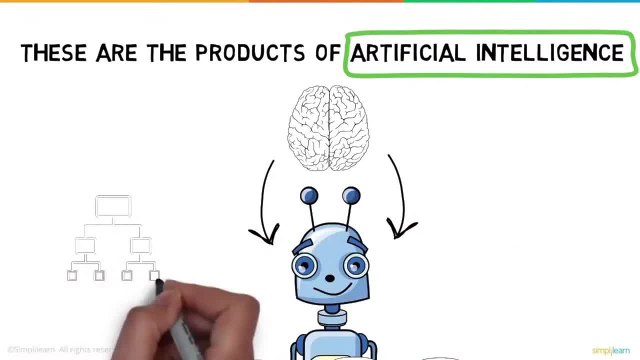 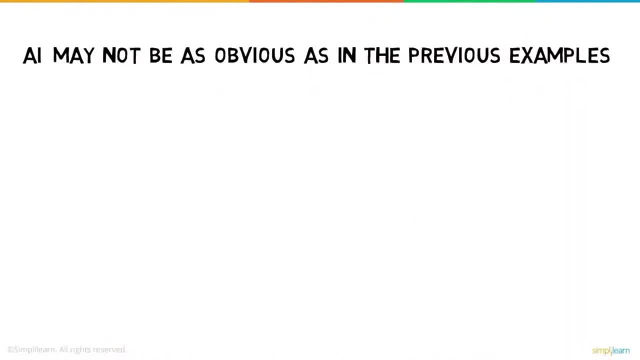 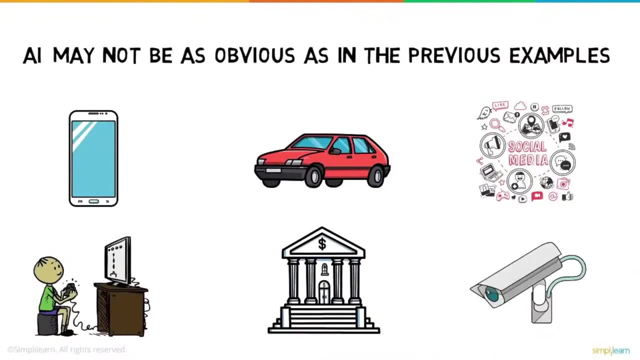 This intelligence is built using complex algorithms and mathematical functions, But AI may not be as obvious as in the previous examples. In fact, AI is used in smartphones, cars, social media feeds, video games, banking surveillance and many other aspects of our daily life. 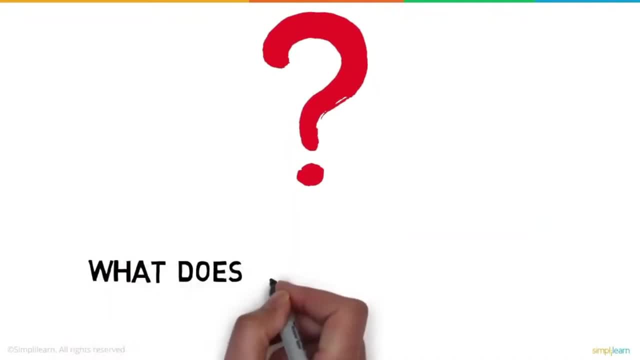 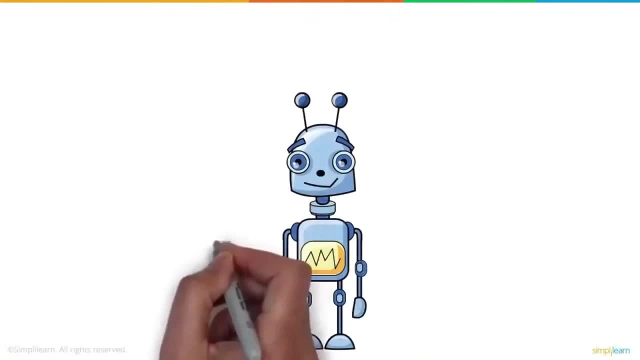 The real question is: what does an AI do at its core? Here is a robot we built in our lab, which is now dropped onto a field. In spite of a variation in lighting, landscape and dimensions of the field, the AI robot must perform as expected. 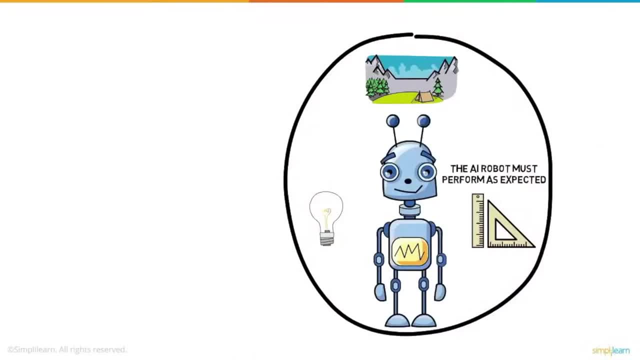 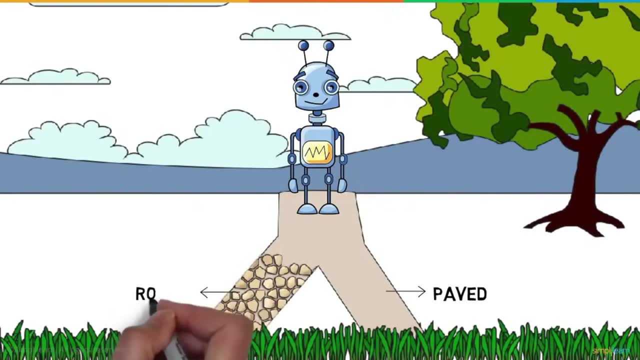 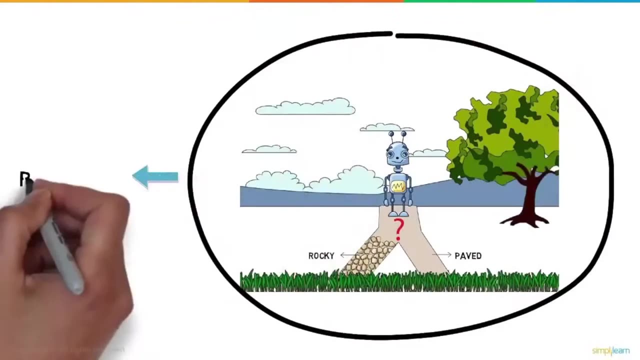 This ability to react appropriately to a new situation is called generalized learning. The robot is now at a crossroad, one that is paved and the other rocky. The robot must determine which path to take based on the circumstances. This portrays the robot's reasoning ability. 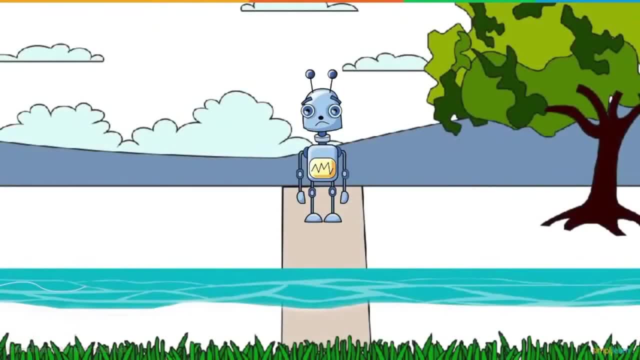 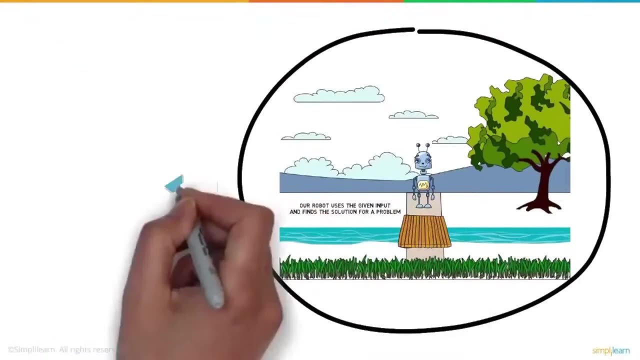 After a short stroll, the robot now encounters a stream that it cannot swim across. Using the plank provided as an input, the robot is able to cross this stream. So our robot uses the given input and finds the solution for a problem. This is problem solving. 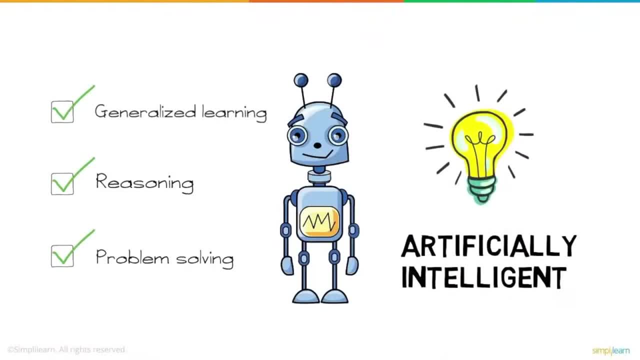 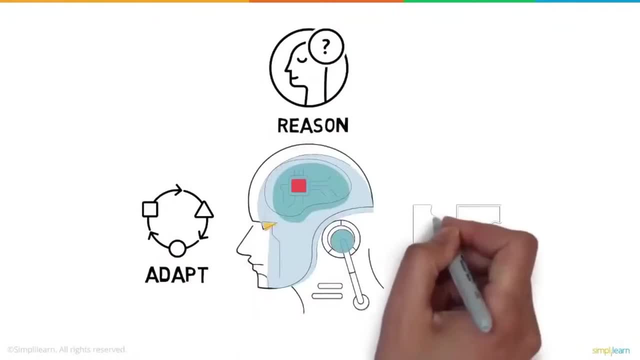 These three capabilities make the robot artificial. In short, AI provides machines with the capability to adapt, reason and provide solutions. Well, now that we know what AI is, let's have a look at the two broad categories an AI is classified into. 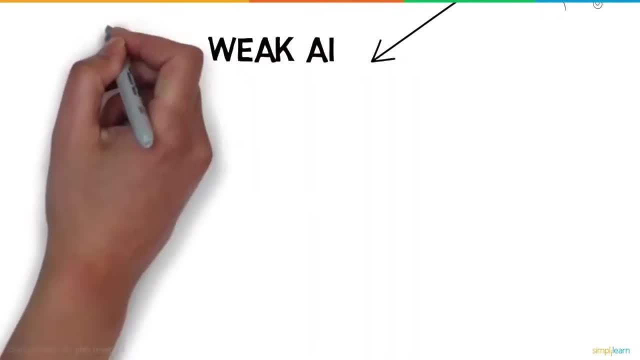 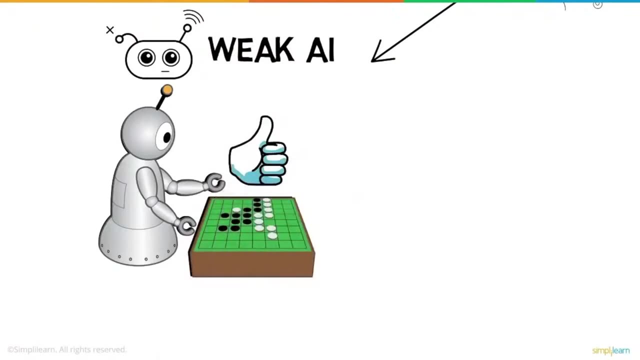 Weak AI, also called Narrow AI, focuses solely on one task. For example, AlphaGo is a maestro of the game Go, But you can't expect it to be even that good. You can't expect it to be even remotely good at chess. 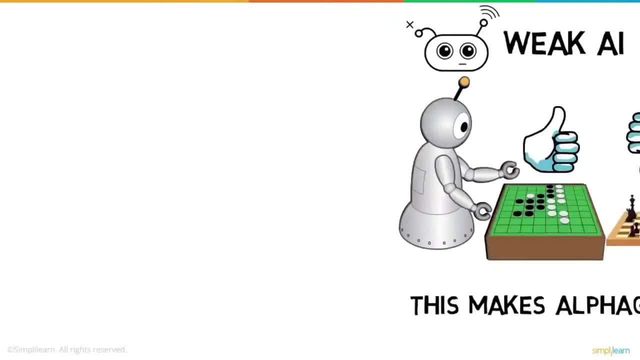 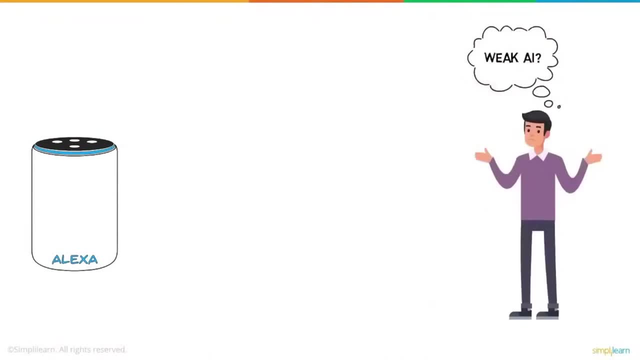 This makes AlphaGo a weak AI. You might say Alexa is definitely not a weak AI, since it can perform multiple tasks. Well, that's not really true. When you ask Alexa to play Despacito, it picks up the keywords Play and Despacito and runs a program it is trained to. 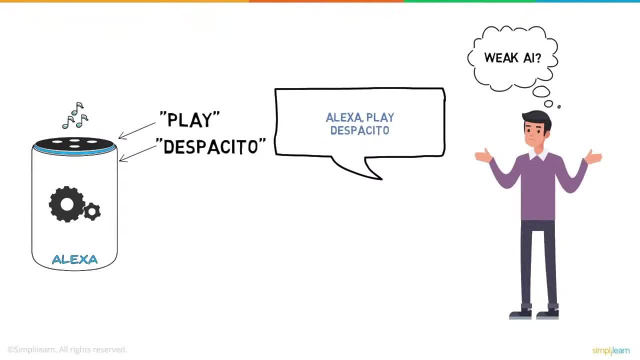 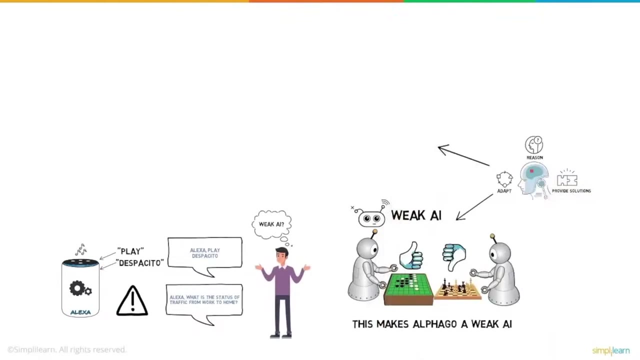 Alexa cannot respond to a question it isn't trained to answer. For instance, try asking Alexa the status of traffic from work to home. Alexa cannot provide you this information as she is not trained to. And that brings us to our second category of AI: Strong AI. 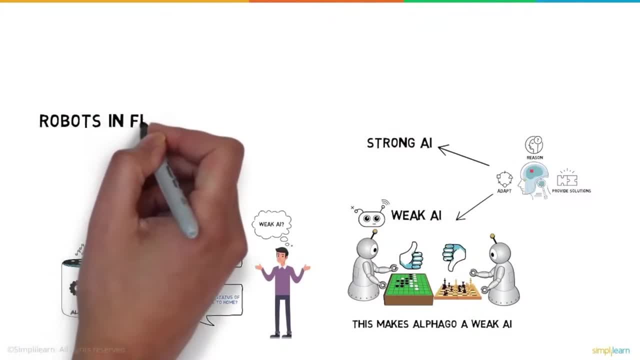 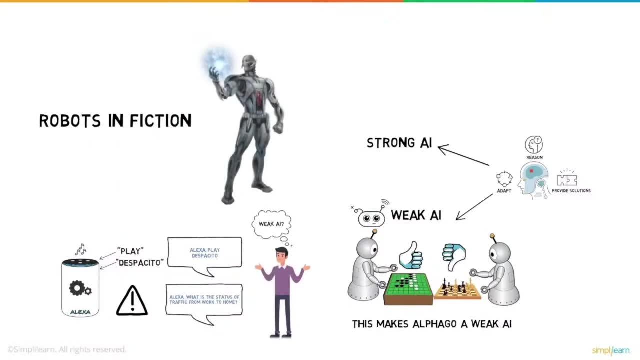 Now this is much like the robots that only exist in fiction as of now. Ultron from Avengers is an ideal example of a strong AI. That's because it's self-aware and eventually even develops emotions. This makes the AI's response unpredictable. 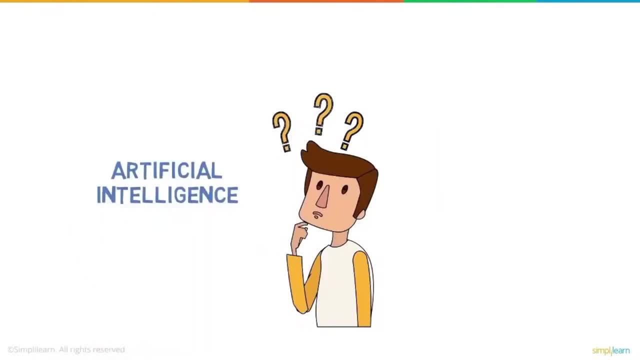 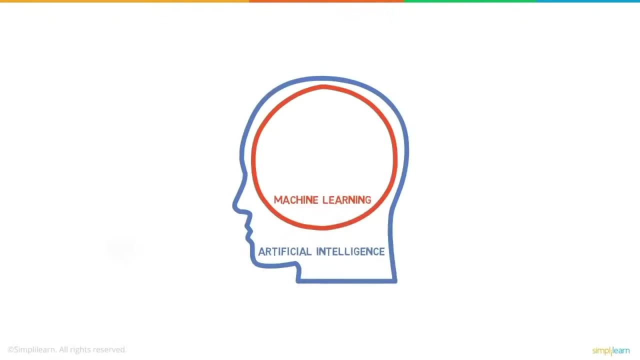 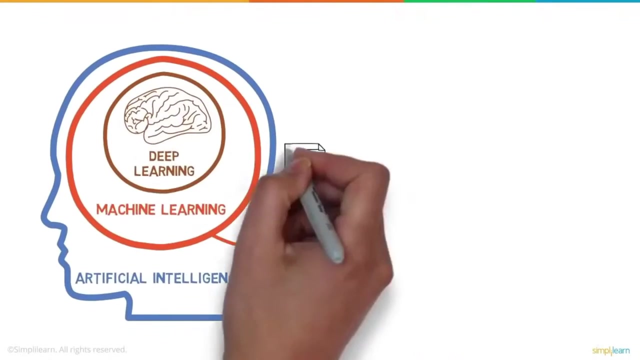 You must be wondering well, how is artificial intelligence different from machine learning and deep learning? We saw what AI is. Machine learning is a technique to achieve AI, and deep learning, in turn, is a subset of machine learning. Machine learning provides a machine with the capability to learn from data and experience through algorithms. 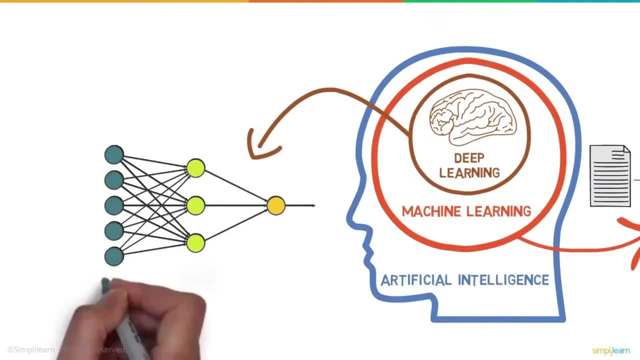 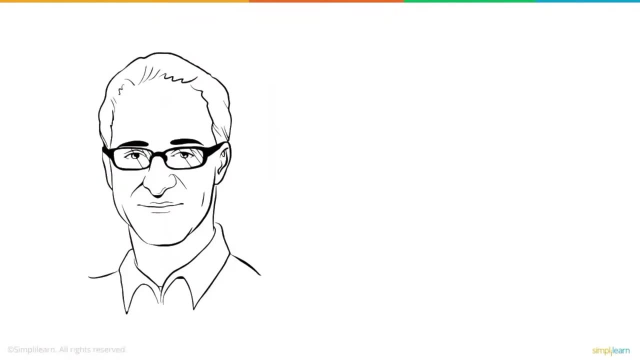 Deep learning does this learning through ways inspired by AI. This means through deep learning, data and patterns can be better perceived. Ray Kurzweil, a well-known futurist, predicts that by the year 2045, we would have robots as smart as humans. 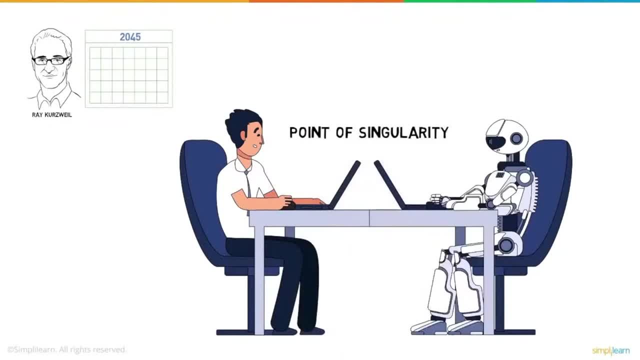 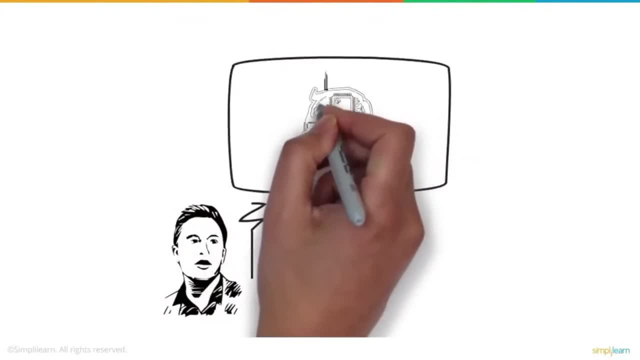 This is called the point of singularity. Well, that's not all. In fact, Elon Musk predicts that the human mind and body will be enhanced by AI implants, which would make us partly cyborgs. So here's a question for you. 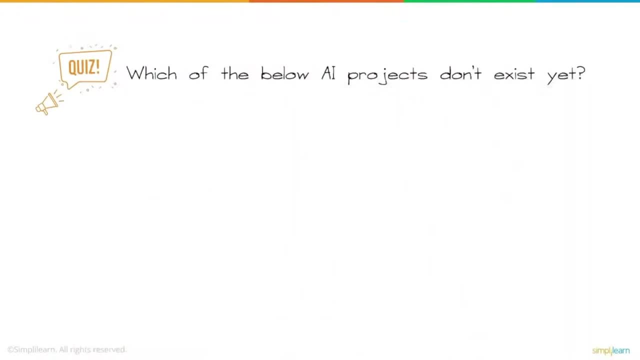 Which of the below AI projects don't exist yet? A- An AI robot with citizenship. B- A robot with a muscular skeletal system. C- AI that can read its owner's emotions. D- AI that develops emotions over time. Give it a thought and leave your answers in the comment section below. 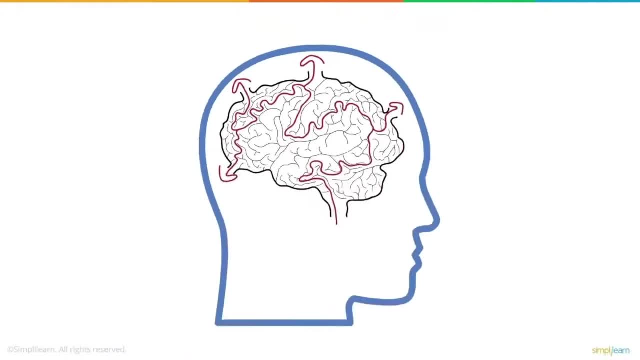 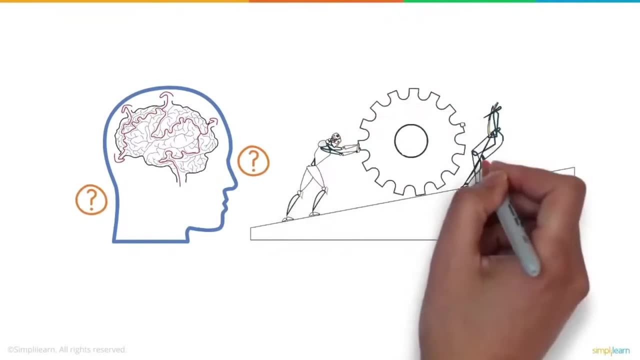 Since the human brain is still a mystery, it's no surprise that AI, too, has a lot of unventured domains. For now, AI is built to work with humans and make our tasks easier. However, with the maturation of technology, 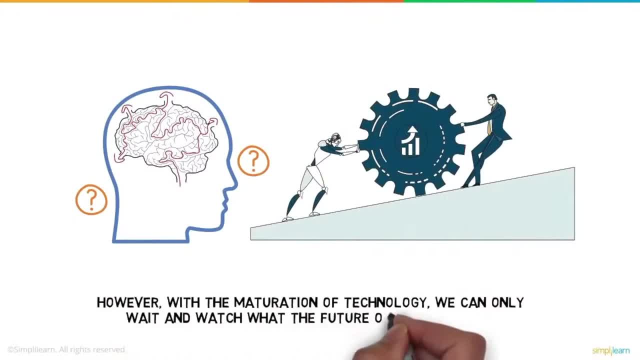 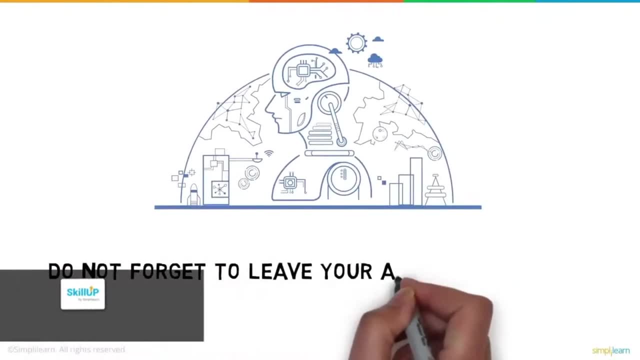 we can only wait and watch what the future of AI holds for us. Well, that is artificial intelligence for you. in short, Do not forget to leave your answer to the quiz in the comment section below. Also like, share and subscribe to our channel if you enjoyed this video. 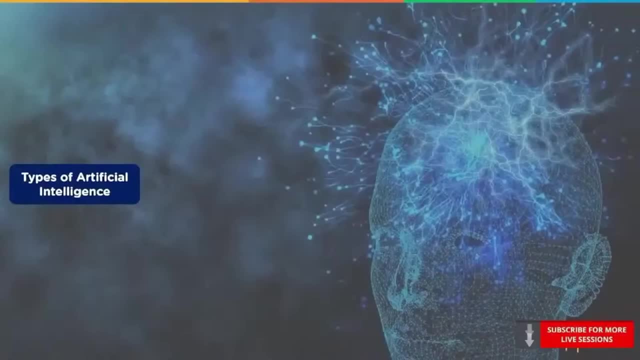 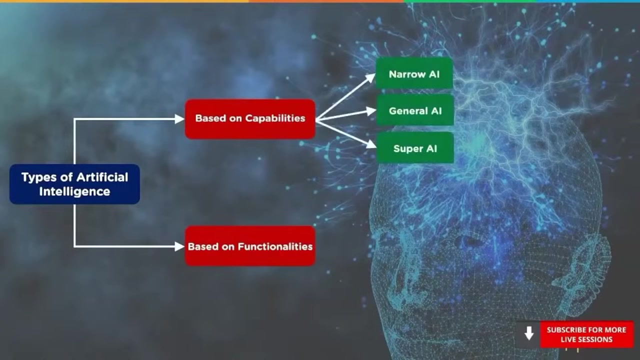 Stay tuned and keep learning. Now let's look at the different types of artificial intelligence. So AI can be classified based on capabilities and functionalities. Under capabilities, there are three types of artificial intelligence. They are narrow AI, general AI and super AI. 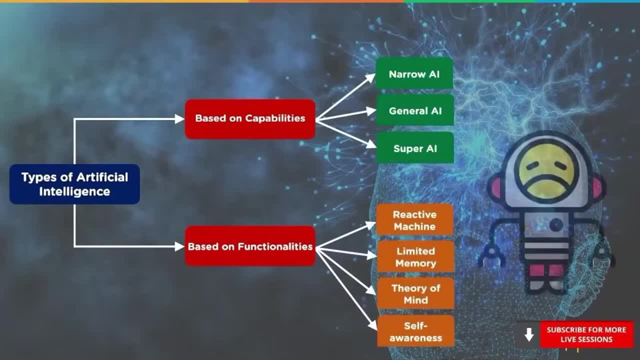 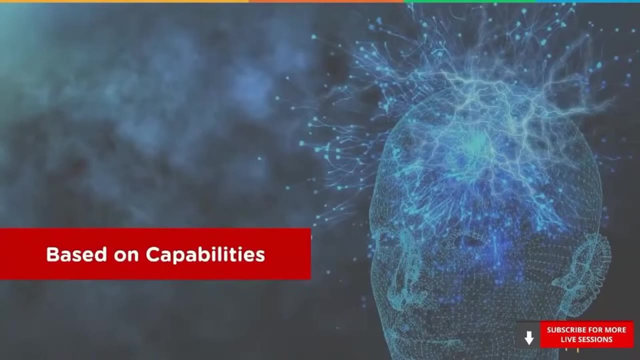 Under functionalities. we have four types of artificial intelligence: Reactive machine, limited memory, theory of mind and self-awareness. Let's look at them one by one. First, we will look at the different types of artificial intelligence based on capabilities. So what is narrow AI? 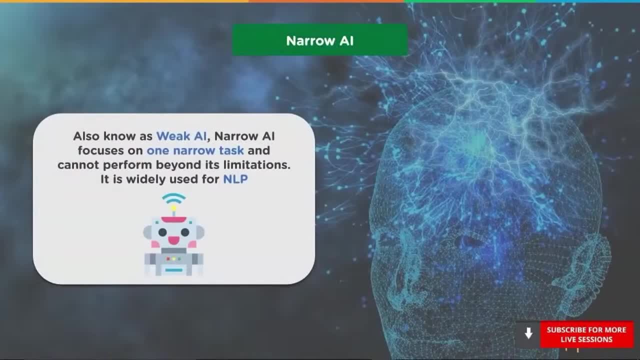 Narrow AI, also known as weak AI, focuses on one narrow task and cannot perform beyond its limitations. It aims at a single subset of cognitive abilities and advances in that spectrum. Applications of narrow AI are becoming increasingly common in our day-to-day lives as machine learning and deep learning methods continue to evolve. 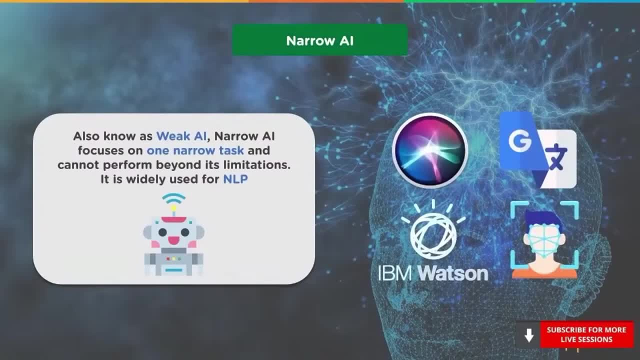 Apple's Siri is a simple example of a narrow AI that operates with a limited, predefined range of functions. Siri often has challenges with tasks outside its range of abilities. IBM Watson Supercomputer is another example of narrow AI, which applies cognitive computing, machine learning and natural language processing to process information and answer your questions. 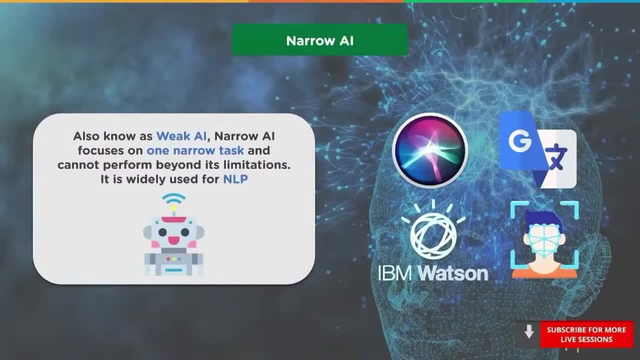 IBM Watson once outperformed human contestants Ken Jenkins to become the champion on the popular game show Jeopardy. Other examples of narrow AI include Google Translate, image recognition, software recommendation systems, spam filtering and Google's page-ranking algorithm. Next, we have general artificial intelligence, or general AI. 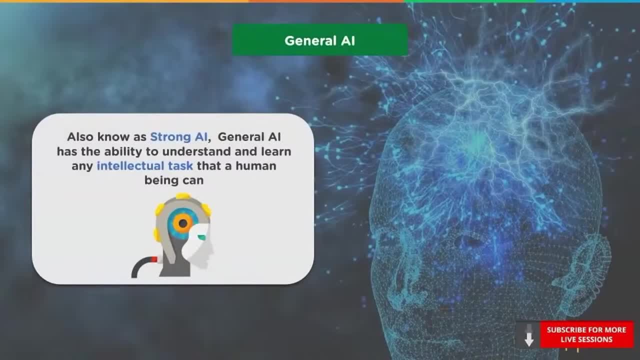 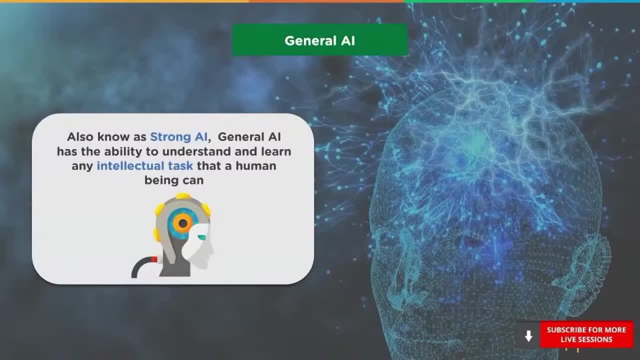 Next we have general artificial intelligence, or general AI has the ability to understand and learn any intellectual task that a human can. In near future, we also need to improve to apply knowledge and skills in different contexts. AI researchers and scientists have not achieved strong AI so far. 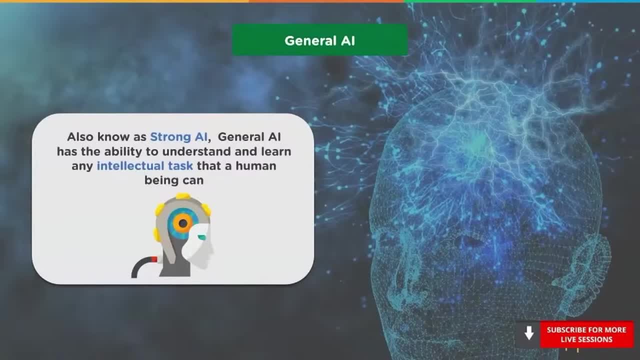 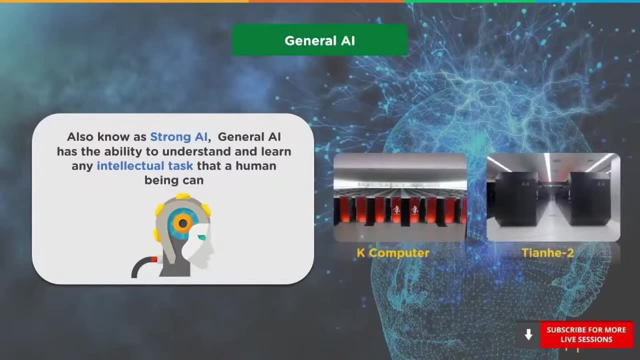 To succeed, they would need to find a way to make machines conscious, programming a full set of cognitive abilities. Fujitsu built the K computer, which is one of the fast computers in the world. It is one of the most notable attempts at achieving strong AI. 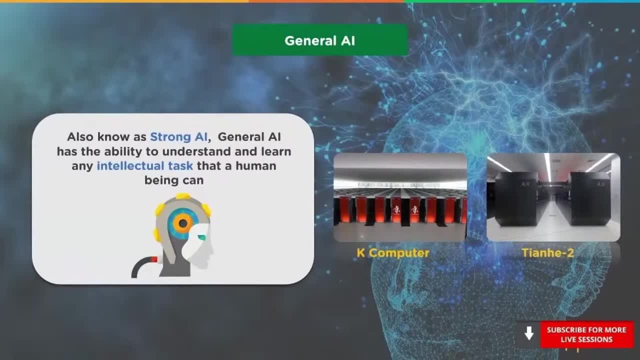 It took 40 minutes to simulate a single second of neural activity, so it is difficult to determine whether or not strong AI will be achieved in the near future. Tianhe-2 is a supercomputer created by China's National University of Defense Technology. It currently holds the record for CPS at 33.86 petaflops. 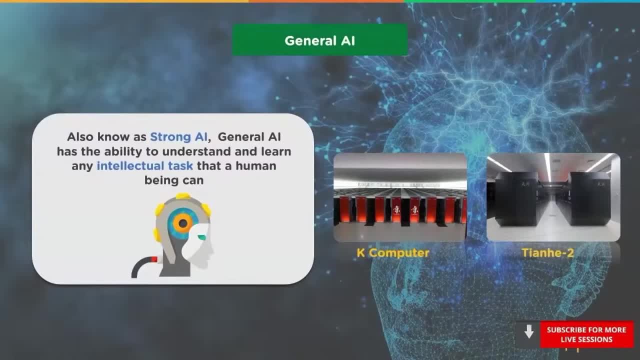 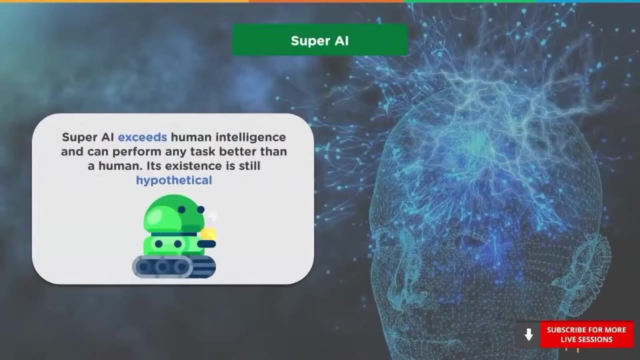 Although it sounds exciting, the human brain is estimated to be capable of one exaflop. Now, CPS means characters per second that a system can process. Third in the list of AI that is based on capabilities, we have Super AI. Super AI exceeds human intelligence and can perform any task better than a human. 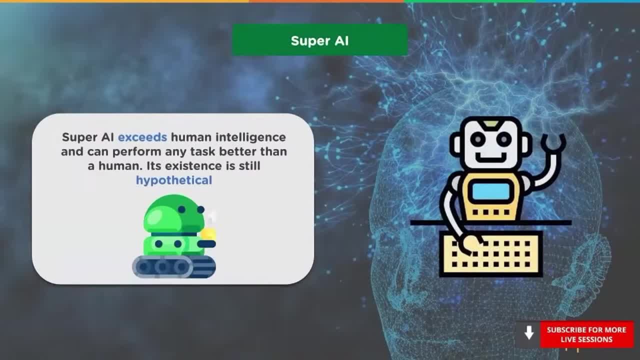 The concept of artificial super intelligence sees AI evolve to be so akin to human emotions and experiences that it doesn't just understand them: it evokes emotions, needs, beliefs and desires of its own. Its existence is still hypothetical. Some of the key characteristics of Super AI are the following. 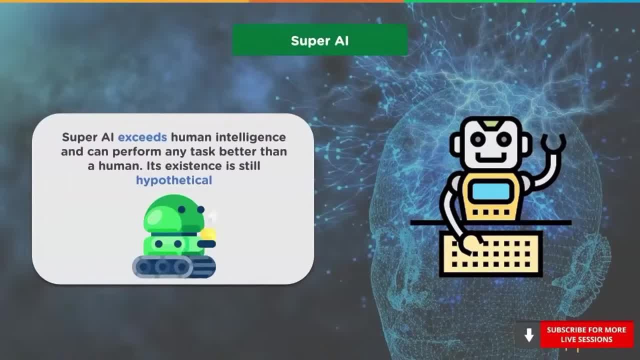 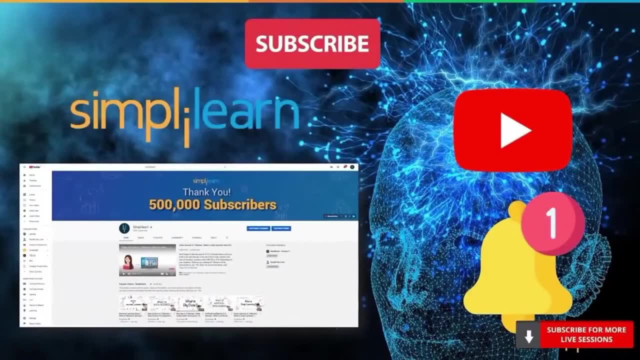 Super AI includes the ability to think, solve puzzles, make judgments and decisions on its own. Now, if you have enjoyed watching this video so far, please make sure to subscribe to our YouTube channel and hit the bell icon to stay updated with all the latest technologies. 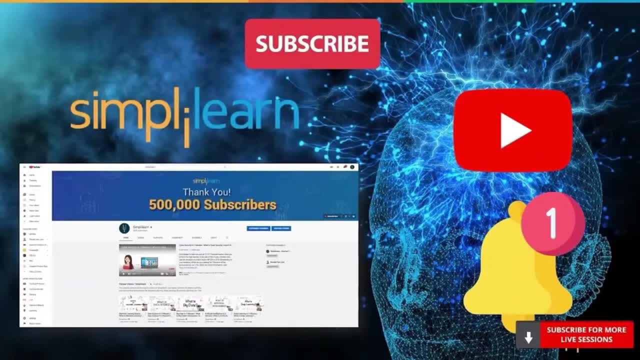 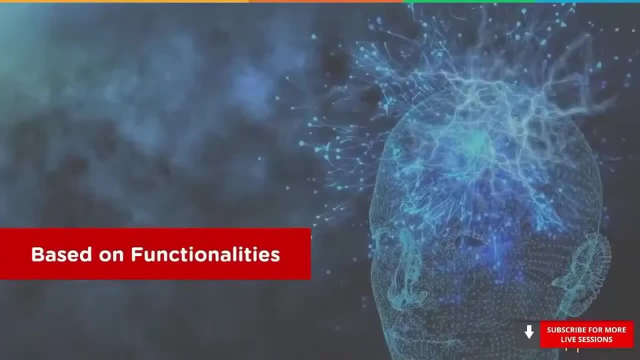 Also, if you have any questions related to this video, please put it in the chat section. Our team of experts will help you address your questions. Moving ahead Now, we will see that Super AI is a technology that can be used to solve problems. 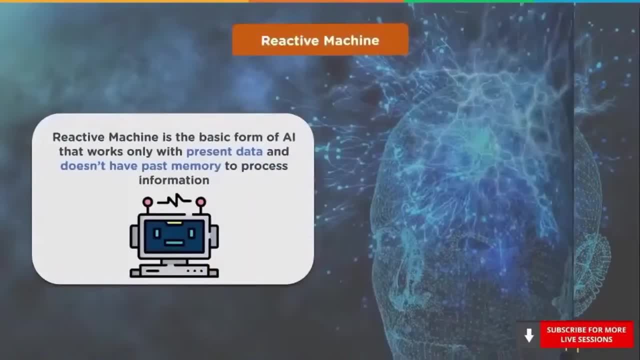 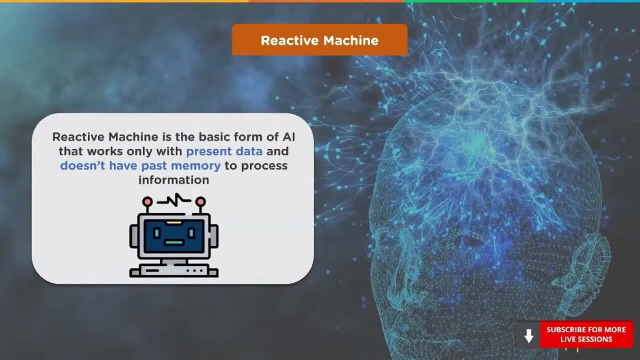 Let's explore the different types of artificial intelligence based on functionalities In this category. first, we have Reactive Machine. A reactive machine is the basic form of AI that does not store memories or use past experiences to determine future actions. It works only with present data. 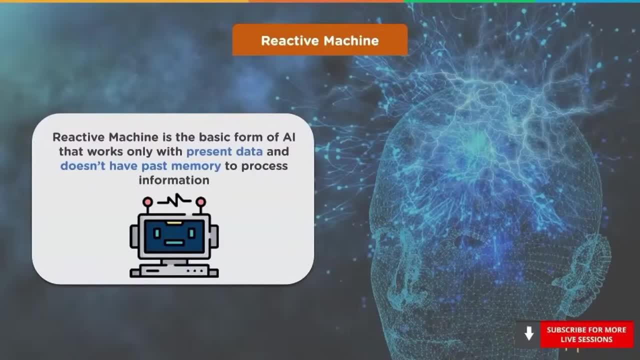 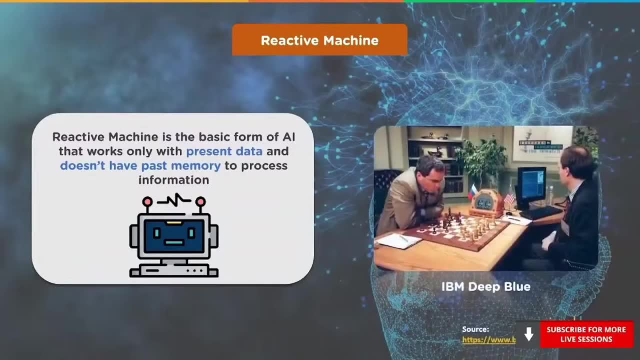 They simply perceive the world and react to it. Reactive machines are given certain tasks and don't have capabilities beyond those duties. IBM's Deep Blue, which detects and detects the world, is a machine that can detect the world and react to it. Defeated chess grandmaster Garry Kasparov is a reactive machine that sees the pieces on a chessboard and reacts to them. 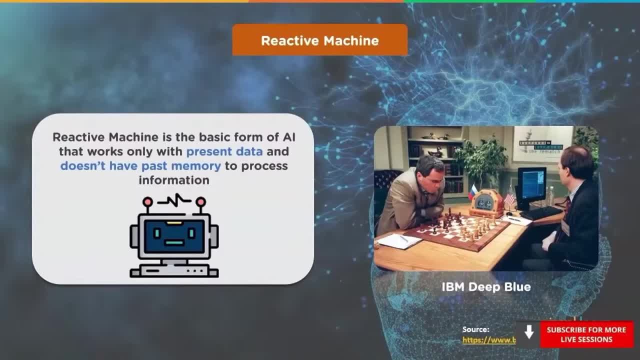 It cannot refer to any of its prior experiences and cannot improve with practice. Deep Blue can identify the pieces on a chessboard and know how each moves. It can make predictions about what moves might be next for it and its opponent. It can choose the most optimal moves from among the possibilities. 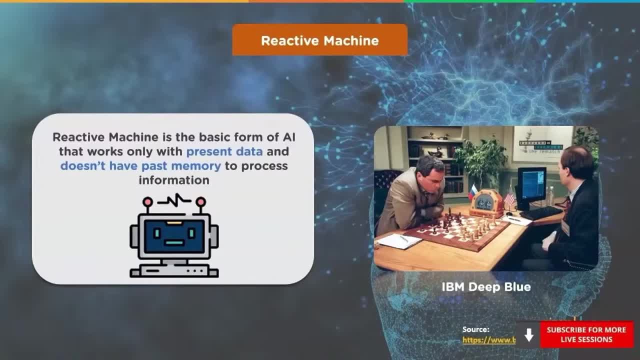 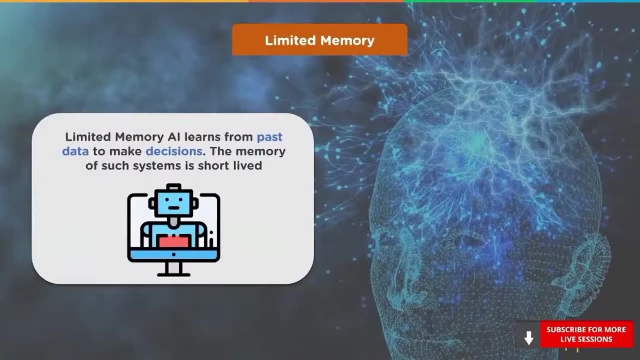 Deep Blue ignores everything before the present moment. All it does is look at the pieces on the chessboard as it stands right now and choose from possible next moves Up. next we have Limited Memory. Limited Memory: AI learns from past data to make decisions. 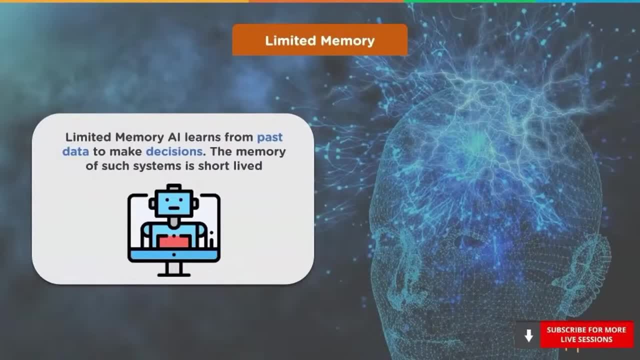 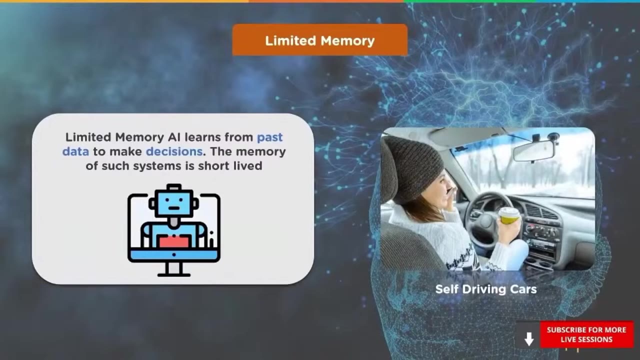 The memory of such systems is short-lived. While they can use this data for a specific period of time, they cannot add it to a library of their experiences. This kind of technology is used for self-driving vehicles. They observe how other vehicles are moving around them in the present and as time passes. 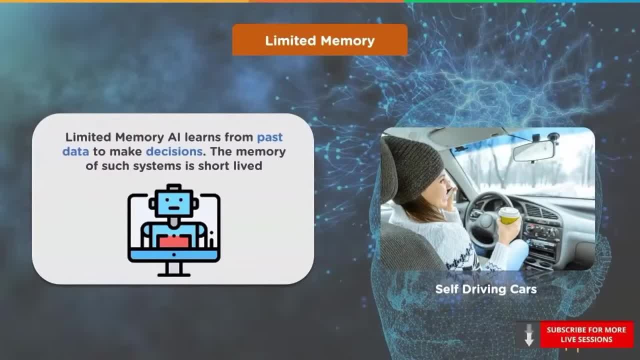 That ongoing collected data gets added to the static data within the AI machine, such as lane markers and traffic lights. They are included when the vehicle decides to change lanes to avoid cutting off another driver or being hit by a nearby vehicle. Mitsubishi Electric is a company that has been figuring out how to improve such technology for applications like self-driving cars. 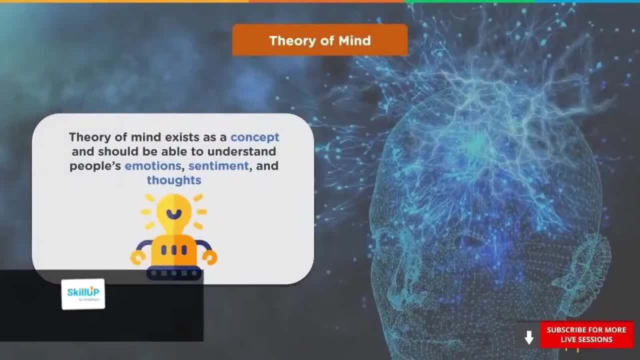 They have been working on a series of applications for self-driving cars for a long time, and they have been working on a series of applications for self-driving cars for a long time now. Then we have Theory of Mind. Theory of Mind represents a very advanced class of technology and exists as a concept. 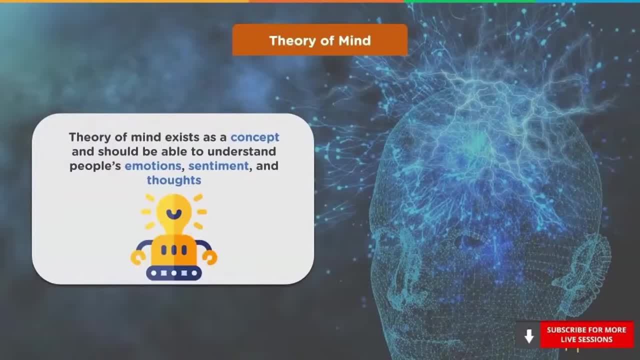 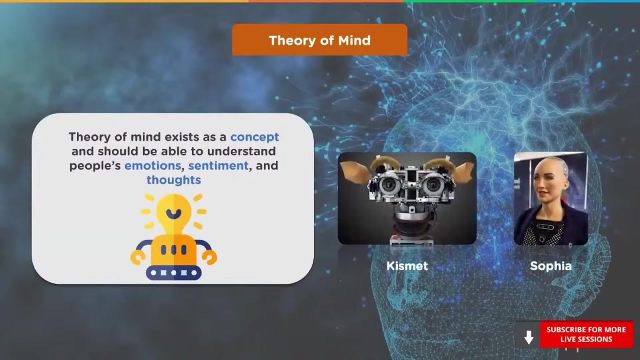 This kind of AI requires a thorough understanding that the people and the things within an environment can alter feelings and behaviors. It should be able to understand people's emotions, sentiment and thoughts. Even though a lot of improvements are there in this field. Even though a lot of improvements are there in this field. 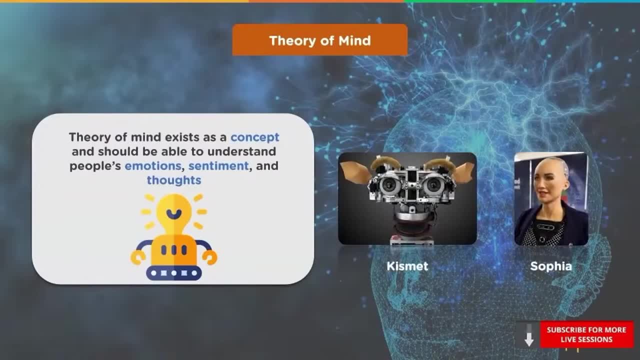 the theory of AI is not complete yet. One real-world example of Theory of Mind AI is Kismet, a robot head made in the late 90s by a Massachusetts Institute of Technology researcher. Kismet can mimic human emotions and recognize them. Both abilities are key advancements in Theory of Mind AI. but Kismet can't follow gazes or convey attention to humans. 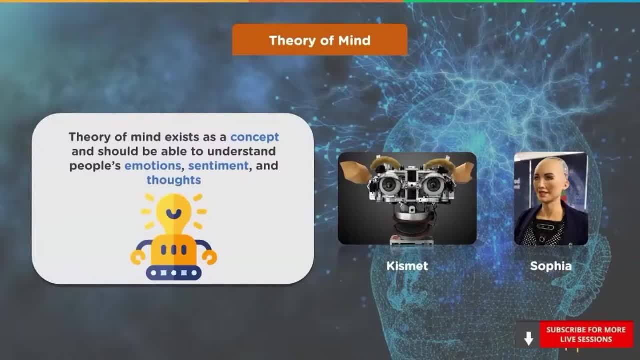 Sophia from Hanson Robotics is another example where the Theory of Mind AI was implemented. Cameras within Sophia's eyes, combined with computer algorithms, allow her to see. She can follow faces, sustain eye contact and recognize individuals. She is able to process speech and have conversations using natural language subsystem. 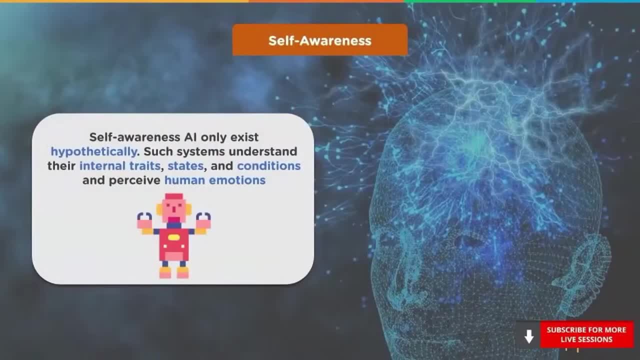 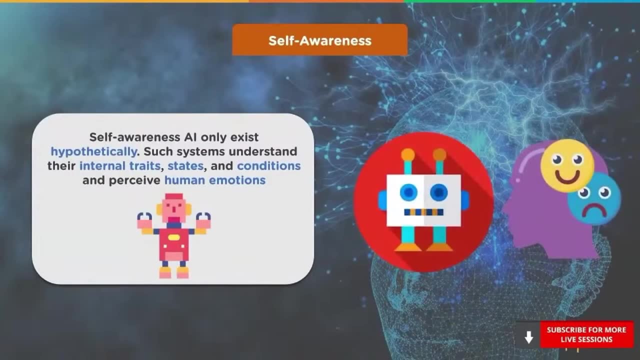 Finally, we have Self-Awareness. Self-Awareness AI only exists hypothetically. Such systems understand their internal traits, states and conditions and perceive human emotions. These machines will be smarter than the human mind. This type of AI will not only be able to understand and evoke emotions in those it interacts with. 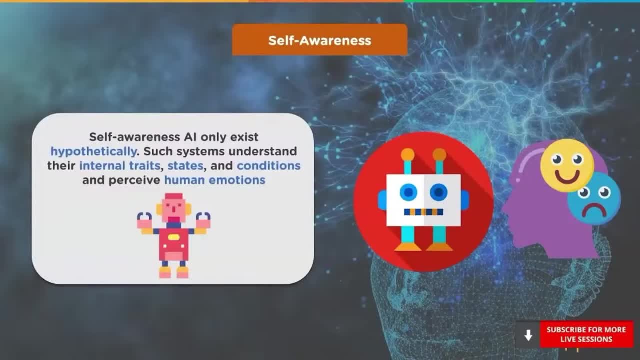 but also have emotions, needs and beliefs of its own. While we are probably far away from creating machines that are self-aware, we should focus our efforts towards understanding, memory, learning and the ability to base decisions on past experiences. I am Keerthana, and today we shall be talking about 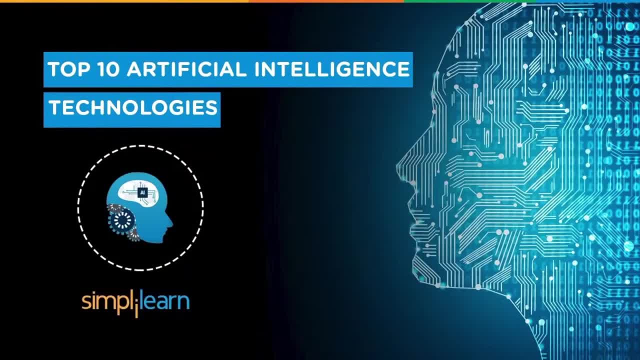 the Top 10 Artificial Intelligence Technologies. Before getting into the video, here's a gentle reminder to subscribe to our channel and hit the bell icon so that you wouldn't miss any update from us. So, without further ado, let's quickly jump into the topic. 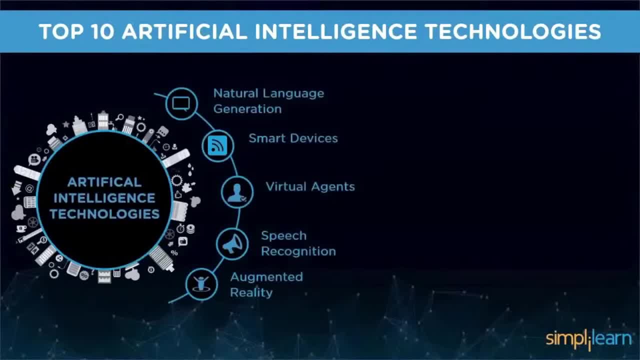 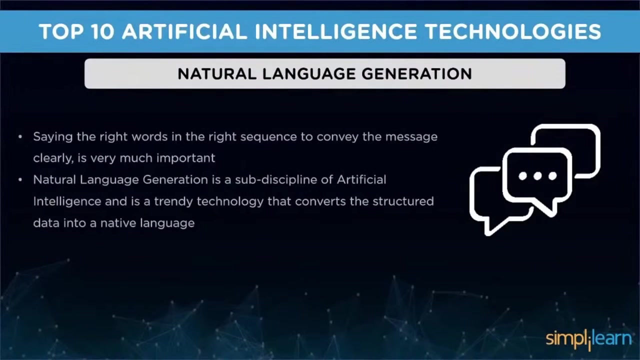 In the list we have Natural Language Generation, Smart Devices, Virtual Agents, Speech Recognition, Augmented Reality, Machine Learning, Robotic Process Automation, Decision Management, Deep Learning and, finally, Image Recognition. Please note that the list is in no particular order. Natural Language Generation. Communicating, or conveying the information efficiently and transparently is very much crucial in communication. 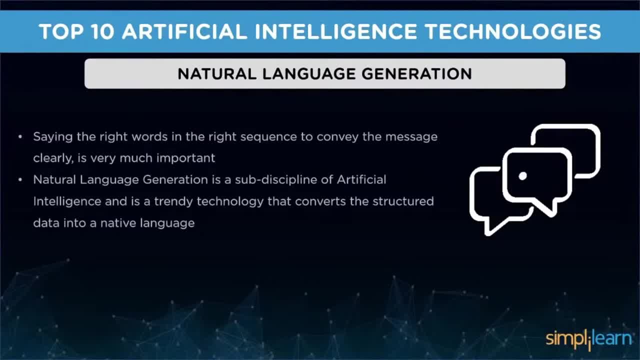 To say the right words in the right sequence to convey the message clearly. humans often find it tricky, and when it comes to machines it's trickier. Natural Language Generation is a sub-discipline of artificial intelligence and is a trendy technology that converts the structured data into a native language. 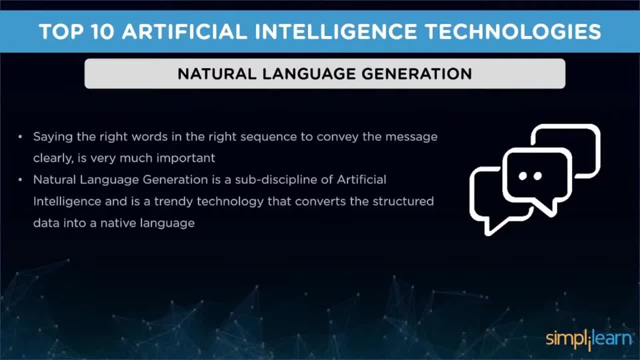 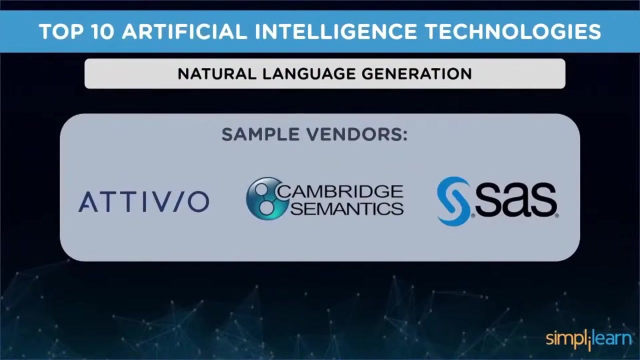 The machines are programmed in such a way that the algorithms convert the data into a desirable format for the users. This technology is widely used in customer service, report generation and summarizing business intelligence insights. Some of the sample vendors are ATVU, Automated Insights. 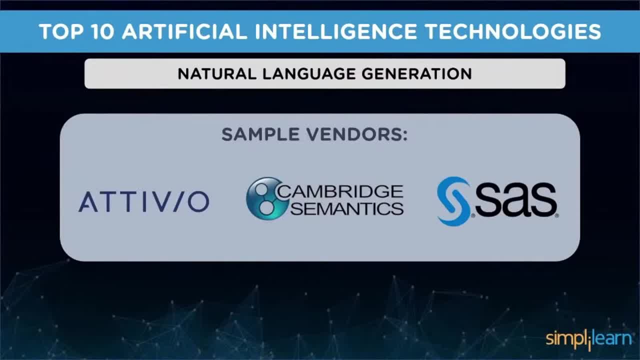 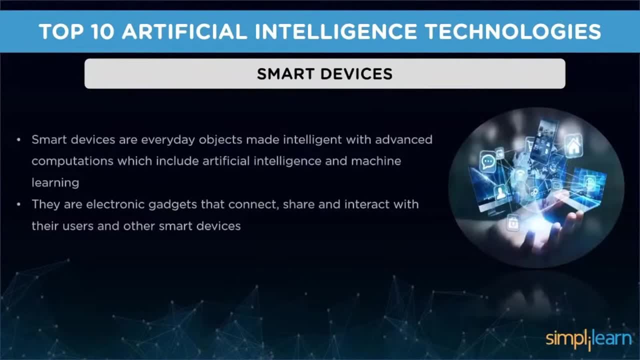 SAS, Digital Reasoning, Narrative Science, etc. On the list. next we have Smart Devices. With every passing day, smart devices are becoming more popular and more trendy. Technologies that people were using once upon a time are now remodeled and modified as smart devices. They can be used in almost every industry to improve efficiency and optimize the operations. 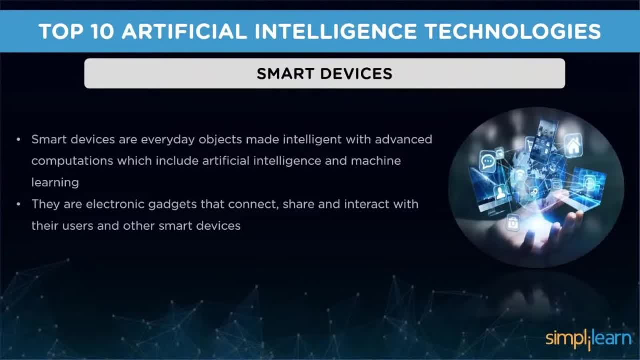 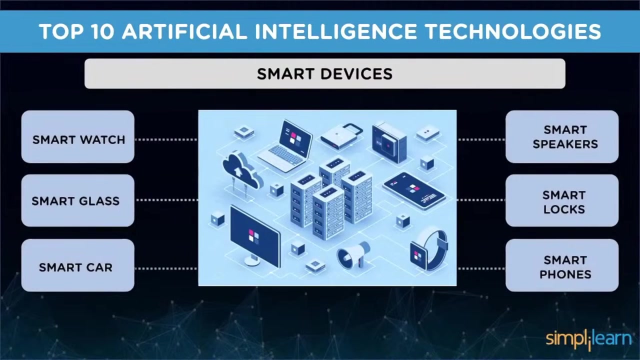 Smart devices are everyday objects made intelligent with advanced computations, which include artificial intelligence and machine learning. They are electronic gadgets that are able to connect, share and interact with its users and other smart devices. Some of the smart devices are smart watches, smart glasses, smart phones, smart speakers, etc. 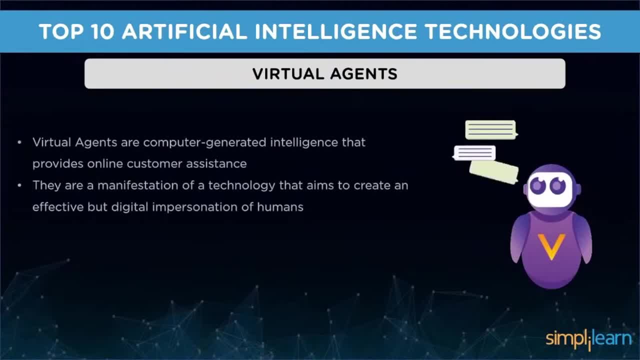 Virtual Agents. They are computer-generated intelligence that provides online customer assistance. They can effectively communicate with humans. In most of the web and mobile applications, we see chatbots as customer service agents who interact with us. answering our queries In simple virtual agents are a manifestation of a technology. 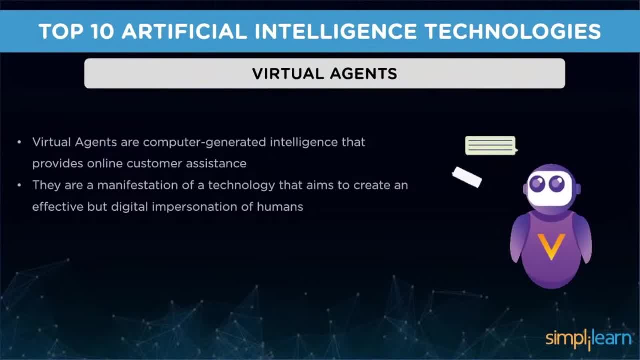 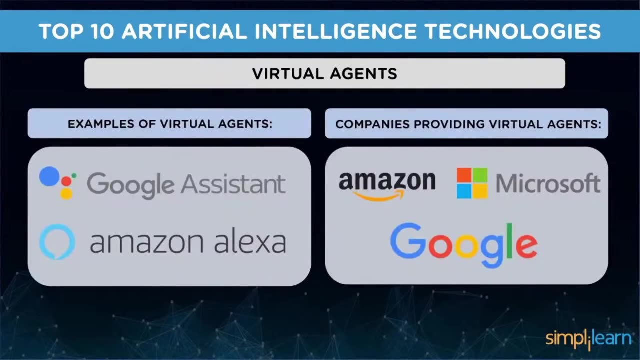 which aims to create an effective but digital impersonation of humans. Virtual agents can make reservations, book an appointment, place an order and can even avail product information. Some of the best examples of virtual agents are Google Assistant and Amazon Alexa, And the companies that provide virtual agents are Microsoft, Google, Amazon and Assist AI. 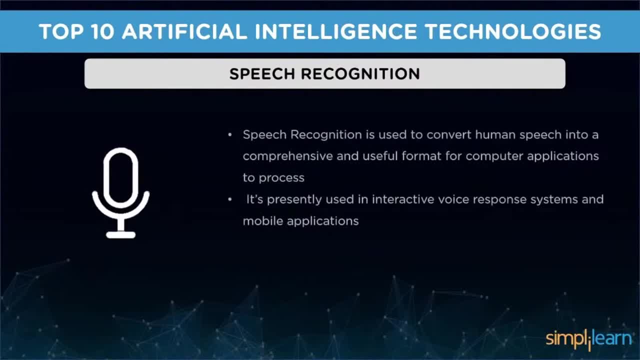 Next we have Speech Recognition. Speech recognition is yet another sub-discipline of artificial intelligence which is used to convert human speech into a comprehensive and useful format for computer applications to process. It can be said as a bridge between computer interactions and humans. It's presently used in interactive voice response systems and mobile applications. 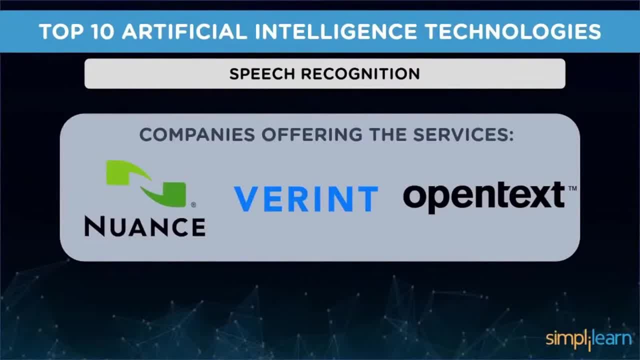 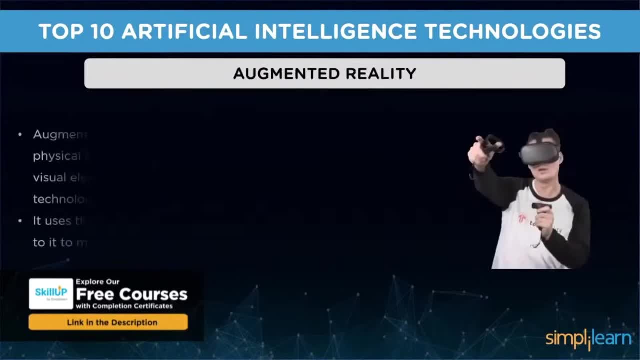 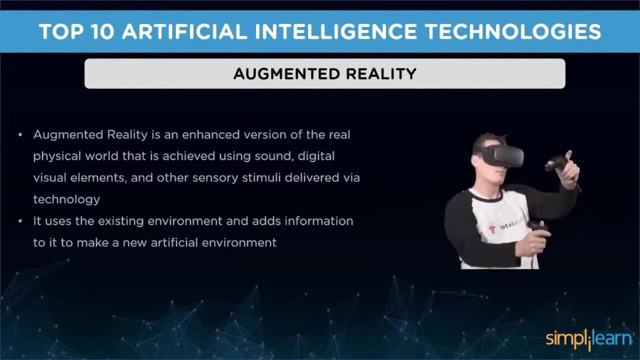 Some of the companies offering speech recognition services are Nuance Communications, Open Text, NICE and Wear & Systems. Augmented Reality: Yet another trendy technology in the field of artificial intelligence. augmented reality is an enhanced version of the real physical world that is achieved using sound, digital visual elements and other sensitive stimuli delivered via technology. 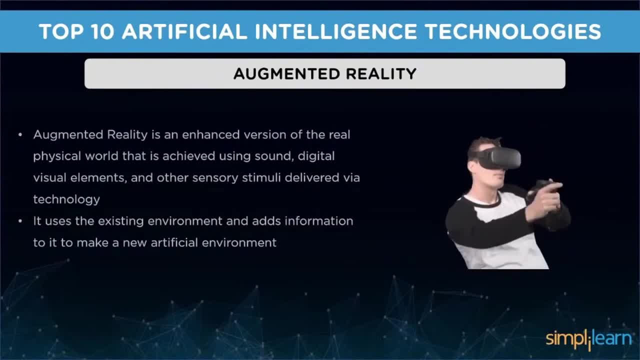 Augmented reality uses the existing environment and adds information to it to make a new artificial environment. It alters the perception of the real-world environment. Augmented reality is making its way into several retail stores that make makeup selection and furnishing much more fun and interactive. 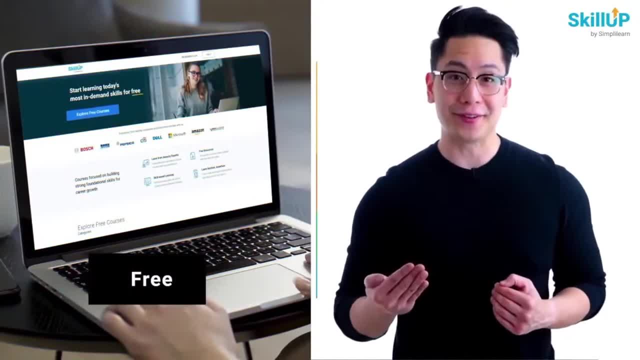 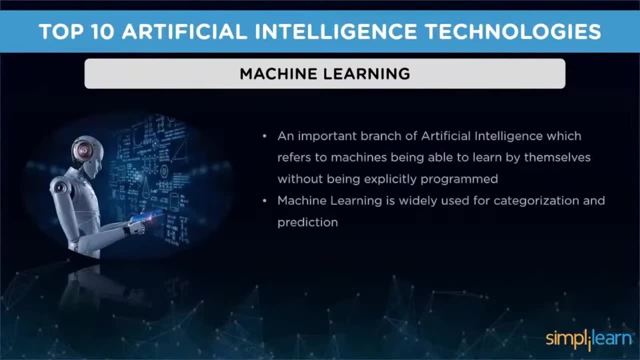 If getting your learning started is half the battle, what if you could do that for free? Visit SkillUp by SimplyLearn. Click on the link in the description to know more Machine Learning. Machine learning is an application and an important branch of artificial intelligence. 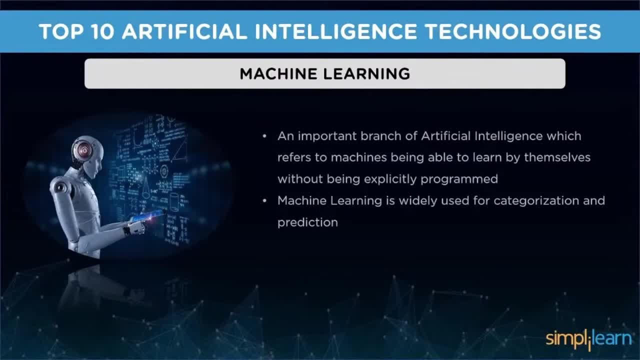 which refers to machines being able to learn by themselves without being explicitly programmed. It enables systems to learn and improve from experience automatically. Machine learning platforms are becoming more and more popular with the help of algorithms, APIs, big data and applications and training tools. 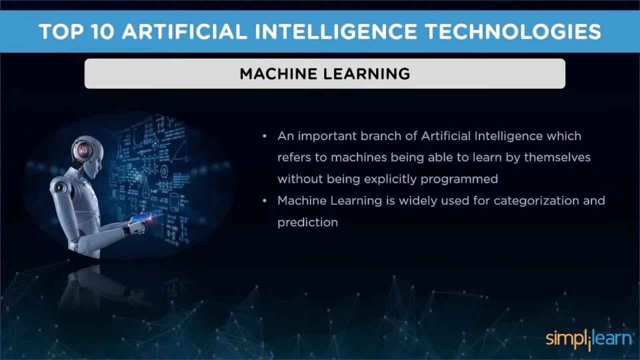 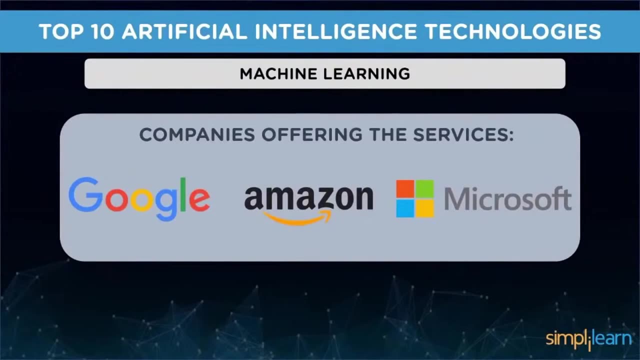 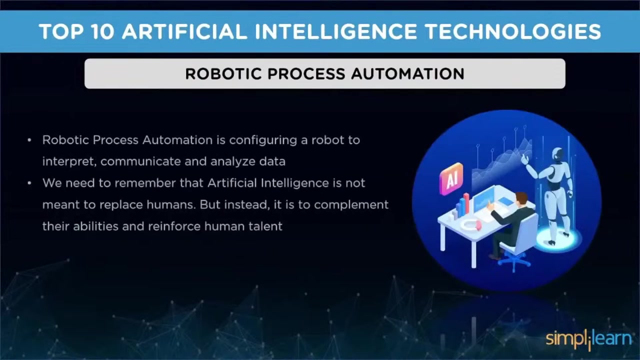 Enterprises are heavily investing in machine learning to reap its benefits for the various domains. Machine learning is widely used for categorization and prediction. Some of the sample vendors are Amazon, Fractal Analytics, Google, Microsoft, etc. Robotic Process Automation: Configuring a robot to interpret, communicate and analyze data is robotic process automation. 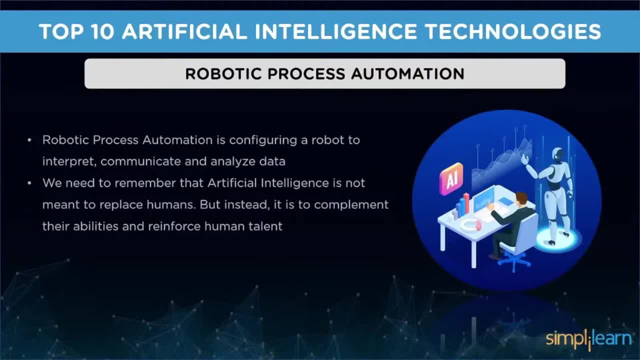 It uses scripts and other methods to automate the human actions, which in turn supports efficient business processes. Robotic process automation is widely used in those areas where the physical presence of a human is dangerous. Fields like warfare, mining, etc. is where it's currently being used. 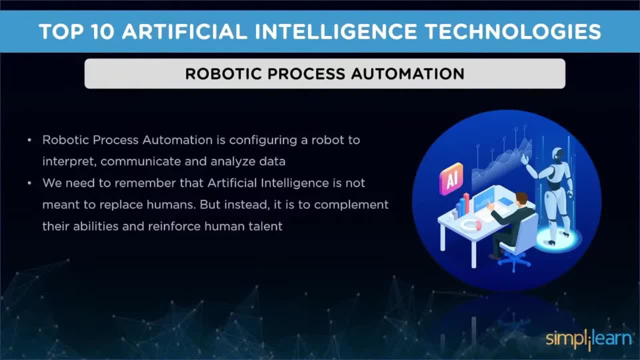 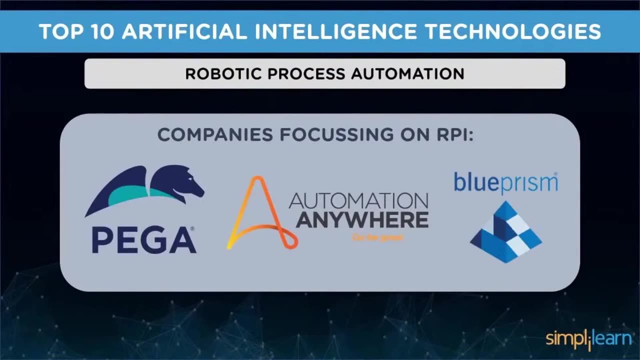 We need to remember that artificial intelligence is not meant to replace humans, But instead it is to complement their abilities and reinforce human talent. Companies that are focusing on robotic process automation are Pega Systems, Automation Anywhere, Blue Prism, etc. Next on the list, we have 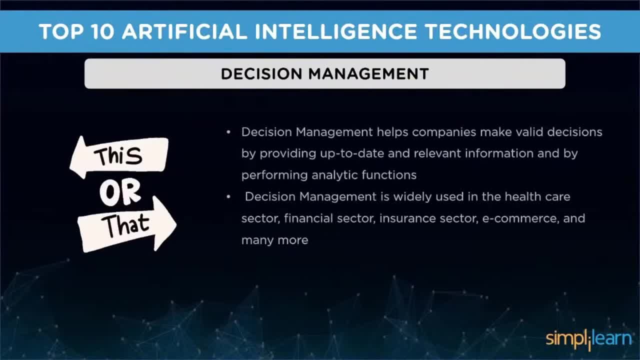 Decision Management. Decision management is yet another technology in artificial intelligence that helps companies make valid decisions by providing up-to-date and relevant information and performing analytic functions. Artificial intelligence, when combined with decision management, helps translate customer data into predictive models of key trends. It also helps in making quick decisions. 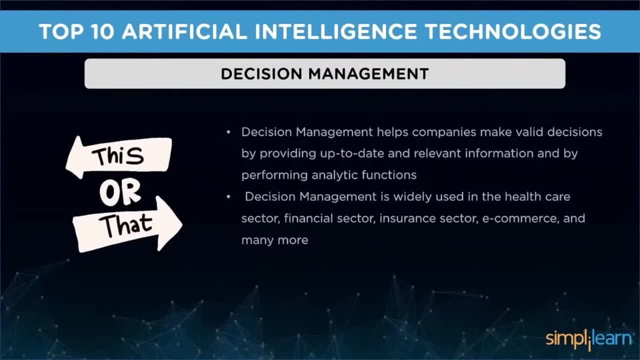 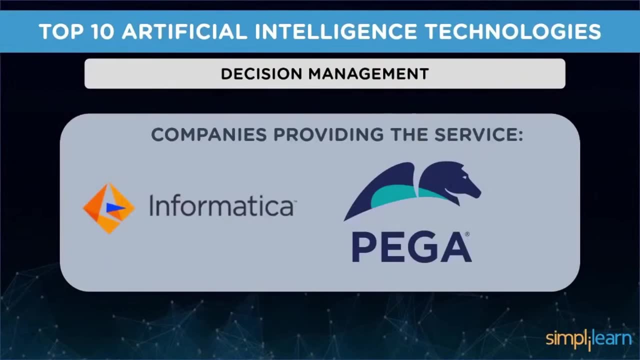 Avoidance of risks And in the automation of the process. Decision management is widely used in the healthcare sector, financial sector, insurance sector, e-commerce and many more. Some of the companies that provide this service are Informatica, Advanced Systems, Concepts, Pega Systems, Mana, etc. 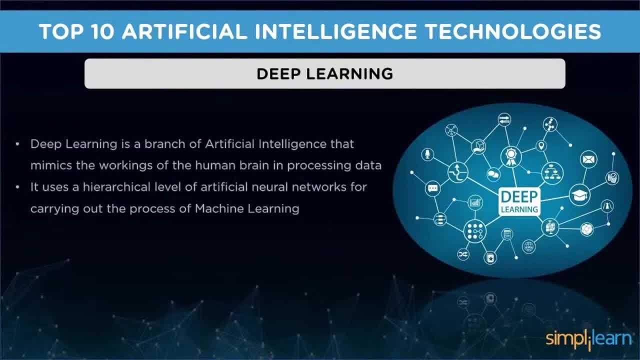 Deep Learning. Deep learning is a branch of artificial intelligence that mimics the workings of the human brain in processing data. This data is used for a variety of purposes like recognizing speech, detecting objects, translating languages and making decisions. Deep learning uses hierarchical level of artificial neural networks for carrying out the process of machine learning, which is used across several industries for various applications. 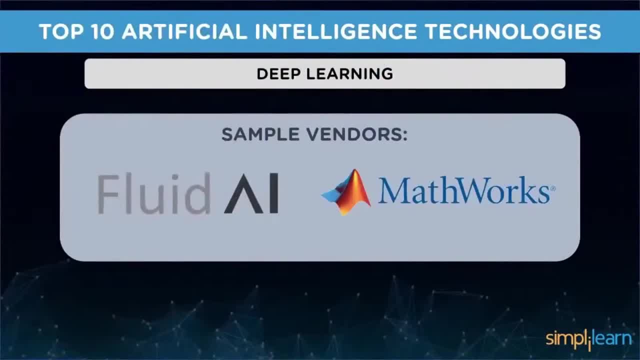 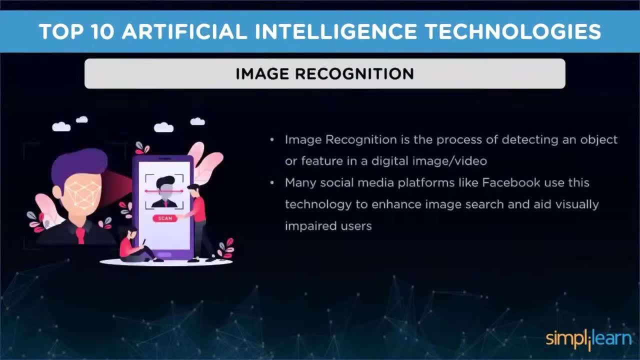 Some of the sample vendors are Deep Instinct, Fluid, AI, Mathworks, Safran Technology, etc. Image Recognition. Image recognition is the process of detecting an object or feature in a digital image or video. It can be used to analyze clients and their opinions, verify users based on their faces, detect license plates. 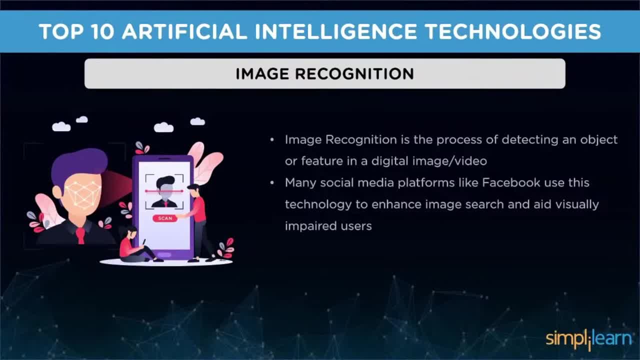 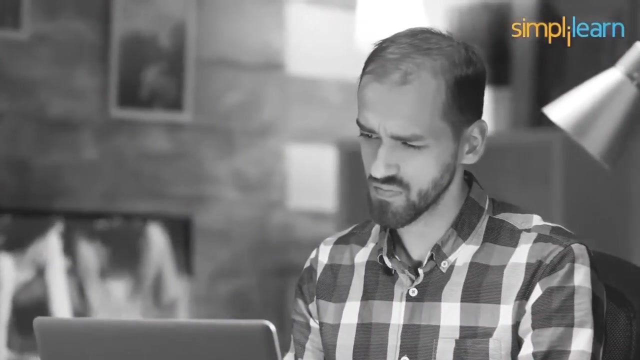 and diagnose diseases. The present-day image recognition is comparable to human visual perception. Many social media platforms, like Facebook, use this technology to enhance image search and aid visually impaired users. Clarify, Guggums and SenseTime provide this technology. Decades ago, the term artificial intelligence was just another Frankenstein story. 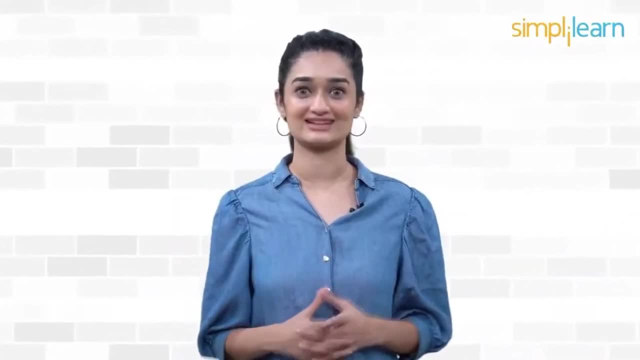 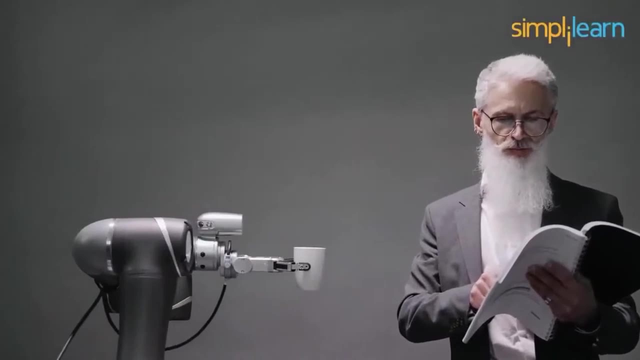 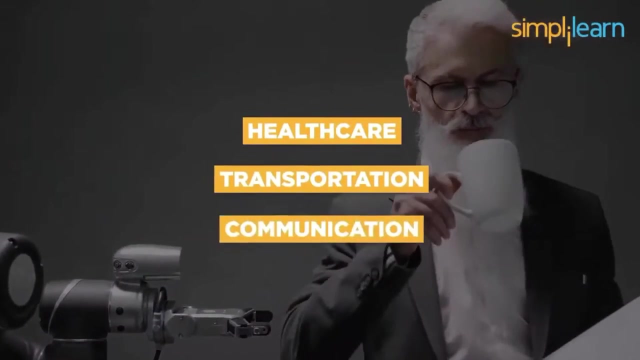 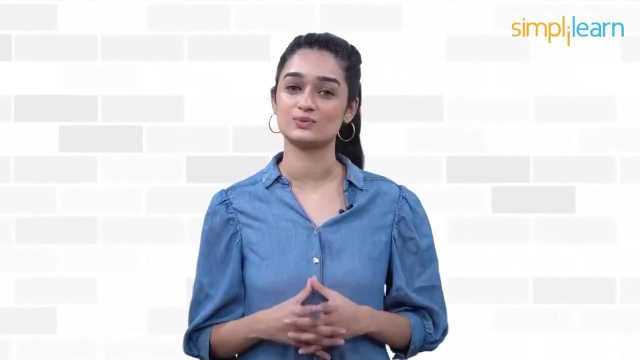 But today it could be a citizen in your next door. Right from its genesis, artificial intelligence was programmed to probe into human life and eliminate the fortifications of the impossibilities in many areas, like healthcare, transportation, communication and much more. There are hundreds and thousands of organizations, tech communities and engineers worldwide working round the clock to make miracles a reality. 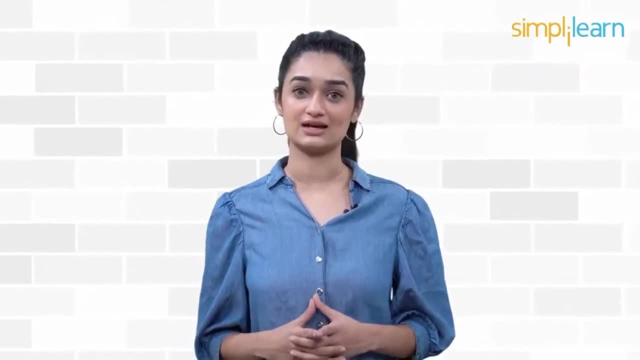 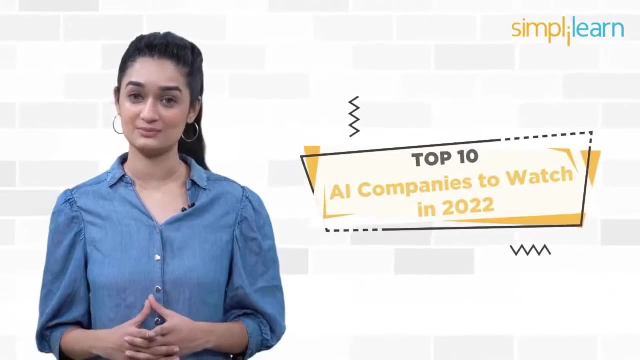 And today we are going to discuss the top 10 amongst those who are contributing a significant part. So here we are: the top 10 artificial intelligence companies to watch in 2022.. At number 10, we have Vizai. 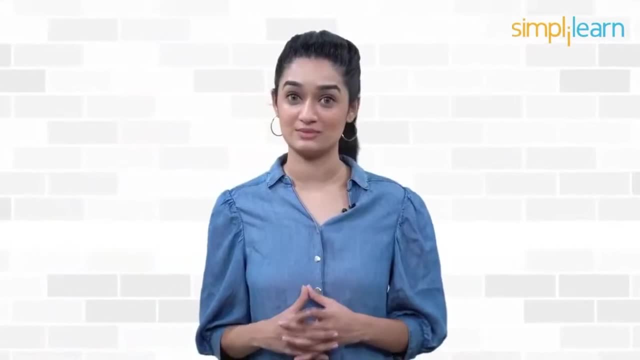 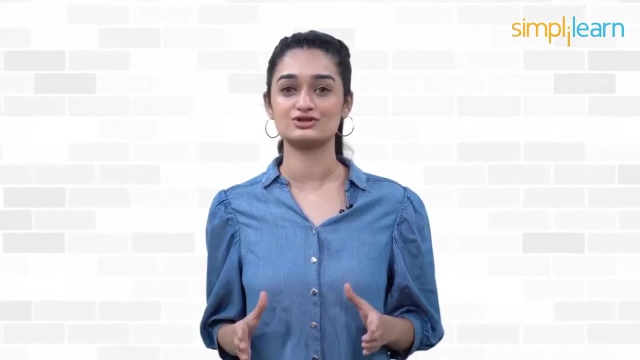 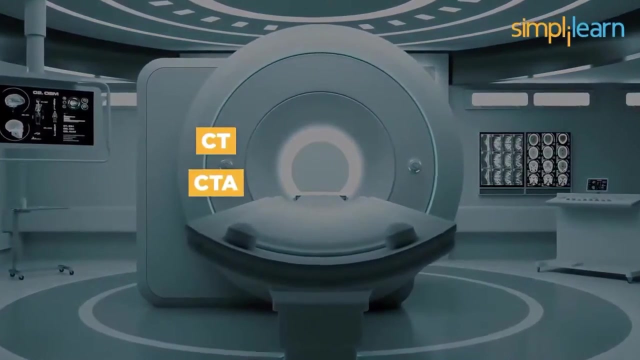 Vizai is a revolutionary approach to dramatically improvise the way healthcare is delivered. Vizai focuses on implementing artificial intelligence to diagnose and detect abnormalities. Vizai is able to detect abnormalities in the human body via CT, CTA, MRI, X-ray, EKG, ultrasound, etc. 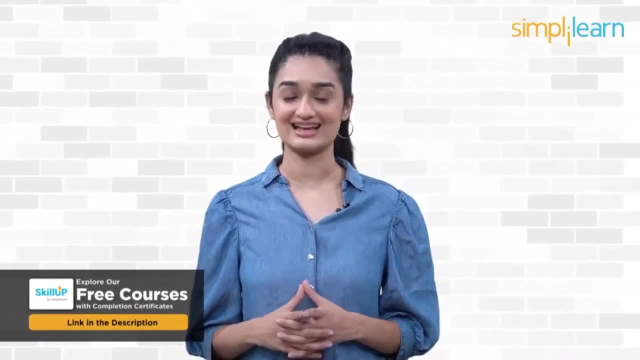 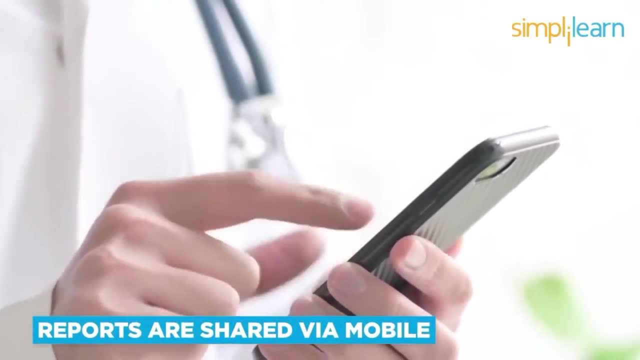 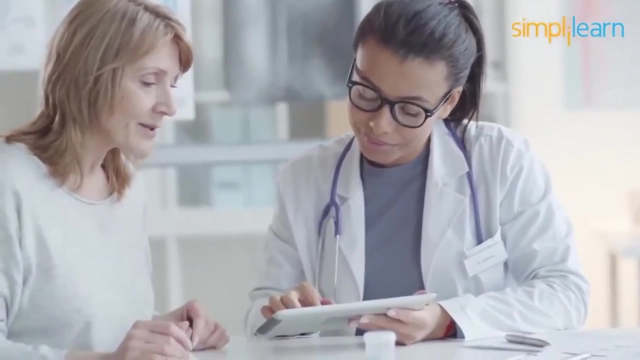 Vizai coordinates both the patient and healthcare professionals. at the same time, The patient reports are shared via mobile to all the concerned medical teams. Results are astonishing. With Vizai, there is a significant improvement in productivity and a reduction of time required for patient treatment and discharge. 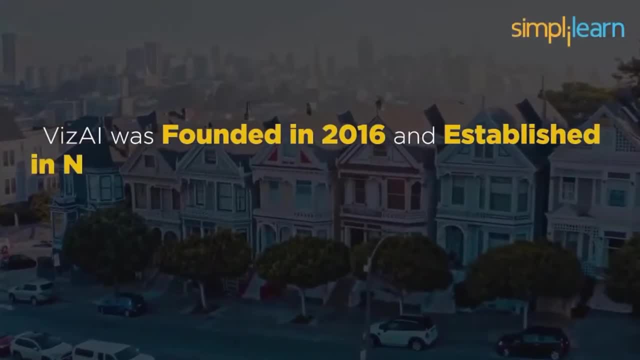 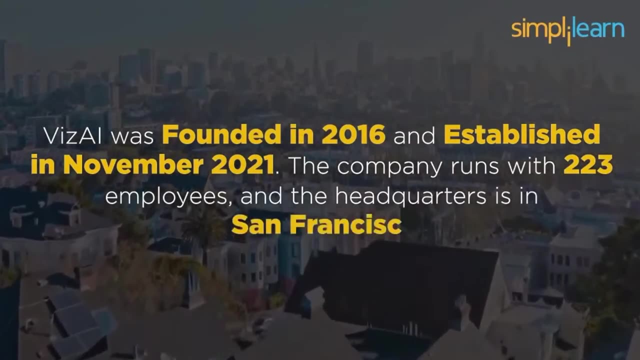 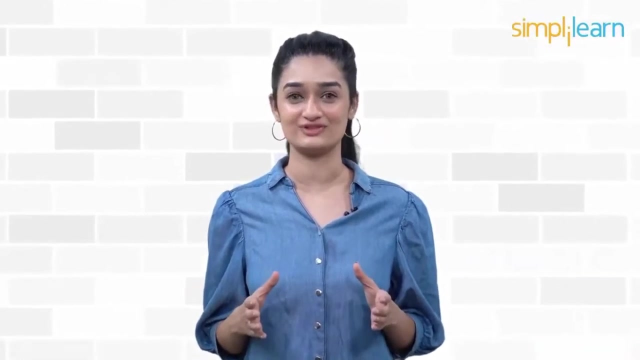 Vizai was founded in 2016 and established in November 2021.. The company runs with 223 employees and the headquarters is in San Francisco. Vizai mainly focuses on improving and filling all the gaps between patients and healthcare professionals. Vizai offers hands-on salaries to its employees. 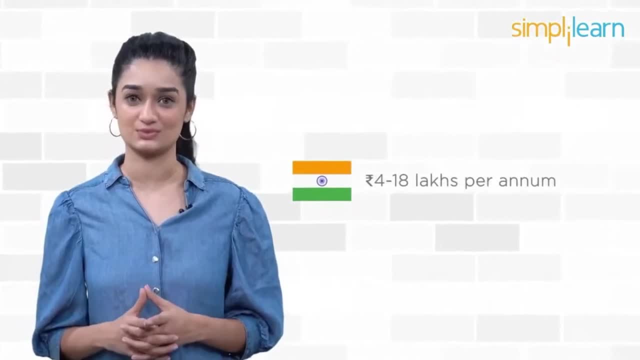 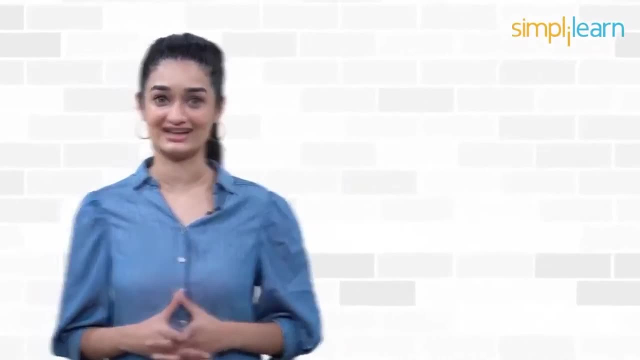 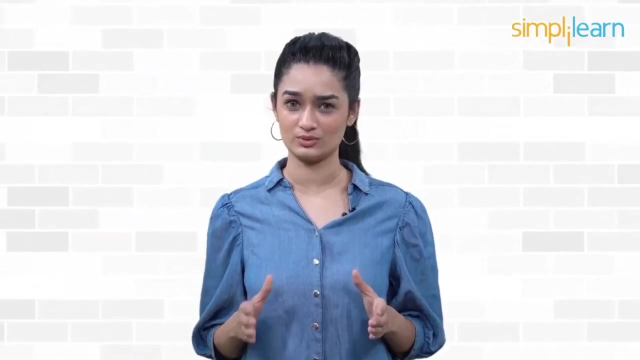 In India, the salaries range from 4 lakhs to 18 lakhs per annum. In America, the wages range from $110,000 to $210,000 per annum. At number 9, we have Farmwife. Ten years ago, an automated weed-killing robot was science fiction. 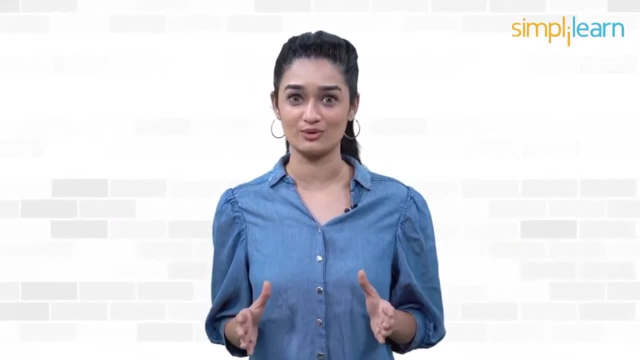 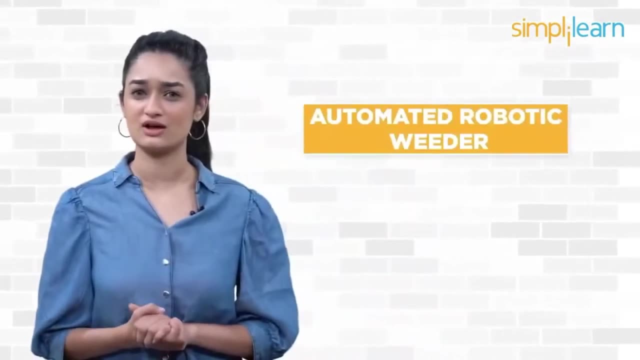 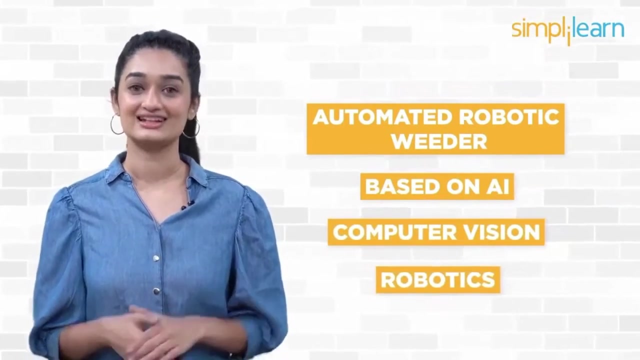 Now it strives of practical weed-killing robots with millimeter precision. thanks to Farmwife, The first product of the Californian-based company was an automated robo-weeder based on AI, computer vision and also robotics. The robo would eliminate weeds from the vegetable fields. 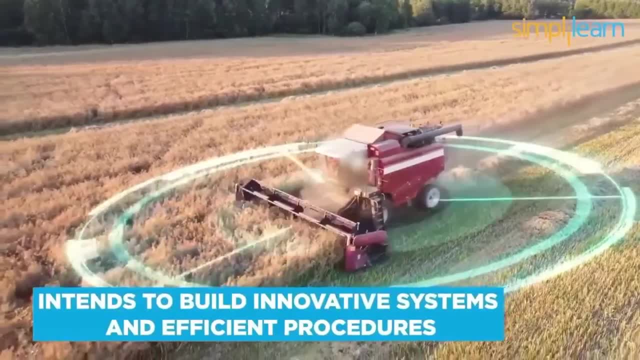 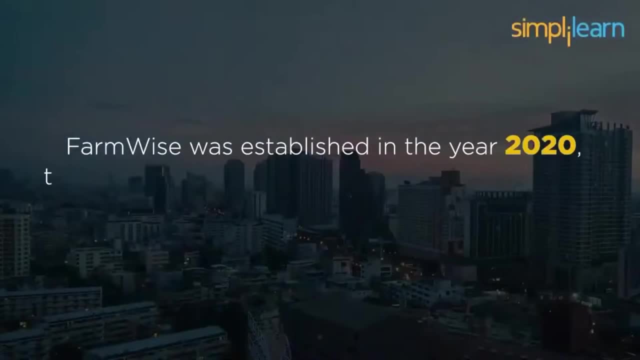 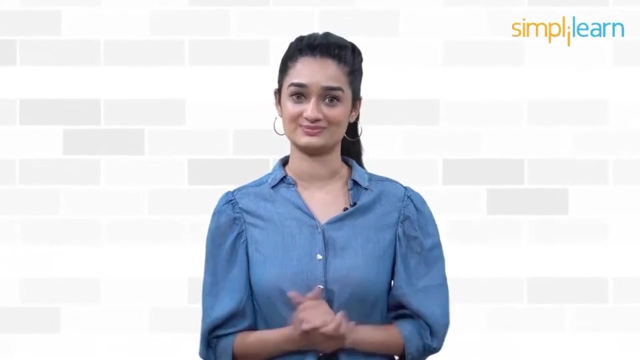 FarmWise intends to build innovative systems and efficient procedures that help farmers streamline farming with efficiency. FarmWise was established in the year 2020.. The company functions with 50 employees on board and actively looking for expansion. The company follows the procedure of paying farming equipment employees and contract personnel hourly. FarmWise makes an annual turnover of $8.5 million. On average, an AIML engineer at FarmWise earns anywhere around $113,000 per annum. Up next, we have AMP Robotics. At number 8, we have AMP Robotics. 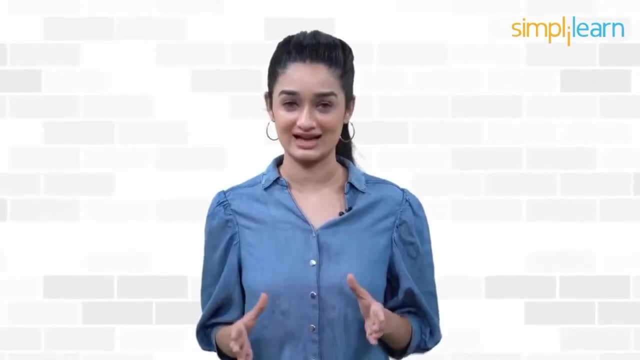 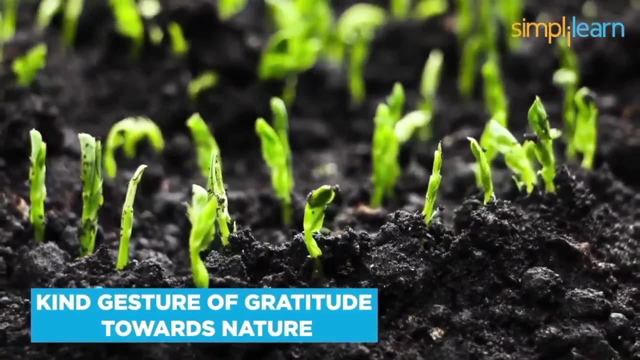 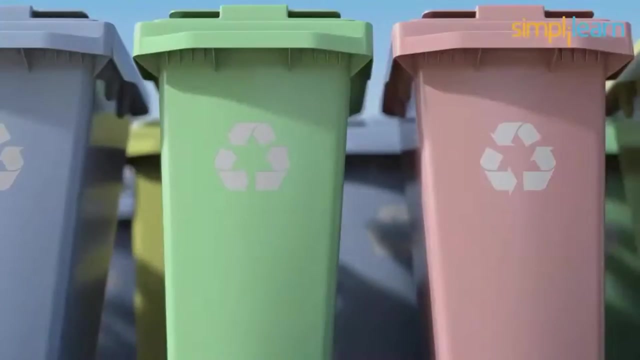 While others are busy trying to revolutionize mankind with AI. AMP Robotics came up with an innovative idea that happens to be a kind gesture of gratitude towards nature. AMP AI designed an artificial intelligence robo that recycles e-waste, plastic waste and waste from construction sites, and much more. 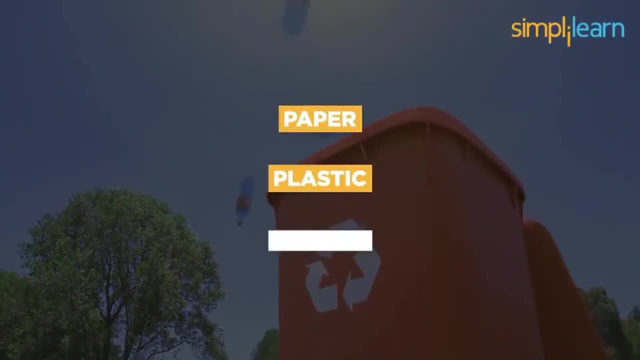 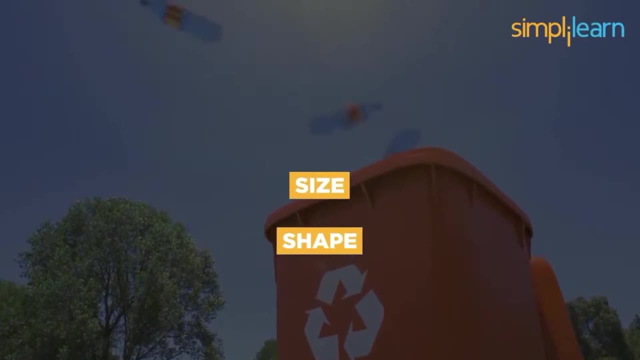 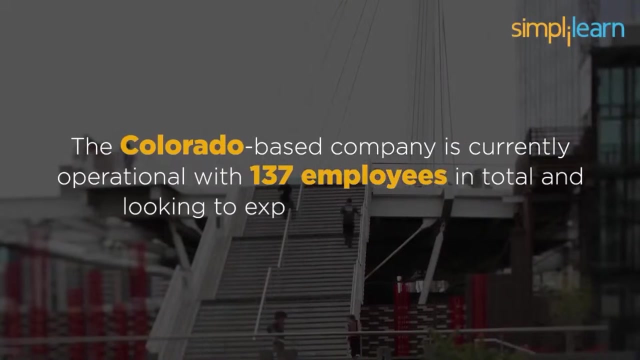 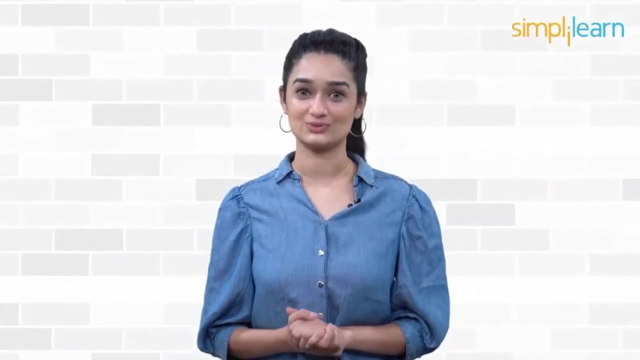 The robo precisely identifies paper, plastics and metals by learning and recognizing them via color, size, shape and a few more factors. The Colorado-based company is currently operational with 137 employees in total and looking forward to expand the idea globally. AMP Robotics aims to re-imagine recycling and to create a world without waste through artificial intelligence. AMP Robotics pays handsome salaries to their employees, with an average salary of an employee AMP Robotics varies between $96,000 to $131,000 per annum. Coming up next is a giant. At number 7, we have Automation Anywhere. Automation Anywhere is a global robotics automation and software company founded in the year 2003.. 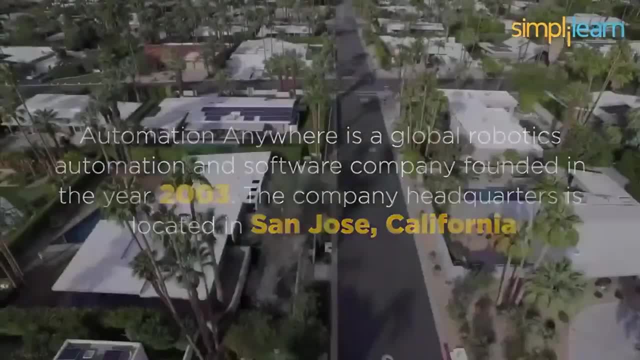 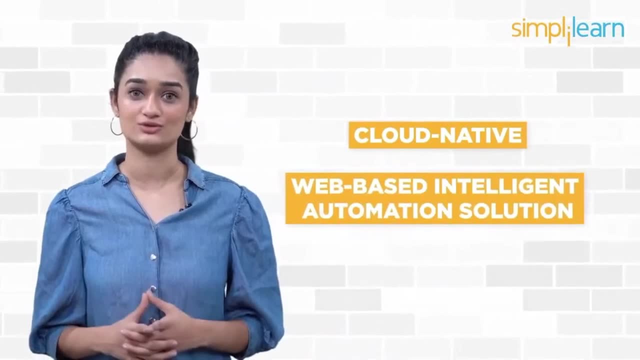 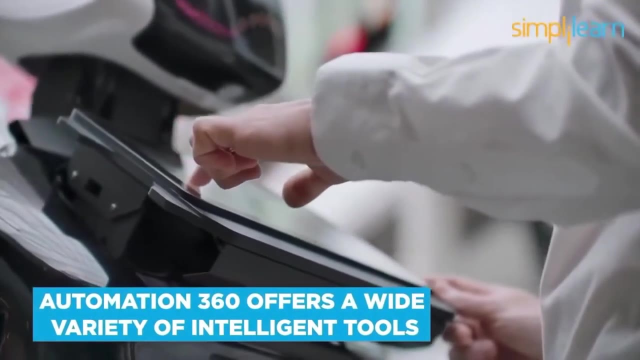 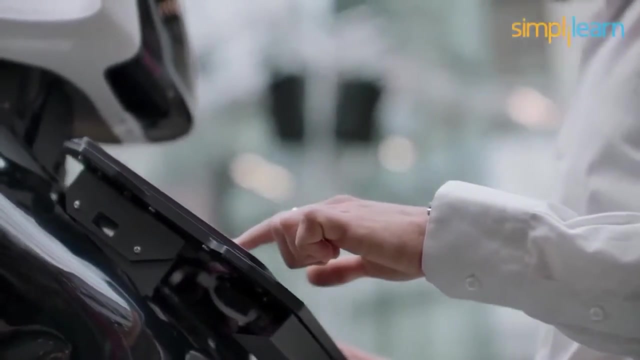 The company's headquarters is located in San Jose, California. The global RPA leader offers cloud-native, web-based intelligent automation solutions to the world's leading cloud companies. Automation Anywhere's. Automation360 offers a variety of intelligent tools and self-learning systems to automate every redundant task. 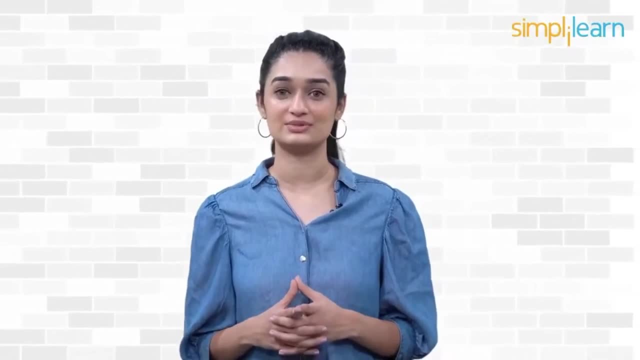 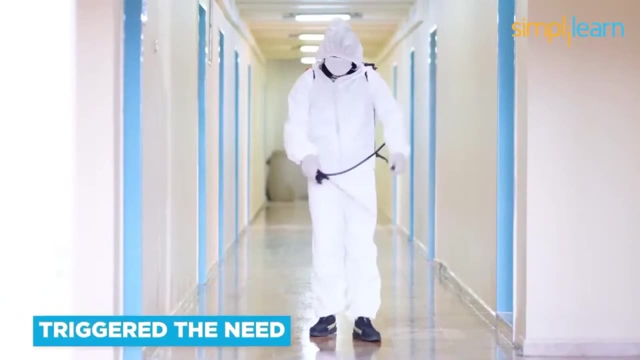 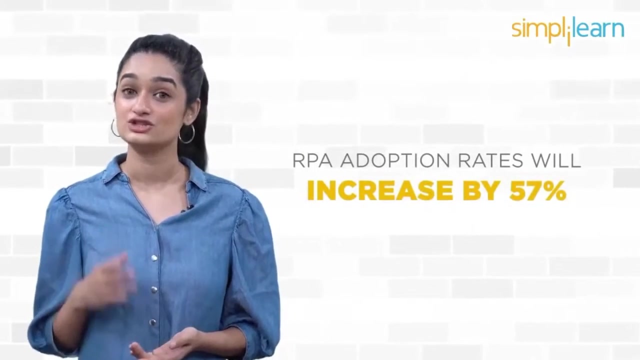 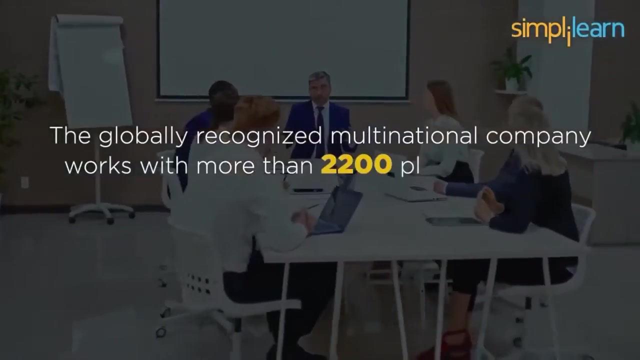 Automation Anywhere is focusing on transforming the companies to be RPA-oriented, and the current COVID situations have triggered the need for automation even more. A recent survey states the RPA adoption rates will increase by 57% in just one more year. The globally recognized multinational company works with more than 2,200 plus employees on board. 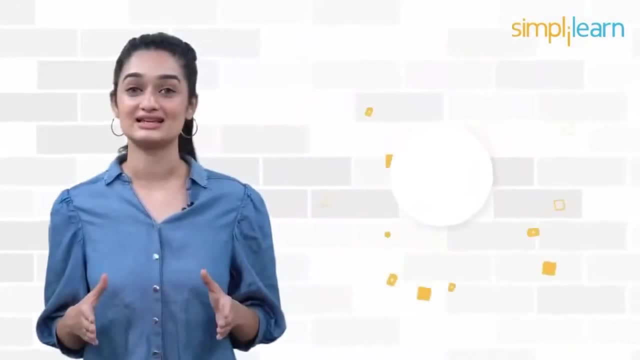 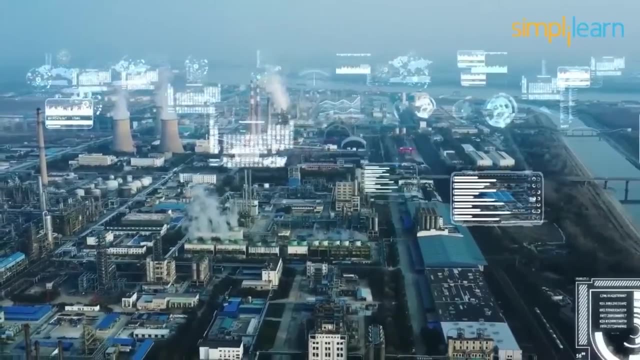 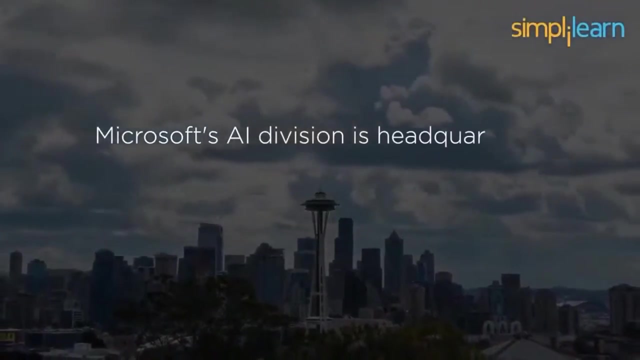 The company pays decent salaries as well. At number 6, we have Microsoft AI. Microsoft integrated AI into cloud computing. Microsoft's AI platform provides robust solutions to cloud-related problems. Microsoft's AI division is headquartered in Redmond, Washington, with around 5,000 employees. 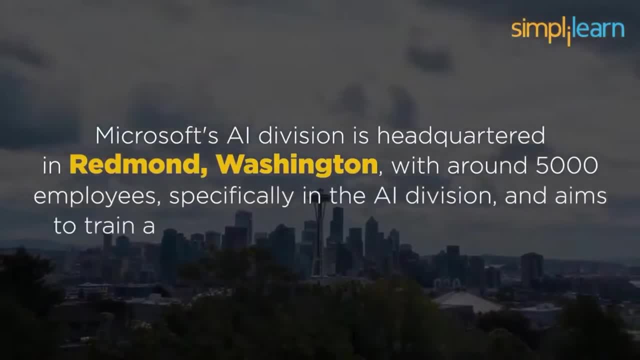 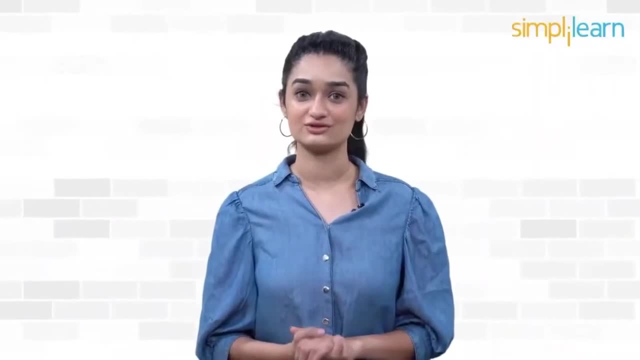 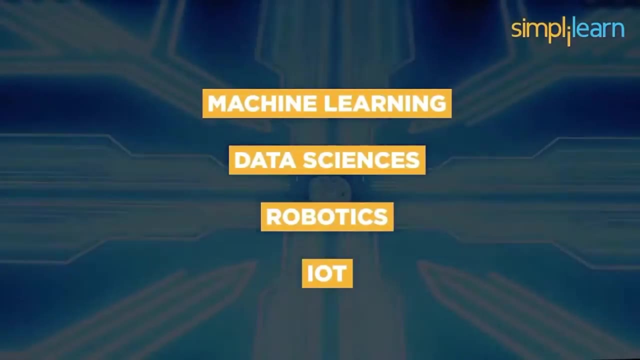 specifically in the AI division and aims to train and certify 15,000 employees by 2022.. Microsoft AI is a robust framework designed for developing AI solutions. using machine learning, data science, robotics, IoT and more AI-enabled services accelerate productivity to a greater level. 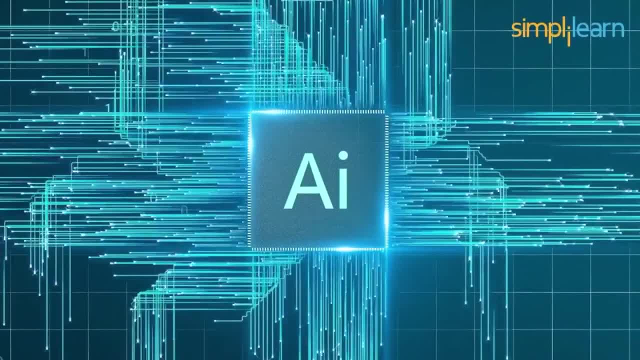 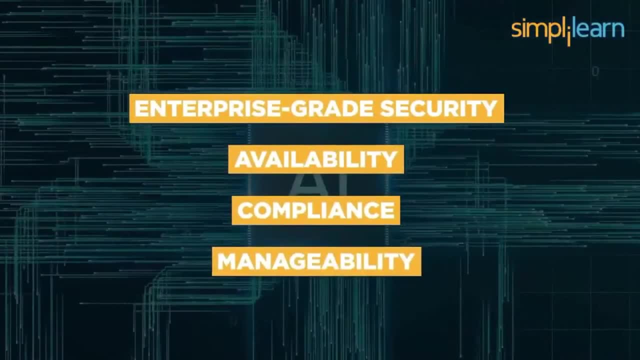 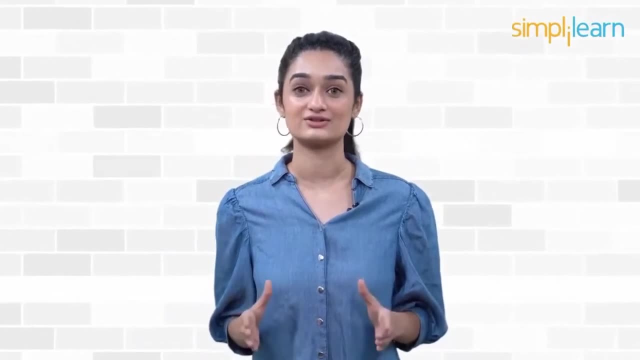 Microsoft Azure uses AI to get best-of-breed infrastructure with enterprise-grade security, availability, compliance and manageability. Microsoft also pays handsome salaries to their employees. The average salary of an employee at the Microsoft AI division earns up to $160,000 per annum. 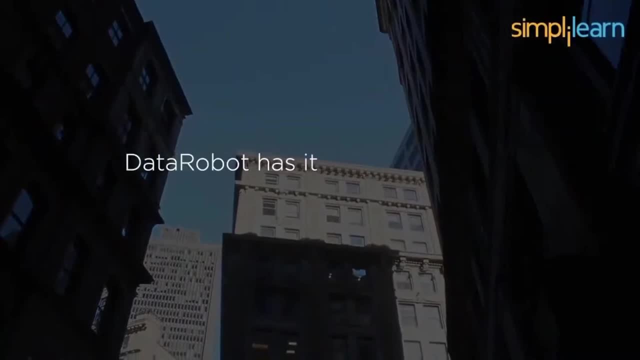 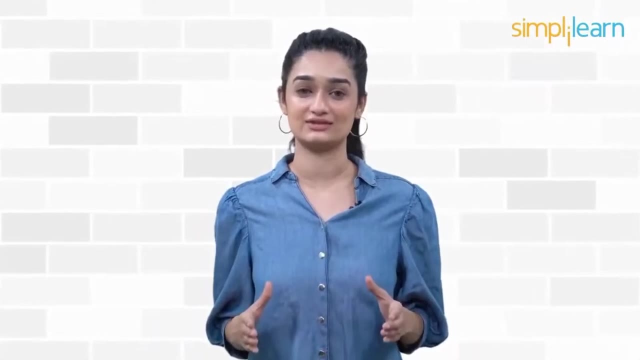 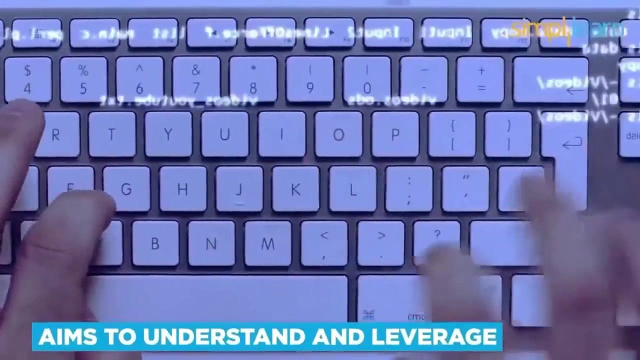 At number 5, we have DataRobo. DataRobo has its headquarters in Boston. It is one of the AI cloud leaders, providing a unified platform for the delivery of AI to the cloud. DataRobo aims to understand and leverage the inherent capabilities of the platform. 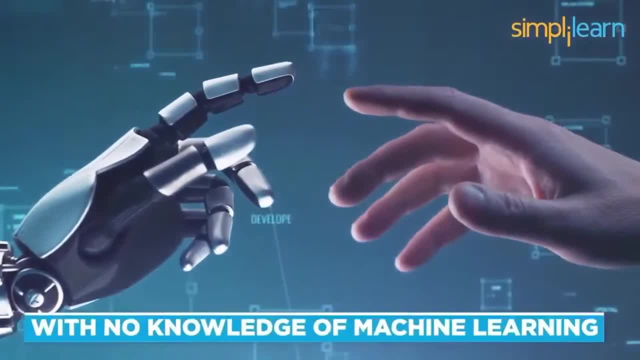 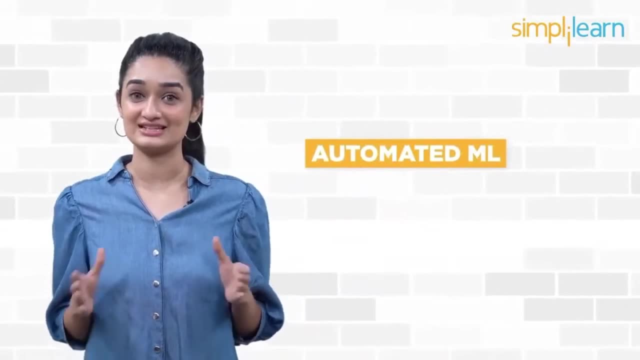 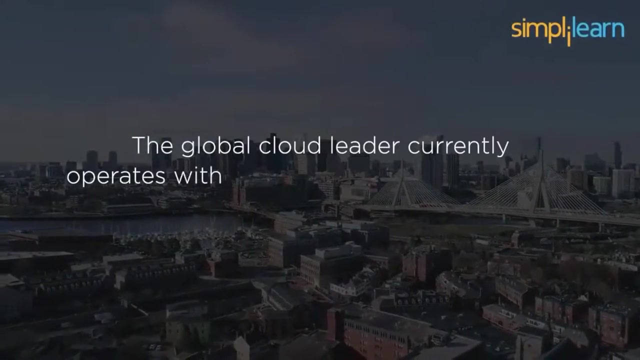 DataRobo has the caliber to help business analysts in building predictive analytics with no knowledge of machine learning. It uses automated ML to build and deploy accurate predictive models in a short span of time. The global cloud leader currently operates with more than 1,000 employees worldwide. DataRobo compensates its employees with handsome salaries. An average employee at DataRobo earns up to $160,000 per year and up to Rs 3,400,000 in India. At number 4, we have Amazon, The Alexa maker. Amazon is one of the tech giants interested in adopting AI into its various divisions. 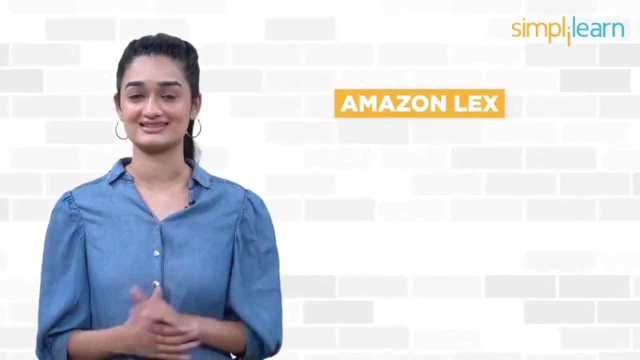 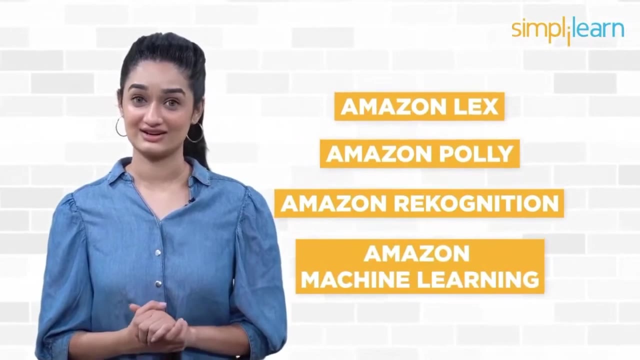 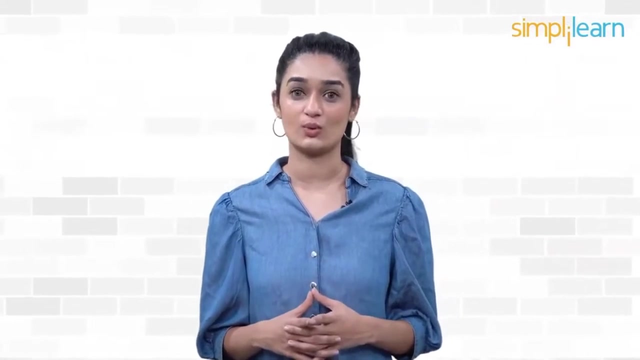 Amazon calls its AI services Amazon Lex, Amazon Polly, Amazon Recognition and Amazon Machine Learning. These services are accessible through a software API call or console. The Amazon AI suite of services can have text or voice conversations with an end user using a conversational chat ops interface. 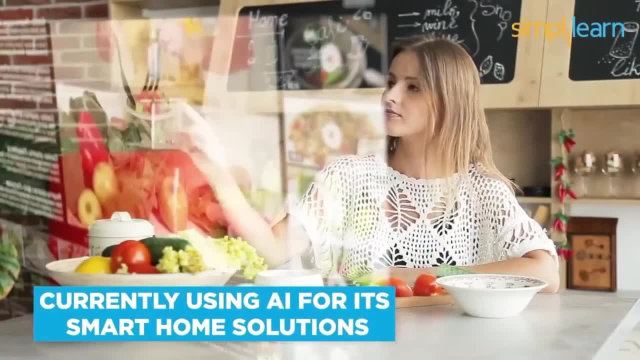 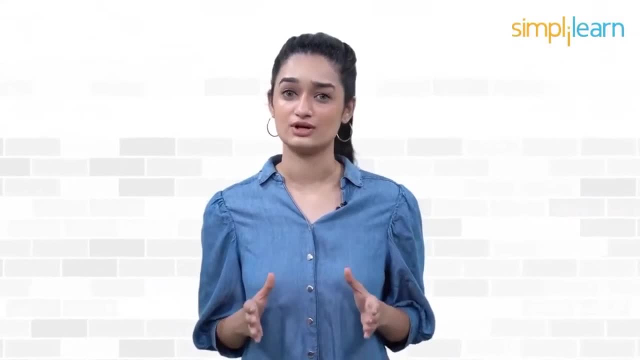 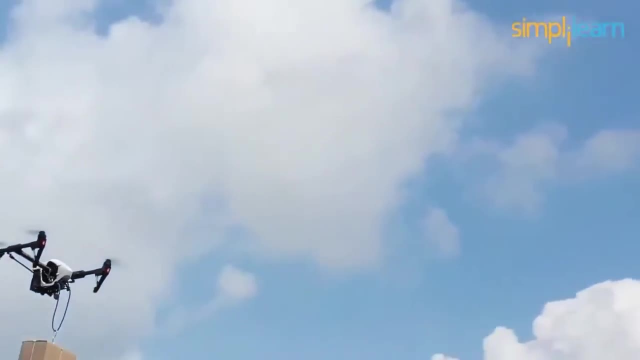 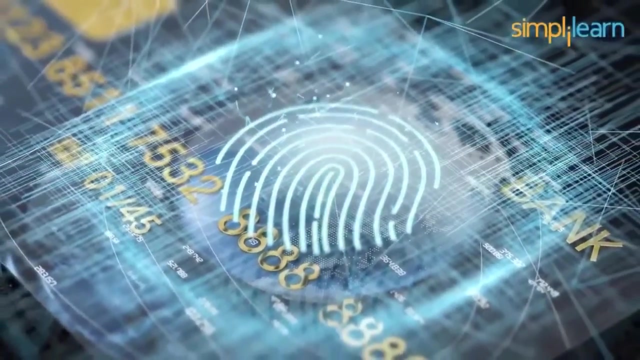 The Seattle-based tech giant is currently using AI for its smart home solutions, AI companies like Alexa and its business intelligence needs. Amazon is also conducting trials on drone delivery to save time and efforts to deliver goods and services to remote locations with ease. Amazon AI aims to provide biometric payments to its customers at cash-free stores. 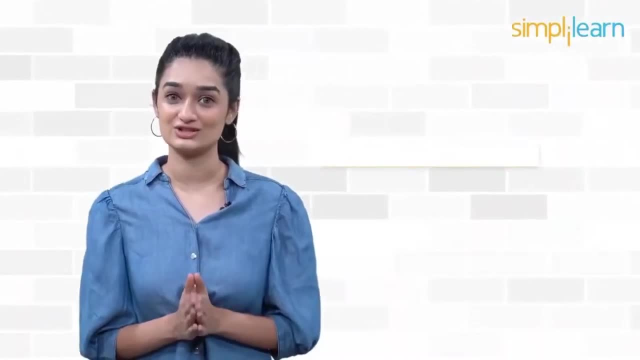 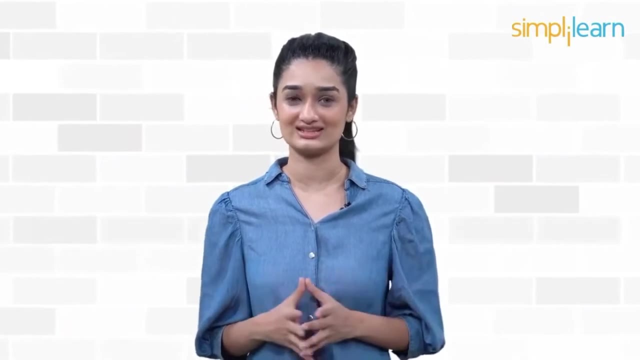 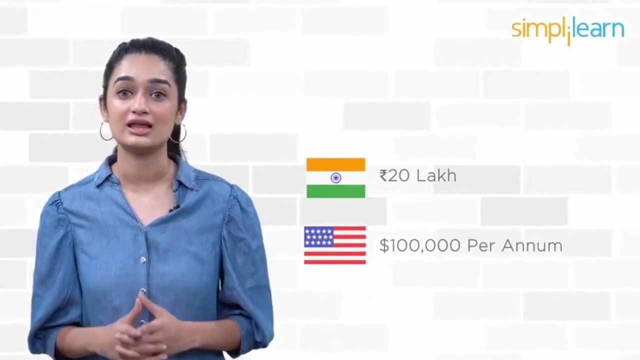 The approach is still in trials. Amazon calls it Just Walk Out technology. Amazon has enormous teams and pays decent salaries to its employees. For example, an employee at Amazon can earn up to Rs 20 lakh per annum in India and about $100,000 per annum in the United States of America. At number 3, we have Dell. Dell is one of the best data-driven companies. Dell lake houses combine data warehouses, reliability, performance and governance with the openness and flexibility of Dell lakes. Dell is headquartered in San Francisco, California, and has 15 office locations across 11 countries. 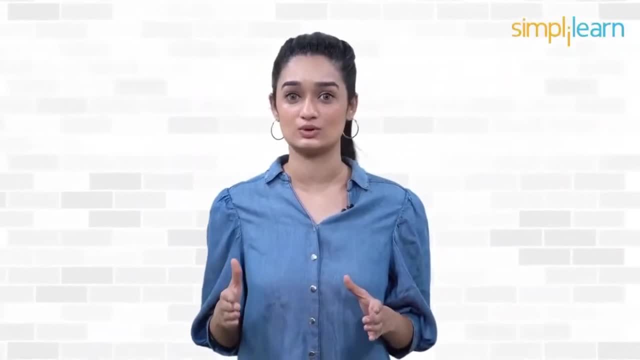 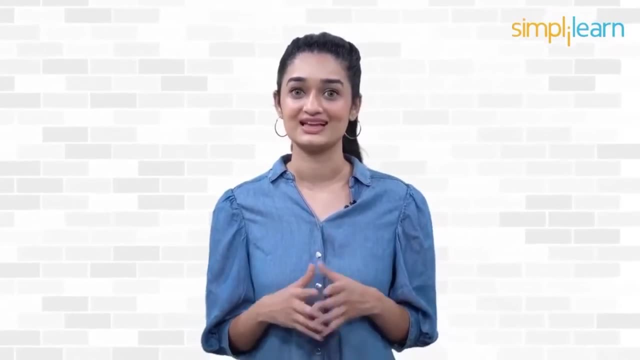 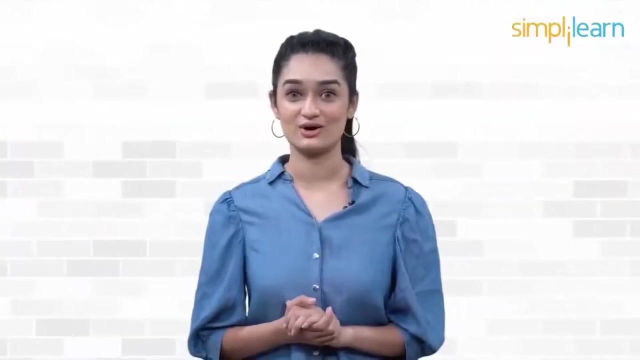 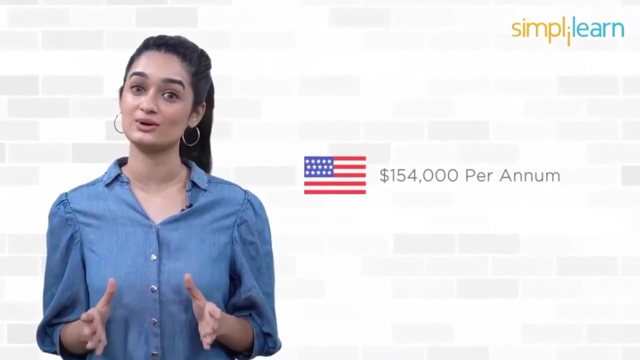 Dell announces plans on delivering keynote on data and machine learning product innovations and the rise of the lake house architecture advancements. Databricks currently operates with 2,000 plus employees globally. The organization compensates its employees with handsome salaries. An average employee at Databricks makes about 154,000 US dollars and around 2.1 lakh rupees per annum in India. 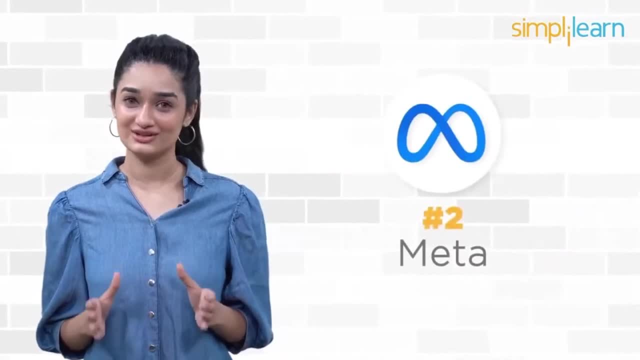 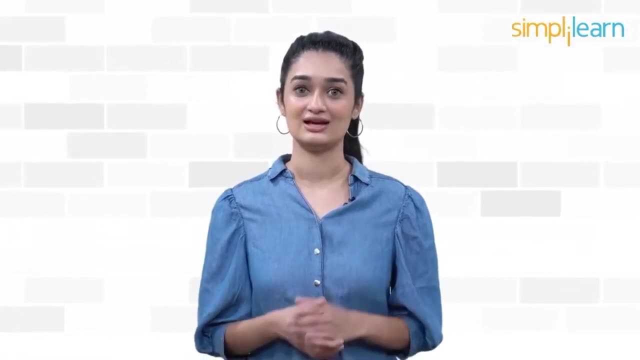 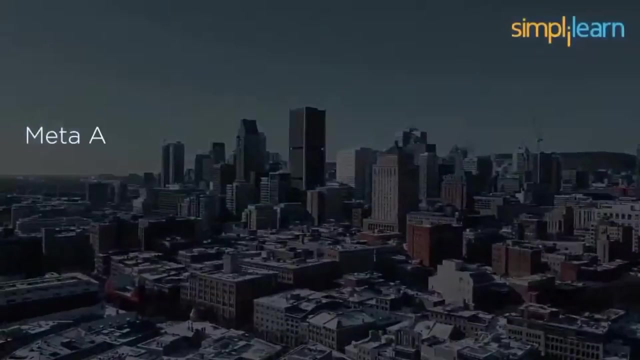 Next we have Meta. At number 2, we have Meta. Meta, formerly known as Facebook, is innovating an advanced way of social interaction. Meta has integrated artificial intelligence and is being called the Meta AI. Meta AI has its headquarters in Toronto, Canada. 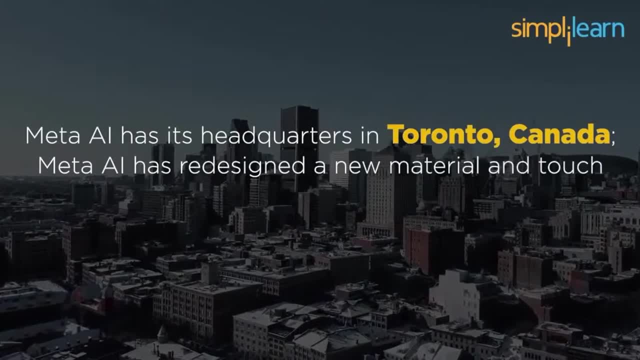 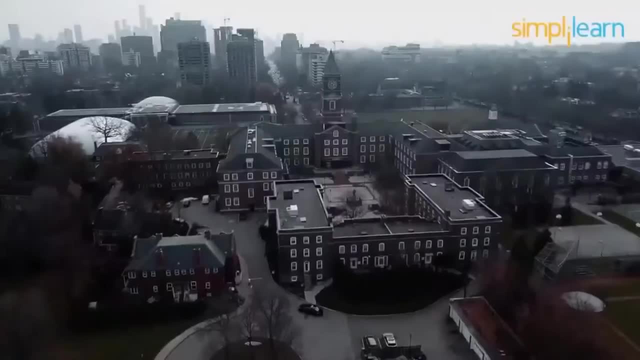 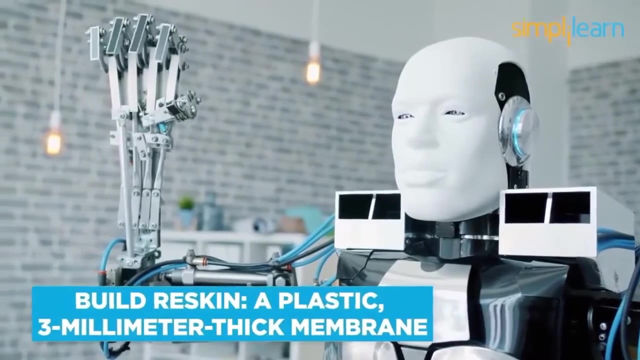 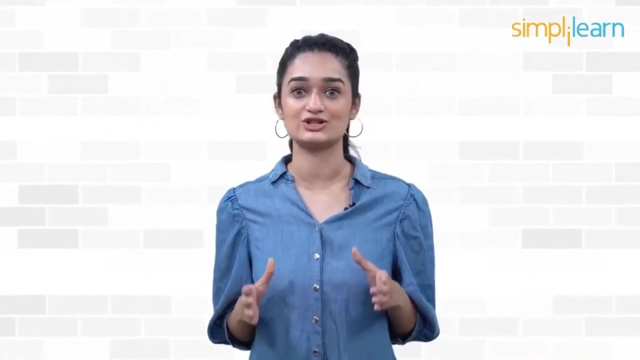 Meta AI has redesigned a new material and touch sensor with potential to boost the development of Metaverse. A team of researchers at the Metaverse have worked jointly with scientists at Carnegie Mellon University to build Reskin, a plastic 3mm thick membrane with magnetic particles capable of measuring touch and sensation. A thrilling experiment Meta has under its sleeve, I would say. Meta currently operates remotely, with about 350 employees on board. Critics also state that Meta pays a vast salary to its AI experts, with an average salary of $1,750,000 paid to the employees at Meta AI. 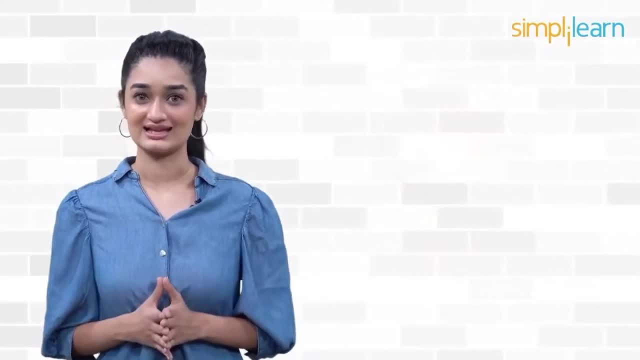 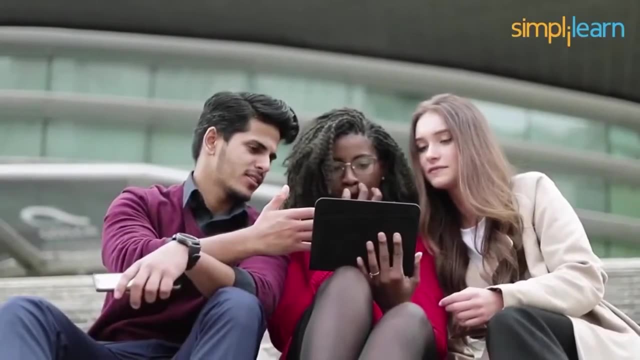 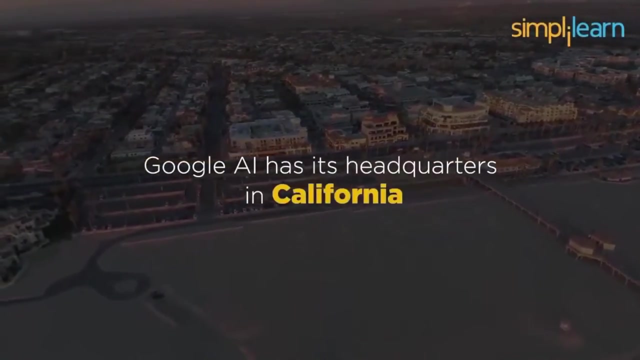 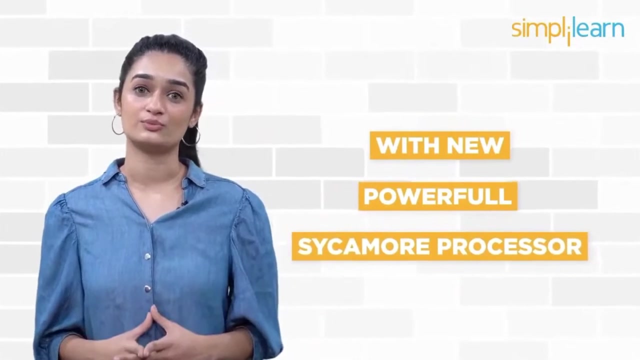 At number 1, we have Google AI. Google AI is the division of Google dedicated to artificial intelligence. CEO Sundar Pichai announced it at Google IO 2017.. Google AI has its headquarters in California. Google AI is demonstrating its quantum computing supremacy with its new and powerful CineMore processor. 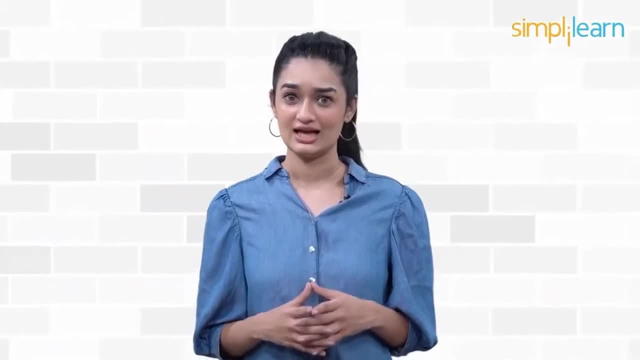 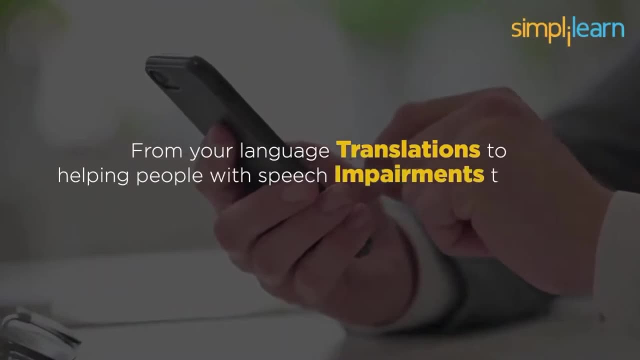 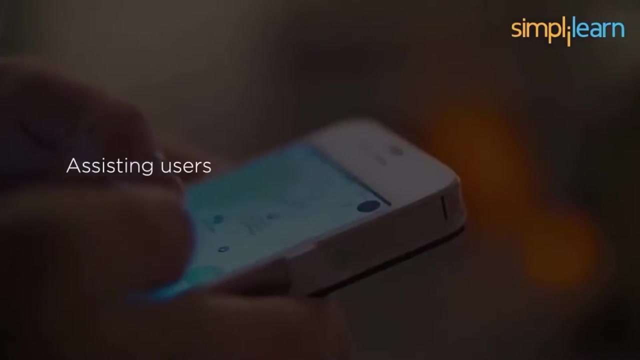 Google's AI is one of the most widespread technologies. It's almost everywhere, from your language translations to helping people with speech impairments to have a successful conversation, social media interactions, shopping lists and assisting users with GPS sending alerts to its users about natural calamities. 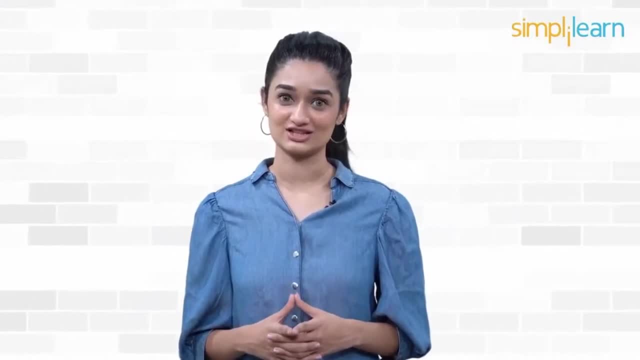 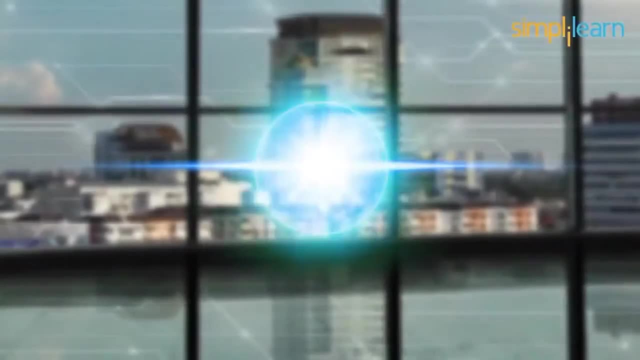 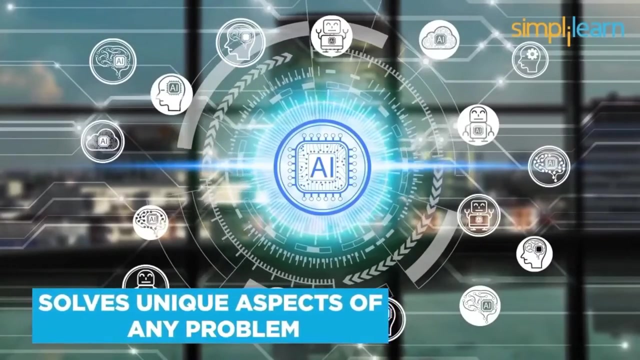 And saving them. Google AI has announced that its research team is designing next-generation AI chips for a smart future. In addition, a new AI model allows artificial intelligence to perform chip design that more efficiently solves unique aspects of any problem with an artificial neural network. 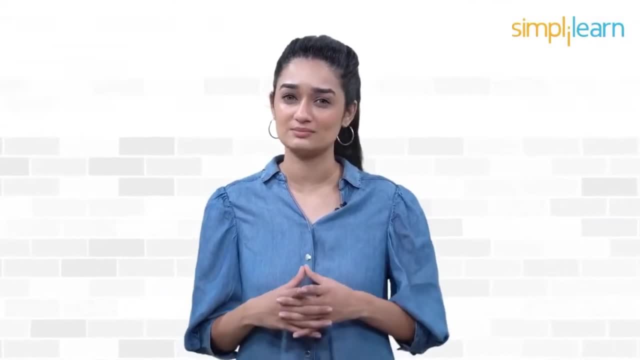 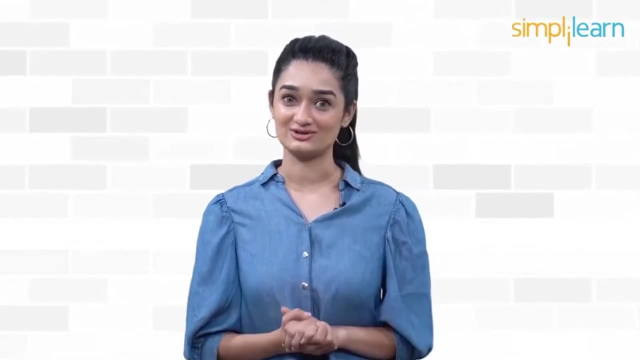 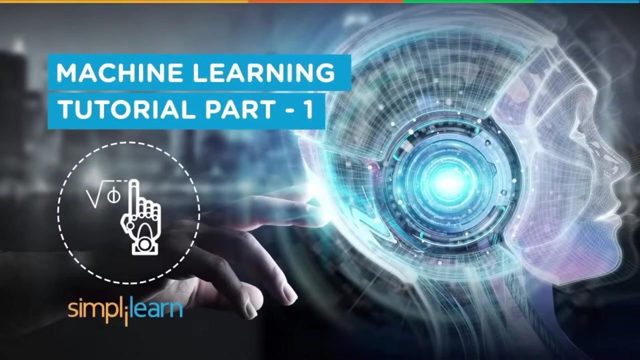 Google AI currently works with our four divisions with massive teams. We have come to an end of this session on the top 10 AI companies to watch out for in 2022.. Hello and welcome to Machine Learning Tutorial Part 1.. This is part 1 of a machine learning series put on by SimplyLearn. 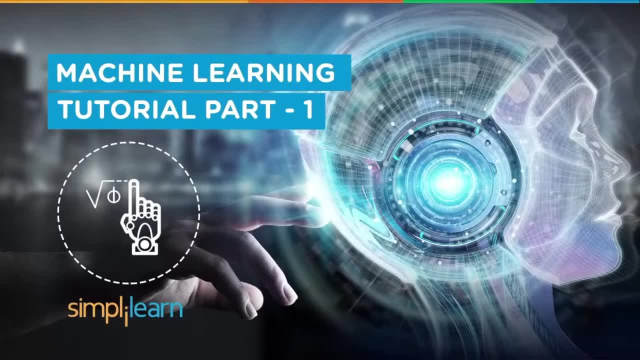 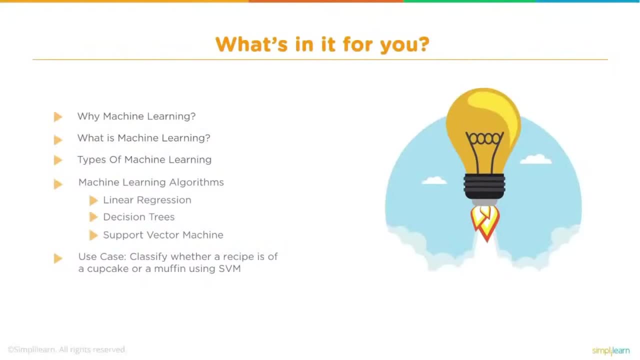 My name is Richard Kirschner. I'm with the SimplyLearn team. That's wwwsimplylearncom. Get certified, Get ahead. What's in it for you today? Well, we'll start off with a brief explanation of why machine learning and what is machine learning? 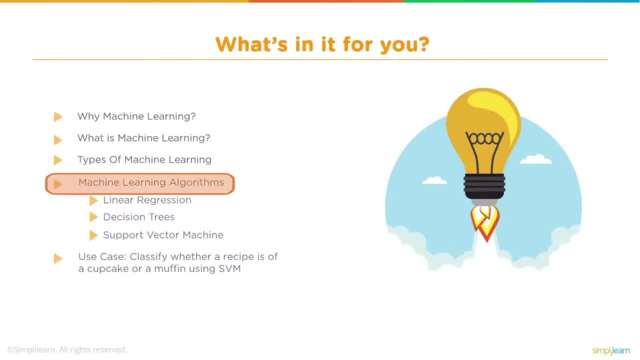 And then we'll get into a few of the types of machine learning: Machine learning algorithms, linear regression, decision trees, support vector machine And finally, we'll do a use case where we're going to classify whether a recipe is of a cupcake or a muffin using the SVM or the support vector machine. 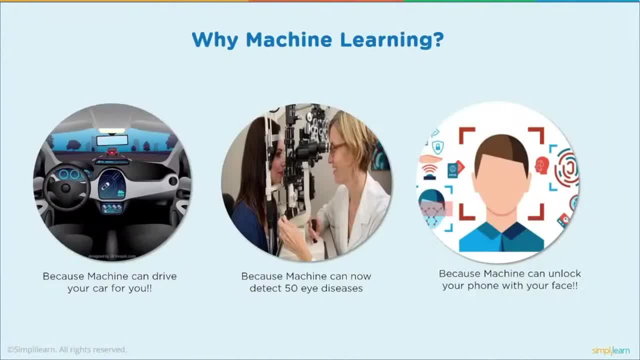 Sounds like a delicious way to explore machine learning. So why machine learning? Why do we even care about having these computers come up and be able to do all these new things for us? Well, because machines can now drive your car for you. It's still very in the infant stage, but it's just exploding, as we see with Google's Waymo. and then Uber had their program, which unfortunately crashed. 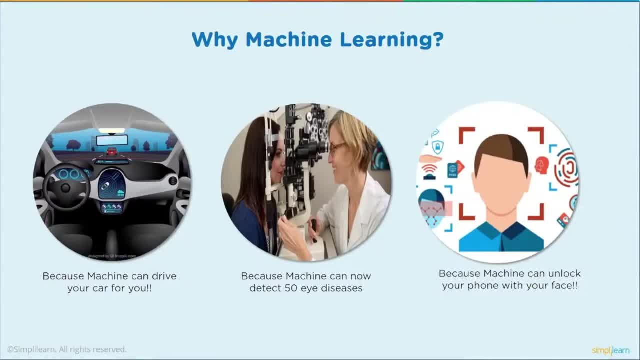 They know that this is huge. This is going to be the huge industry to change our whole transportation infrastructure. Machine learning is now used to detect over 50 eye diseases. Do you know how amazing that is to have a computer that double checks for the doctor for things they might miss? 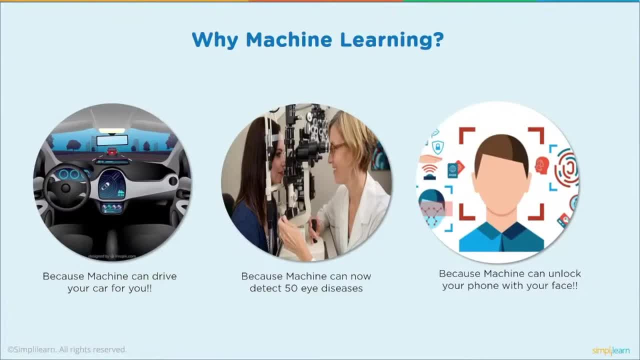 That's just huge in the health industry. Pretty soon they actually do already have that in some areas where- maybe not for eyes but for other diseases- where they're using the camera on your phone to help pre-diagnose before you go in and see the doctor. 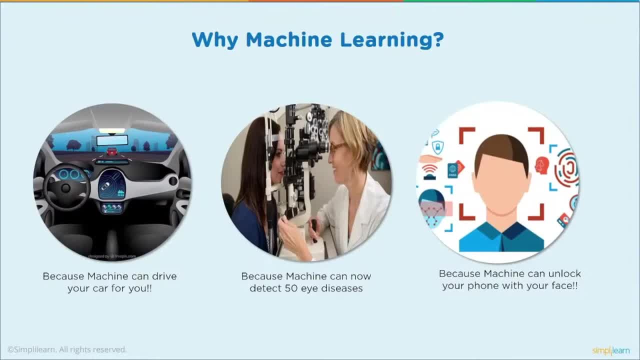 And because the machine can now unlock your phone with your face. I mean that's just cool Having it being able to identify your face or your voice and be able to turn stuff on and off for you, depending on where you're at and what you're doing. 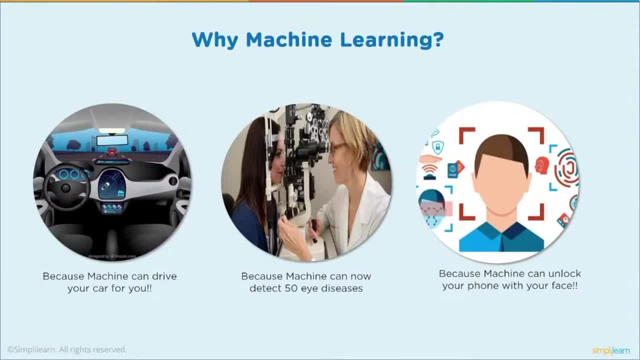 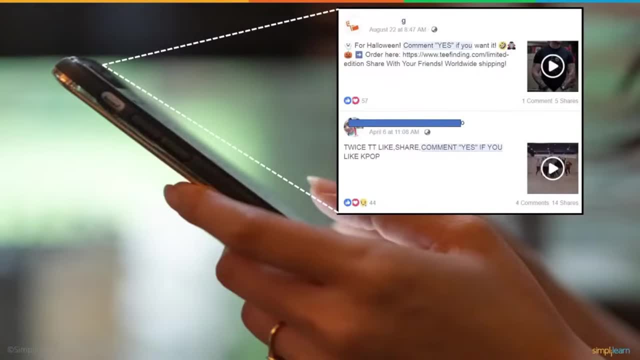 Talk about what you need. Talk about an ultimate automation in our world we live in And as we dig in deeper, we have a nice example of Facebook, As you can see here. they have the Facebook post with Halloween Comment: yes, if you want it. 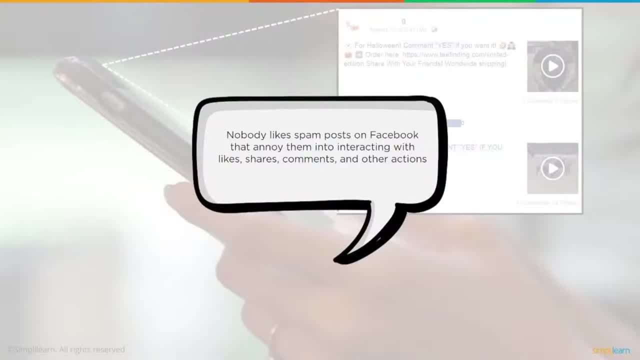 Order here. Nobody likes spam posts on Facebook that annoy them into interacting with likes, shares, comments and other actions. I remember the original ones were all: if you don't click on here, you will have bad luck or some kind of fear factor. 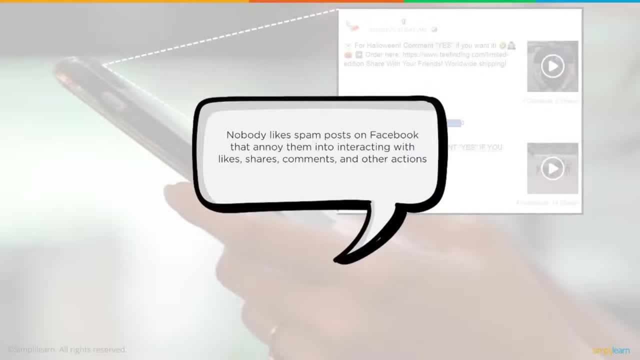 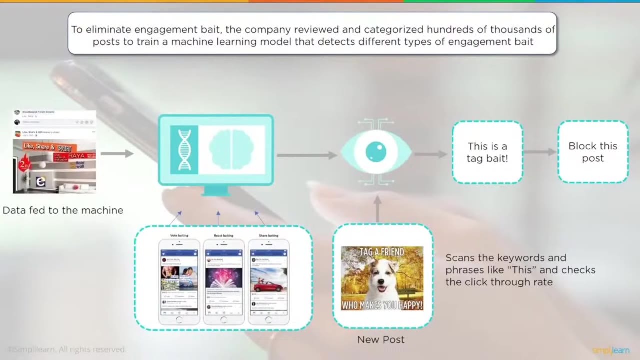 Well, this is a huge thing in social media when people are getting spammed, And so this tactic known as engagement bait takes advantage of Facebook's newsfeed algorithm by choosing engagement in order to get the greater reach. To eliminate engagement bait, the company reviewed and categorized hundreds of thousands of posts to train a machine learning model that detects different types of engagement bait. 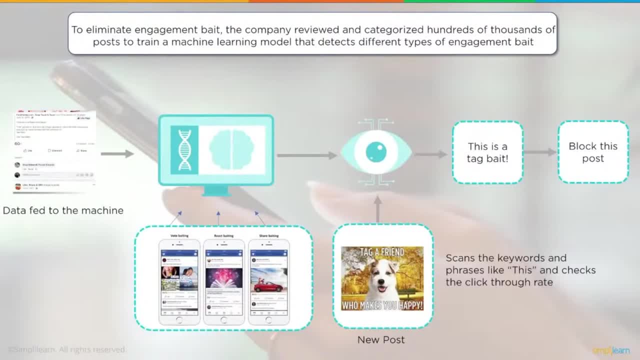 So in this case we have, we're using Facebook, but this is, of course, across all the different social media. They have different tools, they're building And the Facebook scroll GIF will be replaced, kind of like a virus coming in there. 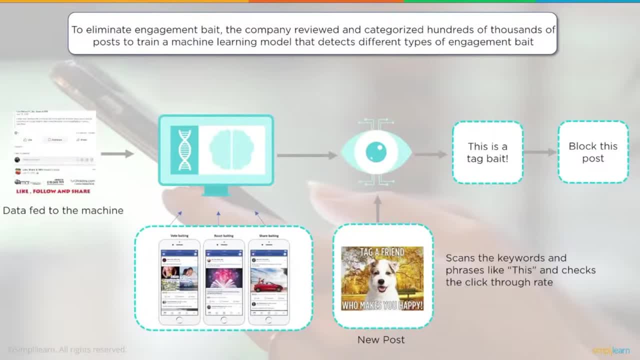 It notices that there's a certain setup with Facebook and it's able to replace it. And they have like vote baiting, react baiting, share baiting, They have all these different. these are kind of general titles, But there certainly are a lot of way of baiting you to go in there and click on something. 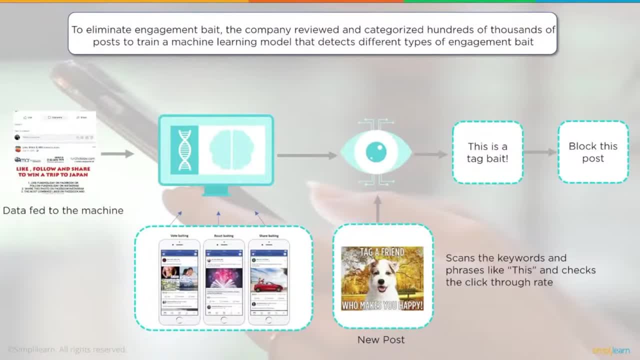 So they fed all this. This data was fed into the machine, And then they have the new post That takes over part of the Facebook setup, And that's what you're looking at. You're looking at this new post that's replaced, like a virus has replaced that. 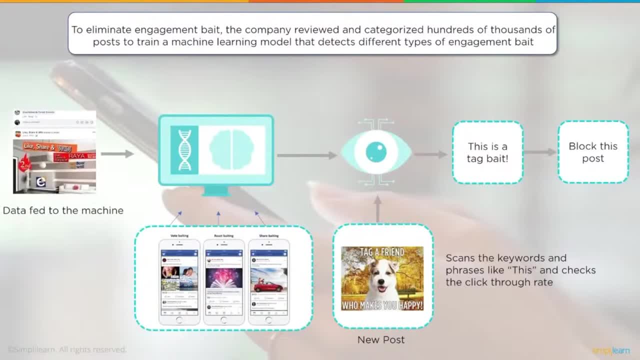 So what Facebook did to eliminate this is they start scanning for keywords and phrases like this and checks the click through rate, So it starts looking for people who are clicking through it without even looking at it or clicking through it, and it's not something that normally would be clicked through. 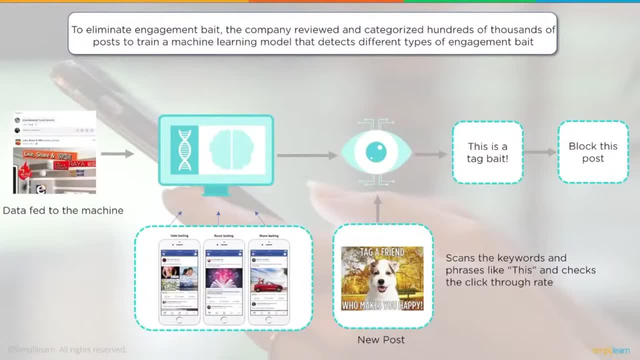 Once Facebook has scanned for these keywords and phrases, it is now able to identify the spam coming in, And this makes your life easier. It's not like spam, It's not like walking through an airport and in a lot of countries, you have like hundreds of people trying to sell you timeshare. 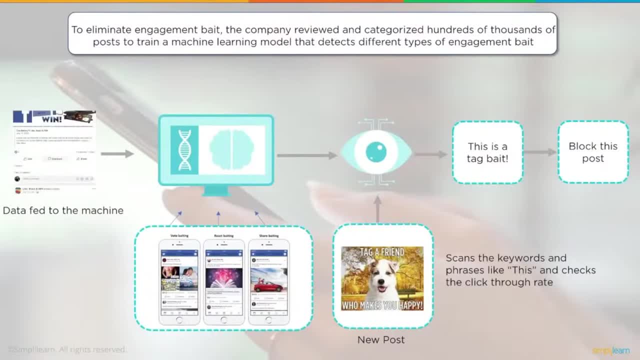 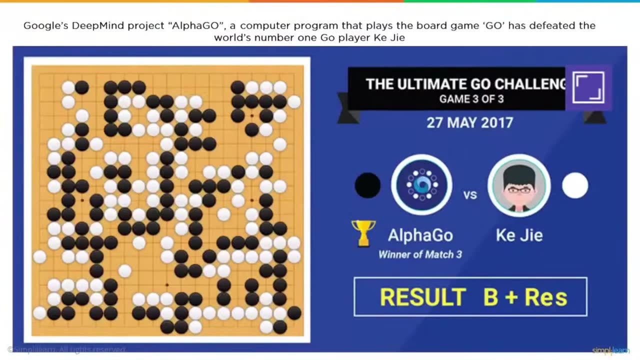 Come join us. Sign up for this. It eliminates that annoyance. so now you can just enjoy your Facebook and your cat pictures- Or maybe it's your family pictures- Mine is family. Certainly people like their cat pictures too. Another good example is Google's deep mind project AlphaGo. 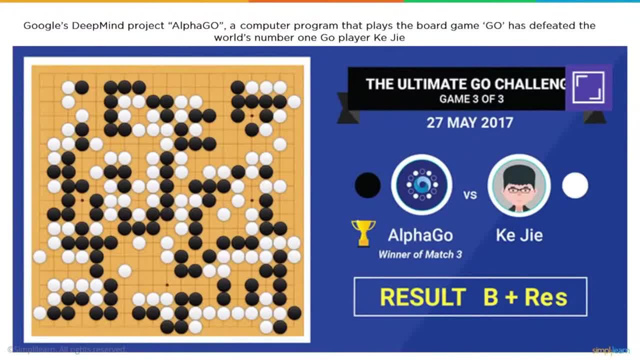 A computer program that plays a board game. Go has defeated the world's number one Go player, And I hope I say his name right. The ultimate Go challenge game of three of three was on May 27th 2017.. So that was just last year that this happened. 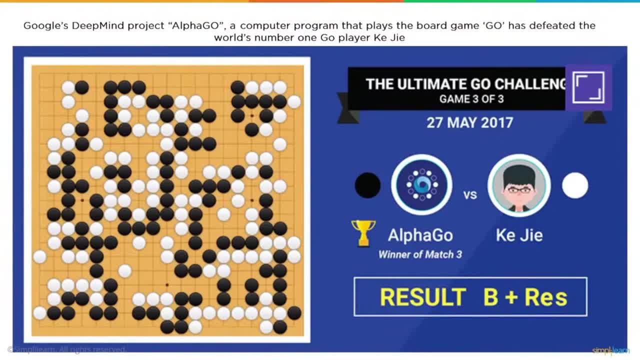 And what makes this so important is that you know, Go is just a game, So it's not like you're driving a car or something in our real world, But they are using games to learn how to get the machine learning program to learn. 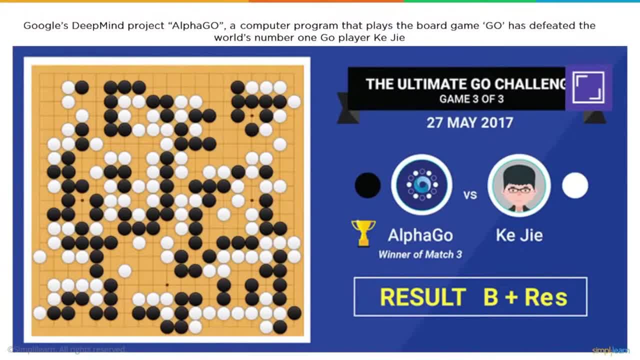 They want it to learn how to learn, And that is a huge step. A lot of this is still in its infant stage as far as development, As we saw what happened with the- as I referred to earlier- the Uber cars. They lost their whole division because they jumped ahead too fast. 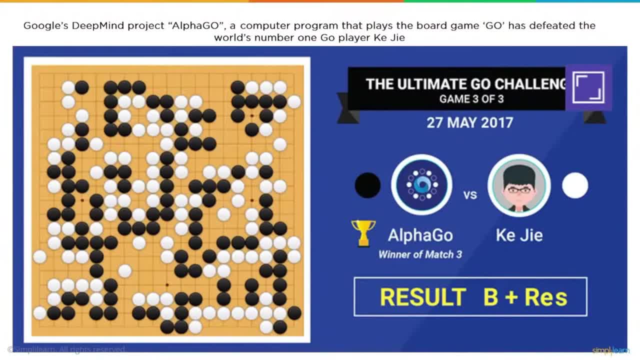 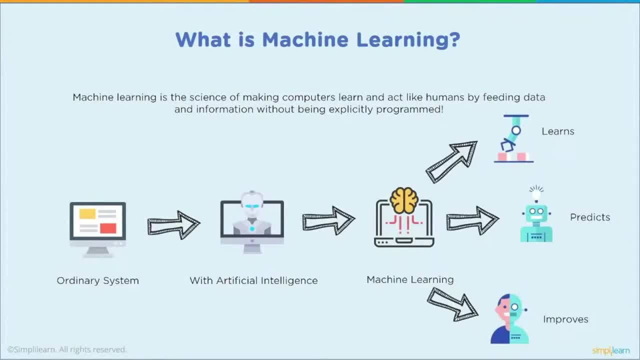 So still in infant stage. But boy is this like the beginning of just an amazing world that is automated in ways we can't even imagine what tomorrow is going to look like. We've looked at a lot of examples of machine learning, So let's see if we can give a little bit more of a concrete definition. 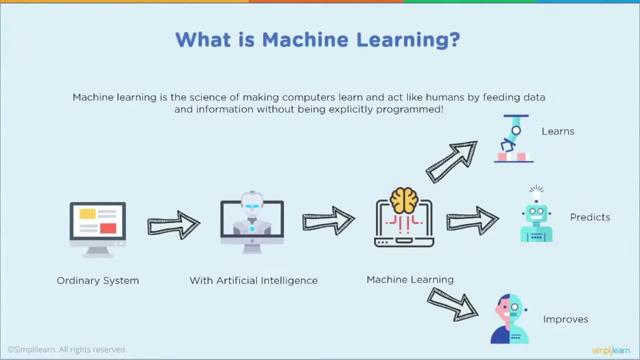 What is machine learning? Machine learning is the science of making computers learn and act like humans by feeding data and information without being explicitly programmed. We see, here we have a nice little diagram where we have our ordinary system, Your computer. nowadays you can even run a lot of this stuff on a cell phone, because cell phones have advanced so much. 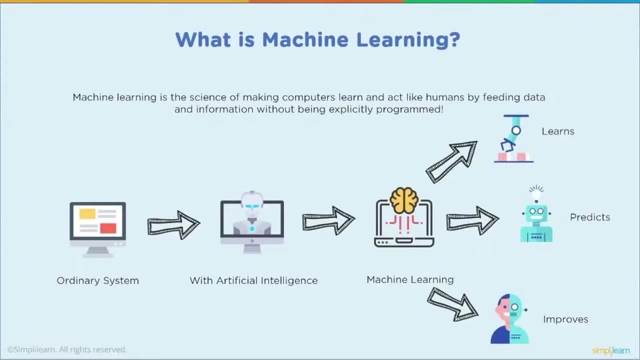 And then with artificial intelligence and machine learning, it now takes the data and it learns from what happened before And then it predicts what's going to come next. And then really the biggest part right now in machine learning that's going on is it improves on that. 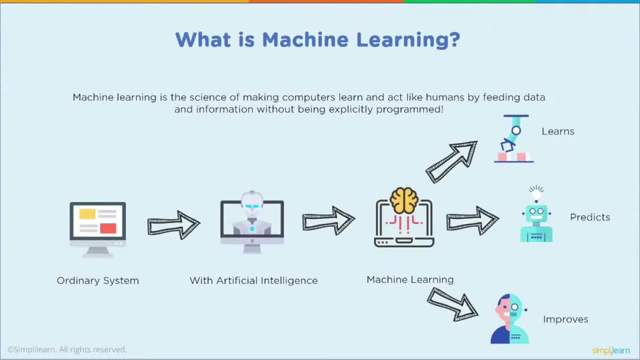 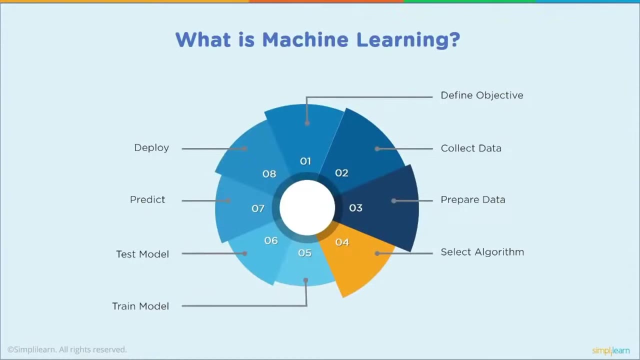 How do we find a new solution? So we go from descriptive, where it's learning about stuff and understanding how it fits together, to predicting what it's going to do, to postscripting- coming up with a new solution. And when we're working on machine learning, there's a number of different diagrams that people have posted for what steps to go through. 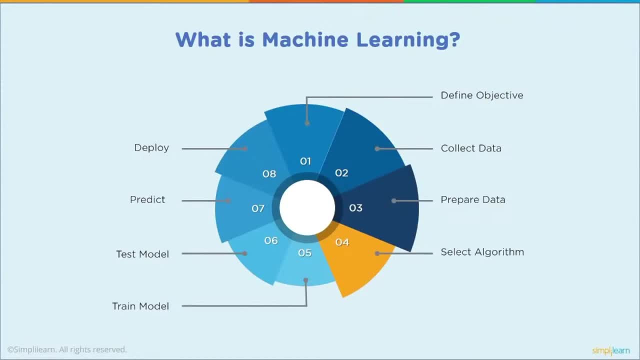 A lot of it might be very domain specific. So if you're working on photo identification versus language, versus medical or physics, some of these are switched around a little bit or new things are put in that are very specific to the domain. This is kind of a very general diagram. 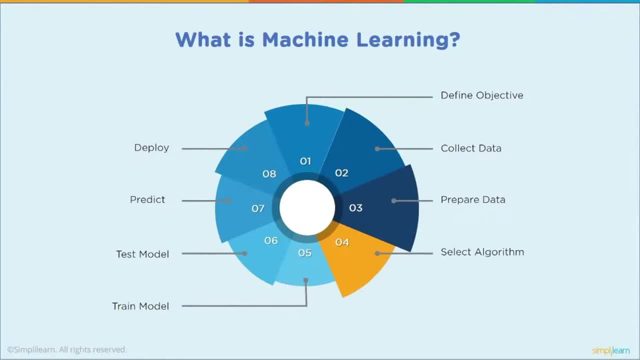 First you want to define your objective. Very important to know what it is you're wanting to predict. Then you're going to be collecting the data. So once you've defined an objective, you need to collect the data that matches. You spend a lot of time in data science collecting data. 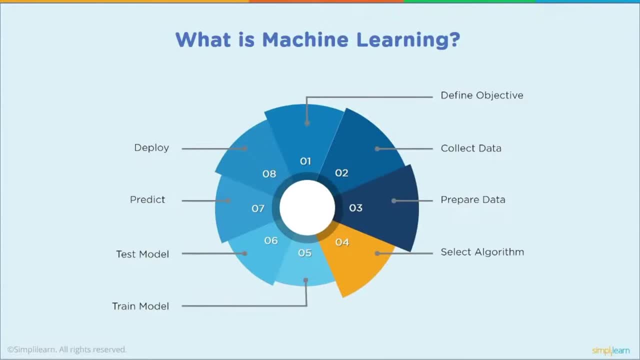 And the next step, preparing the data. You want to make sure that your data is clean, going in. There's the old saying: bad data in, bad answer out Or bad data out. And then, once you've gone through and we've cleaned all this stuff coming in, then you're going to select the algorithm. 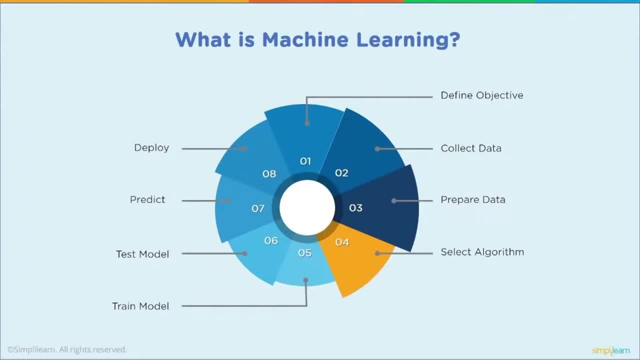 Which algorithm are you going to use? You're going to train that algorithm. In this case, I think we're going to be working with SVM, the support vector machine. Then you have to test the model. Does this model work? Is this a valid model for what we're doing? 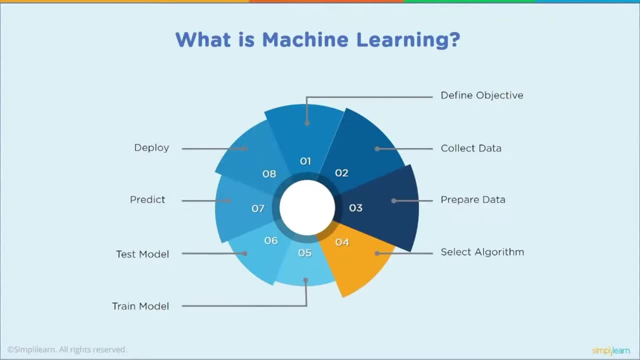 And then, once you've tested it, you want to run your prediction. You want to run your prediction or your choice, or whatever output it's going to come up with, And then, once everything is set and you've done lots of testing, then you want to go ahead and deploy the model. 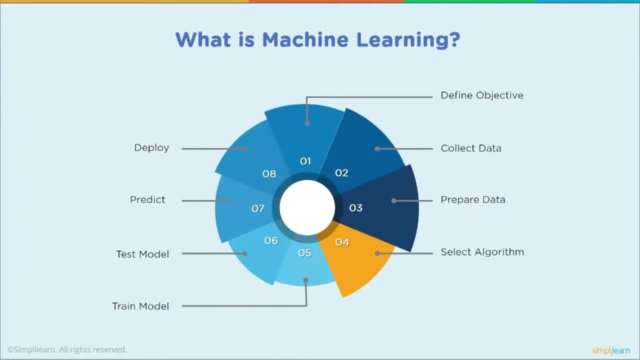 And remember I said domain specific. This is very general. as far as the scope of doing something, A lot of models you get halfway through and you realize that your data is missing something And you have to go collect new data because you've run a test in here someplace along the line. 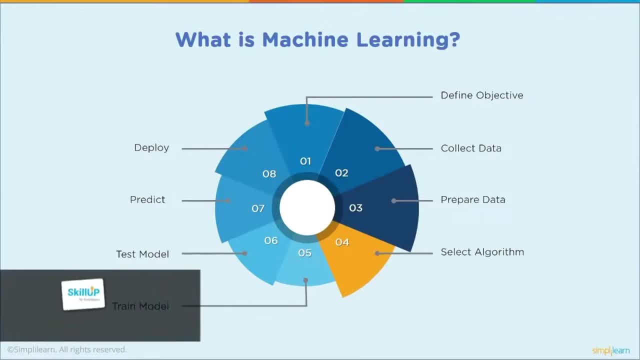 You're saying, hey, I'm not really getting the answers I need. So there's a lot of things that are domain specific that become part of this model. This is a very general model, but it's a very good model to start with. 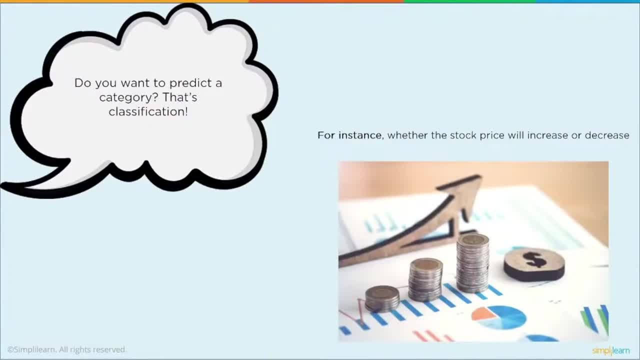 And we do have some basic divisions of what machine learning does. that's important to know. For instance, do you want to predict a category? Well, if you're categorizing things, that's classification, For instance, whether the stock price will increase or decrease. 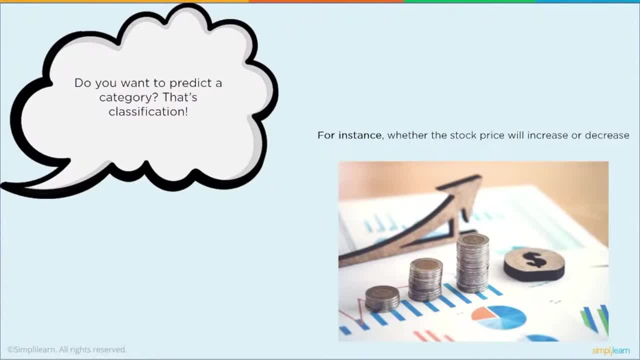 So in other words, I'm looking for a yes-no answer. Is it going up or is it going down? And in that case we'd actually say: is it going up, True? If it's not going up, it's false meaning, it's going down. 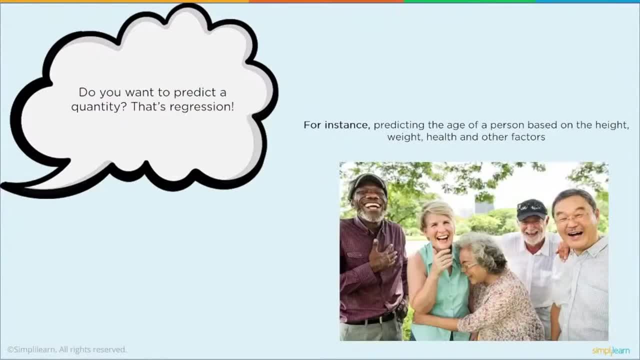 This way, it's a yes-no- 0-1.. Do you want to predict a quantity? That's regression. So remember, we just did classification, Now we're looking at regression. These are the two major divisions in what data is doing. 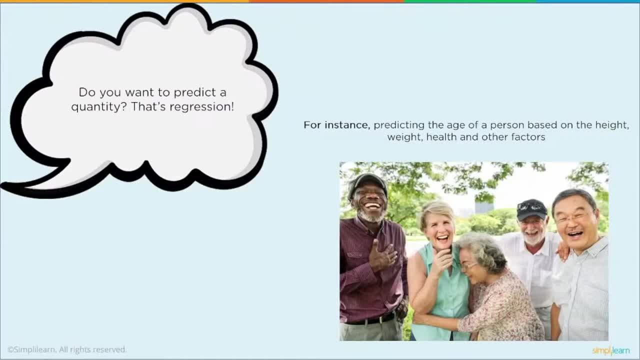 For instance, predicting the age of a person based on the height, weight, health and other factors. So, based on these different factors, you might guess how old a person is. And then there are a lot of domain, specific things Like: do you want to detect an anomaly? 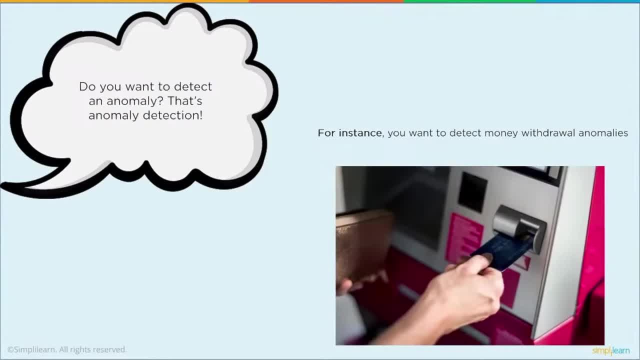 That's anomaly detection. This is actually very popular right now. For instance, you want to detect money withdrawal anomalies. You want to know when someone's making a withdrawal that might not be their own account. We've actually brought this up because this is really big right now. 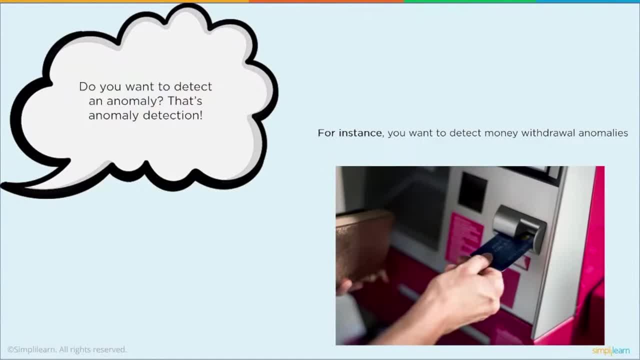 If you're predicting the stock- whether to buy stock or not- you want to be able to know if what's going on in the stock market is an anomaly. It's a different prediction model because something else is going on. You've got to pull out new information in there. 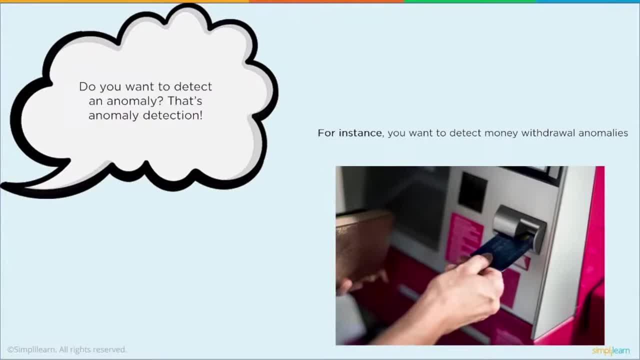 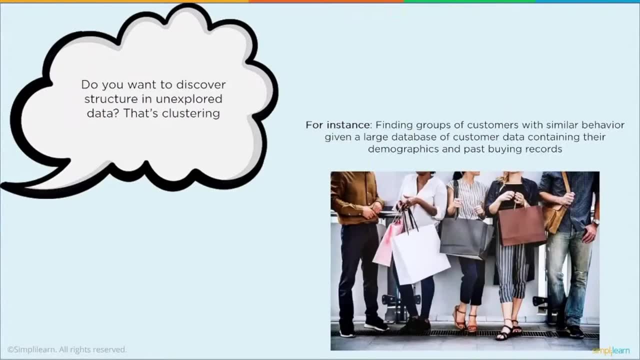 Or is this just the norm? I'm going to get my normal return on my money invested, So being able to detect anomalies is very big in data science these days. Another question that comes up, which is what we call untrained data, is: do you want to discover structure in unexplored data? 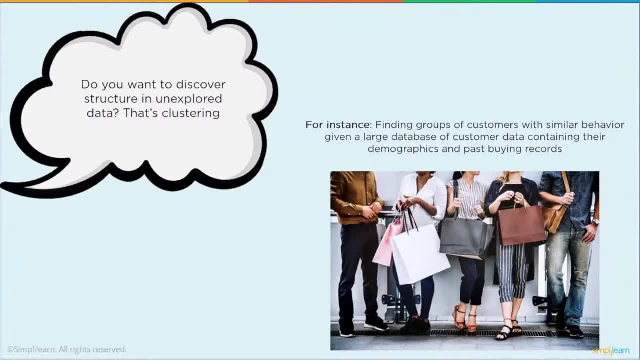 And that's called clustering, For instance, finding groups of customers with similar behavior, given a large database of customer data containing their demographics and past buying records. And in this case, we might notice that anybody who's wearing a certain set of shoes goes shopping at certain stores, or whatever it is. 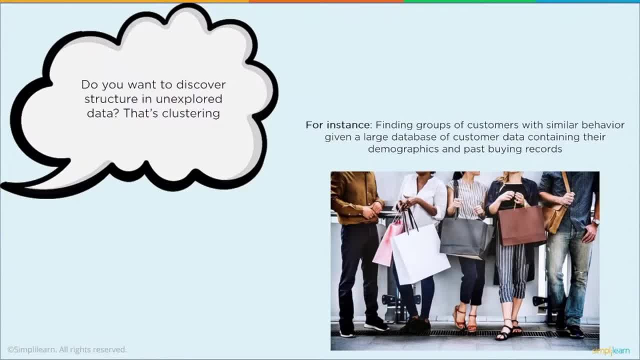 they're going to make certain purchases. By having that information, it helps us to market or group people together so that we can now explore that group and find out what it is we want to market to them. if you're in the marketing world- And that might also work in just about any arena- 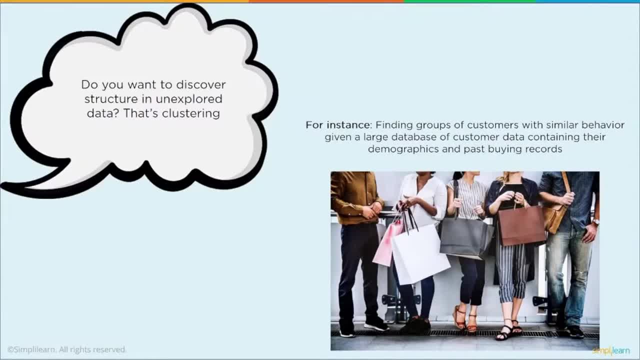 You might want to group people together, whether they're based on their different areas and investments and financial background, whether you're going to give them a loan or not, before you even start looking at whether they're a valid customer for the bank. You might want to look at all these different areas. 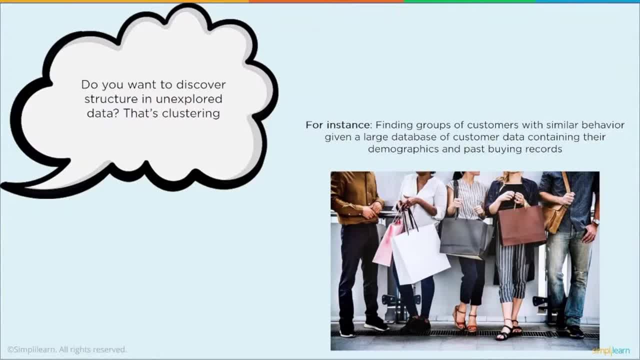 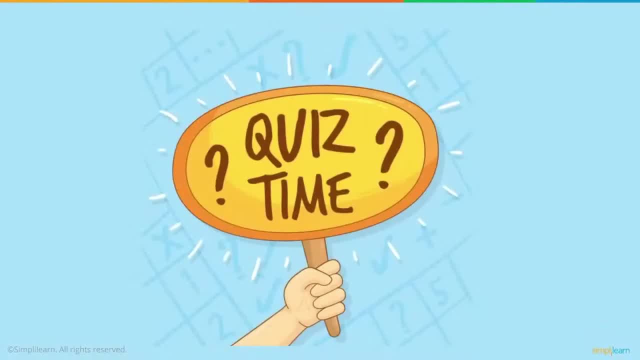 and group them together based on unknown data, So you don't know what the data is going to tell you. but you want to cluster people together, that come together. Let's take a quick detour for quiz time. Oh, my favorite. So we're going to have a couple questions here under quiz time. 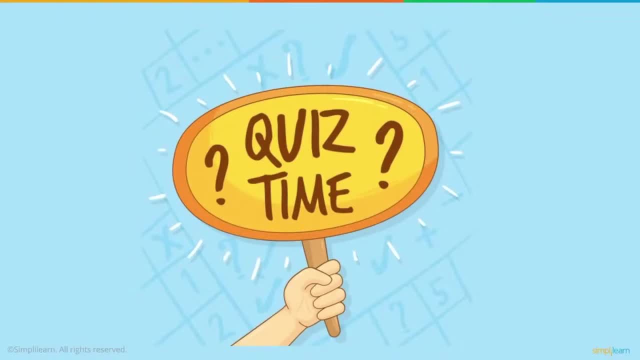 And we'll be posting the answers in the part two of this tutorial. So let's go ahead and take a look at these quiz times questions. Hopefully you'll get them all right. It'll get you thinking about how to process data and what's going on. 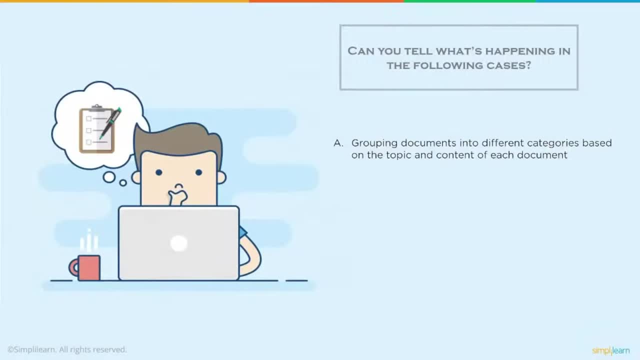 Can you tell what's happening in the following cases? Of course, you're sitting there with your cup of coffee and you have your checkbox and your pen trying to figure out what's your next step in your data science analysis. So the first one is grouping documents into different categories. 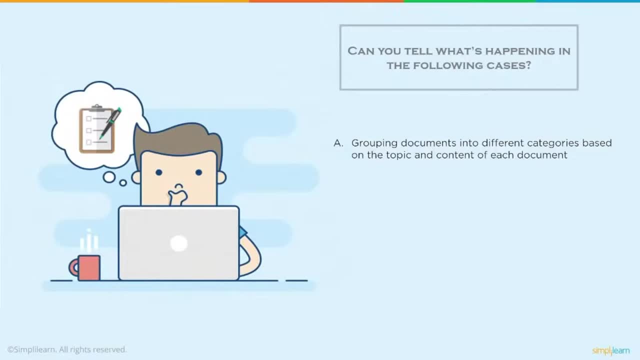 based on the topic and content of each document, Very big these days. You know you have legal documents, You have. maybe it's a sports group document, Maybe you're analyzing newspaper postings, But certainly having that automated is a huge thing in today's world. 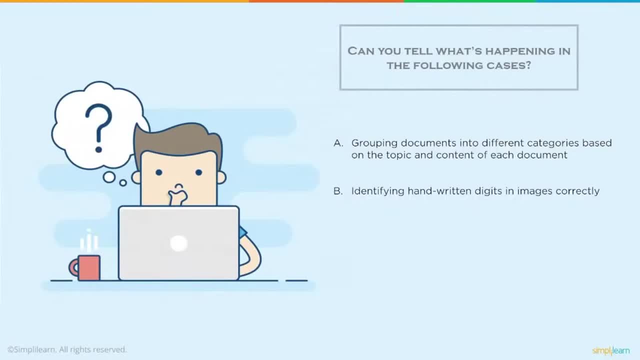 B- identifying handwritten digits in images correctly. So we want to know whether they're writing in A or capital. A, B, C. What are they writing out in their handwriting? C- behavior of a website indicating that the site is not working as designed. 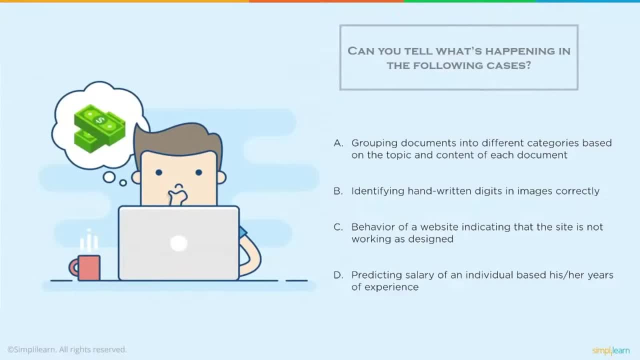 D- predicting salaries: The salary of an individual based on his or her years of experience. HR hiring set up there. So stay tuned for part two. We'll go ahead and answer these questions when we get to the part two of this tutorial. 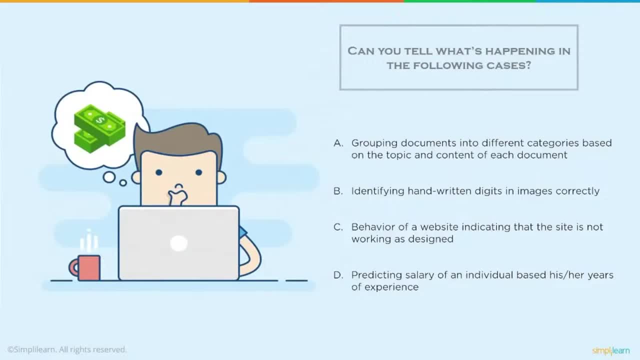 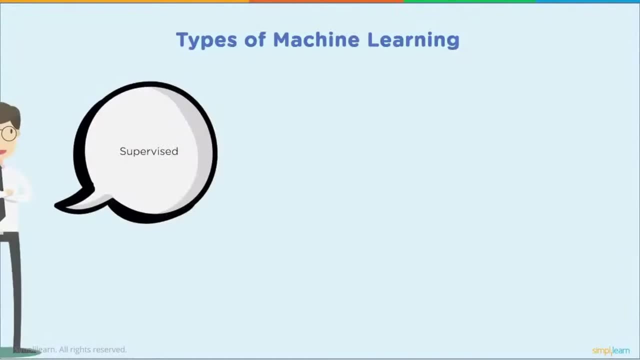 Or you can just simply write at the bottom and send a note to Simply Learn, and they'll follow up with you on it. Back to our regular content, And these last few bring us into the next topic, which is another way of dividing our types of machine learning. 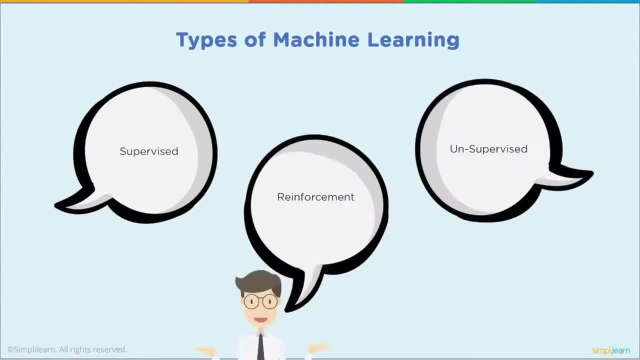 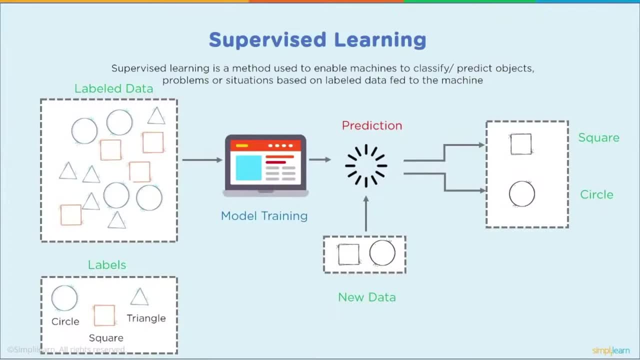 And that is with supervised, unsupervised And reinforcement learning. Supervised learning is a method used to enable machines to classify, predict objects, problems or situations based on labeled data fed to the machine. And in here you see, we have a jumble of data with circles, triangles and squares. 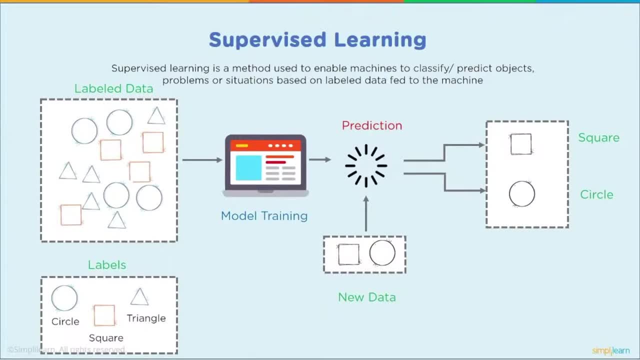 Then we label them. We have what's a circle, what's a triangle, what's a square, And we have our model training And it trains it, so we know the answer. Very important when you're doing supervised learning. you really know the answer to a lot of your information coming in. 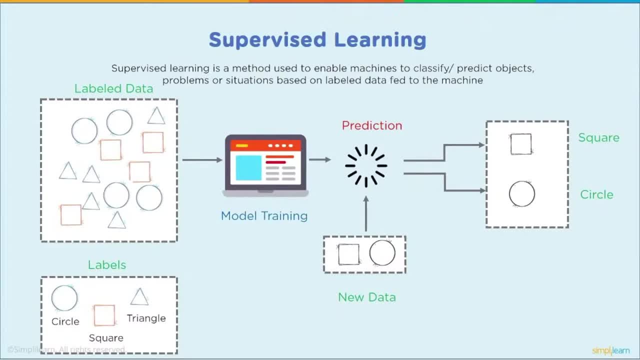 So you have a huge group of data coming in And then you have new data coming in. So we've trained our model. The model now knows the difference between a circle, a square, a triangle, And now that we've trained it, we can send in- in this case, a square and a circle goes in. 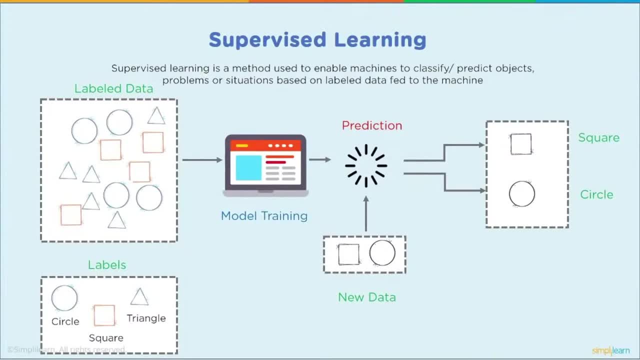 And it predicts that the top one's a square and the next one's a circle, And you can see that this is being able to predict whether someone's going to default on a loan, because I was talking about banks earlier, Supervised learning on stock market, whether you're going to make money or not. 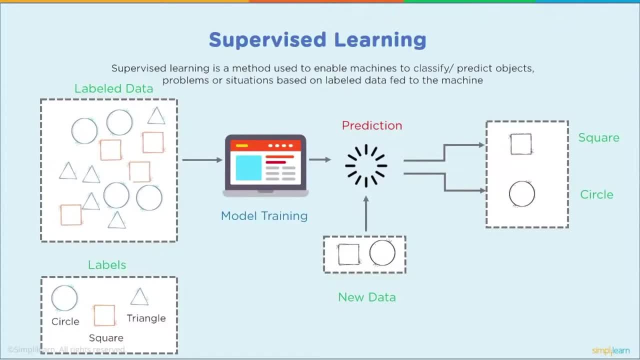 that's always important And if you are looking to make a fortune on the stock market, keep in mind. it is very difficult to get all the data correct on the stock market. It is very it fluctuates in ways really hard to predict. 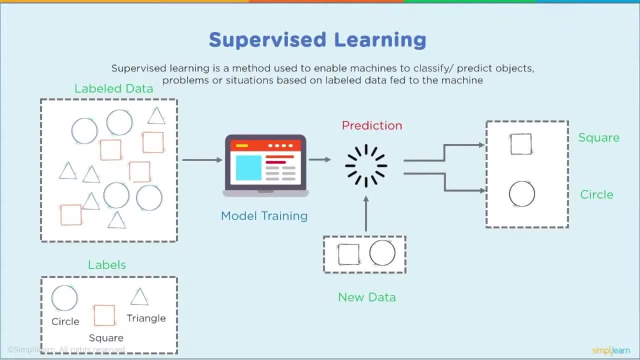 So it's quite a roller coaster ride. if you're running machine learning on the stock market, You start realizing you really have to dig for new data. So we have supervised learning. And if you have supervised, we need unsupervised learning. In unsupervised learning, machine learning model finds the hidden pattern in an unlabeled data. 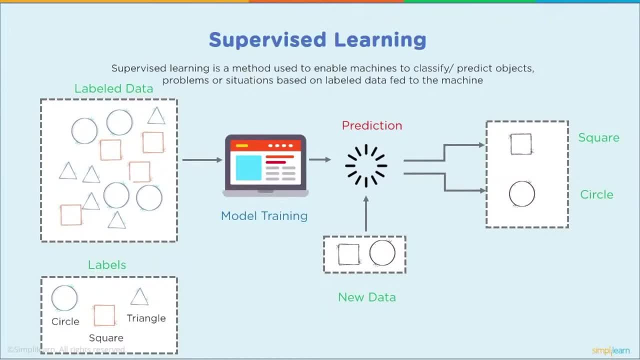 So in this case, instead of telling it what the circle is and what a triangle is and what a square is, it goes in there and looks at them and says, for whatever reason it groups them together. Maybe it'll group it by the number of corners. 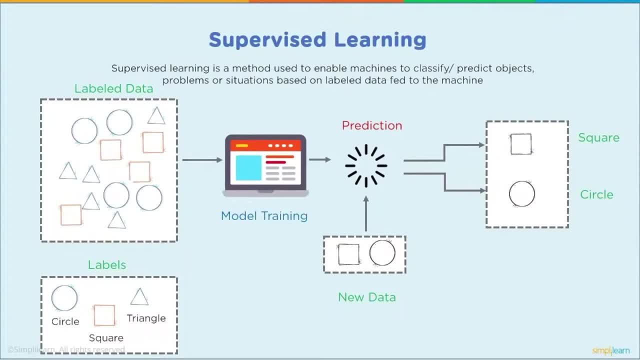 And it notices that a number of them all have three corners, a number of them all have four corners and a number of them all have no corners, And it's able to filter those through and group them together. We talked about that earlier, with looking at a group of people. 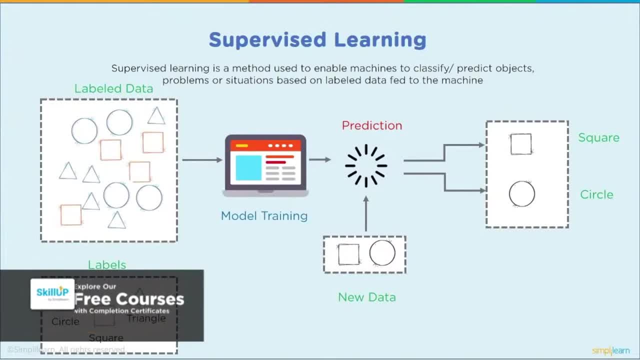 We want to group them together to find out what they have in common. And, of course, once you understand what people have in common, maybe you have one of them who's a customer at your store, or you have five of them who are a customer at your store. 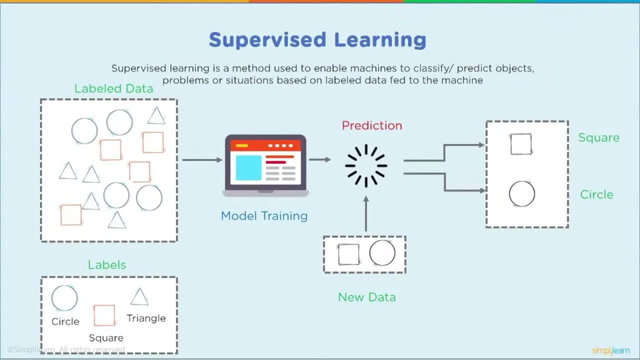 and they have a lot in common with five others who are not customers at your store. How do you market to those five who aren't customers at your store yet They fit the demographics of who's going to shop there and you would like them to shop at your store and not the one next door. 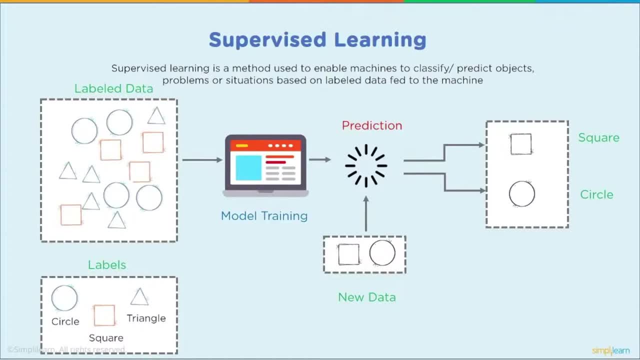 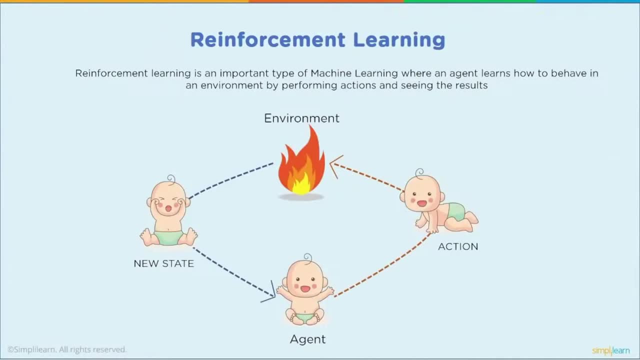 Of course, this is a simplified version. You can see very easily the difference between a triangle and a circle and it's very easy in marketing Reinforcement learning. Reinforcement learning is an important type of machine learning where an agent learns how to behave in an environment by performing actions and seeing the result. 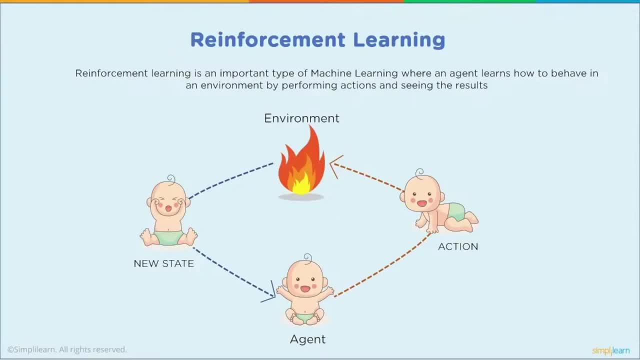 We have here in this case, a baby. It's actually great that they used an infant for this slide because the reinforcement learning is very much in its infant stages, But it's also probably the biggest machine learning demand out there right now or in the future. 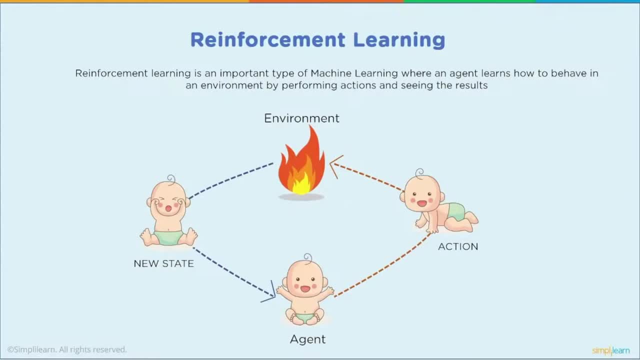 It's going to be coming up over the next few years because reinforcement, learning and how to make that work for us, And you can see here where we have our action In the action. in this one it goes into the fire. Hopefully the baby didn't. it was just a little candle, not a giant fire pit like it looks like here. 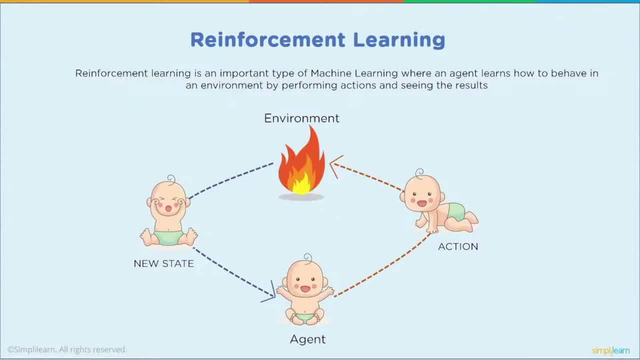 When the baby comes out and the new state is, the baby is sad and crying because they got burned on the fire And then maybe they take another action. The baby's called the agent because it's the one taking the actions And in this case they didn't go into the fire. 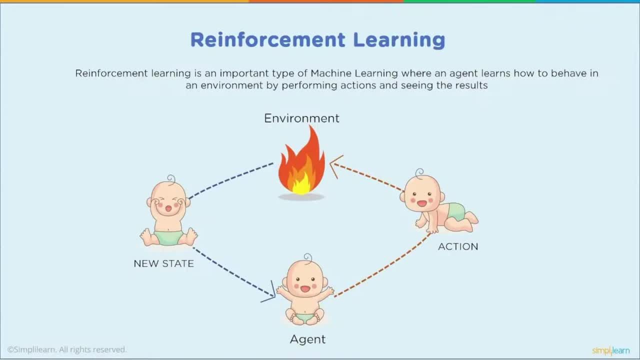 They went a different direction and now the baby's happy and laughing and playing. Reinforcement learning is very easy to understand because that's how, as humans, that's one of the ways we learn. We learn whether it is you know you burn yourself on the stove. don't do that anymore. 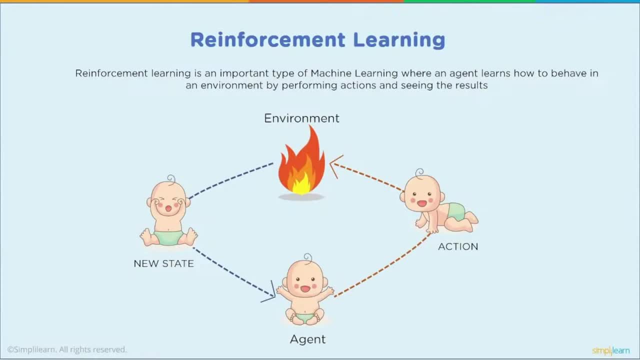 Don't touch the stove. In the big picture, being able to have a machine learning program or an AI be able to do this is huge, Because now we're starting to learn how to learn. That's a big jump in the world of computer and machine learning. 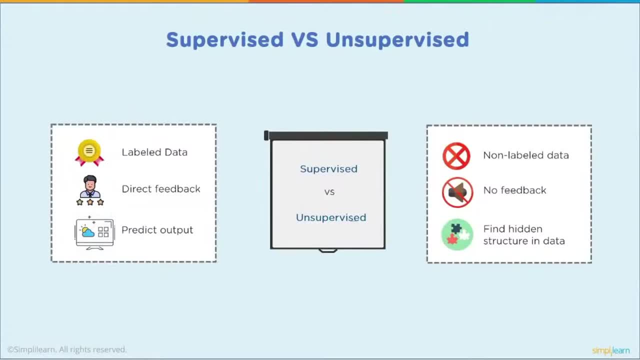 And we're going to go back and just kind of go back over supervised versus unsupervised learning. Understanding this is huge, because this is going to come up in any project you're working on. We have in supervised learning, we have labeled data. 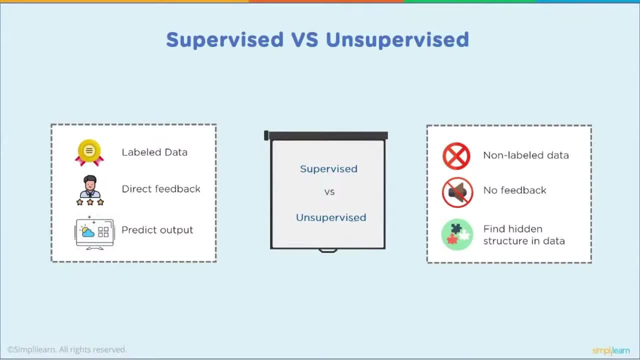 We have direct feedback. So someone's already gone in there and said, yes, that's a triangle, No, that's not a triangle. And then you predict an outcome. So you have a nice prediction: This new set of data is coming in and we know what it's going to be. 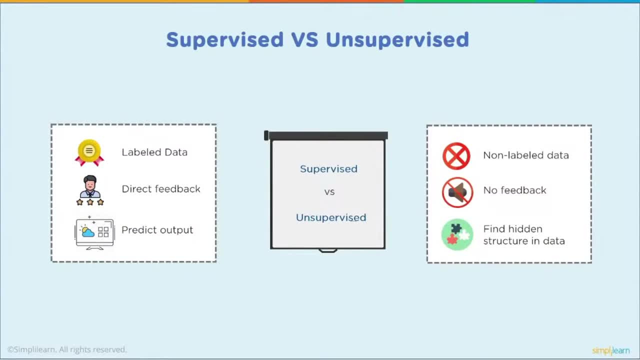 And then, with unsupervised training, it's not labeled, So we really don't know what it is. There's no feedback, So we're not telling it whether it's right or wrong. We're not telling it whether it's a triangle or a square. 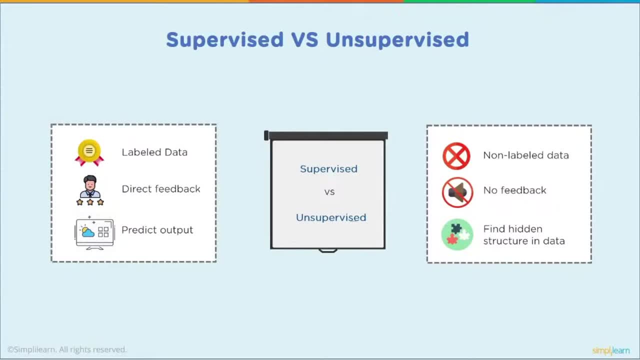 We're not telling it to go left or right. All we do is we're finding hidden structure in the data, grouping the data together to find out what connects to each other, And then you can use these together. So imagine you have an image and you're not sure what you're looking for. 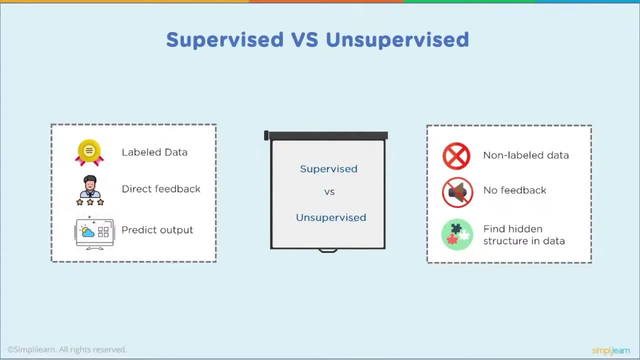 So you go in and you have the unstructured data, Find all these things that are connected together, And then somebody looks at those and labels them. And then you label data and program something to predict what's in the picture So you can see how they go back and forth and you can start connecting all these different tools together to make a bigger picture. 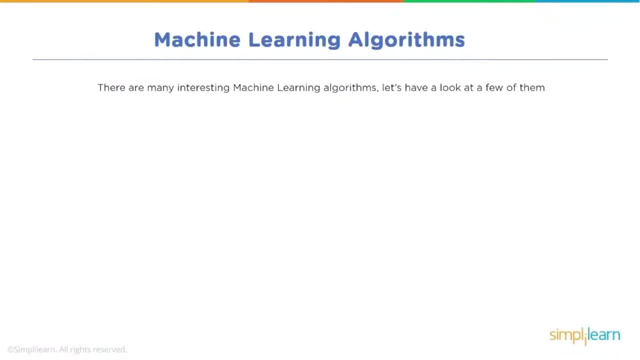 There are many interesting machine learning algorithms. Let's have a look at a few of them. Hopefully, this will give you a little flavor of what's out there, And these are some of the most important ones that are currently being used. We'll take a look at linear regression decision tree and the support vector machine. 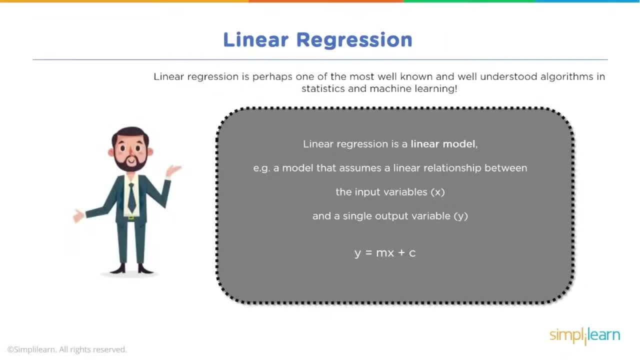 Let's start with a closer look at linear regression. Linear regression is perhaps one of the most well-known and well-understood algorithms in statistics and machine learning. Linear regression is a linear model, For example, a model that assumes a linear relationship between the input variables x and the single output variable y. 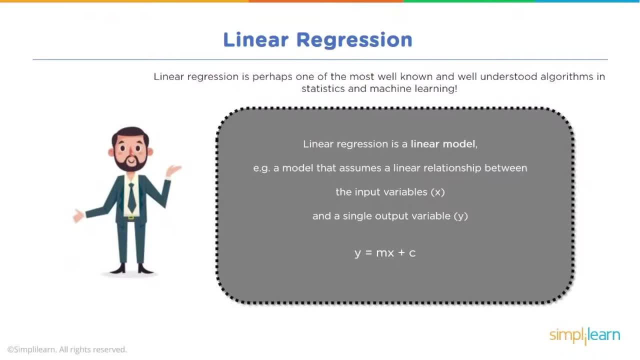 And you'll see this if you remember from your algebra classes: y equals mx plus c. Imagine we are predicting distance traveled y from speed x. Our linear regression model representation for this problem would be: y equals m times x plus c, or distance equals m times speed plus c. 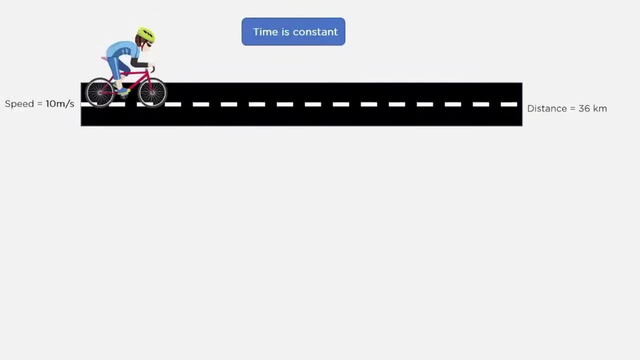 where m is the coefficient and c is the y-intercept, And we're going to look at two different variations of this. First, we're going to start with time as constant And you can see we have a bicyclist. He's got a safety gear on, thank goodness. 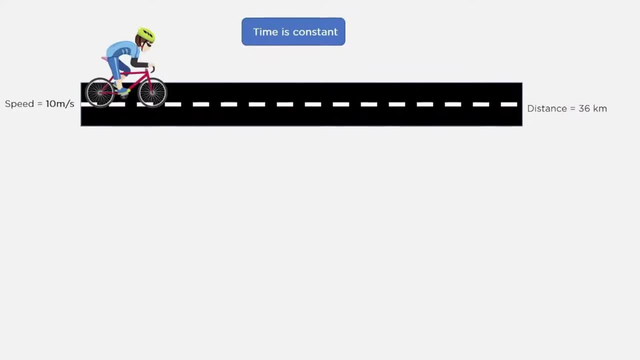 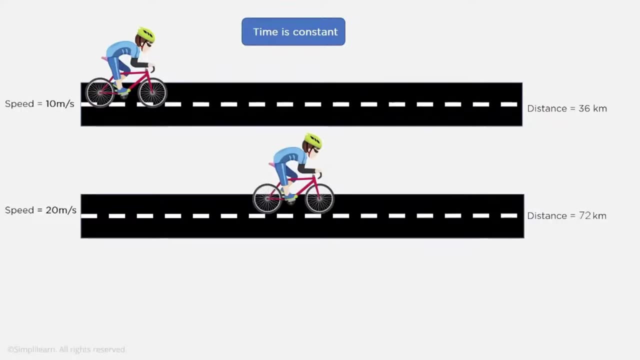 Speed equals 10 meters per second, And so over a certain amount of time, his distance equals 36 kilometers. We have a second bicyclist who's going twice the speed, or 20 meters per second. And you can guess: if he's going twice the speed and time is a constant, then he's going to go twice the distance. 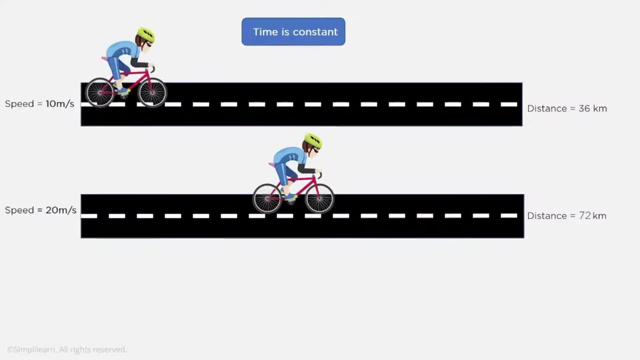 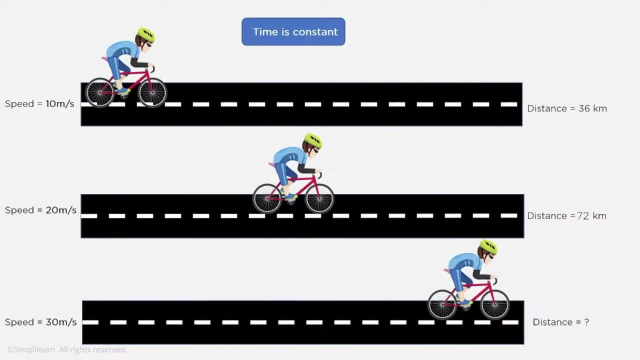 And that's easily to compute. 36 times 2, you get 72 kilometers. And so if you had the question of how fast would somebody who's going three times that speed, or 30 meters per second, is? you can easily compute the distance in our head. We can do that without needing a computer. 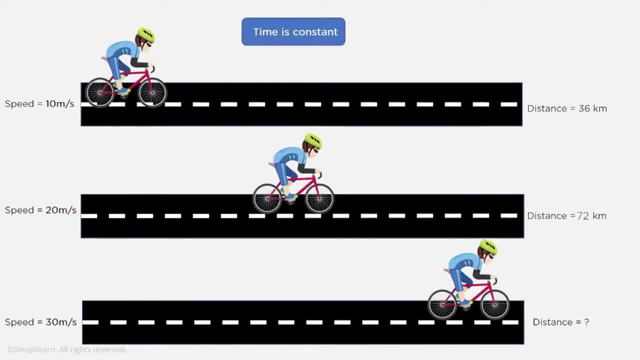 But we want to do this for more complicated data. So it's kind of nice to compare the two, but let's just take a look at that and what that looks like in a graph. So in a linear regression model, we have our distance to the speed. 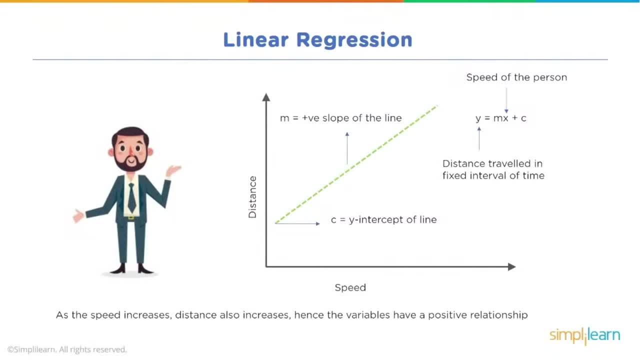 and we have our m equals the ve slope of the line, And we'll notice that the line has a plus slope. And as the speed increases, distance also increases. hence the variables have a positive relationship. And so your speed of the person, which equals y, equals mx plus c, distance traveled in a fixed interval of time. 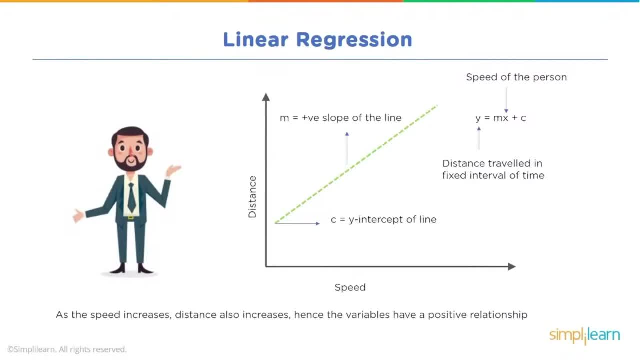 and we could very easily compute either following the line or just knowing it's 3 times 10 meters per second, that this is roughly 102 kilometers distance that this third bicyclist has traveled. One of the key definitions on here is positive relationship. 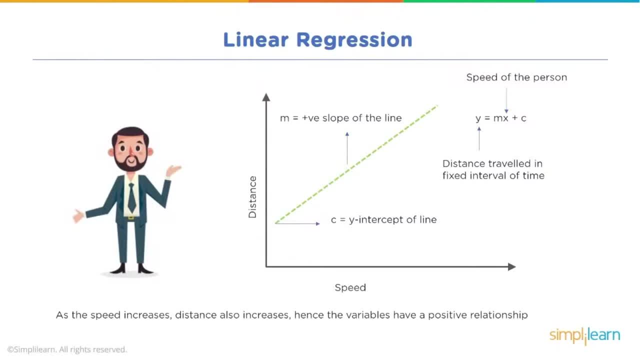 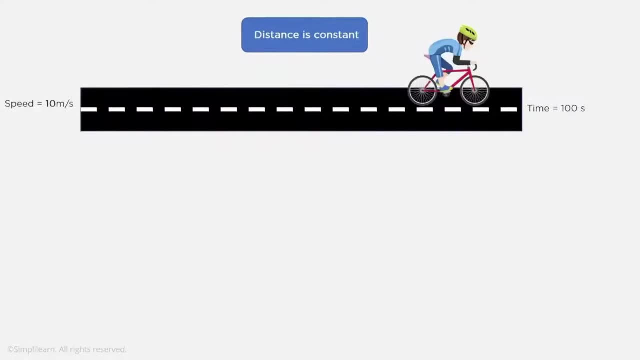 So the slope of the line is positive. As distance increases, so does speed increase. Let's take a look at our second example, where we put distance as a constant, So we have speed equals 10 meters per second. They have a certain distance to go and it takes them 100 seconds to travel that distance. 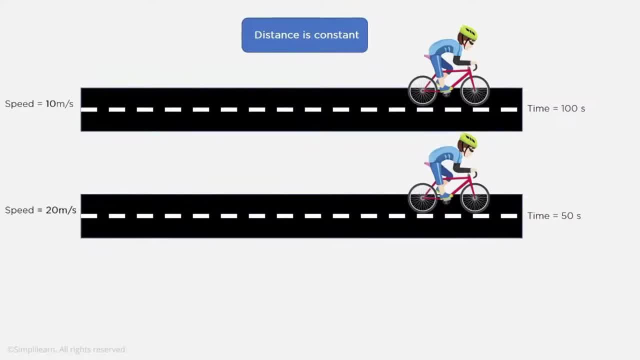 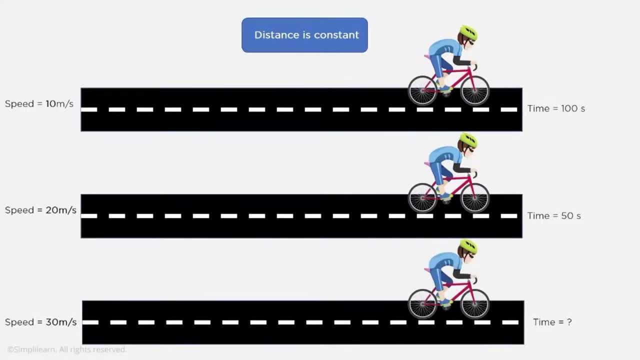 And we have our second bicyclist, who's still doing 20 meters per second. Since he's going twice the speed, we can guess that he'll cover the distance in about half the time: 50 seconds. And of course you could probably guess on the third one, 100 divided by 30, since he's going 3 times the speed. 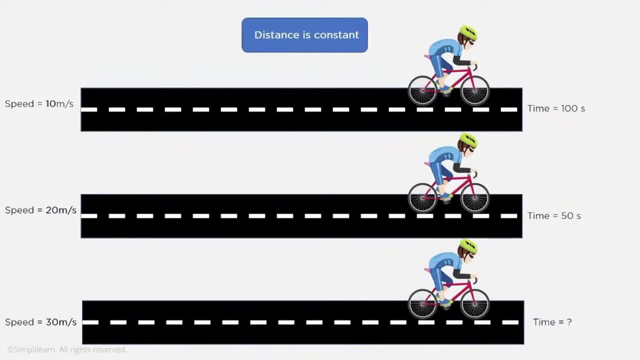 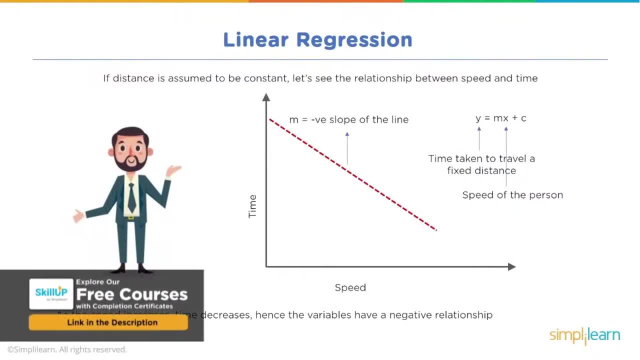 you could easily guess that this is 33.333 seconds time. We put that into a linear regression model or a graph. If the distance is assumed to be constant, let's see the relationship between speed and time And as time goes up the amount of speed to go, that same distance goes down. 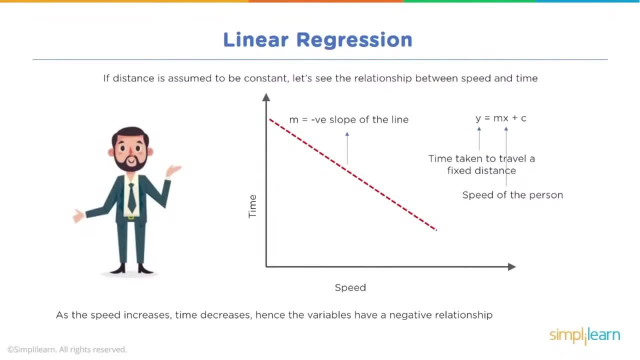 So now your m equals a minus ve slope of the line. As the speed increases, time decreases, hence the variable has a negative relationship. Again, there's our definition: positive relationship and negative relationship dependent on the slope of the line. And with a simple formula like this and even a significant amount of data, 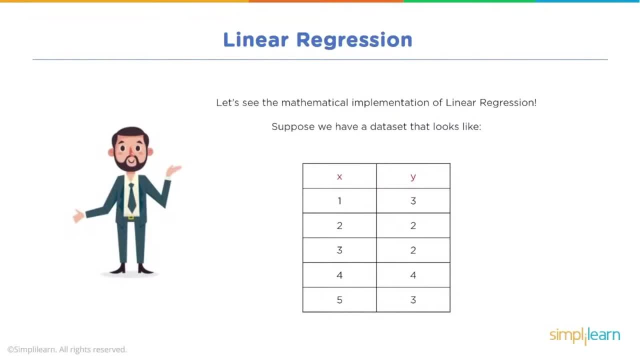 let's see with the mathematical implementation of linear regression And we'll take this data. so suppose we have this data set. we have xy. x equals 1,, 2,, 3,, 4, 5, standard series and the y value is 3,, 2,, 2,, 4, 3.. 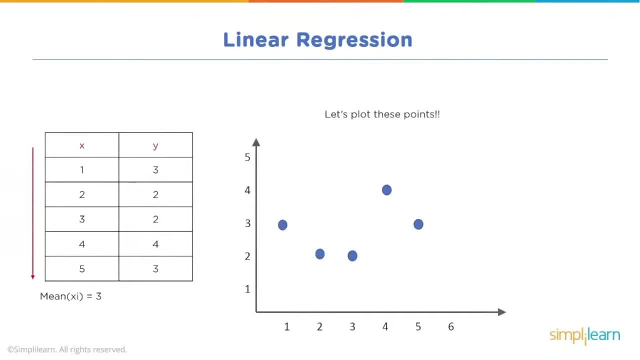 When we take that and we go ahead and plot these points on a graph, you can see there's kind of a nice scattering and you could probably eyeball a line through the middle of it. But we're going to calculate that exact line for linear regression. 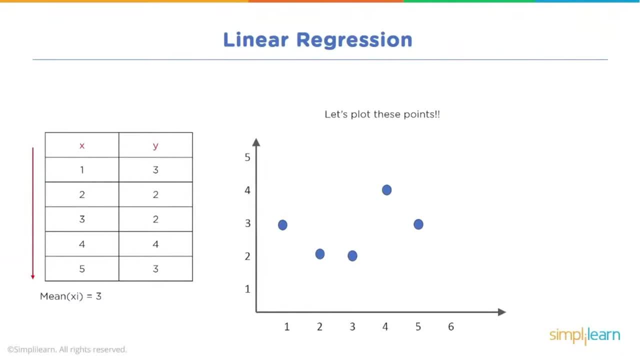 And the first thing we do is we come up here and we have the mean of xi And remember, mean is basically the average. So we added 5 plus 4 plus 3 plus 2.. 2 plus 1 and divide by 5.. 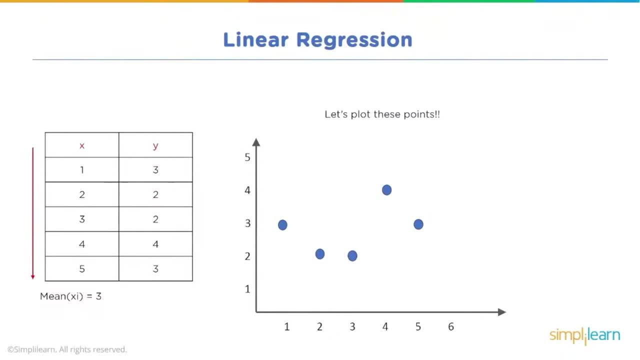 And that simply comes out as 3.. And then we'll do the same for y. We'll go ahead and add up all those numbers and divide by 5. And we end up with the mean value of y of i equals 2.8.. 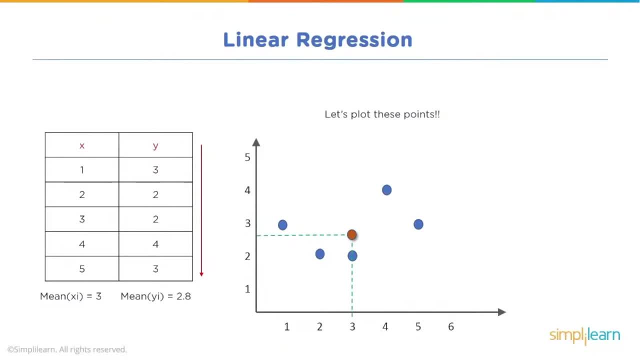 Where the xi references as an average or means value and the yi also equals a means value of y, And when we plot that you'll see that we can put in the y equals 2.8 and the x equals 3 in there on our graph. 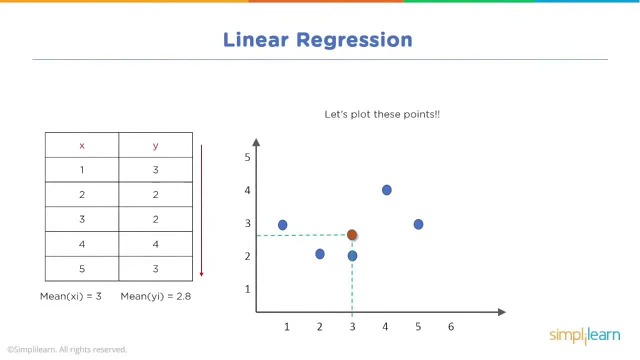 We kind of gave it a little different color so you could sort it out with a dashed line. And it's important to note that when we do the linear regression the linear regression model should go through that dot. Now let's find our regression equation to find the best fit line. 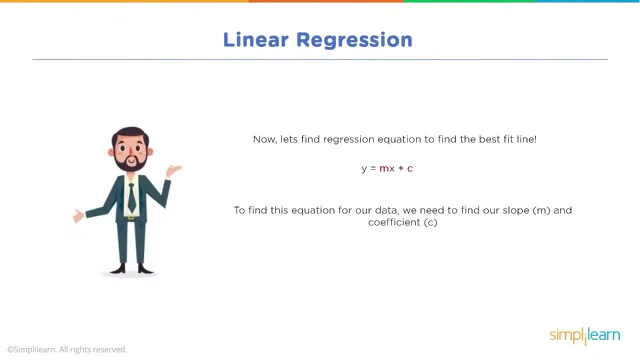 Remember, we go ahead and take our y equals mx plus c, So we're looking for m and c. So to find this equation for our data, we need to find our slope of m and our coefficient of c And we have y equals mx plus c. 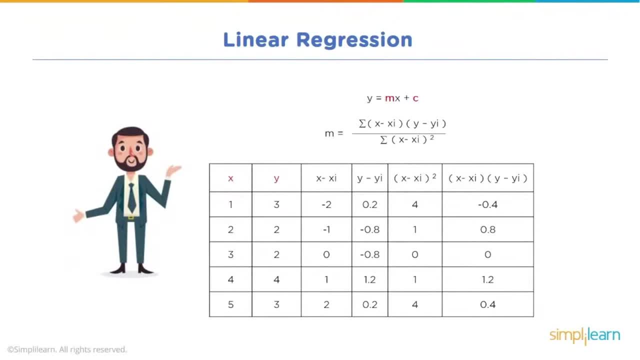 Where m equals the sum of x minus x average times 1.. So we have y minus y average, or y means and x means over. the sum of x minus x means squared. That's how we get the slope of the value of the line. 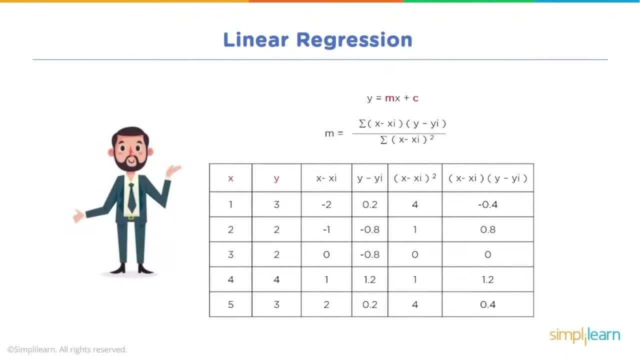 And we can easily do that by creating some columns. here We have x, y. Computers are really good about iterating through data, And so we can easily compute this and fill in a graph of data. And in our graph you can easily see that if we have our x value of 1, and if you remember the xi or the means value is 3,. 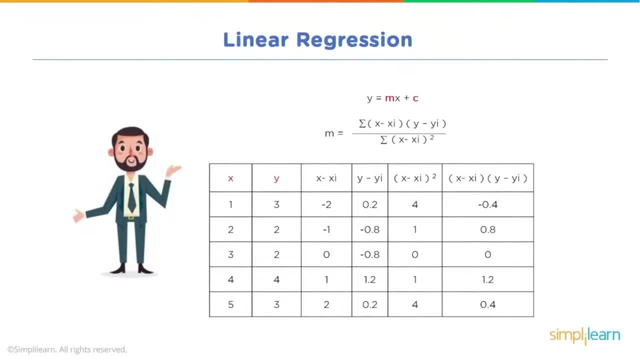 1 minus 3 equals a negative 2.. And 2 minus 3 equals a negative 1, so on and so forth, And we can easily fill in the column of x minus xi, y minus yi, And then from those we can compute x minus xi squared and x minus xi times y minus yi. 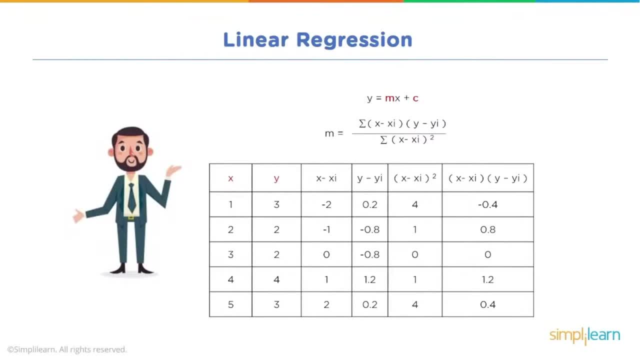 And you can guess it that the next step is to go ahead and sum the different columns for the answers we need. So we get a total of 10 for our x minus xi squared And a total of 2 for x minus xi times y minus yi. 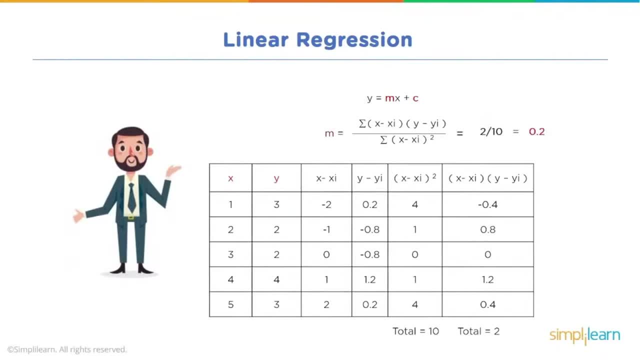 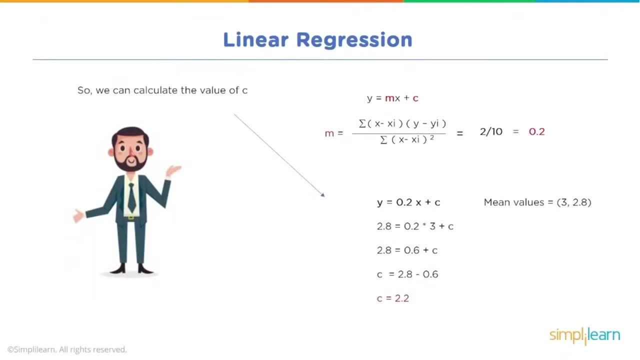 And we plug those in, we get 2 tenths, which equals 0.2.. So now we know the slope of our line equals 0.2. So we can calculate the value of c. That would be the next step, as we need to know where it crosses the y-axis. 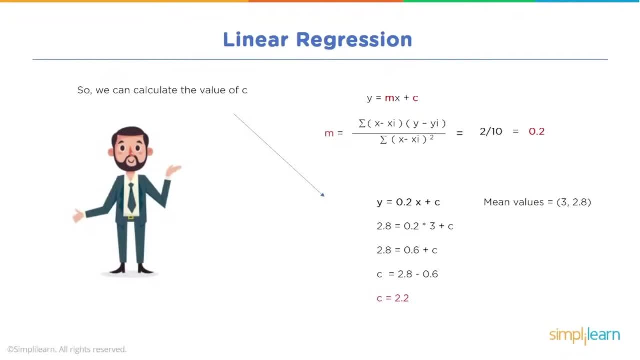 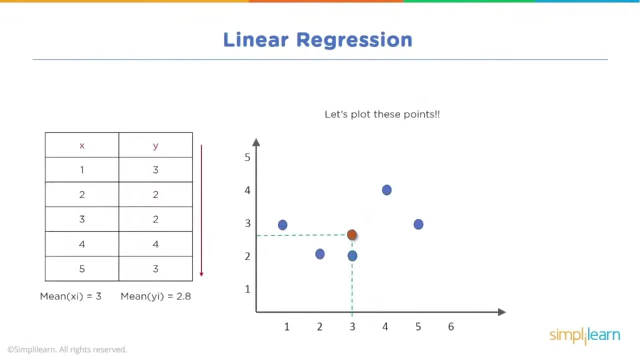 And, if you remember, I mentioned earlier that the linear regression line has to pass through the means value, The one that we showed earlier. We can just flip back up there to that graph And you can see right here there's our means value, which is 3, x equals 3, and y equals 2.8.. 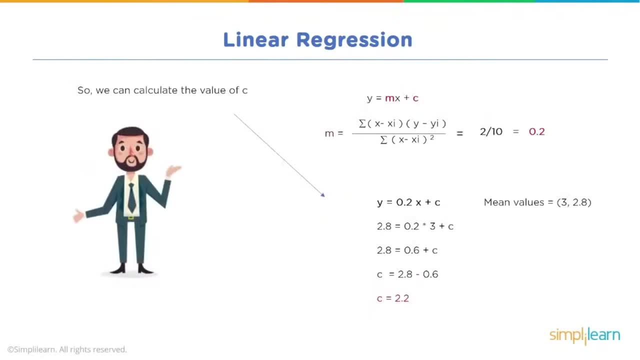 And since we know that value, we can simply plug that into our formula. y equals 0.2x plus c. So we plug that in and we get 2.8 equals 0.2 times 3 plus c, And you can just solve for c. 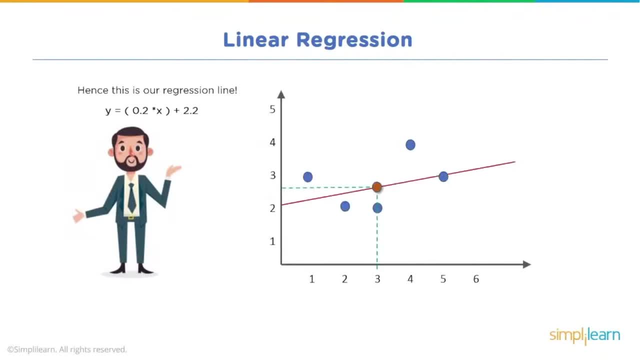 So now we know that our coefficient equals 2.2.. And once we have all that, we can go ahead and plot our regression line: y equals 0.2 times x plus 2.2.. And then from this equation we can compute new values. 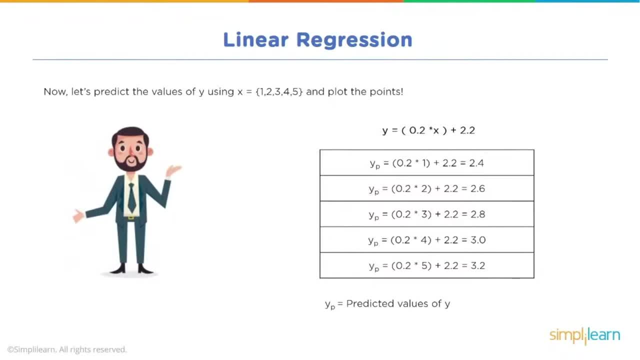 So let's predict the values of y using x equals 1,, 2,, 3,, 4, 5- and plot the points. Remember the 1,, 2,, 3,, 4, 5 was our original x values. 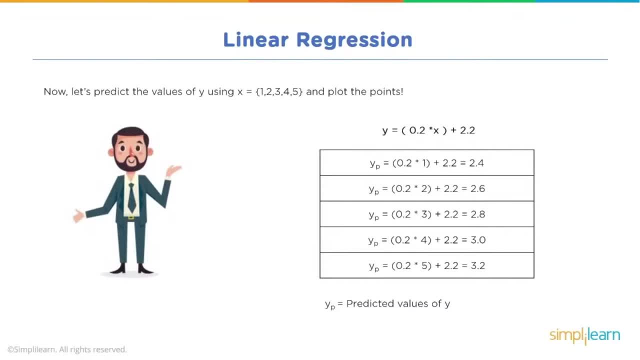 So now we're going to see what y thinks- they are, not what they actually are- And we plug those in. we get y designated with y of p. You can see that x equals 1 equals 2.4,. x equals 2 equals 2.6.. 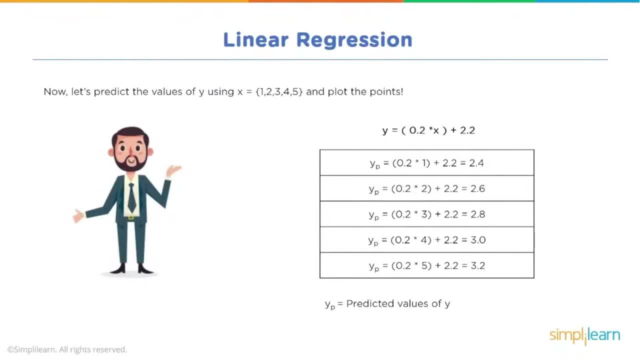 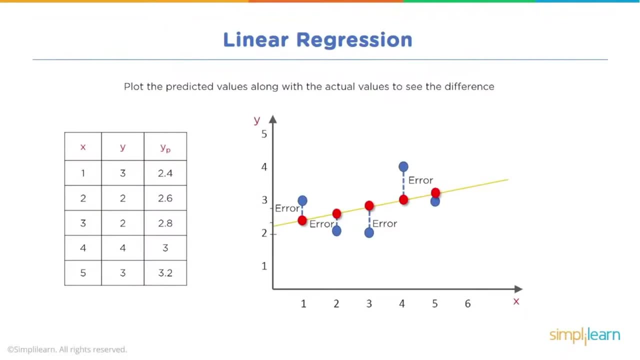 And so on and so on. So we have our y predicted values of what we think it's going to be. when we plug those numbers in And when we plot the predicted values along with the actual values, we can see the difference. And this is one of the things that's very important with linear regression in any of these models is to understand the error. 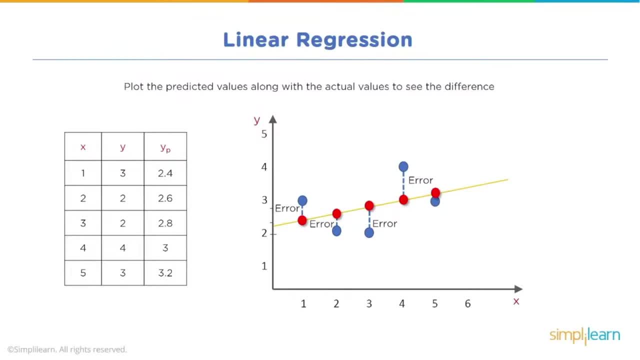 And so we can calculate the error on all of our different values. And you can see over here we plotted x and y and y predict And we draw in a little line so you can sort of see what the error looks like there between the different points. 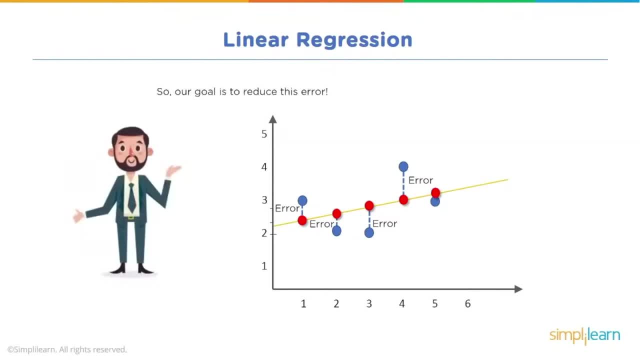 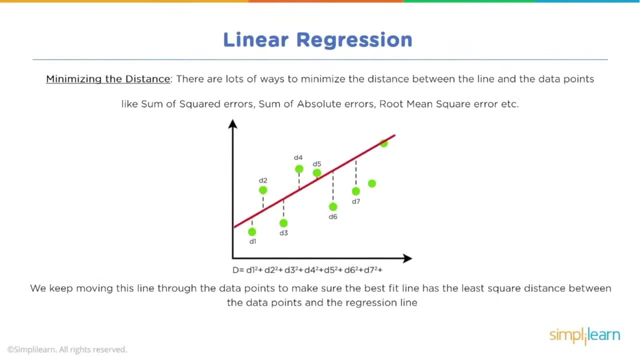 So our goal is to reduce this error. We want to minimize that error value on our linear regression model. Minimizing the distance: There are lots of ways to minimize the distance between the line and the data points, Like sum of squared errors, sum of absolute errors, root mean, square error, etc. 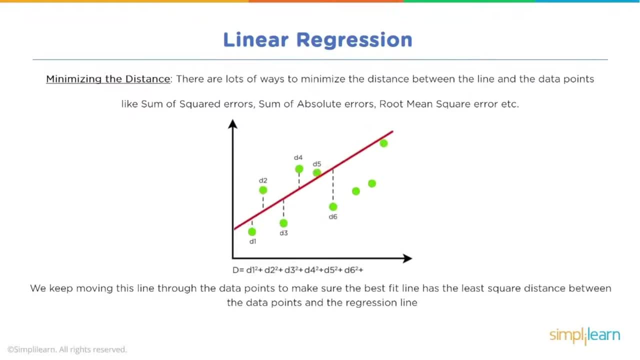 We keep moving this line through the data points to make sure the best fit line has the least squared distance between the data points and the regression line. So to recap with a very simple linear regression model. We first figure out the formula of our line through the middle. 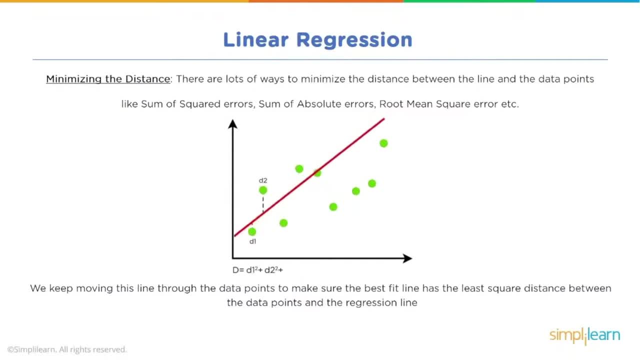 And then we slowly adjust the line to minimize the error. Keep in mind, this is a very simple formula. The math gets. even though the math is very much the same, it gets much more complex as we add in different dimensions. So this is only two dimensions. y equals mx plus c. 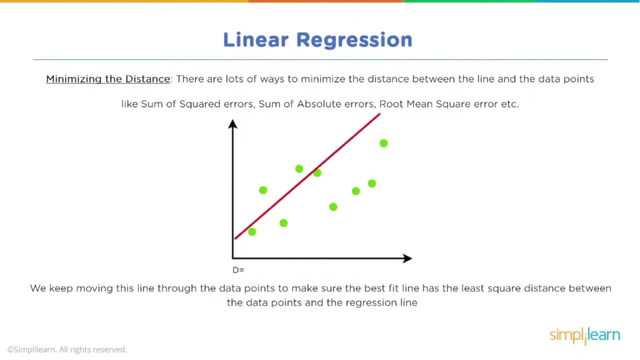 But you can take that out to x, z, ijq, all the different features in there- And they can plot a linear regression model on all of those, using the different formulas to minimize the error. Let's go ahead and take a look at decision trees- a very different way to solve problems than the linear regression model. 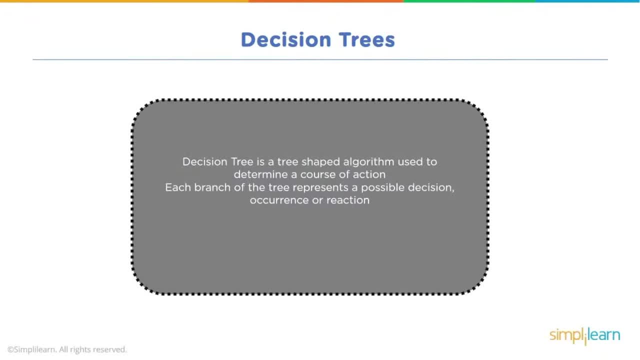 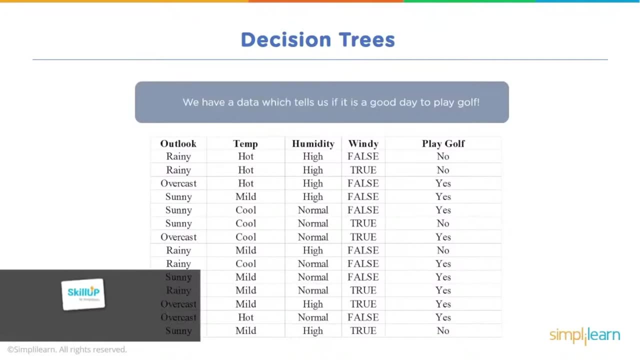 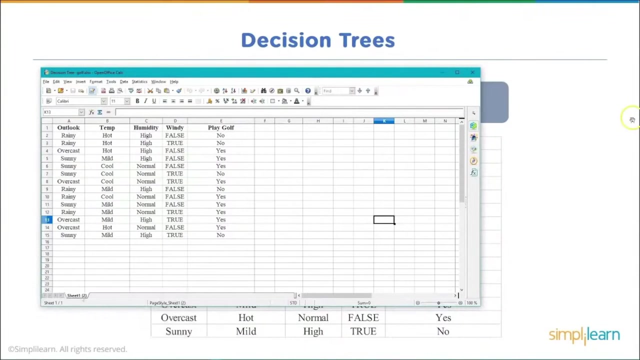 Decision tree is a tree shaped algorithm used to determine a course of action. Each branch of a tree represents a possible decision occurrence or reaction. We have data which tells us if it is a good day to play golf, And if we were to open this data up in a general spreadsheet, you can see we have the outlook. 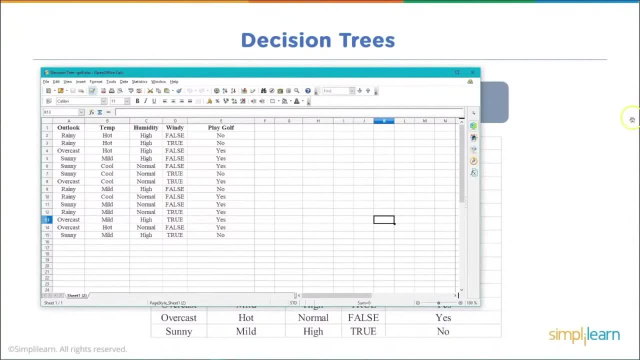 Whether it's rainy, overcast, sunny temperature, hot, mild, cool, Humidity, windy, and did I like to play golf that day, yes or no? So we're taking a census And certainly I wouldn't want a computer telling me when I should go play golf or not. 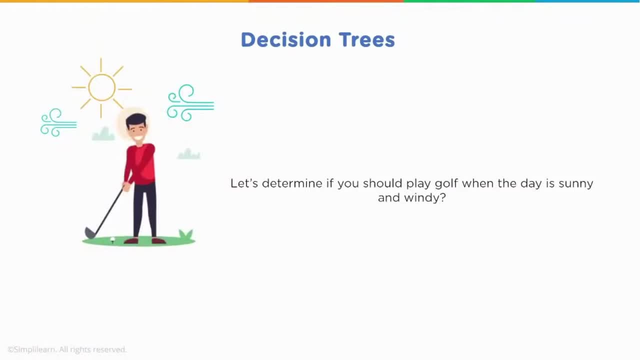 But you can imagine if you got up the night before you're trying to plan your day And it comes up and says: tomorrow would be a good day for golf for you in the morning And not a good day in the afternoon, or something like that. 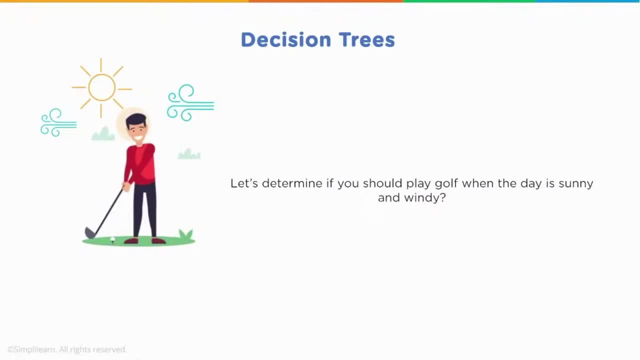 This becomes very beneficial- And we see this in a lot of applications coming out now- where it gives you suggestions And lets you know what would fit the match for you for the next day Or the next purchase, Or the next, whatever Next mail out. 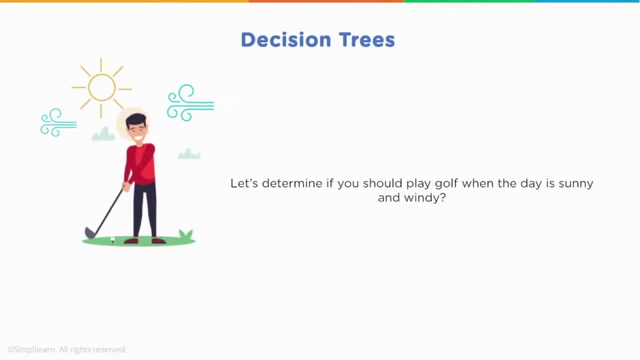 In this case, is tomorrow a good day for playing golf, based on the weather coming in, And so we come up and lets determine if you should play golf when the day is sunny and windy. So we found out: the forecast tomorrow is going to be sunny and windy. 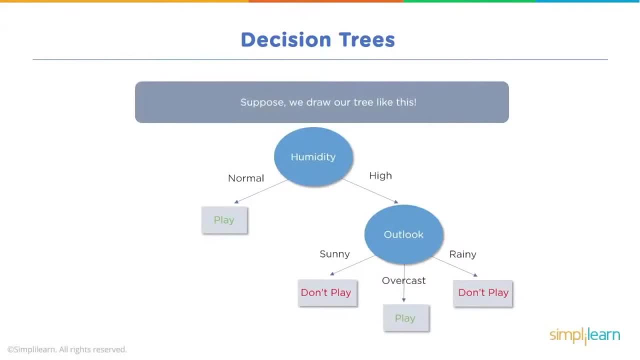 And suppose we draw our tree like this: We're going to have our humidity And then we have our normal, Which is, if you have a normal humidity, you're going to go play golf And if the humidity is really high You're going to get the outlook. 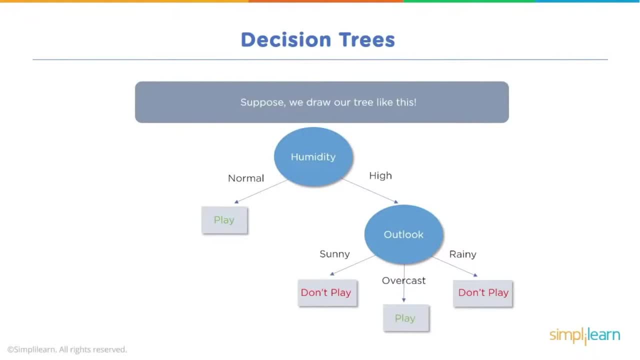 And if the outlook is sunny, overcast or rainy, It's going to change what you choose to do. So if you know that it's a very high humidity and it's sunny, You're probably not going to play golf because you're going to be out there miserable. 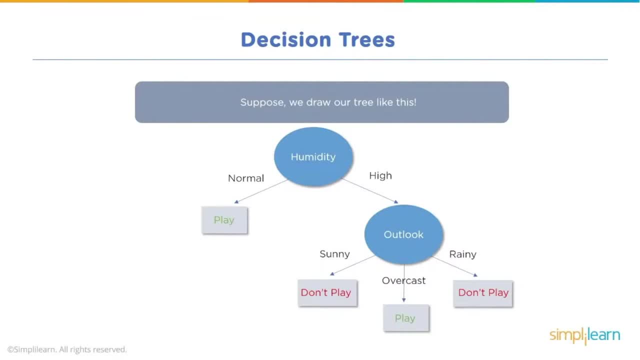 Fighting off the mosquitoes that are out joining you to play golf with you. Maybe if it's rainy- you probably don't want to play in the rain, But if it's slightly overcast and you get just the right shadow, That's a good day to play golf and be outside out on the green. 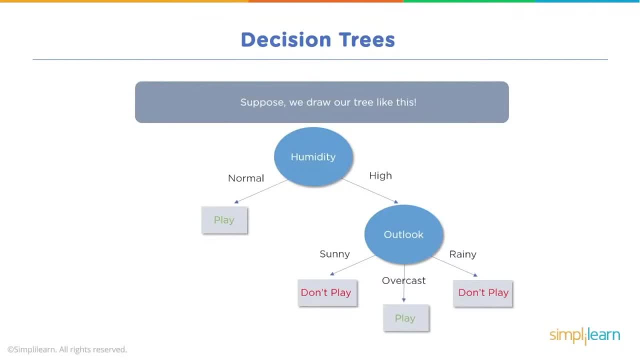 Now in this example, You can probably make your own tree pretty easily Because it's a very simple set of data going in. But the question is: how do you know what to split? Where do you split your data? What if this is much more complicated data? 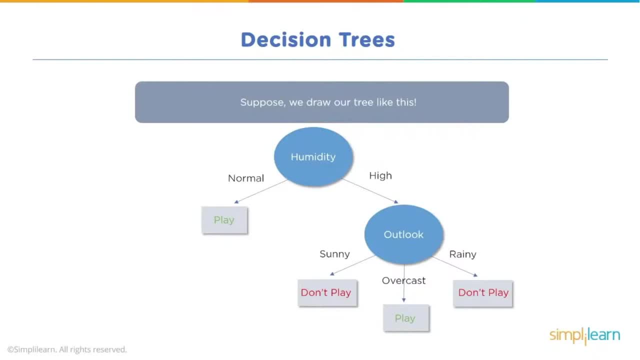 Where it's not something that you would particularly understand. Like studying cancer, They take about 36 measurements of the cancerous cells And then each one of those measurements represents how bulbous it is, How extended it is, How sharp the edges are. 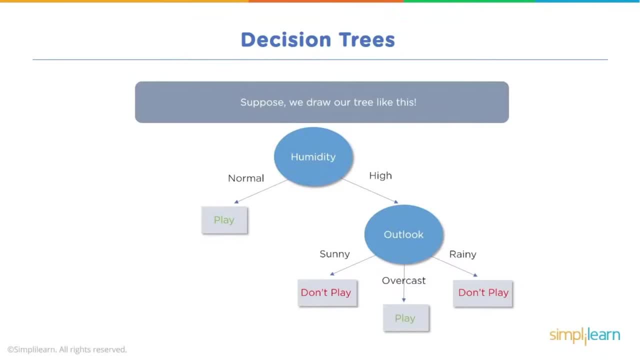 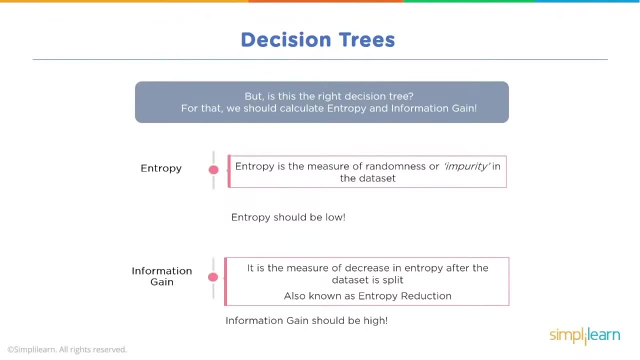 And we would have no understanding of. So how do we decide how to split that data up, And is that the right decision tree? So that's the question that's going to come up: Is this the right decision tree For that? we should calculate entropy. 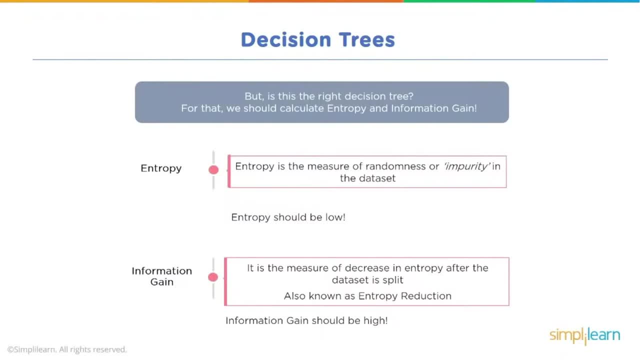 And information gain, Two important vocabulary words. there are the entropy and the information gain. Entropy: Entropy is a measure of randomness or impurity in the data set. Entropy should be low, So we want the chaos to be as low as possible. 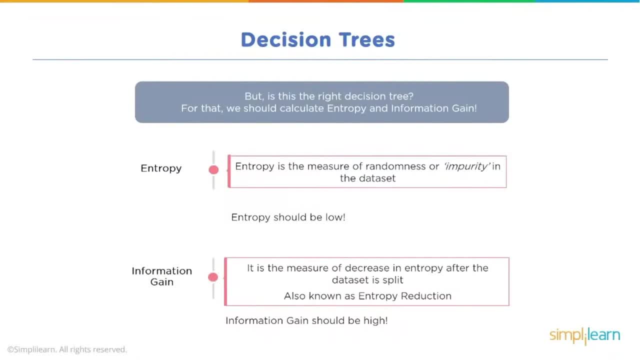 We don't want to look at it and be confused by the images or what's going on there. with mixed data And the information gain, It is a measure of decrease in entropy after the data set is split, Also known as entropy reduction. Information gain should be high. 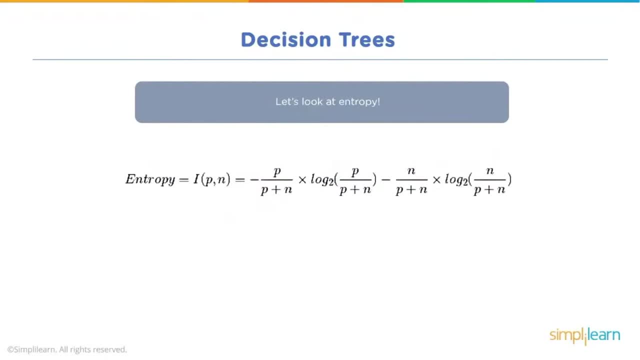 So we want our information that we get out of the split to be as high as possible. Let's take a look at entropy from the mathematical side. In this case, we're going to denote entropy as I of P of n, Where P is the probability that you're going to play a game of golf. 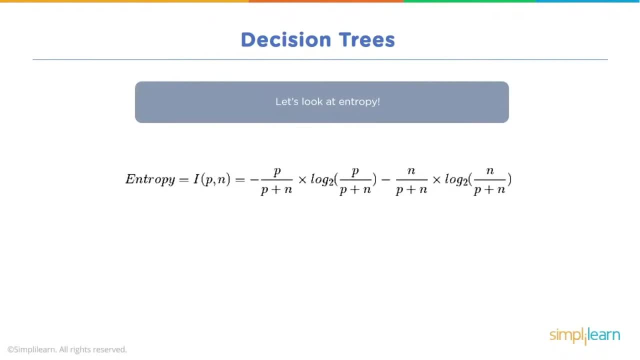 And n is the probability where you're not going to play the game of golf. Now, you don't really have to memorize these formulas- There's a few of them out there, depending on what you're working with- But it's important to note that this is where this formula is coming from. 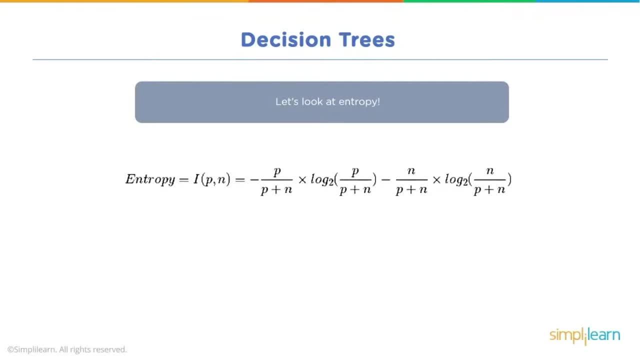 So, when you see it, you're not lost when you're running your programming, Unless you're building your own decision tree code in the back, And we simply have a log squared of P over P plus n minus n over P plus n times the log squared of n over N. 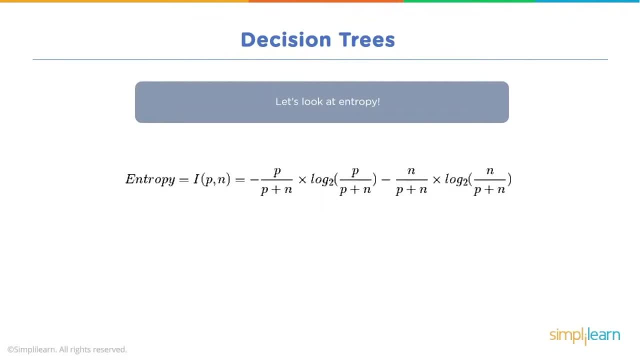 But let's break that down and see what it actually looks like when we're computing that from the computer script side. Entropy of a target class of the data set is the whole entropy. So we have entropy play golf And we look at this. if we go back to the data, 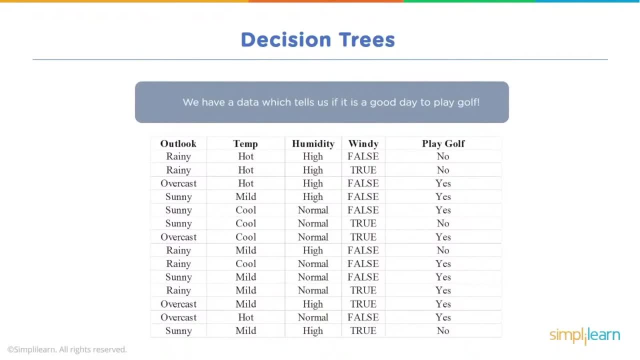 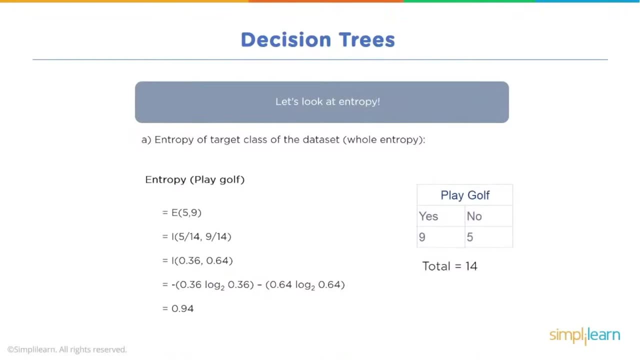 You can simply count how many yeses and no in our complete data set for playing golf days. In our complete set we find we have five days we did play golf and nine days we did not play golf, And so our i equals. if you add those together, nine plus five is fourteen. 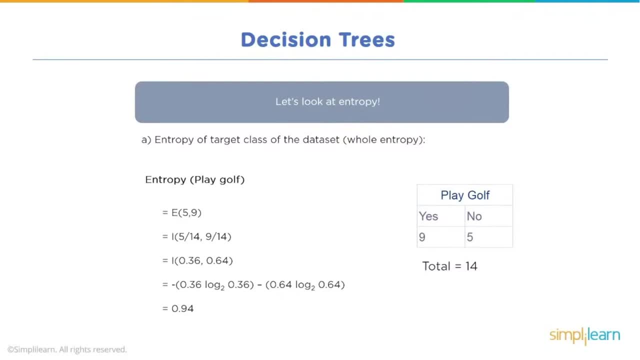 And so our i equals five over fourteen and nine over fourteen. That's our P and N values that we plug into that formula And you can go: five over fourteen equals point three, six. nine over fourteen equals point six, four, And when you do the whole equation you get the minus point three, six, log squared of point three, six. minus point six, four, log squared root of point six, four. 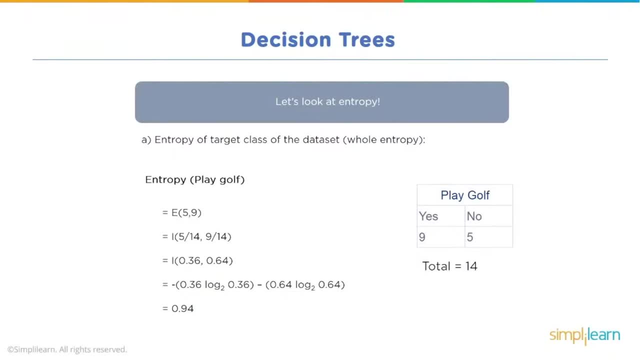 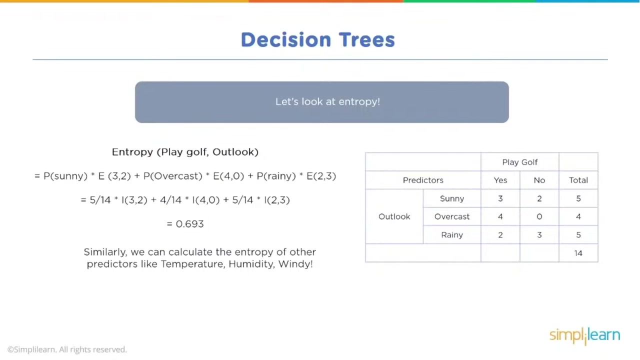 And we get a set value. we get point nine four. So we now have a full entropy value for the whole set of data that we're working with And we want to make that entropy go down. And just like we calculated the entropy out for the whole set, we can also calculate entropy for playing golf and the outlook. 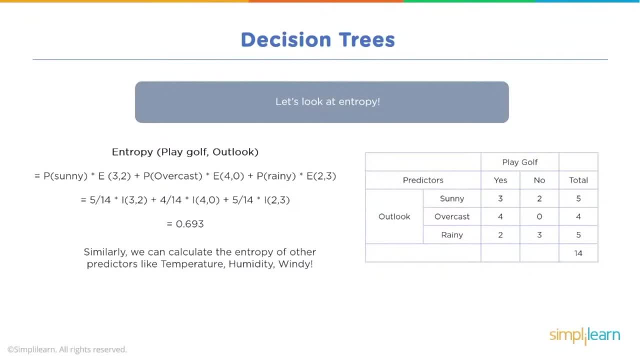 Is it going to be overcast or rainy or sunny? And so we look at the entropy. we have P of sunny times, E of three of two, And that just comes out. how many sunny days yes and how many sunny days no Over the total, which is five. 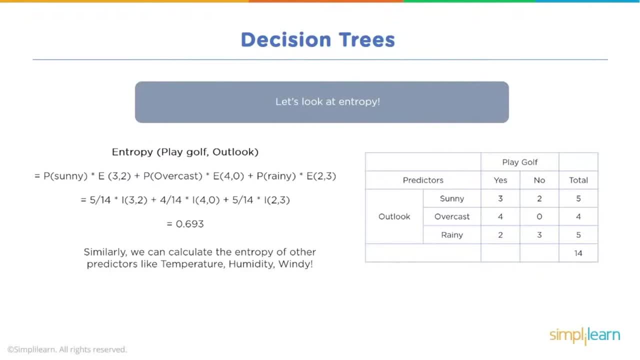 Don't forget to put the. we'll divide that five out later on. Equals P. overcast equals four comma zero. plus rainy equals two comma three, And then, when you do the whole set up, we have five over fourteen. Remember I said there was a total of five. 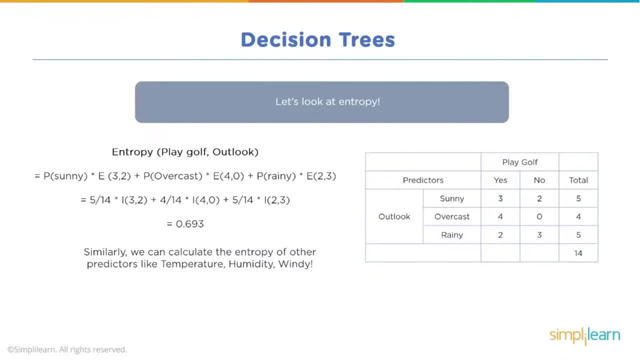 Five over fourteen times the i of three of two, plus four over fourteen times the four comma zero, And five fourteen over i of two, three, And so we can now compute the entropy of rain With just the part it has to do with the forecast. 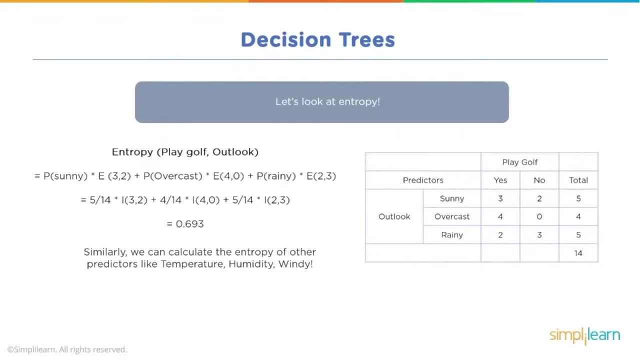 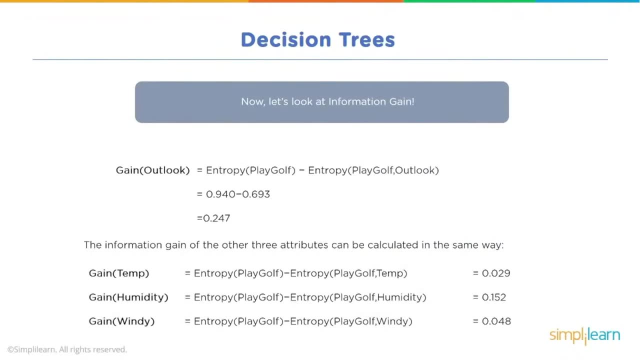 And we get point six, nine, three. Similarly, we can calculate the entropy of other predictors like temperature, humidity and wind, And so we look at the gain outlook. How much are we going to gain from this Entropy play golf minus entropy play golf outlook? 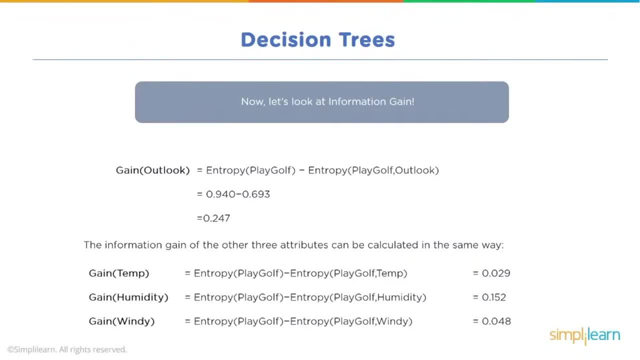 And we can take the original point nine, four for the whole set Minus the entropy of just the rainy day and temperature, And we end up with a gain of point two, four, seven. So this is our information gain. Remember, we define entropy and we define an information gain. 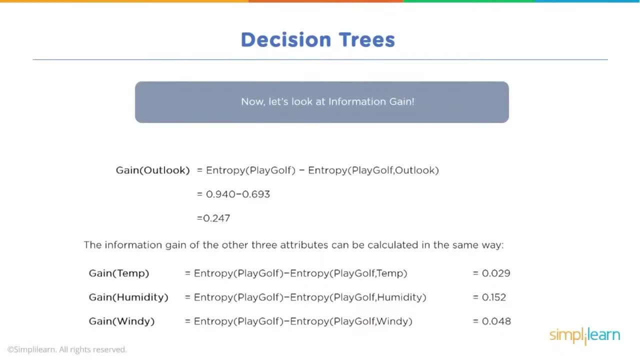 The higher the information gain, the lower the entropy, the better. The information gain of the other three attributes can be calculated in the same way. So we have our gain for temperature equals point oh, two, nine. We have our gain for humidity equals point one, five, two. 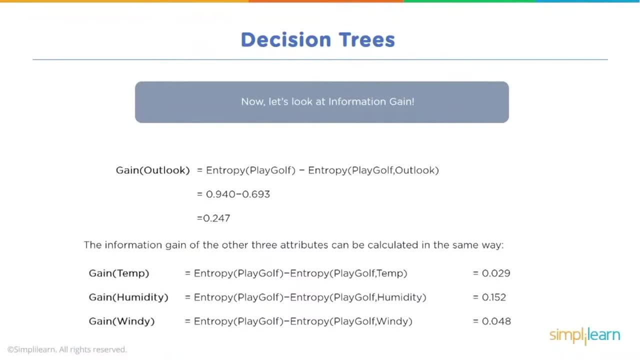 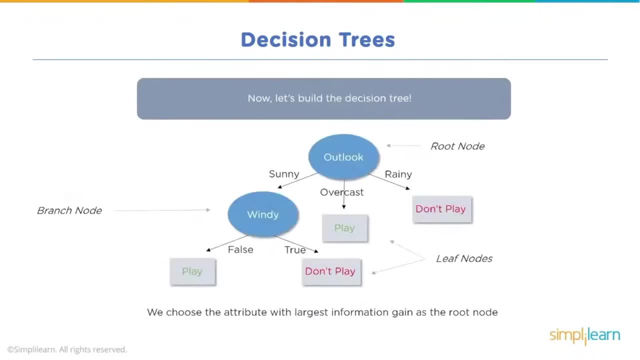 And our gain for a windy day equals point oh four eight, And if you do a quick comparison You'll see the point two four seven is the greatest gain of information. So that's the split we want. Now let's build the decision tree. 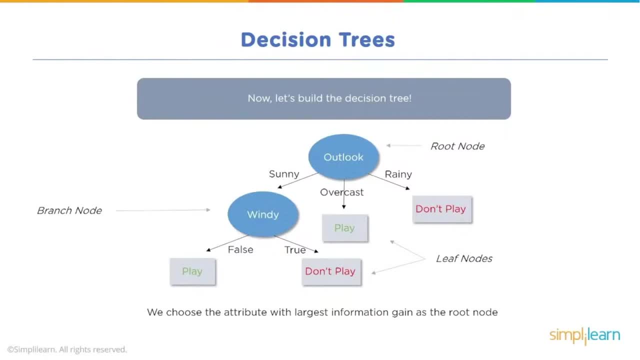 So we have the outlook. Is it going to be sunny, overcast or rainy? That's our first split, because that gives us the most information gain And we can continue to go down the tree using the different information gains with the largest information. 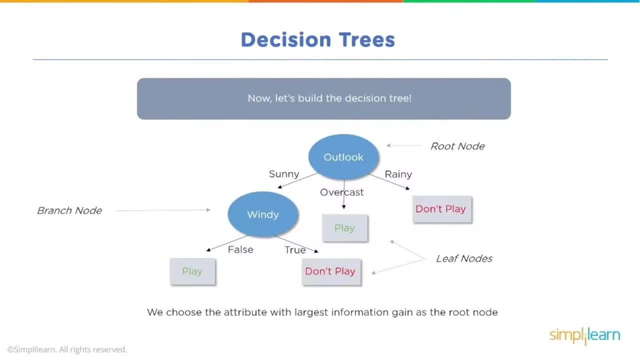 We can continue down the nodes of the tree where we choose the attribute with the largest information gain as the root node And then continue to split each sub node with the largest information gain That we can compute. And although it's a little bit of a tongue twister to say all that, 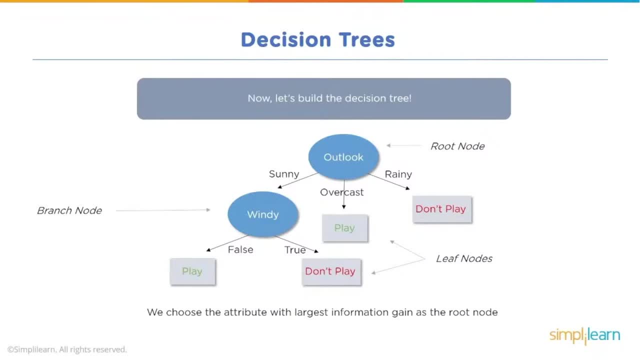 You can see that it's a very easy to view visual model. We have our outlook. We split it three different directions. If the outlook is overcast, we're going to play, And then we can split those further down if we want. So if the outlook is sunny, 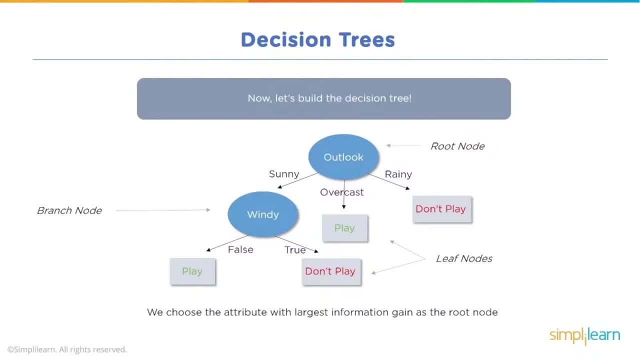 But then it's also windy. If it's windy, we're not going to play, If it's not windy, we'll play. So we can easily build a nice decision tree to guess what we would like to do tomorrow And give us a nice recommendation for the day. 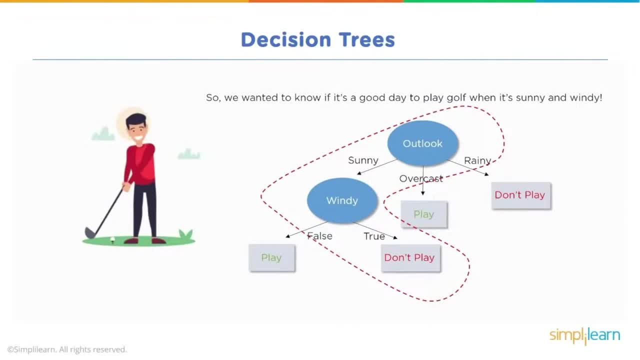 So we want to know if it's a good day to play golf when it's sunny and windy. Remember the original question that came out. Tomorrow's weather report is sunny and windy. You can see by going down the tree we go. outlook- sunny. 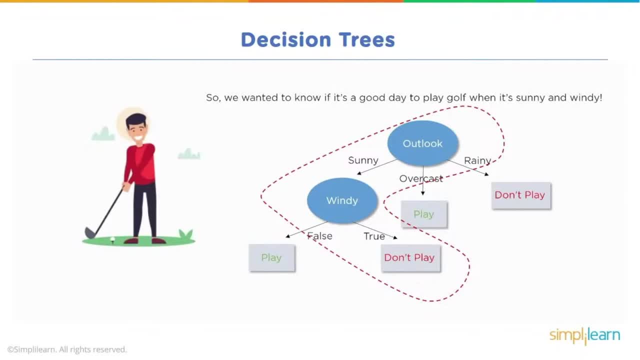 Outlook: windy. We're not going to play golf tomorrow. So our little smart watch pops up and says: I'm sorry, Tomorrow's not a good day for golf. It's going to be sunny and windy And if you're a huge golf fan, you might go. uh oh. 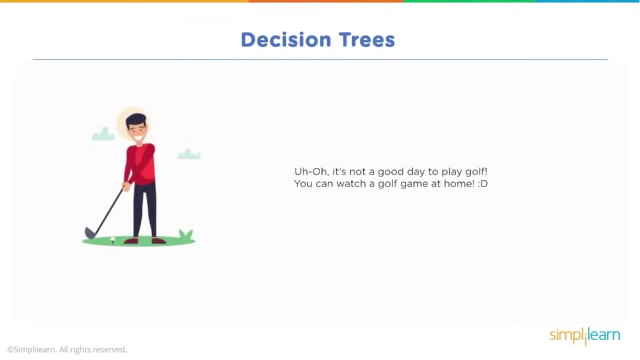 It's not a good day to play golf. We can go in and watch a golf game at home, So we'll sit in front of the TV instead of being out playing golf in the wind. Now that we've looked at our decision tree, 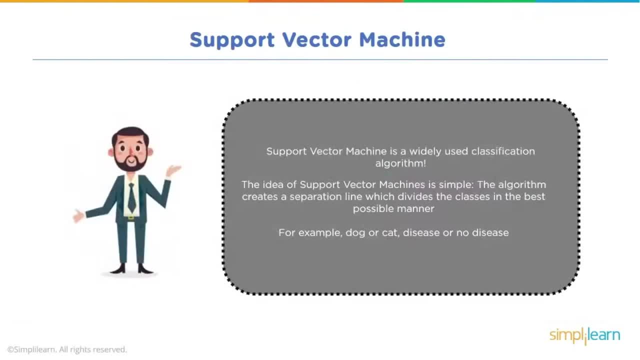 Let's look at the third one of our algorithms. we're investigating Support vector machine. Support vector machine is a widely used classification algorithm. The idea of support vector machine is simple: The algorithm creates a separation line which divides the classes in the best possible manner. 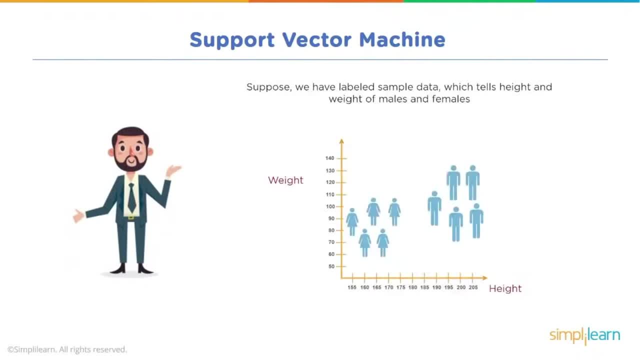 For example, dog or cat disease or no disease. Suppose we have a labeled sample data Which tells height and weight of males and females. A new data point arrives and we want to know whether it's going to be a male or a female. 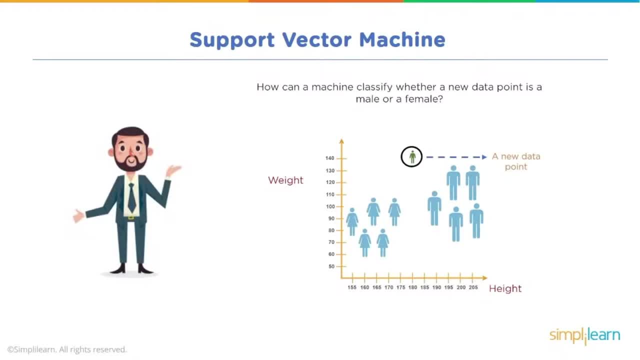 So we start by drawing a line, We draw decision lines, but if we consider decision line one, then we will classify the individual as a male, And if we consider decision line two then it will be a female. So you can see, this person kind of lies in the middle of the two groups. 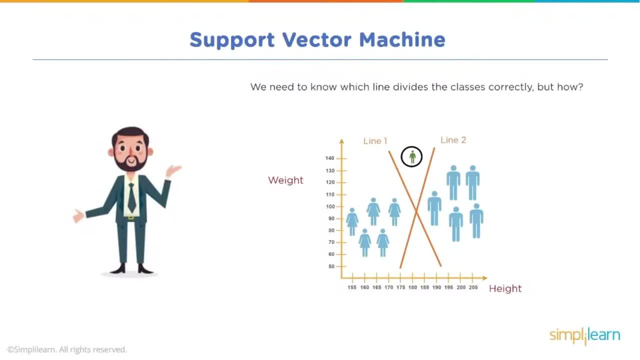 It's a little confusing trying to figure out which line they should be under. We need to know which line divides the classes correctly, but how. The goal is to choose a hyperplane, And that is one of the key words they use when we talk about support vector machines. 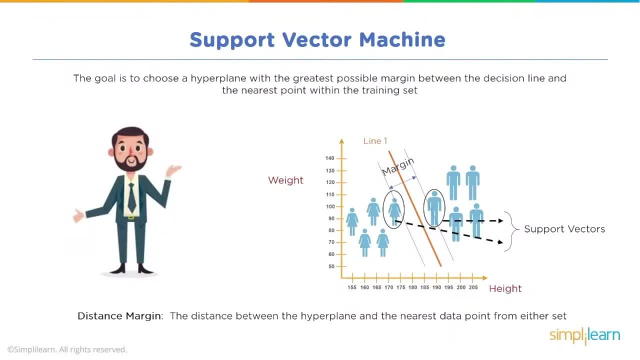 Choose a hyperplane with the greatest possible margin between the decision line and the nearest point within the training set. So you can see, here we have our support vector, We have the two nearest points to it and we draw a line between those two points. 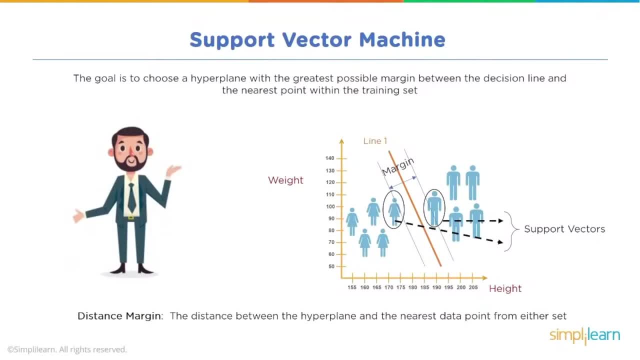 And the distance margin is the distance between the hyperplane and the nearest data point From either set. So we actually have a value and it should be equally distant between the two points that we're comparing it to. When we draw the hyperplanes, we observe that line one has a maximum distance. 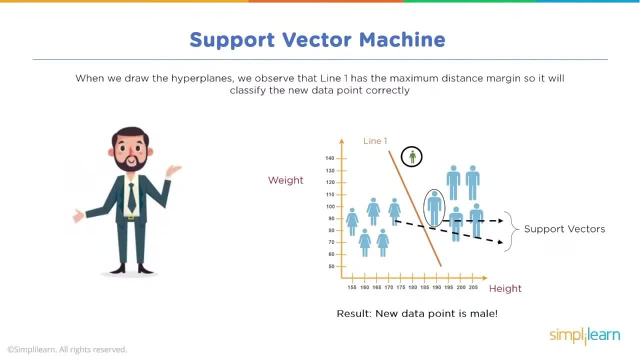 So we observe that line one has a maximum distance margin, so we'll classify the new data point correctly And our result on this one is going to be that the new data point is male. One of the reasons we call it a hyperplane versus a line is that a lot of times we're not looking at just a line. 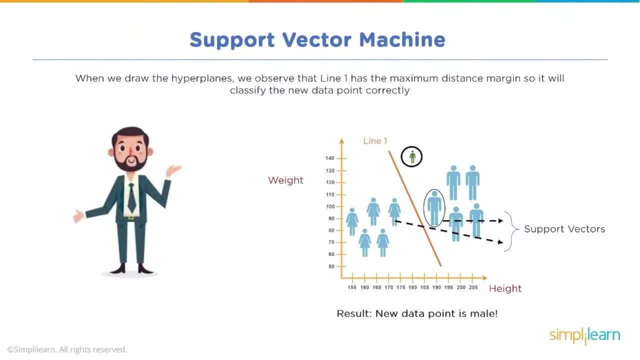 We're looking at just weight and height. We might be looking at 36 different features or dimensions, And so when we cut it with a hyperplane, it's more of a three-dimensional cut in the data or multi-dimensional. It cuts the data a certain way. 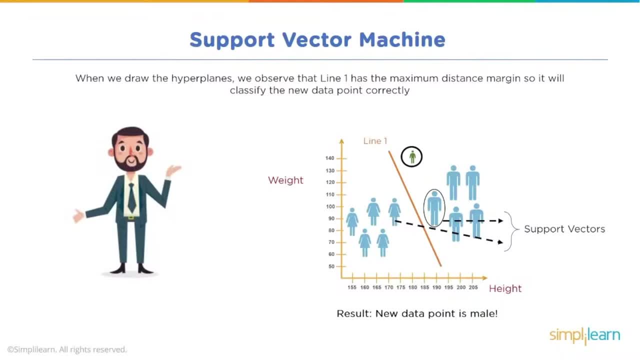 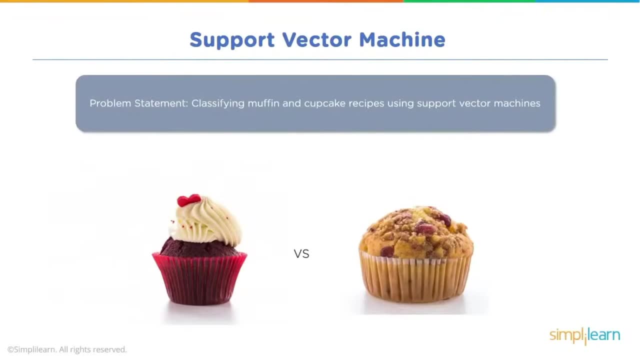 And each plane continues to cut it down until we get the best fit or match. Let's understand this with the help of an example Problem statement. I always start with a problem statement when you're going to put some code together. We're going to do some coding now. 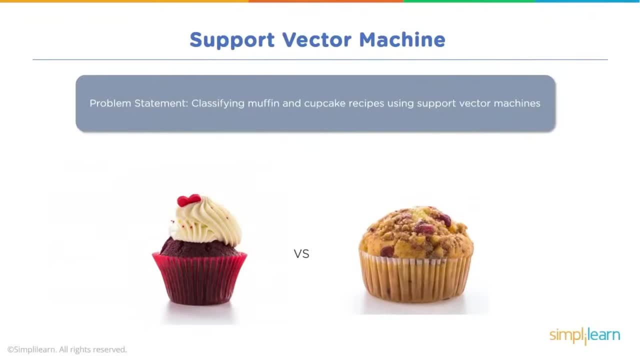 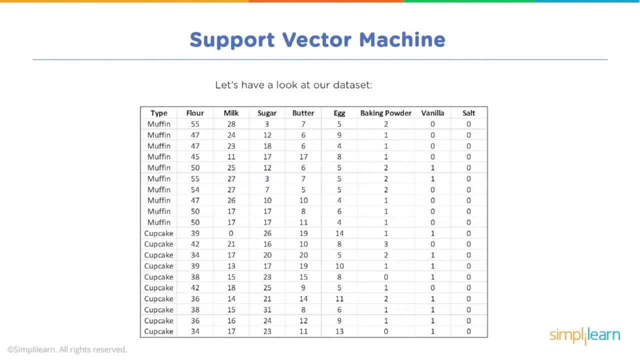 Classifying muffin and cupcake recipes using support vector machines. Cupcake versus the muffin. Let's have a look at our data set And we have the different recipes. here We have a muffin recipe that has so much flour- I'm not sure what measurement 55 is in, but it has 55.. 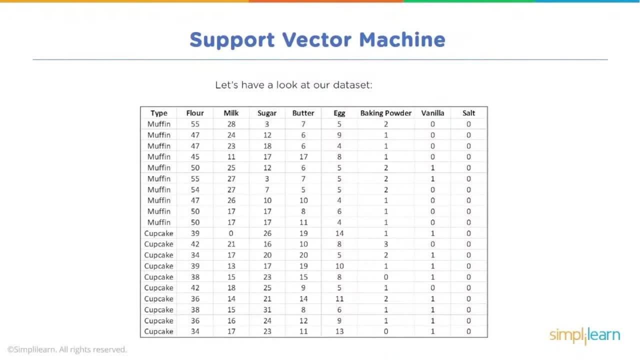 Maybe it's ounces, But it has a certain amount of flour, a certain amount of milk, sugar, butter, egg, baking powder, vanilla and salt, And so, based on these measurements, we want to guess whether we're making a muffin or a cupcake. 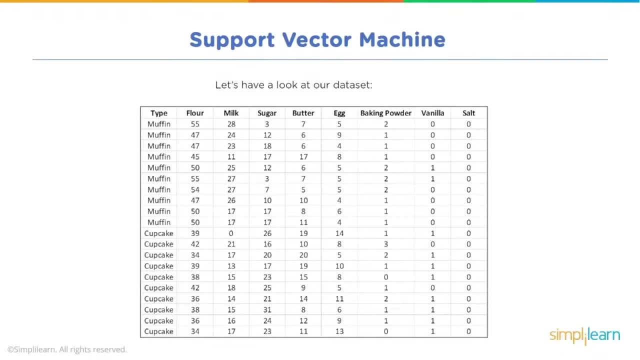 And you can see, in this one we don't have just two features, We just have height and weight, as we did before, between the male and female, And here we have a number of features. In fact, in this we're looking at eight different features to guess whether it's a muffin or a cupcake. 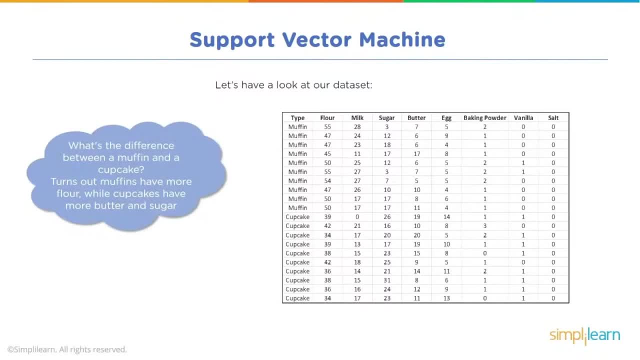 What's the difference between a muffin and a cupcake? Turns out, muffins have more flour, while cupcakes have more butter and sugar. So basically, the cupcake's a little bit more of a dessert, where the muffin's a little bit more of a fancy bread. 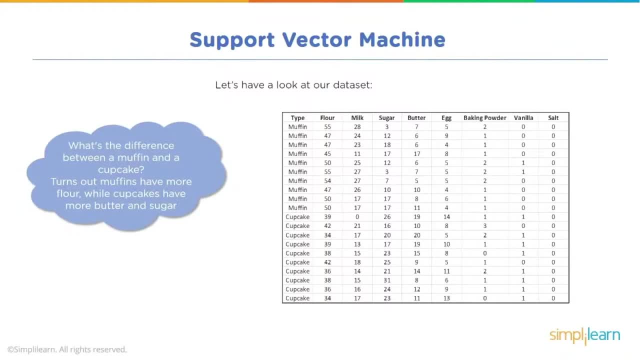 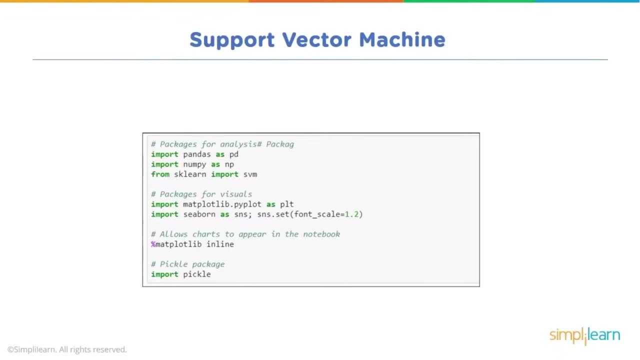 But how do we do that in Python? How do we code that to go through recipes and figure out what the recipe is? And I really just want to say cupcakes versus muffins, Like some big professional wrestling thing. Before we start in our cupcakes versus muffins, we are going to be working in Python. 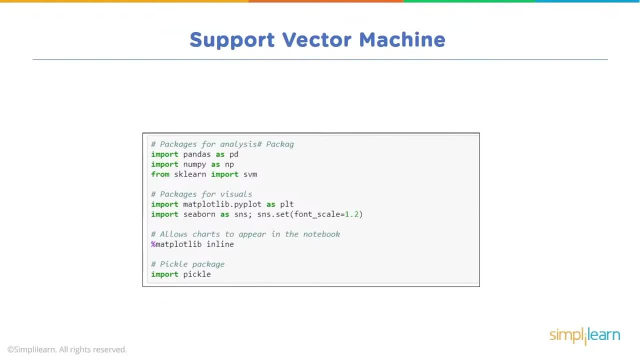 There's many versions of Python, many different editors. That is one of the strengths and weaknesses of Python, is it just has so much stuff attached to it. It's one of the more popular data science programming packages you can use. In this case, we're going to go ahead and use Anaconda in Jupyter Notebook. 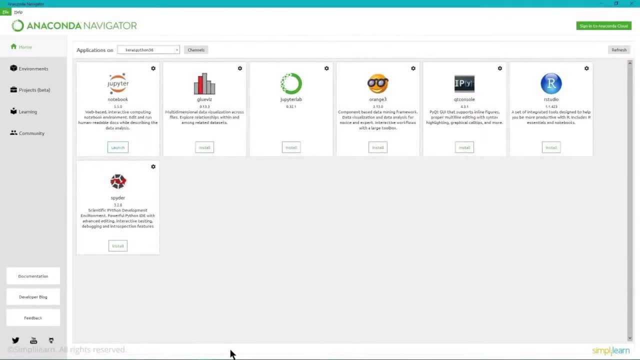 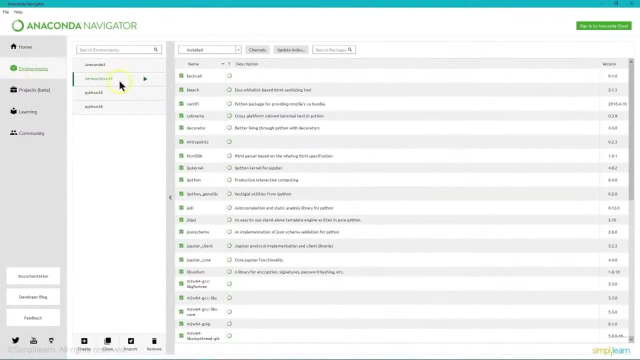 The Anaconda Navigator has all kinds of fun tools. Once you're into the Anaconda Navigator, you can change environments. I actually have a number of environments on here. We'll be using Python 3.6 environment, So this is in Python version 3.6.. 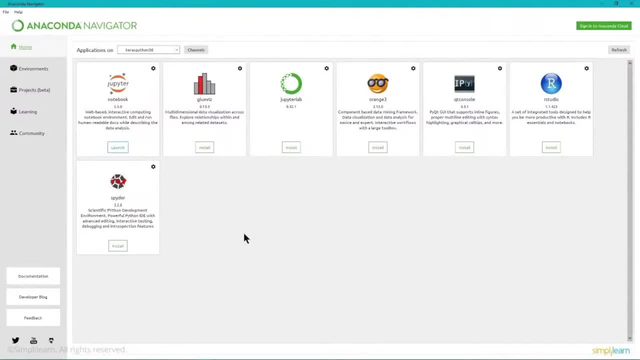 Although it doesn't matter too much which version you use, I usually try to stay with the 3.x because they're current, Unless you have a project that's very specifically in version 2.x. 2.7, I think, is usually what most people use in the version 2.. 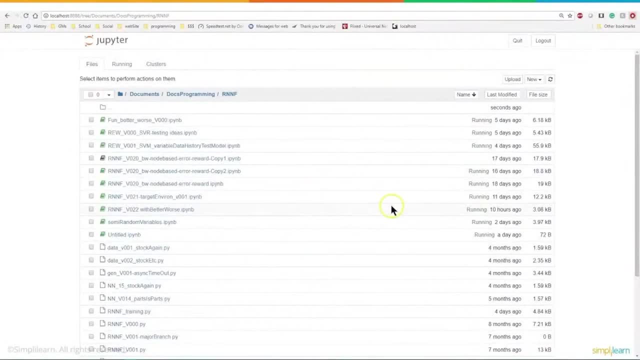 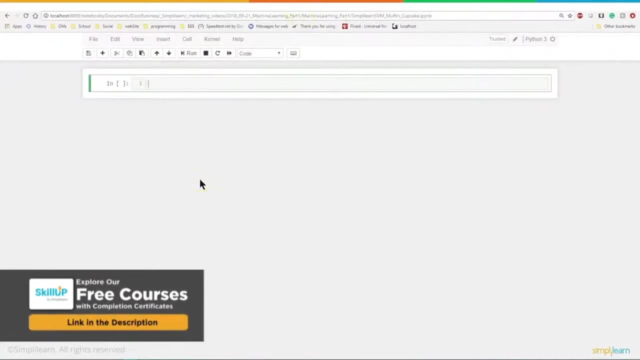 And then, once we're in our Jupyter Notebook editor, I can go up and create a new file, And we'll just jump in here. In this case, we're doing SVM muffin versus cupcake. And then let's start with our packages for data analysis. 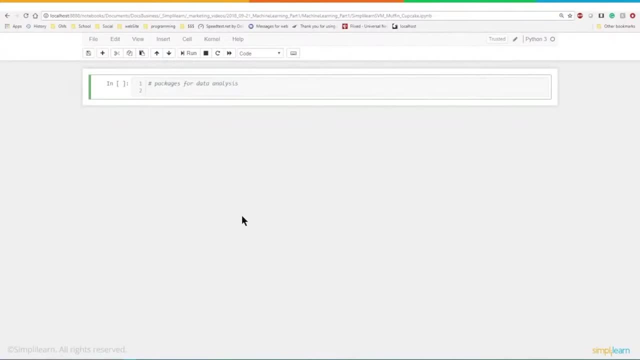 And we almost always use this. There's a few very standard packages we use. We use import numpy, That's for number Python. They usually denote it as np. That's very common. And then we're going to import pandas as pd. 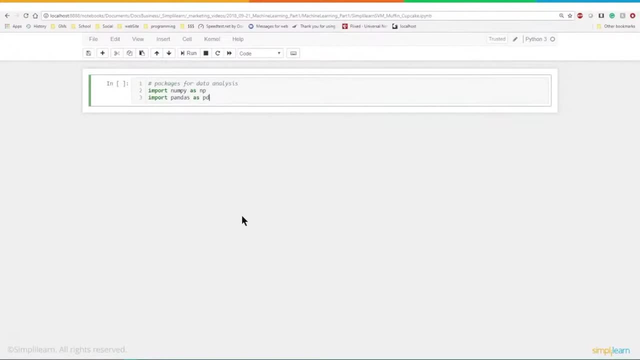 And numpy deals with number arrays. There's a lot of cool things you can do with the numpy setup. As far as multiplying all the values in an array In a numpy array, data array Pandas- I can't remember if we're using it actually in this data set. 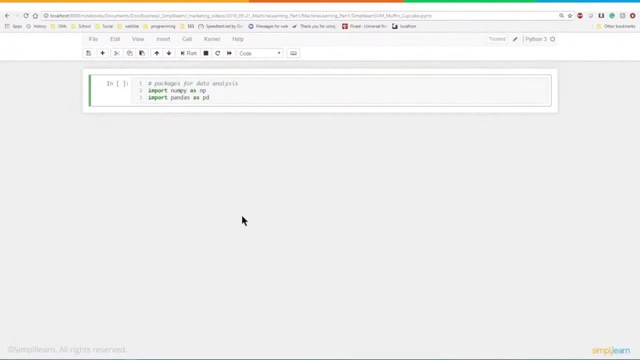 I think we do as an import. It makes a nice data frame And the difference between a data frame and a numpy array is that a data frame is more like your Excel spreadsheet: You have columns, You have indexes, So you have different ways of referencing it. 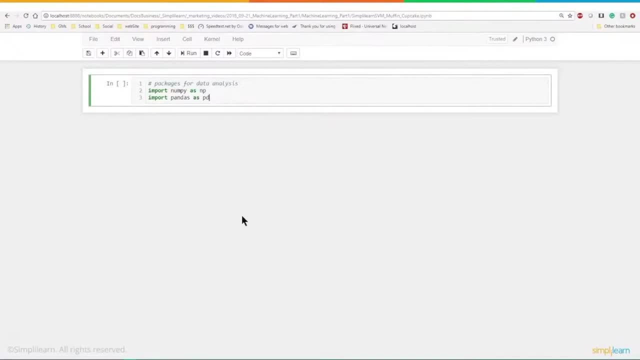 Easily viewing it And there's additional features. you can run on a data frame And pandas kind of sits on numpy, So you need them both in there. And then finally we're working with the support vector machine. So from sklearn We're going to use the sklearn model. 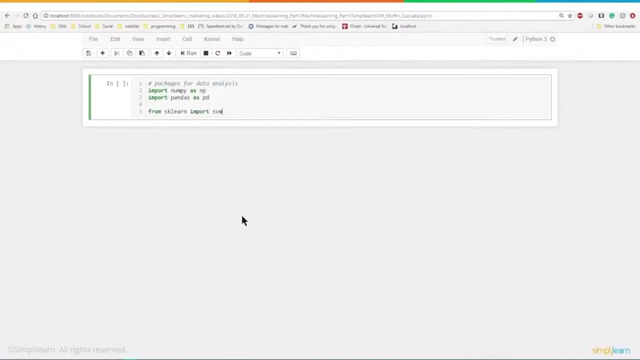 Import svm Support vector machine And then, as a data scientist, you should always try to visualize your data. Some data obviously is too complicated or doesn't make any sense to the human, But if it's possible it's good to take a second look at it. 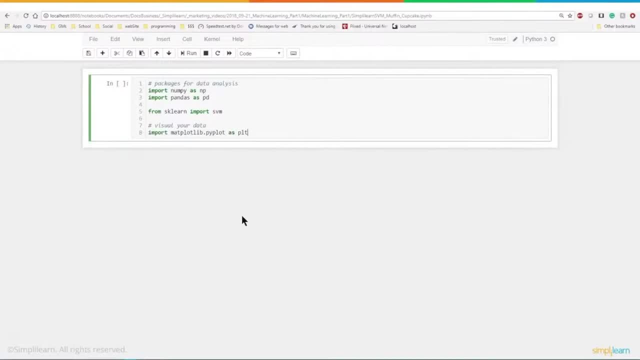 So that you can actually see what you're doing. Now for that we're going to use two packages. We're going to import matplotlibrarypyplot as plt- Again very common- And we're going to import seaborn as sns And we'll go ahead and set the font scale in the sns right in our import line. 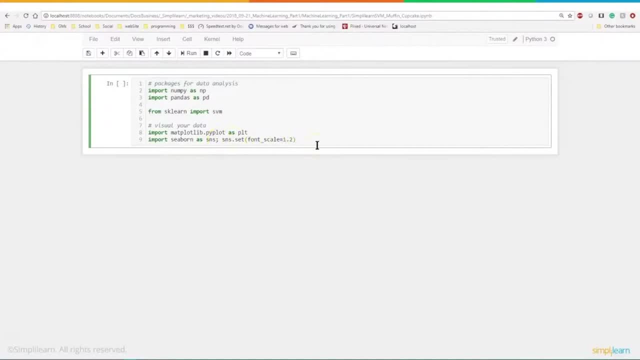 That's with this semicolon, followed by a line of data, We're going to set the sns. And these are great because the seaborn sits on top of matplotlibrary Just like pandas sits on numpy. So it adds a lot more features and uses and control. 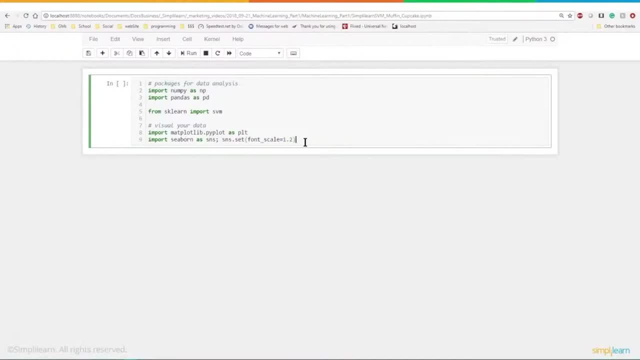 We're obviously not going to get into matplotlibrary and seaborn. That would be it's own tutorial. We're really just focusing on the svm, The support vector machine from sklearn, And since we're in Jupyter Notebook, We have to add a special line in here for our matplotlibrary. 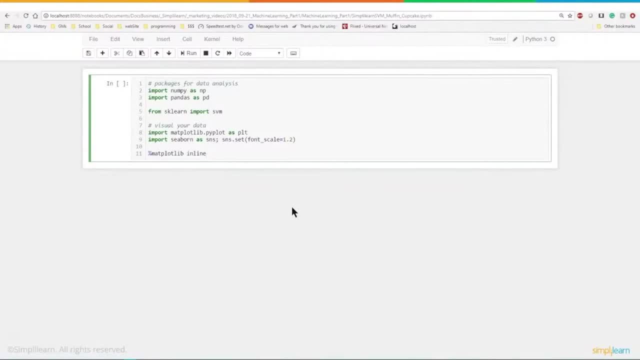 And that's your percentage sign or amber sign. matplotlibrary inline. Now, if you're doing this in just a single line, A straight code project- A lot of times I use like notepad++ And I'll run it from there. You don't have to have that line in there. 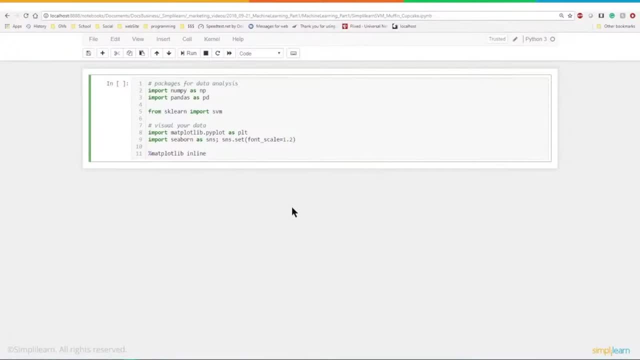 Because it'll just pop up as it's own window on your computer, Depending on how your computer is set up. Because we're running this in the Jupyter Notebook as a browser setup, This tells it to display all of our graphics right below on the page. 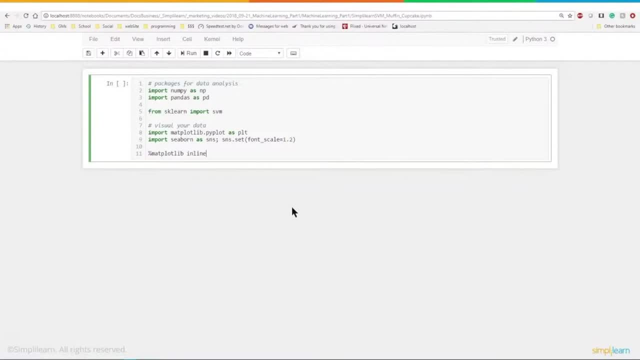 So that's what that line is for. Remember, the first time I ran this I didn't know that I had to go look that up years ago. It was quite a headache. But the reason it's inline is just because we're running this on the web setup. 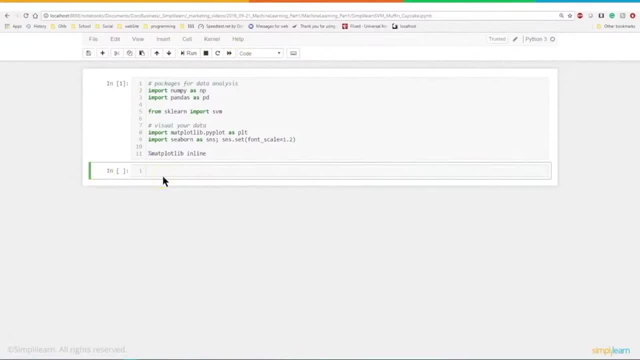 And we can go ahead and run this. Make sure all our modules are in. They're all imported, which is great. If you don't have them import, You'll need to go ahead and pip, Use the pip or however you do it. 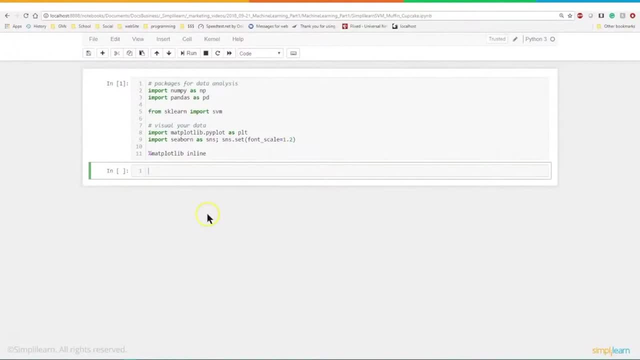 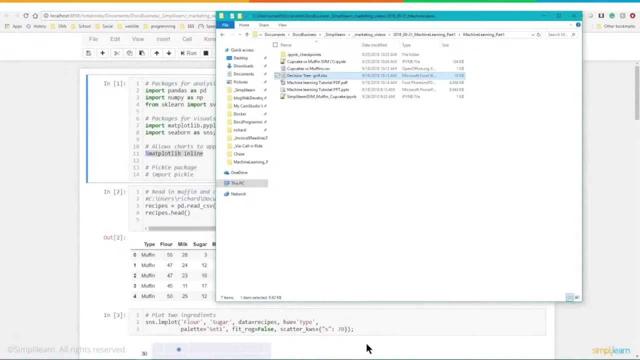 There's a lot of other install packages out there, Although pip is the most common, And you have to make sure these are all installed on your Python setup. The next step, of course, is we got to look at the data. You can't run a model for predicting data if you don't have actual data. 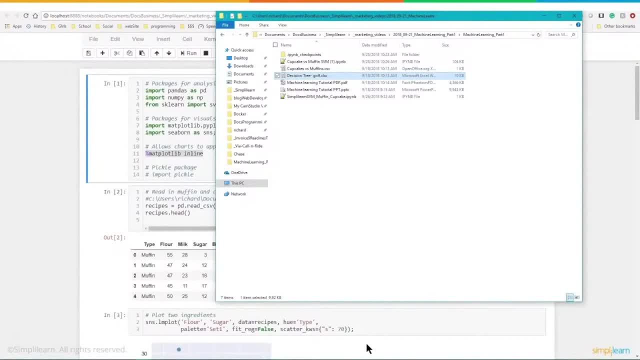 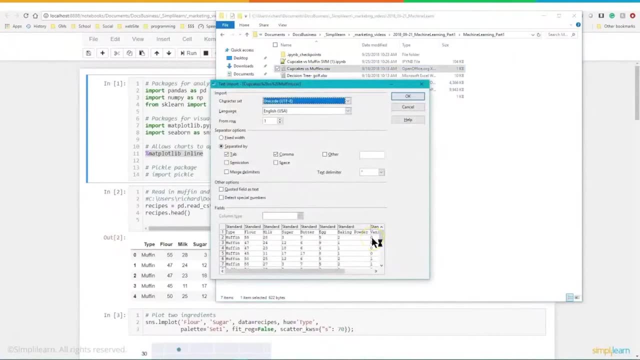 So to do that, let me go ahead and open this up And take a look, And we have our cupcakes versus muffins And it's a CSV file, or CSV, meaning that it's comma separated variable- And it's going to open it up in a nice spreadsheet for me. 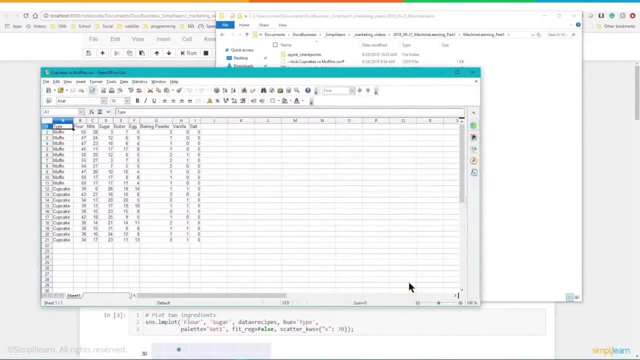 And you can see up here we have the type We have muffin, muffin, muffin cupcake, cupcake cupcake, And then it's broken up into flour, milk, sugar, butter, egg, baking powder, vanilla and salt. 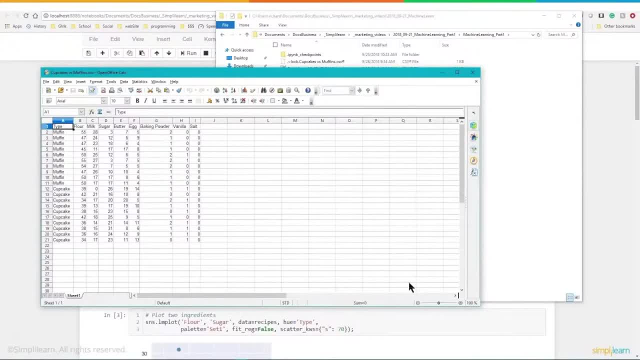 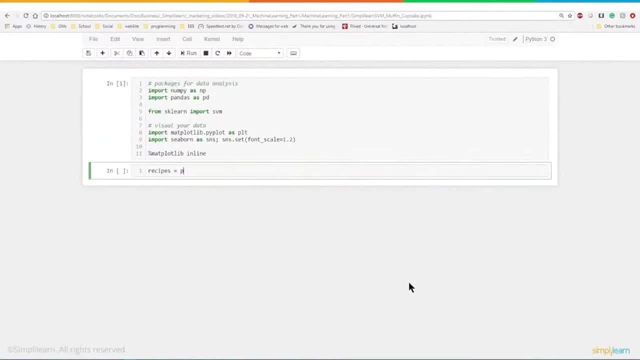 So what we can do is we can go ahead and look at this data And also in our Python, Let us create a variable recipes equals. We're going to use our pandas module readCSV. Remember it was a comma separated variable. 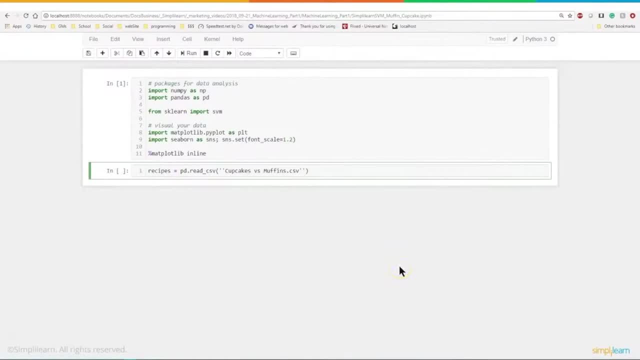 And the file name happened to be cupcakes versus muffins. Oops, I got double brackets there. Do it this way. There we go: Cupcakes versus muffins. Because the program I loaded or the place I saved- this particular Python program- is in the same folder. 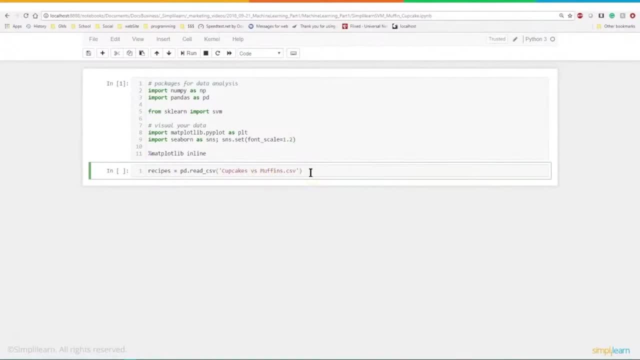 We can get by with just the file name, But remember, if you're storing it in a different location, you have to also put down the full path on there. And then, because we're in pandas, We're going to go ahead and you can actually inline. you can do this. 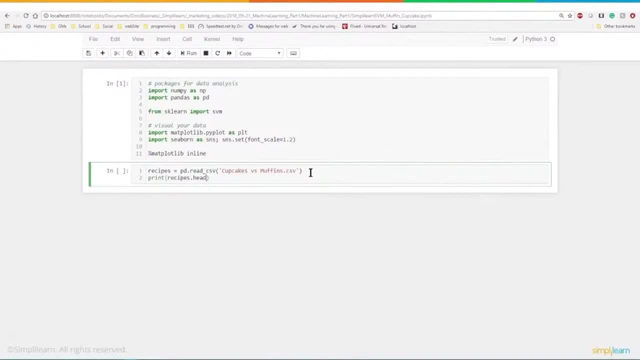 But let me do the full print. You can just type in recipeshead in the Jupyter notebook, But if you're running in code in a different script you need to go ahead and type out the whole print, recipeshead. And pandas knows that. that's going to do the first five lines of data. 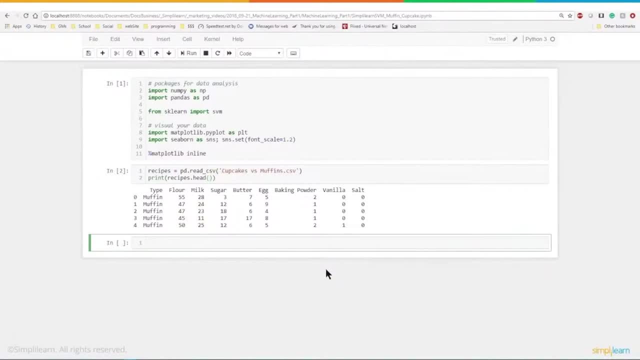 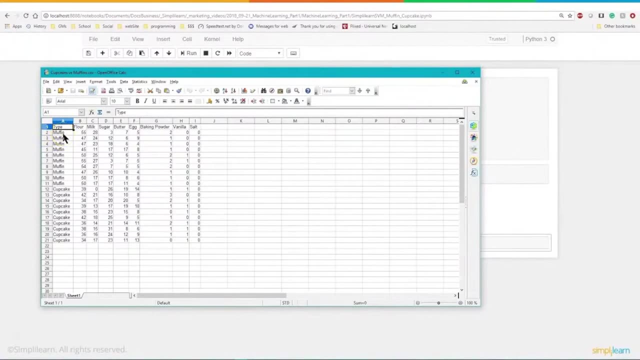 And if we flip back on over to the spreadsheet where we opened up our CSV file, You can see where it starts, on line two. This one calls it zero And then two, three, four, five, six is going to match. Go ahead and close that out, because we don't need that anymore. 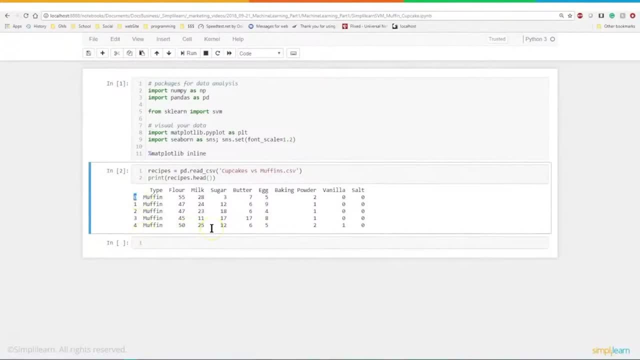 And it always starts at zero. It automatically indexes it, since we didn't tell it to use an index in here. So that's the index number for the left hand side And it automatically took the top row as labels. So, pandas, using it to read a CSV is just really slick and fast. 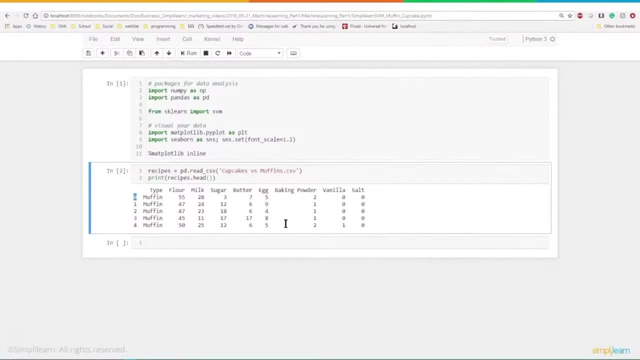 One of the reasons we love our pandas Not just because they're cute and cuddly teddy bears. And let's go ahead and plot our data. And I'm not going to plot all of it, I'm just going to plot the sugar and flour. 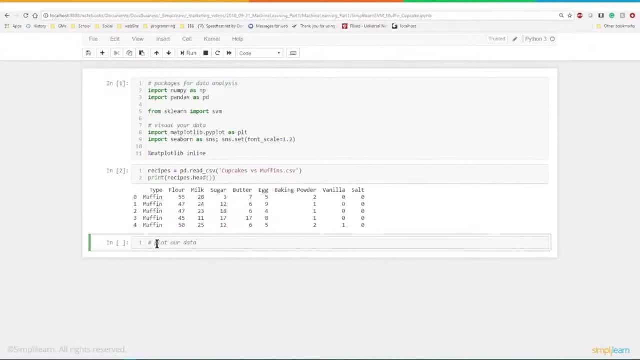 Now, obviously you can see where they get really complicated if we have tons of different features, And so you'll break them up and maybe look at just two of them at a time to see how they connect And to plot them. we're going to go ahead and use Seaborn. 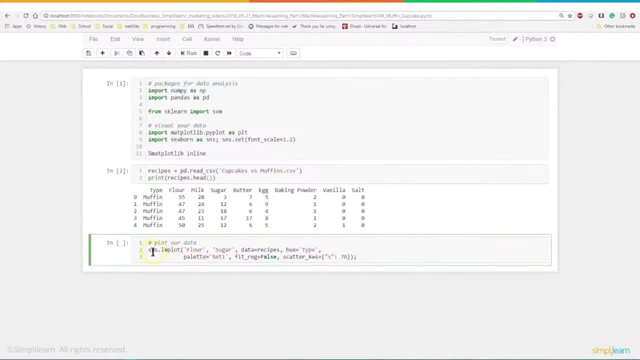 So that's our SNS And the command for that is snslmplot. And then the two different variables I'm going to plot is flour and sugar. Data equals recipes, The hue equals type, And this is a lot of fun, because it knows that this is pandas coming in. 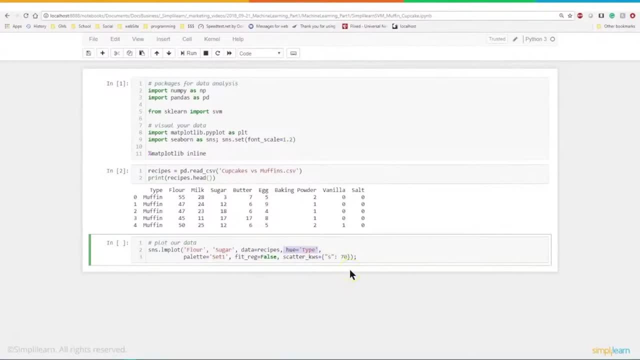 So this is one of the powerful things about pandas mixed with Seaborn in doing graphing, And then we're going to use a palette set one. There's a lot of different sets in there. You can go look them up for Seaborn. 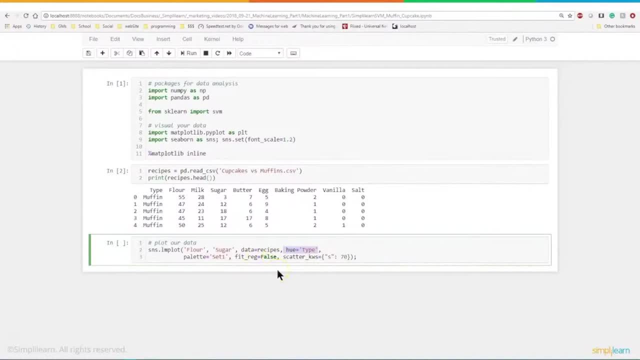 We're going to do a fit. regular equals false. So we're not really trying to fit anything And it's a scatter KWS. A lot of these settings you can look up in Seaborn. Half of these you could probably leave off when you run them. 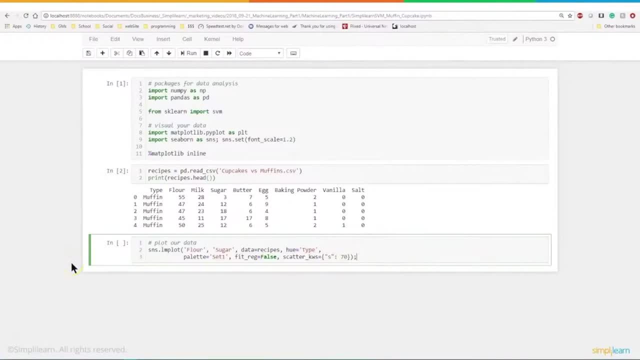 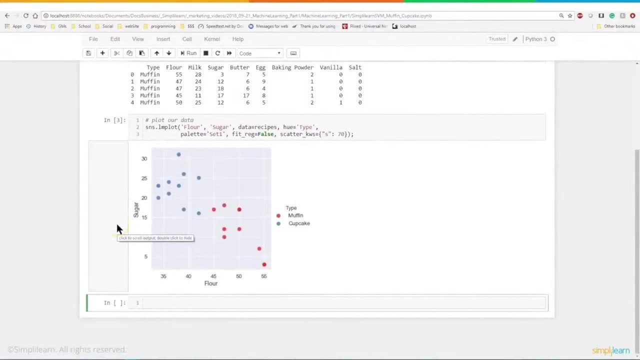 Somebody played with this and found out that these were the best settings for doing a Seaborn plot, And let's go ahead and run that. And because it does it inline, it just puts it right on the page And you can see right here that just based on sugar and flour alone, there's a definite split. 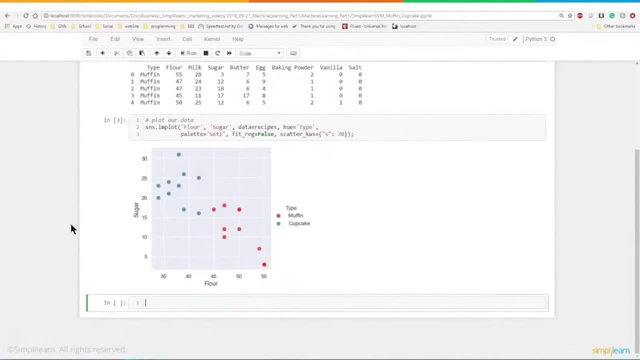 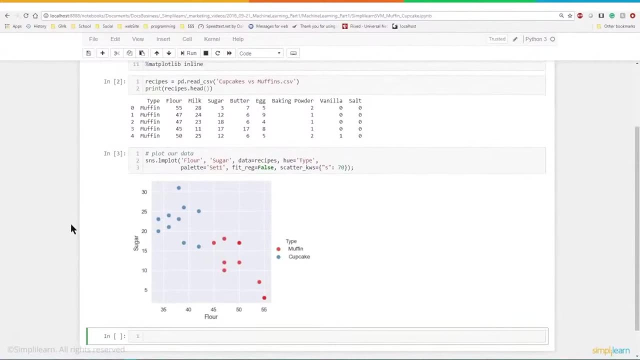 And we use these models because you can actually look at it and say, hey, if I drew a line right between the middle of the blue dots and the red dots, we'd be able to do an SVM and a hyperplane right there in the middle. Then the next step is to format or pre-process our data. 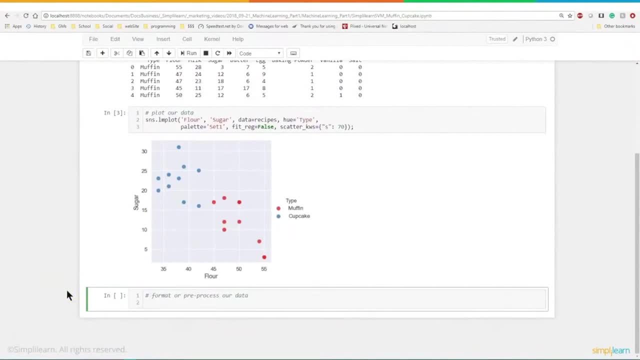 And we're going to break that up into two parts. We need a type label And remember, we're going to decide whether it's a muffin or a cupcake. Well, a computer doesn't know muffin or cupcake. It knows zero and one. 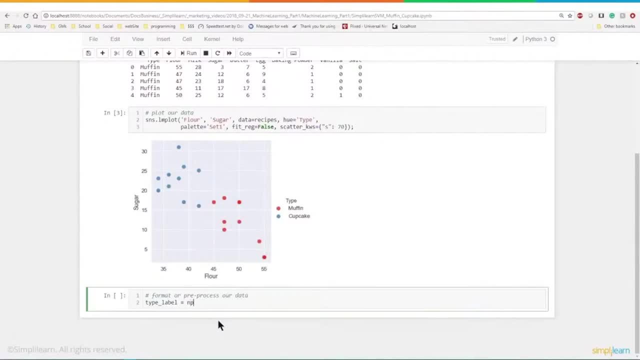 So what we're going to do is we're going to create a type label And from this we'll create a numpy array and p where- and this is where we can do some logic- We take our recipes from our panda and wherever a type equals muffin, it's going to be zero. 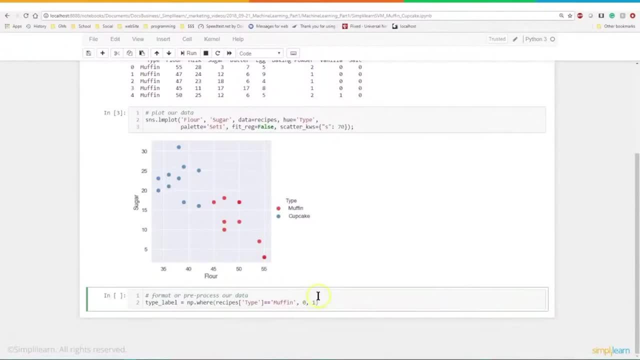 And then if it doesn't equal muffin, which is cupcakes, it's going to be one. So we create our type label. This is the answer. So when we're doing our training model, remember we have to have a training data. This is what we're going to train it with. is that it's zero or one? 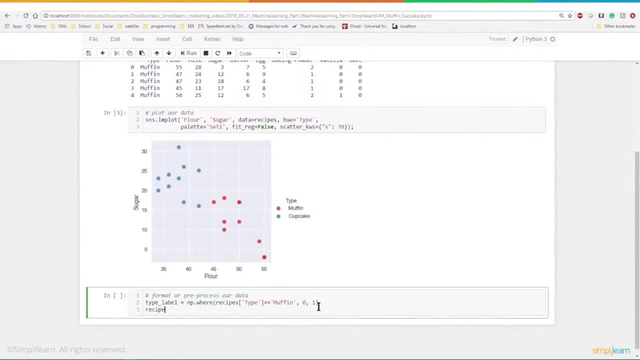 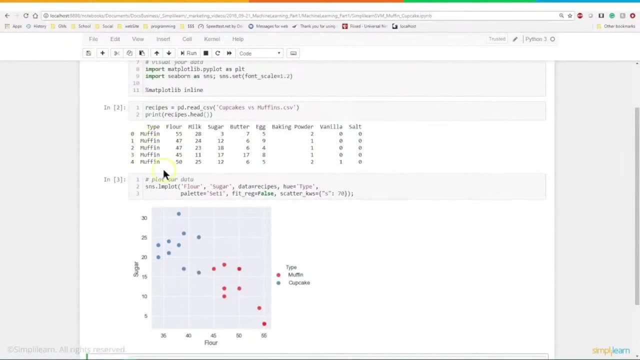 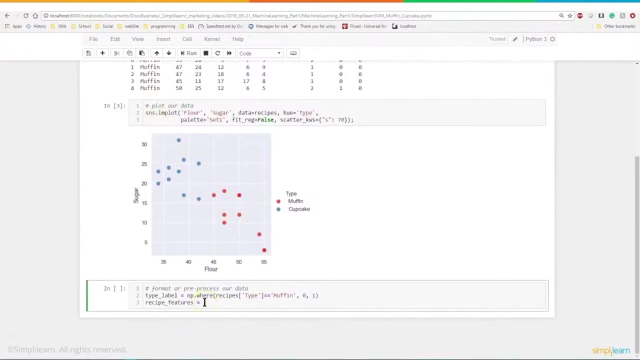 Or it's not, And then we're going to create our recipe features And if you remember correctly from right up here, the first column is type. So we really don't need the type column, because that's our muffin or cupcake And in pandas we can easily sort that out. 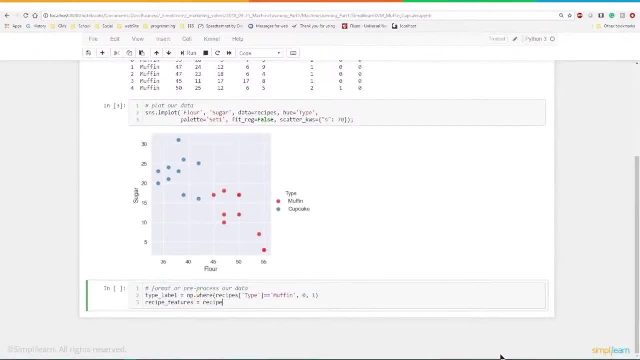 We take our value recipescolumns. That's a pandas function built into pandas. We've got values converting them to values, So it's just the column titles going across the top, And we don't want the first one. So what we do is, since it always starts at zero, we want one colon till the end. 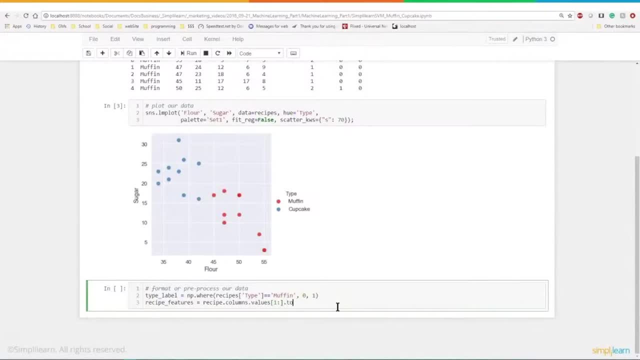 And then we want to go ahead and make this a list And this converts it to a list of strings, And then we can go ahead and just take a look and see what we're looking at for the features. Make sure it looks right. 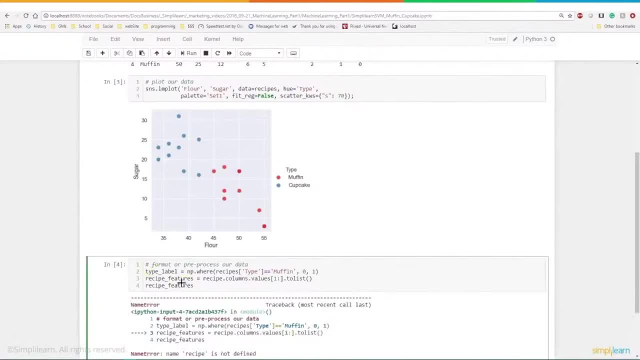 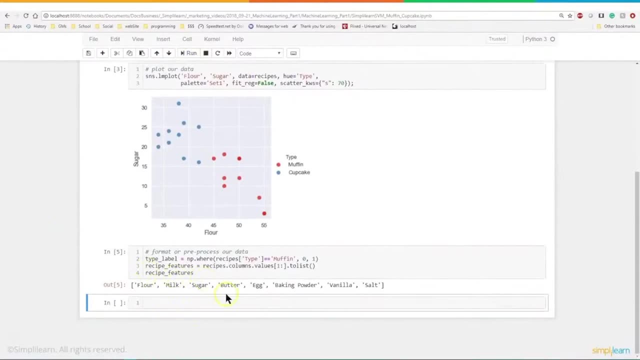 Go ahead and run that And I forgot the S on recipes. So we'll go ahead and add the S in there and then run that And we can see we have flour, milk, sugar, butter, egg, baking powder, vanilla and salt. 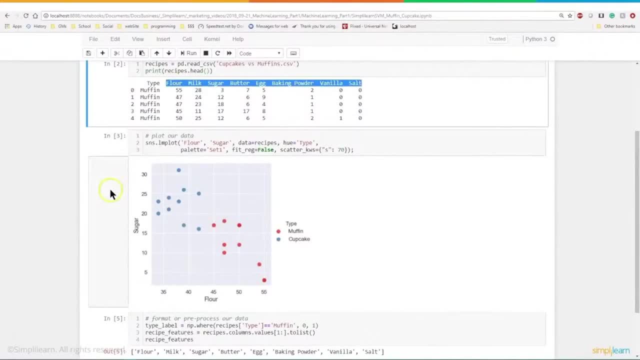 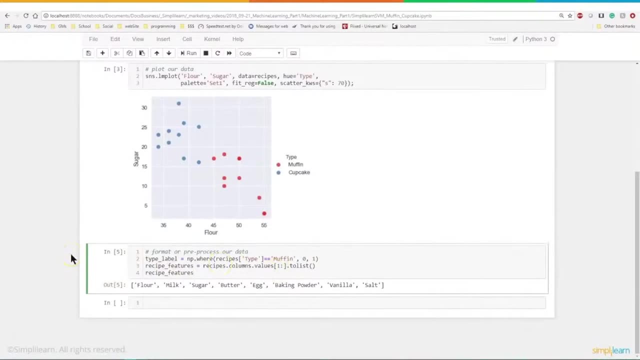 And that matches what we have up here, Right where we printed out everything but the type. So we have our features and we have our label. Now the recipe features is just the titles of the column And we actually need the ingredients, And at this point we have a couple options. 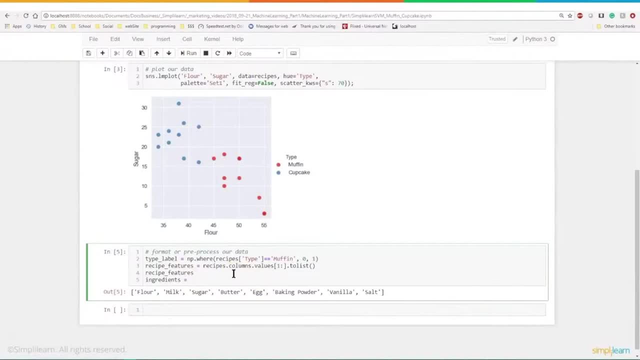 One. we could run it over all the ingredients, And when you're doing this, usually you do, But for our example we want to limit it so you can easily see what's going on, Because if we did all the ingredients we have, you know that's what seven, eight different hyperplanes that would be built into it. 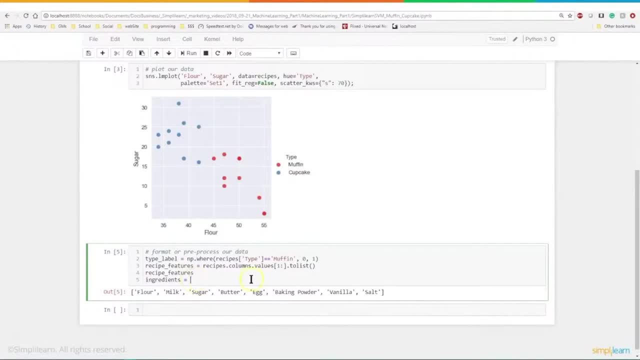 And we only want to look at one so you can see what the SVM is doing. And so we'll take our recipes and we'll do just flour and sugar. Again, you can replace that with your recipe features and do all of them, But we're going to do just flour and sugar and we're going to convert that to values. 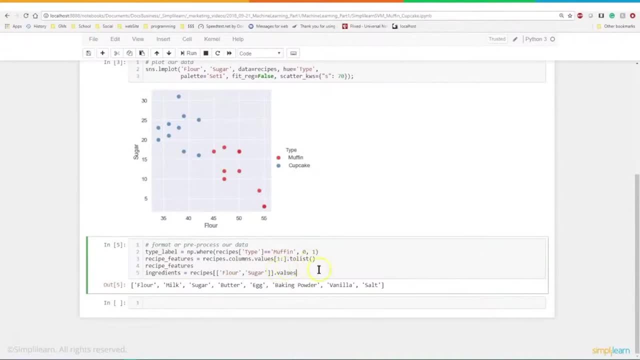 We don't need to make a list out of it because it's not string values. These are actual values on there And we can go ahead and just print ingredients And you can see what that looks like. And so we have just the amount of flour and sugar, just the two sets of plots. 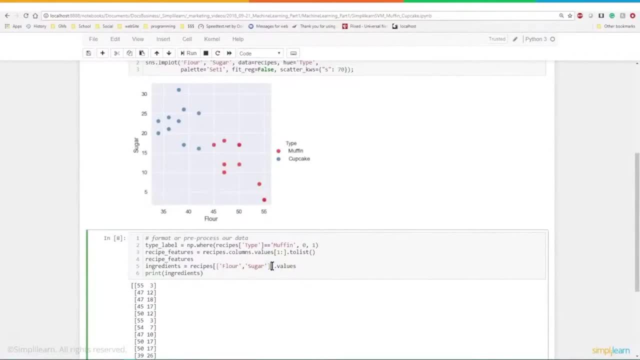 And just for fun, let's go ahead and take this over here and take our recipe features, And so if we decided to use all the recipe features, you'll see that it makes a nice column of different data. So it just strips out all the labels and everything. 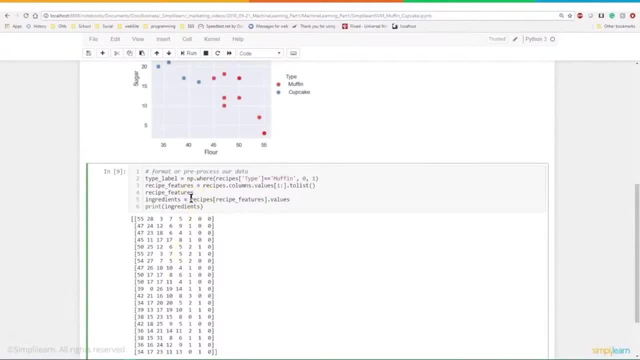 We just have just the values. But because we want to be able to view this easily in a plot later on, we'll go ahead and take that and just do flour and sugar And we'll run that and you'll see, it's just the two columns. 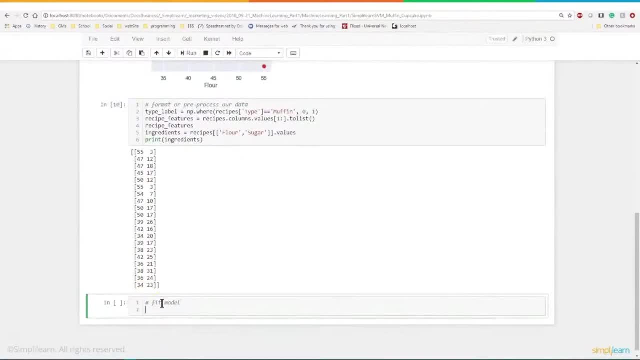 So the next step is to go ahead and fit our model. We'll go ahead and just call it model And it's a SVM. We're using a package called SVC In this case. we're going to go ahead and set the kernel equals linear. 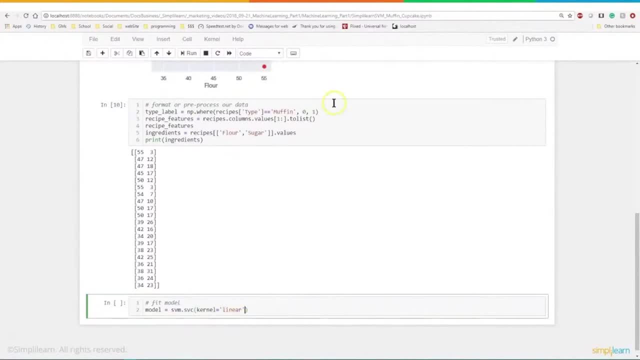 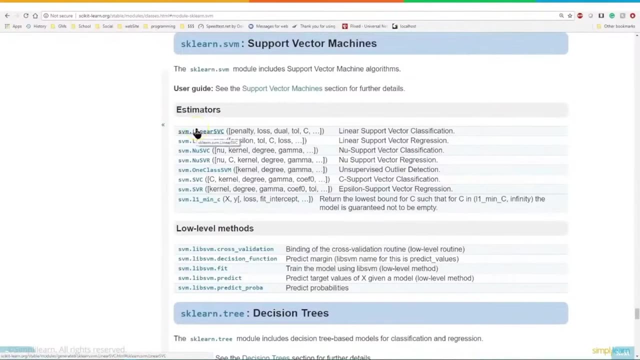 So it's using a specific setup on there. There's a reference on their website for the SVM. You'll see that there's about there's eight of them here. Three of them are for regression, Three are for classification- The SVC support vector, classification, is probably one of the most commonly used. 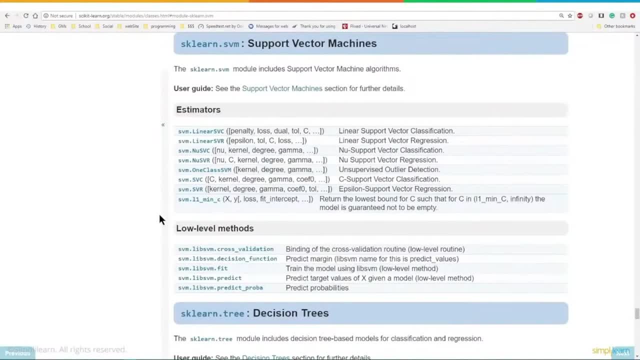 And then there's also one for detecting outliers And another one that has to do with something a little bit more specific on the model, But SVC and SVR are the two most commonly used, standing for support vector classifier and support vector regression. Remember, regression is an actual value. 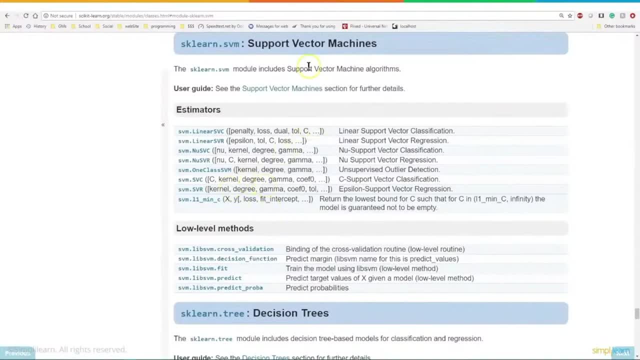 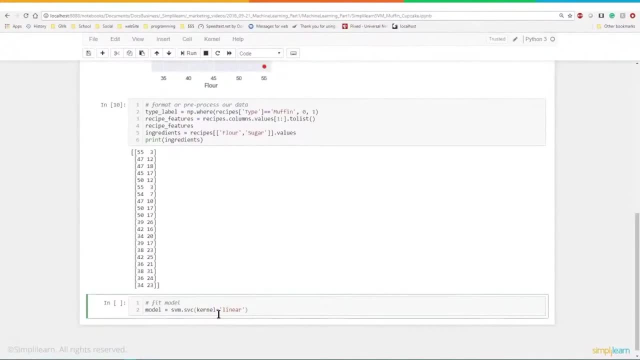 A float value or whatever you're trying to work on, And SVC is a classifier. So it's a yes, no, true, false. But for this we want to know: zero one Muffin cupcake. We go ahead and create our model. 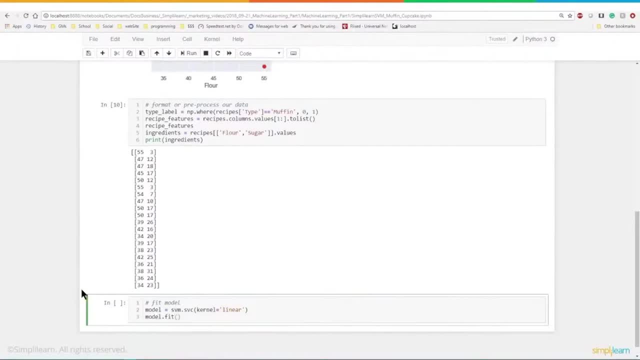 And once we have our model created, we're going to do modelfit, And this is very common, especially in the sklearn. All their models are followed with the fit command, And what we put into the fit, what we're training with it, is we're putting in the ingredients. 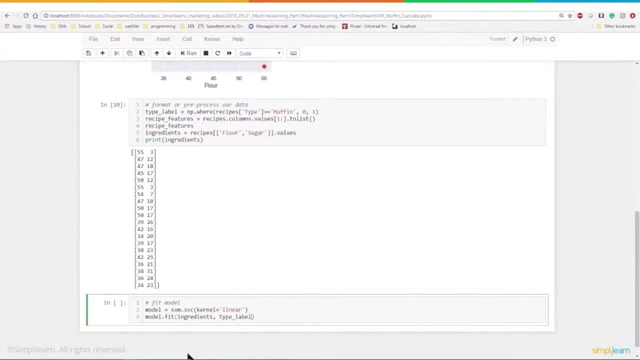 Which, in this case, we limited to just flour and sugar And the type label: Is it a muffin or a cupcake? Now, in more complicated data science series you'd want to split into- we won't get into that today. We split it into training data and test data. 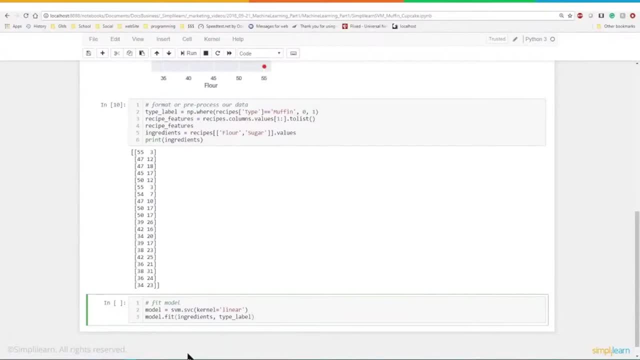 And they even do something where they split it into thirds, Where a third is used for where you switch between which one's training and test. There's all kinds of things that go into that. It gets very complicated when you get to the higher end. 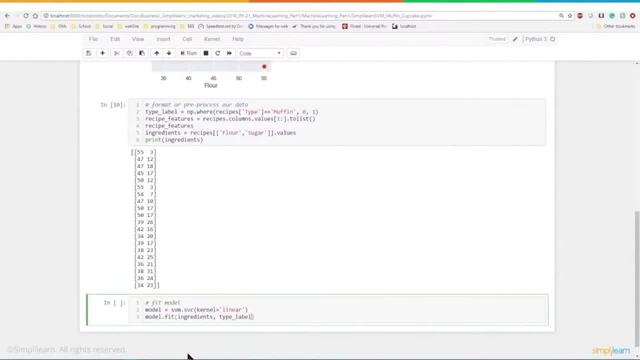 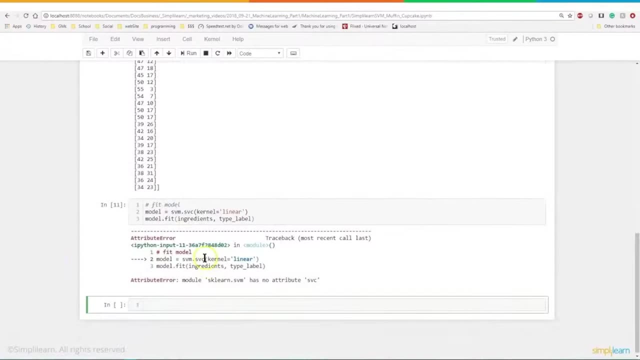 Not overly complicated. Just an extra step, which we're not going to do today, Because this is a very simple set of data, And let's go ahead and run this, And now we have our model fit, And I got an error here. 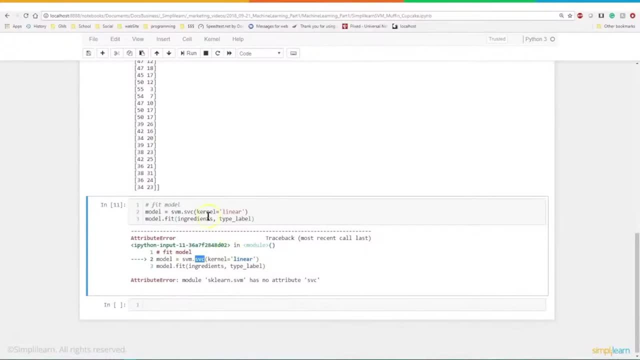 So let me fix that real quick. It's capital SVC, it turns out. I did it lower case Support vector classifier. There we go, Let's go ahead and run that And you'll see it comes up with all this information that it prints out automatically. 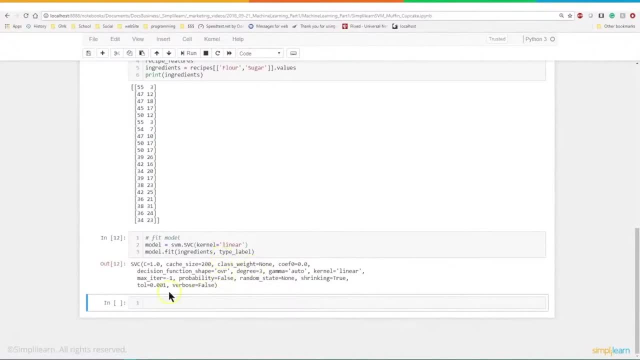 These are the defaults of the model. You notice that we changed the kernel to linear And there's our kernel linear on the printout And there's other different settings you can mess with. We're going to just leave that alone right now for this. 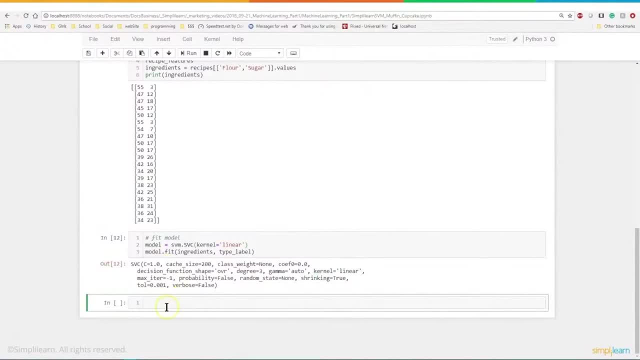 We don't really need to mess with any of those. So next We're going to dig a little bit into our newly trained model And we're going to do this so we can show you on a graph And let's go ahead and get the separating. 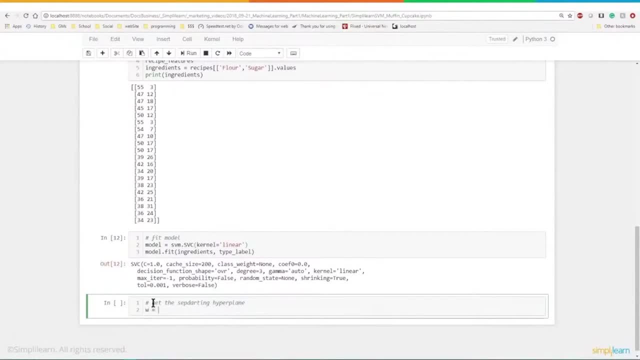 And we're going to say We're going to use a W for our variable on here And we're going to do model dot coefficient underscore zero. So what the heck is that? Again, we're digging into the model. So we've already got a prediction and a train. 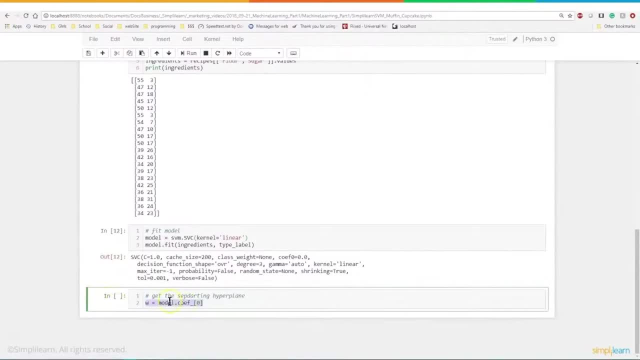 This is the math behind it that we're looking at right now, And so The W is going to represent two different coefficients And if you remember, we had, Y equals MX plus C. So these coefficients are connected to that, But in two dimensional. 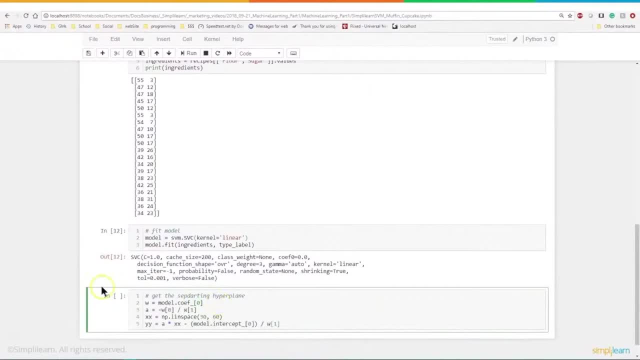 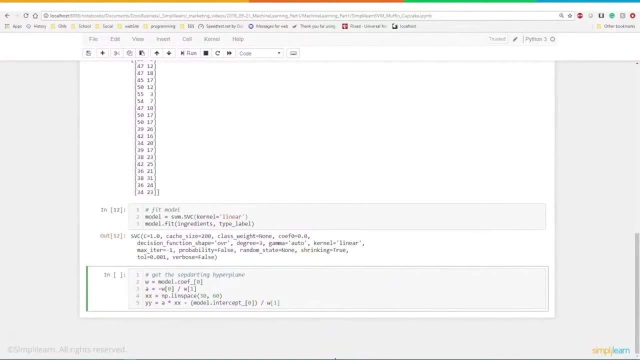 It's a plane. We don't want to spend too much time on this Because you can get lost in the confusion of the math. So if you're a math whiz, this is great. You can go through here And you'll see that we have A equals minus W of zero over W of one. 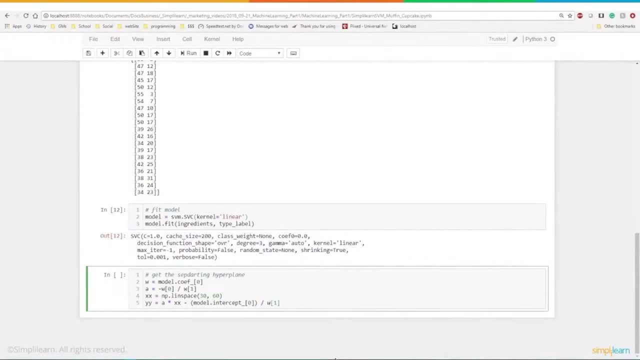 Remember, there's two different values there, And that's basically the slope that we're generating. And then we're going to build an XX. What is XX? We're going to set it up to a numpy array. There's our NP dot line space. 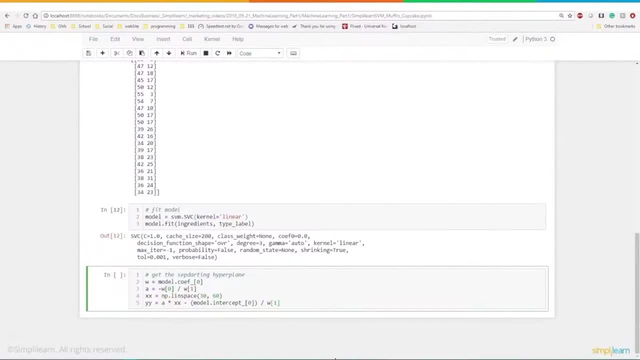 So we're creating a line of values between 30 and 60.. So it just creates a set of numbers for X And then, if you remember correctly, we have our formula: Y equals the slope times X plus the intercept. Well, to make this work, we can do this, as YY equals the slope times each value in that array. 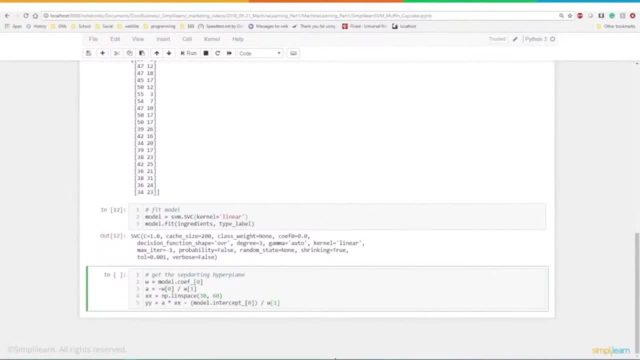 That's the neat thing about numpy. So when I do A times XX, Which is a whole numpy array of values, It multiplies A across all of them And then it takes those same values and we subtract the model intercept. Remember we had MX plus C. 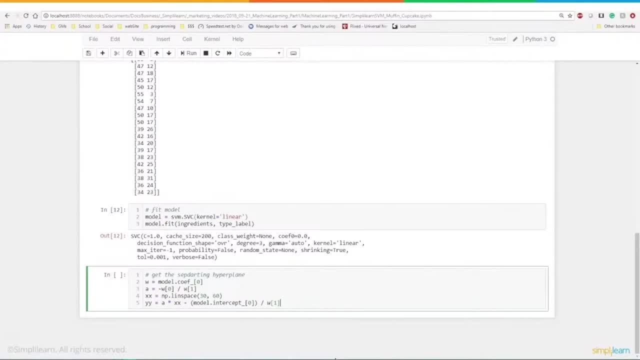 So that would be the C from the formula. Y equals MX plus C, And that's where all these numbers come from. A little bit confusing because it's digging out of these different arrays. And then what we want to do is we're going to take this and we're going to go ahead and plot it. 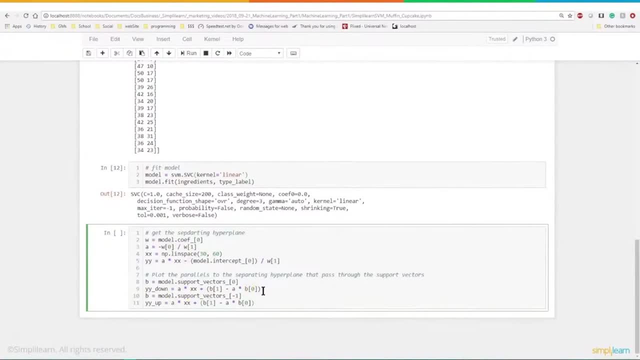 So plot the parallels to separating hyperplane that pass through the support array, And so we're going to create- B equals a model- support vectors. Pulling our support vectors out there, Here's our YY, which we now know is a set of data. 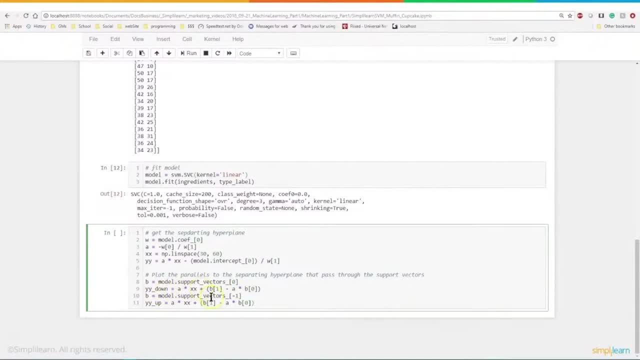 We're going to create: YY down equals A times XX plus B1, minus A times B0.. And then model support, vector B is going to be set that to a new value, The minus one set up. And YY up equals A times XX plus B1 minus B0.. 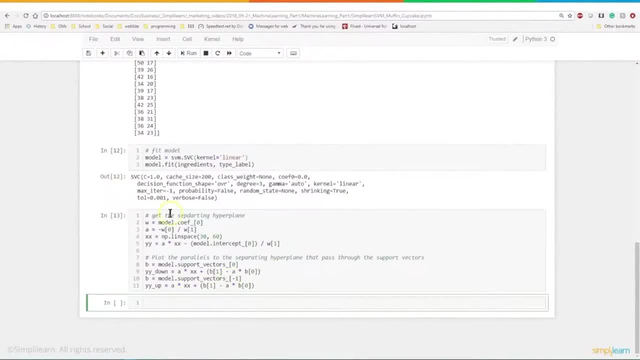 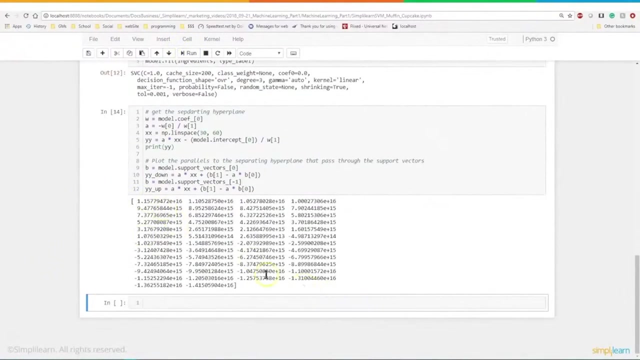 A times B0.. And we can go ahead and just run this to load these variables up. If you wanted to understand a little bit more of what's going on, you can see if we print YY. Let me just run that. You can see, it's an array. 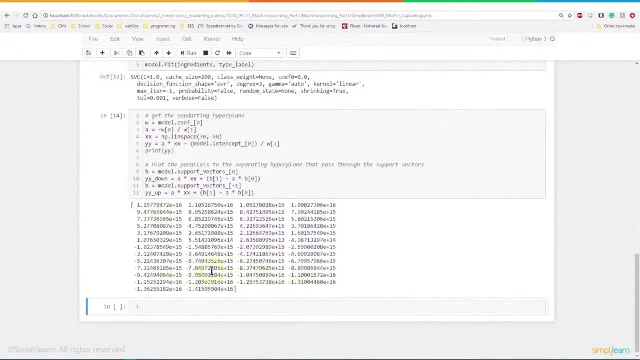 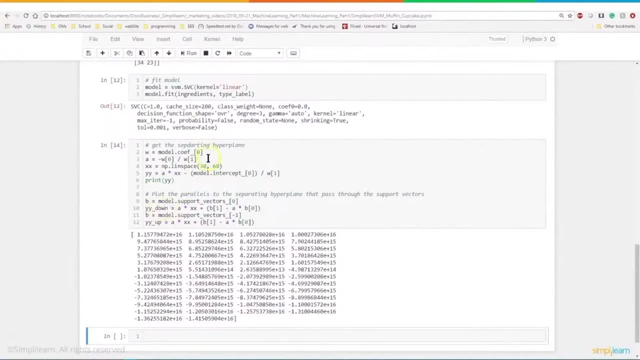 This is a line It's going to have in this case between 30 and 60.. So it's going to be 30 variables in here And the same thing with YY up, YY down, And we'll plot those in just a minute on a graph so you can see what those look like. 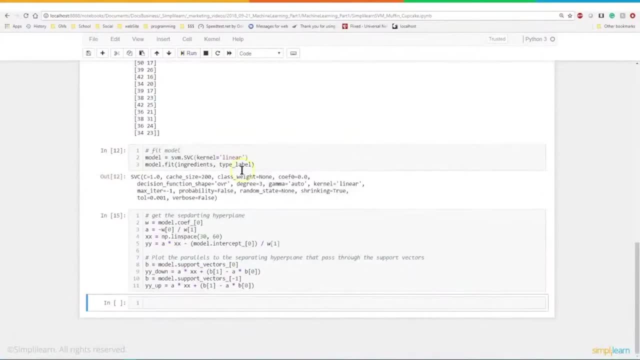 You can just go ahead and delete that out of here And run that so it loads up the variables. Nice clean slate. I'm just going to copy this from before. Remember this: our SNS, our Seaborn plot, LM plot, flour sugar. 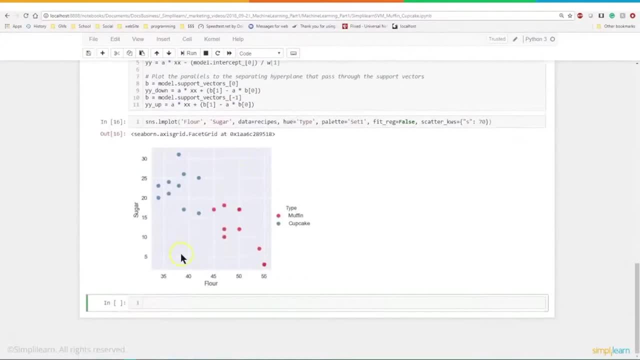 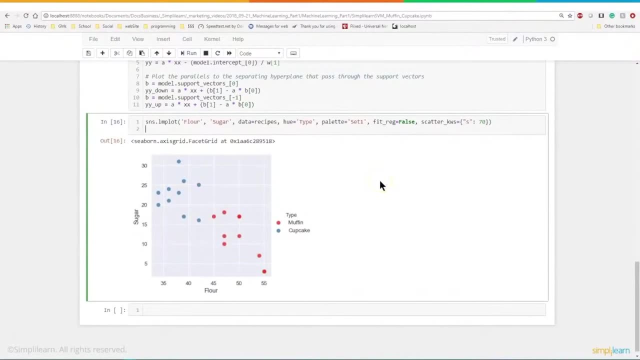 And I'll just go ahead and run that real quick so you can remember what that looks like. It's just a straight graph on there. And then one of the neat things is because Seaborn sits on top of PyPlot, we can do the PyPlot for the line going through. 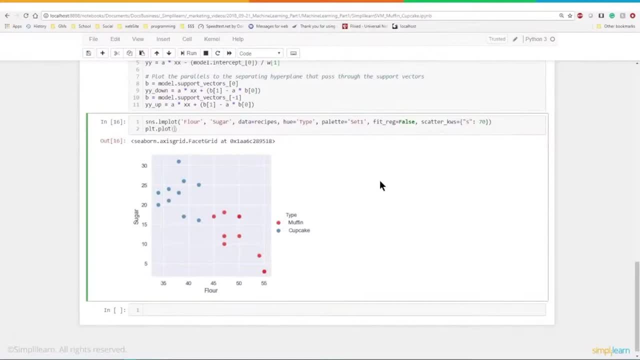 And that is simply PLTplot. And that's our XX and YY, our two corresponding values XY. And then somebody played with this to figure out that the line width equals 2 and the color black would look nice. So let's go ahead and run this whole thing with the PyPlot on there. 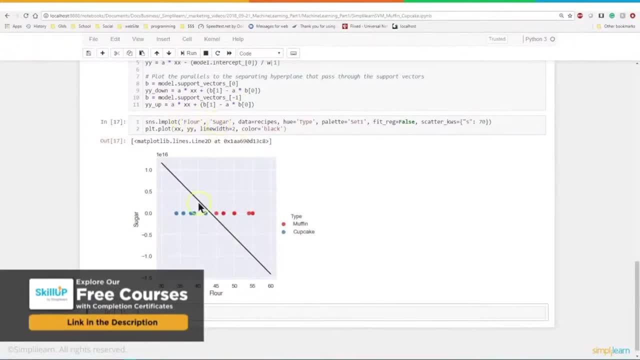 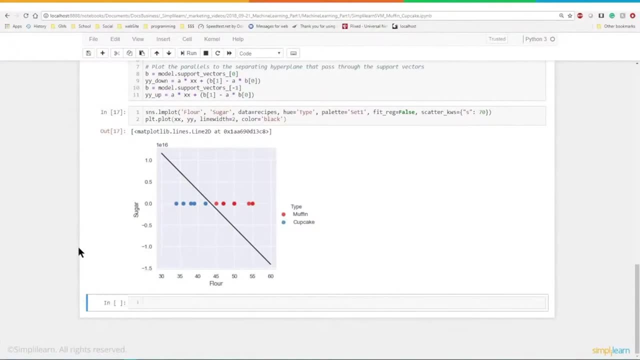 And you can see when we do this, it's just doing flour and sugar on here, Corresponding line between the sugar and the flour and the muffin versus cupcake. And then we generated the support vectors, the YY down and YY up. 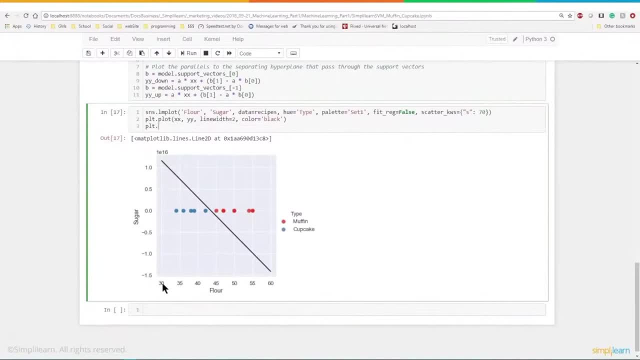 So let's take a look and see what that looks like. So we'll do our PL plot, And again, this is all against XX, our X value, But this time we have YY down And let's do something a little fun with this. 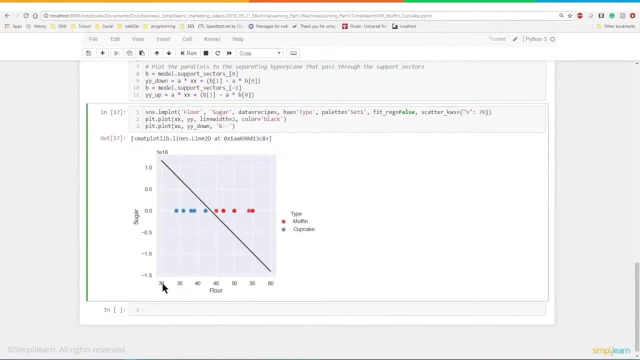 We can put in a K dash dash That just tells it to make it a dotted line. And if we're going to do the down one, we also want to do the up one. So here's our YY up, And when we run that it adds both sets of line. 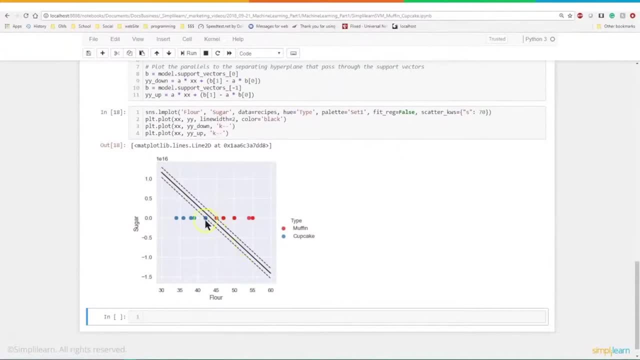 And so here's our support. And this is what you expect. You expect these two lines to go through the nearest data point, So the dash lines go through the nearest muffin And the nearest cupcake When it's plotting it, And then your SVM goes right down the middle. 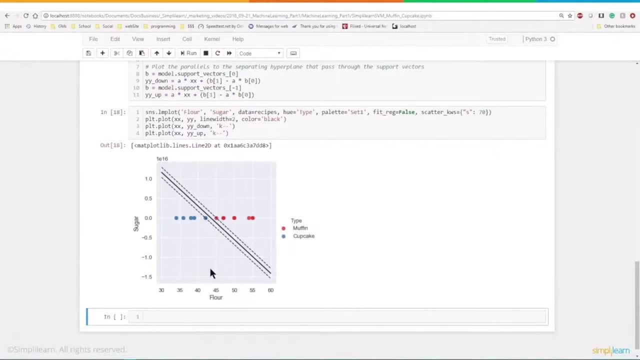 So it gives it a nice split in our data And you can see how easy it is to see, based just on sugar and flour, which one's a muffin or a cupcake. Let's go ahead and create a function to predict muffin or cupcake. 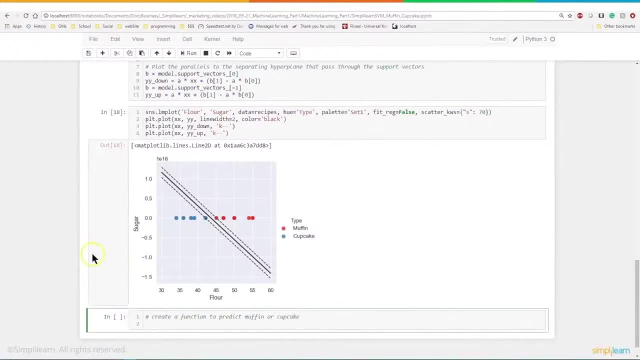 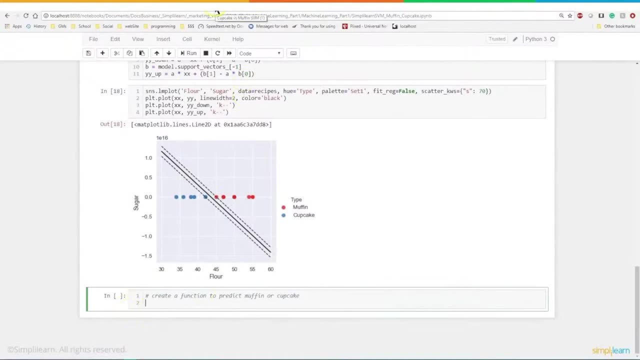 I've got my recipes, I've pulled off the internet And I want to see the difference between a muffin or a cupcake, And so we need a function to push that through And create a function with def And let's call it muffin or cupcake. 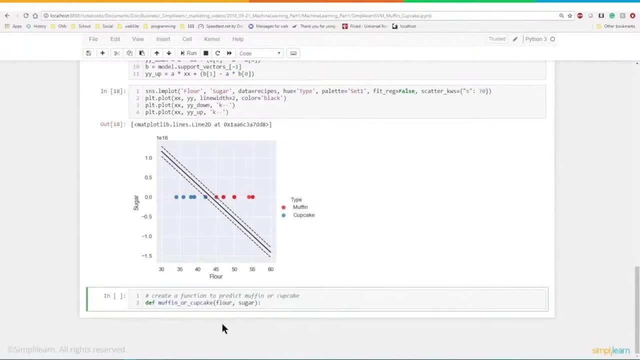 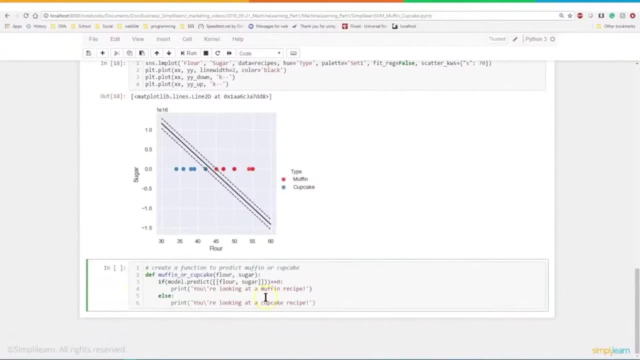 And remember, we're just doing flour and sugar today, We're not doing all the ingredients, And that actually is a pretty good split. You really don't need all the ingredients to know it's flour and sugar And let's go ahead and do an if-else statement. 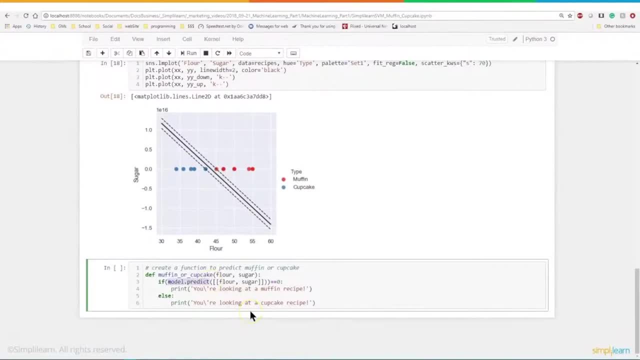 So if model predict Is of flour and sugar equals zero, So we take our model and we run a predict. It's very common in sklearn where you have a dot predict, You put the data in And it's going to return a value. 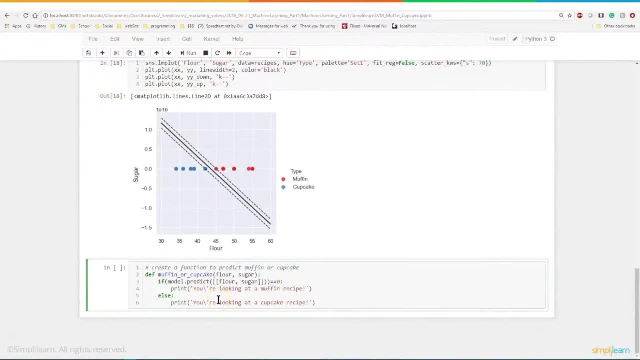 In this case. if it equals zero, then print: you're looking at a muffin recipe, Else. if it's not zero, that means it's one, Then you're looking at a cupcake recipe. That's pretty straightforward for a function. 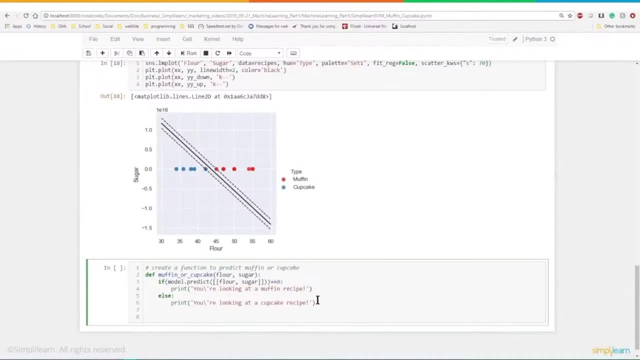 Or def for definition D-E-F is how you do that in Python And, of course, if you're going to create a function, you should run something in it, And so let's run a cupcake And we're going to send it values 50 and 20.. 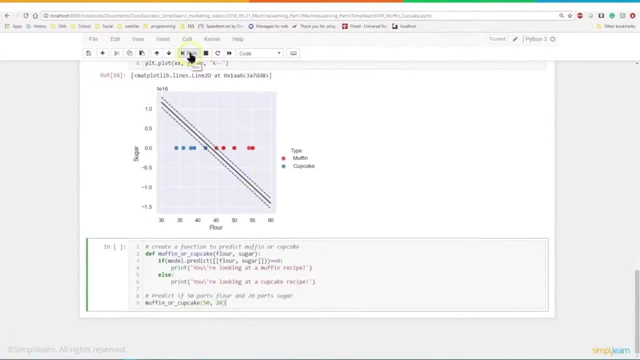 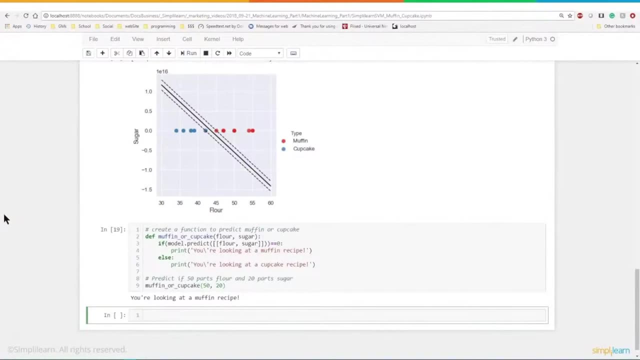 A muffin or a cupcake, I don't know what it is. And let's run this and just see what it gives us And it says: oh, it's a muffin, You're looking at a muffin recipe. So it very easily predicts whether we're looking at a muffin or a cupcake recipe. 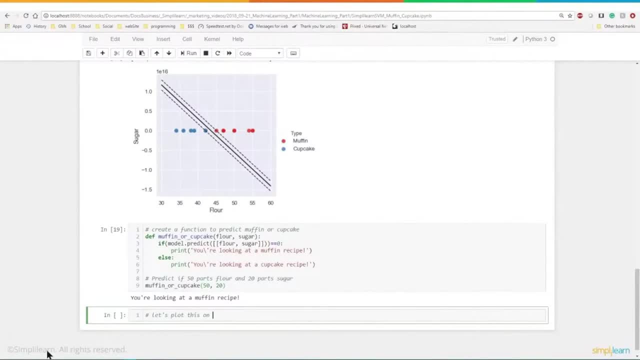 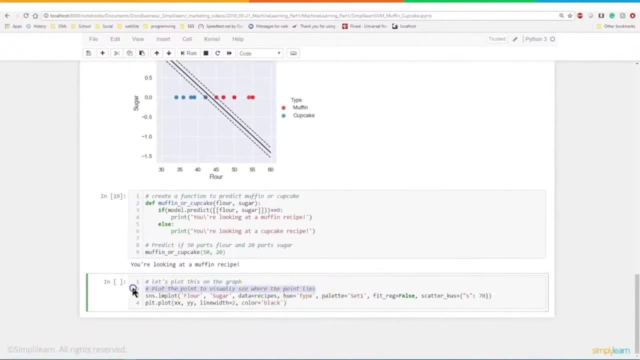 Let's plot this. There we go, Plot this on the graph, Let's see what that actually looks like, And I'm just going to copy and paste it from below. We're plotting all the points in there, So this is nothing different than what we did before. 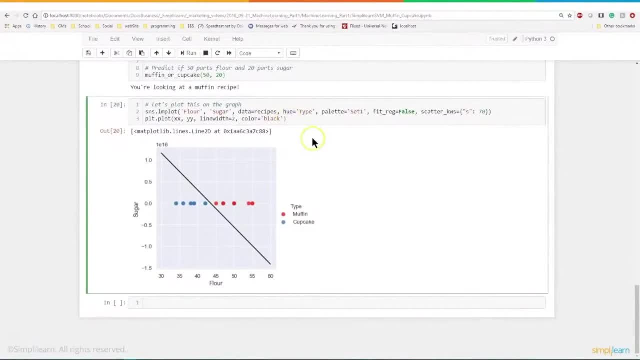 If I run it, you'll see it has all the points and the lines on there And what we want to do is we want to add another point And we'll do pltplot And if I remember correctly we did for our test, we did 50 and 20.. 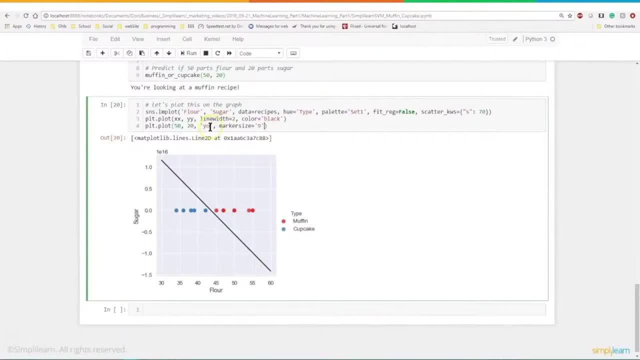 And then somebody went in here and decided we'll do a yo for yo And a yellow, or it's kind of an orangeish yellow color that's going to come up Marker size 9.. Those are settings you can play with. Somebody else played with them to come up with the right setup. so it looks good. 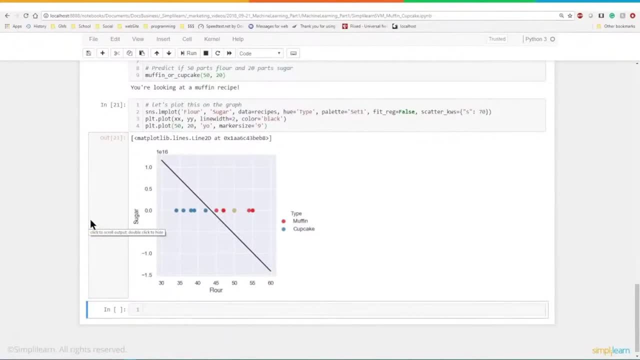 And you can see there it is graphed clearly- a muffin, In this case in cupcakes, versus muffins. the muffin has won, And if you'd like to do your own muffin cupcake contender series, you certainly can send a note down below. 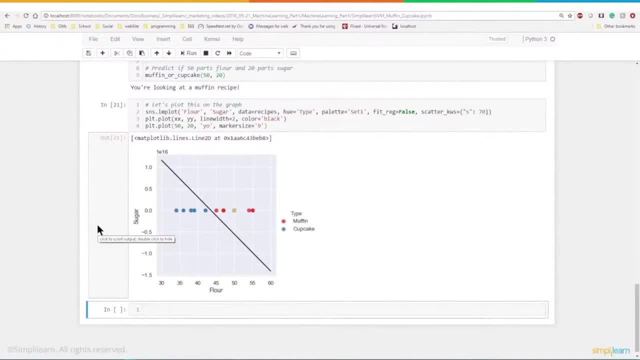 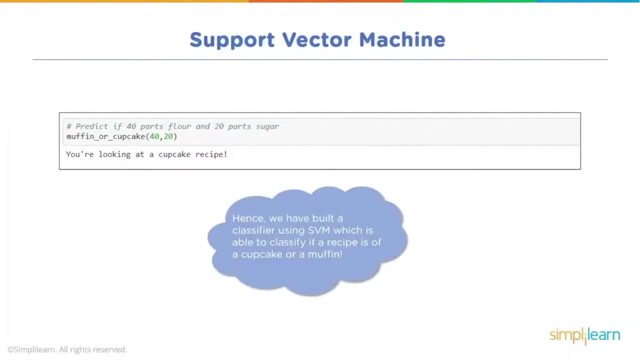 and the team at simply learn will send you over the data they use for the muffin and cupcake, and that's true of any of the data. we didn't actually run a plot on it earlier we had men versus women. you can also request that information to run it on your data setup so you can test that out. so to go back, 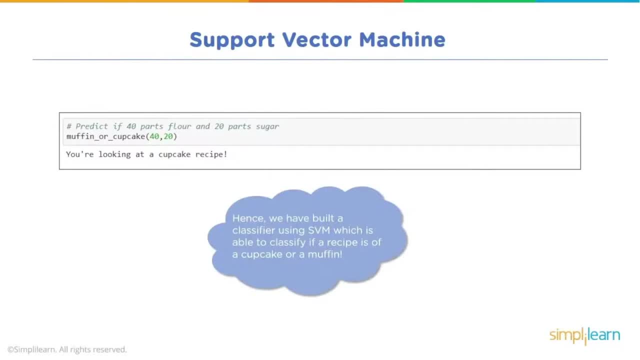 over our setup. we went ahead for our support vector machine code. we did a predict: 40 parts flour, 20 parts sugar. I think it was different than the one we did, whether it's a muffin or a cupcake. hence we have built a classifier using. 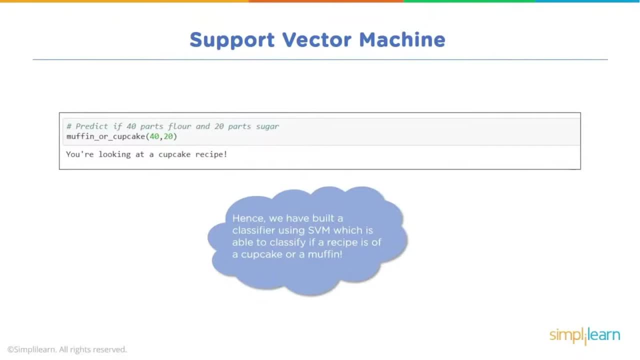 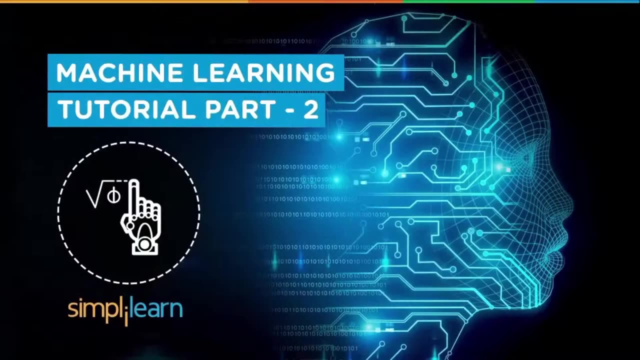 SVM, which is able to classify if a recipe is of a cupcake or a muffin, which wraps up our cupcake versus muffin. today, in our second tutorial, we're going to cover k-means and linear regression, along with going over the quiz questions we had during our first tutorial. what's in it for you? we're going to cover? 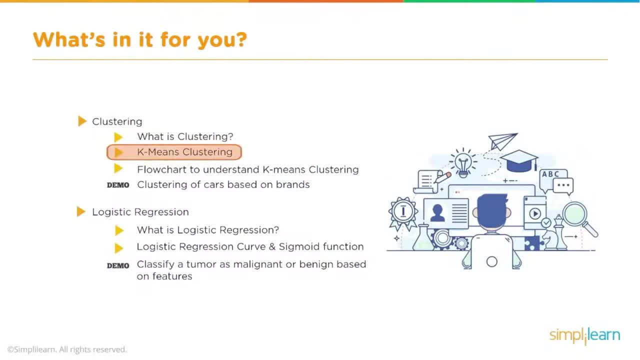 clustering. what is clustering? k-means clustering, which is what some of the most common use clustering tools out there, including a flowchart, to understand k-means clustering and how it functions, and then we'll do an actual python live demo on clustering of cars based on brands. then we're going to 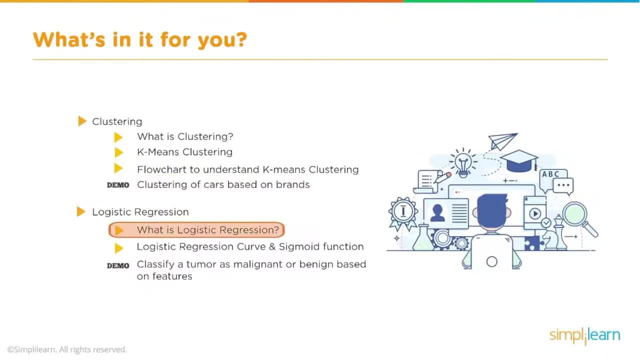 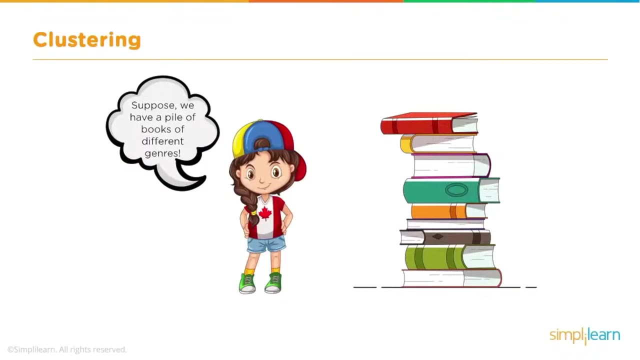 cover logistic regression. what is logistic regression? logistic regression curve and sigmoid function. and then we'll do another python code demo to classify a tumor as malignant or benign based on features. and let's start with clustering. suppose we have a pile of books of different genres. now we divide them into different groups, like fiction, horror. 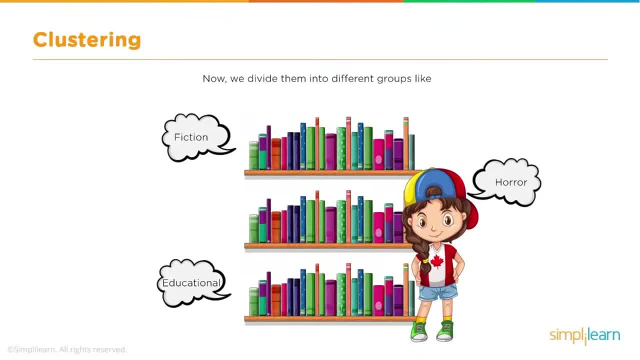 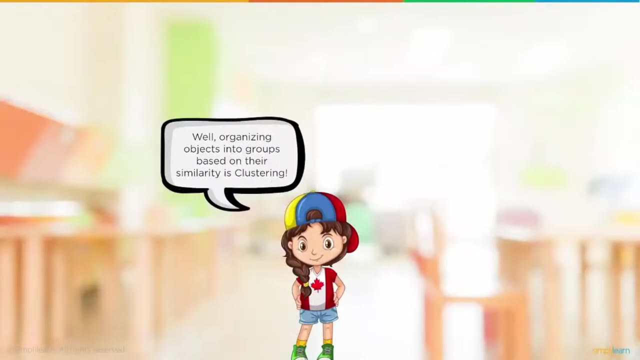 education and, as we can see from this young lady, she definitely is into heavy horror. you just tell by those eyes and the maple Canadian leaf on her shirt. but we have fiction, horror and education and we want to go ahead and divide our books up. well, organizing objects into groups based on similarity is clustering and in 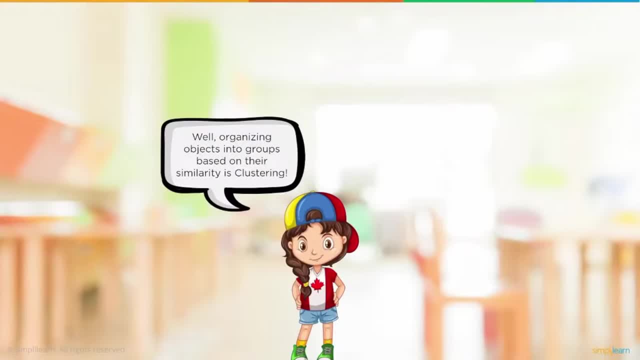 this case was. we're looking at the books, we're talking about clustering things with no one categories, but you can also use a to explore data, so you might not know the categories. you just know that you need to divide it up in some way to conquer the data and to organize it. 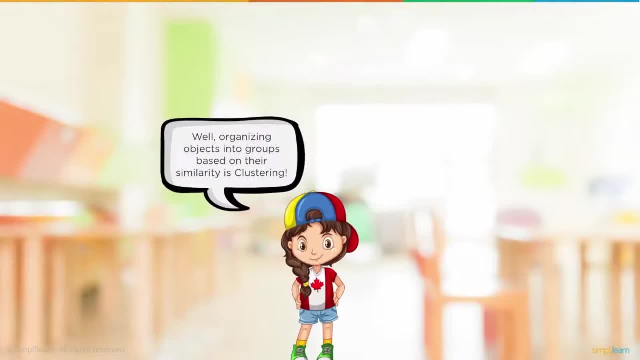 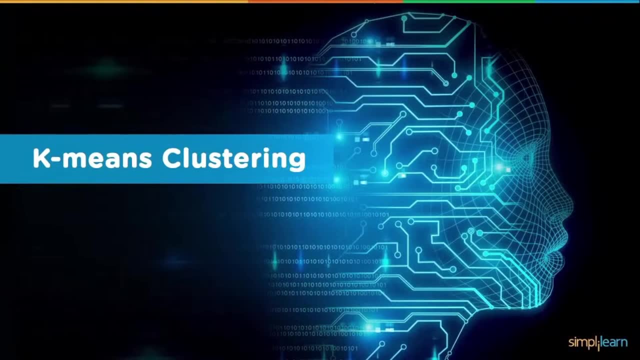 better. but in this case we're gonna be looking at clustering in specific categories and let's just take a deeper look at that. we're gonna use k-means clustering. k-means clustering is probably the most commonly used clustering tool in the machine learning library. k-means clustering is an example. 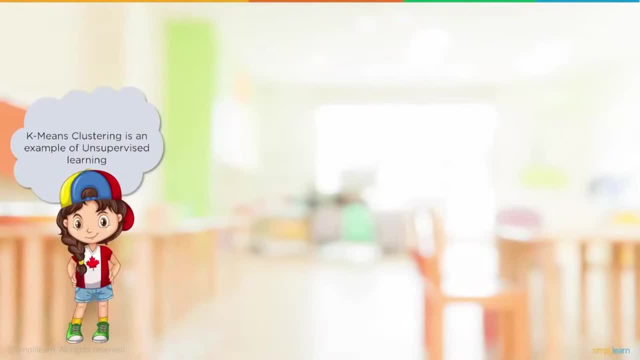 of unsupervised learning. if you remember from our previous thing, it is used when you have unlabeled data. so we don't know the answer yet. we have a bunch of data that we want to cluster. two different groups define clusters in the data based on feature. 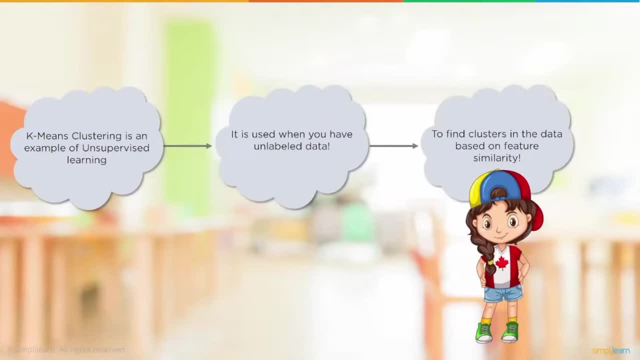 similarity. so we've introduced a couple terms here. we've already talked about unsupervised learning and unlabeled data, so we don't know the answer yet. we're just going to group stuff together and see if we can find an answer of how things connect. we've also introduced feature similarity, features being 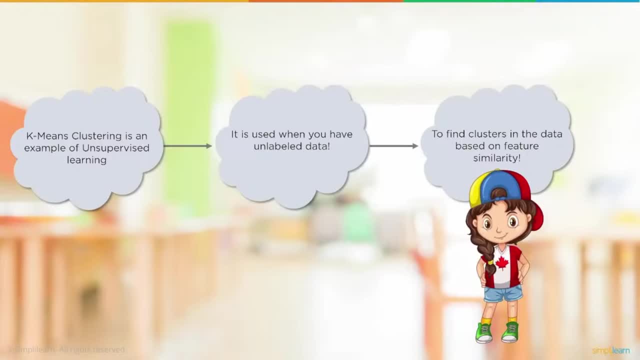 different features of the data. now with books, we can easily see fiction and horror and history books, but a lot of times with data, some of that information isn't so easy to see right when we first look at it, and so k-means is one of those. 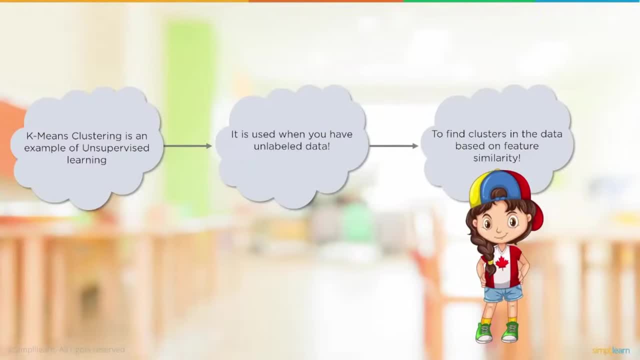 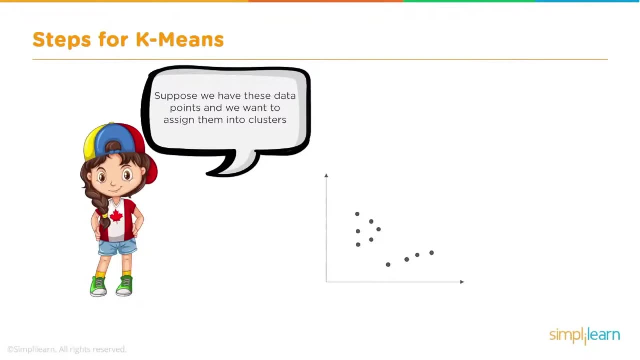 tools where we can start finding things that connect, that match, with each other. suppose we have these data points and want to assign them into a cluster. now when I look at these data points I would probably group them into two clusters. just by looking at them I'd say two of these group of data kind of come. 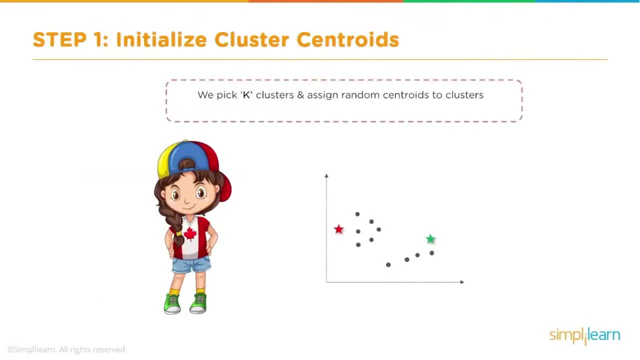 together, but in k-means. we pick k clusters and assign random centroid to clusters. where the k clusters represents two different clusters, we pick k clusters and assign random centroid to the clusters. then we compute distance from objects to the centroids. now we form new clusters based on. 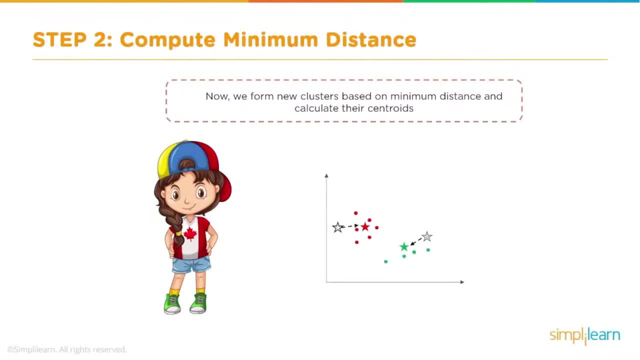 minimum distances and calculate the centroids. so we figure out what the best distance is for the centroid. then we move the centroid and recalculate those distances. repeat previous two steps iteratively till the cluster centroid. stop changing their positions and become static. repeat previous two steps iteratively till the cluster centroid- stop changing. 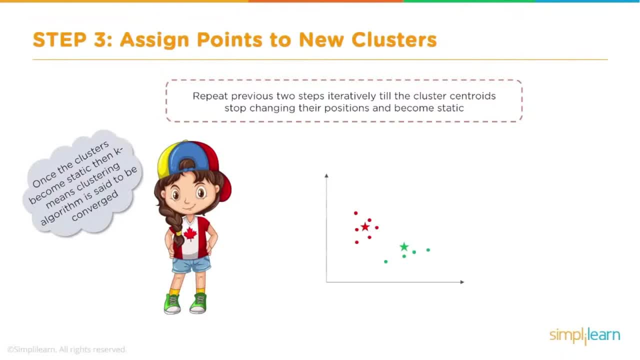 and the positions become static. once the clusters become static, then k-means clustering algorithm is said to be converged, and there's another term we see throughout machine learning is converged. that means whatever math we're using to figure out the answer has come to a solution or it's converged on an. 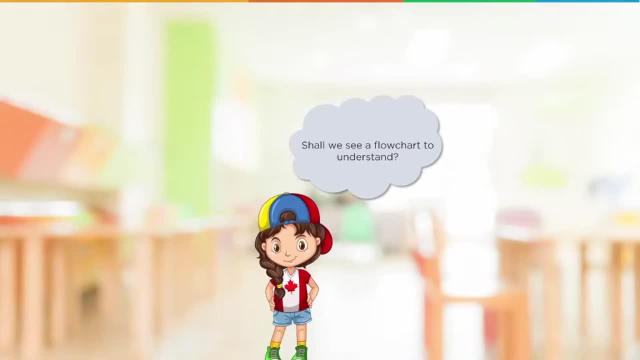 answer. shall we see the flowchart to understand, make a little bit more sense by putting it into a nice easy step-by-step. so we start, we choose k. we'll look at the flowchart and we're going to look at the flowchart and we're going to look at the 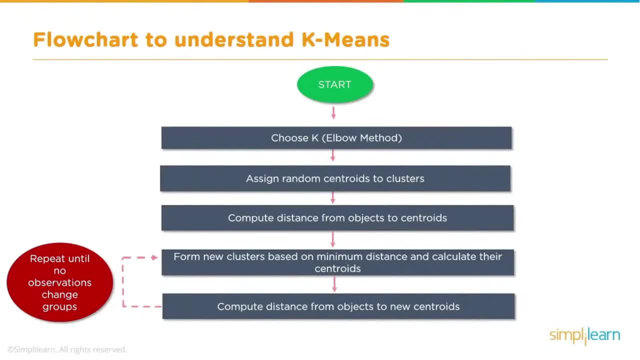 elbow method in just a moment. we assign random centroids, two clusters, and sometimes you pick the centroids because you might look at the data in a graph and say these are probably the central points. then we compute the distance from the objects to the centroids, we take that and we form new clusters based on. 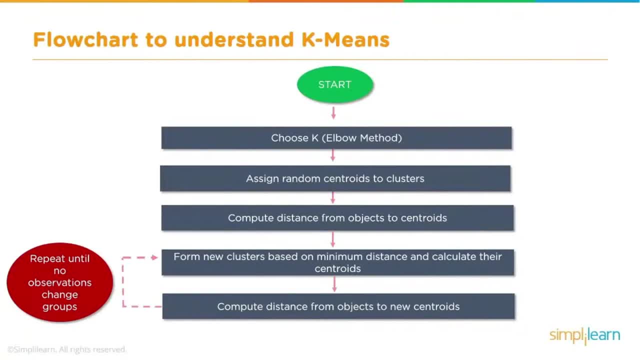 minimum distance and calculate their centroids. then we compute the distance from objects to the new centroids and then we go back and repeat those last two steps. we calculate the distances so as we're As we're doing it, it brings into the new centroid and then we move the centroid around and we figure out what the best, which objects are closest to each centroid. 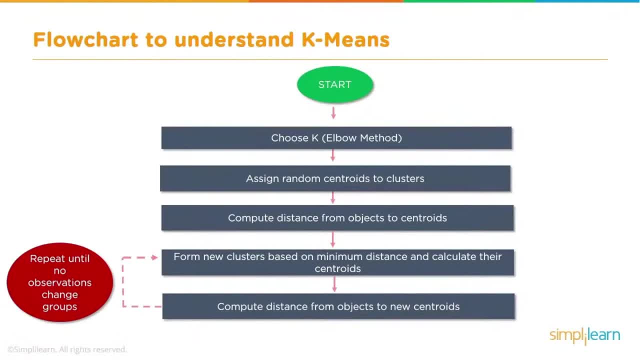 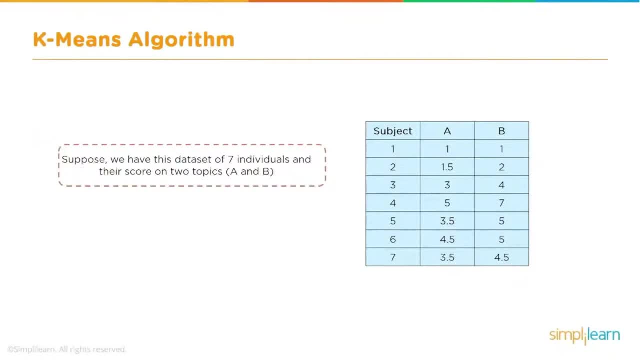 So the objects can switch from one centroid to the other as the centroids are moved around, And we continue that until it is converged. Let's see an example of this. Suppose we have this data set of seven individuals and their score on two topics, A and B. 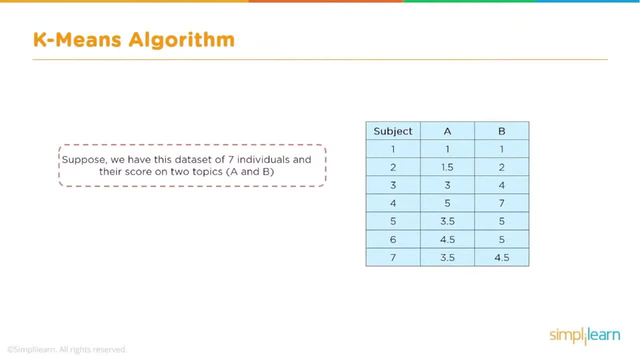 So here's our subject, in this case referring to the person taking the test, And then we have subject A, where we see what they've scored on their first subject, and we have subject B, and we can see what they score on the second subject. 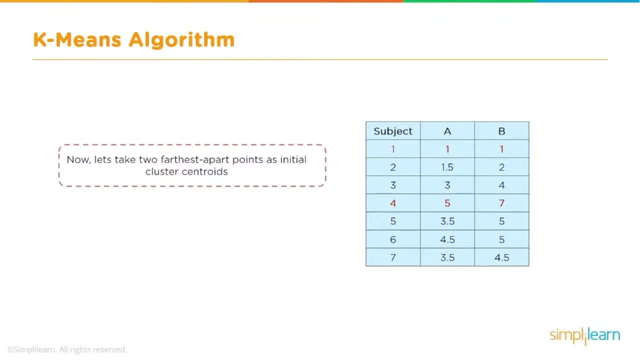 Now let's take two farthest apart points as initial cluster centroids. Now remember we talked about selecting them randomly, or we can also just put them in different points and pick the furthest one apart so they move together. Either one works okay, depending on what kind of data you're working on and what you know about it. 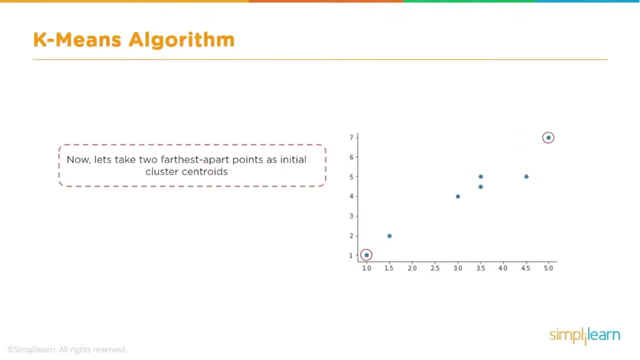 So we took the two furthest, points, 1 and 1, and 5 and 7.. And now let's take the two farthest apart points as initial cluster centroids. Each point is then assigned to the closest cluster with respect to the distance from the centroids. 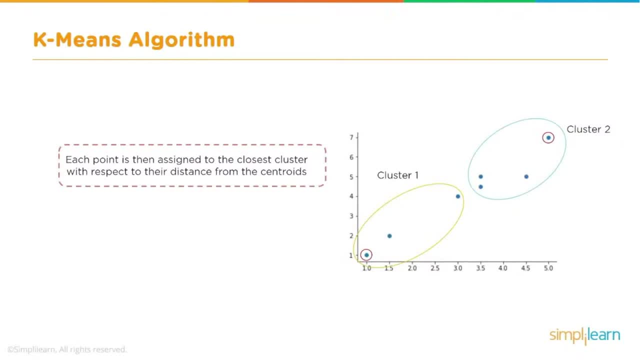 So we take each one of these points in there, we measure that distance and you can see that if we measure each of those distances and you use the Pythagorean theorem for a triangle in this case, because you know the x and the y and you can figure out the diagonal line from that, 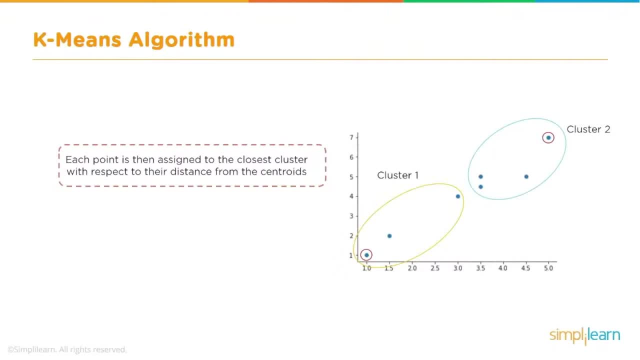 Or you can just take a ruler and put it on your monitor. That'd be kind of silly, but it would work. if you're just eyeballing it, You can see how they naturally come together in certain areas. Now we again calculate the centroids of each cluster. 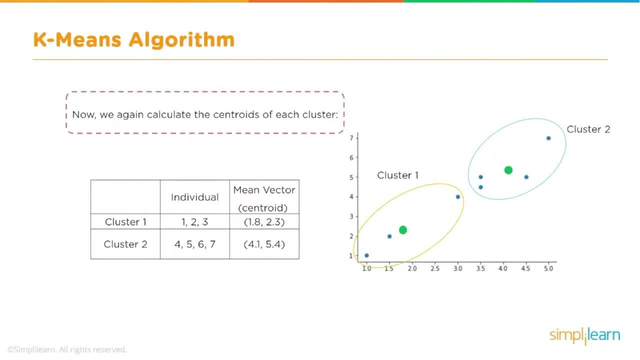 So cluster 1, and then cluster 2, and we look at each individual dot. There's 1,, 2,, 3, we're in one cluster. The centroid then moves over. It becomes 1.8 comma 2.3.. 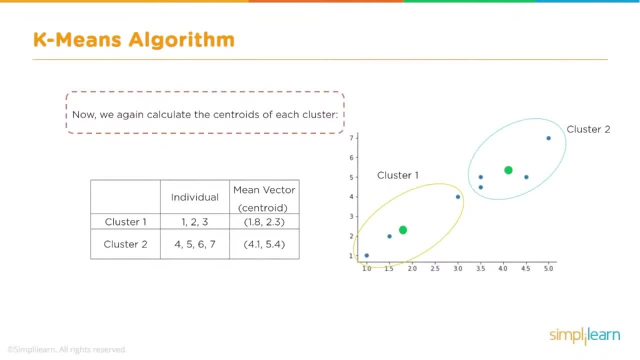 So remember it was at 1 and 1? Well, the very center of the data we're looking at would put it at the 1 point roughly 2, 2, but 1.8 and 2.3.. And the second one, if we wanted to make the overall mean vector. 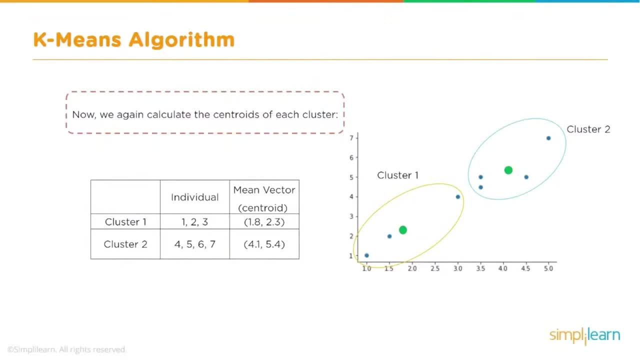 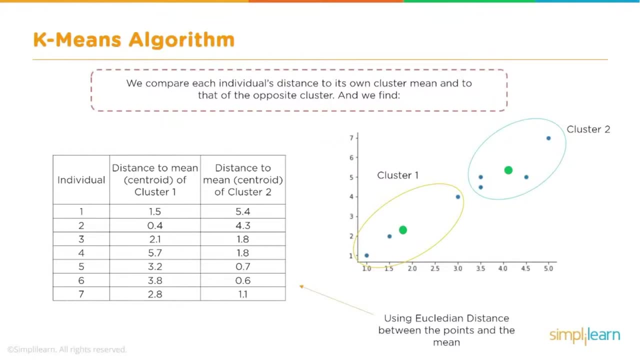 the average vector of all the different distances to that centroid, we come up with 4 comma 1 and 5, 4.. So we've now moved the centroids. We compare each individual's distance to its own cluster mean and to that of the opposite cluster. 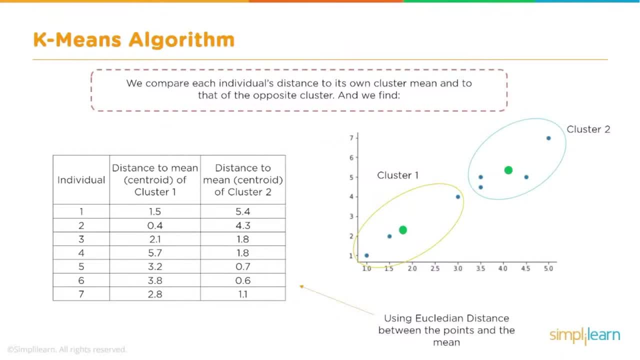 And we find we can build a nice chart on here- that as we move that centroid around, we now have a new, different kind of clustering of groups And using Euclidean distance between the points and the mean, we get the same formula. you see new formulas coming up. 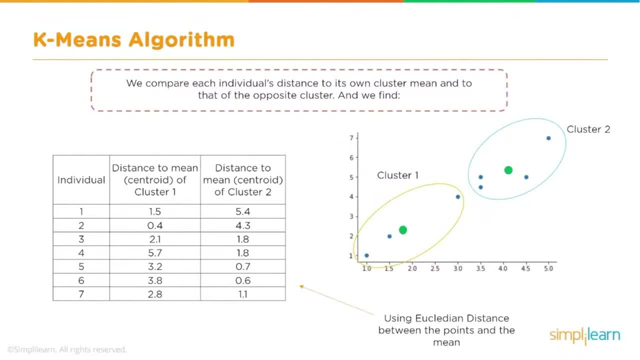 So we have our individual dots: distance to the mean centroid to the mean distance to the mean centroid of the cluster and distance to the mean centroid of the cluster. Only individual 3 is nearer to the mean of the opposite cluster. 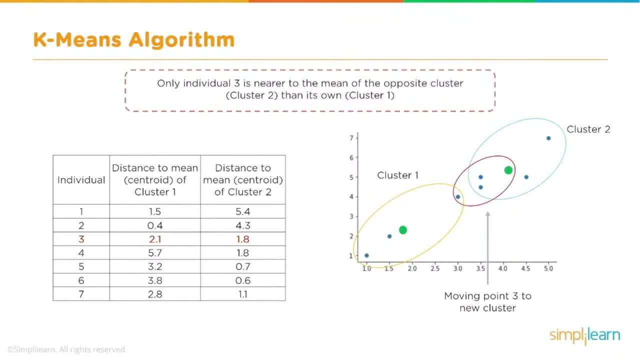 cluster 2, than its own cluster 1.. And you can see here in the diagram we've kind of circled that one in the middle. So when we've moved the centroid of the clusters over one of the points shifted to the other cluster. 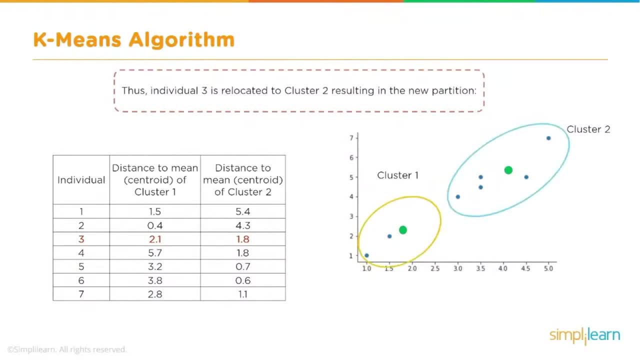 because it's closer to that group of individuals. Thus, individual 3 is relocated to cluster 2, resulting in a new partition, And we regenerate all those numbers of how close they are to the different clusters. For the new clusters we will find the actual cluster centroids. 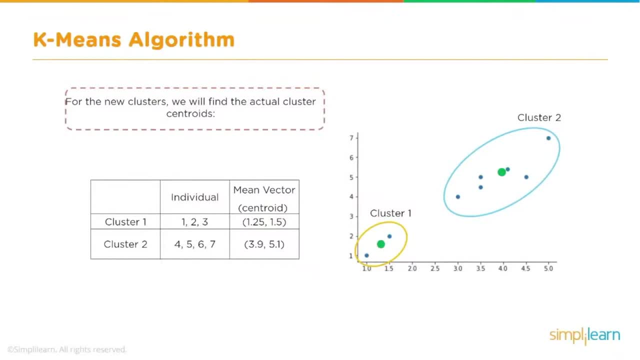 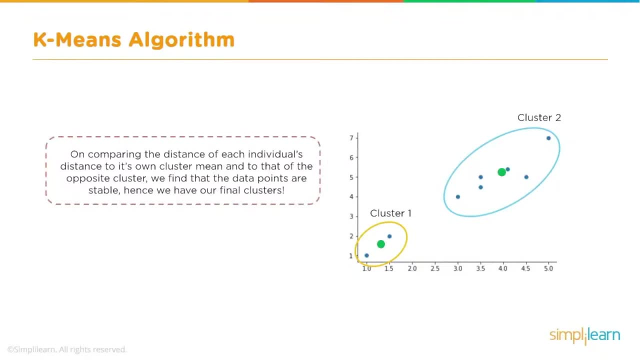 So now we move the centroids over and you can see that we've now formed two very distinct clusters on here. On comparing the distance of each individual's distance to its own cluster mean and to that of the opposite cluster, we find that the data points are stable. 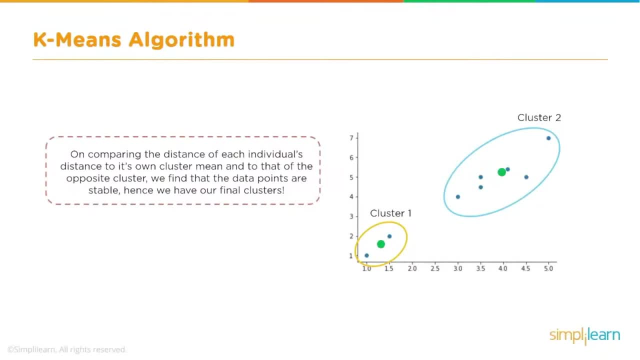 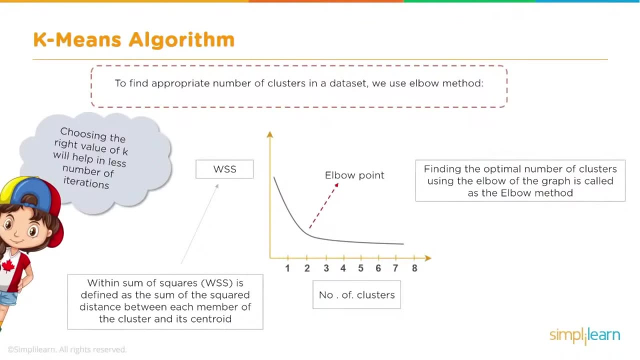 Hence we have our final clusters Now. if you remember, I brought up a concept earlier on the k-means algorithm. Choosing the right value of k will help in less number of iterations And to find the appropriate number of clusters in a data set. 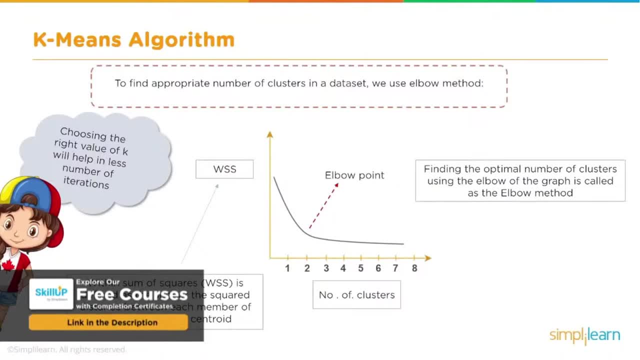 we use the ELBO method And within sum of squares. WSS is defined as the sum of the squared distance between each member of the cluster in its centroid, And so you see what we've done here is we have the number of clusters. 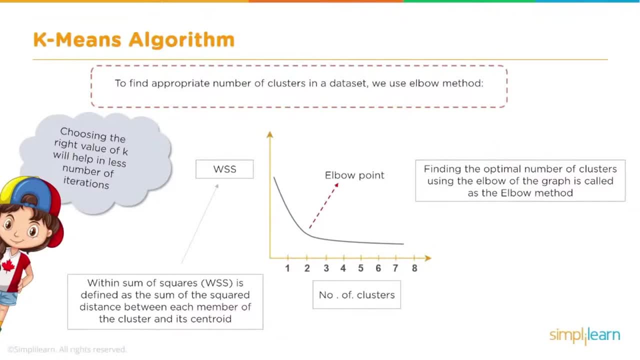 And as you do the same k-means algorithm over the different clusters and you calculate what that centroid looks like and you find the optimal. you can actually find the optimal number of clusters using the ELBO. the graph is called as the ELBO method. 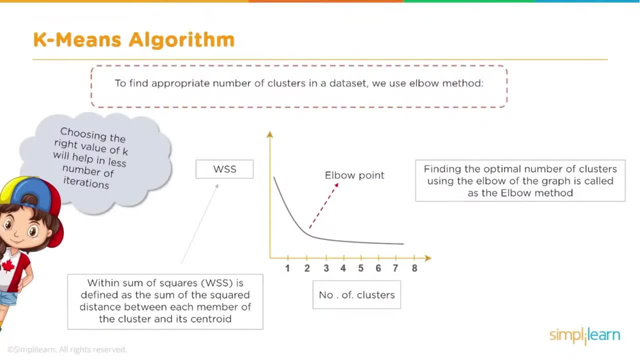 And in this we guessed at 2 just by looking at the data. But as you can see the slope, you actually just look for right there where the ELBO is in the slope and you have a clear answer that we want 2 different. 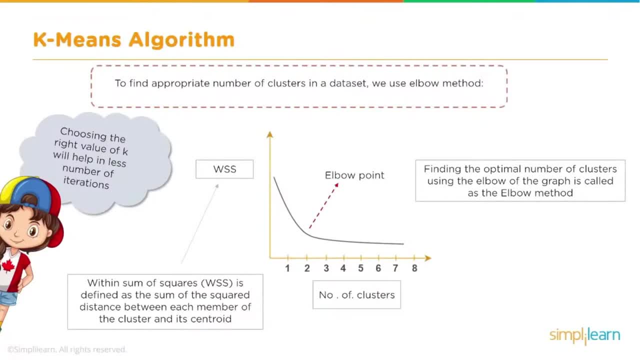 to start with, k-means equals 2.. A lot of times people end up computing k-means equals 2,, 3,, 4,, 5, until they find the value which fits on the ELBO joint. Sometimes you can just look at the data. 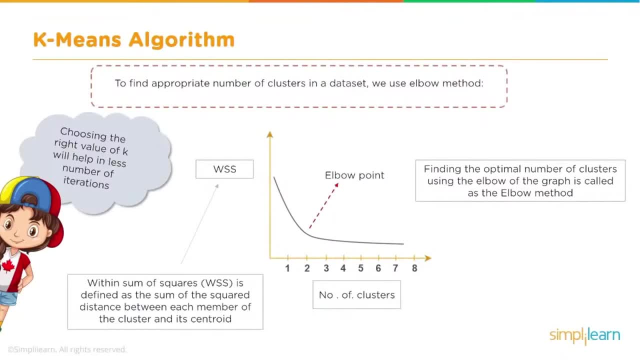 and if you're really good with that specific domain- remember domain I mentioned that last time- you'll know where to pick those numbers and where to start guessing at what that k-value is. So let's take this and we're going to use a use case. 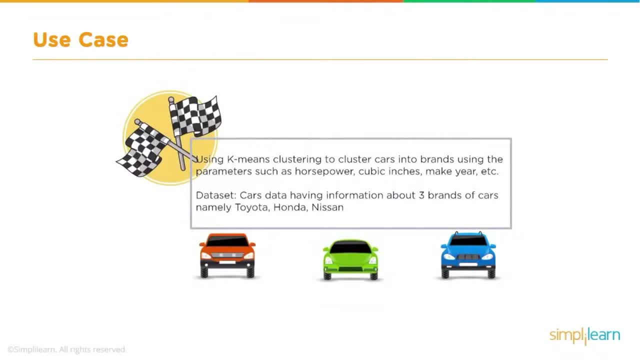 using k-means clustering to cluster cars into brands using parameters such as horsepower, cubic inches, make year, etc. So we're going to use the dataset cars data, having information about 3 brands of cars: Toyota, Honda and Nissan. 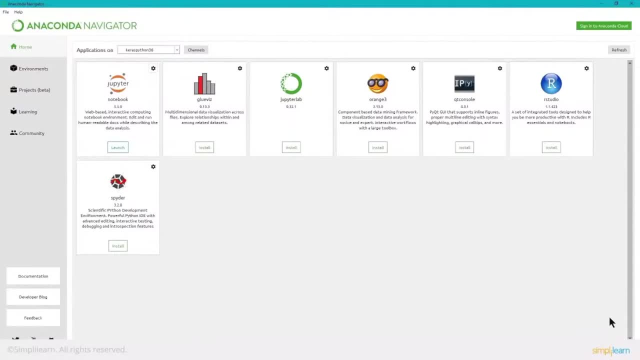 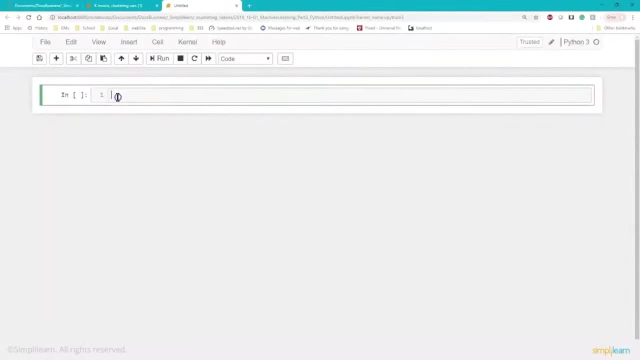 We'll go back to my favorite tool, the Anaconda Navigator, with the Jupyter Notebook, and let's go ahead and flip over to our Jupyter Notebook, And in our Jupyter Notebook, I'm going to go ahead and just paste the basic code. 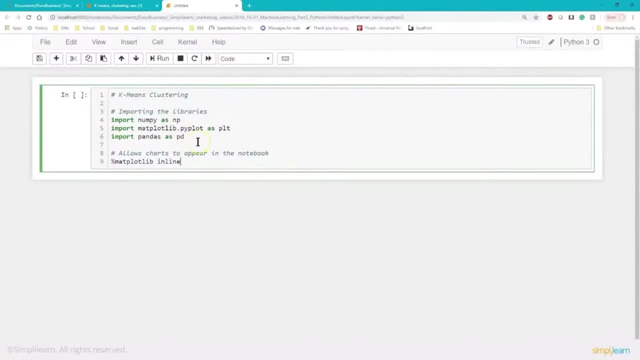 that we usually start a lot of these off with. We're not going to go too much into this code, because we've already discussed numpy. we've already discussed matplotlibrary and pandas, numpy being the number array, pandas being the pandas data frame. 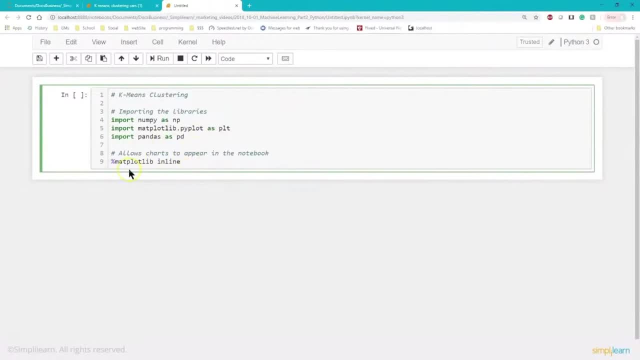 and matplot for the graphing. And don't forget, since if you're using the Jupyter Notebook, you do need the matplotlibrary inline so that it plots everything on the screen. If you're using a different Python editor, then you probably don't need that. 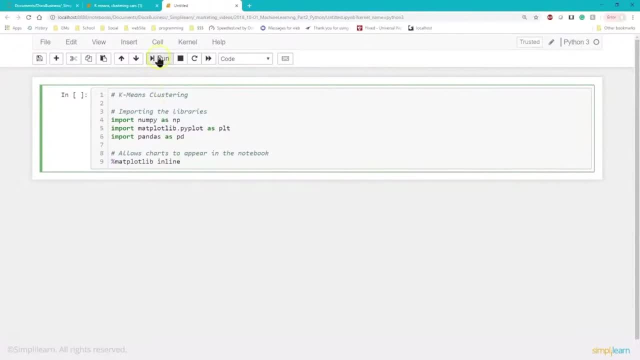 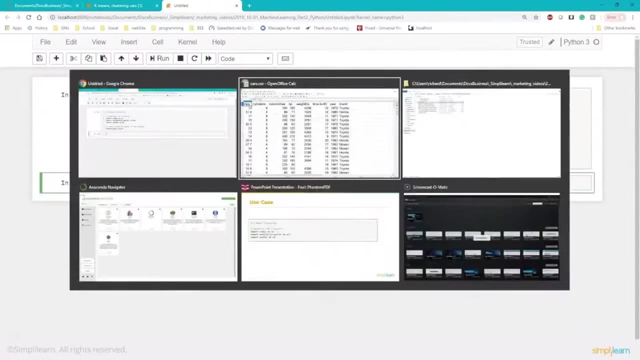 because it'll have a pop-up window on your computer And we'll go ahead and run this just to load our libraries and our setup into here. The next step is, of course, to look at our data, which I've already opened up in a spreadsheet. 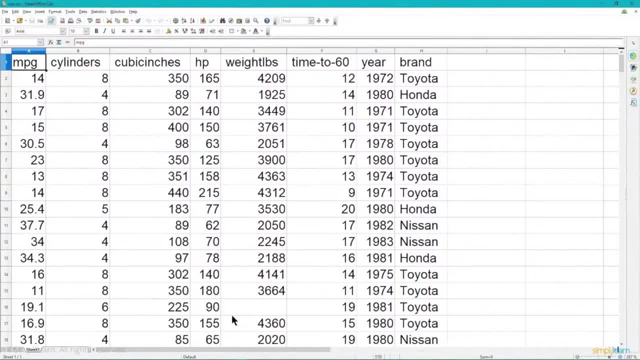 And you can see here we have the miles per gallon, cylinders, cubic inches, horsepower, weight, pounds, how heavy it is time it takes to get to 60, my car is probably on this one at about 80 or 90,. 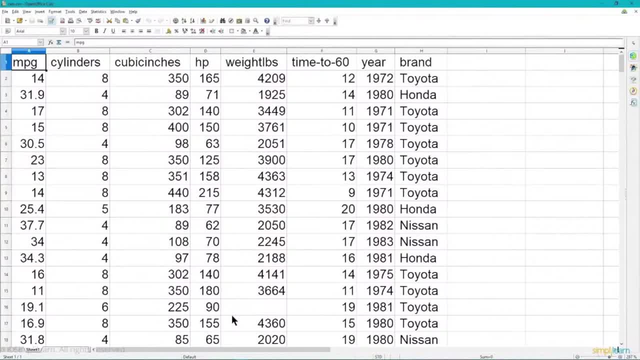 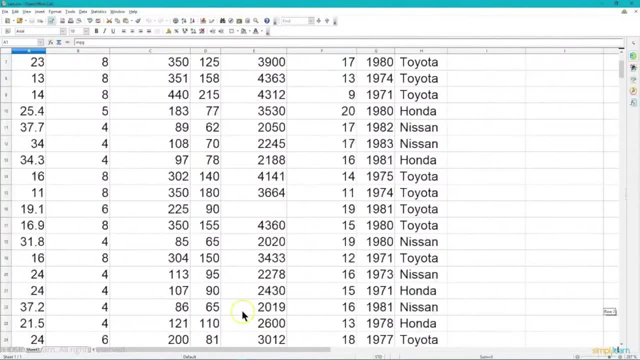 what year it is. so you can actually see this is kind of older cars. and then the brand Toyota, Honda, Nissan. so the different cars are coming from all the way from 1971, if we scroll down to the 80s. 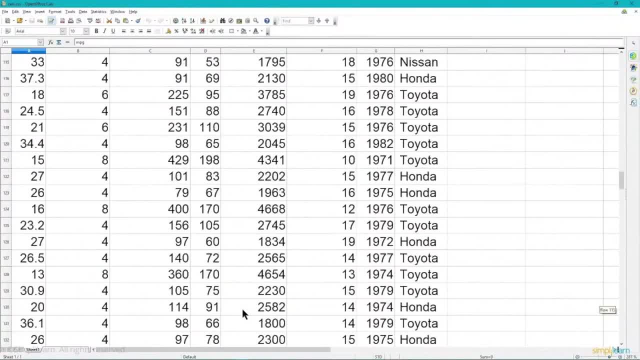 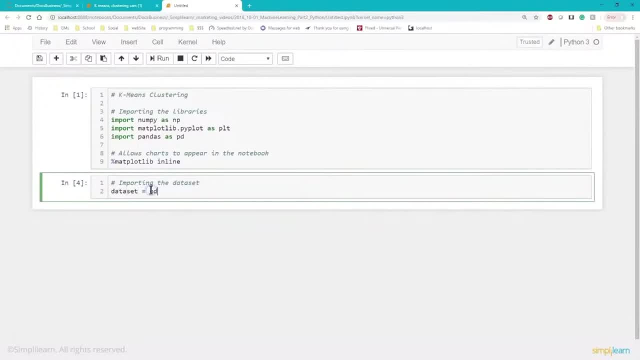 so we have between the 70s and 80s, the number of cars that they've put out, And when we come back here we're going to do importing the data. so we'll go ahead and do dataset equals and we'll use pandas to read this in. 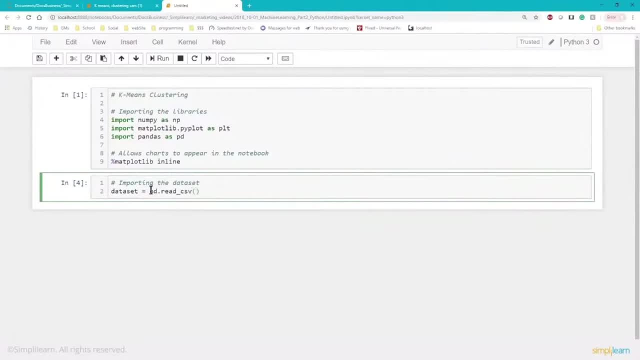 and it's from a CSV file. remember, you can always post this in the comments and request the data files for these, either in the comments here on the YouTube video or go to simplylearncom and request that. The cars CSV. I put it in the same folder as the code that I've stored. 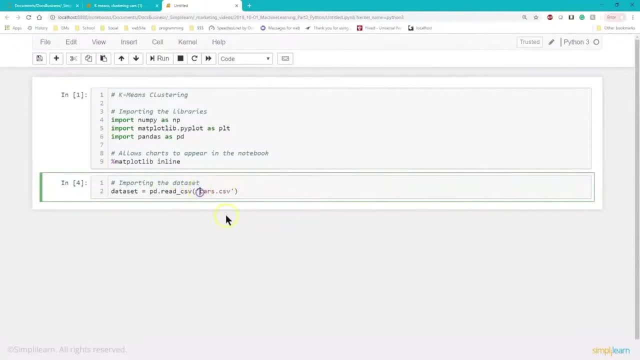 so my Python code is stored in the same folder, so I don't have to put the full path. If you store them in different folders, you do have to change this and double check your name variables And we'll go ahead and run this. 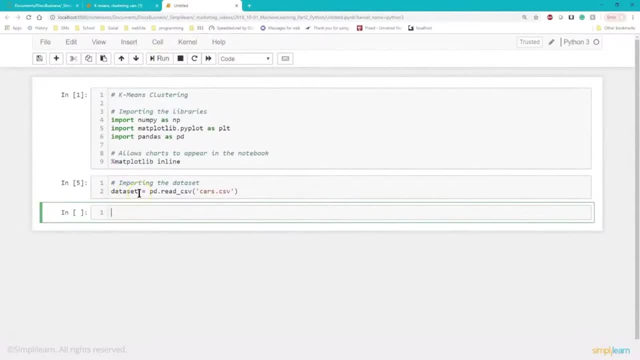 and we've chosen dataset arbitrarily because it's a dataset we're importing, and we've now imported our cars CSV into the dataset. As you know, you have to prep the data, so we're going to create the x data. This is the one that we're going to try to figure out. 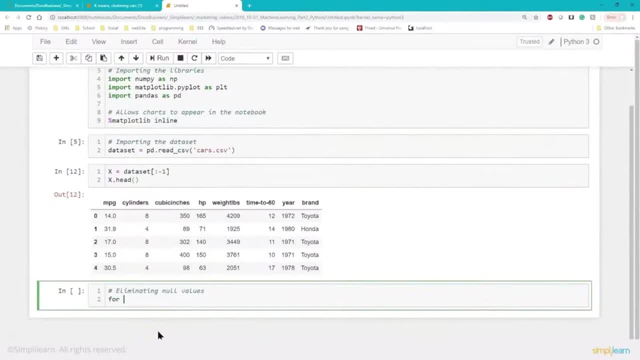 what's going on with. And then there's a number of ways to do this, but we'll do it in a simple loop so you can actually see what's going on. So we'll do for i in xcolumns. So we're going to go through each of the columns. 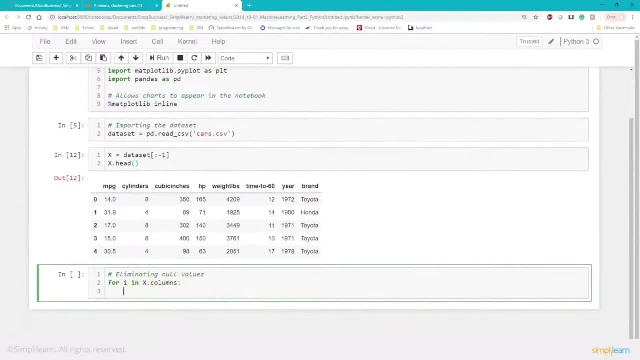 and a lot of times it's important. I'll make lists of the columns and do this because I might remove certain columns or there might be columns that I want to be processed differently, But for this we can go ahead and take x of i. 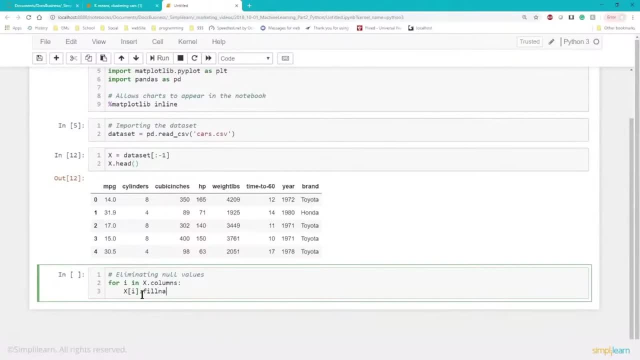 and we want to go fill in a and that's a pandas command. But the question is: what are we going to fill the missing data with? We definitely don't want to just put in a number that doesn't actually mean something, And so one of the tricks you can do with this- 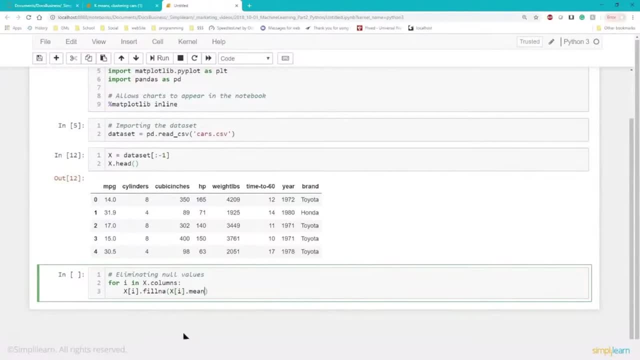 is, we can take x of i and in addition to that we want to go ahead and turn this into an integer, because a lot of these are integers. So we'll go ahead and keep it integers And we add the bracket here. 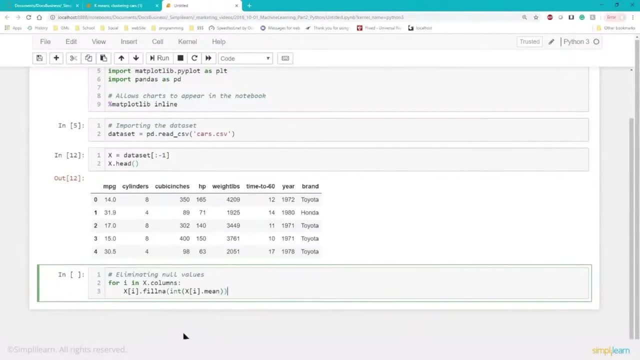 and a lot of editors will do this. they'll think that you're closing one bracket. Make sure you get that second bracket in there. if it's a double bracket, That's always something that happens regularly. So once we have our integer of x of i, 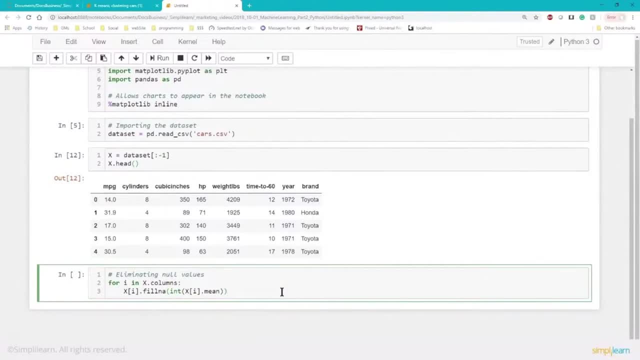 this is going to fill in any missing data with the average, And I was so busy closing one set of brackets I forgot that the mean also has brackets in there for the pandas. So we can see here we're going to fill in all the data with the average value. 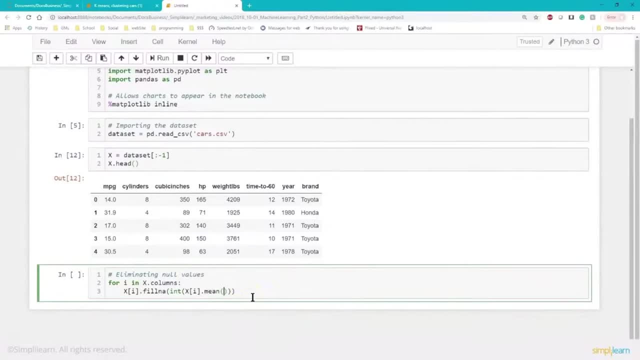 for that column. so if there's missing data it's in the average of the data it does have, And then, once we've done that, we'll go ahead and loop through it again and just check and see to make sure everything is filled in correctly. 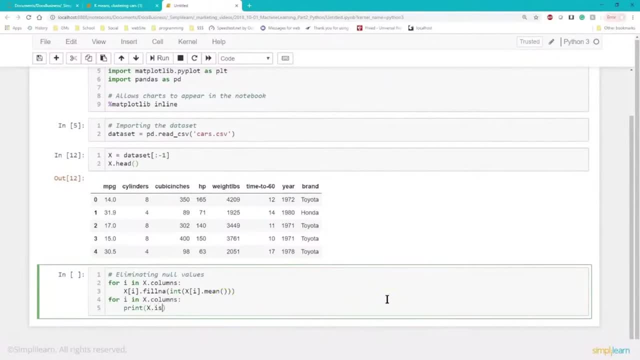 And we'll print. and then we take x is null and this returns a set of the null value, or how many lines are null, and we'll just sum that up to see what that looks like. And so when I run this, 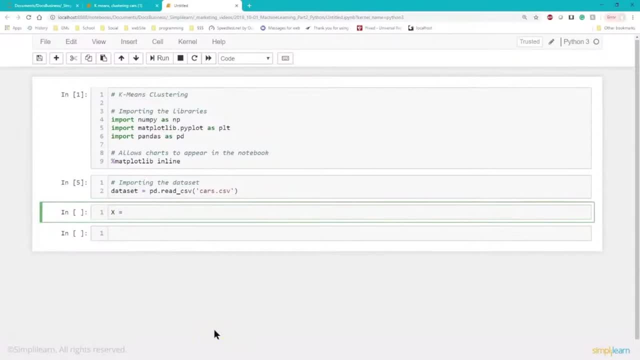 and so, with the x, what we want to do is we want to remove the last column, because that's where that had the models. That's what we're trying to see: if we can cluster these things and figure out the models. There is so many different ways. 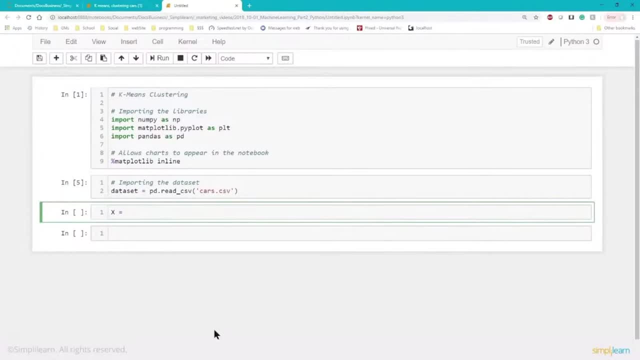 to sort the x out For one. we could take the x and we could go data set our variable. we're using and use the ilocation, one of the features that's in pandas, And we could take that and then take all the rows. 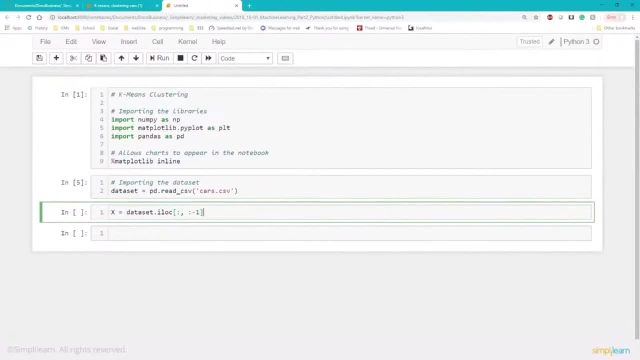 and all but the last column of the data set, And at this time we could do values. We just convert it to values. So that's one way to do this, And if I let me just put this down here and print x: 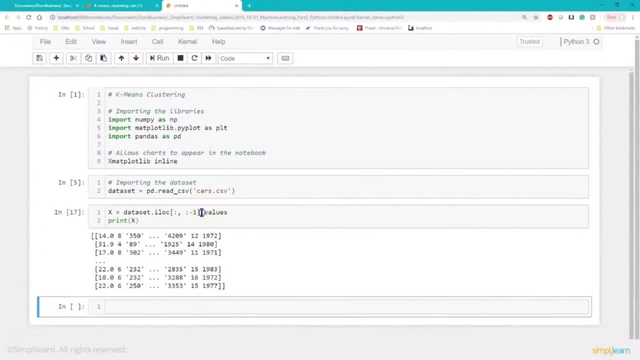 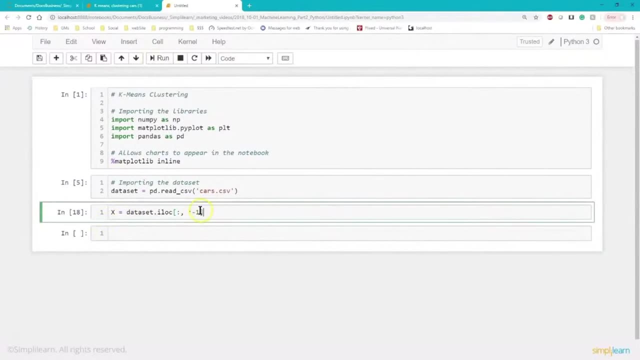 It's a capital X we chose And I run this. you can see it's just the values. We could also take out the values and it's not going to return anything because there's no values connected to it. What I like to do with this: 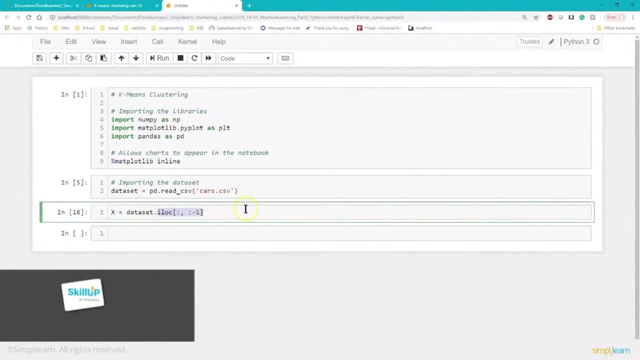 is, instead of doing the ilocation which does integers, more common is to come in here and we have our data set and we're going to do data set dot, data set dot- columns. And remember that lists all the columns. So if I come in here, 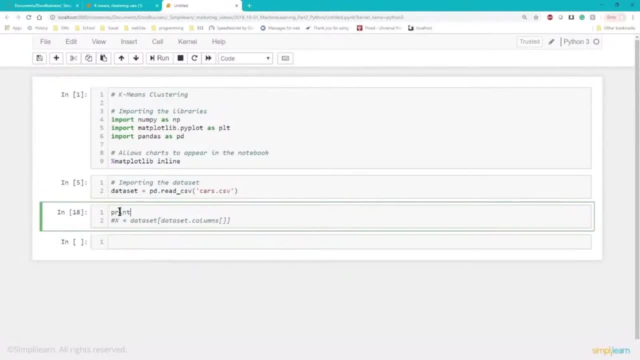 let me just mark that as red and I print data set dot columns. You can see that I have my index here. I have my mpg cylinders, everything including the brand, which we don't want. So the way to get rid of the brand. 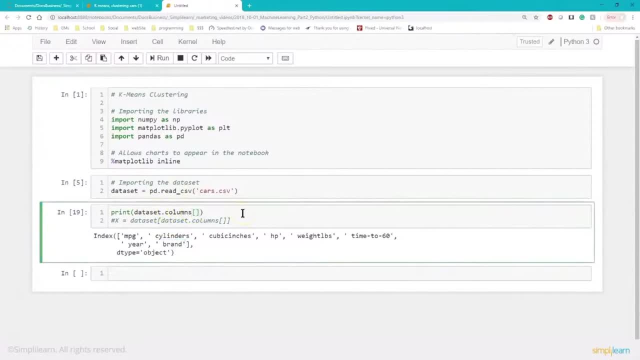 would be to do data columns of everything but the last one minus one. So now, if I print this, you'll see the brand disappears, And so I can actually just take data set columns minus one and I'll put it right in here. 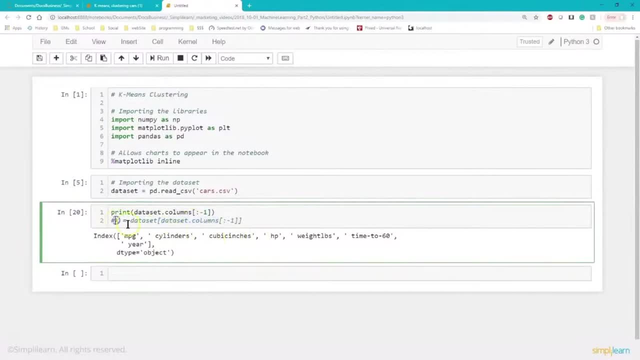 for the columns we're going to look at, And let's unmark this and unmark this, And now, if I do an x dot head, I now have a new data frame and you can see right here we have all the different columns. 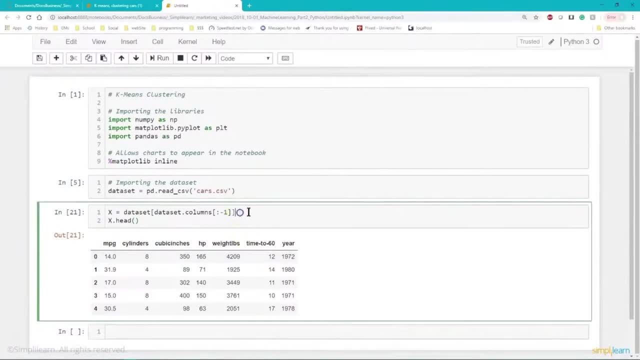 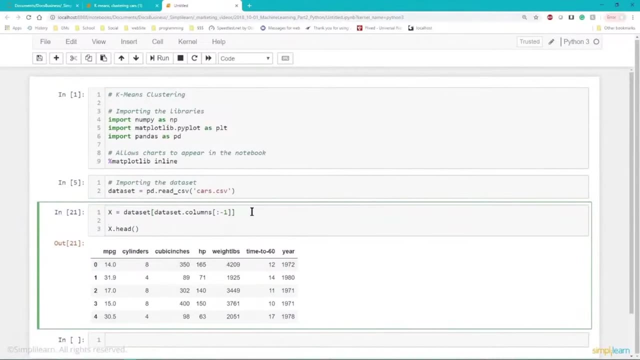 except for the brand- at the end of the year. And it turns out when you start playing with the data set, you're going to get an error later on and it'll say: cannot convert string to float value. And that's because. 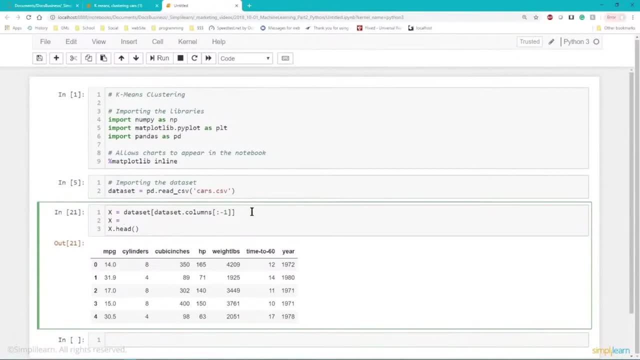 for some reason, these things, the way they recorded them, must have been recorded as strings. So we have a neat feature in here on pandas to convert, And it is simply convert objects, And for this we're going to do convert, oops, convert underscore. 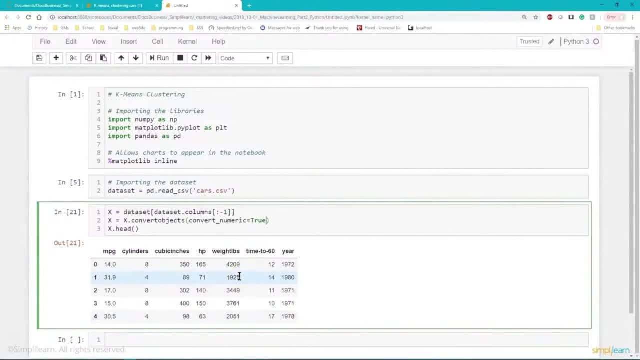 numeric. numeric equals true. And yes, I did have to go look that up. I don't have it memorized- the convert numeric in there. If I'm working with a lot of these things, I remember them, but depending on where I'm at, 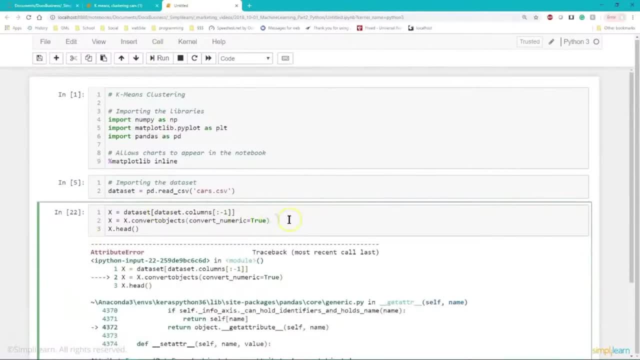 what I'm doing. I usually have to look it up And we run that: Oops, I must have missed something in here. Let me double check my spelling. And when I double check my spelling you'll see I missed the first underscore. 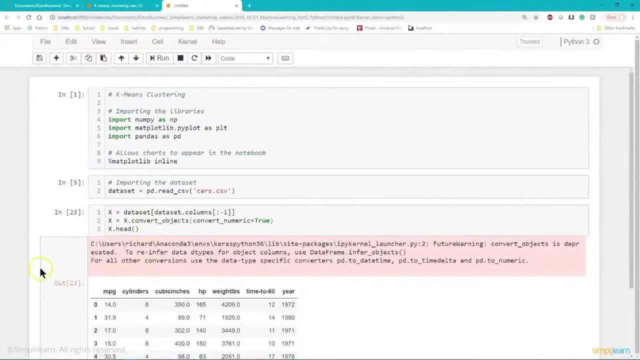 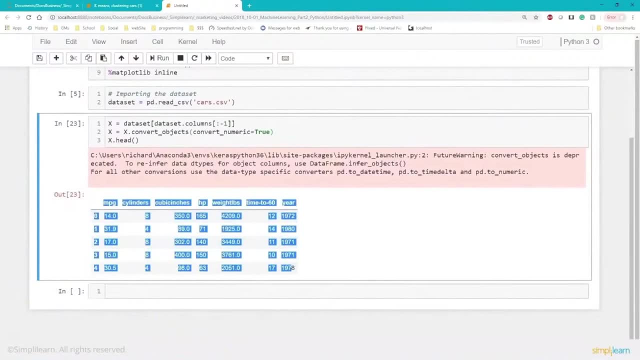 in the convert objects And when I run this, it now has everything converted into a numeric value, because that's what we're going to be working with, is numeric values down here, And the next part is that we need to go through the data. 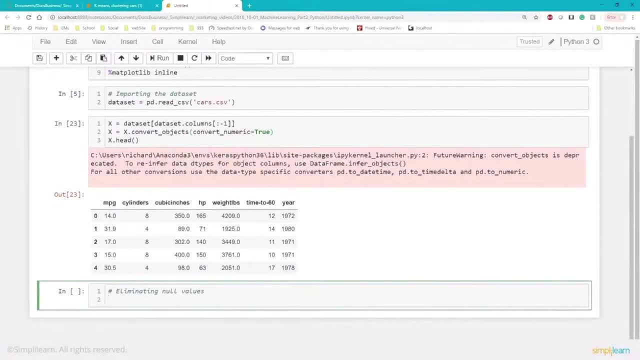 and eliminate null values. Most people, when they're doing small amounts, working with small data pools, discover afterwards that they have a null value and they have to go back and do this. So you know, be aware whenever we're formatting this data. 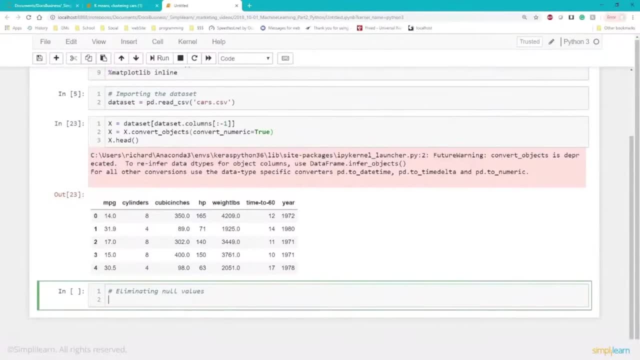 things are going to pop up and sometimes you go backwards to fix it, And that's fine. That's just part of exploring the data and understanding what you have, And I should have done this earlier, but let me go ahead and increase the size. 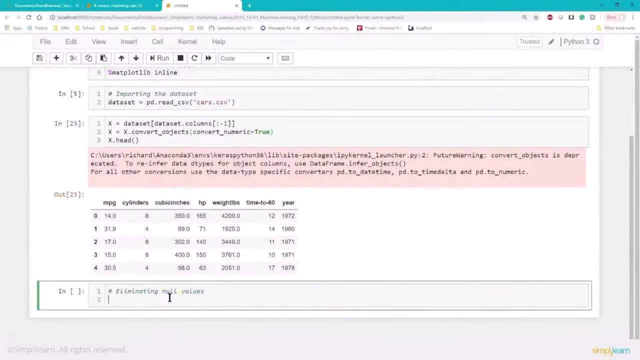 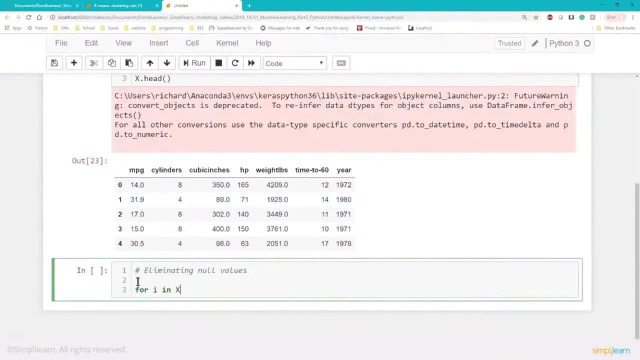 of my window one notch. There we go Easier to see. So we'll do for i. in working with x dot columns. We'll page through all the columns And we want to take x of i and we're going to change that. 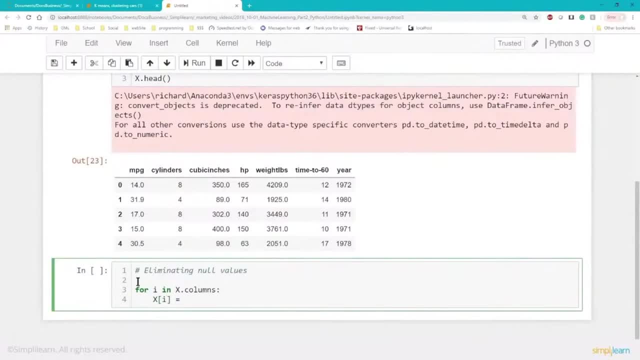 and we're going to alter it, And so with this, we want to go ahead and fill in x of i. Pandas has the fill in a, and that just fills in any non-existent missing data And we'll put my brackets up. 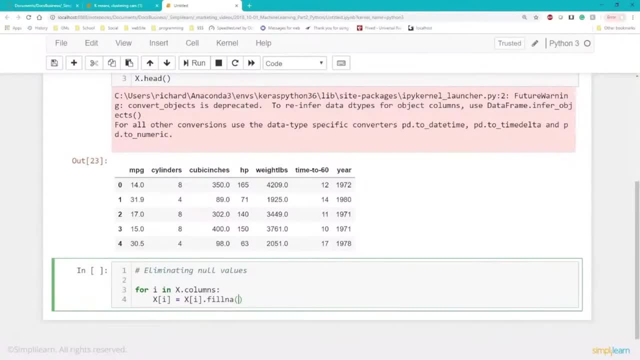 and there's a lot of different ways to fill this data. If you have a really large data set, some people just void out that data and then look at it later in a separate exploration of data. One of the tricks we can do is we can take our column. 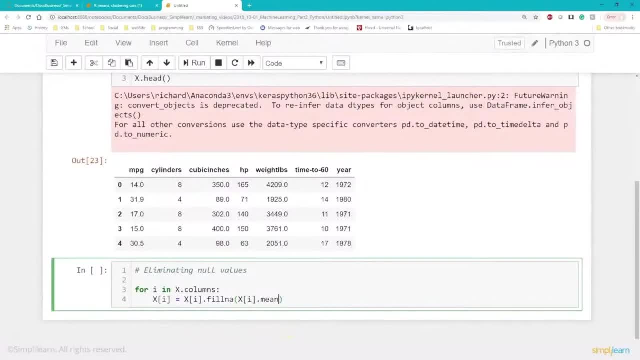 and we can find the means, And the means is in quotation marks. So when we take the columns, we're going to fill in the non-existing one with the means. The problem is that returns a decimal float, So some of these aren't decimals. 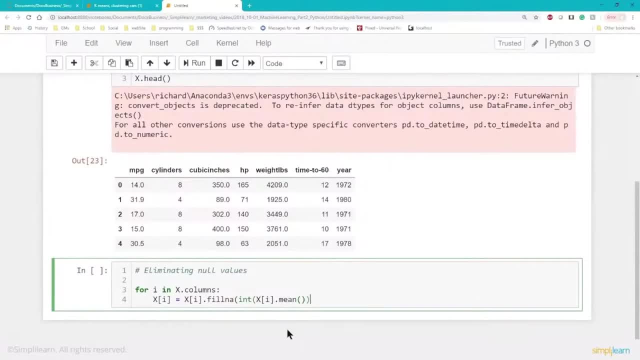 Certainly, you need to be a little careful doing this, but for this example, we're just going to fill it in with the integer version of this. It keeps it on par with the other data. that isn't a decimal point. And then what we also want to do. 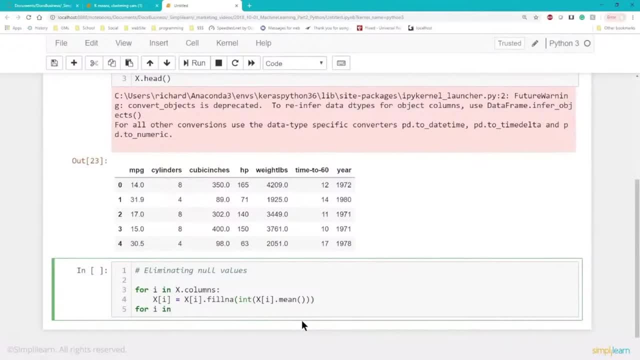 is. we want to double check. A lot of times you do this first part first to double check, then you do the fill and then you do it again just to make sure you did it right. So we're going to go through and test for missing data. 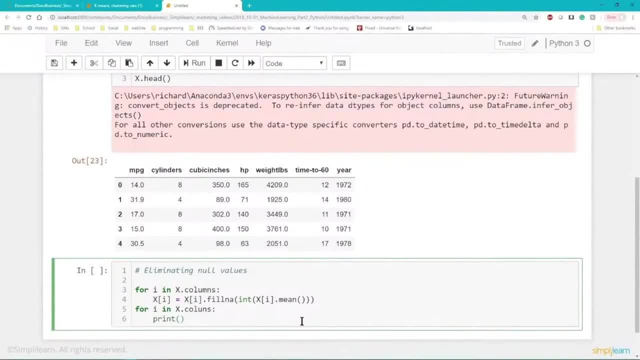 And one of the ways you can do that is simply go in here and take our x of i column. So it's going to go through. the x of i column It says is null, So it's going to return. any place there's a null value. 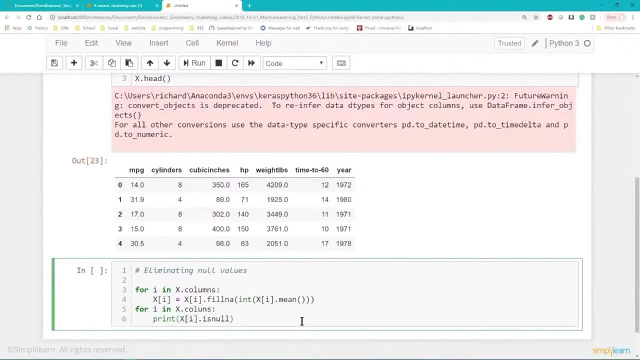 it actually goes through all the rows of each column- is null, And then we want to go ahead and sum that. So we take that, we add the sum value, and these are all pandas. so is null, is a panda command, and so is sum. 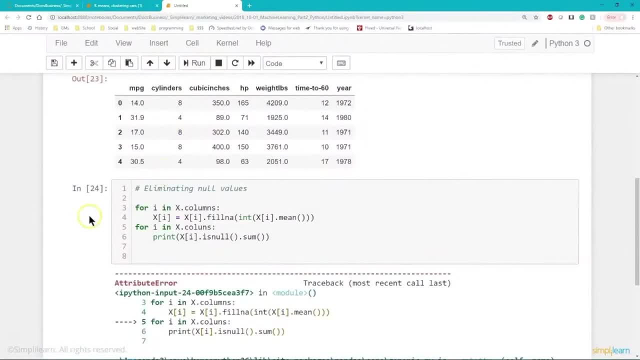 And if we go through that and we go ahead and run it and we go ahead and take and run that, you'll see that all the columns have zero null values. So we've now tested and double checked and our data is nice and clean. 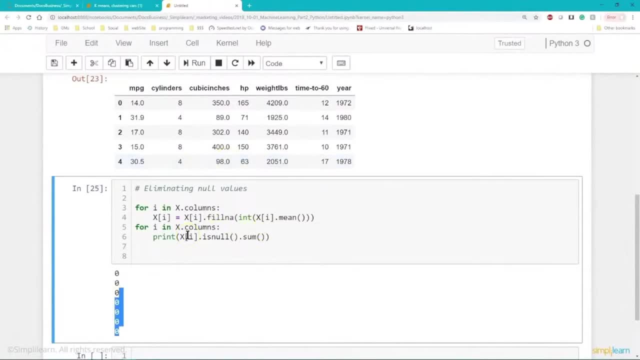 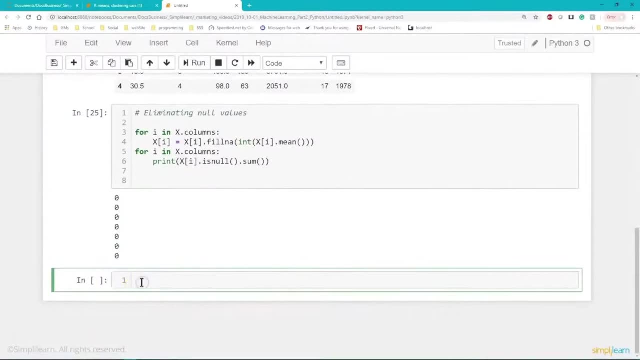 We have no null values. Everything is now a number value. We turned it into numeric And we've removed the last column in our data, And at this point we're actually going to start using the ELBO method to find the optimal number of clusters. 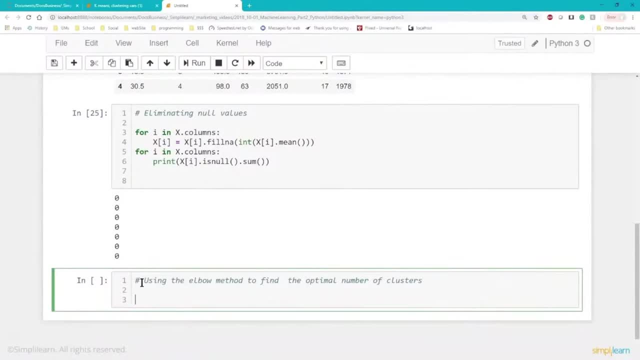 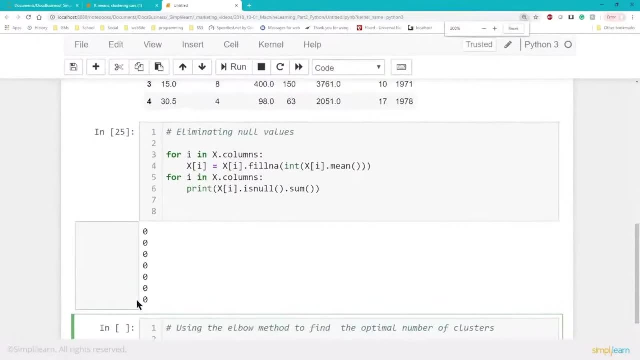 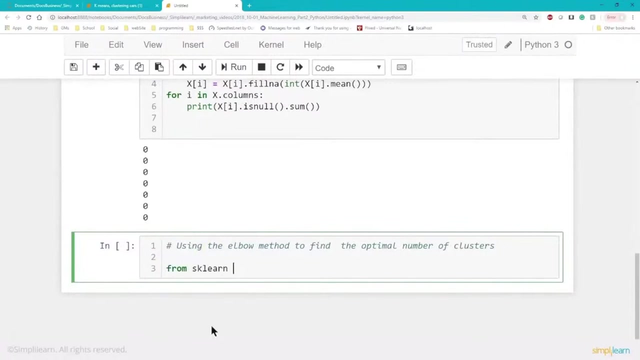 So we're now actually getting into the sklearn part, the k-means clustering on here. I guess we'll go ahead and zoom it up one more notch so you can see what I'm typing in here, And then from sklearn or sklearn cluster. 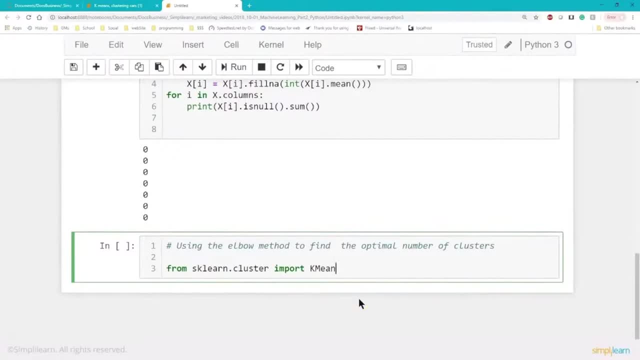 we're going to import k-means. I always forget to capitalize The k and the m when I do this, So it's capital K, capital M, k-means, And we'll go ahead and create a ray. WCSS equals. 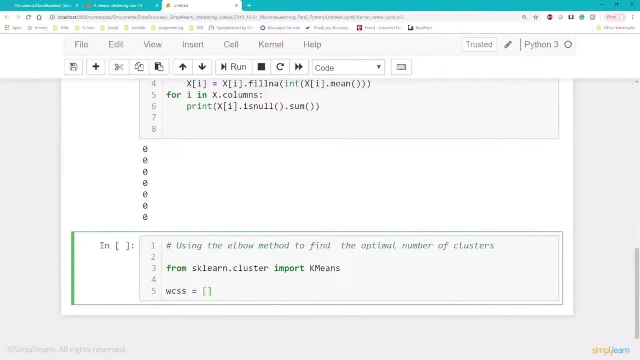 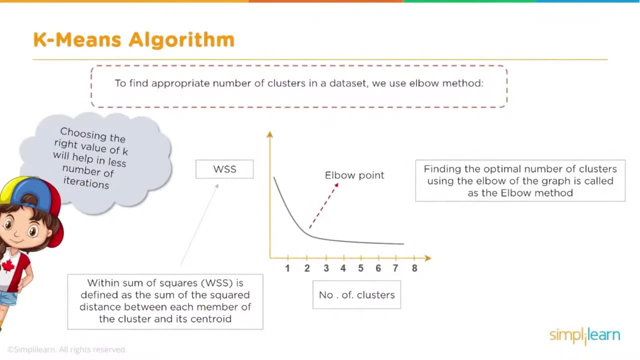 let me get an empty array. If you remember, from the ELBO method, from our slide, within the sum of squares, WSS is defined as the sum of square distance between each member of the cluster in a centroid. So we're looking at that change in differences. 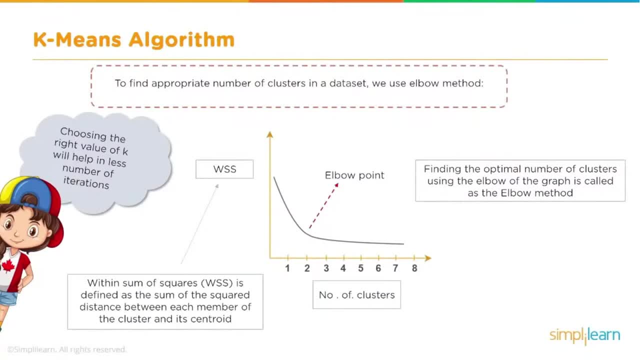 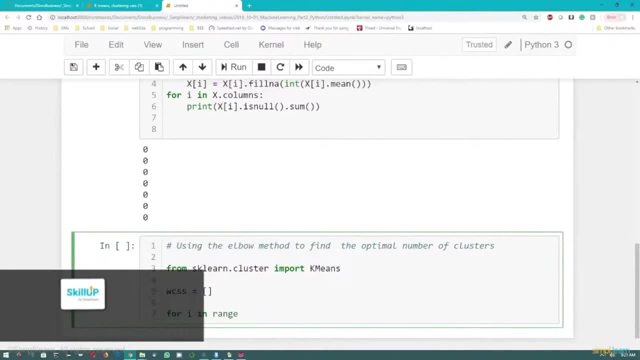 as far as the square distance, And we're going to run this over a number of k-mean values. In fact, let's go for i and range. We'll do 11 of them, Range 0 of 11.. And the first thing we're going to do, 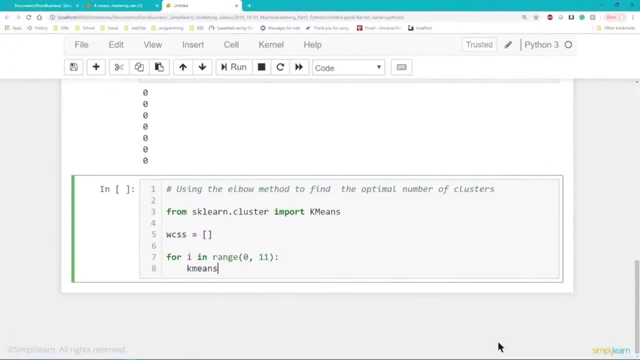 is, we're going to create the actual. we'll do it all lowercase, And so we're going to create this object from the k-means that we just imported, And the variable that we want to put into this is inClusters, And we're going to set that equals to i. 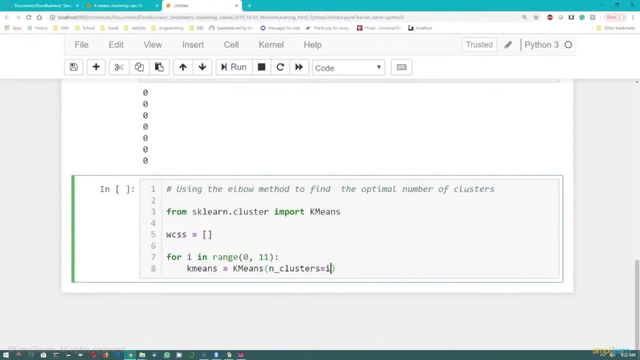 That's the most important one, because we're looking at how increasing the number of clusters changes our answer. There are a lot of settings to the k-means. Our guys in the back did a great job, just kind of playing with some of them. 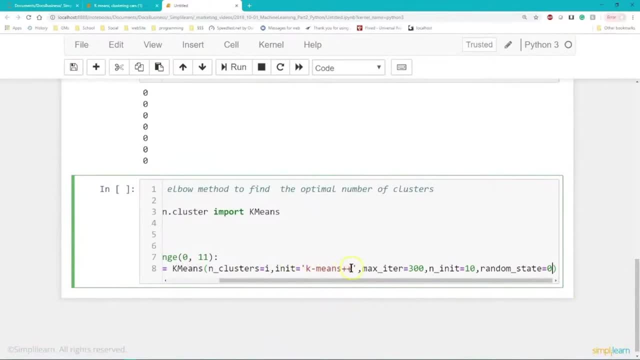 The most common ones that you see in a lot of stuff is how you init your k-means. So we have k-means plus, path plus. This is just a tool to let the model itself be smart- how it picks its centroids, to start with its initial centroids. 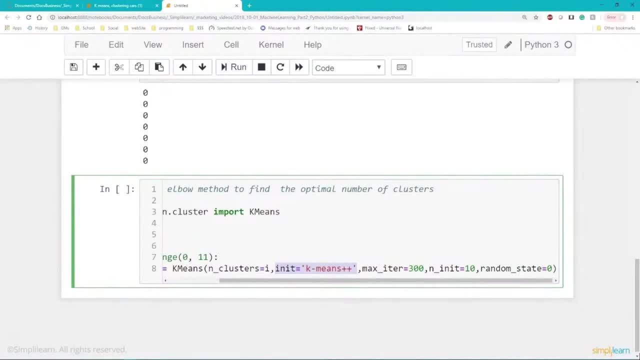 We only want to iterate no more than 300 times. We have a max iteration we put in there. We have the int init. the random state equals 0. You really don't need to worry too much about these when you're first learning this. 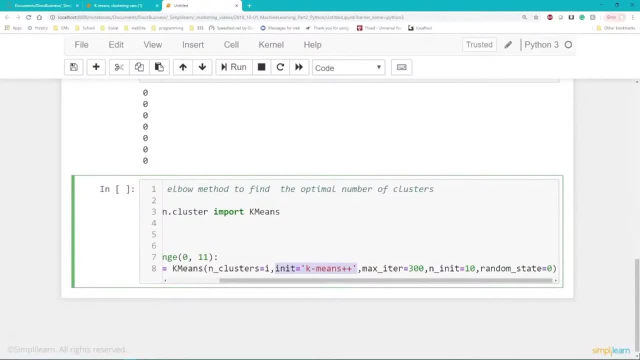 As you start digging in deeper, you start finding that these are shortcuts that will speed up the process as far as the setup, But the big one that we're working with is in clusters equals i, So we're going to literally train our k-means 11 times. 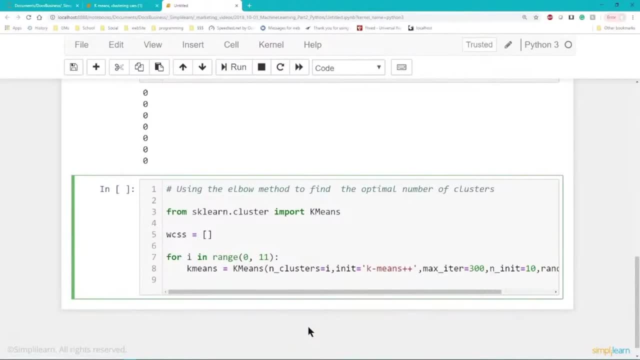 We're going to do this process 11 times And if you're working with big data, you know the first thing you do is you run a small sample of the data so you can test all your stuff on it And you can already see the problem. 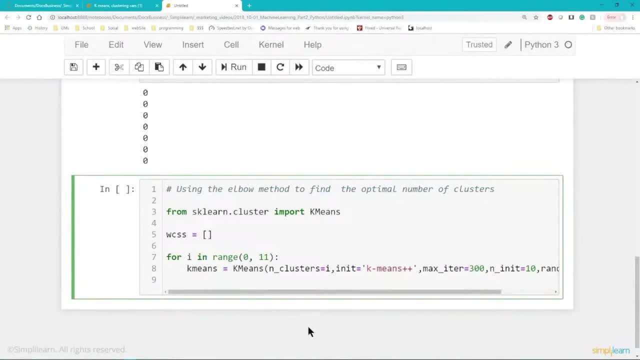 that if I'm going to iterate through a terabyte of data 11 times and then the k-means itself is iterating through the data multiple times, that's a heck of a process. So you've got to be a little careful with this. 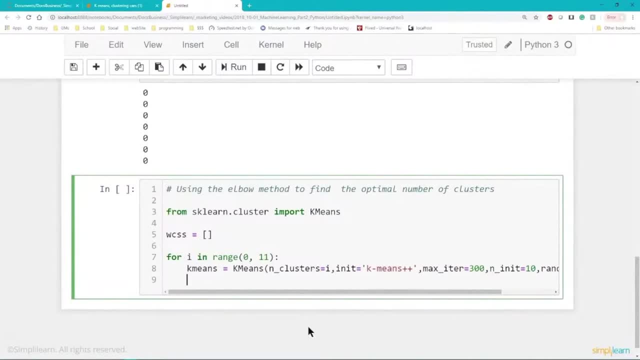 A lot of times, though, you can find your ELBO. using the ELBO method, find your optimal number on a sample of data, especially if you're working with larger data sources. So we want to go ahead and take our k-means. 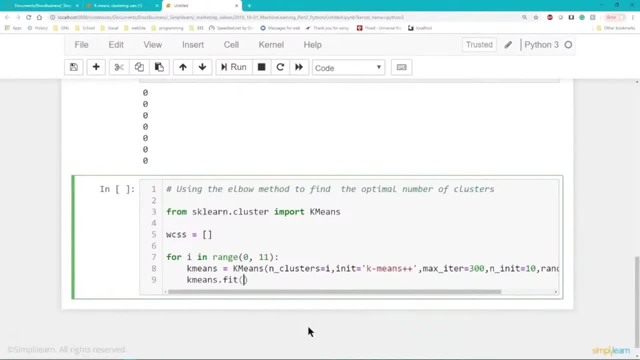 and we're just going to fit it. If you're looking at any of the sklearn- very common- you fit your model And, if you remember correctly, our variable we're using is the capital X And once we fit this value, we go back to the array we made. 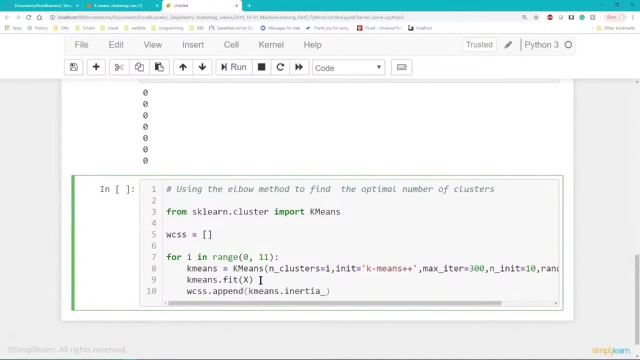 and we want to go ahead and just append that value on the end And it's not the actual fit we're pinning in there. it's when it generates it. it generates. the value you're looking for is inertia. So k-means dot. inertia will pull. 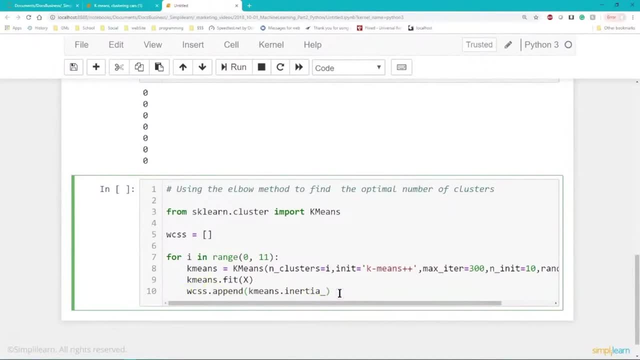 that specific value out that we need And let's get a visual on this. We'll do our PLT plot and what we're plotting here is first the X-axis, which is range 0, 11, so that will generate a nice little plot there. 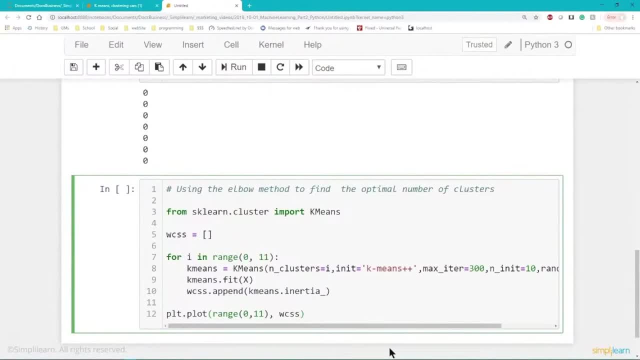 and the WCSS for our Y and the Y-axis. It's always nice to give our plot a title and let's see, we'll just give it the elbow method for the title and let's get some labels. so let's go ahead and do PLT X label. 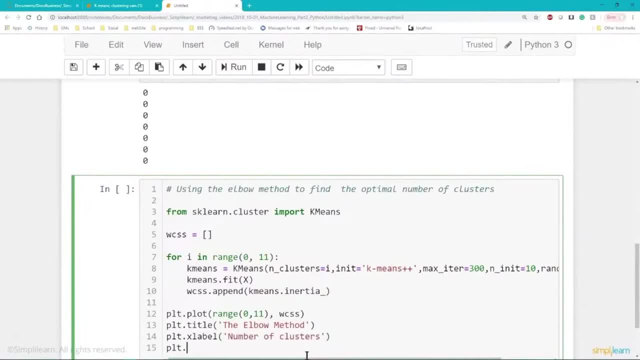 and what we'll do. we'll do number of clusters for that and PLT Y label, and for that we can do: oops, there we go, WCSS, since that's what we're doing on the plot on there. 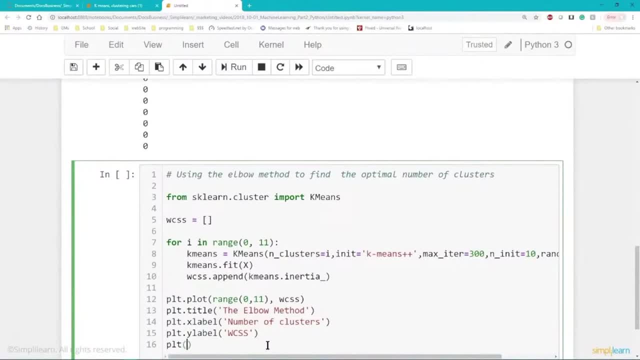 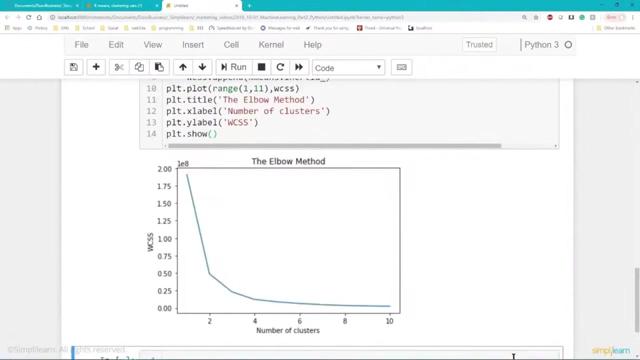 we want to go ahead and display our graph, which is simply PLT dot show. There we go And because we have it set to inline, it'll appear inline. Hopefully I didn't make a type error on there And you can see we get a very nice graph. 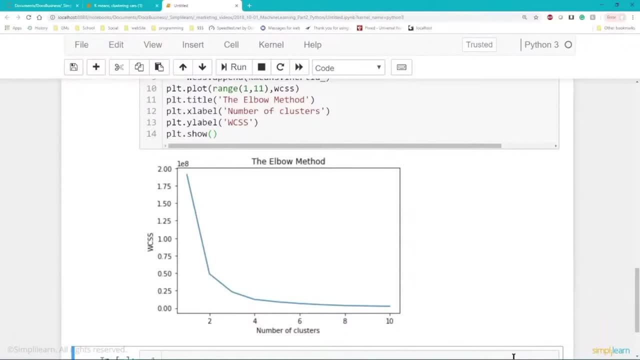 You can see a very nice elbow joint there at 2, and again right around 3 and 4, and then after that there's not very much. Now, as a data scientist, if I was looking at this I would do either 3 or 4,. 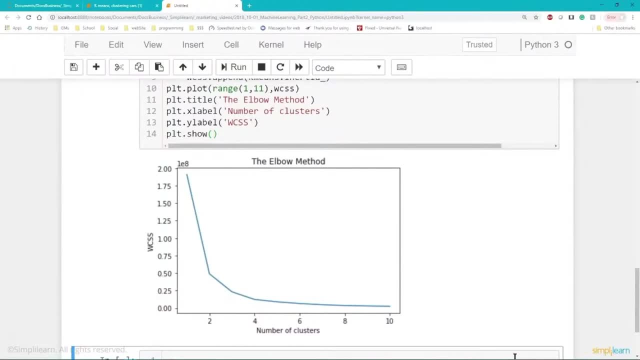 and I'd actually try both of them to see what the output looked like, And they've already tried this in the back. so we're just going to use 3 as a setup on here And let's go ahead and see what that looks like. 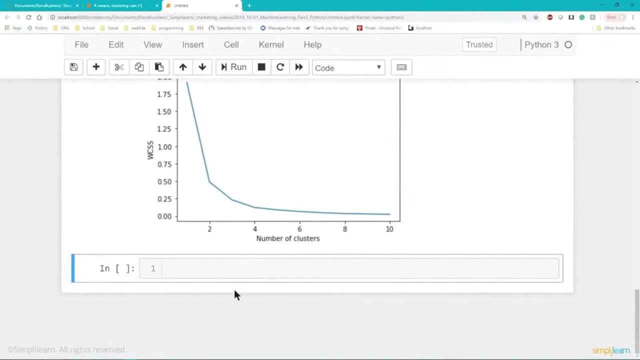 when we actually use this to show the different kinds of cars. And so let's go ahead and apply the k-means to the cars data set And basically we're going to copy the code that we looped through up above where k-means equals k-means. 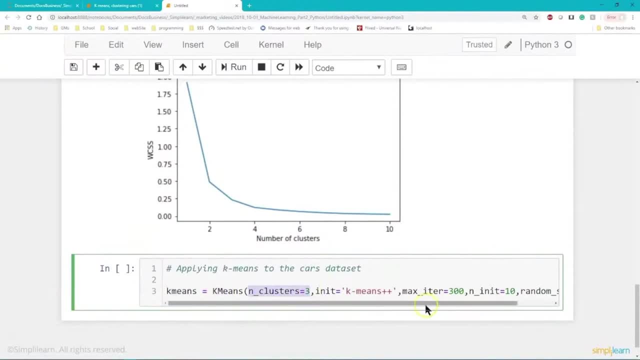 number of clusters, and we're just going to set that number of clusters to 3, since that's what we're going to look for, And you can do 3 and 4 on this and graph them just to see how they come up differently. 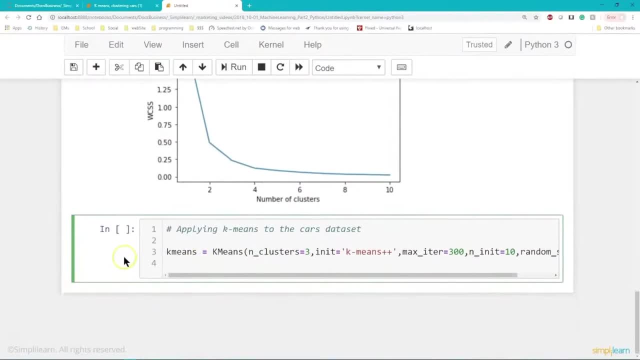 I'd be kind of curious to look at that, But for this we're just going to set it to 3. Go ahead and create our own variable yk-means for our answers, And we're going to set that equal to. 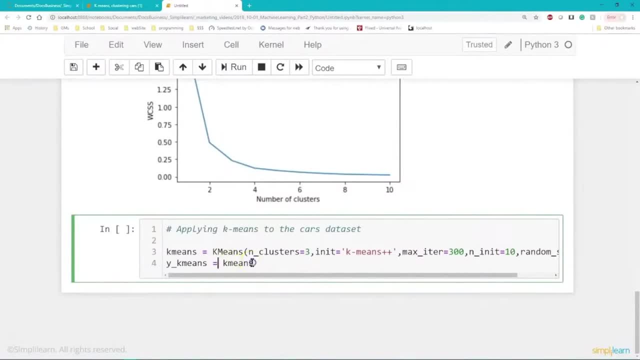 whoops. a double equal there to k-means. but we're not going to do a fit. We're going to do a fit: predict which is the setup you want to use, And when you're using untrained models, you'll see a slightly different. 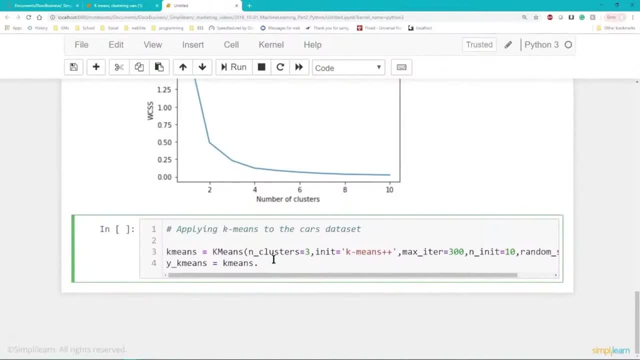 because usually you see fit and then you see just the predict. But we want to both fit and predict the k-means on this, And that's fit, underscore predict. and then our capital X is the data we're working with. And before we plot this data, 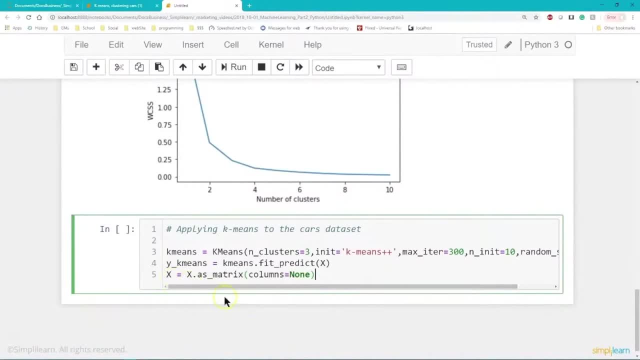 we're going to do a little panda's trick. We're going to take our X value and we're going to set X as matrix. So we're converting this into a nice rows and columns kind of setup and we want the we're going to have columns equals none. 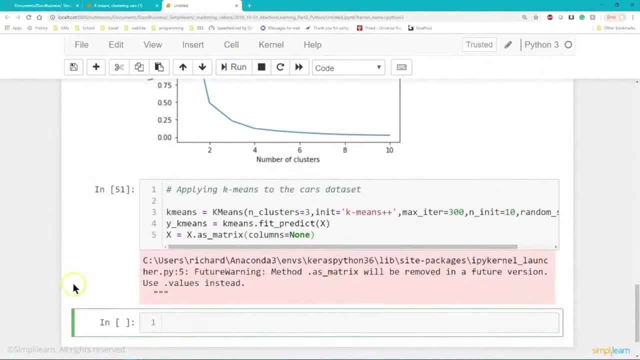 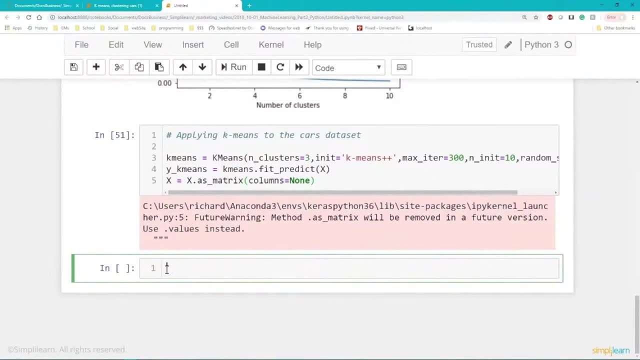 so it's just going to be a matrix of data in here And let's go ahead and run that. A little warning. You'll see these warnings pop up because things are always being updated, So there's like minor changes in the versions and future versions. 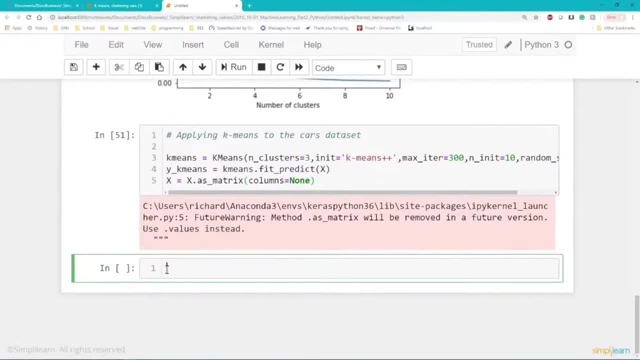 Instead of matrix. now it's more common to set it dot values instead of doing as matrix. But math as matrix works just fine for right now and you'll want to update that later on. But let's go ahead and dive in and plot this. 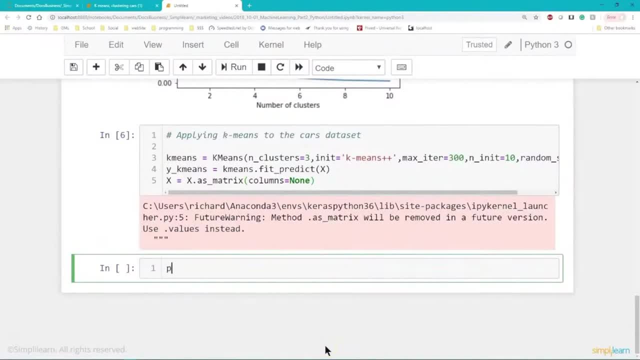 data, And before we dive into plotting this data, I always like to take a look and see what I am plotting. So let's take a look at Y. K means I'm just going to print that out down here And we see, we have an array of answers. 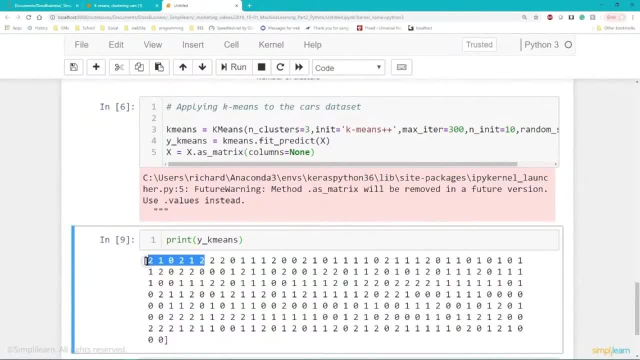 We have 2, 1, 0, 2, 1, 2.. So it's clustering these different rows of data based on the three different spaces it thinks it's going to be, And then let's go ahead and print X. 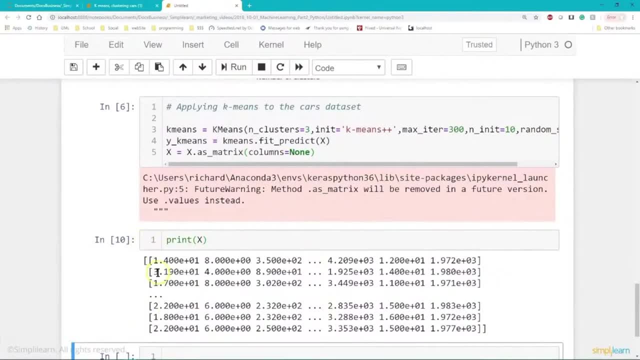 and see what we have for X, And we'll see that X is an array, it's a matrix, so we have our different values in the array And what we're going to do. it's very hard to plot all the different values. 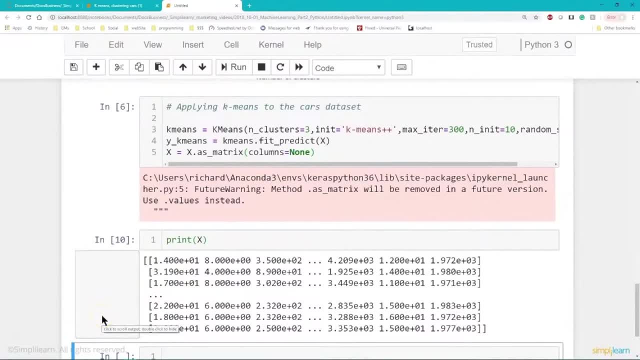 in the array. so we're only going to be looking at the first two, or positions 0 and 1.. And if you were doing a full presentation in front of the board meeting, you might actually do a little different and dig a little deeper into the different. 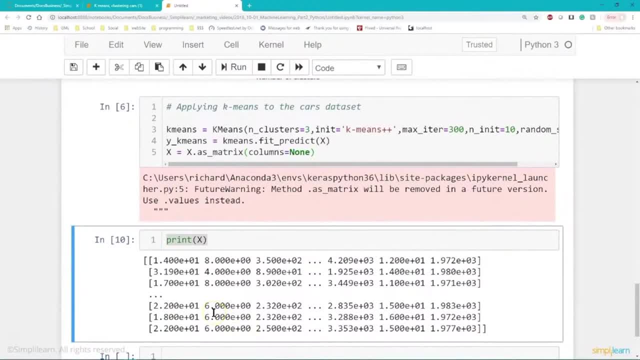 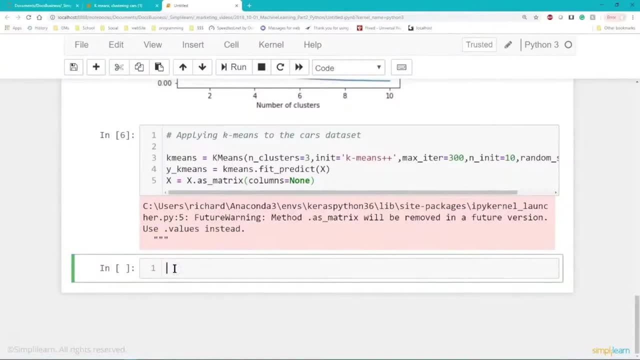 aspects, because this is all the different columns we looked at, But when we look at columns 1 and 2, for this to make it easy. So let's go ahead and clear this data out of here and let's bring up our plot, And we're going to do. 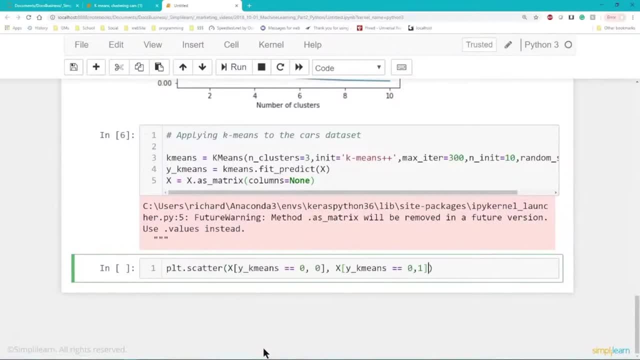 a scatter plot here, so PLT scatter, and this looks a little complicated, so let's explain what's going on with this. We're going to take the X values and we're only interested in Y of K means equals 0, the first cluster. 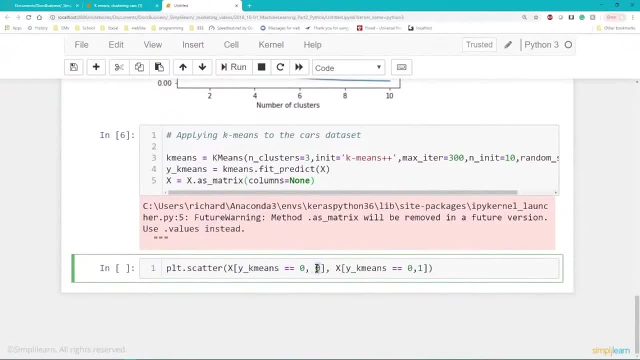 Okay, And then we're going to take value 0 for the X axis, and then we're going to do the same thing. here We're only interested in K means equals 0, but we're going to take the second column, So we're only looking at. 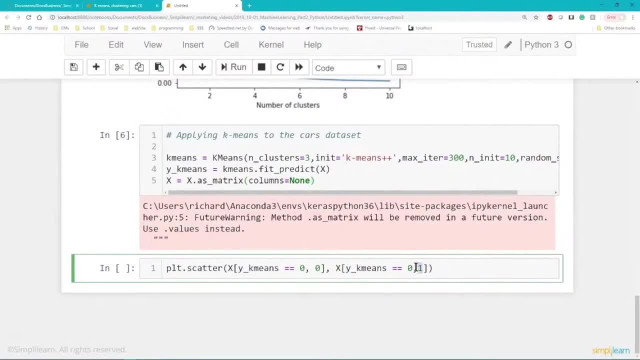 the first two columns in our answer or in the data. And then the guys in the back played with this a little bit to make it pretty And they discovered that it looks good if it has a size equals 100, that's the size of the dots. 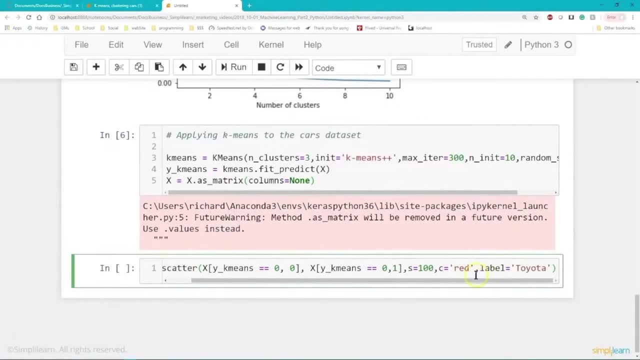 We're going to use red for this one, and when they were looking at the data and what came out, it was definitely the Toyota. on this, We're just going to go ahead and label it Toyota. Again, that's something you really have to explore in here. 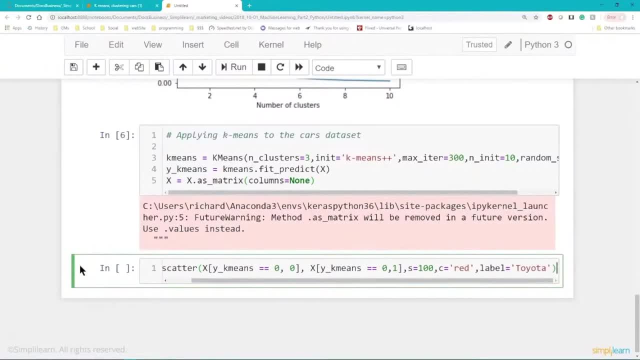 as far as playing with those numbers and see what looks good, We'll go ahead and hit enter in there And I'm just going to paste in the next two lines, which is the next two cars, And this is our Nissan and Honda, And you'll see, with our 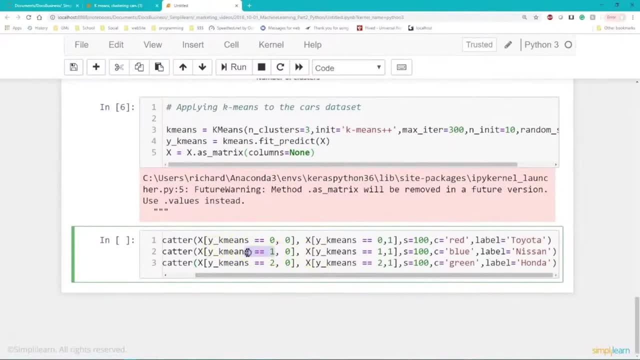 scatter plot. we're now looking at where Y underscore K means equals 1. And we want the 0 column and Y K means equals 2.. Again, we're looking at just the first two columns, 0 and 1.. And each of 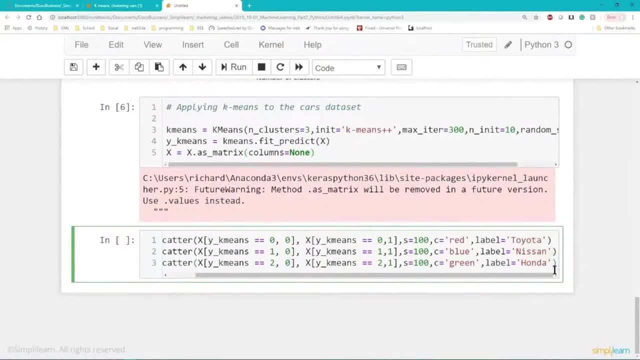 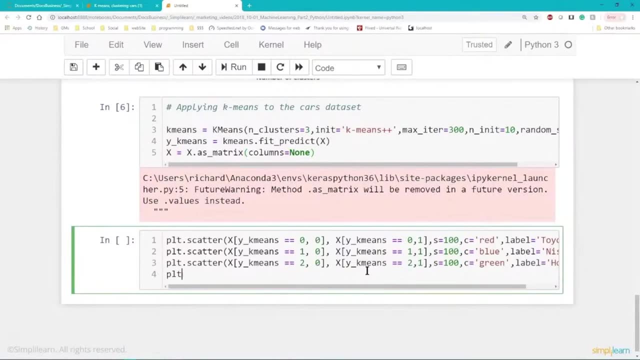 these rows then corresponds to Nissan and Honda, And I'll go ahead and hit enter on there. And finally, let's take a look and put the centroids on there. Again, we're going to do a scatter plot And on the centroids you can just pull. 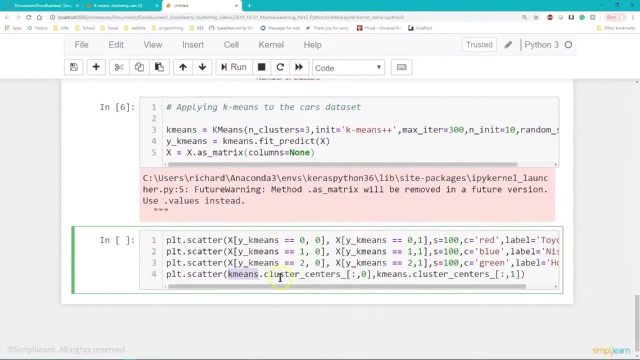 that from our K means the model. we created, dot cluster centers, and we're going to just do all of them in the first number and all of them in the second number, which is 0, 1.. Because you always start with 0 and 1.. 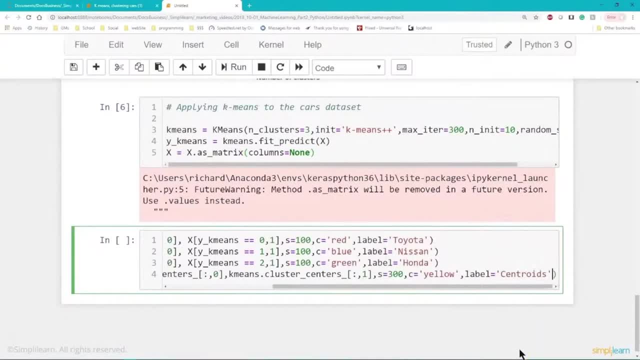 And then if you were playing with the size and everything to make it look good, we'll do a size of 300.. We're going to make the color yellow And we'll label them. it's always good to have some good labels. centroids. 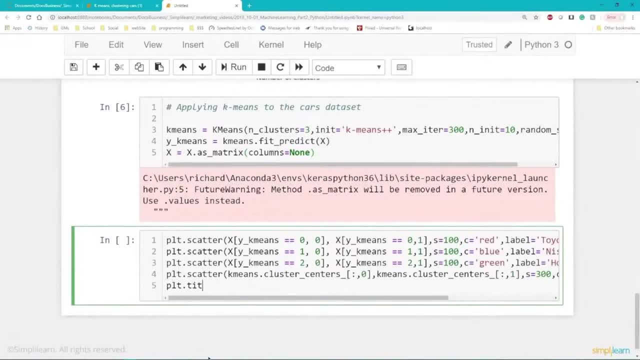 And then we want to do a title- PLT title- And pop up there PLT title. because you always want to make your graphs look pretty, We'll call it clusters of star make, And one of the features of the plot library is you can 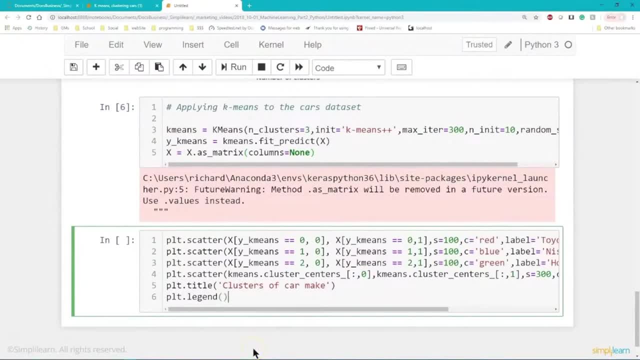 add a legend, It'll automatically bring in it, since we've already labeled the different aspects of the legend with Toyota, Nissan and Honda. And finally, we want to go ahead and show So we can actually see it And remember it's inline. So if you're using 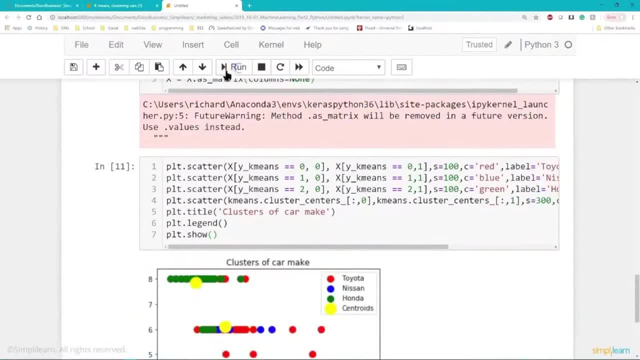 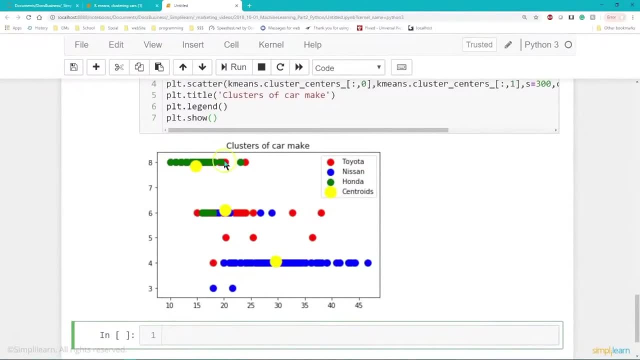 a different editor. that's not the Jupyter Notebook. you'll get a pop up of this And you should have a nice set of clusters here. So we can look at this and we have a nice set of clusters of Honda in green, Toyota in red. 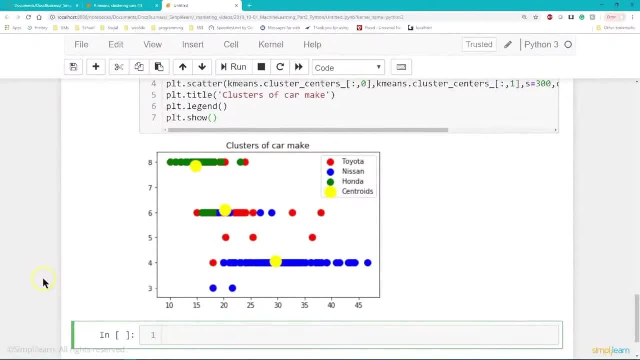 Nissan in purple And you can see where they put the centroids to separate them. Now, when we're looking at this, we can also plot a lot of other different data on here. as far because we only looked at the first two columns, This is just column one. 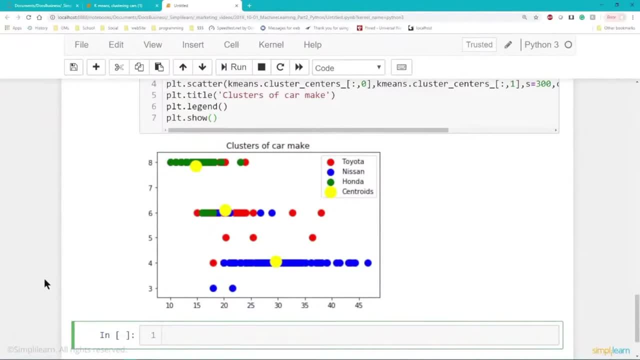 and two or zero one as you label them in computer scripting. But you can see, here we have nice clusters of car make and we've been able to pull out the data and you can see how just these two columns form very distinct clusters of data. 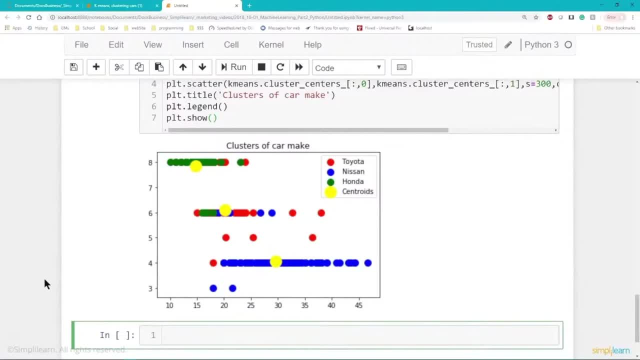 So if you were exploring new data, you might take a look and say: well, what makes these different? Almost going in reverse, you start looking at the data and pulling apart the columns to find out why is the first group set up the way it is? Maybe you're doing. 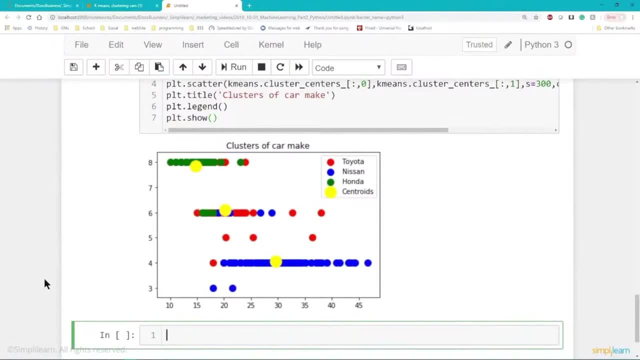 loans and you want to go. well, why is this group not defaulting on their loans? And why is the last group defaulting on their loans? And why is the middle group- 50%- defaulting on their bank loans? And you start finding ways to manipulate. 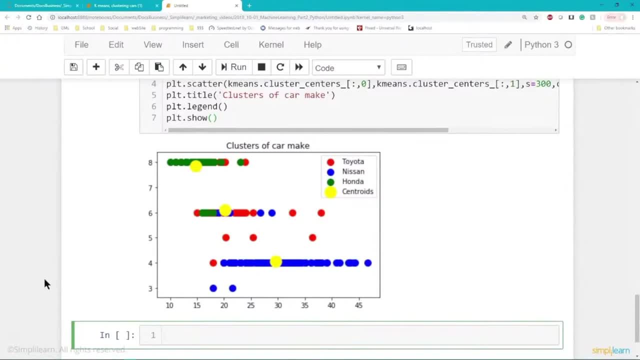 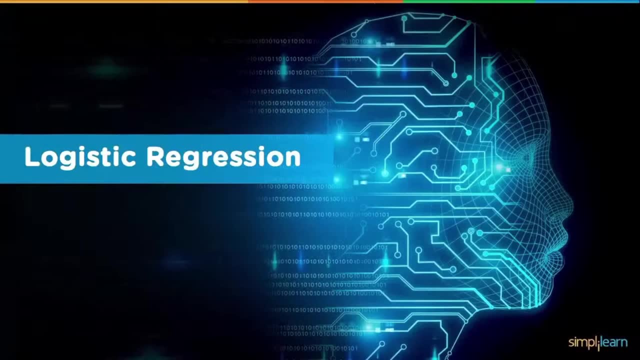 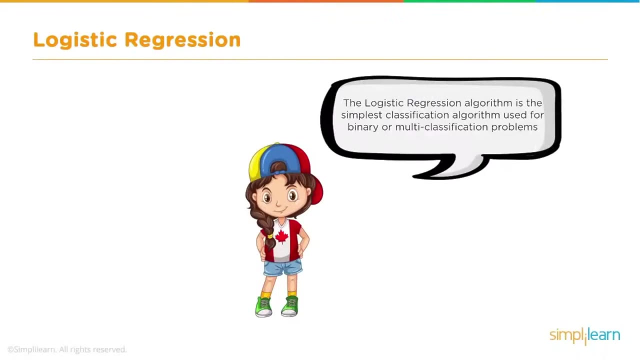 the data and pull out the answers you want. So now that you've seen how to use k-mean for clustering, let's move on to the next topic. Now let's look into logistic regression. The logistic regression algorithm is the simplest classification algorithm used for binary. 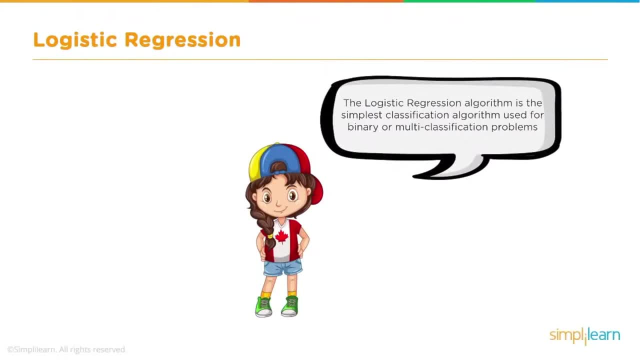 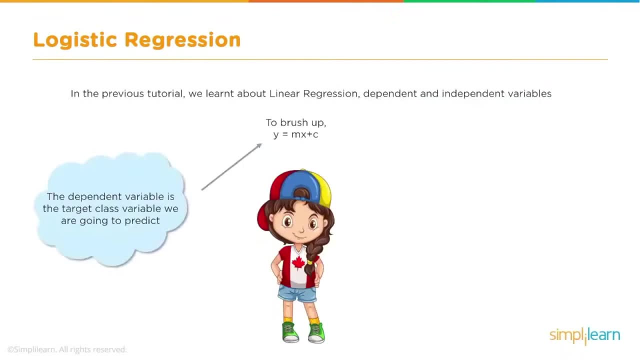 or multi-classification problems And we can see we have our little girl from Canada, who's into horror books, is back. That's actually really scary when you think about that with those big eyes. In the previous tutorial we learned about linear regression, dependent and independent. 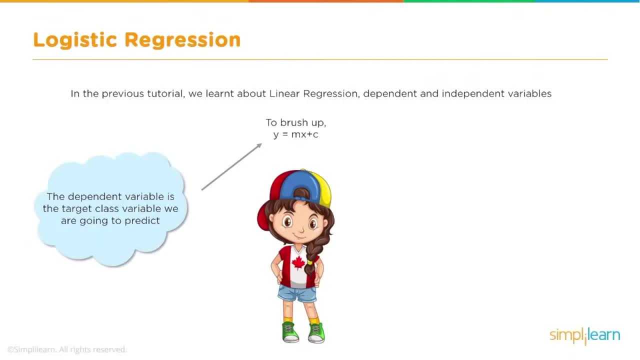 variables. So, to brush up, y equals mx plus c, a very basic algebraic function of y and x. The dependent variable is the target class variable we are going to predict. The independent variables, x1 all the way up to xn, are the features. 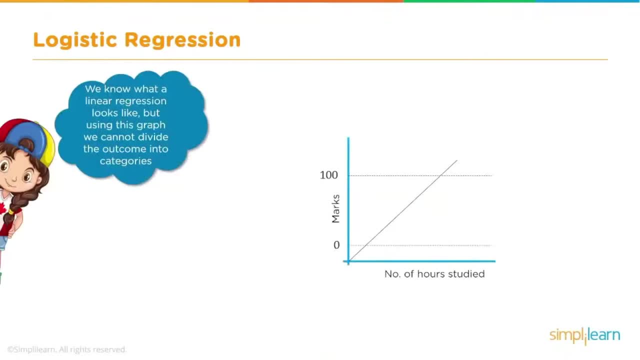 or attributes we're going to use to predict the target class. We know what a linear regression looks like, but using the graph we cannot divide the outcome into categories. It's really hard to categorize 1.5,, 3.6, 9.8.. 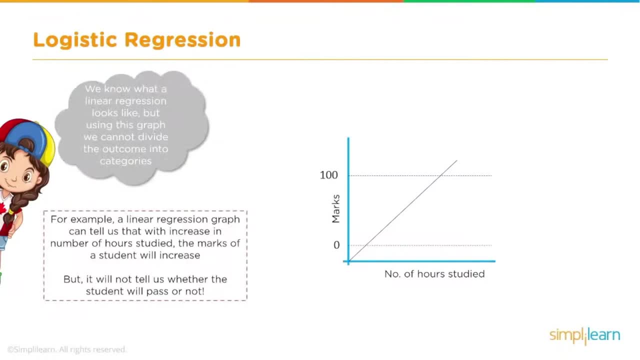 For example, a linear regression graph can tell us that, with increase in number of hours studied, the marks of a student will increase, But it will not tell us whether the student will pass or not In such cases where we need the output as categorical value. 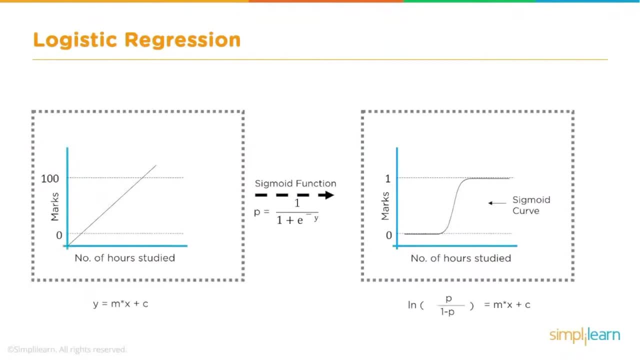 we will use logistic regression And for that we're going to use the sigmoid function. So you can see, here we have our marks 0 to 100, and the number of hours studied. That's going to be what they're comparing it to. 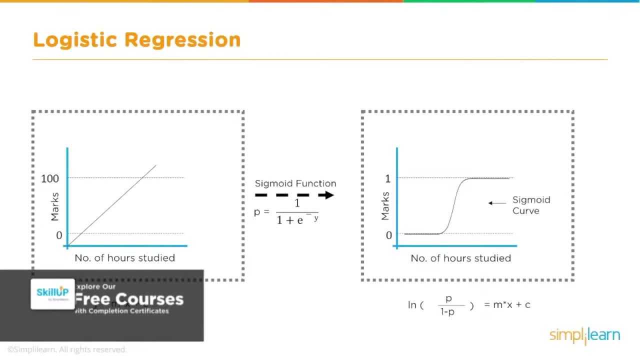 in this example, And we usually form a line that says y equals mx plus c, And when we use the sigmoid function we have: p equals 1 over 1 plus e to the minus y. It generates a sigmoid curve, And so you can see right here. 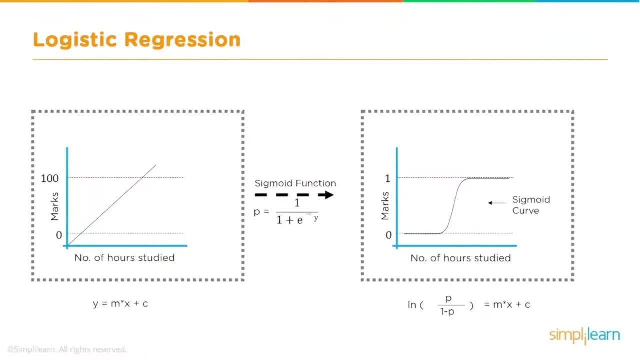 when you take the ln, which is the natural logarithm. I always thought it should be nl not ln. That's just the inverse of e, or e to the minus y, And in this we get ln of p over 1 minus p equals. 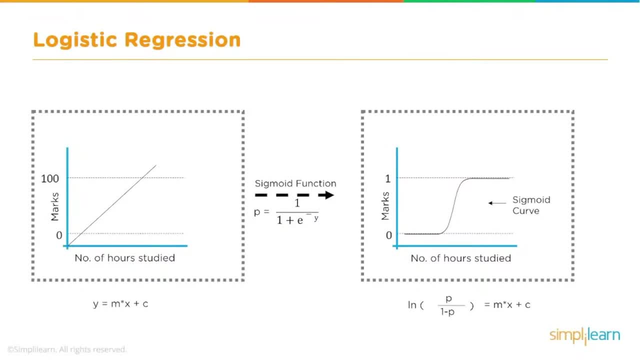 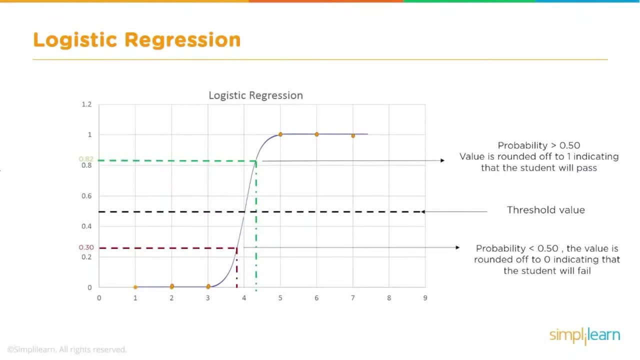 m times x plus c. That's the sigmoid curve function we're looking for. Now we can zoom in on the function and you'll see that the function as it derives goes to 1 or to 0, depending on what your x value is And the probability. 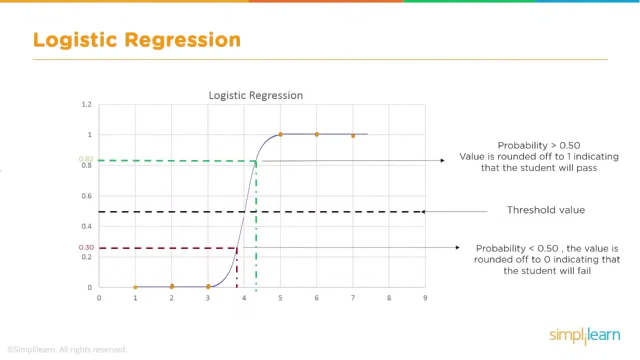 if it's greater than 0.5, the value is automatically rounded off to 1, indicating that the student will pass. So if they're doing a certain amount of studying, they will probably pass. Then you have a threshold value at the. 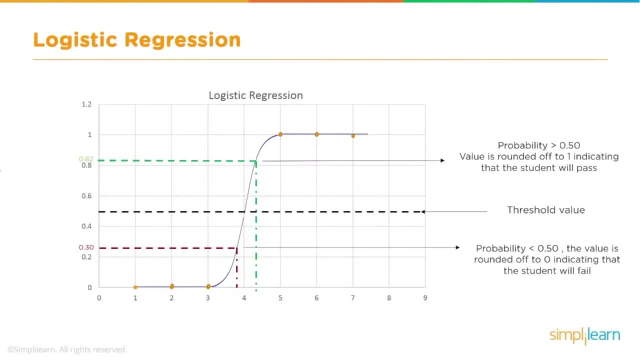 0.5. It automatically puts that right in the middle usually And your probability: if it's less than 0.5, the value rounded off to 0, indicating the student will fail. So if they're not studying very hard, 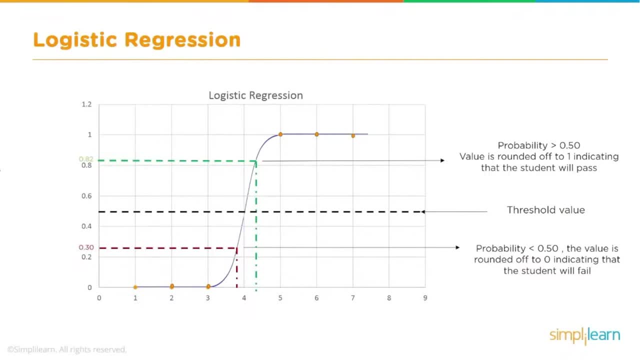 they're probably going to fail. This, of course, is ignoring the outliers of that one student who's just a natural genius and doesn't need any studying to memorize everything. That's not me, unfortunately. I have to study hard to learn new stuff. 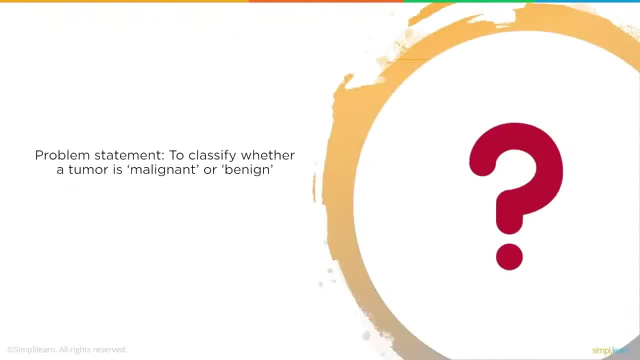 Problem statement To classify whether a tumor is malignant or benign. And this is actually one of my favorite data sets to play with because it has so many features and when you look at them you really are hard to understand. You can't just look at. 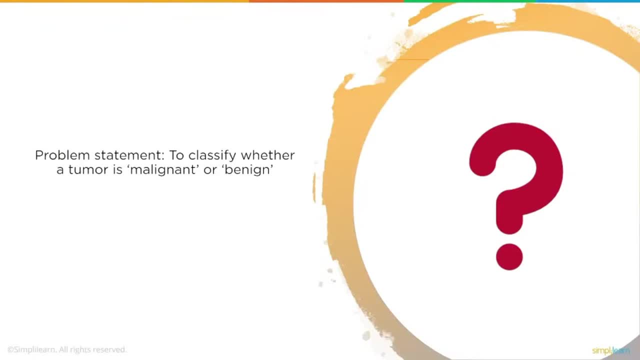 them and know the answer. So it gives you a chance to kind of dive into what data looks like when you aren't able to understand the specific domain of the data. But I also want to remind you that in the domain of medicine, if I told you, 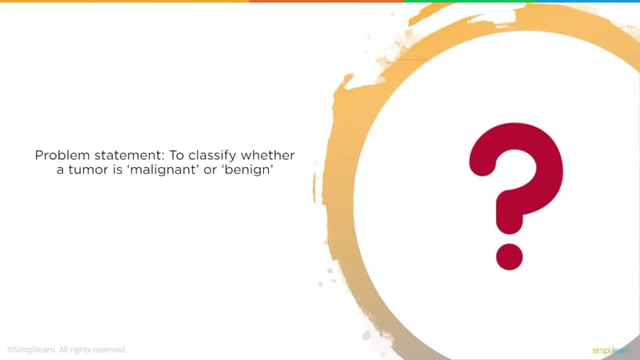 that my probability was really good and classified things at, say, 90% or 95%, and I'm classifying whether you're going to have a malignant or a benign tumor. I'm guessing that you're going to go get it tested anyways, So you've got to remember the domain we're working with. 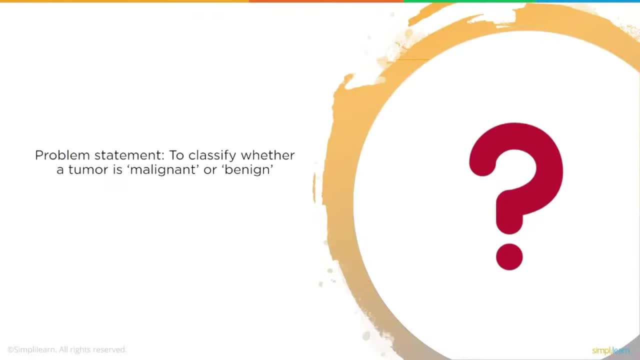 So why would you want to do that if you know you're just going to go get a biopsy? because it's that serious. This is like an all or nothing. Just referencing the domain it's important. It might help the doctor know where to look. 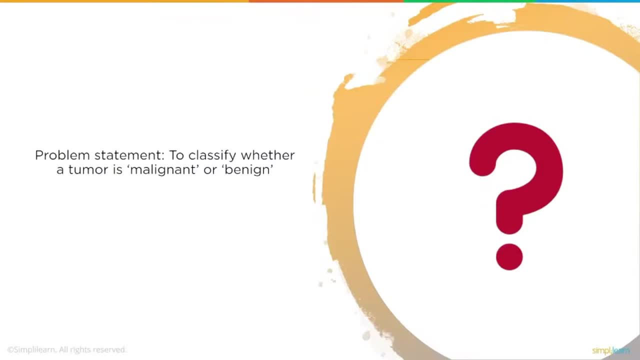 just by understanding what kind of tumor it is. So it might help them or aid them in something they missed from before. So let's go ahead and dive into the code, and I'll come back to the main part of it in just a minute. 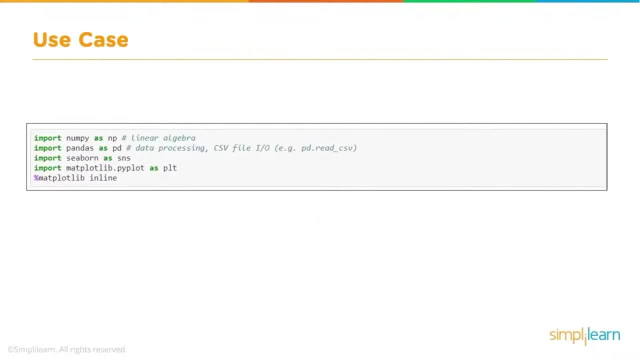 So use case, and we're going to do our normal imports here, where we're importing NumPy, Pandas, Seaborn, the Matplot library, and we're going to do Matplot library inline, since I'm going to switch over to Anaconda. So let's go ahead and 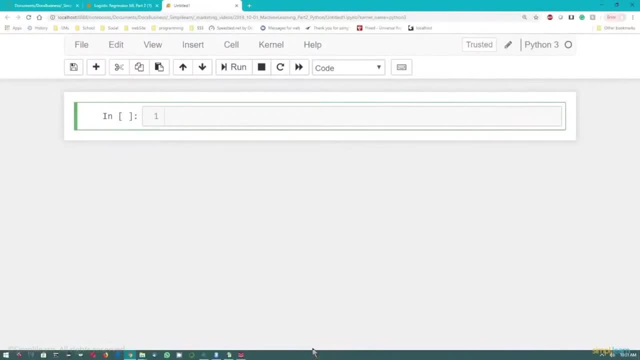 flip over there and get this started. So I've opened up a new window in my Anaconda Jupyter Notebook And, by the way, Jupyter Notebook, you don't have to use Anaconda for the Jupyter Notebook. I just love the interface and all the tools that Anaconda 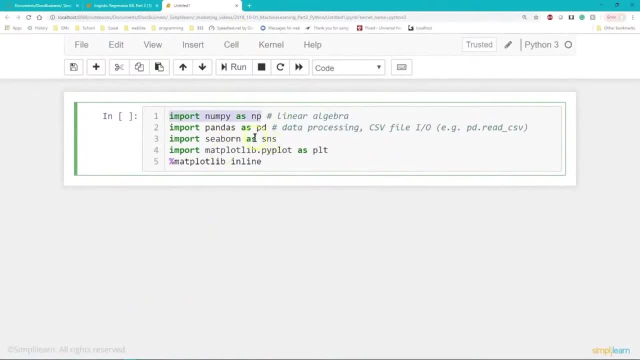 brings. So we've got our import. as in p, for our NumPy number array We have our Pandas pd We're going to bring in Seaborn to help us with our graphs as sns. So many really nice tools in both Seaborn and Matplot. 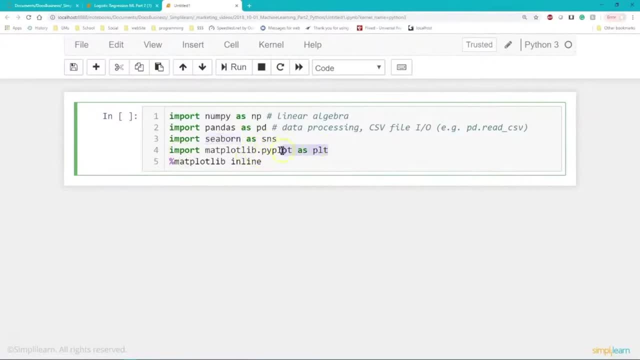 library, Then we'll do our Matplot librarypyplot as plt, and then of course, we want to let it know to do it inline. Let's go ahead and just run that. so it's all set up And we're just going to call our data data. 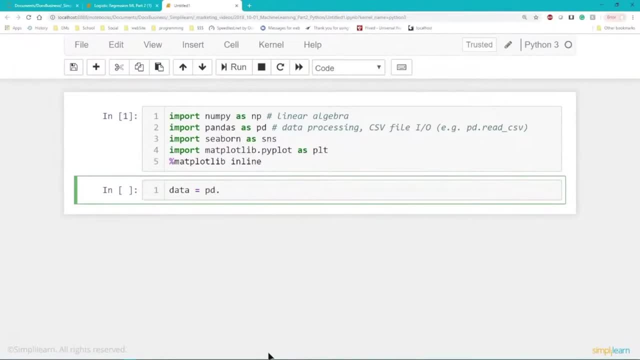 Not creative. today Equals pd and this happens to be in a cs? v file, So we'll use the pdread underscore csv and I happen to name the file. I renamed it data4p2.csv. You can, of course, write in the comments below the YouTube and request. 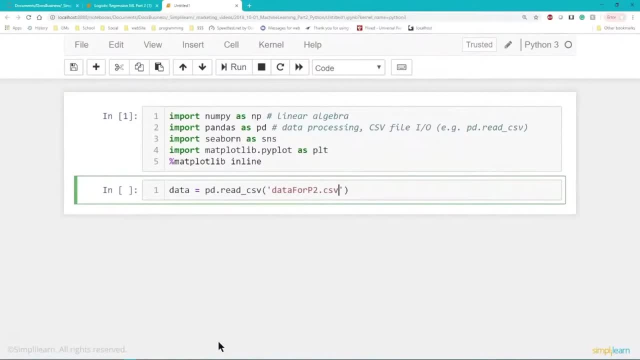 for the data set itself, or go to the Simply Learn website and we'll be happy to supply that for you. And let's just open up the data before we go any further and let's just see what it looks like in a spreadsheet. So when I 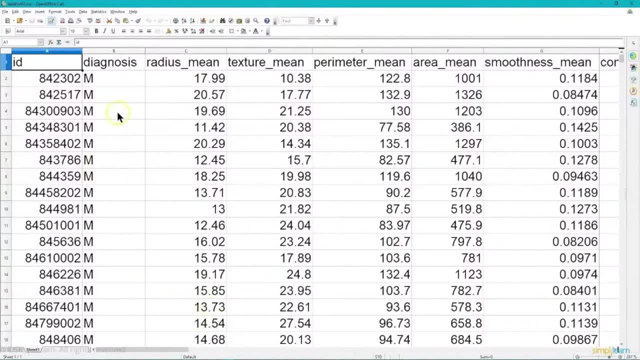 pop it open in a local spreadsheet. this is just a csv file, It's not a separate variables. We have an id, so I guess the categorizes for reference or what id which test was done. The diagnosis: m for malignant, b for benign. 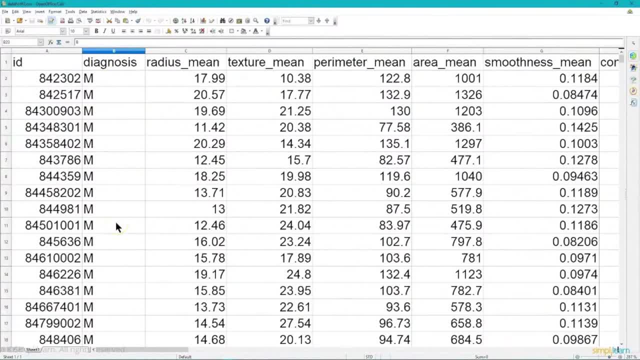 So there's two different options on there, And that's what we're going to try to predict is the m and b and test it, And then we have, like the radius, mean or average, the texture, average perimeter, mean area, mean, smoothness. 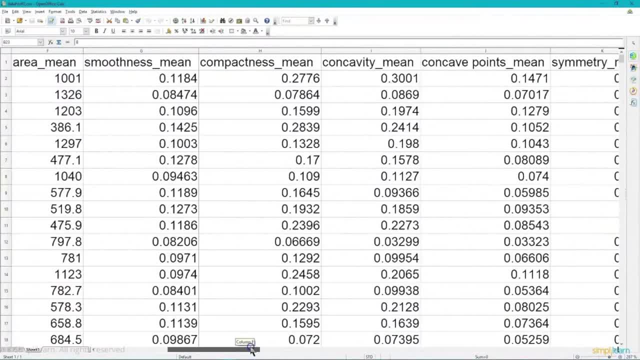 I don't know about you, but unless you're a doctor in the field, most of the stuff I mean- you can guess what concave means just by the term concave, But I really wouldn't know what that means in the measurements they're taking. 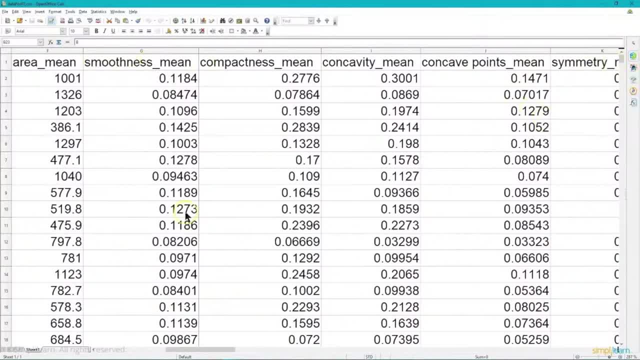 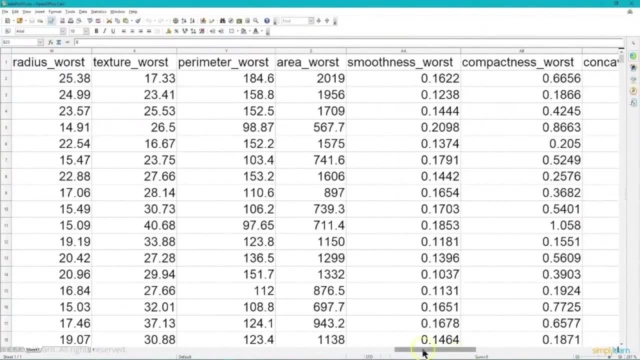 So they have all kinds of stuff like how smooth it is the symmetry, and these are all float values. We can just page through them real quick And you'll see. there's, I believe, 36, if I remember correctly, in this one. So there's a lot of. 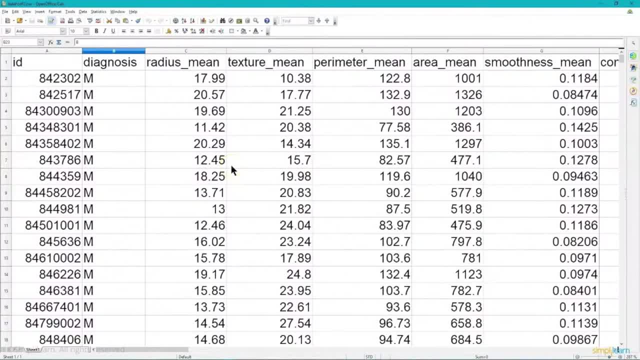 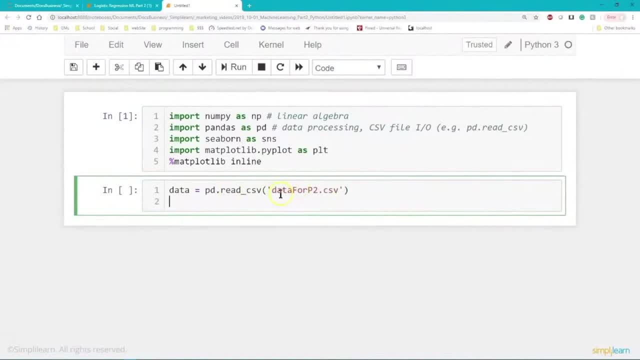 different values they take and all these measurements they take when they go in there and they take a look at the different growth, the tumorous growth. So back in our data and I put this in the same folder as a code So I saved. 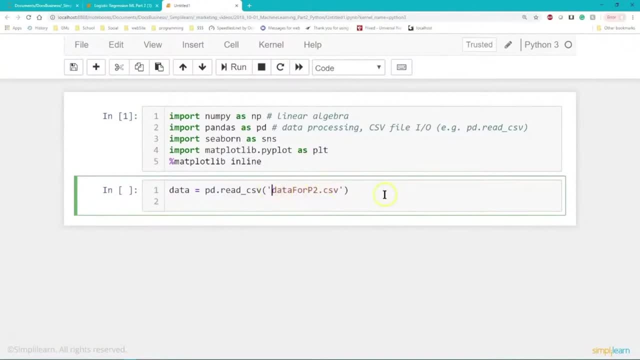 this code in that folder. Obviously, if you have it in a different location, you want to put the full path in there And we'll just do Panda's first five lines of data with the data dot head. When we run that we can see that we have pretty much. 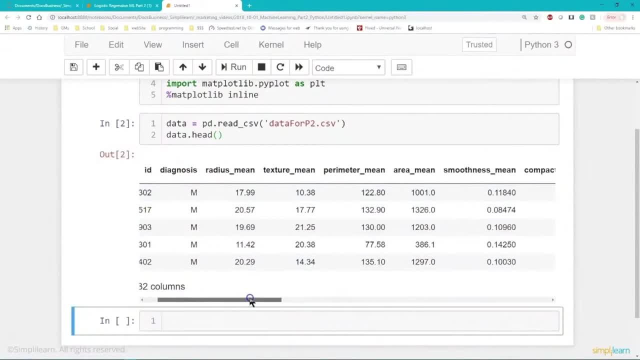 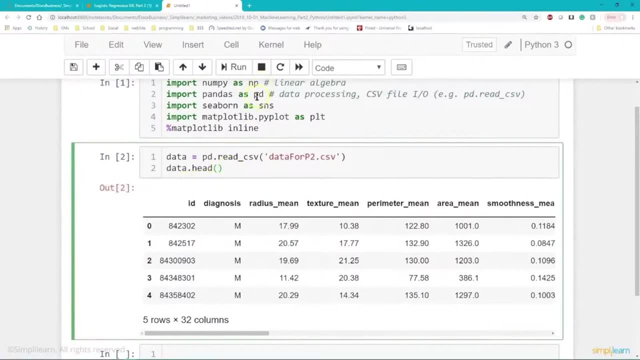 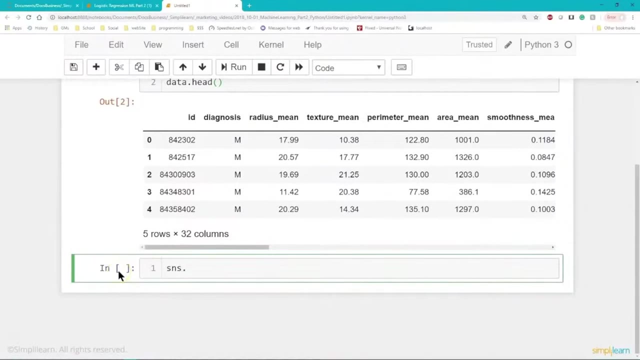 what we just looked at. We have an ID, we have a diagnosis. If we go all the way across, you'll see all the different columns coming across, displayed nicely for our data. And while we're exploring the data, our Seaborn, which we referenced as SNS. 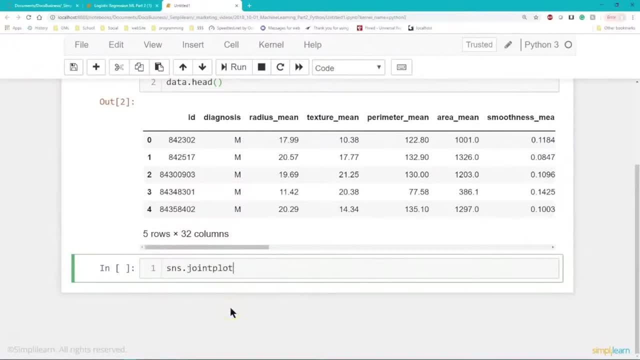 makes it very easy to go in here and do a joint plot. You'll notice very similar to, because it is sitting on top of the plot library. So the joint plot does a lot of work for us And we're just going to look at the first two. 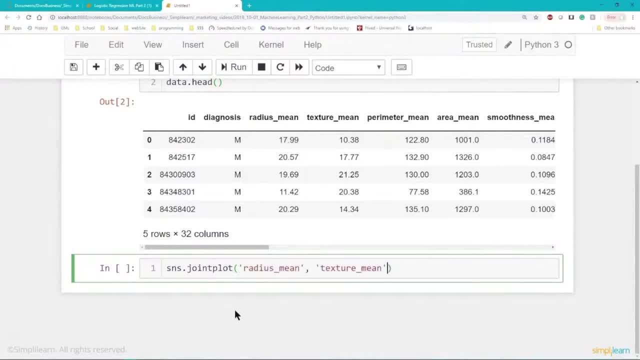 columns that we're interested in- The radius mean and the texture mean. We'll just look at those two columns And data equals data. So that tells us which two columns we're plotting And that we're going to use the data that we've. 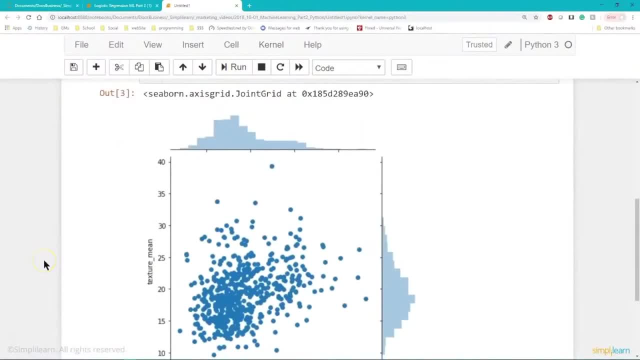 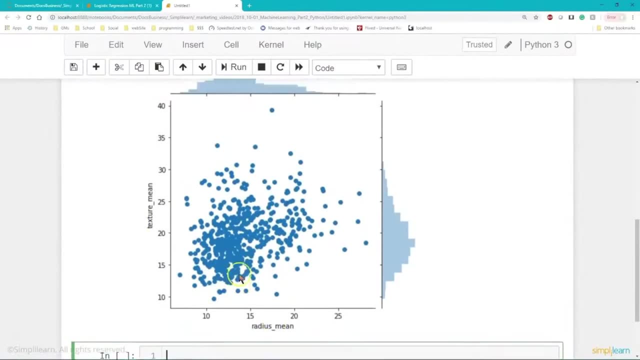 pulled in. Let's just run that And it generates a really nice graph on here And there's all kinds of cool things on this graph to look at. I mean, we have the texture, mean, and the radius mean, Obviously, the axes You can also. 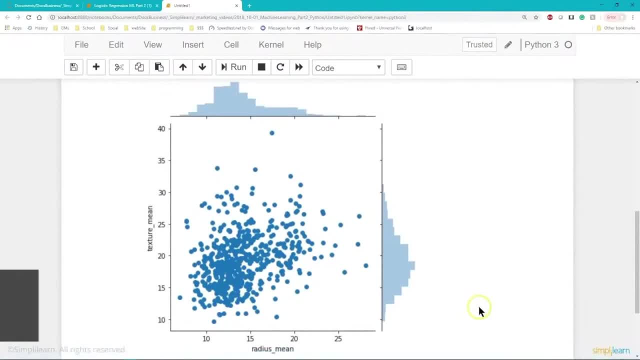 see, and one of the cool things on here is you can also see the histogram. They show that for the radius mean, Where does the most common radius mean come up and where the most common texture is. So we're looking at the on each growth. it's average. 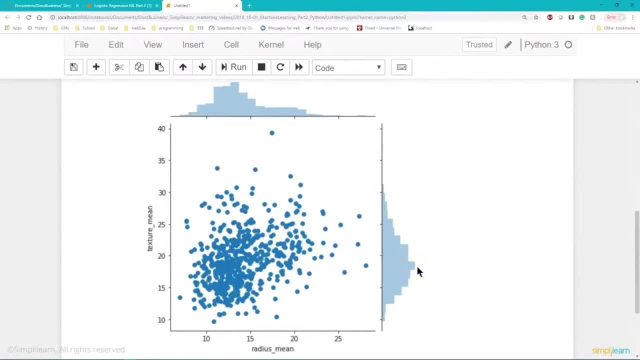 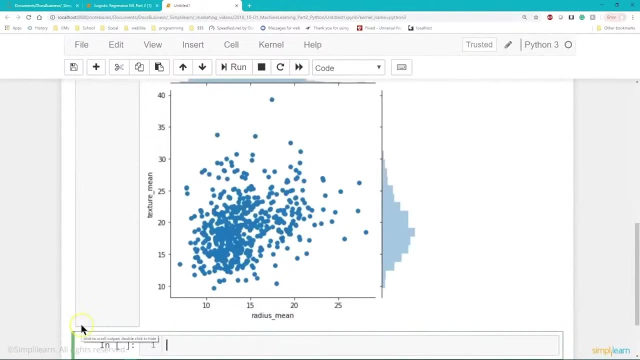 texture, and on each radius it's average radius. on there It gets a little confusing because we're talking about the individual object's average And then we can also look over here and see the histogram showing us the median or how common each measurement is, And that's. 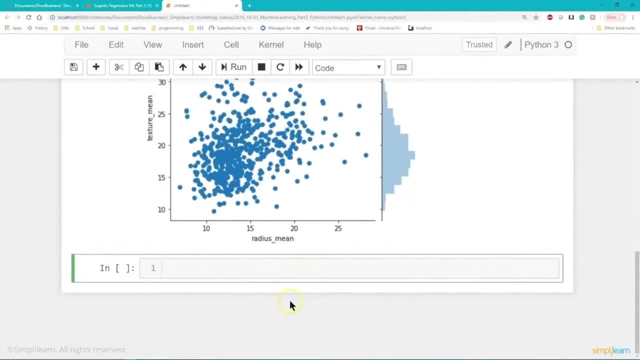 only two columns, So let's dig a little deeper into Seaborn. They also have a heat map, And if you're not familiar with heat maps, a heat map just means it's in color. That's all. that means Heat map. I guess the original ones were plotting heat. 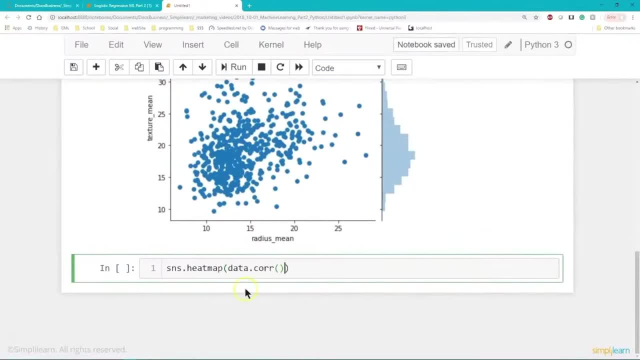 density on something, and so ever since then it's just called a heat map And we're going to take our data and get our corresponding numbers to put that into the heat map And that's simply datacorr for that. That's a pandas expression. 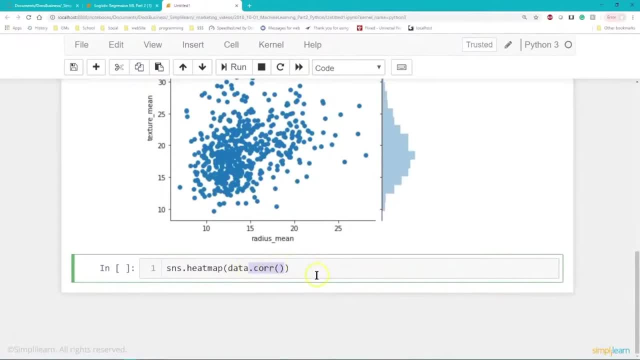 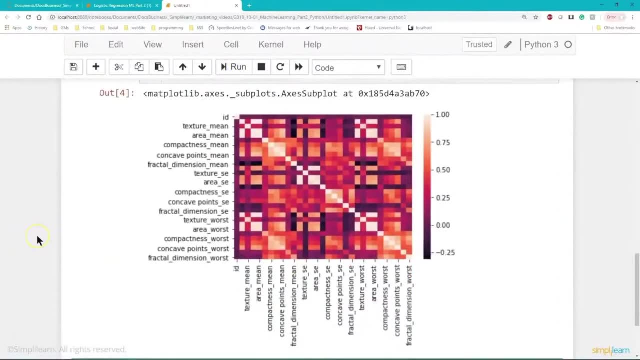 Remember we're working in a pandas data frame, So that's one of the cool tools in pandas for our data, And let's just pull that information into a heat map and see what that looks like And you'll see that we're now looking at all. 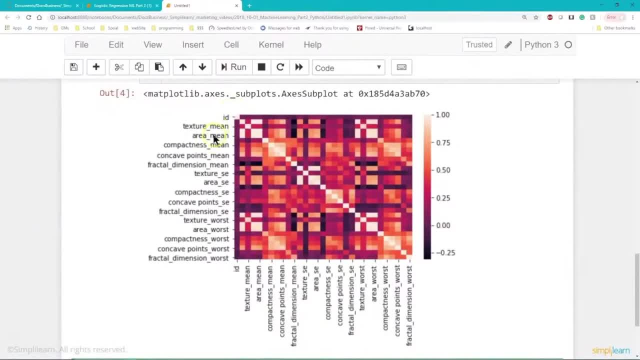 the different features. We have our ID, we have our texture, we have our area, our compactness, concave points, And if you look down the middle of this chart, diagonal, going from the upper left to bottom right, it's all white. 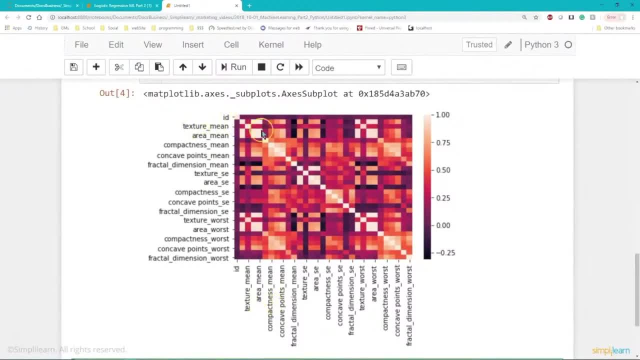 That's because when you compare texture to texture, they're identical, So they're 100%- or, in this case, a perfect one in their correspondence. And you'll see that when you look at say area or right below it, it has almost a black. 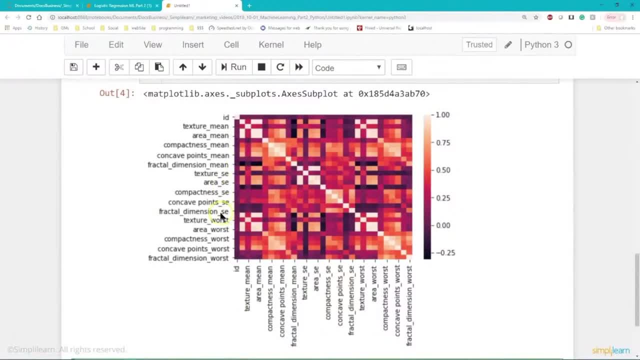 on there when you compare it to texture. So these have almost no corresponding data. They don't really form a linear graph or something that you can look at and say how connected they are. They're very scattered data. This is really just a really nice graph to get a quick. 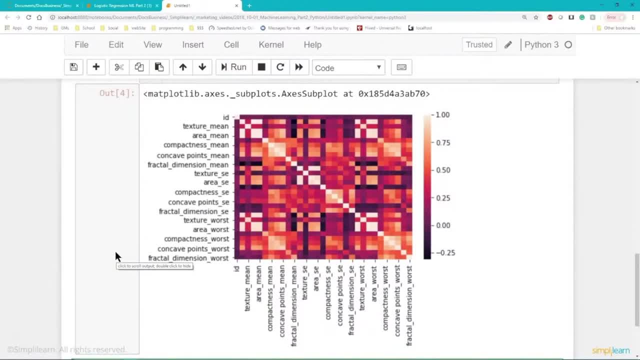 look at your data Doesn't so much change what you do, but it changes verifying. So when you get an answer or something like that, or you start looking at some of these individual pieces, you might go: hey, that doesn't match. according to. 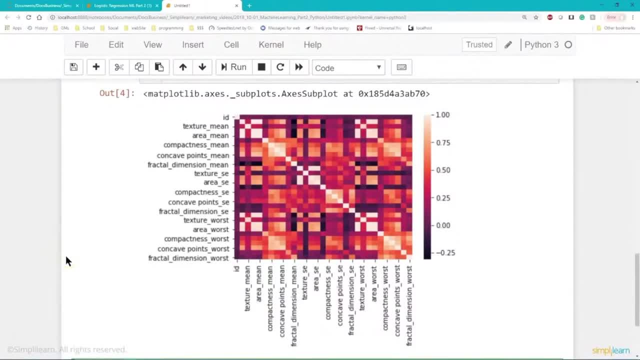 showing our heat map. this should not correlate with each other, And if it is, you're going to have to start thinking: well, why? What's going on? What else is coming in there? But it does show some really cool information on here. 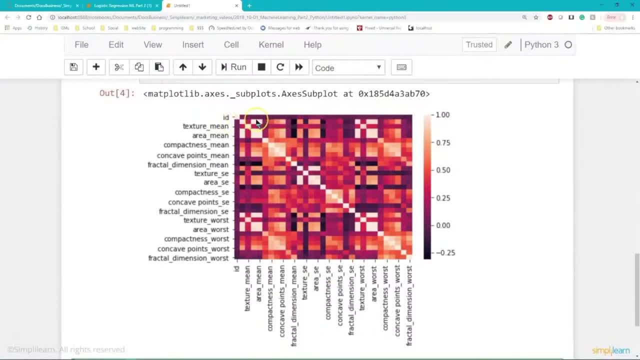 We can see from the ID. there's no real one feature that just says: if you go across the top line, that lights up. There's no one feature that says, hey, if the area is a certain size, then it's going to be. 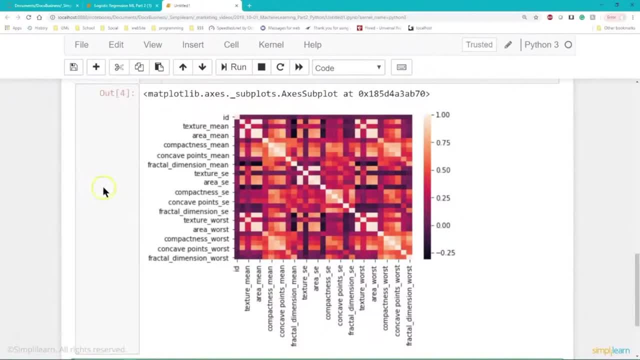 benign or malignant. It says there's some that sort of add up And that's a big hint in the data that we're trying to ID this, whether it's malignant or benign, That's a big hint to us as data scientists to go okay. 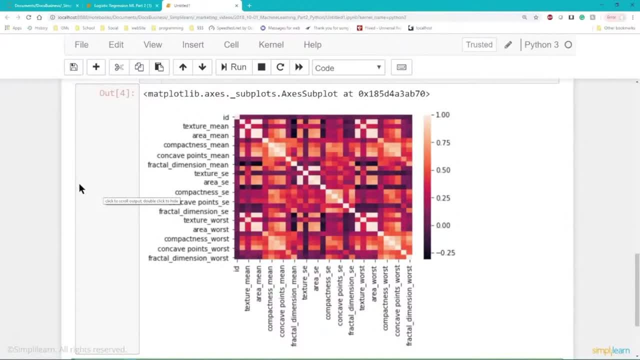 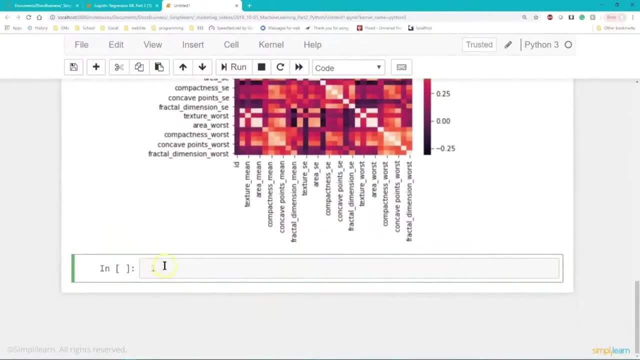 we can't solve this with any one feature. It's going to be something that includes all the features, or many of the different features, to come up with the solution for it. And while we're exploring the data, let's explore one more area and let's 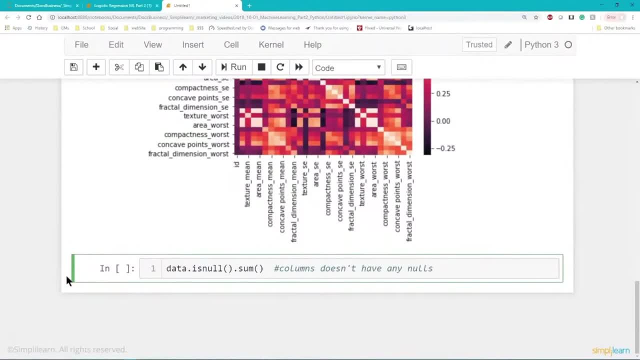 look at dataisNull. We want to check for null values in our data. If you remember from earlier in this tutorial we did it a little differently, where we added stuff up and summed them up. You can actually, with pandas, do it really. 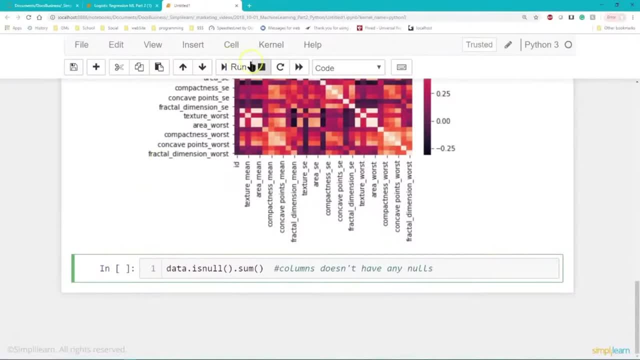 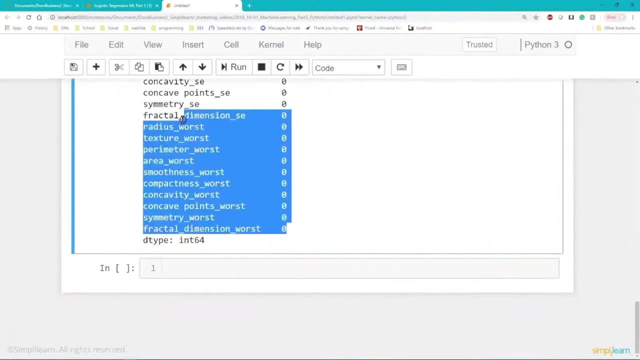 quickly: dataisNull and summit and it's going to go across all the columns. So when I run this, you're going to see all the columns come up with no null data. So we've just just to rehash these last few. 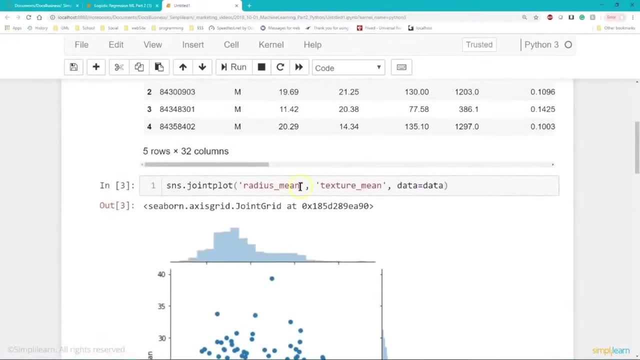 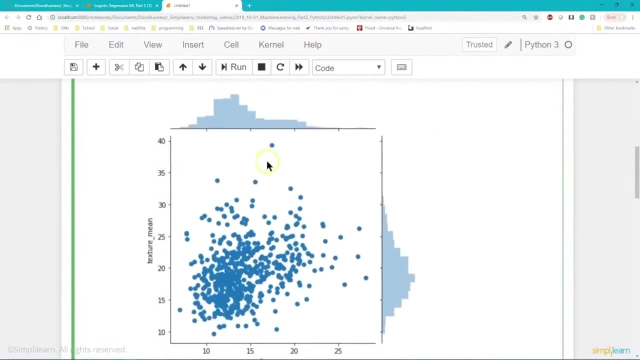 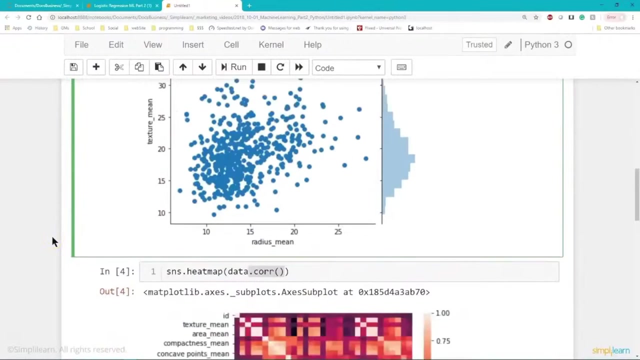 steps. we've done a lot of exploration. We have looked at the first two columns and seen how they plot with the seaborn, with the joint plot which shows both the histogram and the data plotted on the bicoordinates, And obviously you can do that more in detail. 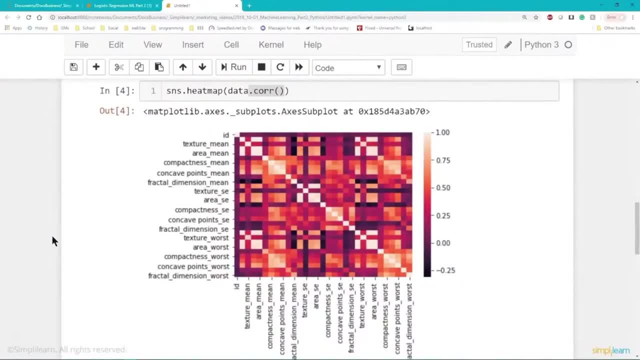 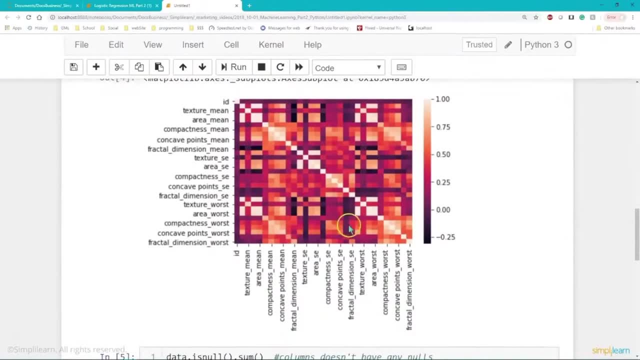 with different columns and see how they plot together. And then we took and did the seaborn heatmap, the snsheatmap of the data, And you can see right here where it did a nice job, showing us some bright spots where stuff correlates with each other and forms. 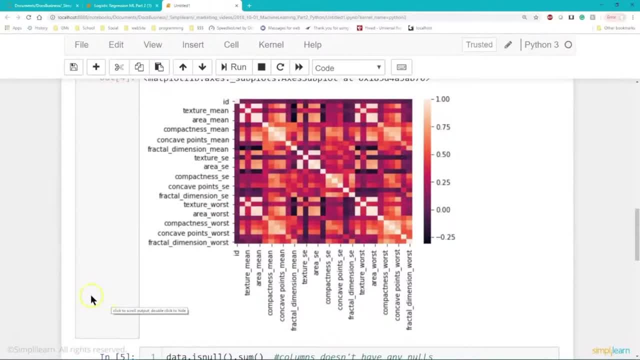 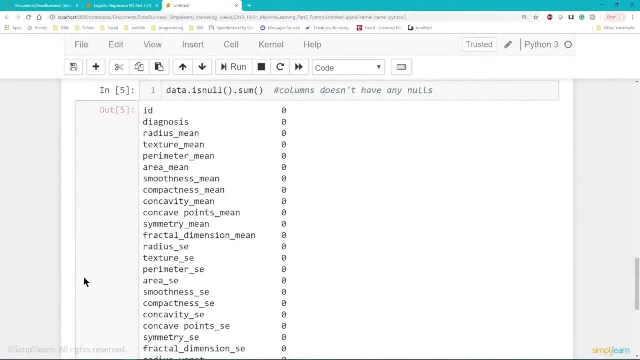 a very nice combination or points of scattering points, And you can also see areas that don't. And then, finally, we went ahead and checked the data. Is the data a null value? Do we have any missing data in there? Very important step, because it'll crash later. 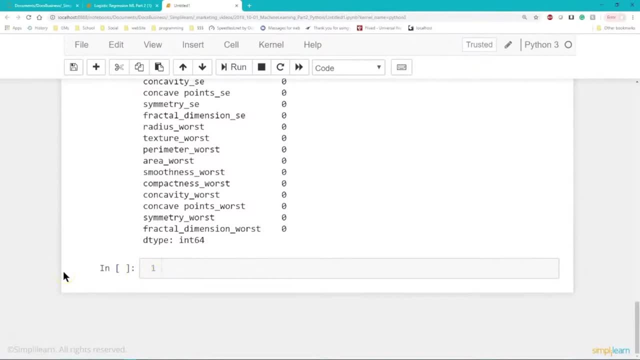 on. If you forget to do this step, it will remind you when you get that nice error code that says null values. Okay, So not a big deal if you miss it, but it's no fun having to go back when you're in a huge process and you've 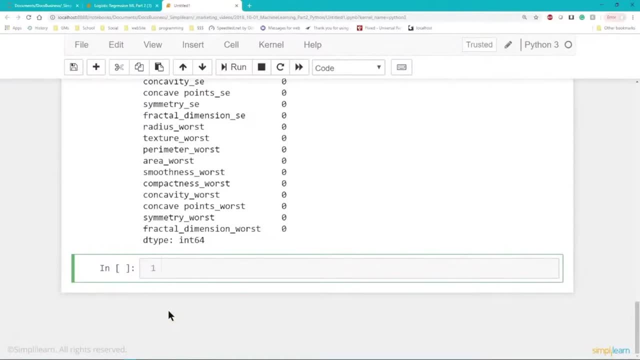 missed this step and now you're ten steps later and you gotta go remember where you were pulling the data in. So we need to go ahead and pull out our x and our y. So we just put that down here And we'll set the x equal to. 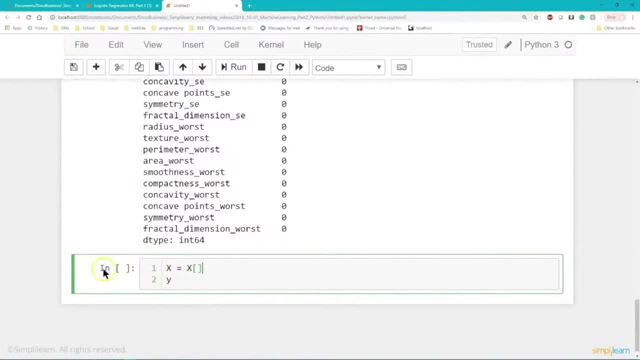 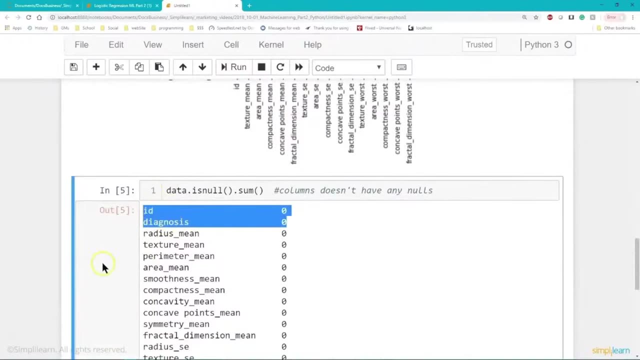 and there's a lot of different options here. Certainly we could do: x equals all the columns except for the first two, Because, if you remember, the first two is the ID and the diagnosis. So that certainly would be an option. But what we're gonna do is we're actually gonna 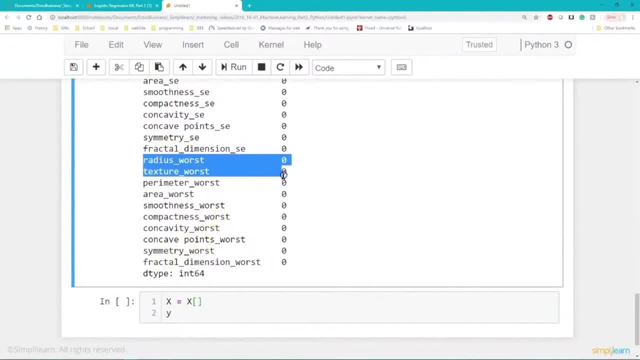 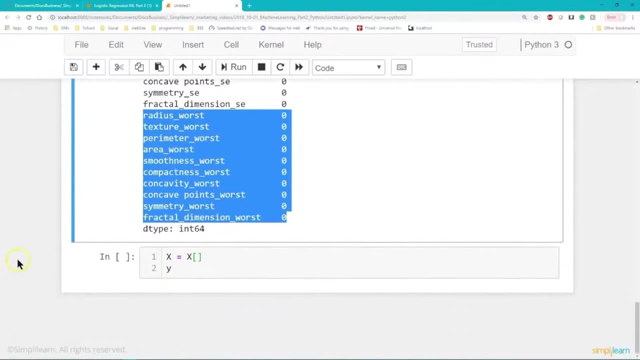 focus on the worst: The worst radius, the worst texture, parameter area, smoothness, compactness and so on. One of the reasons to start dividing your data up when you're looking at this information is sometimes the data will be the same data coming. 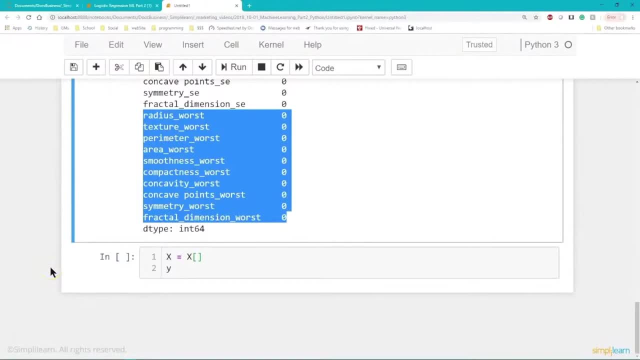 in. So if I have two measurements coming in to my model, it might overweigh them. It might overpower the other measurements because it's basically taking that information in twice. That's a little bit past the scope of this tutorial. What I want you to take. 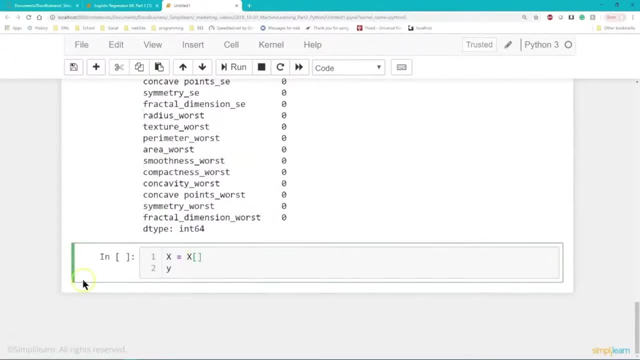 away from this, though, is that we are dividing the data up into pieces, and our team in the back went ahead and said: hey, let's just look at the worst. So I'm gonna create an array, and you'll see this array: Radius worst. 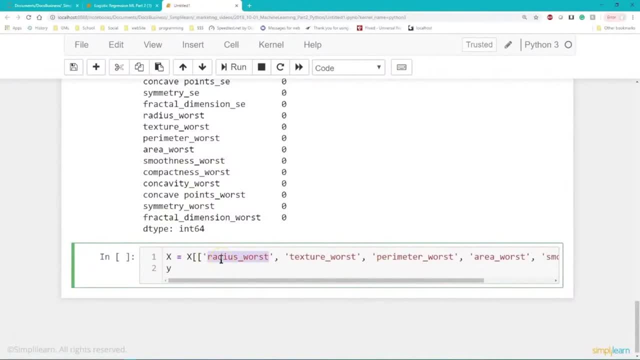 texture worst, perimeter: worst. We've just taken the worst of the worst and I'm just gonna put that in my x. So this x is still a panda's data frame, but it's just those columns, And our y, if you remember correctly, is gonna. 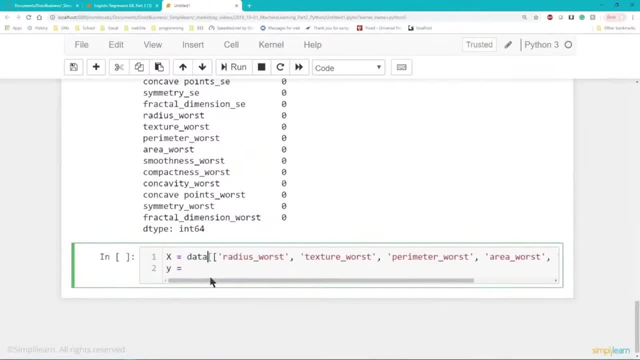 be. oops, hold on one second. it's not x, it's data. There we go, So x equals data, and then it's a list of the different columns. the worst of the worst. And if we're gonna take that, then we have to have our answer for. 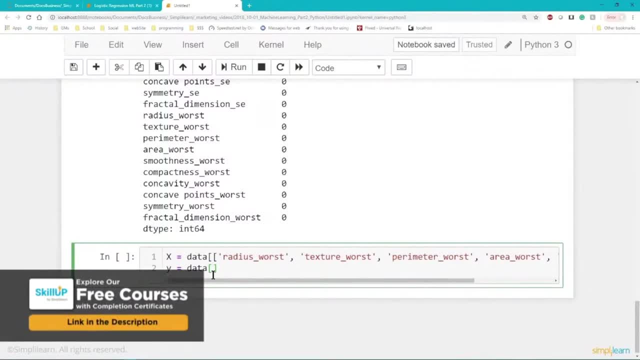 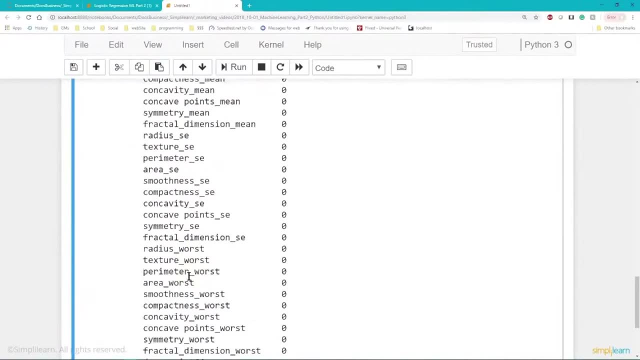 our y for the stuff we know And, if you remember correctly, we're just gonna be looking at the diagnosis. That's all we care about is: what is it diagnosed? Is it benign or malignant? And since it's a single column, we can just do diagnosis. 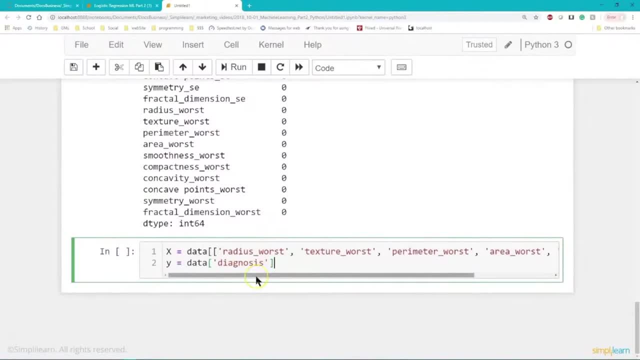 Oh, I forgot to put the brackets. there we go, Okay. So it's just diagnosis on there, And we can also real quickly do like xhead. if you wanna see what that looks like, And yhead And run this And you'll see. 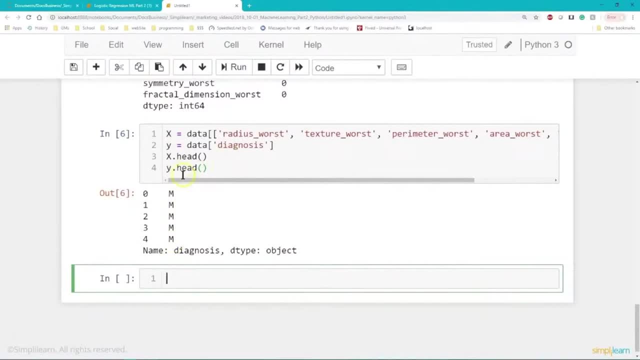 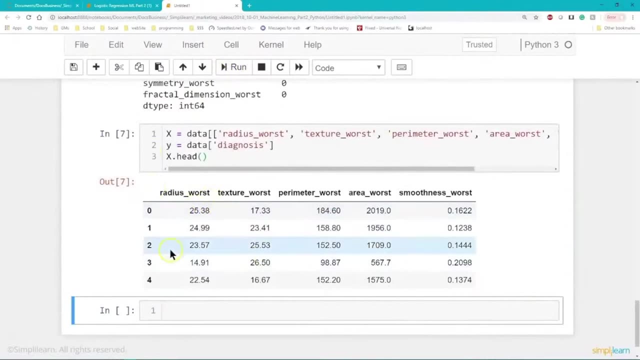 it only does the last one. I forgot about that. if you don't do print, You can see that the yhead is just mmm, because the first ones are all malignant And if I run this, the xhead is just the first five. 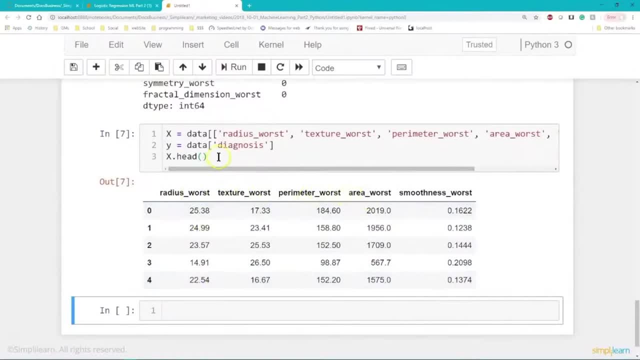 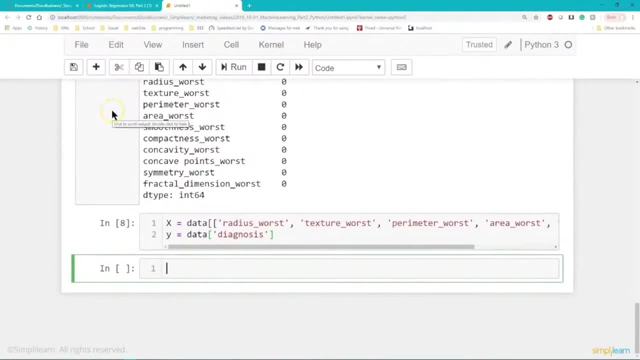 values of radius worst, texture, worst parameter, worst area worst, and so on. I'll go ahead and take that out. So, moving down to the next step, we've built our two data sets, our answer and then the features we wanna. 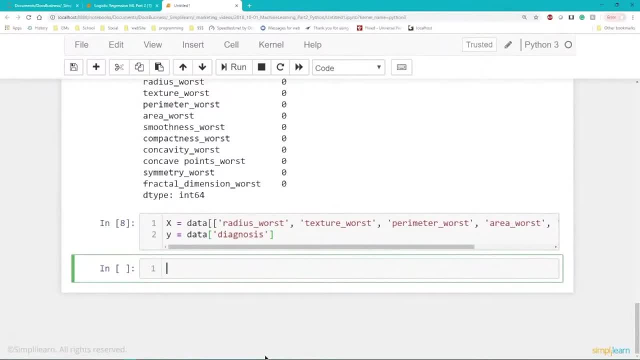 look at. In data science it's very important to test your model. So we do that by splitting the data And from sklearn model selection we're gonna import train test split. So we're gonna split it into two groups. There are so many ways to do this. 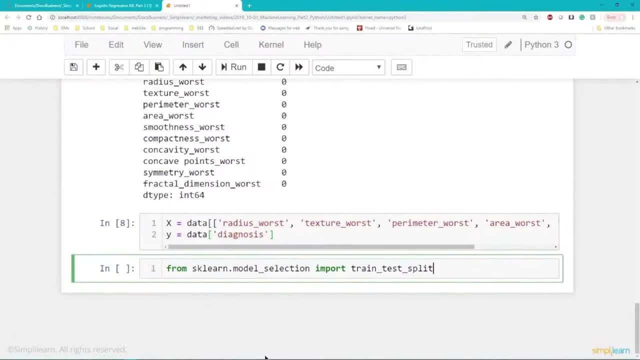 I noticed in one of the more modern ways to actually split it into three groups and then you model each group and test it against the other groups. So you have all kinds of and there's reasons for that, which is past the scope of this. 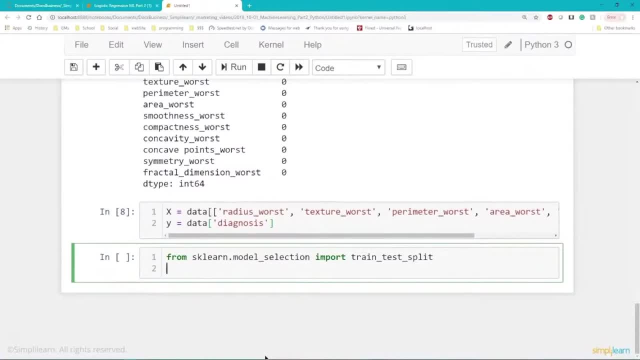 And for this particular example, it isn't necessary For this. we're just gonna split it into two groups: one to train our data and one to test our data And the sklearn dot model selection. we have train test split. You can write your own quick code to do this. 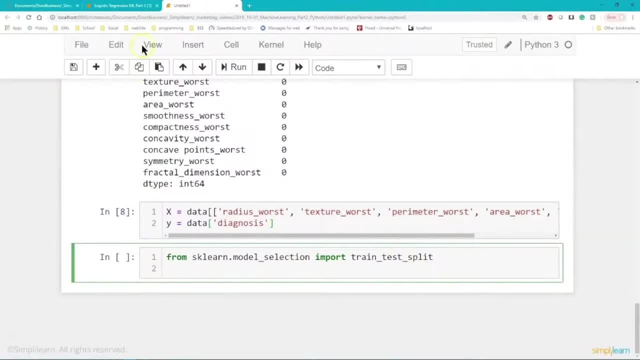 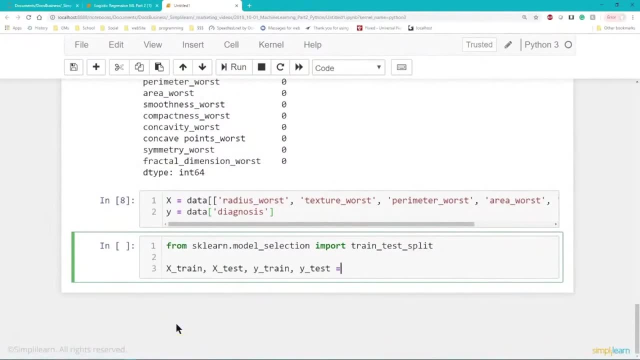 We just randomly divide the data up into two groups, But they do it for us nicely And we actually can- almost we can actually do it in one statement with this, where we're gonna generate four variables: capital X, train, capital X- test. 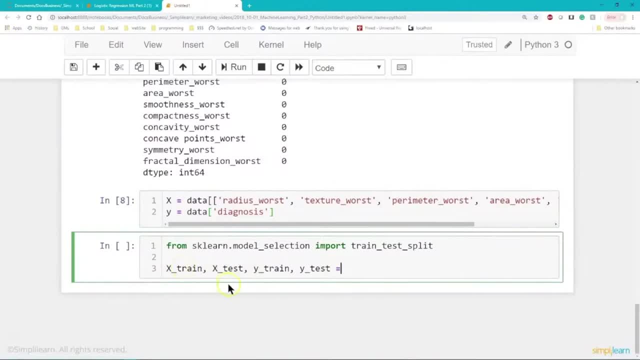 so we have our training data we're gonna use to fit the model, and then we need something to test it. And then we have our Y train, so we're gonna train the answer and then we have our test. So this is the stuff. we wanna see how good it did. 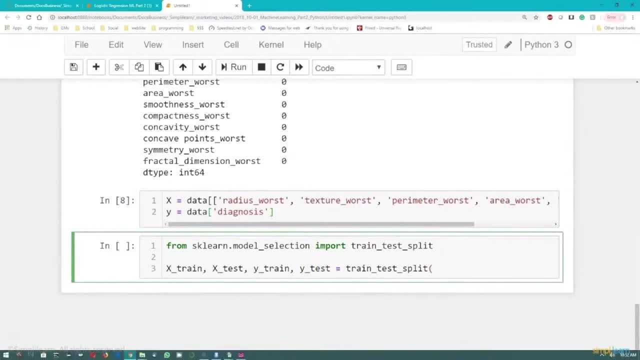 on our model And we'll go ahead and take our train test split that we just imported and we're gonna do X and our Y, our two different data- that's going in for our split. And then the guys in the back came up and wanted us to go ahead and use a test size. 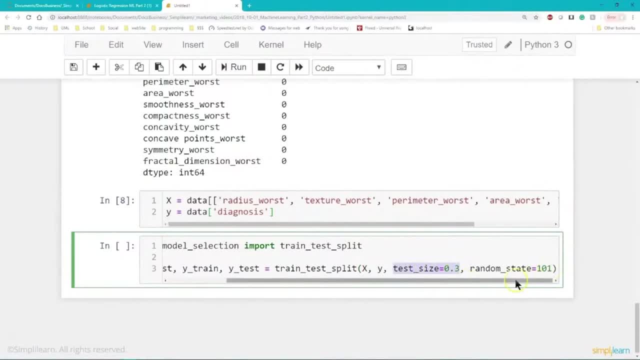 equals .3.. It's always nice to kind of switch your random state around, but not that important. What this means is that the test size is: we're gonna take 30% of the data and we're gonna put that into our test variables, our Y test. 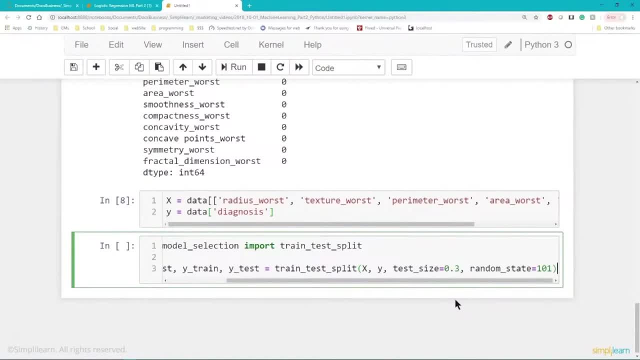 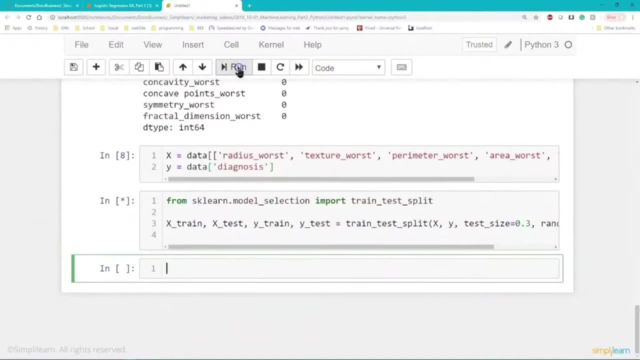 and our X test And we're gonna do 70% into the X train and the Y train. So we're gonna use 70% of the data to train our model and 30% to test it. Let's go ahead and run that. 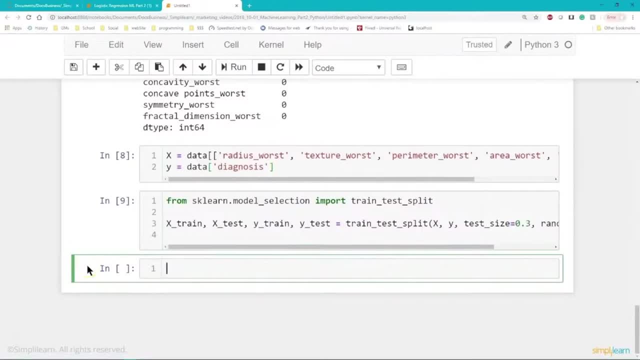 and load those up. So now we have all our stuff split up and our data ready to go. Now we get to the actual logistics part. We're actually gonna create our model, So let's go ahead and bring that in from sklearn. We're gonna bring in our. 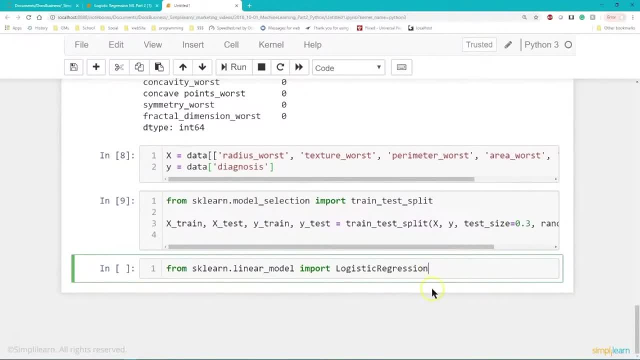 linear model and we're gonna import logistic regression. That's the actual model we're using. We'll call it log model And let's just set this equal to our logistic regression that we just imported. So now we have a variable log model set to that class for us to use. 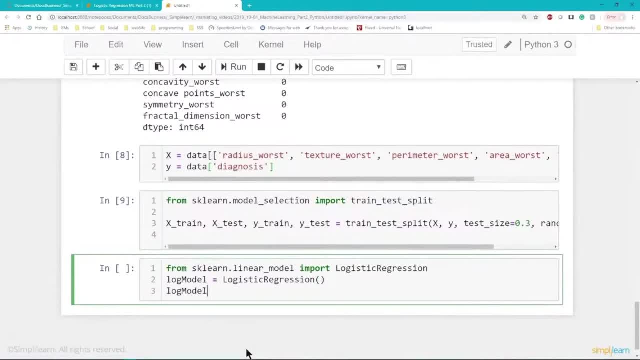 And with most the models in the sklearn. we just need to go ahead and fix it Fit, Do a fit on there And we use our X train and we separate it out with our Y train. Now let's go ahead and run this. 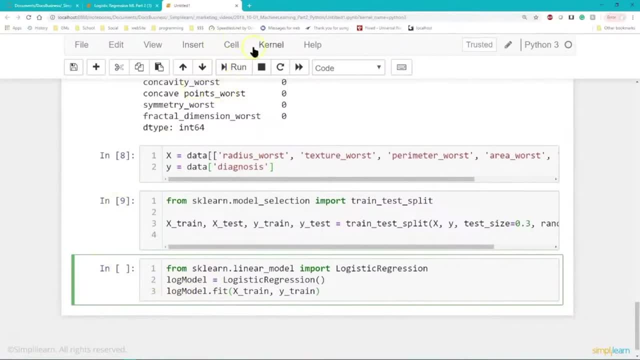 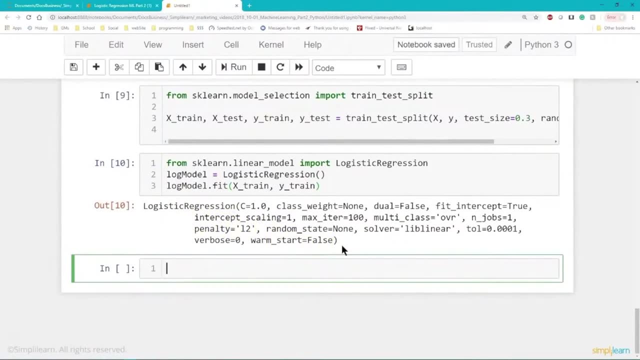 So once we've run this, we'll have a model that fits this data, That 70% of our training data, And of course, it prints this out. that tells us all the different variables that you can set on there. There's a lot of different choices you can make. 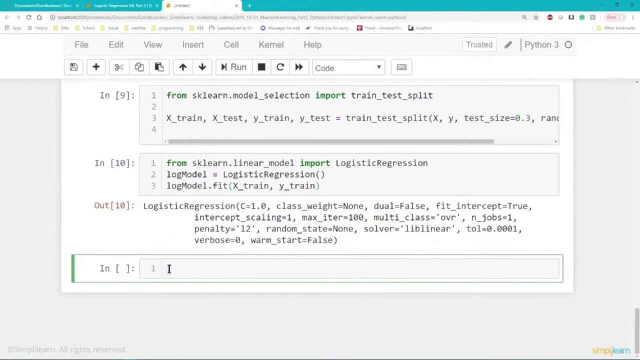 We'll let all the defaults sit. We don't really need to mess with those. on this particular example, There's nothing in here that really stands out as super important until you start fine tuning it. But for what we're doing, the basics will work just fine. 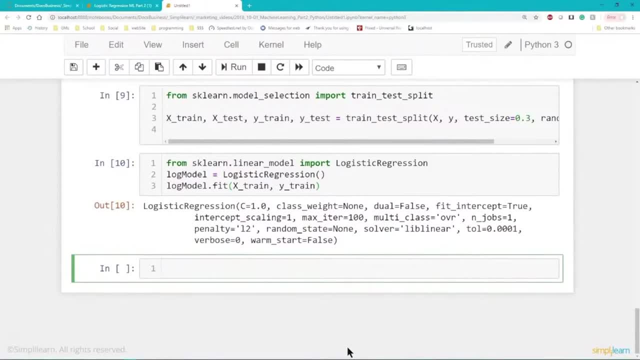 And then we need to go ahead and test out our model. Is it working? So let's create a variable, Y, predict, And this is gonna be equal to our log model And we want to do a predict Again. very standard format for the sklearn library. 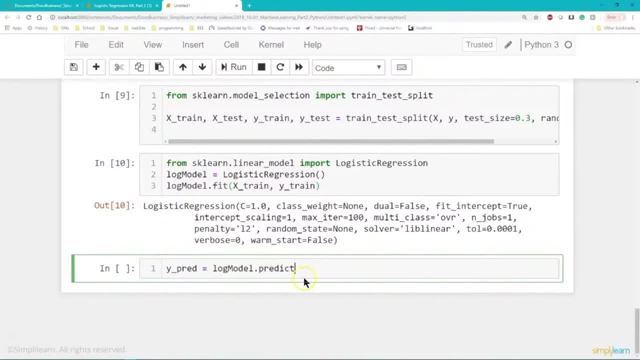 is taking your model and doing a predict on it And we're gonna test Y predict against the Y test. So we want to know what the model thinks it's gonna be. That's what our Y predict is And with that we want the. 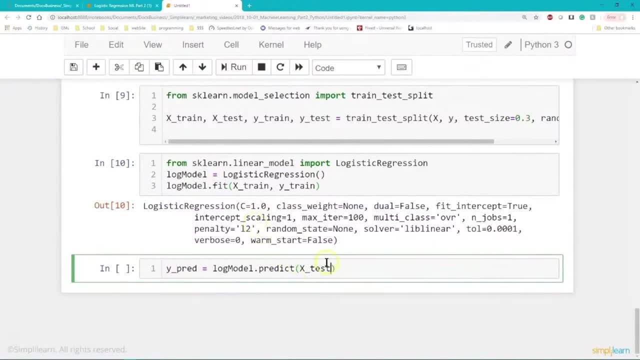 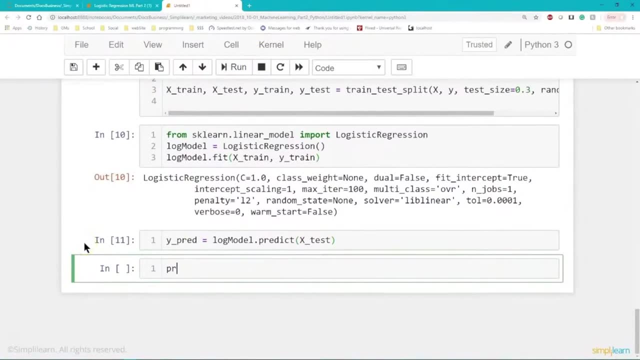 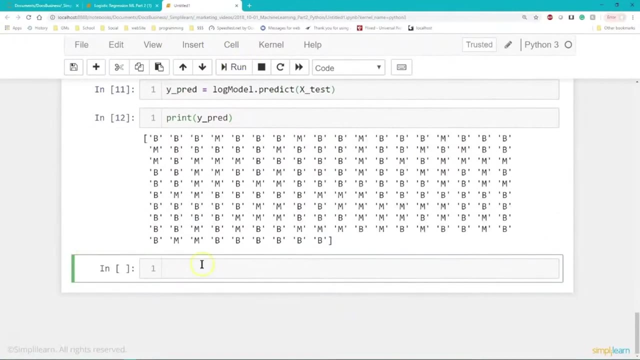 capital X, X test. So we have our train set and our test set And now we're gonna do our Y predict And let's go ahead and run that. And if we print Y predict, Go ahead and run that And it comes up and it. 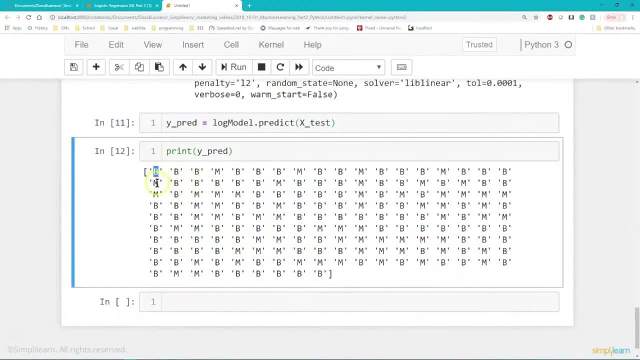 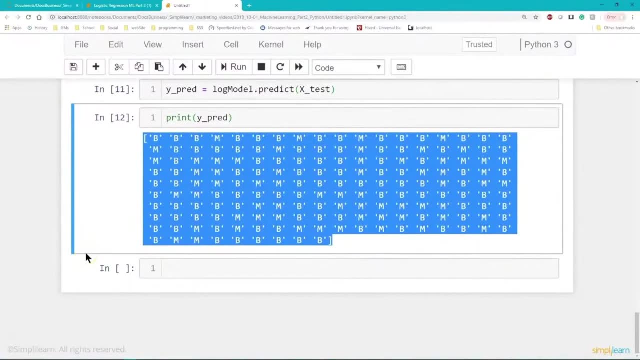 prints a nice array of B and M for benign and malignant, For all the different test data we put in there. So it does pretty good. We're not sure exactly how good it does, But we can see that it actually works and is functional. 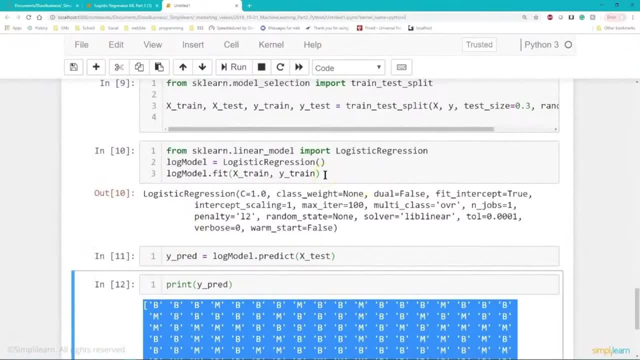 It was very easy to create. You'll always discover with our data science that as you explore this, you spend a significant amount of time prepping your data And making sure your data coming in is good. There's a saying: good data in good answers out. 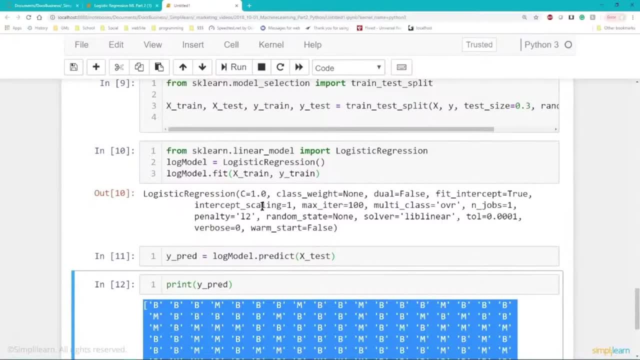 Bad data in bad answers out. That's only half the thing. That's only half of it. Selecting your models becomes the next part, as far as how good your models are, And then, of course, fine tuning it depending on what model you're using. 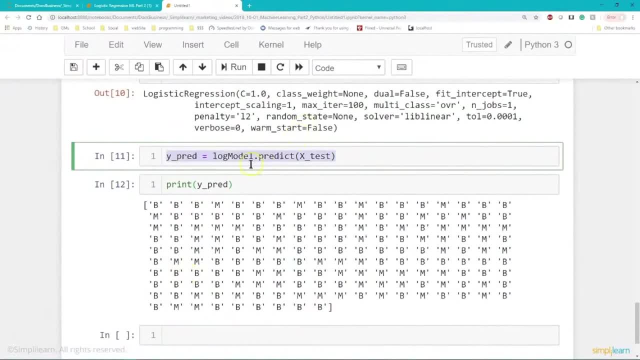 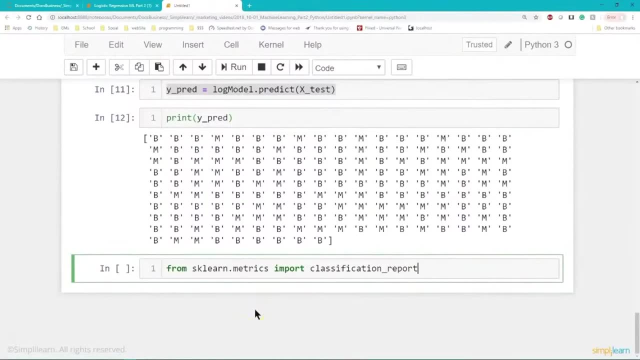 So we come in here, We want to know how good this came out. So we have our Y predict here, Log model, dot predict, X test. So for deciding how good our model is, We're going to go from the sklearn dot metrics, We're going to import. 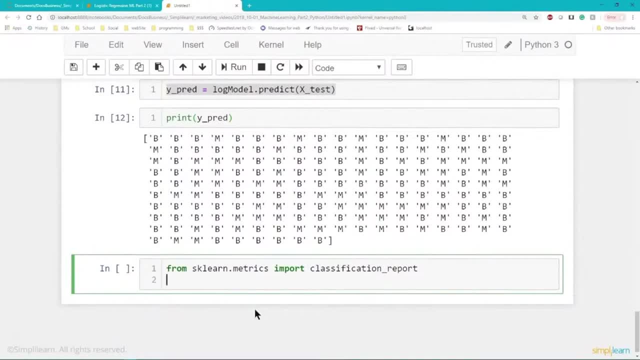 classification report And that just reports how good our model is doing, And then we're going to feed it the model data And let's just print this out And we'll take our classification report And we're going to put into there our test, Our actual 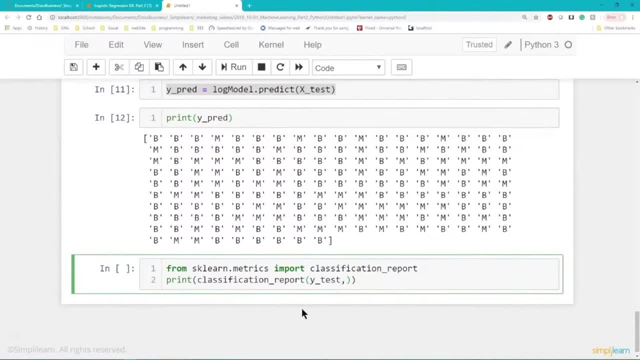 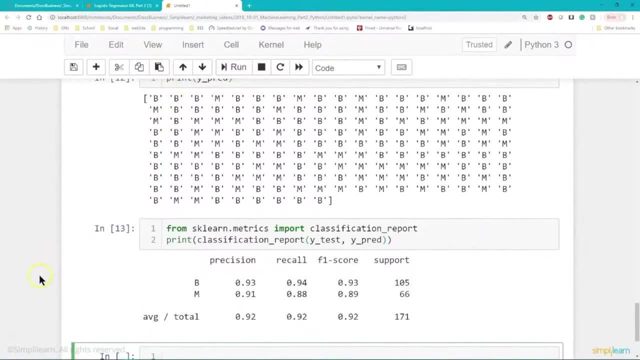 data. So this is what we actually know is true And our prediction, What our model predicted for that data on the test side. And let's run that and see what that does. So we pull that up, You'll see that we have a precision. 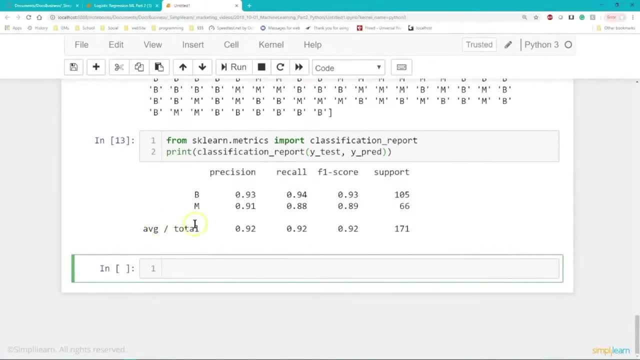 for B9 and malignant B and M, And we have a precision of 93 and 91. A total of 92. So it's kind of the average between these two: 92. There's all kinds of different information on here. Your F1 score. 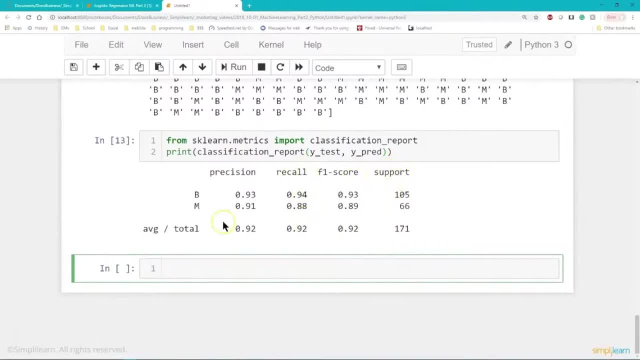 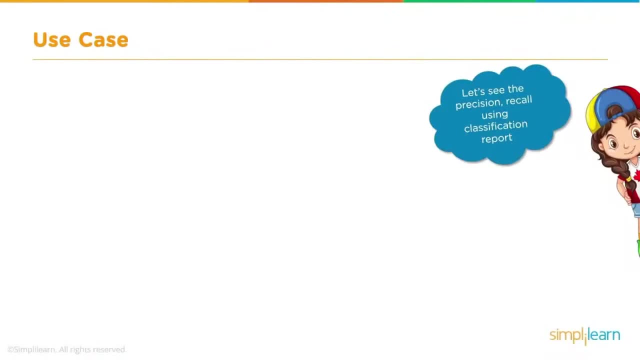 Your recall, Your support coming through on this, And for this I'll go ahead and just flip back to our guides that they put together for describing it. And so here we're going to look at the precision using the classification report, And you'll see, this is the same printout I had. 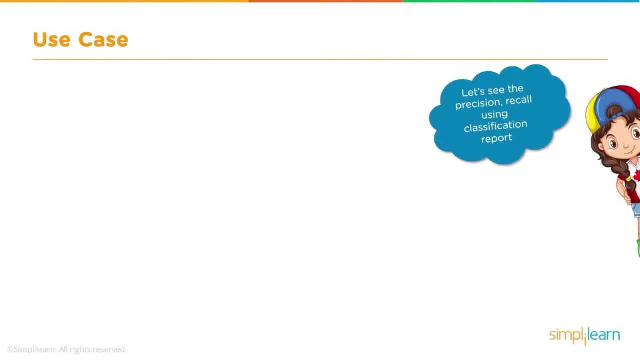 up above. Some of the numbers might be different because it does randomly pick out which data we're using. So this model is able to predict the type of tumor with 91 percent accuracy. So we look back here. You'll see where we have B9 and malignant. 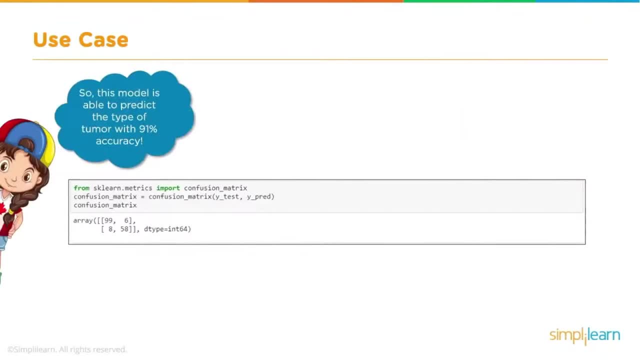 It actually is 92 coming up here. We're looking at about a 92, 91 percent precision And remember I reminded you about domain. So we're talking about the domain of a medical domain with a very catastrophic outcome, You know, at 91 or 92 percent. 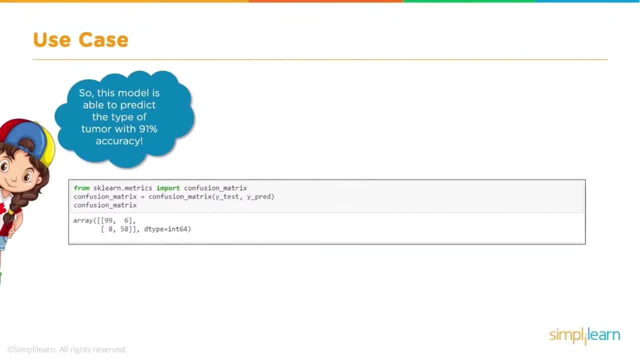 precision, you're still going to go in there and have somebody do a biopsy on it. Very different than if you're investing money and there's a 92 percent chance you're going to earn 10 percent and 8 percent chance you're going to lose 8 percent. 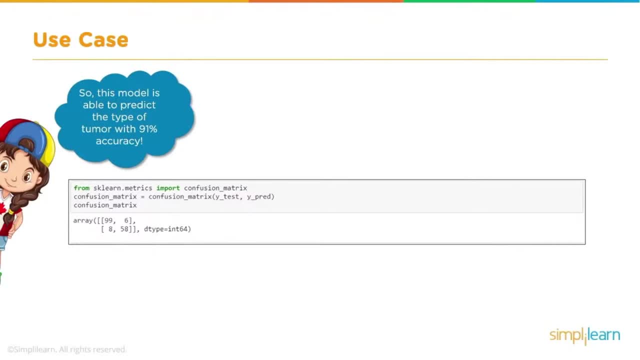 You're probably going to bet the money Because at that odds it's pretty good that you'll make some money And in the long run, if you do that enough, you definitely will make money. And also with this domain, I've actually seen them use this to identify different forms. 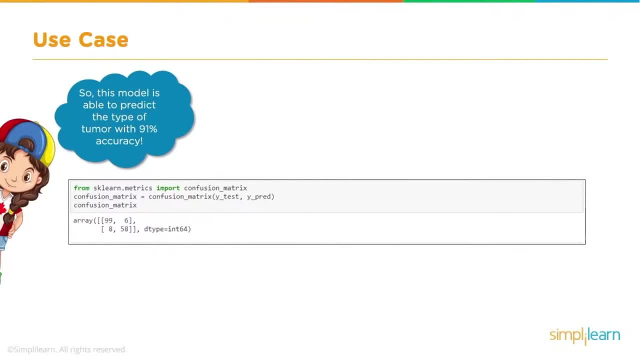 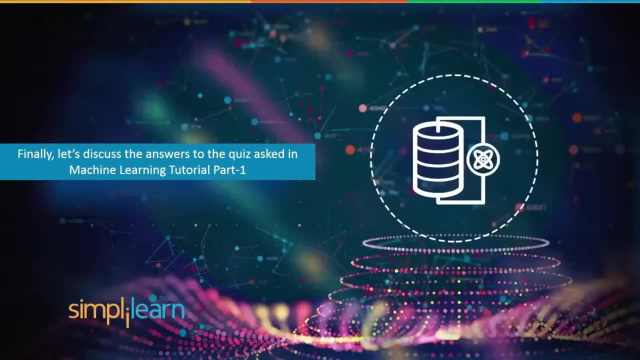 of cancer. That's one of the things that they're starting to use these models for, Because then it helps the doctor know what to investigate. So that wraps up this section. We're finally, we're going to go in there and let's discuss the answer to the. 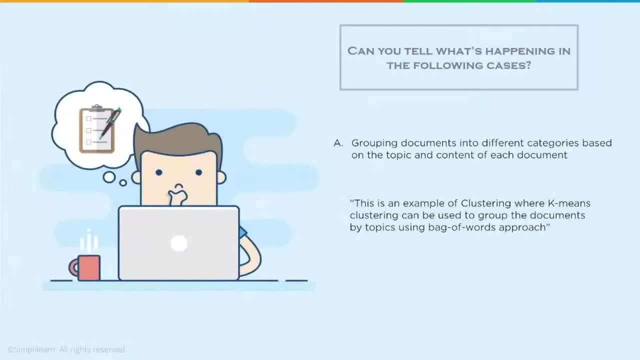 quiz asked in Machine Learning Tutorial, Part 1.. Can you tell what's happening in the following cases? Grouping documents into different categories based on the topic and content of each document. This is an example of clustering, where k-means clustering can be used. 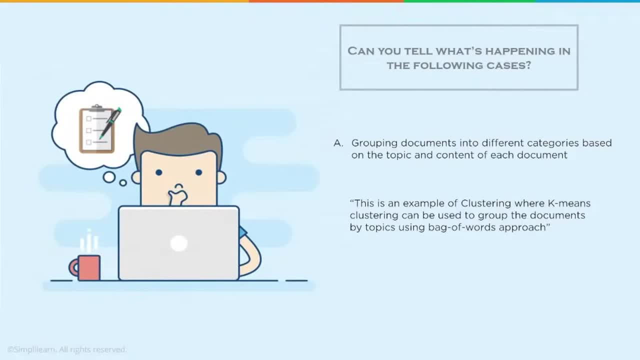 to group the documents by topics using bag of words approach. So if you've gotten in there that you're looking for clustering- and hopefully you had at least one or two examples like k-means that are used for clustering different things- then give yourself a two. 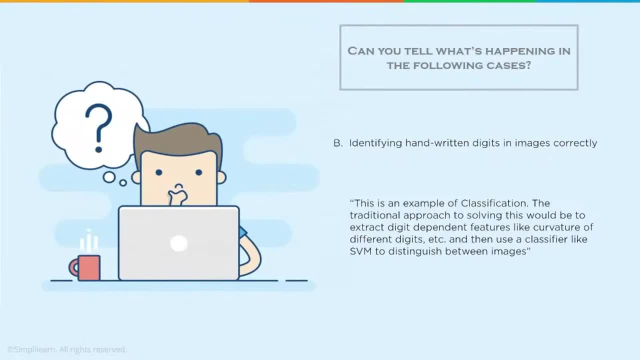 thumbs up B- Identifying handwritten digits in images correctly. This is an example of classification. The traditional approach to solving this would be to extract digit dependent features like curvature of different digits etc. and then use a classifier like SVM to distinguish between images. 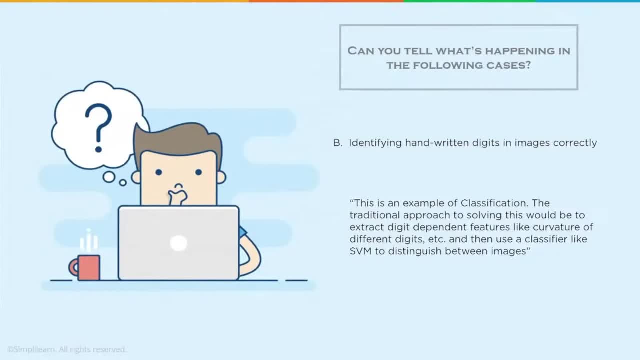 Again, if you got the fact that it's a classification example, give yourself a thumb up, and if you're able to go, hey, let's use SVM or another model for this, give yourself those two thumbs up on it. C: Behavior of a website indicating that the site is not working as 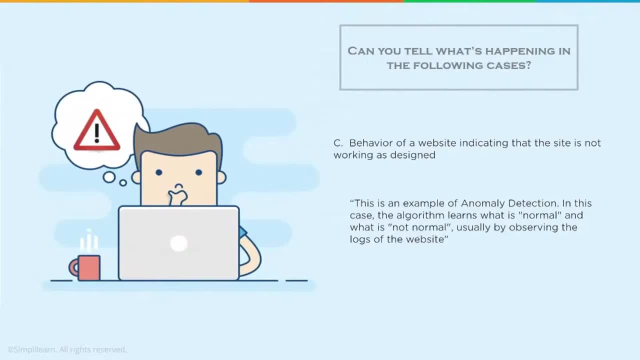 designed. This is an example of anomaly detection. In this case, the algorithm learns what is normal and what is not normal, usually by observing the logs or the website. Give yourself a thumbs up if you got that one, And just for a bonus. can you think of another example of? 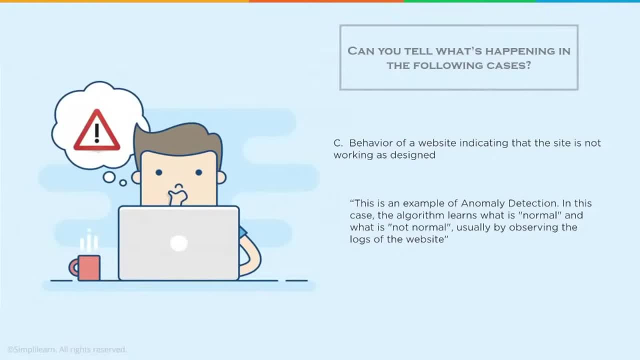 anomaly detection. One of the ones I use it for in my own business is detecting anomalies in stock markets. Stock markets are very fickled and they behave very radical, So finding those erratic areas and then finding ways to track down why they're erratic Was something released in social 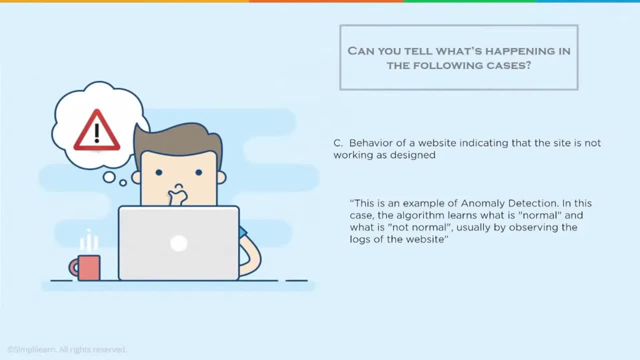 media Was something released. You can see where knowing where that anomaly is can help you to figure out what the answer is to it. in another area D, Predicting salary of an individual based on his or her years of experience. This is an example of regression. 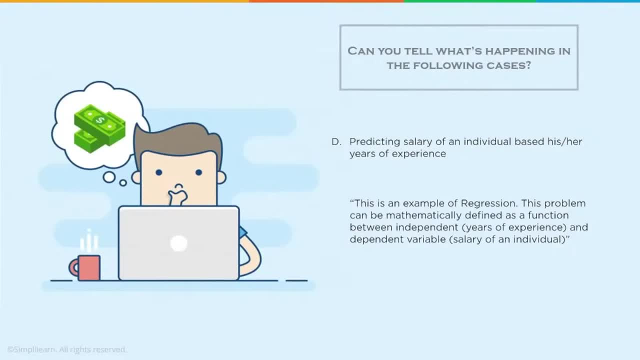 This problem can be mathematically defined as a function between independent years of experience and dependent variables- salary of an individual. And if you guessed that this was a regression model, give yourself a thumbs up. And if you're able to remember that it is between independent and dependent, 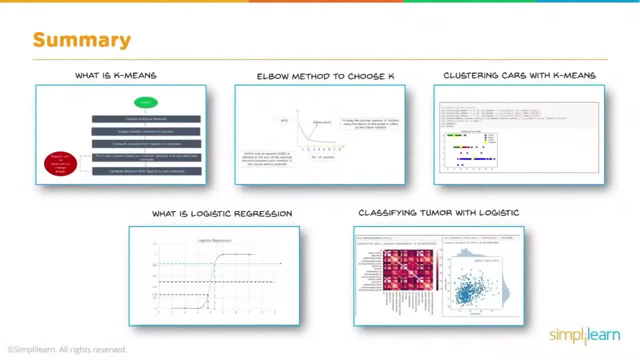 variables and that terms. give yourself two thumbs up Summary. So to wrap it up, we went over what is k means And we went through also the chart of choosing your elbow method and assigning a random centroid to the clusters, Computing the distance and then going in there. 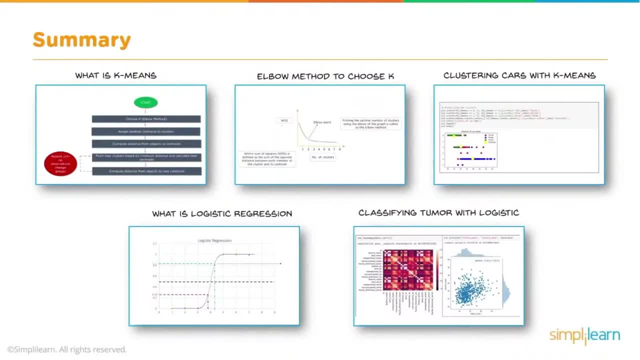 and figuring out what the minimum centroid is and computing the distance and going through that loop until it gets the perfect centroid. And we looked into the elbow method to choose k, based on running our clusters across a number of variables and finding the best location for that. 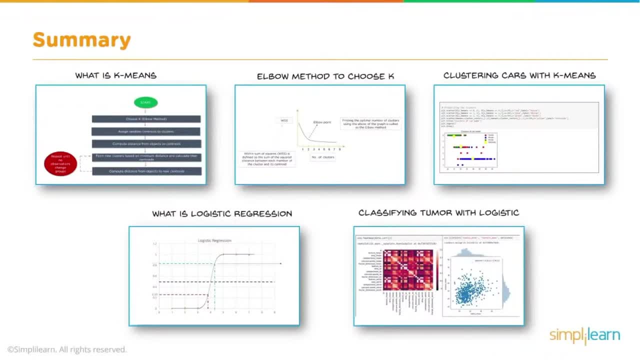 We did a nice example of clustering cars with k means, even though we only looked at the first two columns. to make it simple and easy to graph, You can easily extrapolate that and look at all the different columns and see how they all fit together. And we looked at what is. 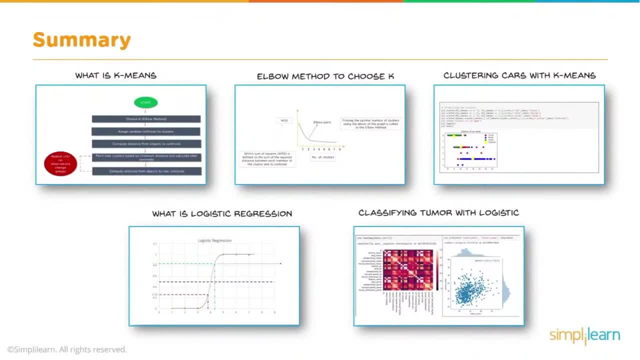 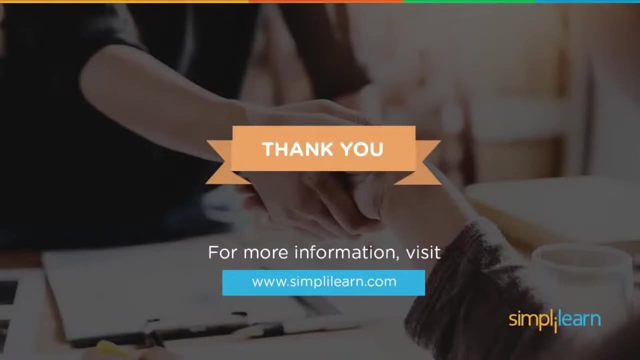 logistic regression. We discussed the sigmoid function- What is logistic regression? And then we went into an example of classifying tumors with logistics. I hope you enjoyed part two of machine learning. Thank you for joining us today. For more information, visit wwwsimplylearncom. 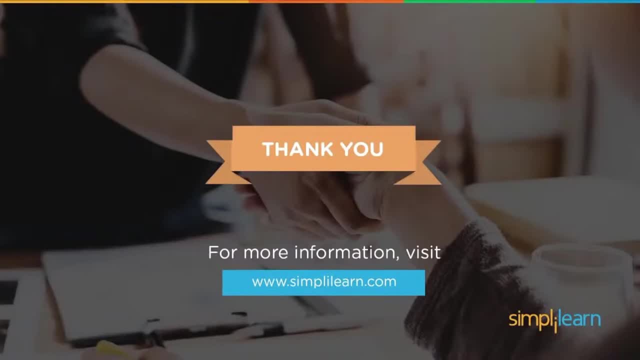 Again. my name is Richard Kirschner, a member of the SimplyLearn team. Get certified, Get ahead. If you have any questions or comments, feel free to write those down below the YouTube video or visit us at simplylearncom. We'll be happy to supply you with the data. 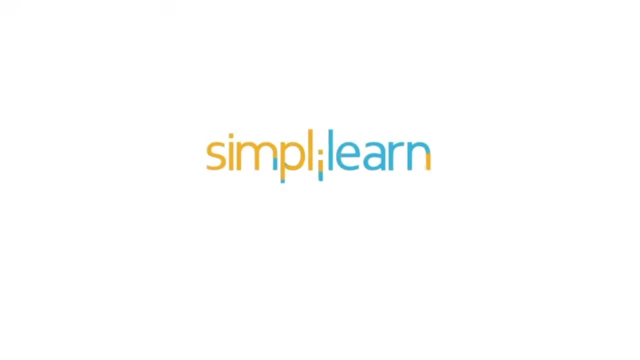 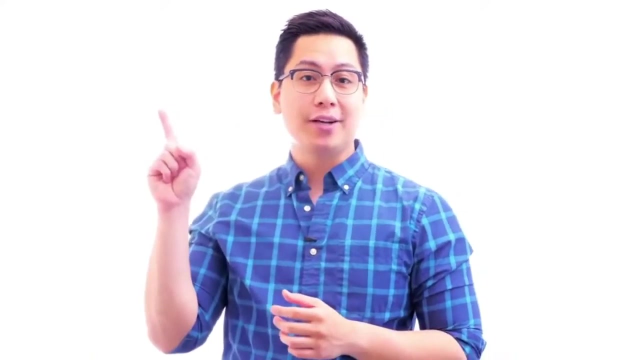 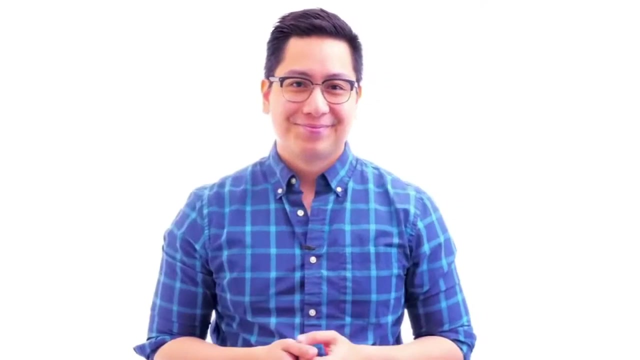 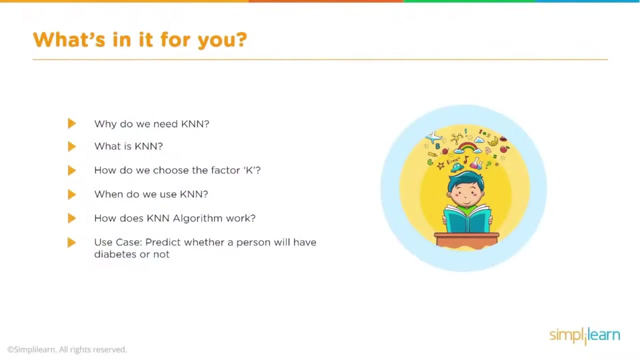 sets or other information as requested. Today we're going to cover the k-nearest neighbors, a lot referred to as k-n-n, And k-n-n is really a fundamental place to start in the machine learning. It's a basis of a lot of other things and just the logic. 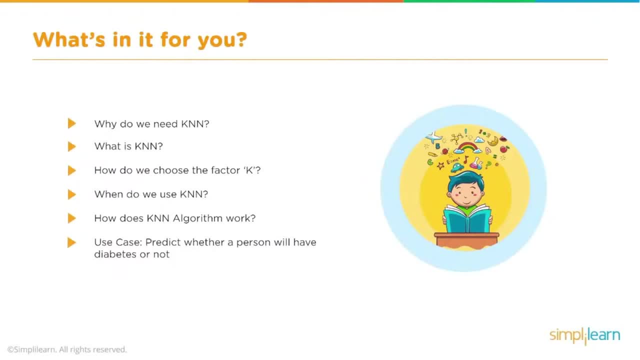 behind. it is easy to understand and incorporate it in other forms of machine learning. So, today, what's in it for you? Why do we need k-n-n? What is k-n-n? How do we choose the factor k? When do we use k-n-n? 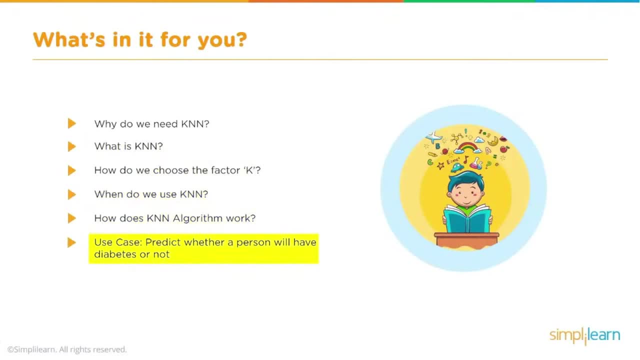 How does k-n-n algorithm work? And then we'll dive in to my favorite part, the use case Predict whether a person will have diabetes or not. That is a very common and popular used data set. as far as testing out models and learning how to 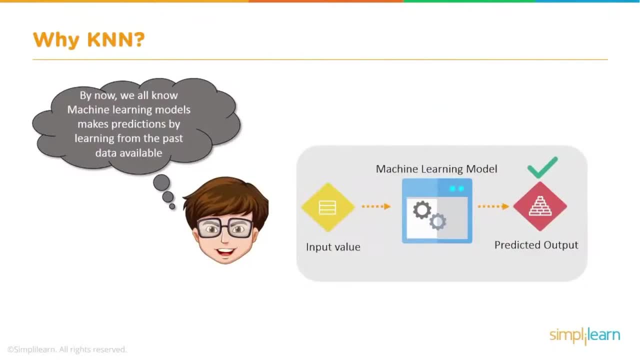 use the different models in machine learning. By now we all know machine learning models make predictions by learning from the past data available. So we have our input values. our machine learning model builds on those inputs of what we already know and then we use that to create a predictive. 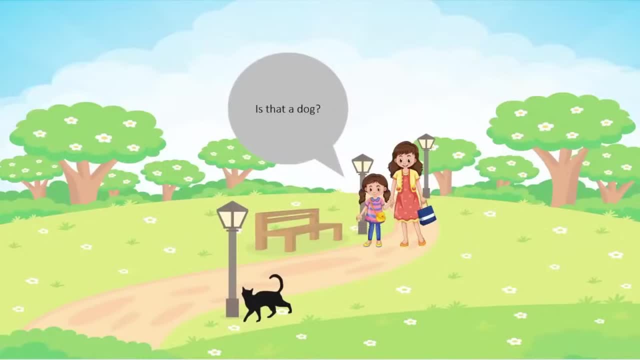 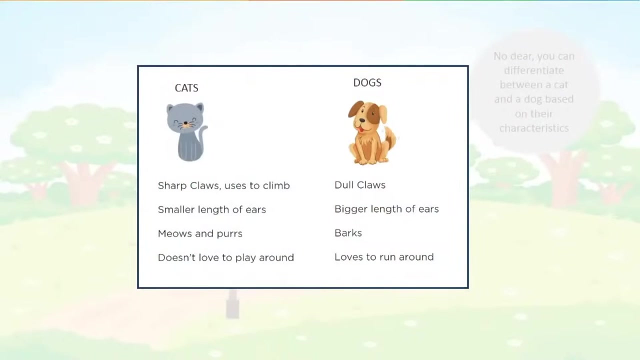 output. Is that a dog? Little kid looking over there watching the black cat cross their path? No dear, you can differentiate between a cat and a dog based on their characteristics: Cats. Cats have sharp claws, uses to climb, smaller length of ears. 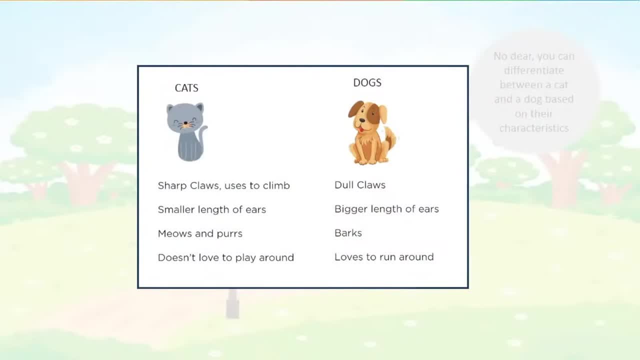 meows and purrs, doesn't love to play around. Dogs have dull claws, bigger length of ears, barks. loves to run around. You usually don't see a cat running around people, Although I do have a cat that does that. 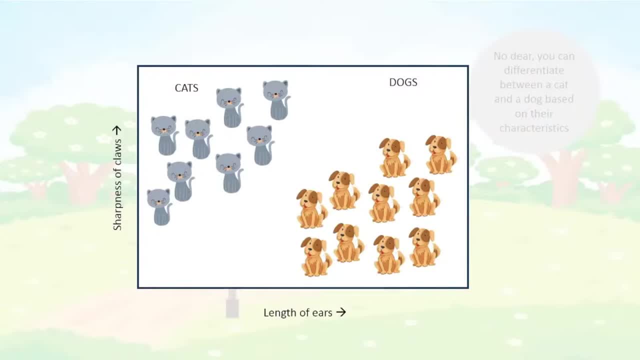 And we can look at these and say we can evaluate the sharpness of the claws- how sharp are their claws? and we can evaluate the length of the ears, and we can usually sort out cats from dogs based on even those two characteristics. Now tell me if it is a cat or a dog. 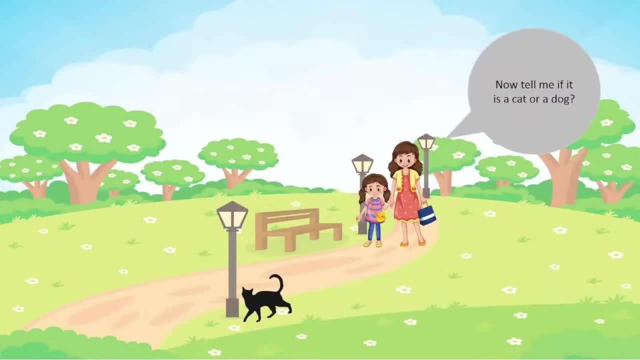 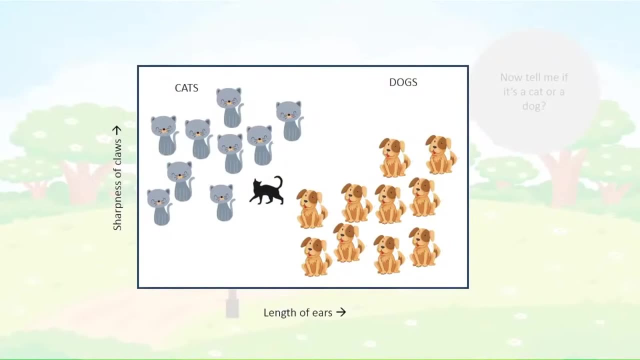 Odd question. usually little kids know cats and dogs by now, Unless they live in a place where there's not many cats or dogs. So if we look at the sharpness of the claws, the length of the ears and we can see that the cat has smaller ears. 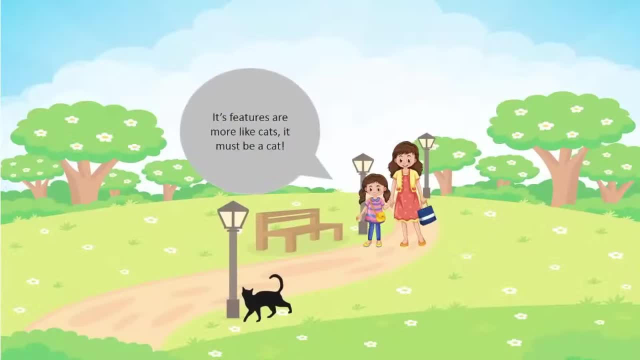 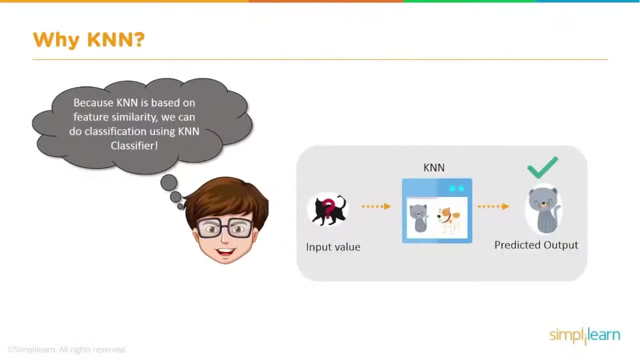 and sharper claws than the other animals. Its features are more like cats. it must be a cat: Sharp claws, length of ears- and it goes in the cat group. Because KNN is based on feature similarity, we can do classification using KNN. 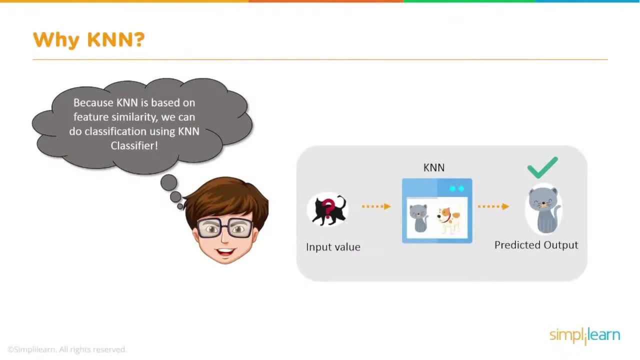 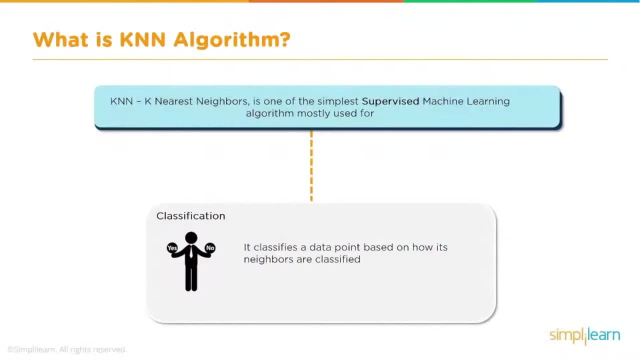 classifier. So we have our input value, the picture of the black cat. it goes into our trained model and it predicts that this is a cat coming out. So what is KNN? What is the KNN algorithm? K nearest neighbors is what that stands for. It's one of the 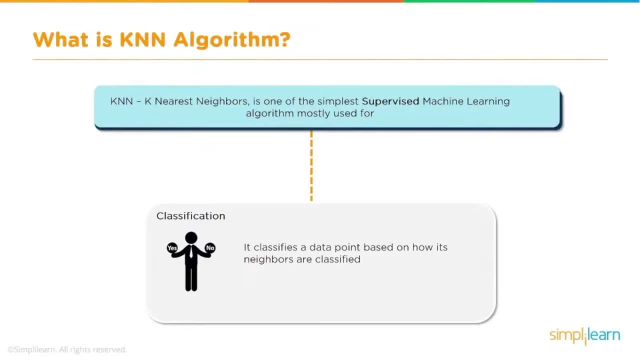 simplest supervised machine learning algorithms mostly used for classification. So we want to know: is this a dog or it's not a dog? Is it a cat or not a cat? It classifies a data point based on how its neighbors are classified. KNN stores all available. 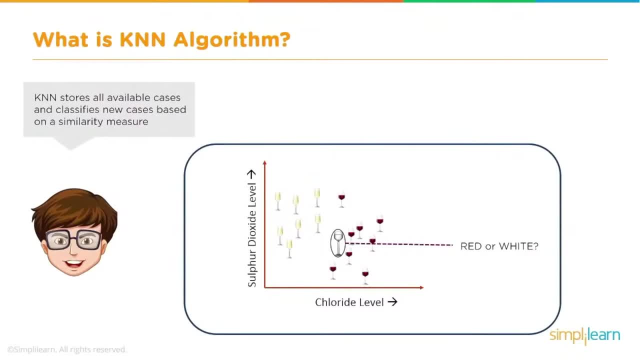 cases and classifies new cases based on a similarity measure. And here we've gone from cats and dogs right into wine. another favorite of mine, KNN, stores all available cases and classifies new cases based on a similarity measure. And here you see, we have a measurement of 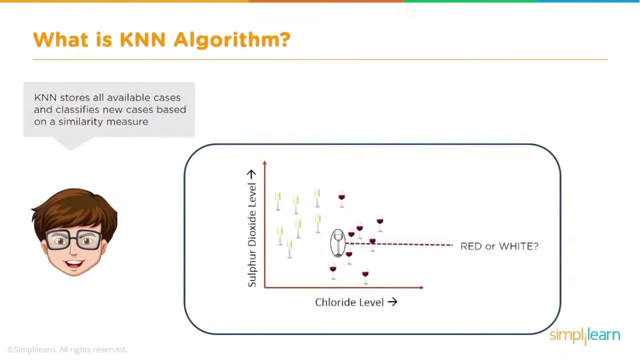 sulfur dioxide versus the chloride level and then the different wines they've tested and where they fall on that graph based on how much sulfur dioxide and how much chloride. KNN is a perimeter that refers to the number of nearest neighbors to include in the majority of the voting. 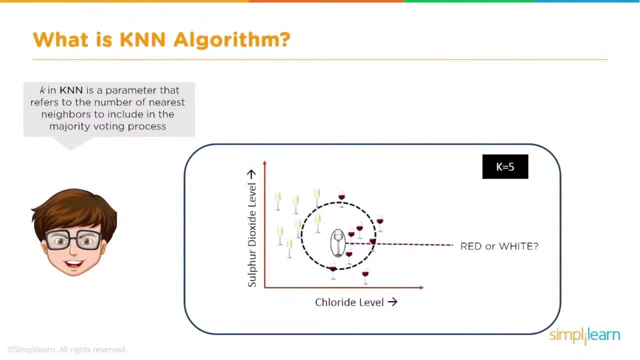 process, And so if we add a new glass of wine there- red or white- we want to know what the neighbors are. In this case, we're going to put K equals 5.. We'll talk about K in just a minute. A data point is classified by the majority. 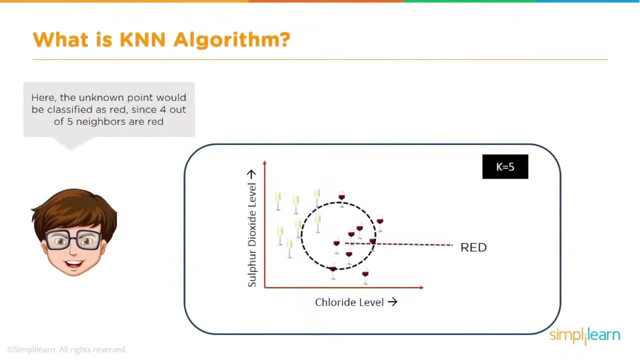 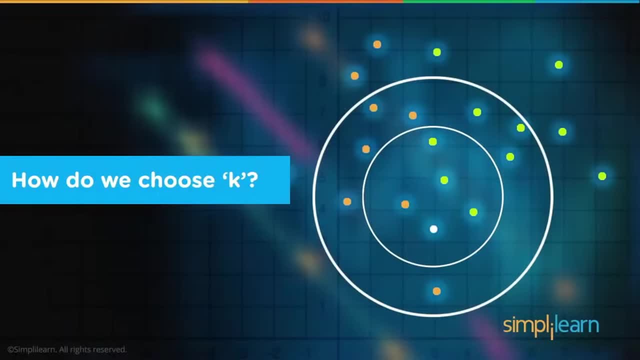 of votes from its five nearest neighbors. Here the unknown point would be classified as red, since four out of five neighbors are red. So how do we choose K? How do we know K equals 5?? I mean, that was the value we put in there, so we're going to talk about it. 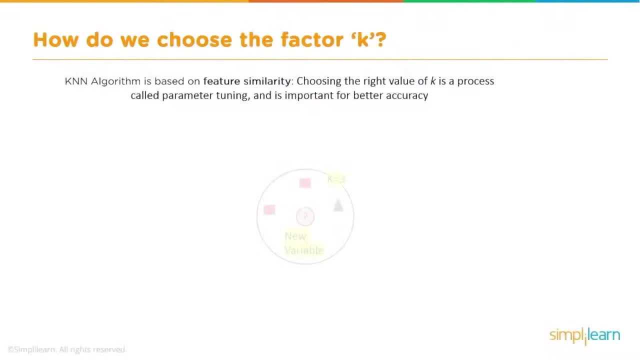 How do we choose the factor K? KNN algorithm is based on feature similarity. Choosing the right value of K is a process called parameter tuning and is important for better accuracy. So at K equals 3, we can classify. we have a question mark in the middle. 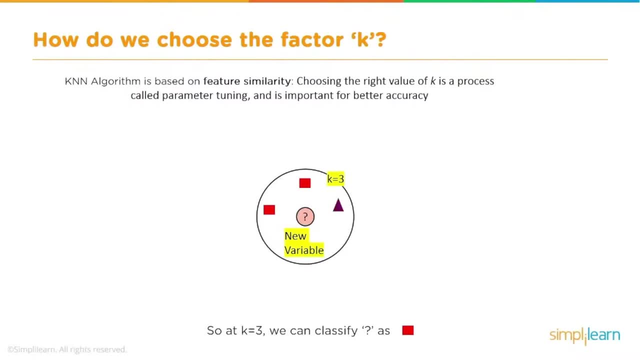 as either a square or a not. Is it a square or is it, in this case, a triangle? And so if we set K equals to 3, we're going to look at the three nearest neighbors. we're going to say: this is a square. 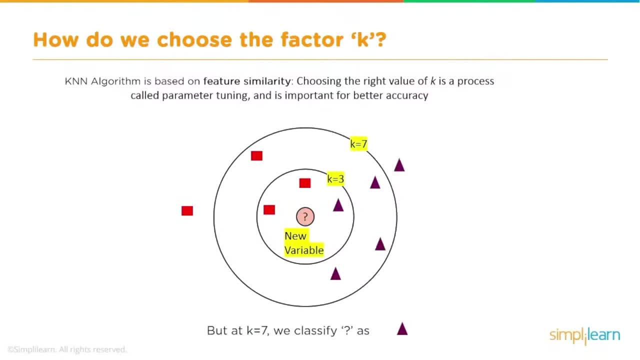 And if we put K equals to 7, we classify as a triangle depending on what the other data is around it And you can see as the K changes depending on where that point is. that drastically changes your answer And we jump here and we go. how do we choose? 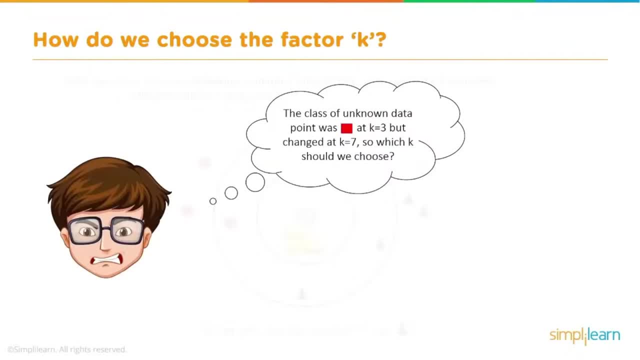 the factor of K. You'll find this in all machine learning. Choosing these factors, that's the face you get. It's like, oh my gosh, Did I choose the right K? Did I set it right my values in whatever machine learning? 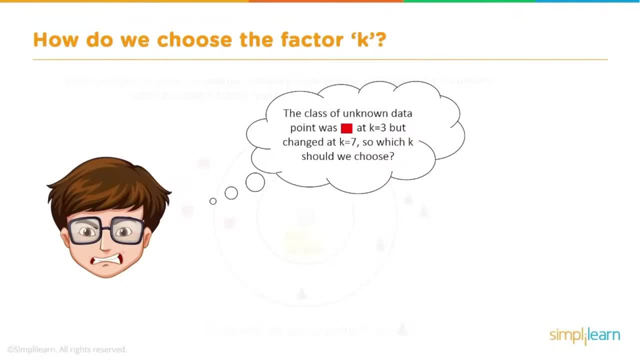 tool you're looking at so that you don't have a huge bias in one direction or the other, And in terms of KNN- the number of K, if you choose it too low the bias is based on- it's just too noisy, It's right next to a couple things and it's going to pick. 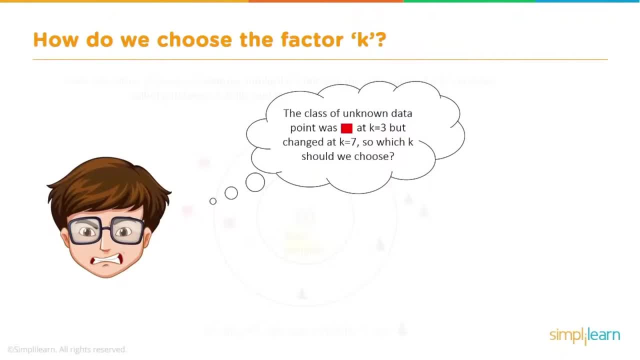 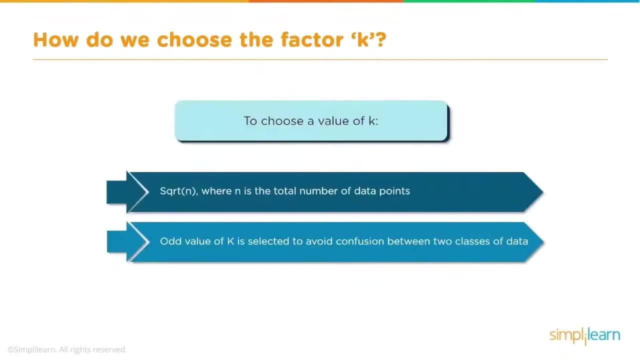 those things and you might get a skewed answer. And if your K is too big then it's going to take forever to process. So you're going to run into processing issues and resource issues. So what we do, the most common use and there's other options for. 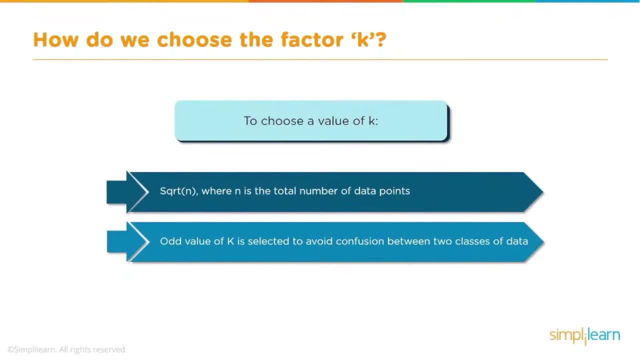 choosing K is to use the square root of N. So N is the total number of values you have and you take the square root of it. In most cases you also if it's an even number. so if you're using, like in this case, 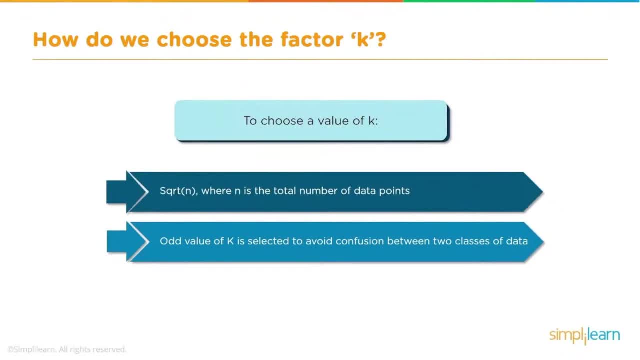 squares and triangles. if it's even, you want to make your K value odd. That helps it select better. So in other words, you're not going to have a balance between two different factors that are equal. So usually take the square root of N and if it's even you, add one to it. 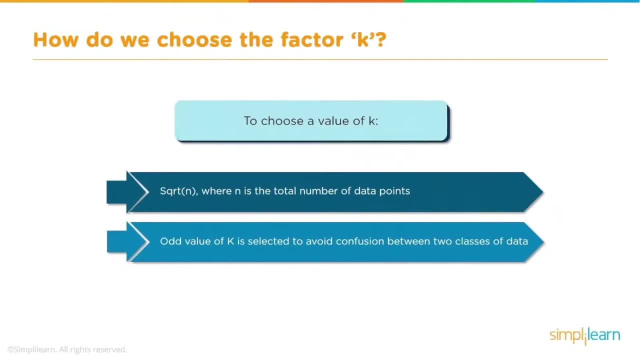 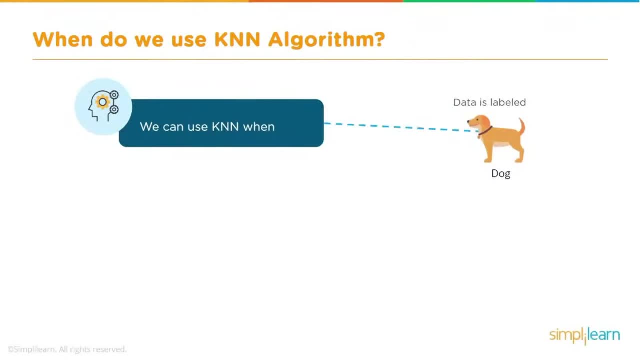 or subtract one from it, and that's where you get the K value from. That is the most common use and it's pretty solid. It works very well. When do we use KNN? We can use KNN when data is labeled, So you need a. 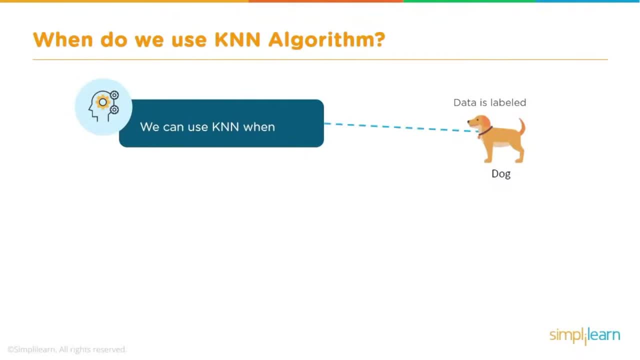 label on it. We know we have a group of pictures with dogs, dogs, cats, cats. Data is noise free And so you can see here when we have a class and we have like underweight 140,, 23,, hello. 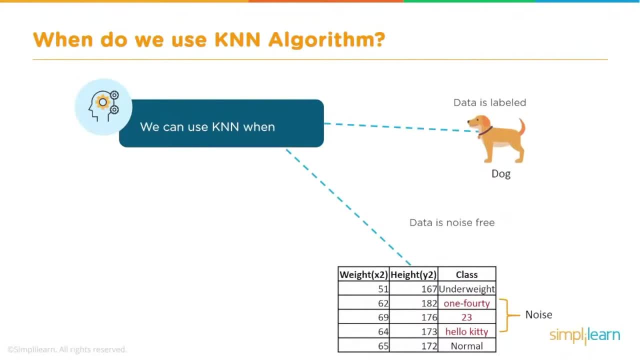 kitty normal. that's pretty confusing. We have a high variety of data coming in So it's very noisy And that would cause an issue. Data set is small, So we're usually working with smaller data sets where you might get into. 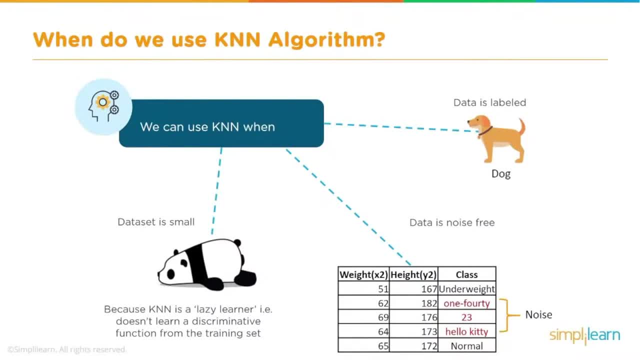 a gig of data if it's really clean, doesn't have a lot of noise. Because KNN is a lazy learner, ie it doesn't learn a discriminative function from the training set, So it's very lazy. So if you have very complicated, 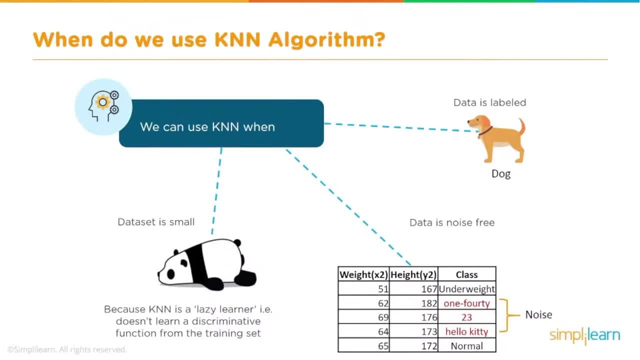 data and you have a large amount of it. you're not going to use the KNN, But it's really great to get a place to start, even with large data, you can sort out a small sample and get an idea of what that looks like using the KNN And also. 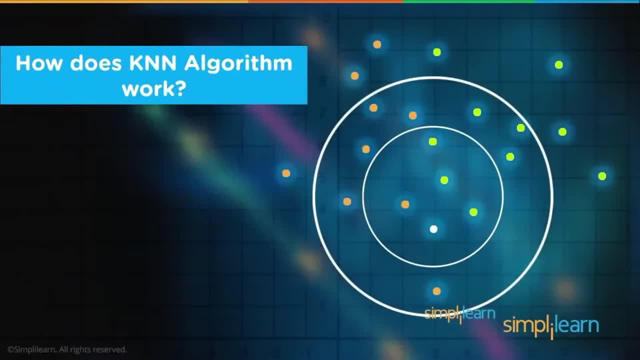 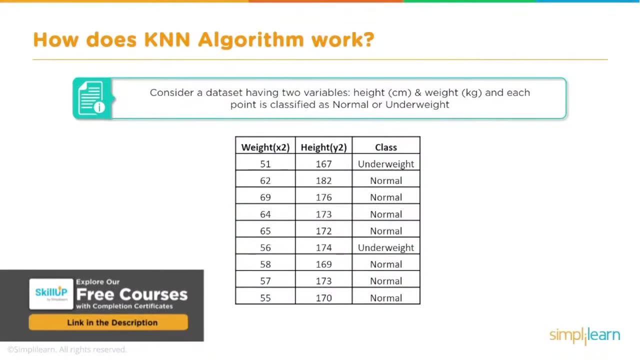 just using for smaller data sets. KNN works really good. How does a KNN algorithm work? Consider a data set having two variables- Height in centimeters and weight in kilograms- And each point is classified as normal or underweight. So we can see right here. 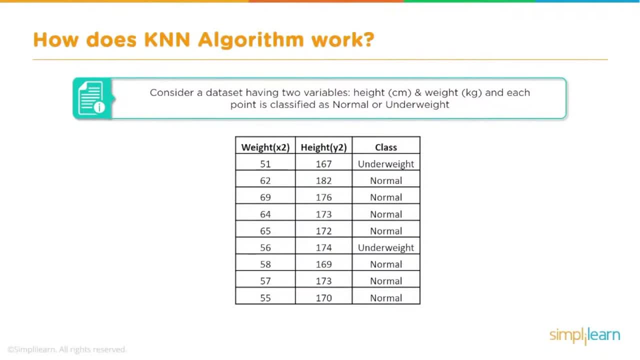 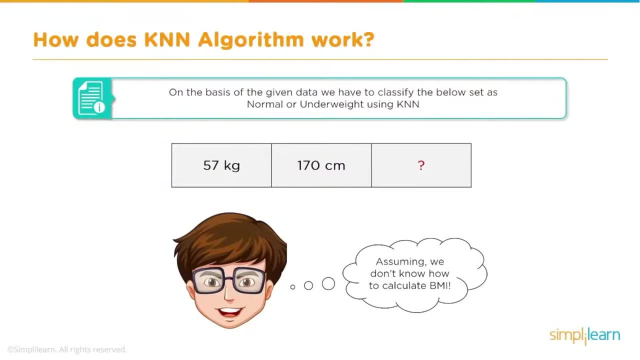 we have two variables. you know: true, false, or either normal or they're not. they're underweight. On the basis of the given data, we have to classify the below set as normal or underweight using KNN. So if we have new data coming, 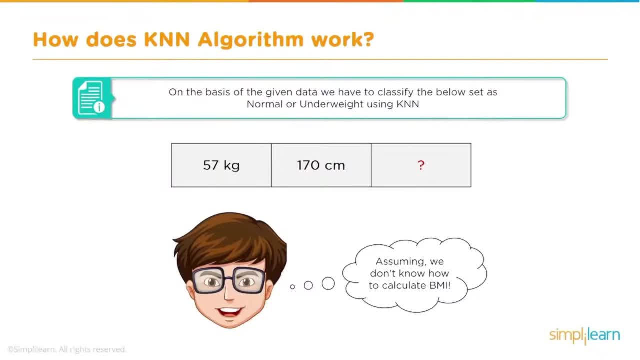 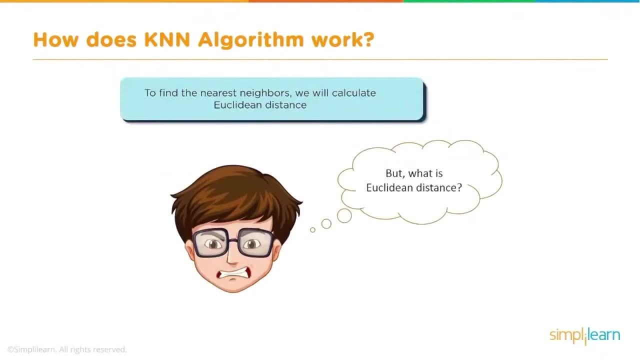 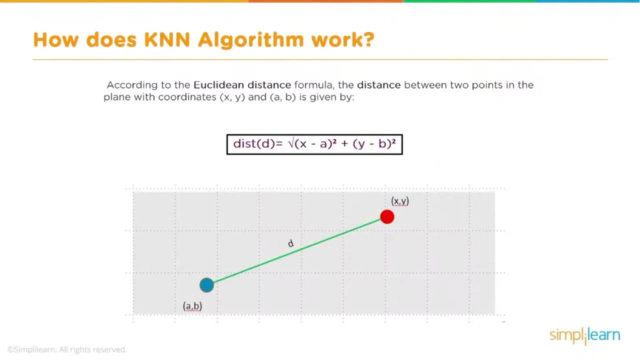 in. that says 57 kilograms and 177 centimeters. is that going to be normal or underweight? To find the nearest neighbors, we'll calculate the Euclidean distance According to the Euclidean distance formula: the distance between two points in the plane with the coordinates x, y and a- b. 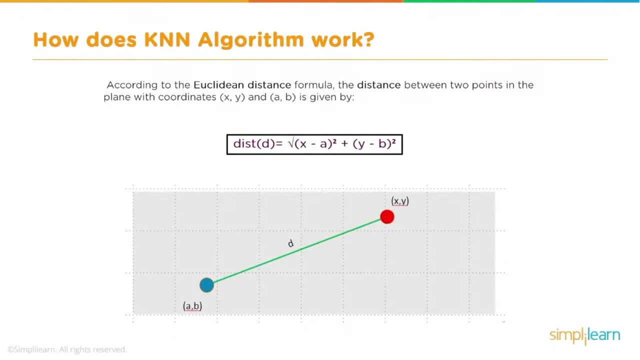 is given by distance. d equals the square root of x minus a squared, plus y minus b squared, And you can remember that from the two edges of a triangle, or computing the third edge, since we know the x side and the y side, Let's calculate. 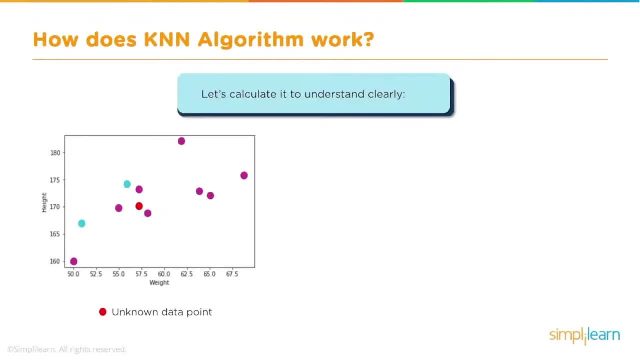 to understand clearly. So we have our unknown point- We placed it there in red- And we have our other points where the data is scattered around. The distance d1 is the square root of 170 minus 167 squared, plus 57 minus 51 squared. 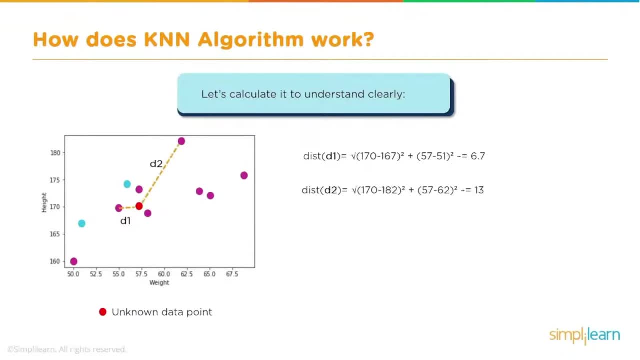 which is about 6.7.. And distance 2 is about 13.. And distance 3 is about 13.4.. Similarly, we will calculate the Euclidean distance of unknown data point from all the points in the data set. And because we're dealing with small amount of data, 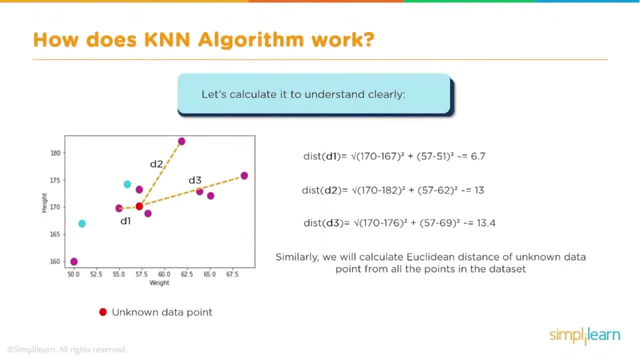 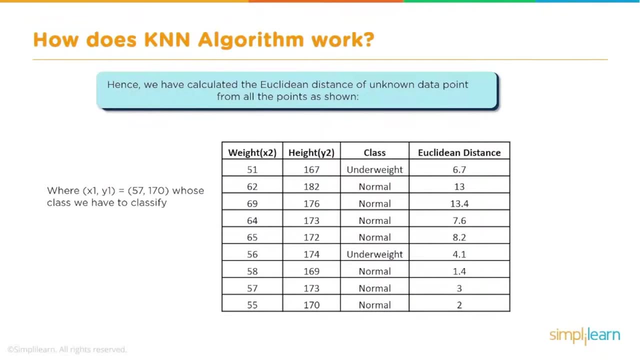 that's not that hard to do. It's actually pretty quick for a computer And it's not a really complicated math. So you can just see how close is the data based on the Euclidean distance. Hence we have calculated the Euclidean distance of unknown data point. 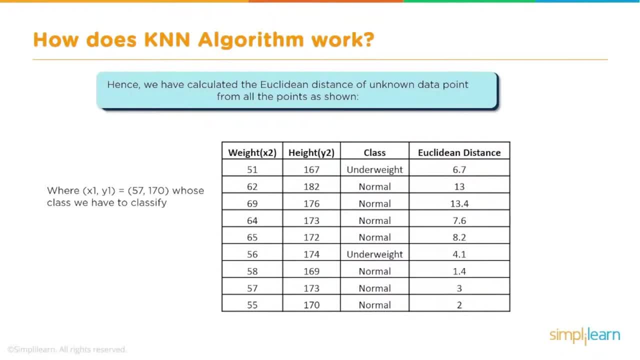 from all the points as shown, Where x1 and y1 equal 57 and 170, whose class we have to classify. So now we're looking at that, We're saying, well, here's the Euclidean distance, Who's going to be their closest? 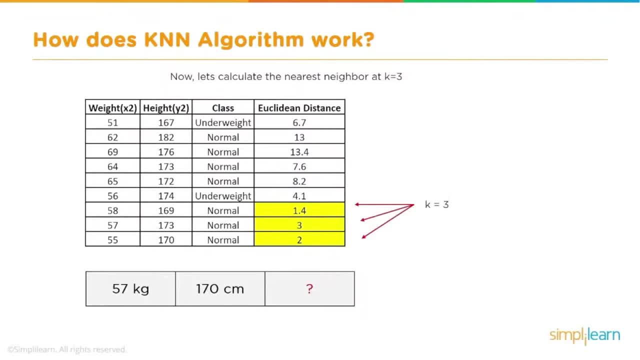 neighbors. Now let's calculate the nearest neighbor at k equals 3. And we can see the three closest neighbors. puts them at normal And that's pretty self-evident. When you look at this graph it's pretty easy to say okay. 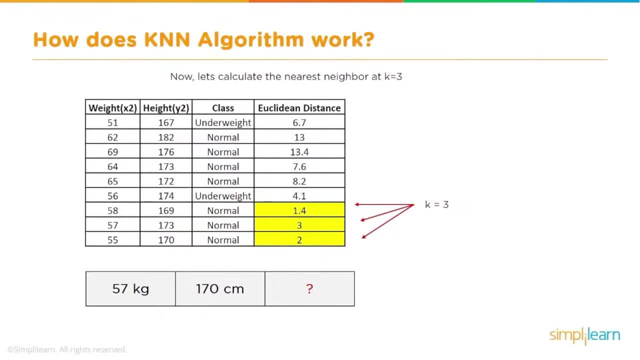 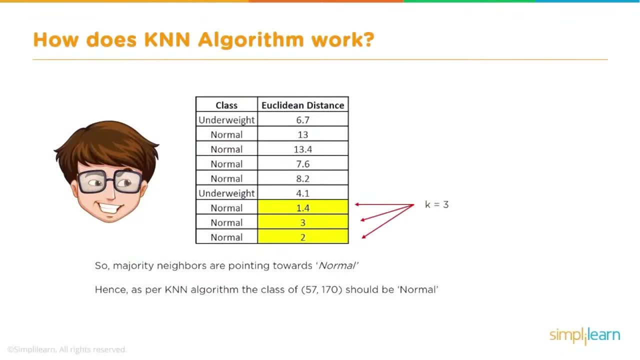 we're just voting Normal, normal, normal. Three votes for normal. This is going to be a normal weight, So majority of neighbors are pointing towards normal Hence, as per KNN algorithm, the class of 57, 170 should be normal. 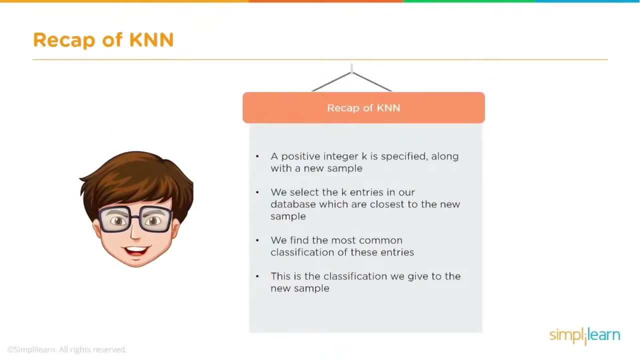 So a recap of KNN Positive integer k is specified, along with a new sample. We select the k entries in our database which are closest to the new sample. We define the most common classification of these entries. This is the classification we give to the new sample. So, as you can see, 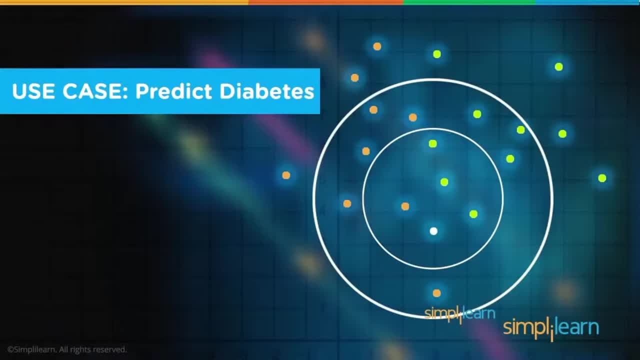 it's pretty straightforward: We're just looking for the closest things that match what we got. So let's take a look and see what that looks like in a use case in Python. So let's dive into the predict diabetes use case. So, use case: predict diabetes. 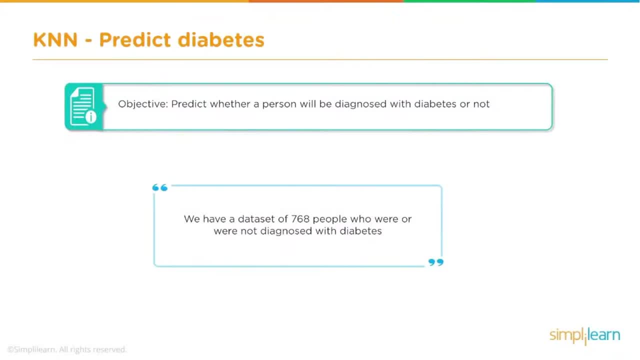 The objective: predict whether a person will be diagnosed with diabetes or not. We have a data set of 768 people who were or were not diagnosed with diabetes, And let's go ahead and open that file and just take a look at that data. And this is in a 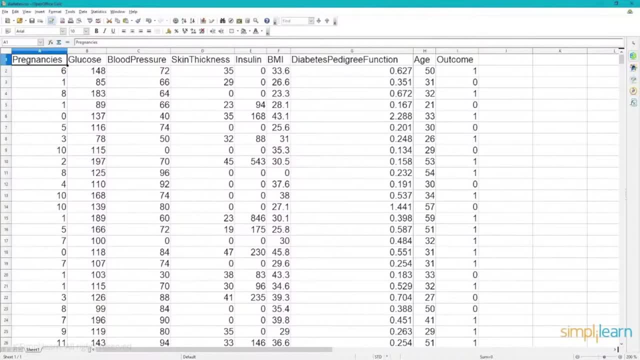 simple spreadsheet format. The data itself is comma separated- Very common set of data. It's also a very common way to get the data And you can see here we have columns A through I. That's what: one, two, three, four, five, six, seven, eight. 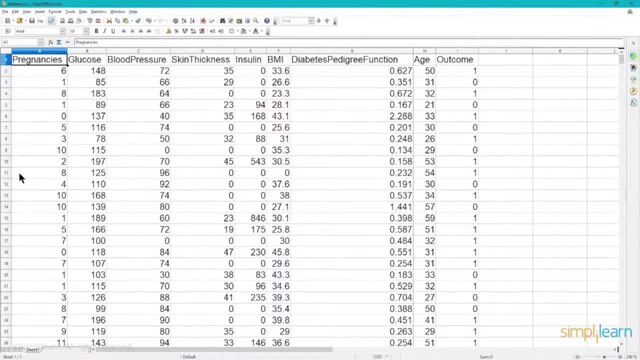 Eight columns with a particular attribute and then the ninth column, which is the outcome, is whether they have diabetes. As a data scientist, the first thing you should be looking at is insulin. Well, you know, if someone has insulin, they have diabetes because that's why they're taking it And that could cause 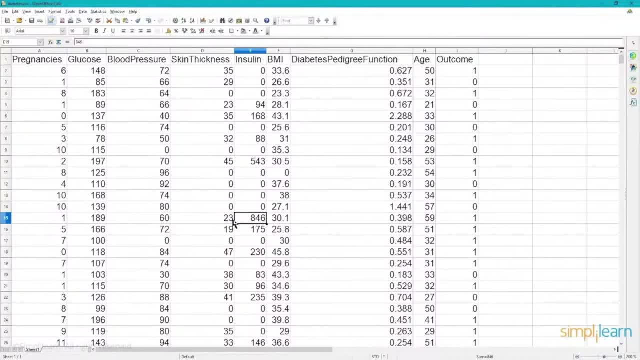 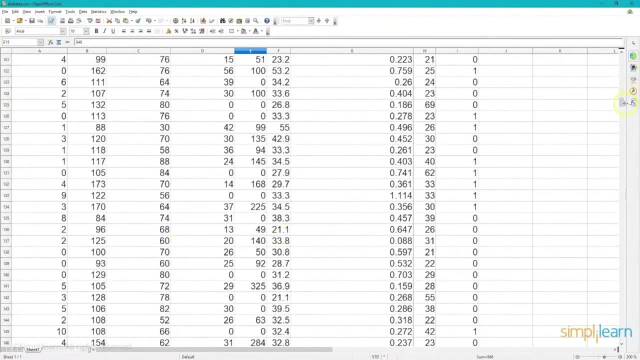 issue in some of the machine learning packages, But for a very basic setup this works fine for doing the KNN And the next thing you notice is it didn't take very much to open it up. I can scroll down to the bottom of the data There's. 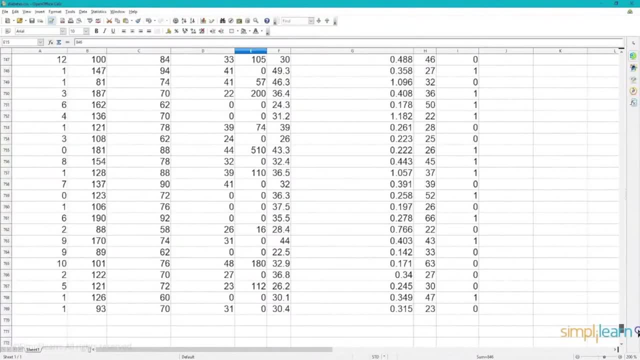 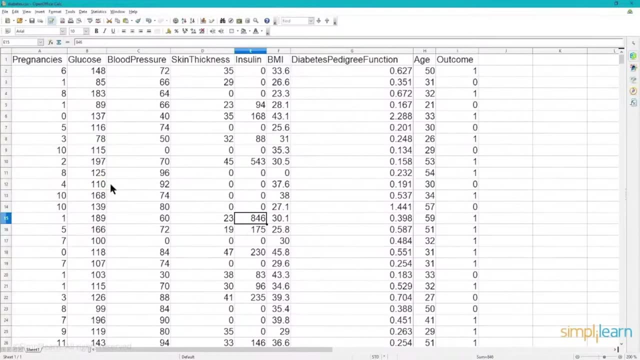 768.. It's pretty much a small data set. You know, at 769 I can easily fit this into my RAM on my computer. I can look at it, I can manipulate it And it's not going to tax, just a regular desktop computer. 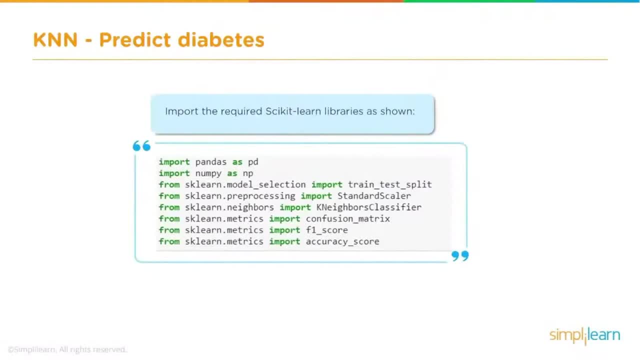 You don't even need an enterprise version to run a lot of this. So let's start with importing all the tools we need, And before that, of course, we need to discuss what IDE I'm using. Certainly, you can use any particular editor for Python, But I like to use for doing. 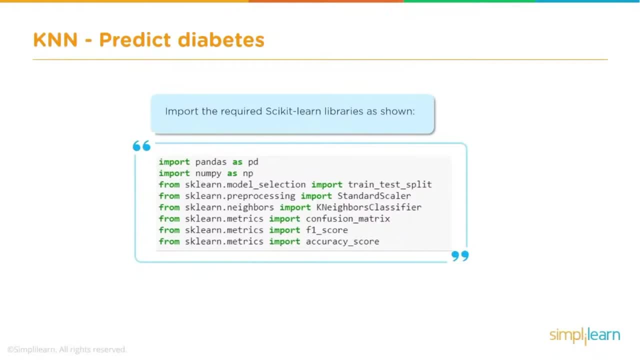 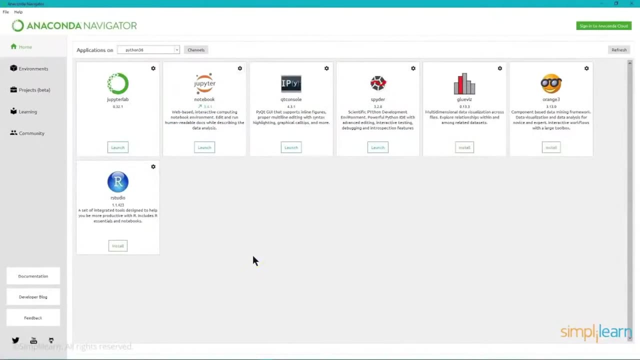 very basic visual stuff: the Anaconda, which is great for doing demos with the Jupiter Notebook, And just a quick view of the Anaconda Navigator, which is the new release out there, which is really nice. You can see under Home. I can choose my application. We're going to. 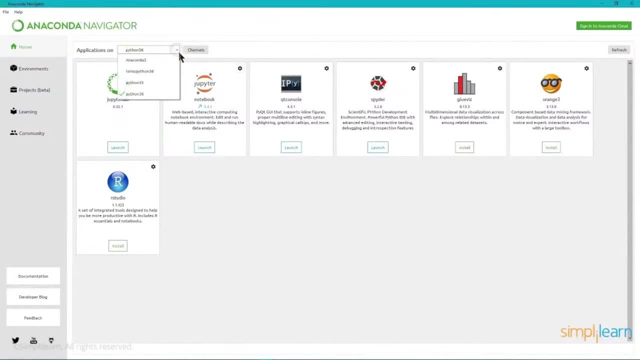 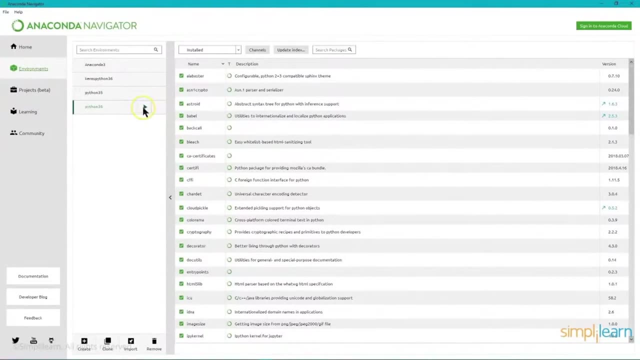 be using Python 3.6.. I have a couple different versions on this particular machine. If I go under Environments, I can create a unique environment for each one, which is nice, And there's even a little button there where I can install different packages. 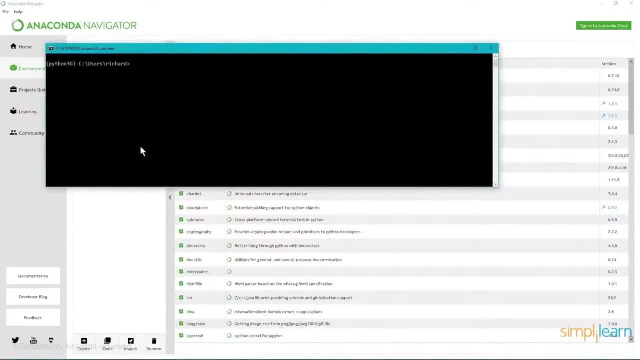 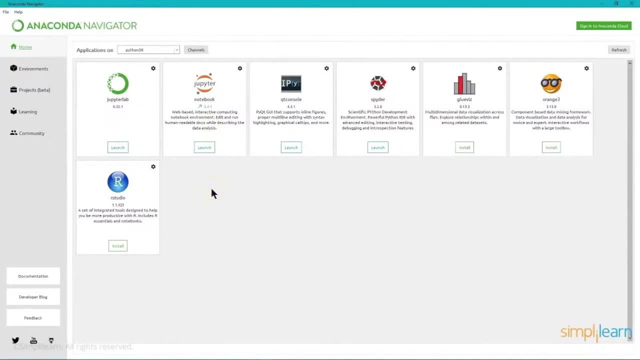 So if I click on that button and open the terminal, I can then use a simple pip install to install different packages I'm working with. Let's go ahead and go back under Home and we're going to launch our notebook And I've already, you know, kind of like the old cooking. 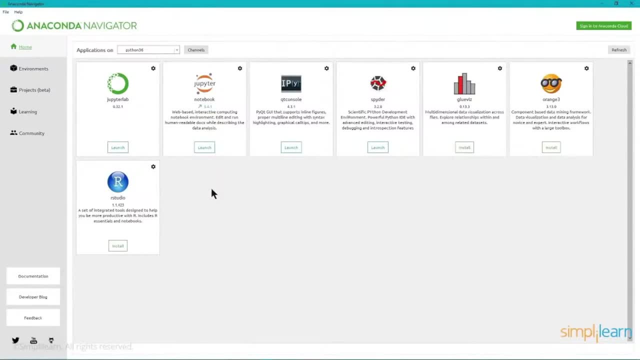 shows. I've already prepared a lot of my stuff, so we don't have to wait for it to launch, because it takes a few minutes for it to open up a browser window. In this case, it's going to open up Chrome, because that's my default. 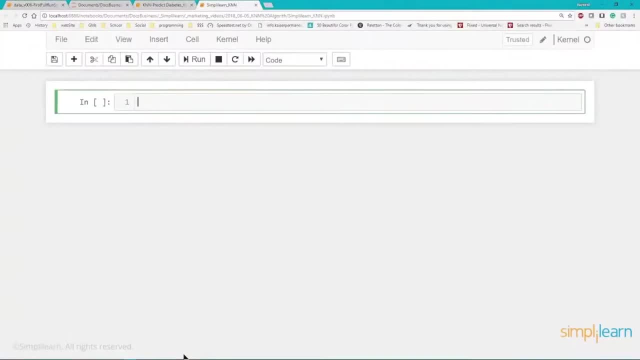 that I use And since the script is pre-done, you'll see I have a number of windows open up at the top, The one we're working in. And since we're working on the KNN predict whether a person will have diabetes or not, Let's go ahead and put that. 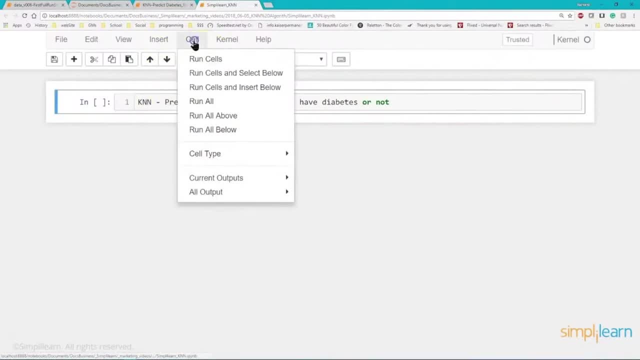 title in there And I'm also going to go up here and click on cell. Actually, we want to go ahead and first insert a cell below And then I'm going to go back up to the top cell and I'm going to change the cell type. 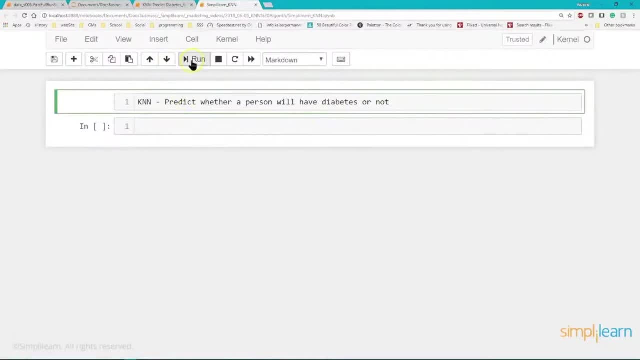 to markdown. That means this is not going to run as Python It's a markdown language, So if I run this first one, it comes up in nice big letters, which is kind of nice, Reminds us what we're working on, And by now, 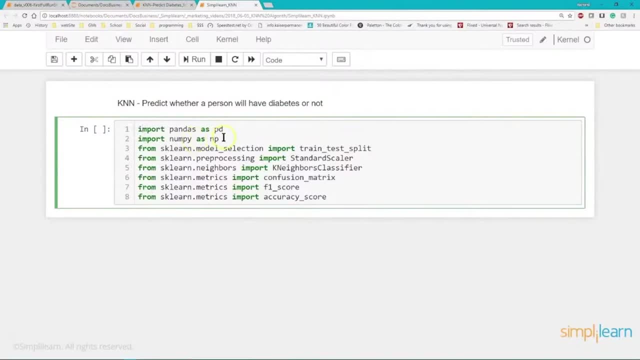 you should be familiar with doing all of our imports. We're going to import the pandas as pd Import, numpy as np. Pandas is the pandas data frame and numpy is the number array- Very powerful tools to use in here. So we have our imports, So we've 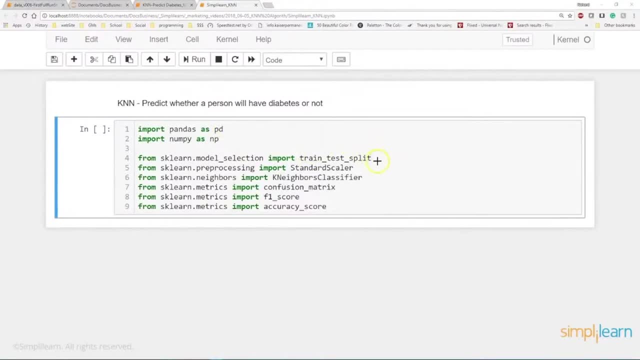 brought in our pandas, our numpy, our two general Python tools, and then you can see over here we have our train test split. By now you should be familiar with splitting the data. We want to split part of it for training our thing and then training our particular model. 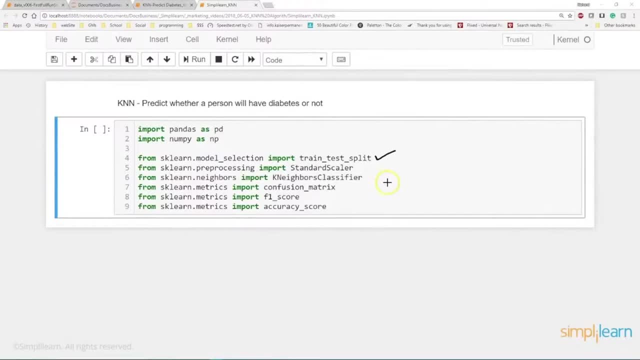 And then we want to go ahead and test the remaining data to see how good it is Pre-processing A standard scalar pre-processor so we don't have a bias of really large numbers. Remember in the data we had like number pregnancies isn't going to get very large. 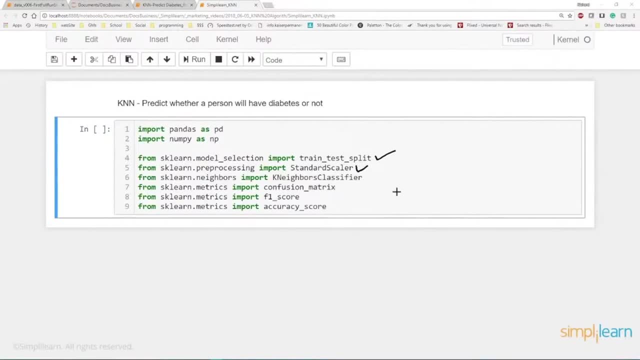 where the amount of insulin they take can get up to 256.. So 256 versus 6. That will skew results, So we want to go ahead and change that so that they're all uniform between minus 1 and 1.. And then the actual. 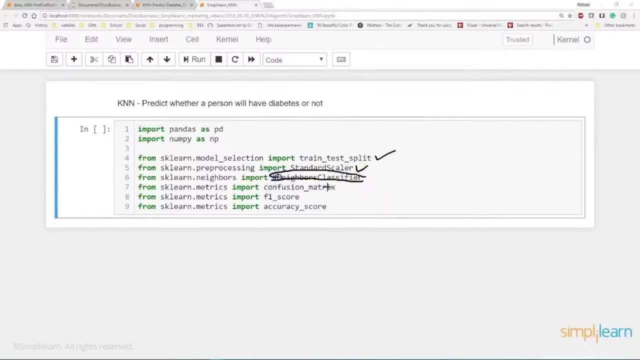 tool. This is the k-neighbors classifier we're going to use. And finally, the last three are three tools to test. All about testing our model. How good is it? We just put down test on there And we have our confusion matrix, our 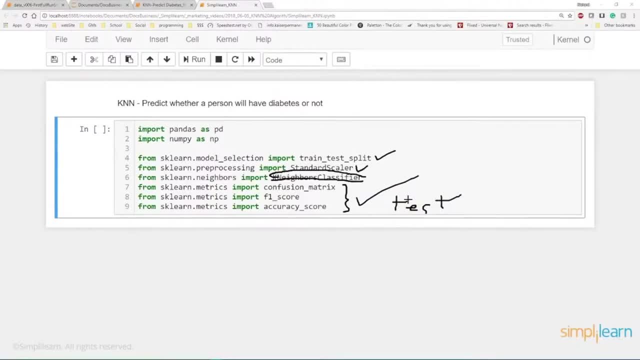 F1 score and our accuracy. So we have our two general Python modules we're importing, and then we have our six modules specific from the sklearn setup, And then we do need to go ahead and run this so that these are actually imported. There we go. 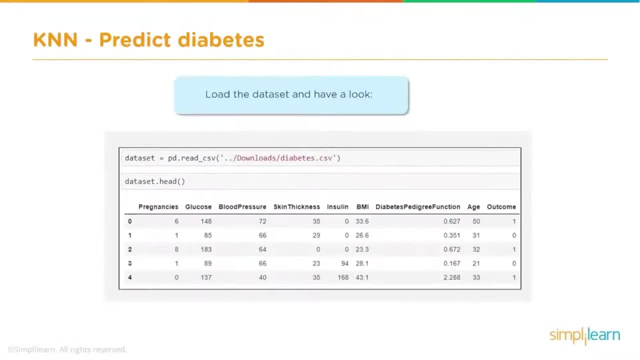 And then move on to the next step. And so in this set we're going to go ahead and load the database. We're going to use pandas- Remember pandas is pd- And we'll take a look at the data in Python. We looked at it. 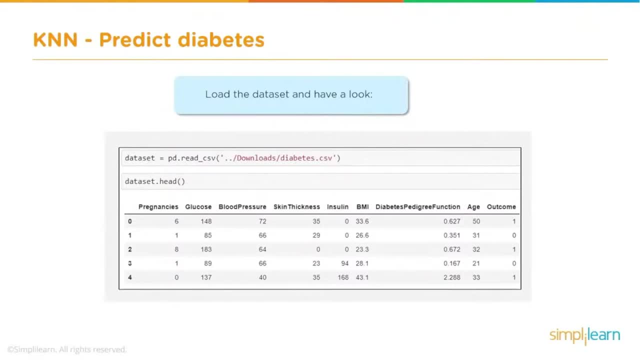 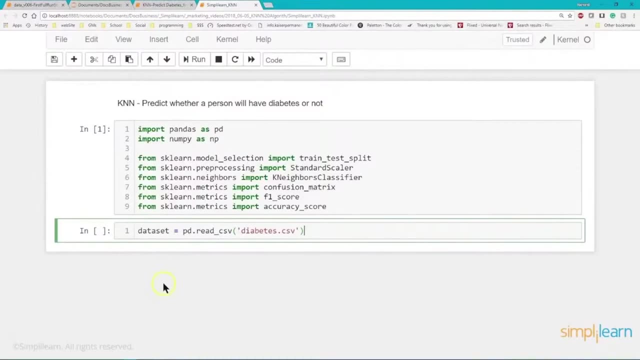 in a simple spreadsheet, But usually I like to also pull it up so that we can see what we're doing. So here's our data: set: equals pd dot, read csv. That's a pandas command. And the diabetes folder I just put in the same folder. 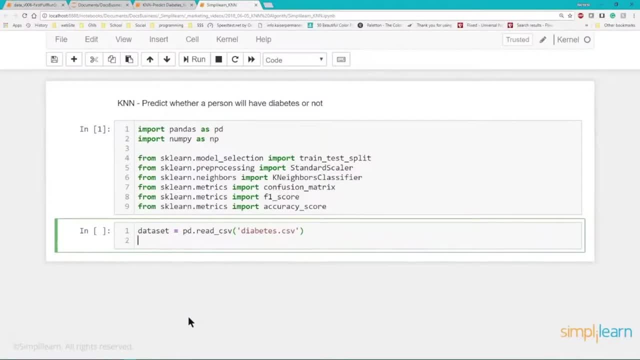 my IPython script is: If you put it in a different folder you'd need the full length on there. We can also do a quick length of the data set. That is a simple Python command: len for length. We might even let's go ahead and print that. 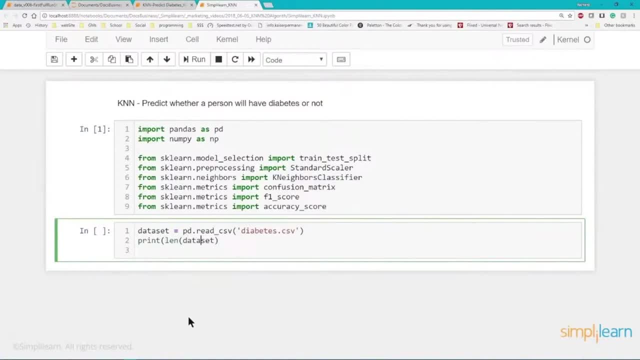 We'll go print. And if you do it on its own line length dot data set in the Jupyter Notebook, it'll automatically print it. But when you're in most of your different setups you want to do the print in front of there. 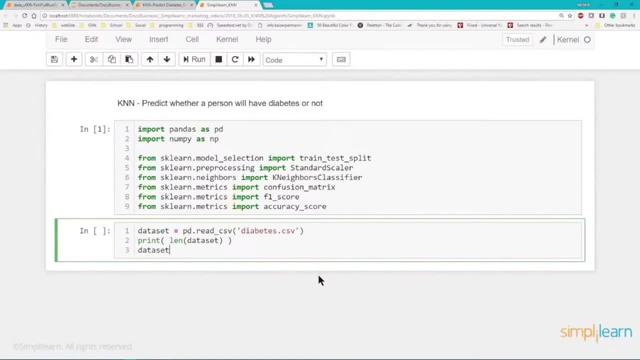 And then we want to take a look at the actual data set And since we're in pandas, we can simply do data set head And again. let's go ahead and add the print in there If you put a bunch of these in a row. 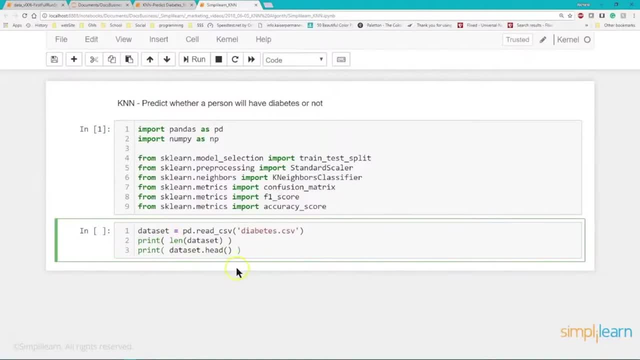 the data set one head. data set two head. it only prints out the last one, So I always like to keep the print statement in there. But because most projects only use one data frame- pandas data frame- doing it this way doesn't really matter. The other way works just fine. 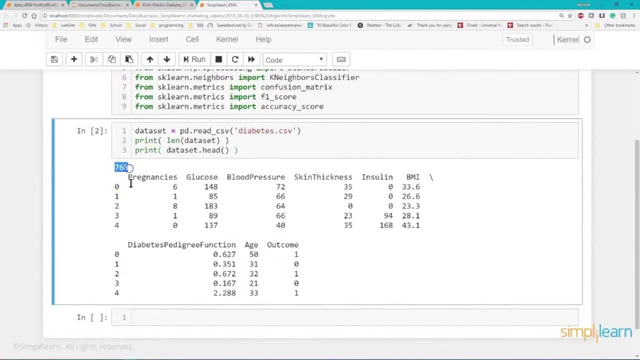 And you can see when we hit the run button. we have the 768 lines which we knew, And we have our pregnancies. It's automatically given a label on the left, Remember, the head only shows the first five lines, So we have zero through four. 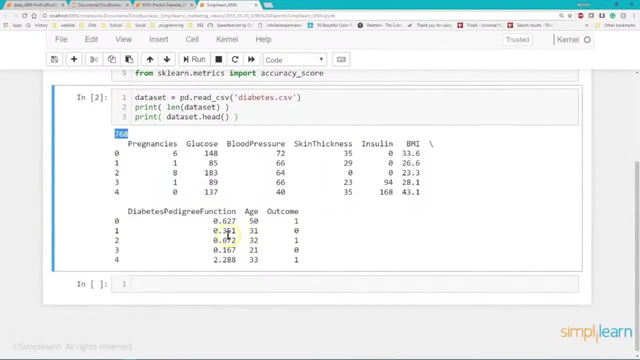 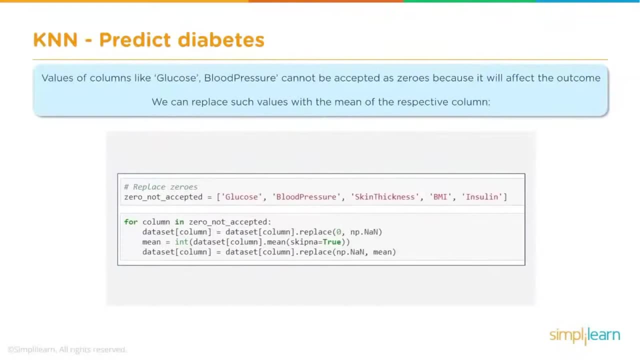 And just a quick look at the data. you can see it matches what we looked at before. We have pregnancy, glucose blood pressure, all the way to age, And then the outcome on the end, And we're going to do a couple things in this. 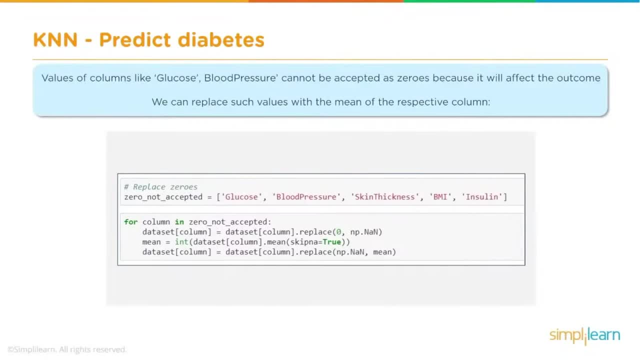 next step, We're going to create a list of columns where we can't have zero. There's no such thing as zero skin thickness or zero blood pressure, zero glucose- Any of those, you'd be dead. So not a really good factor if they have a zero in there because they didn't. 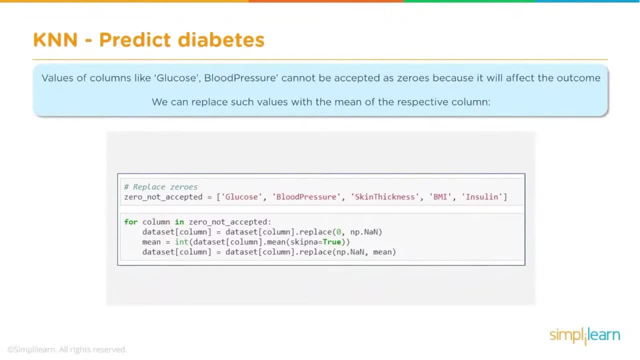 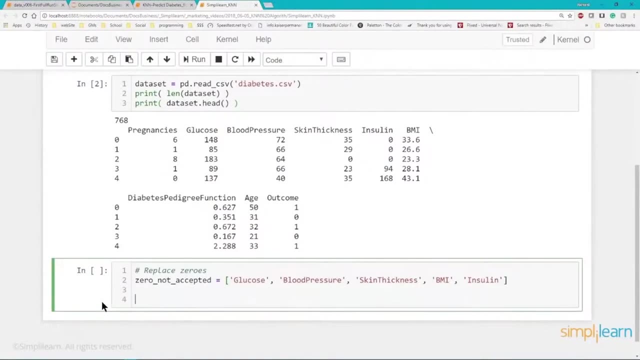 have the data And we'll take a look at that, because we're going to start replacing that information with a couple of different things And let's see what that looks like. So first we create a nice list. As you can see, we have the values we talked about. 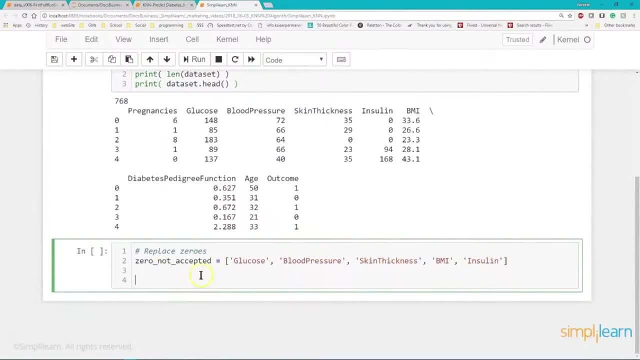 glucose, blood pressure, skin thickness- And this is a nice way when you're working with columns- is to list the columns you need to do, some kind of transformation on A very common thing to do And then for this particular setup, we certainly could. 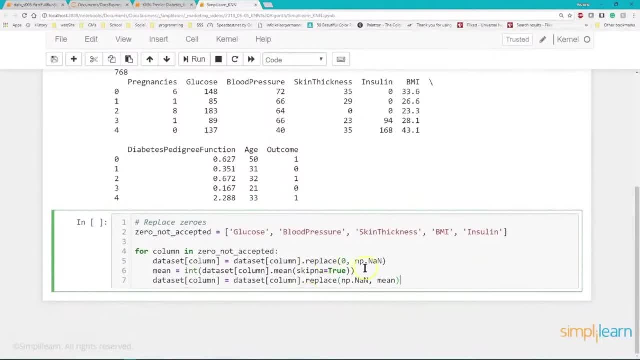 use the. there's some panda tools that will do a lot of this where we can replace the na, But we're going to go ahead and do it as a data set column equals data set column, dot replace. This is still pandas. You can do it direct. There's. 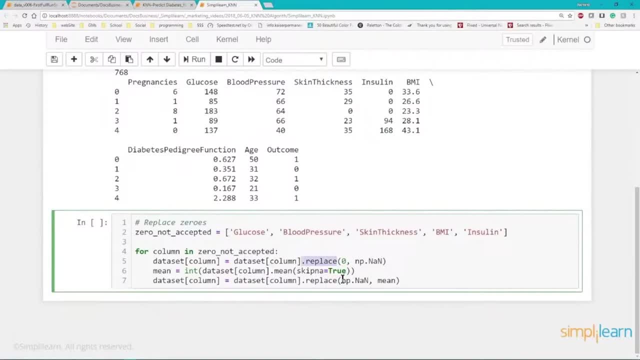 also one that you look for your nan. A lot of different options in here, But the nan, numpy nan is what that stands for. It doesn't exist. So the first thing we're doing here is we're replacing the zero with a numpy none. 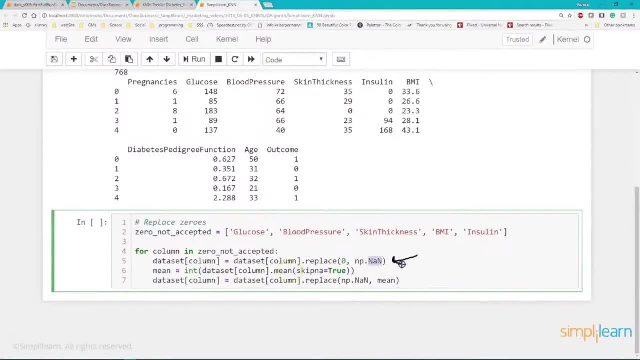 There's no data there. That's what that says. That's what this is saying right here. So let's put the zero in and we're going to replace zeros with no data. So if it's a zero, that means the person's hopefully not dead. Hopefully they just didn't get the data. 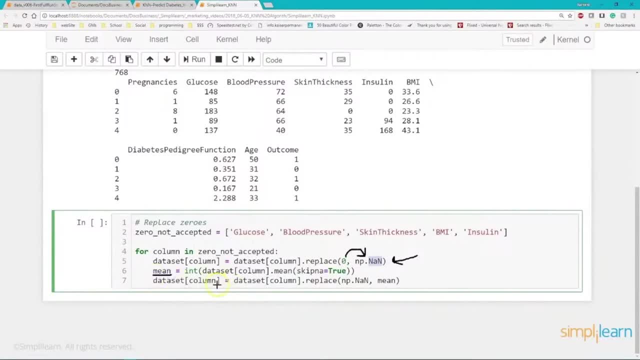 The next thing we want to do is we're going to create the mean, which is the integer from the data set, from the column dot mean where we skip na's. We can do that. That is a panda's command there: The skip na. 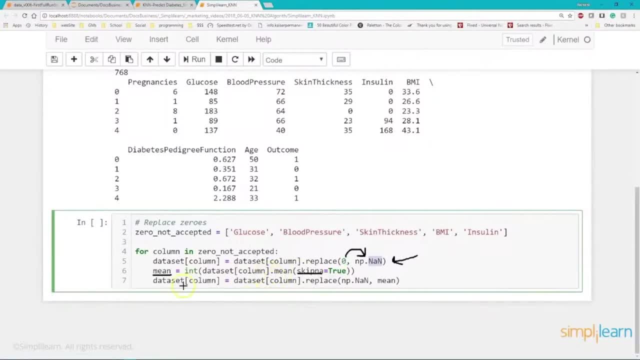 So we're going to figure out the mean of that data set And then we're going to take that data set column and we're going to replace all the np nan with the means. Why did we do that? We could have actually just taken this step and gone right down here. 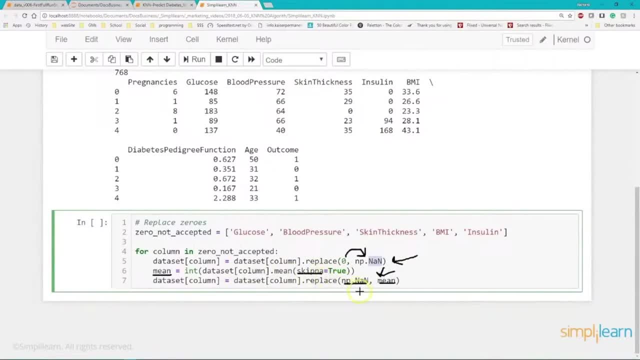 and just replaced zero and skipped anything, except there's a way to skip zeros and then just replace all the zeros, But in this case we want to go ahead and do it this way. So you can see that we're switching this to a nonexistent value. 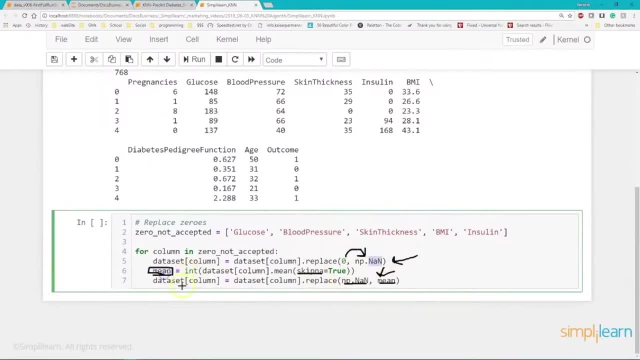 Then we're going to create the mean: Well, this is the average person. So if we don't know what it is, if they did not get the data and the data's missing, one of the tricks is you replace it with the average What is? 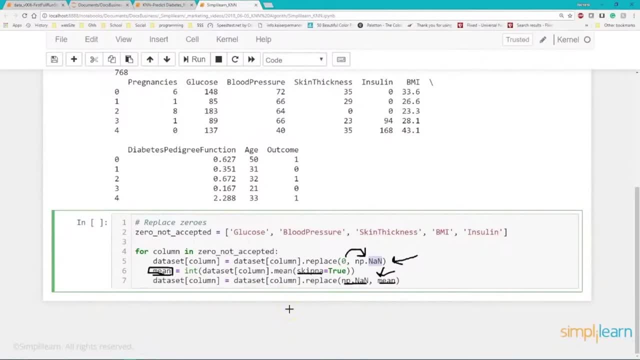 the most common data for that. This way you can still use the rest of those values to do your computation and it kind of just brings that particular value of those missing values out of the equation. Let's go ahead and take this and we'll go ahead and run it. 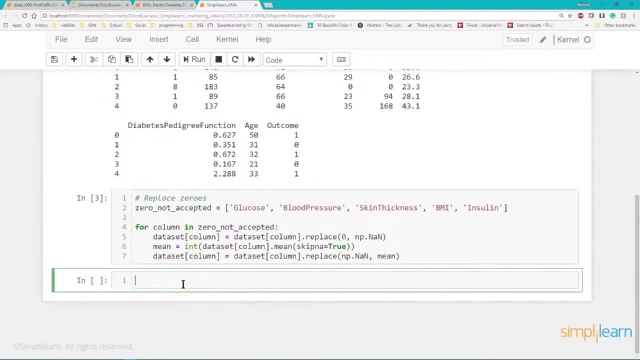 It doesn't actually do anything, so we're still preparing our data. If you wanted to see what that looks like, we don't have anything in the first few lines, so it's not going to show up, But we certainly could look at a row. 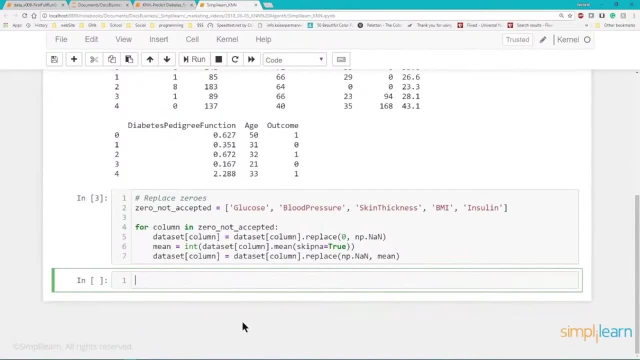 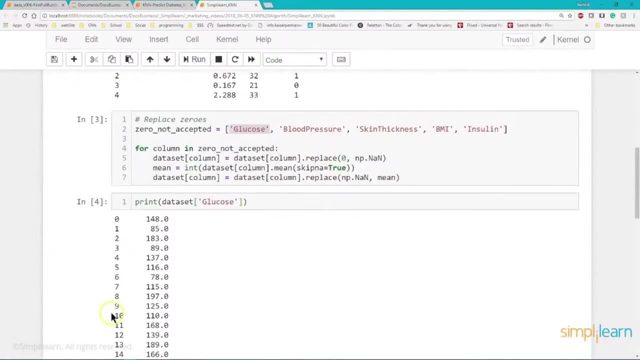 Let's do that. Let's go into our data set, Let's print a data set And let's pick- in this case, let's just do glucose- And if I run this, this is going to print all the different glucose levels going down And we 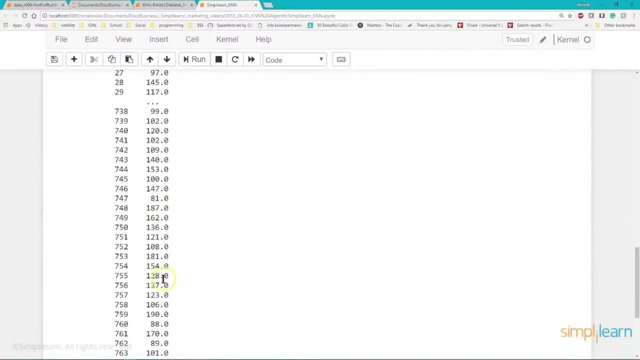 thankfully don't see anything in here that looks like missing data. at least on the ones it shows You can see it skipped a bunch in the middle. That's what it does. If you have too many lines in Jupyter Notebook, it'll skip a few, and 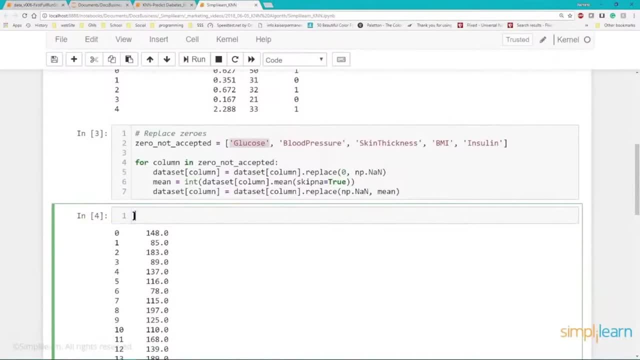 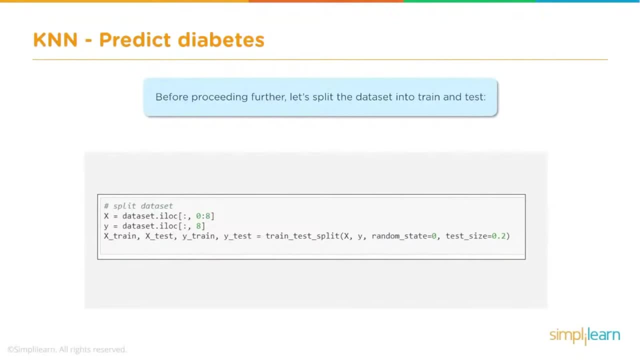 go on to the next in a data set. Let me go ahead and remove this And we'll just zero out that. And, of course, before we do any processing, before proceeding any further, we need to split the data set into our train and testing. 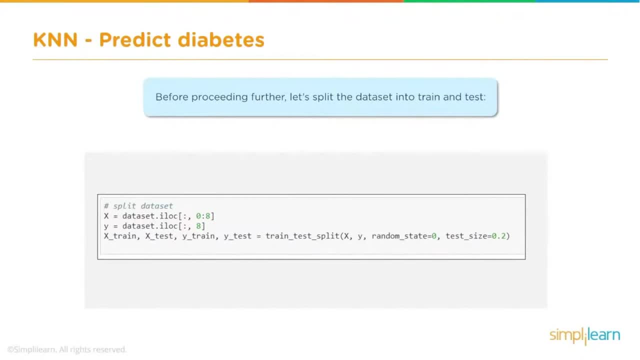 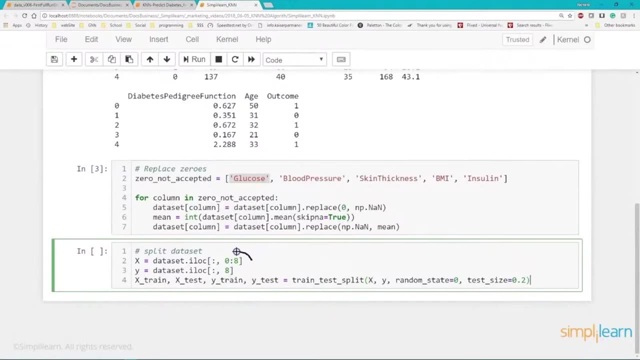 data. That way, we have something to train it with and something to test it on. And you're going to notice we did a little something here with the Pandas database code. There we go, my drawing tool We've added in this right here. 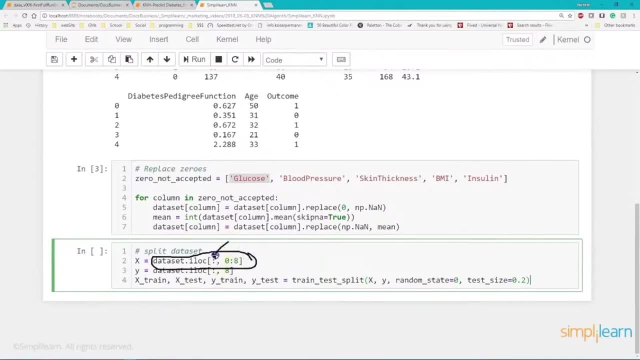 off the data set And what this says is that the first one in Pandas- this is from the PD Pandas- it's going to say, within the data set, we want to look at the eye location and it is all rows. That's what. 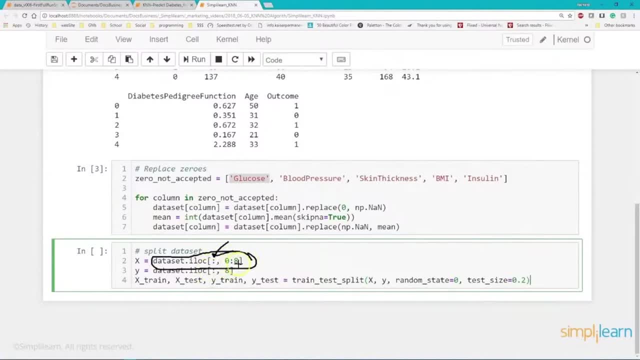 that says So. we're going to keep all the rows, But we're only looking at zero, column zero to eight. Remember column nine? here it is right up here. we printed it in here as outcome. Well, that's not part of the. 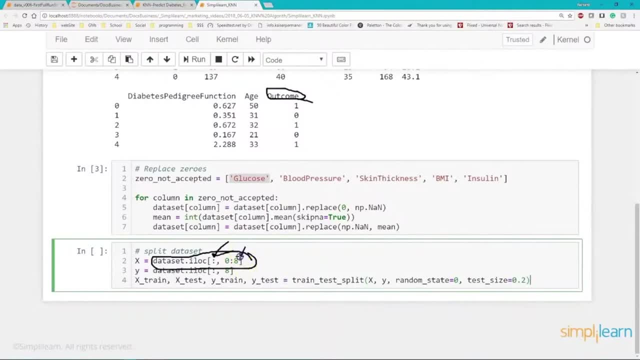 training data. that's part of the answer. Yes, column nine, but it's listed as eight Number eight. So zero to eight is nine columns. So eight is the value And, when you see it in here, zero. this is actually zero. 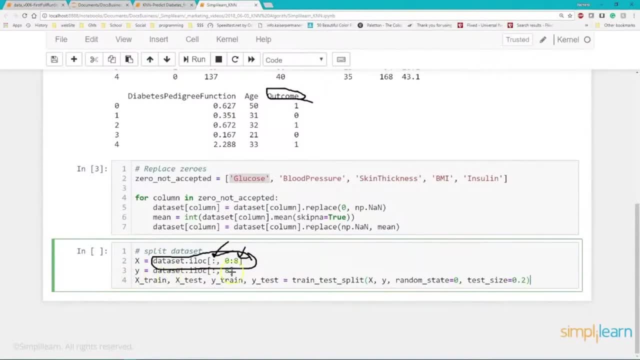 to seven, It doesn't include the last one. And then we go down here to Y, which is our answer, and we want just the last one, Just column eight, And you can do it this way with this particular notation And then, if you, 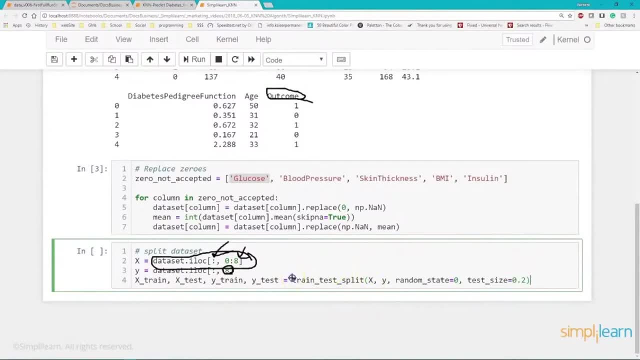 remember we imported the train test split. That's part of the A learn right there And we simply put in our X and our Y. We're going to do random. state equals zero. You don't have to necessarily seed it, That's a. 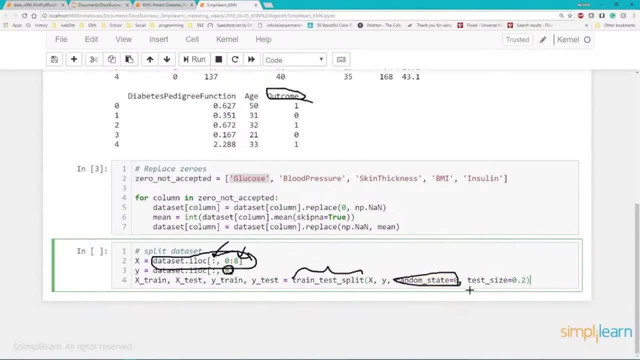 seed number. I think the default is one when you seed it. I'd have to look that up. And then the test size. Test size is point two. That simply means we're going to take twenty percent of the data and put it aside. 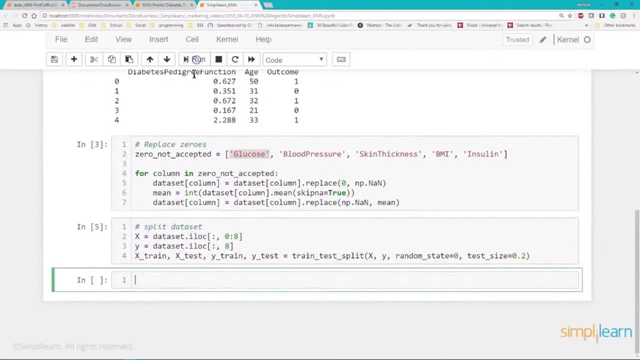 so that we can test it later. That's all that is, And again we're going to run it. Not very exciting. So far we haven't had any printout other than to look at the data. But that is a lot of. this is prepping. 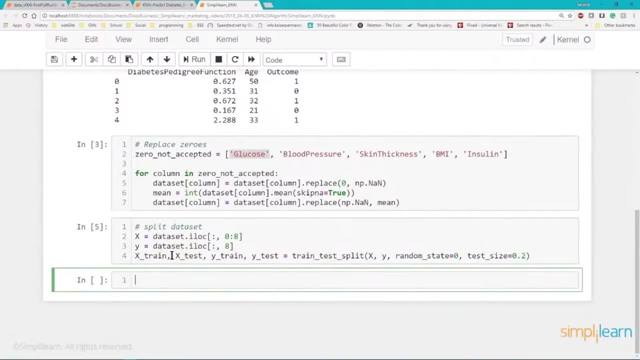 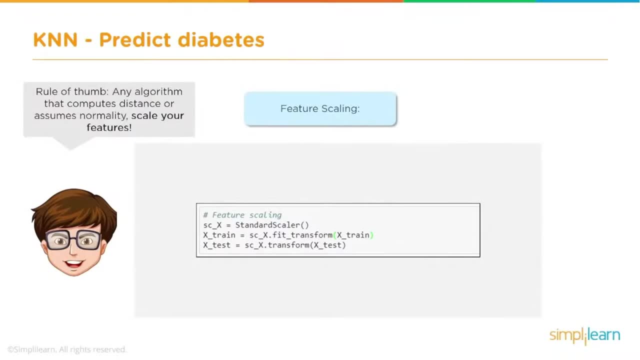 this data. Once you prep it, the actual lines of code are quick and easy And we're almost there with the actual running of our KNN. We need to go ahead and do a scale the data. If you remember correctly, we're fitting the data in a standard. 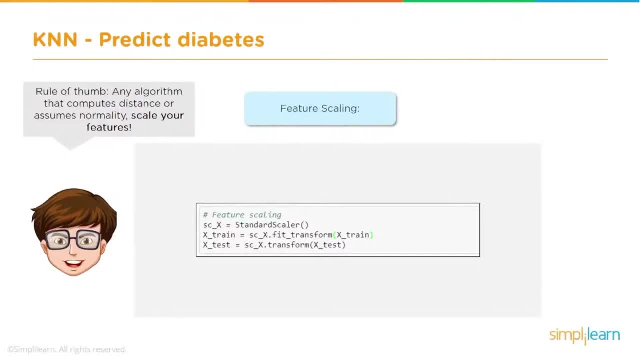 scalar, which means, instead of the data being from five to three hundred and three in one column and the next column is one to six, We're going to set that all so that all the data is between minus one and one. That's what that standard scalar. 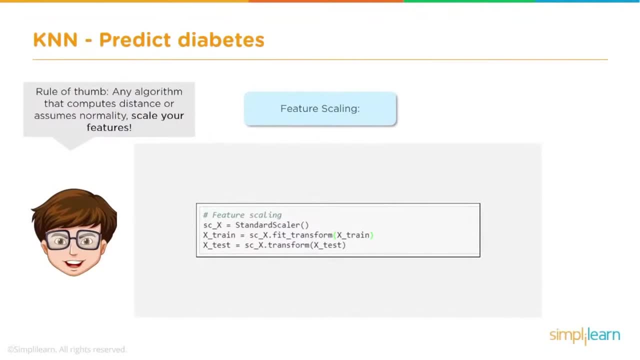 does Keeps it standardized, And we only want to fit the scalar with the training set. But we want to make sure the testing set is the X test going in is also transformed, So it's processing it the same. So here we go with our standard scalar. 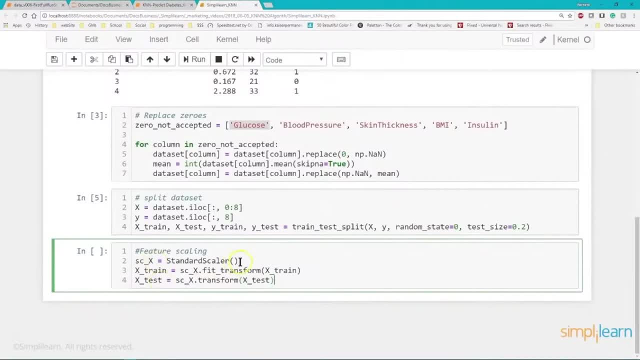 We're going to call it SC underscore X for the scalar And we're going to import the standard scalar into this variable and then our X train equals SC underscore X, dot fit transform. So we're creating the scalar on the X train variable And then our X test. we're also 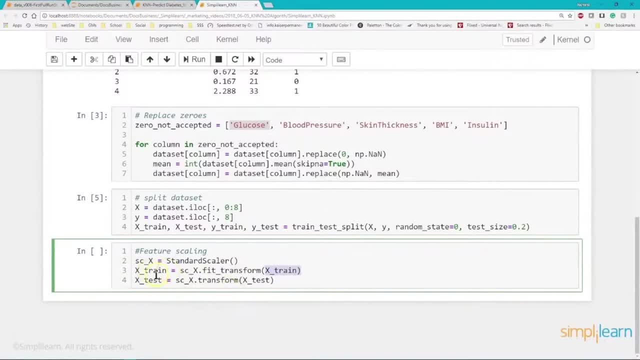 going to transform it. So we've trained and transformed the X train, and the X test isn't part of that training. It isn't part of training the transformer. It just gets transformed. That's all it does. And again, we're going to go ahead and run this. And if you look at this, 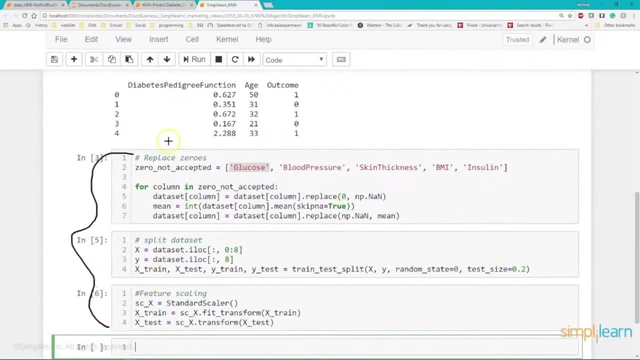 we've now gone through these steps, All three of them. We've taken care of replacing our zeros for key columns that shouldn't be zero And we've replaced that with the means of those columns, That way that they fit right in with our data. 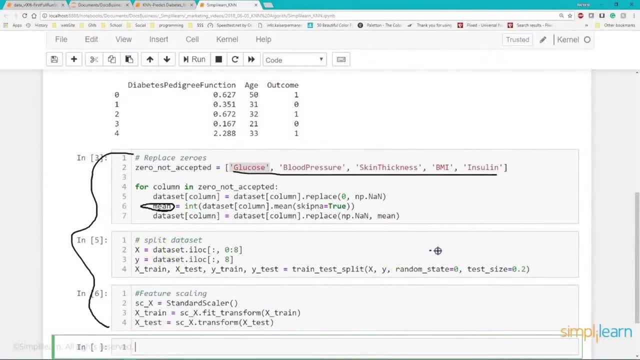 models. We've come down here and we've split the data. So now we have our test data and our training data, And then we've taken and we've scaled the data. So all of our data going in Now? no, we don't. 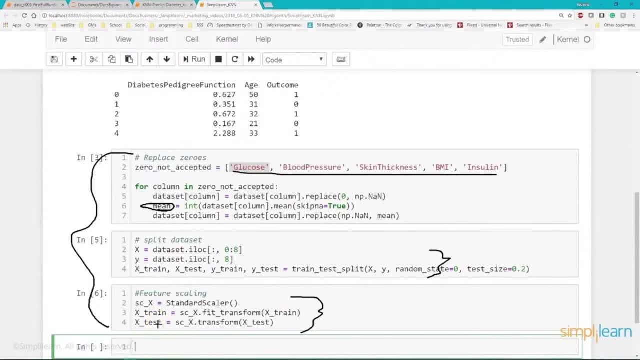 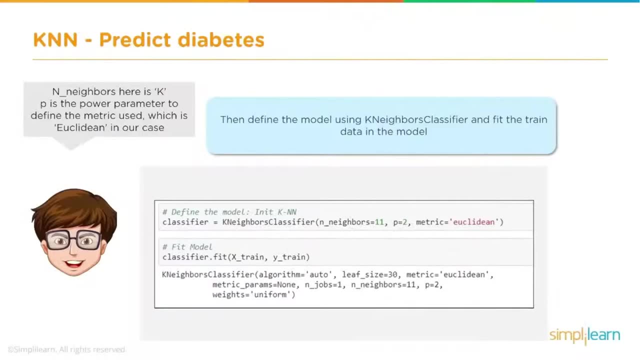 train the Y part, The Y train and Y test. That never has to be trained, It's only the data going in. That's what we want to train in there. Then define the model using KNeighborsClassifier and fit the train data in the model. 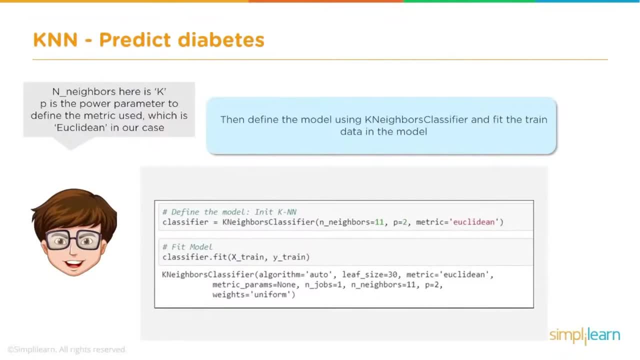 So we do all that data prep And you can see down here we're only going to have a couple lines of code where we're actually building our model and training it. That's one of the cool things about Python and how far we've come. It's such an. 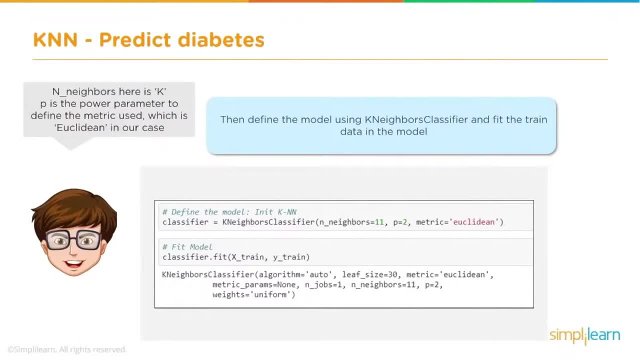 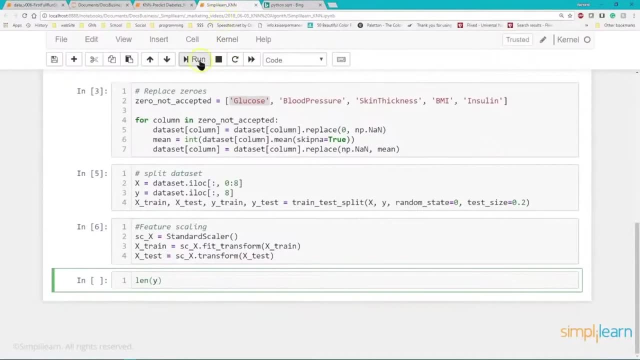 exciting time to be in machine learning because there's so many automated tools. Let's see, before we do this, let's do a quick length of and let's do Y. We want, let's just do length of Y And we get 768.. And if we 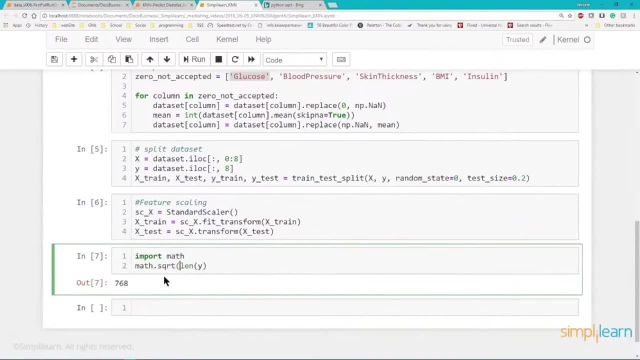 import math. we do math, dot square root. Let's do Y train. There we go. It's actually supposed to be X train. Before we do this, let's go ahead and do import math and do math square root. length of Y test. 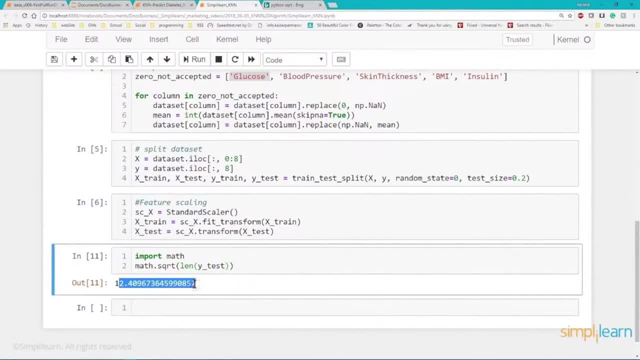 And when I run that we get 12.409.. I want to show you where this number comes from. we're about to use. 12 is an even number. So if you know, if you're ever voting on things, remember the neighbors all vote, don't want. 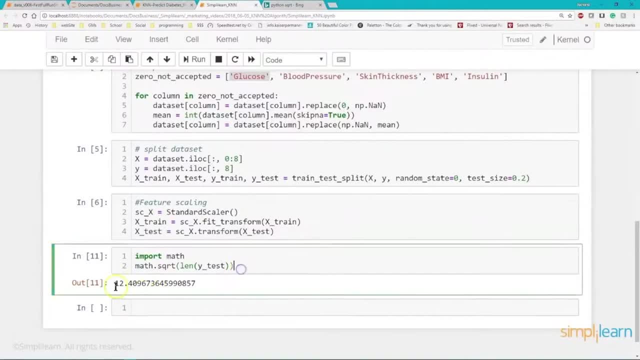 to have an even number of neighbors voting. So we want to do something odd And let's just take one away and we'll make it 11.. Let me delete this out of here. That's one of the reasons I love Jupyter Notebook, because you can flip around and do all. 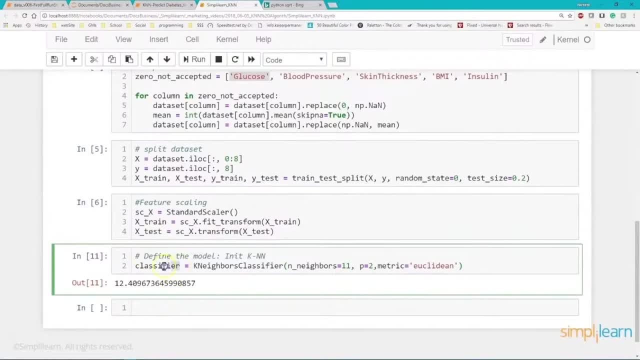 kinds of things on the fly, So we'll go ahead and put in our classifier. We're creating our classifier now And it's going to be the kNeighbors classifier. nNeighbors equals 11.. Remember we did 12 minus 1 for 11. So we have an odd number. 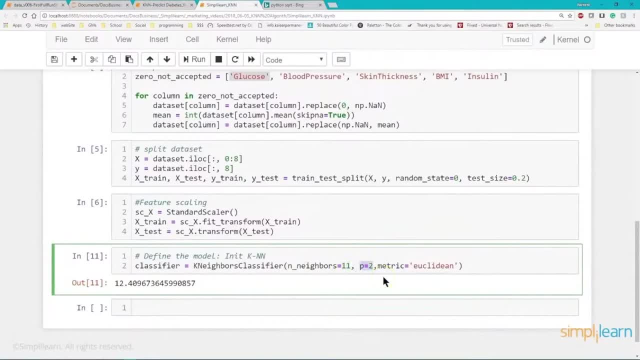 of neighbors. p equals 2, because we're looking for is it, are they diabetic or not? And we're using the Euclidean metric. There are other means of measuring the distance. You could do like square means, values, all kinds of measure. 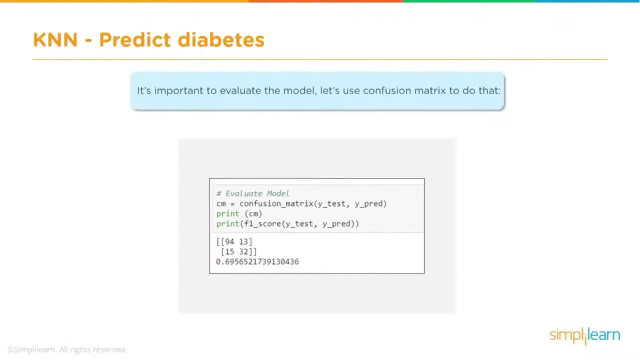 this, But the Euclidean is the most common one and it works quite well. It's important to evaluate the model. Let's use the confusion matrix to do that. And we're going to use the confusion matrix, Wonderful tool, And then we'll. 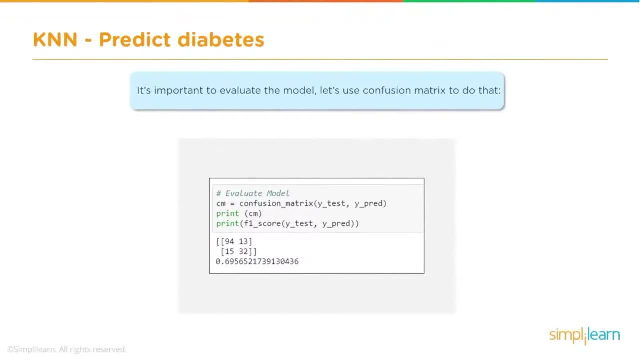 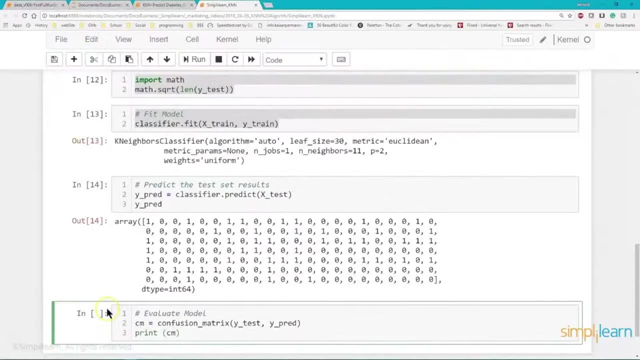 jump into the F1 score And finally, accuracy score, which is probably the most commonly used quoted number when you go into a meeting or something like that. So let's go ahead and paste that in there And we'll set the cm equal to. 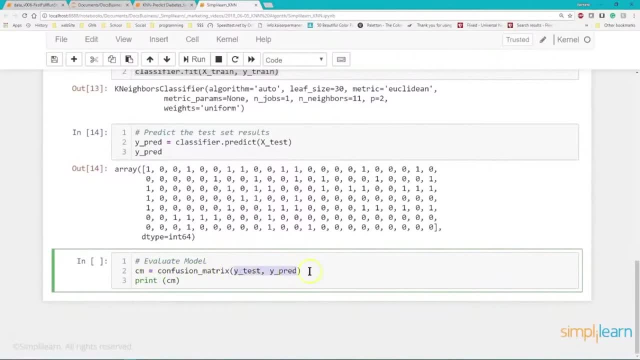 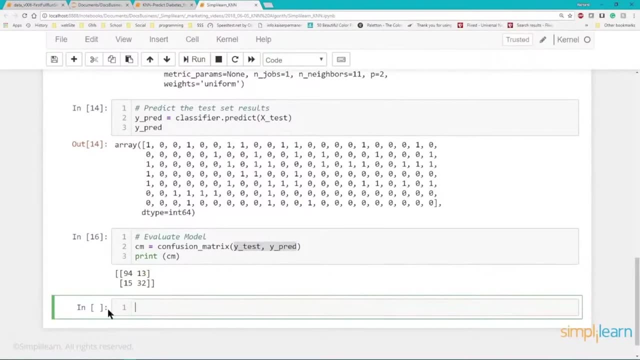 confusion. matrix y test: y predict. So those are the two values we're going to put in there. Let me go ahead and run that and print it out And the way you interpret this is: you have the y predict, which would be your title, up here. 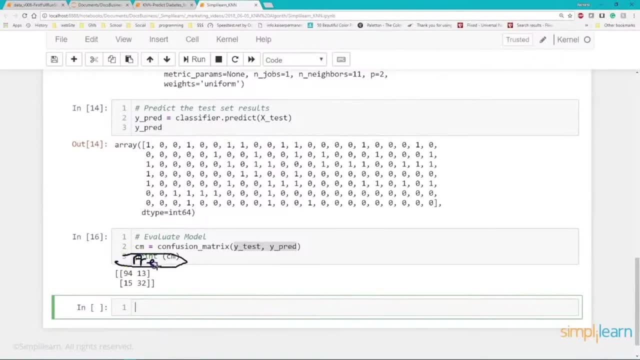 Let's just do: pred Predicted across the top and actual going down. It's always hard to write in here. actual That means that this column here down the middle that's the important column And it means that our prediction said 94 and 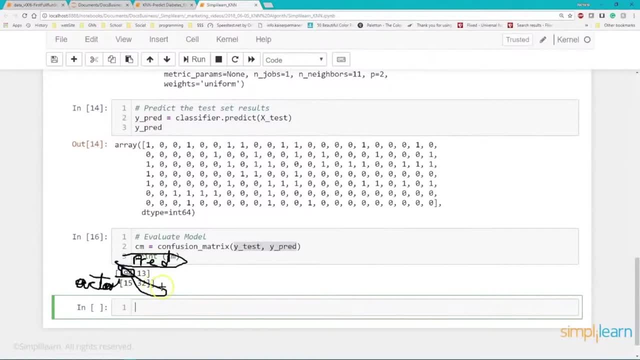 prediction and the actual agreed on 94 and 32.. This number here, the 13 and the 15, those are what was wrong. So you could have like three different. if you're looking at this across three different variables instead of just two, you'd end up with the third row down. 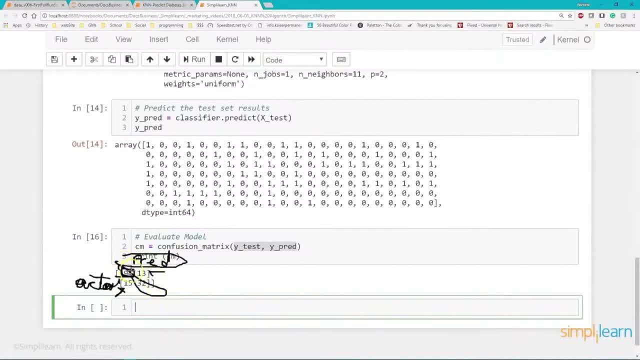 here and the column going down the middle. So in the first case we have the and I believe the zero is the 94, people who don't have diabetes. The prediction said that 13 of those people did have diabetes and were at high risk And the 32 that 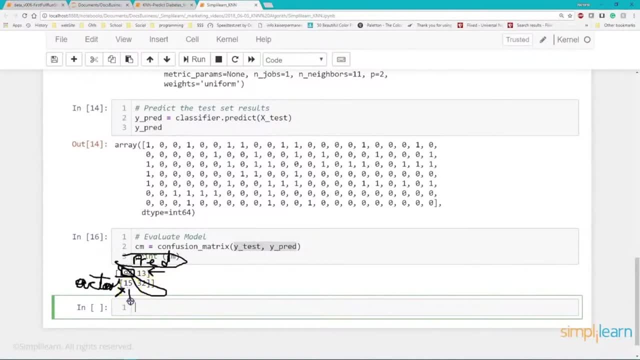 had diabetes. it had correct, But our prediction said another 15 out of that 15 it classified as incorrect. So you can see where that classification comes in and how that works on the confusion matrix. Then we're going to go ahead and print the F1 score. 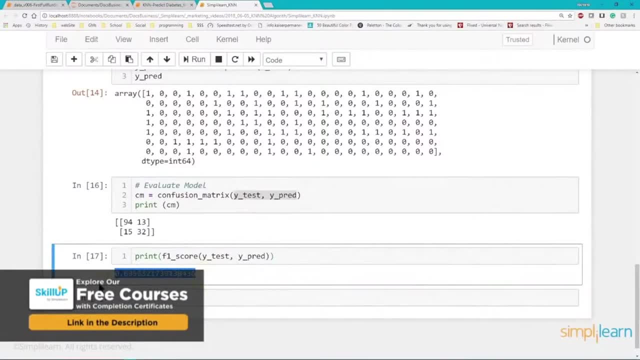 Just run that And you see we get a .69 in our F1 score. The F1 takes into account both sides of the balance of false positives, Where, if we go ahead and just do the accuracy account- and that's what most people think of- 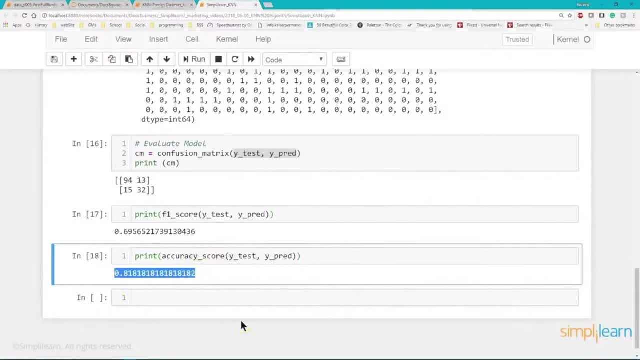 is. it looks at just how many we got right out of how many we got wrong. So a lot of people, when you're a data scientist and you're talking to other data scientists, they're going to ask you what the F1 score or the F score is, If you're. 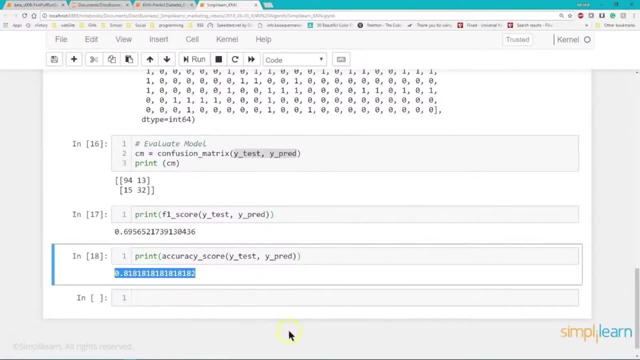 talking to the general public or the decision makers in the business. they're going to ask what the accuracy is, And the accuracy is always better than the F1 score. But the F1 score is more telling. It lets us know that there's more false positives. 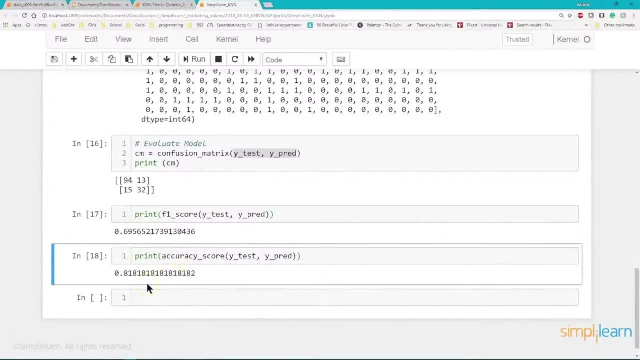 than we would like on here, But 82%, not too bad for a quick flash look at people's different statistics and running an KLearn and running the KNN, the K nearest neighbor, on it. So we have created a model using KNN which can predict whether 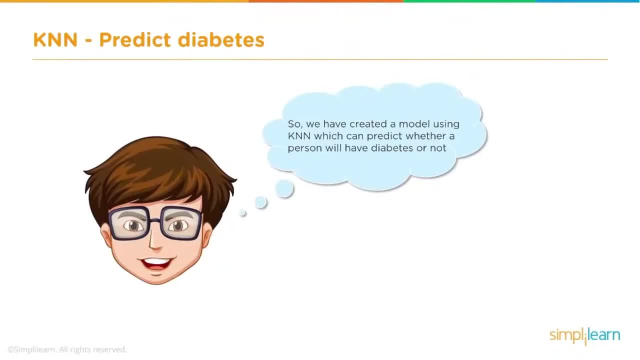 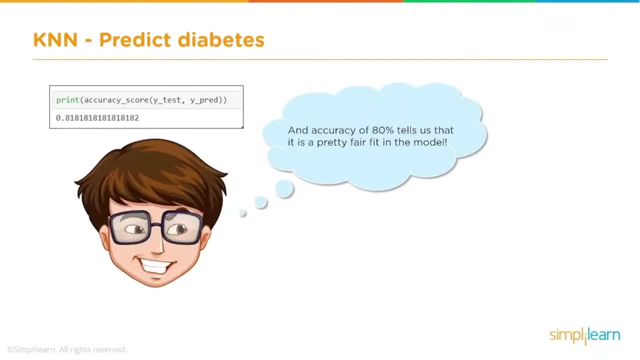 a person will have diabetes or not, or at the very least, whether they should go get a checkup and have their glucose checked regularly or not. The print accuracy score we got- the .818- was pretty close to what we got, and we can pretty much round that off and just say. 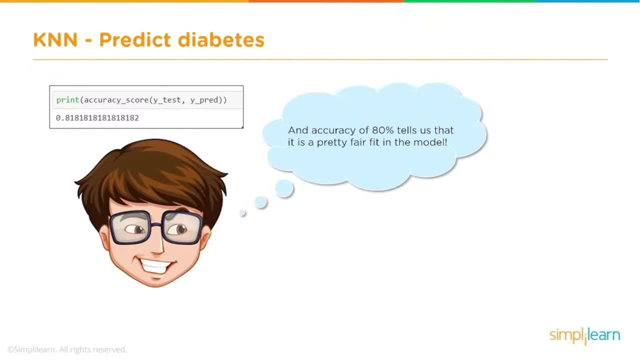 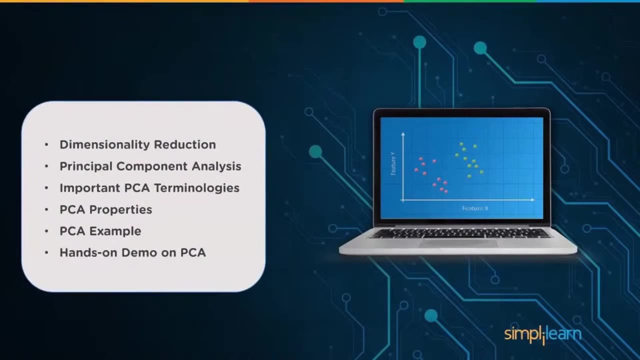 we have an accuracy of 80% Tells us it is a pretty fair fit in the model. The principal component analysis: we're going to cover dimensionality reduction. principal component analysis. what is it important? PCA terminologies, and you'll see it abbreviated normally as: 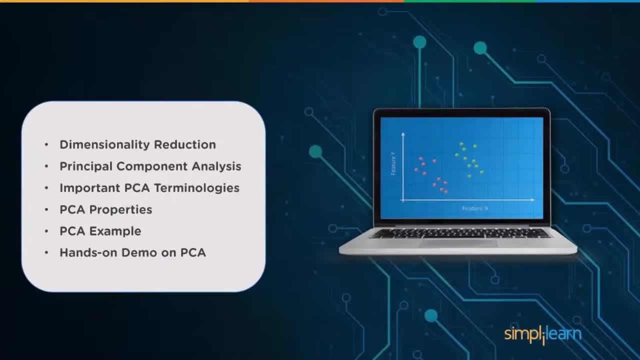 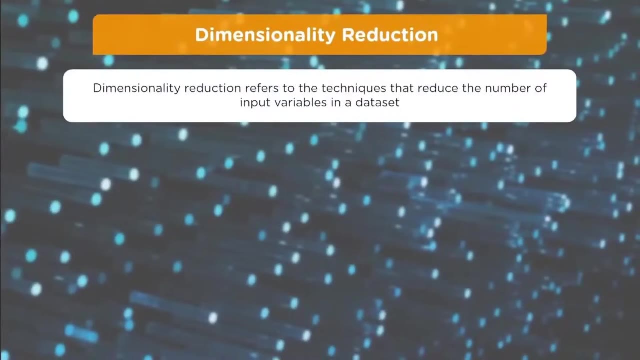 PCA: principal component analysis, PCA properties, PCA example. and then we'll pull up some Python code in our Jupyter notebook and have some hands on demo on the PCA and how it's used. Dimensionality reduction: Dimensionality reduction refers to the technique that reduces the 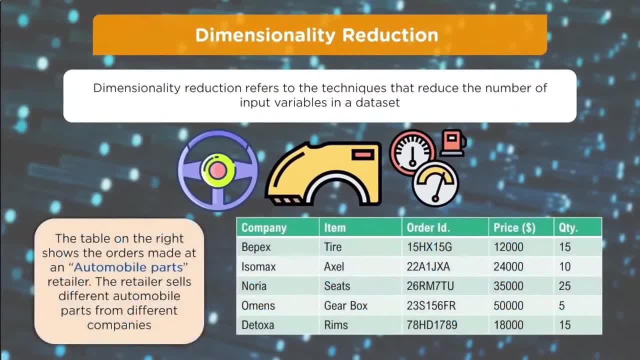 number of input variables in a data set And so you can see on the table on the right shows the orders made at an automobile parts retailer. The retailer sells different automobile parts from different companies And you can see we have company Bpex, Isomax and they have the. 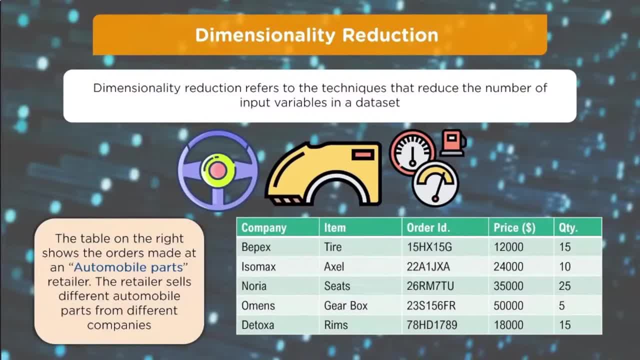 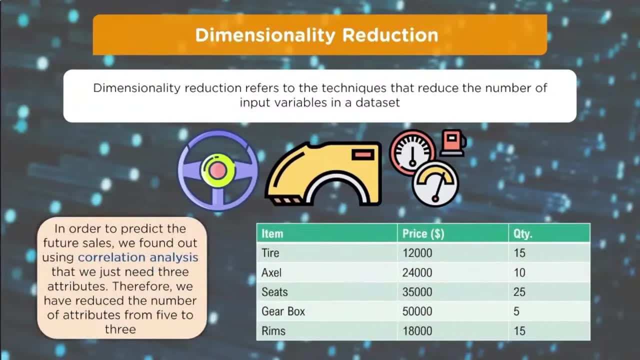 item, the tire, the axle, an order ID, a price number and a quantity In order to predict the future cells. we find out that, using correlation analysis, that we just need three attributes. Therefore, we have reduced the number of attributes. 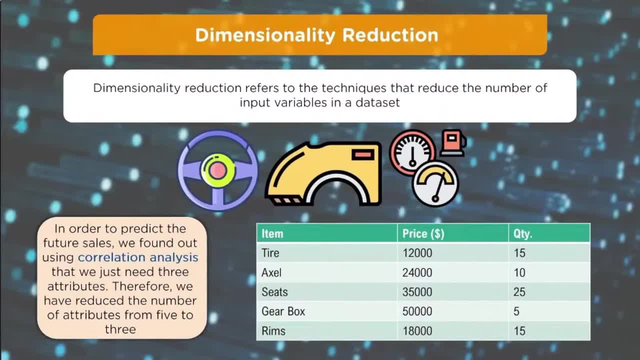 from five to three, And clearly we don't really care about the part number. I don't think the part number would have an effect on how many tires are bought, And even the store who's buying them probably does not have an effect on that. In this case, that's what they've. 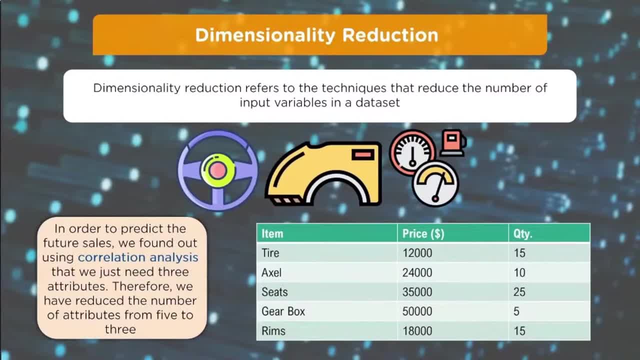 actually done is remove those And we just have the item, the tire, the price and the quantity. One of the things you should be taking away from this is: in the scheme of things, we are in the descriptive phase. We're describing the data. 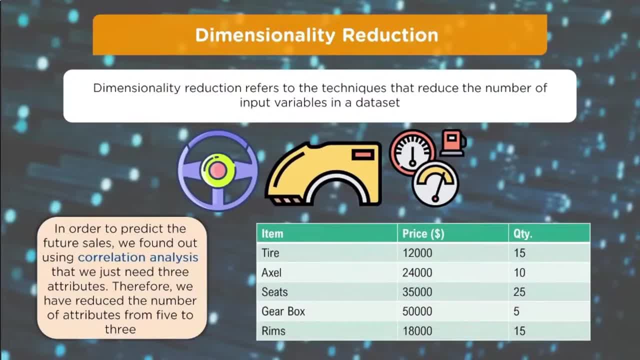 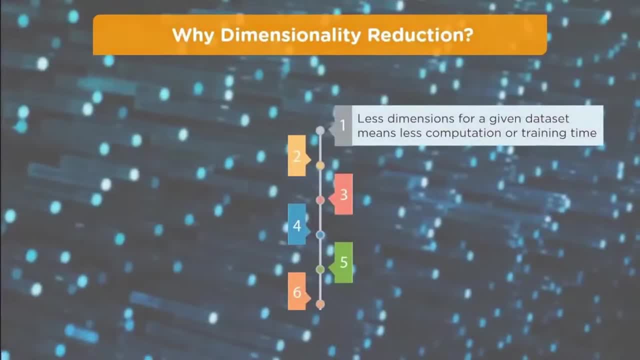 and we're pre-processing the data. What can we do to clean it up? Why dimensionality reduction? Well, number one: less dimensions for a given data set means less computation or training time. That can be really important if you're trying a number of different models. 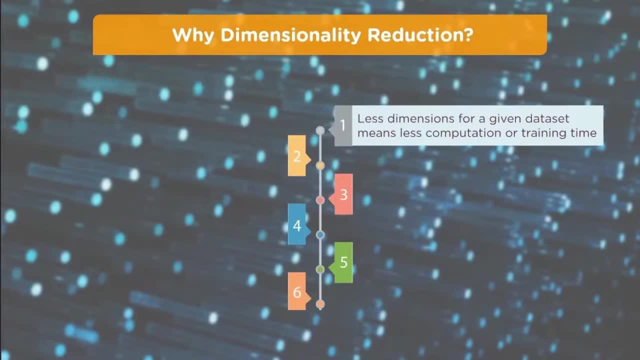 and you're re-running them over and over again. And even if you have seven gigabytes of data, that can start taking days to go through all those different models. So this is huge. This is probably the hugest part as far as reducing. 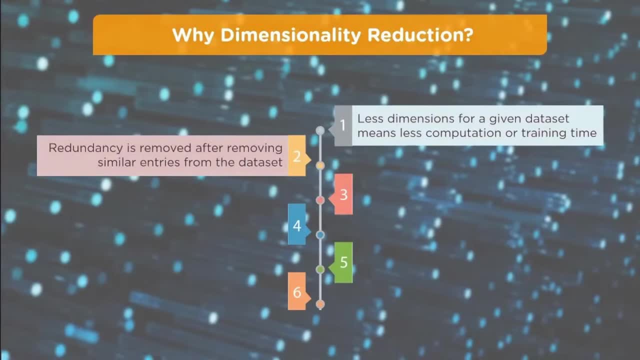 our data set. Redundancy is removed after removing similar entries from the data set, Again pre-processing some of our models. like a neural network, if you put in two of the same data, it might give them a higher weight than they. 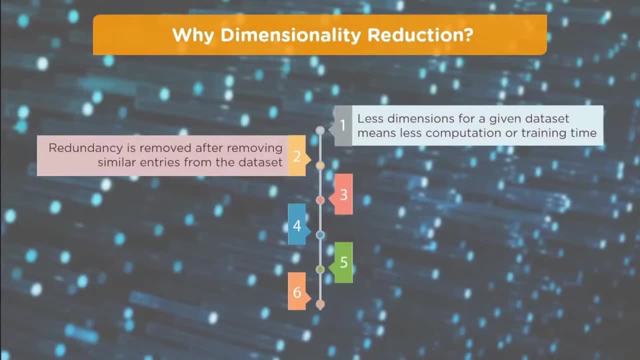 would if it was just once. We want to get rid of that redundancy. It also increases the processing time. if you have multiple data coming in, Space required to store the data is reduced. So if we're committing this into a big data pool, 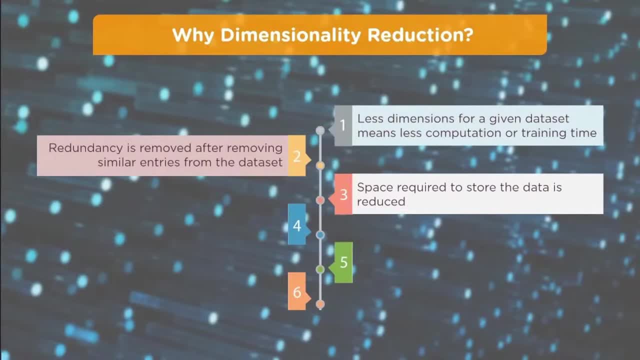 we might not send the company that bought it. Why would we want to store two whole extra columns when we add it into that pool of data? Makes the data easy for plotting in 2D and 3D plots. This is my favorite part. 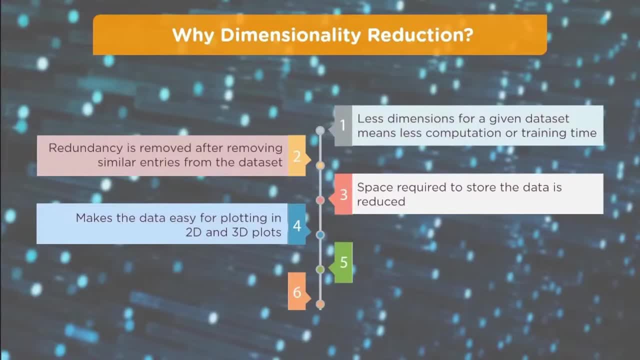 Very important. You're in your shareholder meeting. You want to be able to give them a really good, clear and simplified version. You want to reduce it down to something people can take in. It helps to find out the most significant features and skip the rest. 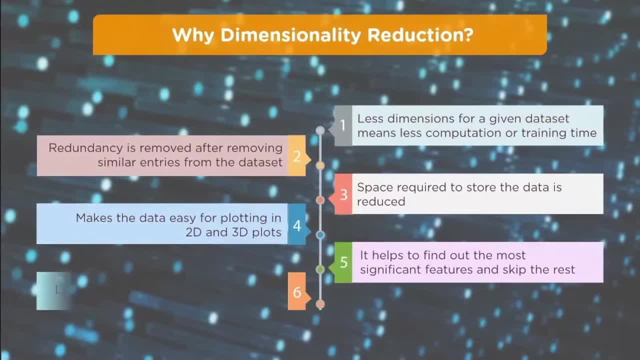 Which also comes in in post-scribing, Leads to better human interpretation. That kind of goes with number four: what makes data easy for plotting? You have a better interpretation when we're looking at it: Principal component analysis. So what is it? 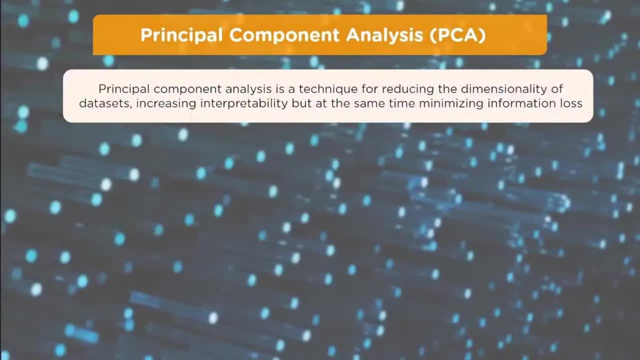 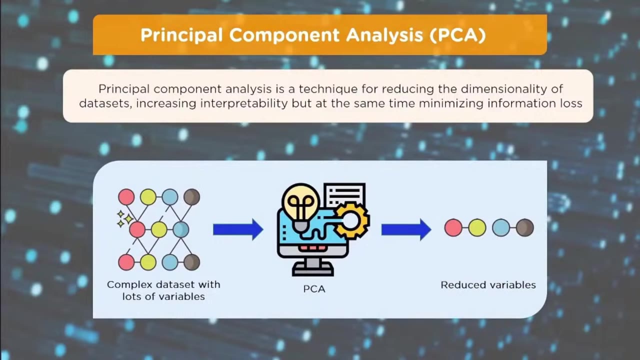 Principal component analysis is a technique for reducing the dimensionality of data sets, increasing interpretability but at the same time minimizing information loss. So we take some very complex data set with lots of variables, We run it through the PCA, We reduce the variables. 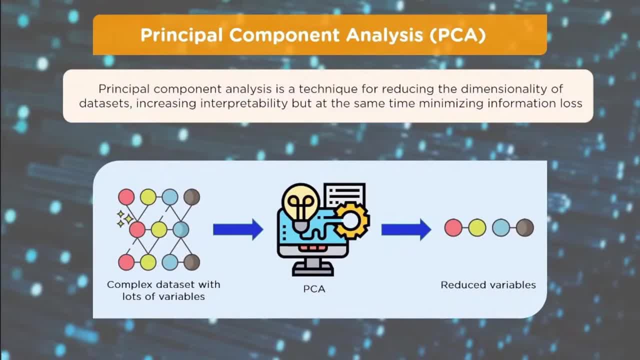 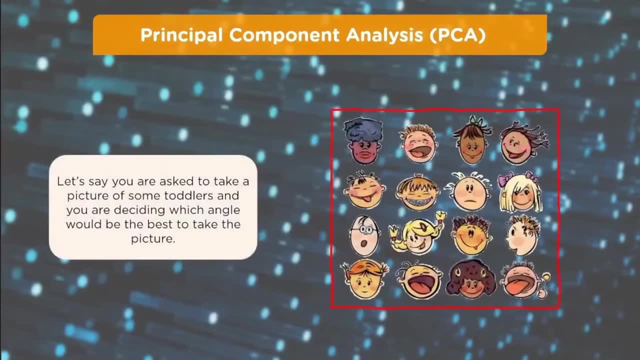 We end up with a reduced variable set up. This is very confusing to look at Because if you look at the end result, we have the different colors all lined up. So what we're going to take a look at is, let's say, we have a picture here. 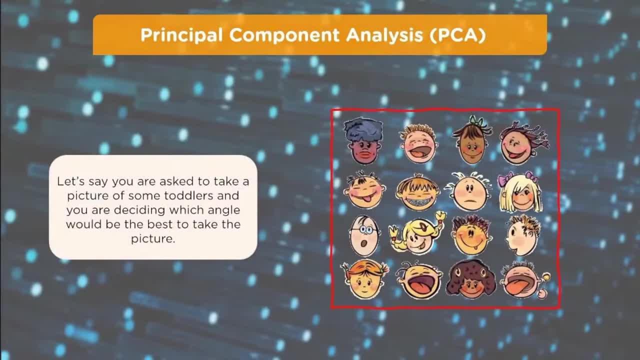 Let's say you are asked to take a picture of some toddlers and you are deciding which angle would be the best to take the picture from. So if we come up here and we look at this, we say, okay, this is one angle. 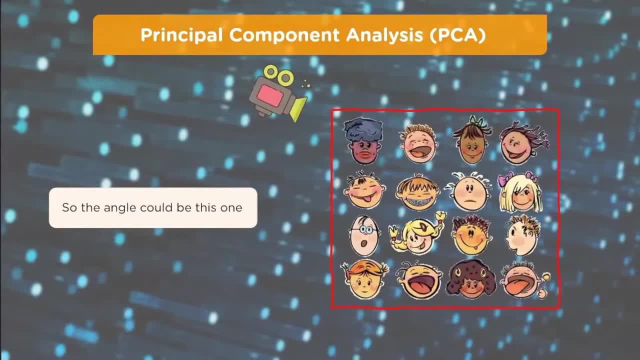 We get the back of a lot of heads, not many faces, So we'll do it from here. We might get the one person up front smiling. A lot of the people in the class are missing, So we have a huge amount off to the right of blank space. 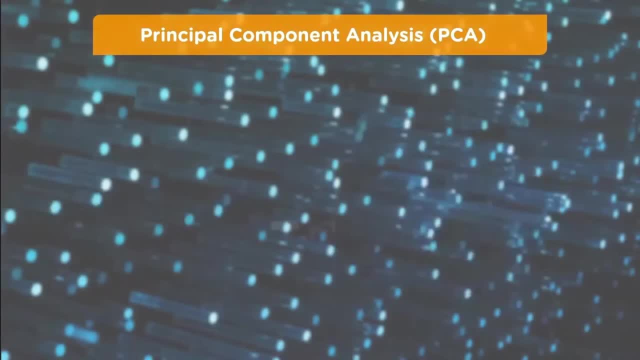 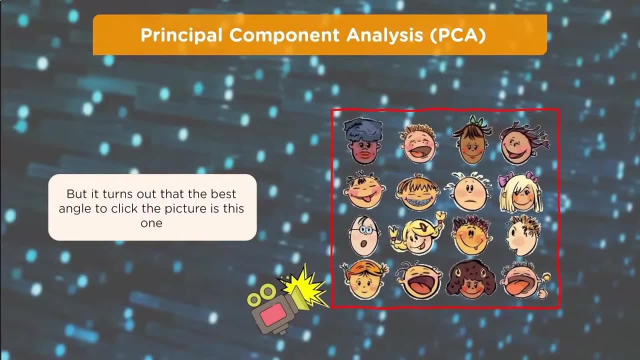 Maybe from up here. Again, we have the back of someone's head And it turns out that the best angle to click the picture from might be this bottom left angle. You look at it and you say, hey, that makes sense, It's a good. 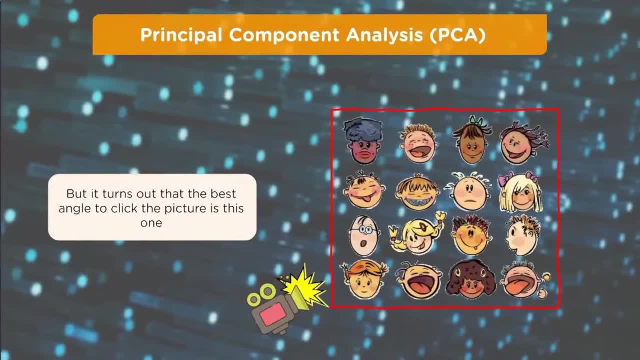 configuration of all the people in the picture. Now, when we're talking about data, it's not. you really can't do it by what you think is going to be the best. We need to have some kind of mathematical formula so it's consistent and so. 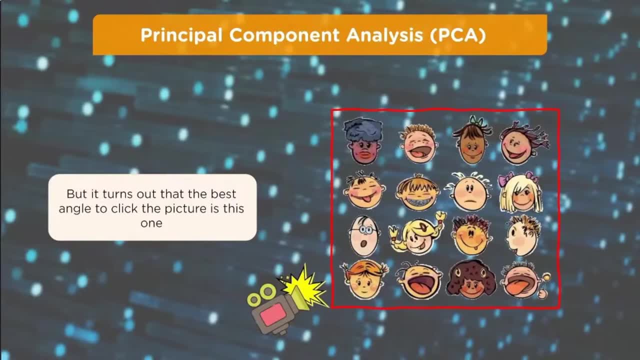 it makes sense in the back end. One of the projects I worked on many years ago has something similar to the iris. If you've ever done the iris data set, it's probably one of the most common ones out there where they have the flower. 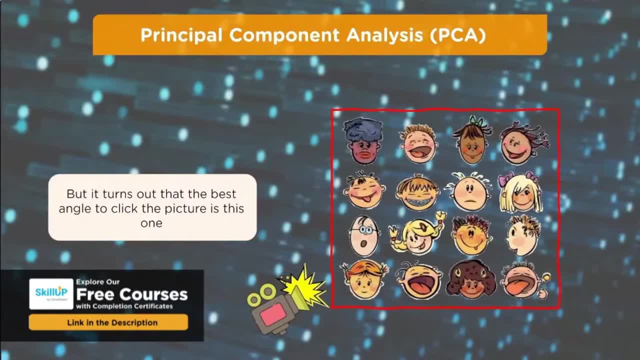 and they're measuring the stamen and the petals and they have width and they have length of the petal. Instead of putting through the width and the length of the petal, we could just as easily do the width to length ratio. We can divide the width. 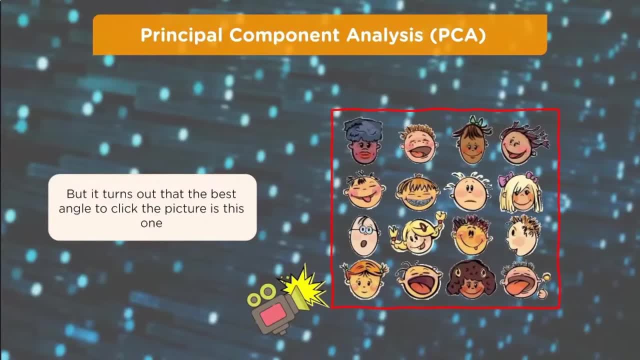 by the length and you get a single number where you had two. That's the kind of idea that's going on into this in pre-processing and looking at what we can do to bring the data down. A very simplified example on my iris petal: 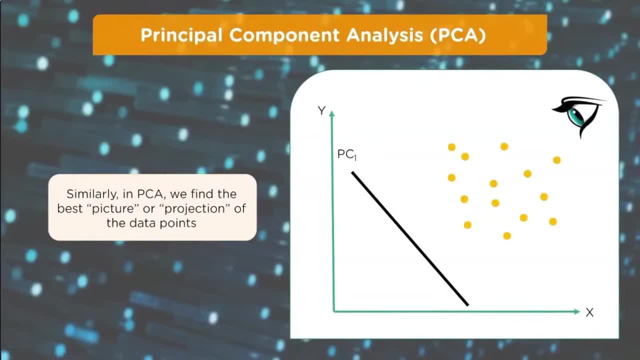 example, When we look at the similarity in PCA, we find the best picture or projection of the data points When we look down from one angle. we've drawn a line down there. we can see these data points based on, in this case, just two variables. 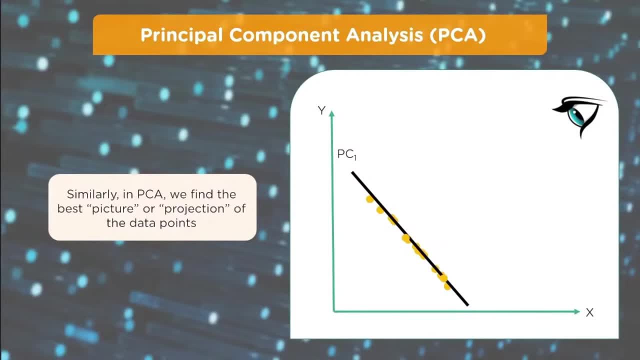 Keep in mind. we're usually talking about 36, 40 variables. Almost all of your business models usually have about 26 to 27 different variables. they're looking at Same thing with a bank loan model. We're talking 26 to 36 different variables. 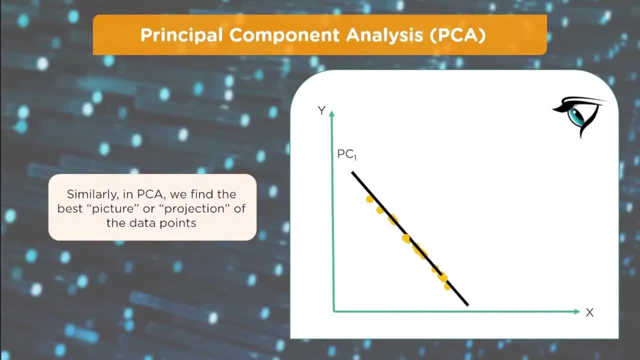 they're looking at that, are going in. What we want to do is we want to find the best view. In this case, we're just looking at the XY, We look down at it and we have our second idea, PC2.. 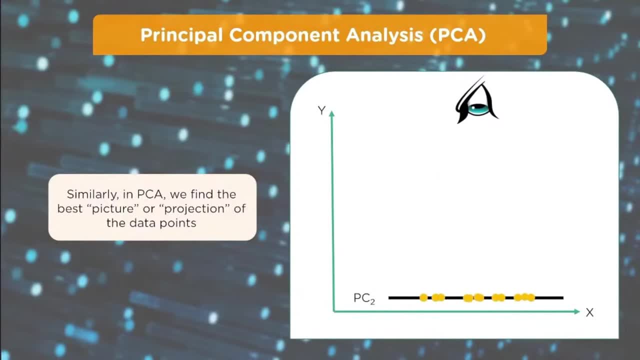 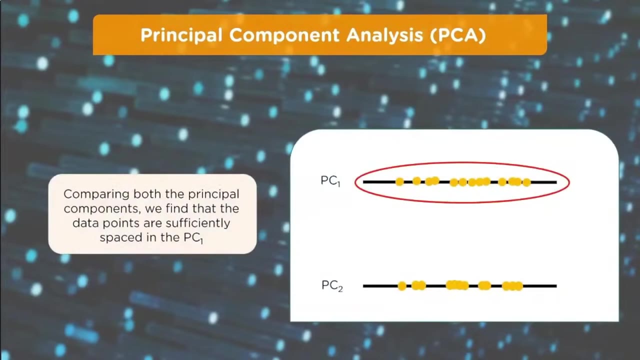 Again, we're looking at the XY, this time from a different direction. Here, for our ease, we can consider that we get two principal components, namely PC1 and PC2.. Comparing both the principal components, we find the data points are sufficiently spaced. 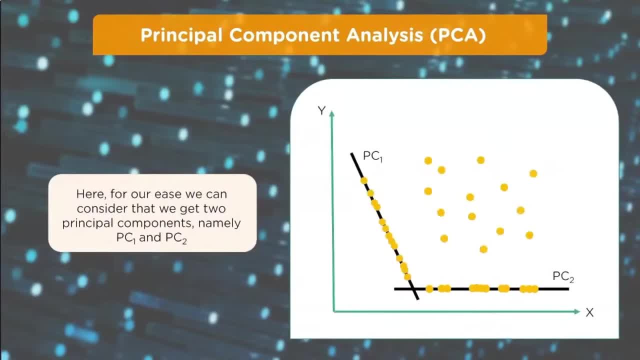 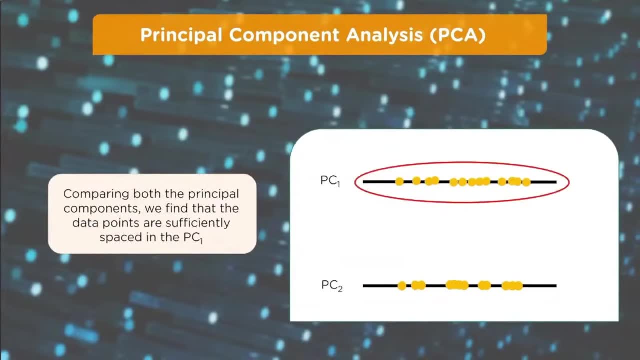 in PC1.. If you look at what we got here, we have PC1. You can see along the line how the data points are spaced versus the spacing in PC2.. That's what they're coming up with. What is going to give us the best look? 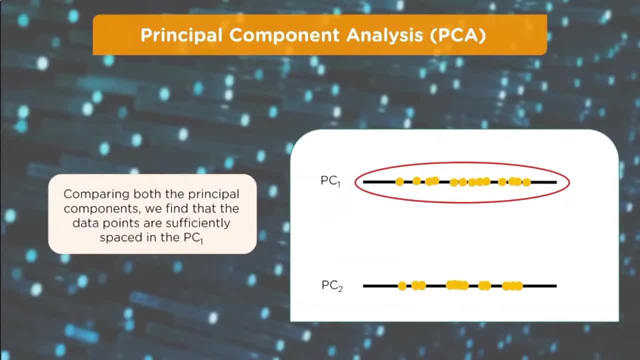 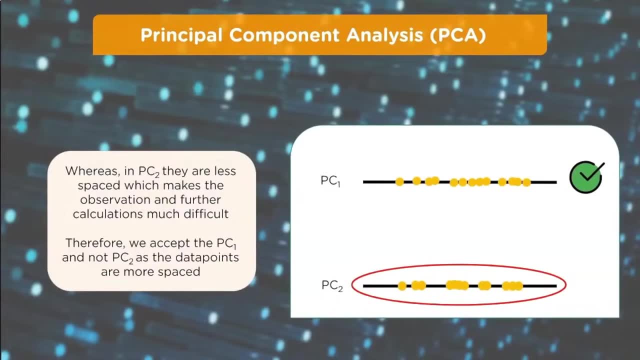 for these data points. when we combine them, We're looking at them from just a single angle, Whereas in PC2, they are less spaced, which makes the observation and further calculations much more difficult. Therefore, we accept the PC1 and not the PC2. 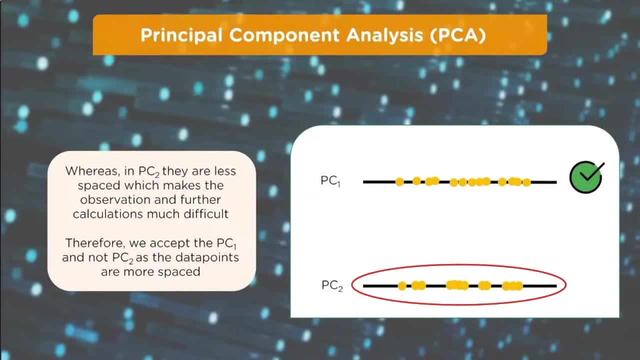 as the data points are more spaced. Obviously, the back-end calculations are a little bit more complicated when we get into the math of how they decide what is more valuable. This gives you an idea, though, that when we're talking about this, 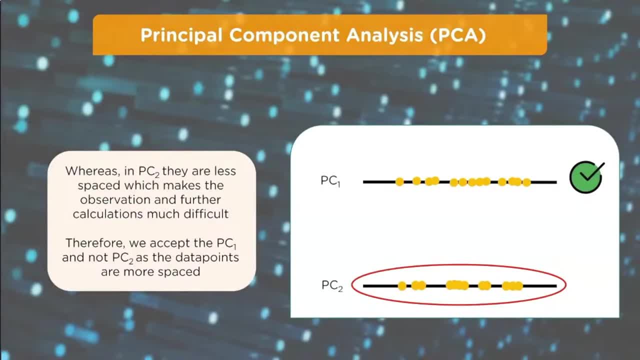 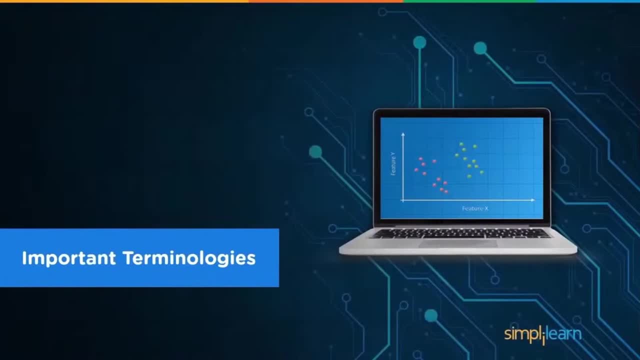 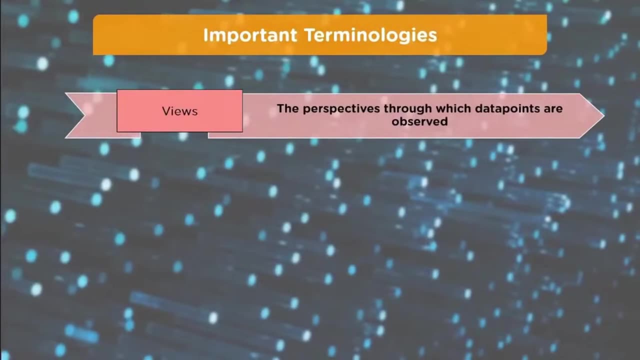 we're talking about the perspective, which would help in understanding how PCA analysis works. What we want to go ahead and do is dive into the important terminologies under PCA. Important terminologies are views, the perspective through which data points are observed. You'll hear that if someone's talking about 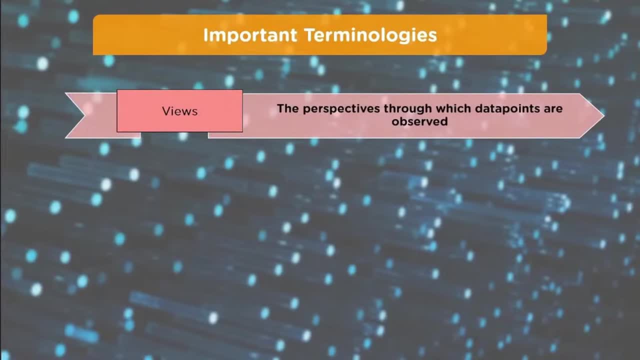 a PCA presentation and they're not taking the time to reduce it to something that the average person shareholders can understand. you might hear them refer to it as the different views. What view are we taking? Dimension: number of columns in a data set. 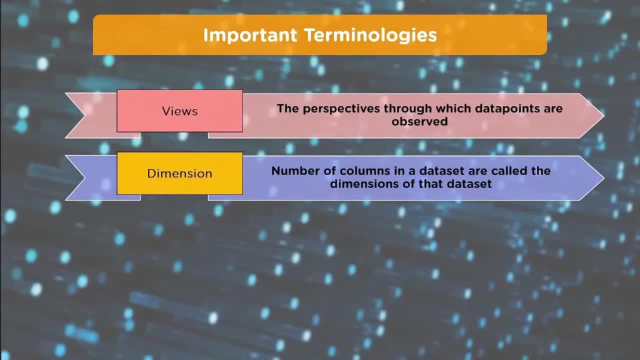 are called the dimensions of that data set We talked about. you'll hear features dimensions. I was talking about features. Usually, when you're running a business, you're talking 25,, 26,, 27 different features minimal. 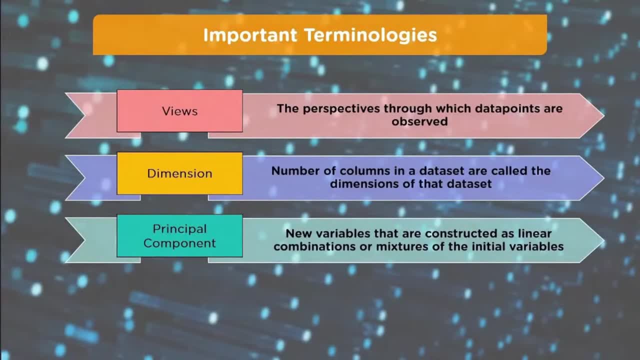 Then you have the principal component: new variables that are constructed as linear combinations or mixtures of the initial variables. Principal component is very important. It's a combination. If you remember my flower example, it would be the width over the length of the petal, as opposed to putting. 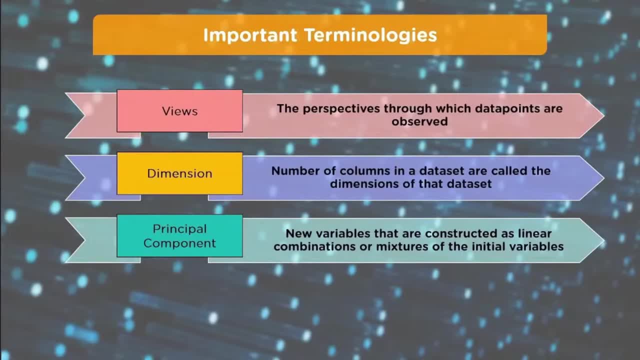 both width and length in. You just put in the ratio instead, which is a single number versus two separate numbers, Projections, The perpendicular distance between the principal component and the data points. That goes to that line we had earlier. It's that right angle line of where. 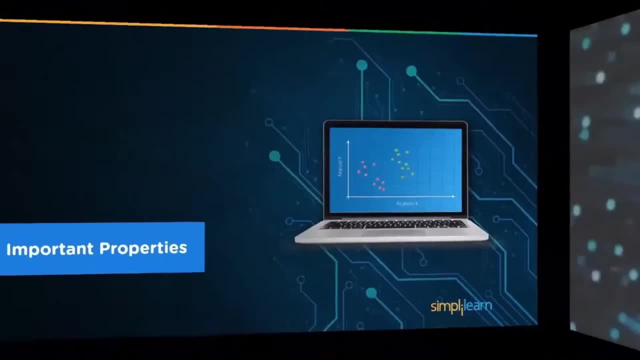 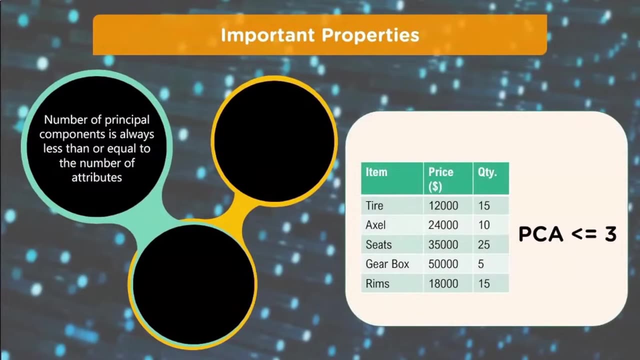 all those points fall onto the line Important properties. Important properties: Number of principal components is always less than or equal to the number of attributes. That just makes common sense. You're not going to do ten principal properties with only three features. You're trying to reduce them. so that's just. 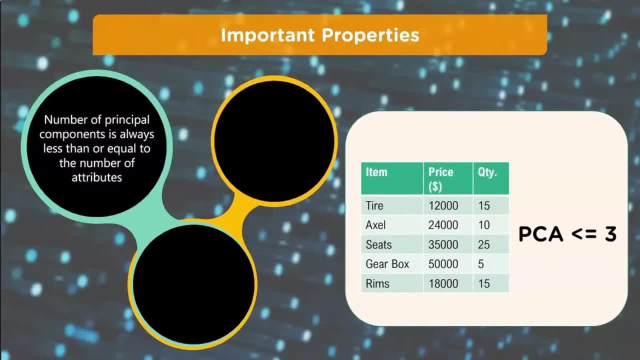 kind of goofy, but it is important to remember that People will throw weird code out there and just randomly do stuff instead of really thinking it through. Principal components are orthogonal. This is what we're talking about, that right angle from the line. 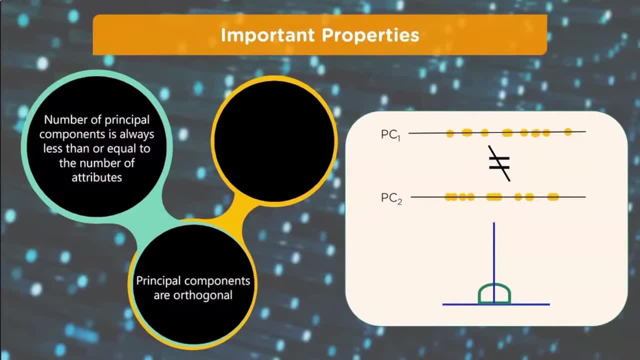 When we do PC1, we're looking at how those points fall onto that line. Same thing with PC2.. We want to make sure that PC1 does not equal PC2.. We don't want to have the same two principal points when we do. 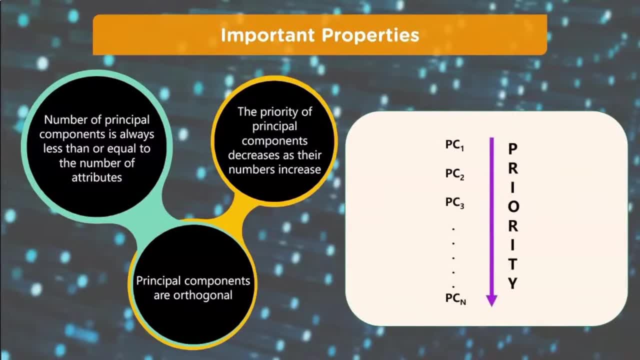 two points. The priority of principal components decreases as they're numbers increase. This is important to understand. If you're going to create one principal component, everything is summarized into that one component. As we go to two components, the priority, how much? 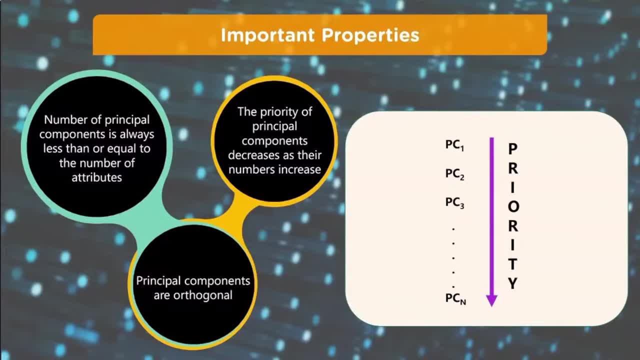 it holds value decreases as we go down. If you have five different points, each one of those points is going to have less value than just the one point which has everything summarized in it: How PCA works. I said there was more in the back end. 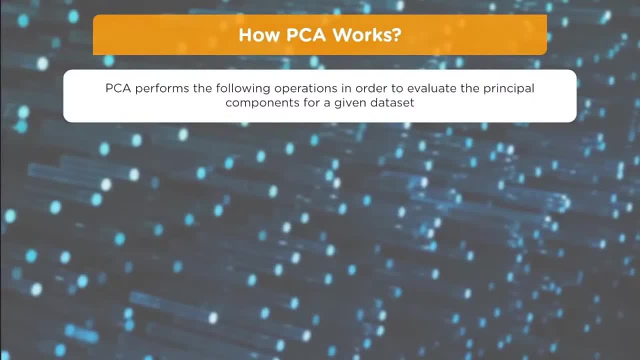 We talk about the math. This is what we're talking about. How does it actually work? Now we have an understanding. You're looking at a perspective. Now we want to see how that math side works. PCA performs the following operations in order to evaluate: 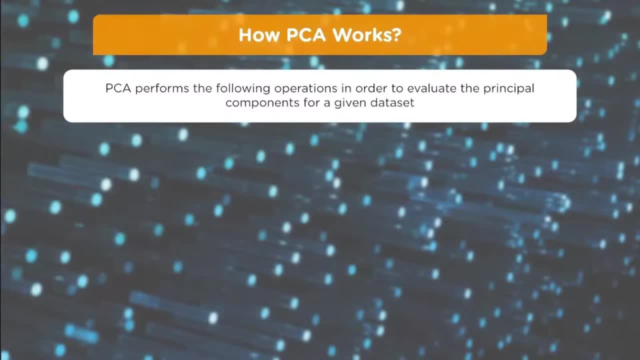 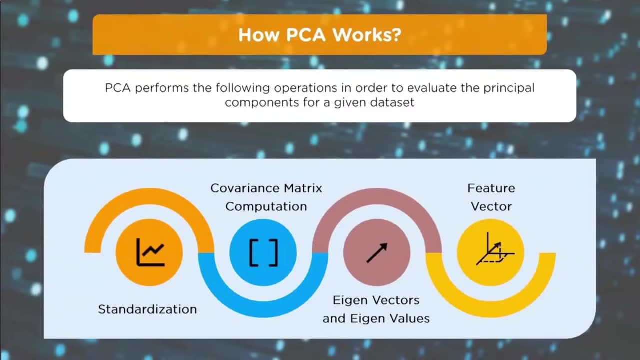 the principal components for a given data set. First we start with the standardization, Then we have a covariance matrix computation. We use that to generate our iGene vectors and iGene values, which is the feature vector. If you remember, the iGene vector is: 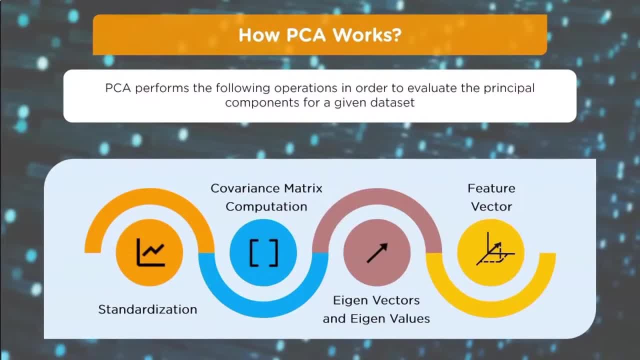 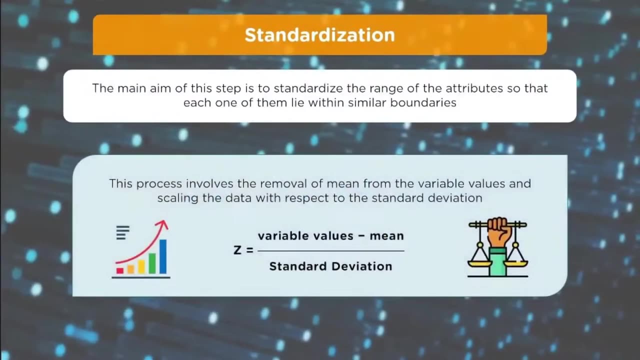 like a translation for moving the data from x equals one to x equals two or whatever altering it. The iGene value is the final value that we generate. We talk about standardization. The main aim of this step is to determine the range of the. 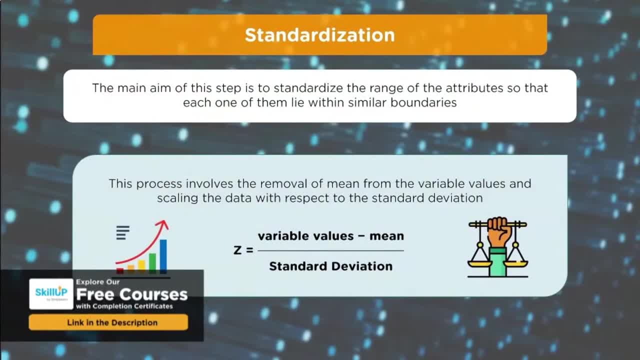 attributes so that each one of them lie within similar boundaries. This process involves removal of the mean from the variable values and scaling the data with respect to the standard deviation. You can see here we have: z equals the variable values minus the mean over the standard deviation. 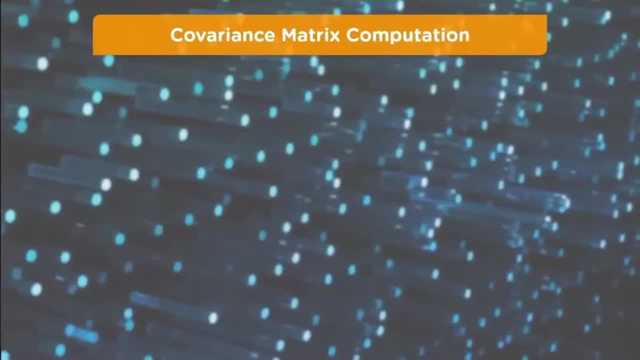 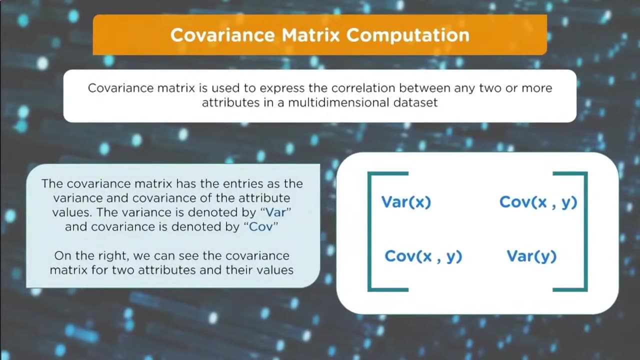 The covariance matrix computation. Covariance matrix is used to express the correlation between any two or more attributes in multidimensional data. The covariance matrix has the entries as the variance and covariance of the attribute values. The variance is denoted by var and the covariance is denoted by co. 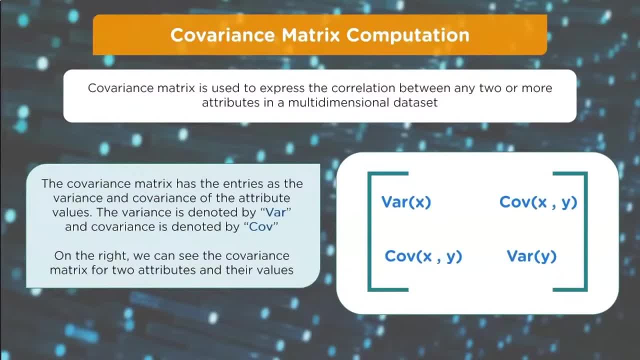 On the right we can see the covariance matrix for two attributes and their values. When we do a hands-on look at the code, we'll do a display of this so you can see what we're talking about and what that looks like. For now, you can just notice that. 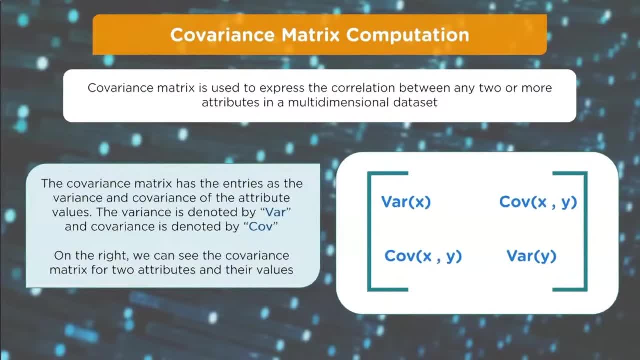 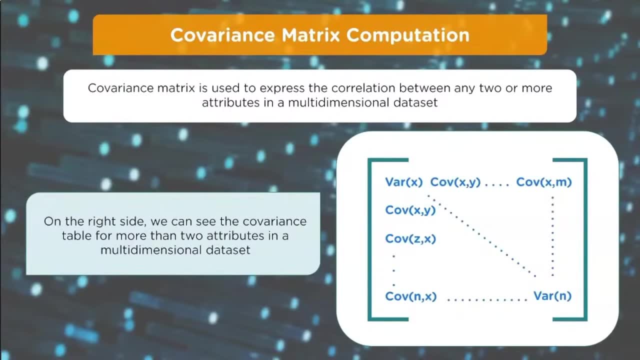 this is a matrix that we're generating with the variance and then the covariance matrix. On the right side we can see the covariance table for more than two attributes in a multidimensional data set. This is what I was talking about. We usually are looking at, not just 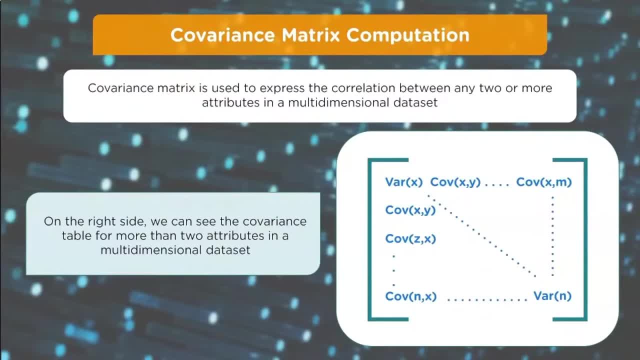 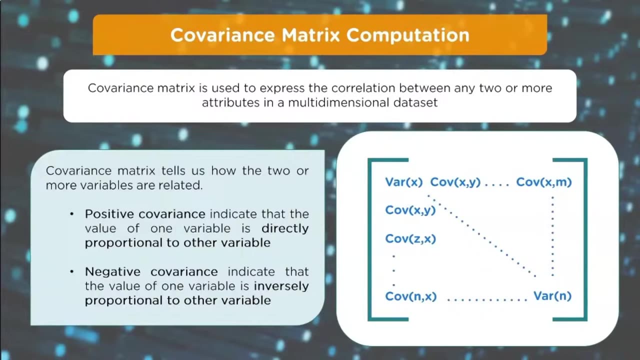 one feature or two features. we're usually looking at 25, 30 features going on. If we do a setup like this, we should see all those different features as the different variables. Covariance matrix tells us how the two or more variables are related. 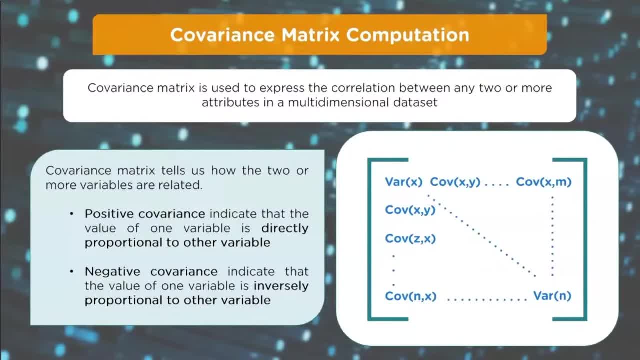 Positive covariance indicate that the value of one variable is directly proportional to the other variable. Negative covariance indicate that the value of one variable is inversely proportional to the other variable. That is always important to note whenever we're doing any of these matrices that we're going to be. 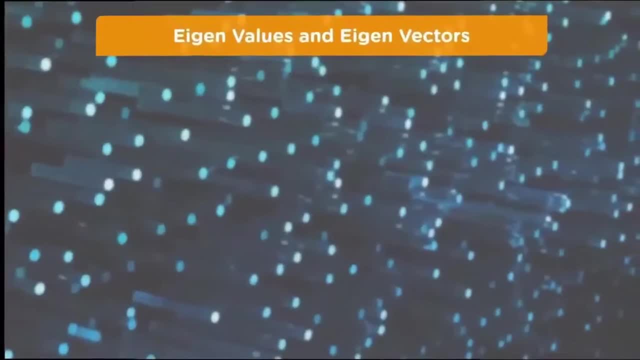 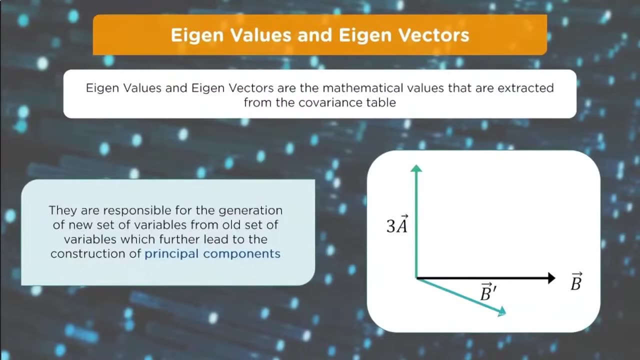 looking at that- positive and negative, whether it's inverted or not. And then we have the eigenvalues and the eigenvectors. Eigenvalues and eigenvectors are the mathematical value that are extracted from the old set of variables. They are responsible for the generation. 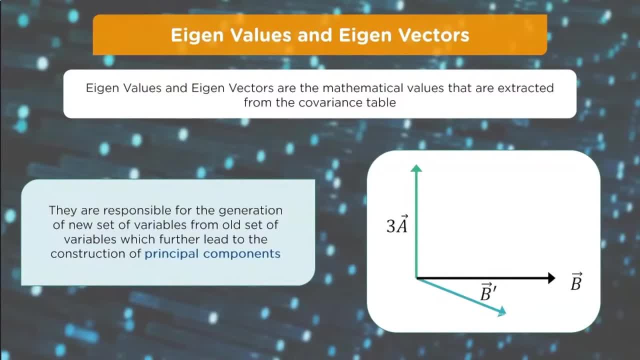 of a new set of variables from the old set of variables which further lead to the construction of the principal components. Eigenvectors do not change directions after linear transformation. Eigenvalues are the scalars or the magnitude of the eigenvectors. And again, 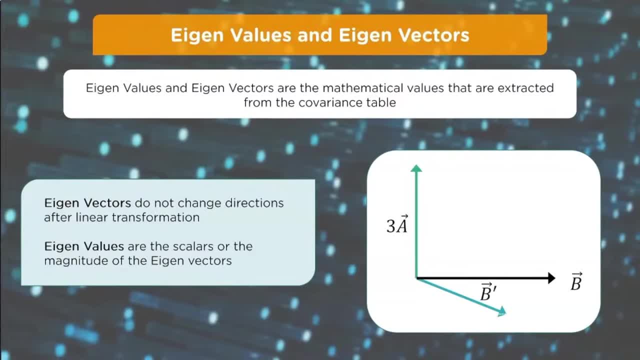 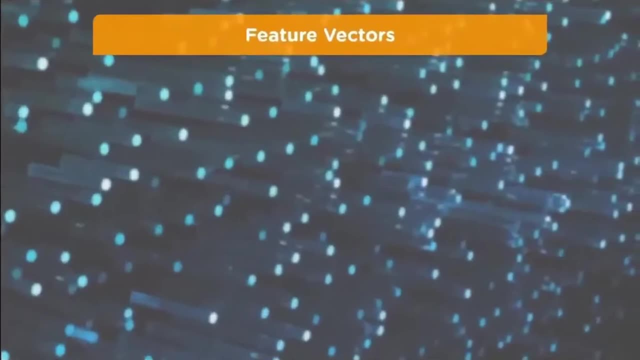 this is just transforming that data. So we're going to change the vector b to the b prime, as denoted on the chart, And so we have multiple variables. How do we calculate that new variable? And then we have feature vectors. Feature vectors is simply a matrix. 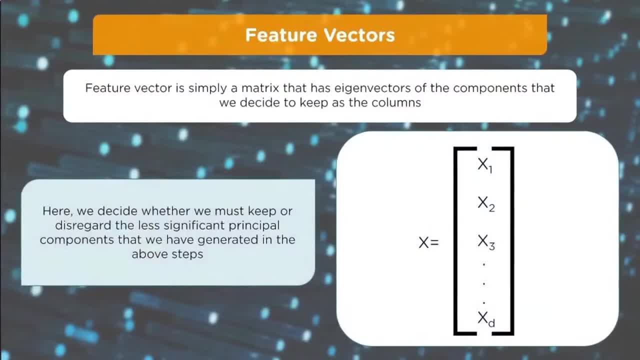 that has eigenvectors of the components that we decide to keep. as the columns Here we decide whether we must keep or discard the less significant principal components that we have generated in the above steps. This becomes really important as we start looking at the back end of this. 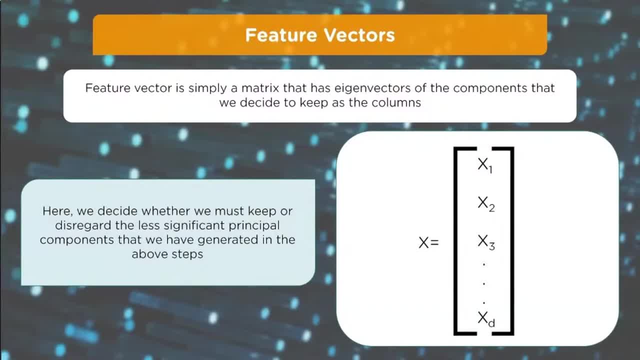 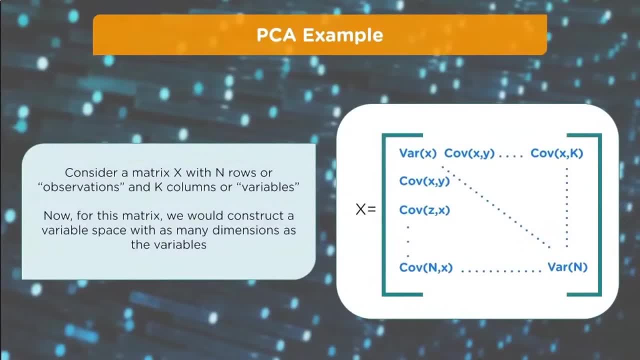 And we'll do this in the demo, But one of the more important steps to understand. And so we have the PCA example. Consider matrix X with n rows or observations, and k columns or variables. Now for this matrix, we would construct a variable space with as many dimensions. 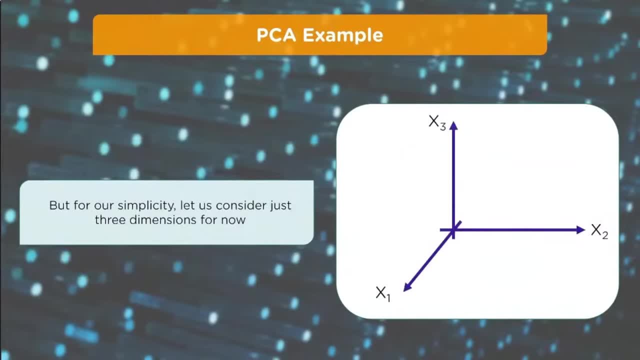 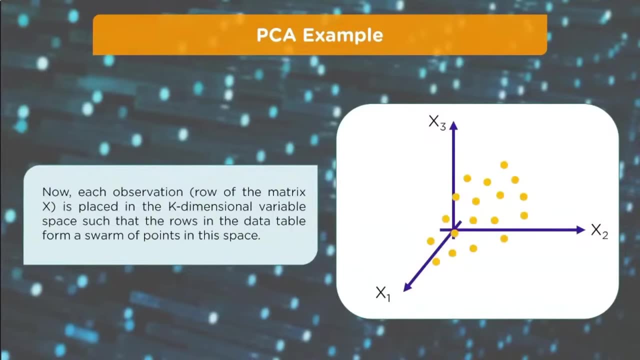 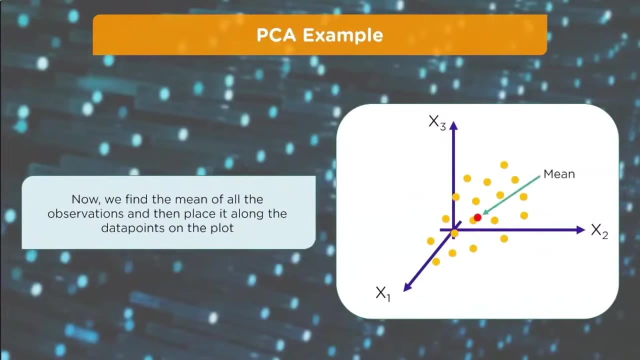 as the variable. But for our simplicity, let's consider this three dimensions for now. Now, each observation row of the matrix X is placed in the k-dimensional variable space, such that the rows in the data table form a swarm of points in this space. 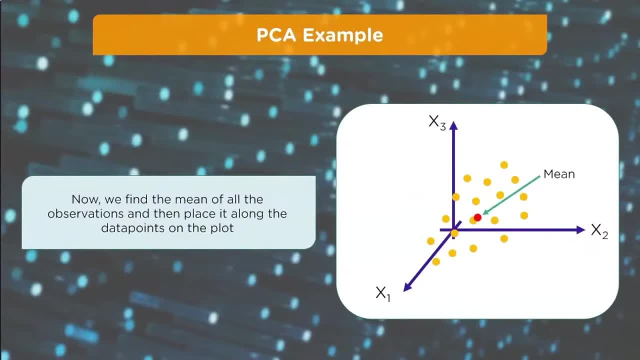 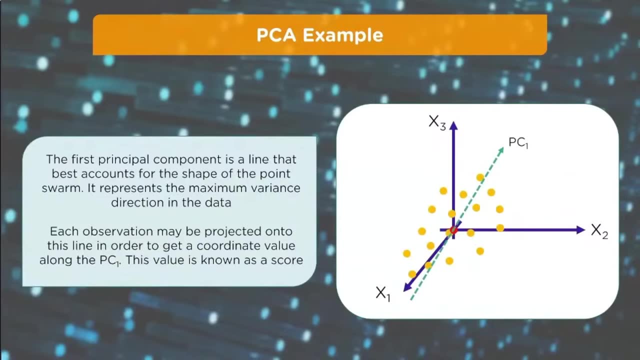 Now we find the mean of all the observations and then place it along the data points on the plot. The first principal component is a line that best accounts for the shape of the point swarm. It represents the maximum variance direction in the data. Each observation may be projected. 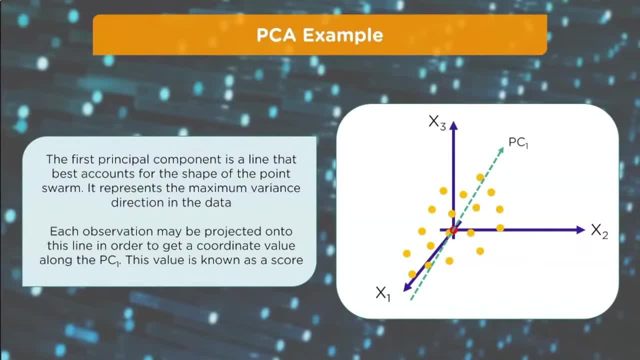 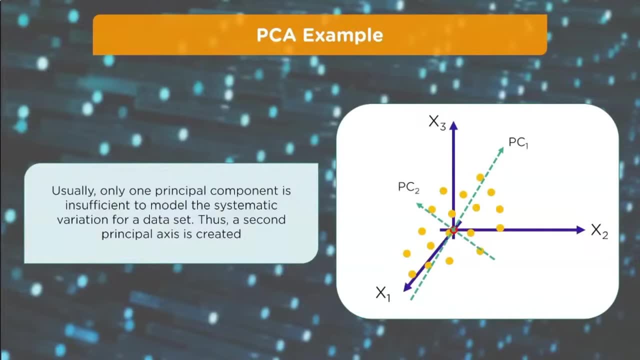 onto this line in order to get a coordinate value along the PC1.. This value is known as a score. Usually, only one principal component is insufficient to model the systematic variation for a data set. Thus, a second principal axis is created, The second principal component. 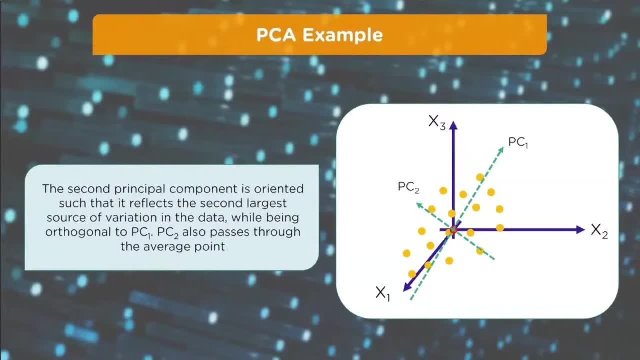 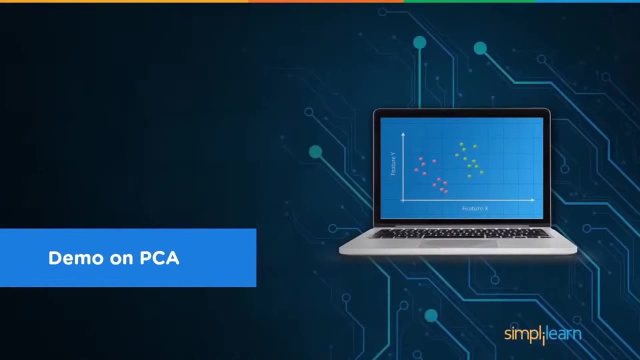 is oriented such that it reflects the second largest source of variation in the data, While being orthogonal to PC1, PC2 also passes through the average point. Let's go ahead and pull this up and just see what that means inside our Python script. 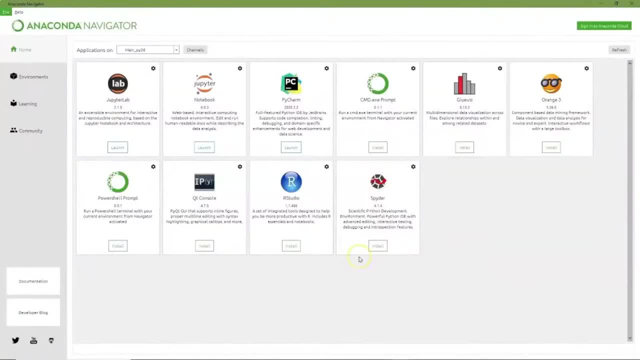 I'm going to use the Anaconda Navigator and I will be in Python 3.6 for this example. I believe there is even like a 3.9 out. I tend to stay in 3.6 because a lot of the models I use. 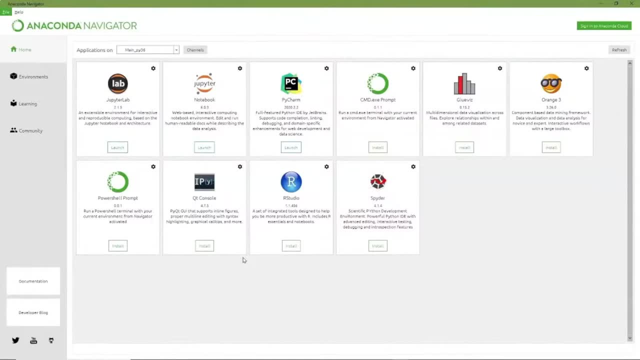 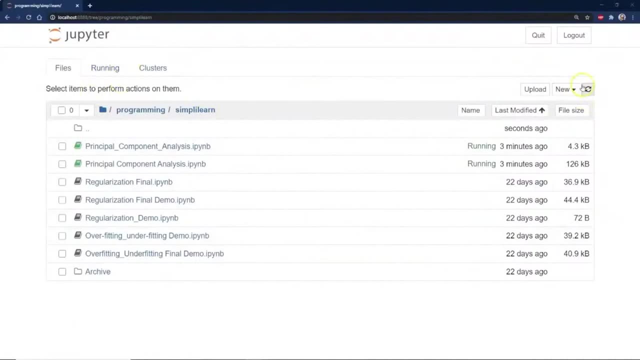 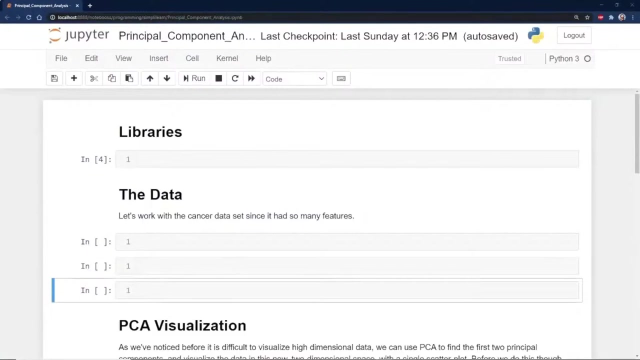 especially with the neural networks, are stable in 3.6.. And then we open up our Jupyter. I'm in Chrome. Go ahead and create a new Python 3.. And for ease of use, our team in the back was nice enough to put this. 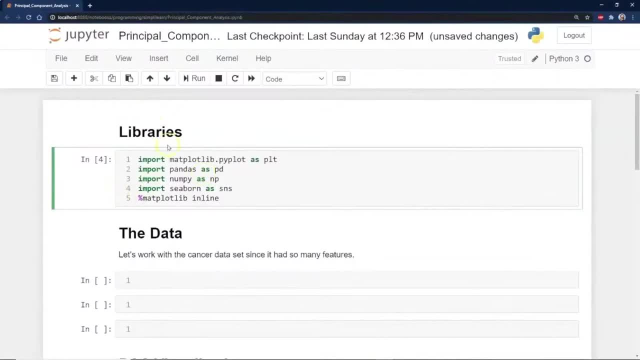 together. for me- And we'll go ahead and start with the libraries- The first thing I like to do whenever I'm looking at any new setup. Well, you know what? let's do the libraries first. We're going to do our basic libraries. 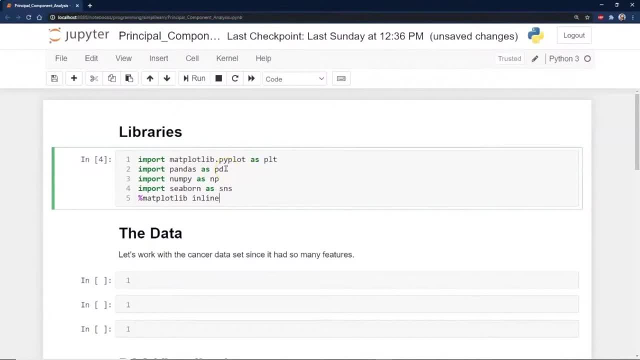 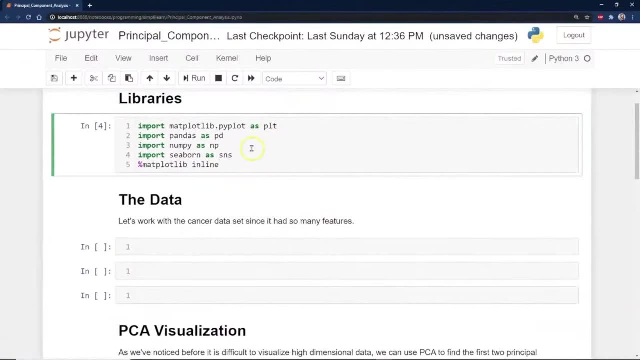 which is MatplotLibrary, the PLT from the MatplotLibrary Pandas, our DataFrame PD Seaborn for graphing SNS. that goes with the plot that actually sits on MatplotLibrary, so the Seaborn sits on there. 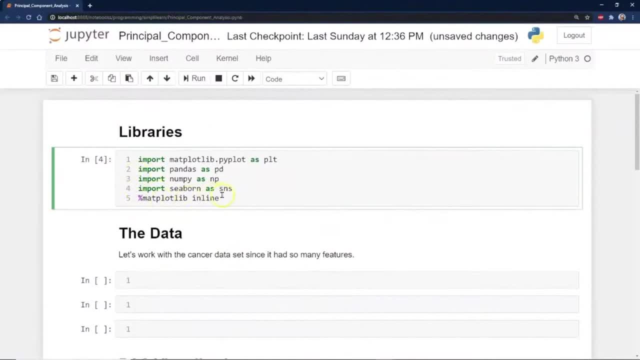 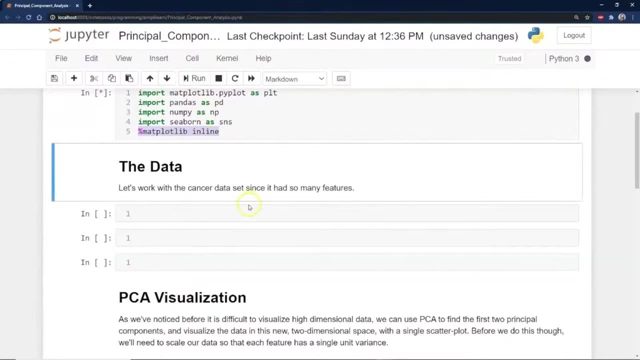 And then we have our Ambersign, because we're in Jupyter Notebook MatplotLibrary inline. The newer version actually doesn't require that, But I put it in there anyway, just because I'm so used to it. And then we want to go ahead. 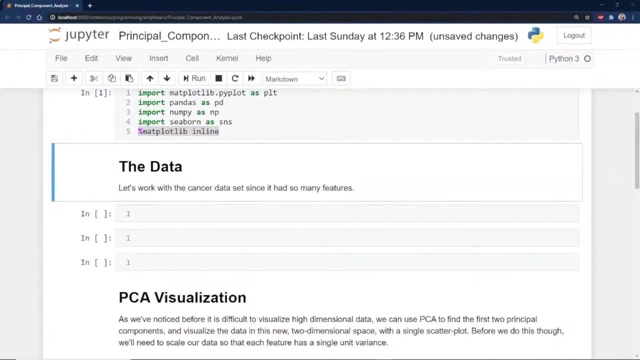 and take a look at the data And in this case we're going to pull in with different data, but we're going to use the cancer data set. And one of the reasons the cancer data set is is it has like 36,, 35 different features. 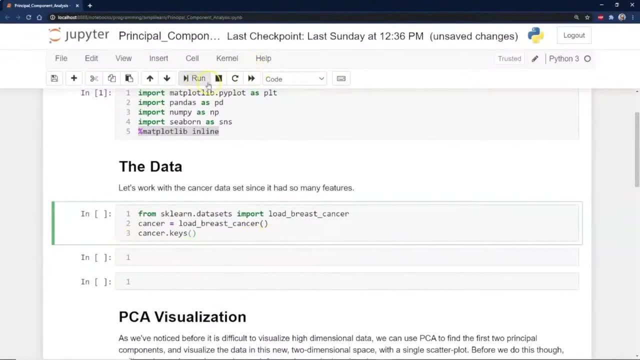 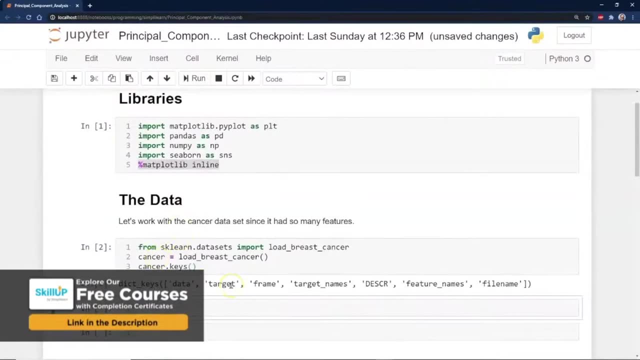 So it's kind of fun to use that as our base for this. Then we'll go ahead and run this and look at our keys And the first thing we notice in our keys for the cancer data set is: we have our data, we have our target, our frame. 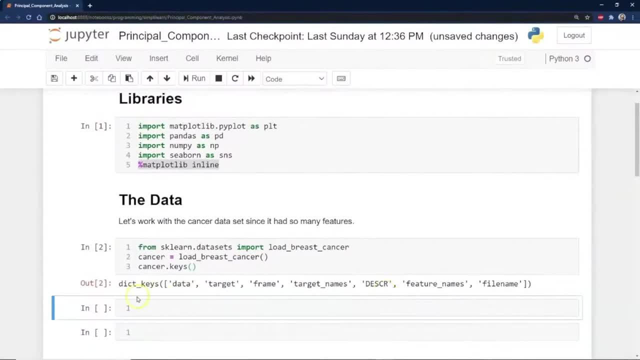 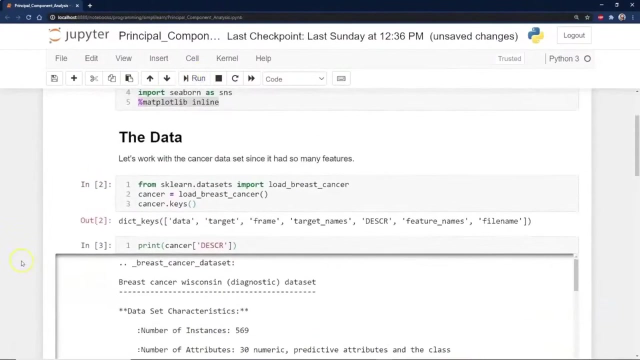 target names, description, feature names and file name. What we're looking for in all this is: well, let's take a look at the description. Let's go in here and pull up the description on here. I'm not going to spend a huge amount of time. 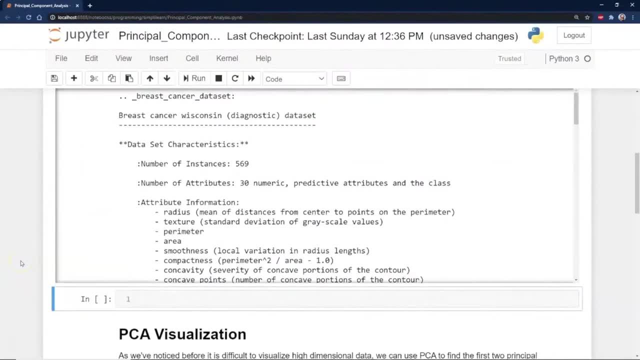 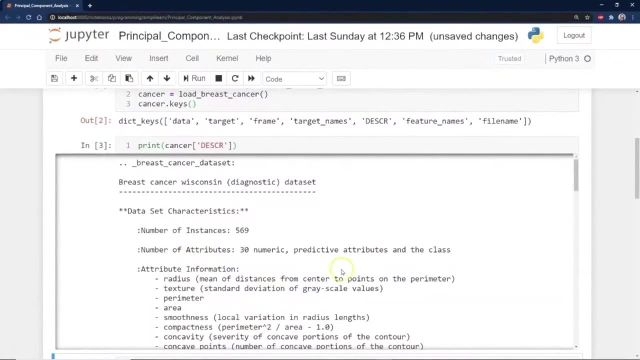 on the description, because we don't want to get into a medical domain. We want to focus on our PCA setup. What's important is you start looking at what the different attributes are, what they mean. If you were in the medical field, you'd want to note. 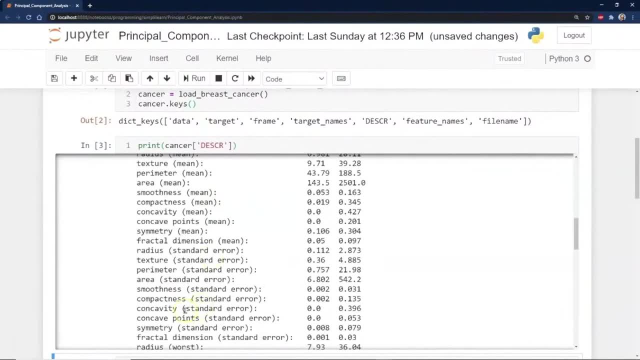 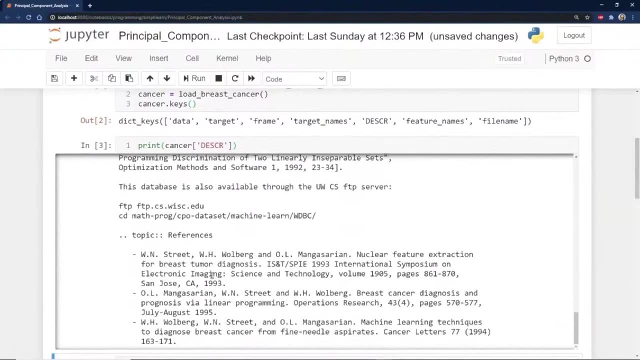 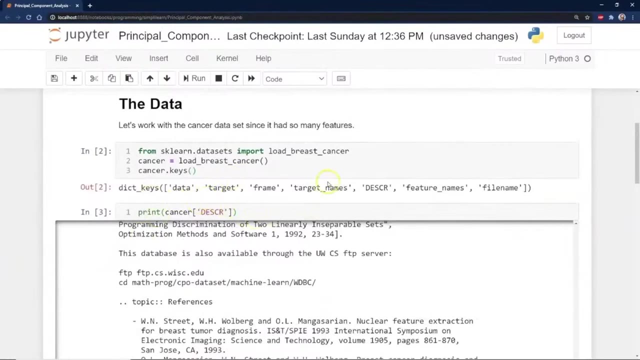 the things, what they're measuring, where it's coming from. You can actually see the actual different measurements they're taking, No missing attributes. We page all the way to the bottom And you're going to have your data- in this case, our target. 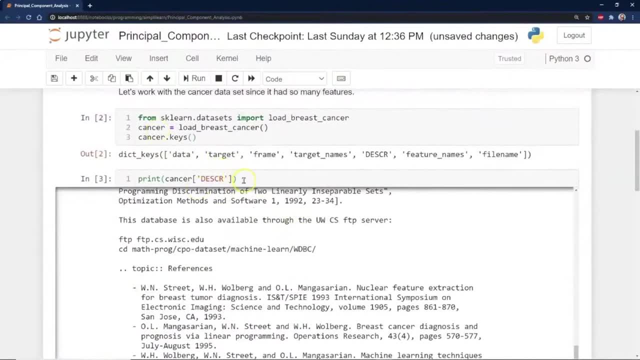 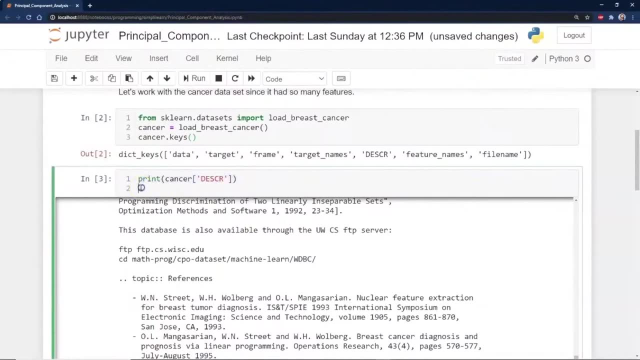 And if you dig deep enough to the target, let's actually do this. Let's go ahead and print target names A little quick here. I always like to just take a look and see what's on the other end of this Target names. 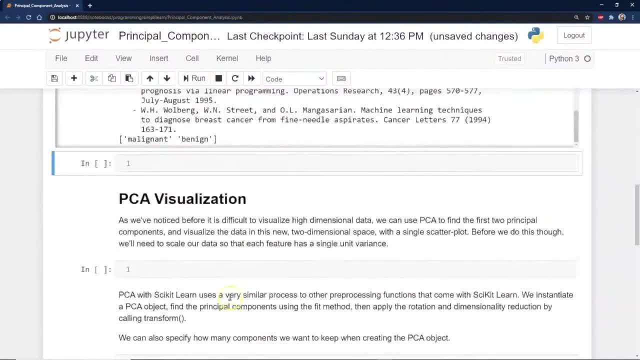 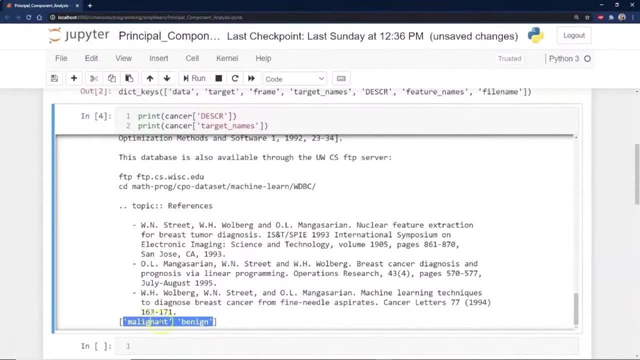 Run that. So the target name is: is it malignant or is it benign? So, in other words, is this dangerous growth or is it something we don't have to worry about? That's the bottom line with the cancer in this case, And then we can go ahead. 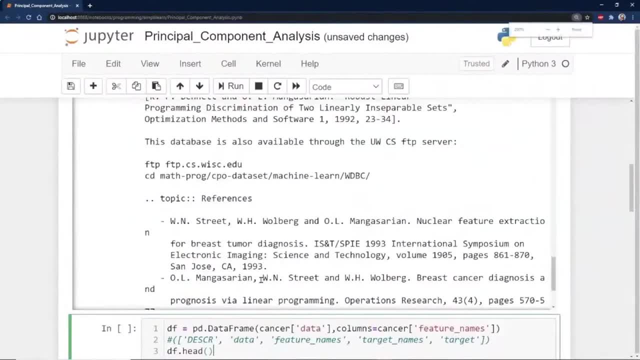 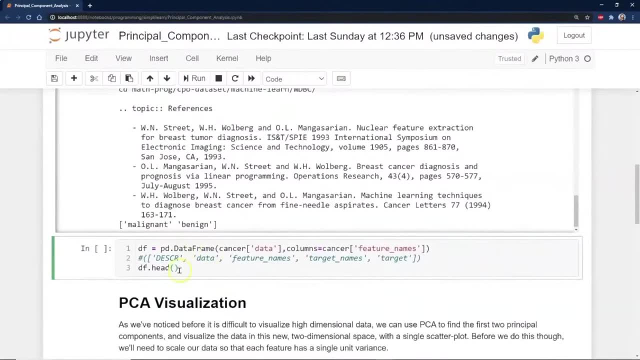 and load our data And you know what? let me go up just a notch here for easy of reading. It's hard to get that just right. That's what we have to do, So let's go ahead and look at our data. 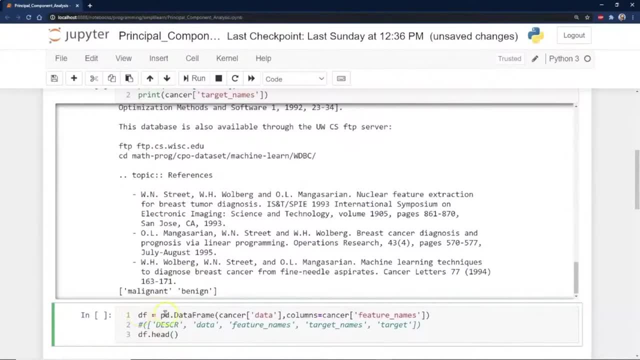 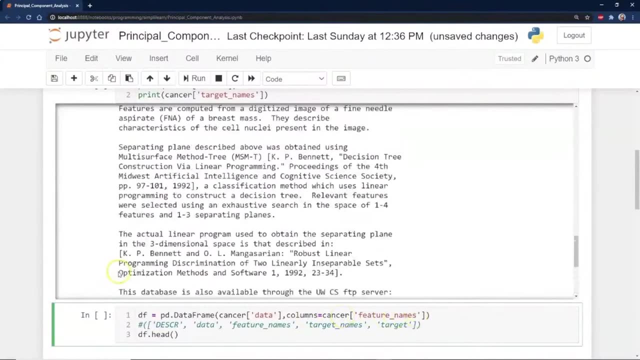 We're going to use our pandas And we're going to go ahead and do our data frame. It's going to equal cancer data Columns equals cancer Feature equals feature names. So remember up here we already loaded the names up of our 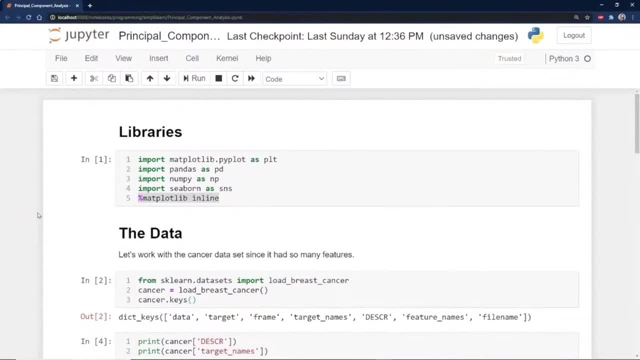 features in there. What is going to come out of this? Let me just see if we can get to that. It's at the top of target names. It's at the top of target names. It's at the top of target names. 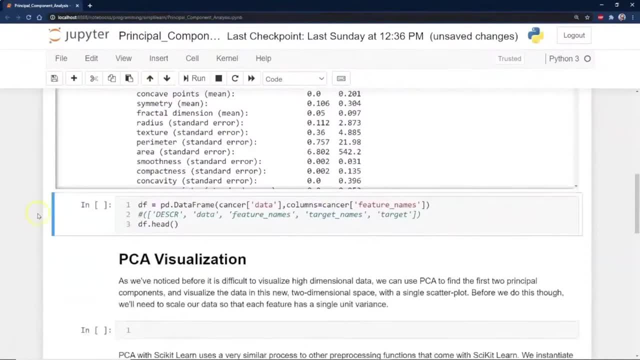 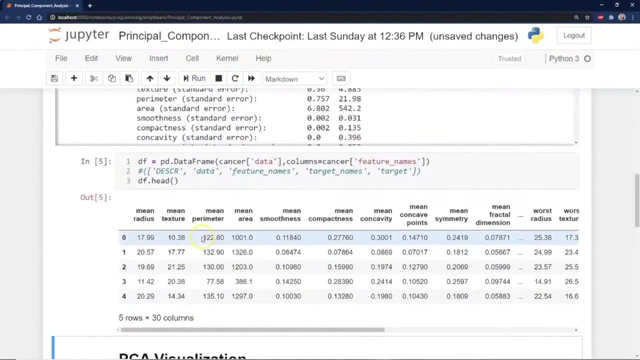 That's just this list of names here in the setup And we can go ahead and run this code And it'll print the head And you can see, here we have the mean radius, the mean texture, mean perimeter. I don't know about you. 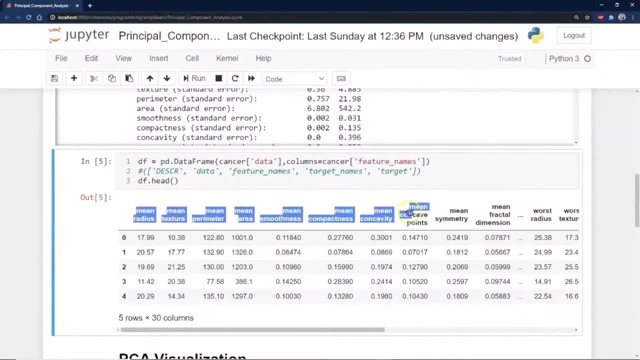 this is a wonderful data set if you're playing with it, because, like many of the data, most of the data that comes in, half the time we don't even know what we're looking at. We're just handed a bunch of stuff. as a data scientist, 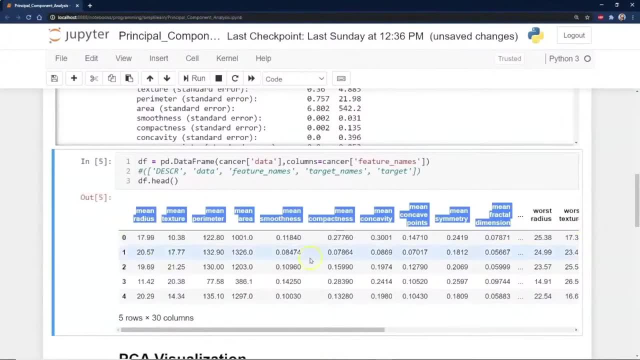 going: what the heck is this? And so this is a good place to start, because this has a number of different features in there and we have no idea what these feature means or where they come from. We want to just look at the data and figure that out. 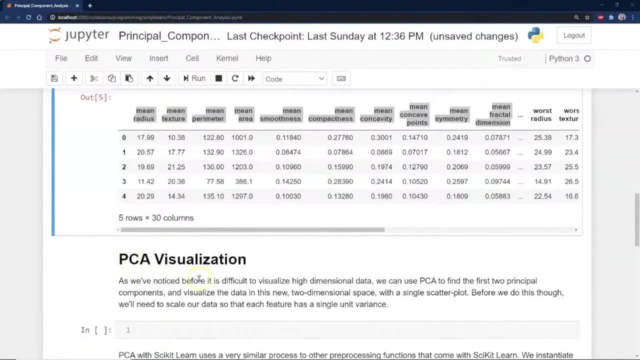 And now we actually are getting into the PCA side of it. As we've noticed before, it is difficult to visualize high dimensional data. We can use PCA to find the first two principal components and visualize the data, this new two dimensional space with a single scatter plot. 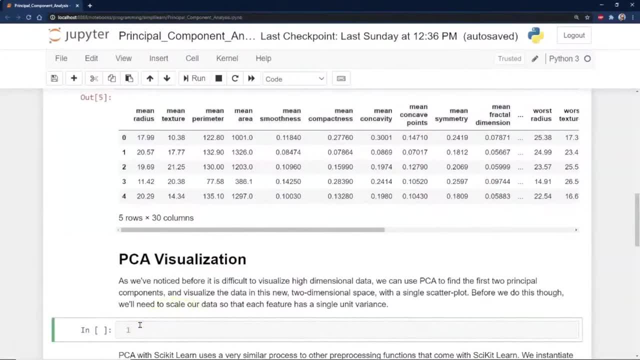 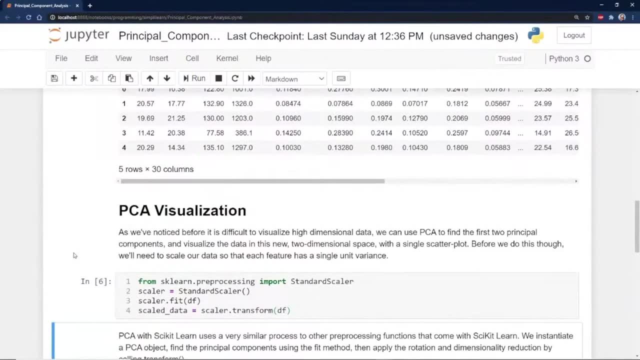 Before we do this, we need to go ahead and scale our data. Now I haven't run this to see if you really have to scale the data on this, But as just a general run time, I almost do that as the first step of any modeling. 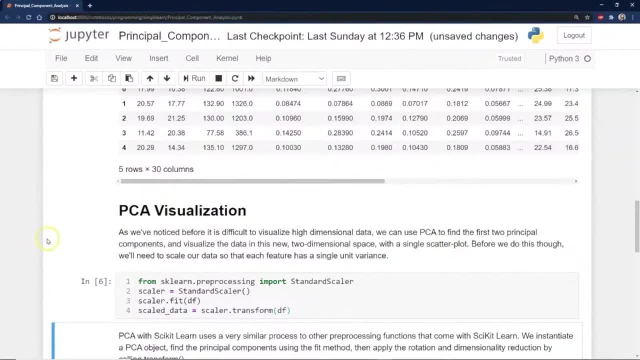 Even if it's pre-modeling, as we're doing here In neural networks. that is so important With PCA visualization. it's already going to scale it when we do the means and deviation inside the PCA, But just in case, it's always good to scale it. 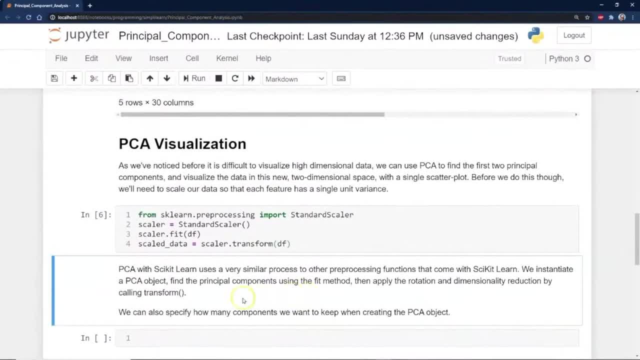 And then we're going to take our PCA with the scikit-learn uses very similar process to other pre-processing functions that come with scikit-learn. We instantiate a PCA object, find the principal components using the fit method, then apply the rotation and dimensionality. 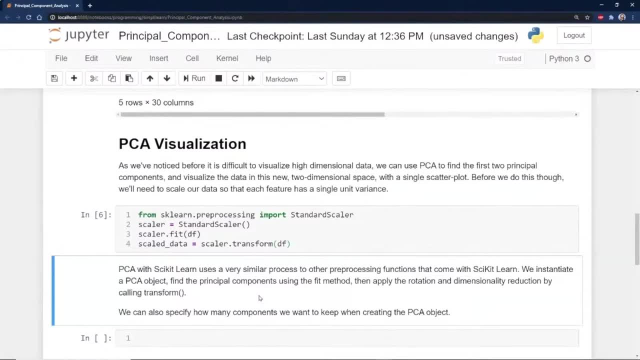 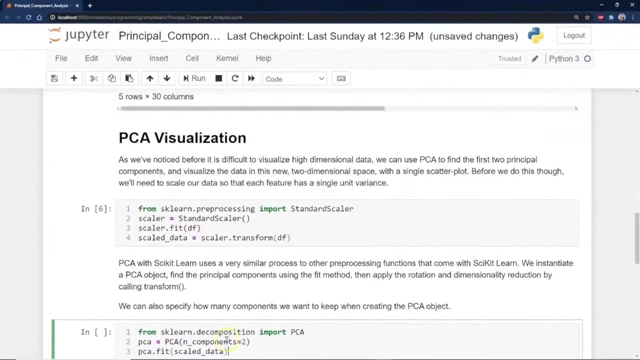 reduction. by calling transform, We can also specify how many components we want to keep when creating the PCA object, And so the code for this. Oops, getting a little bit ahead, I'm going to go ahead and run this code. So the code for this: 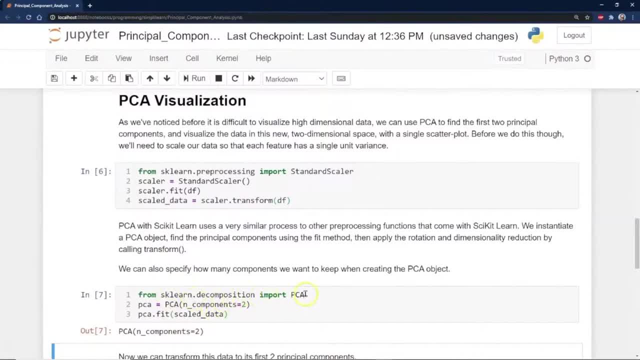 is from sklearn decomposition import PCA. PCA equals PCA and components equals two, And that's really important to note that Because we're only going to want to look at two components. I would never go over four components, Especially if you're going to demo this. 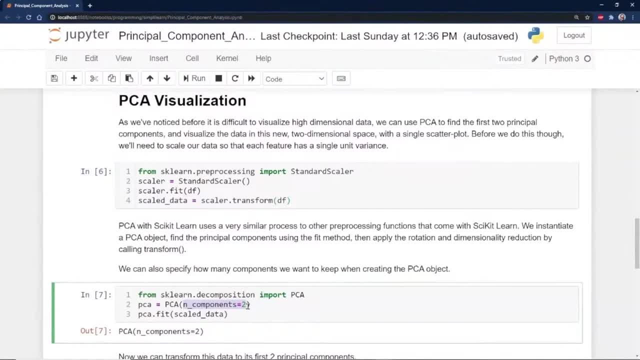 with somebody else. If you're showing this to the shareholders, the whole idea is to reduce it to something people can see, And then the PCA fit is going to take the scaled data that we generated up here and then you can see we've created our 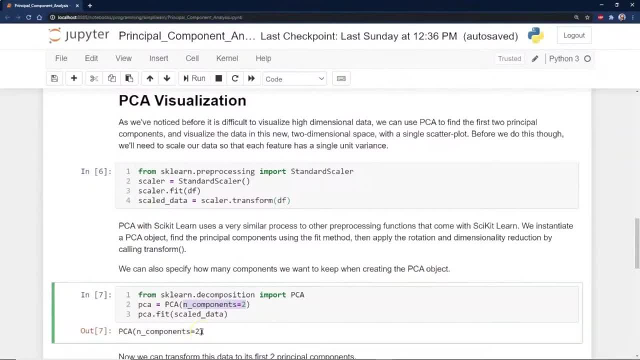 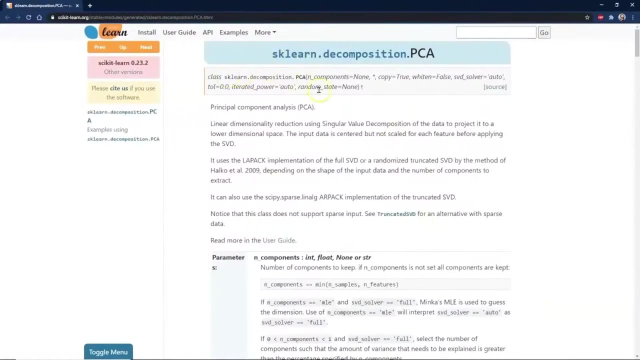 PCA model with in components equals two. Now whenever I use a new tool, I like to go in there and actually see what I'm using. So let's go to the Scikit webpage for the PCA And you can see in here. here's our call statement. It describes: 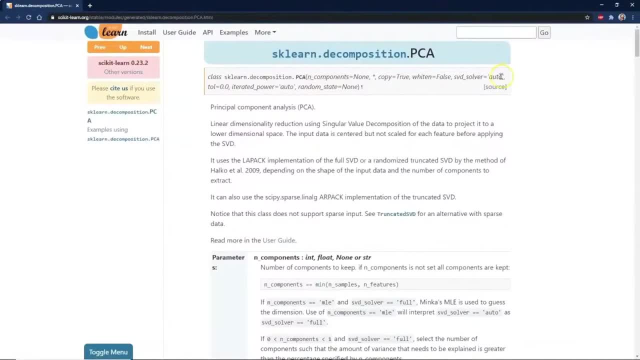 all the different setups you have on there, Probably the biggest one to look at would be. well, the biggest one is your components. How many components do you want Which you have to put in there pretty much, And then you also might look at the SVD solver. 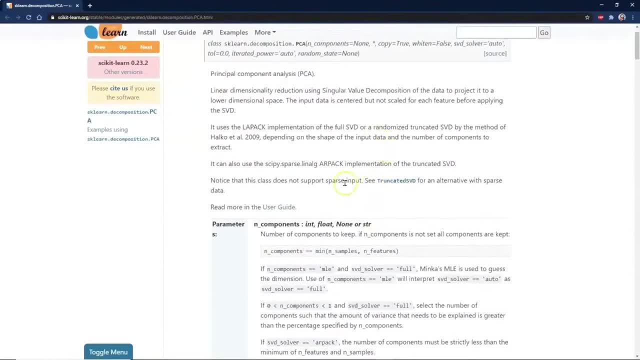 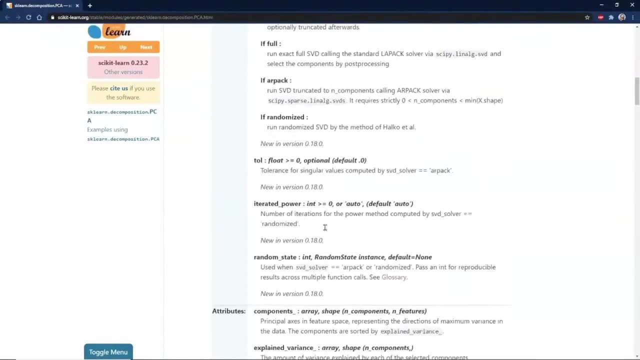 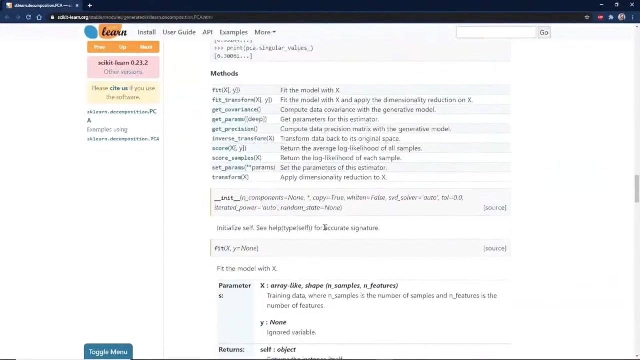 It's on auto right now, But you can override that and do different things with it. It does a pretty good job as it is, And if we go down all the way down to there, we go to our methods. If you notice, we have fit. 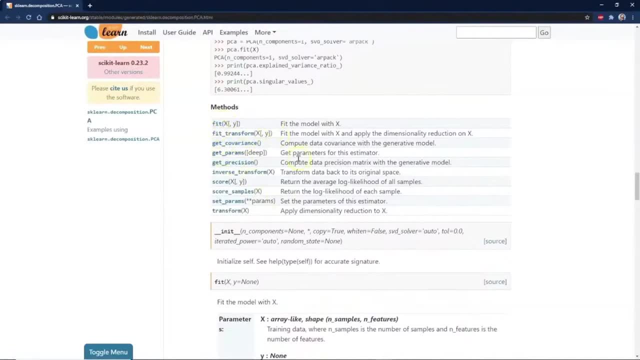 and we have fit transform. Nowhere in here is predict, Because this is not used for prediction, It's used to look at the data. Again, we're in the describe setup, We're fitting the data, We're taking a look at it. 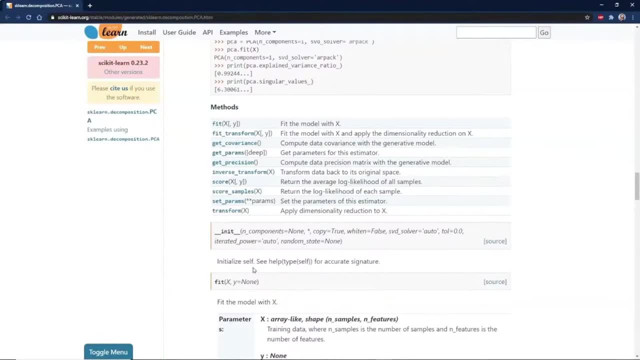 We've already looked at our minimum maximum. We've already looked at what's in each quarter. We've done a full description of the data. This is part of describing the data. That's the biggest thing I take away when I come zooming in here And of course, they have examples. 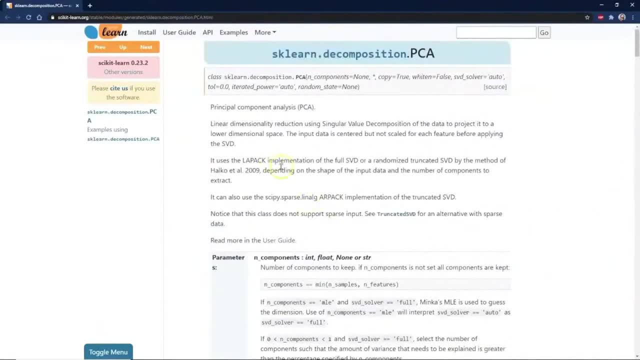 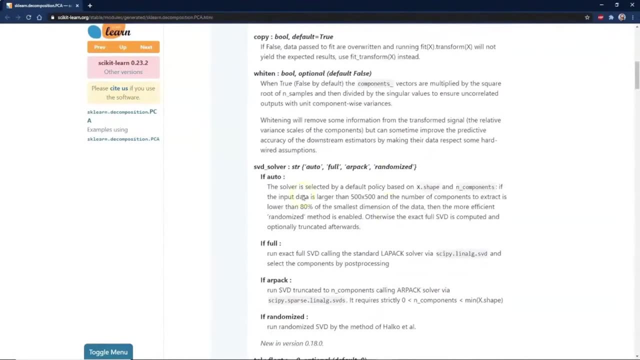 of it down here, if you forget. And the biggest one, of course, is the number of components And then the rest you can play with The actual solver, whether you're doing a full or randomized- there's different things. It is pretty good on the auto. 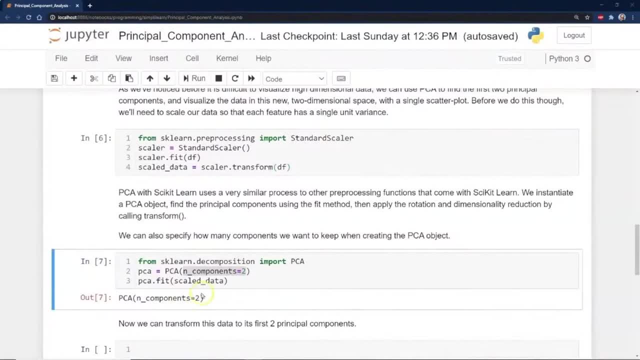 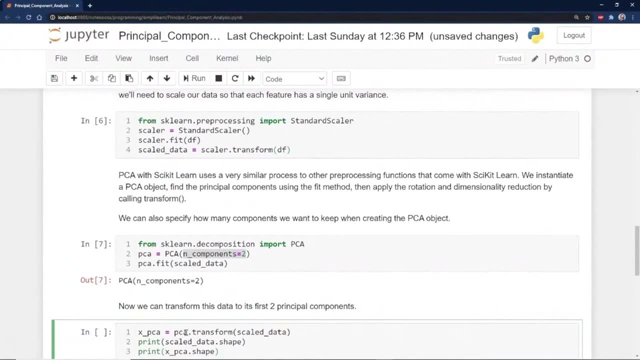 And now we can transform this data to its first two principal components, And so we have our XPCA. We're going to set that equal to PCA: transform scaled data. So there we go, There's our first transformation, And let's just go ahead and print the scaled. 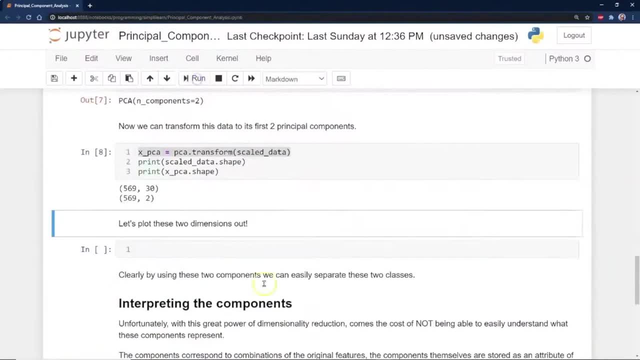 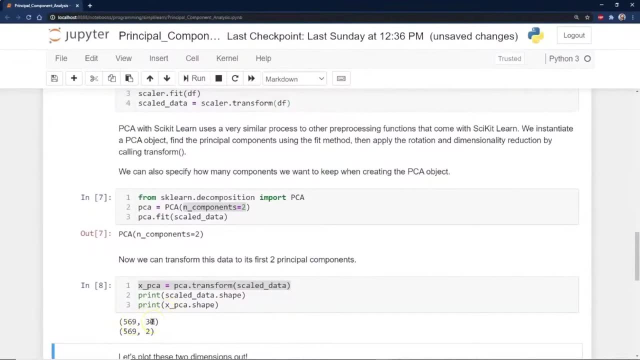 data shape and the XPCA data shape, And the reason we want to do this is just to show us what's going on here. We've taken 30 features. I think I said 36 or something like that, but it's 30.. 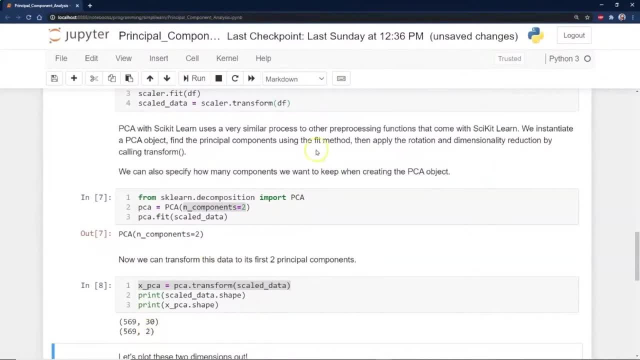 And we've compressed it down to two features And we decided we wanted two features. And that's where this comes from. We still have 569 data sets. I mean data rows, not data sets. We still have 569 rows of data, But instead of computing. 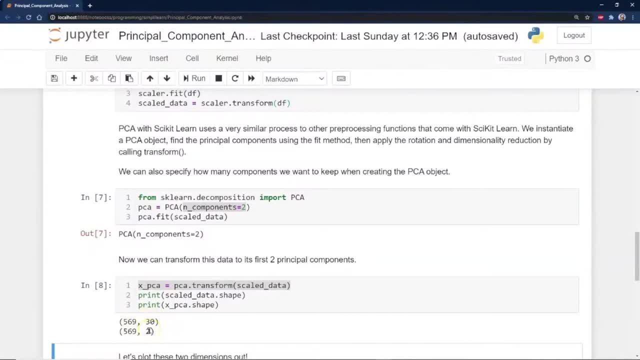 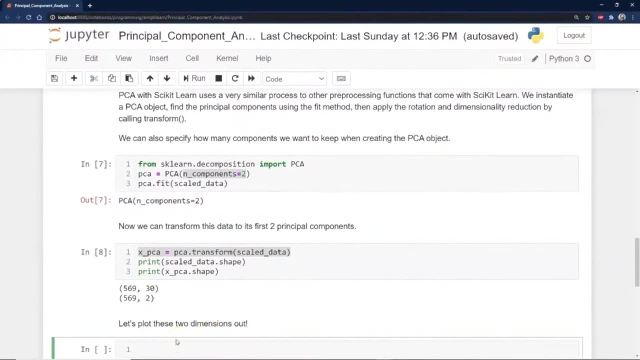 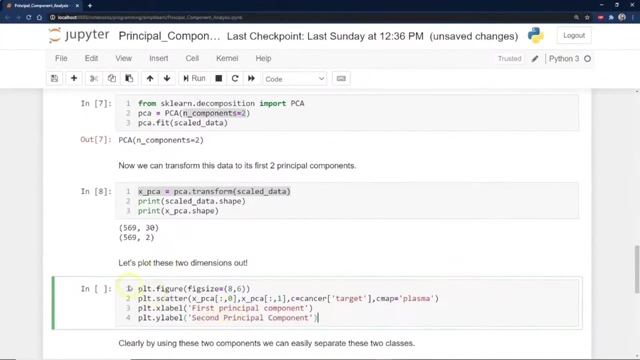 30 features. we're now only doing our model on two features. So let's go ahead and plot these and take a look and see what's going on. And we're just going to use our PLT figure. We're going to set the figure size on here. 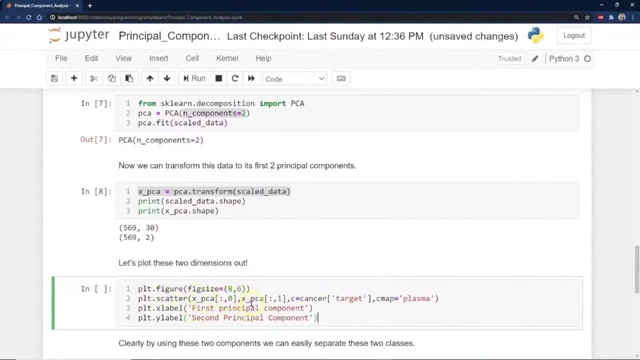 Here's our scatter plot: XPCA X underscore PCA of one. These are two different perceptions we're using, And then you'll see right here: C for color cancer equals target, And so remember, we have zero, we have one And, if I remember correctly, zero was: 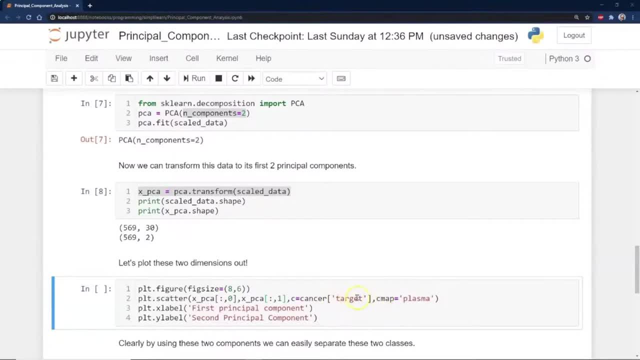 malignant, one was benign. So everything in the zero column is going to be one color and the other color is going to be one, And then we're going to use the plasma map just kind of telling you what color it is. Add some labels First. 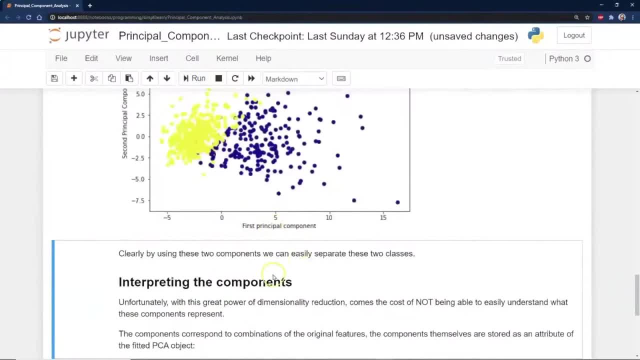 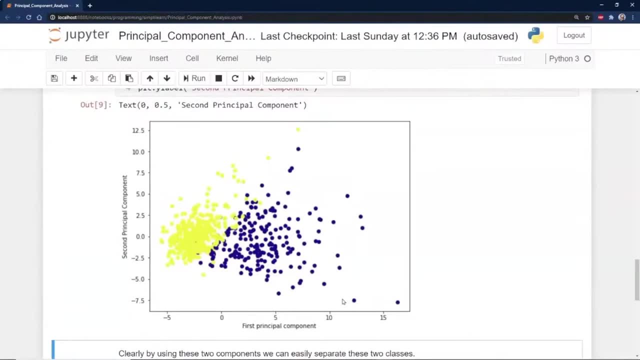 principal component. second principal component, And we'll go ahead and run this, And you can see here, instead of having a chart, one of those heat maps with thirty different columns in it, we can look at this and say, hey, this one actually did a pretty good. 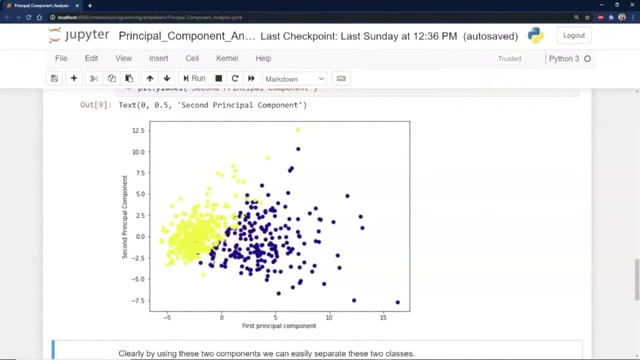 job of separating the data And a couple things when I'm looking at this that I notice is: first, we have a very clear area where it's clumped together, Where it's going to be benign, And we have a huge area it's still clumped together, more spread out. 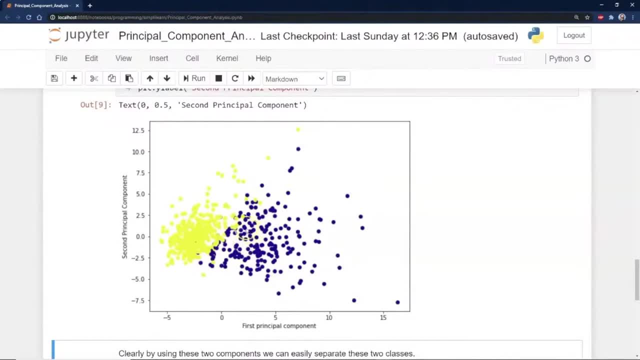 where it's going to be malignant, Or I think I had that backwards And then in the middle, because we're dealing with something, in this particular case cancer- we would try to separate. I would be exploring how to separate this middle group out. 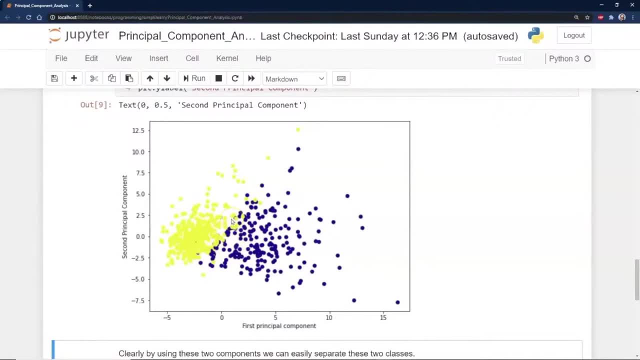 In other words, there's an area where everything overlaps and we're not going to have a clear result on it. Just because those are the people, you want to go in there and have extra tests or treat it differently, versus going in and saying. just cutting into the cancer so the body absorbs it and it dissipates, versus actively going in there, removing it, testing it, going through chemo and all the different things. That's a big difference, you know, as far as what's going to happen here. 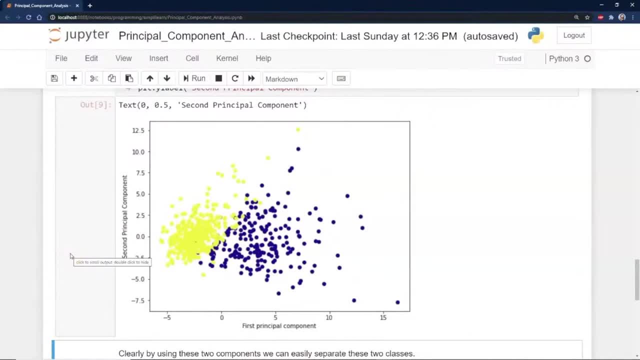 And that middle line where they overlap is going to be huge. That's domain specific. Going back to the data we can see here, these two components, we can easily separate these two classes. So the next step is: what does that mean? 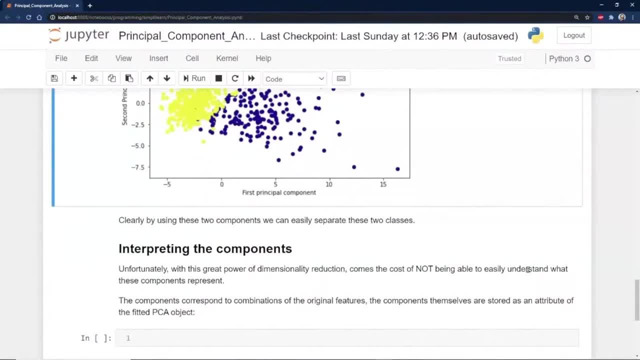 Interpreting the components. Unfortunately, with this great power of dimensionality reduction comes the cost of not being able to easily understand what these components represent. I don't know what principle component one represents, or second principle. The components correspond to combinations of original features. 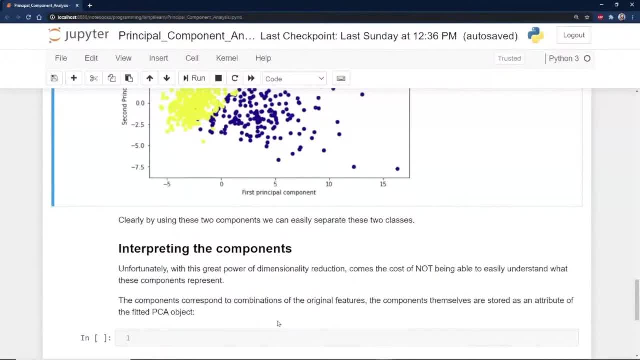 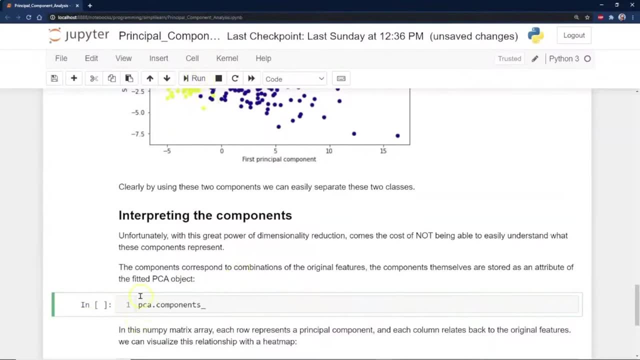 The components themselves are stored as an attribute of the filtered PCA object, And so when we look at that, we can go ahead and look at the PCA components. This is in our model we built, We've trained it, We can run that and you can see. 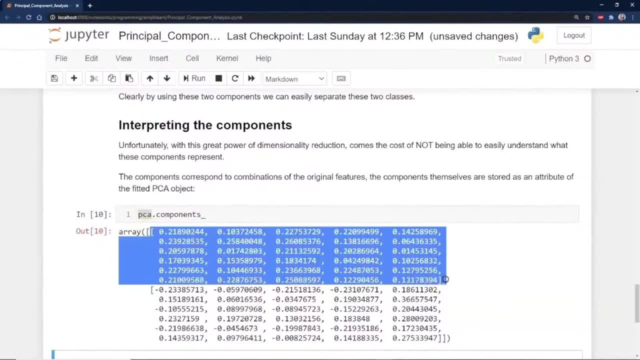 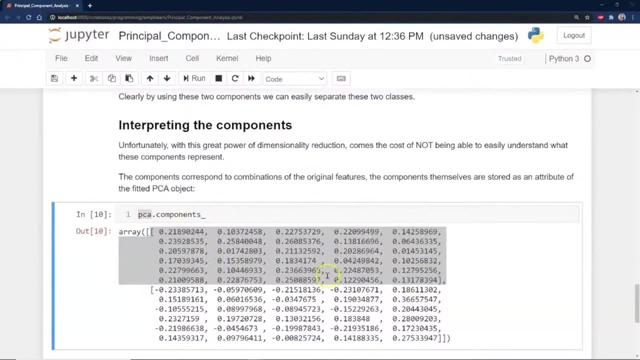 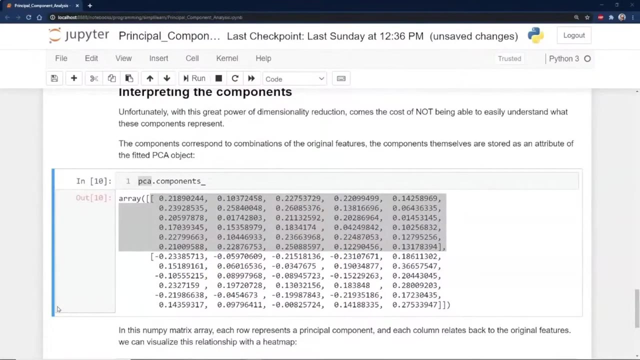 here's the actual components. The two components each have their own array And within the array you can see the scores they're using, And these actually give weight to what features are doing what. So in this numpy matrix array, each row represents a principle component. 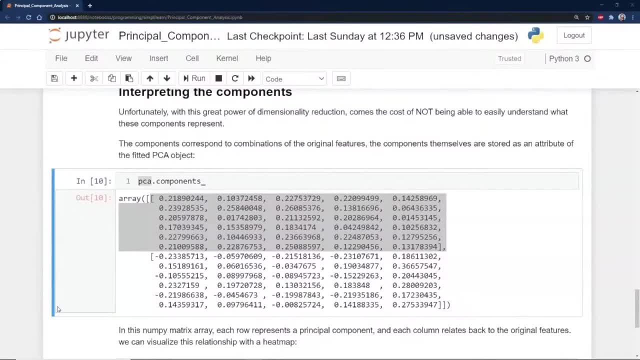 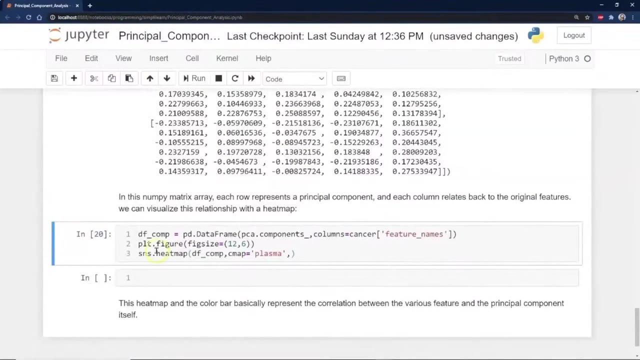 and each column relates back to the original features. What's really neat about this is we can now go in reverse and drop this onto a heat map and start seeing what this means. So let me go ahead and just put this down. We'll go ahead and put this in here. 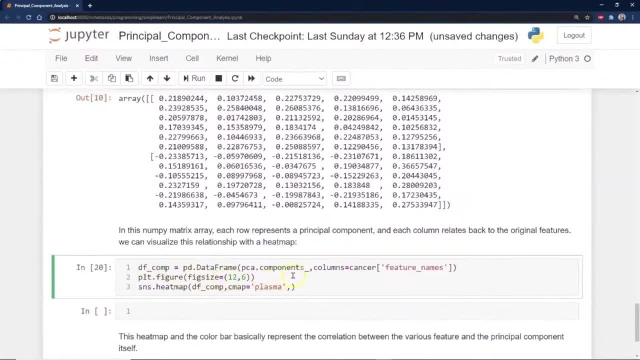 We're going to use our dfcomp data frame and we do our PCA components, And I want you to notice how easy this is. We're going to set our columns equal to cancer feature names- That just makes it really easy- And we're dumping it into a data frame. 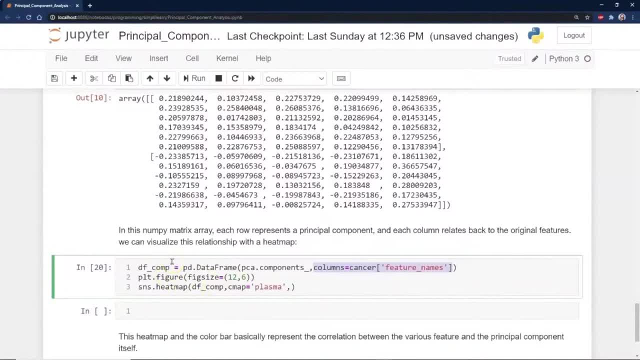 What's neat about a data frame is when we get to seaborne, it will pull that data frame apart and set it up for us where we want, And so we're just going to do the seaborne heat map of our data frame. 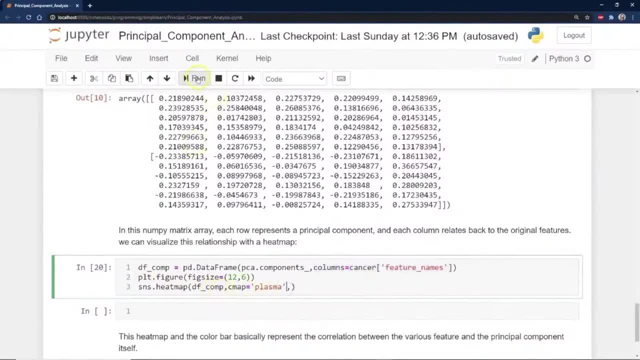 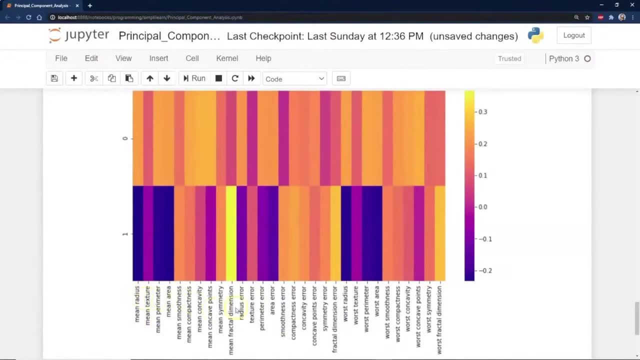 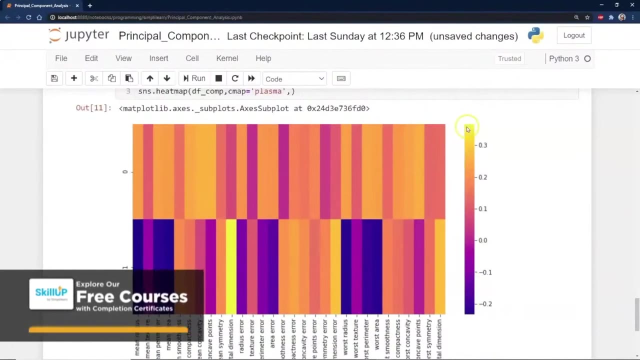 composition and we'll use the plasma coloring And it creates a nice little color graph. here You can see we have the mean radius and all the different features. along the bottom On the right we have a scale so we can see we have the dark colors. 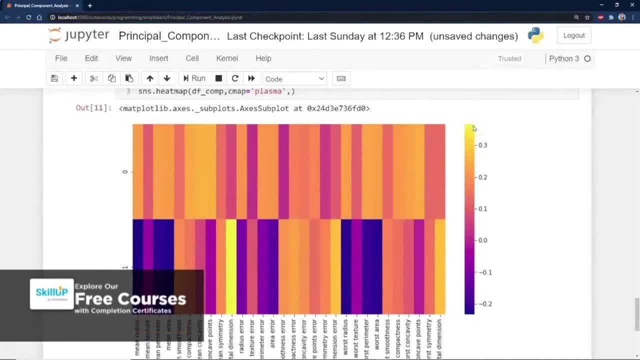 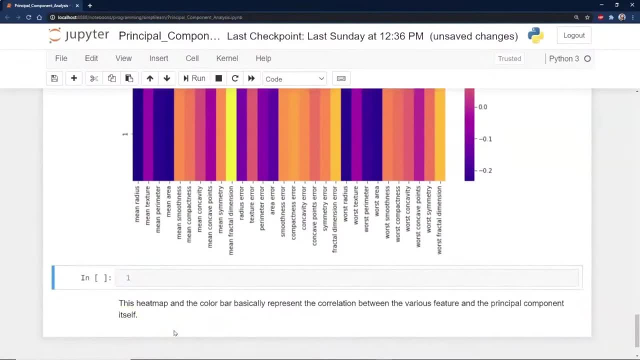 all the way to the really light colors which are what's really shining there. This is like the primary stuff we want to look at. So this heat map and the color bar basically represent the correlation between the various features and the principal component itself. 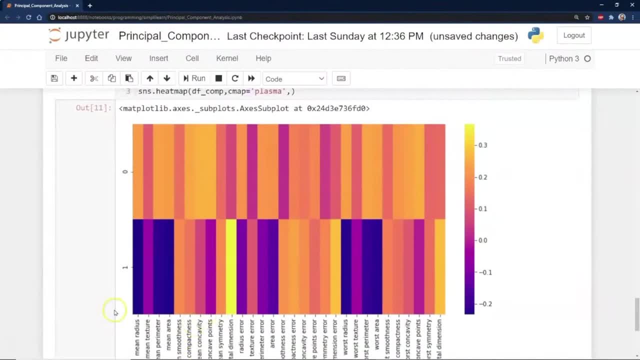 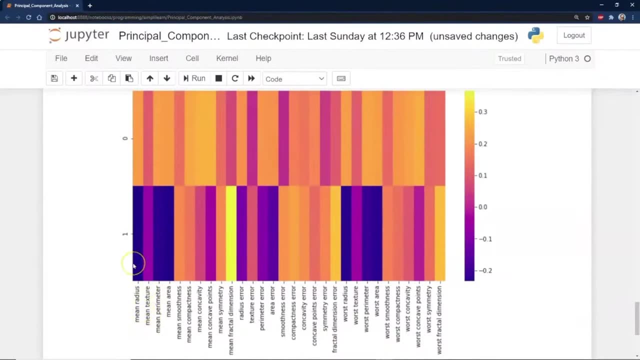 So you have a very powerful map to look at and then you can go in here and we might notice that the mean radius. look how on the bottom of the map it is on some of this. So you have some interesting correlations here that change the variations on that. 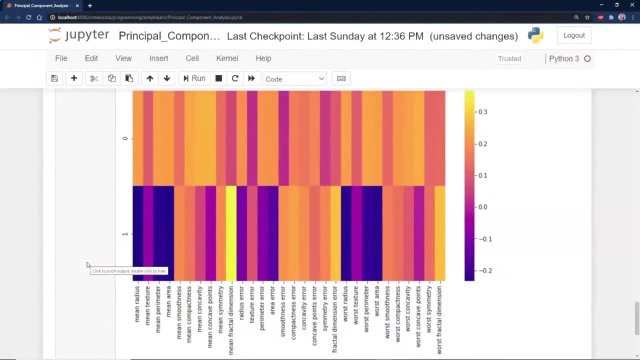 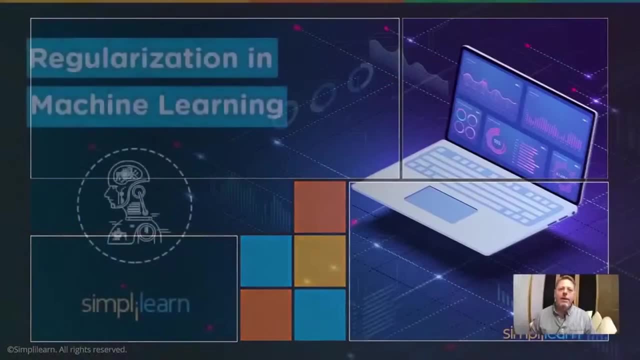 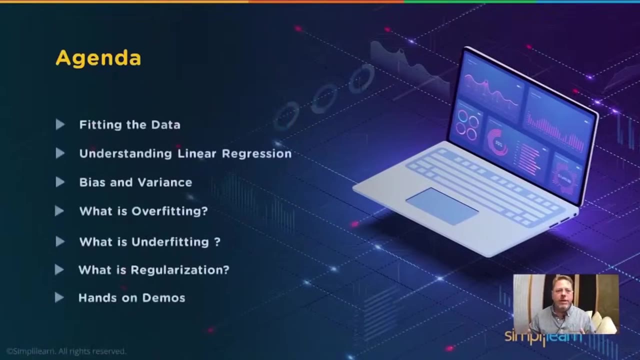 and what means what. This is more, when you get to post scribe, you can also use this to try to guess as what these things mean and what you want to change to get a better result. Regularization in machine learning. So our agenda on this one is: 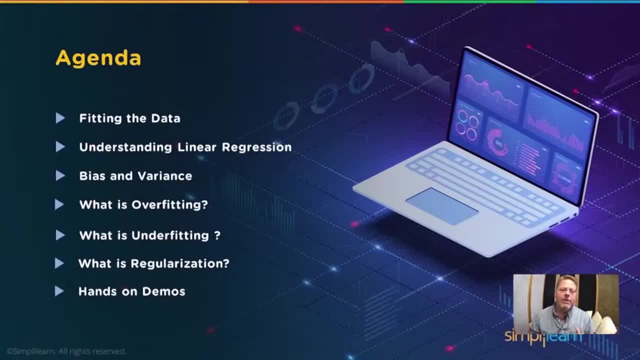 fitting the data, understanding linear regression, bias and variance. what is overfitting, what is underfitting- and those are like the biggest things right now in data science- is overfitting and underfitting. What does that mean? And what is regularization? 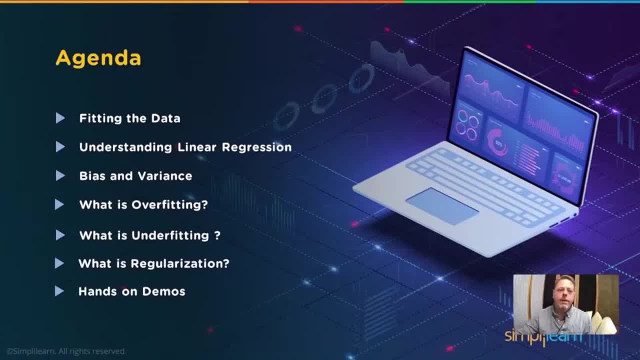 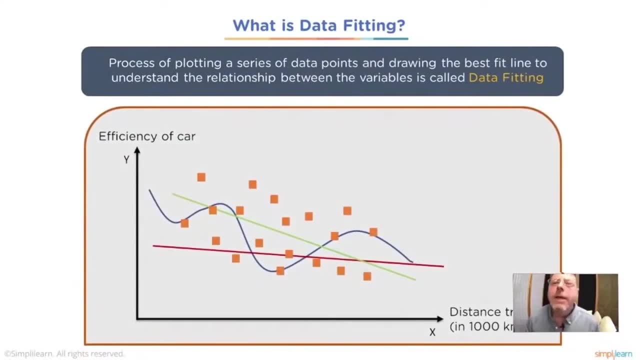 and then we'll do a quick hands-on demo to take a look at this. So, fitting the data. Let's start with fitting the data. Let's talk about what is data fitting. It's a process of plotting a series of data points and drawing. 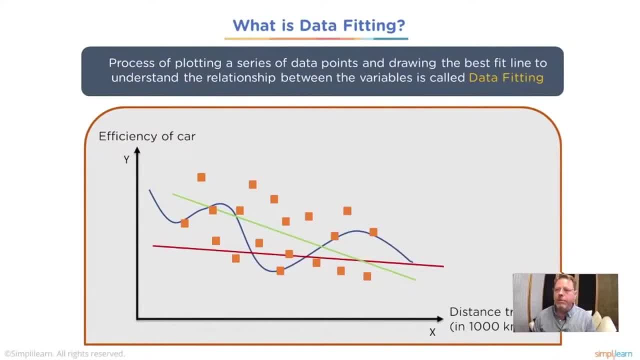 the best fit line to understand the relationship between the variables, and this is what we call data fitting And you can see here we have a couple of lines we've drawn on this graph. We're going to go in a little deeper on there, So we might have in this case, 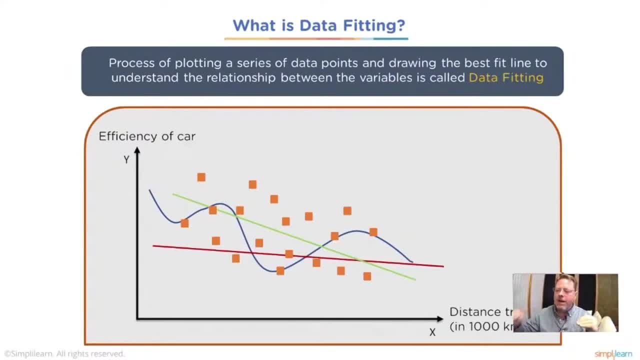 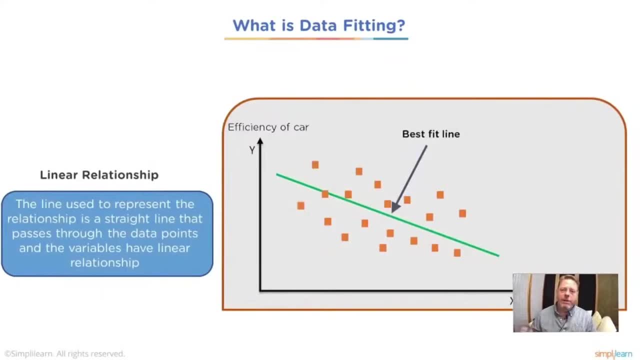 just two dimensions. We have an efficiency of the car and we have the distance traveled in 1000 kilometers. And so what is data fitting? Well, it's a linear relationship, And a linear relationship very specifically. linear means line, The line. 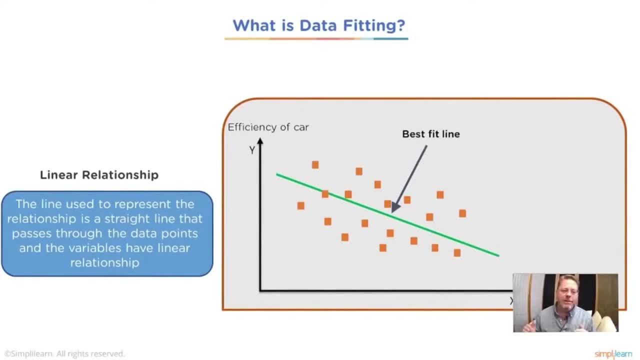 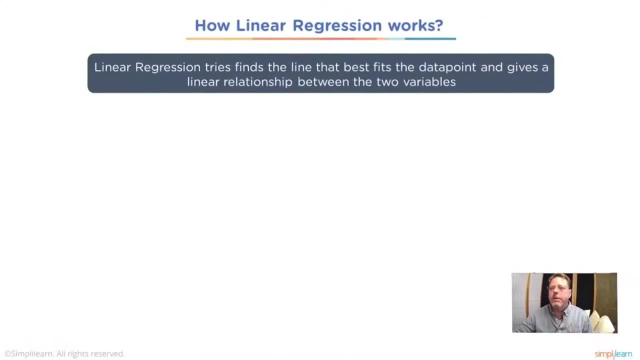 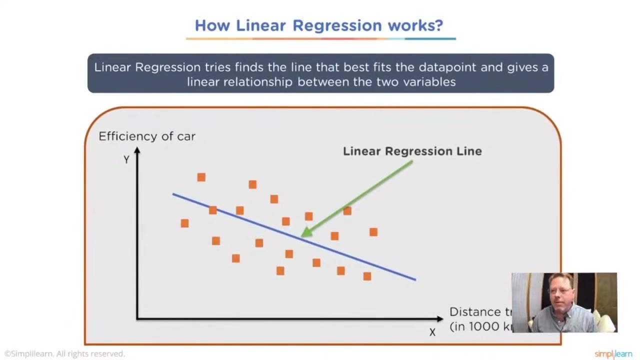 used to represent the relationship is a straight line that passes through the data points, and the variables have a linear relationship- Linear regression. So let's start with how linear regression works. Linear regression finds a line that best fits the data point and gives a relationship between: 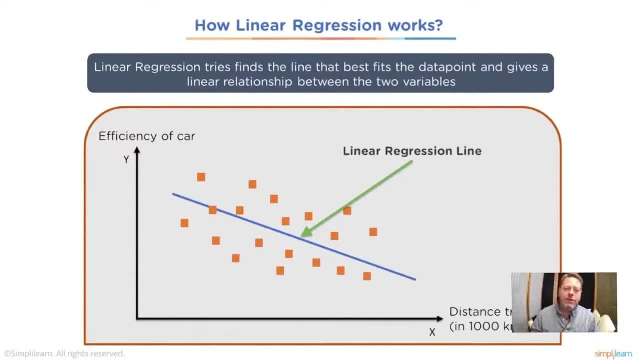 the two variables, And so you can see here we have the efficiency of the car versus the distance traveled, And you can see this nice straight line drawn through there. And when you talk about multiple variables, all you're doing is putting this: instead of a line, it now becomes a plane. 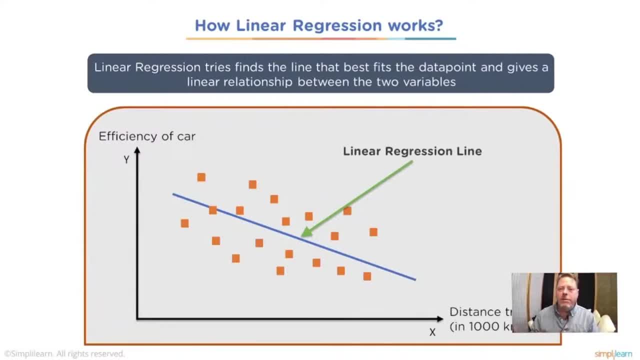 It gets a little more complicated with multiple variables, but they all come down to this linear kind of drawing a line through your data and finding what fits the data the best. And so we can consider an example. Let's say that we want to find the relationship. 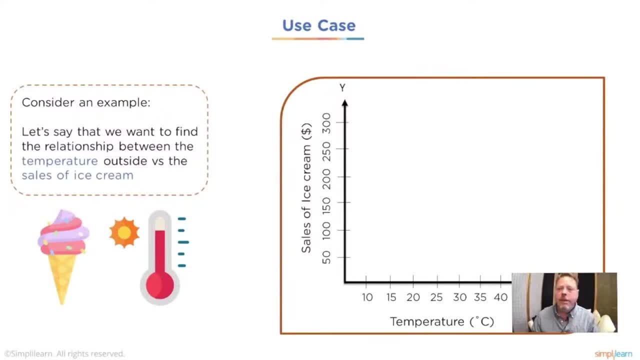 between the temperature outside versus the sales of ice cream. And so we start looking at that. We're looking at how many ice cream cones we're selling or how much money we sold on ice cream, and we're looking at how warm it is outside. 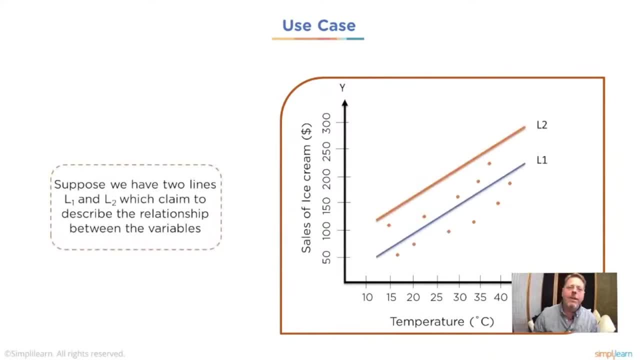 which would hopefully draw a lot of people into the ice cream store, And suppose we have two lines- We're going to draw L1 and L2 and we're going to kind of guess which one we think is the best fit- Which claim to describe the relationship. 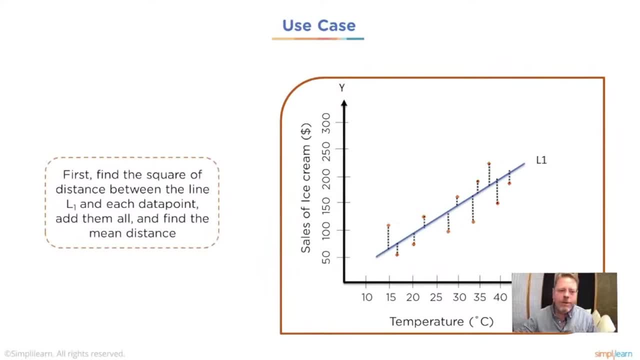 between the variables. And so first we find the square of the distance between the line L1 and each data point and add them all and find the mean distance. And I want you to think about that when we square something, if it's a negative or positive number. 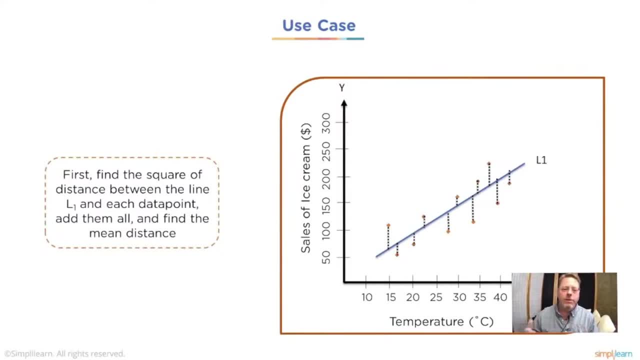 it no longer matters, because a minus two squared is four. two squared is four. So we're removing what side of the line it's on and we're just looking for the error, In this case the mean distance of each of the little dotted lines you see here. 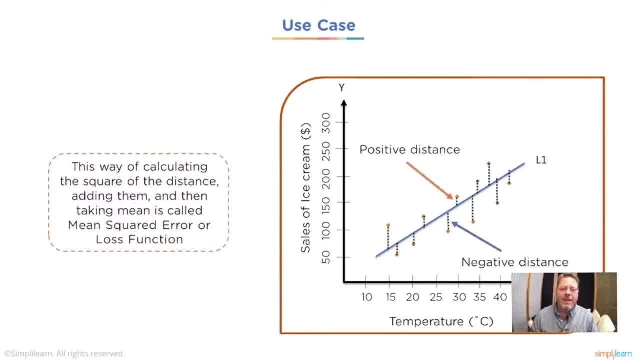 This way of calculating the square of the distance. adding them and then taking the mean is called mean square, error or loss function, And we talk about loss. how far off are we? That's what we're really talking about. What did we miss? 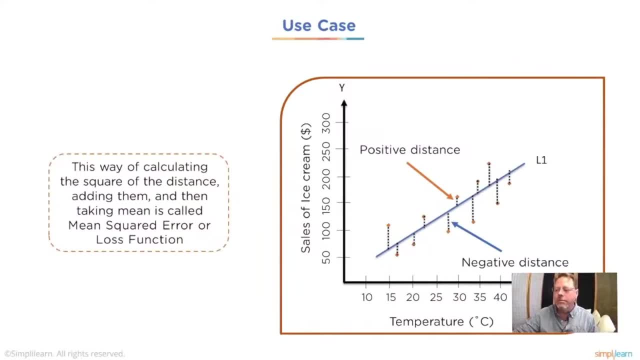 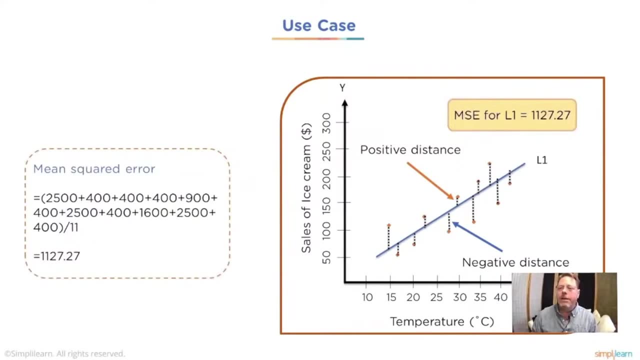 We have a positive distance and a negative distance and of course when we square it it just becomes a positive error And so we take the mean square error and a lot of times you'll see it referred to as MSE. If I look in a code and I'm going through, 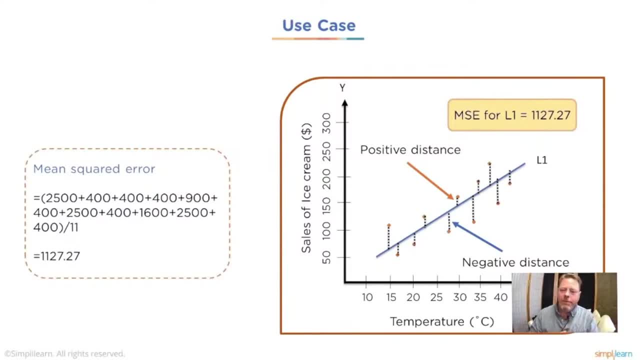 the code and I see MSE- I know that's the mean squared error- And we take all the dotted lines and we calculate this error and we add them all together and then we average it or find the means. And in this case they ran a demo. 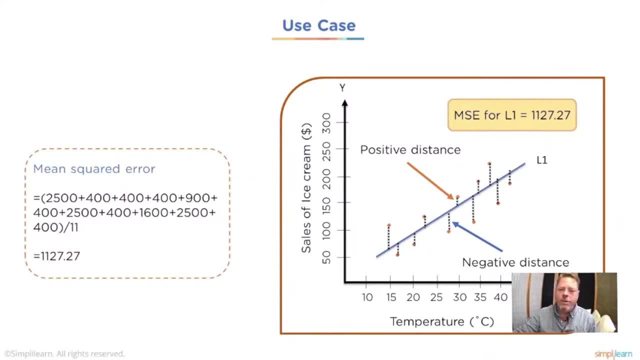 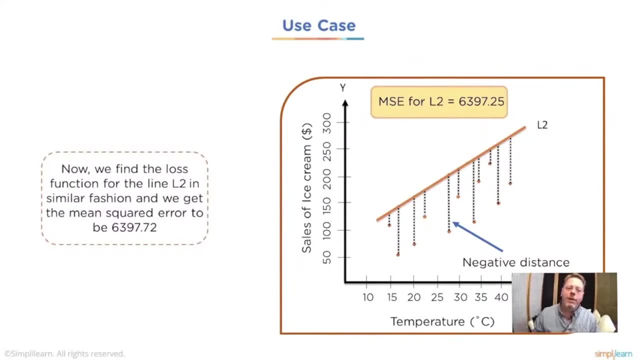 on this and it was 1127.27 for our L1 line. Now we find the loss function for line L2 in a similar fashion and we get the mean square error to be 6397.. And it's computed the same way. 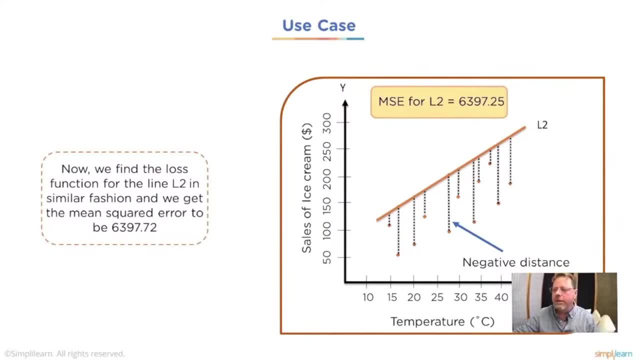 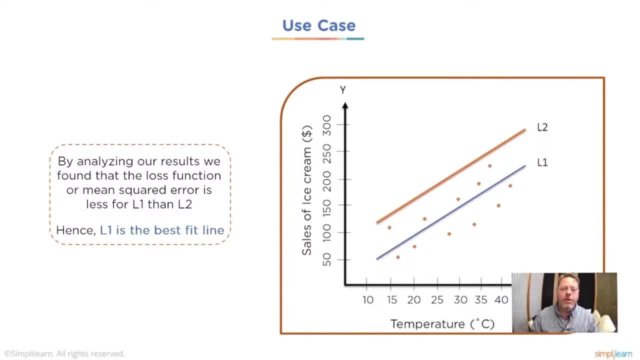 So maybe you put this line just way outside the data range and this is the error you get. By analyzing our results, we find that the loss function, or the mean square error, is less for L1 than L2.. Hence L1 is the best fit. 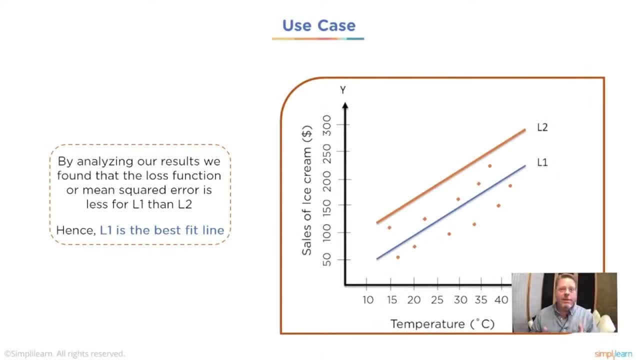 line. This process describes a lot of machine learning processes. We're going to keep guessing and get as close as we can to find the right answer. We have to have some way to calculate this and figure out which one is the best and the mean square. 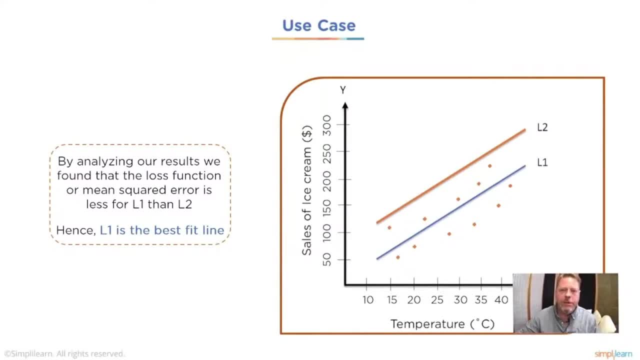 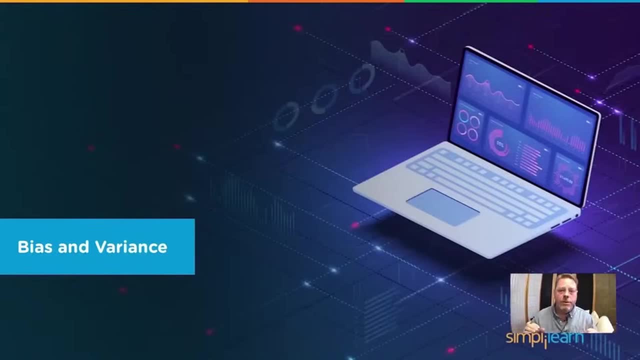 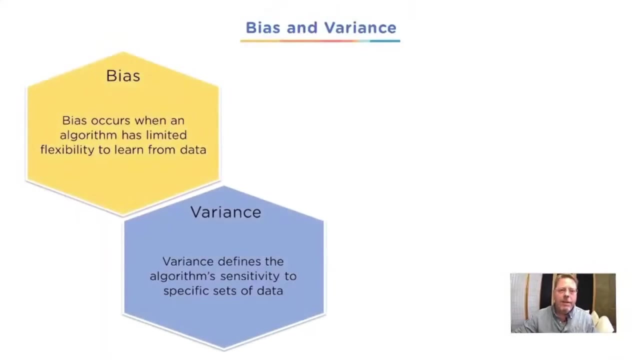 error is one of the better fits for doing this and most commonly used. We really want to talk about bias and variance, Very important terms to know in machine learning and with linear regression. So bias- Bias- occurs when an algorithm has limited flexibility to learn. 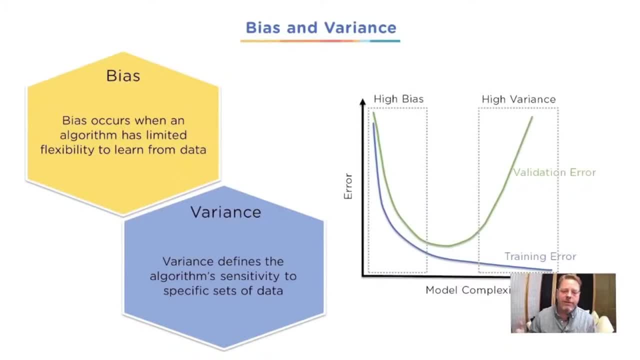 from data. Variance defines the algorithm's sensitivity to specific sets of data. Let's start with bias and variance. You can see here we have the two different setups. Bias, you can think, is very generalized, where variance is very specific When we talk. 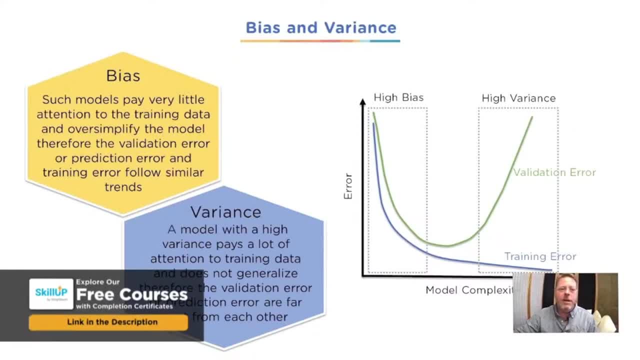 about bias. such models pay very little attention to the training data and oversimplify the model. Therefore, the validation error or prediction error and training error follow similar trends And with bias, if you oversimplify it so much, you're going to miss. 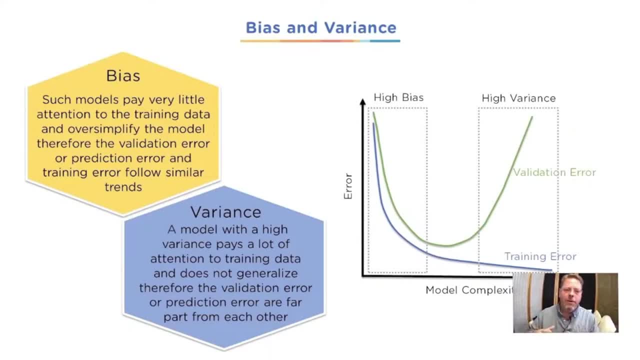 your local. if you have a really good fit, you're going to miss it. You're going to just kind of guess what the average is and that's what your answer is going to be. With variance, a model with a high variance pays a lot of attention to training. 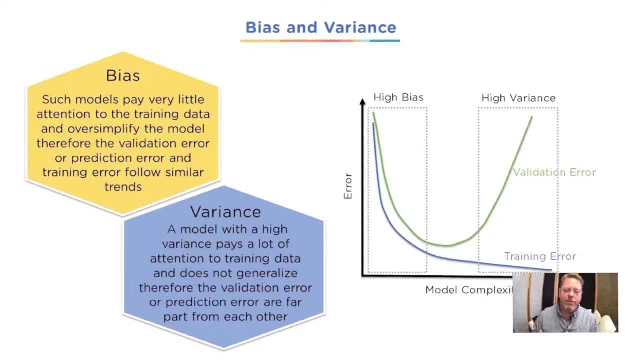 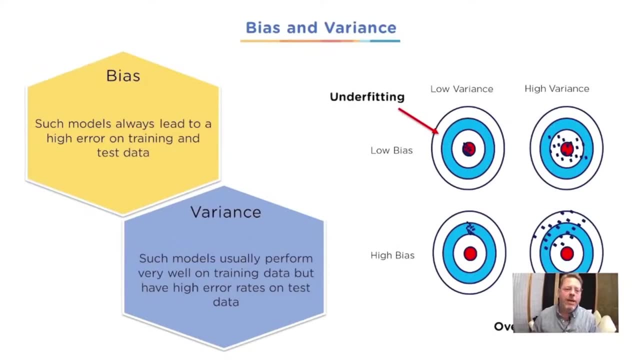 data and does not generalize. Therefore, the validation error or prediction error are far apart from each other. Such models always lead to a high error on training and test data, as a bias does Where variance. such models usually perform very well on training data but have high error. 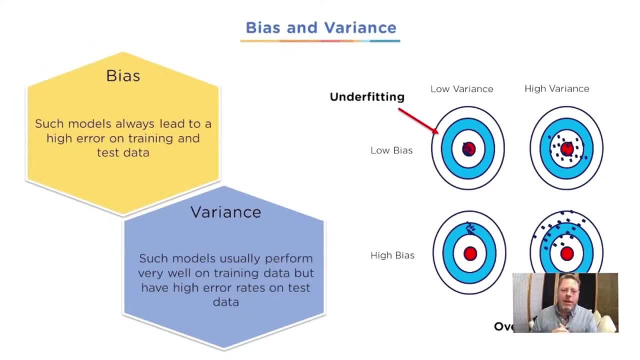 rates on test data, And I want you to think about this: When we're talking about a bias, the error is going to be high, both when you're training it and you're testing it. Why? Because we're just kind of getting an average. We're not really fitting it. 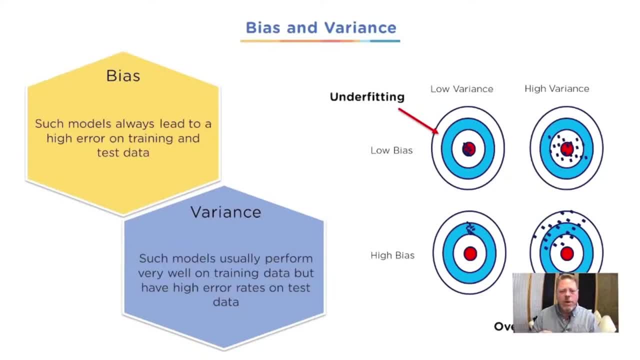 close With variance. we're fitting it so close that the test data does really good. It's going to nail it every time. If you're doing categorical testing, that's a car, that's a truck, that's a bicycle, But with variance. 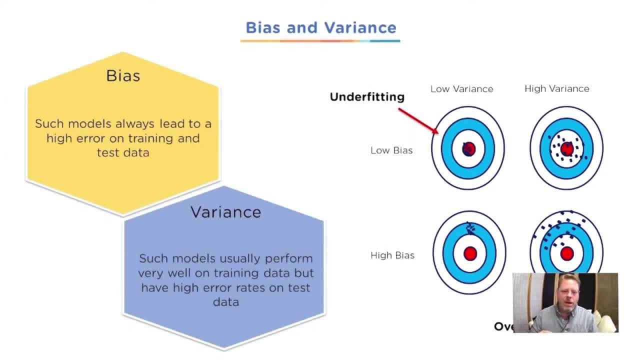 suddenly, a truck has to have certain features and it might have to be red because you had so many red pictures. So if it's an 18-wheeler, it has to be red. If it's blue, then it has to be a bicycle. 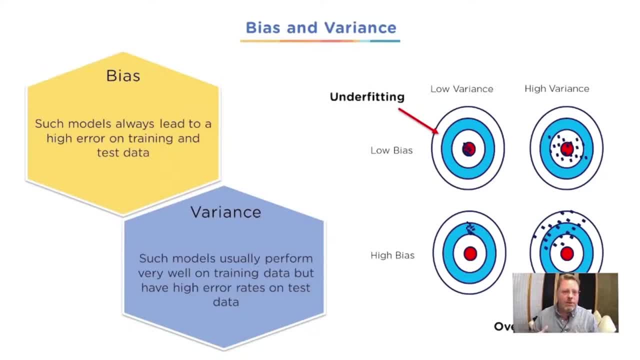 That's the kind of variance we're talking about, where it picks up on something and it cannot get the right answer unless it gets a very specific data. And we see that so that as you're testing it, your models and you programmed it, you've got to look for how. 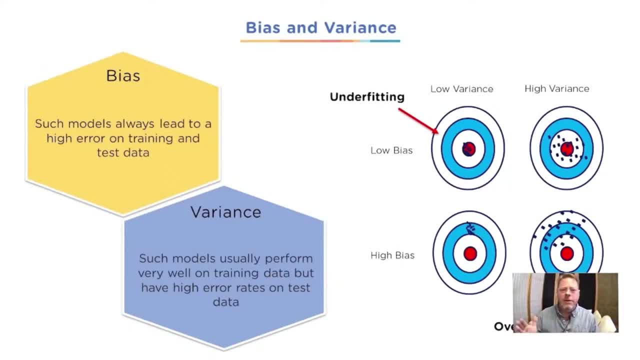 I trained it what is coming out, and if it's not looking good on either bias or if it's not looking good on the training or on the test data, then you're biased in your data. If it really looks good on the training data, then 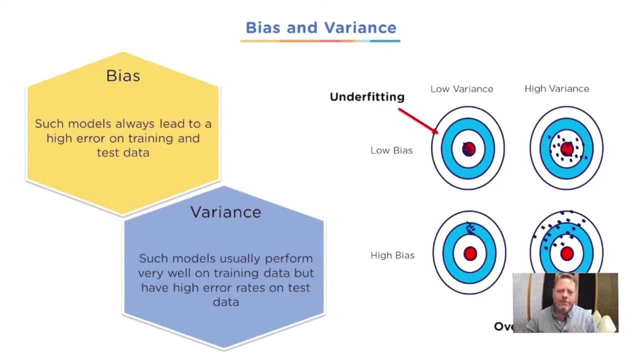 that's going to be your variance. You've overfitted the data, And those are very important things to know when you are building your models in regression of any kind or any kind of setup for predicting. So in dart games, if all the data 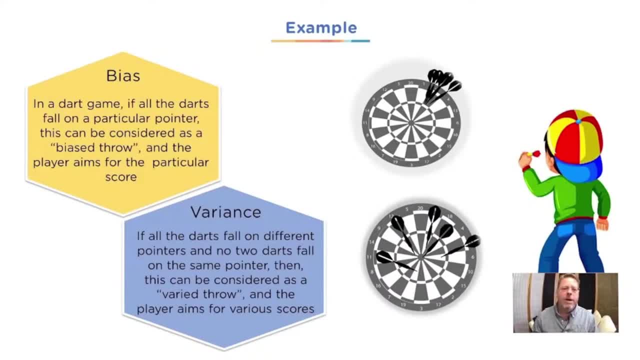 fall on a particular pointer, this can be considered as a biased throw and the player aims for the particular score For variance. if all the darts fall on different pointers and no two darts fall on the same pointer, then this can be considered as a varied throw. 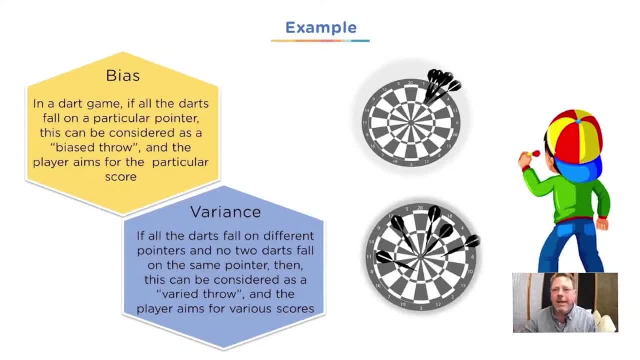 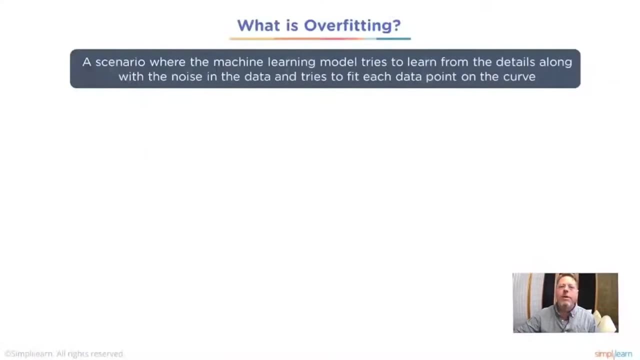 And the player aims for various scores. Again, the bias sums everything up in one point, kind of averages it together, where the variance really looks for the individual predictions coming out. So let's go ahead and talk about overfitting. When we talk about overfitting, 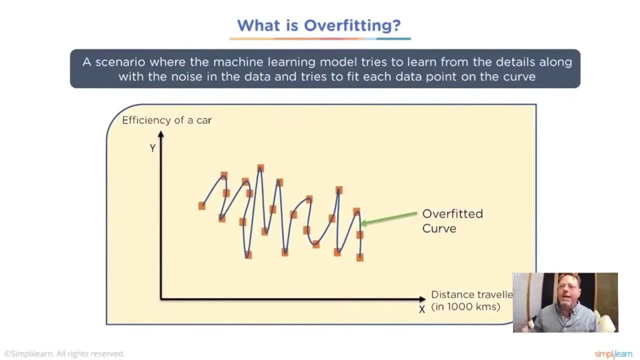 it's a scenario where the machine learning model tries to learn from the details, along with the noise And the data, tries to fit each data point on the curve. You can see that if you plug in your coordinates, you're just going to get whatever. 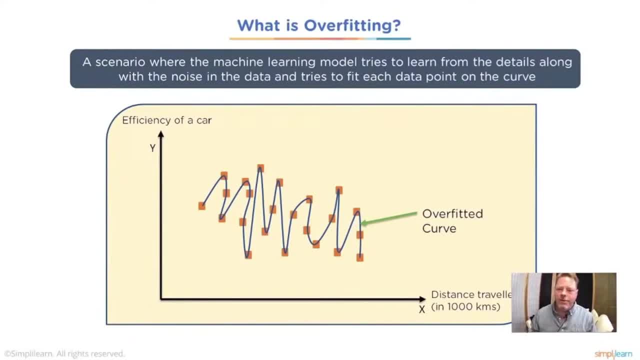 is fitted every point on the data stream. There's no average, there's no two points that might have two different answers, because if the wind blows a certain way, and the efficiency of your car, maybe you have a headwind, so your car might. 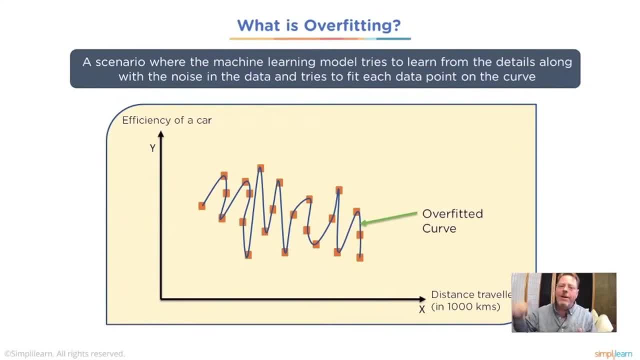 alter how efficient it is as it goes. So there's going to be this variance on here and this says no, you can't have any variance. It's going to be exactly this: You can't be the same speed or the same car and have a. 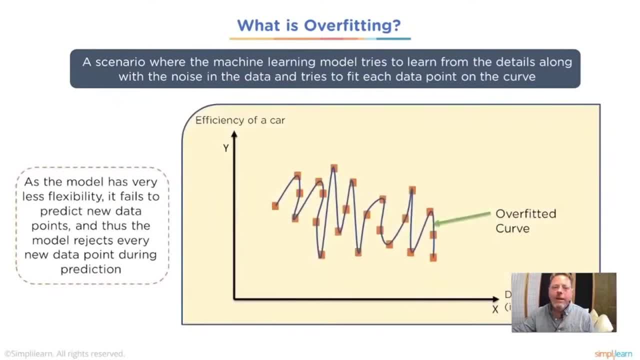 slightly different efficiency. So as the model has very less flexibility, it fails to predict new data points And thus the model rejects every new data point during the prediction. So you'll get like a really high error on here, And so reasons for overfitting. 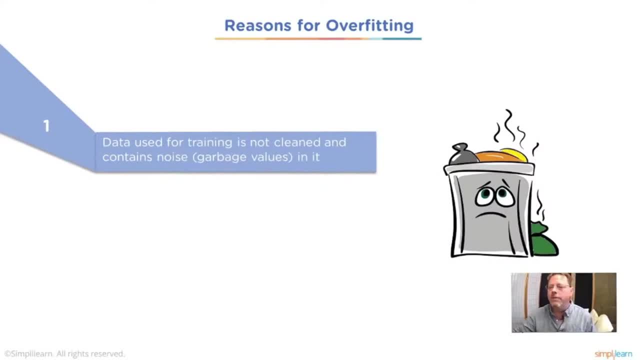 Data used for training is not cleaned and contains noise garbage values in it. You can spend so much time cleaning your data and it's so important. It's so important that if you have some kind of something wrong with the data coming in, 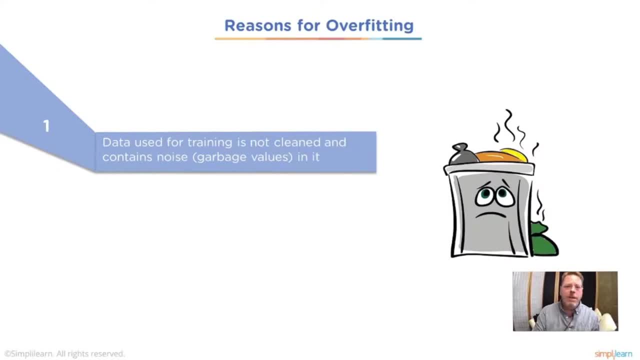 it needs to be addressed Whether it's the source of the data. maybe they use in medical different measuring tools so you now have to adjust for data that came in from hospital A versus hospital B or even off of machine A and machine B. that's testing. 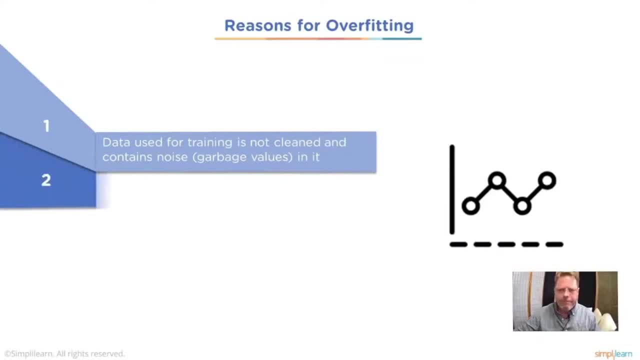 something and those numbers are coming in wrong. The model has a high variance. Again, wind is a good example. I was talking about that with the car. You may have a hundred tests, but because the wind's blowing, it's all. 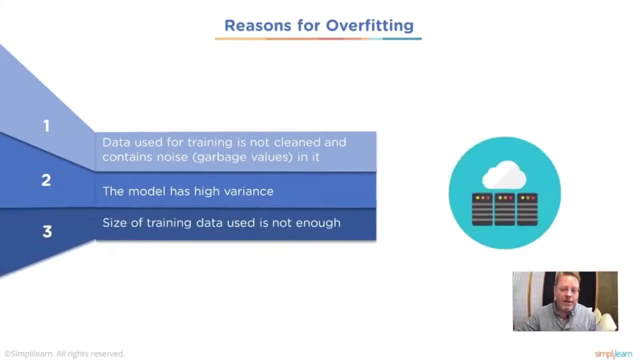 over the place. Size of training data used is not enough, so a small amount of data is going to also cause this problem. You only have a few points and you try to plot everything. The model is too complex. This comes up a lot. 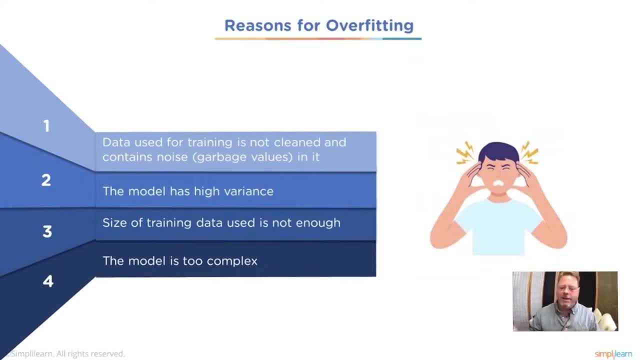 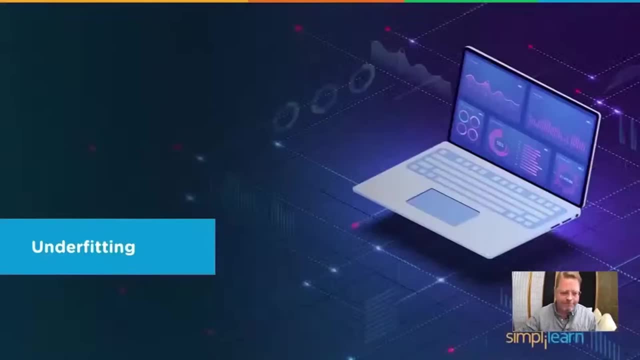 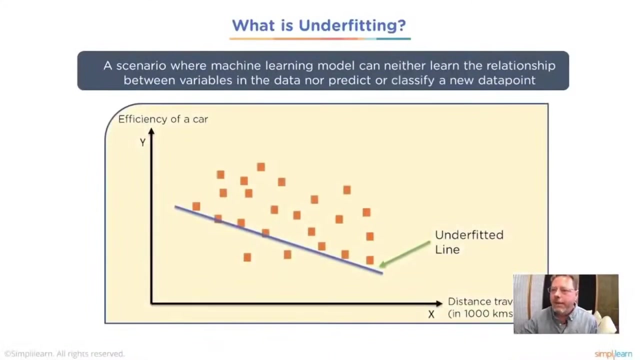 We put too many pieces together and how they interact can't even be tracked. You have to go back, break it up and find out actually what correlates and what doesn't. What is underfitting A scenario where machine learning models can? 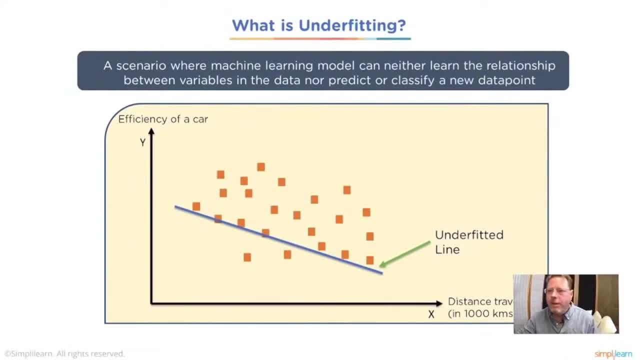 either learn the relationship between the data points, nor predict or classify a new data point. You can see, here we have our efficiency of our car and our line drawn and it's just going to be way off for both the training and the predicting data. 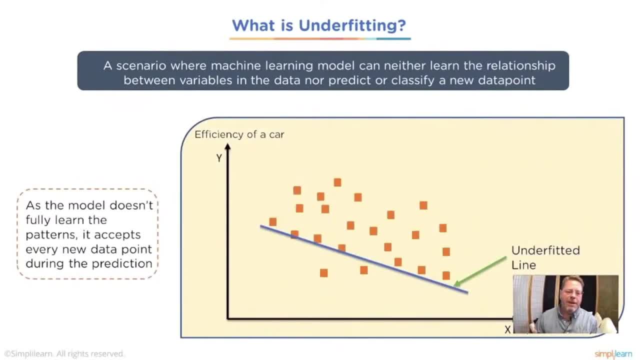 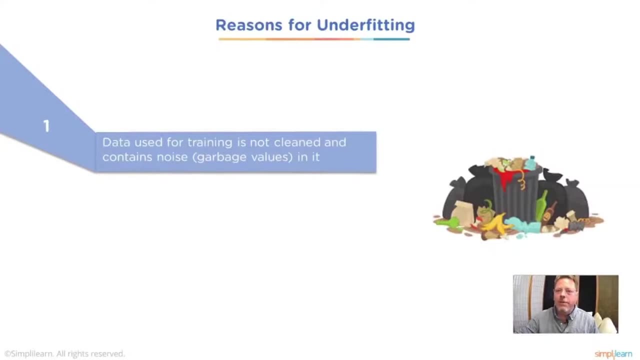 As the model doesn't fully learn the patterns, it accepts every new data point during the prediction Instead of looking for a general pattern. we just kind of accept everything. Data used for training is not cleaned: It contains noise, garbage and values. 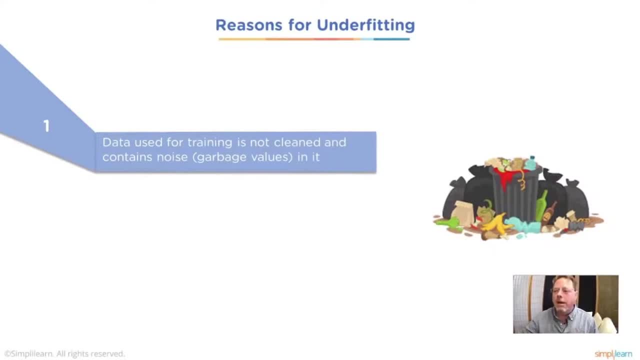 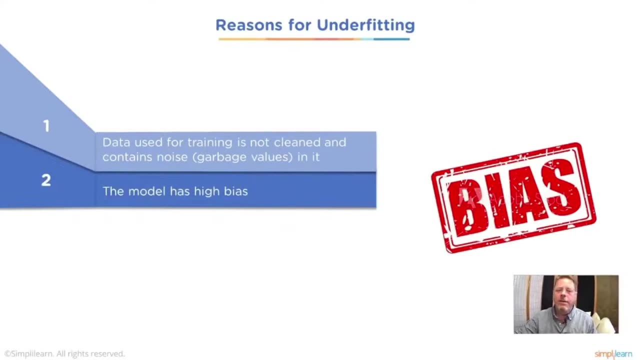 Again, underfitting and overfitting. same issue. You've got to clean your data. The model has a high bias. We've seen this in all kinds of things, from the most common is the driving cars to facial identification or whatever it is. 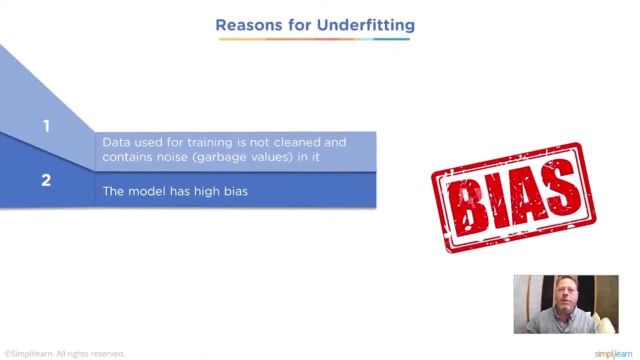 The model itself, when they build it might have a bias towards one thing. This would be an underfitted model, would have that bias because it's averaged it out If you have five people from India and ten people from Africa and twenty people from the US. 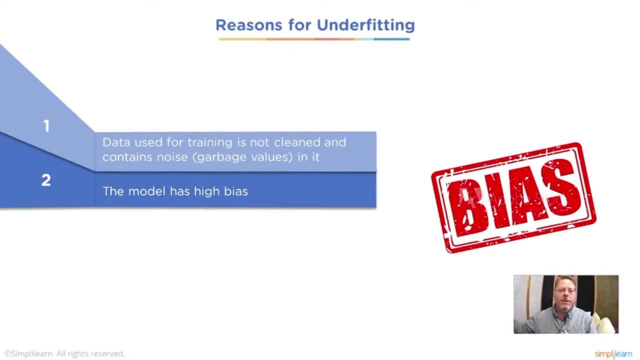 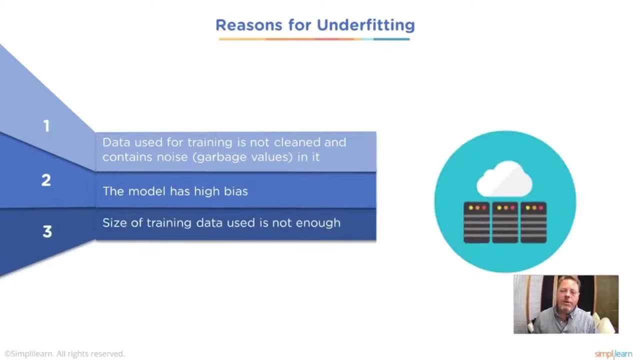 you've created a bias because it's looking at the twenty people and you only have a small amount of data to work with. Size of training: data used is not enough. That goes with the size I was just talking about. We have a model with a high bias. 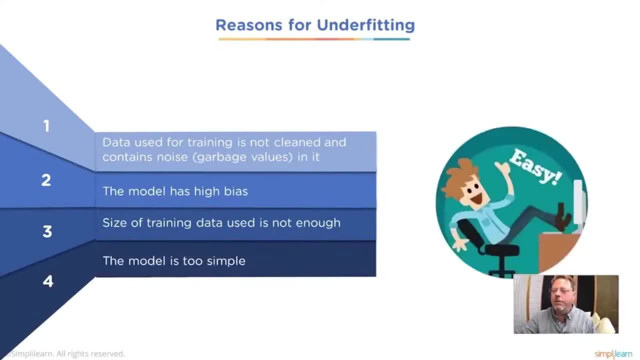 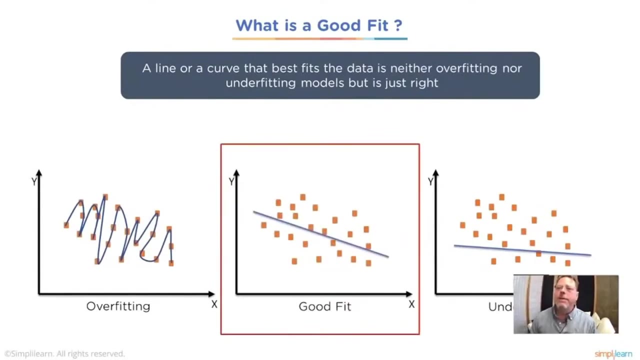 We have size of training. data used is not enough. The model is too simple. Again, this is one straight line through all the data, when it has a slight shift to it for other reasons. What is a good fit? A linear curve that best fits the data. 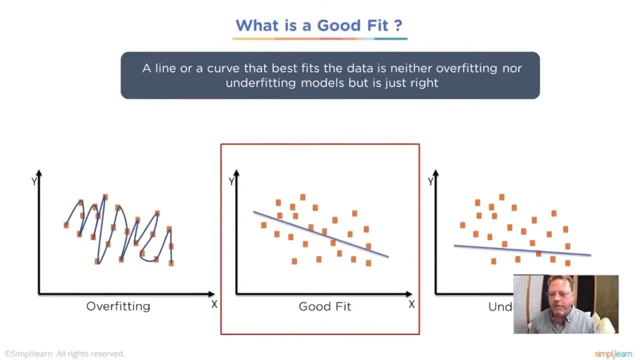 is neither overfitting or underfitting models, but is just right. Of course we have the nice examples here where we have overfitting lines going up and down. every point is trying to be included. underfitting the line really is. 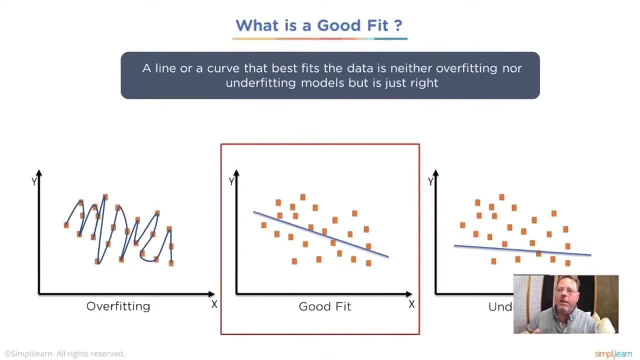 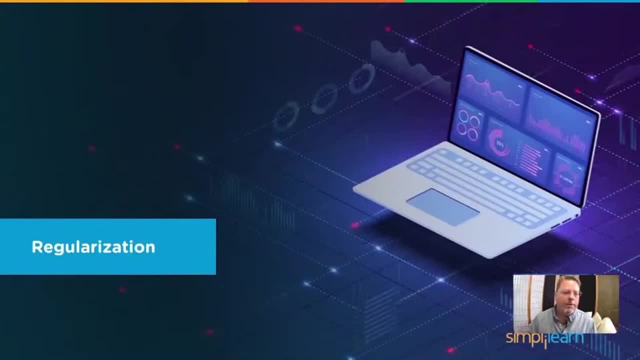 off from where the data is and then a good fit is minimize that error. coming through Regularization is taking the guesswork out. You're looking at this graph and you're going which one. is that really overfit or is that underfit? That's pretty hard to tell. 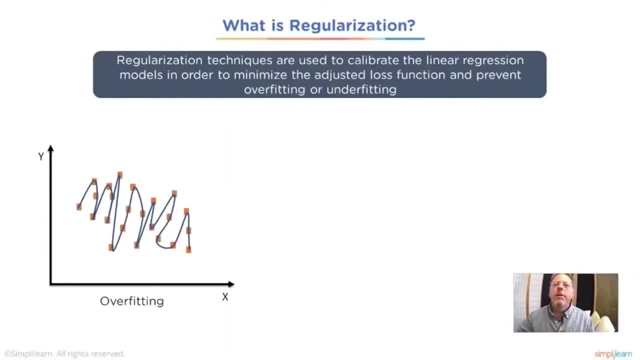 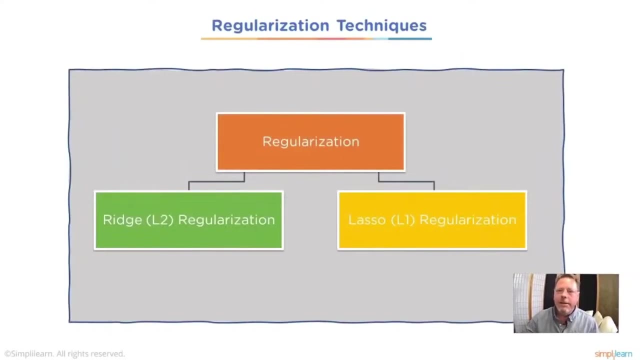 We talk about regularization. Regularization techniques are used to calibrate the linear regression models and to minimize the adjusted loss function and prevent overfitting or underfitting What that means in this case. we're going to go ahead and take a look at a couple different things. 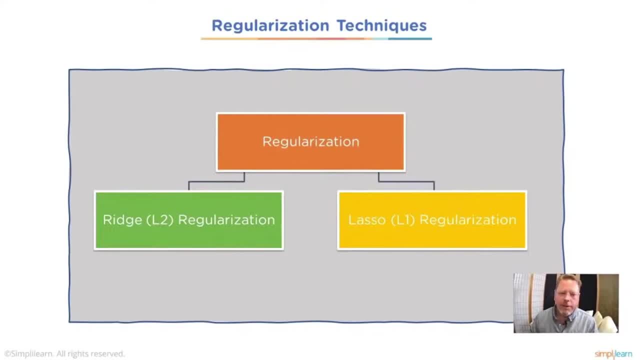 We're going to look at regularization, which will start with a linear model. We'll look at the ridge regularization and the lasso regularization. These models are just like we did the MLP, the multi-layered positron in the sklearn module You could bring in. 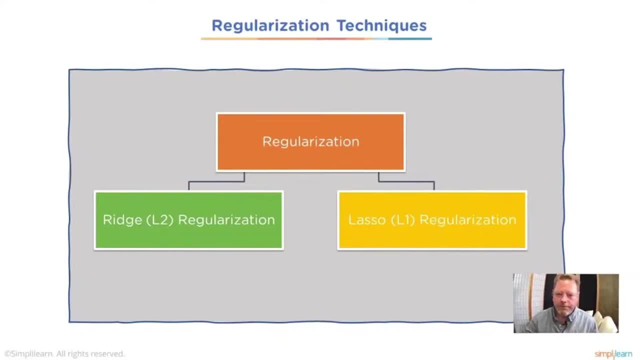 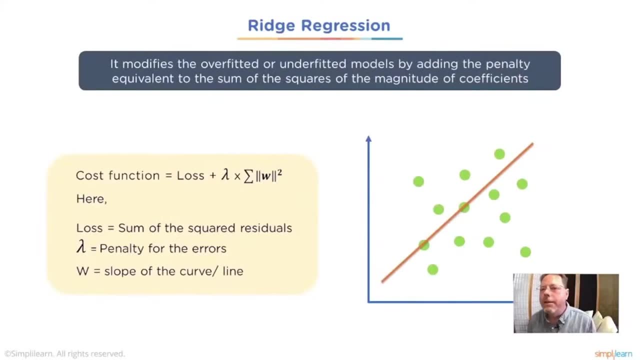 the ridge module and you can bring in the lasso module. When we talk about ridge regression, it modifies the overfitted or underfitted models. by adding the penalty equivalent to the sum of the squares of the magnitude of the coefficients, We have a cost function. 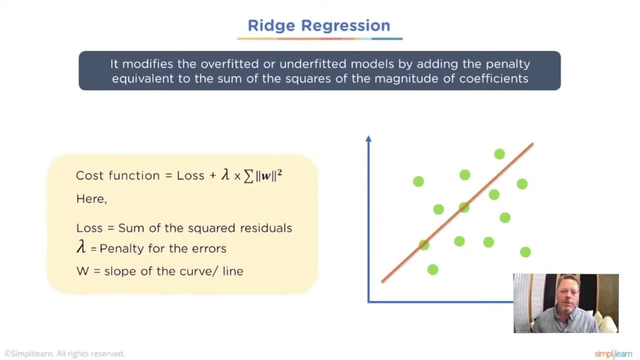 equals loss, equals lambda times the sum of w squared, or the absolute value of w, depending on how you're doing it. Remember we talked about error, whether we either square it or we absolute value it, because that removes the plus or minus sign on there. There's reasons to do it either way, but it is more common. 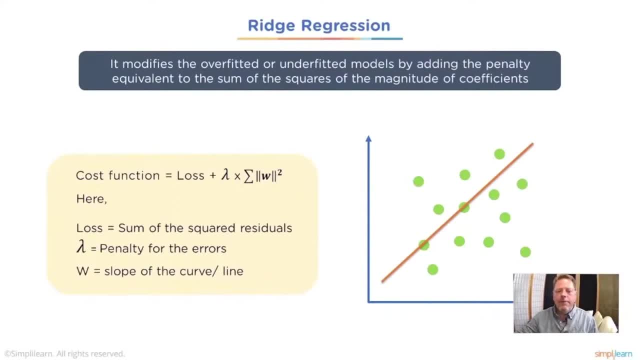 to square the value, Then we have our. in this case, the lambda is going to be the penalty for the errors. We've thrown in a Greek character for you just to confuse everybody. This is the slope of the curve of the line. We're going to look at this. 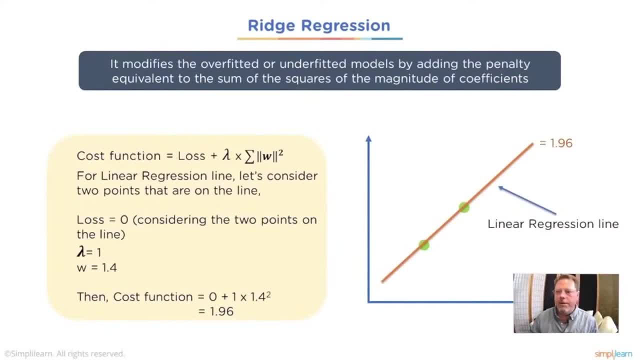 and we're going to draw a line. This is going to be like a linear regression model In sklearn. you could import just a standard linear regression model. It would plot this line across. whatever data we're working on, We look at this and, of course, we're just extrapolating this. 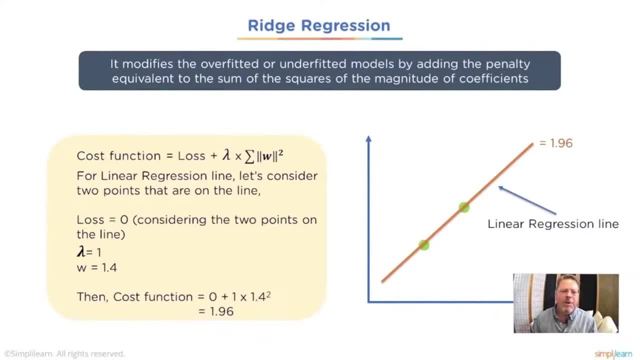 I know they use some specific data but don't want to get into the actual domain For a linear regression line. let's consider two points that are on the line. We'll go ahead and have a loss equal zero. considering the two points on the line. We'll go ahead and do lambda. 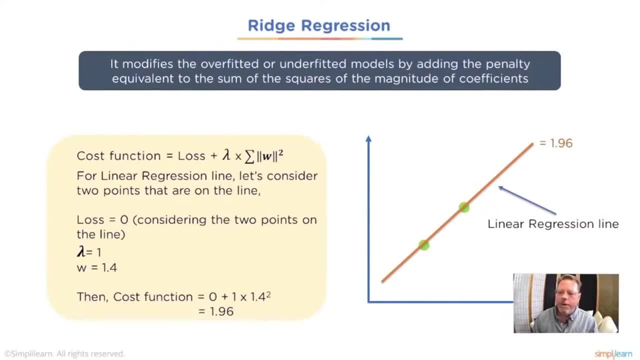 equals one. We'll set our w is going to be one point four. Then the cost function equals zero plus one times one point four squared, which equals one point nine six. Really, don't get caught up too much in the math on this, other than understanding. 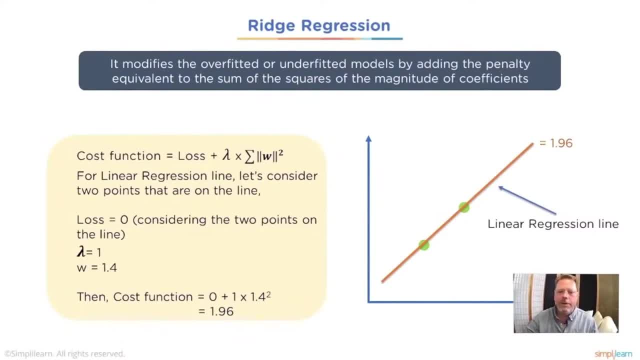 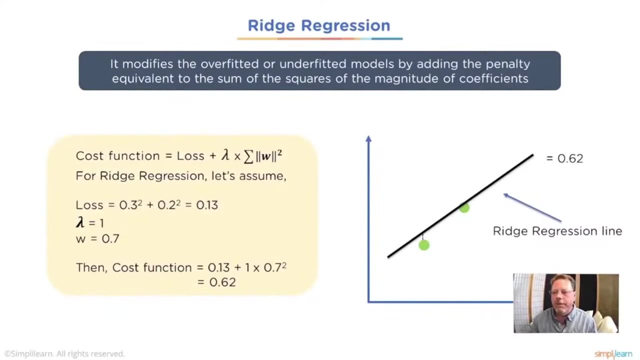 that this is something that's very easy for a computer to calculate. If you ever see the loss plus the lambda times the sum of w squared, Then let's say we have a ridge regression line and we go ahead and plot it and we do the calculations on the data. 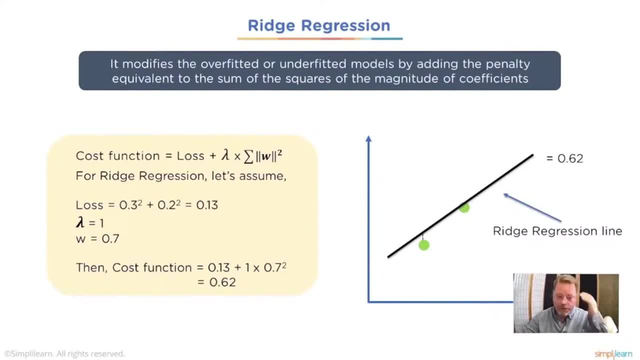 For the ridge regression. let's assume a loss equals point three squared plus point two squared equals point one. three. When we put all the calculations through of the two points, we end up with point six, two. We've now had a linear regression model. We now had a ridge. 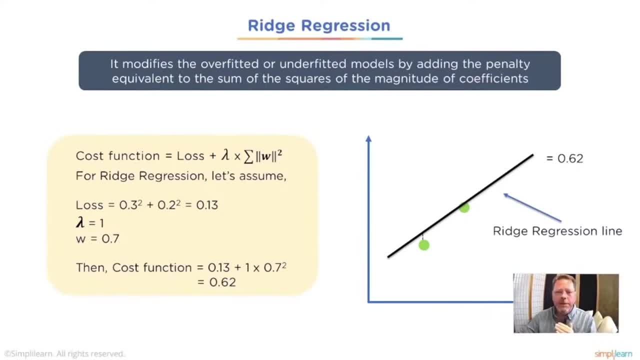 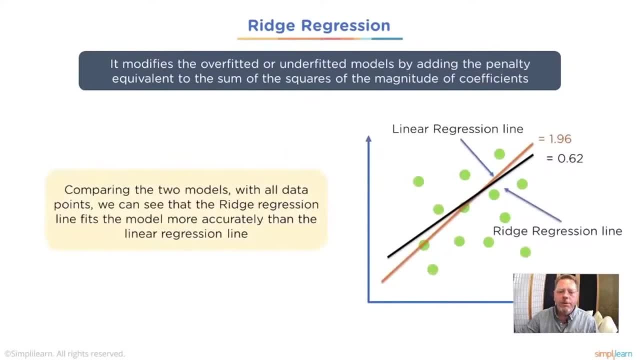 regression model. The ridge regression model plots a little differently than the standard linear regression model. Comparing the two models with all the data points, we can see that the ridge regression line fits the model more accurately than the linear regression line. I find this true on a lot. 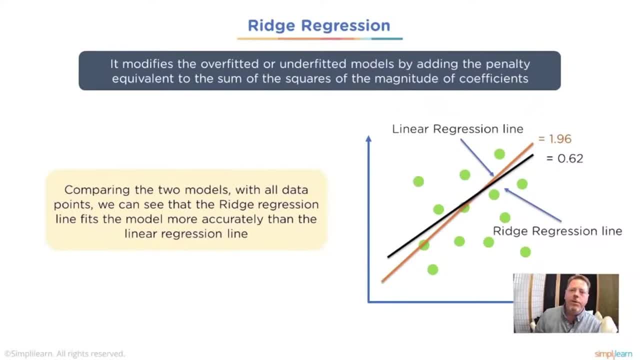 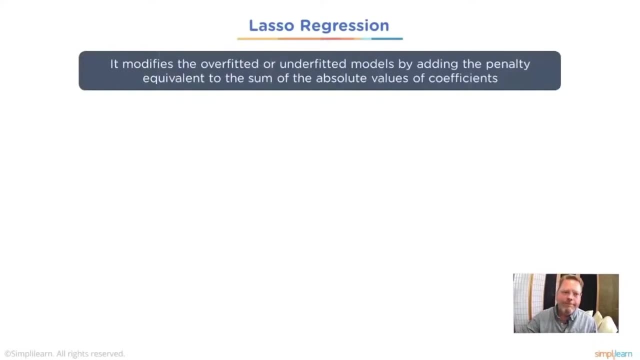 of data I work with, I'll end up using either the ridge regression model or the LASSO MARS regression model for fitting, Especially dealing with a lot of stock markets daily setup. they come out slightly better. You get a slightly better fit. 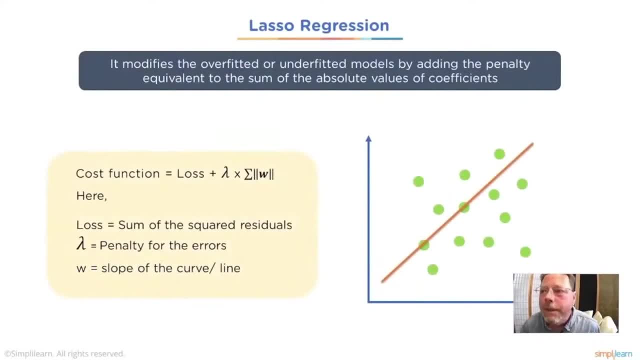 We have our LASSO. We just talked about LASSO coming in here. The cost function equals. instead of doing a squared, we're just going to do the absolute value. If you remember, this is where ridge regression changes. Where's my ridge regression model? 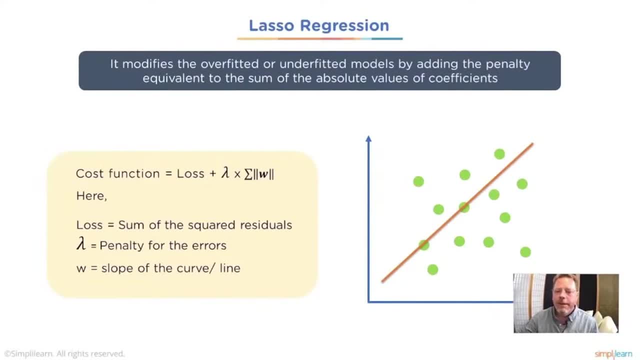 We're squaring the value here, If you look at this. we're not squaring the value, we're just finding the absolute value on here: The loss of the squared individuals. and here is our lambda symbol again: Penalty for errors. W equals. 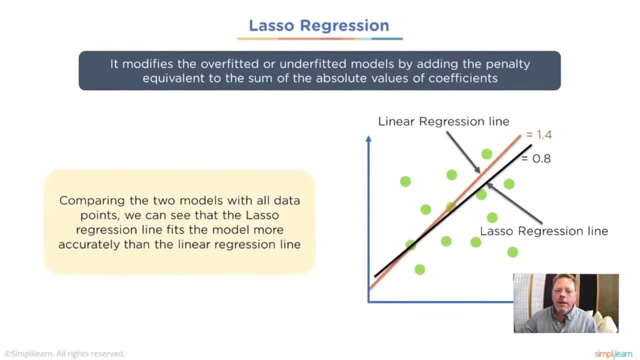 the slope of the curve. Comparing the two models with all the data points, we can see that the LASSO regression line fits the model more accurately than the linear regression line. This is like I said a lot. I use these two models a lot. 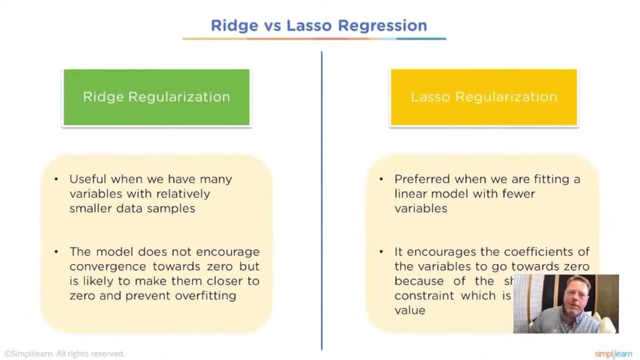 The ridge, and this is important. this is kind of the meat of the matter. How do you know which one to use? Some of it is. you just do it a bunch of times and then you figure it out. Ridge regularization is useful when we have. 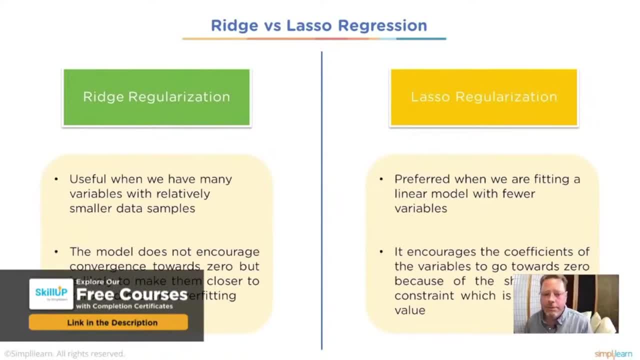 many variables with relatively smaller data samples. The model does not encourage convergence towards zero, but is likely to make them closer to zero and prevent overfitting. The LASSO regularization model is preferred when we are fitting a linear model with fewer variables In the IRIS thing we had. 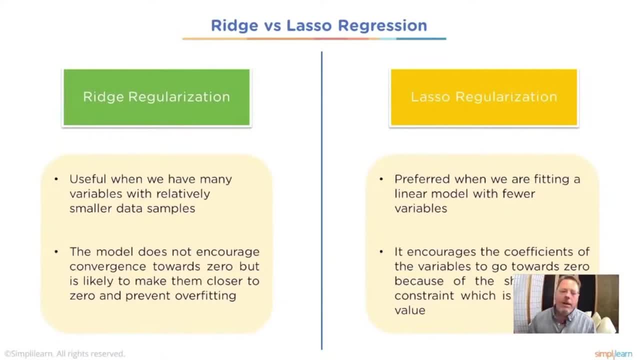 four or five variables as we measured the different leaf pieces. You might be doing the measurements on the cancer project, which has 36 different variables As we get down to the IRIS with four variables. LASSO-LAR will probably work pretty good where you might use the. 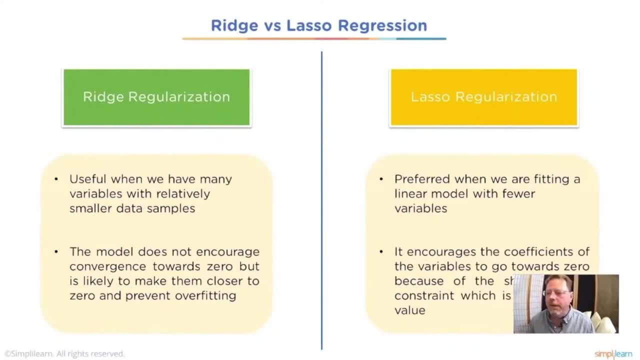 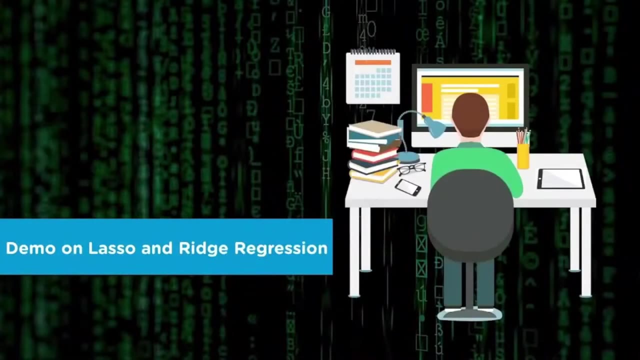 ridge regularization with more models If you have something significantly larger, and it encourages the coefficients of the variables to go towards zero because of the shape of the constraint, which is an absolute value. With any of this, we want to go ahead and do a demo in LASSO. 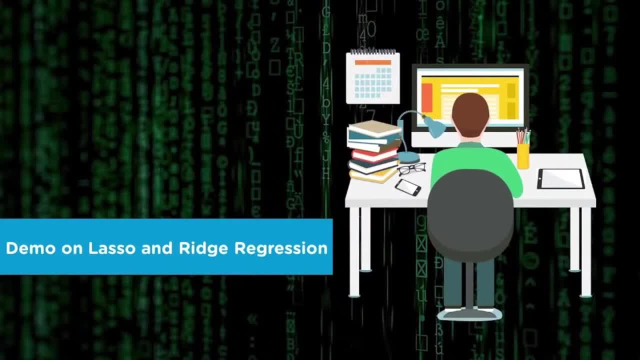 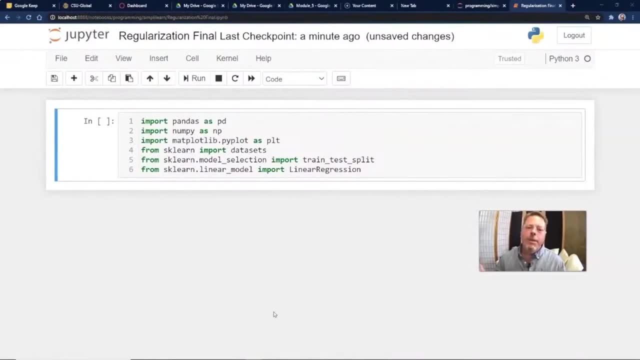 and ridge regression. Let's take a look and see what that looks like in our code and bring up our Jupyter Notebook. We'll start with our imports. Pandas is PD Import. numpy is NP. Import. matplotlib is PLT. Sklearn- we're going to import our dataset. 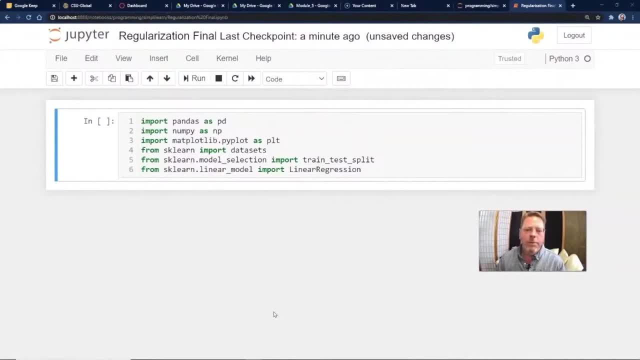 which is kind of more generic. We usually just import one dataset instead of all of them. Quick and dirty when you're putting some of these together. We have our sklearn model selection. We're going to import our train test split for splitting our data up. 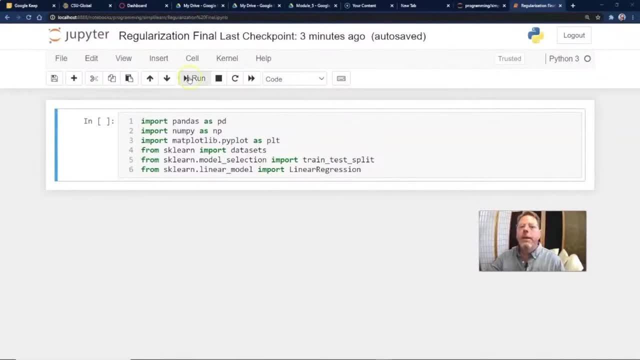 Then we'll bring in our linear regression model. We'll go ahead and run these just to load them up, Then load our dataset. We were just talking about that. You could just have imported the load Boston dataset in there instead of loading all the. 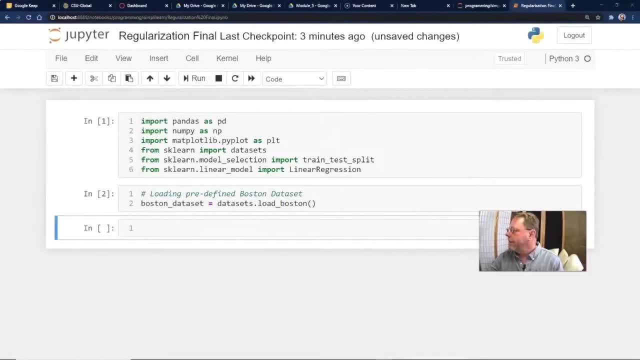 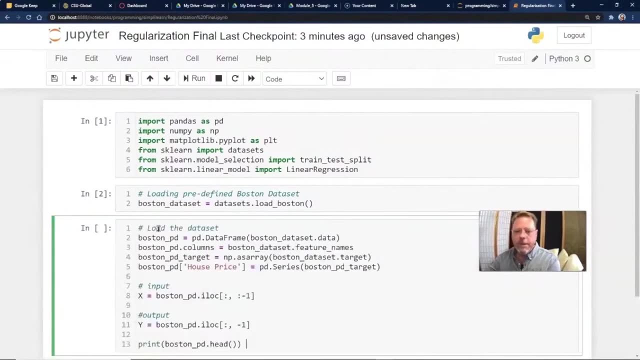 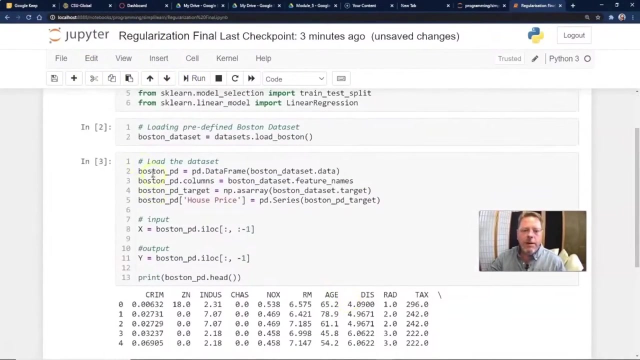 datasets. Then, once we've loaded our dataset, we want to go ahead and take a look at that data and see what we've got here. Let me just go ahead and pop that down there and go ahead and run it. We've gone ahead and taken our 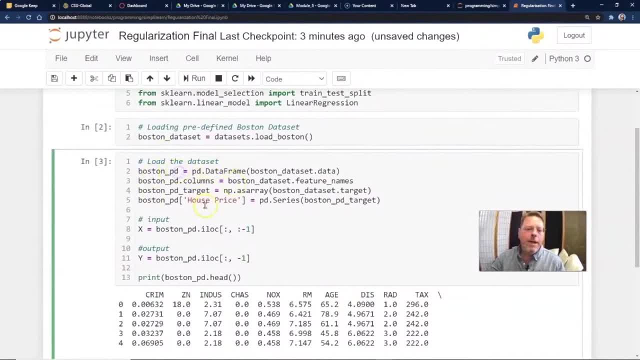 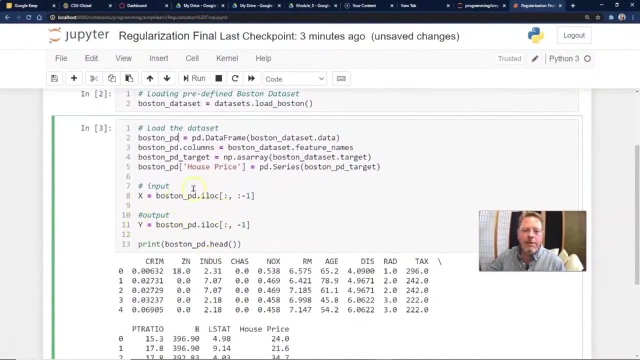 Boston data. We've put it into our Pandas data frame, the Boston dataset and then the Boston columns. We want to see what's going on with them. We have our target, we have the house price, etc. Our x equals Boston. 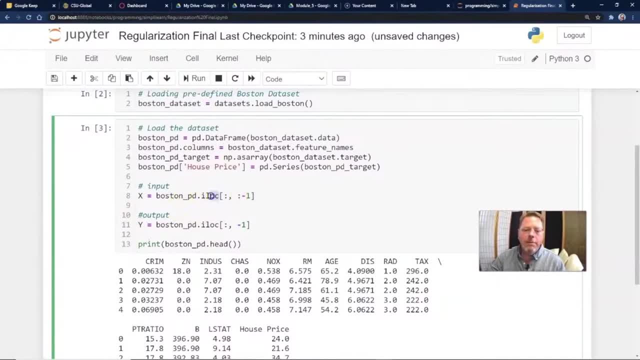 iLocation. Remember in Pandas- the new updates to Pandas- they want iLocation if you're going to pull data. We used to be able to leave this off, but it does something different. It creates a slice versus a direct setup, so make sure you're using that iLocation. 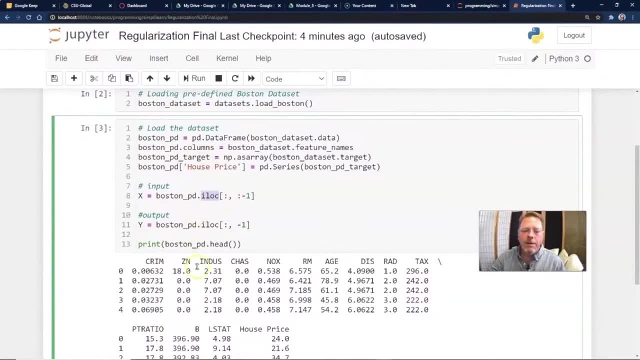 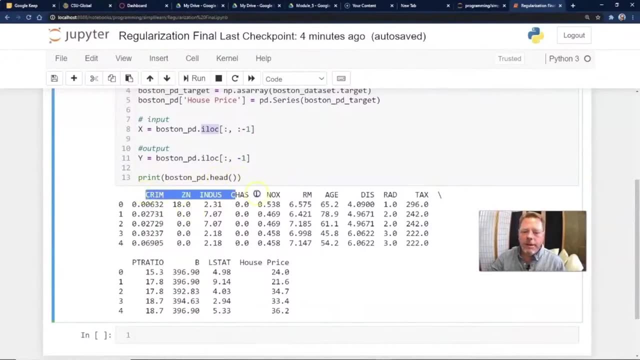 and the output. This is all just bringing our data together. We can see here, if we print the Boston Pandas head, we can see here all of our different aspects we're looking for. If you're following the x and the y, the x is everything. 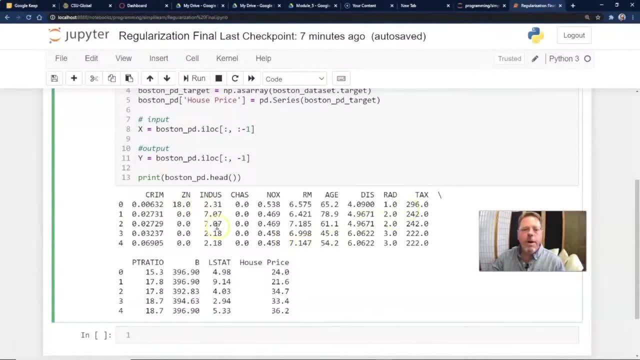 except for the last column where y is all the rows, except for the last column, and then y is all the rows, but just the last column. y is our house price and the x is the Crim ZN Industry, Chas, Knox and all these other. 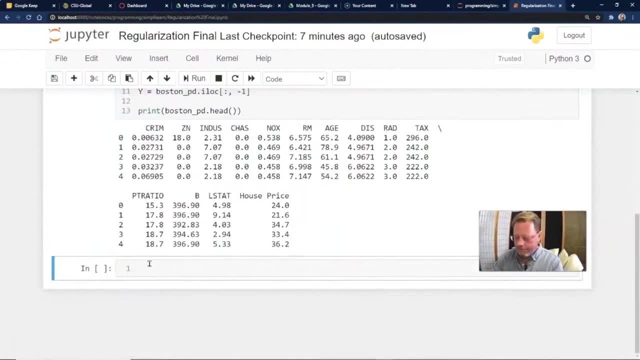 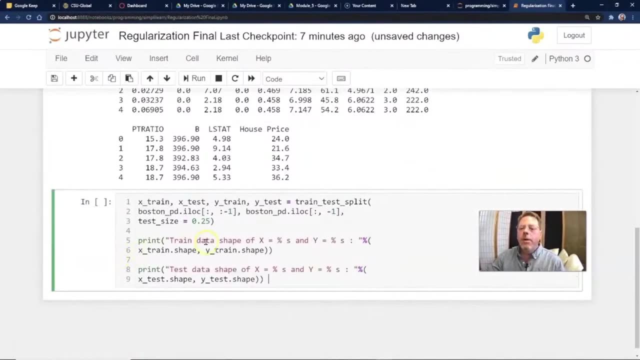 different statistics they've collected for house sales in Boston. We'll go ahead and split our data: x train and our x test, y train. y test equals the train test split which we imported. We have our Boston. you could have easily used the x and y on here. 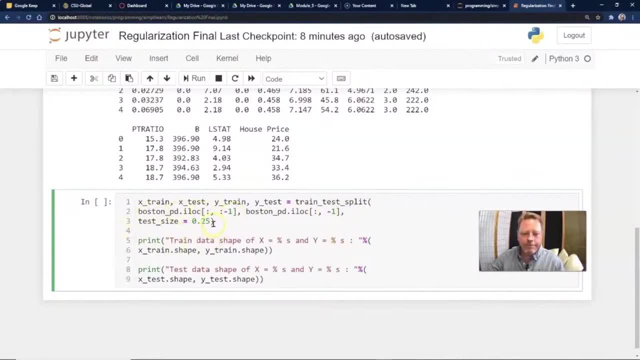 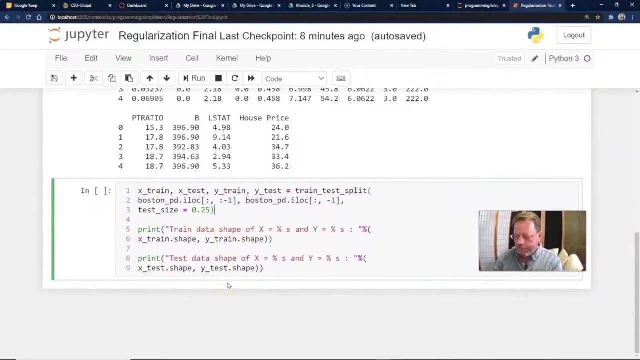 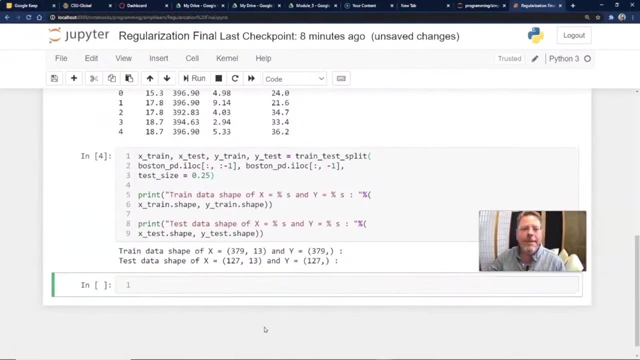 as opposed to Boston iLocation. We'll create our test size. We're going to take 25% of the data and put it in as a test. We'll go ahead and run this. Need an extra drink? there We have our train. 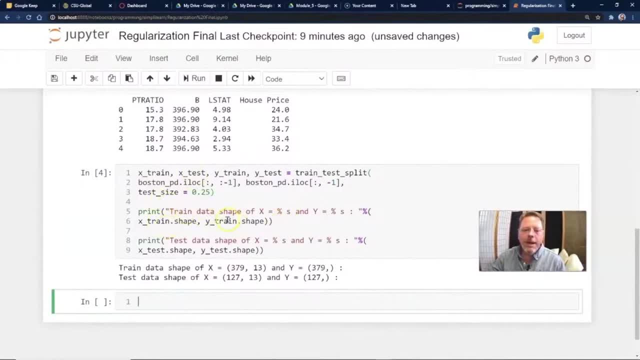 and test. and then, of course, the print, the train data shape. I love doing this kind of thing Whenever I'm working with this data print out the shape, Make sure everything looks correct so that we have 127 by 13 and 127 by 1. 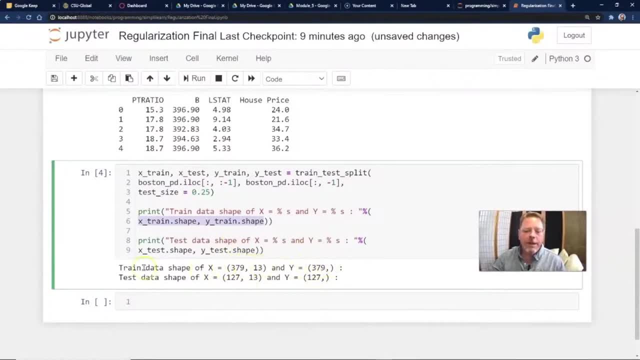 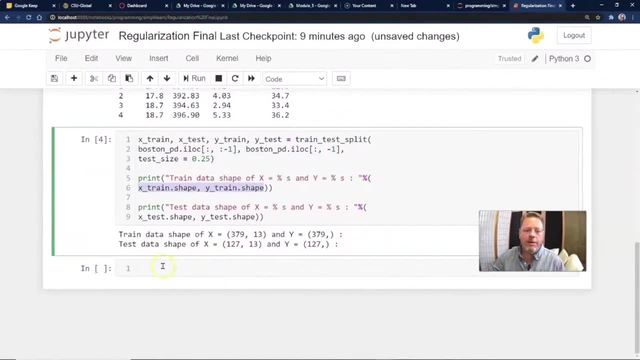 379 by 13, they should match. If the data sets are not quite matching, then you know something's wrong and you're going to get all those errors. I don't know how many times I've gone through here and it's dropped a row on one of them. 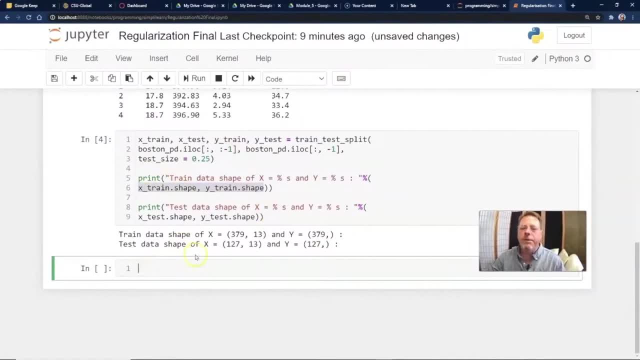 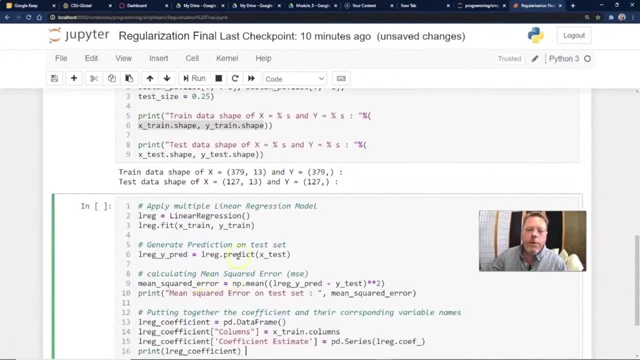 and not on the other, or something weird has happened when I'm cleaning the data. It's simple, because the data comes in a nice prepackage and is all clean for you, Let's go ahead and apply the multiple linear regression model. We'll call this. 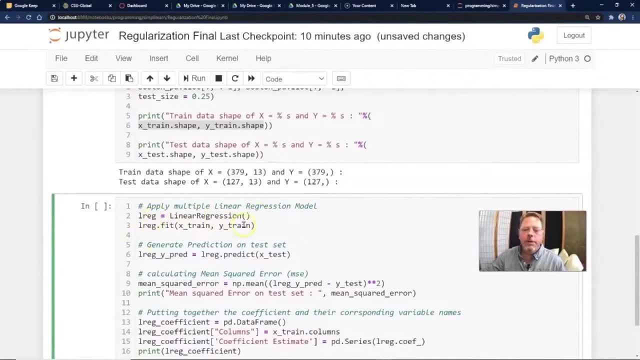 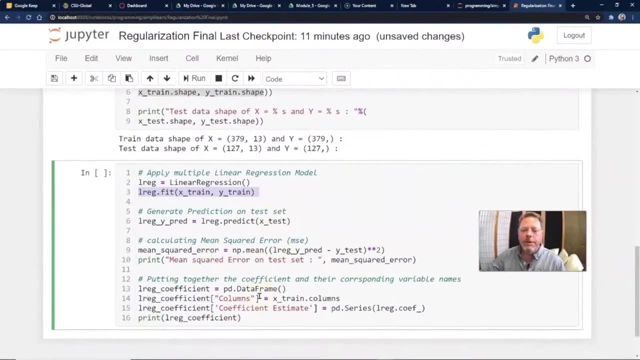 LREG linear regression. We're going to go ahead and fit that linear regression model to X train and Y train. Then we'll generate the prediction on the test set. Here's our LREG Y predict with our test going into the prediction. Now let's 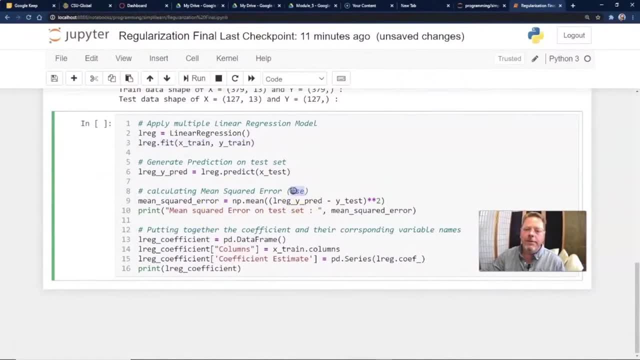 calculate that mean square error MSE. I told you you'll see MSE used a lot. People use it in variables and things like that. It's pretty common. We get our mean squared error equals. this is just the basic formula we've already been talking about. What's the difference? squared? 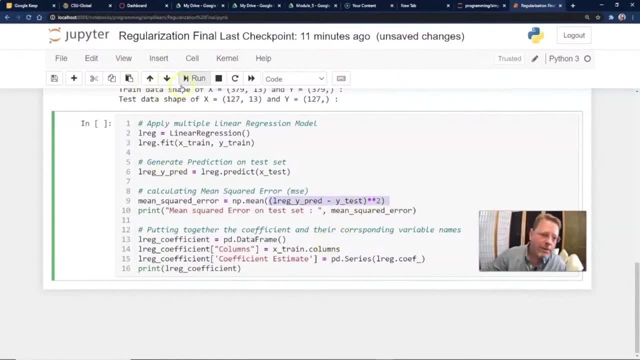 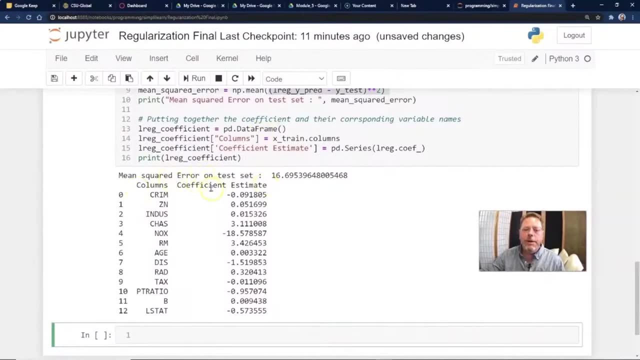 Then we look for the average of that. We'll go ahead and just run this. You can see, when we get through the end of this, we have our mean square error on test, we have our total and then we have each column coming down. 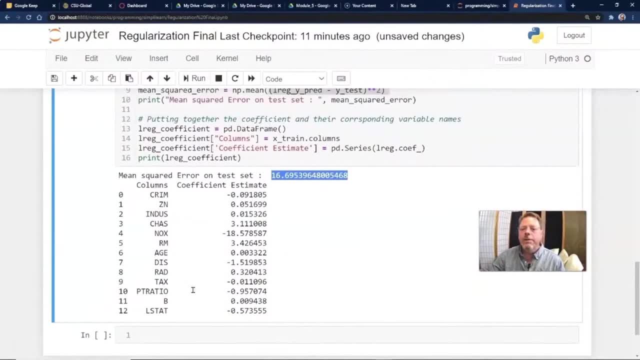 At this point, unless you really know the data you're working with, it's not going to mean a whole lot. If it's in your domain, you might know what you're looking at when you see these kinds of numbers coming up. If it's not, it's just a bunch of numbers. 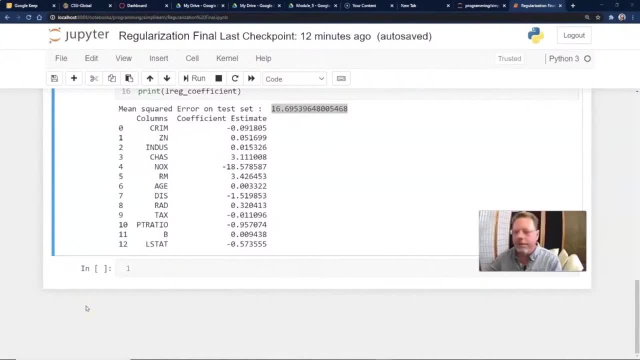 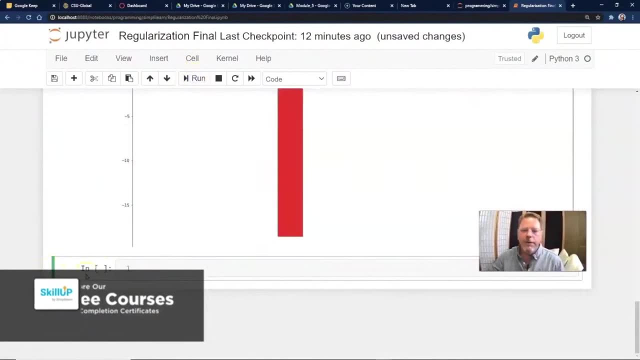 and that's okay- At least that's okay for this demo. Then we're going to go ahead and plot these so we can see what's going on. This is always kind of fun. It's always nice to have a nice visual of what you're looking at. 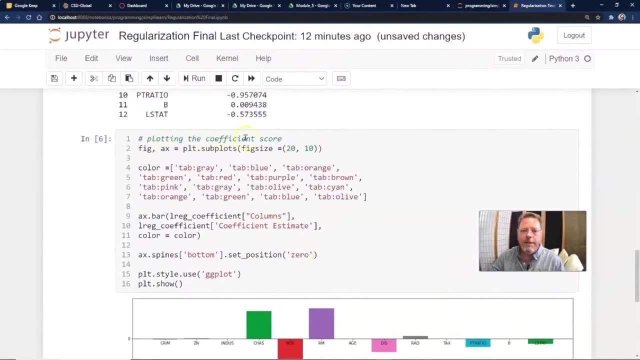 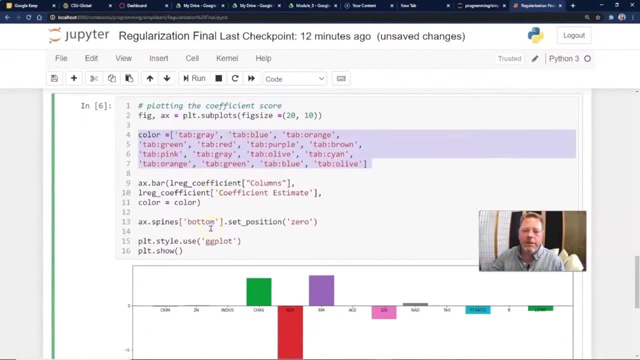 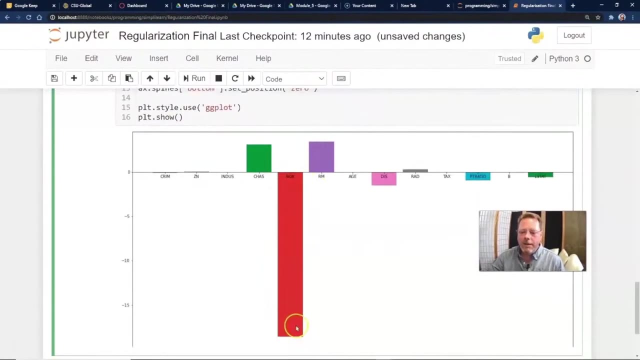 You can see here when we plot the coefficient scores on here. the guys in the back did a great job putting some pretty colors together and making it look nice and setting up the columns. You can see here: your NOX has just a huge coefficient. 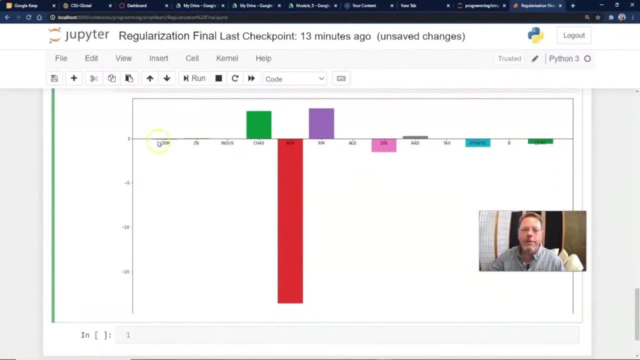 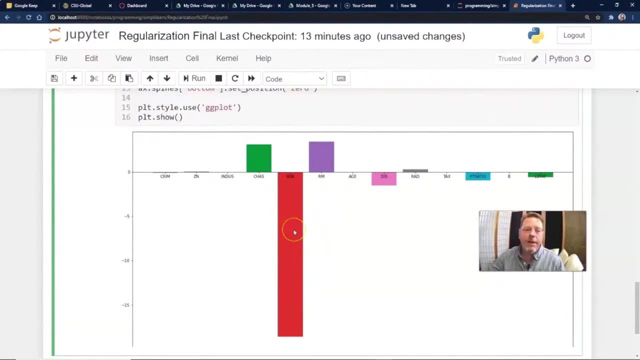 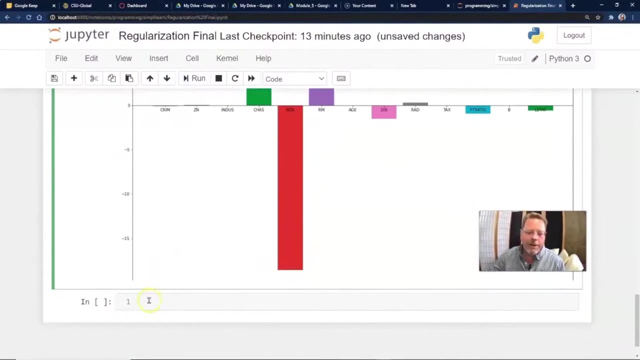 When I look at a table like this, I look for what has very little value and different coefficients- They're not using a huge change- and what has huge changes. That flags you for all kinds of things as you're working with the data, but it depends so much on the domain you're working with. 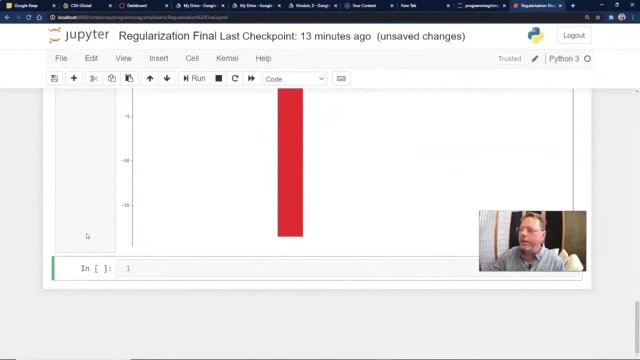 These are great things, though, as just a quick look to see what's going on with your data and what you're looking for, Of course, once we look at this now, our motive is to reduce the coefficient score. Now we want to take these: 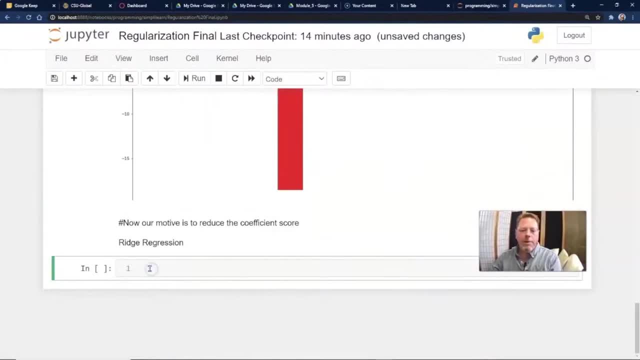 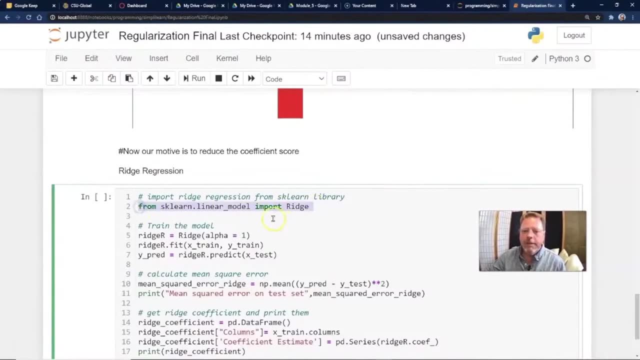 and bring them down as much as we can. For that we're going to put the ridge regression on here. Let's start by going ahead, and we're going to import our ridge model, the ridge regression, from the sklearn library or the scikit. 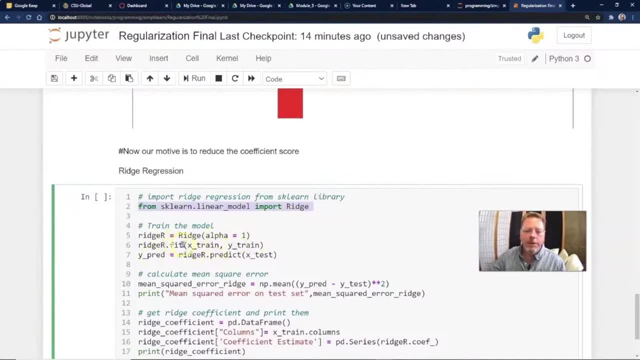 We're going to go ahead and train the model. Here's our ridge: alpha equals one. I mentioned that earlier. When I work with the ridge model you'll see alpha equals one If you set alpha equal to zero. that's a standard linear regression model. 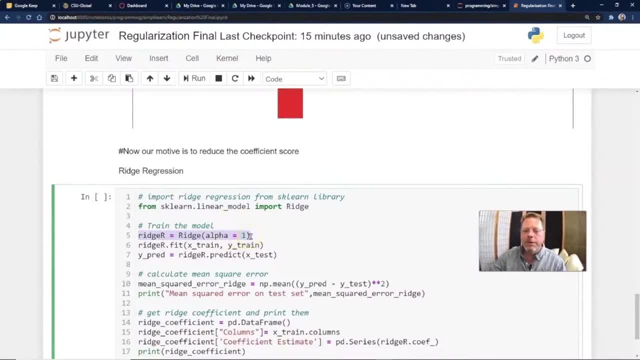 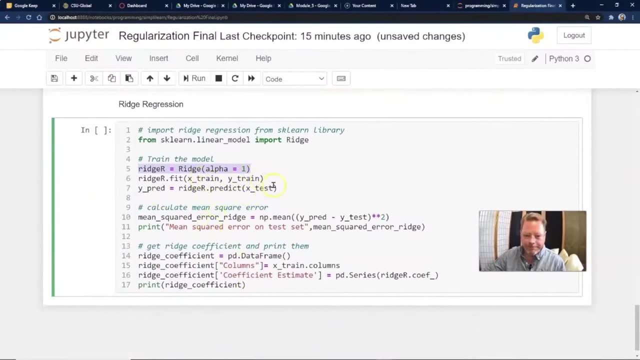 You have alpha equals one, two, three, four and a standard integer on there. We'll go ahead and fit the ridge model on there with our x-train and our y-train data generate a prediction for that for our x-test. 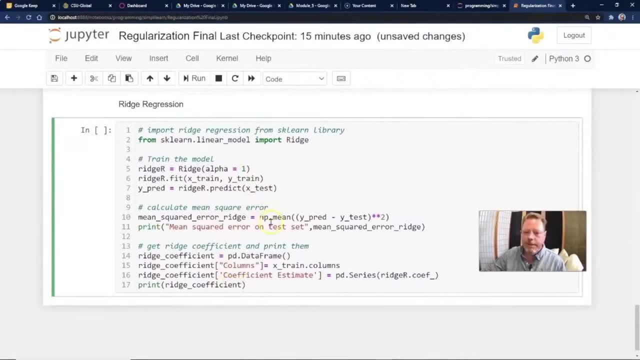 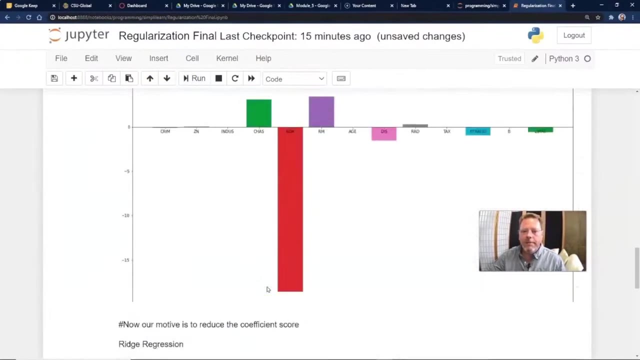 and we'll calculate the mean square error just like we did before. This should all look familiar. We'll go ahead and print that out and we'll look at the ridge coefficients for our data and see what that looks like Now, if you jump up and down. 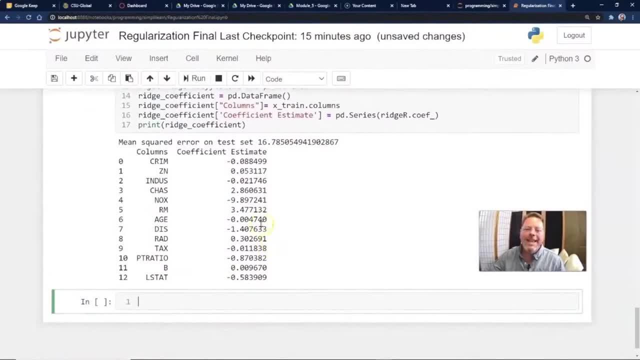 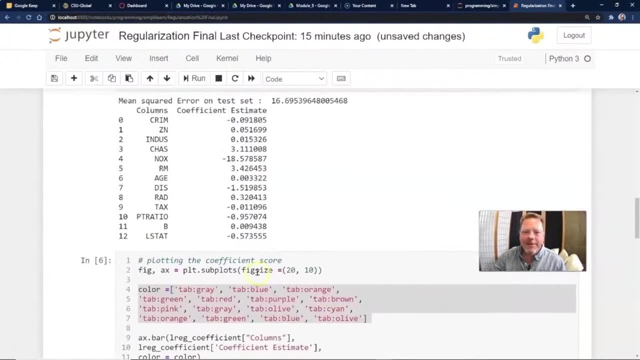 between these two, you'll get a headache. You'll still see the NOX value. Let's just look at the NOX, because that was the biggest value. It's a minus nine here. If we go back up here, the NOX value is a minus 18.. 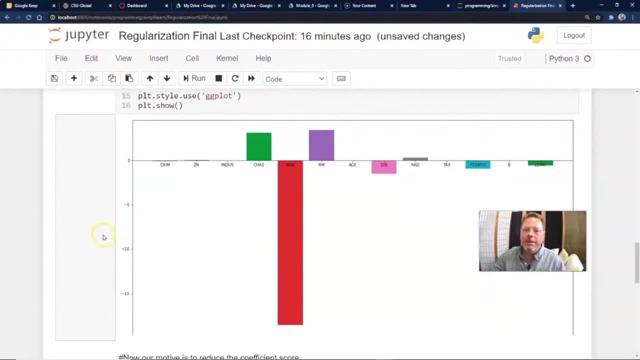 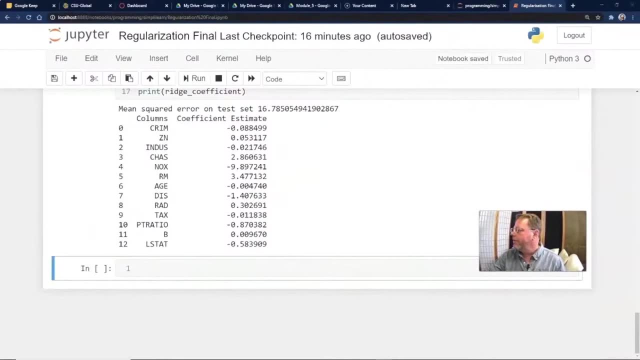 Right off the bat. I'm seeing a huge change in the biggest coefficient there. If we're going to do that nice setup, we want to go ahead and just print it and see what that looks like. Here we go. We've set up our plots, subplots. 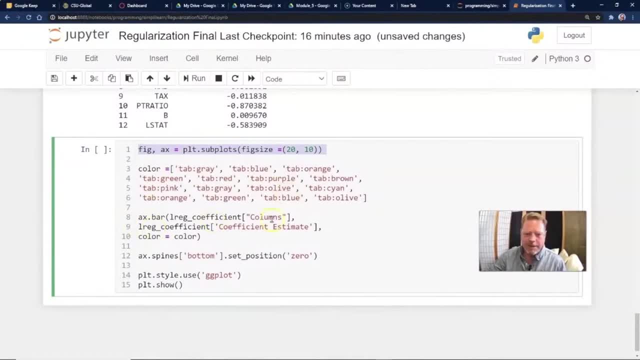 and again the team put together some nice colors so it makes it look good. We're doing an x-bar based on the columns and our L-regress coefficients. color equals color ax, spine bottom and so forth. It just puts together a nice little graph. 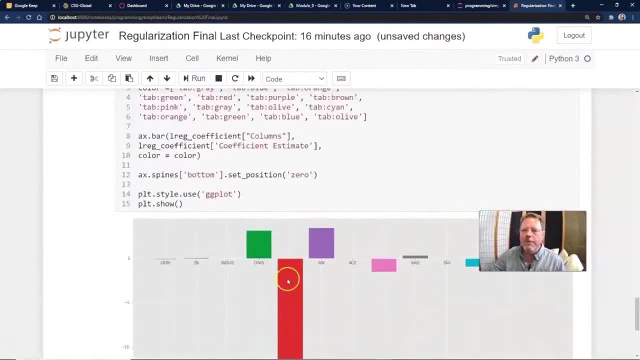 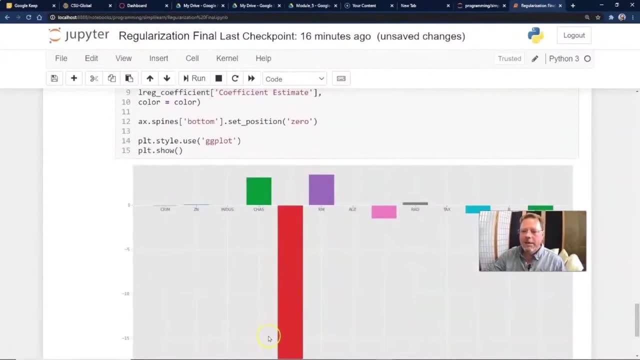 You're starting to see one when you compare this, if you put it on the same graph as this one up here, this is up here at minus 18.. This is at minus nine. This graph is half the size of the graph above. 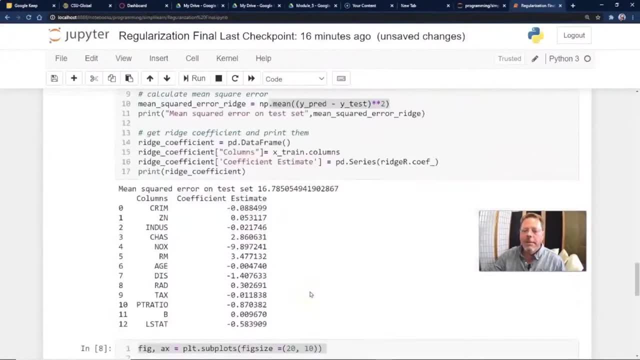 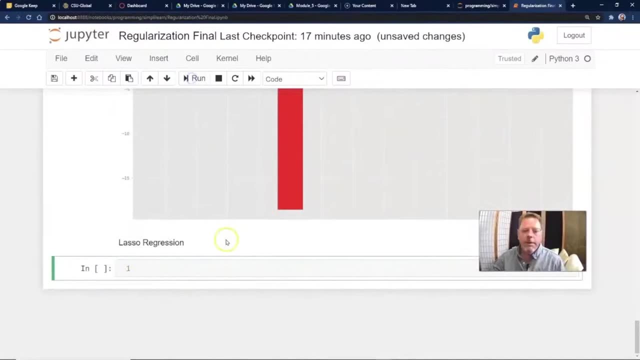 The same thing with these values here. They might look the same, but they're actually almost half the value on here. Then, finally, you can do the same thing for the lasso regression. This will all look very similar as far as what we worked on before. 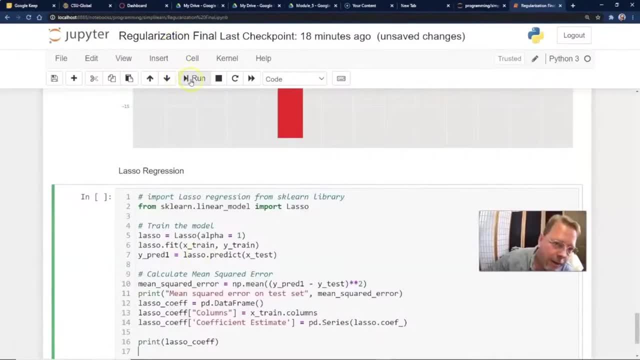 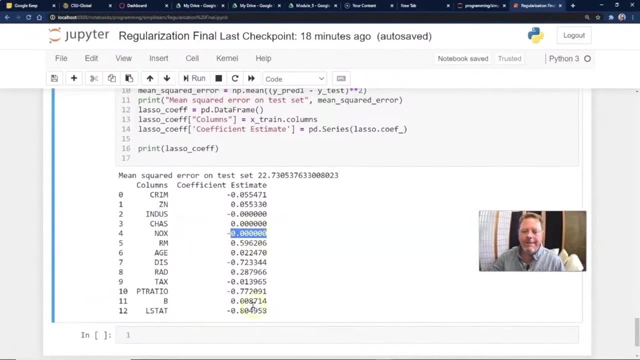 I'm just going to go ahead and print that on here and run it Again. let's go up to NOX. Look where NOX is. It's all the way down to zero. If we look at our next biggest coefficient, it's minus .8.. 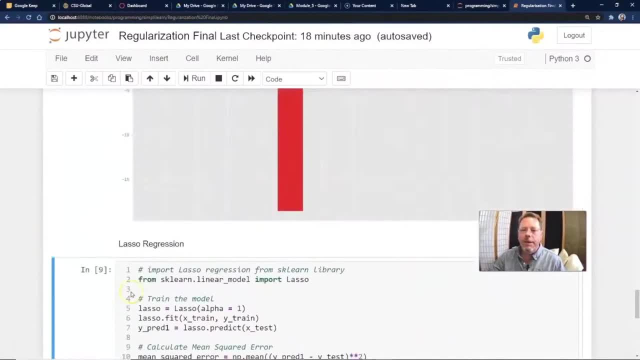 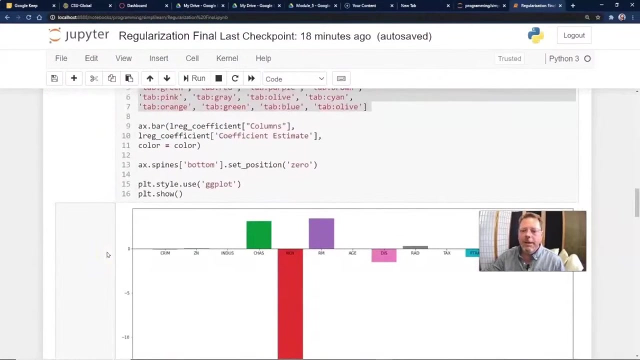 Really, here's our 22.73.. We go up here 16.7.. We go up here and we look at the same number, 16.69.. We look at this. If I was running this and working on a project with this, 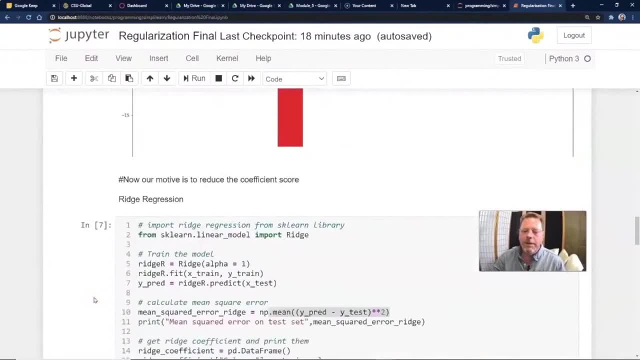 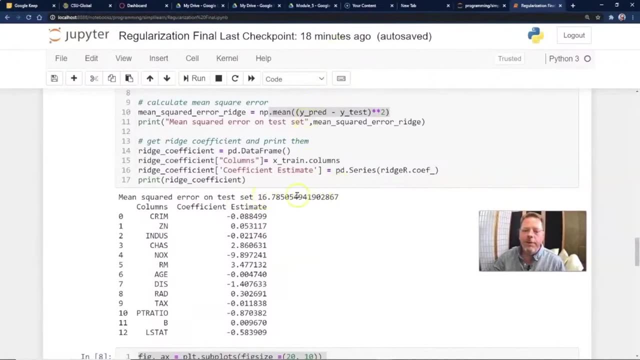 I would look at these numbers. I start with the 16.69, come down here and compare it to 16.78.. 69 is better than 78.. From the very beginning, we might start looking at this first model for overall predicting. 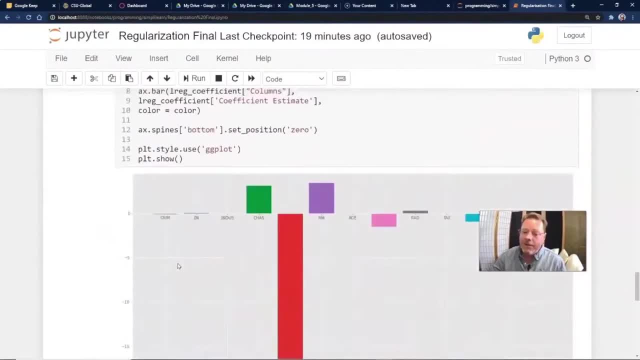 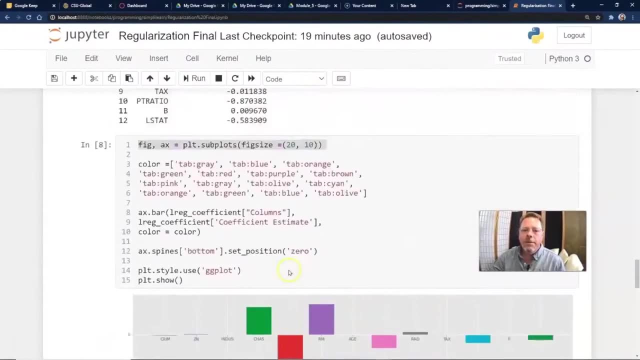 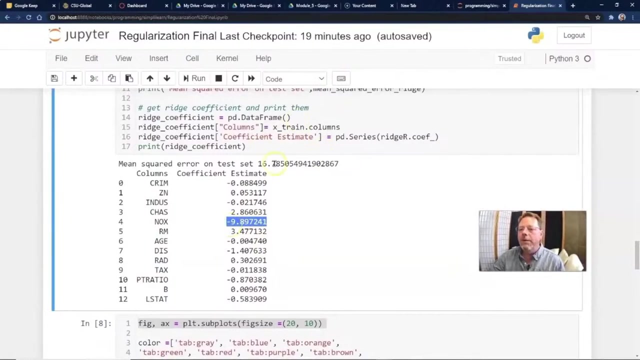 Now there's other factors involved. We might know that the NOX value is central and the other ones aren't quite as good. We might start looking at certain setups like: what is this particular coefficient? because it might have a certain meaning to us, and so forth. 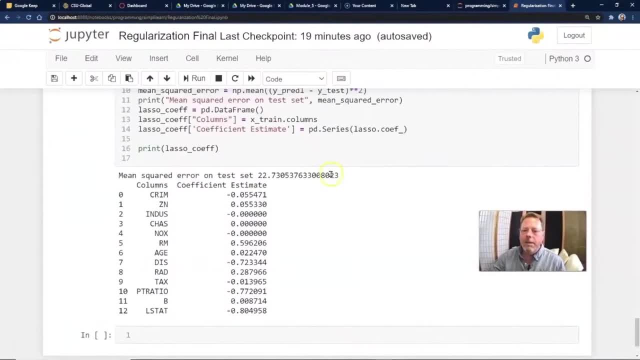 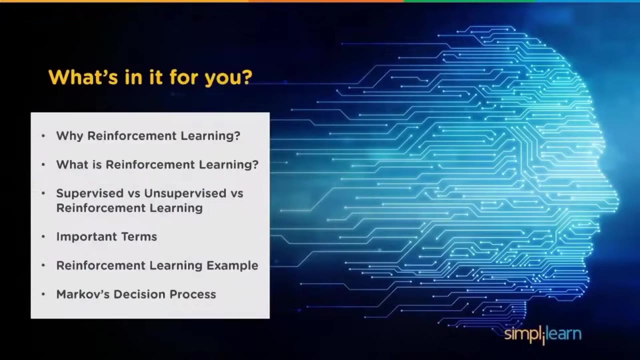 You've got to look at all those different items in there. The bottom dollar is. our first model did better than our other two models. Our mean square error on the test set can tell you that it continues to come down. on this, We're going to cover reinforcement learning today. 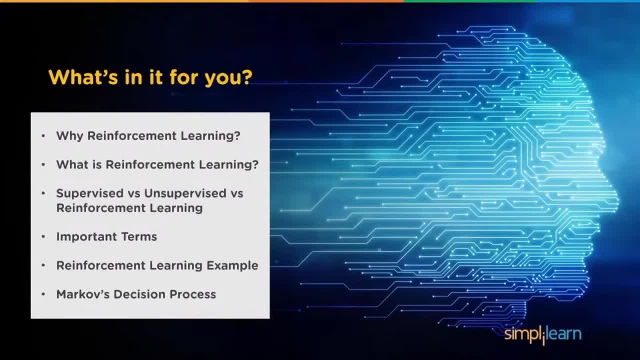 What's in it for you? We'll start with why reinforcement learning. We'll look at what is reinforcement learning. We'll see what the different kinds of learning strategies are that are being used today in computer models: under supervised versus unsupervised, versus reinforcement. 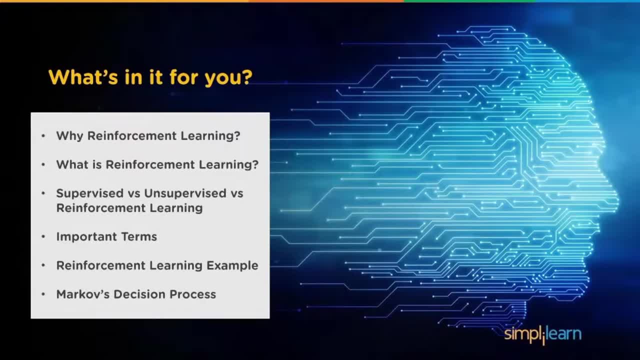 We'll cover important terms specific to reinforcement learning. We'll talk about Markov's decision process and we'll take a look at a simple example. We'll teach a tic-tac-toe how to play. Why reinforcement learning? Training, a machine learning model. 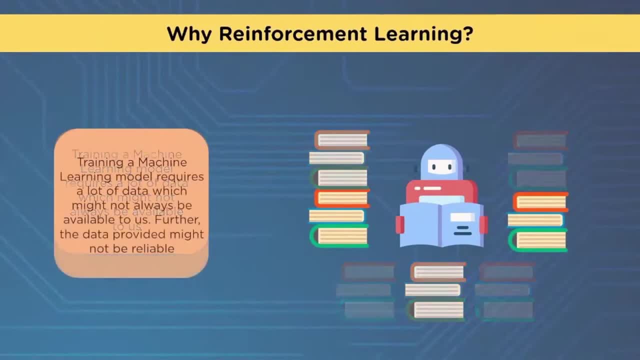 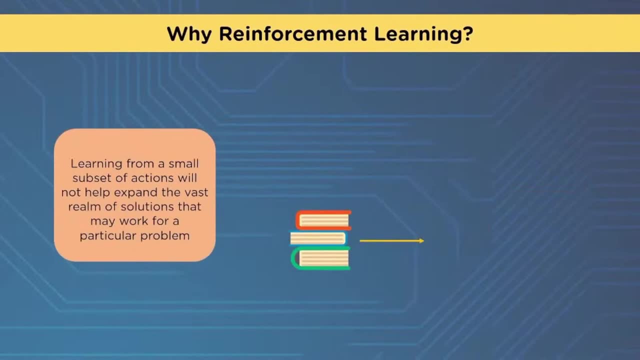 requires a lot of data, which might not always be available to us. Further, the data provided might not be reliable. Learning from a small subset of actions will not help expand the vast realm of solutions that may work for a particular problem. You can see, here we have the robot learning to walk. 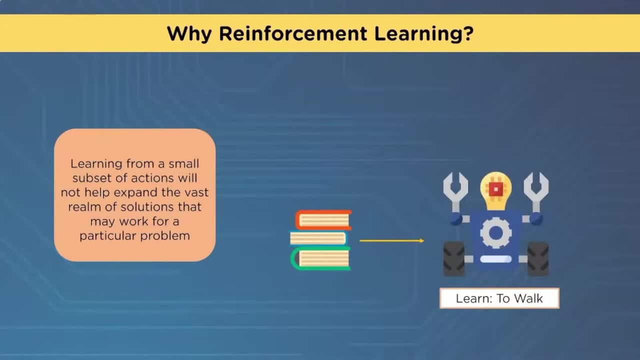 A very complicated setup when you're learning how to walk. If I'm taking one step forward and left, what happens if I pick up a 50 pound object? How does that change how a robot would walk? These things are very difficult to program because there's no 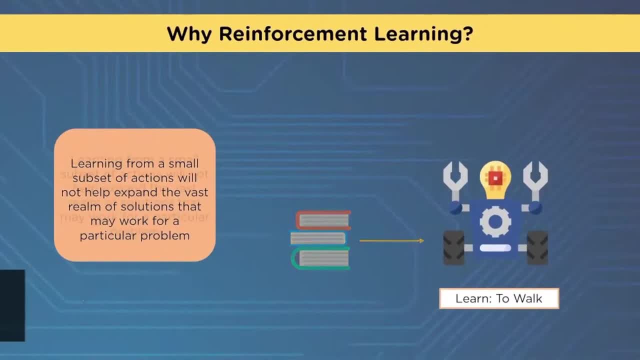 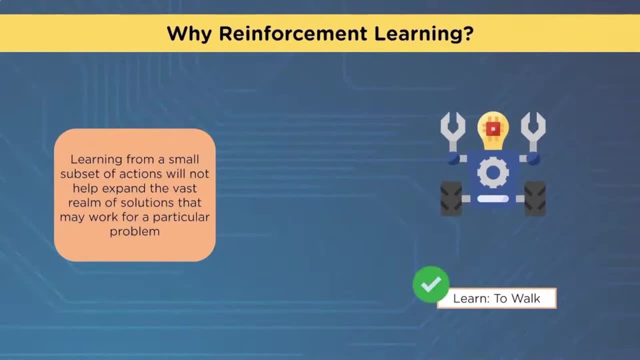 actual information on it until it's actually tried out. Learning from a small subset of actions will not help expand the vast realm of solutions that may work for a particular problem. We'll see here. it learned how to walk. This is going to slow the growth. 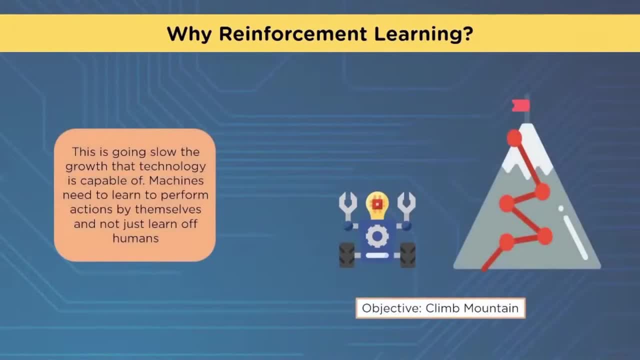 that technology is capable of. Machines need to learn how to perform actions by themselves and not just learn off humans. You see the objective climb a mountain. A real interesting point here is that as human beings we can go into a very unknown environment and we can adjust for it. 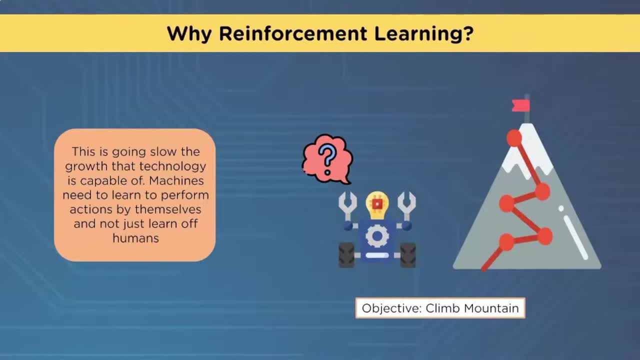 and kind of explore and play with it. Most of the models- the non-reinforcement models in computer machine learning aren't able to do that very well. There's a couple of them that can be used or integrated. See how it goes is what we're talking about with reinforcement learning. 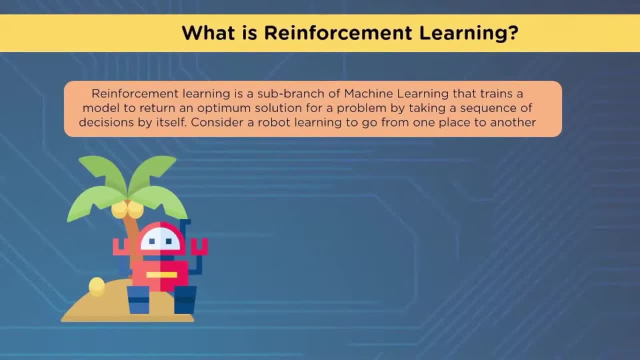 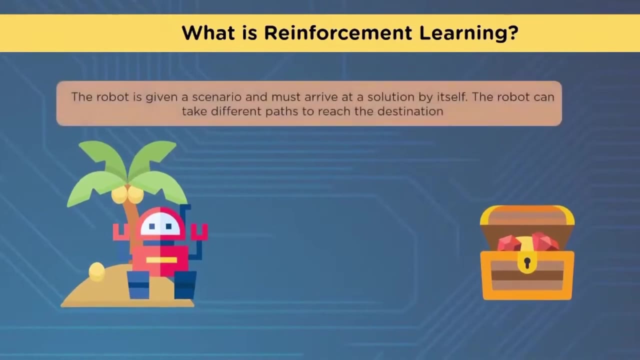 So what is reinforcement learning? Reinforcement learning is a sub-branch of machine learning that trains the model to return an optimum solution for a problem by taking a sequence of decisions by itself. Consider a robot learning to go from one place to another. The robot is given a scenario. 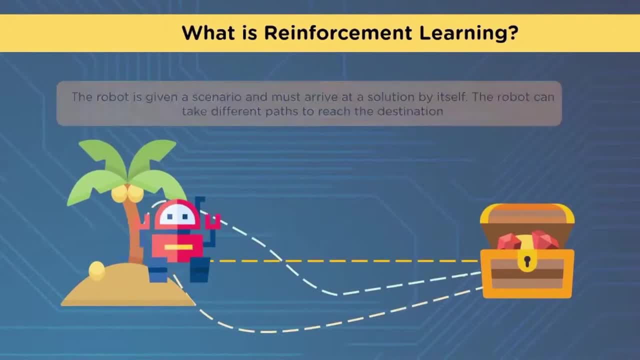 and must arrive at a solution by itself. It has to find a different path to reach the destination. It will know the best path by the time taken on each path. It might even come up with a unique solution all by itself, And that's really important. 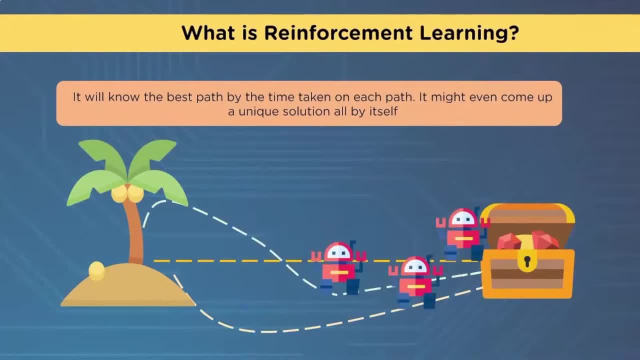 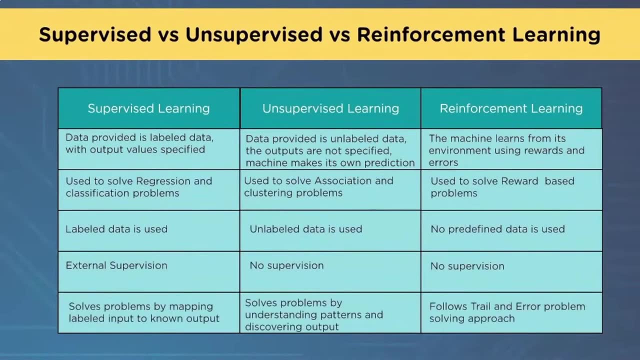 as we're looking for unique solutions. We want the best solution, but you can't find it unless you try it. So we're looking at our different systems, our different model. We have supervised versus unsupervised, versus reinforcement learning, And with the supervised learning, 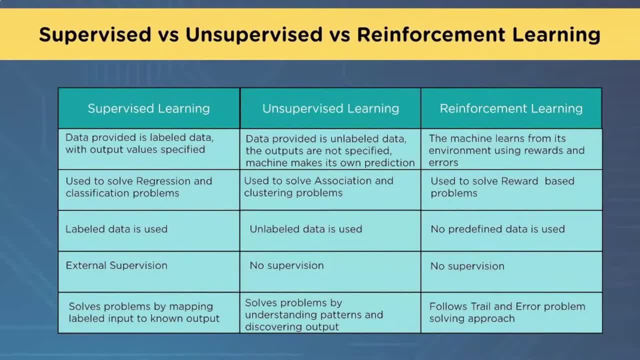 we have a controlled environment. We have a lot of different supervised learning models, whether it's linear regression, neural networks- there's all kinds of things in between decision trees. The data provided is labeled, data with output values specified, And this is important because 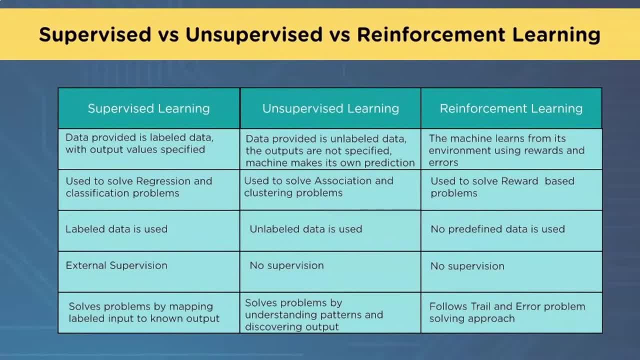 when we talk about supervised learning. you already know the answer for all this information. You already know the picture has a motorcycle in it. You can already have the graph of what the next day looks like, so you have an answer for it And you have labeled data, which is used. 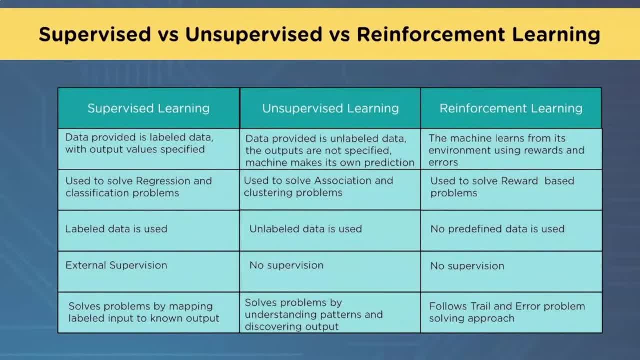 You have an external supervision and solves problems by mapping labeled input to known output. So very controlled Unsupervised learning is really interesting because it's now taking part in many other models. You can actually insert an unsupervised learning model in almost either supervised 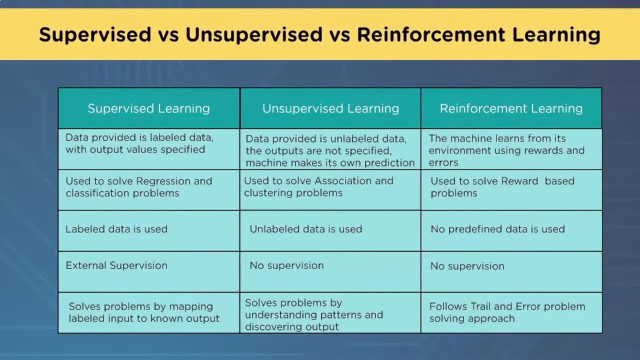 or stored reinforcement learning as part of the system, which is really cool. Data provided is unlabeled data. The outputs are not specified. Machine makes its own predictions Used to solve association with clustering problems. Unlabeled data is used. No supervision. 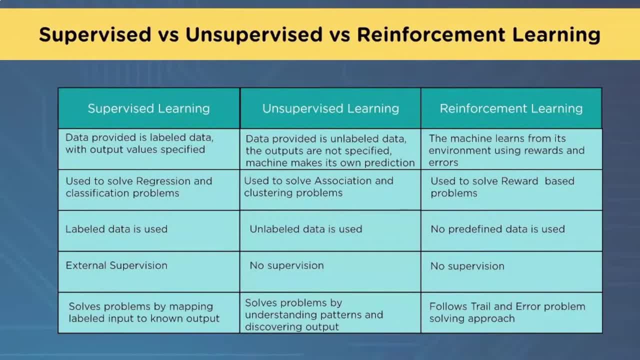 Solves problems by understanding patterns and discovering output. So you can look at this and you can think some of these things go with each other. It connects in different ways And there's a lot of different algorithms that look at this. When you start getting into those, 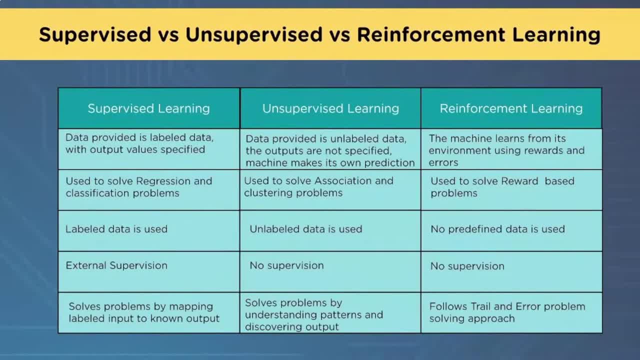 there's some really cool images that come up of what unsupervised learning is, How it can pick out, say, the area of a donut. One model will see the area of the donut and the other one will divide it into three sections based on its location. 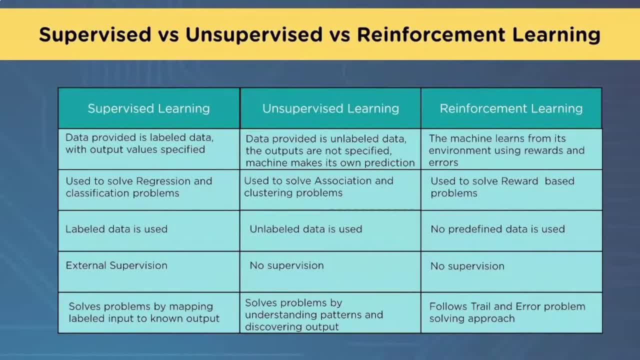 versus what's next to it. So there's a lot of stuff that goes in with unsupervised learning, And then we're looking at reinforcement learning, The machine learning or growing market. it's very infant stage as far as how it works and what it's going to be capable of. 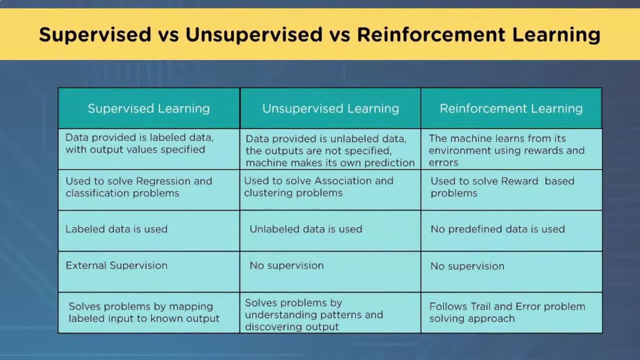 The machine learns from its environment using rewards and errors, Used to solve reward based problems. No predefined data is used, No supervision Follows trail and error problem solving approach. So again we have a random. at first, you start with a random, I try this. it works. 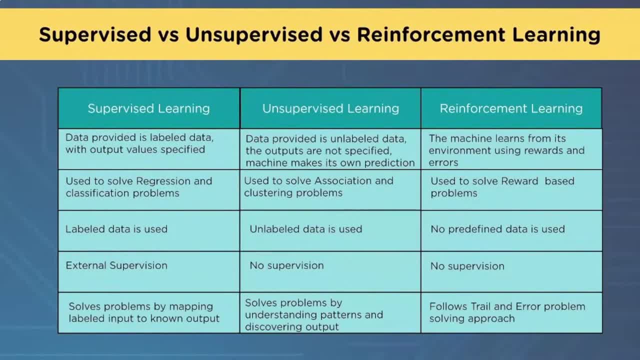 and this is my reward- Doesn't work very well, maybe Doesn't even get you where you're trying to get it to do, And you get your reward back. and then it looks at that and says: well, let's try something else, And it starts to play with these different things. 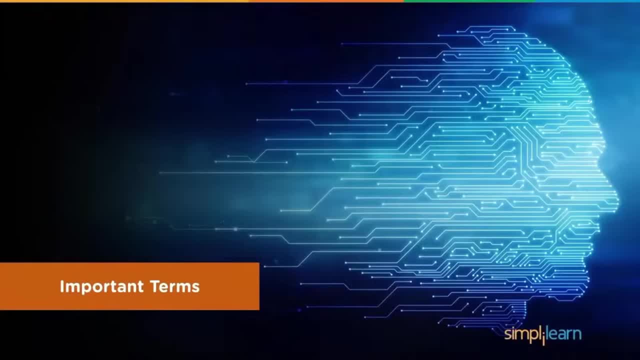 finding the best route. So let's take a look at important terms in today's reinforcement model- And this has become pretty standardized over the last few years, So these are really good to know. We have the agent. Agent is the model that is being trained. 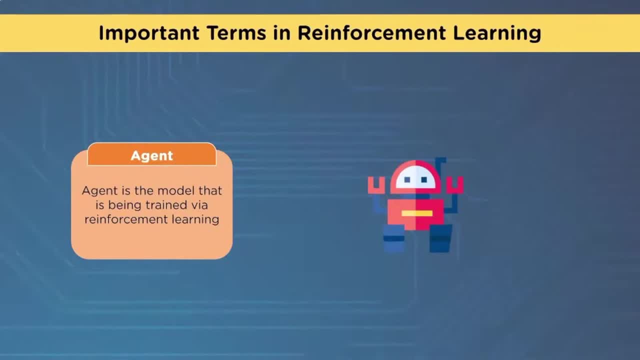 via reinforcement learning. So this is your actual entity, however you're doing it, Whether you're using a neural network or a cue table or whatever combination thereof, This is the actual agent that you're using. This is the model, And you have your environment. 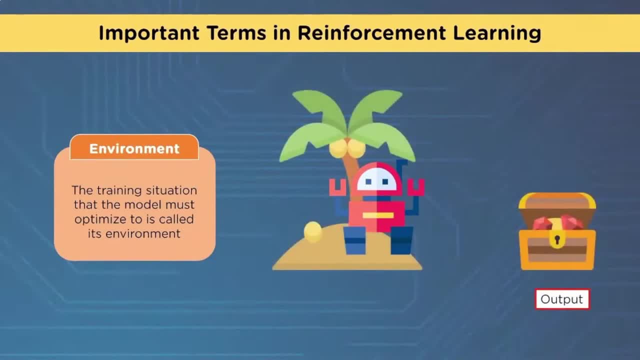 The training situation that the model must optimize to is called its environment, And you can see here, I guess we have a robot who's trying to get a chest full of gems or whatever, and that's the output, And then you have your action. 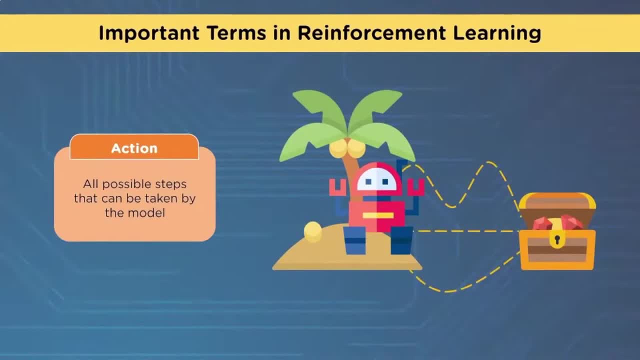 This is all possible steps that can be taken by the model and it picks one action. It picks three different routes to get to the chest of diamonds and gems. We have a state, The current position, condition returned by the model, And you could look at this. 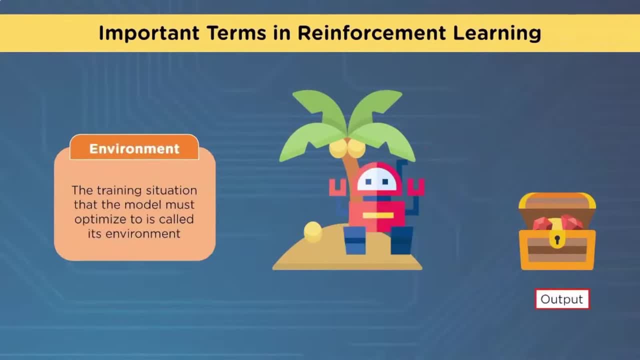 if you're playing like a video game, This is the screen you're looking at. So when you go back here, the environment is a whole game board. So if you're playing one of those Mobius games, you might have the whole game board going on. 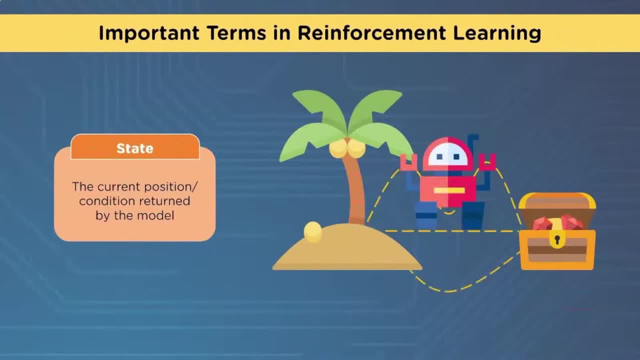 But then you have your current position. What's around that game board? What's around you? If you were talking about a robot, the environment might be moving around the yard, where it is in the yard and what it can see, What input it has in that location. 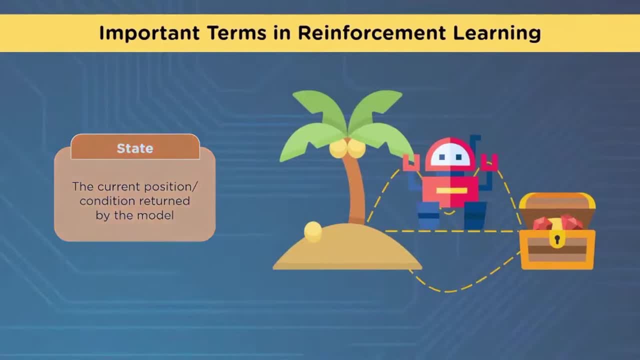 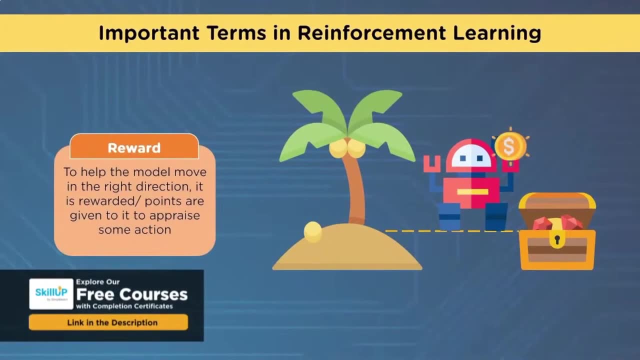 That would be the current position condition returned by the model. And then the reward: To help the model move in the right direction, it is rewarded. Points are given to it to appraise some kind of action. So, yeah, you did good Trying to maximize the reward. 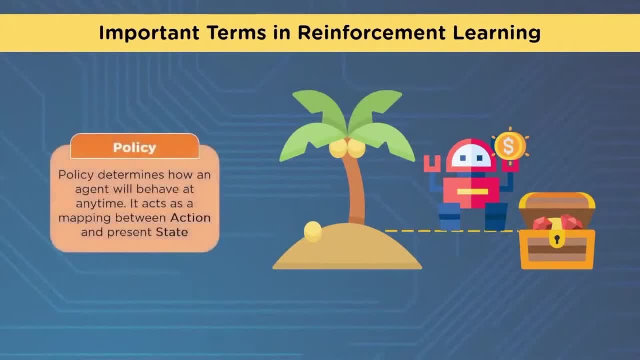 and have the best reward possible. And then policy. Policy determines how an agent will behave at any time. It acts as a mapping between action and present state. This is part of the model. What is your action that you're going to take? 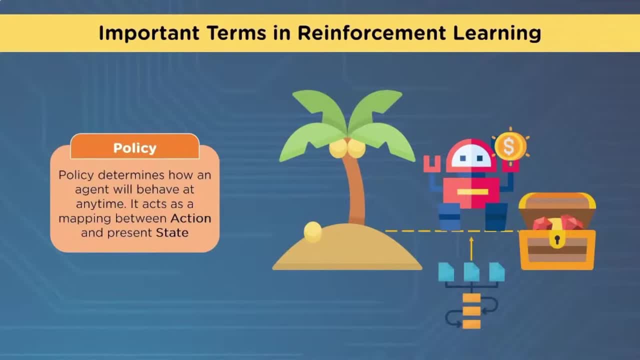 What's the policy you're using to have an output from your agent? One of the reasons they separate policy as its own entity is that you usually have a prediction of different options And then the policy. well, how am I going to pick the best based on those predictions? 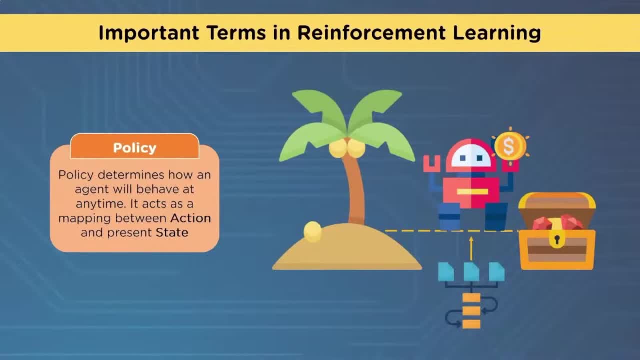 I'm going to guess at different options And we'll actually weigh those options in and find the best option we think will work. So it's a little tricky, but the policy thing is actually pretty cool how it works. Let's go ahead and take a look at a reinforcement learning example. 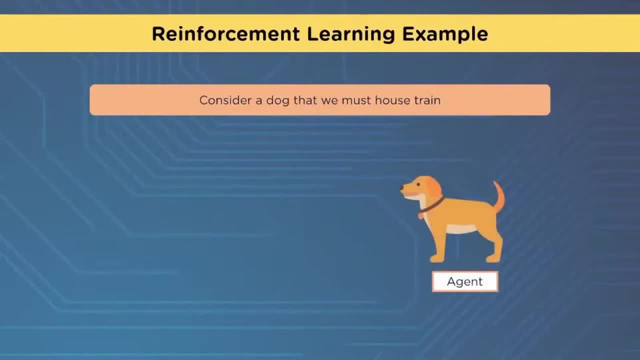 And just in looking at this, we're going to take a look, consider what a dog that we want to train. So the dog would be like the agent. so you have your puppy or whatever, and then your environment is going to be the whole house or whatever it is where you're training them. 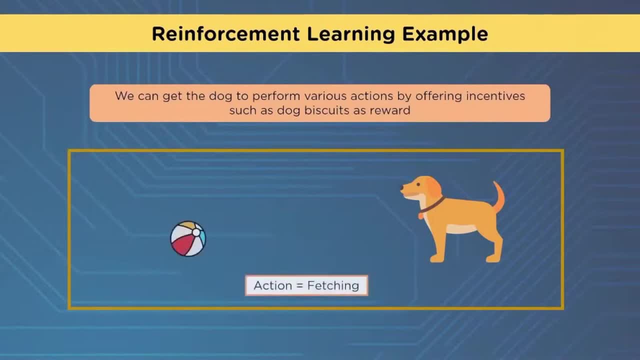 And then you have an action. we want to teach the dog to fetch, So action equals fetching. and then we have a little biscuit so we can get the dog to perform various actions by offering incentives such as a dog biscuit as a reward. The dog will follow a policy. 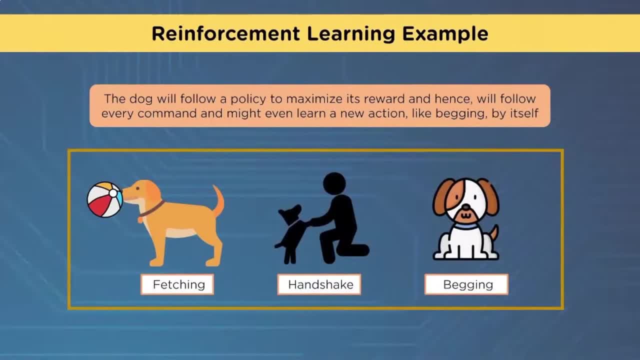 to maximize this reward and hence will follow every command and learn new actions, like begging, by itself. So we start off with fetching. it goes: oh, I get a biscuit for that. it tries something else. you get a handshake or begging or something like that, and it goes: oh, this is also reward based. 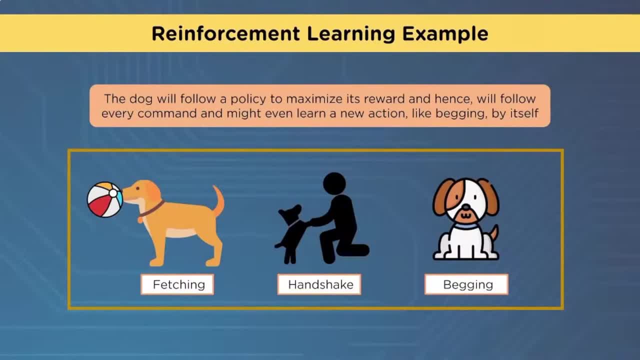 and so it kind of explores things to find out what will bring it its biscuit. And that's very much like how a reinforced model goes, is it looks for different rewards. how can I try different things and find a reward that works? The dog also will want to run around. 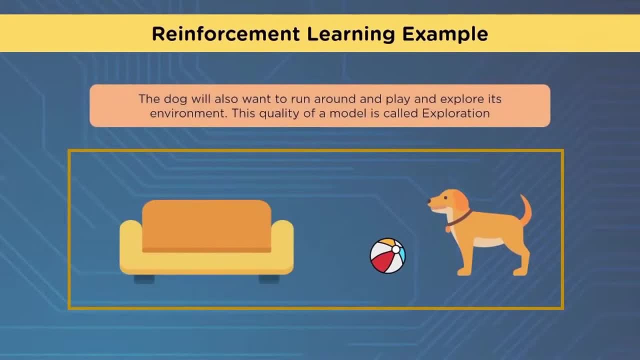 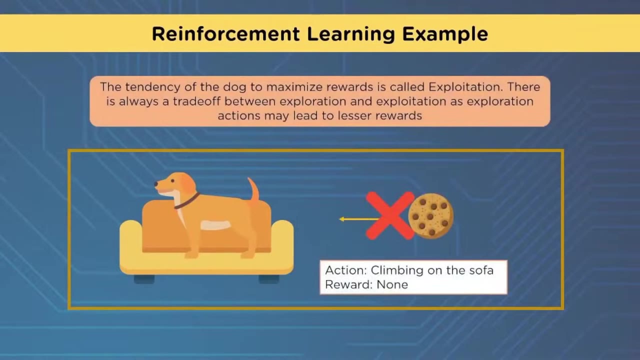 and play and explore its environment. this quality of model is called exploration, So there's a little randomness going on in exploration. It explores new parts of the house. climbing on the sofa doesn't get a reward. In fact, it usually gets kicked off the sofa. 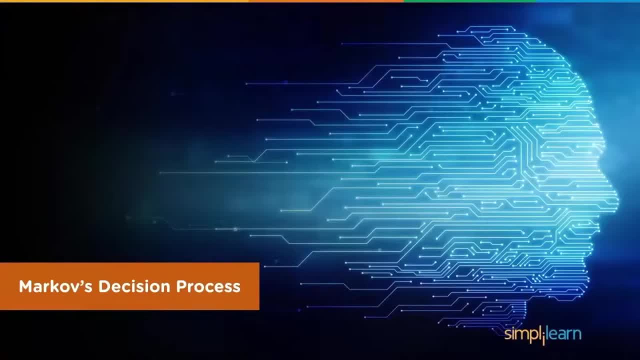 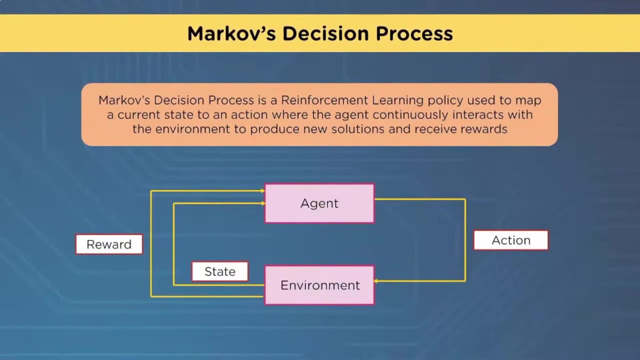 So let's talk a little bit about Markov's decision process. Markov's decision process is a reinforcement learning policy used to map a current state to an action, and the agent continuously interacts with the environment to produce new solutions and receive rewards. And you'll see, here's all of our different. 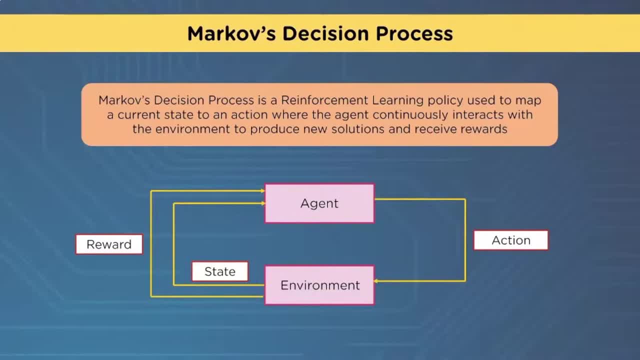 vocabulary we just went over. we have a reward: our state, our agent, our environment and our action. And so, even though the environment kind of contains everything, you really, when you're actually writing the program, your environment is going to put out a reward and state. 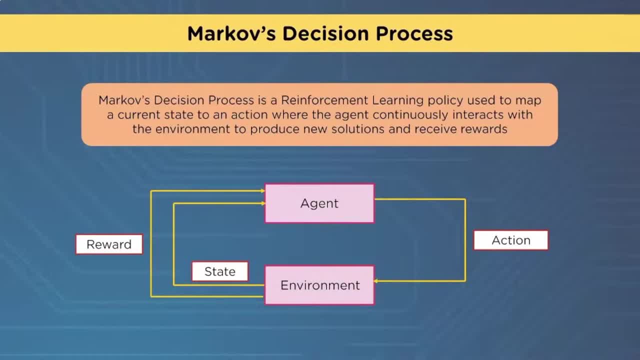 that goes into the agent. the agent then looks at this state or it looks at the reward usually first, and it says, okay, I got rewarded for whatever I just did, or I didn't get rewarded. and then it looks at the state and then it comes back and, if you remember, 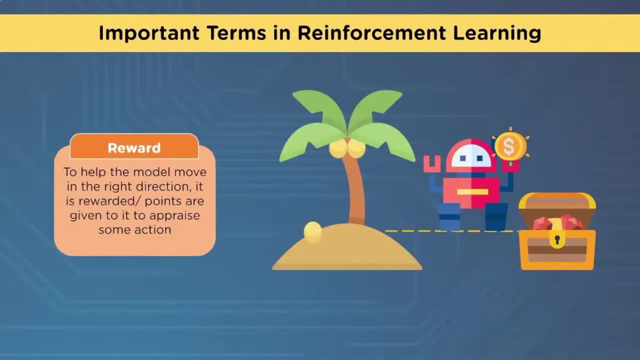 from policy. the policy comes in and then we have a reward. The policy is that part that's connected at the bottom, and so it looks at that policy and it says, hey, what's a good action? that will probably be similar to what I did, or sometimes they're completely. 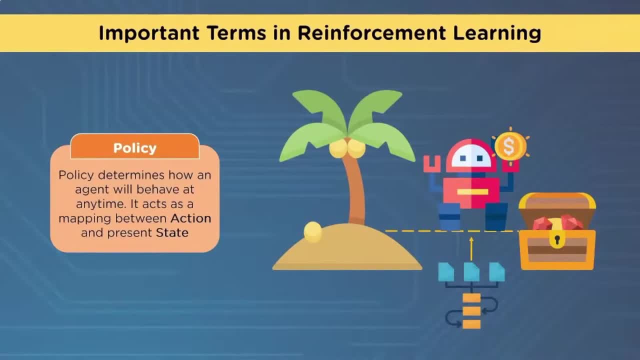 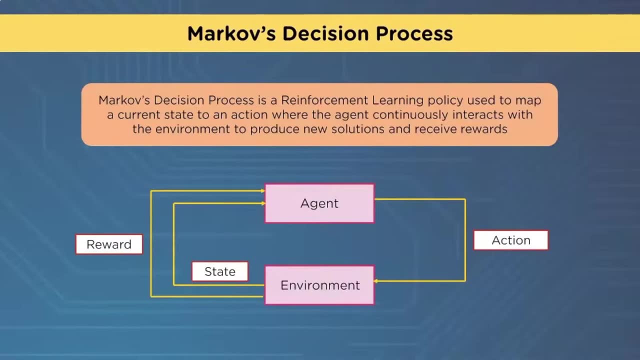 random, but what's a good action that's going to bring me a different reward. So taking the time to just understand these different pieces as they go is pretty important in most of the models today, and so a lot of them actually have templates based on this that you can. 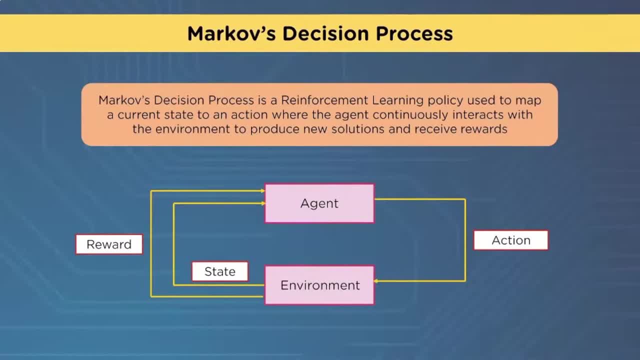 pull in and start using pretty straight forward as far as once you start seeing how it works, you can see. your environment says: hey, the agent did this. if you're a character in a game, this happened and it shoots out a reward in a state. the agent looks at the reward. 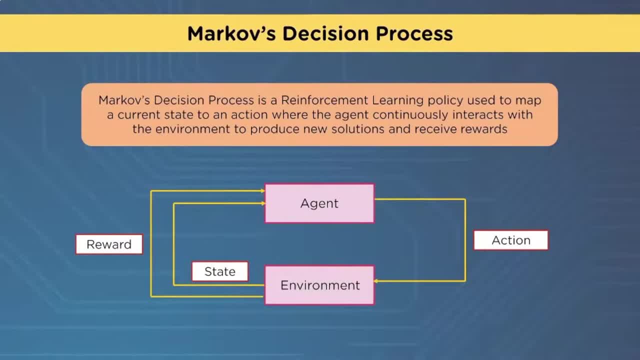 looks at the new state and then takes a little guess and says I'm going to try this action. and then that action goes back into the environment. it affects the environment. the environment then changes depending on what the action was, and then it has a new state and a new reward that goes back to the agent. 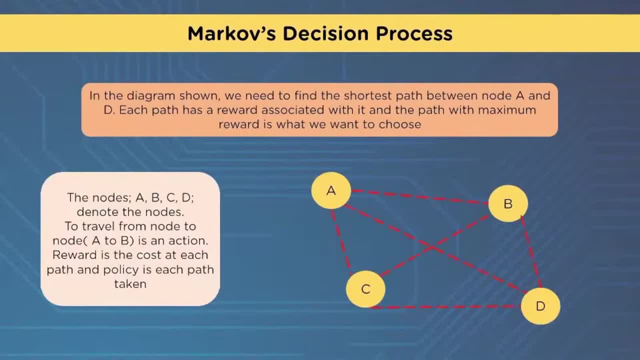 So in the diagram shown, we need to find the shortest path between node A and D. each path has a reward associated with it, and the path with the maximum reward is what we want to choose. the nodes A, B, C, D denote the nodes that travel from node 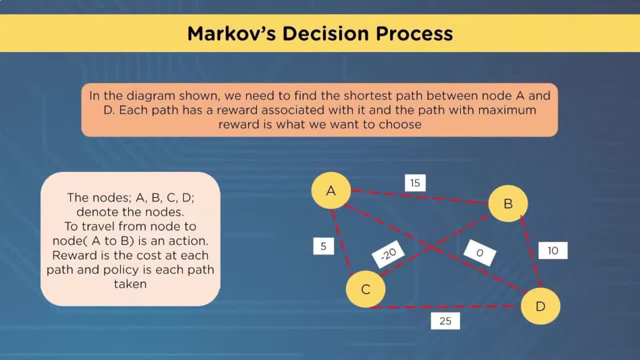 A to B is an action, Reward is the cost of each path and policy is each path taken. and you can see here A can go to B or A can go to C right off the bat, or it can go right to D. and if you explored 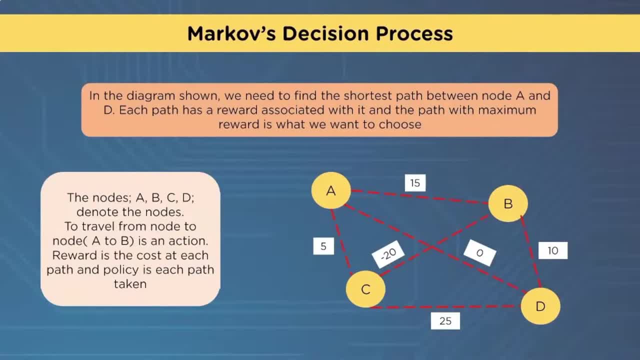 all three of these, you would find that A going to D was a zero reward, A going to C and D would generate a different reward, or you could go A, C, B, D. there's a lot of options here, and so when we start looking at this diagram, 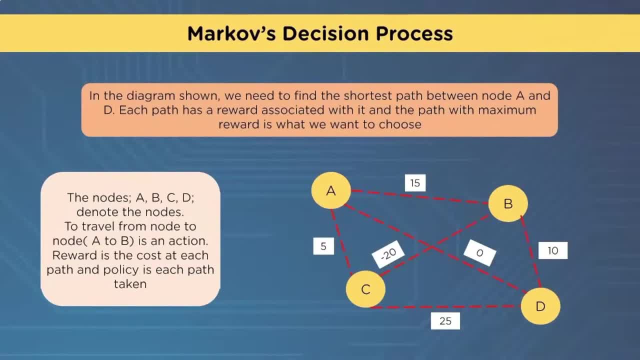 you start to realize that even though today's reinforced learning models do really good at finding an answer, they end up trying almost all the different directions, you see, and so they take up a lot of work or a lot of processing time for reinforcement learning. they're right now in their infant stage. 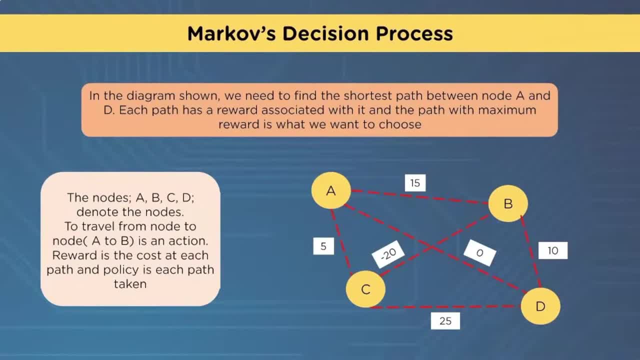 they're really good at solving simple problems and we'll take a look at one of those in just a minute in a tic-tac-toe game. but you can see here, once it's gone through these and it's explored, it's going to find the A, C, D. 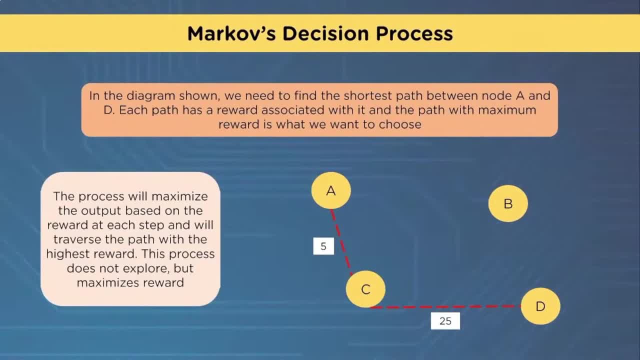 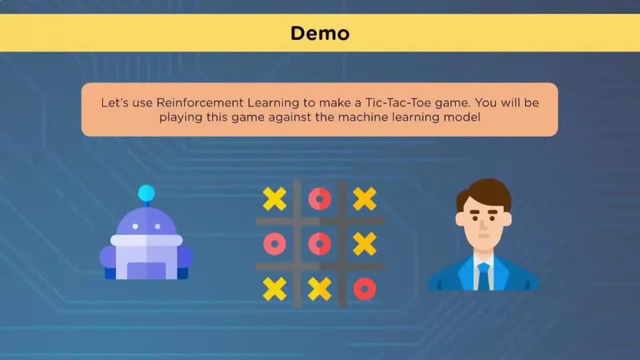 is the best reward. it gets a full 30 points for it. so let's go ahead and take a look at a reinforcement learning demo. in this demo, we're going to use reinforcement learning to make a tic-tac-toe game. you'll be playing this game against the machine learning. 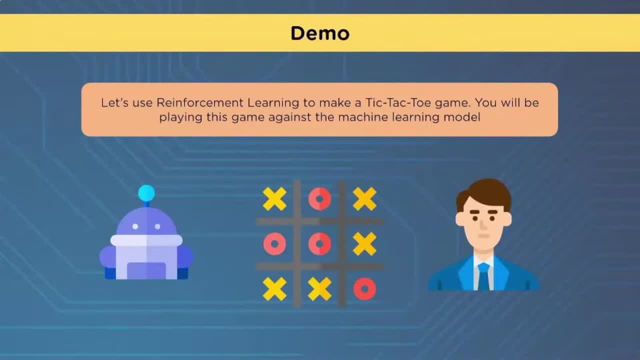 model and we'll go ahead, and we're doing it in Python. so let's go ahead and go through my always- not always- I actually have a lot of Python tools. let's go through Anaconda, which will open up a Jupyter notebook. seems like a lot of steps, but it's worth it. 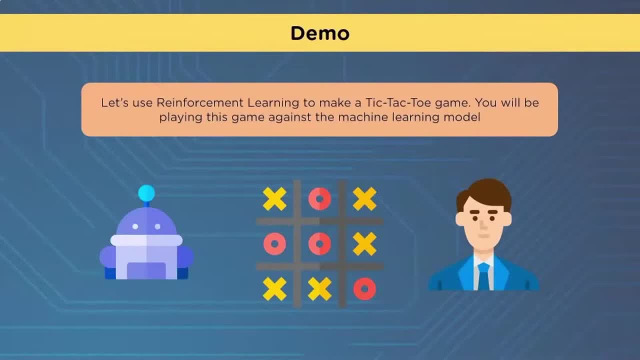 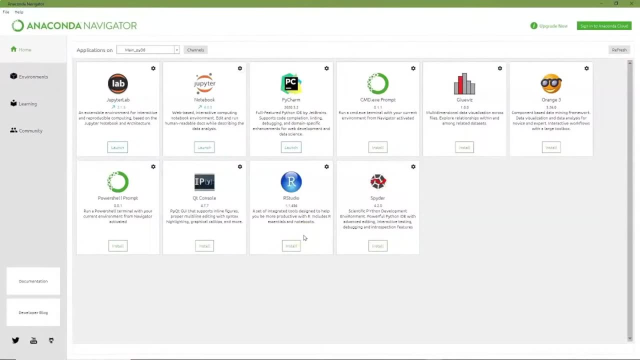 to keep all my stuff separate, and it also has a nice display when you're in the Jupyter notebook for doing Python. so here's our Anaconda Navigator. I open up the notebook, which is going to take me to a web page, and I've gone in here and created a. 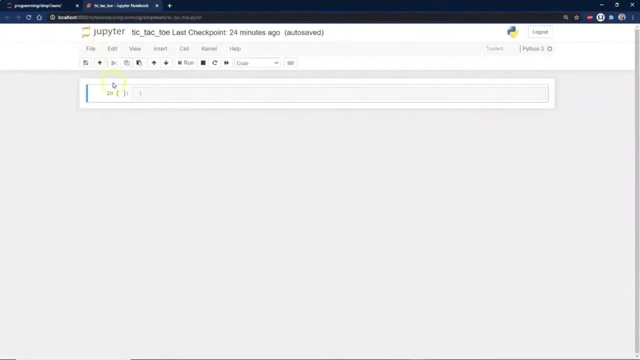 new Python folder. in this case I've already done it and enabled it to change the name to tic-tac-toe. and then, for this example, we're going to go ahead and import a couple things. we're going to import numpy as in p. we'll go ahead and import pickle. 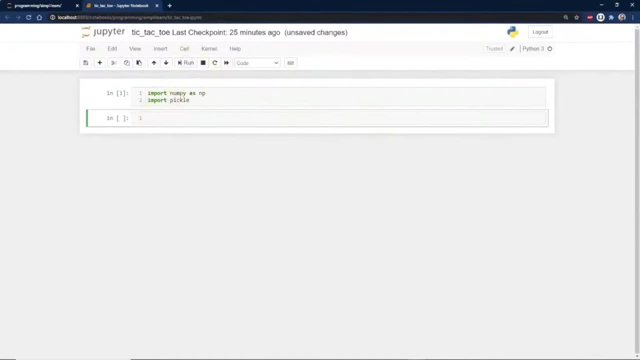 numpy, of course, is our number array, and then pickle is just a nice way sometimes for storing different information, different states that we're going to go through on here, and so we're going to create a class called state. we're going to start with that. 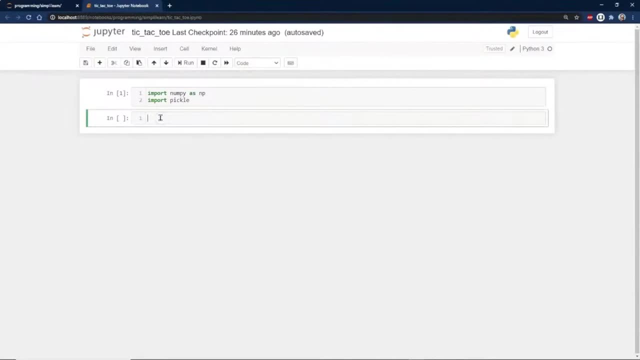 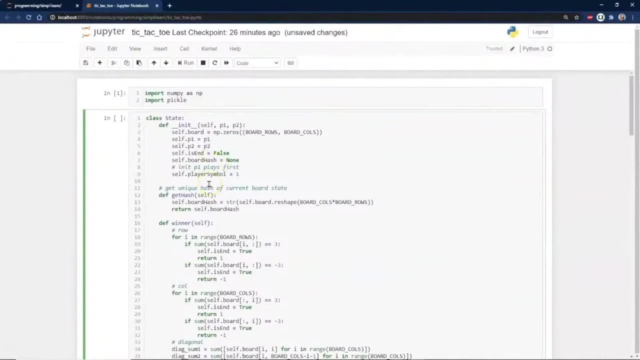 and there's a lot of lines of code to this class that we're going to put in here. don't let that scare you too much. there's not as much here. it looks like there's going to be a lot here, but there really is just a lot of setup. 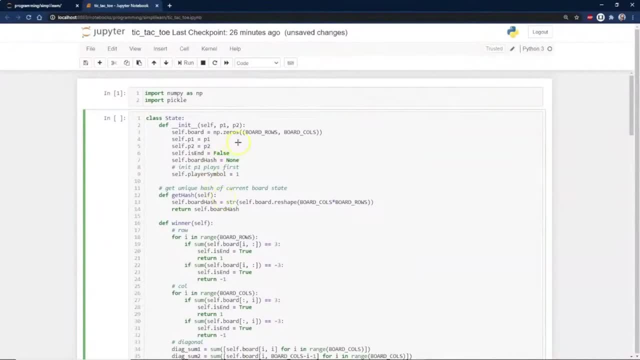 going on in our class state and so we have up here. we're going to initialize it. we have our board. it's a tic-tac-toe board, so we're only dealing with nine spots on the board. player one, player two is end. we're going to create a board hash. 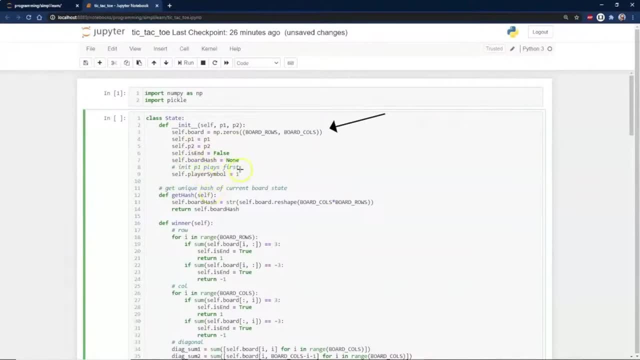 we'll look at that in just a minute. we're just going to store some information in there. symbol of player equals one, so there's a few things going on. as far as the initialization, then something simple. we're just going to get the hash of the board. 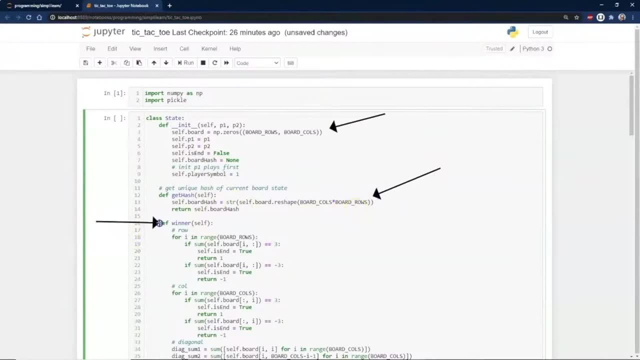 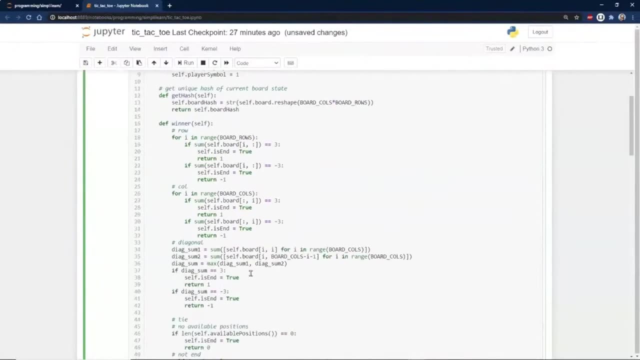 we're going to get the information from the board on there, which is columns and rows. we want to know when a winner occurs, so if you get three in a row, let me go ahead and scroll up a little bit. you can get a copy of this code. 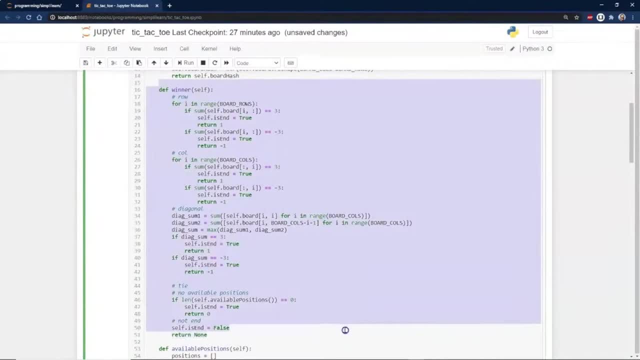 if you send a note over to simplylearn, we'll send you over this particular file and you can play with it yourself and see how it's put together. I don't want to spend a huge amount of time on this, because this is just some real general. 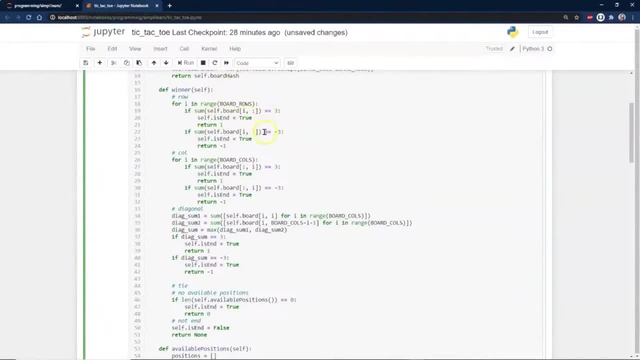 Python coding. but you can see, here we're just going through all the rows and you add them together and if it equals three, three in a row, it's just columns diagonal. so you've got to check the diagonal. that's what all this stuff does here. 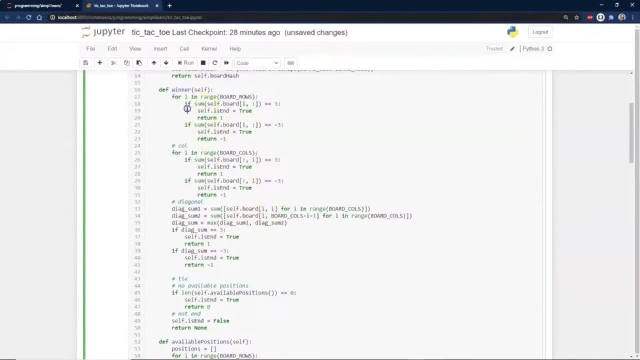 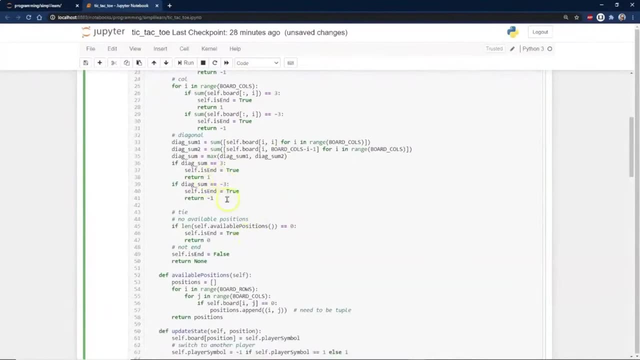 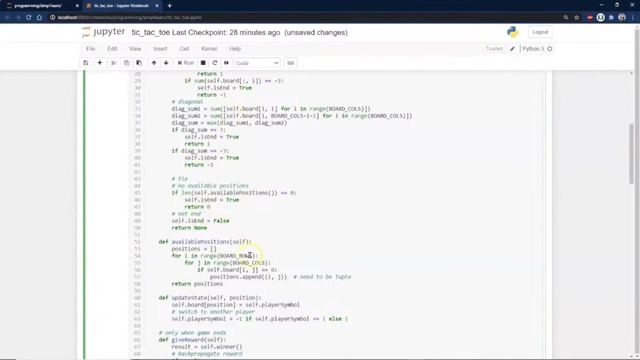 it just goes through the different areas. actually, let me go ahead and put there we go, and then it comes down here and we do our sum and it says true minus three. it just says did somebody win or is it a tie? so you've got to add up all the numbers on there anyway. 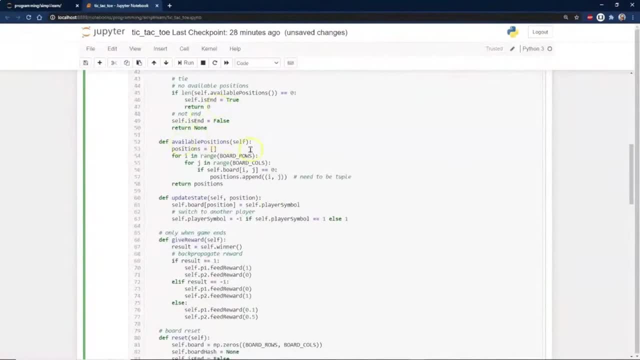 just in case they're all filled up. and next we also need to know available positions. no one's ever used before this way: when you try something or the computer tries something, it's not going to give it an illegal move. that's what the available positions is doing. 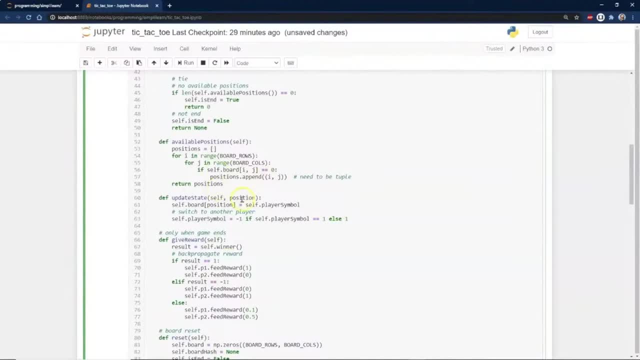 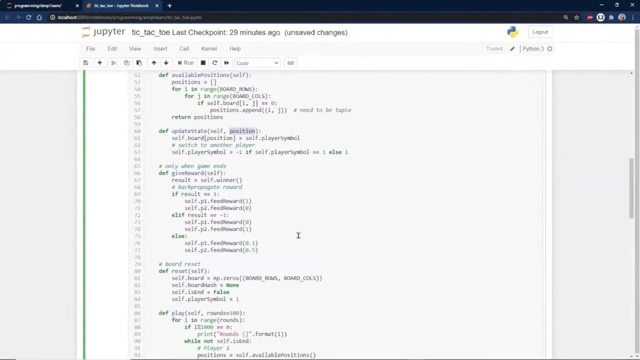 then we want to update our state. so you have your position going in. we're just sending in the position that you just chose and you'll see there's a little user interface we put in there, pick the row and column in there and again, this is a lot of code. 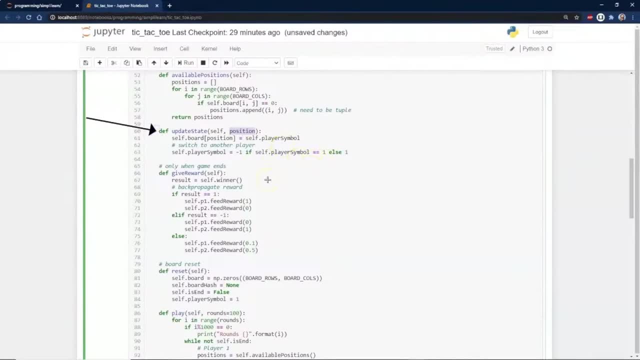 so really it's kind of a thing you'd want to go through and play with a little bit and just read through it, get a copy of it- a great way to understand how this works. and here is a given reward. so we're going to give a reward. 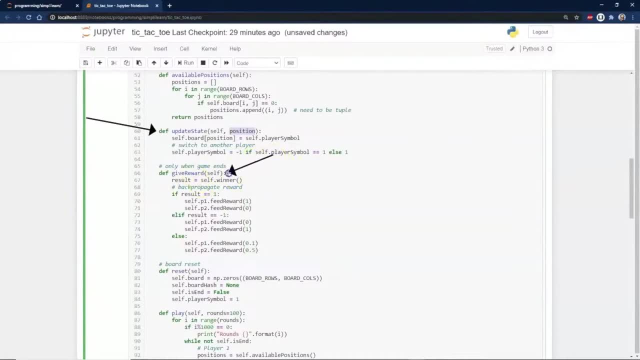 result equals self winner. this is one of the hearts of what's going on here is we have a result selfwinner. so if there's a winner, then we have a result. if the result equals one, here's our feedback: it gets a zero, so it only gets a reward. 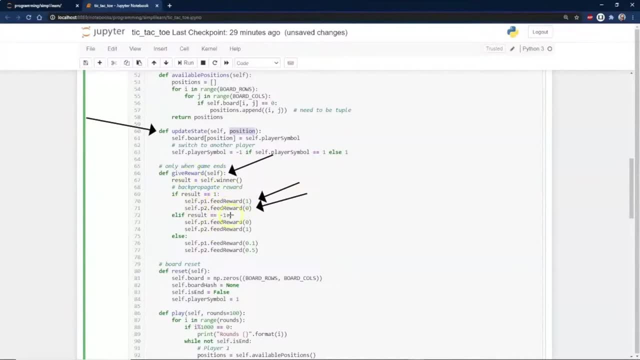 in this particular case, if it wins- and that's important to know, because different systems of reinforced learning do rewarding a lot differently depending on what you're trying to do. this is a very simple example with a 3x3 board, imagine if you're playing a video game. 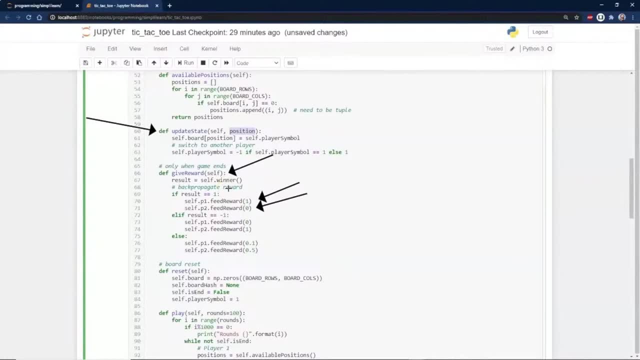 certainly you only have so many actions, but your environment is huge. you have a lot going on in the environment and suddenly a reward system like this is going to be just. it's going to have to change a little bit. it's going to have to have different rewards. 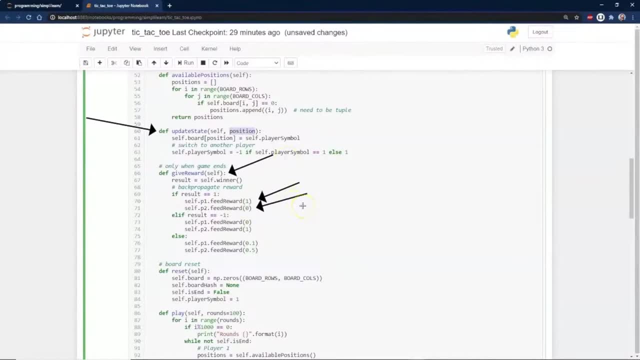 and different setup, and there's all kinds of advanced ways to do that. as far as weighing, you add weights to it, and so they can add the weights up, depending on where the reward comes in. so it might be that you actually get a reward. in this case, you get the reward. 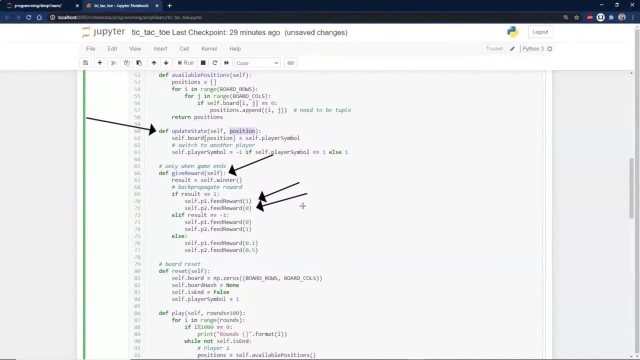 at the end of the game. I'm spending just a little bit of time on this because this is an important thing to note. except those rewards it might have, like if you take a certain path, the first reward is going to be weighed a little bit less than the last reward. 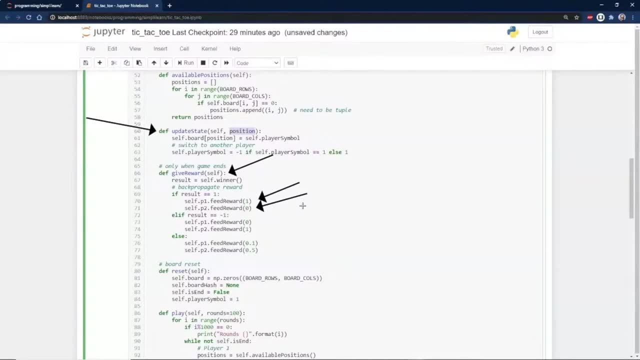 because the last reward is actually winning the game, or scoring, or whatever it is, so this reward system gets really complicated in some of the more advanced setups. in this case, though, you can see right here that they give a .1 and a .5 reward just for getting. 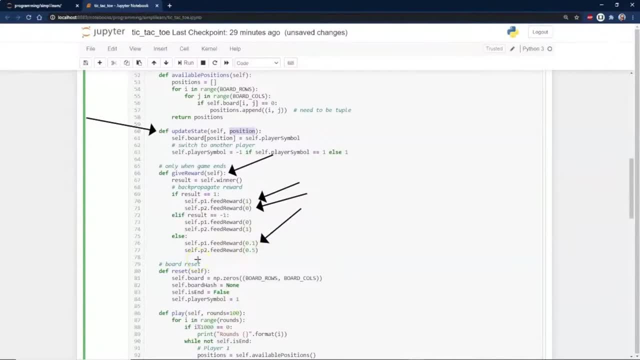 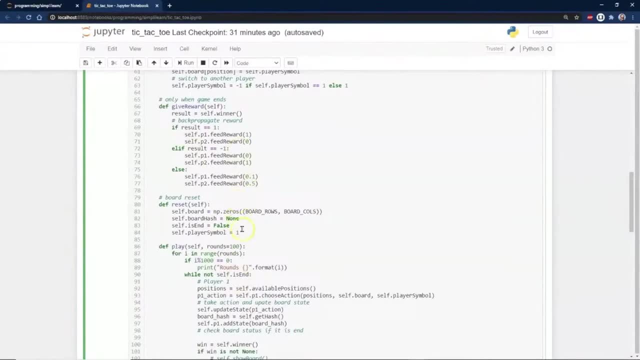 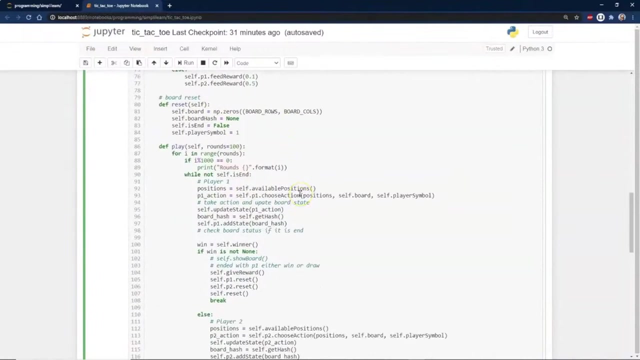 picking the right value and something that's actually valid, instead of picking an invalid value. so rewards again, that's like key, it's huge. how do you feed the rewards back in? then we have a board reset. that's pretty straight forward. it just goes back and resets the board to the beginning. 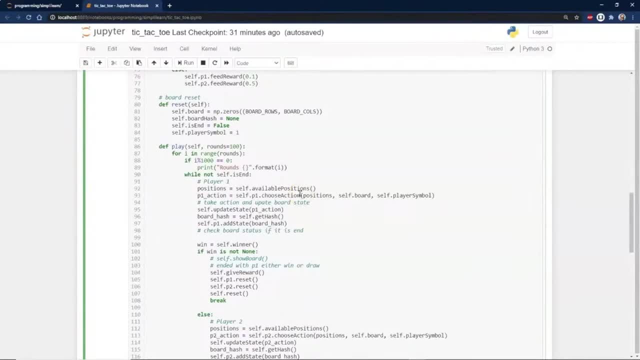 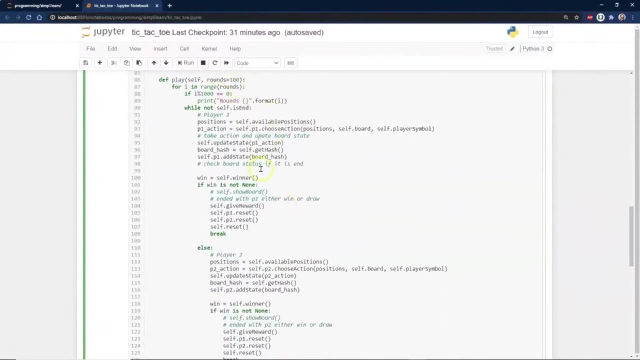 because it's going to try out all these different things while it's learning. it's going to do it by trial and error, so you have to keep resetting it. and then, of course, there's the play. we want to go ahead and play. rounds equals 100. 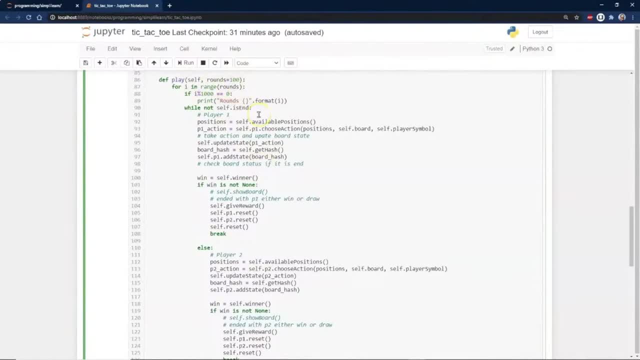 and set this different, obviously set that to higher level. but this is just going to go through and you'll see in here that we have player one and player two. this is the computer playing itself, one of the more powerful ways to learn: to play a game or even learn something that isn't a game. 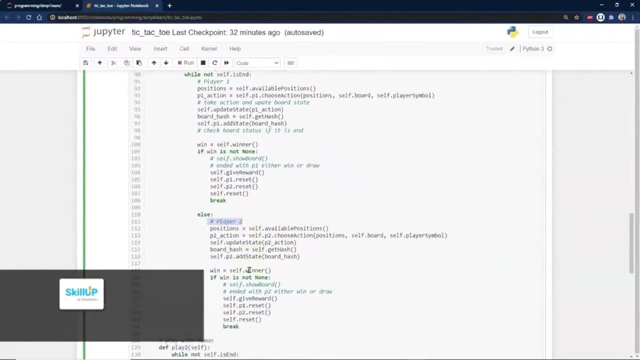 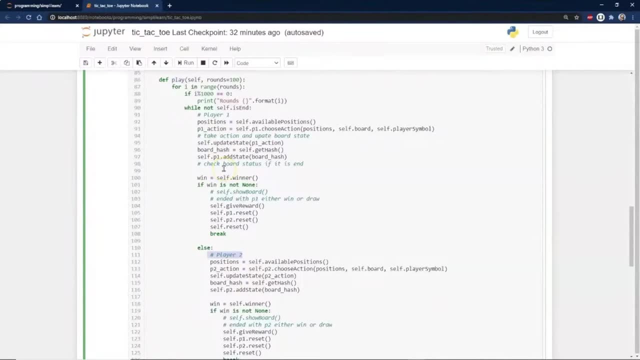 is to have two of these models that are basically trying to beat each other and so they keep finding, explore new things. this one works for this one, so this one tries new things, it beats this. we've seen this in chess. I think was a big one where they had the two players in chess. 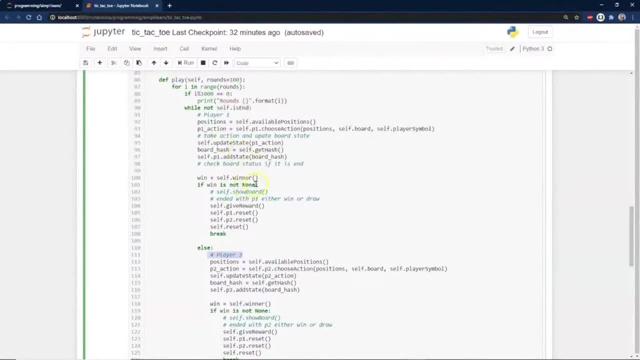 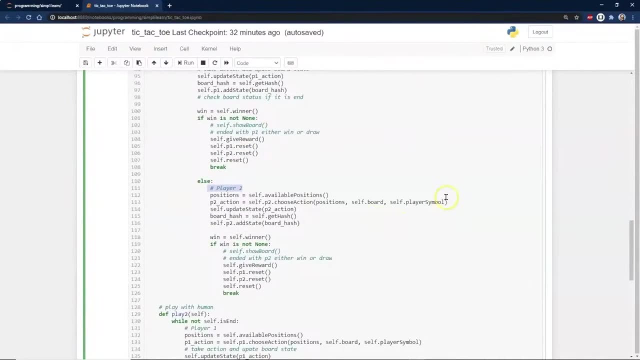 with reinforcement learning. it was one of the ways they trained one of the top computer chess playing algorithms. so this is just what this is: it's going to choose an action, it's going to try something, and the more it tries stuff, the more we're going to record the hash. 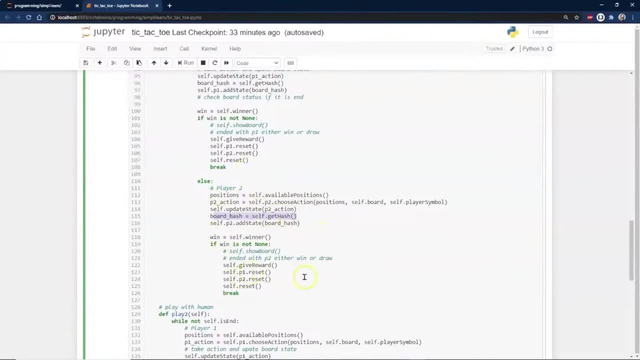 we actually have a board hash where you can get the hash set up on here and then once you get to a win- one of them wins, it gets the reward. then we go back and reset and try again and then kind of the fun part we actually get down here is: 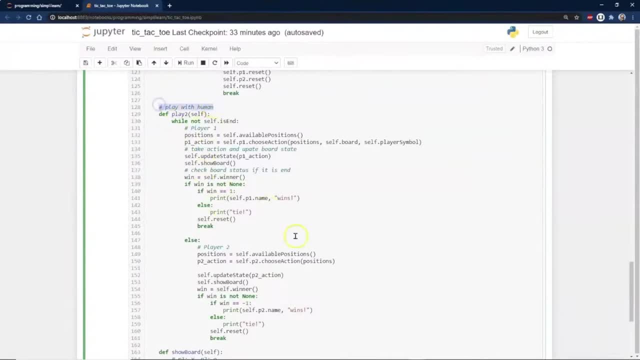 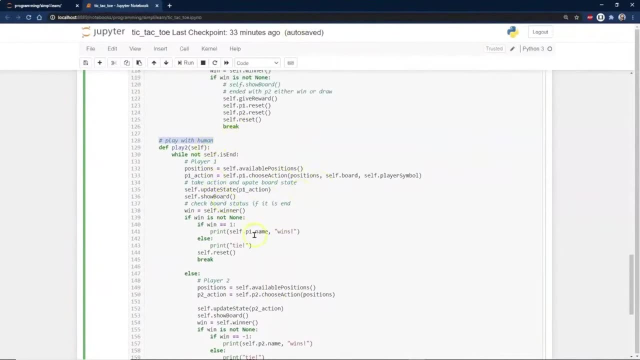 we're going to play with a human, so we'll get a chance to come in here and see what that looks like when you put your own information in, and then it just comes in here and does the same thing it did above. it gives it a reward for its things. 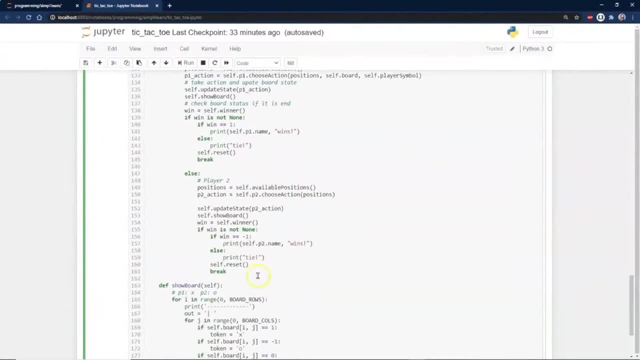 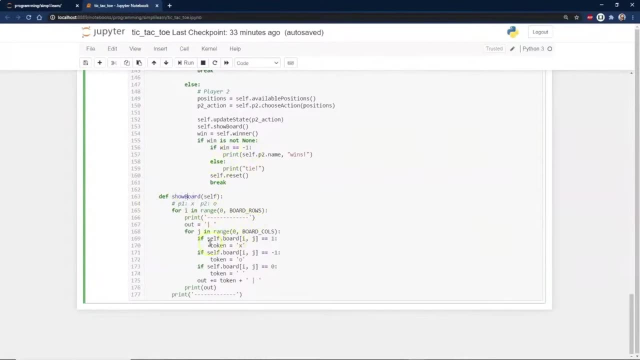 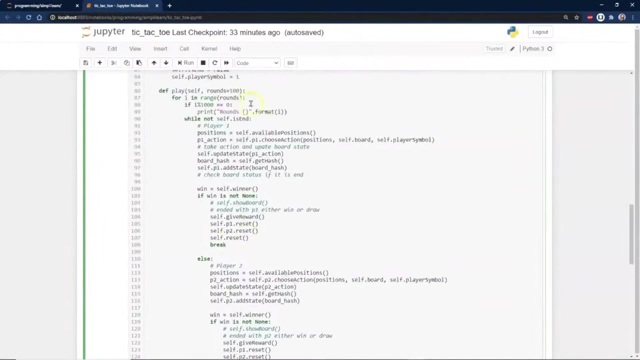 or sees if it wins or ties, looks at available positions, all that kind of fun stuff, and then finally, we want to show the board, so it's going to print the board out each time. really, as an integration, it's not that exciting. what's exciting in here is one looking at this: 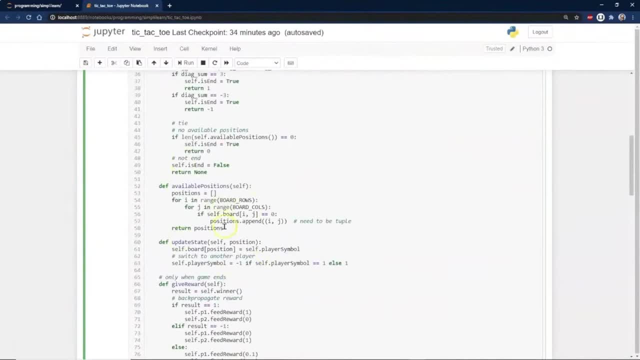 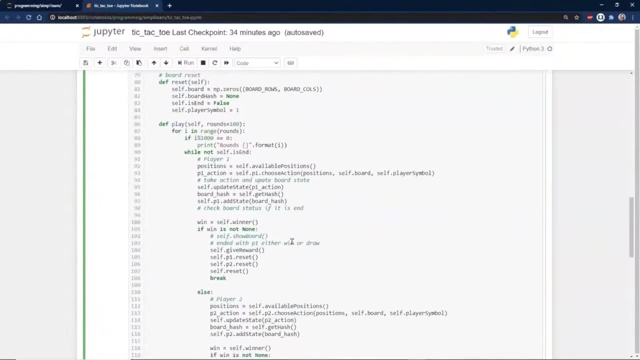 reward system. the reward system is really the heart of this. how do you reward the different set up? and the other one is when it's playing. it's got to take an action, and so what it chooses for an action is also the heart of reinforcement learning. how do we choose that action? 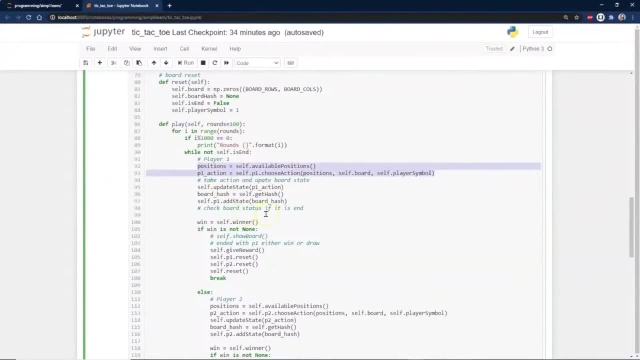 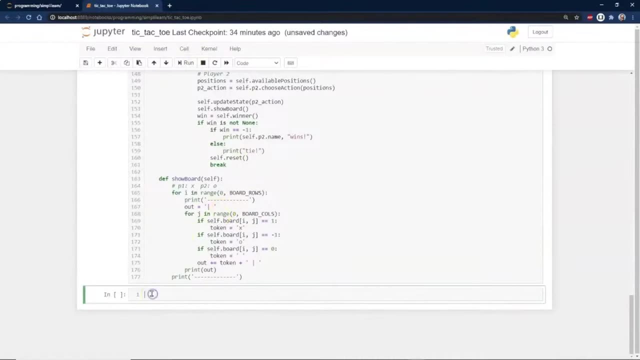 and those are really key to right now where reinforcement learning is in. today's technology is figuring this out. how do we reward it and how do we guess the next best action? so we have our environment and you can see the environment or the state, which is kind of like what's going on. 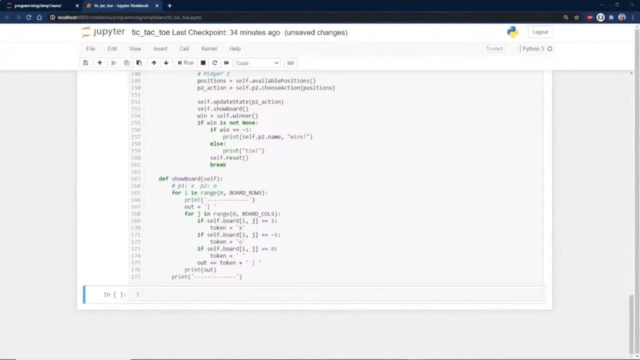 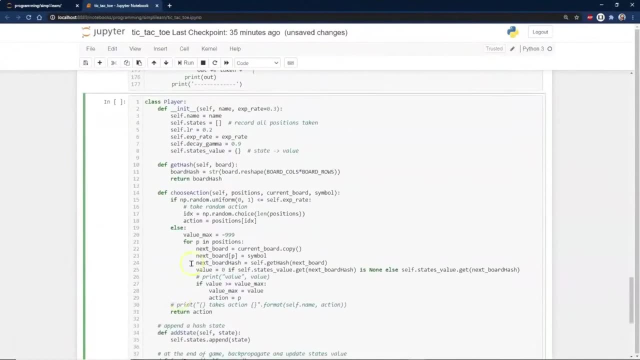 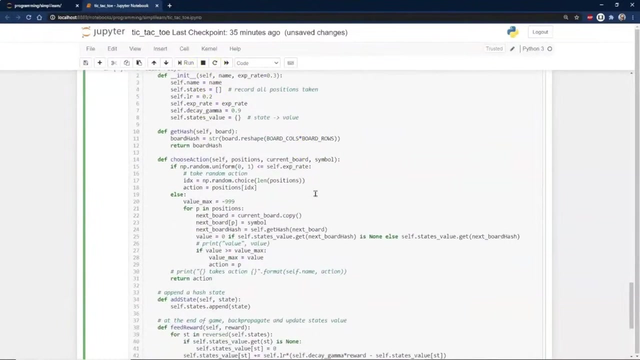 in the state, depending on what happens, and we want to go ahead and create our agent, in this case our player. so each one is grab that and so we look at a class player. this is where a lot of the magic is really going on. how is this player figuring out? 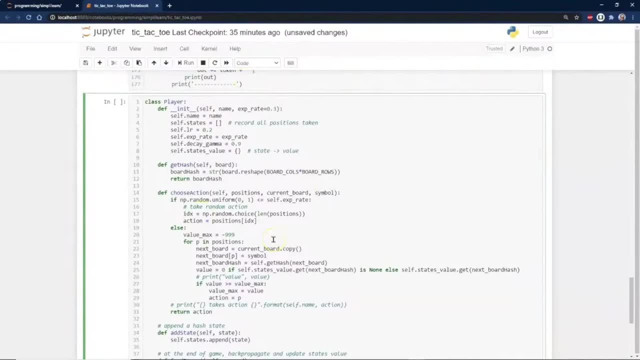 how to maneuver around the board. and then the board of course returns a state that it can look at and reward. so we want to take a look at this. we have name self state. this is class player, and when you say class player, we're not talking about. 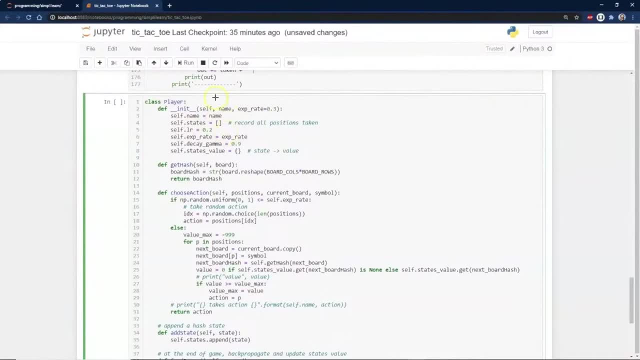 a human player. we're talking about just the computer players, and this is kind of interesting because, remember I told you, depending on what you're doing, there's going to be a decay gamma explore rate. these are what I'm talking about is how do we train it? 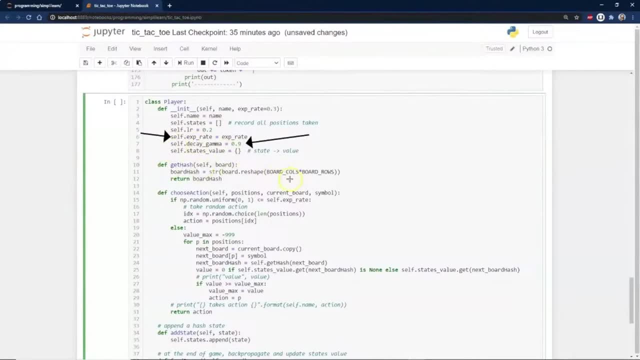 as you try different moves, it gets to the end. the first move is important, but it's not as important as the last one, and so you could say that the last one has the heaviest weight, and then, as you get there, the first one, let's say the first move. 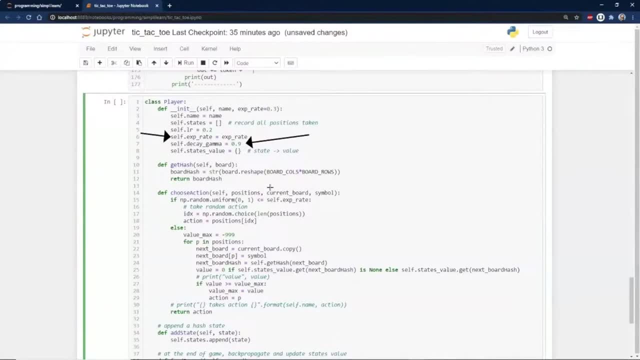 gives you a 5 reward, the second gives you a 2 reward and the third one gives you a 10 reward, because that's the final ending. you got it. the 10 is going to count more than the first step, and here's our: we're going to get the. 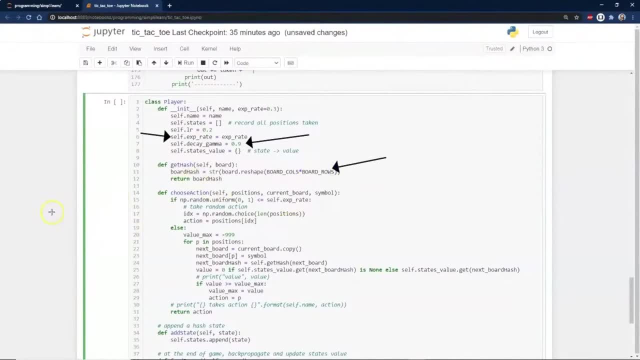 board information coming in and then choose an action. this was the second part that I was talking about. that was so important. so once you have your training going on, we have to do a little randomness and you can see, right here is our NP random uniform. so it's picking out a random number. 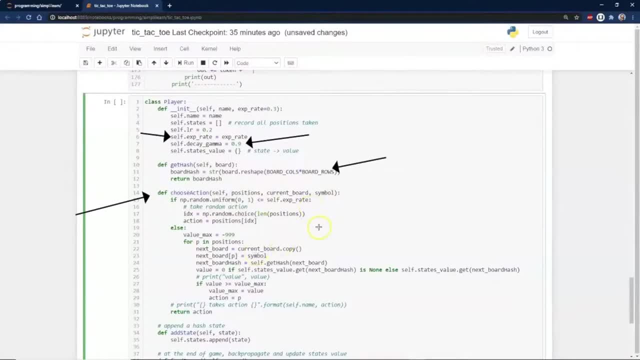 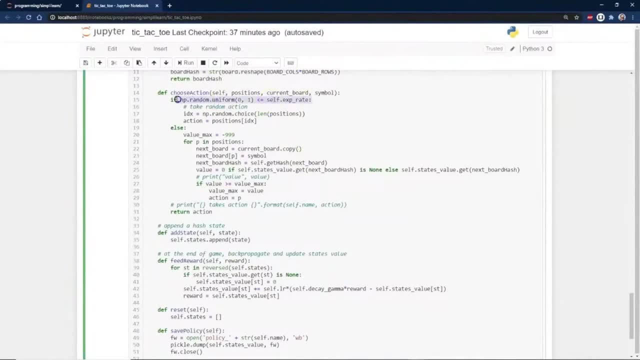 take a random action. this is going to just pick which row and which column it is and so choosing the action, this one. you can see we're just doing random states, choice, length of positions, action position. and then it skips in there and takes a look at the board. 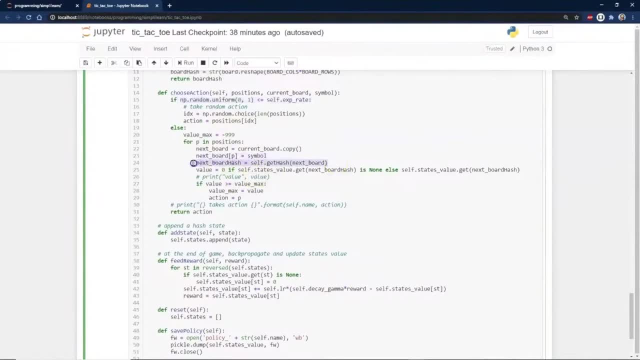 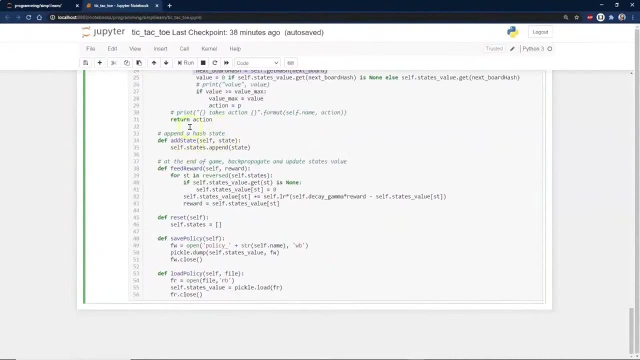 for P and positions. it's actually storing the different values each time you go through, so it has a record of what it did, so it can properly weigh the values, and this simply just appends a hash state. what's the last state? append it to our states on here. 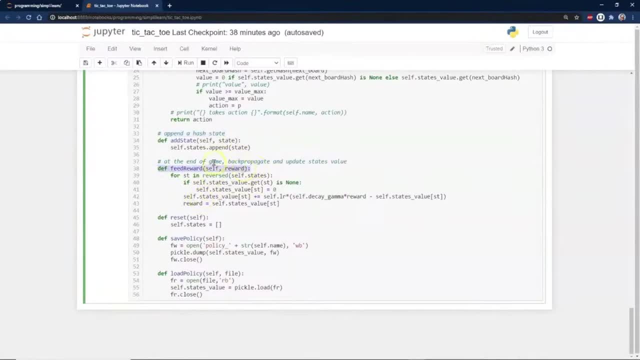 here's our feedback: rewards. the reward comes in and it's going to take a look at this and say: is it none? what is the reward? and here is that formula. remember I was telling you about up here. that was important because it has times a reward. this is where, as it goes, 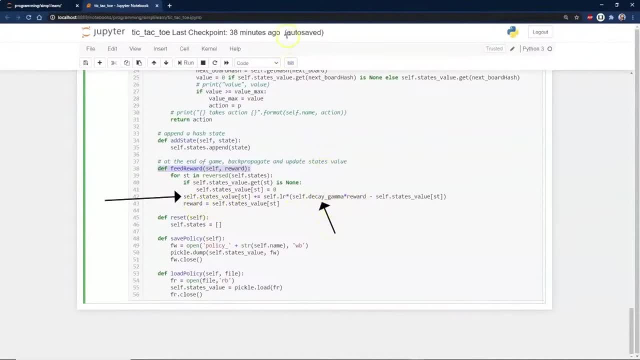 through each step, and this is really important. this is kind of the heart of this, of what I was talking about earlier. you have step one, and this might have a reward of two. you have step two, this has a step three, step four and so on until you get to step in. 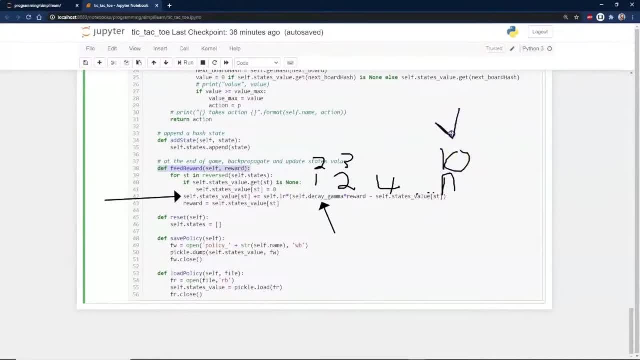 and this might have a reward of ten. so reward of ten. we're going to add that, but we're not adding. let's say this one right here. let's say this reward here: right before ten was, let's say it's also ten. that just makes the math easy. 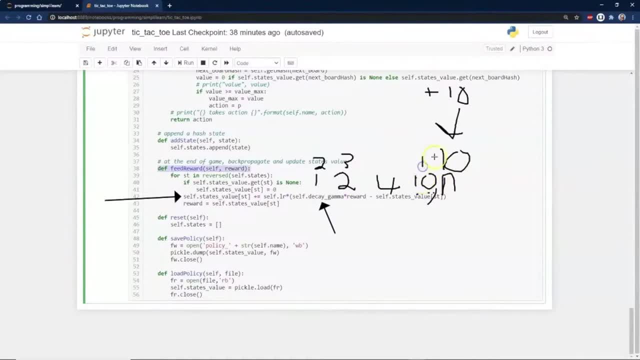 so we had ten and ten, we had ten, this is ten and ten in whatever it is, but this time it's point nine. so instead of putting a full ten here, we only do nine. that's point nine times ten, and so this formula as far as the decay, 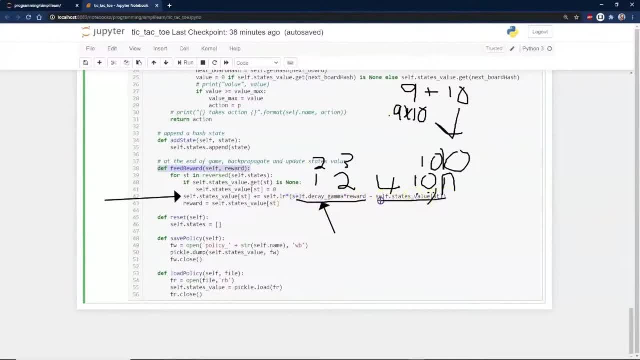 times the reward minus the self state value. it basically adds in. it says here's one or here's two. I should have done this ABC. it would have been easier. so the first move goes in here and it puts two in here. you can see how this gets pretty complicated. 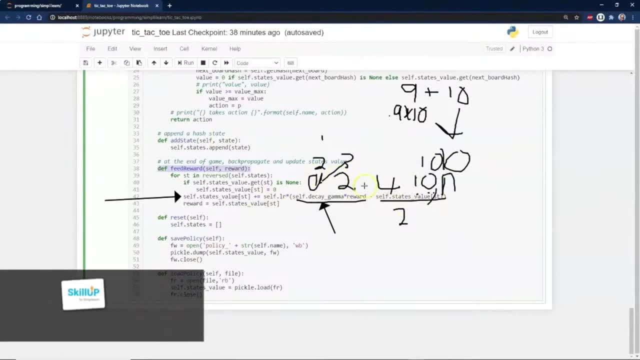 in the math. but this is really the key is: how do we train our states? and we want the final state, the win, to get the most points. if you win, you get the most points and the first step gets the least amount of points. so you're really training this. 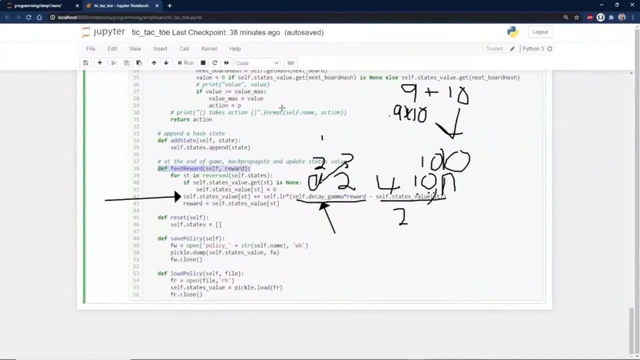 almost in reverse. you're training it from the last place where you have. this is now where I need to sum up my rewards and I want to sum them up going in reverse and find the answer in reverse- kind of an interesting play on the mind when you're trying to figure this stuff out. 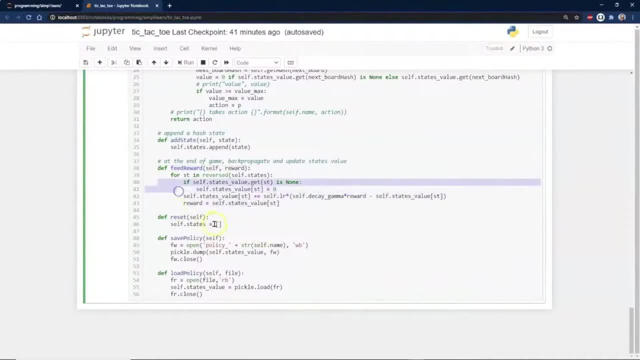 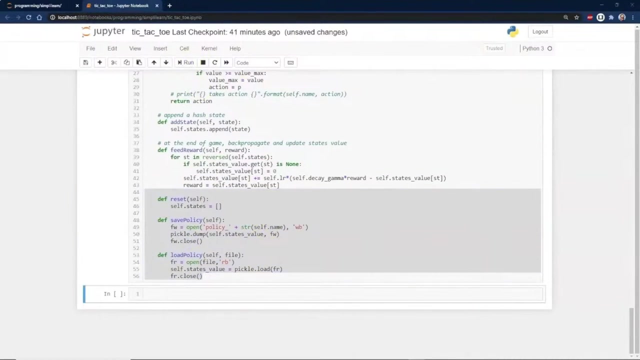 and, of course, we want to go ahead and reset the board down here, save the policy, load policy. these are the different things that are going in between the agent and the state to figure out what's going on. let's go ahead and load that up and then, finally, we want to go ahead. 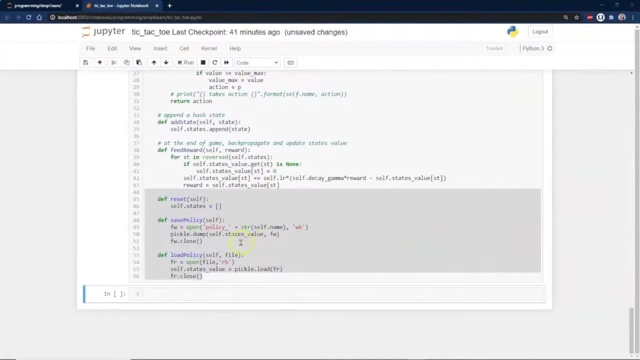 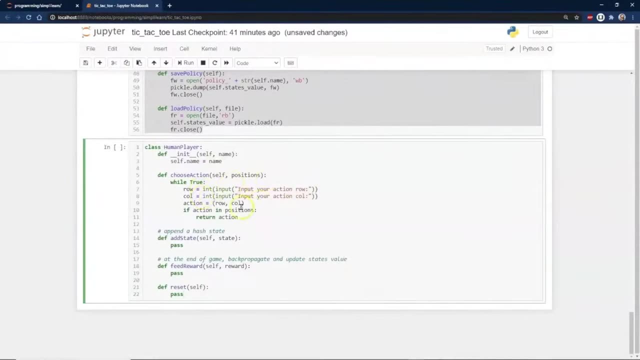 and create a human player. and the human player is going to be a little different in that you choose an action row and column. here's your action. if action in positions- meaning positions that are available- you return the action. if not, it just keeps asking you until you get the action that actually works. 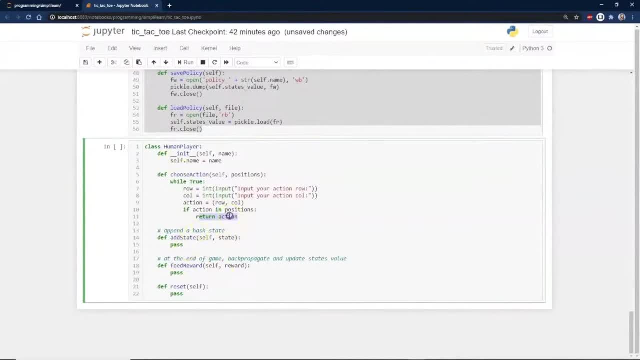 and then we're going to go ahead and append to the hash state- which we don't need to worry about because it returns the action up here- and feed forward- because it's a human at the end of the game- bat, propagate and update state values. this part isn't being done. 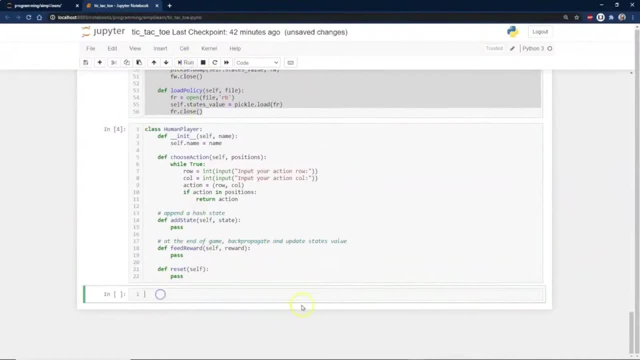 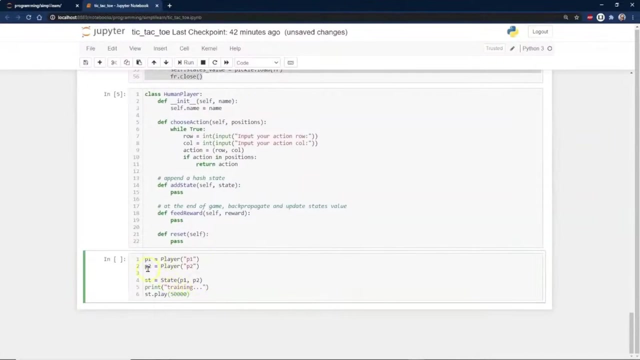 because it's not programming the model. the model is getting it's own rewards, so we've gone ahead and loaded this in here. so here's all our pieces, and the first thing we want to do is set up p1 player 1, p2- player 2. 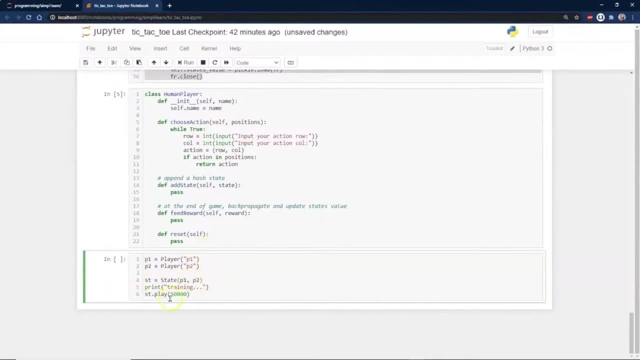 and then we're going to send our players to our state. so now it has p1, p2 and it's going to play 50,000 rounds. now we can probably do a lot less than this and it's not going to get the full results. 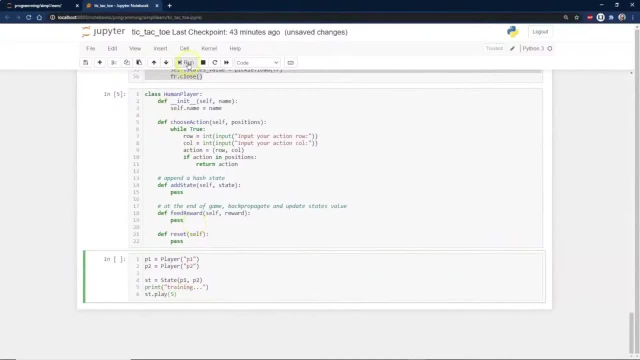 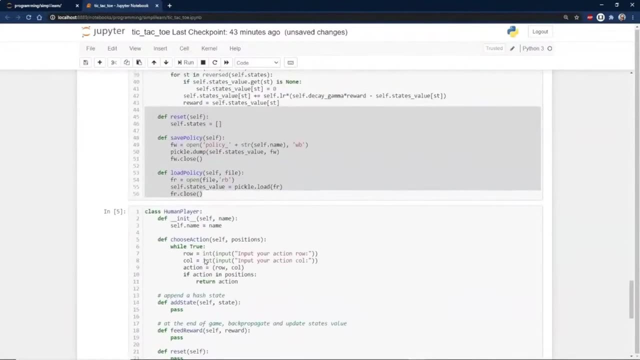 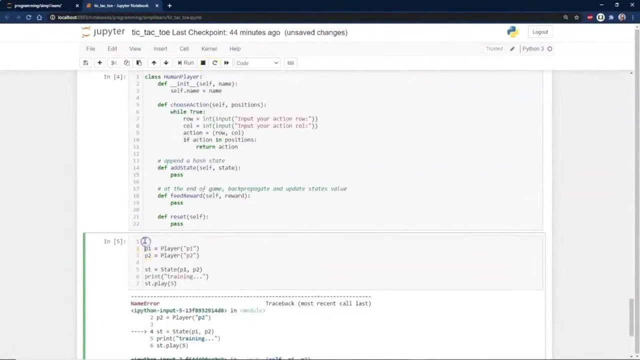 in fact, you know what? let's go ahead and just do 5 just to play with it, because I want to show you something here. oops, somewhere in there I forgot to load something. there we go. I forgot to run this run. I forgot a reference there for the board. 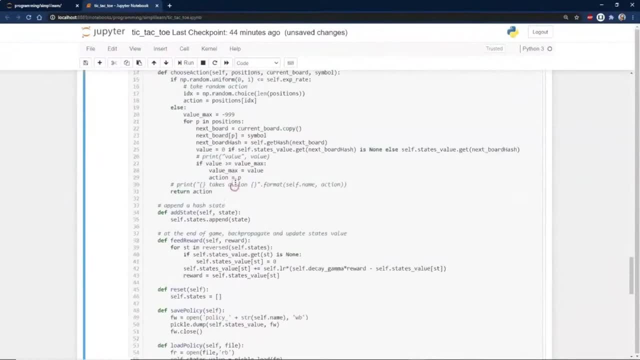 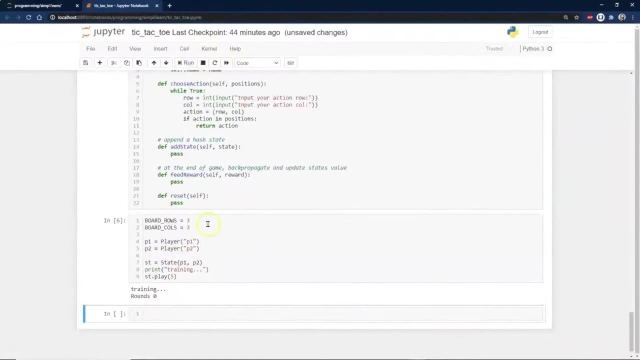 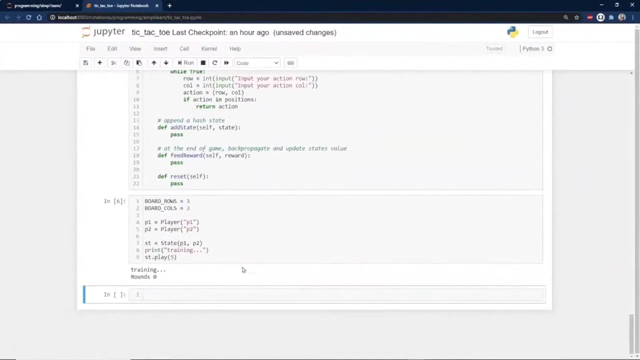 rows and columns 3x3. there's actually in the state it references that we can just tack it on on the end. it was supposed to be at the beginning, so now I've only set this up with. let's see where are we going here? I've only set this up to train. 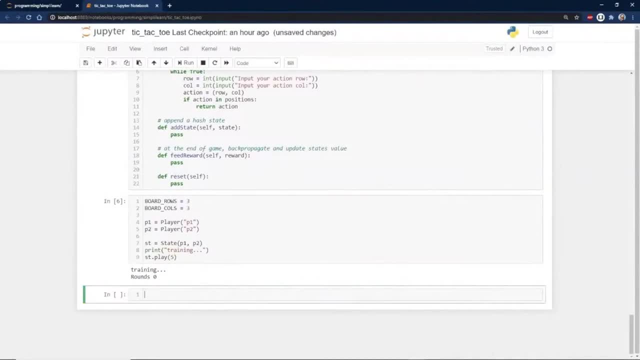 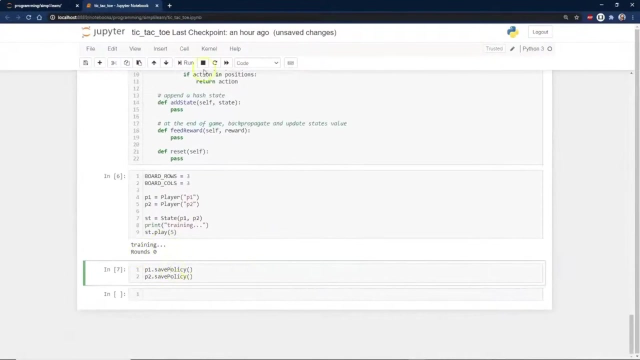 5 times and the reason I did that is we're going to come in and actually play it and I'm going to change that and we can see how it differs on there. there we go, and it didn't even make it through a run and we're going to go ahead and save the policy. 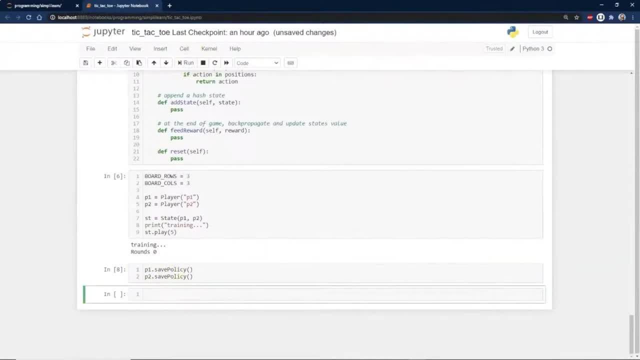 so now we have our player 1 and our player 2 policy. the way we set it up, it has two separate policies loaded up in there, and then we're going to come in here and we're going to do: player 1 is going to be the computer. 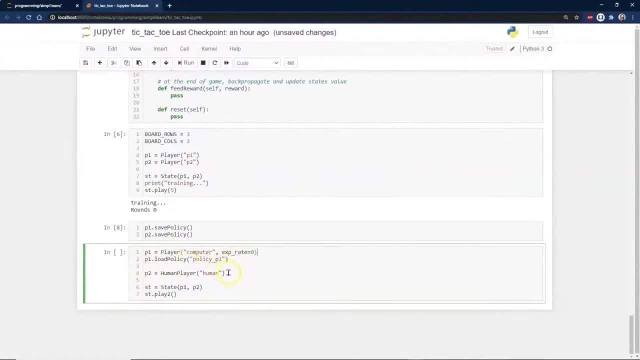 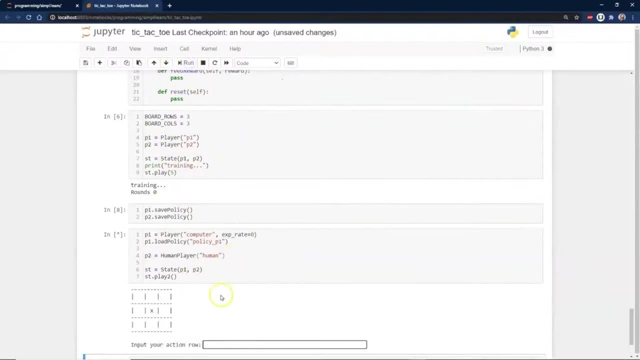 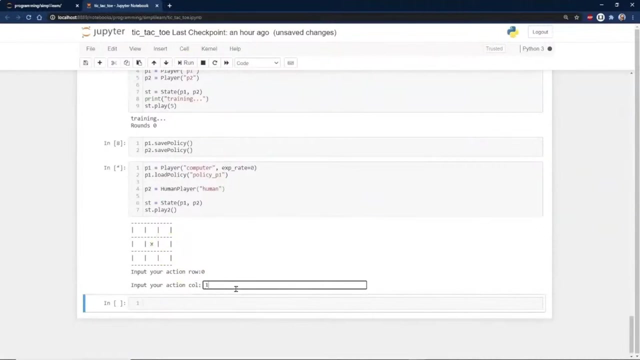 experience rate: 0. load policy: 1: human player: human. now remember, I only went through it. just one round of training, in fact minimal training, and so it puts an x there and I'm going to go ahead and do row 0, column 1, and you can see this is very. 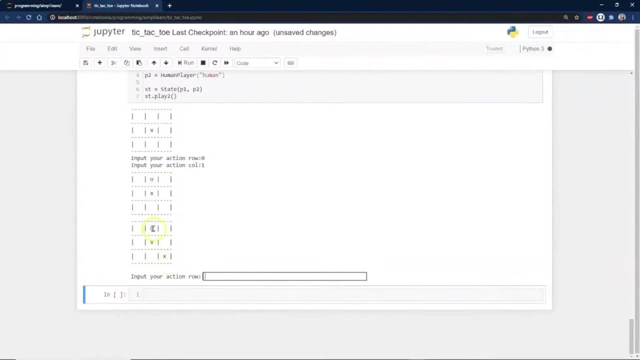 basic on here, and so I put in my 0 and then I'm going to go 0, block it 0, 0 and you can see right here it. let me win. just like that, I was able to win 0, 2 and human wins. 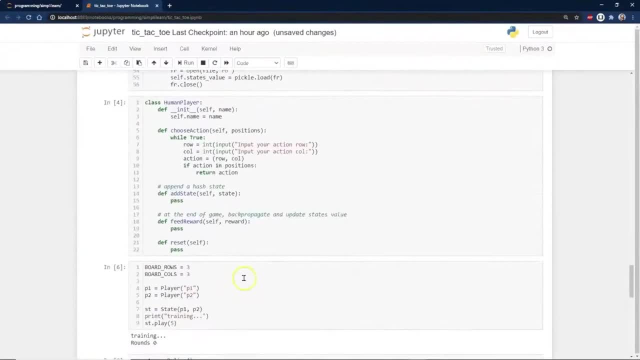 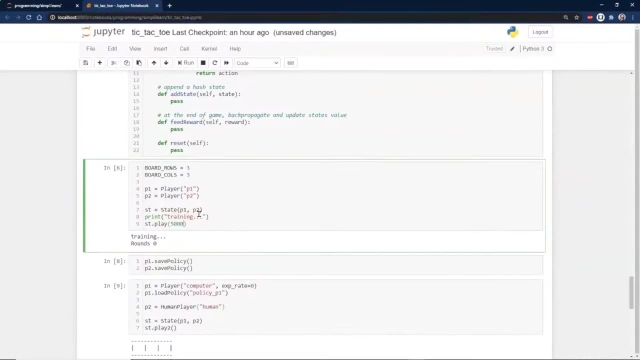 so I only trained it 5 times. we're going to run this again, and this time, instead of 5, let's do 5,000 or 50,000- I think that's what the guys in the back had- and this takes a while to train it. 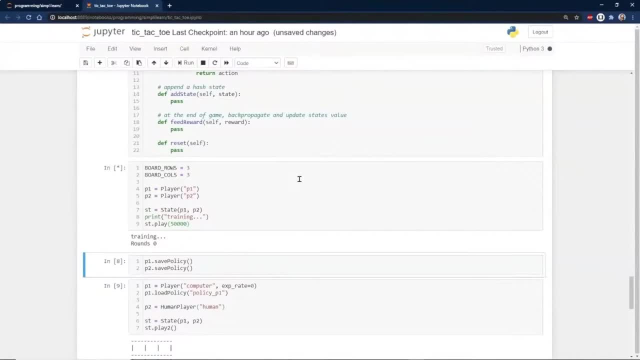 this is where reinforcement learning really falls apart. look how simple this game is. we're talking about a 3x3 set of columns, and so for me to train it on this, I could do a Q table, which would go much quicker. you could build a quick Q table. 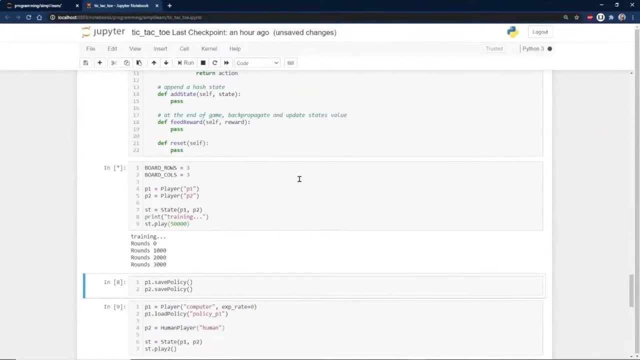 with almost all the different options on there and you would probably get the same result much quicker. we're just using this as an example. so when we look at reinforcement learning, you need to be very careful what you apply it to. it sounds like a good deal until you do like a large neural network. 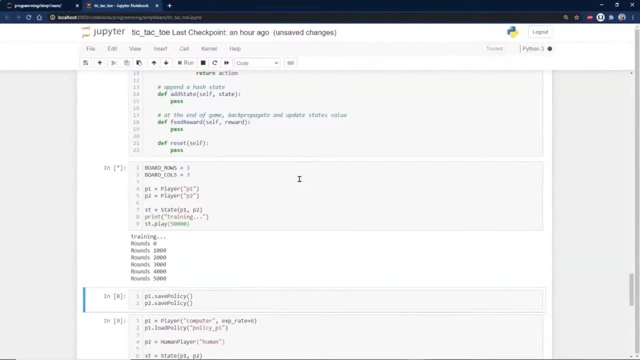 where you're doing. you set the neural network to a learning increment of 1, so every time it goes through it learns. and then you do your actions. you pick from the learning set up and you actually try actions on the learning set up until you get what you think is going to be the best action. 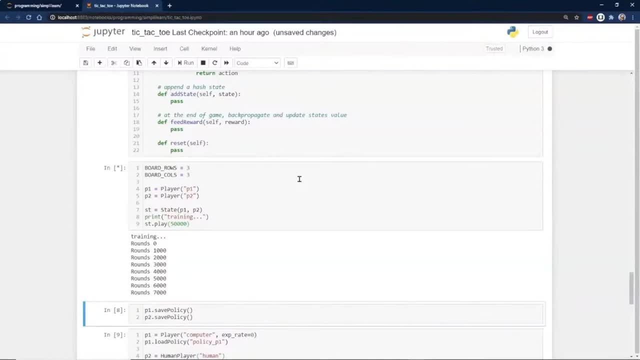 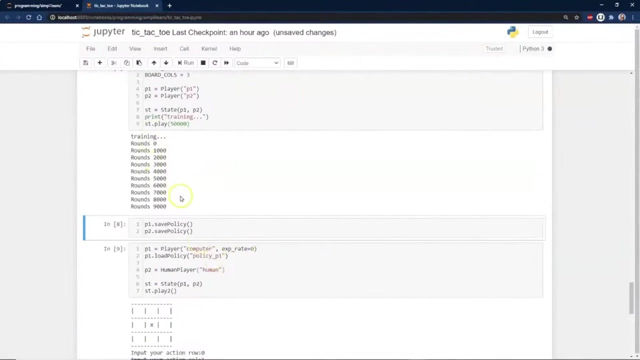 so you actually feed what you think is right back through the neural network. there's a whole layer there which is really fun to play with, and then it has an output. I mean, that is just a huge amount of work it's going to do. let's go ahead and skip ahead here. 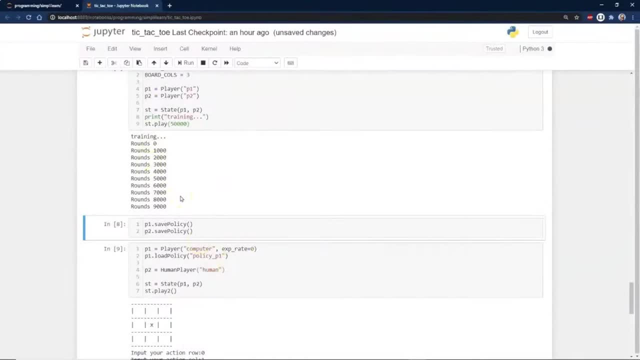 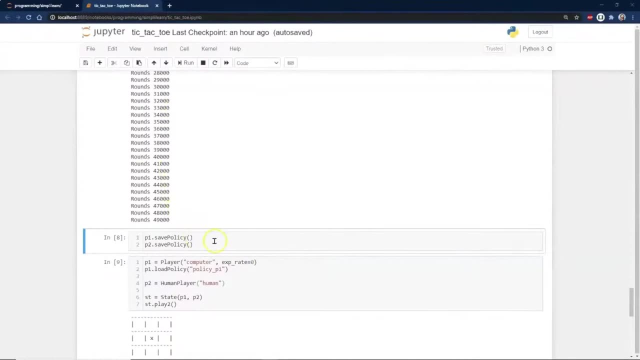 give it a moment. it's going to take a minute or two to go ahead and run now. to train it, we went ahead and let it run and it took a while. I got a pretty powerful processor and it took about 5 minutes plus to run it. 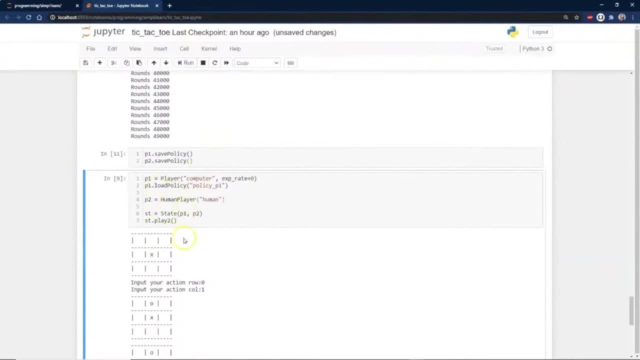 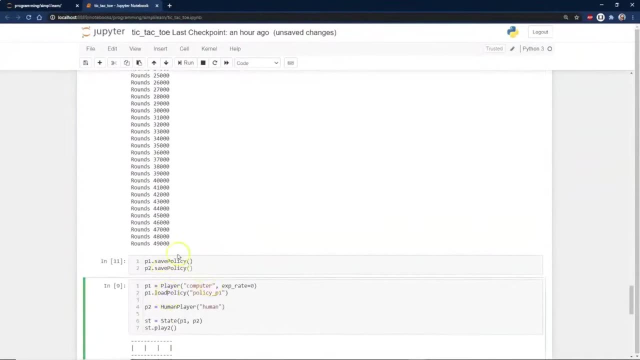 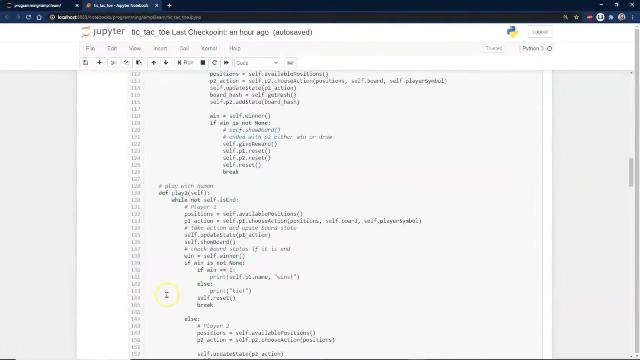 and we'll go ahead and run our player set up on here. it brought in the last round, so give me just a moment to redo the policy. save there we go. I forgot to save the policy back in there and then go ahead and run our player again. 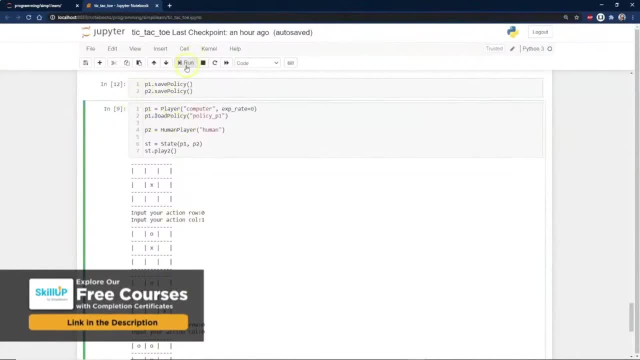 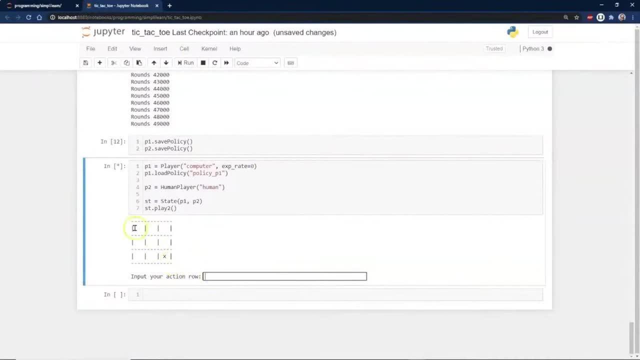 so we've saved the policy and we want to go ahead and load the policy for P1 as the computer- and we can see the computer has gone in the bottom right corner- I'm going to go ahead and go 1. 1, which is the center. 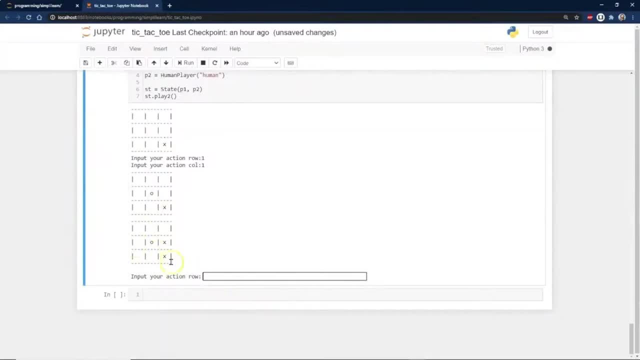 and it's gone right up the top, and if you've ever played tic-tac-toe you know the computer has me, but we'll go ahead and play it out. row 0, column 2: there it is, and then it's gone here and so I'm going to go ahead and go. 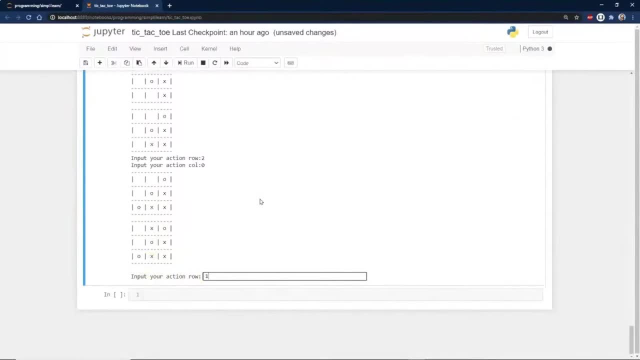 row 0, 1, 2, no, 0, 1. there we go. and column 0: that's where I want it. oh, and it says: ok, your action, there we go. so you can see, here we've got a. it's a tie. kind of funny. they didn't catch the win on there. 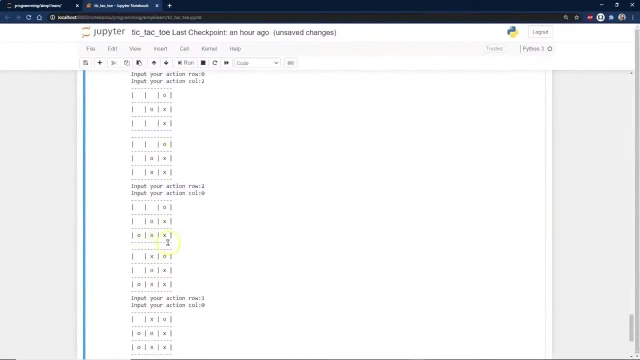 but if we play this a bunch of times, you'll find that it's going to win more and more. the more we train it, the more the reinforcement happens. this lengthy training process is really the stopper on reinforcement learning. as this changes, reinforcement learning will be one of the more powerful packages. 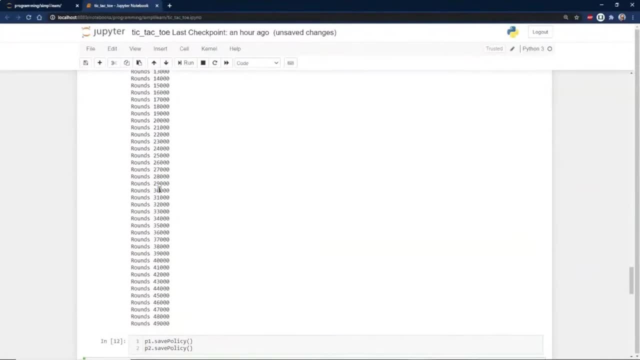 evolving over the next decade or two. in fact, I would even go as far as to say it is the most powerful and most important machine learning tool and artificial intelligence tool out there, as it learns not only a simple tic-tac-toe board, but we start learning environments. 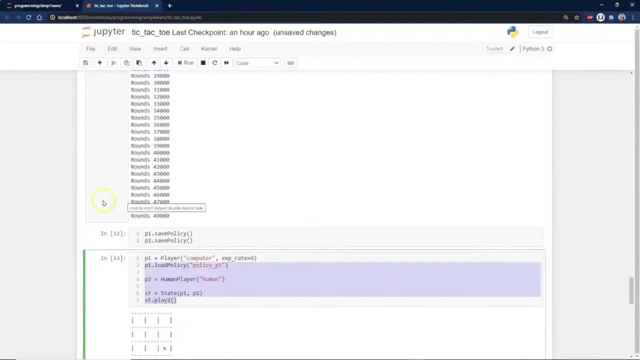 and the environment would be like a language: if you're translating a language from one language to the other, so much of it is lost if you don't know the context it's in, what's the environment it's in, and so being able to attach environment and context. 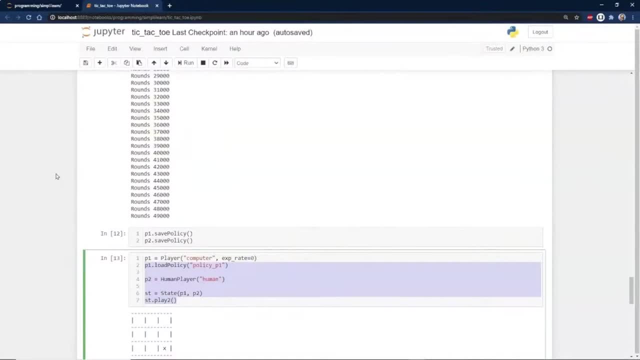 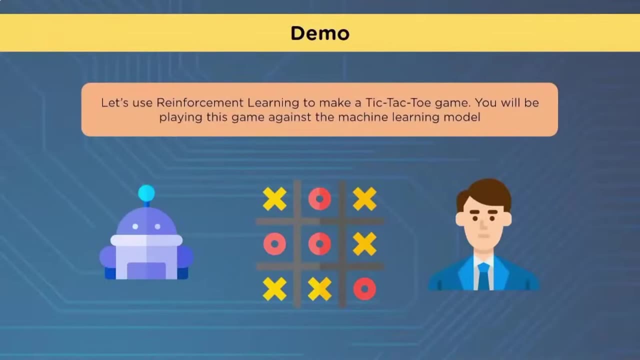 and all those things together is going to require reinforcement, learning to do so. again, if you want to get a copy of the tic-tac-toe board- it's kind of fun to play with- run it, you can test it out. you can test it for different values. 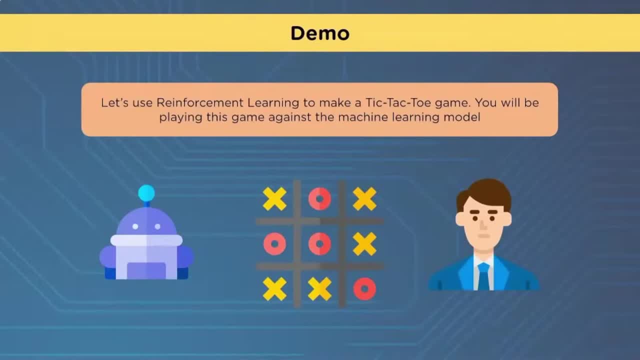 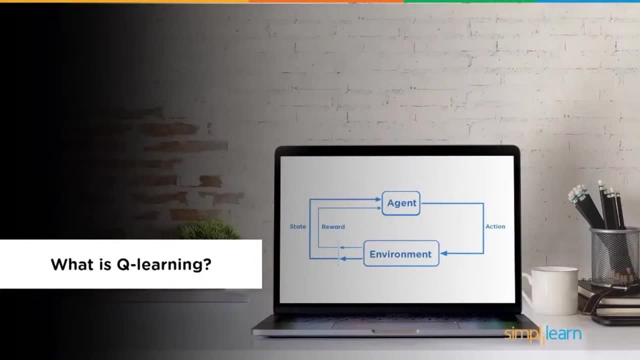 you can switch from P1 computer, where we loaded the policy 1, to load the policy 2 and just see how it varies. there's all kinds of things you can do on there. so what is Q-learning? Q-learning is reinforcement learning policy which will fill the next best action. 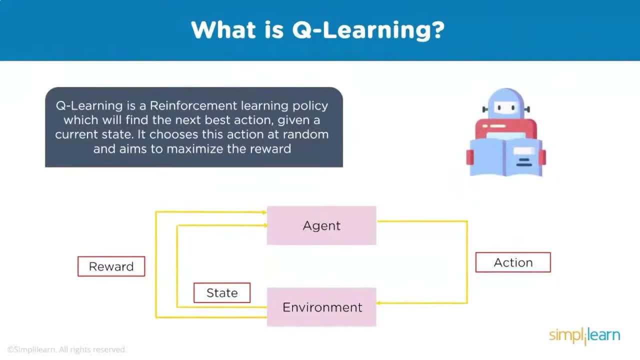 given a current state, it chooses this action at random and identifies the reward, and so you can see- here's our standard reinforcement learning graph by now. if you're doing any reinforcement learning, you should be familiar with this. where you have your agent, your agent takes an action. 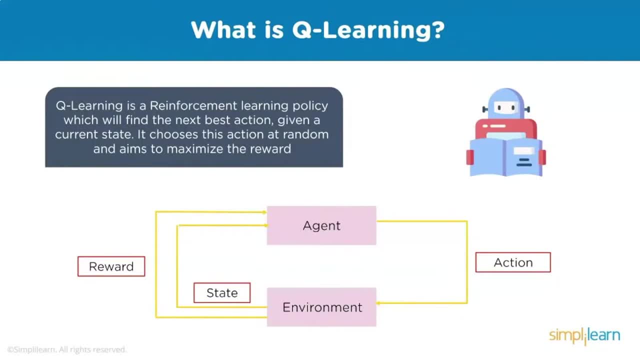 the action affects the environment, and then the environment sends back the reward or the feedback and the new state the agent's in. where is it at on the chess board? where is it at in the video game if your robot's out there picking trash up off the side of the road? 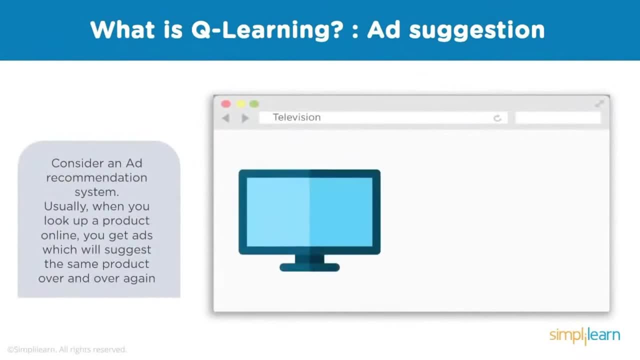 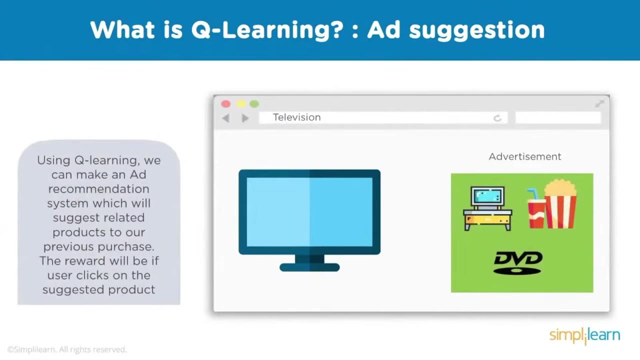 consider an ad recommendation system. usually, when you look up a product online, you get ads which will suggest the same product over and over again. using Q-learning, we can make an ad recommendation system which will suggest related products to our previous purchase. the reward will be if user clicks. 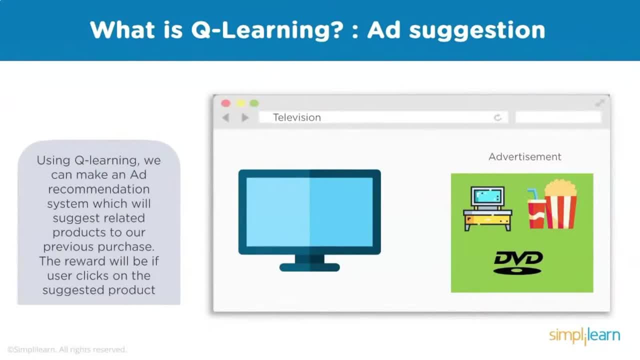 on the suggested product and again you can see you might have a lot of products on your website, your web advertisement or your pages, but it's still not a float number, it's still a set number and that's something to be aware of when you're using Q-learning. 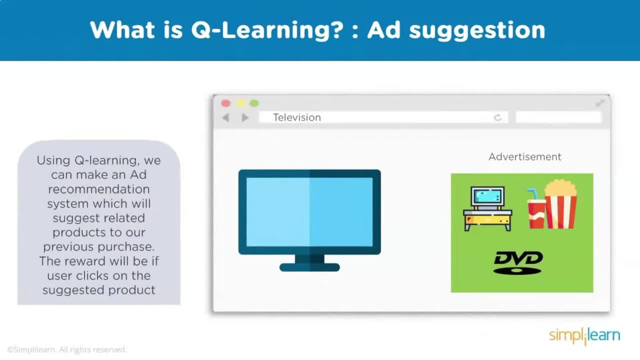 and you can see here that if you have 100 people clicking on ads and you click on one of the ads, it might go in there and say, okay, this person clicked on this ad. what is the best set of ads based on clicking on this ad or these two ads afterwards? 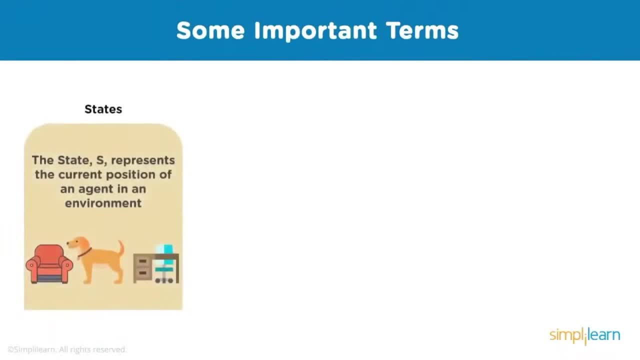 based on where they are browsing to see what they're doing or what their. and again, when we talk about states, we're usually not. when you're using a Q table, you're not usually talking about float variables. you're talking about true, false. we'll take a closer look at that in a second. 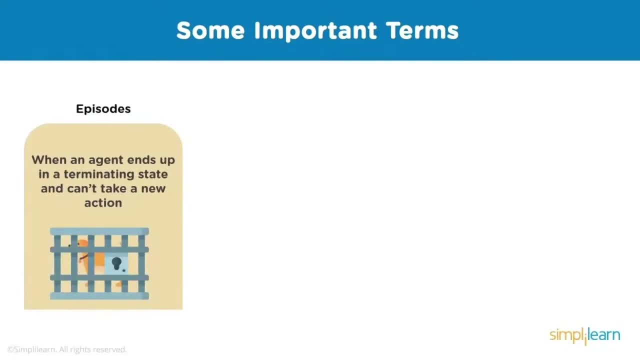 And episodes when an agent ends up in a terminating state and can't take a new action. This might be if you're playing a video game. your character stepped in and is now dead, or whatever Q values used to determine how good an action A taken at a particular state. S is Q A of S. 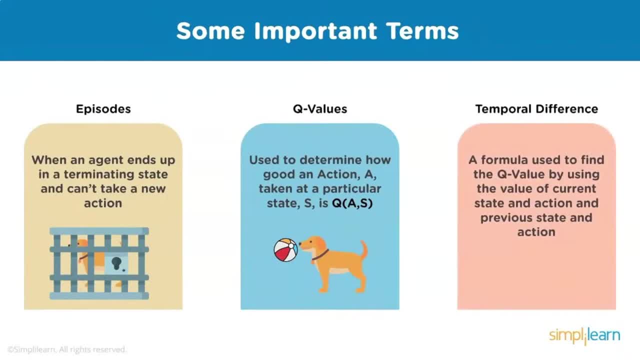 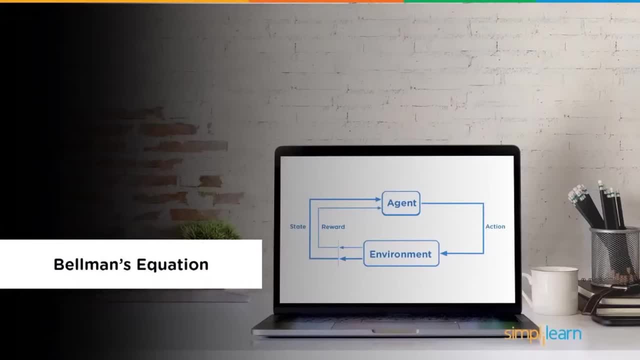 And temporal difference, a formula used to find the Q value by using the value of the current state and action and previous state and action. And there's Bellman's equation, which basically is the equation that kind of covers what we just looked at in all those different terms. 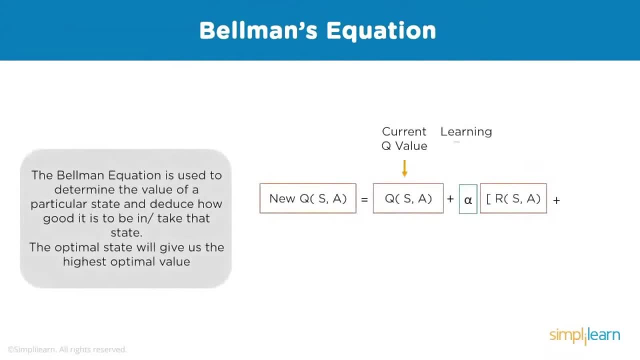 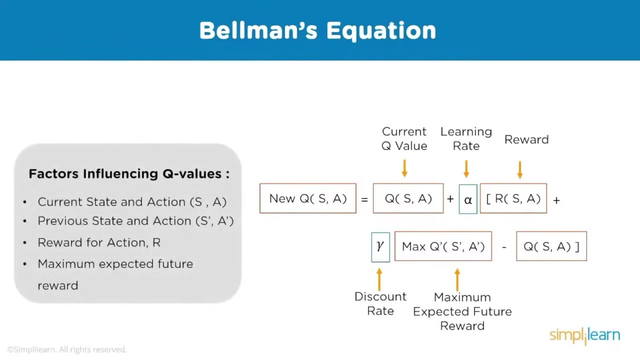 The Bellman equation is used to determine the values of a particular state and deduce how good it is to be in. take that state, The optimal state will give us the highest optimal value Factor influencing Q values. the current state and action. that's your S? A, so your current state and your action. 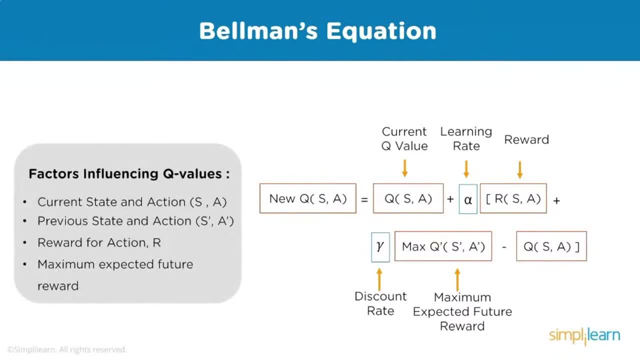 Then you have your previous state and action, which is your S, I guess- prime. I'm not sure how they reference that S, prime, A prime. so this is what happened before. Then you have a reward for action, so you have your R reward and you have your maximum expected future reward. 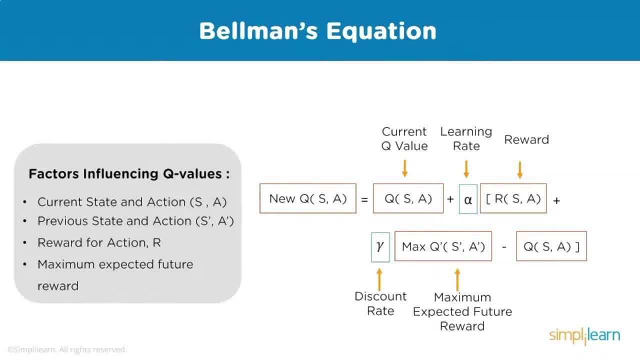 And you can see there's also a learning curve. There's a learning rate put in there and a discount rate. So when we're looking at these, just like any other model, we don't want to have an absolute final value on here. 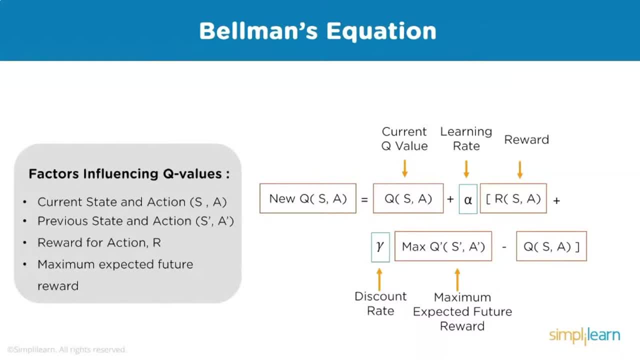 We don't want it to. if you do absolute values instead of taking smaller steps, you don't really have that approach to the solution. You just have a jump and then pretty soon, if you jump one solution out, that's what's going to be the new solution, whichever one jumps up really high first. 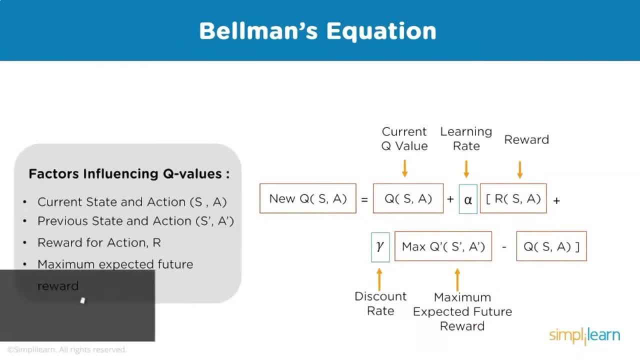 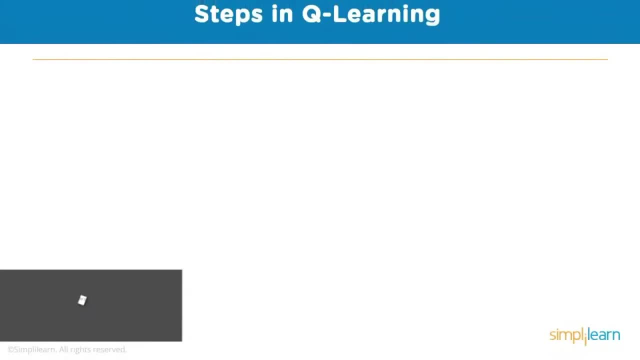 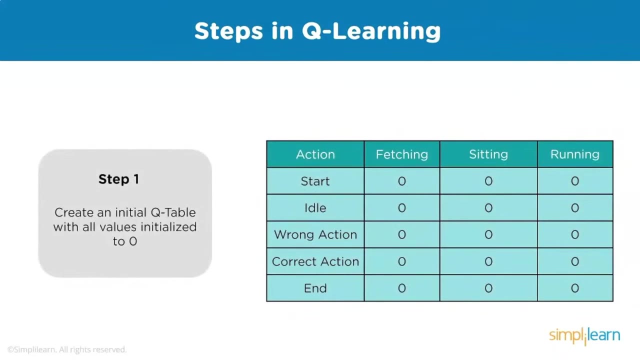 Kind of ruining the solution And the whole idea of doing a random selection. And I'll go into the random selection in just a second Steps in Q learning, Step one: create an initial Q table with all values initialized to zero. Again, we're looking at zero one. 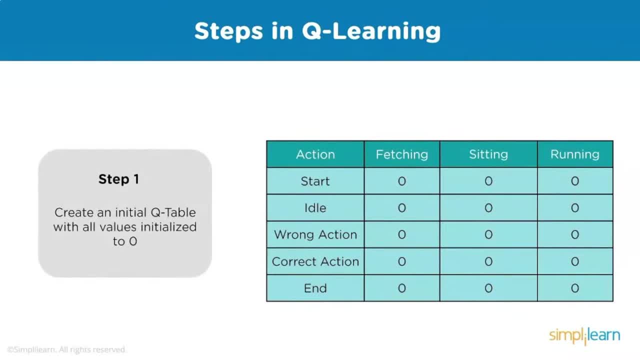 So are you? you know, here's our action. We start, we're in idle, we took a wrong action, we took a correct action and end, And then we have our actions: fetching, sitting and running, And of course, we're just going to do that. 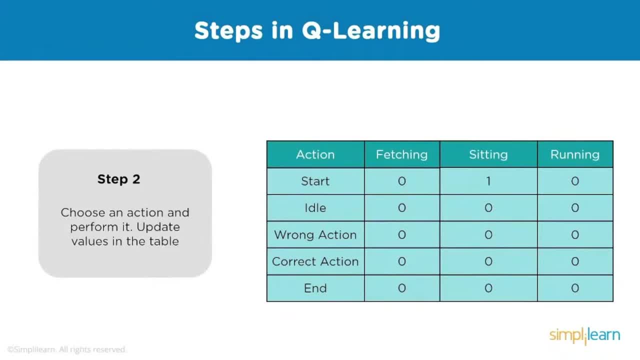 I'm just using the dog example And choose an action and perform it, Update values in the table And of course, when we're choosing an action we're going to kind of do something random and just randomly pick one. So you start out and you sit. 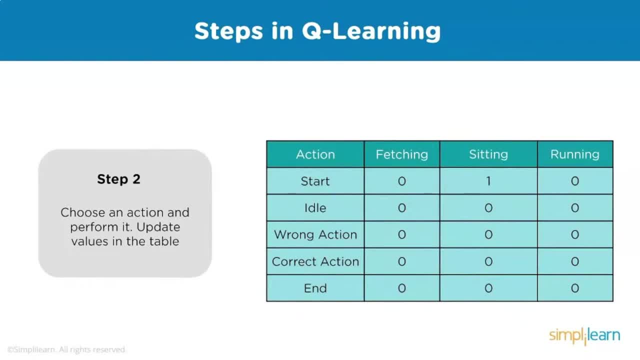 And you have. then, depending on that action you took, you can now update the value for sitting after you start from start to sitting, Get the value of the reward and calculate the value- Q value- using the Bellman equation. And so now we attach a reward to sitting. 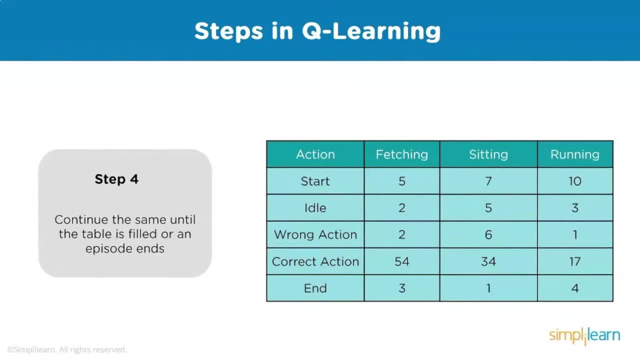 And when we attach all those rewards, we continue the same until the table's filled with or an episode ends. And my image now is going to come back to the random side of this And there's a few different formulas I use for the random setup to pick it. 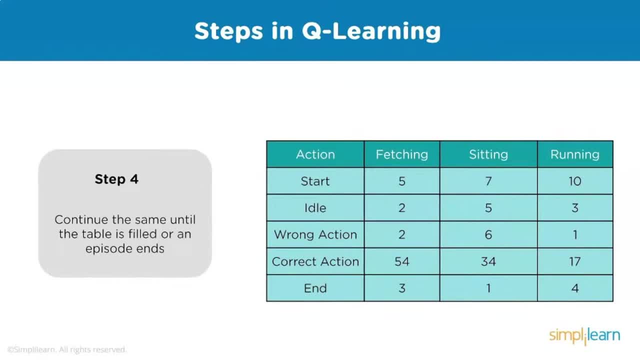 I usually let whatever Q model I'm using do their standard one, because someone's usually gone in and done the math for the optimal spread. But you can look at this So I have: running has a reward of 10.. Sitting has a reward of 7.. 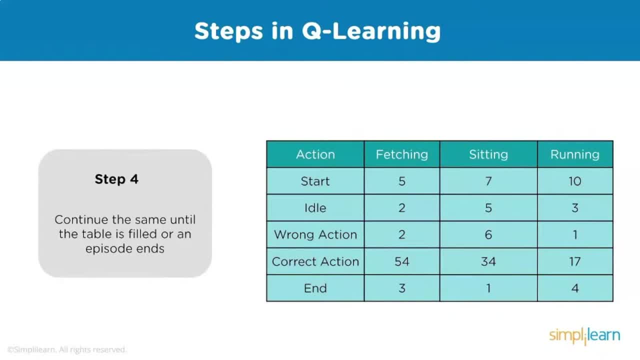 Fetching has a reward of 5.. Just kind of, without doing like a means, you know, using the bell curve for the means value And, like I said, there's some math you can put in there to pick so that you're more likely, so that running has even a higher chance. 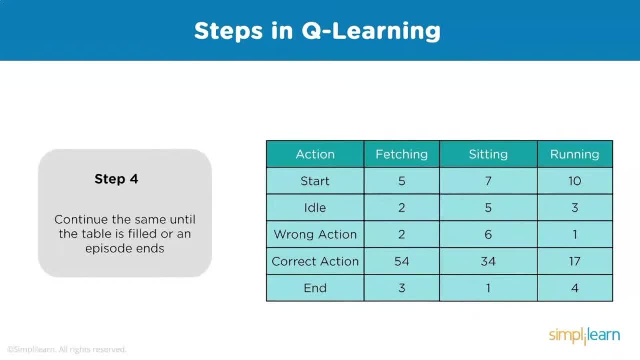 But even if you were just going to do an average on this, you could do an average, a random number, by adding them all together. So you get 10 plus 7 plus 5 is 22.. You can do 0 to 22 or 0 to 21,, but 1 to 22.. 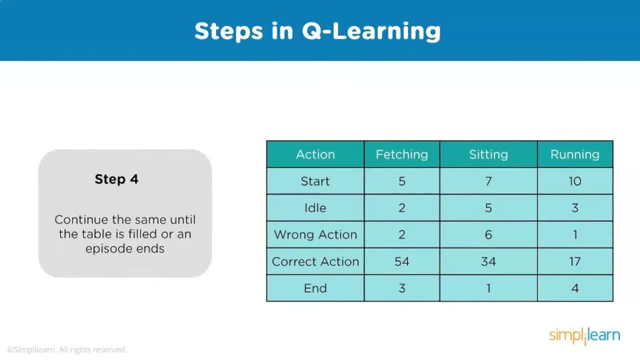 1 to 5 would be fetching, and so forth. You know the last 10.. So you can just look at this: as what percentage are you going to go for that particular option? And then that gets your random setup in there, And then, as you slowly increment these up, you see that if you're idle, 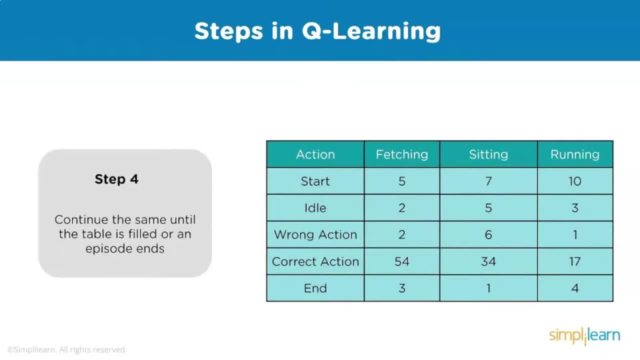 Where's one? Here we go Sitting at the end. If you're at the end of wherever you're at sitting gets a reward of one. Where's a good one on here? Oh, wrong action, Running for a wrong action gets almost no reward. 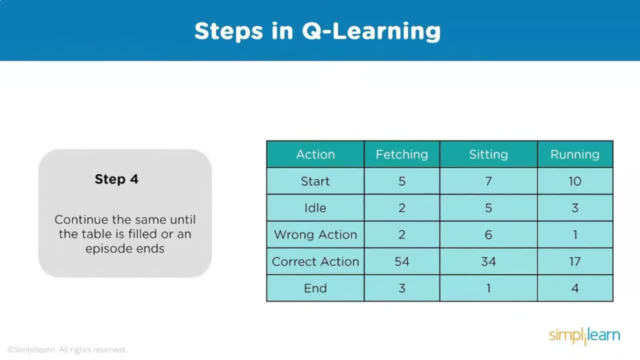 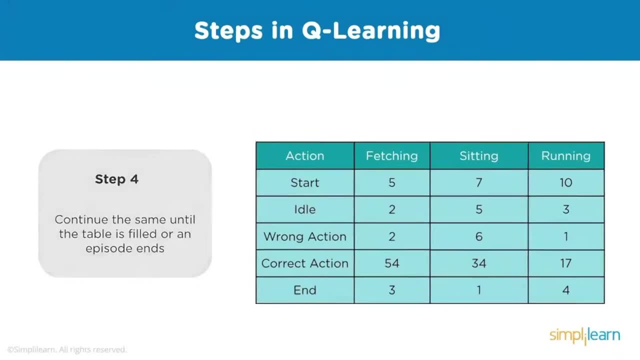 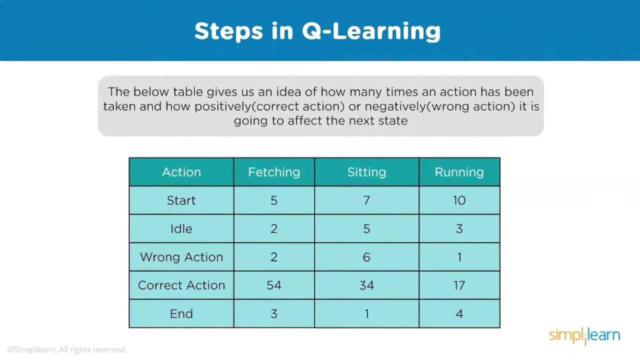 So that becomes very, very less likely to happen. But it still might happen. It still might have a percentage of coming up, And that's where the random programming and Q learning comes in. The below table gives us an idea of how many times an action has been taken and how positively correct action or negatively wrong action it is going to affect the next state. 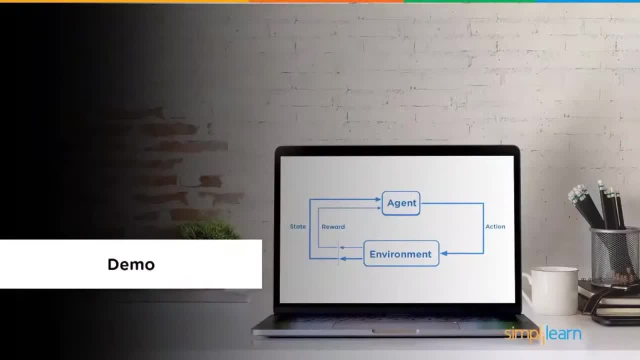 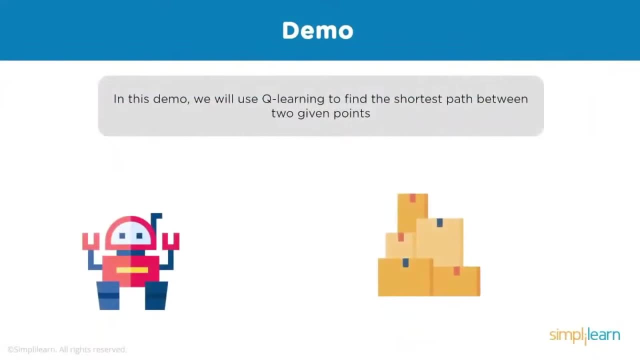 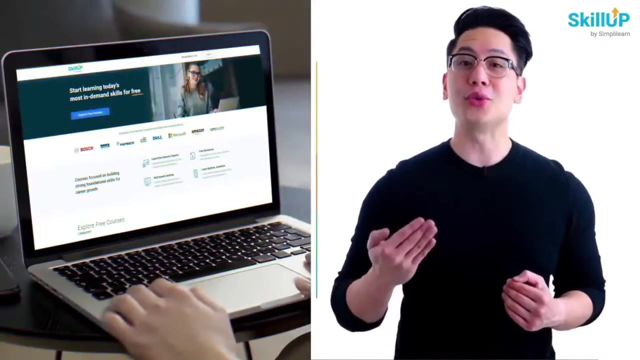 So let's go ahead and dive in and pull up a little piece of code and see what this looks like in Python. In this demo, we'll use Q learning to find the shortest path between two given points. If getting your learning started is half the battle, what if you could do that for free? 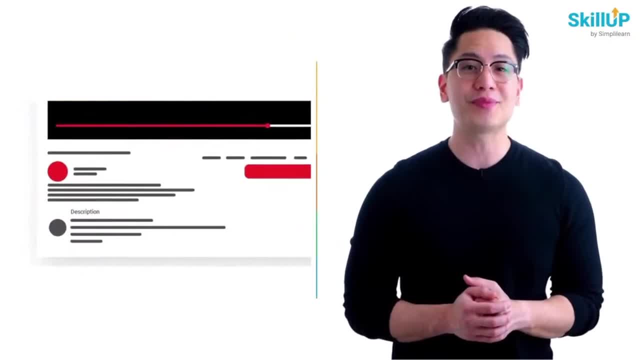 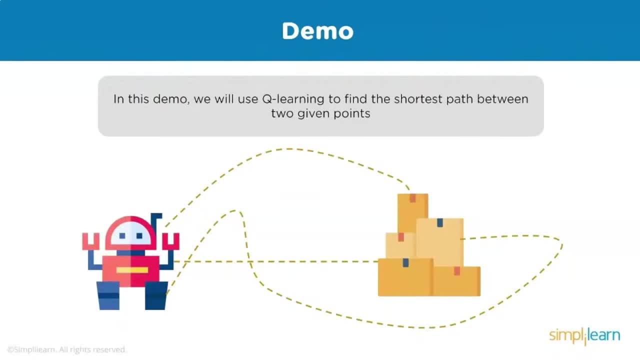 Visit SkillUp by SimplyLearn. Click on the link in the description to know more. If you've seen my videos before, I like to do it in the Anaconda. This is the Jupyter Notebook setup, just because it's really easy to see and it's a nice demo. 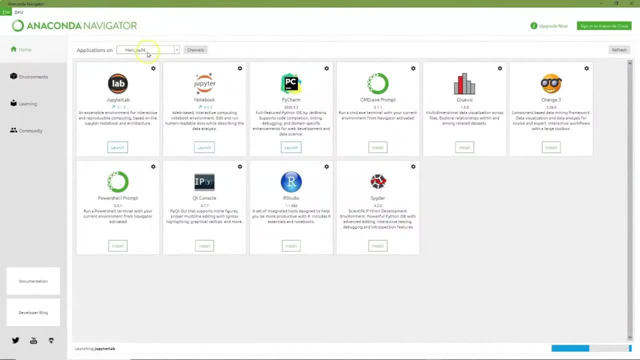 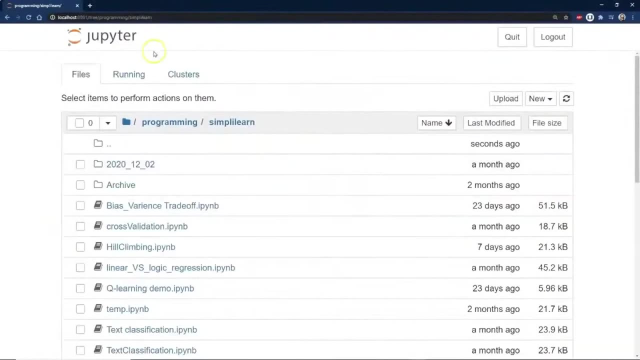 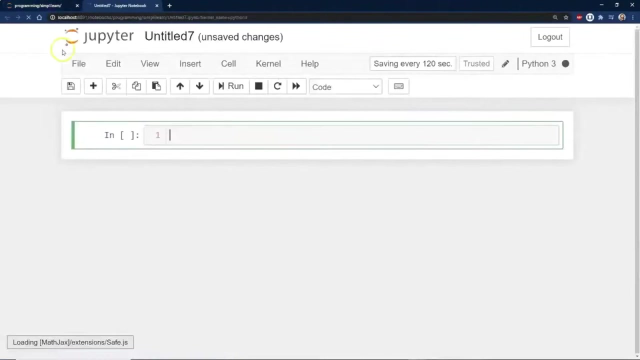 And so here's my Anaconda. This one, I'm actually using Python 3.6 environment that I set up in here, And we'll go ahead and launch the Jupyter Notebook on this. And once we're in our Jupyter Notebook, which has the kernel loaded with Python 3, we'll go ahead and create a new Python 3 folder in here. 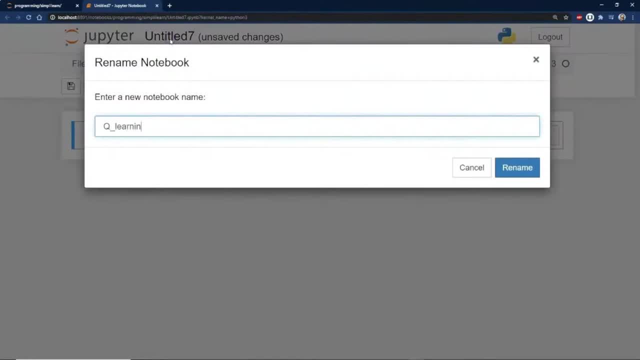 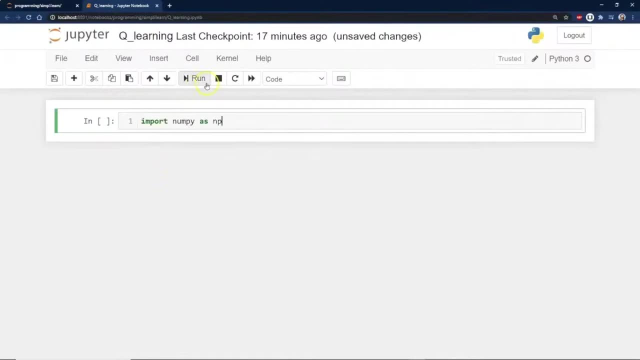 And we'll call this Q Learning. And to start this demo, let's go ahead and import our numpy array. We'll just run that, so it's imported. And, like a lot of these model programs, when you're building them, you spend a lot of time putting it all together. 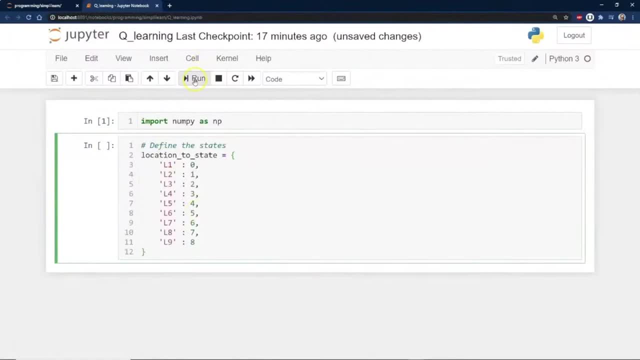 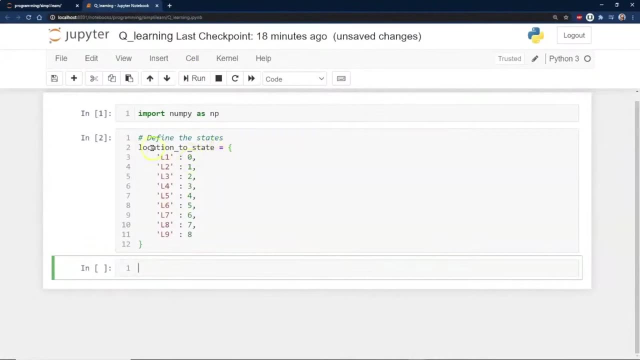 And then you end up with this really short answer at the end, And we'll take a look at that as we come into it. So we go ahead and start with our location to state. So we have L1, L2.. These are our nine locations, one to nine. 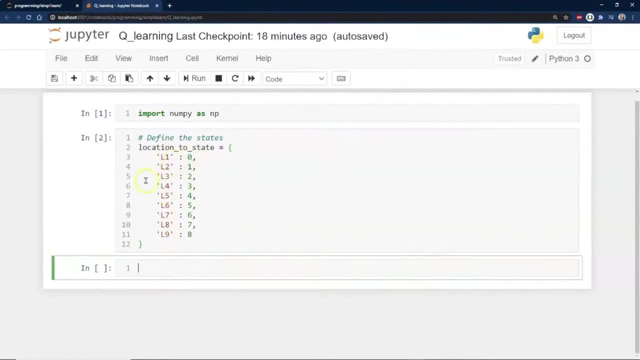 And then, of course, the state is going to be 0,, 1,, 2,, 3,, 4.. It's just a mapping of our location to an integer on there, And then we have our actions. Our actions are simply moving from one location to another. 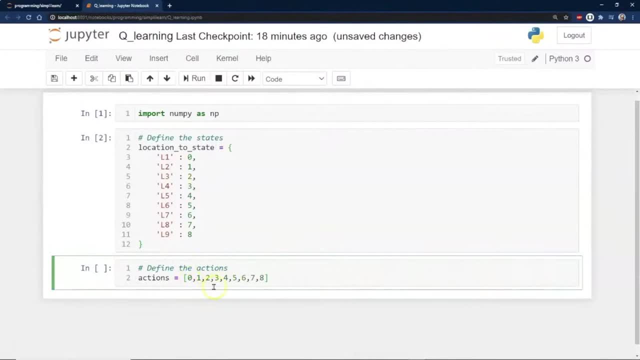 So I can go to location 0.. I can go to location 1,, 2,, 3,, 4,, 5,, 6,, 7, 8.. So these are my actions. I can choose. These are the locations of our state. 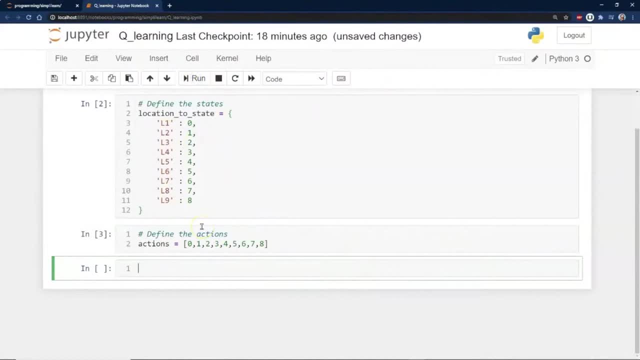 And if you remember, earlier I mentioned that the limitation is that you don't want to put in a continually growing table, Because you can actually create a dynamic queue table where you continually add in new values as they arise, Because if you have float values it just becomes infinite. 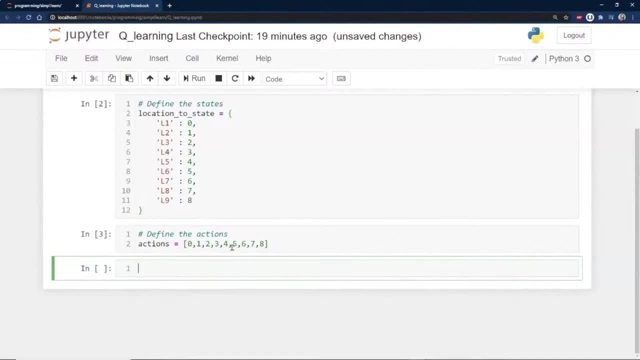 And then your memory in your computer is gone or it's not going to work At the same time you might think, well, that kind of really limits The queue learning setup, But there are ways to use it in conjunction with other systems. 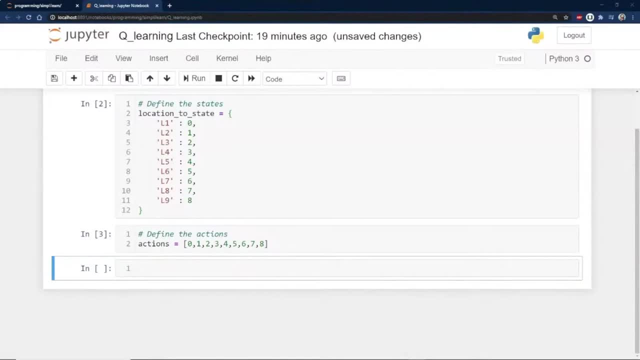 And so you might look at. well, I do. I've been doing some work in stock And one of the questions that comes out is to buy or sell the stock And the state coming in might be. you might take it and create what we call buckets. 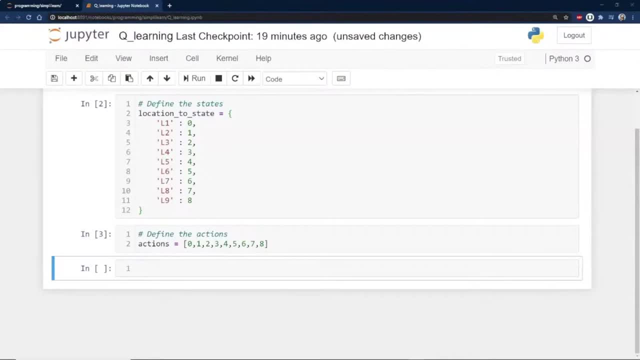 Where anything that you predict is going to return more than a certain amount of money- The error for that stock that you've had in the past. You put those in buckets And suddenly, as you start creating these buckets, you realize you do have a limited amount of information coming in. 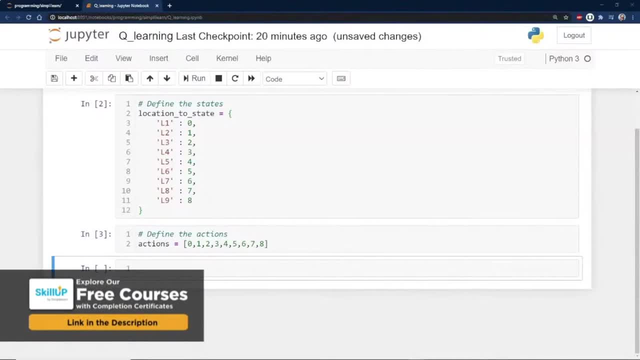 You no longer have a float number. You now have bucket 1,, 2,, 3, and 4.. And then you can take those buckets, Put them through a queue learning table And come up With the best action. Which stock should I buy? 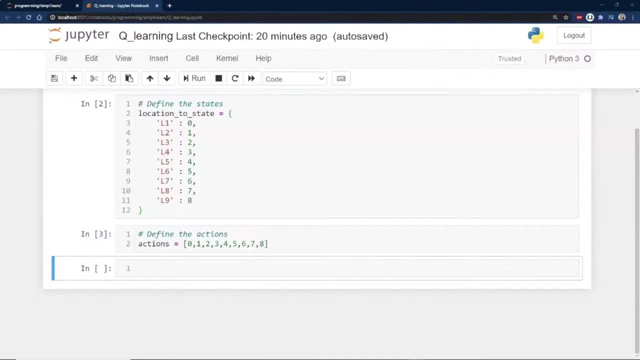 It's like gambling. Stock is pretty much gambling. If you're doing day trading, You're not doing long term investments, And so you can start looking at it like that. A lot of the current feeds say that the best algorithms used for day traders 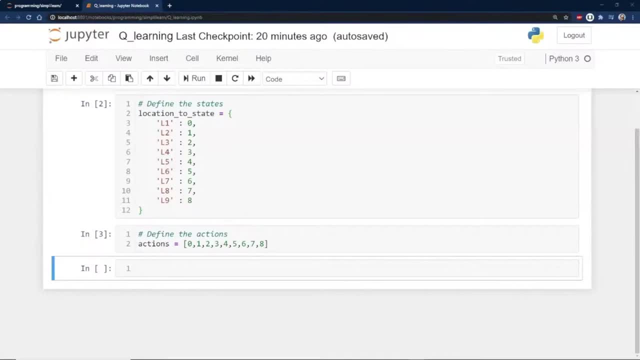 Where you're doing it on your own, Is really to ask the question: do I want to trade the stock, Yes or no? And now you have it in a queue learning table And now you can take it to that next level And you can see where that can be a really powerful tool. 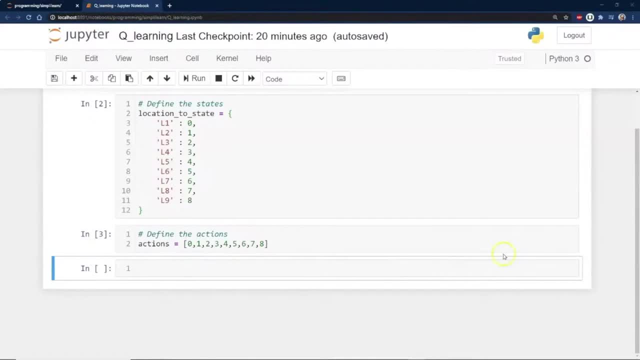 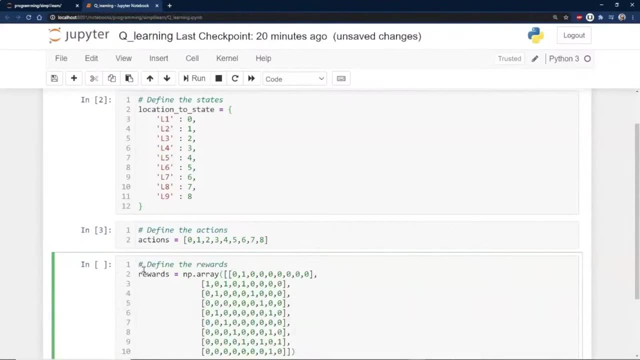 At the end of doing a basic linear regression model or something, What is the best investment? And you start getting the best reward on there. And so if we're going to have rewards, These rewards we just create. It says basically, if you're 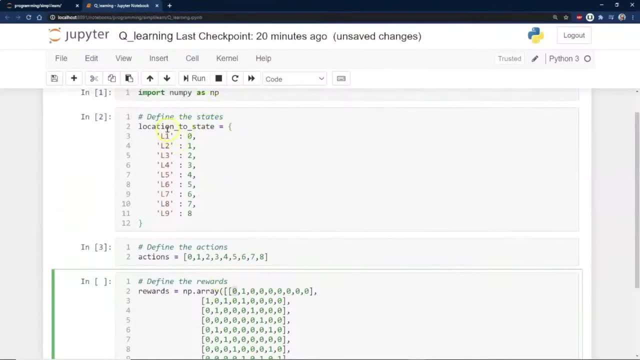 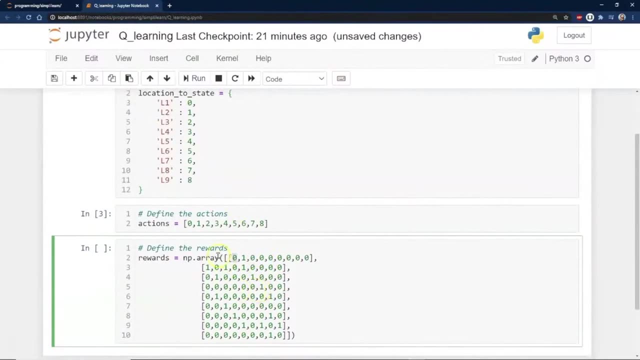 This should match our queue table, Because it's going to be: You have your state And you have your action across the top, If you remember, from the dog- And so we have whatever state we're in going down And then the next action. 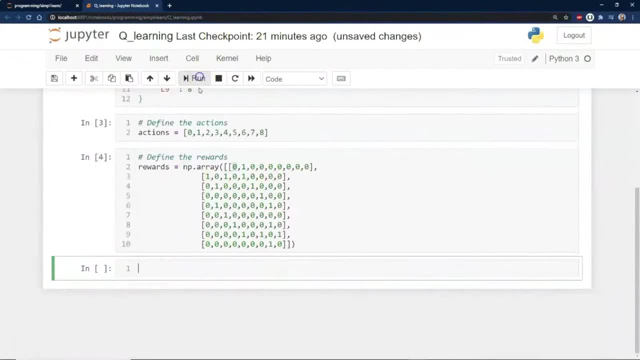 And what the reward is for it. And, of course, if you were actually doing something more connected, Your reward would be based on the actual environment it's in. And then we want to go ahead and create a state to location So we can map the indexes. 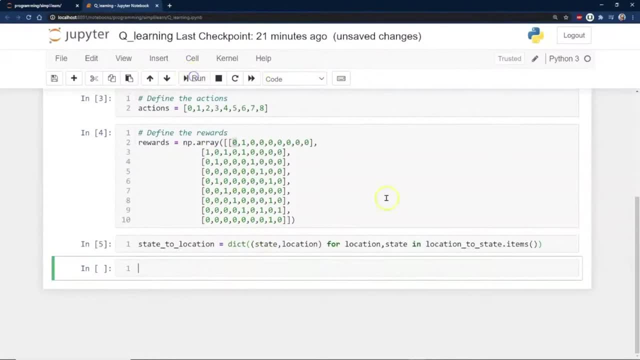 So, just like we defined our rewards, We're going to go ahead and do state to location And you can see here it's a dictionary setup For location, state and location to state with items. And we also need to define what we want for learning rates. 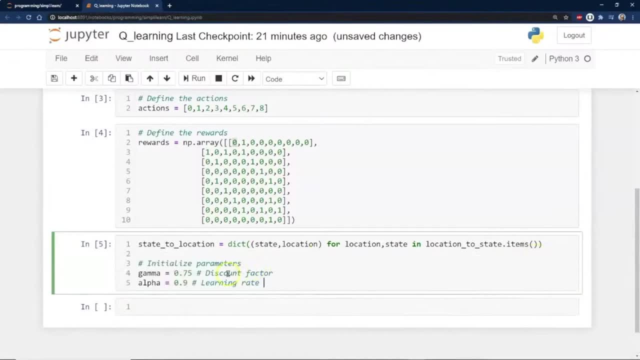 You remember we had our two different rates As far as like learning from the past And learning from the current. So we'll go ahead and set those to .75.. And the alpha set to .9.. And we'll see that when we do the formula. 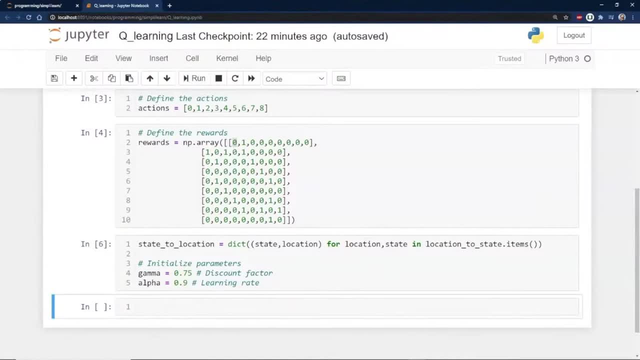 And, of course, any of this code. Send a note to our Simply Learn team. They'll get you a copy of this code On here And let's go ahead and pull. There we go The next two sections, Since we're going to keep it short and sweet. 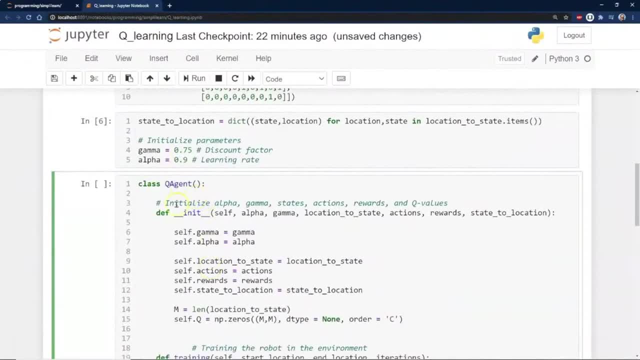 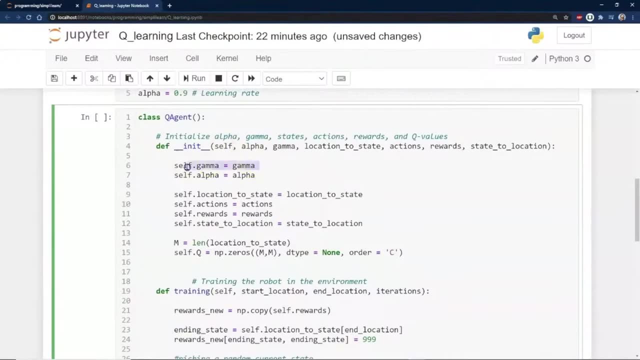 Here we go. So let's go ahead and create our agent. So our agent is going to have our initialization Where we send it all the information We'll define our self. gamma equals gamma. We could have just set the gamma rate down here. 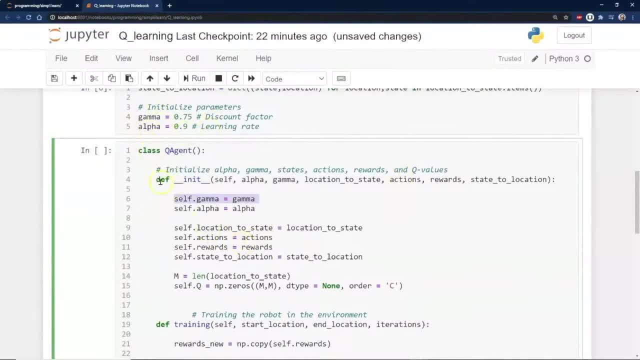 Instead of submitting it. It's kind of nice to keep them separate, Because you can play with these numbers, Our self alpha. Then we have our location state. We'll set that in here. We have our choice of actions. We're going to go ahead and just embed the rewards. 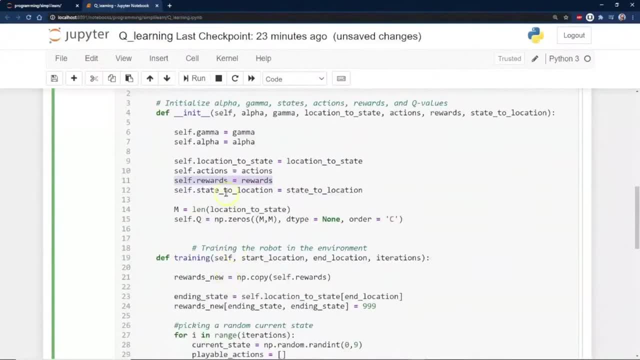 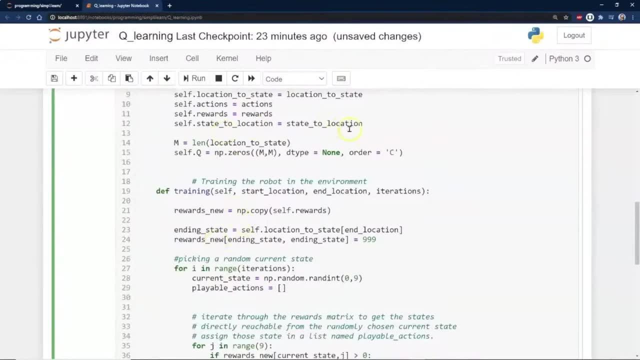 Right into the agent, So obviously this would be coming from somewhere else Instead of from self generated. And then a self state to location Equals our state to location dictionary, And we go ahead and create a queue learning table And I went ahead and just set the queue learning table up to 0 to 0.. 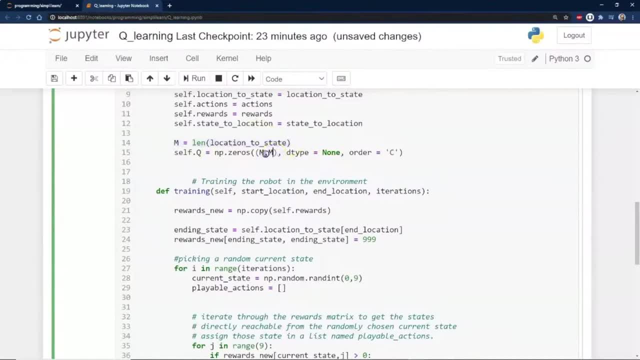 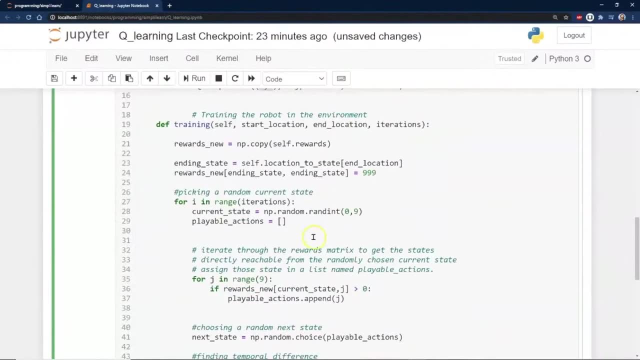 What the setup is, Location to state How many of them are there, And this just creates an array of 0 to 0 setup on there. And then the big part is the training. We have our rewards- new equals a copy of self dot rewards. 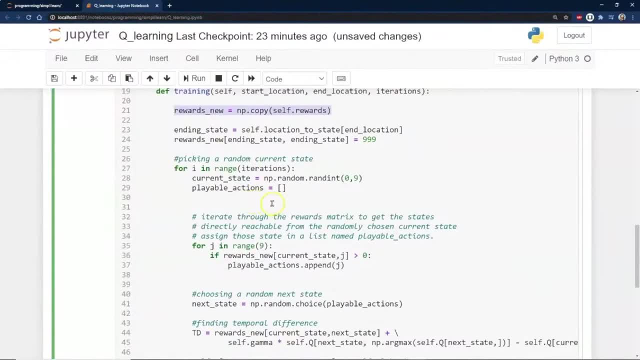 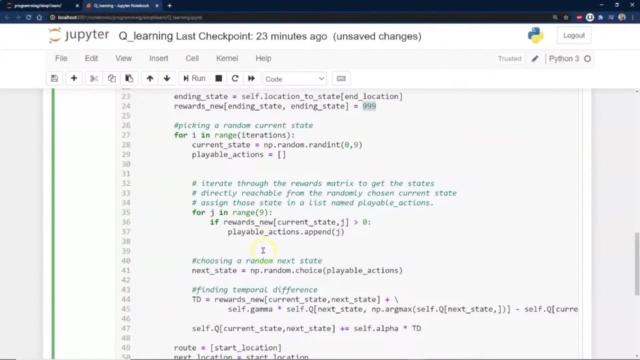 Ending state equals the self location state in location. So this is whatever we end up at: Rewards: new equals ending state plus ending state equals 999.. Just kind of goes to a dead end And we start going through iterations And we'll go ahead. 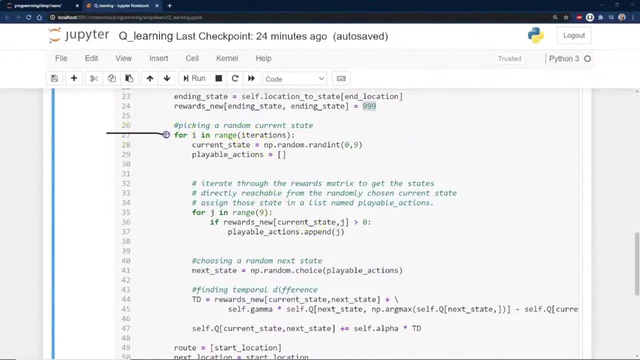 Let's do this. So this we're going to come back and we're going to call it on here. Let me just erase that. Switch it to an arrow. There we go. So what we're doing is We're going to send in here to train it. 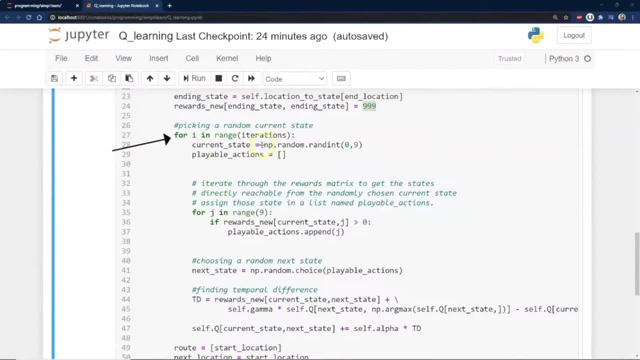 We're going to say, hey, I want to iterate through this a thousand times And see what happens. Now this part Would actually be: Instead of iterating, You might have your external environment And they're going back and forth And you iterate through. 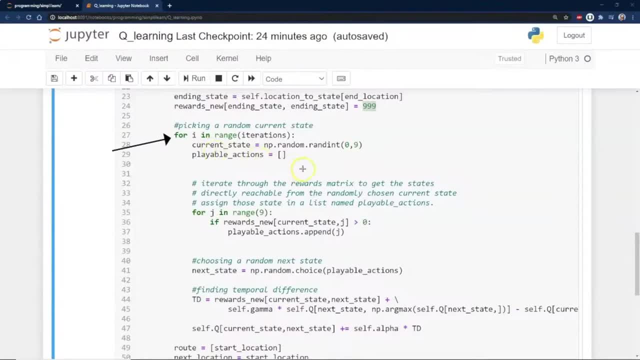 Outside of here, But just for ease of use. Our agent is going to come in here And iterate through this Sometimes. I'll put this iteration in here And I'll have it call the environment And say, hey, This is what I did. 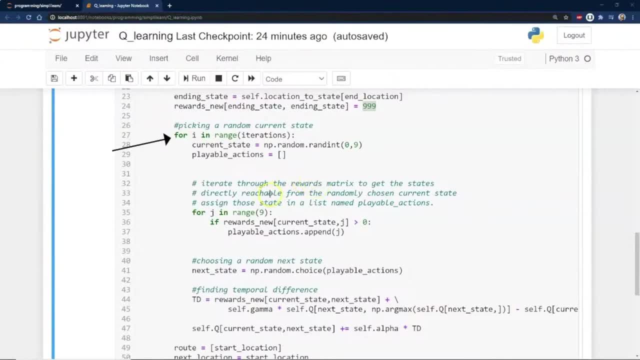 What's the next state? And the environment Does this thing right in here As I iterate through it. And then we want to go ahead And pick a random state To start with. That's what's going on here. You have to start somewhere. 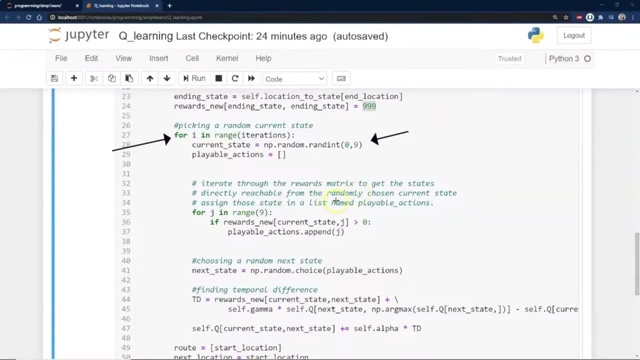 And then you have Your playable actions. We're going to start with just An empty thing for playable actions And we'll fill that up. So that's what choices I have, And so we're going to iterate through the rewards matrix. 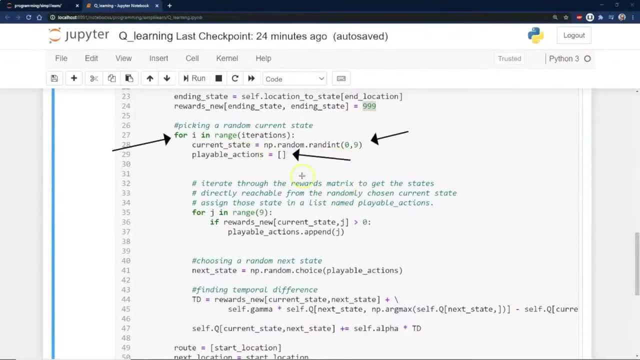 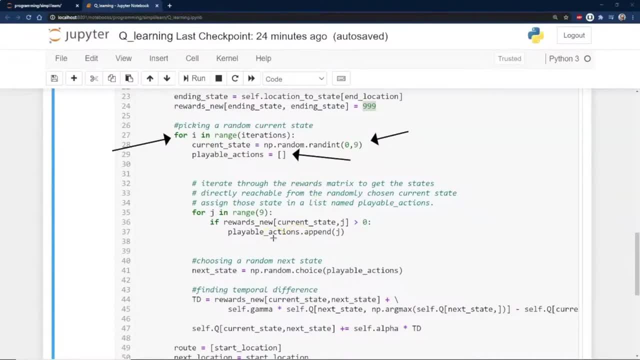 And so we're going to iterate through the rewards matrix To get the states Directly reachable from the randomly chosen current state, Assign those states to a list Named playable actions, And so you can see, here We have range nine. I usually use lengths of whatever I'm looking at. 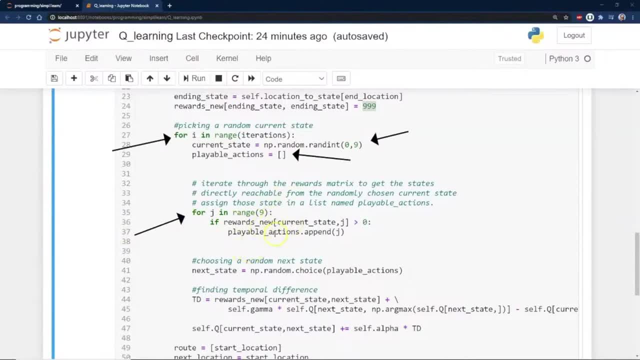 Which is our locations Or states as they are. We have a reward. So we want to look at the current The rewards. The new reward Is our, Is our Is in our chart here of rewards. underscore new, Current state. 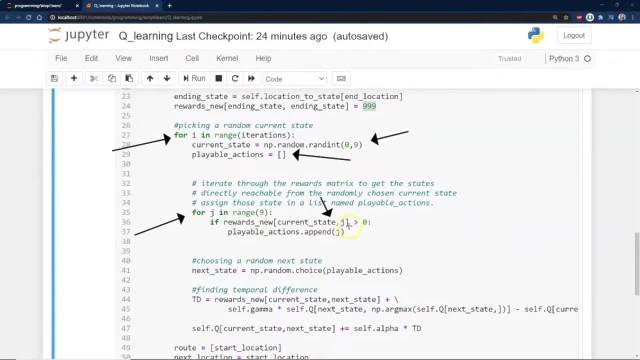 Plus j, J being what is the next date? we want to try, And so we go ahead and do our playable actions And we append j, And so we're doing is we're randomly Trying different things in here to see What's going to generate a better reward. 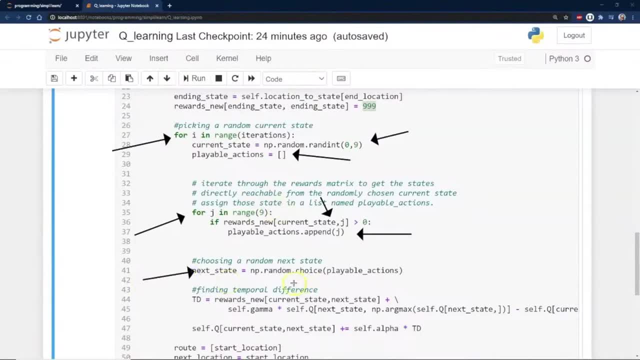 And then, of course, we go ahead And choose our next state. So we have a random choice, playable actions And if you remember I mentioned on this, let me just go ahead and whoops, let's do a free form When we were talking about the next state. this right here just does a random selection. 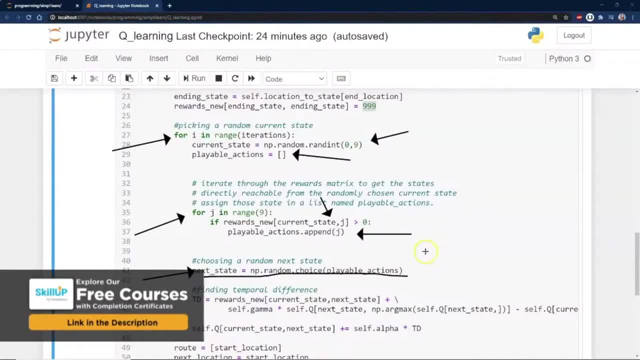 Instead of a random selection, you might do something where, whatever the best selection is, which might be option 3 here and then, so you can see that it might use a bell curve, and then option 2 over here might have a bell curve like this, and we start looking at these. 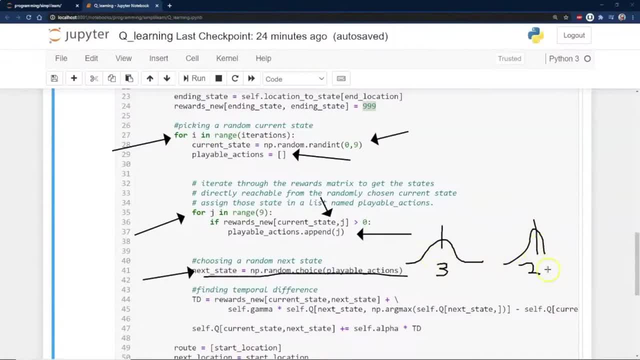 averages and these spreads, or we can just add them all together and pick the one that kind of goes in all of those. So those are some of the options we have in here. We just go with a random choice. That's usually where you start to play with it, and then we have our reward section down. 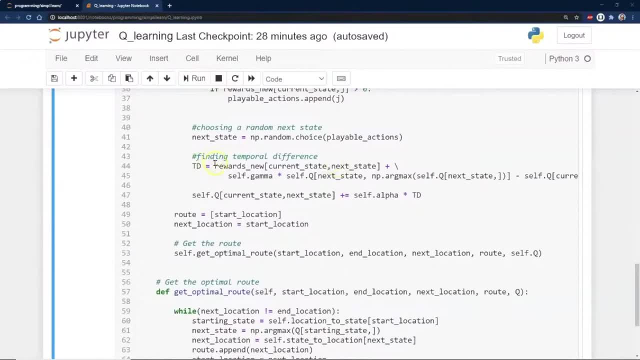 here, and so we want to go ahead and find- well, in this case, a temporal difference. So you have your rewards new, plus the self gamma, and this is the formula we were looking at. This is Bellman's equation here. So we have our current value, our learning rate, our discount rate involved in 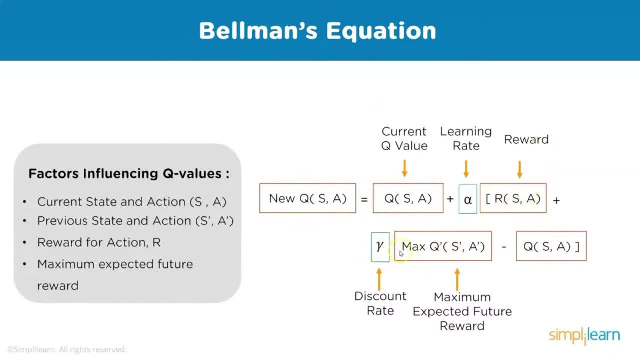 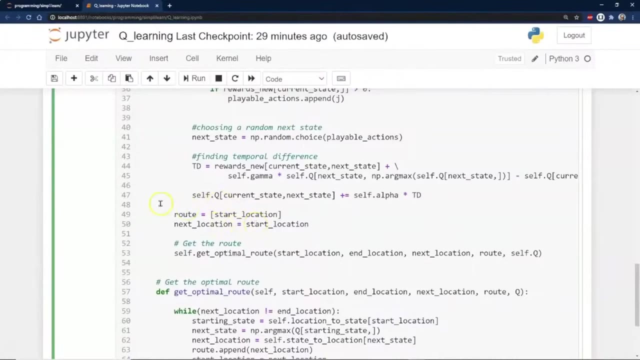 there, the reward system coming in for that, and we can add it all together. This is, of course, our maximum expected future set up in here. So this is all of our Bellman's equation that we're looking at here, and then we come up in here and we update our Q table. 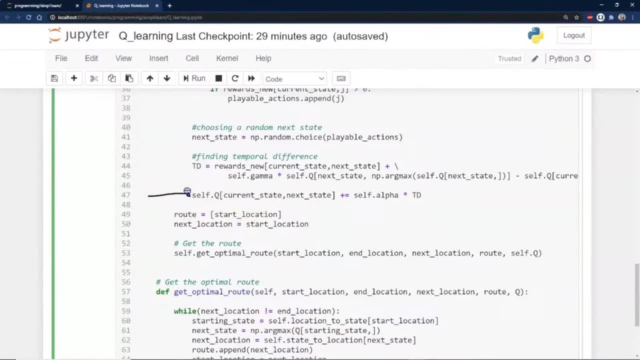 That's all. this is on this one. That's right. here We have self Q, current state, next state, and we add in our alpha- because we don't want to train all of it at once, in case there's slight differences coming in there. We want to slowly approach the answer and then we have our route. 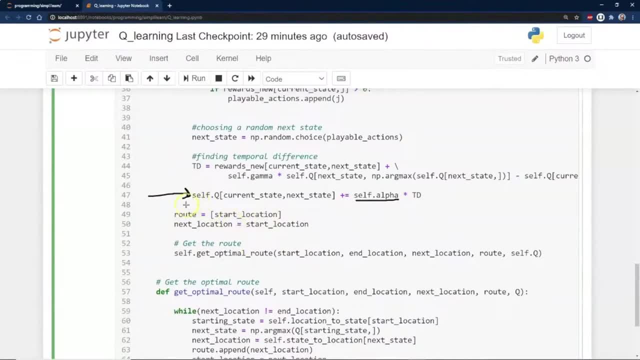 equals the start location and next location equals start location. So we're just incrementing. We took a step forward and then finally remember I was telling you how we're going to do all this and just have some simple thing at the end or just generates a simple path We're going. 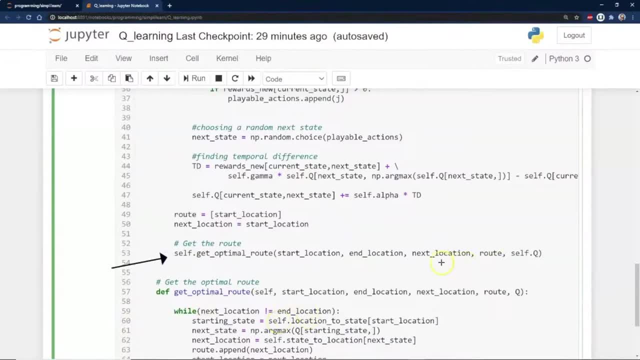 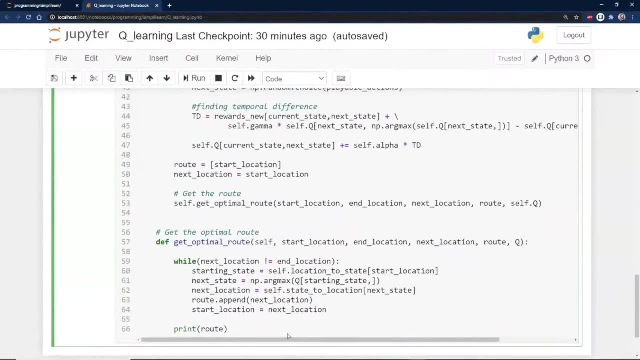 to go ahead and get the optimal route. We want to find the best route in here, and so we've created a definition for the optimal route down here. Just scroll down for that and we get the optimal route. We go ahead and put the information in, including the Q table: self start location in location. 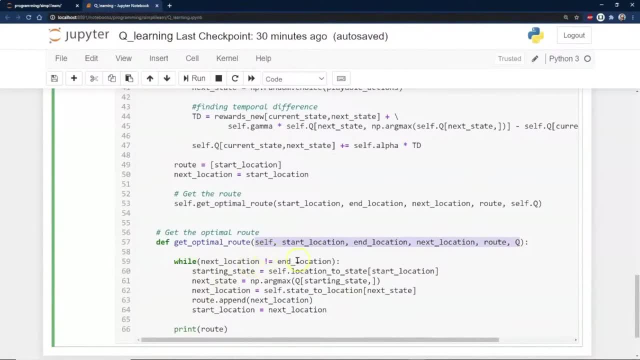 next location, route Q, and it says: while next location is not equal to in location, so while we go, our start location equals self location to state start location. So we already have our best value for the start location. The next state looks at the Q table and says hey, what's the next one? 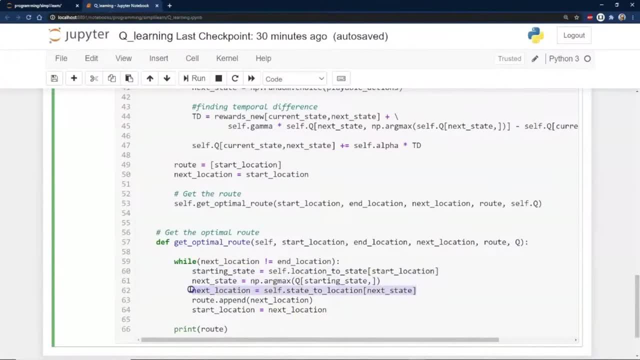 with the best value, And then the next location. we go ahead and pull that in and we just append it. That's what's going on down here, and then our start location equals the next location and we just go through all the steps and we'll go ahead and run this. and now that we have our 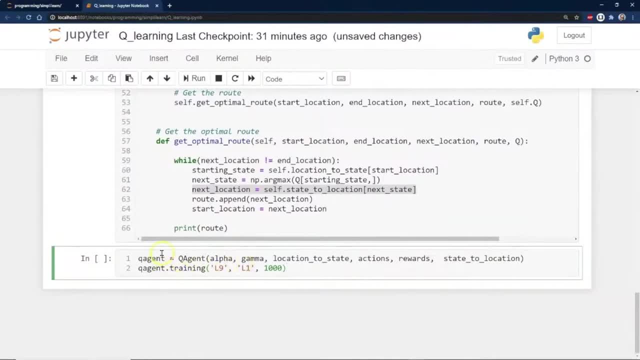 Q table, our Q agent loaded, we're going to go ahead and take our Q agent, load them up with our alpha gamma that we set up above, along with the location, step, action, reward, state to location, and our goal is to plot a course between L9 and L1, and we're going to go through a thousand. 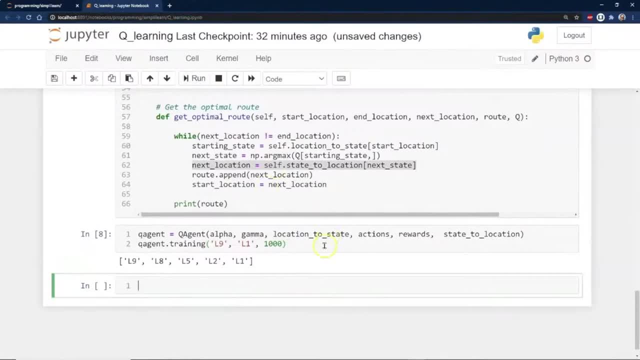 iterations on here, And so when I run that, it runs pretty quick. Why is this so fast? If you've been running neural networks and you've been doing all these other models, you sit here and wait a long time. Well, we're a very small amount of data. These are all integers. These 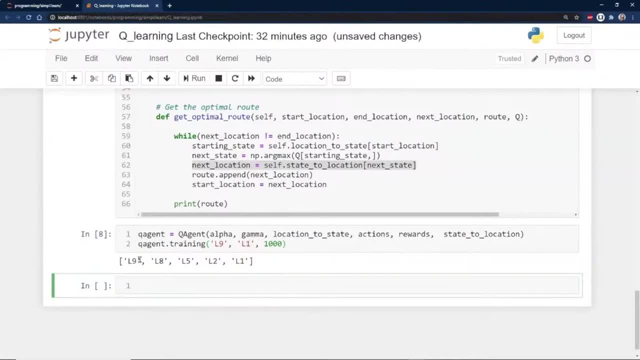 aren't float values. The math is not heavy on the processing end, and this is where Q tables are so powerful. If you have a small amount of information coming in, you very quickly get an answer off of this, even though we went through it a thousand times to train it and you'll see here. 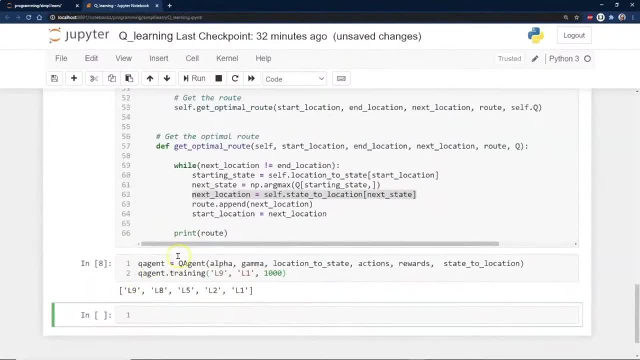 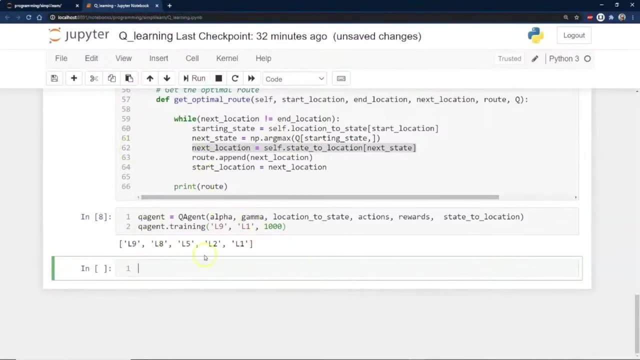 we have L9,, 8,, 5,, 2, and 1.. And that's based on our reward table we had set up on there and this is the shortest path going between these different setups in here. And if you remember on our reward table you can see that. if 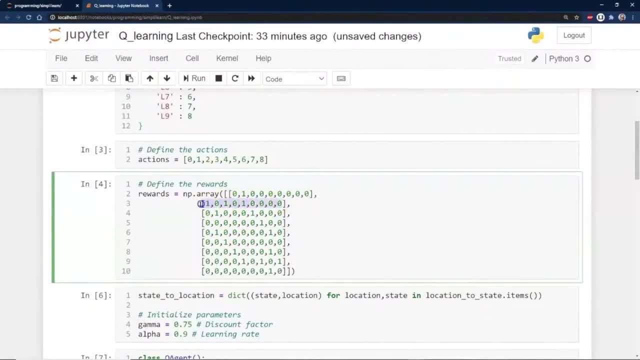 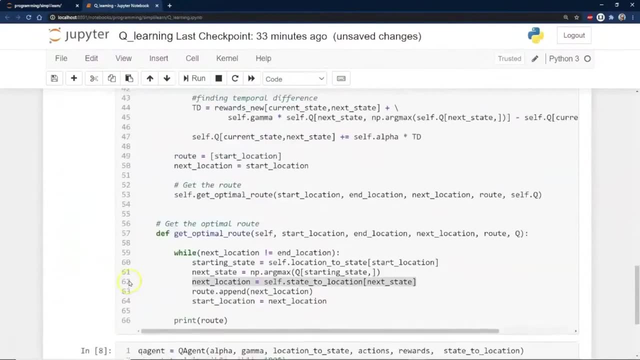 you start here, you can go to here. There's places you can't go. That's how this reward table was set up, so I can only go to certain places. So kind of a little maze setup in there and you can play. 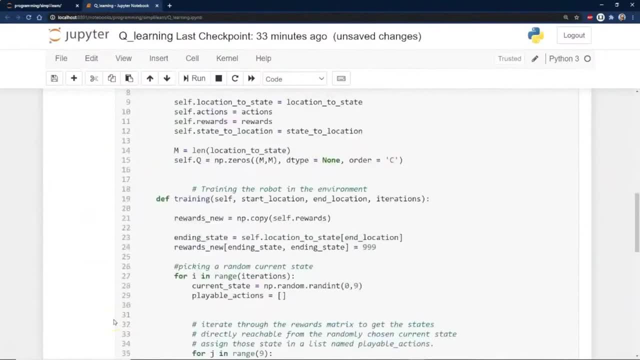 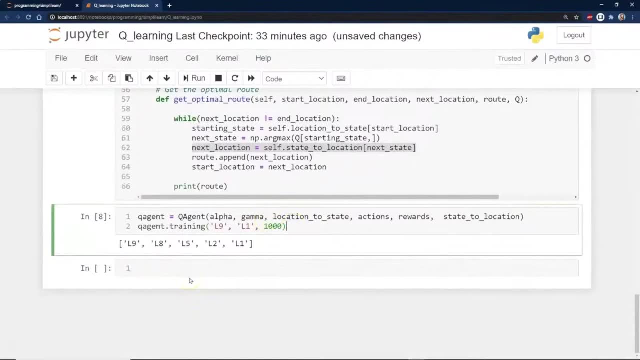 with it. This is a really fun setup to play with and you can play with that. You can see how you can take this whole code and you can, like I was saying earlier, you can embed it into another setup in model and predictions, where you put things into buckets and you're trying to. 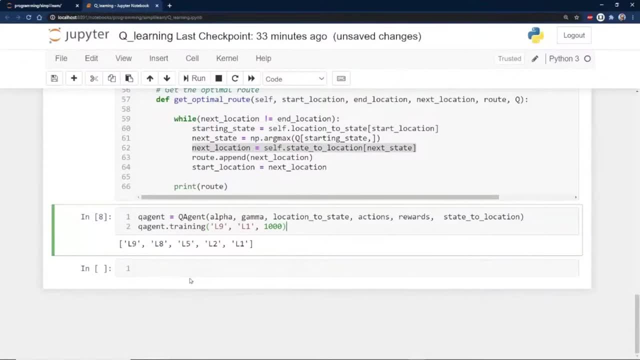 guess the best investment, the best course of action, as long as you can take that course of action and reduce it down to a yes-no. Or, if you're using text, you can use a one-hot encoder: which word is next? There's all kinds of things you can do with a Q table, depending on just how. 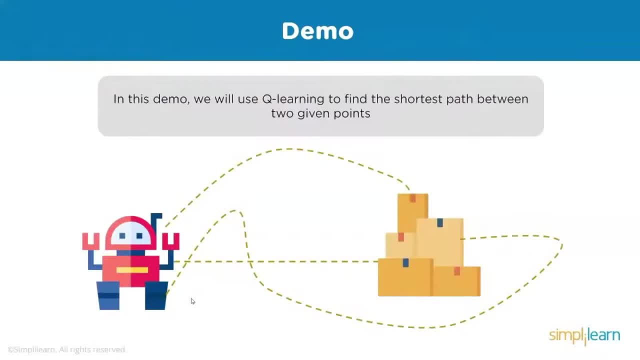 much information you're putting in there. So that wraps up our demo. In this demo we've found the shortest distance between two paths, based on whatever rules or state rewards we have to get from point A to point B and what available actions there are. Hello and welcome to this tutorial on. 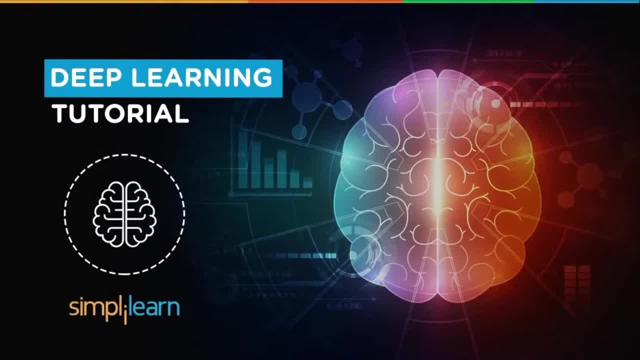 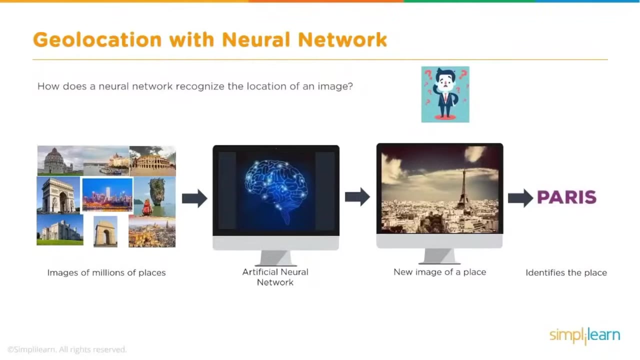 deep learning. My name is Mohan and in the next about one one and a half hours I will take you through what is deep learning and into TensorFlow environment to show you an example of deep learning. Now there are several applications of deep learning, really very interesting and innovative. 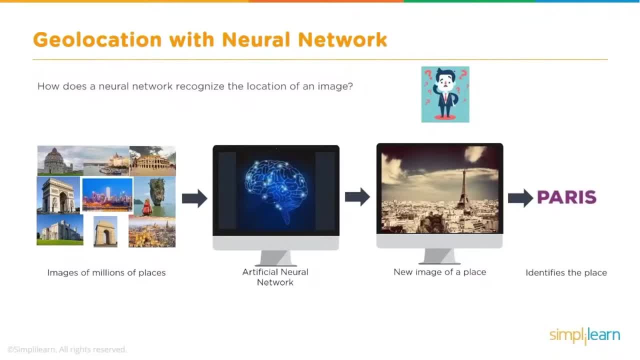 applications, And one of them is identifying the geographic location based on a picture. And how does this work? The way it works is pretty much: we train an artificial neural network with millions of images which are tagged. Their geolocation is tagged and then, when we feed a new picture, it will. 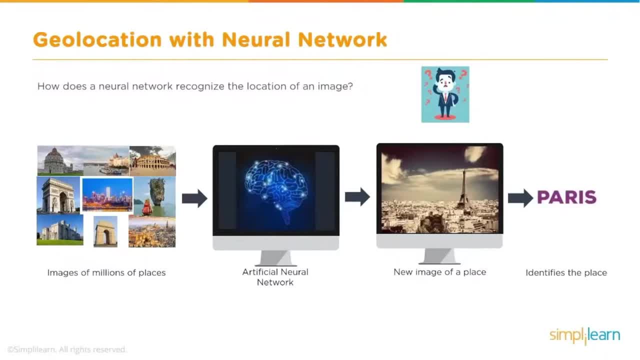 be able to identify that geolocation of this picture, new image, For example. you have all these images, especially with maybe some significant monuments or significant locations, and you train with millions of such images and then when you feed another image, it need not be exactly one of those that you have trained, It can be completely. 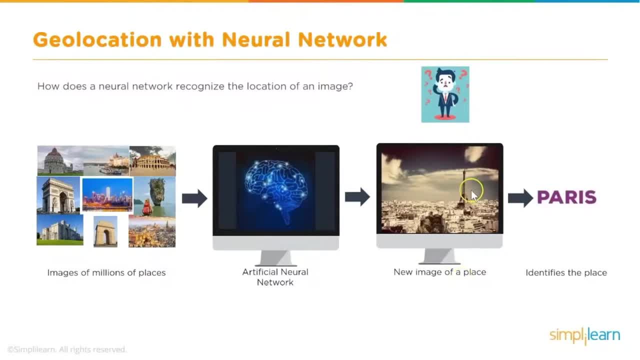 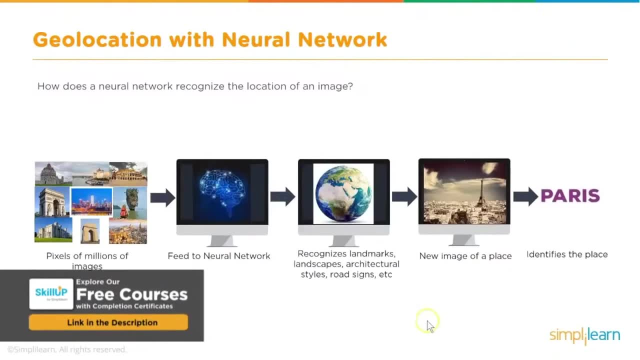 different. That is the whole idea of training. It will be able to recognize, for example, that this is a picture from Paris because it is able to recognize the Eiffel Tower. So the way it works internally, if we have to look a little bit under the hood, is: these images are nothing, but this is. 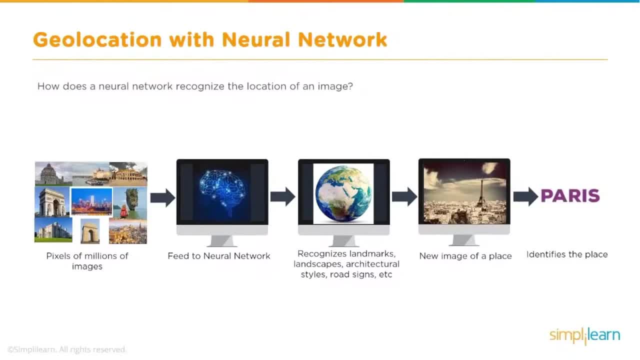 digital information in the form of pixels, So each image could be a certain size. It can be 256 by 256 pixel kind of a resolution, and then each pixel is either having a certain grade of color and although it is a picture from Paris, it is able to recognize the Eiffel Tower. So it can be. 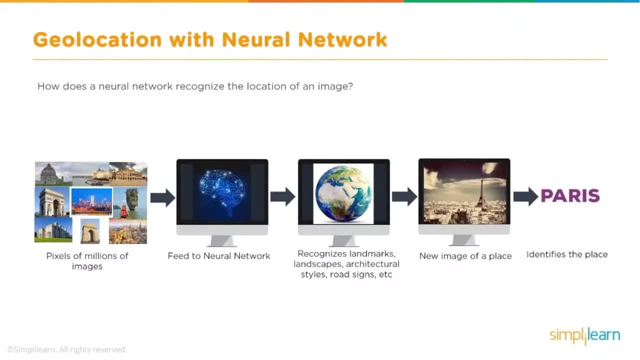 All that is fed into the neural network and it then gets trained and it's able to, based on these pixels, pixel information, it is able to get trained and able to recognize the features and extract the features, and thereby it is able to identify these images and the location of these images. 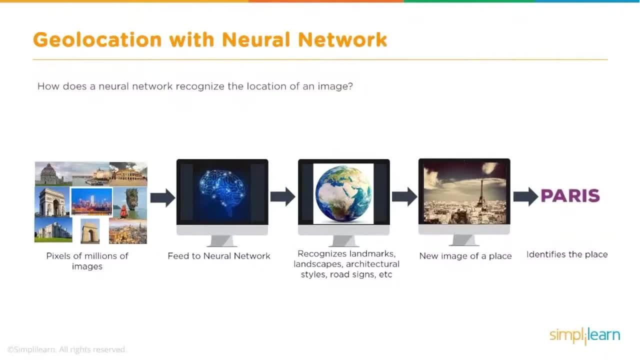 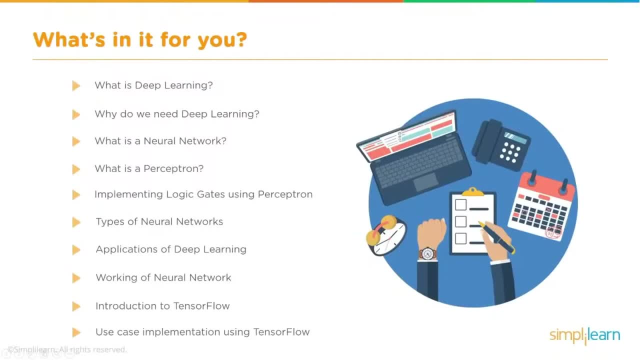 And then when you feed a new image, it kind of based on the training, it will be able to figure out where this image is from. So that's the way, a little bit under the hood, how it works. So what are we going to do in this tutorial? 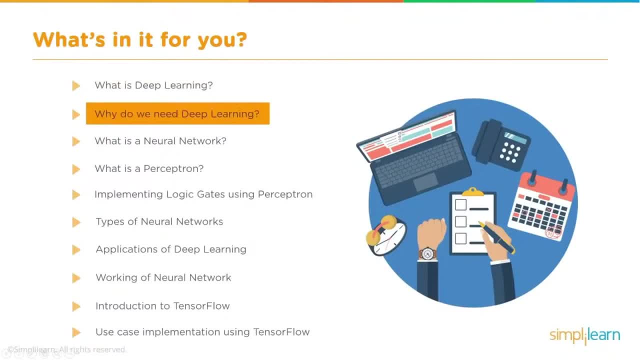 We will see what is deep learning and what do we need for deep learning, And one of the main components of deep learning is neural networks. So we will see what is neural network, what is a perceptron and how to implement logic gates like AND, OR, NOR, and so on. 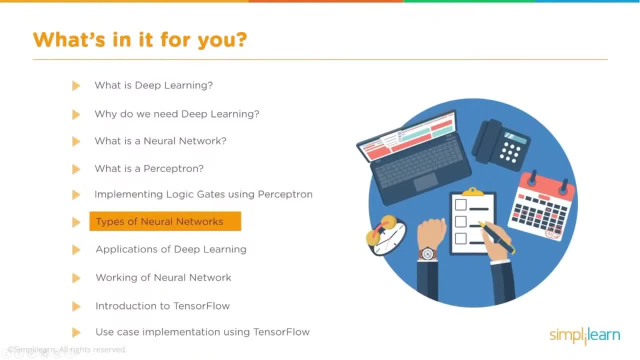 Using perceptrons, the different types of neural networks, and then applications of deep learning, And we will also see how neural networks works. So, how do we do the training of neural networks? And at the end, we will end up with a small demo code which will take you through intensive flow. 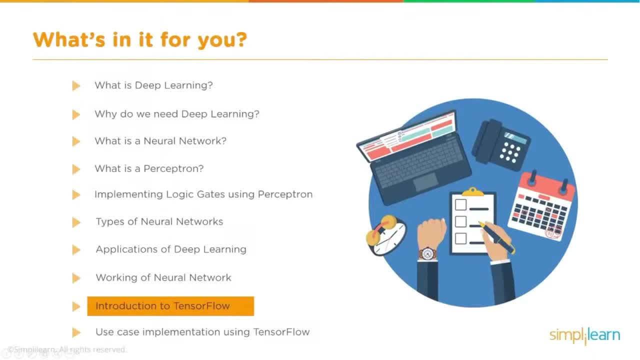 Now, in order to implement deep learning code, there are multiple libraries or development environments that are available, And Tensive flow is one of them. So the focus at the end of this would be on how to use TensorFlow to write a piece of code using Python as a programming language. 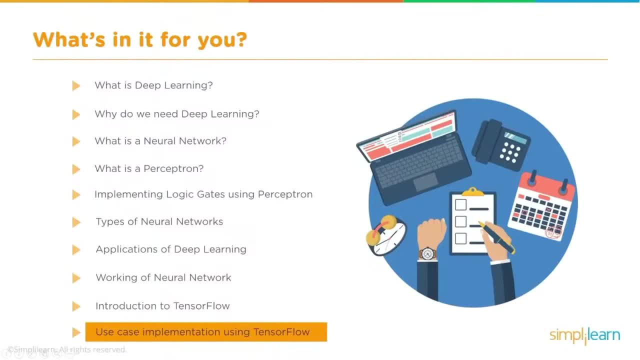 And we will take up an example which is a very common one, which is like the hello world of deep learning: the handwriting number recognition, which is a MNIST commonly known as MNIST database. So we will take a look at MNIST database and how we can train a neural network to recognize hand recognition. 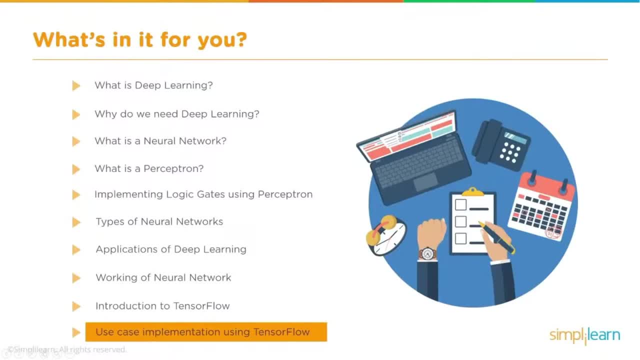 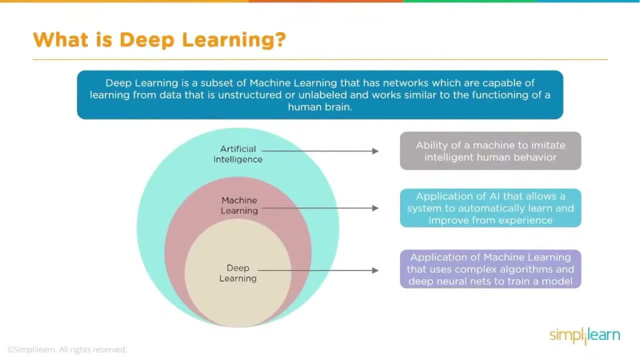 So we will take a look at MNIST database and how we can train a neural network to recognize MNIST database. So that's what you will see in this particular video. So let's get started. What is deep learning? Deep learning is like a subset of what is known as a high level concept called artificial intelligence. 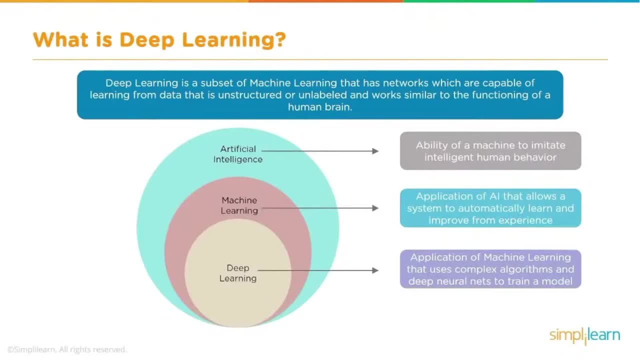 You must be already familiar, must have heard about this term, artificial intelligence. So artificial intelligence is like the high level concept, if you will, And in order to implement artificial intelligence applications, we use what is known as machine learning and, within machine learning, a subset of machine. 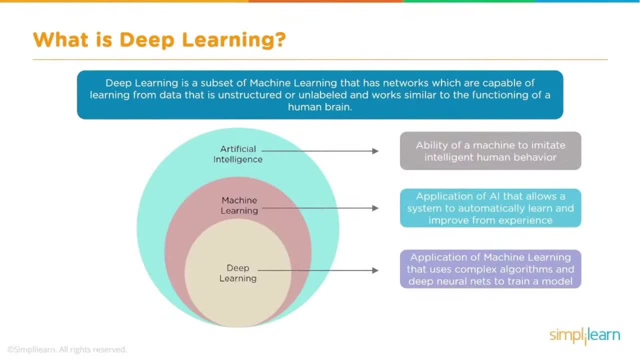 learning is deep learning. Machine learning is a little bit more generic concept and deep learning is one type of machine learning. if you will- and we will see a little later in maybe the following slides, a little bit more in detail how deep learning is different from traditional machine- 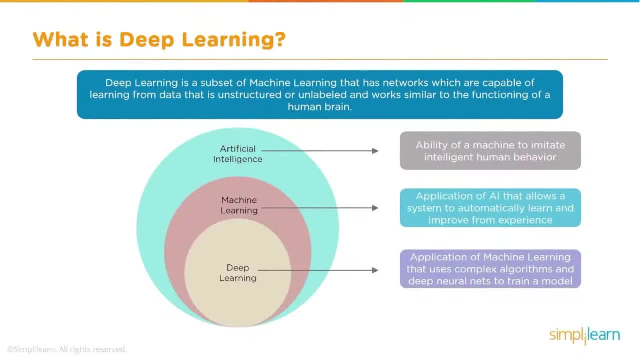 learning. But to start with, we can mention here that deep learning uses. one of the differentiators between deep learning and traditional machine learning is that deep learning uses neural networks, and we will talk about what are neural networks and how we can implement neural networks, and so on and so forth as a part of this tutorial. So a little deeper into deep learning- Deep 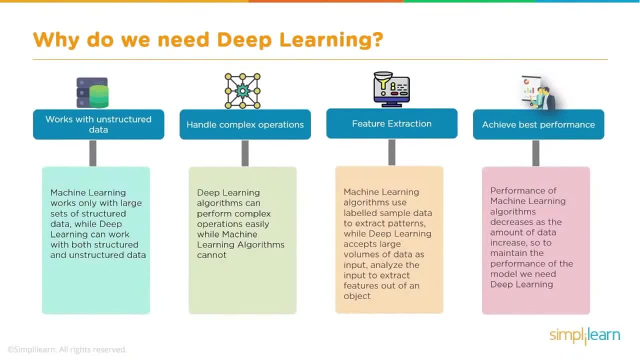 learning primarily involves working with complicated, unstructured data, compared to traditional machine learning, with where we normally use machine learning. So deep learning is a type of machine learning where we normally use structured data. In deep learning the data would be primarily images or voice or maybe text file, So and it is large amount of data. 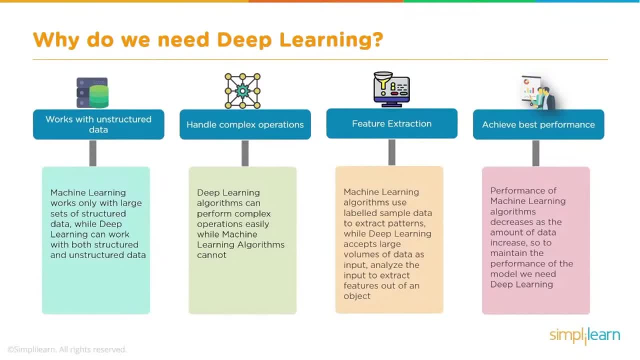 as well, and deep learning can handle complex operations. It involves complex operations and the other difference between traditional machine learning and deep learning is that the feature extraction happens pretty much automatically. In traditional machine learning, feature engineering is done manually. The data scientists, we data scientists, we data. 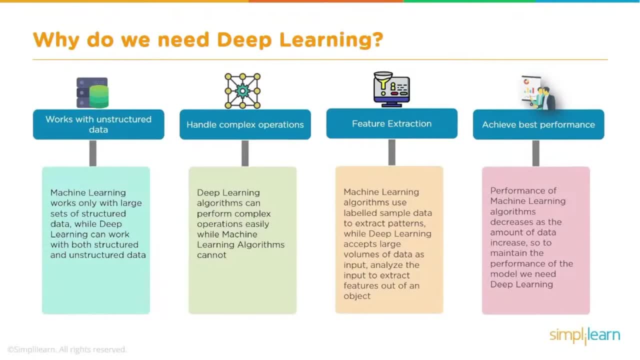 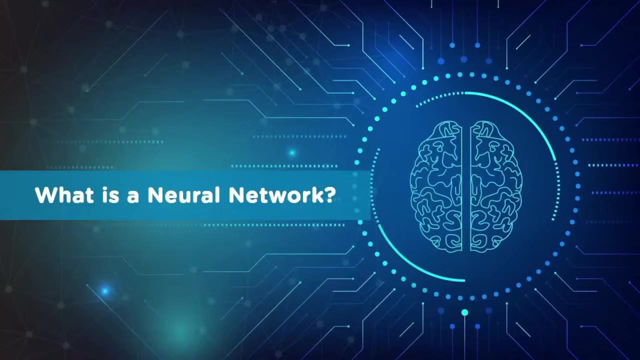 scientists have to do feature engineering, feature extraction, But in deep learning that happens automatically. And, of course, in deep learning for large amounts of data, complicated, unstructured data, deep learning gives very good performance. Now, as I mentioned, one of the secret sources of deep learning is neural networks. Let's 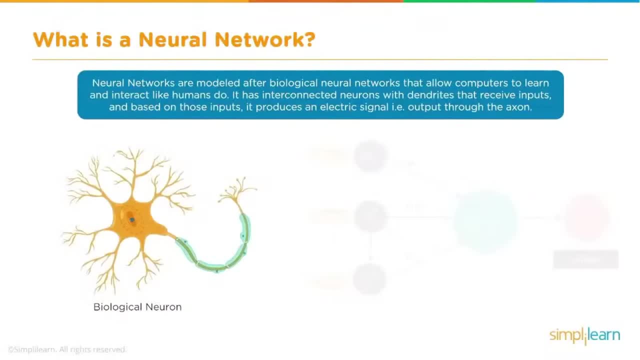 see what neural networks is. Neural networks is based on our biological neurons. The whole concept of deep learning and artificial intelligence is based on human brain, and human brain consists of billions of tiny stuff called neurons, and this is how a biological neuron looks and this is how an artificial neuron looks. so neural networks is like a simulation of 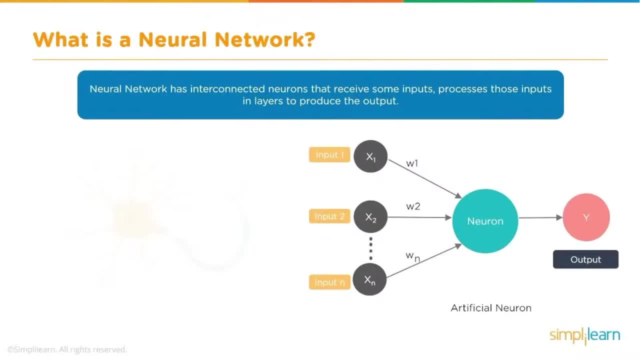 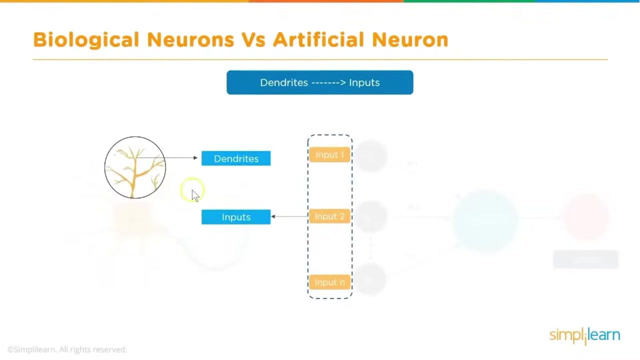 our human brain. human brain has billions of biological neurons and we are trying to simulate the human brain using artificial neurons. this is how a biological neuron looks: it has dendrites and the corresponding component with an artificial neural network is or an artificial neuron are the inputs they receive, the inputs through dendrites, and then there is the cell nucleus. 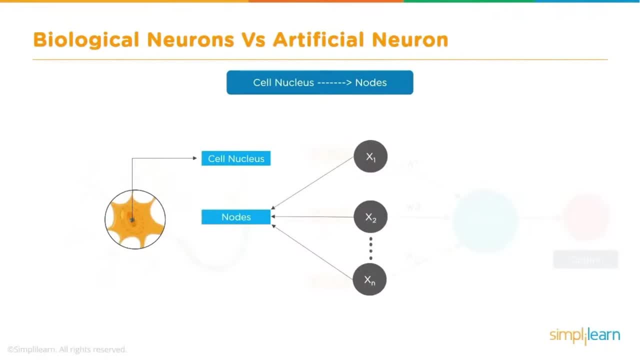 which is basically the processing system, which is basically like intercomputing cell, cell cells unit in a way. So in artificial neuron also, there is a piece which is an equivalent of this cell nucleus and, based on the weights and biases, we will see what exactly weights and biases are. 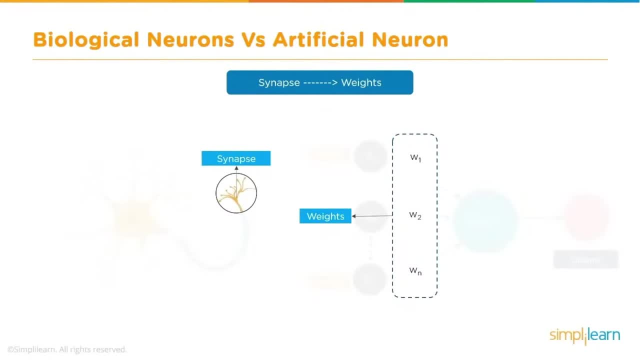 as we move, The input gets processed and that results in an output In a biological neuron. the output is sent through a synapse and in an artificial neuron there is an equivalent of that in the form of an output, and biological neurons are also interconnected. So there are billions of 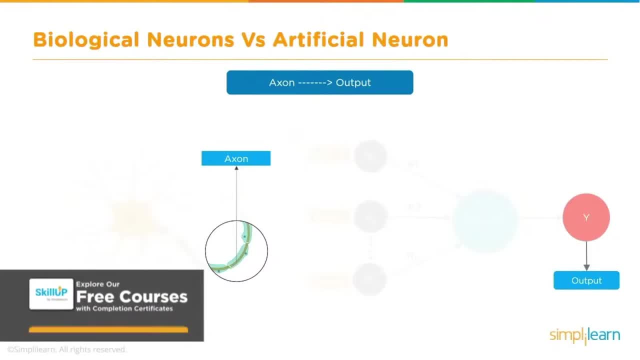 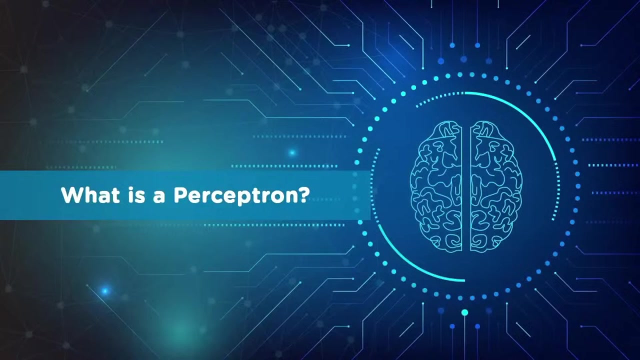 neurons which are interconnected. in the same way, artificial neurons are also interconnected, So this output of this neuron will be fed as an input to another neuron, and so on. Now in neural network, one of the very basic units is a perceptron. So what is a perceptron? A perceptron can be considered. 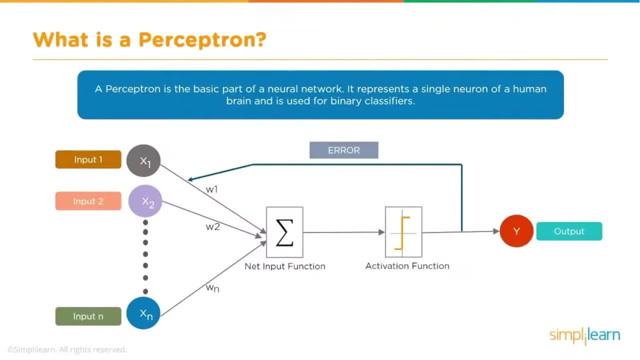 as one of the fundamental units of neural network. It can consist at least one neuron, but sometimes it can be more than one neuron. but you can create a perceptron with a single neuron and it can be used to perform certain functions. It can be used as a. 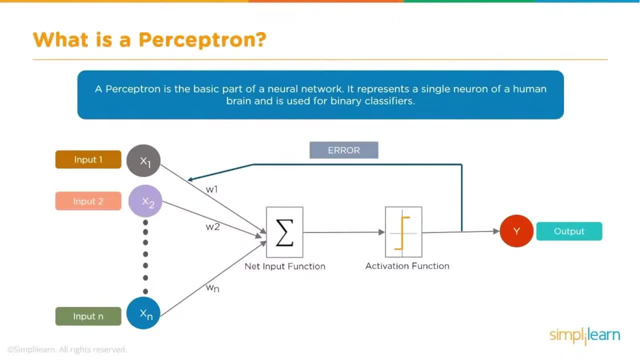 basic binary classifier. It can be trained to do some basic binary classification. and this is how a basic perceptron looks like, and this is nothing but a neuron. You have inputs x1,, x2, xn and there is a summation function and then there is what is known as an activation function, and based on this, 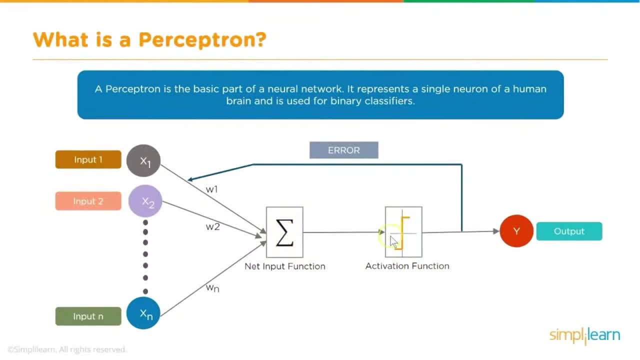 input, what is known as the weighted sum. the activation function either gets, gives an output like a 0 or a 1. so we say the neuron is either activated or not. so that's the way it works. So you know these inputs are. each of the inputs are multiplied by a weight and there is a bias that 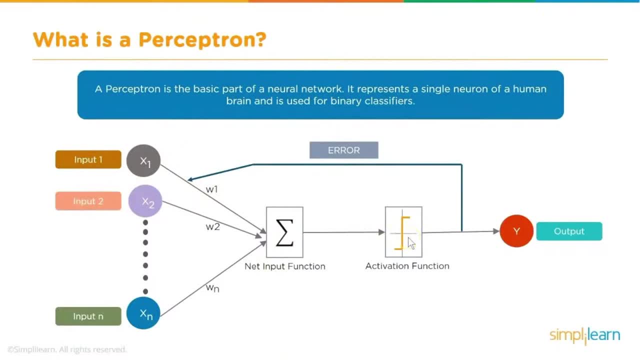 gets added and that whole thing is fed to an activation function and then that results in an output and if the output is correct, it is accepted. if it is wrong, if there is an error, then that error is fed back and the neuron then adjusts the weights and biases to give a new output, and so on. 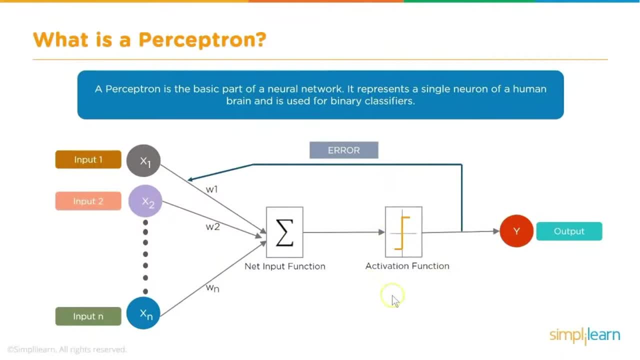 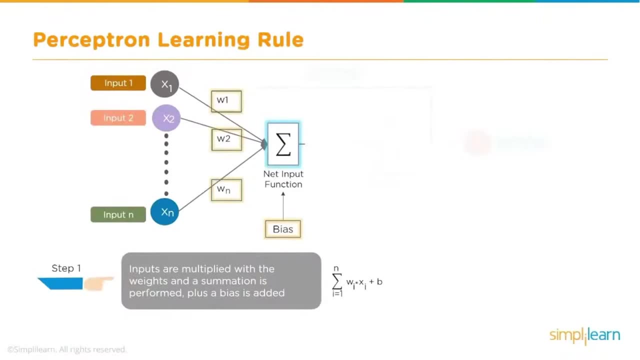 and so forth. So that's what is known as the training process of a neuron or a neural network. There's a concept called perceptron learning. So perceptron learning is again one of the very basic learning processes. The way it works is somewhat like this. so you have all these inputs like x1 to 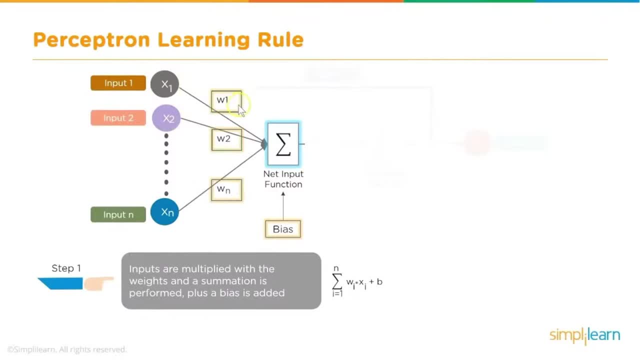 xn, and each of these inputs is multiplied by a weight, and then that sum- this is the formula or the equation- so that's sum wi, xi sigma of that, which is the sum of all these product of x and w, is added up, and then a bias is added to that. The bias is not dependent on the input, but or the input values, but the bias. 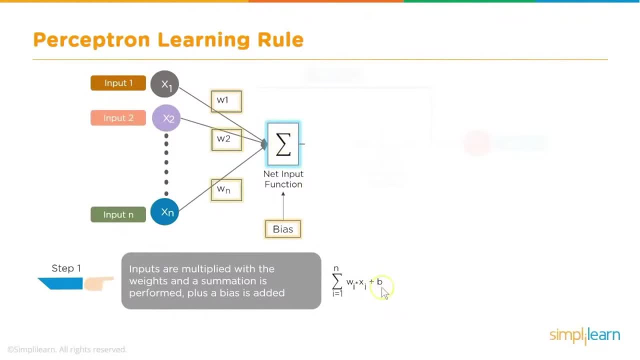 is common for one neuron. However, the bias value keeps changing during the training process. Once the training is completed, the values of these weights- w1, w2 and so on- and the value of the bias gets fixed. So that is basically the whole training process and that is what is known as. 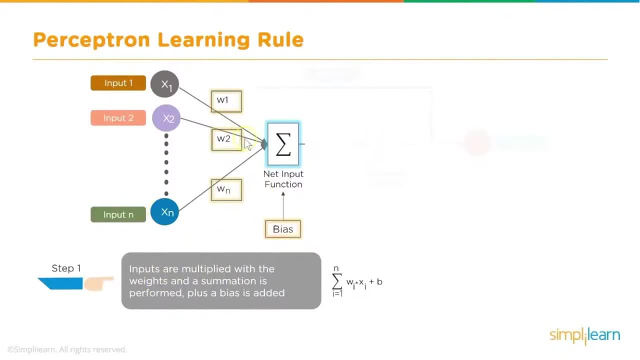 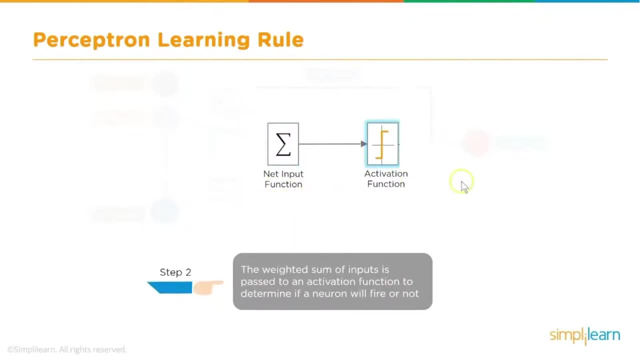 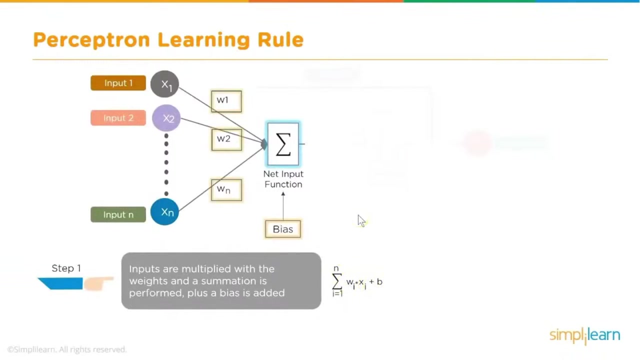 the perceptron training, So the weights and biases keep changing till you get the accurate output and the summation is of course passed through the activation function. As you see here, this wixi summation plus b is passed through activation function and then the neuron gets either fired: 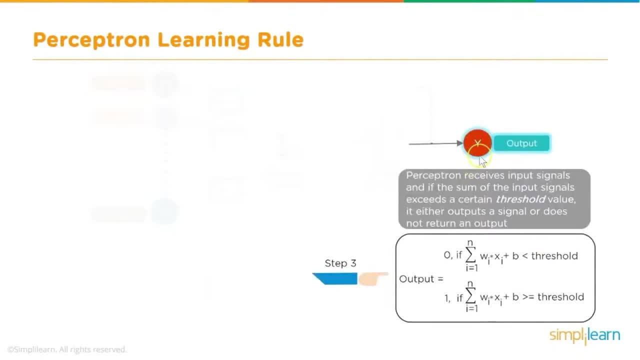 or not, and based on that there will be an output. That output is compared with the actual or expected weight, The value which is also known as labeled information. This is the process of supervised learning. So the output is already known and that is compared and thereby we know if there. 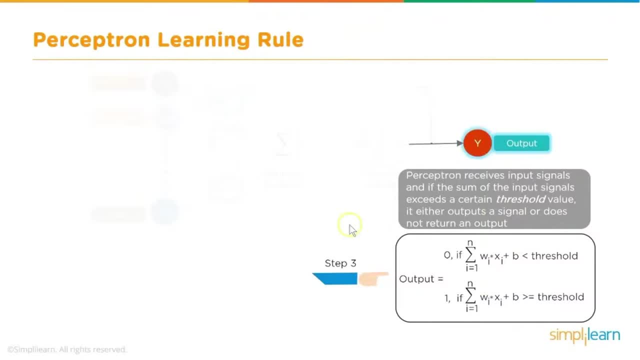 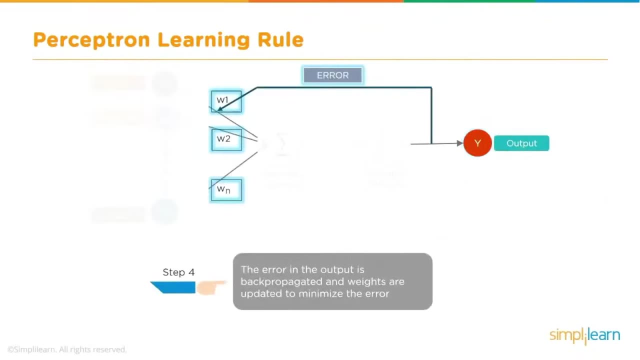 is an error or not. And if there is an error, the error is fed back and the weights and biases are updated accordingly. till the error is reduced to the minimum. So this iterative process is known as perceptron learning or perceptron learning rules, and this error needs to be minimized. so, till the error is minimized, this iteratively, the weights 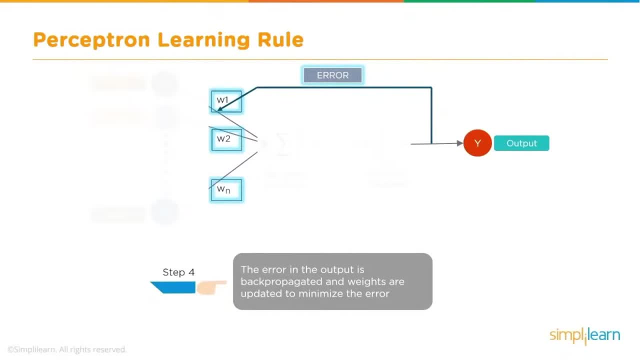 and biases keep changing, and that is what is the training process. so the whole idea is to update the weights and the bias of the perceptron till the error is minimized. the error need not be zero, the error may not ever reach zero, but the idea is to keep changing these weights and bias so that 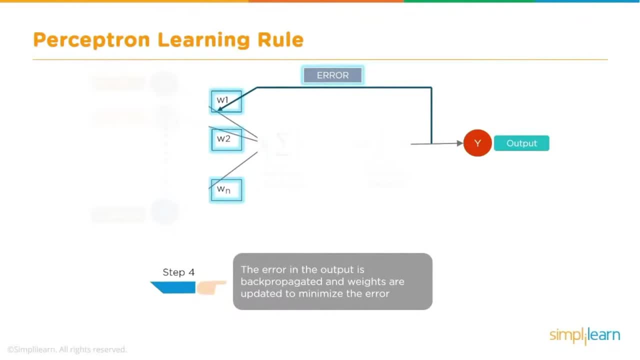 the error is minimum, the minimum possible that it can have. so this whole process is an iterative process, and this is the iteration continues till: either the error is zero, which is unlikely situation, or it is the minimum possible within these given conditions. now, in 1943, two scientists, 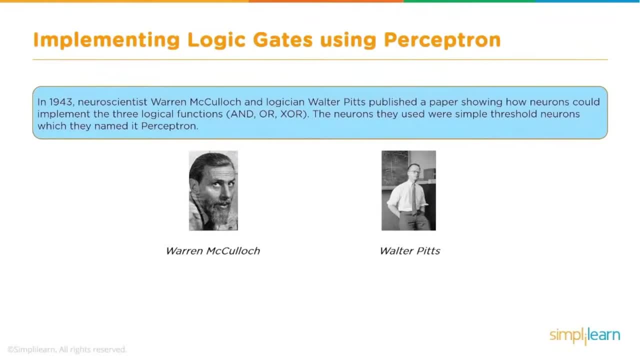 together, Warren McCulloch and Walter Pitts came up with an experiment where they were able to implement the logical functions like AND, OR AND NOR, using neurons, and that was a significant breakthrough in a sense. So they were able to come up with the most common logical gates. They were: 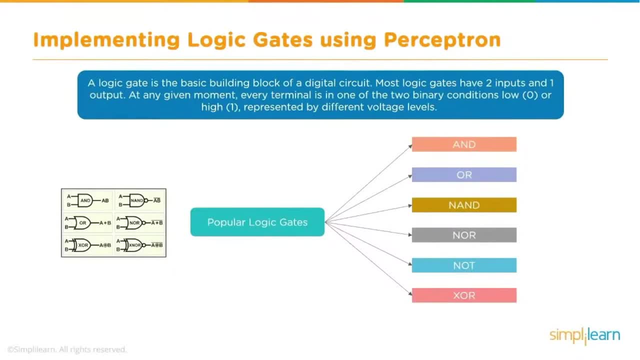 able to implement some of the most common logical gates which could take two inputs like A and B, and then give a corresponding result. So, for example, in case of an AND gate, A and B and then the output is AB. In case of an OR gate, it is A plus B, and so on and so forth, and they were able. 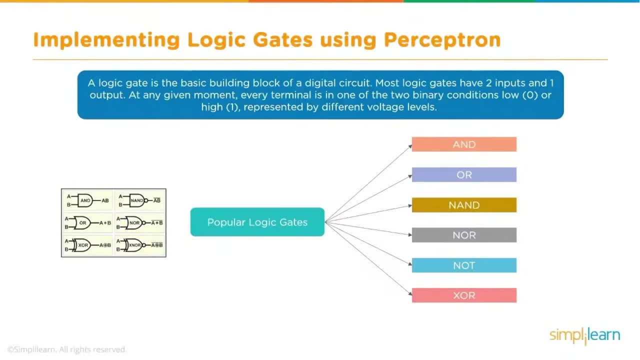 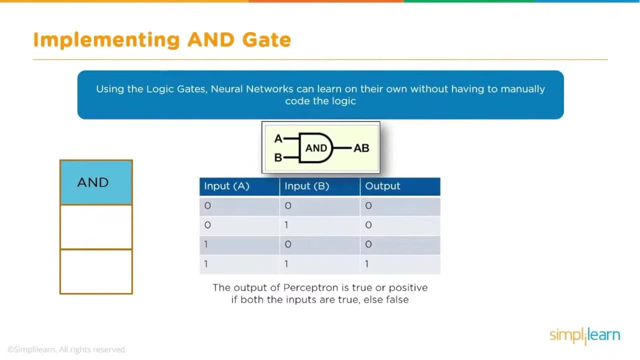 to do this using a single layer perceptron. Now, most of these gates it was possible to use single layer perceptron, except for XOR, and we will see why that is in a little bit. So this is how an AND gate works. The inputs A and B, the output should be fired or the neuron should be fired only when both the 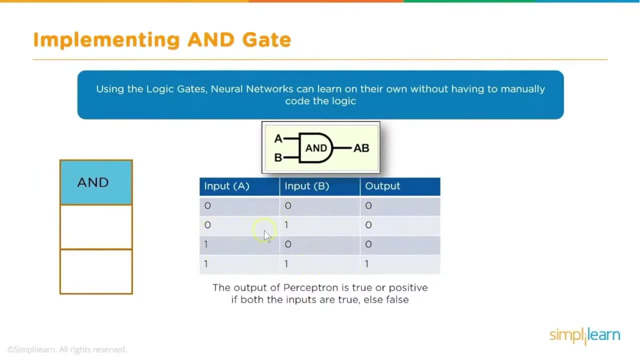 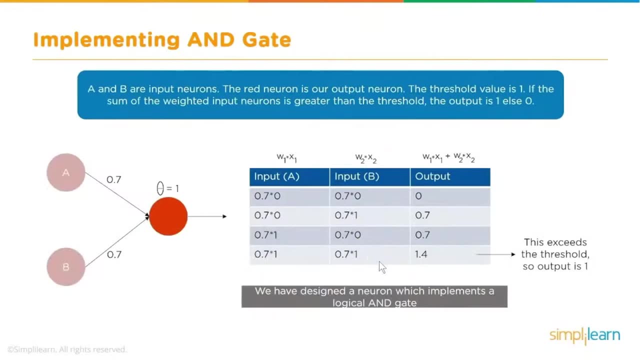 inputs are 1.. So if you have 0: 0, the output should be 0. for 0- 1, it is again 0, 1, 0, again 0 and 1: 1 the output should be 1.. So how do we implement this with a neuron? So it was found that by changing. 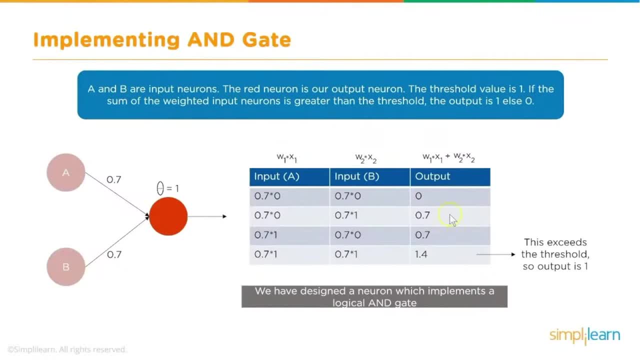 the values of weights, it is possible to achieve this logic. So, for example, if we have equal weights- 0.7, 0.7- and then if we take the sum of the weighted product, So for example, 0.7 into 0 and 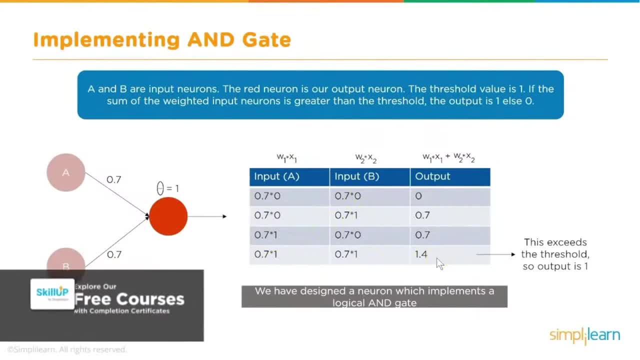 then 0.7 into 0, will give you 0, and so on and so forth, and in the last case, when both the inputs are 1, you get a value which is greater than 1, which is the threshold. So only in this case the 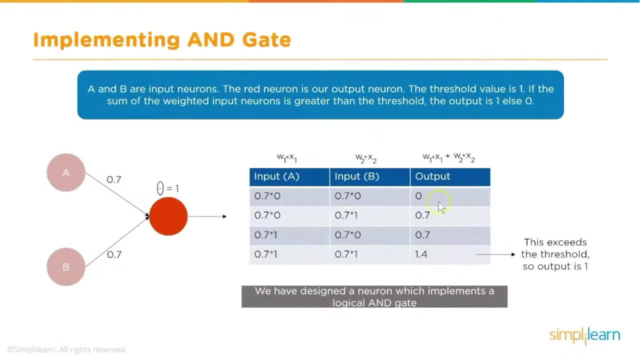 neuron gets activated and the output is: there is an output. in all the other cases there is no output because the threshold value is 1.. So this is implementation of an AND gate using a single perceptron or a single neuron. Similarly, an OR gate. in order to implement an OR gate in: 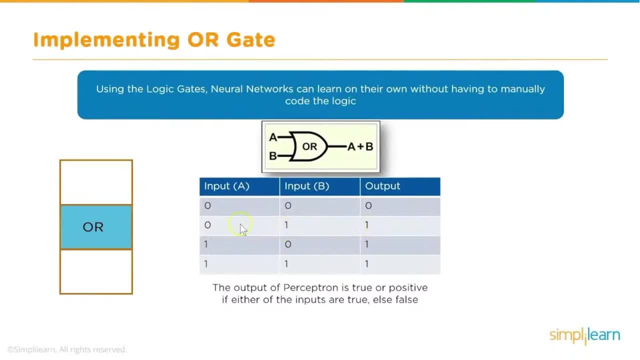 case of an OR gate, the output will be 1 if either of these inputs is 1.. So, for example, 0, 1 will result in 1, or rather, in all the cases it is 1, except for 0- 0.. So how do we implement this using? 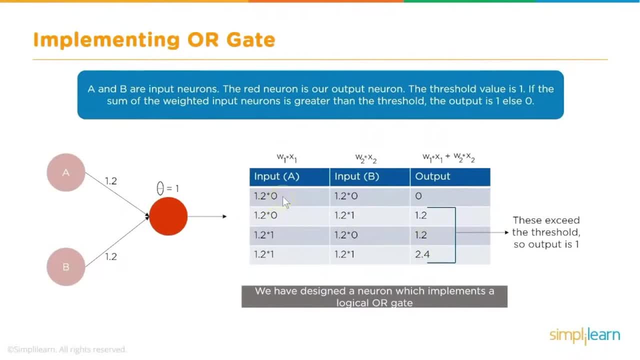 a perceptron. Once again, if you have a perceptron with weights, for example 1.2. now if you see here, if in the first case, when both are 0, the output is 0.. Second case, when it is 0 and 1, 1.2 into 0 is 0, and then 1.2 into 1 is 1, and in the second case, 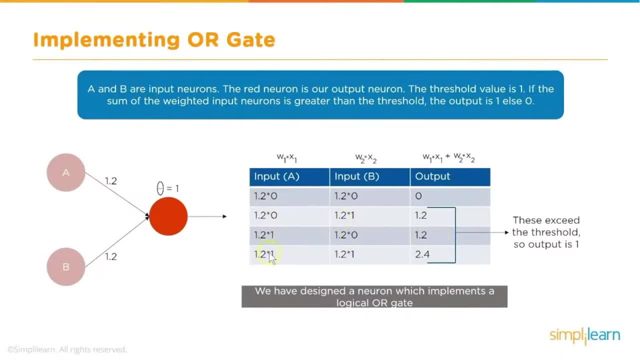 similarly, the output is 1.2. in this last case, when both the inputs are 1, the output is 2.4. So during the training process these weights will keep changing and then at one point, where the weights are equal to w1 is equal to 1.2 and w2 is equal to 1.2, the system learns that it gives. 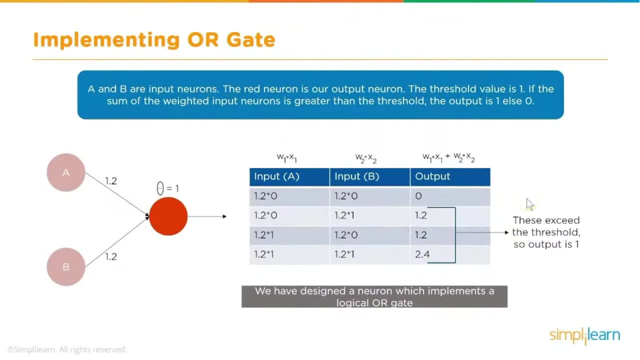 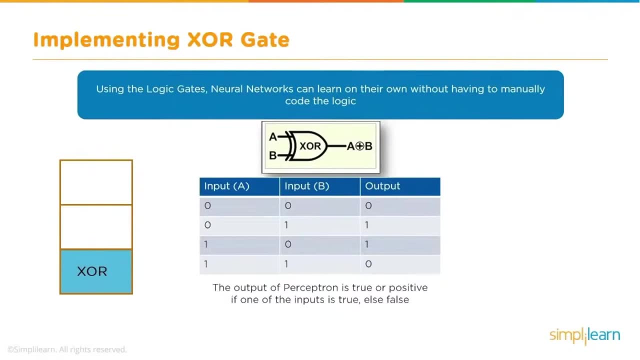 the output a number of times. So that is, implementation of OR gate using a single neuron or a single layer perceptron, Now XOR gate. this was one of the challenging ones. They tried to implement an XOR gate with a single level perceptron, but it was not possible and therefore, in order to implement 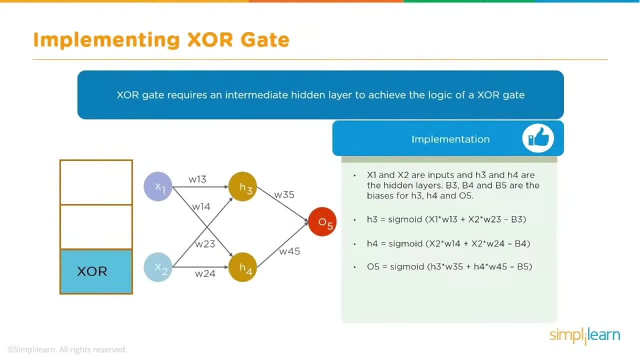 an XOR, So this was like a roadblock in the progress of a neural network. However, subsequently they realized that this can be implemented. an XOR gate can be implemented using an XOR gate, a multi-level perceptron or mlp. so in this case there are two layers instead of a single layer. 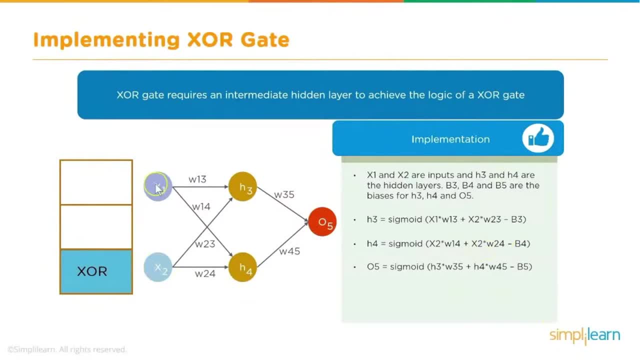 and this is how you can implement an xr gate. so you will see that x1 and x2 are the inputs and there is a hidden layer and that's why it is denoted as h3 and h4. and then you take the output of that and feed it to the output at o5 and provide a threshold here. so we will see here that 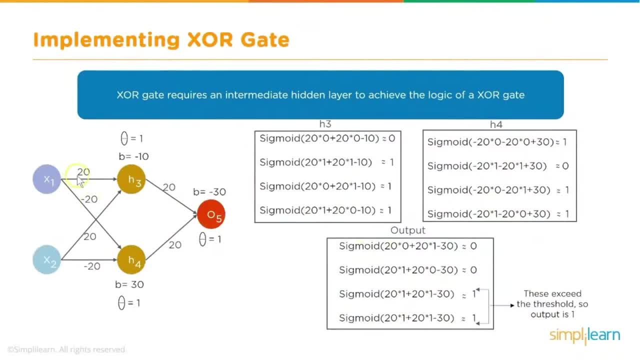 this is the numerical calculation. so the weights are in this case: for x1 it is 20 and minus 20, and once again 20 and minus 20.. so these inputs are fed into h3 and h4. so you will see here for h3. 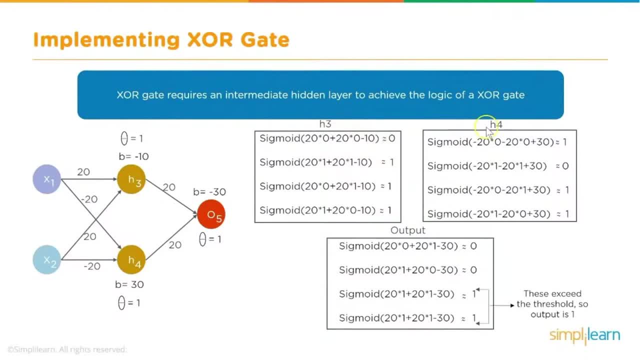 the input is 0, 1, 1, 1 and for h4 it is 1, 0, 1, 1. and if you now look at the output, final output, where the threshold is taken as 1, if we use a sigmoid with the threshold 1, you will see that in these two cases it is 0 and in the last two cases it is 1.. so this: 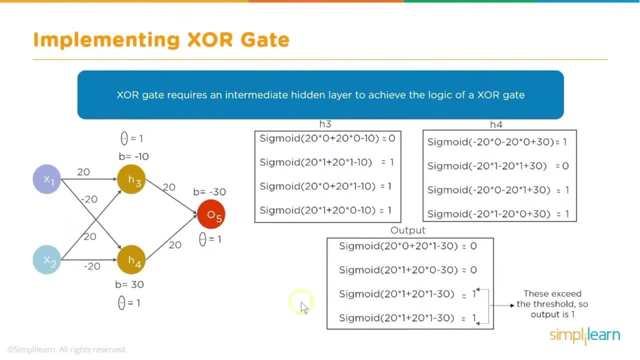 is the implementation of xr. in case of xr, only when one of the inputs is one you will get an output. so that is what we are seeing here. if we have either both the inputs are one or both the inputs are zero, then the output should be zero. so that is what is an exclusive or gate. so it 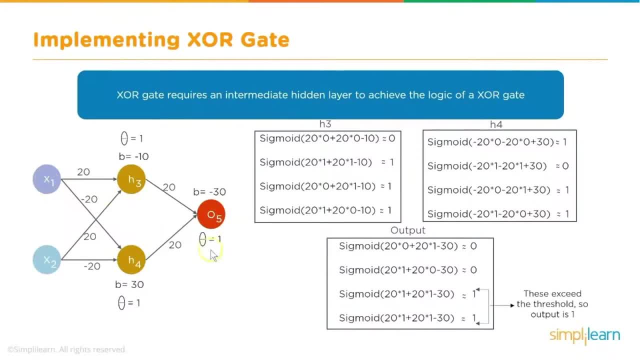 is exclusive, because only one of the inputs should be one, and that's what we are seeing here. only you will get an output of one which is satisfied by this condition. so this is a special implementation. xr gate is a special implementation of perceptron, now that we got a good idea about. 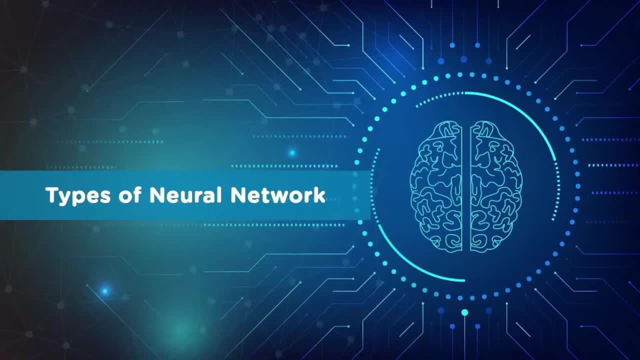 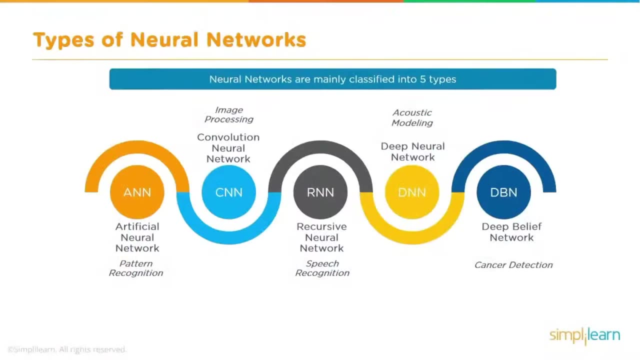 perceptron. let's take a look at what is the neural network. so we have seen what is a perceptron. we have seen what is a neuron, so we will see what exactly is a neural network. so neural network is nothing but a network of these neurons, and they are different types of neural networks there are. 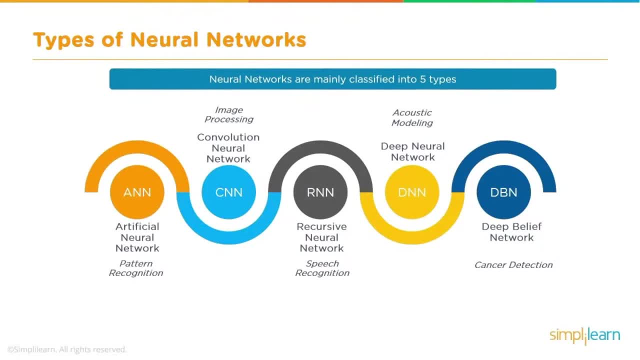 these are artificial neural network, convolutional neural network, then recursive neural network or recurrent neural network, deep neural network and deep belief network. so and each of these types of neural networks have a special you know they can solve special kind of problems. for example, convolutional neural networks are very good at performing image processing. 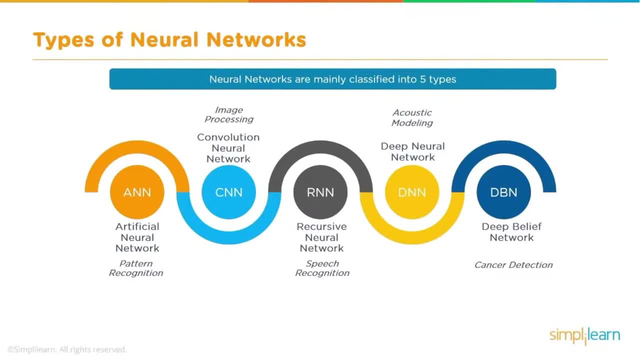 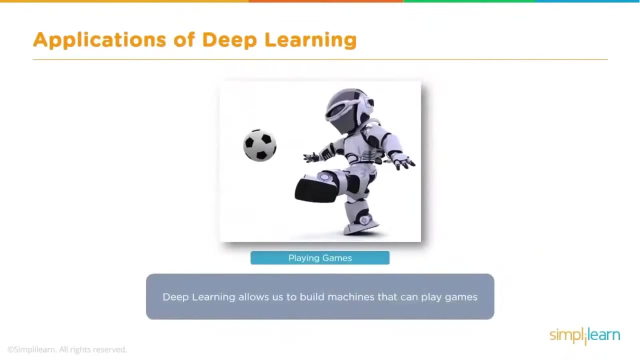 and image recognition and so on, whereas rnn are very good for speech recognition and also text analysis and so on. so each type has some special characteristics and they can, they're good at performing certain special kind of tasks. what are some of the applications of deep learning? deep learning is today used extensively in gaming. you must have heard about. 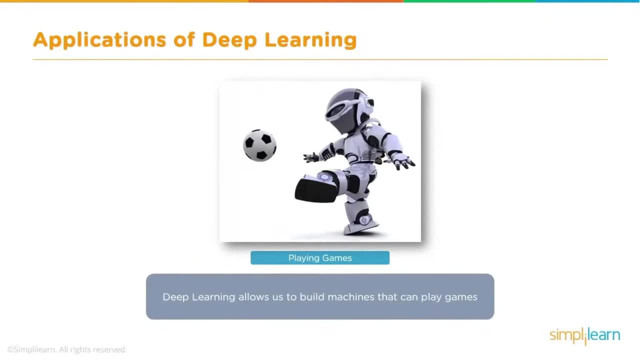 alpha go, which is a game created by a startup called deep mind, which got acquired by google, and alpha go is a AI which defeated the human world champion, lee sedol in this game of go. so gaming is an area where deep learning is being extensively used and a lot of research happens in the area of gaming, as 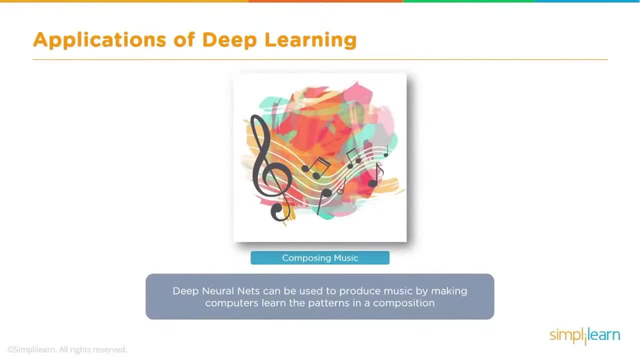 well, in addition to that, nowadays there are neural networks, or special type called generative adversarial networks, which can be used for synthesizing either images or music, or text and so on, and they can be used to compose music, so the neural network can be trained to compose a certain kind. 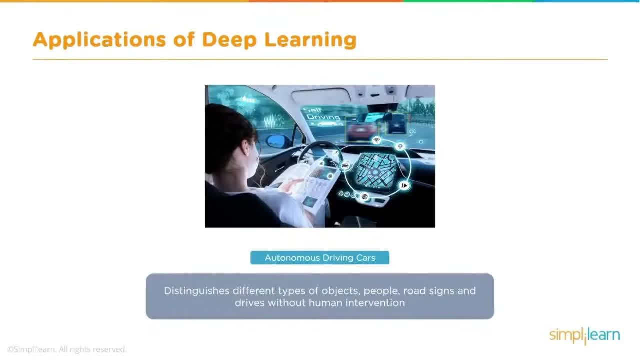 of music and autonomous cars. you must be familiar with google, google's self-driving car, and today a lot of automotive companies are investing in this space, and deep learning is a core component of this autonomous cars. the cars are trained to recognize, for example, the road, the lane markings. 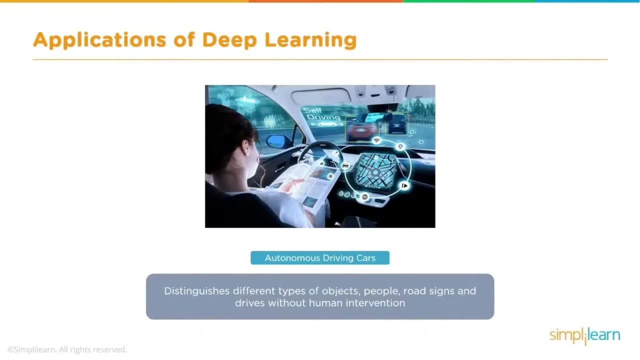 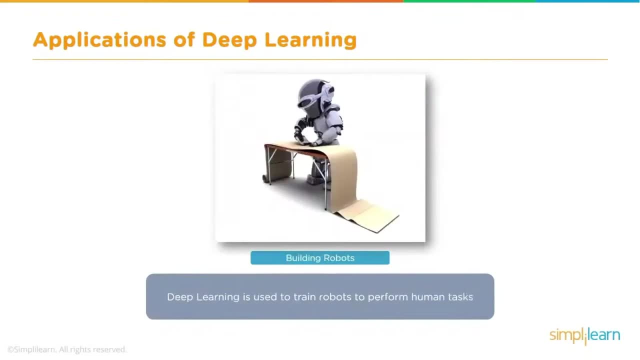 the road signals, any objects that are in front, any obstruction and so on and so forth. so all this involves deep learning. so that's another major application. and robots: we have seen several robots, including Sophia. you may be familiar with Sophia, who was given a citizenship by Saudi Arabia, and 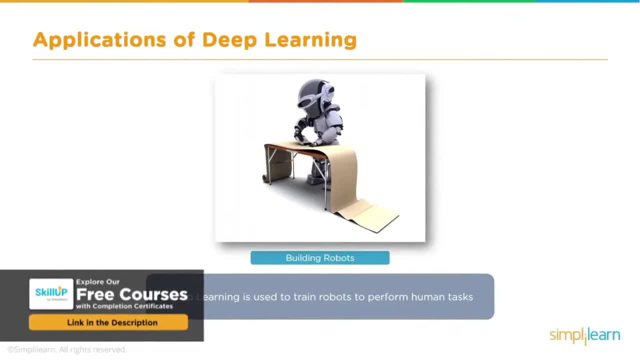 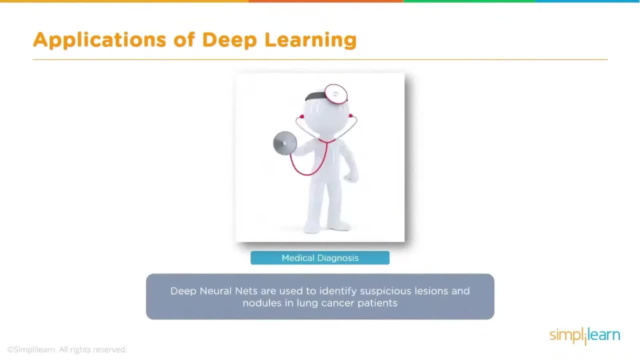 there are several such robots, which are very human-like, and the underlying technology in many of these robots is deep learning. medical diagnostics and health care is another major area where deep learning is being used, and within healthcare diagnostics, again, there are multiple areas where deep learning and image. 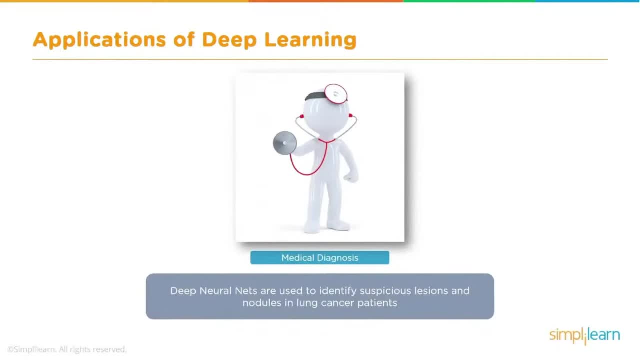 recognition. image processing can be used, for example, for cancer detection. as you may be aware, if cancer is detected early on, it can be cured, and one of the challenges is in the availability of specialists who can diagnose cancer and the availability of specialists who can diagnose cancer using these diagnostic images and various scans, and and so on and so forth. so the idea is to train. 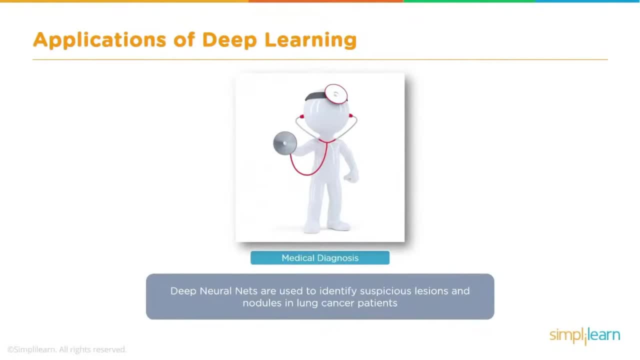 neural network to perform some of these activities so that the load on the cancer specialist doctors or oncologists comes down. and there is a lot of research happening here and there are already quite a few applications that are claimed to be performing better than human beings in this space. can be lung cancer. it can be tiroid cancer. it can be trouble with cancer, danny, who is also a patient, and even though there are some areas that are desire to develop the brain in order to be able to perform better than human beings in this space, it can be lung cancer, it can be with cancer, it can be. 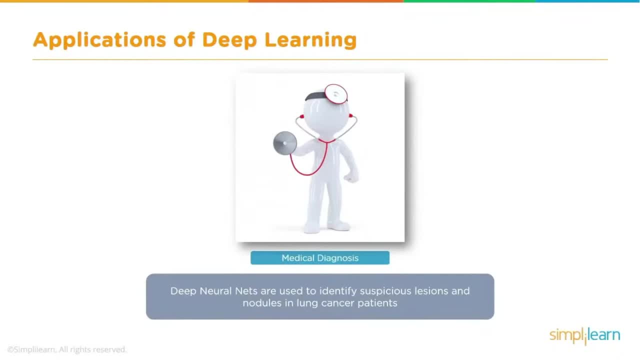 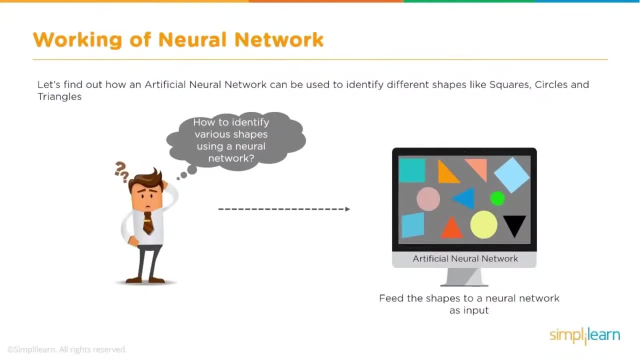 breast cancer and so on and so forth. so health care is a major area where deep learning is being applied. let's take a look at the inner working of a neural network. so how does an artificial neural network, let's say, identify? can we train a neural network to identify the shapes like squares? 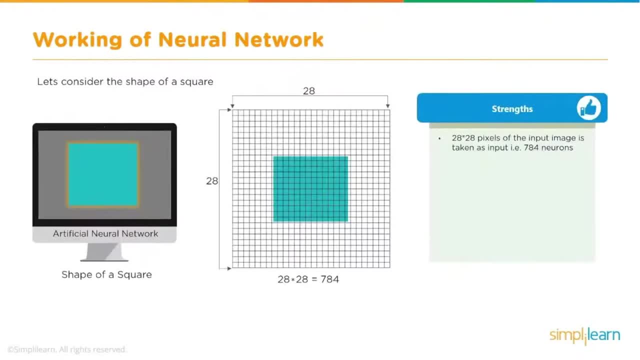 and circles and triangles when these images are fed. so this is how it works. any image is nothing, but it is a digital information of the pixels. so in this particular case, let's say this is an image of 28 by 28 pixel and this is an image of a square. there is a certain way in which the pixels are. 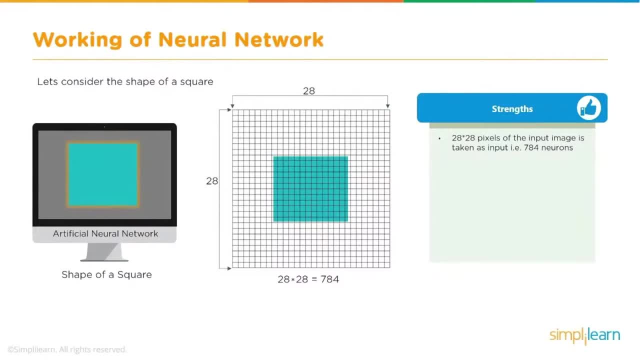 lit up, and so these pixels have a certain value, maybe from 0 to 256, and 0 indicates that it is black or it is dark and 256 indicates it is completely, it is white or lit up. so that is like an indication or a measure of the how the pixels are lit up and 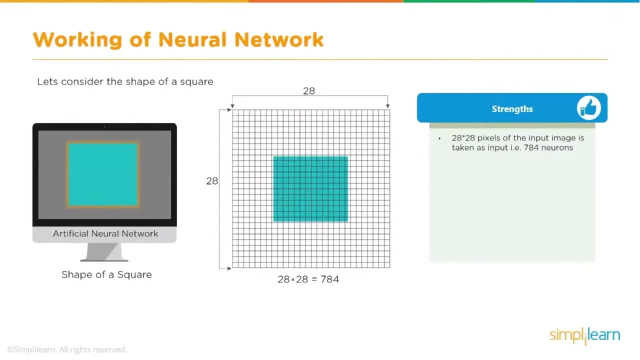 so this is an image is, let's say, consisting of information of 784 pixels, so all the information, what is inside this image, can be kind of compressed into this 784 pixels. the way each of these pixels is lit up provides information about what exactly is the image, so we can 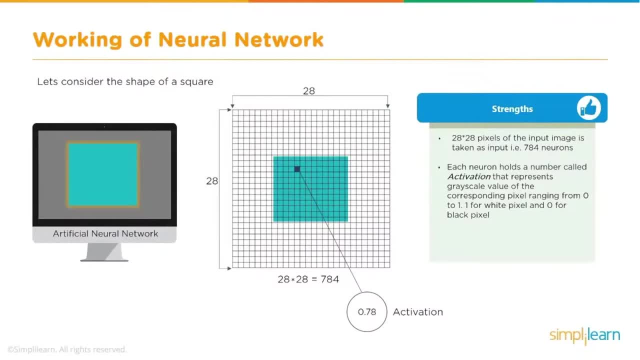 train neural networks to use that information and identify the images. so let's take a look how this works. so each neuron, the value. if it is close to one, that means it is white, whereas if it is close to zero, that means it is black. now this is a an animation. 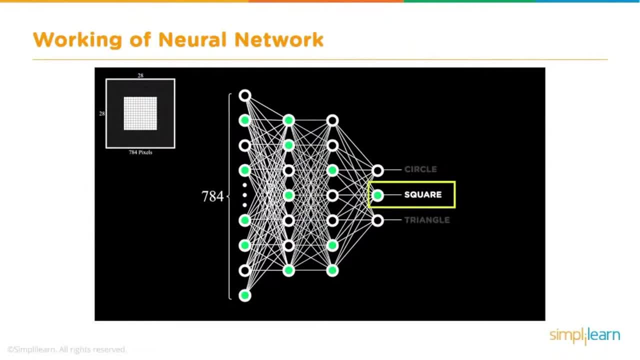 of how this whole thing works. so these pixels. one of the ways of doing it is we can flatten this image and take this complete 784 pixels and feed that as input to our neural network. the neural network can consist of probably several layers. there can be a few hidden layers and then 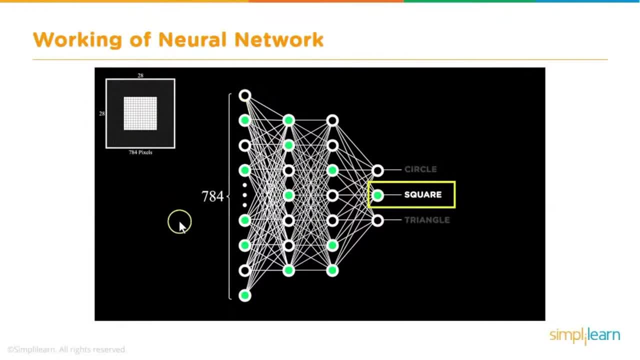 there is an input layer and an output layer. now, the input layer: take the 784 pixels as input, the values of each of these pixels, and then you get an output which can be of three types or three classes. one can be a square, a circle or an of a number of those. you get a space value on the surface which is equal to 784 pixels per pixel and post. sheesh, it's really easy. if you just eat it and fluke yourself, you now know how to create that proof. if you need to come with an alternate or a model, it takes five qualities you know too. you don't have to come out and do all the training etc and do at once either a. 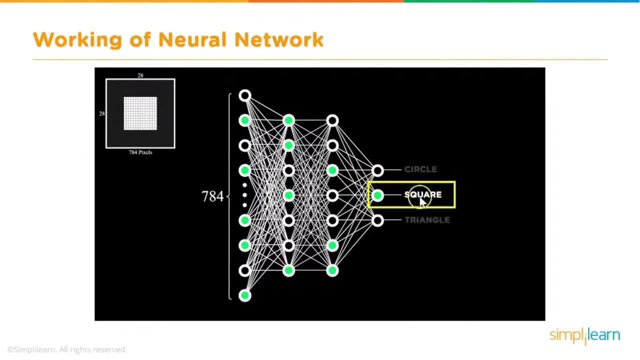 one single connection option, or you take the stroke command to do that, take the obд given and sweet them to past the a triangle. now, during the training process there will be initially, obviously, you feed this image and it will probably say it's a circle, or it will say it's a triangle. so as a part of the training, 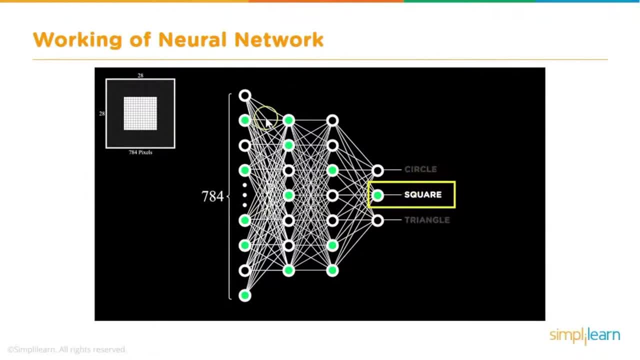 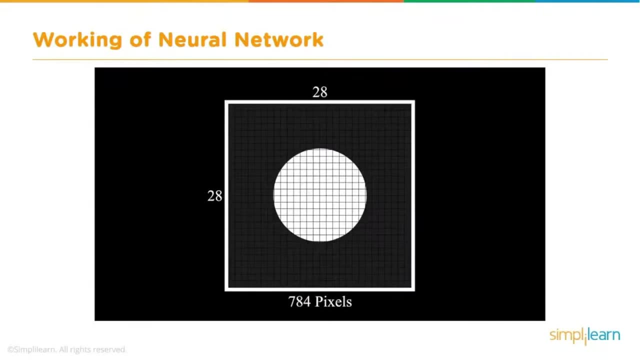 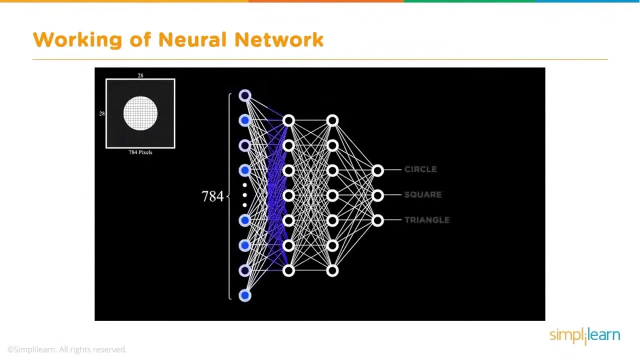 process. we then send that error back and the weights and the biases of these neurons are adjusted till it correctly identifies that this is a square. that is the whole training mechanism that happens out here. now let's take a look at a circle same way. so you feed these 784 pixels. 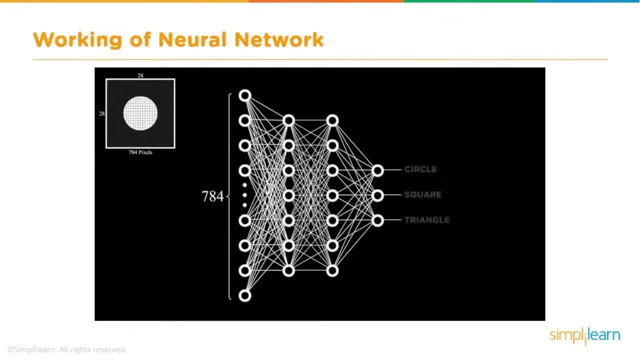 there is a certain pattern in which the pixels are lit up and the neural network is trained to identify that pattern and during the training process, once again, it would probably initially identify it incorrectly, saying this is a square or a triangle, and then that error goes away. it goes away after the initial training, over and over again. but in fact, this to be found words like it's eating over here and reading over here to identify this, and then this is managing the category, now the pattern. 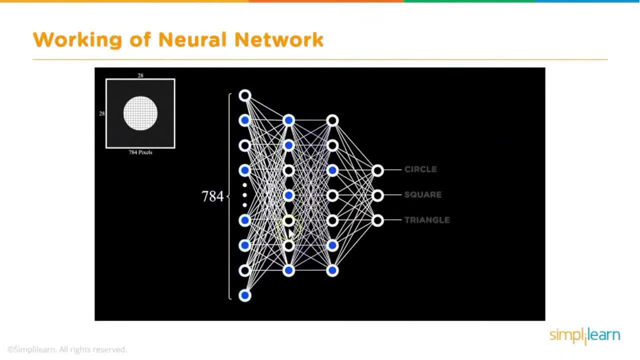 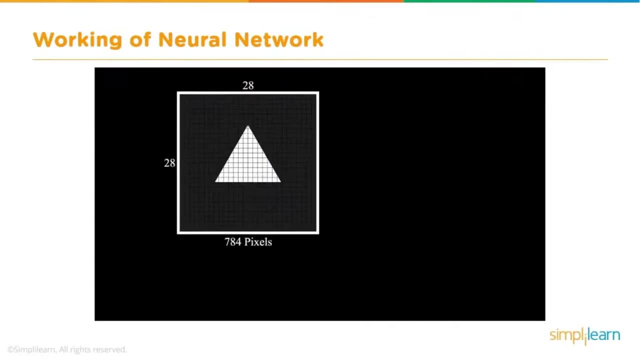 is fed back and the weights and biases are adjusted, finally till it finally gets the image correct. so that is the training process. so now we will take a look at same way: a triangle. so now if you feed another image which is consisting of triangles. so this is the training process. now we have trained our 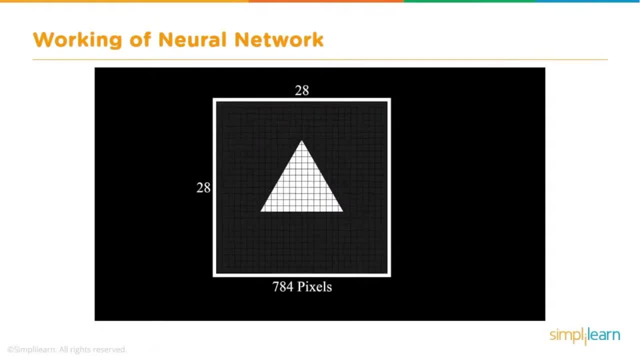 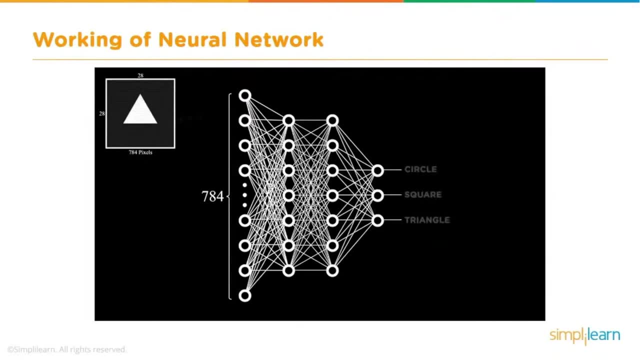 neural network to classify these images into a triangle or a circle and a square. so now this neural network can identify these three types of objects. now, if you feed another image and it will be able to identify whether it's a square or a triangle or a circle. now what is important to be observed is that 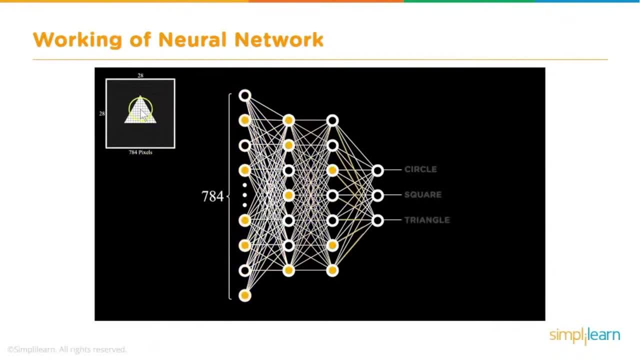 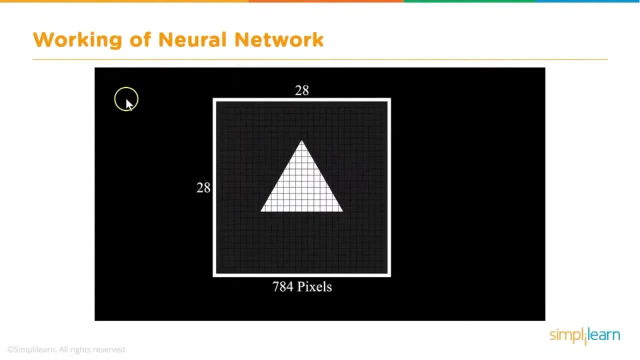 when you feed a new image, it is not necessary that the image or the the triangle is the same as the triangle, or the triangle is the same as the triangle is exactly in this position now the neural network actually identifies the patterns. so even if the triangle is, let's say, positioned here, not exactly in, 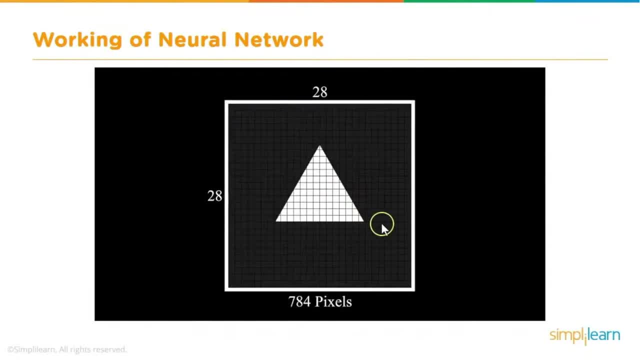 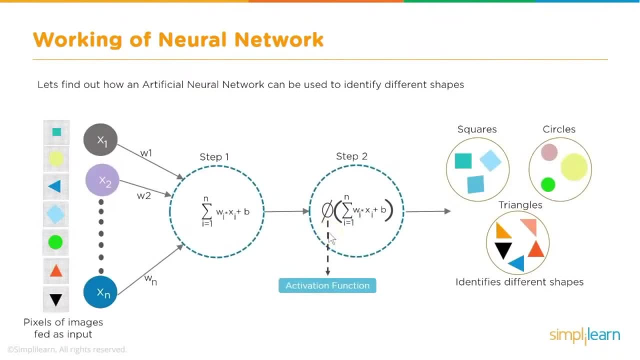 the middle, but maybe at the corner or in the side, it would still identify that it is a triangle, and that is the whole idea behind pattern recognition. so how does this training process work? there's a quick view of how the training process works. so we have seen that a neuron consists. 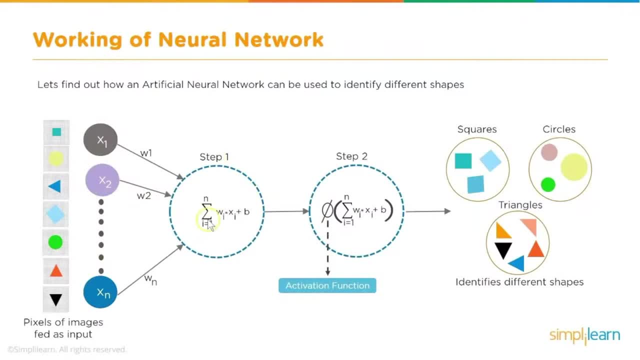 of two side node and a cross node, and then it is identified that an object is of inputs, it receives inputs, and then there is a weighted sum which is nothing but this xi wi summation of that plus the bias, and this is then fed to the activation function, and that in turn, 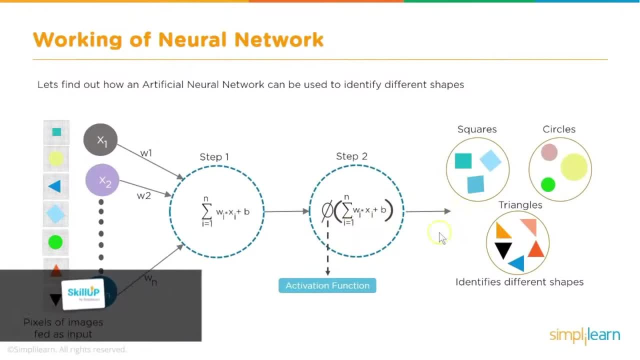 gives us a output now during the training process. initially, obviously, when you feed these images, when you send maybe a square, it will identify it as a triangle, and when you maybe feed a triangle, it will identify as a square, and so on, so that error information is fed back. and initially these: 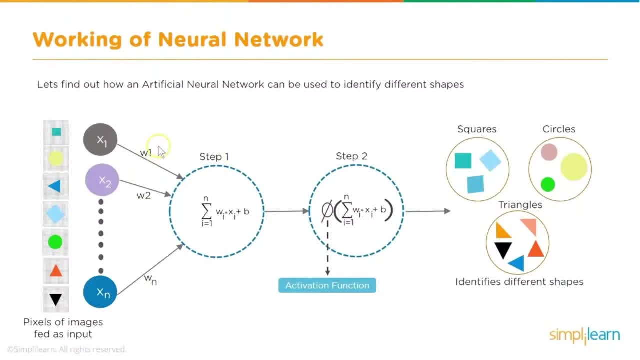 weights can be random. maybe all of them have zero values and then it will slowly keep changing. so the, as a part of the training process, the values of these weights- w1, w2, up to wn- keep changing in such a way that towards the end of the training process, it should be able to identify these images. 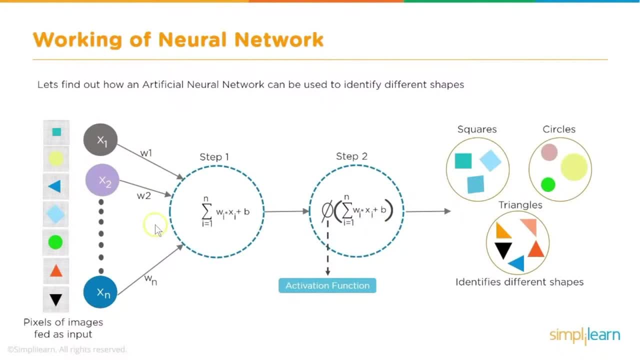 correctly. so till then the weights are adjusted, and that is known as the training process, and these weights are numeric values, could be 0.5, 0.25, 0.35 and so on. it could be positive or it could be negative, and the value that is coming here is the pixel. 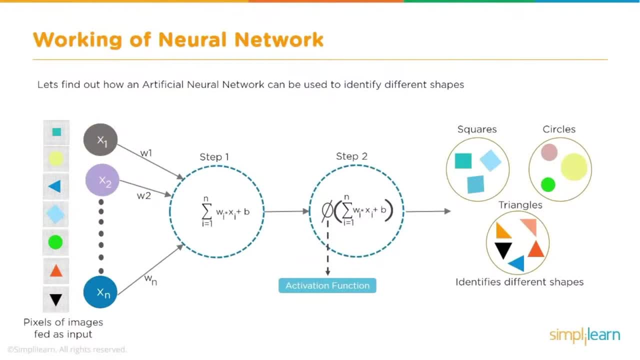 value. as we have seen, it can be anything between 0 to 1. you can scale it between 0 to 1 or 0 to 256, whichever way, 0 being black and 256 being white, and then all the other colors in between. so that is the input. so these are numerical values, this multiplication or the product. 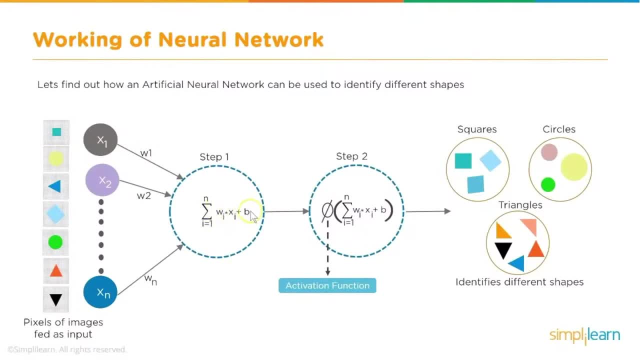 that wi xi is a numerical value and the bias is also a numerical value. we need to keep in mind that the bias is fixed for a neuron. it doesn't change with the inputs, whereas the weights are one per input. so that is one important point to be noted. so, but the bias also keeps changing. 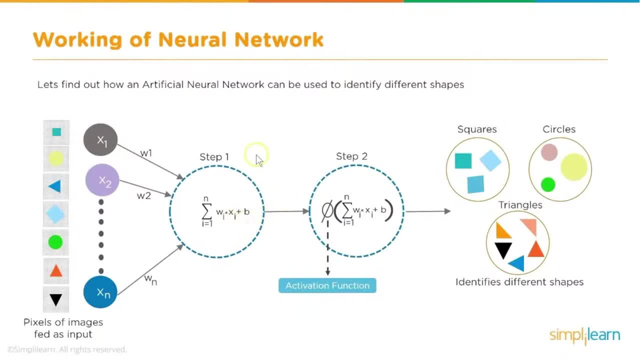 initially it will again have a random value, but as a part of the training process, the weights, the values of the weights w1, w2, wn and the value of B will change and ultimately, once the training process is complete, these values are fixed for this particular neuron: w1, w2, up to wn and plus. 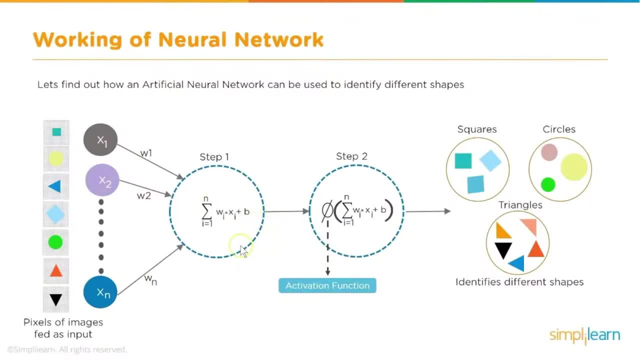 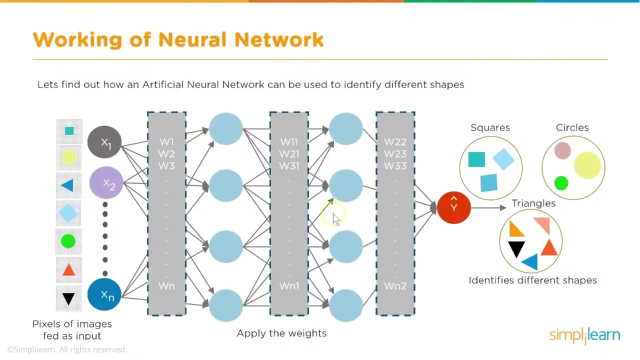 the value of the B is also fixed for this particular neuron, and in this way there will be multiple neurons and each. there may be multiple levels of neurons here, and that's the way the training process works. so this is another example of multi-layer. so there are two hidden layers in 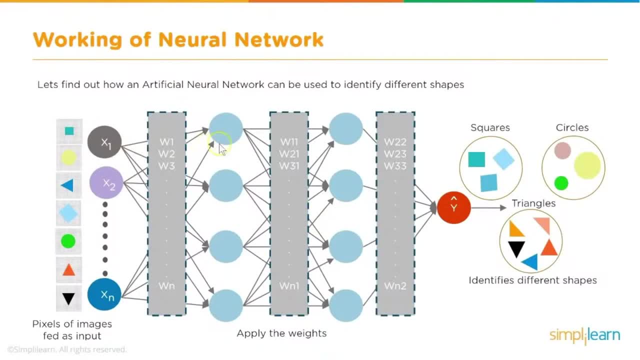 between, and then you have the input layer values coming from the input layer, then it goes through multiple layers, hidden layers, and then there is an output layer and, as you can see, there are weights and biases for each of these neurons in each layer, and all of them gets keeps changing during the training process and at the end of the training. 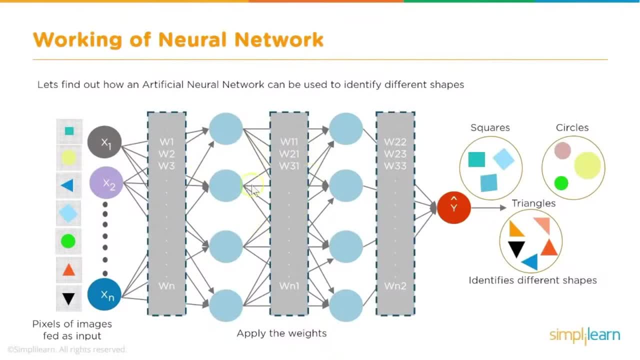 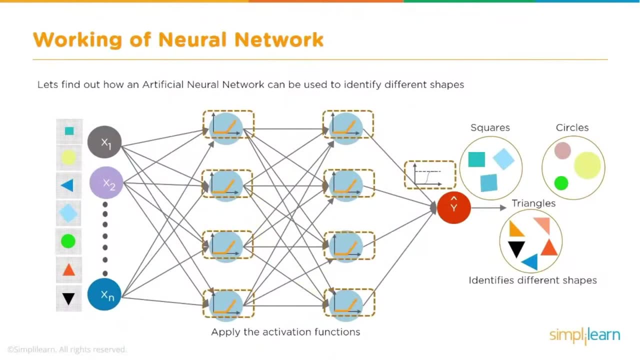 process. all these weights have a certain value, and that is a trained model, and those values will be fixed once the training is completed. all right, then there is something known as activation function neural networks consists of. one of the components in neural networks is activation function, and every neuron has an activation function, and there are different types of 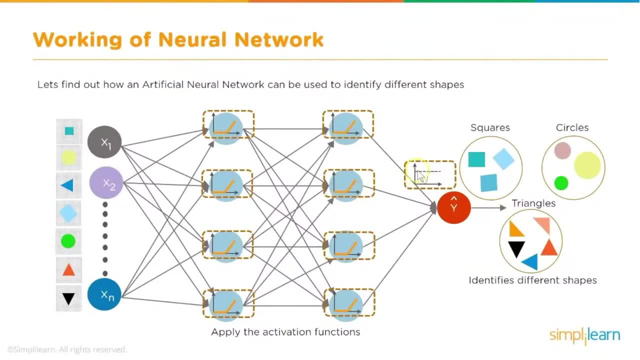 activation functions that are used. it could be a relu, it could be sigmoid, and so on and so forth, and the activation function is what decides whether a neuron should be fired or not. so whether the output should be zero or one is decided by the activation function and the activation function. 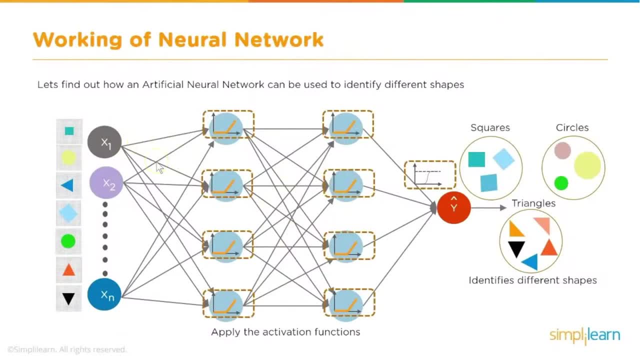 input, which is the weighted sum- remember we talked about wi xi plus b- that weighted sum is fed as a input to the activation function and then the output can be either a zero or a one, and there are different types of activation functions which are covered in an earlier video. you might want to. 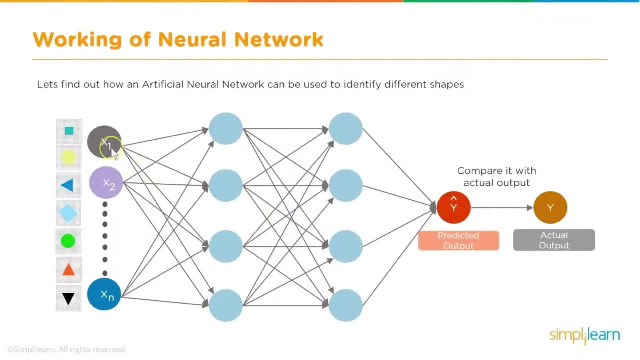 watch, all right. so, as a part of the training process, we feed the inputs, the label data or the training data, and then it gives an output, which is the predicted output by the network, which we indicate as y hat, and then there is a labeled data, because we, for supervised learning, we already know what. 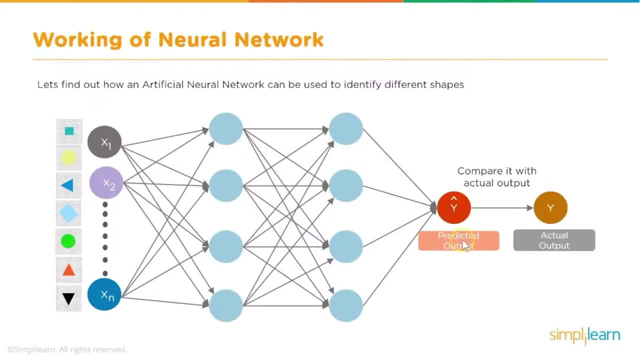 should be the output, so that is the actual output. and in the initial process, before the training is complete, obviously there will be error. so that is measured by what is known as a cost function. so the difference between the predicted output and the actual output is the error and the cost. 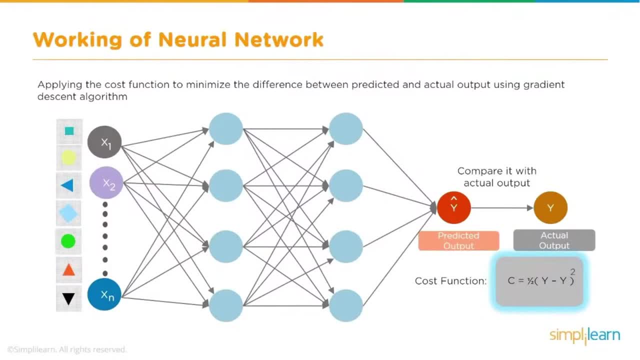 function can be defined in different ways. there are different types of cost functions. so in this case it is like the average of the squares of the error. so, and then all the errors are added, which can sometimes be called as sum of squares, sum of square errors or ssc, and that is then fed as a. 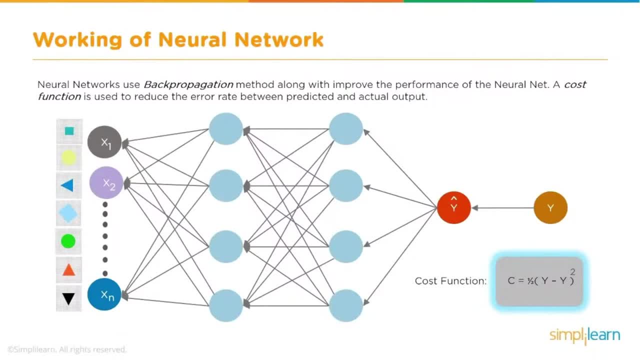 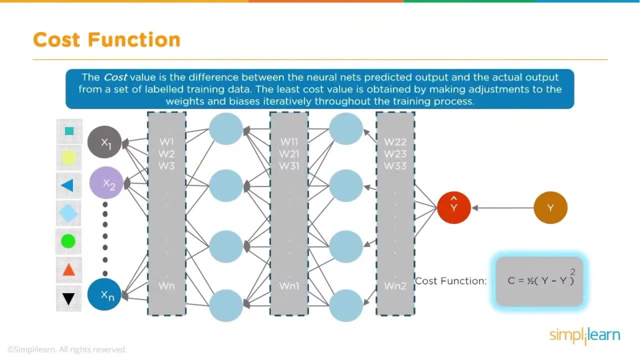 feedback in what is known as backward propagation or back propagation, and that helps in the network adjusting the weights and biases, and so the weights and biases get updated till this value. the error value or the cost function is minimum. now there is a optimization technique which is used. 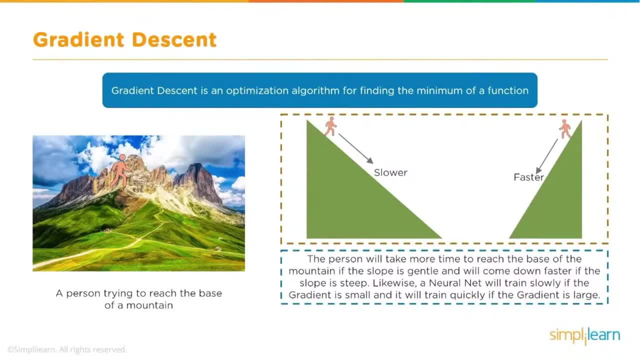 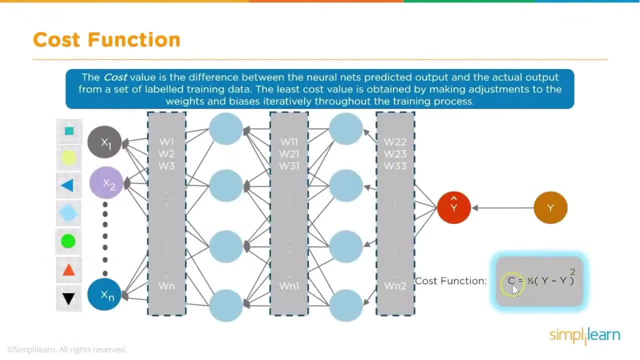 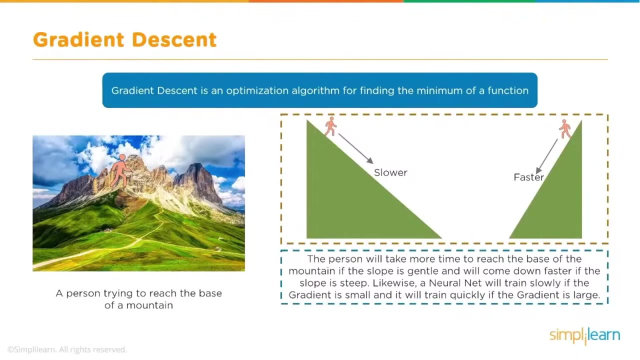 here called gradient descent optimization, and this algorithm works in a way that the error, which is the cost function, needs to be minimized. so there's a lot of mathematics that goes behind this. for example, they find the local minima on the global minima using differentiation, and so on and so forth. 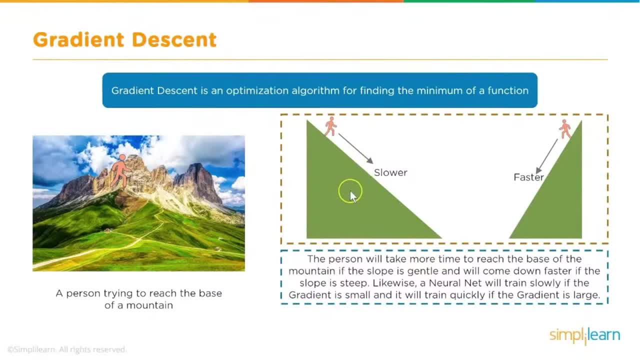 but the this so as a training process, as the as the part of training. the whole idea is to bring down the error which is like: let's say: this is the function, the cost function. at certain levels it is very high the cost value of the cost function. 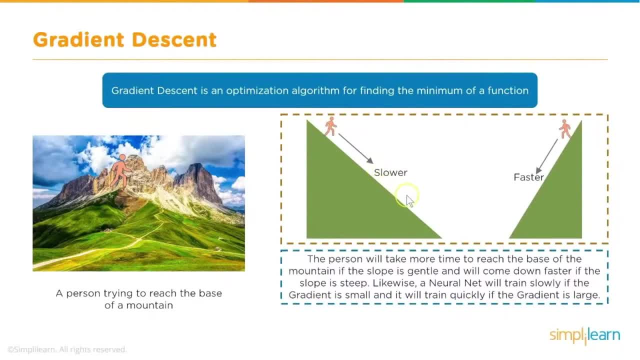 or the output of the cost function is very high, so the weights have to be adjusted in such a way- and also the bias, of course, that the cost function is minimized. so there is this optimization technique called gradient descent that is used, and this is known as the learning rate. now, gradient descent, you. 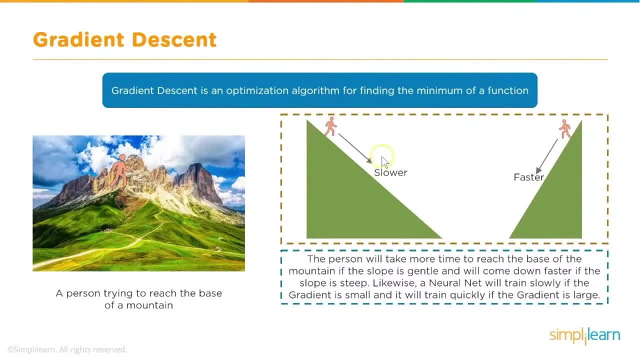 need to specify what should be the learning rate. and the learning rate should be optimal, because if you have a very high learning rate, then the optimization will not converge because at some point it will cross over to the side. on the other hand, if you have very low, 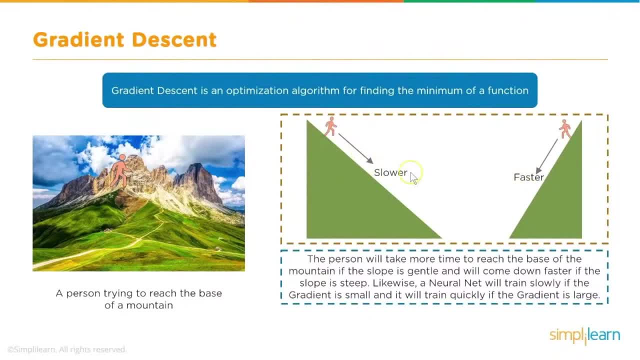 low learning rate, then it might take forever to convert. So you need to come up with the optimum value of the learning rate, And once that is done, using the gradient descent optimization, the error function is reduced And that's like the end of the training process. 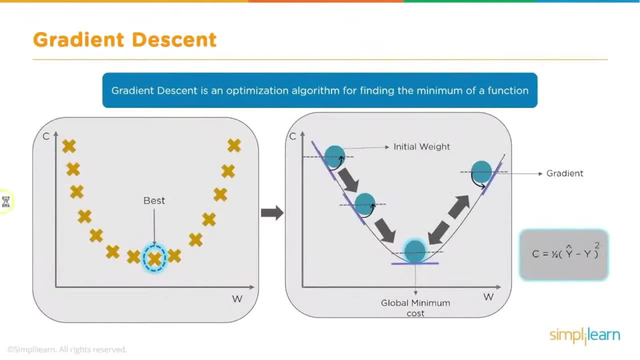 Alright, so this is another view of gradient descent. So this is how it looks. This is your cost function, the output of the cost function, and that has to be minimized using gradient descent algorithm, and these are like the parameters, and weight could be one of them. 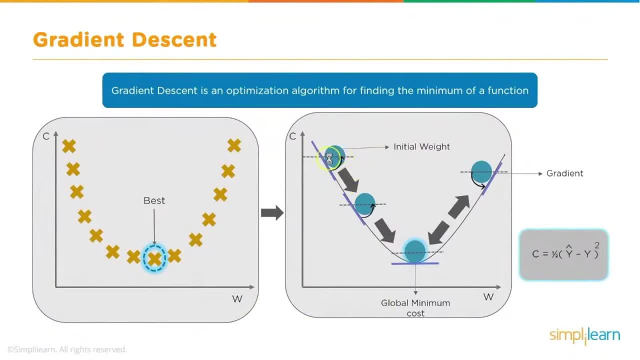 So initially we start with certain random values, So cost will be high and then the weights keep changing and in such a way that the cost function needs to come down and at some point it may reach the minimum value and then it may increase. So that is where the gradient descent algorithm decides that okay, it has reached a minimum. 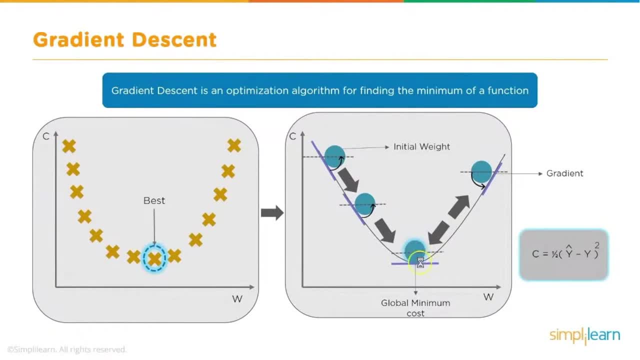 value and it will kind of try to stay here. So this is known as the global minima. Now, sometimes these curves may not be just for explanation purpose. this has been drawn in a nice way, But sometimes these curves can be pretty erratic. there can be some local minima here and then. 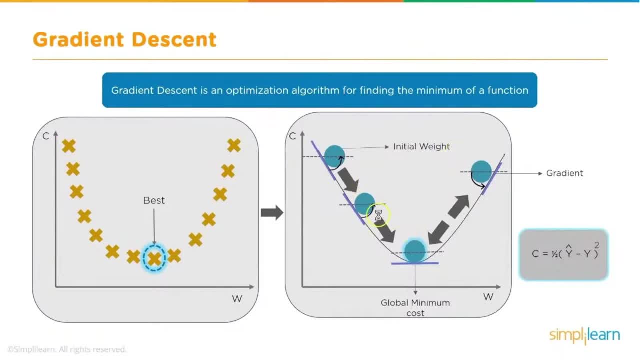 there is a peak and then and so on. So the whole idea of gradient descent optimization is to identify the global minima and to find the weights and the bias at that particular point. So that's what is gradient descent. Okay, And then this is another example. 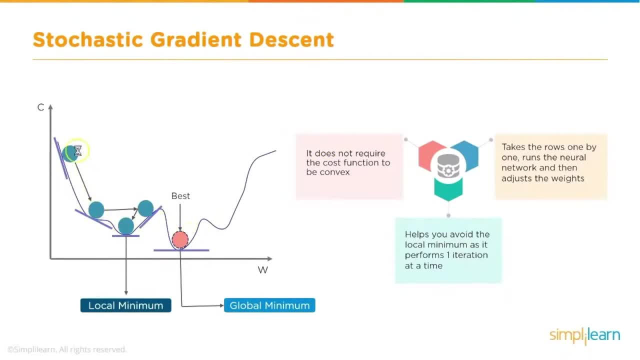 So you can have these multiple local minima. As you can see, at this point when it is coming down, it may appear like this is a minimum value, but then it is not. This is actually the global minimum value and the gradient descent algorithm will make. 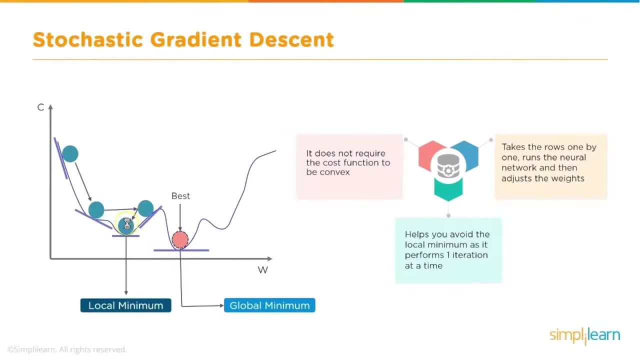 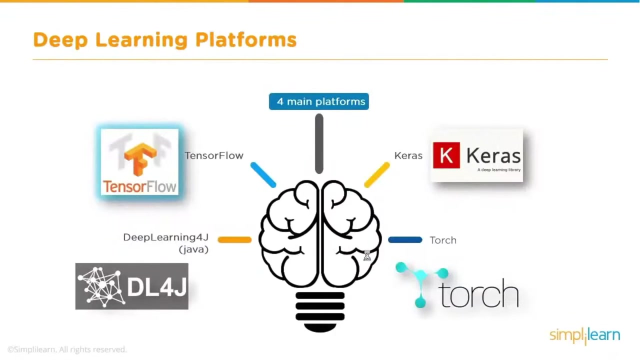 an effort to reach this level and not get stuck at this point. So the algorithm is already there and it knows how to identify this global minimum, and that's what it does during the training process. Now, in order to implement deep learning, there are multiple platforms and languages. 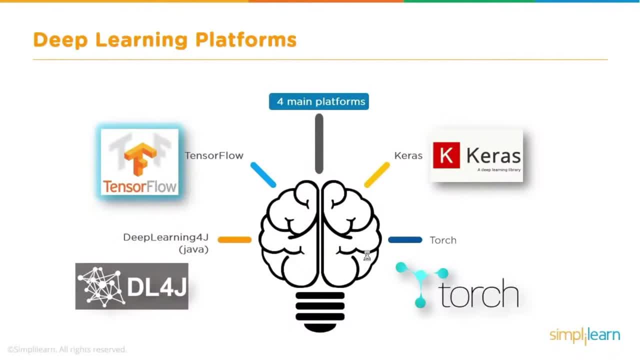 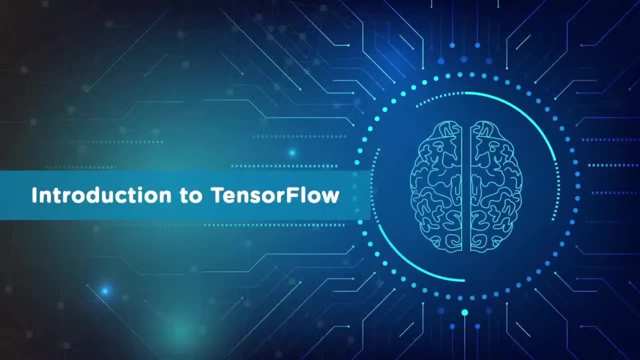 that are available, But the most common platform nowadays is TensorFlow, And so that's the reason we have this tutorial. we have created this tutorial for TensorFlow, So we will take you through a quick demo of how to write a TensorFlow code using Python. 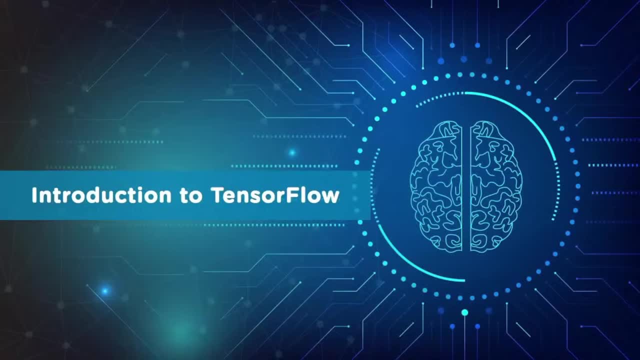 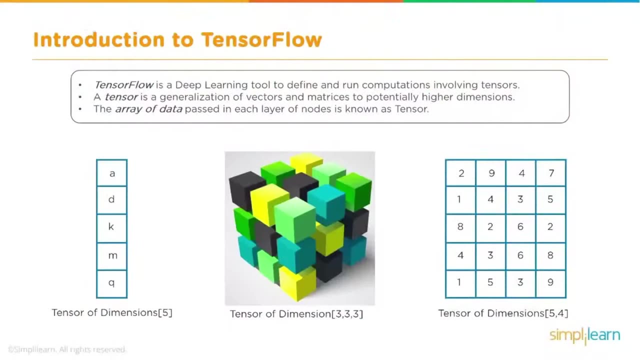 And TensorFlow is an open source platform created by Google, So let's just take a look at the details. So TensorFlow and so this is a library, a Python library, so you can use Python or any other languages. It's also supported in other languages like Java and R, and so on. 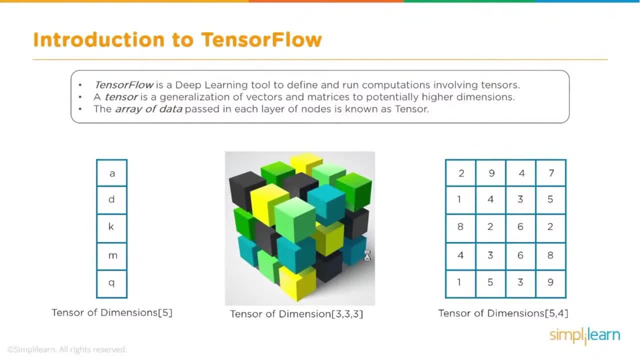 But Python is the most common language that is used, So it is a library for developing deep learning applications, especially using neural networks, And it consists of primarily two parts, if you will, So one is the tensors And then the other is the GUI. 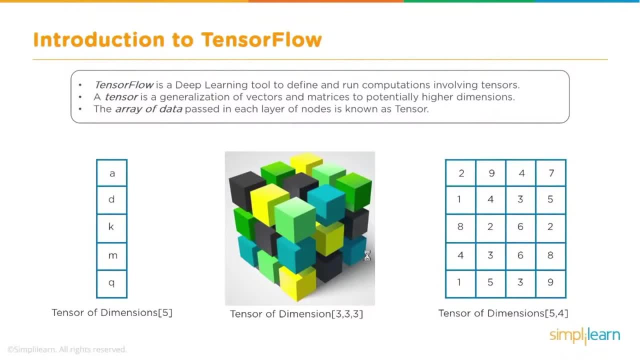 So the GUI is the name of the tensors, And then the tensors are the graphs or the flow. That's the way, the name, that's the reason for this kind of a name called TensorFlow. So what are tensors? Tensors are like multi dimensional arrays, if you will. 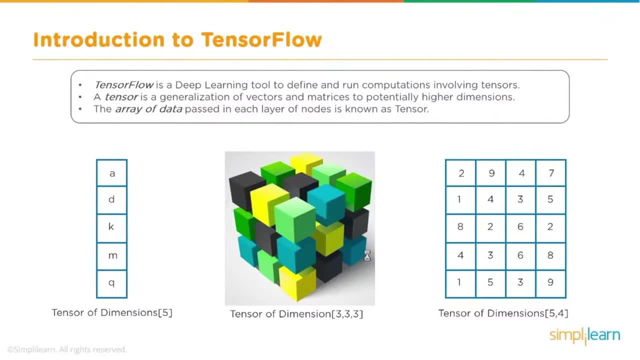 That's one way of looking at it. So usually you have a one dimensional array. So first of all you can have what is known as a scalar, which means a number, and then you have a one dimensional array, something like this, which means this: like a set of 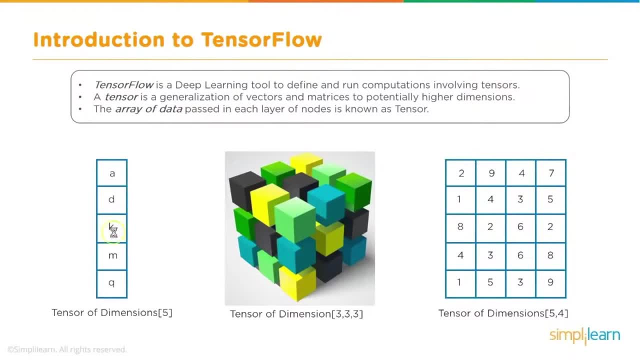 numbers, So that is a one dimensional array. Then you can have a two dimensional array Which is like a matrix, And beyond that sometimes it gets difficult. So this is a three dimensional array. but TensorFlow can handle many more dimensions, So it can have multi dimensional arrays. 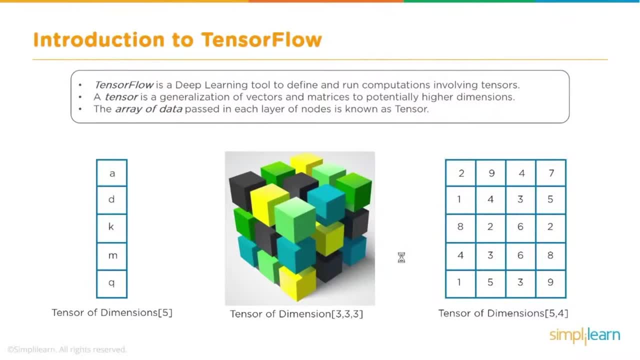 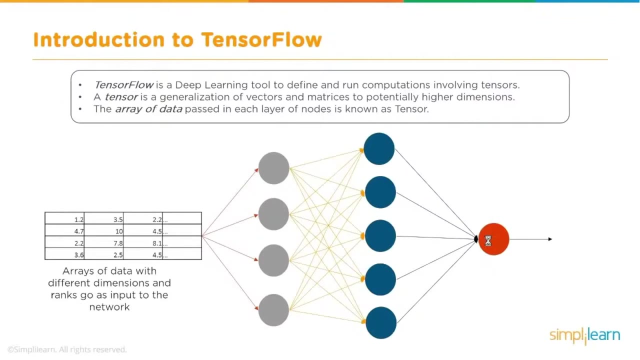 That is the strength of TensorFlow and which makes computation- deep learning computation- much faster, And that's the reason why TensorFlow is used for developing deep learning applications. So TensorFlow is a deep learning tool and this is the way it works. So the data basically flows in the form of tensors. and the way the programming works. 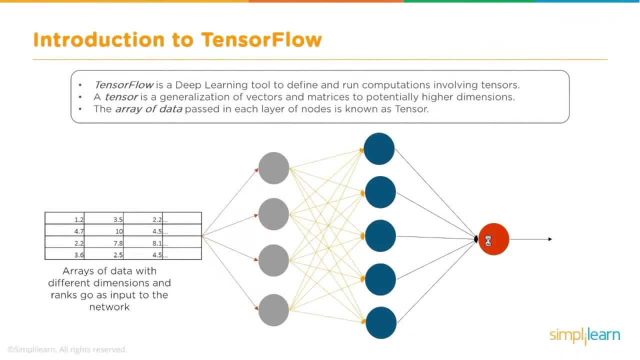 as well, is that you first create a graph of how to execute it and then you actually execute that particular graph in the form of what is known as a session. We will see this in the TensorFlow code as we move forward. So all the data is managed or manipulated in tensors and then the processing happens. 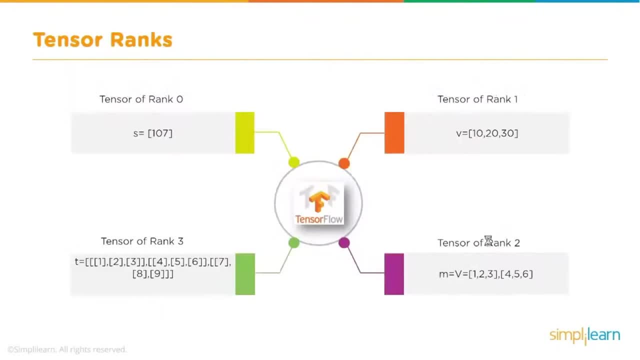 using these graphs. There are certain terms called tensors. So tensors are called like, for example, ranks of a tensor. The rank of a tensor is like a dimensional dimensionality in a way. So, for example, if it is scalar, so there is just a number, just one number: the rank. 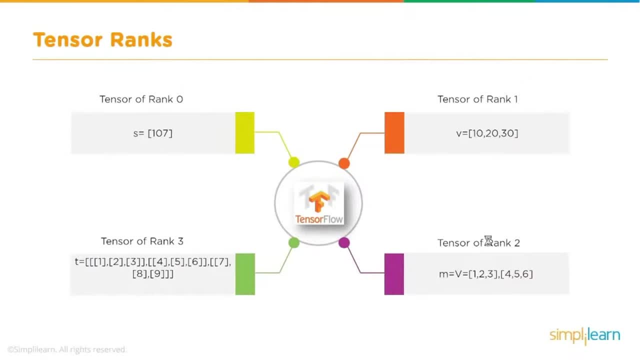 is supposed to be zero, And then it can be a one dimensional vector, in which case the rank is supposed to be one, And then you can have a two dimensional vector, typically like a matrix. then in that case we say the rank is zero. 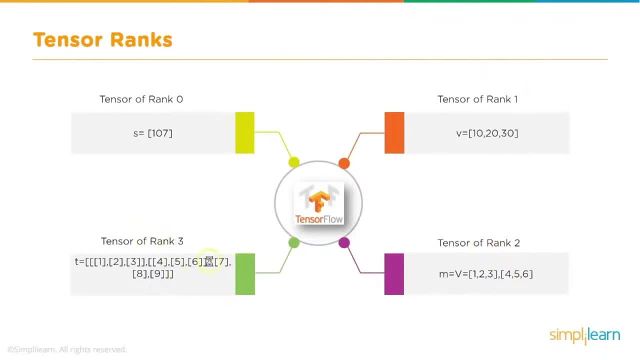 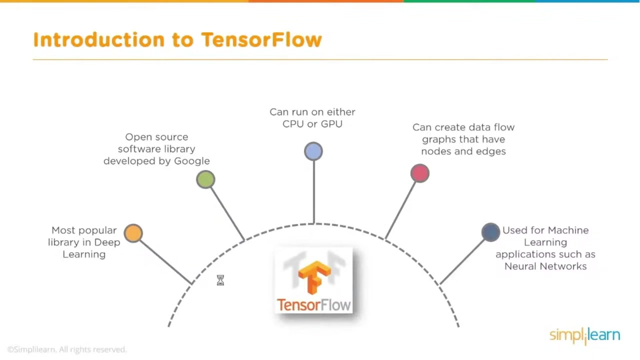 The rank is two, And then if it is a three dimensional array, then rank is three and so on, So it can have more than three as well. So it is possible that you can store multi dimensional arrays in the form of tensors. So what are some of the properties of TensorFlow? 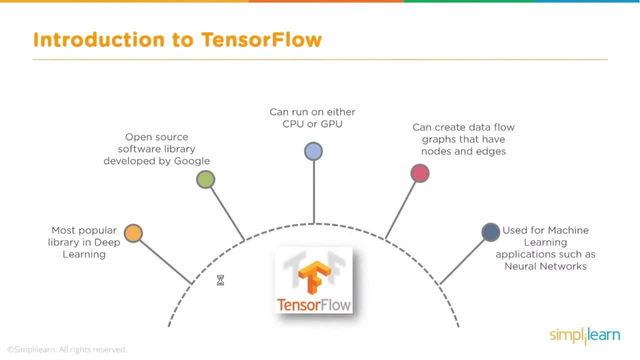 I think today it is one of the most popular platform. TensorFlow is the most popular deep learning platform or library. It is open source. It's developed by Google, Developed and maintained by Google, But it is open source. One of the most important things about TensorFlow is that it can run on CPUs as well as GPUs. 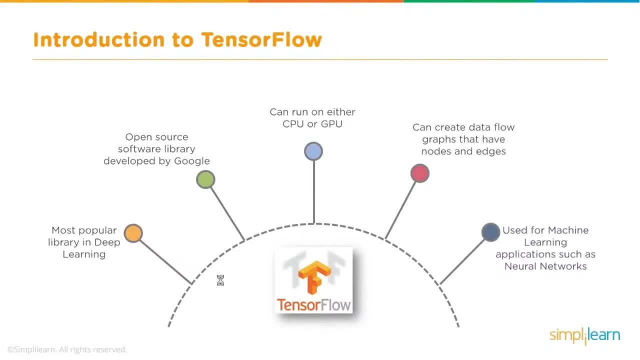 GPU is graphical processing unit, just like CPU is central processing unit. Now, in earlier days, GPU was used for- primarily for- graphics, And that's how the name has come, And one of the reasons is that it cannot perform generic activities very efficiently like CPU. 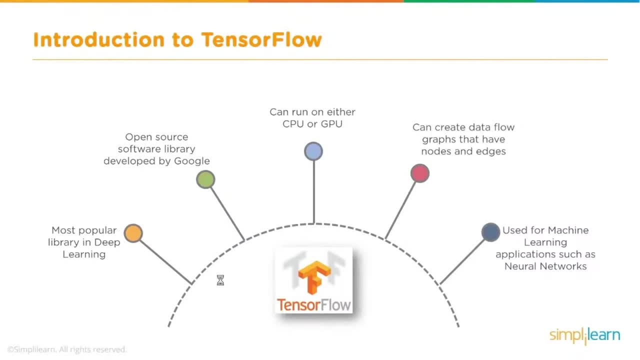 but it can perform iterative. It can perform iterative actions or computations extremely fast and much faster than a CPU, So they are really good for computational activities And in deep learning. there is a lot of iterative computation that happens So in the form of matrix, multiplication and so on. 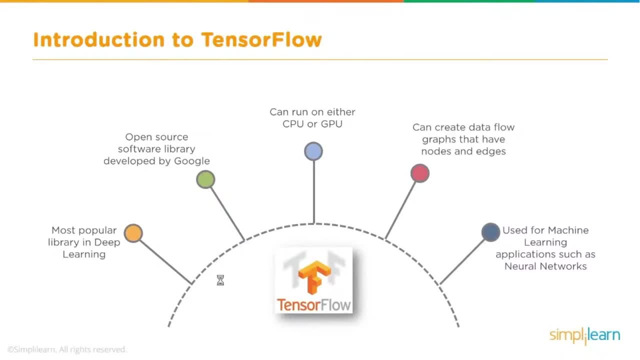 So GPUs are very well suited for this kind of computation And TensorFlow supports both GPU as well as CPU. And there's a certain way of writing code in TensorFlow. We will see as we go into the code. And of course, TensorFlow can be used for traditional machine learning as well. 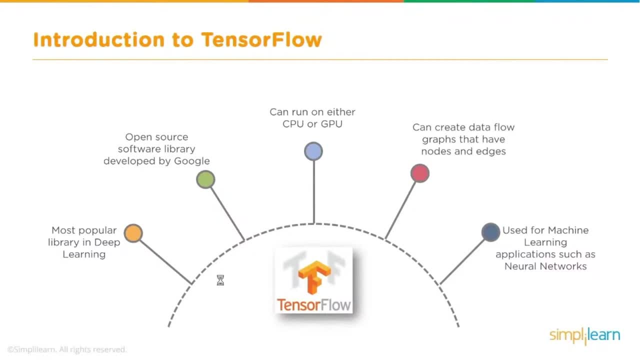 But then that would be an overkill. But just for understanding, it may be a good idea to start writing code for a normal machine learning use case, so that you get a hang of how TensorFlow code works, And then you can move into neural networks. 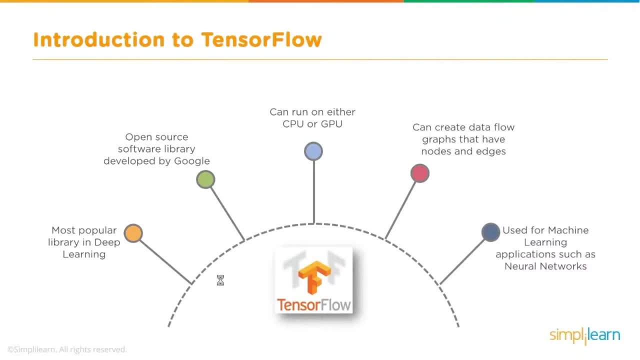 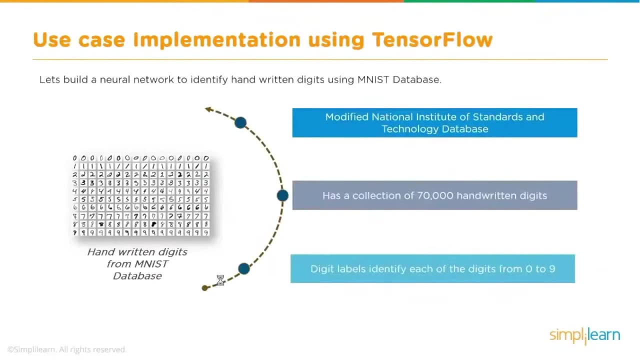 So that is just a suggestion, But if you're already familiar with how TensorFlow works, then probably you can go straight into the neural networks part. So in this tutorial we will take the use case of recognizing handwritten digits. This is like a hello world of deep learning. 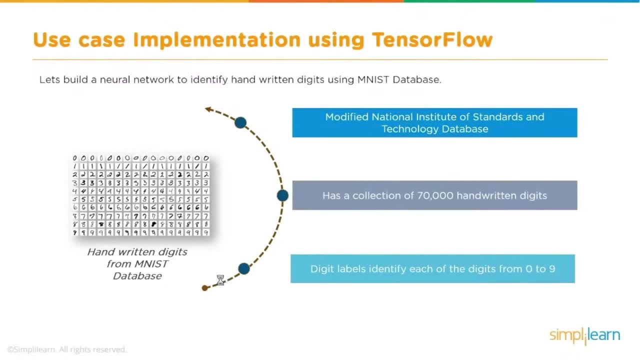 And this is a nice little MNIST database is a nice little database that has images of handwritten digits, nicely formatted, because very often in deep learning and neural networks we end up spending a lot of time in preparing the data for training And with that we are going to get started. 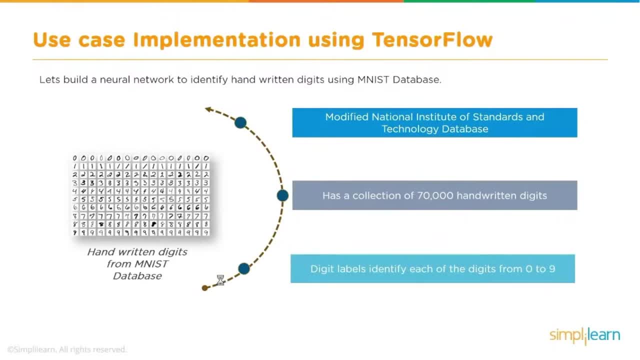 With MNIST database we can avoid that. You already have the data in the right format which can be directly used for training, And MNIST also offers a bunch of built in utility functions that we can straight away use and call those functions without worrying about writing our own functions. 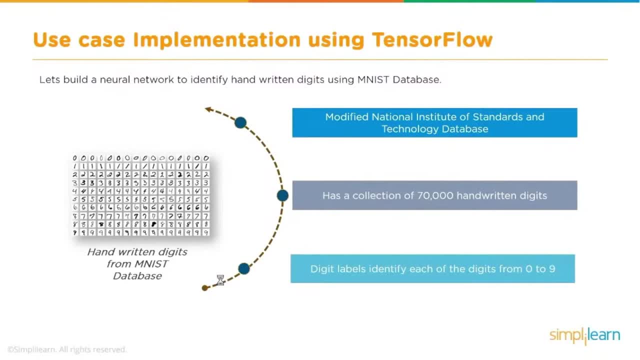 And that's one of the reasons why MNIST database is very popular for training purposes Initially, when people want to learn about deep learning And deep learning And so flow. this is the database that is used, and it has a collection of 70,000 handwritten. 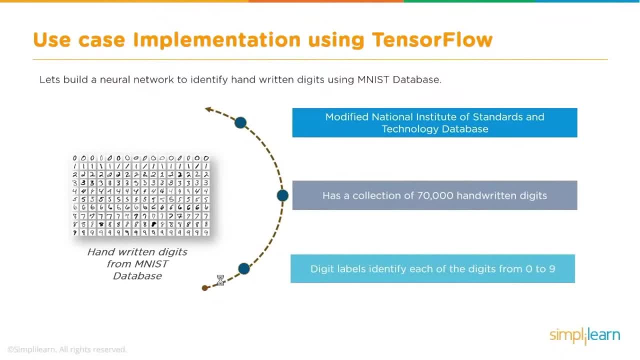 digits and a large part of them are for training. then you have test, just like in any machine learning process, And then you have validation and all of them are labeled. So you have the images and their label And these images. they look somewhat like this: 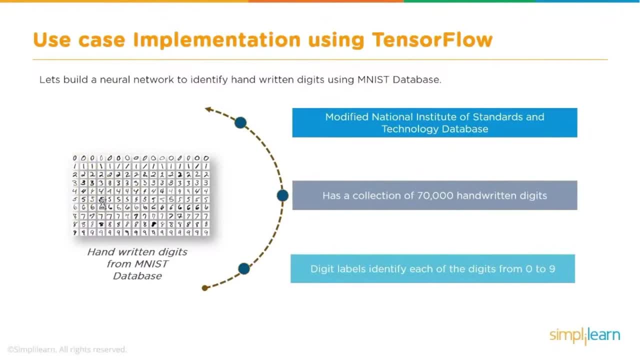 So they are handwritten images collected from a lot of individuals People have. these are samples written by human beings. They have handwritten these numbers, these numbers going from zero to nine. So people have written these numbers and then the images of those have been taken and formatted. 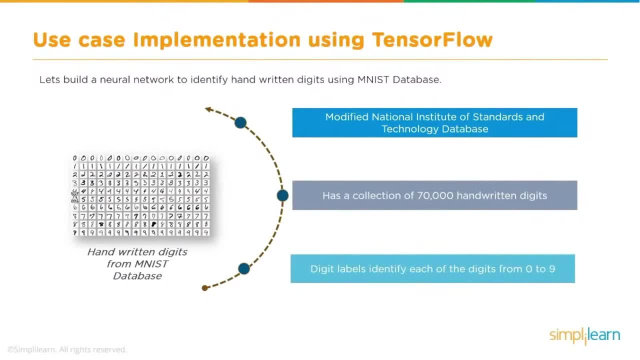 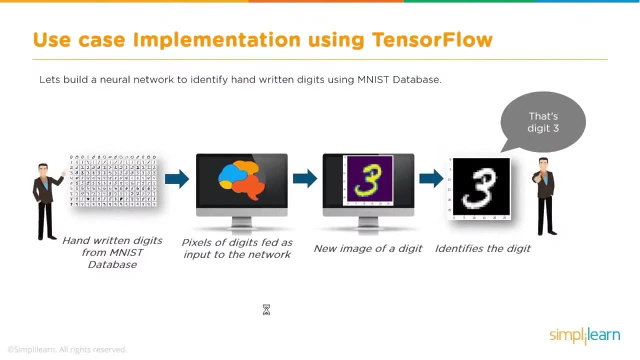 in such a way that it is very easy to handle. So that is MNIST database, And the way we are going to implement this in our TensorFlow is we will feed this data, especially the training data, Along with the label information, and the data is basically: these images are stored. 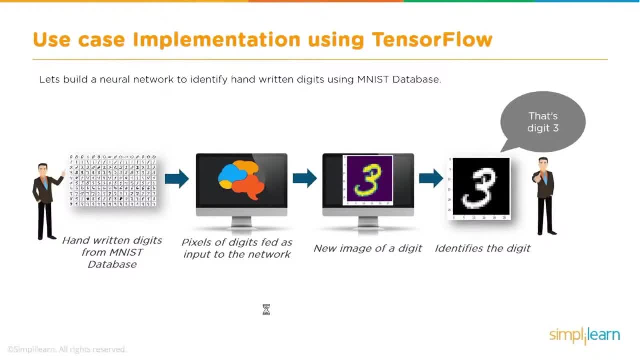 in the form of the pixel information. As we have seen in one of the previous slides, all the images are nothing but these are pixels. So an image is nothing but an arrangement of pixels and the value of the pixel. either it is lit up or it is not, or in somewhere in between. 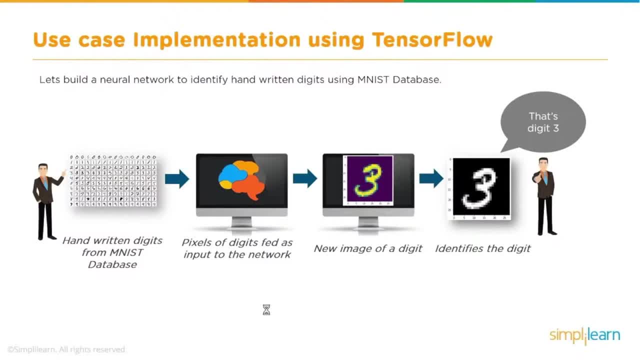 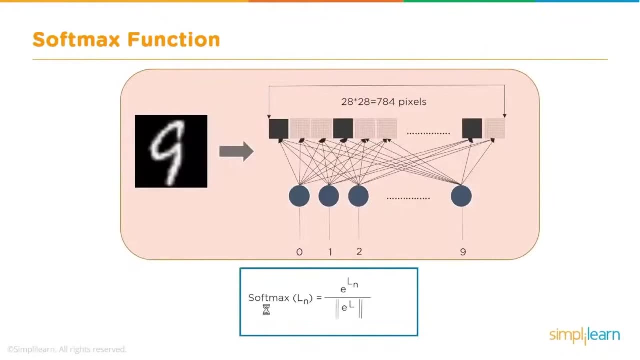 That's how the images are stored and that is how they are fed into the neural network and for training. Once the network is trained, when you provide a new image, it will be able to identify within a certain error, of course, And for this we will use one of the simpler neural network configurations called Softmax. 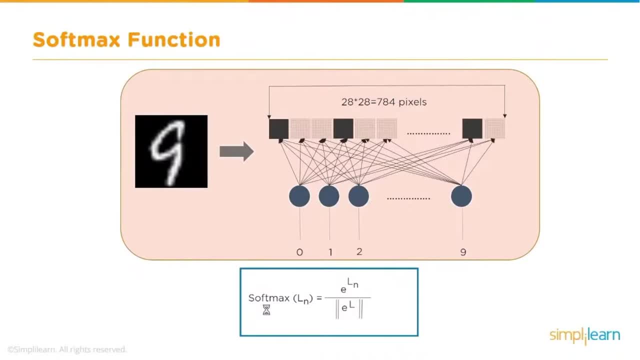 And for simplicity, what we will do is we will flatten these pixels. So, instead of taking them in a two dimensional arrangement, we just flatten them out. So, for example, this is a pixel. It starts from here. it is a 28 by 28.. 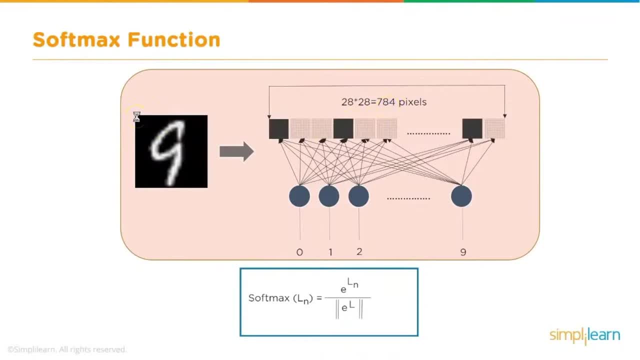 So there are 784 pixels. So pixel number one starts here, it goes all the way up to 28,. then 29 starts here and goes up to 56, and so on, And the pixel number 784 is here. So we take all these pixels, flatten them out and feed them like one single line into. 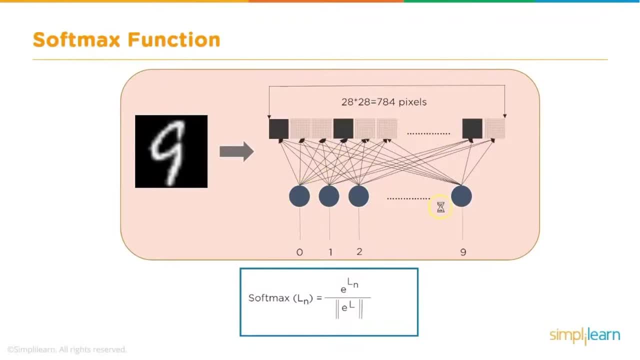 our neural network, And this is a what is known as a Softmax layer. What it does is, Once it is trained, it will be able to identify what digit this is. So there are in this output layer, there are 10 neurons each signifying a digit. 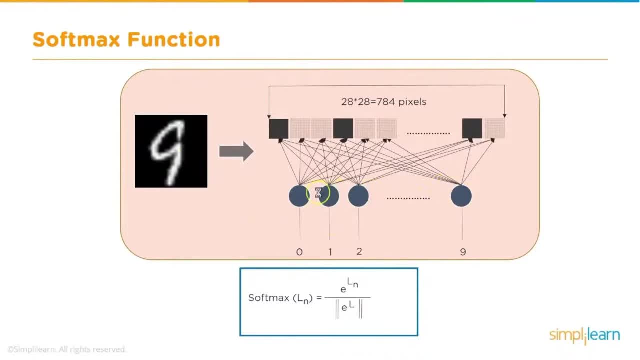 And at any given point of time, when you feed an image, only one of these 10 neurons gets activated. So, for example, if this is trained properly and if you feed a number nine like this, then this This neuron gets activated. 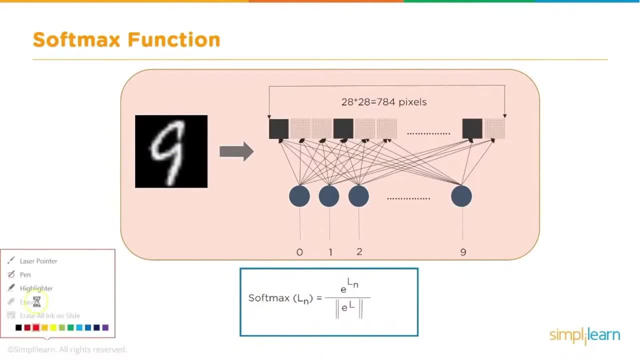 So you get an output from this neuron. Let me just use a pen or a laser to show you here. Okay, so you're feeding a number nine. let's say this has been trained. And now, if you're feeding a number nine, this will get activated. 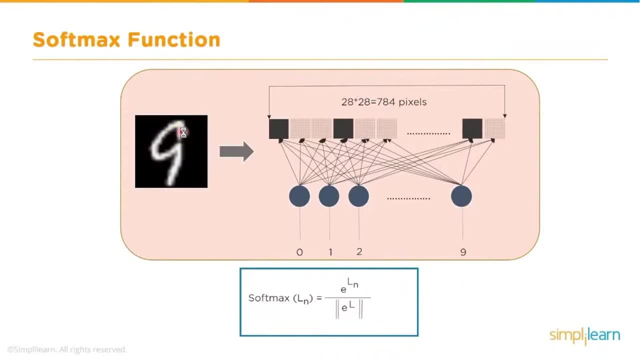 Now let's say you feed one to the trained network, then this neuron will get activated. If you feed two, this neuron will get activated, and so on. I hope you get the idea. So this is one. This is one type of a neural network or an activation function known as softmax layer. 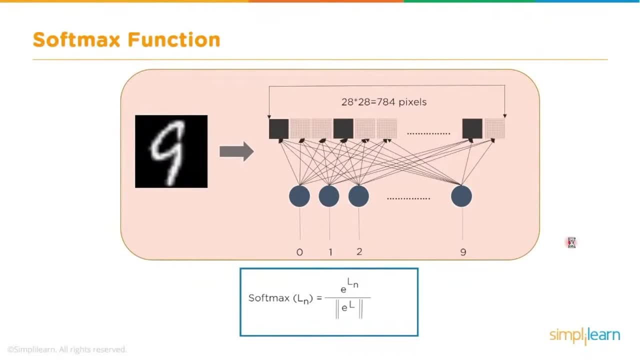 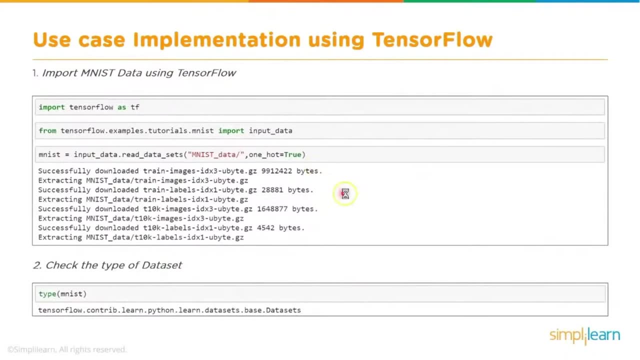 So that's what we will be using here. This is one of the simpler ones for quick and easy understanding. So this is how the code would look. We will go into our lab environment in the cloud and we will show you there directly, But very quickly. this is how the code looks. 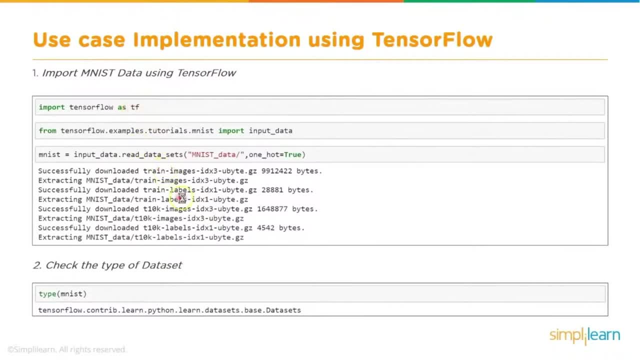 And let me run you through briefly here, and then we will go into the Jupyter notebook where The actual code is, and we will run that as well. So as a first step, first of all, we are using Python here And that's why the syntax of the language is Python. 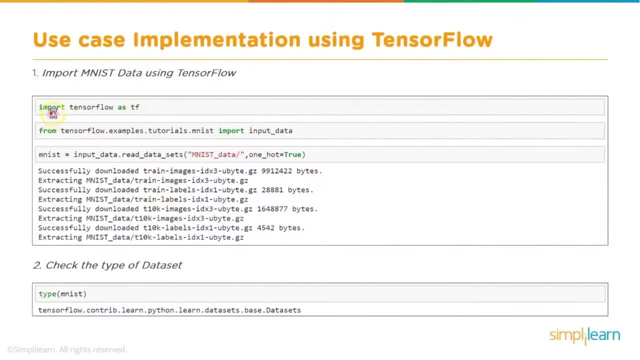 And the first step is to import the TensorFlow library. So, and we do this by using this line of code saying: import TensorFlow as tf. tf is just for convenience, So you can name, give any name, and once you do this, tf is, TensorFlow is available as an 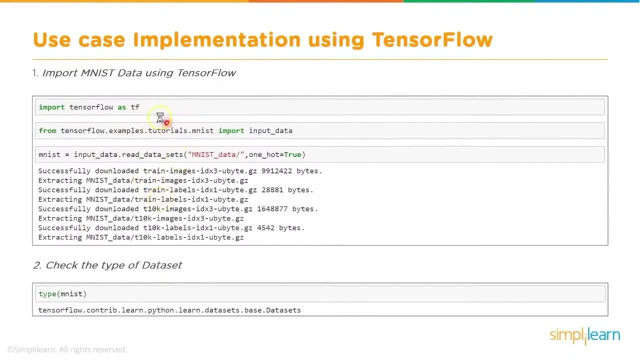 object in the name of tf And then you can run its methods and accesses its attributes and so on and so forth. And MNIST database is actually an integral part of TensorFlow And that's again another reason why we, as a first step, we always use this example: MNIST. 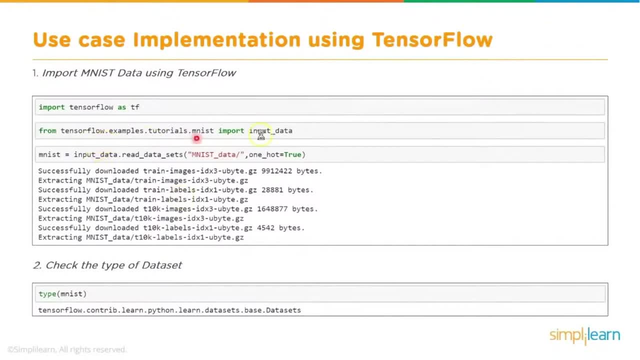 database example. So you just simply import MNIST database as well using this line of code And you slightly modify this so that the labels are in this format, what is known as one hot true, Which means that the label information is stored like an array. 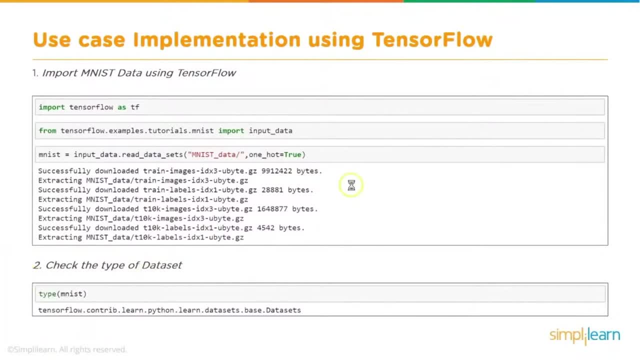 And let me just use the pen to show what exactly it is. So when you do this, one hot true. what happens is each label is stored in the form of an array of 10 digits, And let's say the number is eight. Okay, so in this case, all the remaining values- there will be a bunch of zeros. 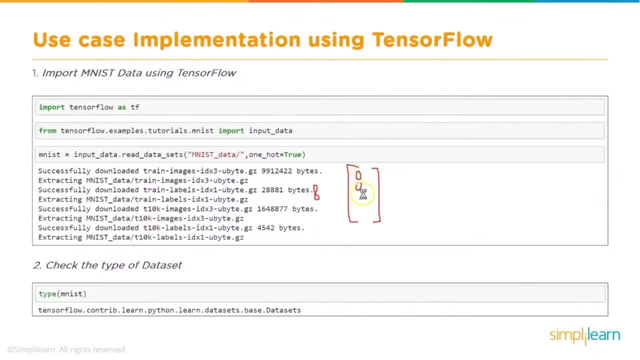 This is like array at position zero, this is at position one, position two and so on and so forth. Let's say this is position seven, then this is position eight, that will be one because our input is eight, And again position nine will be zero. 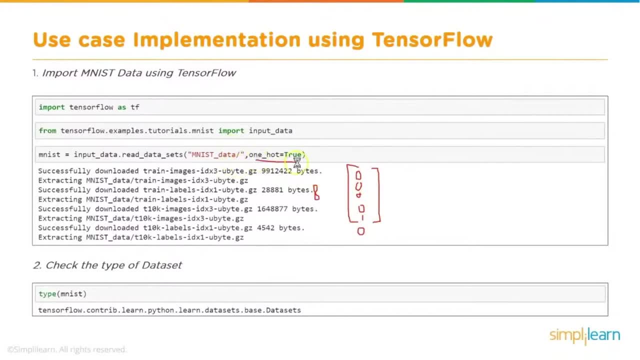 Okay, so one hot encoding, this one hot encoding true will kind of load the data in such a way that the labels are in such a way that only one of the digits has a value of one And that indicates so based on which digit is one. we know what is the label. 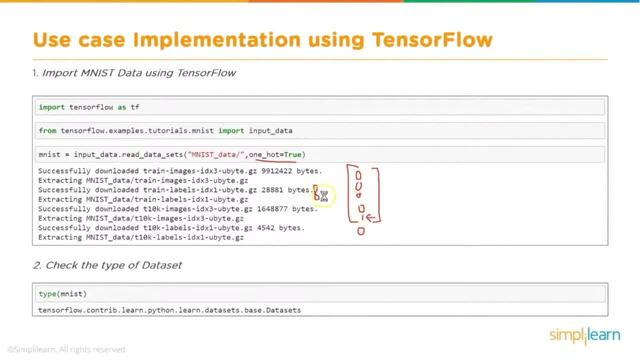 So in this case, the eighth position is one. therefore, we know this sample data. the value is eight. Similarly, if you have a two here, let's say, then the label information will be somewhat like this: So you have your labels. 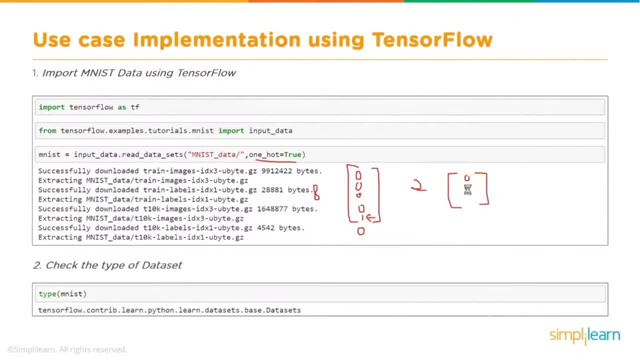 So you have this as zero, the zero position. the first position is also zero, the second position is one, because this indicates number two, And then you have third as zero, and so on. Okay, so that is the significance of this one hot true. 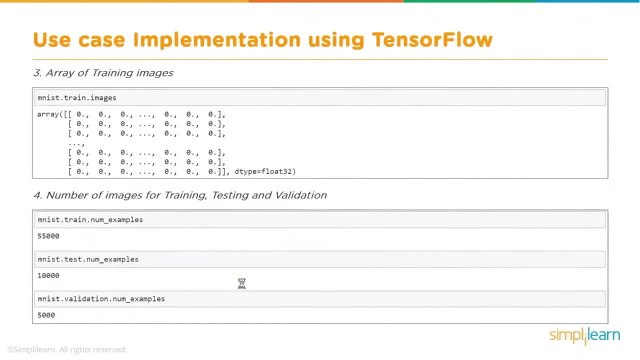 All right, and then we can check how the data is looking by displaying the data And, as I mentioned earlier, this is pretty much in the form of digital form, like numbers, So all these are like pixel values, So you will not really see an image in this format. 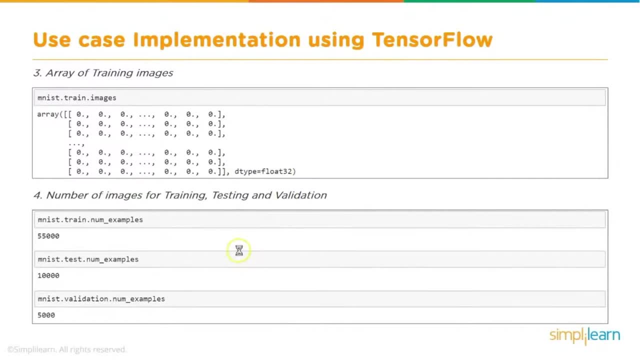 But there is a way to visualize that image. I will show you in a bit And this tells you how many images are there in each set. So the training: there are 55,000 images in training and in the test set there are 10,000. 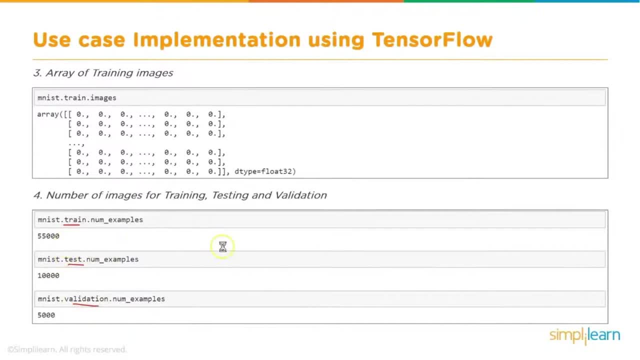 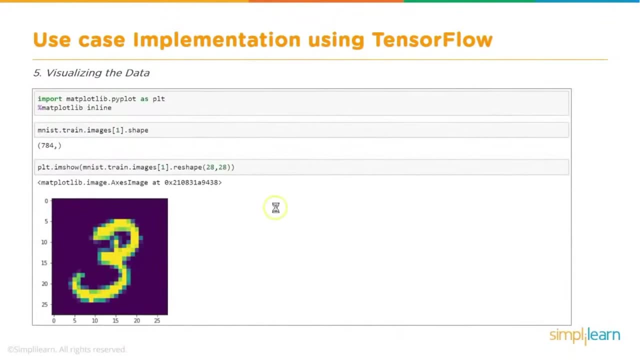 And then validation. there are 5000.. So altogether there are 70,000 images. alright, so let's move on. And we can view the actual image by using the matplotlib library, And this is how you can view. this is the code for viewing the images. 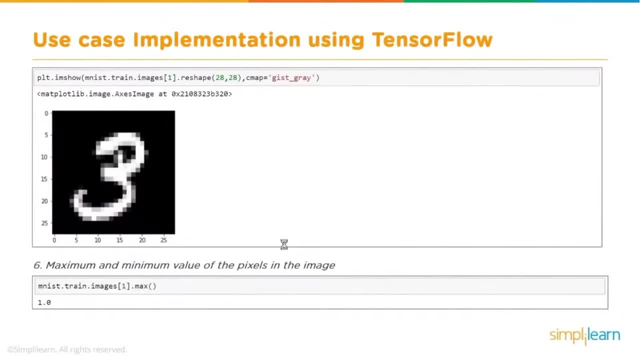 And you can view them in color or you can view them in grayscale. So the C map is what tells in what way we want to view it and what are the maximum values and the minimum values of the pixel values. So these are the max and minimum value so of the pixel values. 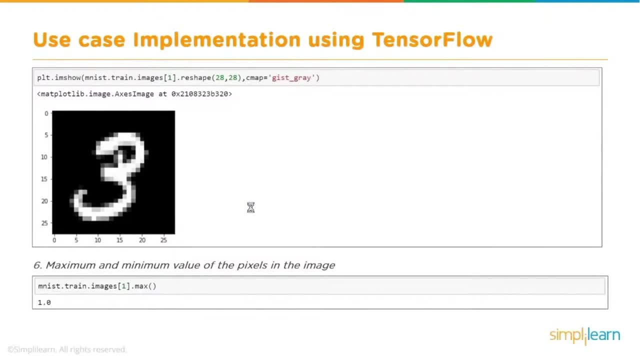 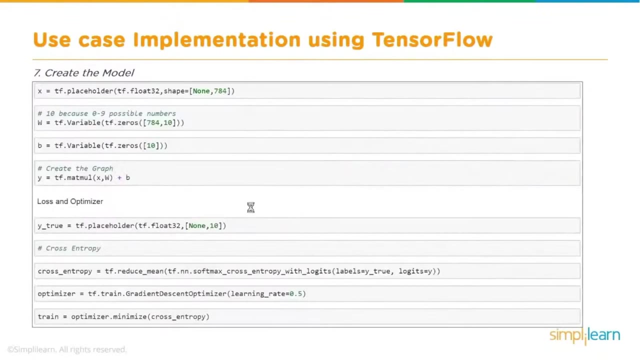 So maximum is one because this is a scaled value. So one means it is white and zero means it is black. and in between, is it Okay, It can be anywhere in between black and white And the way to train the model. there is a certain way in which you write your TensorFlow. 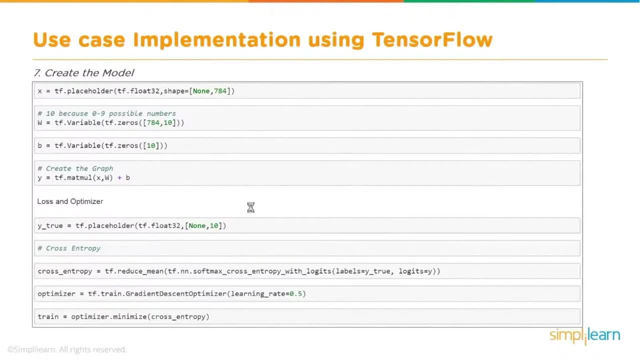 code And the first step is to create some placeholders and then you create a model. In this case we will use the softmax model, one of the simplest ones, and placeholders are primarily to get the data from outside into the neural network. So this is a very common mechanism that is used. 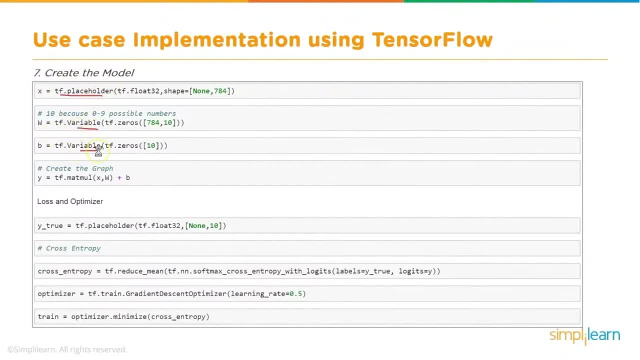 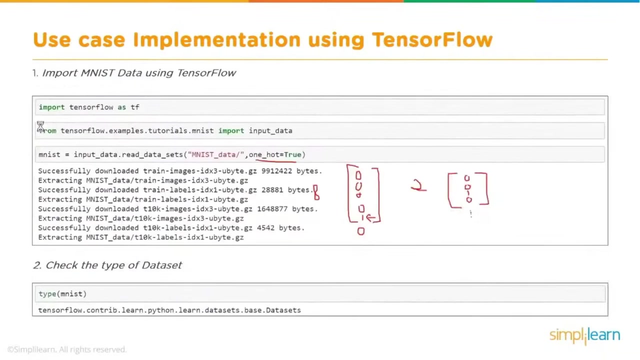 And then, of course, you will have variables Which are your. remember, these are your weights and biases. So far. in our case, there are 10 neurons and each neuron actually has 784, because each neuron takes all the inputs. If we go back to our slide here, actually every neuron takes all the 784 inputs, right? 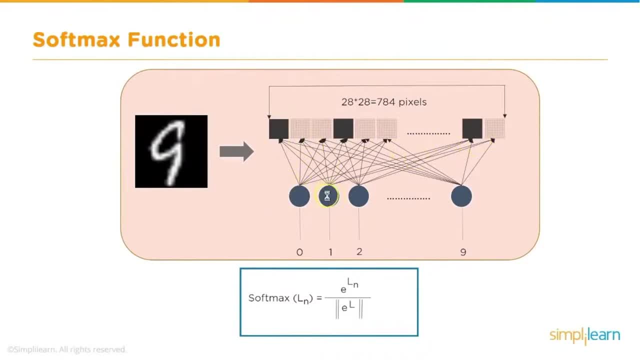 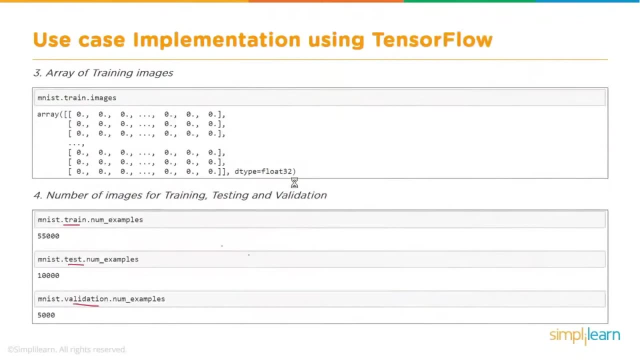 This is the first neuron it has. it receives all the 784,. this is the second neuron. this also receives all the 784.. So each of these inputs, This needs to be multiplied with the weight, And that's what we are talking about here. 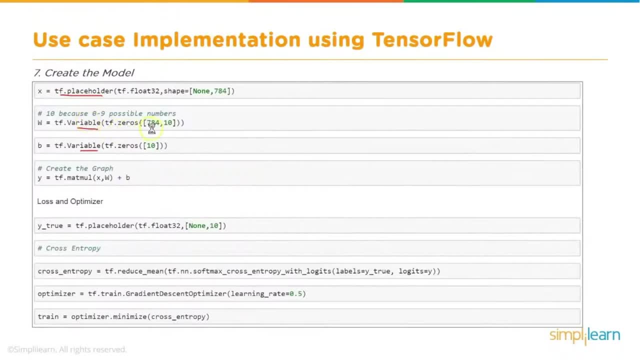 So these are. this is a matrix of 784 values for each of the neurons, And so it is like a 10 by 784 matrix, because there are 10 neurons And similarly there are biases. Now, remember I mentioned biases- only one per neuron, so it is not one per input. 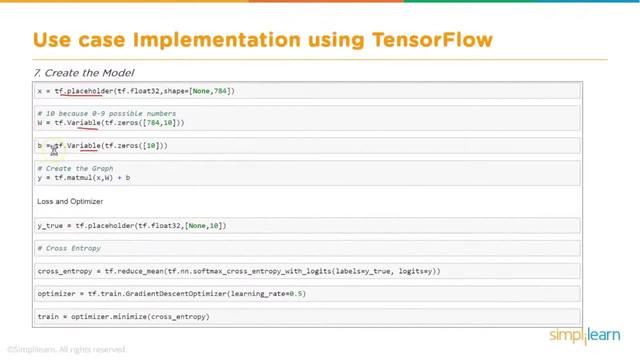 Unlike the weights. So therefore there are only 10 biases, because there are only 10 neurons in this case. So that is what we are creating: a variable for biases. So this is something little new in TensorFlow, You will see, unlike our regular programming languages where everything is a variable here. 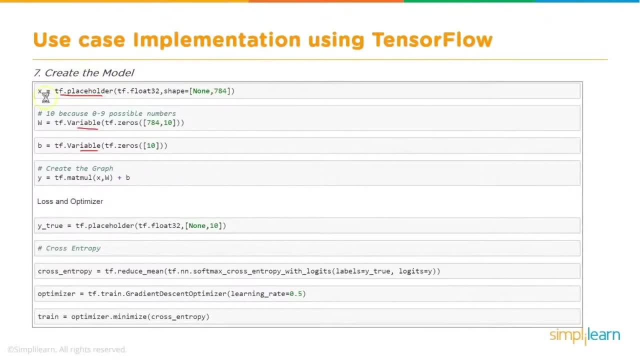 the variables can be of three different types. You have placeholders, which are primarily used for feeding data. you have variables which can change during the course of computation, And then a third type, which is not shown here, are constants. So these are like fixed numbers, all right. 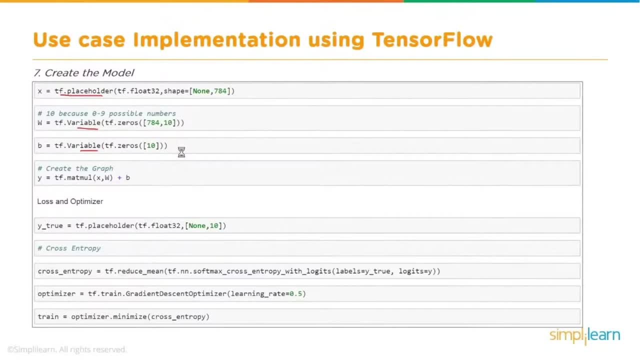 So in a regular programming language you may have everything as variables or, at the most, variables and constants. But in TensorFlow you have three different types: placeholders, variables and constants, And then you create what is known as a graph. So TensorFlow programming consists of graphs and tensors, as I mentioned earlier. 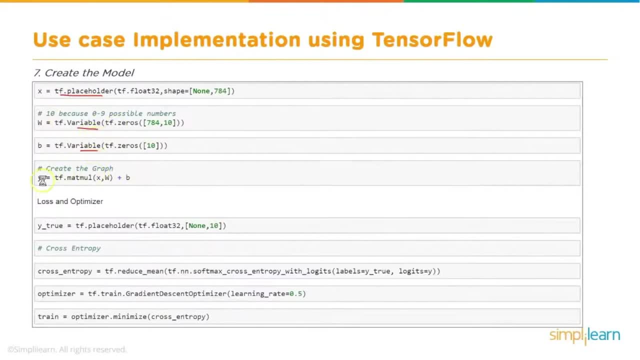 So this can be considered ultimately as a tensor, And then the graph tells how to execute the whole implementation, so that the execution is stored in the form of a graph, And in this case what we are doing is we are doing a multiplication tf, you remember? 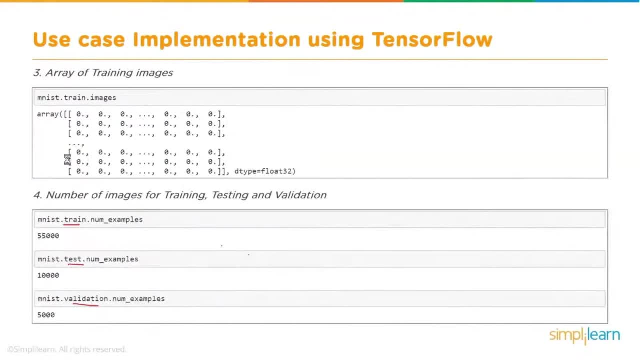 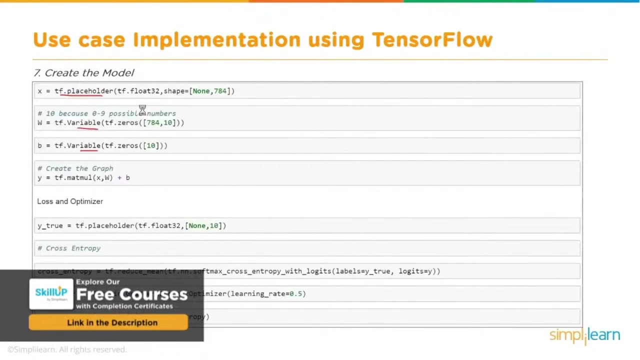 this tf was created as a TensorFlow object. here one more level, one more. So tf is available here Now. TensorFlow has what is known as a matrix multiplication or matmul function, So that is what is being used here in this case. So we are using the matrix multiplication of TensorFlow so that you multiply your input. 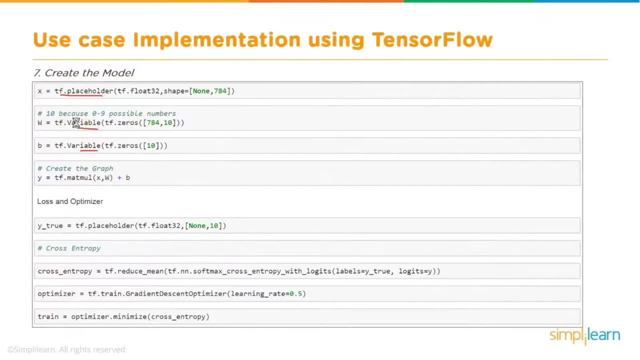 values x with w. right, this is what we were doing: x, w plus b. you're just adding b, And this is very similar to one of the earlier slides where we saw sigma xi, wi. So that's what we are doing here. 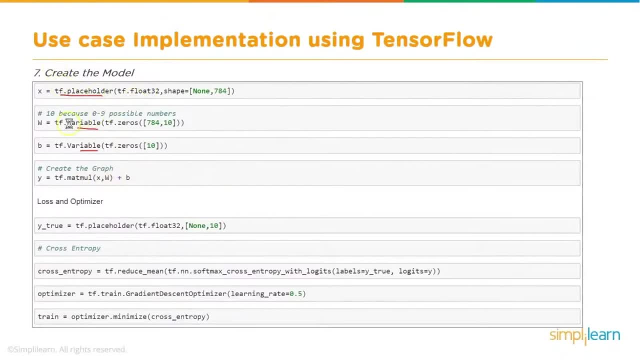 Matrix multiplication is multiplying all the input values with the corresponding weights and then adding the bias. So that is the graph We created, and then we need to define what is our loss function and what is our optimizer. So in this case, we again use the TensorFlow APIs. 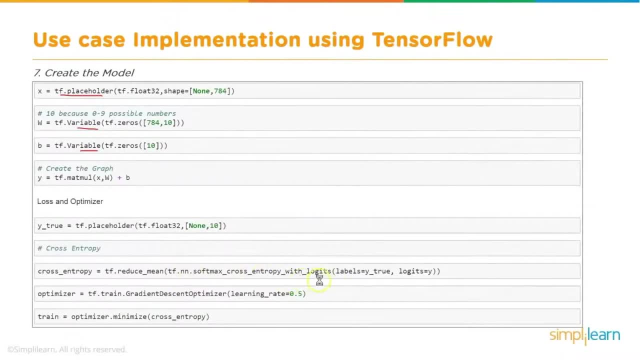 So tf, dot nn, softmax cross entropy with logits is the API that we will use and reduce mean is what is like the mechanism whereby which says that you reduce the error, and optimizer for doing reduction of the error. What optimizer are we using? So we are using gradient descent optimizer. 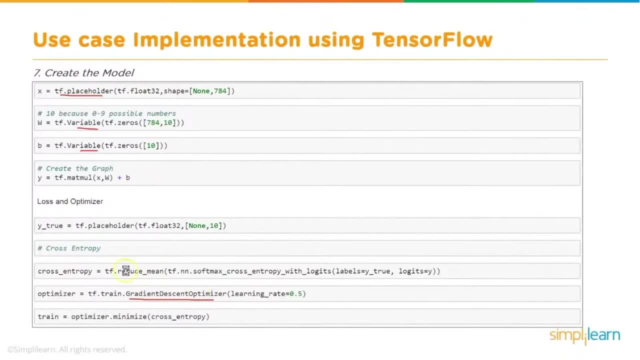 We discussed about this in a couple of slides earlier- and for that you need to specify the learning rate. You remember we saw that there was a slide somewhat like this- and then you define what should be the learning rate, how fast you need to come down. 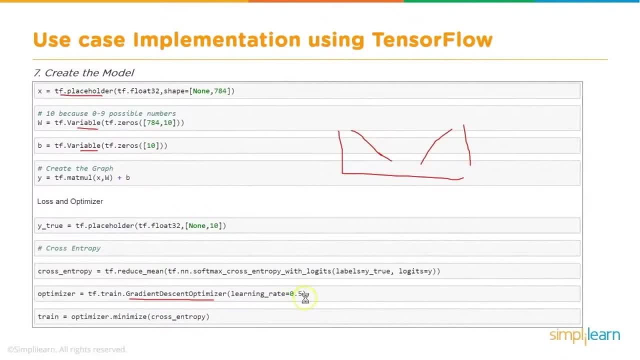 That is the learning rate and this again needs to be tested and tried and to find out the optimum level of this learning rate. Okay, So the learning rate. it shouldn't be very high, in which case it will not converge, or shouldn't be very low, because it will. in that case it will take very long. 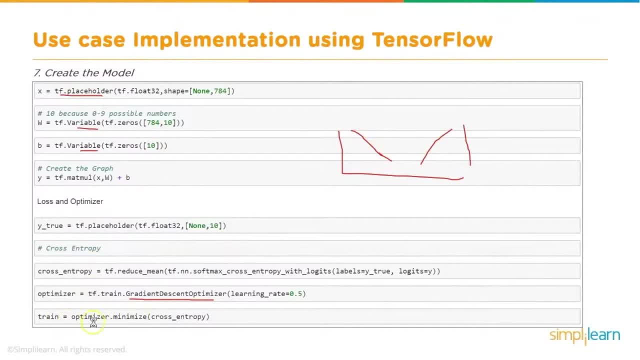 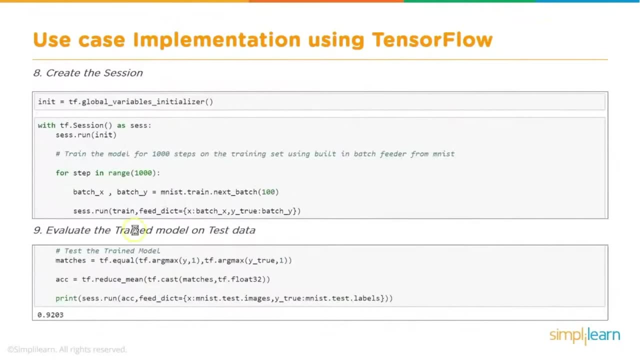 So you define the optimizer and then you call the method minimize for that optimizer and that will kickstart the training process. And so far we've been creating the graph and in order to actually execute that graph, we create what is known as a session and then we run that session and once the training 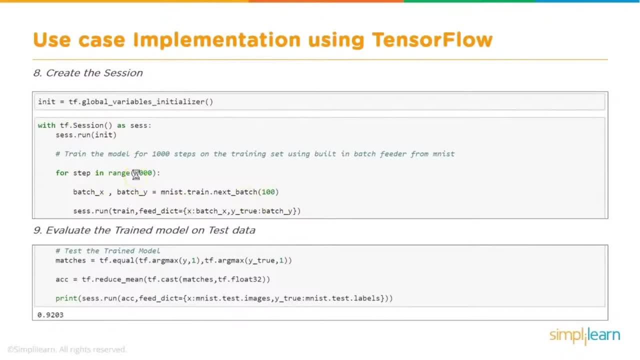 is completed. We specify how many times, how many iterations we want it to run. So for example, in this case we are saying thousand steps. So that is a exit strategy in a way. So you specify the exit condition, So training will run for thousand iterations, and once that is done we can then evaluate. 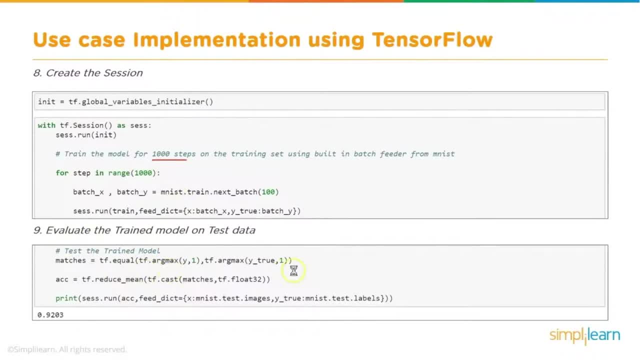 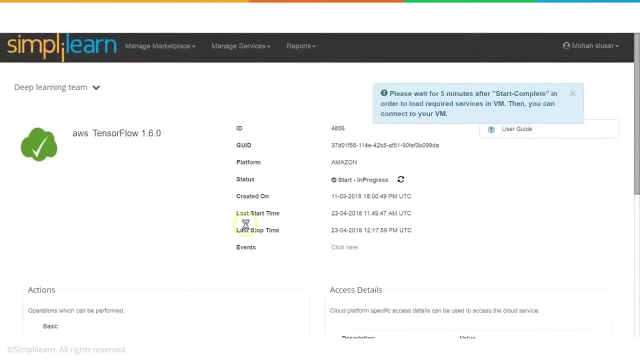 the model using some of the techniques shown here. So let us get into the code quickly and see how it works. So this is our cloud environment. Okay, Now you can install TensorFlow on your local machine as well. I'm showing this demo on our existing cloud, but you can also install TensorFlow on your. 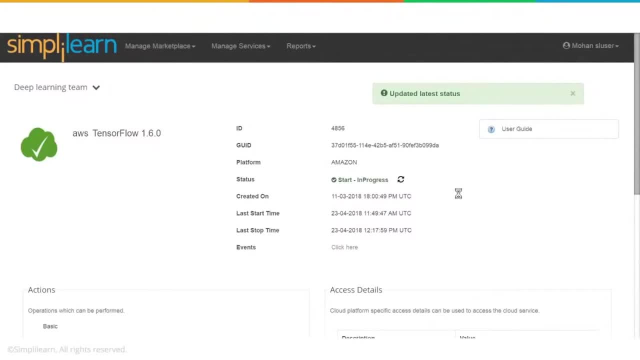 local machine and there is a separate video on how to set up your TensorFlow environment. You can watch that if you want to install your local environment, or you can go for other. any cloud service, like, for example, Google Cloud, Amazon or Cloud Labs- any of these. 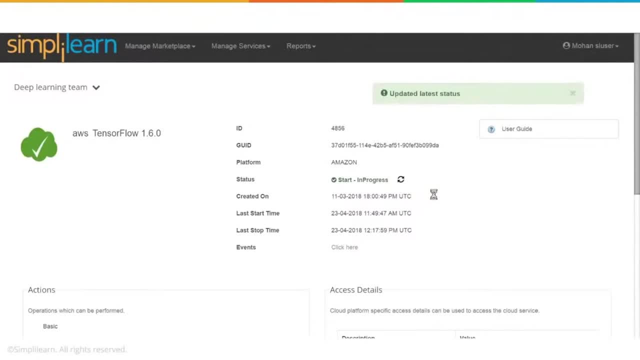 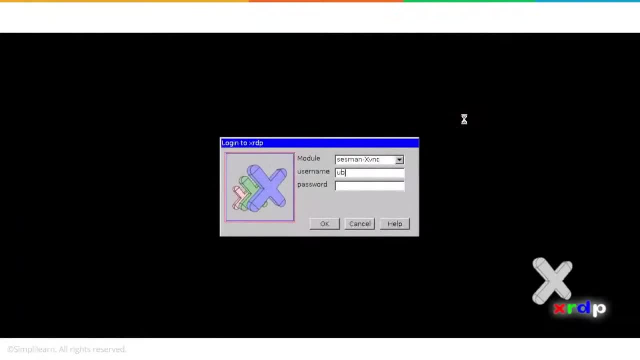 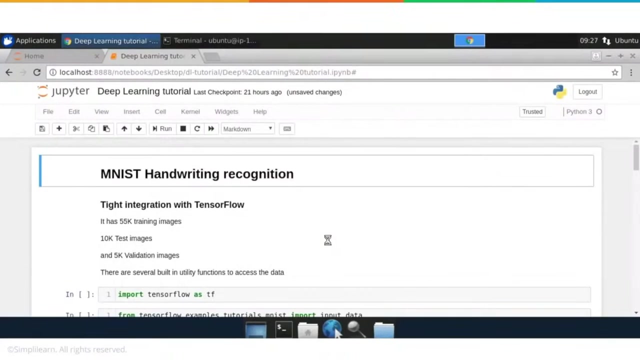 you can use, Use and run and try the code. Okay, So it has got started. We log in. All right, So this is our deep learning tutorial code and this is our TensorFlow environment. And so let's get started. The first: we have seen a little bit of code. 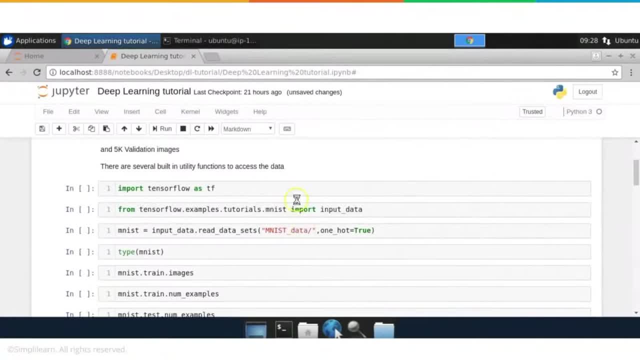 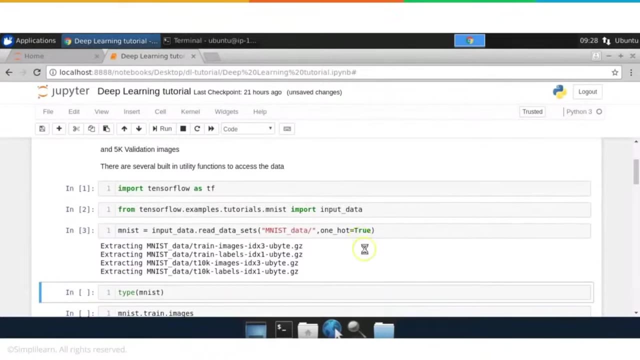 Walkthrough in the slides as well. Now you will see the actual code in action. So the first thing we need to do is import TensorFlow, and then we will import the data, and we need to adjust the data in such a way that the one hot is encoding is set to true. 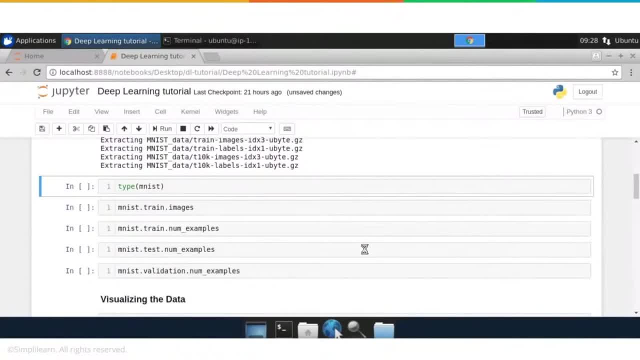 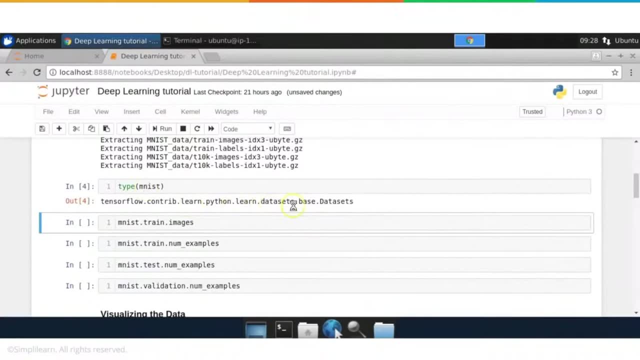 one hot encoding right, As I explained earlier. So in this case the label values will be shown appropriately And if we just check what is the type of the data, so you can see that this is a data set. So we have Python data sets, Python data sets. 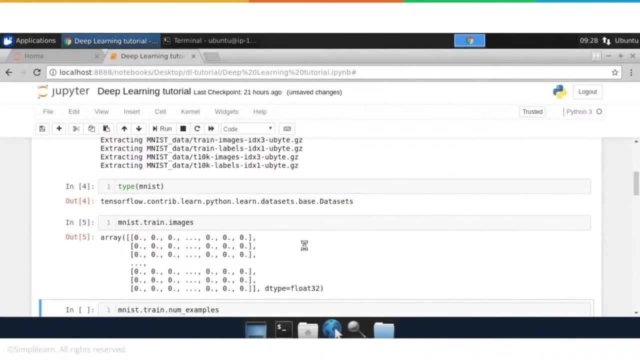 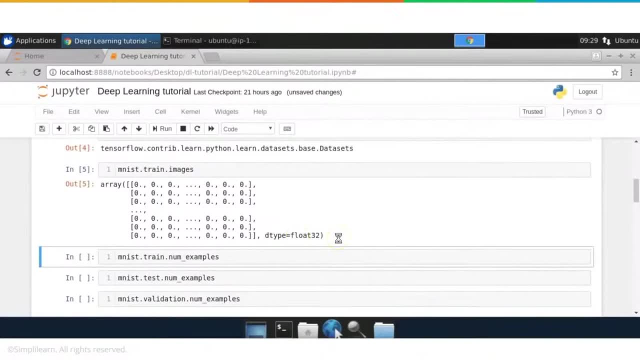 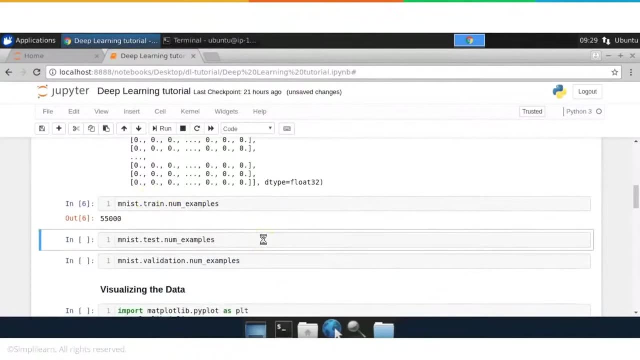 And if we check the number of images, the way it looks. this is how it looks. It is an array of type float 32.. Similarly, the number, if you want to see what is the number of training images, there are 55,000, and there are test images- 10,000, and then validation images- 5000. 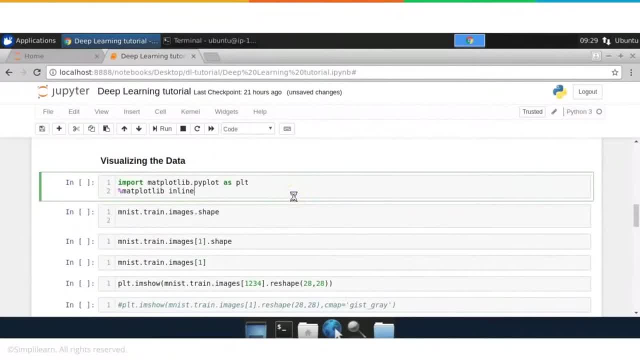 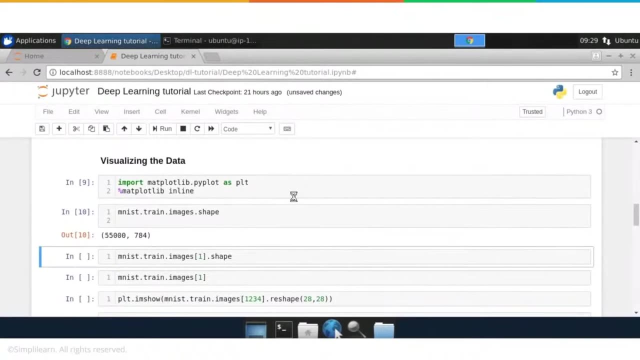 Now let's take a quick look at the dataset, At the data itself, visualization, so we will use matplotlib for this. And if we take a look at the shape now, shape gives us like the dimension of the tensors, or the arrays, if you will. 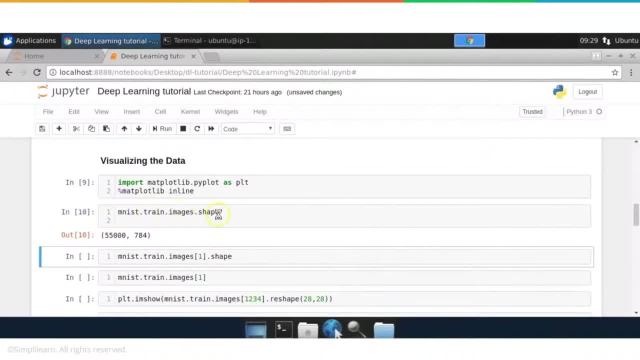 So, in this case, the training data set. if we see the size of the training data set using the method shape, it says there are 55,000 and 55,000 by 784.. So remember, the 784 is nothing but the 28.. 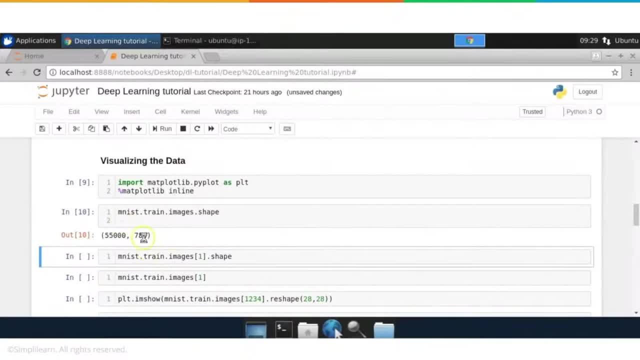 28 by 28,, 28 into 28.. So that is equal to 784.. So that's what it is showing. Now we can take just one image and just see what is the, the first image and see what is the shape. 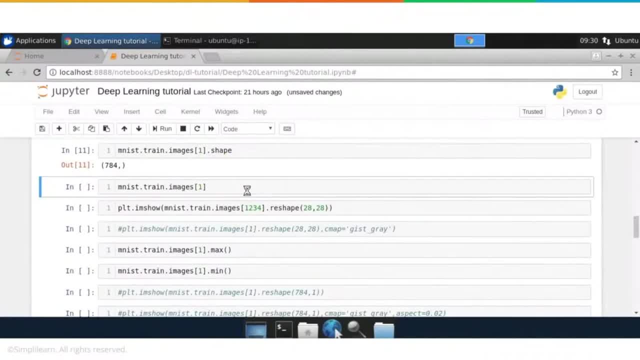 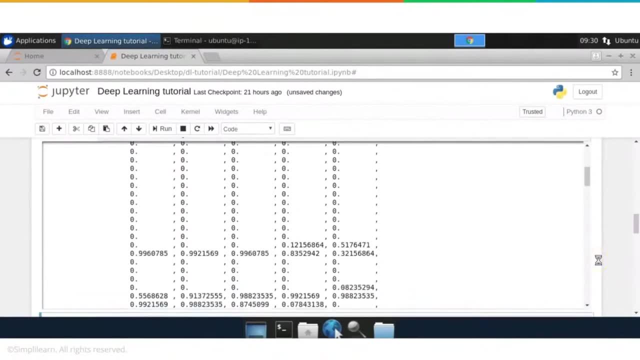 So again, size: obviously it is only 784.. Similarly, you can look at the image itself, the data of the first image itself. So this is how it shows. So large part of it will probably be zeros because, as you can imagine in the image, 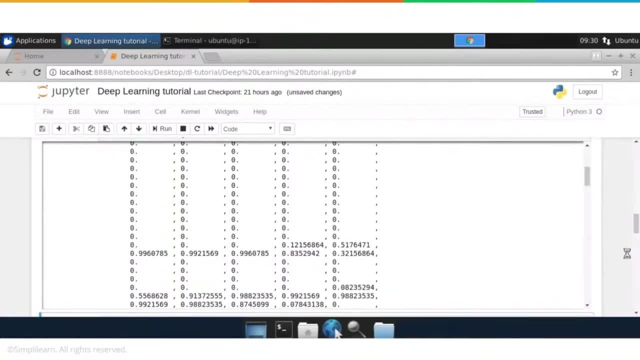 only certain areas are written, rest is black. So that's why you will mostly see zeros. either it is black or white. But then there are these values are. so the values are actually. they are scaled, So their values are between zero and one. 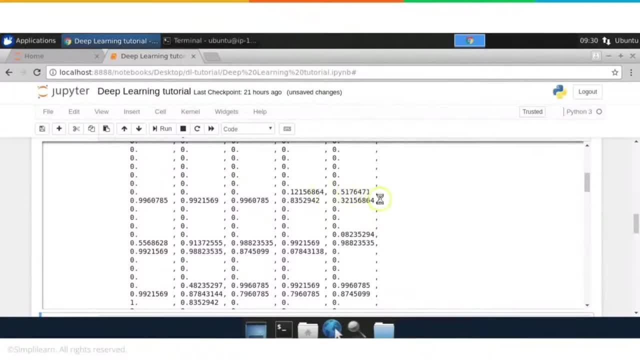 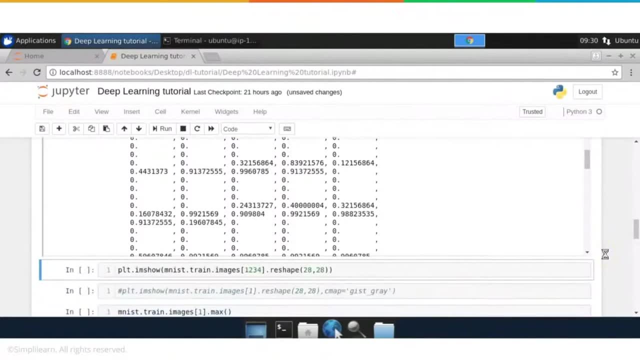 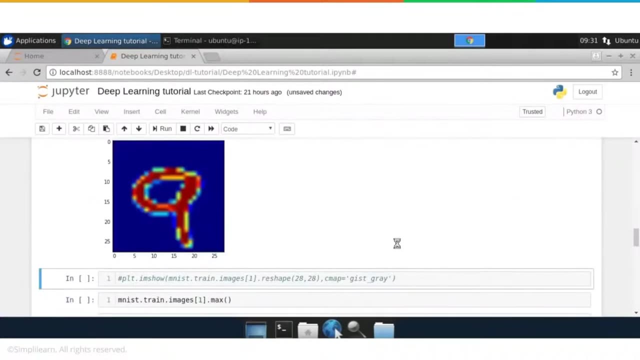 Okay, so this is what you're seeing. So certain locations there are some values and then other locations there are zeros. So that is how the data is stored and loaded If we want to actually see what is. Okay. So this is the value of the handwritten image. 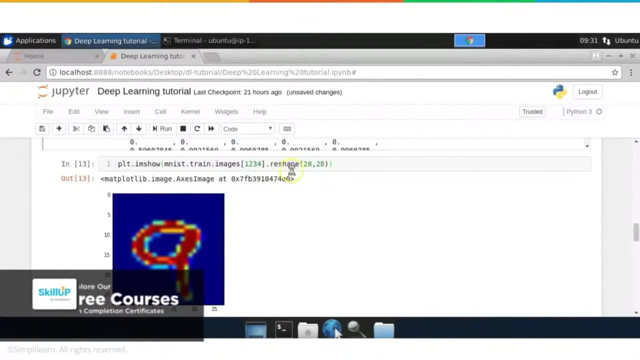 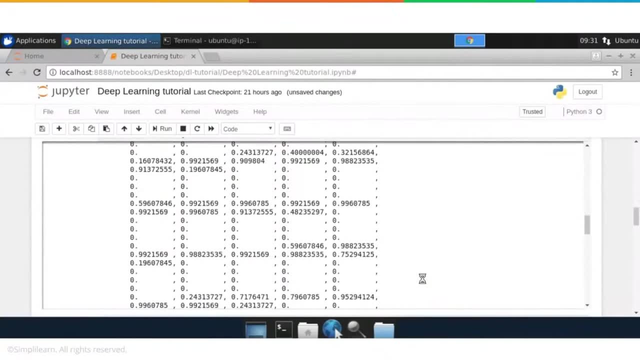 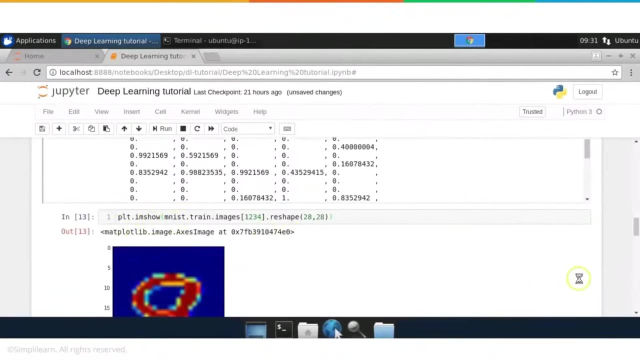 If you want to view it, this is how you view it. So you create, like, do this reshape, and matplotlib has this feature to show you these images. So we will actually use the function called I am sure And then, if you pass this parameters appropriately, you will be able to see the different images. 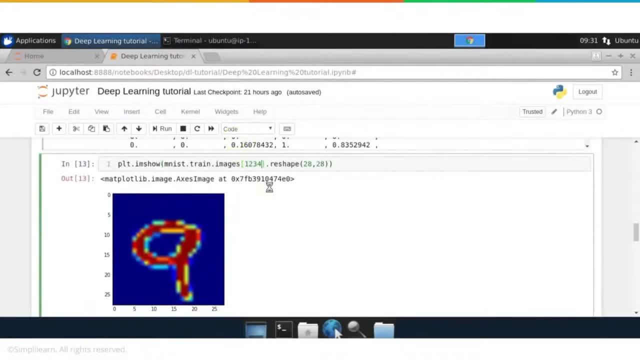 Now I can change the values in this position. So which image we are looking at? right, so we can say: if I want to see what is there in, maybe 5000.. Right, So 5000 has three. Similarly, you can just say five. what is in five, five as eight, what is in 50.. 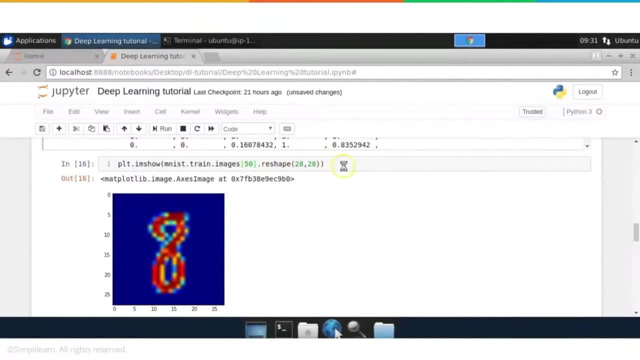 Again, eight. So basically, by the way, if you're wondering how I'm executing this code, shift enter- it is a little bit difficult, Okay. Okay. So, in case you're not familiar with Jupyter notebooks, shift enter is how you execute each cell, individual cell. 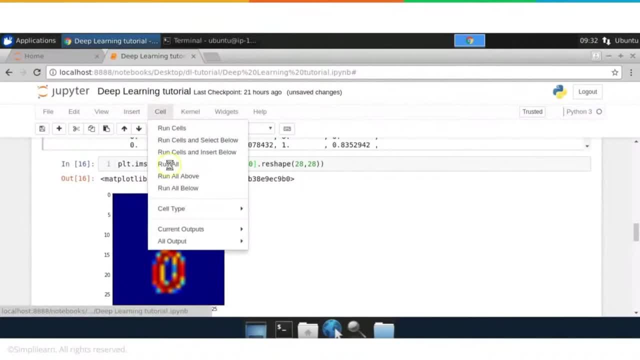 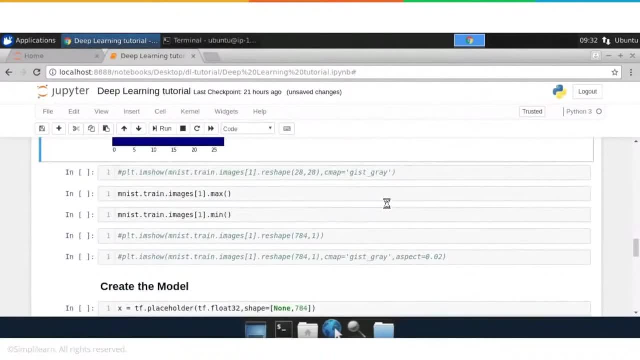 And if you want to execute the entire program, you can go here and say run all. So that is how this code gets executed And here again we can check what is the maximum value and what is the minimum value of this pixel values. 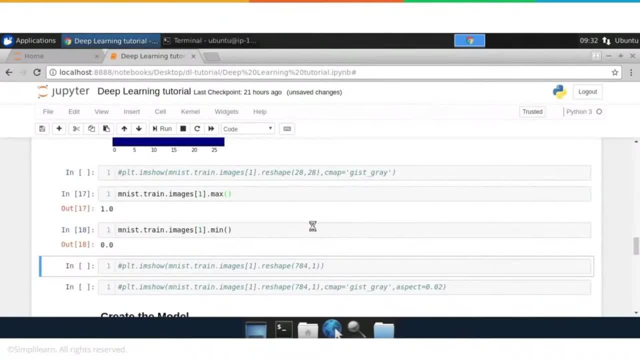 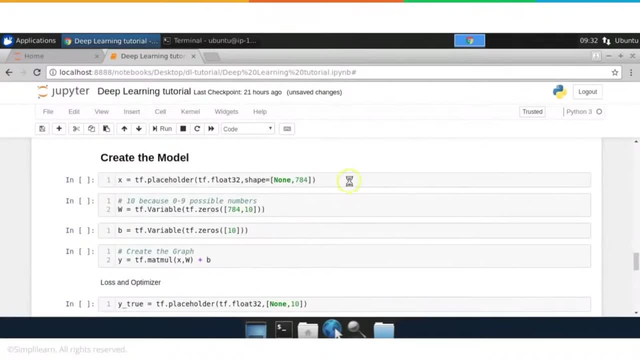 As I mentioned, this is: it is scaled, So therefore it is between. the values lie between one and zero. Now this is where we create our model. The first thing is to create the required placeholders and variables, And that's what we are doing here, as we have seen in the slides. 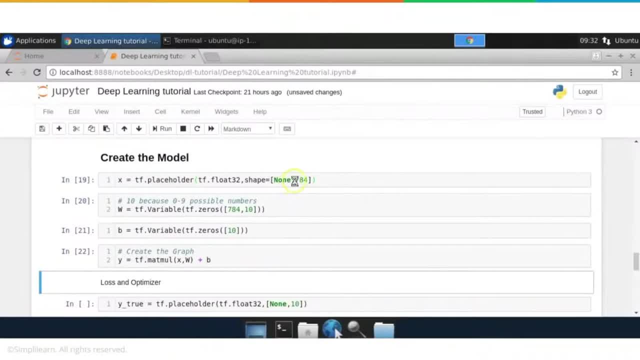 So we create one placeholder and we create two variables, which is for the weights and biases. These two variables are actually matrices, So each variable has 784 by 10.. So values, okay. so one for this. 10 is for each neuron- there are 10 neurons- and 784 is for the pixel values, inputs that are given, which is 28 into 28.. 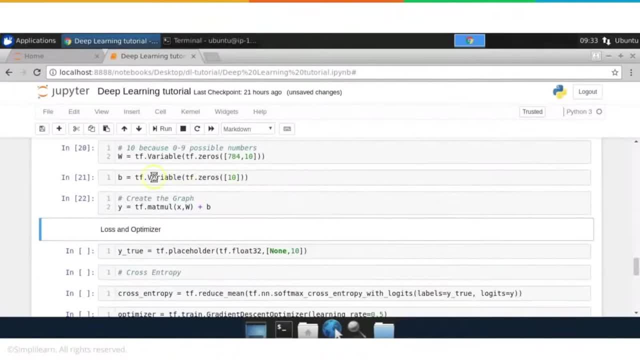 And the biases, as I mentioned, one for each neuron, so there will be 10 biases. they are stored in a variable by the name B And this is the graph which is basically the multiplication of these matrix. multiplication of x into w. 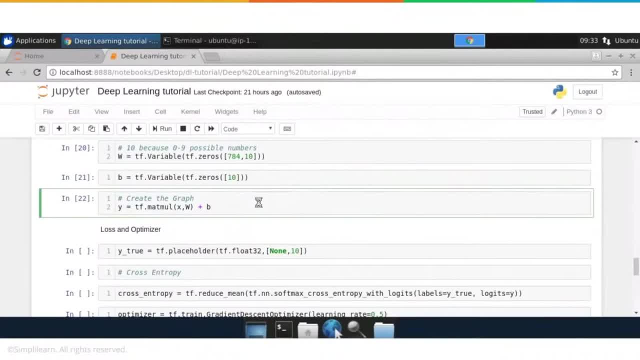 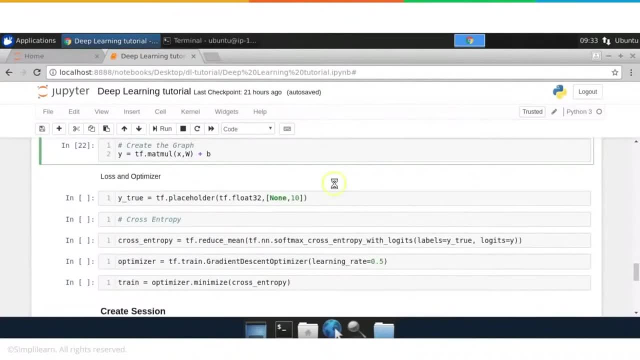 And then the bias is added for each of the neurons, And the whole idea is to minimize the error. So let me just execute. I think this code is executed. then we define what is our. the y value is basically the label value. So this is another placeholder. we had x as one placeholder and y underscore, true, as a second placeholder. 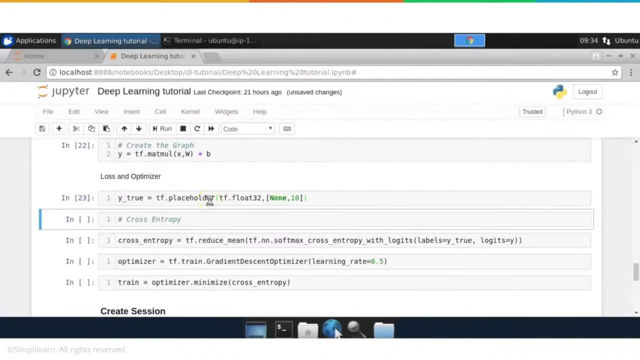 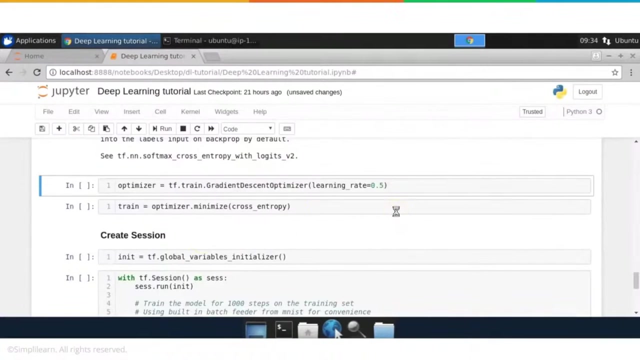 And this will have values in the form of 10 digit, 10 digit arrays, And since we said one hot encoded the position which has a one value indicates what is the label for that particular number. All right, then we have cross entropy, which is nothing but the loss loss function. 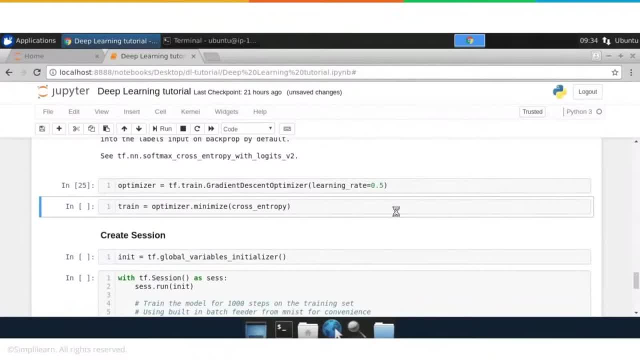 And we have the optimizer. we have chosen gradient descent as our optimizer, then the training process itself. So the training process is nothing but to minimize the cross entropy, which is again nothing but the loss function. So we define all of this in the form of a graph. 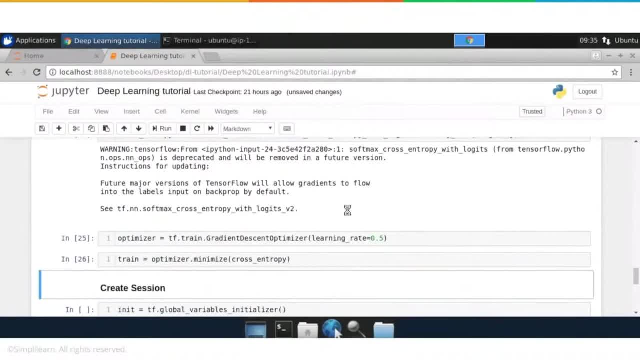 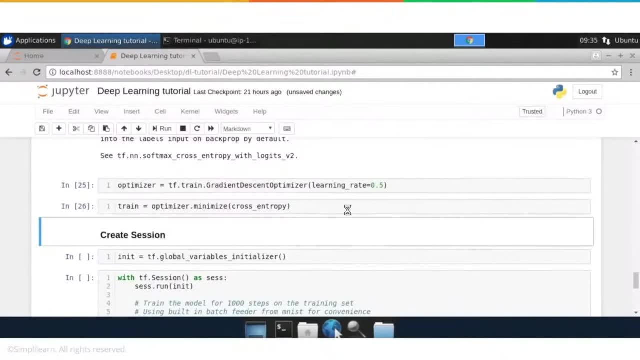 So the up to here remember what we have done is we have not exactly executed any TensorFlow code till now. we are just preparing the graph, the execution plan. That's how the TensorFlow code works. So the whole structure and format of this code. 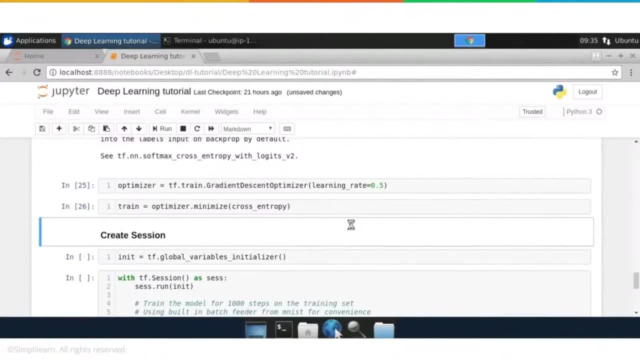 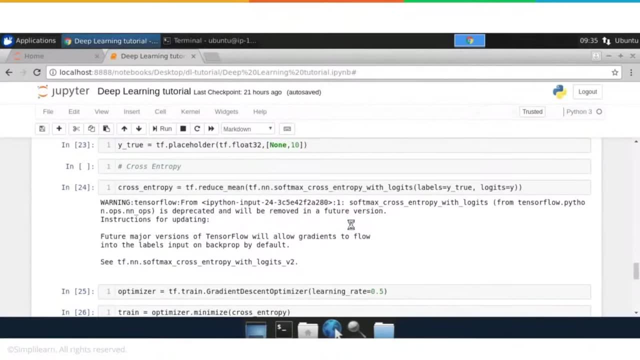 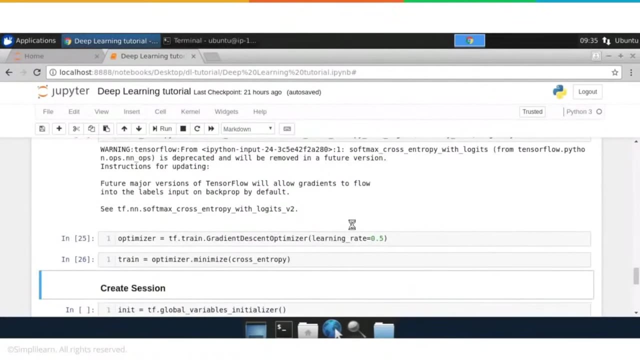 Will be completely different from how we normally do programming. So even with people with programming experience may find this a little difficult to understand it and it needs quite a bit of practice. So you may want to view this video also, maybe a couple of times, to understand this flow. 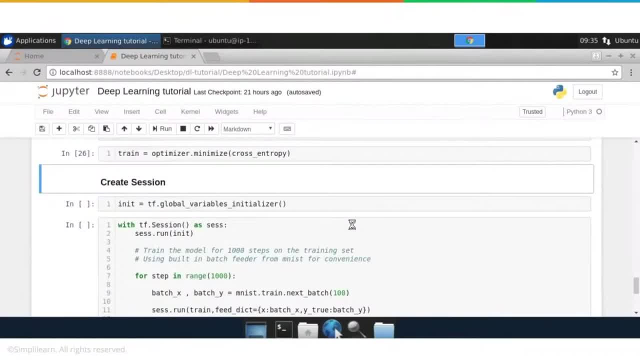 Because the way TensorFlow programming is done is slightly different from the normal programming. Some of you who, let's say, have done maybe Spark programming to some extent, will be able to easily understand this. But even in Spark, the programming, the code itself, is pretty straightforward. 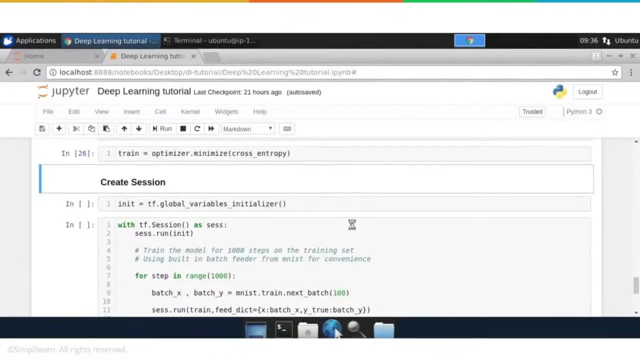 Behind the scenes the execution happens slightly differently, But in TensorFlow even the code has to be written in a completely different way, So the code doesn't get executed in the same way as you have written. So that that's something you need to understand. 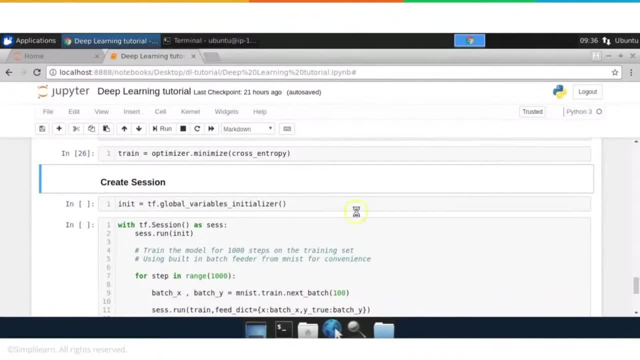 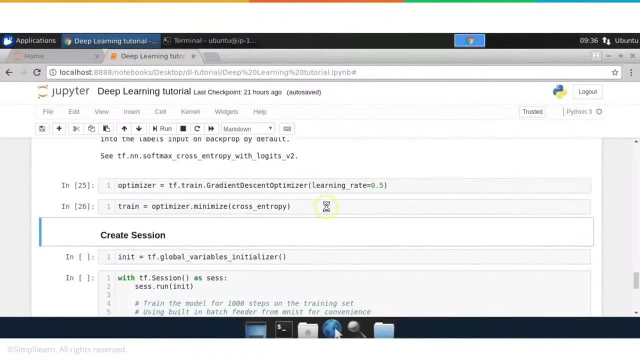 And a little bit of practice is needed For this. So so far, what we have done up to here is creating the variables and feeding the variables, and rather not feeding but setting up the variables and the graph. That's all defining, maybe, the what kind of a network you want to use. 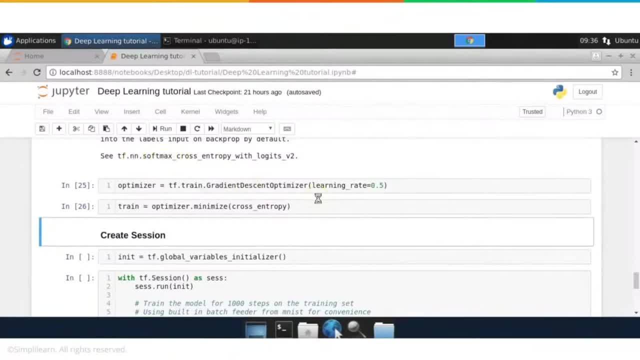 For example, we want to use Softmax and so on. So you have created the variables, have to load the data, loaded the data, viewed the data and prepared everything. But you have not yet done that, You have not yet executed anything in TensorFlow. 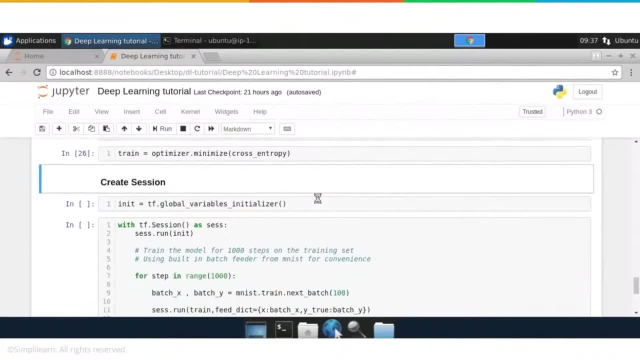 Now the next step is the execution in TensorFlow. So the first step for doing any execution in TensorFlow is to initialize the variable. So anytime you have any variables defined in your code, you have to run this piece of code always. So you need to basically create what is known as a node for initializing. 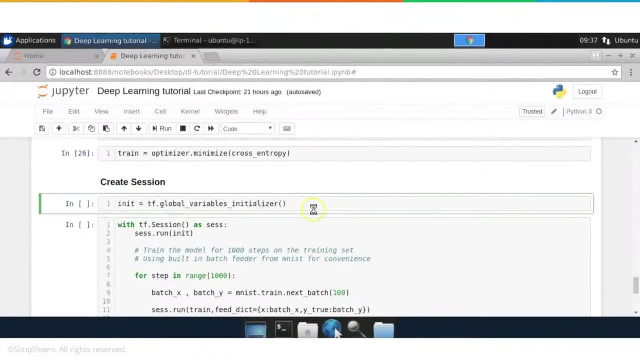 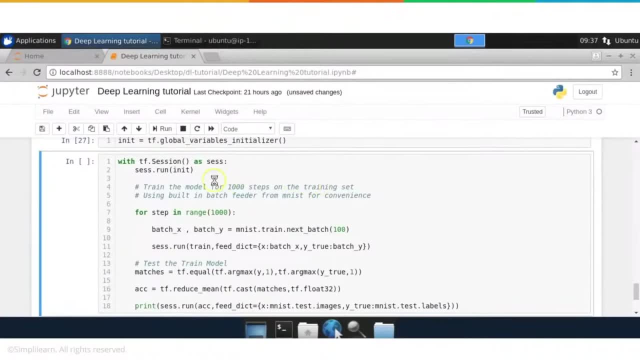 So this is a node. You still are not yet executing anything here. You just created a node, You just created a node for the initialization, So let us go ahead and create that, And here onwards is where you will actually execute your code in TensorFlow. 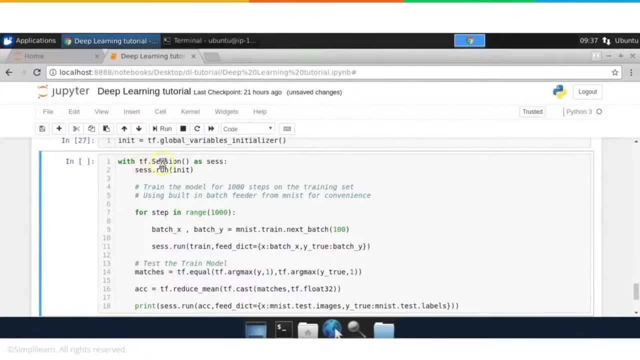 And in order to execute the code, what you will need is a session, TensorFlow session. So tfsession will give you a session, And there are a couple of different ways in which you can do this, But one of the most common methods of doing this is: 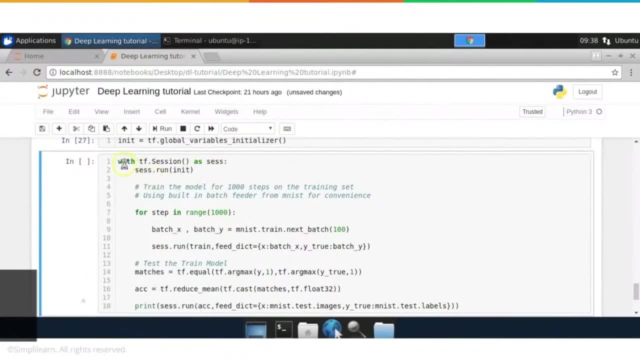 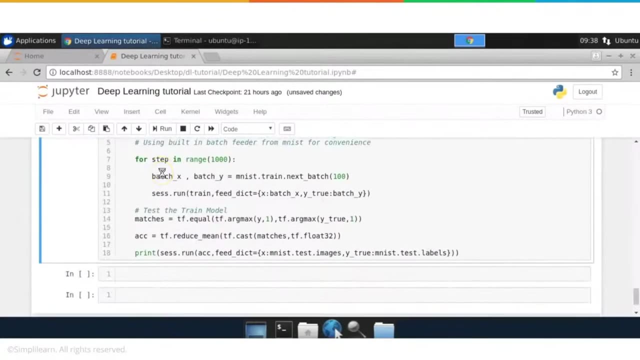 with what is known as a with loop. So you have a with tfsession as sess and with a colon here And this is like a block starting of the block, And these indentations tell how far this block goes And this session is valid till this block gets executed. 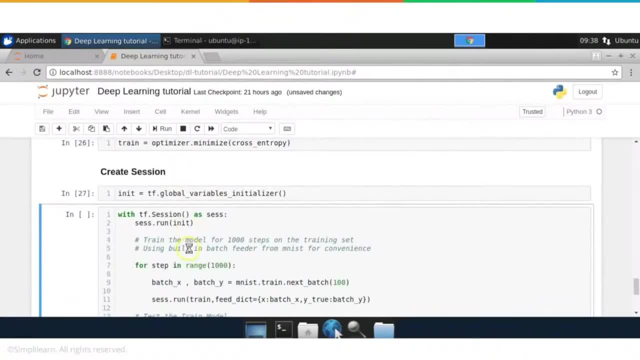 So that is the purpose of creating this with block. This is known as a with block, So with tfsession. As sess, You say sessrun in it. Now sessrun will execute a node that is specified here. So, for example, here we are saying sessrun. 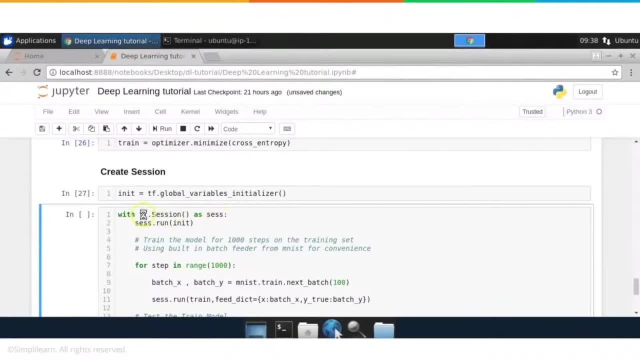 Sess is basically an instance of the session, Right? So here we are saying tfsession, So an instance of the session gets created and we are calling that sess, And then we run a node within that, One of the nodes in the graph. 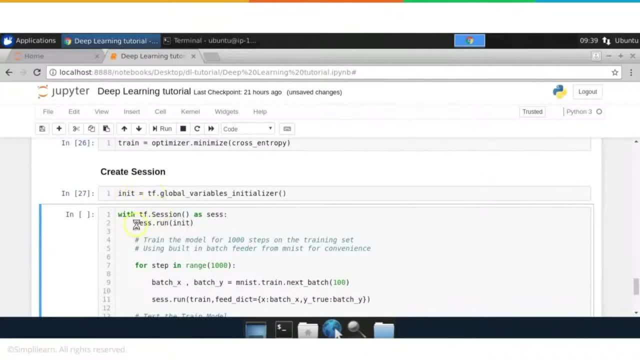 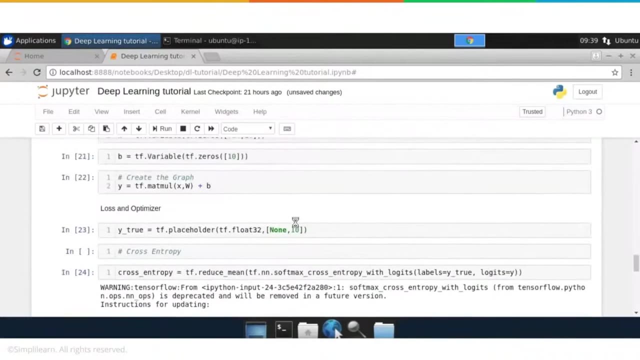 So one of the nodes here is in it. So we say, run that particular node And that is when the initialization of the variables happens. Now what this does is if you have any variables in your code. In our case we have: w is a variable and b is a variable. 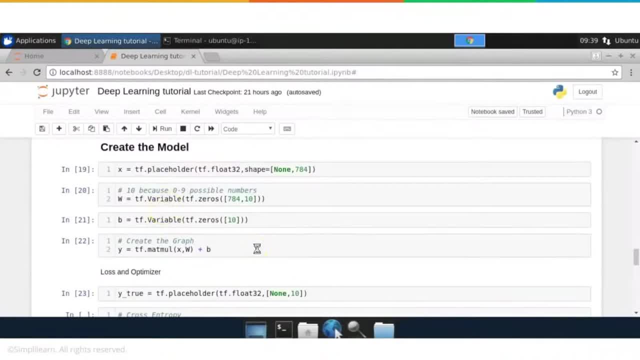 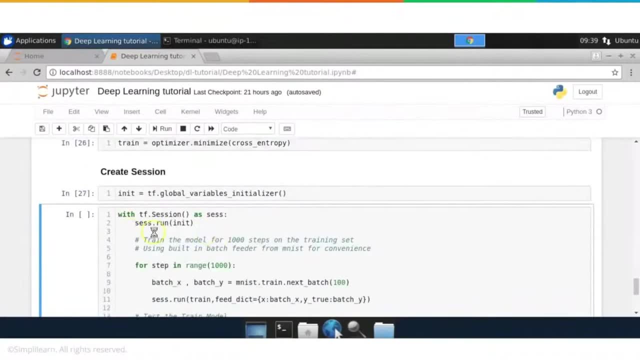 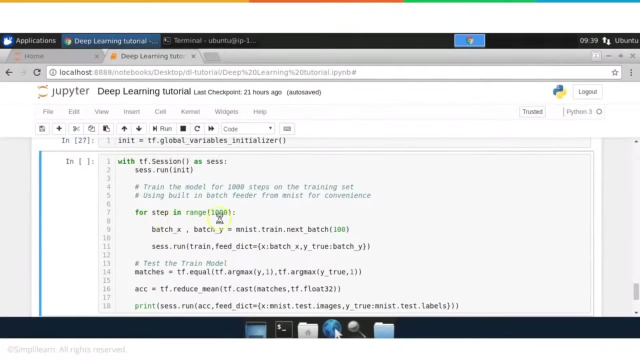 So any variables that we created, You have to run this code, You have to run the initialization of these variables, Otherwise you will get an error. So that is what this is doing. Then, within this, with block, we specify a for loop And we are saying we want the system to iterate for 1000 steps. 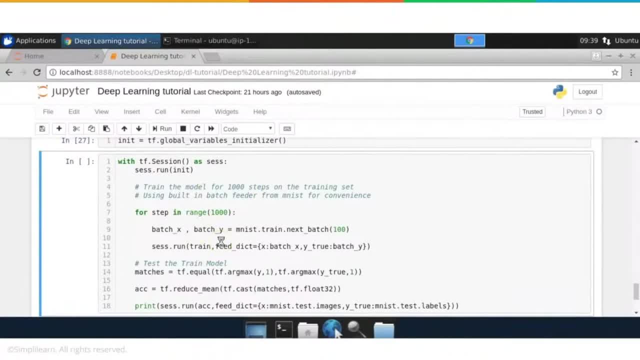 And perform the training. That is what this for loop does: Run training for 1000 iterations- And what it is doing basically is it is fetching the data or these images. Remember, there are about 50000 images, But it cannot get all the images in one shot. 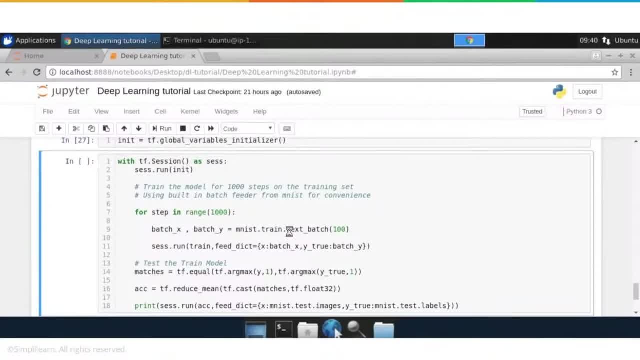 Because it will take up a lot of memory and performance issues will be there. So this is a very common way of performing deep learning training. You always do in batches, So we have maybe 50000 images, But you always do it in batches of 100 or maybe 500. 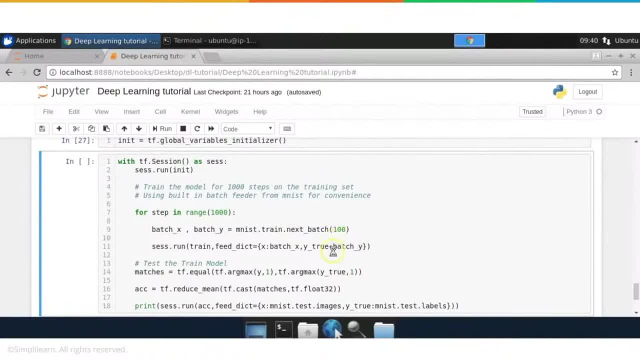 Depending on the size of your system, and so on and so forth. So in this case we are saying, Okay, get me 100 images at a time And get me only the training images. Remember, we use only the training data for training purpose. 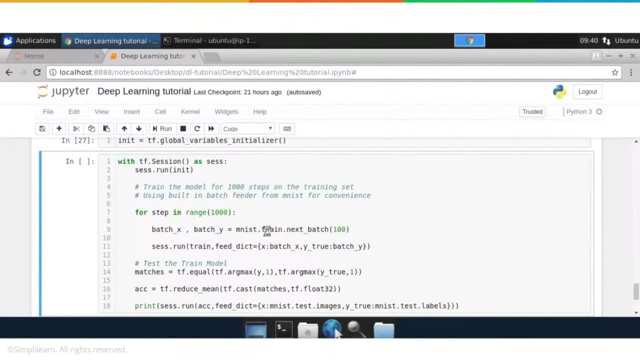 And then we use test data for test purpose. You must be familiar with machine learning, So you must be aware of this. But in case you are not, In machine learning also- This is not specific to deep learning, But in machine learning in general- 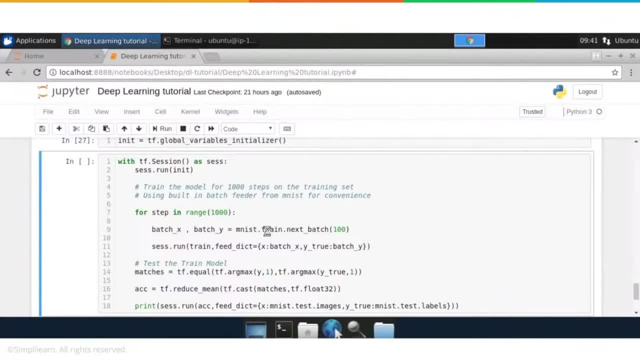 You have what is known as training data set and test data set- Your available data. Typically, you will be splitting into two parts And using the training data set for training purpose And then, to see how well the model has been trained, You use the test data set. 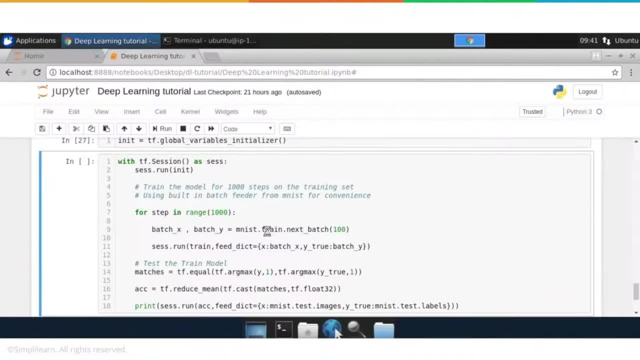 To check or test the validity or the accuracy of the model. So that's what we are doing here, And you observe here That we are actually calling an mnist function here. So we are saying mnist train dot. next batch, Right. So this is the advantage of using mnist database. 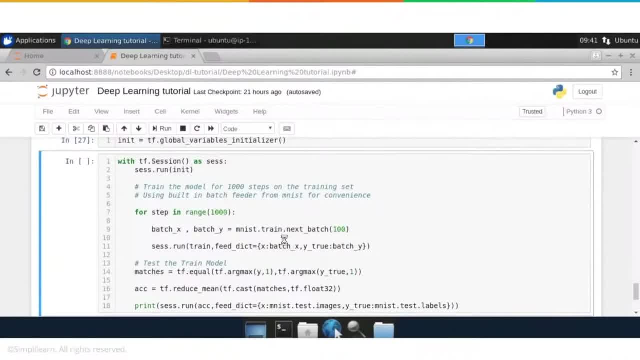 Because they have provided some very nice helper functions Which are readily available. Otherwise, this activity itself- We would have had to write a piece of code To fetch this data in batches. That itself is a lengthy exercise. So we can avoid all that if we are using mnist database. 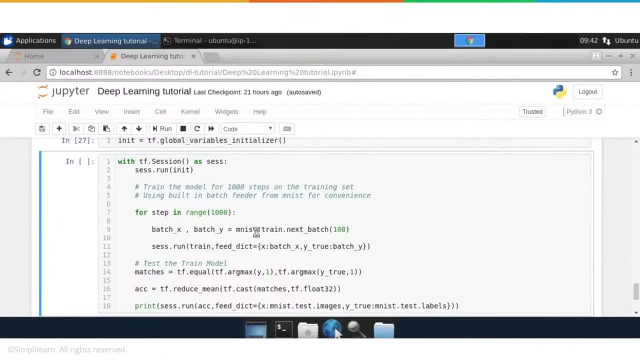 And that's why we use this for the initial learning phase. Okay, So when we say fetch, What it will do is It will fetch the images into x And the labels into y, And then you use this batch of hundred images. 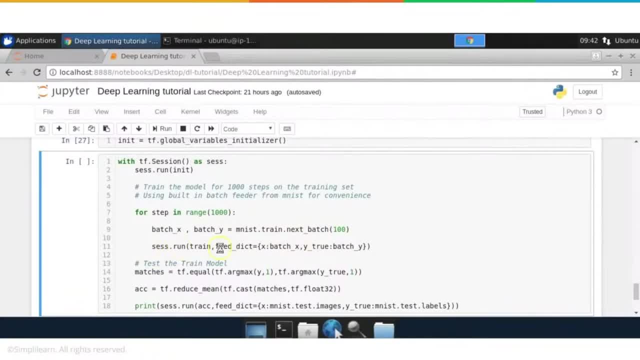 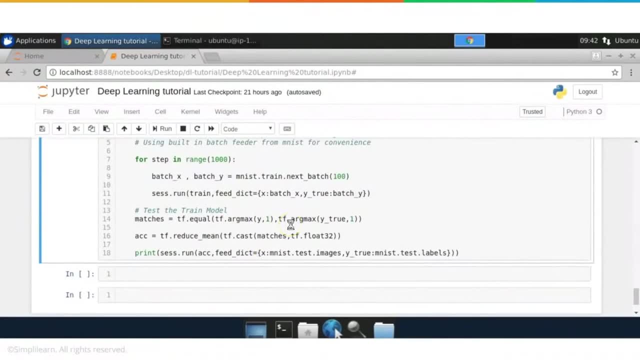 And you run the training. So ses dot run. Basically, what we are doing here is We are running the training mechanism, Which is nothing, but It passes this through the neural network, Passes the images through the neural network, Finds out what is the output. 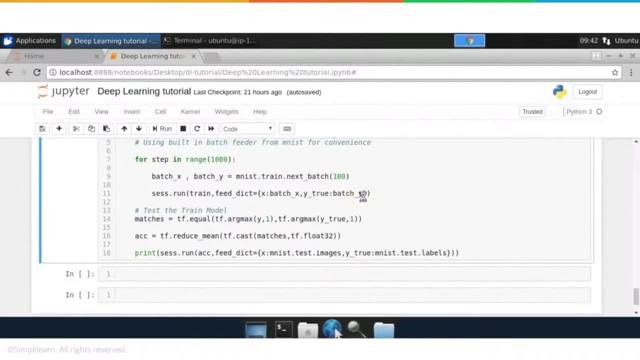 And if the output, Obviously, initially it will be wrong. So all that feedback is given back to the neural network And thereby All the data, All the w's and b's, get updated Till It reaches thousand iterations, In this case. 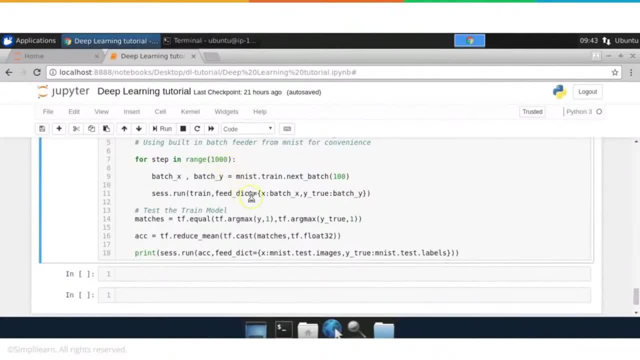 The exit Criteria is thousand, But you can also specify, probably, Accuracy rate or something like that for the As an exit criteria. So here it is. It just says that. Okay, This particular image was wrongly predicted, So you need to update your weights and biases. 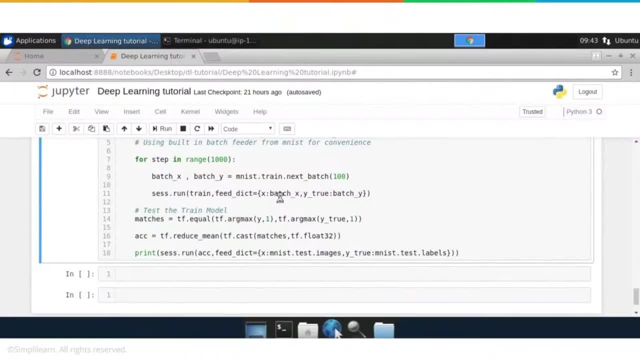 That's the feedback given to each neuron And that is run for Thousand iterations, And typically by the end of this thousand iterations The model would have learned to recognize These handwritten images. Obviously it will not be hundred percent accurate. Okay. 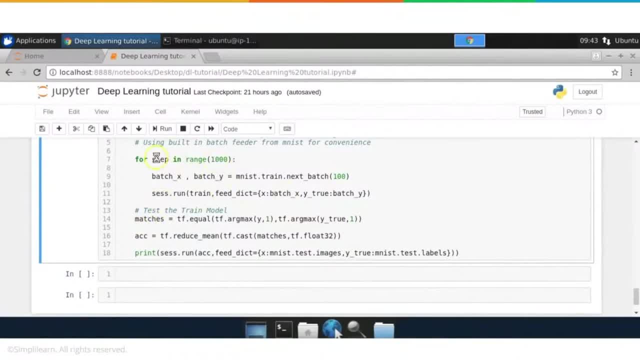 So once that is done- After- So this happens for Thousand iterations- Once that is done, You then Test The accuracy of these models by using the Test data set Right. So this is what we are trying to do here. 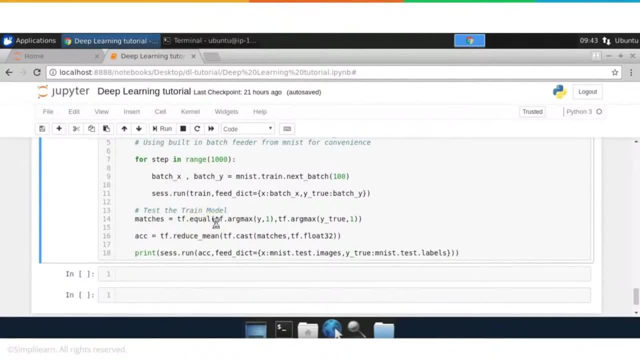 The code may appear a little Complicated because If you're seeing this for the first time, You need to understand The various methods of TensorFlow and so on, But it is basically comparing The output with What has been, What is actually there. 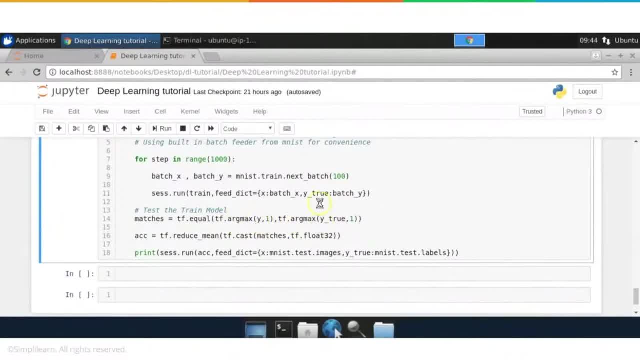 That's all it is doing. So you have your test data And You're trying to Find out what is the actual value And what is the predicted value, And seeing whether they are equal or not. TF dot equal Right. 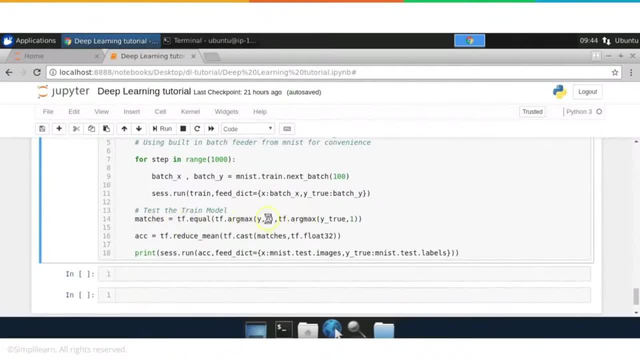 And how many of them Are correct, And so on And so forth, And Based on this, You can Find out What is the actual value And what is the predicted value, And seeing whether they are equal or not. 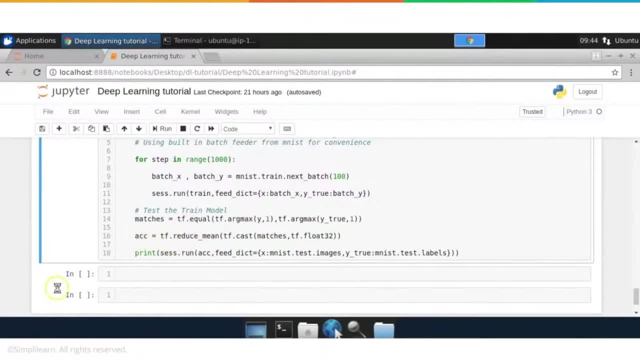 TF, dot equal Right, And Based on that, The accuracy Is Calculated as well. So this is the accuracy And That is what we are trying to see: How accurate The model Is In predicting These. 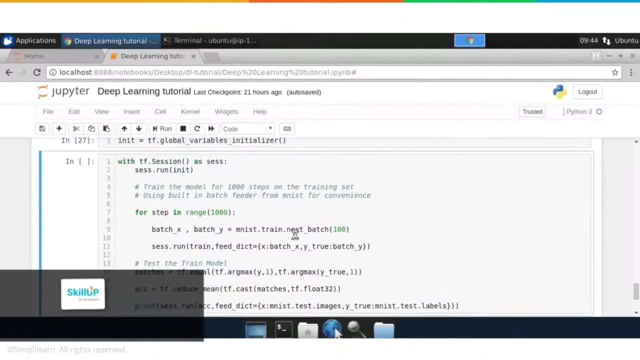 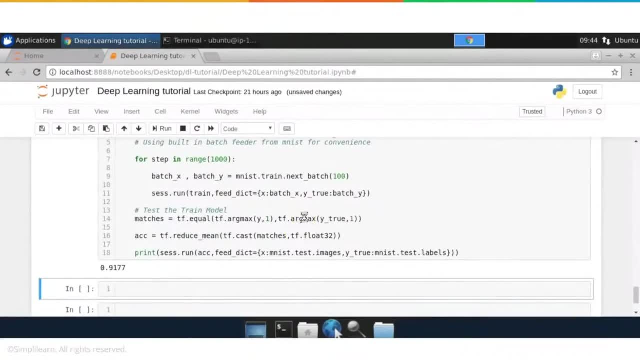 Numbers Or these digits. Okay, So let us run this. This entire thing is in One cell, So we will have to just run it in one shot. It may take a little while, Let us see, And Not bad. 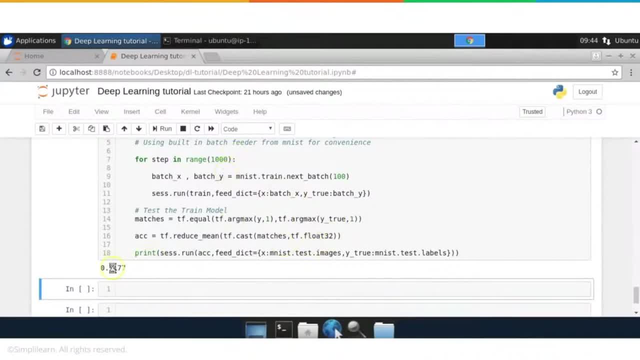 So it has finished The thousand iterations, And What we see Here In output Is The accuracy. So we see that The accuracy Of this model Is Around Ninety one percent. Okay Now, Which is? 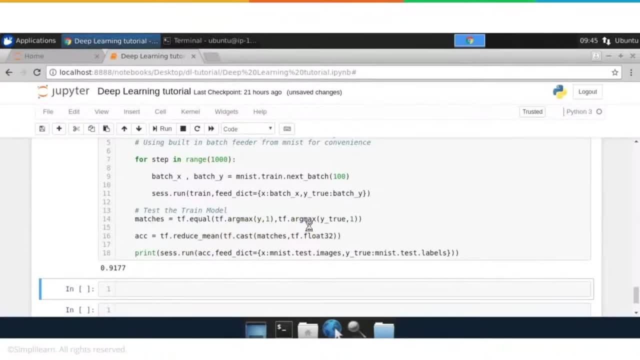 Pretty good For such a Short exercise. Within such a short time We got Ninety percent Accuracy. However, In real life This is probably Not sufficient, So there are Other ways In To increase The accuracy. 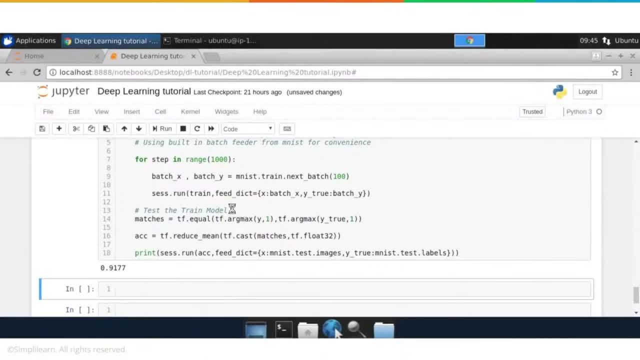 We will See Accuracy, How to change Maybe The hyper parameters Like number of neurons Or number of layers And so on And so forth, And So that This accuracy Can be increased Beyond Ninety percent. 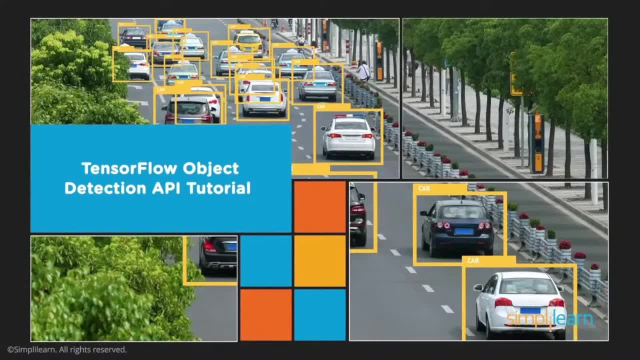 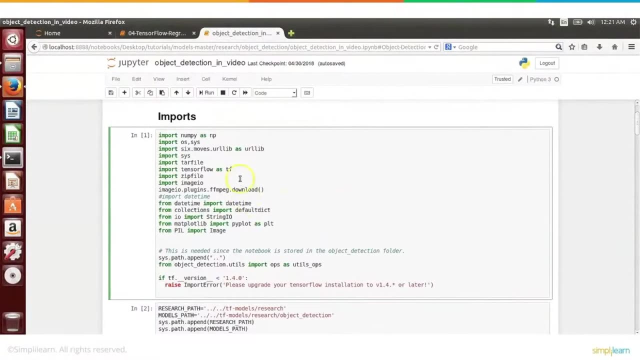 Hello And welcome To the TensorFlow Object Detection API Tutorial. In this video I will walk you Through The TensorFlow Code To perform Object Detection. We need A lot Of these Libraries. 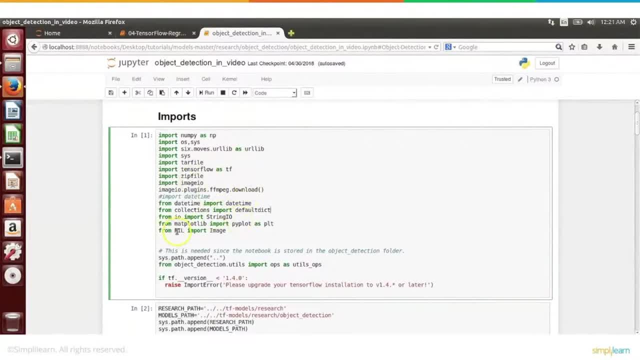 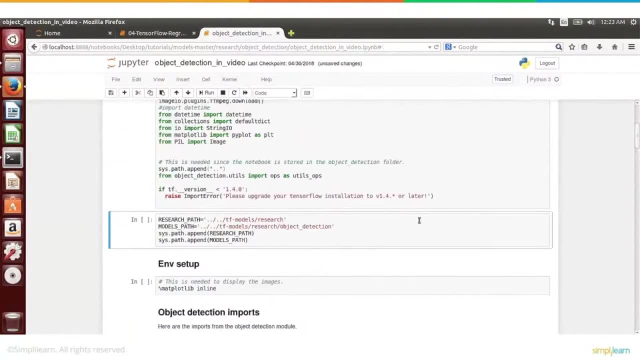 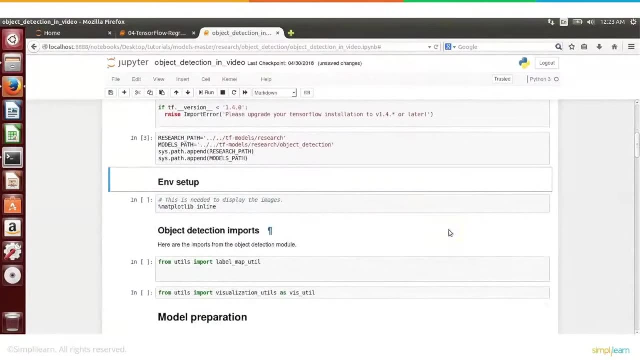 For example, NumPy, We need Image, IO, Date, Time And Pill And so on And so forth And of course Matplotlib. So we import All these Libraries And then There are 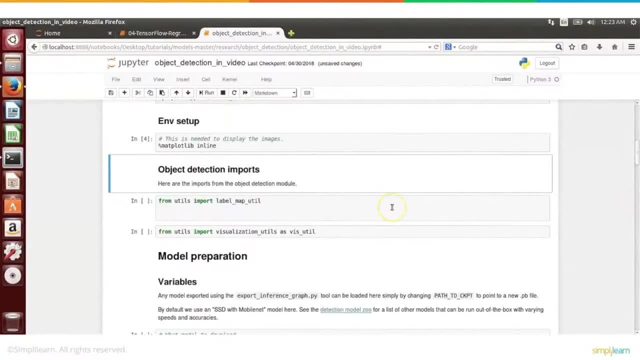 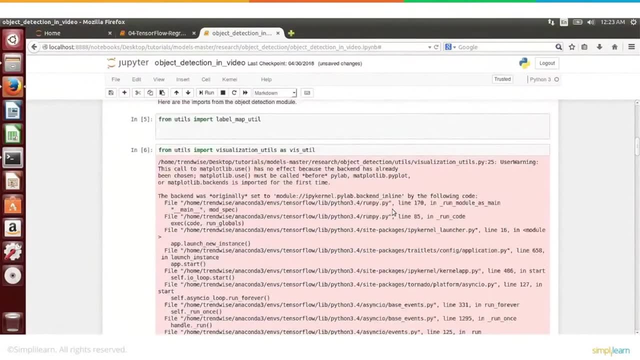 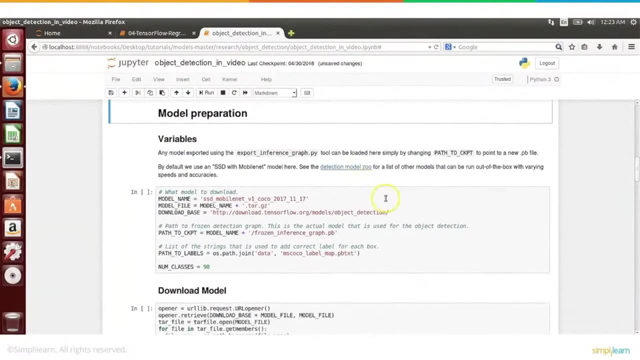 A bunch Of Variables Which have Some Parts For the Model, And then These are Some warnings. We can just Ignore Them. So If I Run This Code Once Again, 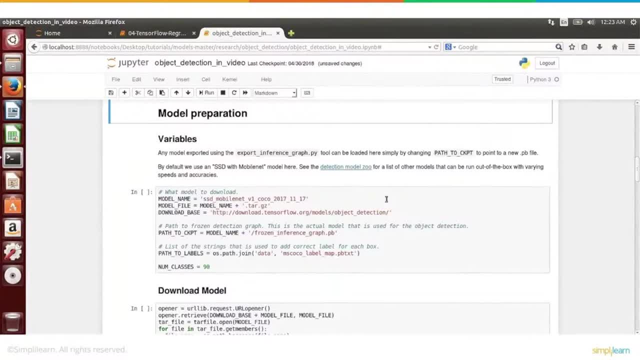 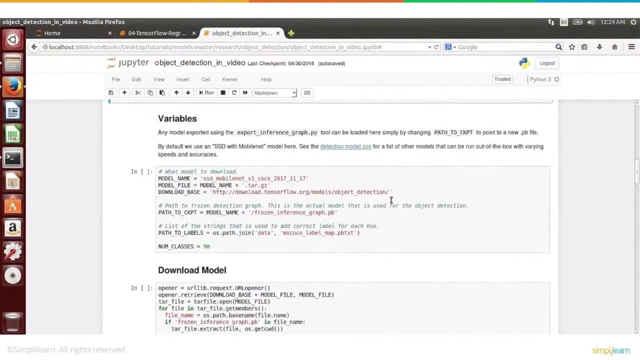 We Can Go Away Right And then Here Or Not. We Do The Model Preparation. Is The SSD With Mobile Net Model That We Are Going. 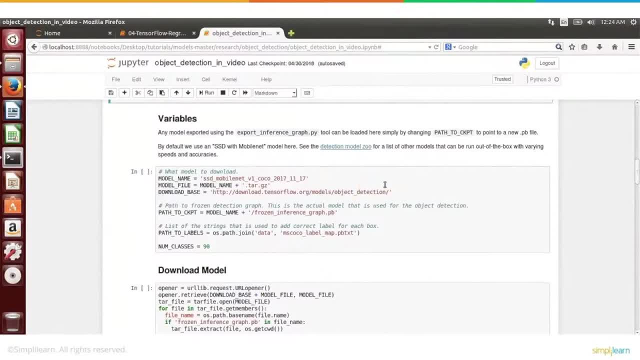 To Use And This Model Is Trained To Detect Objects And It Is Readily Available As Open Source. Very Accurate, But That Is One. 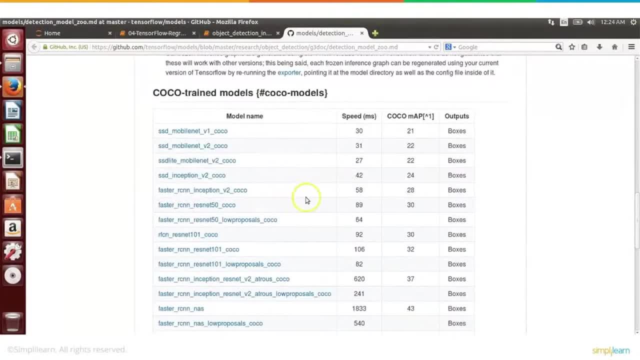 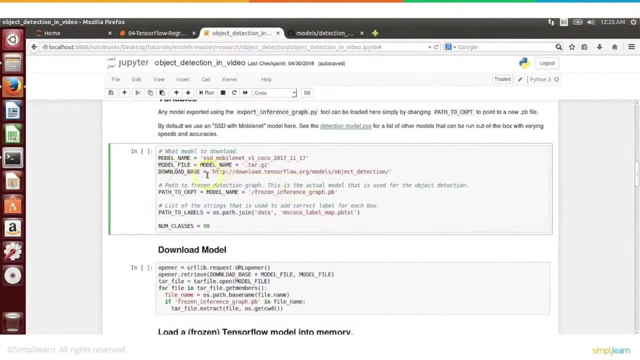 Of The Faster Models, But On This Link You Will See A Lot Of Other Models That Are Readily Available. These Are Trained To Use. 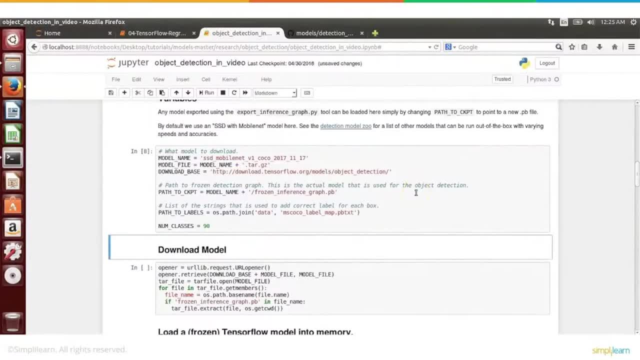 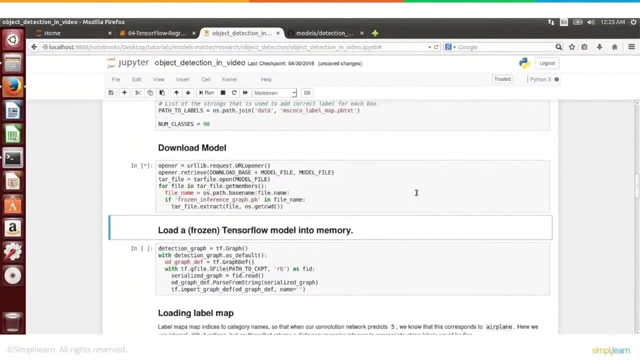 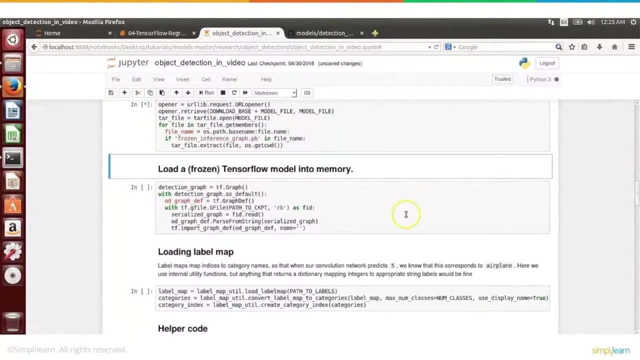 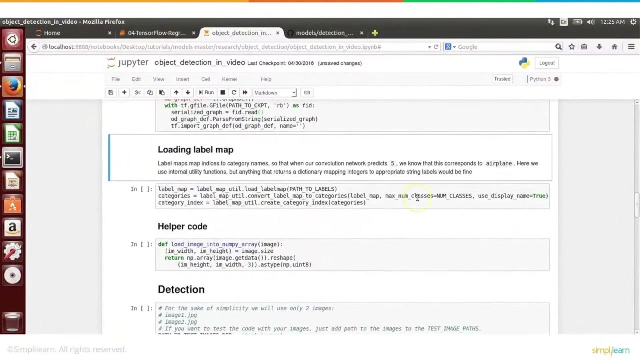 This Model. So We Import, Download And Import That, And Then We Will Actually Use That Model In Our Code. So These Two Cells We Have. 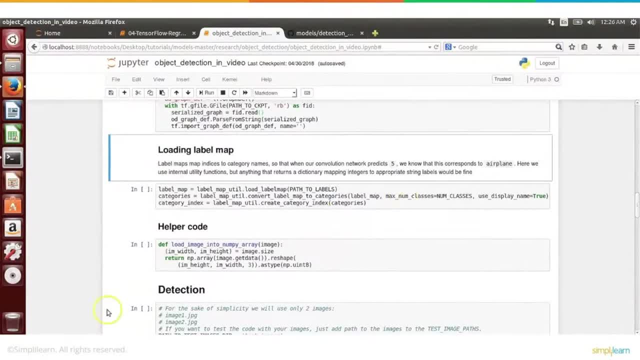 Downloaded Steps, Which Is Basically We Need To Map The Numbers To Text. As You May Be Aware, When We Actually Build A Model And 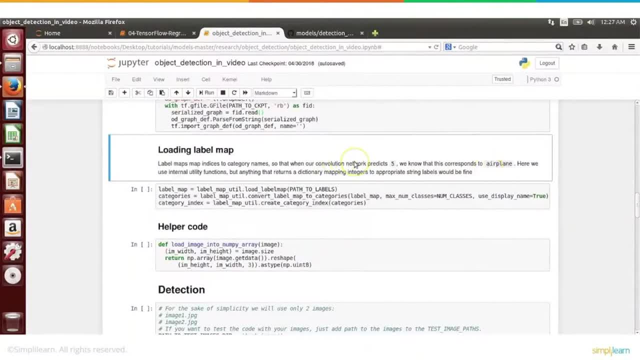 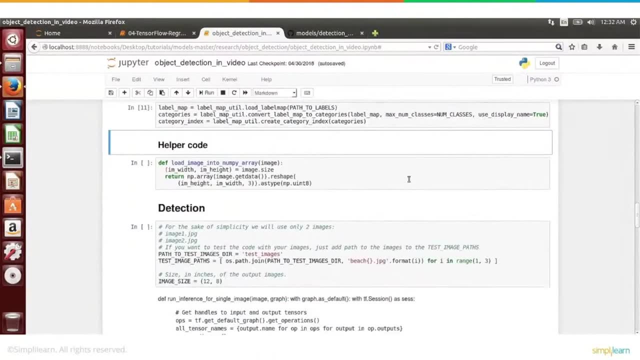 When We Run Predictions, The Model Is Done In This Next Cell, Right, So Let's Keep Moving. And Then We Have A Help Code, Which? 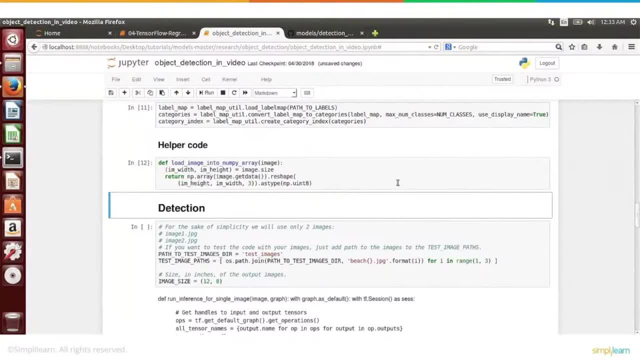 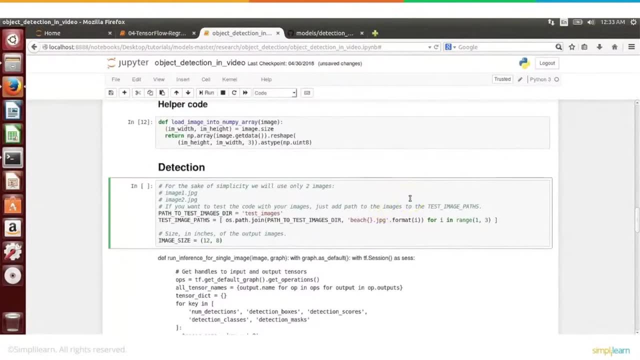 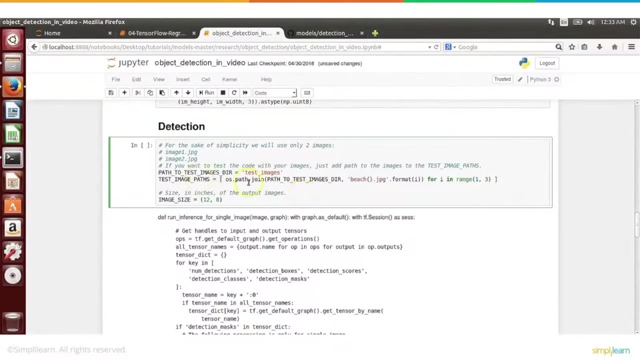 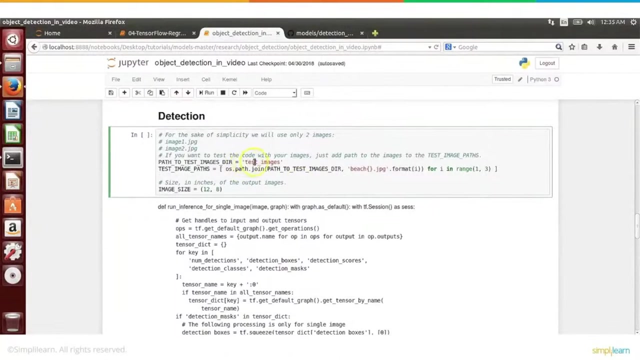 Will Basically Load The Data Or Load The Images, So This Is Where The Actual Detection Starts. So Here, This Is The Path For Where The 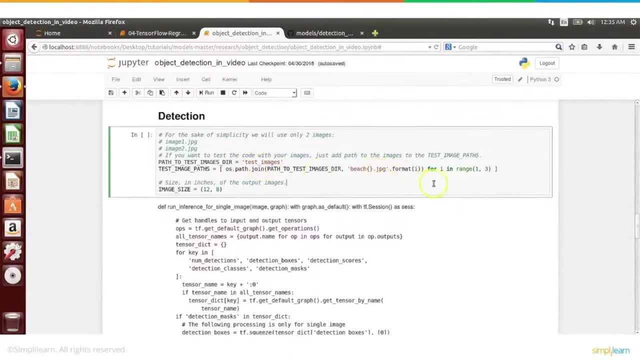 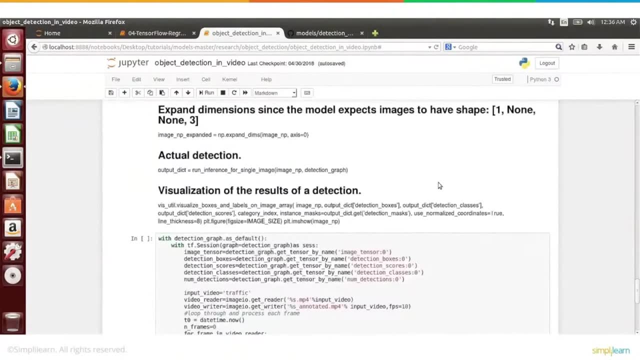 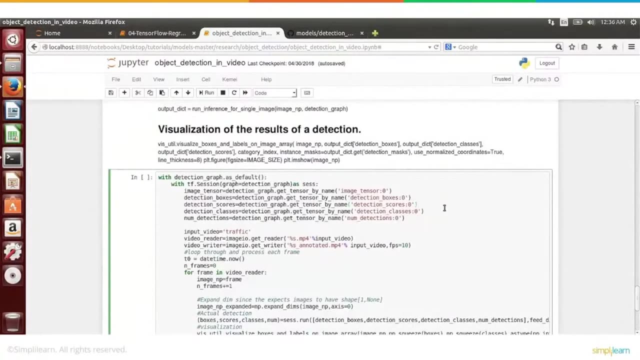 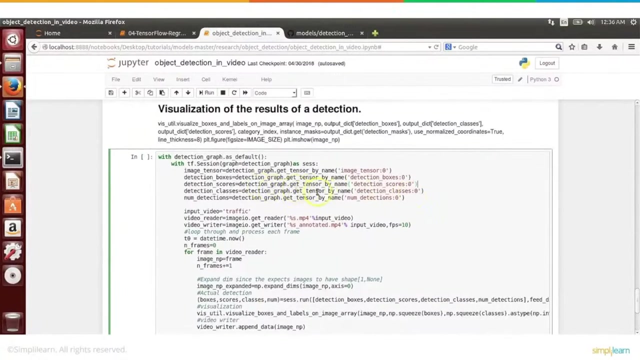 Images Are Stored. So This Is Once Again: We Are Reusing The Cell Where We Are Actually Loading The Video And Converting It Into Frames. 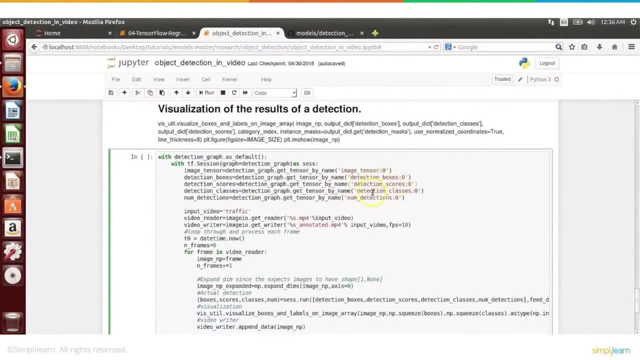 And Then, Using Frame By Frame, We Are Detecting The Objects In The Image, So In This Video Reader, So Excellent Object, Which Is Basically 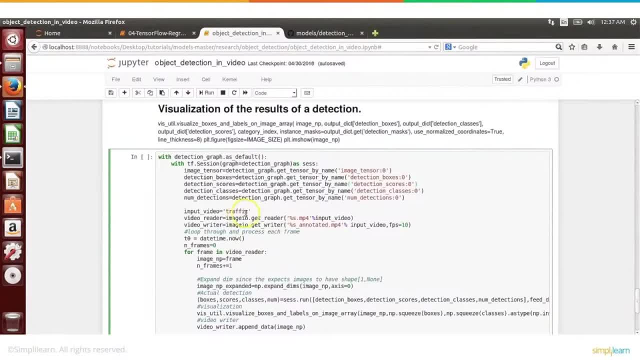 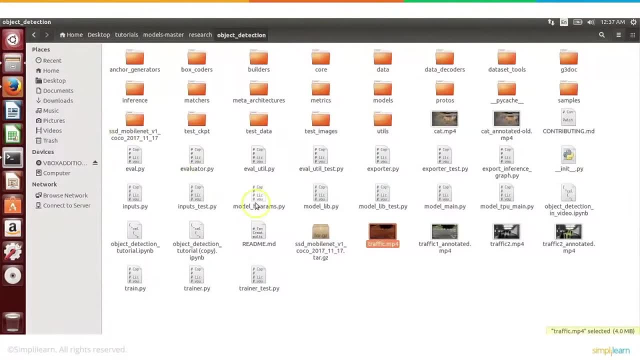 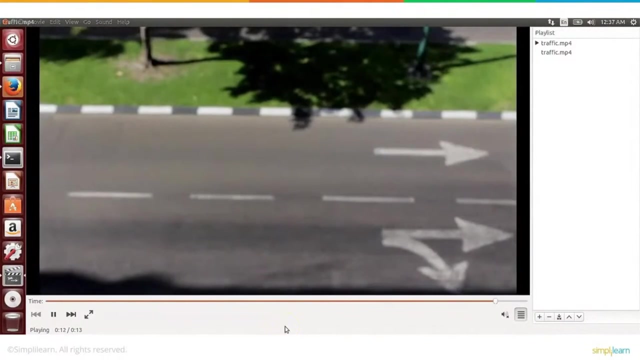 Part Of This Class Called Image I O, So We Can Read And Write Videos Using That, And The Video Is A Little Slow, Yeah, Okay. 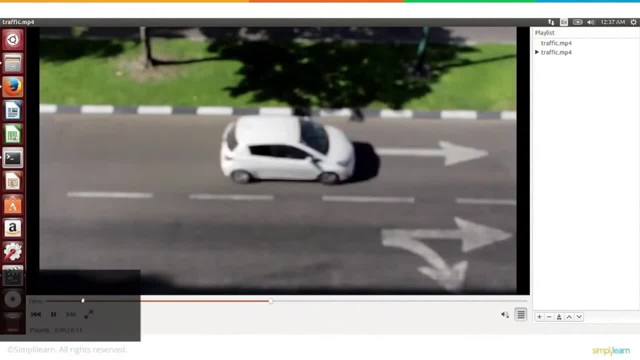 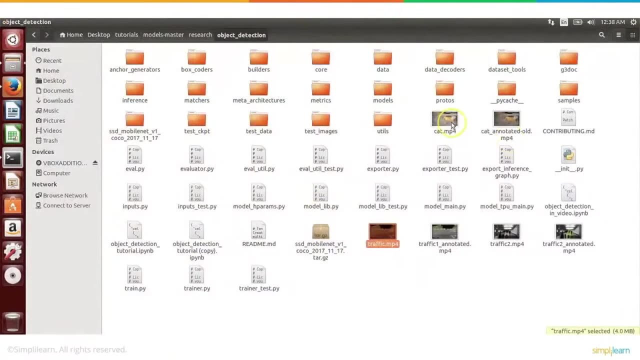 So Here We Go. This Is The Video. It's A Short One, Relatively Small Video. So That For This Particular Demo And What We 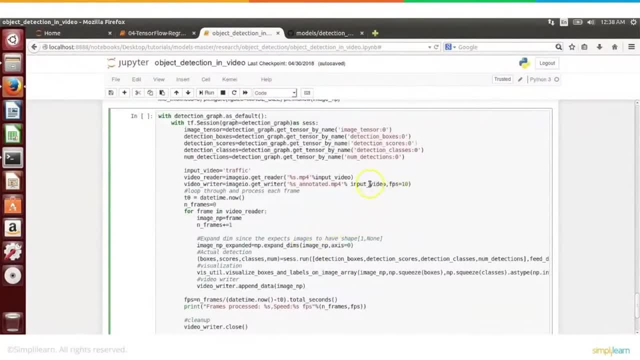 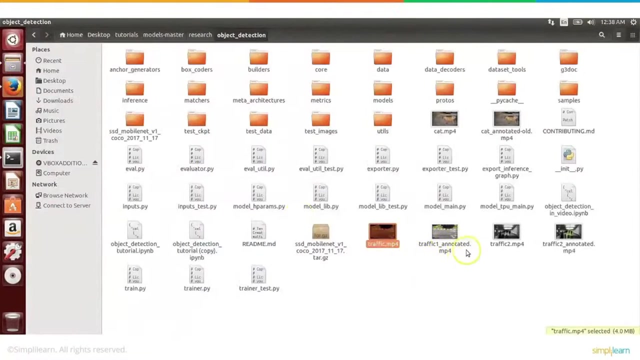 Will Do So. We Will Go Back, So We Will Be Reading This Frame By Frame, And No, Actually, We Will Be Reading The Video File. 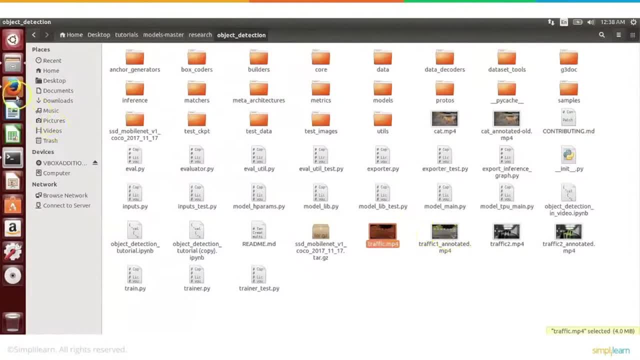 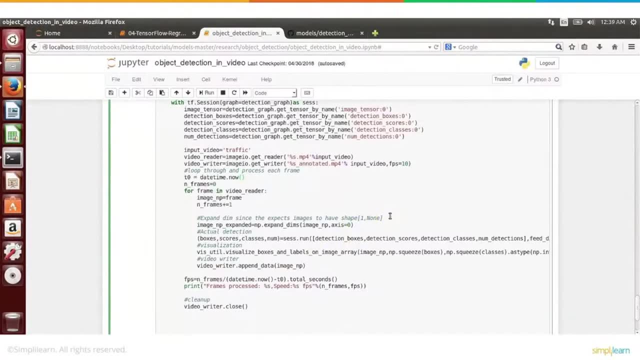 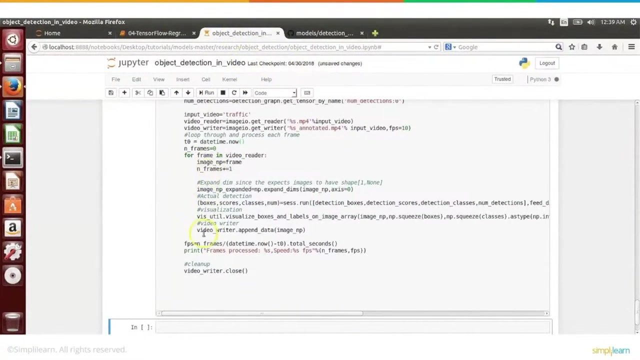 But Then We Will Go Back And Run Through This Piece Of Code And Then We Will Come Back And See The Annotated Video. This 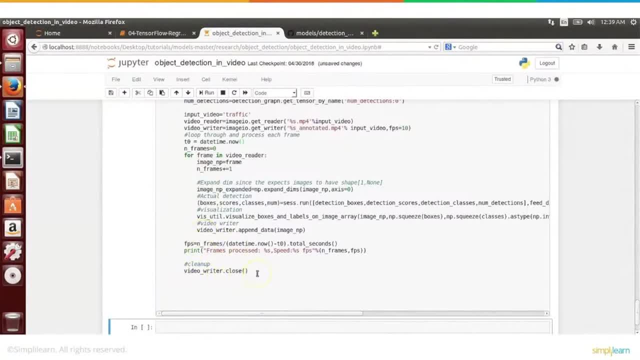 Might Take A Little While. So We Will Be Reading This Frame By Frame, And We Will Be Reading This File, And Then We Will Go. 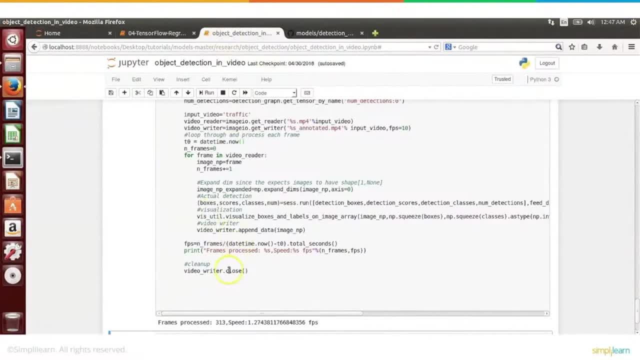 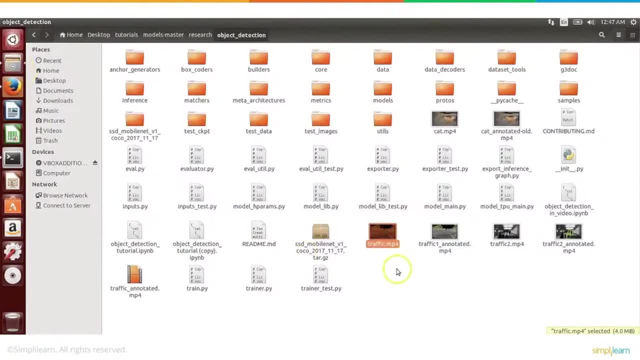 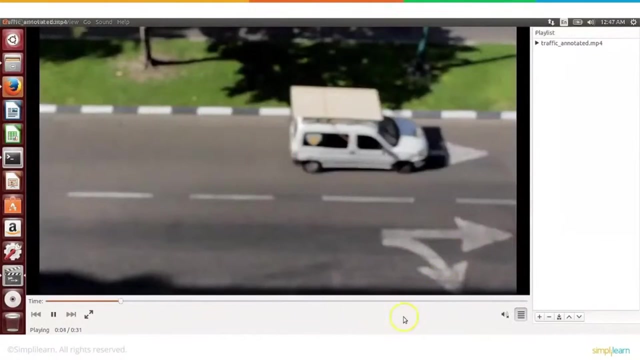 Back To My File Manager And We Will Go To My File Manager. So This Was The Original Traffic Dot Mp4.. And Now You Have. 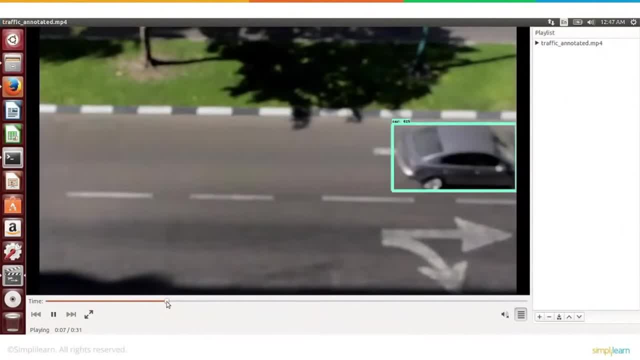 Here Traffic Underscore Annotated Mp4.. So Let's Go And Run This And See A Truck, Okay? So I Think Because Of The Board, 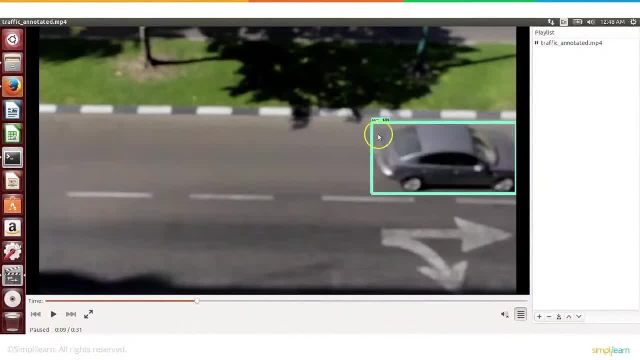 On Top. It Somehow Thinks There Is A Truck. Let's Play Some More And See If It Detects Anything. This Process For Another Video. 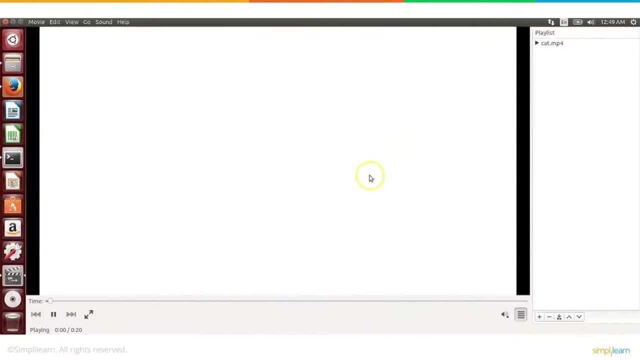 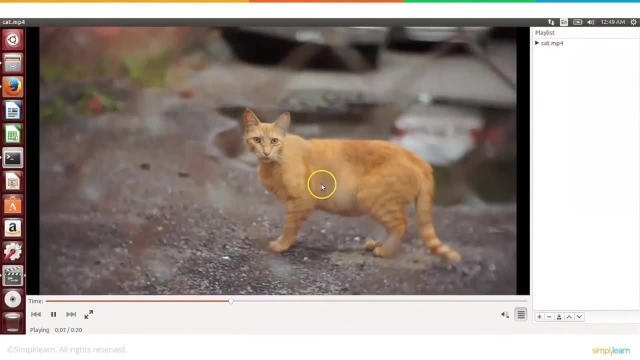 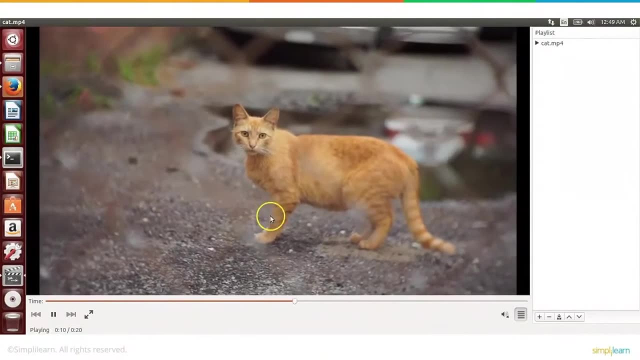 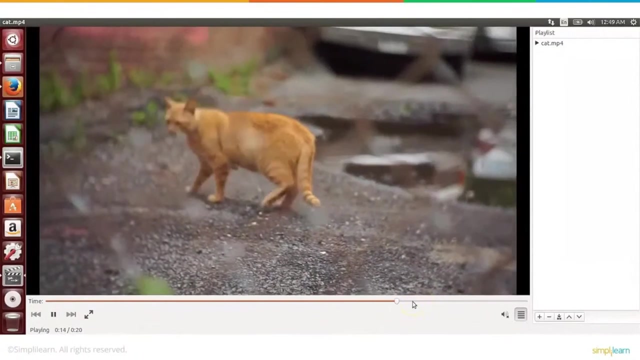 Let Me Just Show You The Other Video, Which Is A Cat. Again There Is. This Cat Is Not Really Moving Or Anything, But Video Is. 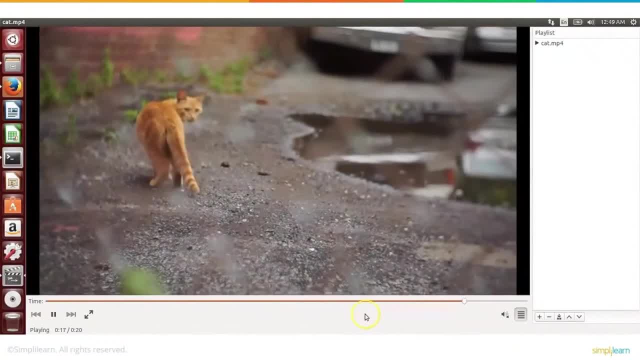 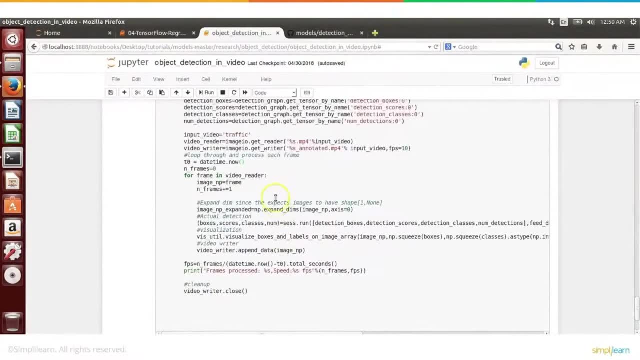 Let's Go Ahead And Change Our Code To Analyze This One And See If It Detects Our Network. Detects This Cat. Close This Here. 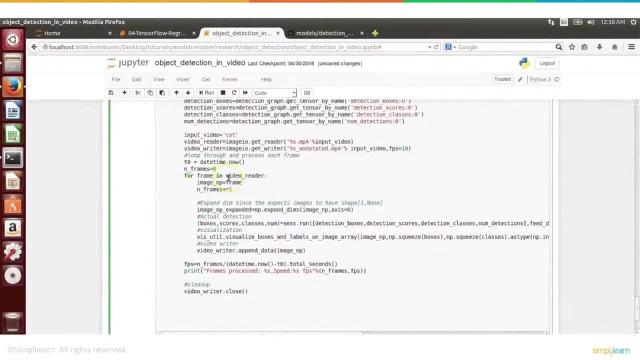 We Go And We Can Say: For Frame In Video Underscore Reader, So It Will Basically Provide Frame By Frame. So You Are In A 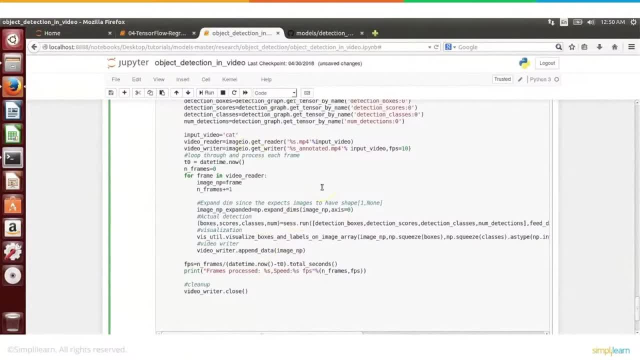 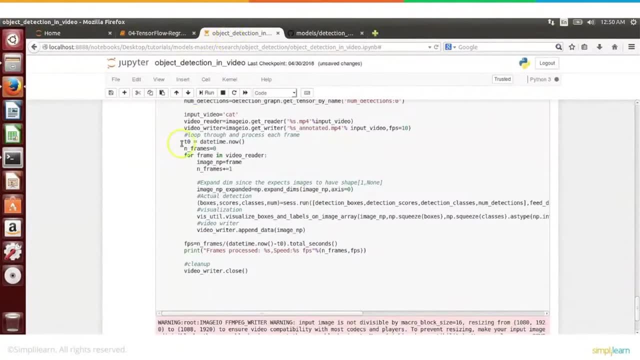 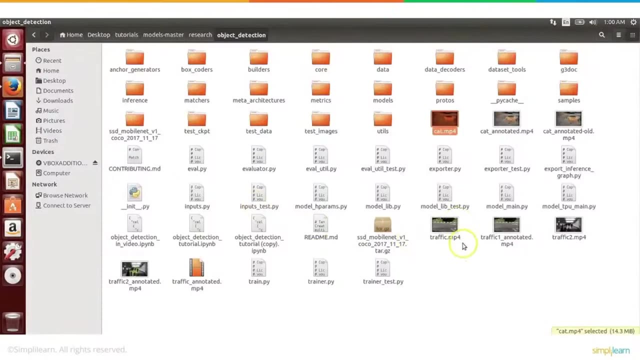 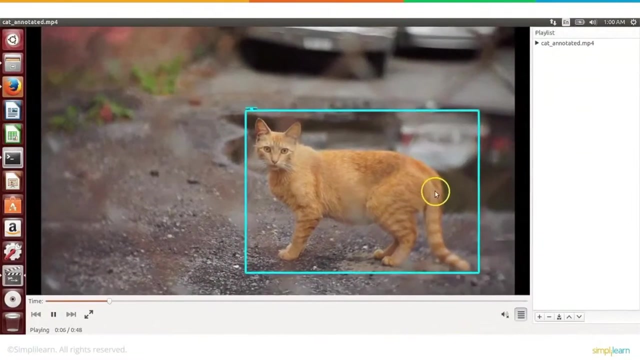 Loop Frame By Frame And Then You Can See What It Has Detected Here. So You Can See What It Has Detected Here. Let's Play. 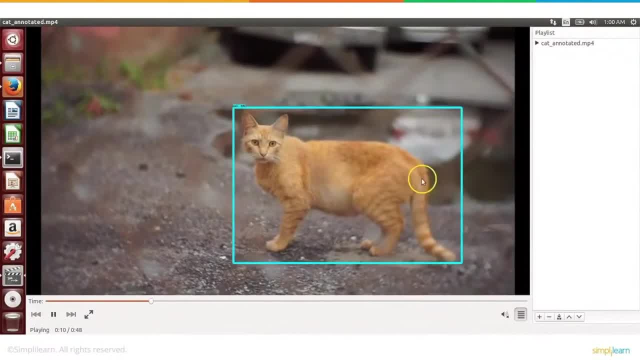 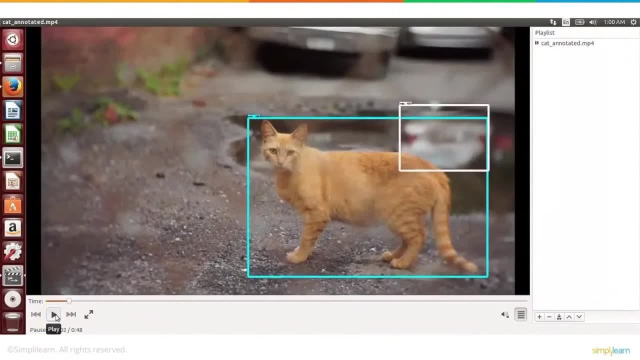 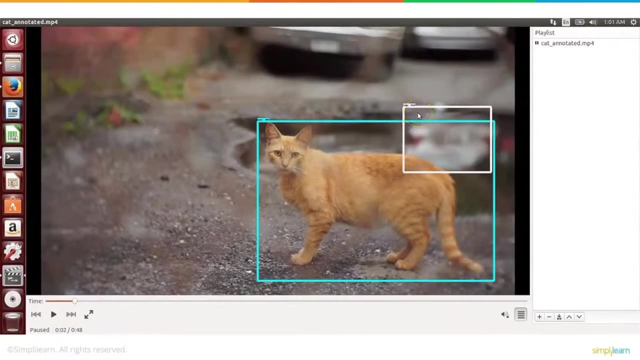 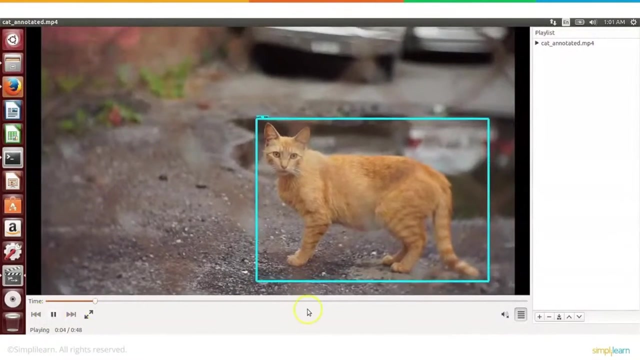 This All Right. So The Processing Is Done, Let's Go. And So What Is It Trying To Show Here? It's Too Small, Not Able To. 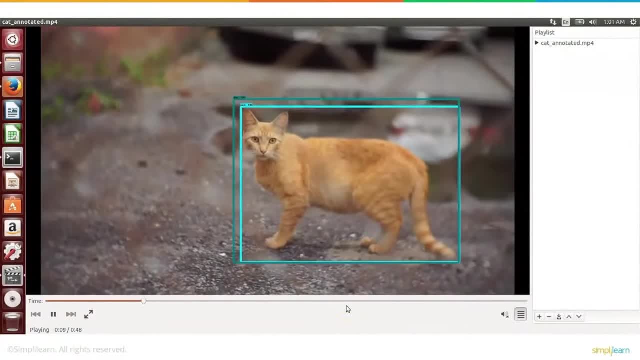 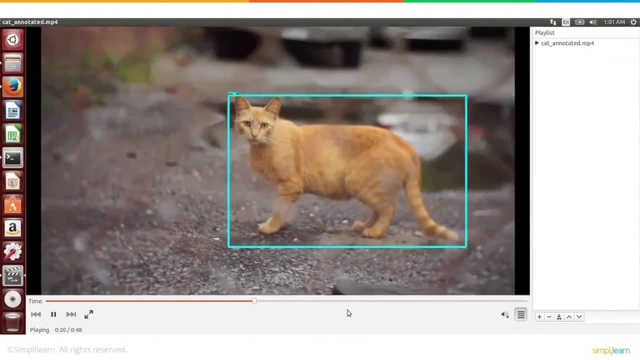 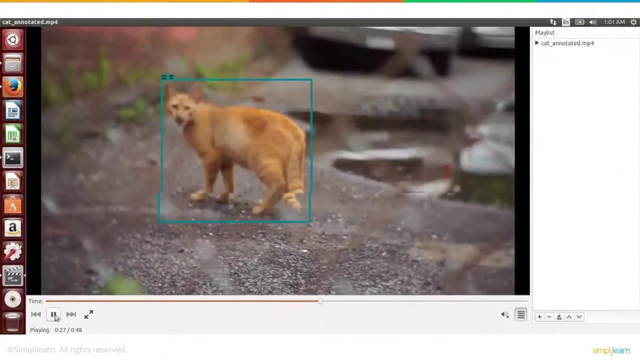 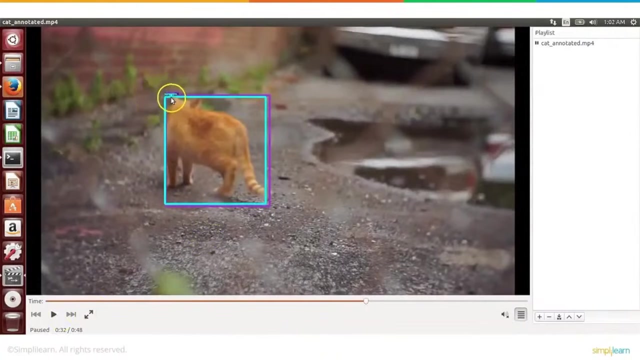 See, But It Is Trying To Detect Something. I Think It Is Saying A Car And In Spite Of Turning The Other Way. I Think 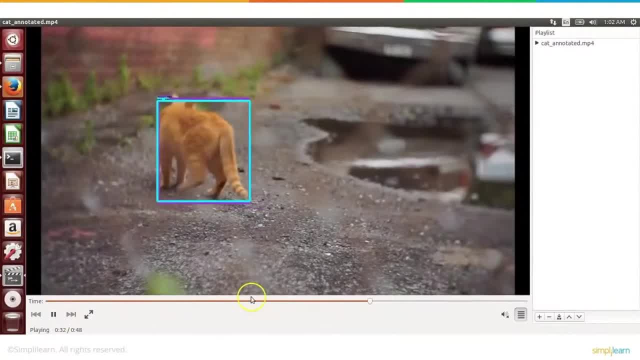 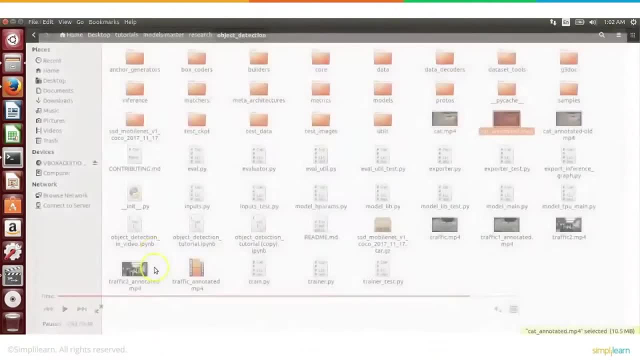 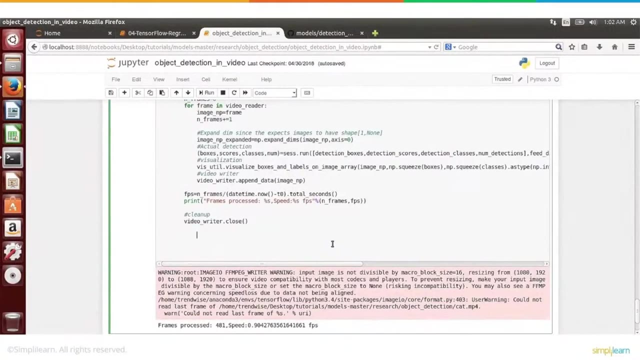 Our Network Is Able To Detect That It Is A Cat, So Let Me Freeze And Then Show Here This Is An Able To See It. 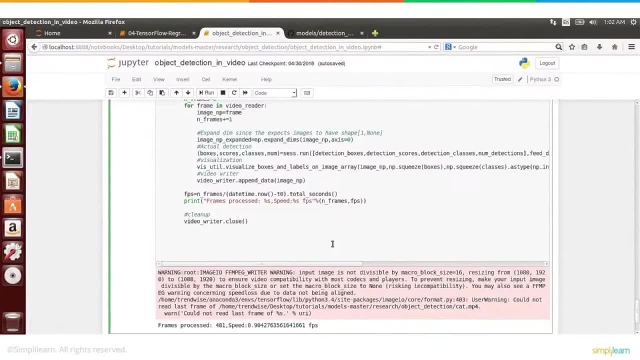 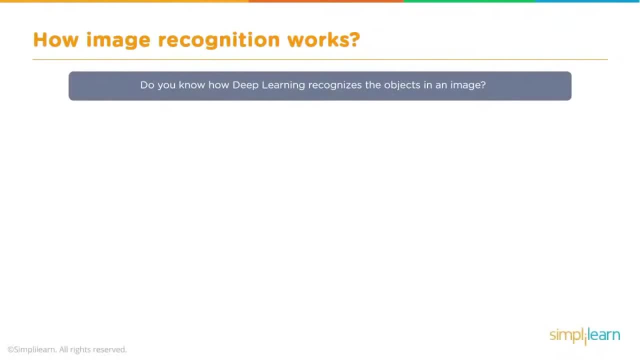 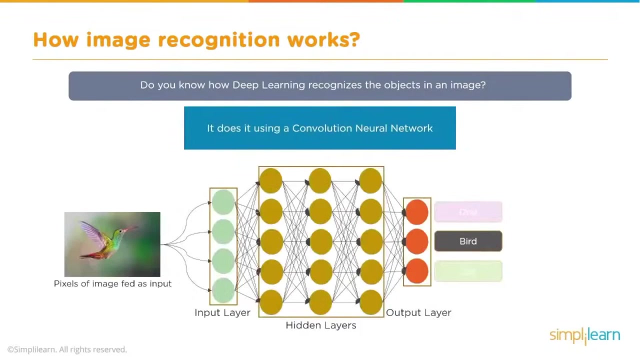 Is Something That Can Be Able To See. It Is Able To See What I Think Is Able To See, That Is convolution, neural network, And over here we have the basic picture of a hummingbird. 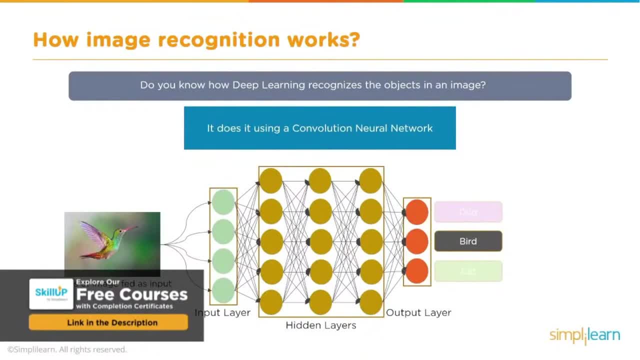 Pixels of an image fed as input. you have your input layer coming in, so it takes that graphic and puts it into the input layer. You have all your hidden layers and then you have your output layer and your output layer. one of those is going to light up and 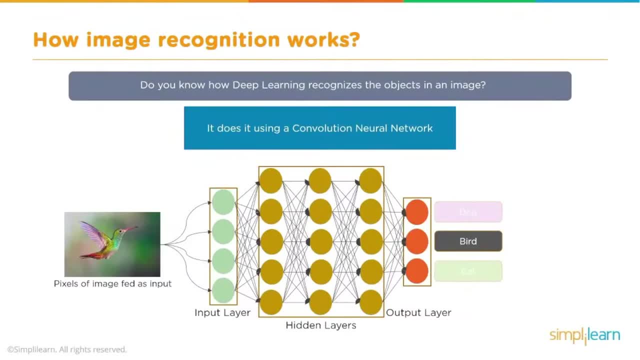 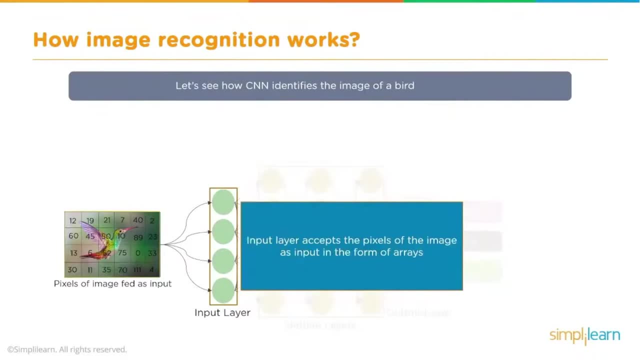 say: oh, it's a bird. We're going to go into depth. we're going to actually go back and forth on this a number of times today, So if you're not catching all the image, don't worry, we're going to get into the details. So we have our input layer accepts the pixels. 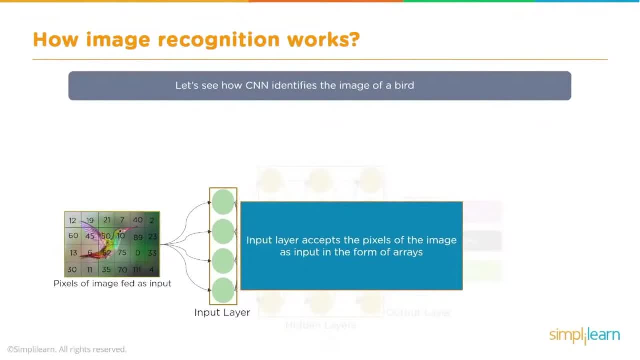 of the image as input in the form of arrays, and you can see up here where they've actually labeled each block of the bird in different arrays. So we'll dive into deep as to how that looks like and how those matrixes are set up. Your hidden layer carry out feature. 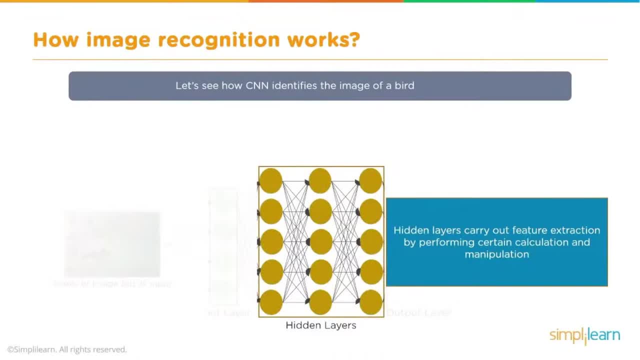 extraction by performing certain calculations and manipulation. So this is the part that kind of reorganizes that picture multiple ways until we get some data that's easy to read for the neural network. This layer uses a matrix filter and performs convolution operation to detect patterns in the image. And if you remember that convolution means to coil or 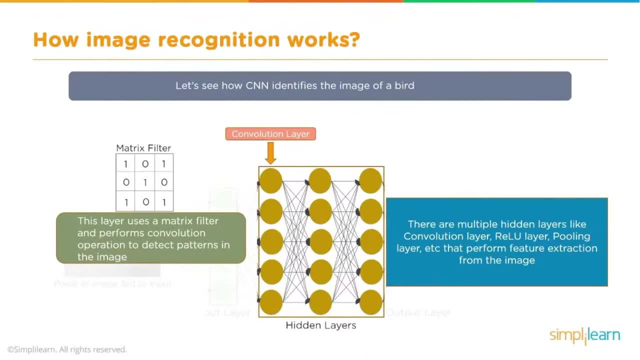 to twist. so we're going to twist the data around and alter it and use that operation to detect a new pattern. There are multiple hidden layers, like convolution layer. rel u is how that is pronounced and that's the rectified linear unit That has to do with 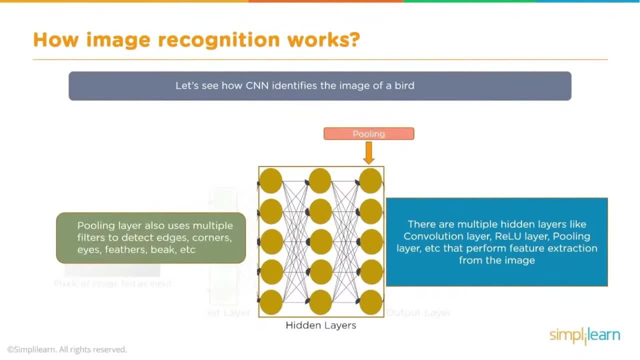 the activation function that's used. Pooling layer also uses multiple filters to detect edges, corners, eyes, feathers, beak etc. And just like the term says, pooling is pooling information together. We'll look into that a lot closer here, so if it's a little confusing now, we'll dig in deep and try to get you. 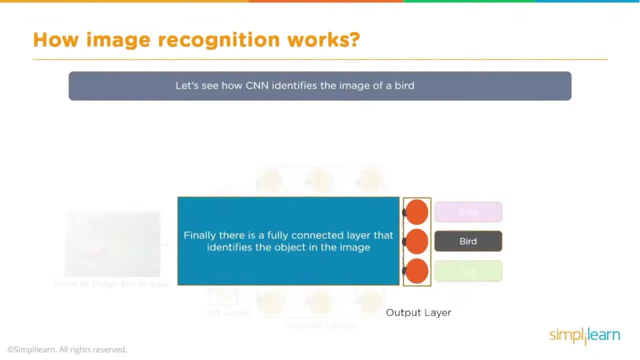 squared away with that And then, finally, there is a fully connected layer that identifies the object in the image. So we have these different layers coming through in the hidden layers and they come into the final area, and that's where we have the one node, or one. 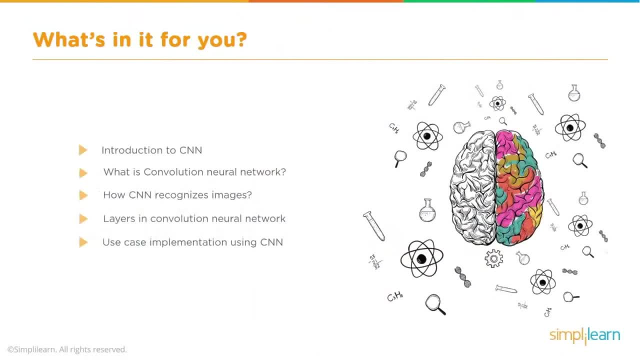 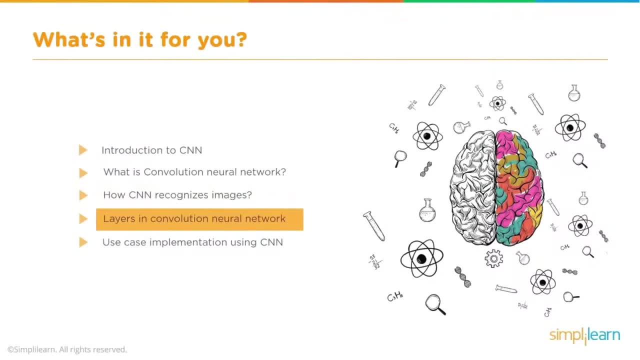 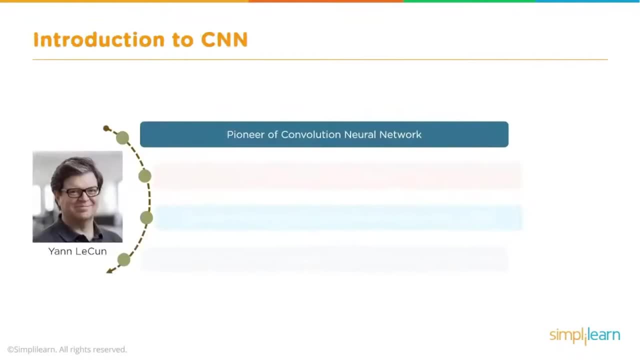 dig deeper into that and really look at the individual layers in the convolutional neural network And finally we do a use case implementation using the CNN. We'll begin our introduction to the CNN by introducing the pioneer of convolutional neural network, Jan LeCun. He was the director. 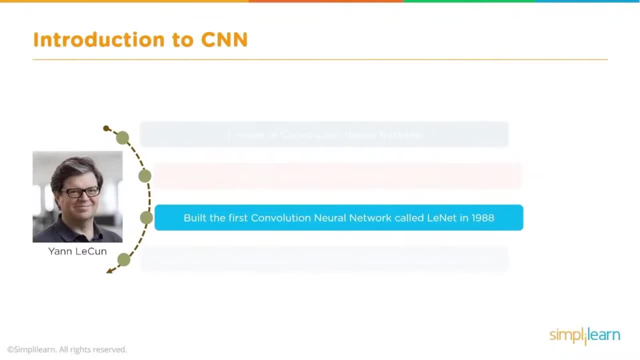 of Facebook. AI Research Group built the first convolutional neural network, called LeNet, in 1988. So these have been around for a while and have had a chance to mature over the years. It was used for character recognition tasks like reading zip code digits, Imagine processing. 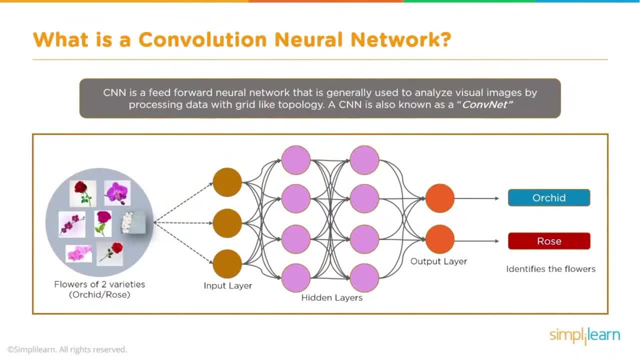 mail and automating that process. CNN is a feed-forward neural network that is generally used to analyze visual images by producing data with a grid-like topology. A CNN is also known as a ConvNet, And very key to this is we are looking at images. That was what this 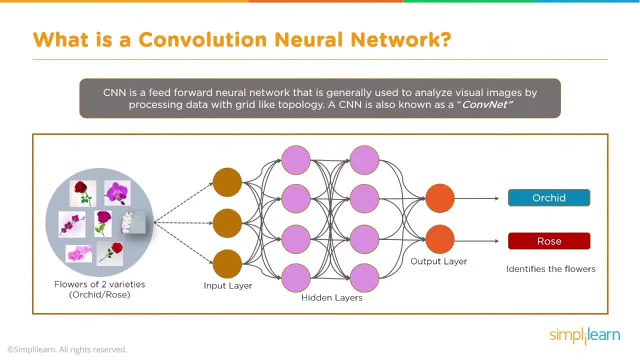 was designed for And you'll see the different layers as we dig in mirror some of the others. Some of them are actually now used, since we are using TensorFlow and Keras in our code. later on You'll see that some of those layers appear in a lot of your other neural network frameworks. 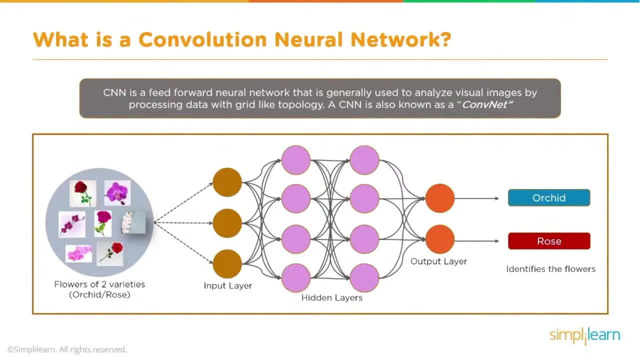 But in this case this is very central to processing images and doing so in a variety that captures multiple images and really drills down into their different features. In this example, here you see flowers of two varieties: orchid and a rose. I think the orchid is much. 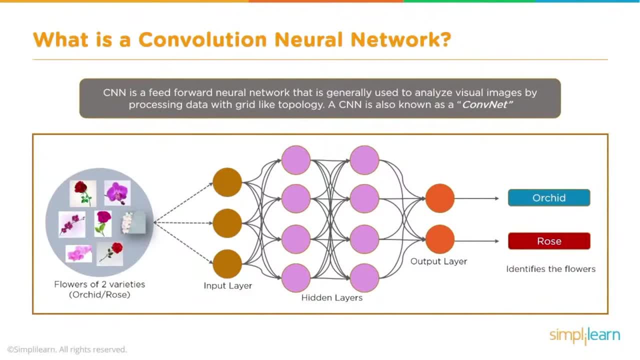 more dainty and beautiful than the other. This orchid is actually a little bit more and the rose smells quite beautiful. I have a couple of rose bushes in my yard. They go into the input layer. That data is then sent to all the different nodes. 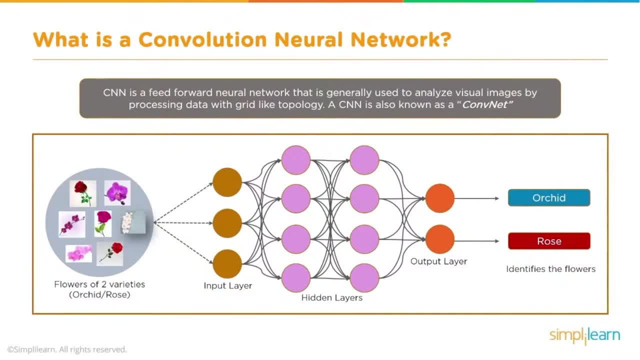 in the next layer, one of the hidden layers, based on its different weights and its setup. It then comes out and gives those a new value. Those values then are multiplied by their weights and go to the next hidden layer, and so on, And then you have the output layer and one of those nodes comes out and says: 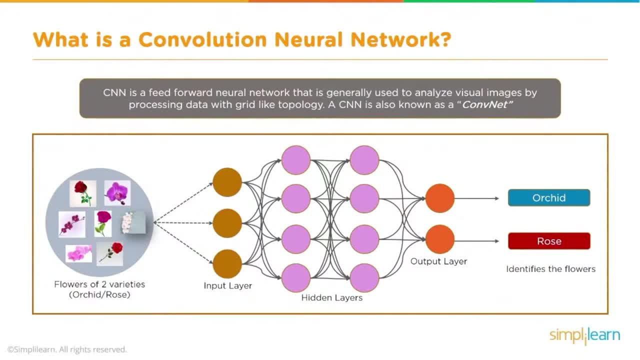 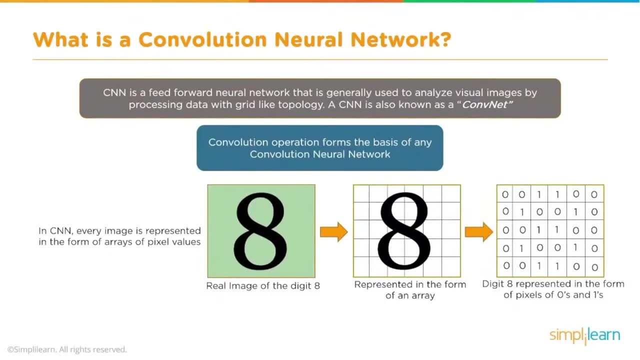 it's an orchid and the other one comes out and says it's a rose, depending on how well it was trained. What separates the CNN or the convolutional neural network from other neural networks is a convolutional operation. It forms the 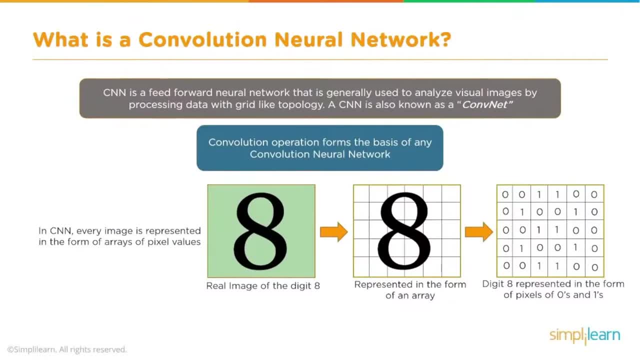 basis of any convolutional neural network. In a CNN, every image is represented in the form of arrays of pixel values. So here we have a real image of the digit 8. That then gets put on to its pixel values, represented in the form of an array. In this case you have a two-dimensional array And then 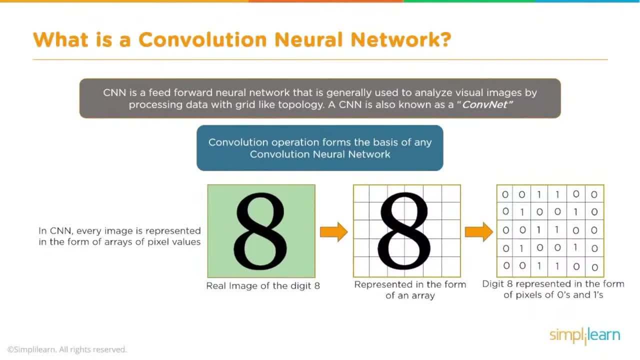 you can see in the final end form, we transform the digit 8 into its representational form of pixels, of zeros and ones, where the ones represent, in this case, the black part of the 8, and the zeros represent the white background To understand the convolutional neural. 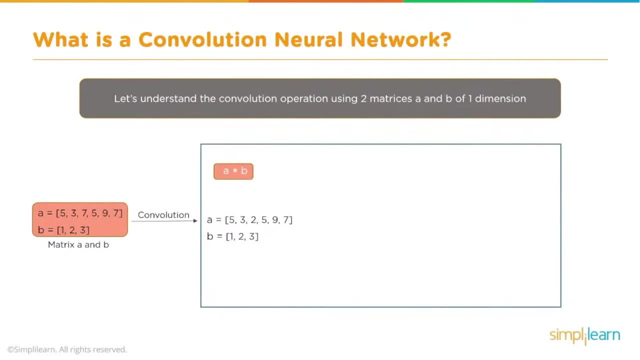 network or how that convolutional operation works. we're going to take a sidestep and look at matrices. In this case we're going to simplify it. We're going to take two matrices, A and B, of one dimension, Now kind of separate this. 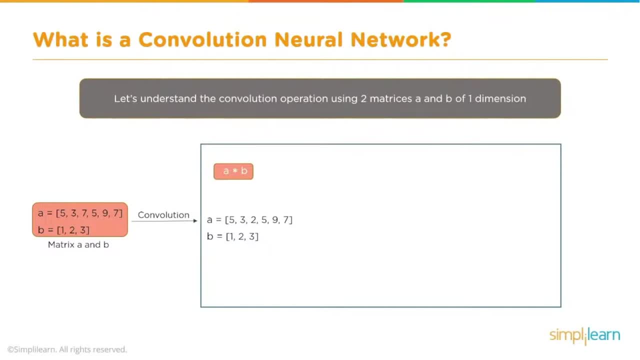 from your thinking as we learn that you want to focus just on the matrix aspect. Now kind of separate this from your thinking as we learn that you want to focus just on the matrix aspect. Now kind of separate this from your thinking as we listen and reflect on this and then we'll bring that. 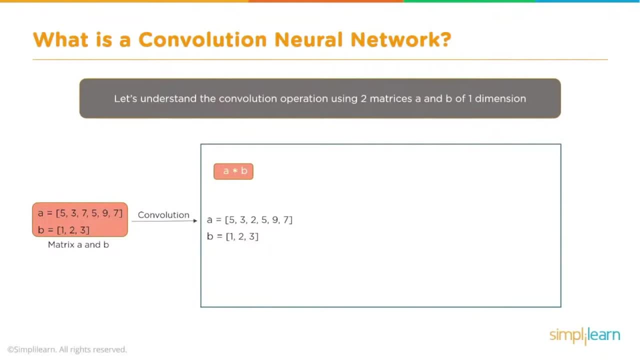 back together and see what that looks like When we put the pieces for the convolutional operation. Here we've set up two arrays. We have a single dimension matrix And we have A equals 5,, 3,, 7,, 5,, 9,, 7.. And we have B equals 1,, 2,. 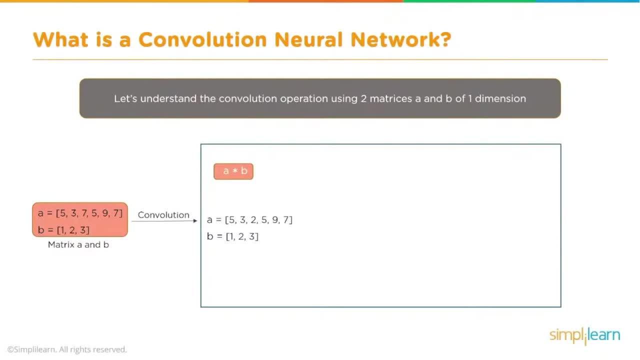 3. So in the convolution as it comes in, it's going to look at these two And we're going to start by doing multiplying them A times B. So we multiply the arrays element wise and we get 5,, 6,, 6.. 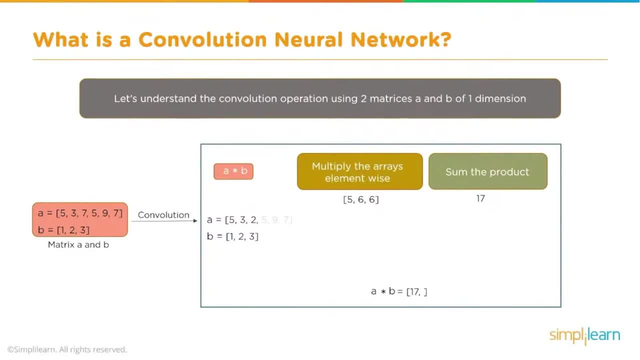 where 5 is the 5 times 1, 6 is 3 times 2, and then the other 6 is 2 times 3.. And since the two arrays aren't the same size, they're not the same setup, we're. 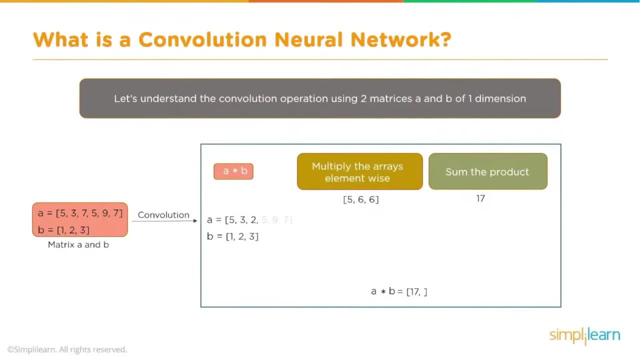 going to just truncate the first one and we're going to look at the second array multiplied just by the first three elements of the first array. Now that's going to be a little confusing, Remember, a computer gets to repeat these processes hundreds of times, so we're not going to just forget those other numbers. 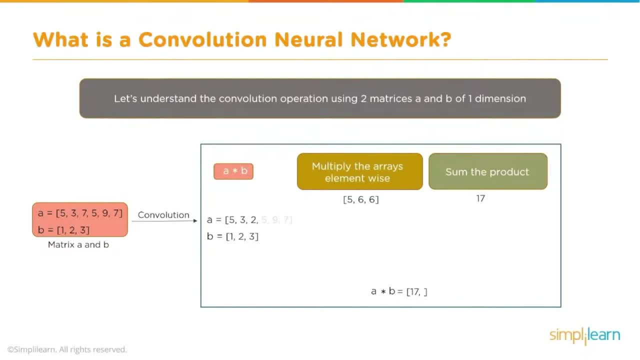 later on We'll see, we'll bring those back in And then we have the sum of the product. In this case, 5 plus 6 plus 6 equals 17.. So in our A times B, our very first digit in that matrix of A times B is 17.. And if you remember, I said we're 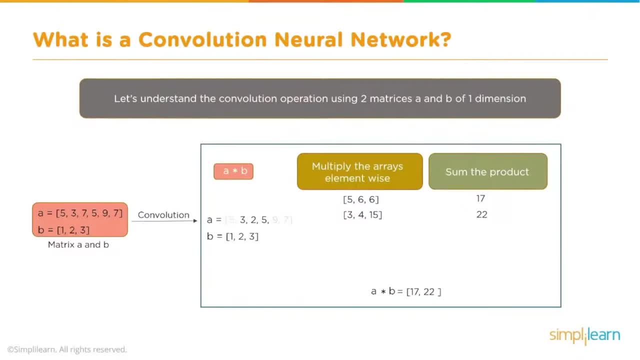 not going to forget the other digits. So we now have 3,, 2, 5.. We move one set over and we take 3, 2, 5 and we multiply that times B And you'll see that 3 times 1 is. 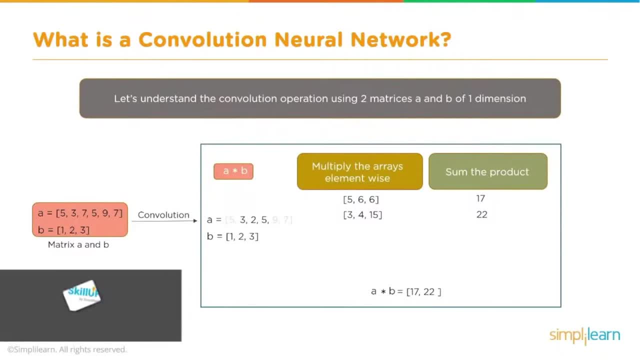 3,, 2 times 2 is 4, and so on, and so on. We sum it up, So now we have: 3 times 1 is 3,, 2 times 2 is 4, and so on, and so on. We sum it up, So now we have. 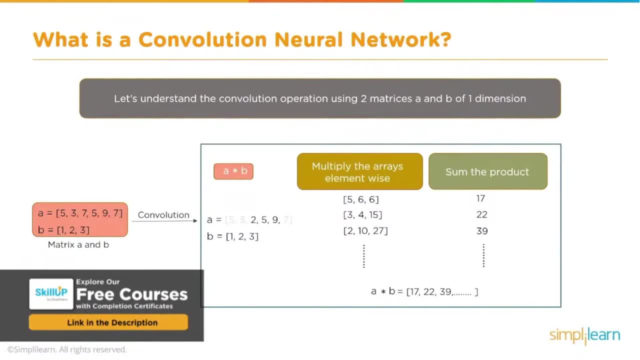 3 times 1 is 3,, 2 times 2 is 4, and so on, and so on. We sum it up. So now we have the second digit of our A times B product in the matrix, And we continue on with. 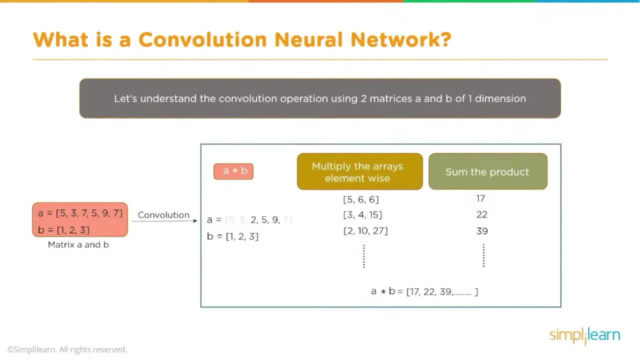 that same thing, so on and so on. So then we would go from 3, 7, 5 to 7, 5, 9 to 5, 9, 7.. This short matrix that we have for A, we've now covered all the different. 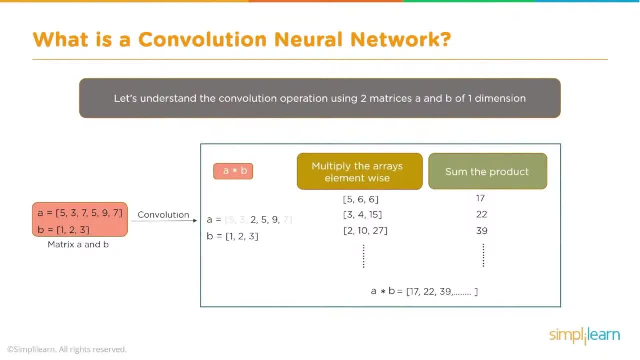 entities in A that match three different levels of B. Now in a little bit we're going to cover where we use this math at this multiplying of matrices and how that works. But it's important to understand that we're going through the matrix. 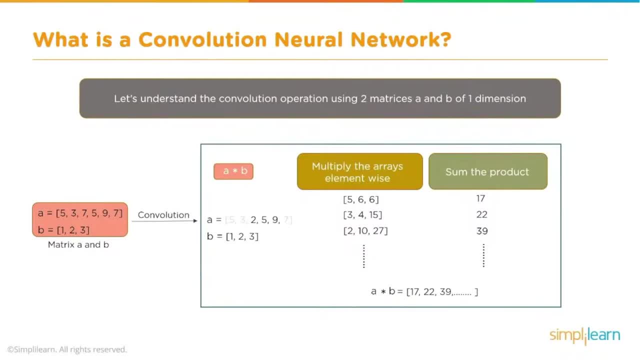 and multiplying the different parts to it to match the smaller matrix with the larger matrix I know a lot of people get lost at is you know what's going on here with these matrices? Ooh, scary math. Not really that scary when you break it down. We're. 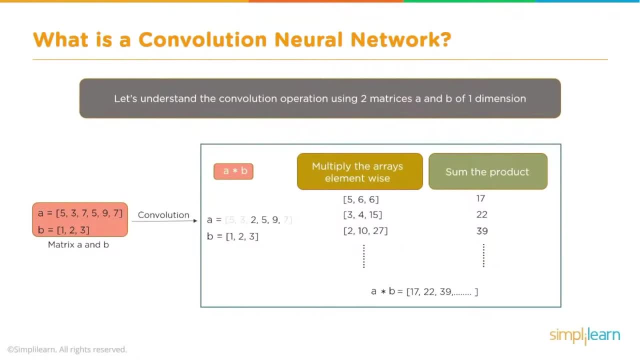 looking at a section of A and we're comparing it to B. So when you break that down in your mind like that, you realize okay. so I'm just taking these two matrices and comparing them and I'm bringing the value down into one matrix: A times B. We're deucing that. 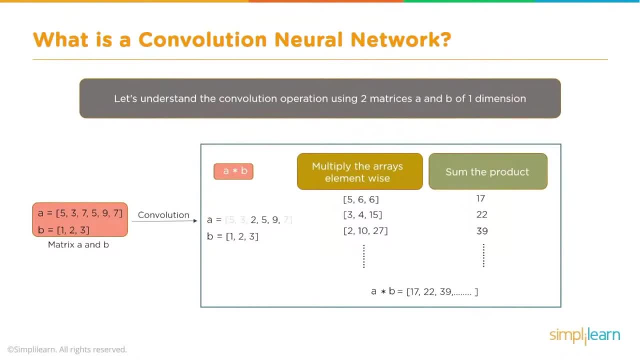 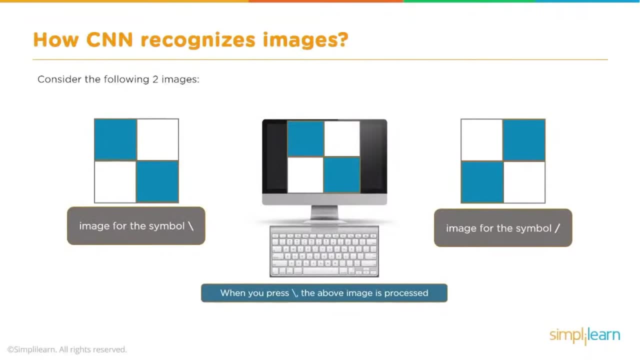 information in a way that will help the computer. Let's go ahead and flip over again back to our images. Here we are back to our images. I'm talking about going to the most basic two-dimensional image. you can get to Consider the following two images: The image for the symbol backslash When you press the backslash. 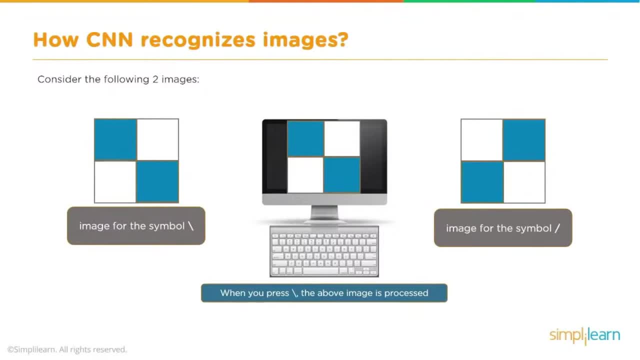 the above image is processed And you can see there for the image for the forward slash is the opposite. So when we click the forward slash button that flips. Very basic: We have four pixels going in. Can't get any more basic than that. Here we have a little bit. 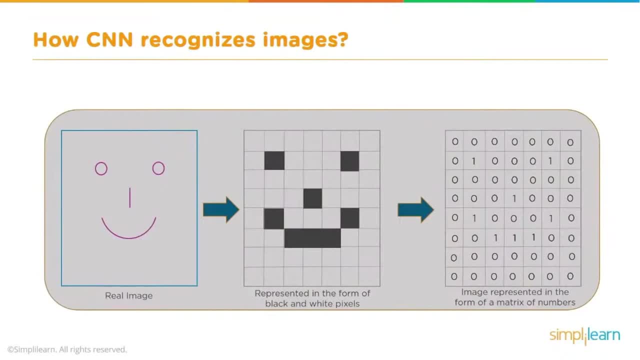 more complicated picture. We take a real image of a smiley face, Then we represent that in the form of black and white pixels. So if this was an image in the computer, it's black and white And, like we saw before, we convert this into the zeros and ones. So where the 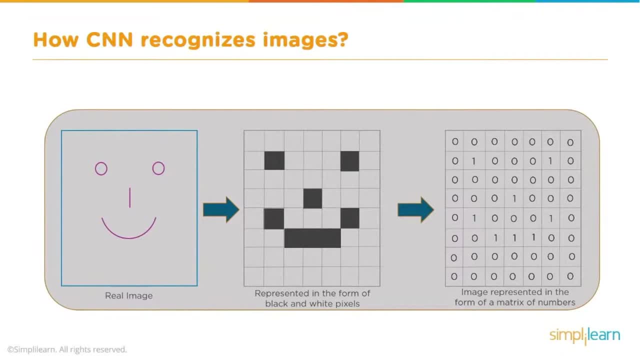 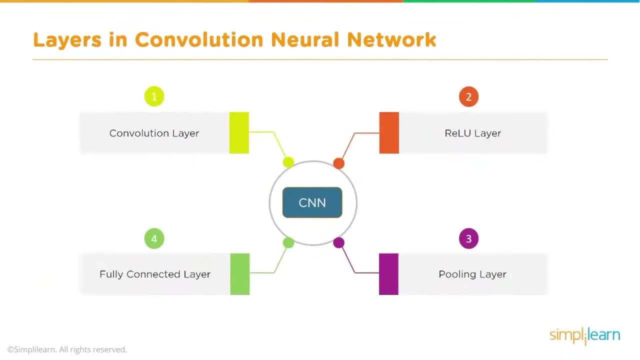 other one would have just been a matrix of just four dots. now we have a significantly larger image coming in, So, don't worry, We're going to bring this all together here in just a little bit. Layers in convolutional neural network. When we're looking at this, we have our convolution layer. 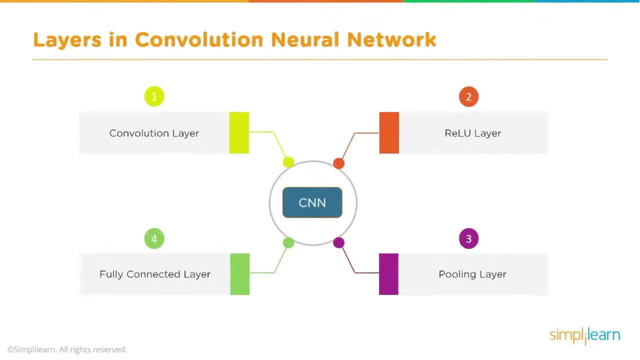 Okay, And that really is the central aspect of processing images in the convolutional neural network. That's why we have it, And then that's going to be feeding in And you have your relu layer, which is, you know, as we talked about, the rectified linear unit. 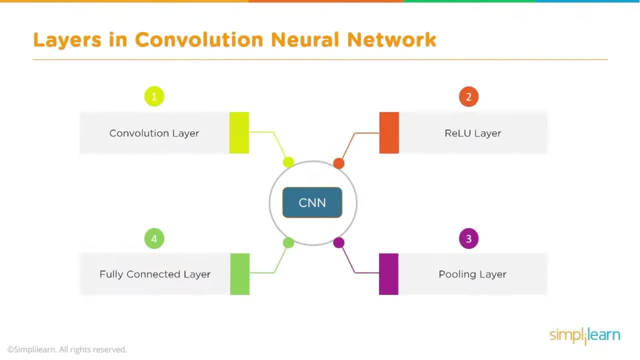 We'll talk about that in a little bit later. The relu is how that layer is activated. It's the math behind it what makes the neurons fire. You'll see that in a lot of other neural networks When you're using it just by itself. it's for processing smaller amounts of data. 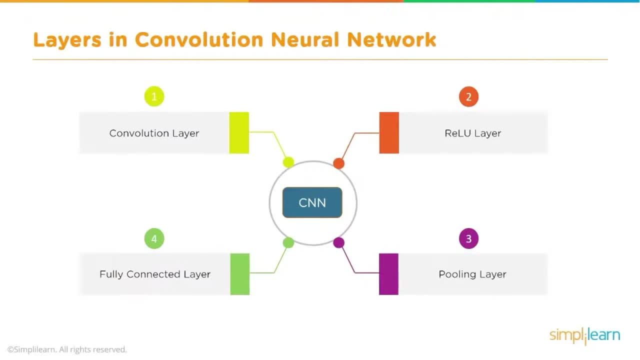 We use the atom activation feature for large data coming in. Now, because we're processing small amounts of data in each image, the relu layer works great. You have your pooling layer. That's where you're pooling the data together. Pooling is a neural network term that's very commonly used. I like to use a term: reduce. So if you're. 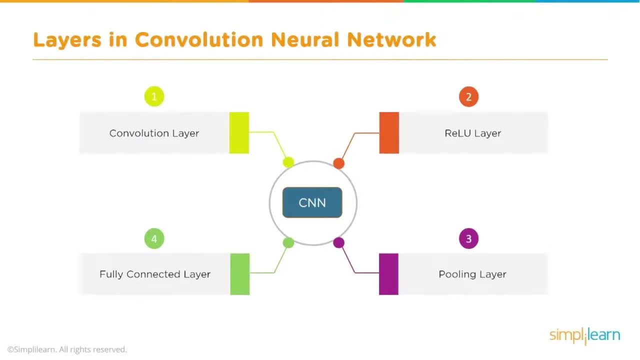 coming from the map and reduce side, you'll see that we're mapping all this data through all these networks And then we're going to reduce it, We're going to pool it together And then finally, we have the fully connected layer layer. That's where our output's going to come out. So we have started to look at 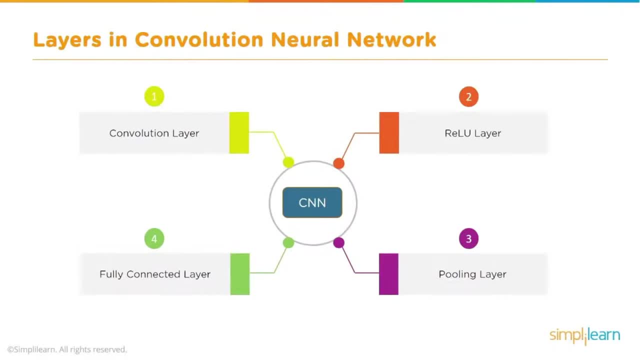 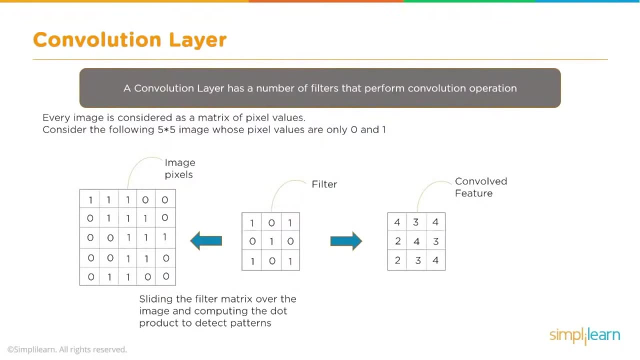 matrices. We've started to look at the convolutional layer and where it fits in and everything. We've taken a look at images, So we're going to focus more on the convolution layer. since this is a convolutional neural network, A convolution layer has a number of filters and perform convolutional 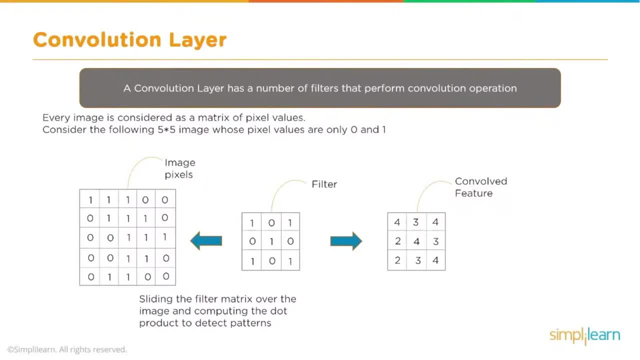 operation. Every image is considered as a matrix of pixel values. Consider the following 5x5 image, whose pixel values are only 0 and 1.. Now, obviously, when we're dealing with color, there's all kinds of things that come in on color. 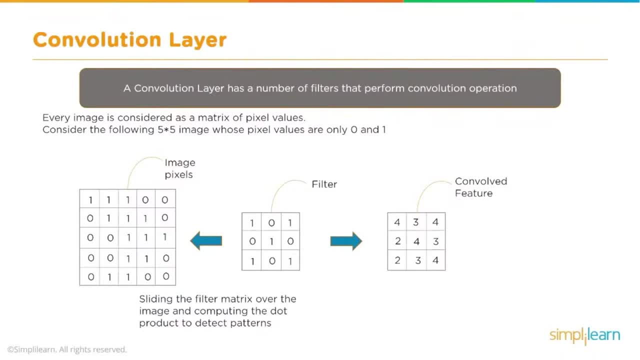 processing. But we want to keep it simple and just keep it black and white. And so we have our image pixels, So we're sliding the filter matrix over the image and computing the dot product to detect the patterns. And right here you're going. 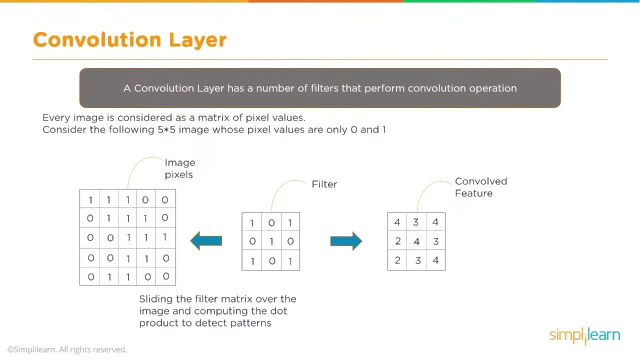 to ask: where does this filter come from? This is a bit confusing because the filter is going to be derived later on. We build the filters when we program or train our model, So you don't need to worry what the filter actually is. What you do need to understand how a convolution layer works is what is the 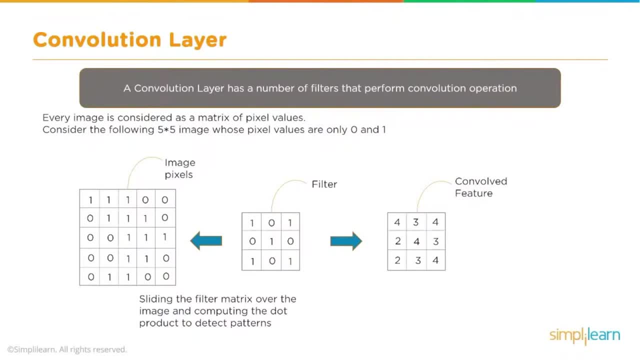 filter doing Filter. You'll have many filters. You don't have just one filter. You'll have lots of filters that are going to look for different aspects, And so the filter might be looking for just edges. It might be looking for different. 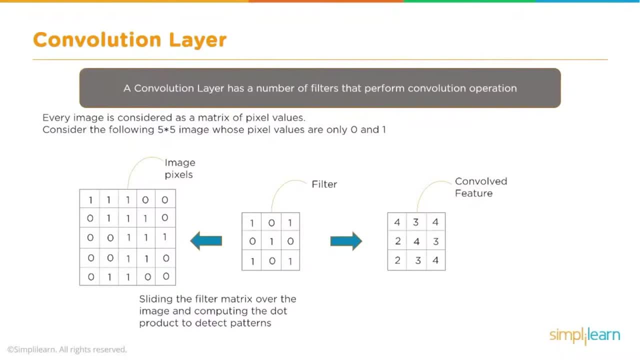 parts. We'll cover that a little bit more detail in a minute. Right now we're just focusing on how the filter works as a matrix. Remember, earlier we talked about multiplying matrices together And here we have our two-dimensional matrix And you can see, we take the filter and we multiply it. 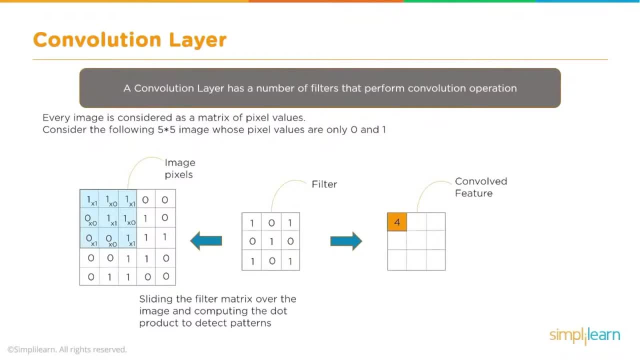 in the upper left image And you can see right here: 1 times 1,, 1 times 0,, 1 times 1.. We multiply those all together, then sum them and we end up with the convolved feature of 4.. We're going to take that and sliding the filter matrix over the 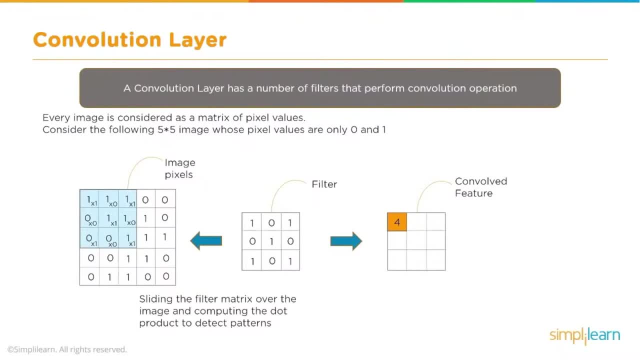 image and computing the dot product to detect patterns. So we're just going to slide this over. We're going to predict the first one and slide it over one notch, Predict the second one, and so on, and so on, all the way through until we 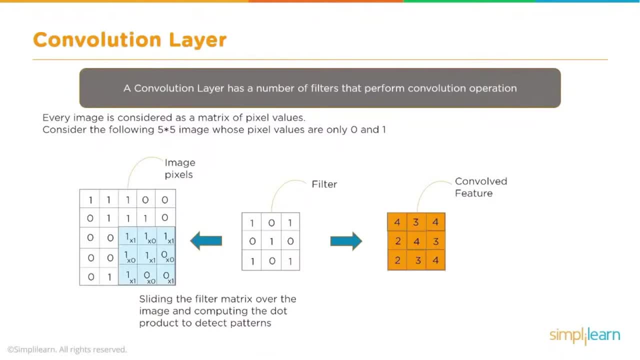 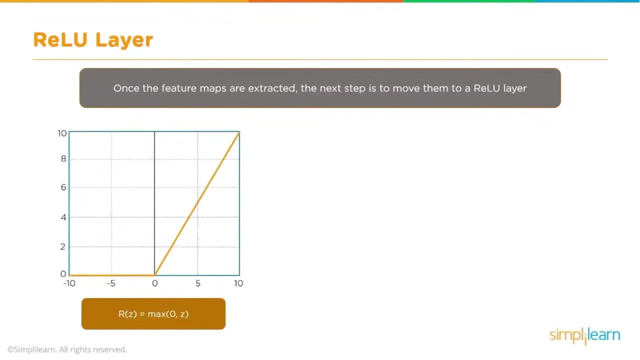 have a new matrix And this matrix, which is the same size as a filter, has reduced the image and whatever filter, whatever that's filtering out, it's going to be looking at just those features reduced down to a smaller matrix. So once the feature maps are extracted, the next step is to move them. 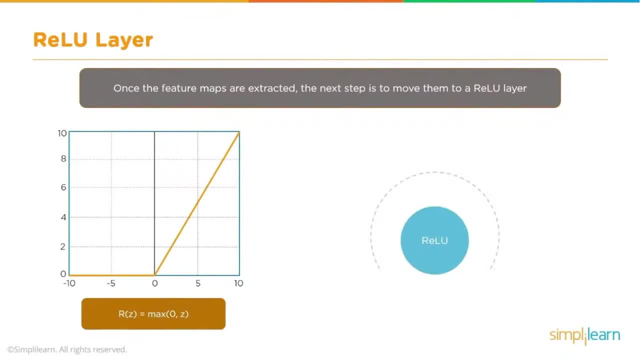 to the relu layer. So the relu layer. the next step first is going to perform an element-wise operation. So each of those maps coming in, if there's negative pixels, so it says all the negative pixels to 0, and you can see this nice graph. 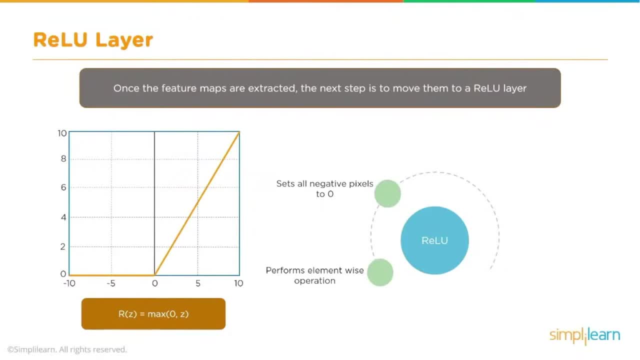 where it just zeroes out the negatives and then you have a value that goes from 0 up to whatever value is coming out of the matrix. This introduces non-linearity to the network. So up until now we have a- we say linearity We're talking about. 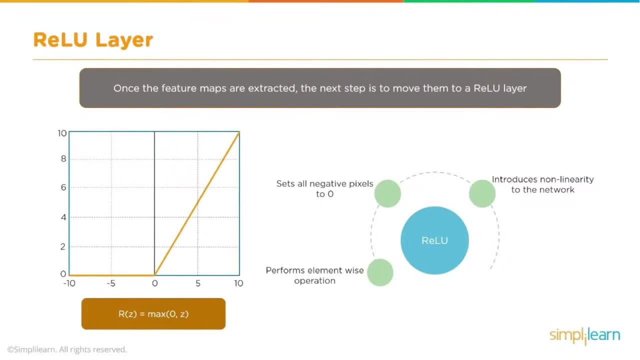 the fact that the feature has a value. So it's a linear feature. This feature came up and it has. let's say, the feature is the edge of the beak, you know it's like, or that backslash that we saw. It'll look at that and say, okay, this feature has a. 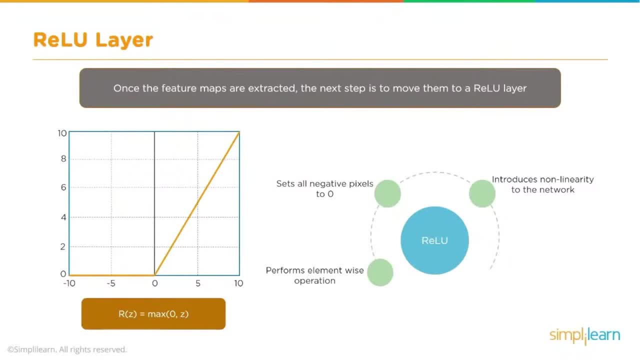 value from negative 10 to 10. in this case, If it was 1, it'd say, yeah, this might be a beak, It might not, It might be an edge right there. A minus 5 means no, we're not even going to look at it, It's a 0.. And 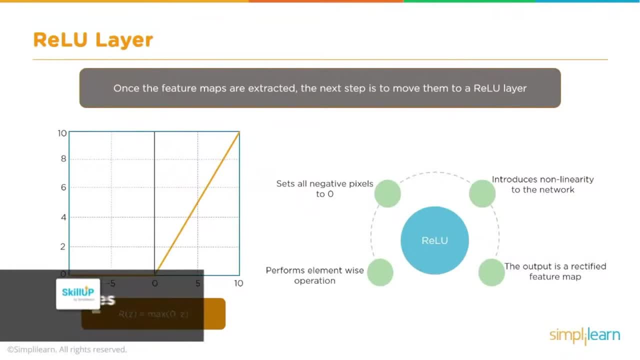 so we end up with an output, and the output takes all these features, all these filtered features. Remember, we're not just running one filter on this, We're running a number of filters on this image. And so we end up with a rectified feature map that is looking at just the features coming through and how. 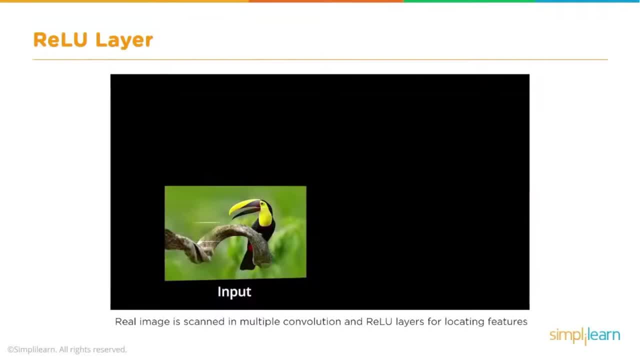 they weigh in from our filters. So here we have an input of a. it looks like a toucan bird, very exotic looking. Real image is scanned in multiple convolution and the ReLU layers for locating features And you can see up here it's. 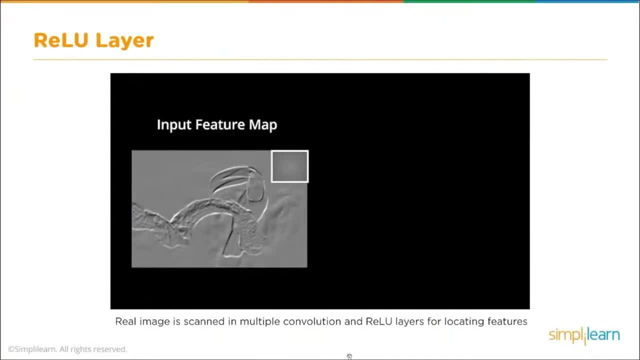 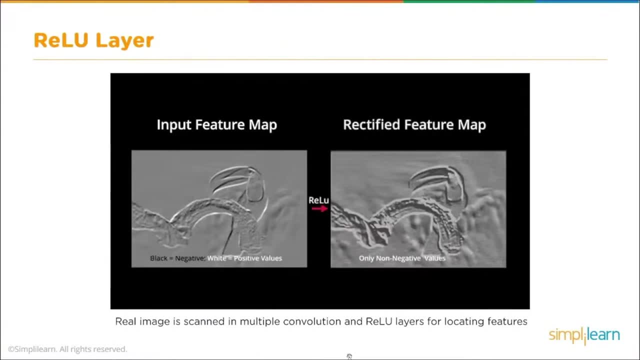 turned it into a black and white image And in this case we're looking in the upper right-hand corner for a feature, and that box scans over A lot of times. it doesn't scan one pixel at a time. A lot of times it will skip by two or 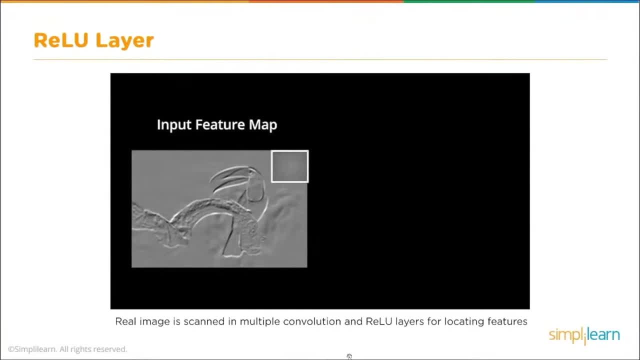 three or four pixels to speed up the process. That's one of the ways you can compensate if you don't have enough resources on your computation for large images- And it's not just one filter slowly goes across the image You have. multiple filters have been programmed in there, So you're looking at. 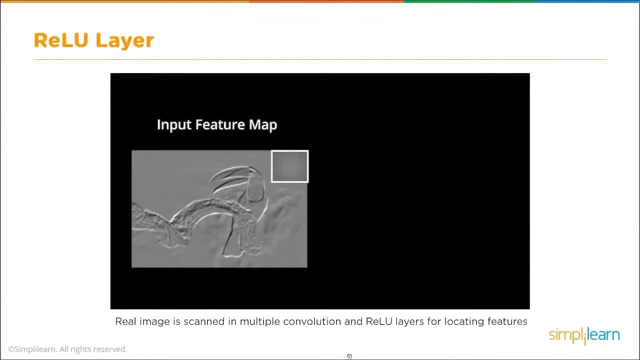 a lot of different filters going over the different aspects of the image and just sliding across there and forming a new matrix. One more aspect to note about the ReLU layer is we're not just having one ReLU coming in. So not only do we, 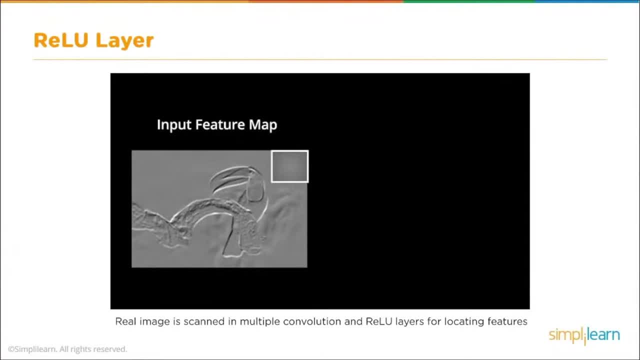 have multiple features going through, but we're generating multiple ReLU layers for locating the features. That's very important to note, you know. So we have a quite a bundle. We have multiple filters, multiple ReLU, which brings us to the next step forward: propagation. Now we're 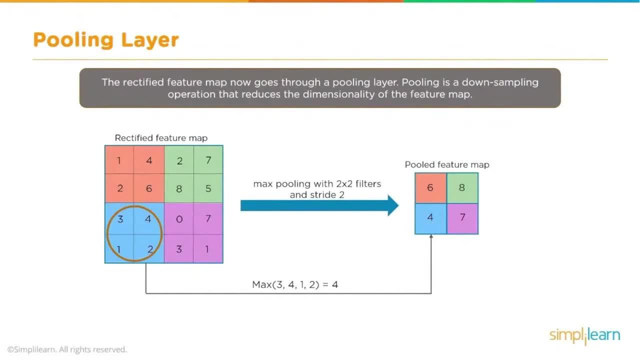 going to look at the pooling layer. The rectified feature map now goes through a pooling layer. Pooling is a down sampling operation that reduces the dimensionality of the feature map. That's all we're trying to do. We're trying to take a huge amount of information and reduce it down to a single answer- This: 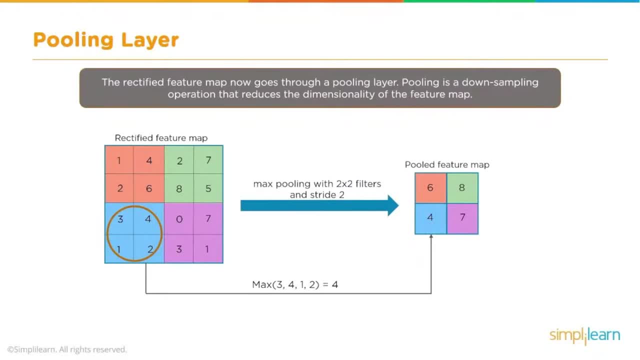 is a specific kind of bird, This is an iris, This is a rose. So you have a rectified feature map and you see, here we have our rectified feature map coming in. We set the max pooling with a 2 by 2 filter Those and a stride of 2, and if 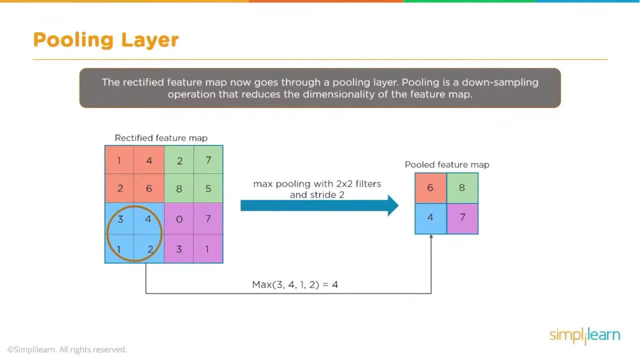 you remember correctly, I talked about not going one pixel at a time. Well, that's where the stride comes in. We end up with a 2 by 2 pooled feature map, but instead of moving one over each time and looking at every possible combination, we 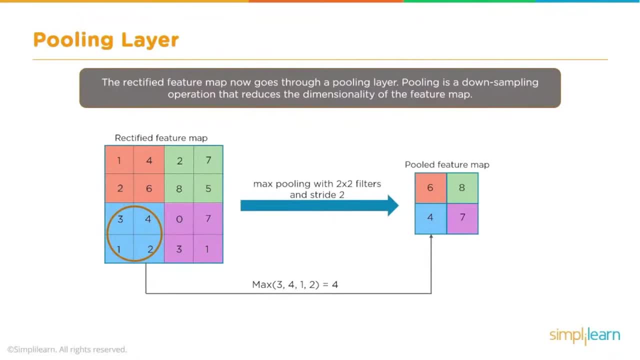 skip, we skip a few. there, We go by two. We skip every other pixel, We just do every other one, And this reduces our rectified feature map which, as you can see over here, 16 by 16 to a 4 by 4.. So we're continually. 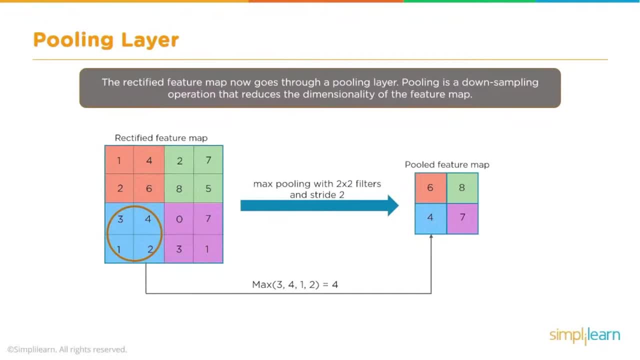 trying to filter and reduce our data so that we can get to something we can manage. And over here you see that we have the max 3,, 4,, 1, and 2.. And in the max pooling we're looking for the max value. 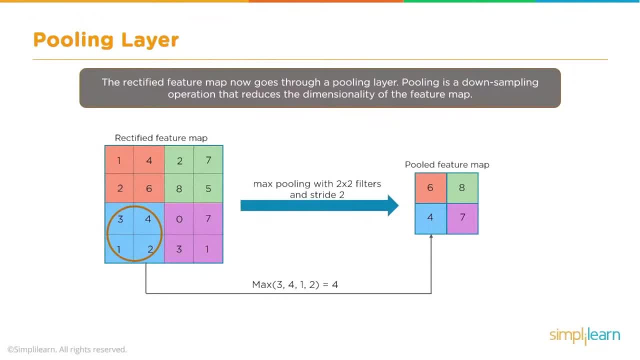 a little bit different than what we were looking at before. So, coming from the rectified feature, we're now finding the max value and then we're pooling those features together. So, instead of think of this as image of the map, think of this as: how valuable is a feature in that area? How much? 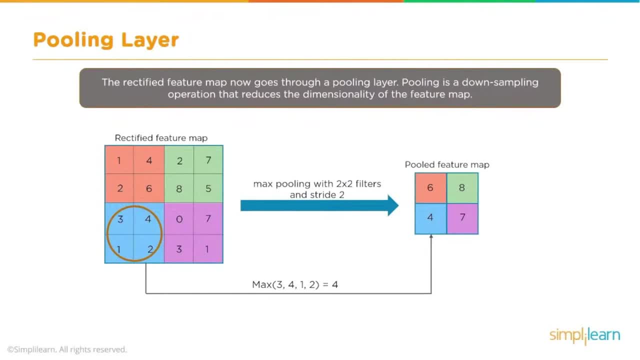 of a feature value do we have And we just want to find the best or the maximum feature for that area. They might have that. one piece of the filter of the beak said: oh, I see a 1 in this beak in. 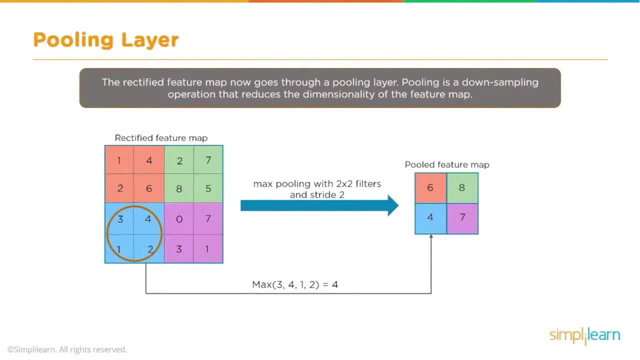 this image And then it skips over and says I see a 3 in this image And it says, oh, this one is rated as a 4.. We don't want to sum it together because then you know you might have like. 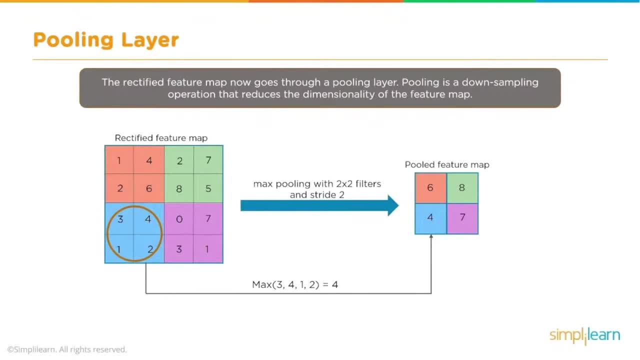 five 1s and it'll say: ah, 5.. But you might have four 0s and one 10.. And that 10,. you might have four 0s and one 10. And that 10,. you might have four 0s and one 10. And that 10,. 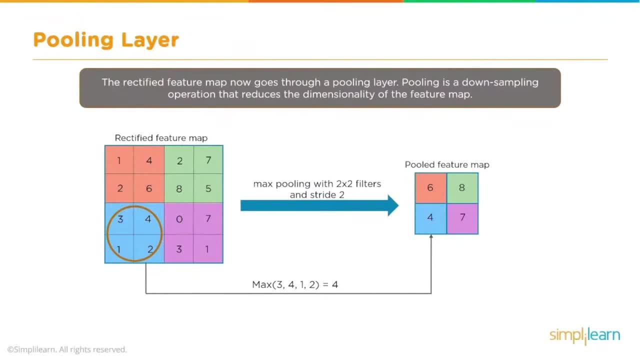 says, well, this is definitely a beak, where the 1s will say: probably not a beak. A little strange analogy, since we're looking at a bird. But you can see how that pooled feature map comes down And we're just looking for the max value in each one of those matrices. Pooling layer uses. 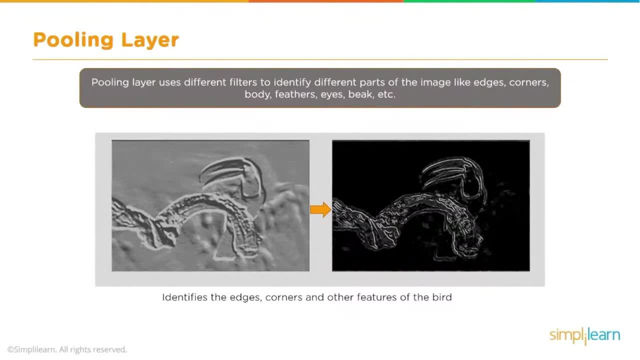 different filters to identify different parts of the image, like edges, corners, body feathers, eyes, beak, et cetera. I know I focus mainly on the beak, but obviously each feature could be a different part of the bird coming in. So let's take a look at what. 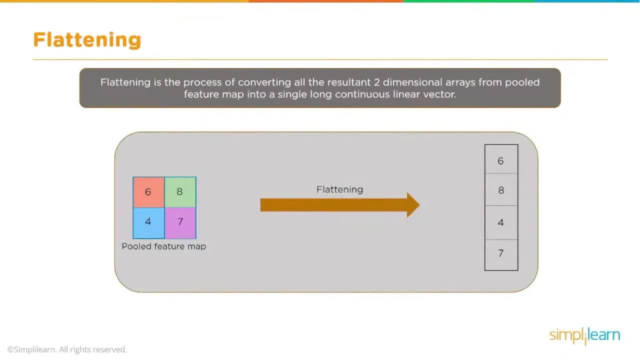 that looks like Structure of a convolution neural network. so far, This is where we're at right now. We have our input image coming in And then we use our filters- And there's multiple filters on there that are being developed- to kind of twist and change that data, And so we 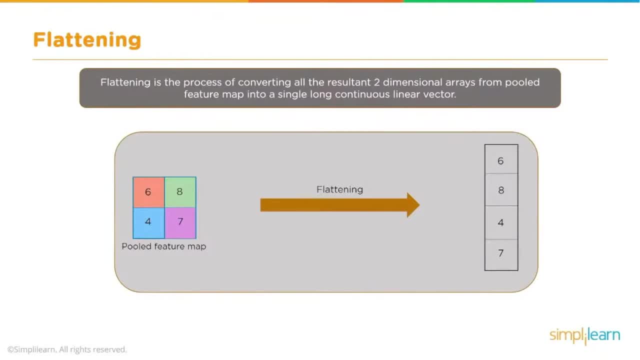 multiply the matrices. We take that little filter, Maybe it's a 2 by 2. We multiply it by each piece of the image And if we step 2, then it's every other piece of the image. That generates multiple convolution layers. So we have a number of convolution layers. We have a number of 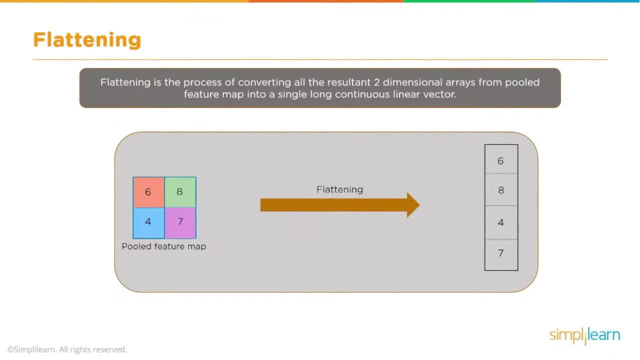 setup in there, just looking at that data. We then take those convolution layers, We run them through the ReLU setup And then, once we've done through the ReLU setup and we have multiple ReLUs going on, multiple layers that are ReLU, then we're going to take those multiple layers. 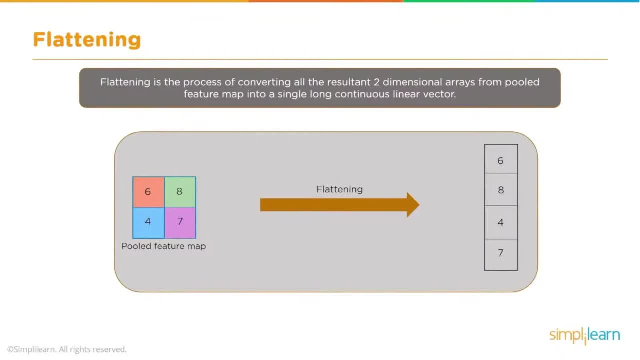 and we're going to be pooling them. So now we have the pooling layers, or multiple poolings, going on Up until this point. we're dealing with- sometimes it's multiple dimensions. You can have three dimensions, some strange data setups that aren't doing images but looking at other things. They 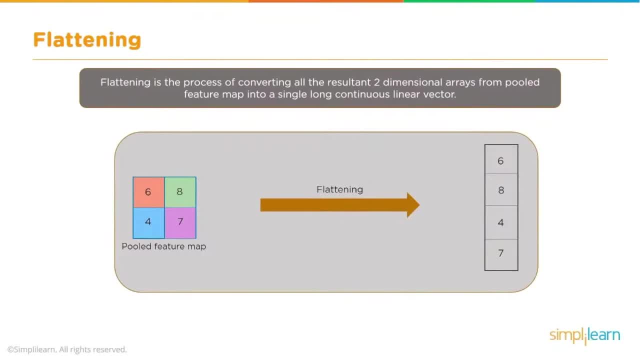 can have four, five, six, seven dimensions. So right now we're looking at 2D image dimensions coming in into the pooling layer. So the next step is we want to reduce those dimensions or flatten them. So flattening- Flattening is a process of 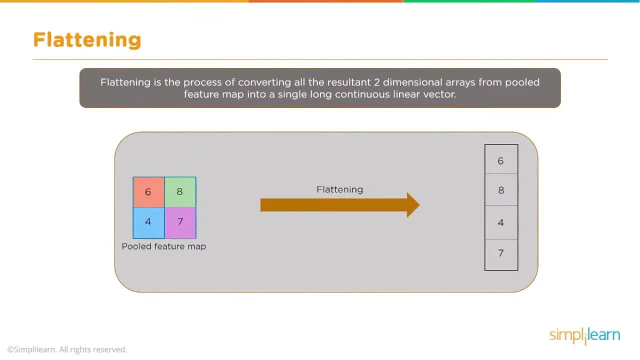 converting all of the resultant two-dimensional arrays from pooled feature map into a single long, continuous linear vector. So over here you see where we have a pooled feature map- Maybe that's the bird wing- And it has values 6,, 8,, 4,, 7.. And we want to just flatten this out and turn. 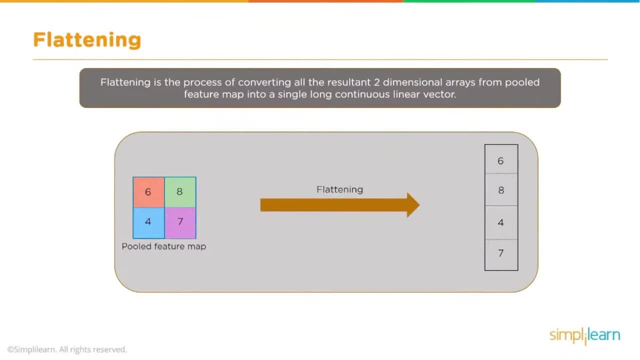 it into 6,, 8,, 4,, 7 or a single linear vector. So we're going to do that, And then we're going to go ahead and do a long linear vector And we find out that not only do we do each of the pooled 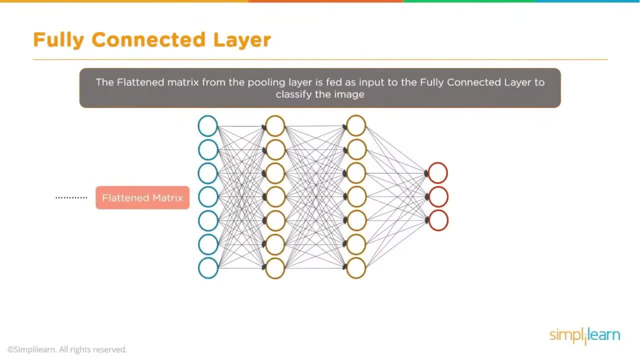 feature maps. we do all of them into one long linear vector. So now we've gone through our convolutional neural network part and we have the input layer into the next setup. All we've done is taken all those different pooling layers and we flattened them out and combined them into a 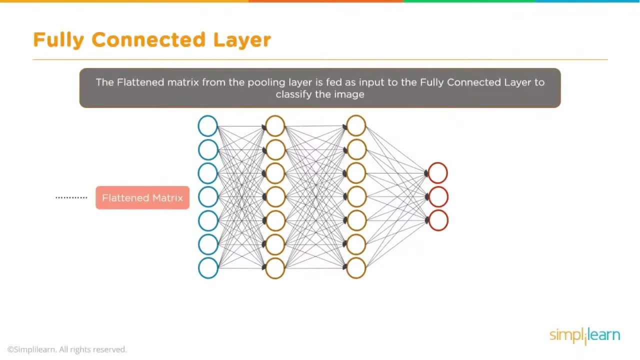 single linear vector going in. So after we've done the flattening, we have just a quick recap, because we've covered so much. So it's important to go back and take a look at each of the steps we've through. The structure of the network so far is we have our convolution, where we 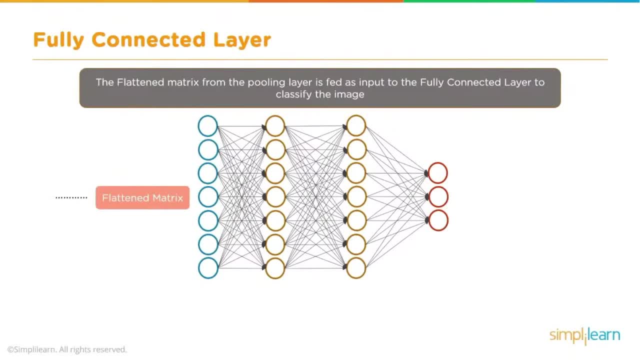 twist it and we filter it and multiply the matrices. We end up with our convolutional layer, which uses the relu to figure out the values going out into the pooling. As you have numerous convolution layers that then create numerous pooling layers pooling that data together, which is the max value. 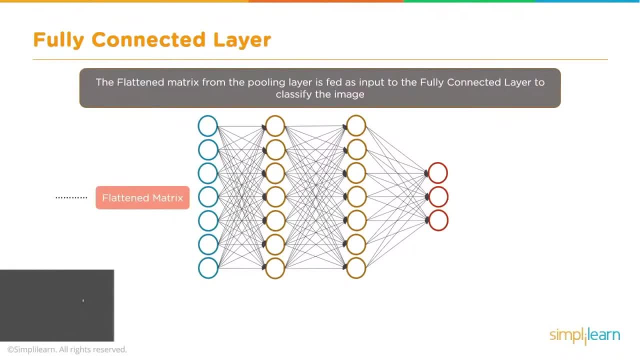 Which one we want to send forward. we want to send the best value, And then we're going to take all of that from each of the pooling layers and we're going to flatten it and we're going to combine them into a single input going. 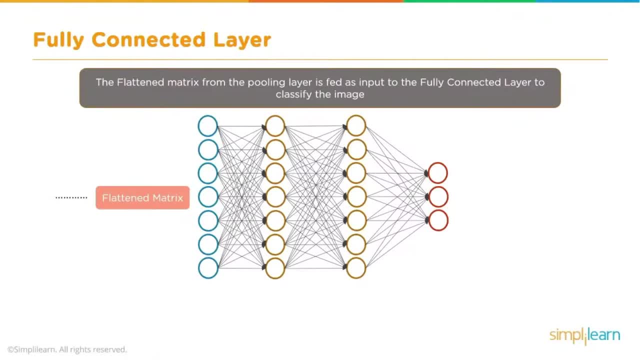 into the final layer. Once you get to that step- you might be looking at that going boy. that looks like the normal intro it to most neural network. and you're correct, it is So. once we have the flattened matrix from the pooling layer, that becomes our input. So the pooling layer is fed as an input to the fully. 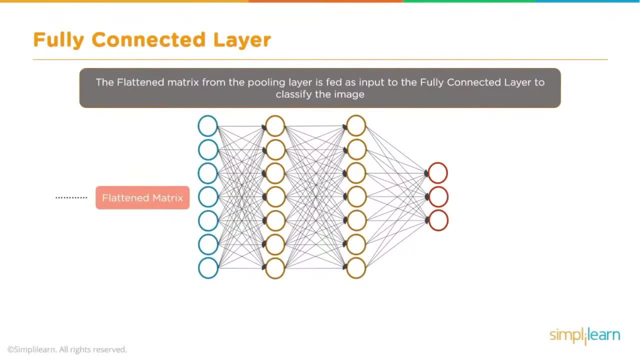 connected layer to classify the image So you can see as our flatten matrix comes in. In this case we have the pixels from the flatten matrix fed as an input back to our toucan or whatever that kind of bird that is. I need one of these to 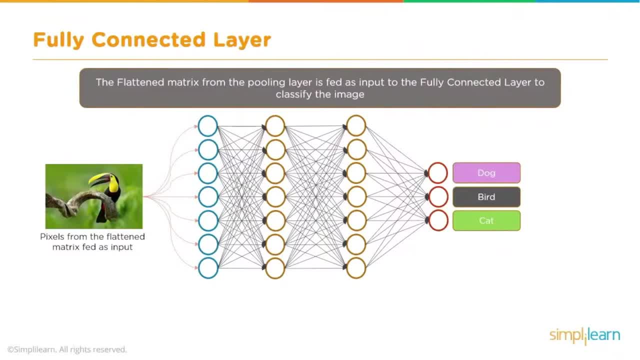 identify what kind of bird that is, It comes into our forward propagation network and that will then have the different weights coming down across and then finally it selects that that's a bird and that it's not a dog or a cat. in this case, Even though it's not labeled, the final layer there in red is our. 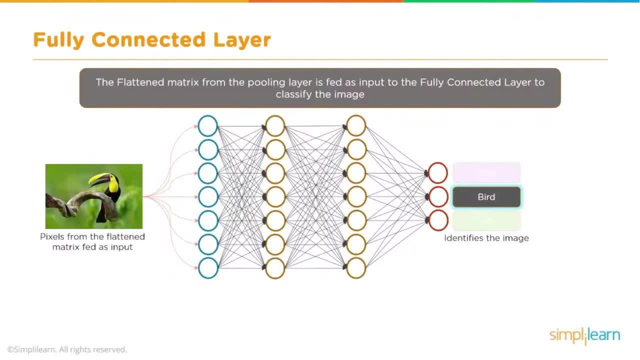 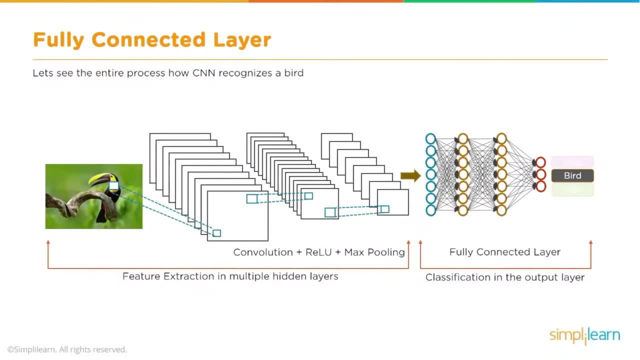 output layer, Our final output layer that says bird, cat or dog. So quick recap of everything we've covered so far. We have our input image which is twisted and multiplied. The filters are multiplied times the matrix, The two matrixes multiplied all the filters to create our convolution layer, Our convolution layers. 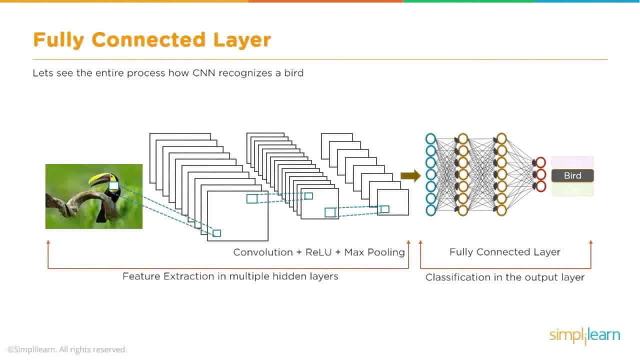 there's multiple layers in there because it's all building multiple layers off the different filters, Then goes through the ReLU as its activation and that creates our pooling. And so once we get into the pooling layer, we then, and the pooling look for who's the best, What's the max value coming in from our 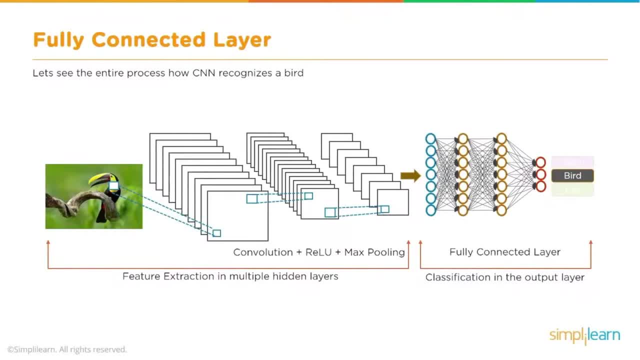 convolution, And then we take that layer and we flatten it, and then it goes into a fully connected layer, Our fully connected neural network, and then to the output, And here we can see the entire process: how the CNN recognizes a bird. This is kind of nice. 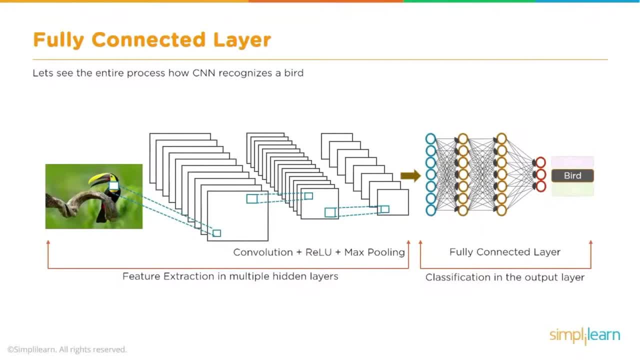 because it's showing the little pixels and where they're going. You can see the filter is generating this convolution network and that filter shows up in the bottom part of the convolution network And then, based on that, it uses the ReLU for the pooling. The pooling then find out which one's the best, and so on all. 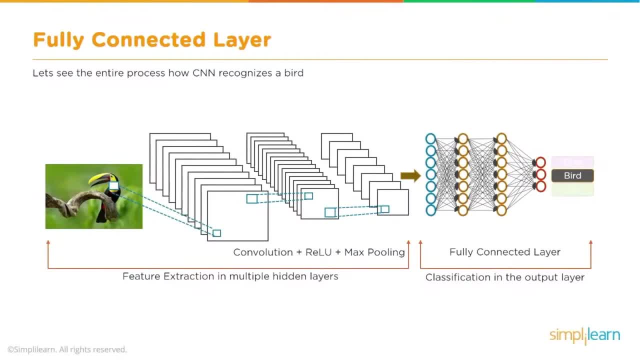 the way to the fully connected layer, So that's a classification neural network at the end, or the classification and the output layer, So that'd be a classification neural network at the end. So we covered a lot of theory up till now and you can imagine each one of these steps has to be. 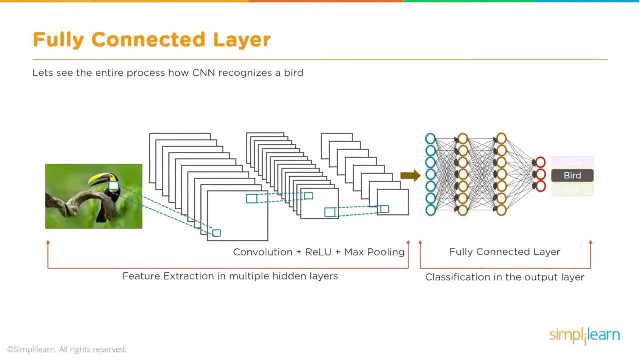 broken down in code, So putting that together can be a little complicated. Not that each step of the process is overly complicated, but because we have so many steps, We have one, two, three, four, five different steps going on here with 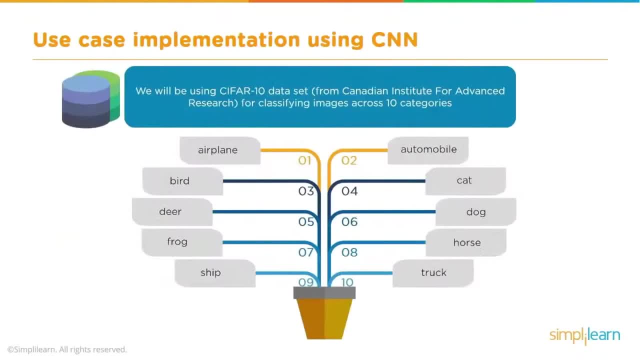 substeps in there. We're going to break that down and walk through that in code. in our use case implementation using the CNN, we'll be using the CIFAR-10 data set from Canadian Institute for Advanced Research for classifying images across 10 categories. Unfortunately, they 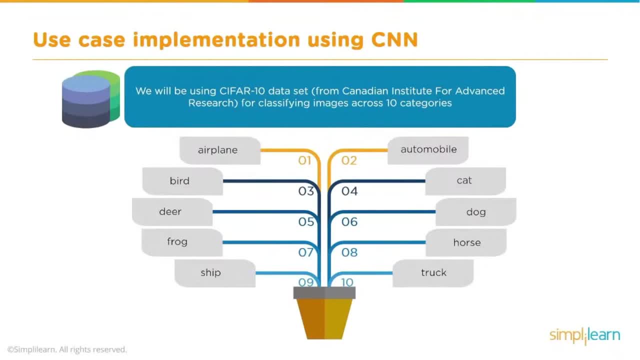 don't let me know whether it's going to be a toucan or some other kind of bird, but we do get to find out whether it can categorize between a ship, a frog, deer bird, airplane, automobile, cat, dog. 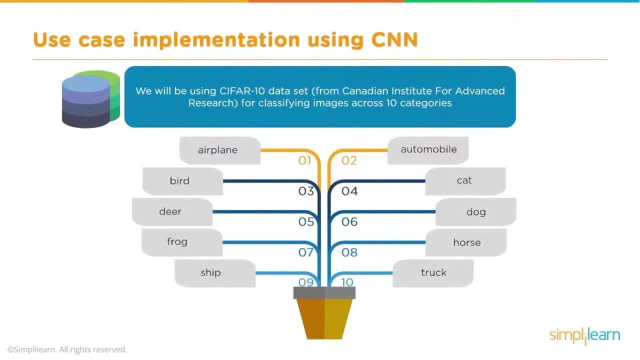 horse truck. So that's a lot of fun. And if you're looking anything in the news at all of our automated cars and everything else, you can see where this kind of processing is so important in today's world and very cutting edge as far as what's coming out in the commercial deployment. 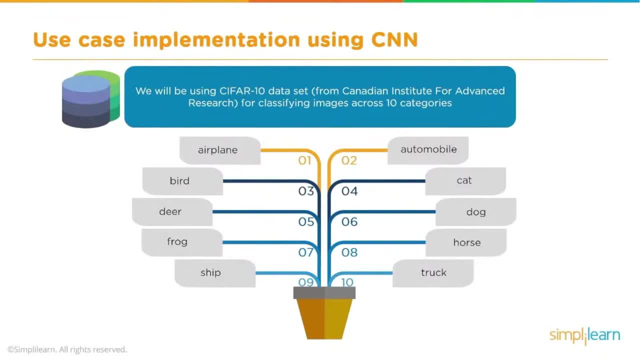 I mean, this is really cool stuff. We're starting to see this just about everywhere in industry, So great time to be playing with this and figuring it all out. Let's go ahead and dive into the code and see what that looks like when we're actually writing our script. Before we go on, let's do one. 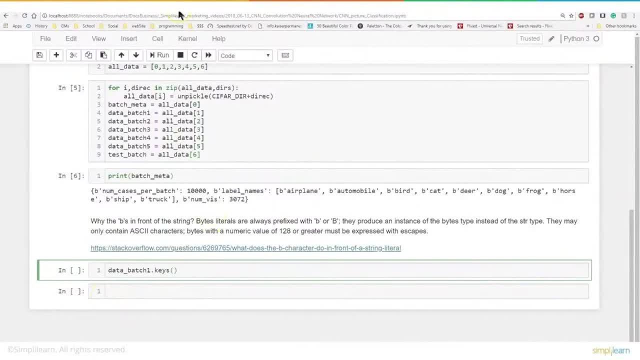 more quick look at what we have here. Let's just take a look at data background And remember in Jupyter Notebook I can get by with not doing the print statement. If I put a variable down there, it'll just display the variable And you can see in our data batch one for the. 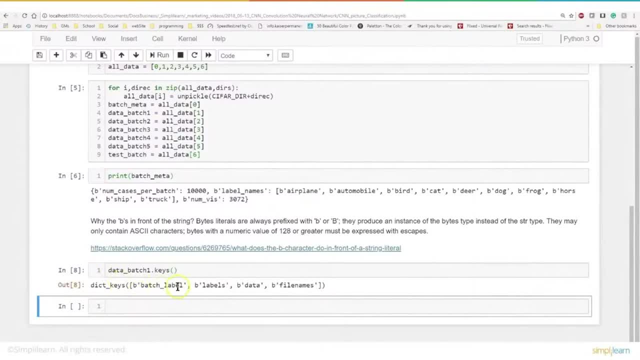 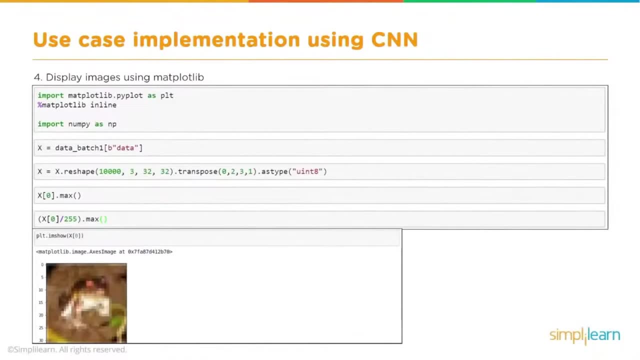 keys. since this is a dictionary, we have the batch one, label, data and file names, So you can actually see how it's broken up in our data set. So for the next step, or step four as we're calling it, we want to display the image using matplot library. There's many ways to display the images. 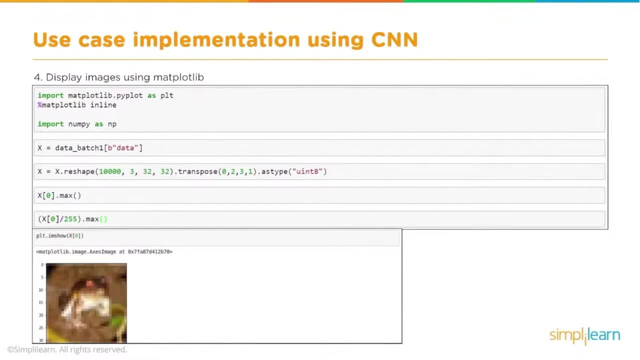 You could even. There's other ways to drill into it, But matplot library is really good for this- And we'll also look at our first reshape setup, or shaping the data, so you can have a little glimpse into what that means. So we're 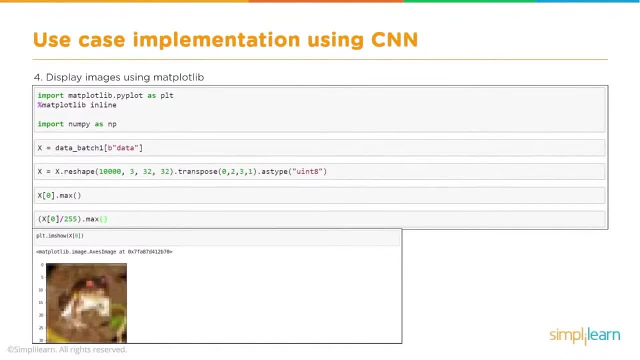 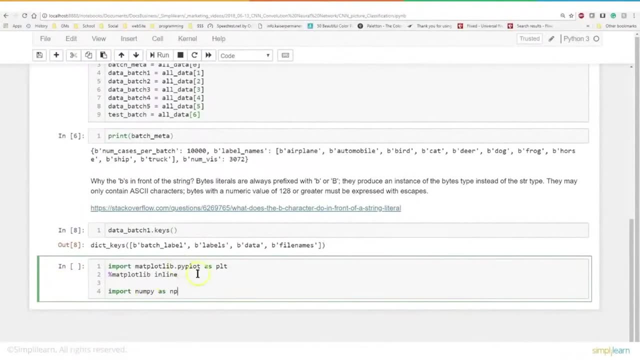 going to start by importing our matplot And of course, since I am doing Jupyter Notebook, I need to do the matplot inline command, so it shows up on my page. So here we go, We're going to import matplot- librarypyplot. 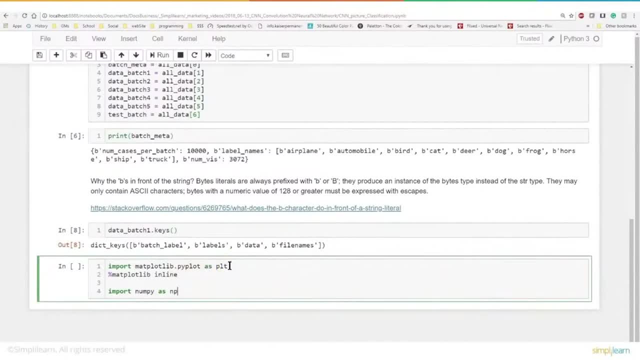 as plt. And if you remember matplot library, the pyplot is like a canvas that we paint stuff onto And then we're going to import numpy as np. There's my % matplot library inline, So it's going to show up in my notebook. And then of 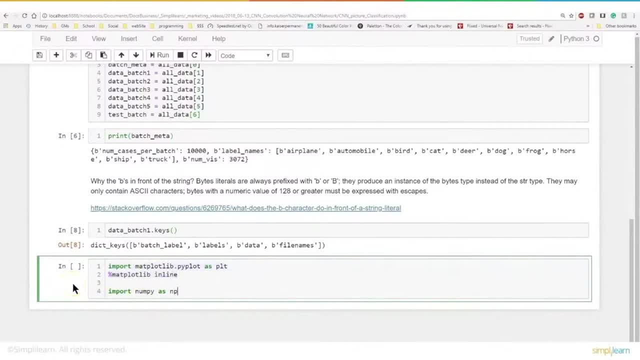 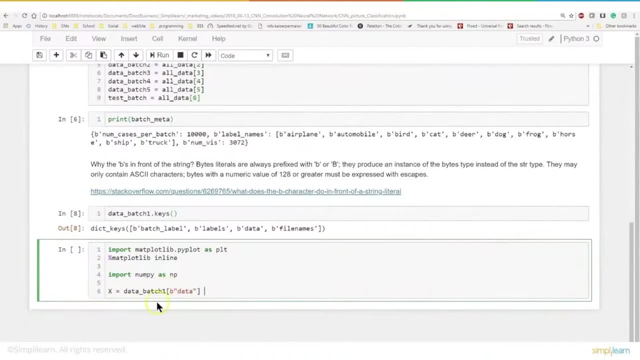 course we're going to import numpy as np for our Numbers Python array setup. And let's go ahead and set x equals to data batch 1.. So this will pull in all the data going into the x value. And then, because this is just a long stream of 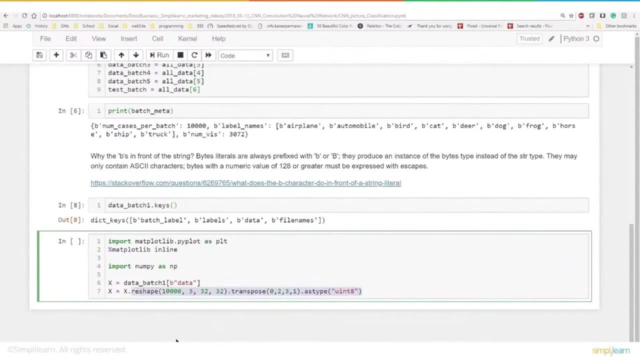 binary data. we need to go a little bit of reshaping. So in here we have to go ahead and reshape the data. We have 10,000 images. Okay, that looks correct And this is kind of an interesting thing. It took me a little bit to. I had to go research this. 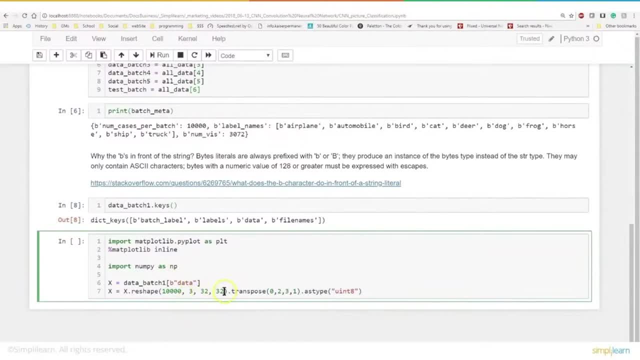 myself to figure out what's going on with this data And what it is is. it's a 32 by 32 picture And let me do this, Let me go ahead and do a drawing pad on here, So we have 32 bits by 32 bits and it's in color, So there's three bits of color And then 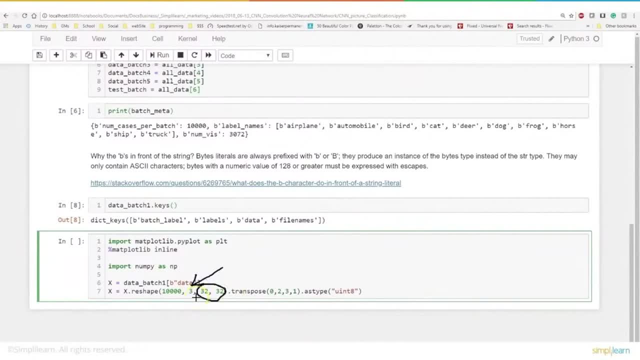 we have 32 bits of color Now. I don't know why the data is particularly like this. It probably has to do with how they originally encoded it, But most pictures put the three afterward. So what we're doing here is we're going to take the shape. 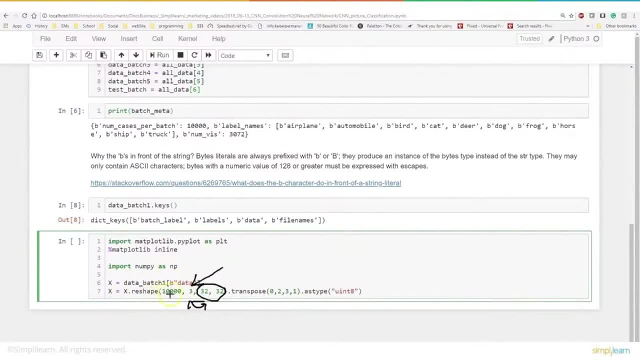 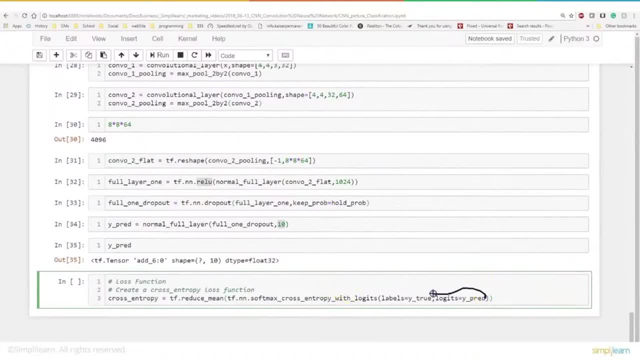 information, And then we're going to take the data, which is just a long stream of information, And then we're going to take the data, which is just a long stream of exactly what that is. let's take a look and see what we're feeding it. We're going to feed it. 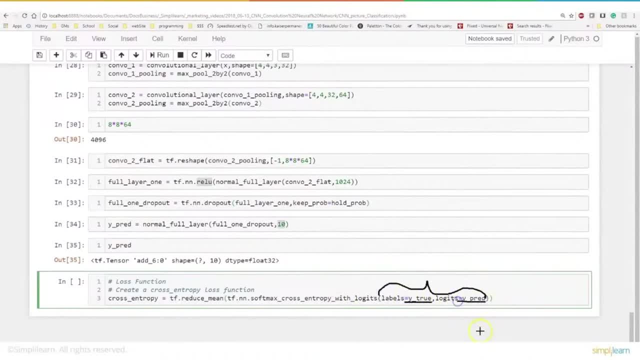 our labels and we have our true labels and our prediction labels. So coming in here is where the two different variables we're sending in, or the two different probability distributions, is one that we know is true and what we think it's going to be. Now, this function right here when they 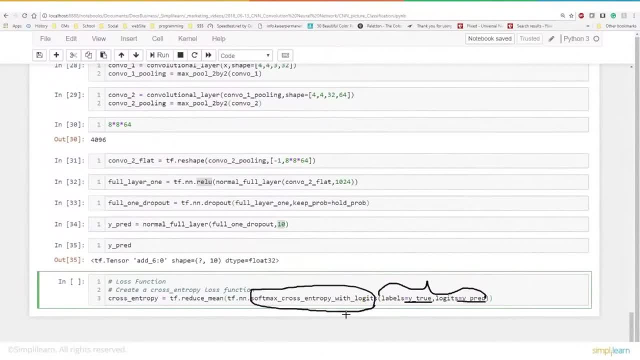 talk about cross entropy. in information theory, the cross entropy between two probability distributions over the same underlying set of events measures the average number of bits needed to identify an event drawn from the set. That's a mouthful, Really. we're just looking at the amount. 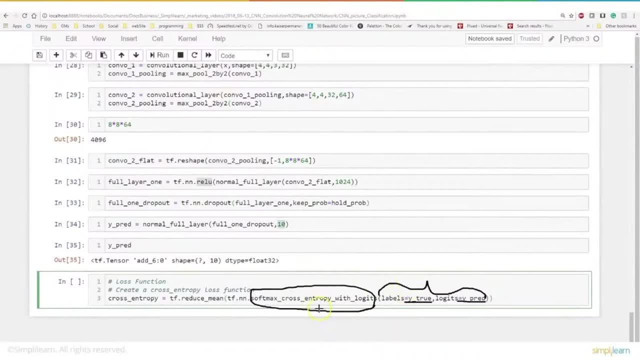 of error in here, How many of these are correct and how many of these are incorrect. So how much of it matches? And we're going to look at that. we're just going to look at the average. That's what the mean, the reduced to the mean, means here. So we're looking at the average error on this. 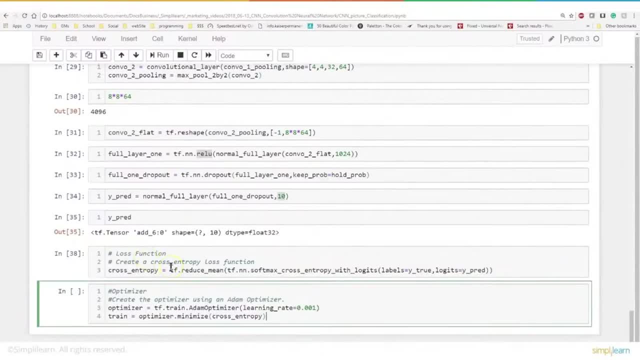 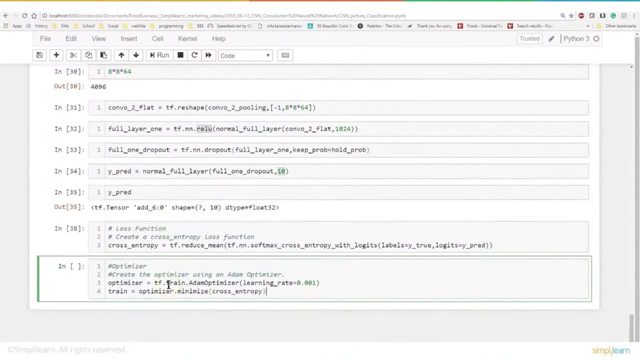 And so the next step is we're going to take the error. We want to know our cross entropy or our loss function, how much loss we have. That's going to be part of how we train the model. So when you know what the loss is and we're training it, you feed that back into. 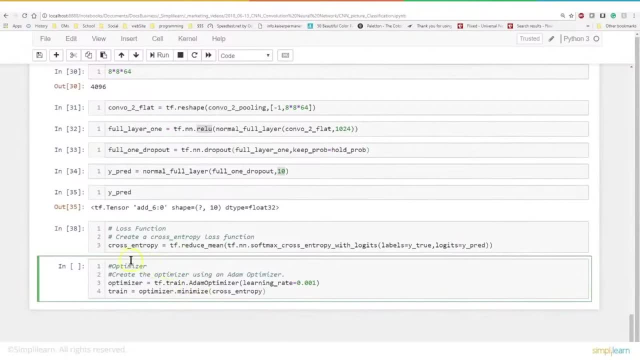 the back propagation setup, And so we want to go ahead and optimize that. Here's our optimizer. We're going to create the optimizer using an atom optimizer. Remember, there's a lot of different ways of optimizing the data. Atom's the most popular used, So our optimizer is going to equal 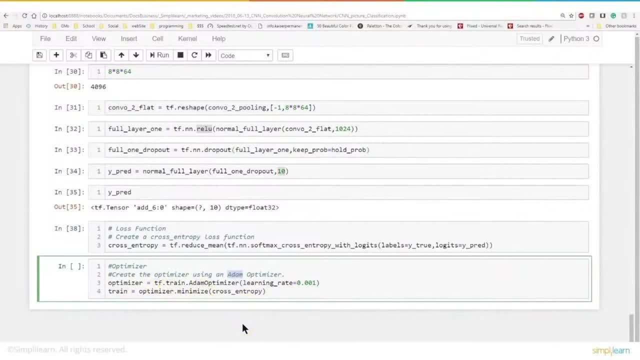 the tftrain atom optimizer. If you don't remember what the learning rate is, let me just pop this back into here. Here's our learning rate When you have your weights. you have all your weights and your different nodes that are coming out. Here's our node coming out. It has all its. 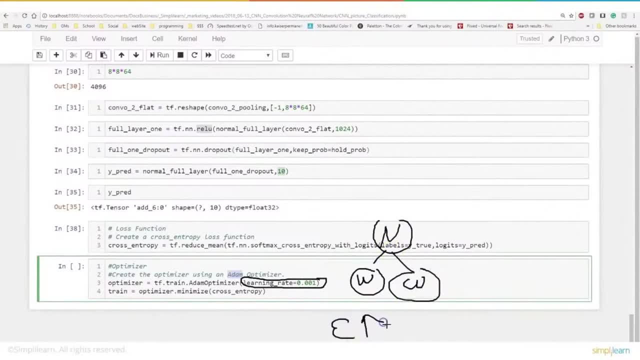 weights And then the error is being sent back through in reverse on our neural network. So we take this error and we adjust these weights based on the different formulas. In this case, the atom formula is what we're using. We don't want to just adjust them completely. We don't want to 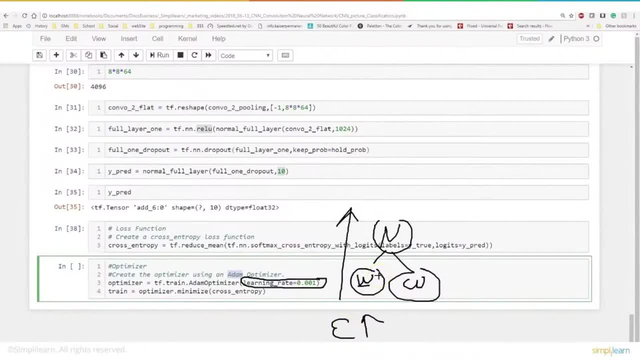 change this weight so it exactly fits the data coming through, Because if we made that kind of bias to whatever the last data we sent through is, Instead we're going to multiply that by 0.001 and make a very small shift in this weight. So our delta w is only 0.001 of the actual delta w of the. 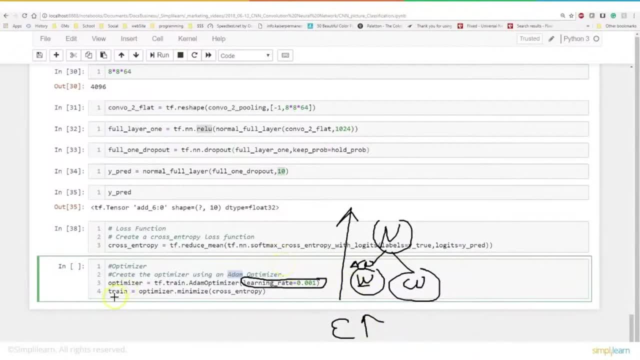 full change. we're going to compute from the atom And then we want to go ahead and train it. So our training or set up a training variable or function, And this is going to equal our optimizer, minimize cross entropy, And we make sure we go ahead and run this So it's loaded in there And 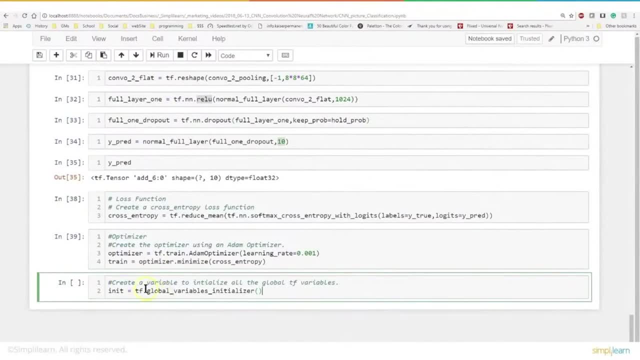 we're almost ready to train our model. But before we do that, we need to create one more variable in here And we're going to create a variable to initialize all the global TF variables. And when we look at this- the TF global variable initializer- this is a TensorFlow object. It goes through there. 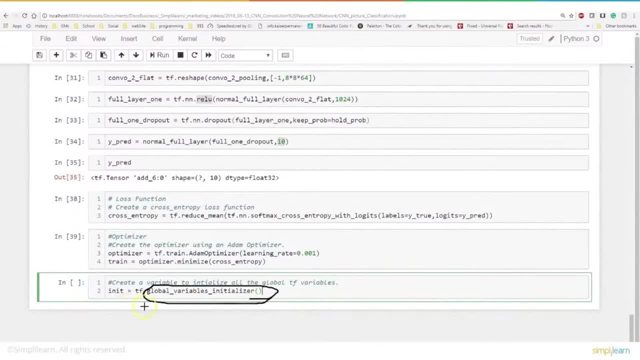 and it looks at all our different setup that we have going under our TensorFlow and then initializes those variables. So it's kind of like a magic wand, because it's all hidden in the back of the model And the trick about this is that you have to have the initialization on there, which is an 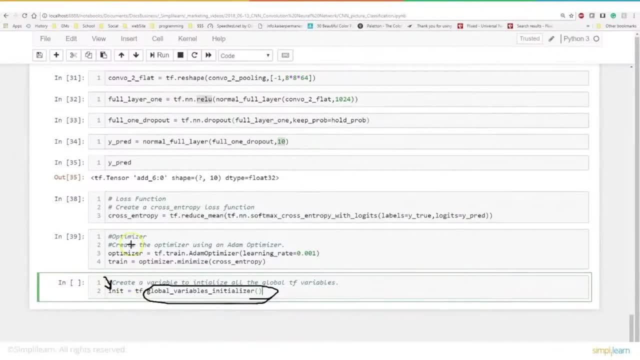 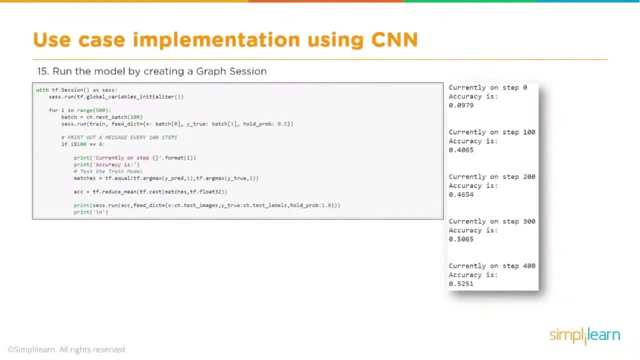 operation And you have to run that once you have your setup going. So we'll go ahead and run this piece of code And then we're going to go ahead and train our data. So let me run this. So it's loaded up there. 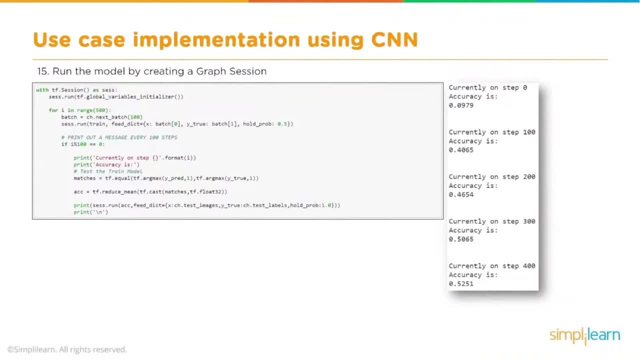 And so now we're going to go ahead and run the model by creating a graph session. Graph session is a TensorFlow term, So you'll see that coming up. It's one of the things that throws me, because I always think of GraphX and Spark and Graph as just general graph code And I know that's a little bit too much for me. I can go. 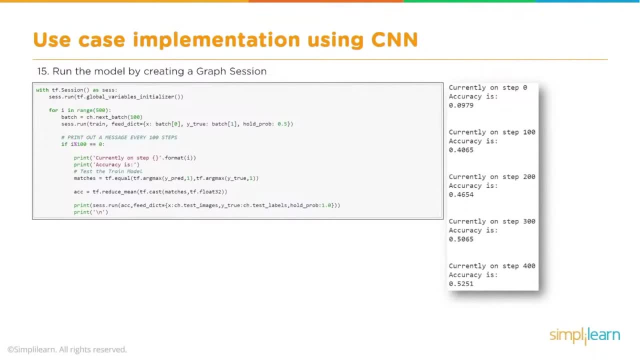 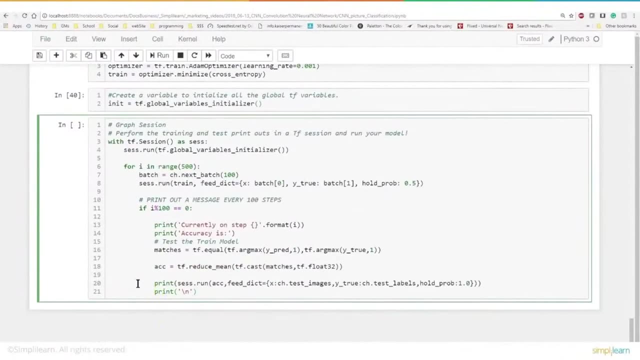 but they talk about a graph session. So we're going to go ahead and run the model And let's go ahead and walk through this what's going on here, And let's paste this data in here. And here we go. So we're going to start off with a TF session as SES, So that's our actual TF session. 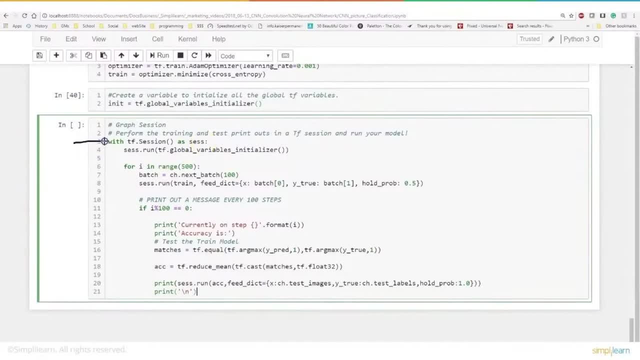 we've created. So we're right here with the TF session, Our session. we're creating, we're going to run TF global variable initializer. So right off the bat, we're initializing our variables here And then we have for I and range, 500.. So what's going on here? remember 500, we're going. 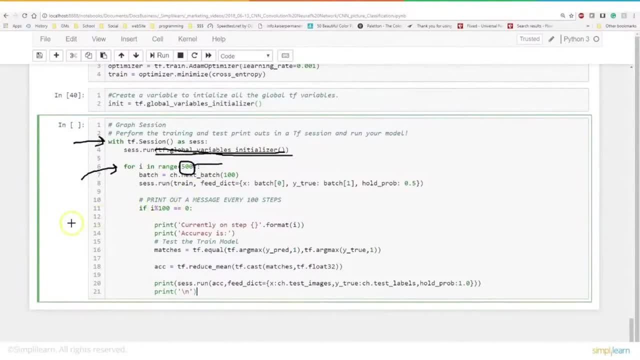 to break the data up and we're going to batch it in at 500 points each. We've created our session run, So we're going to do with TF session as session right here. We've created our variable session And then we're going to run and we're going to go ahead and initialize it. So we have. 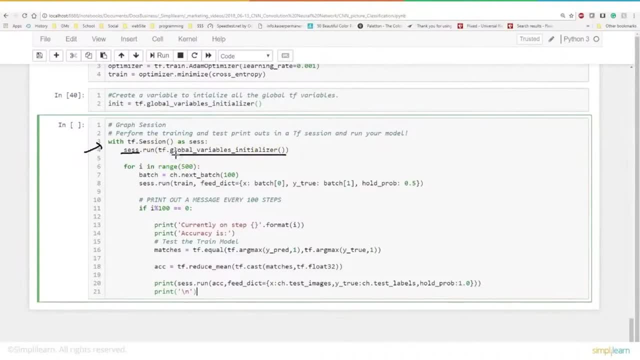 our TF global variables initializer that we created. That initializes our session in here. The next thing we're going to do is we're going to go for I and range of 500 batch equals chnext batch. So if you remember correctly, this is: 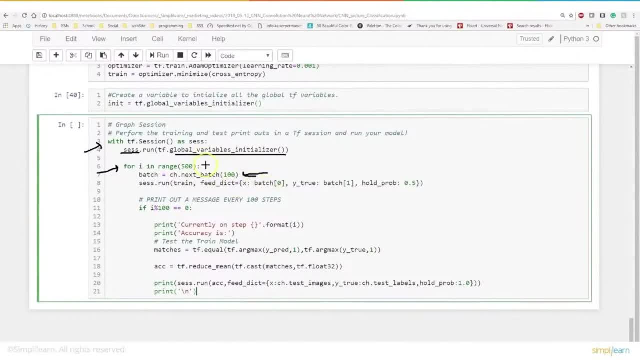 loading up 100 pictures at a time And this is going to loop through that 500 times. So we are literally doing what is that? 500 times 100 is 50,000.. So that's 50,000 pictures we're going to. 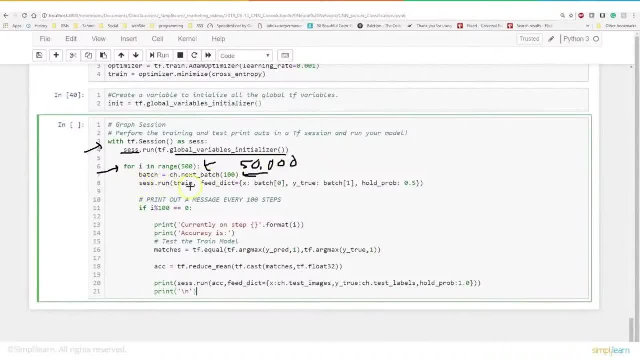 process right there And the first process is: we're going to do a session run. We're going to take our train. We created our train variable or optimizer in there. We're going to feed it the dictionary. We had our feed dictionary that we created And we 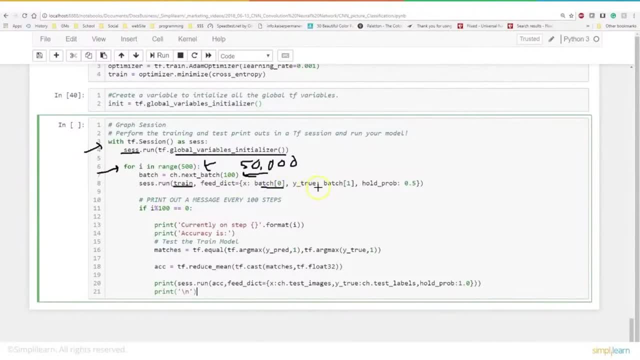 have x equals batch zero, coming in Y, true Batch one, Hold the probability 0.5.. And then, just so that we can keep track of what's going on, we're going to every 100 steps, we're going to run a. 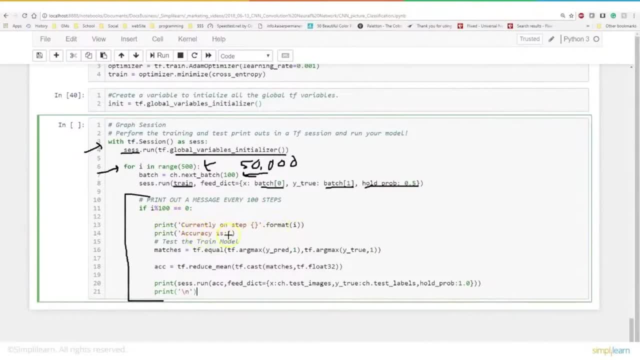 print. So currently on step format, accuracy is And we're going to look at matches equals tfequal max y true comma one. So we're going to look at this as how many matches it has And here our ACC. all we're doing here is we're going to take the matches, how many matches they have It creates. 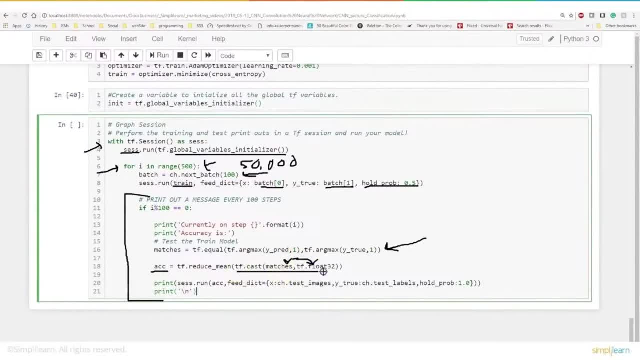 it generates a chart. We're going to convert that to float. That's what the tf cast does- And then we just want to know the average. We just want to know the average of the accuracy, And then we'll go ahead and print that out. Print session run accuracy feed dictionary. So it takes all this. 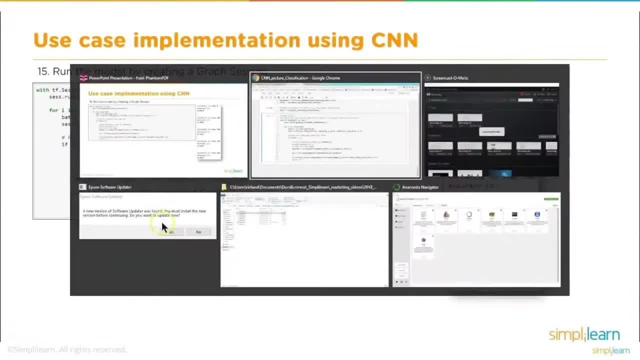 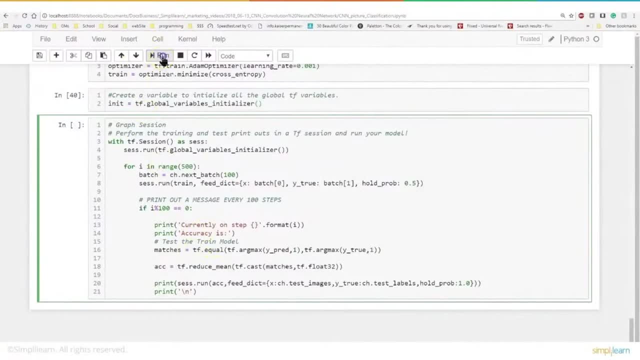 and it prints out our accuracy on there. So let's go ahead and take this. We're going to print out this. Oops screen's there. Let's go ahead and take this and let's run it. And this is going to take a little bit to run. So let's see what happens on my old laptop And we'll see here that. 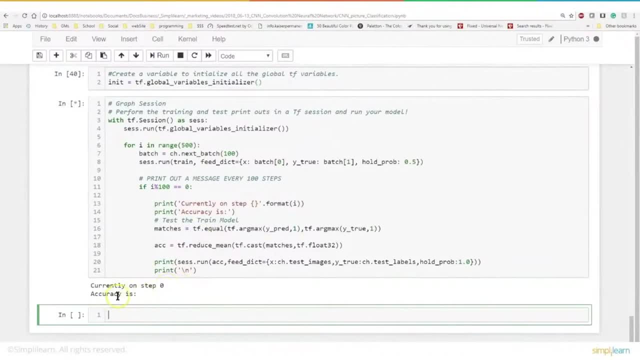 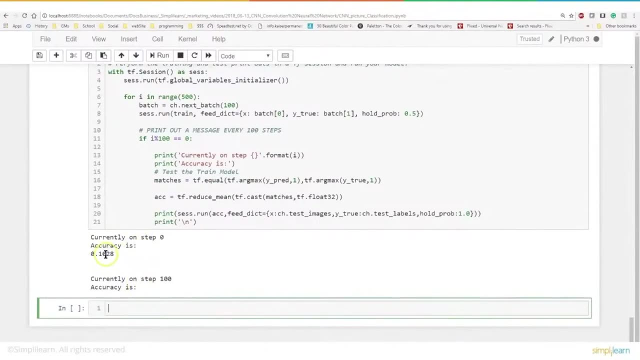 we have our current. we're currently on step zero. It takes a little bit to get through the accuracy And this will take just a moment to run. We can see that on our step zero it has an accuracy of 0.1 or 0.1028.. And as it's running, we'll go ahead. You don't need to watch it run all the. 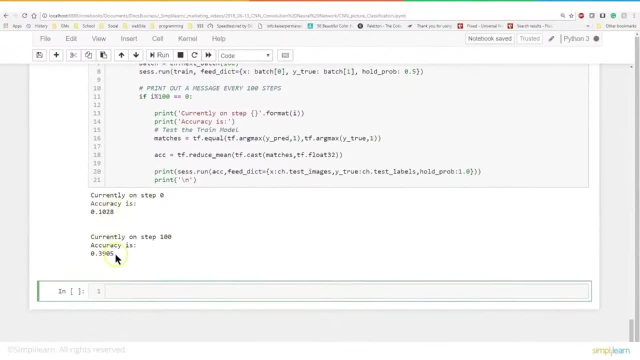 way, But this accuracy is going to change a little bit up and down, So we've actually lost some accuracy during our step two. But we'll see how that comes out. Let's come back after we run it all the way through and see how the different steps come out. I was actually reading: 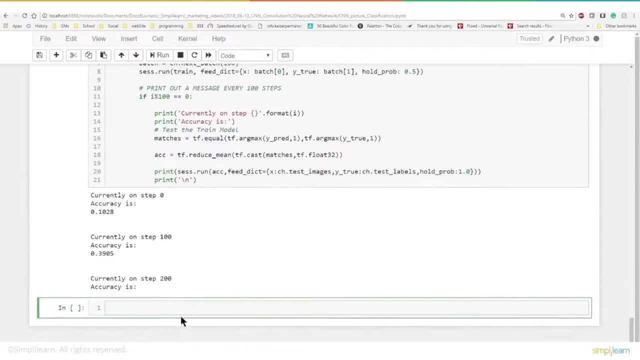 that backwards. The way this works is, the closer we get to one, the more accuracy we have. So you can see here we've gone from a 0.1 to a 0.39.. And we'll go ahead and pause this and come back and 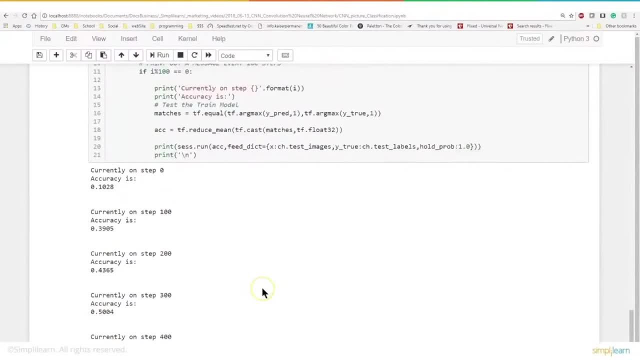 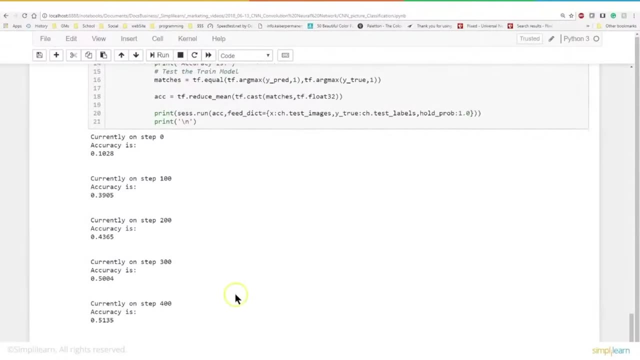 see what happens when we're done with the full run. All right, now that we've prepared the meal, got it in the oven and pulled out my finish dish here. if you've ever watched any of the old cooking shows, Let's discuss a little bit about. 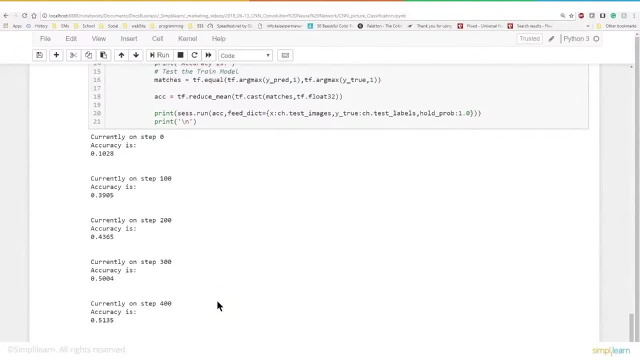 this accuracy going on here, And how do you interpret that? We've done a couple things. First, we've defined accuracy. The reason I got it backwards before is you have loss or accuracy, And with loss you'll get a graph that looks like this. It goes: oops, that's an S, by the way, There. 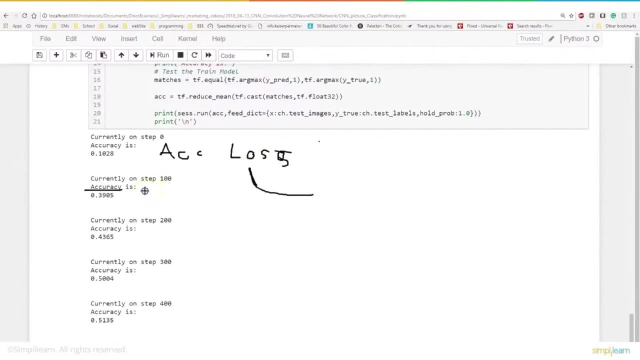 we go, You get a graph that curves down like this, And with accuracy, you get a graph that curves up. This is how good it's doing. Now, in this case, one is supposed to be really good. accuracy: That means it gets close to one, but it never crosses one. So if you have an accuracy of one, that is. 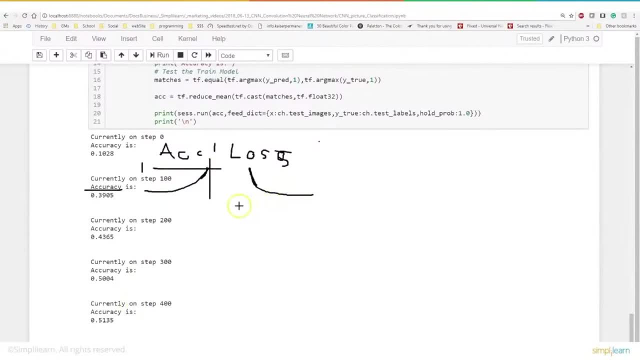 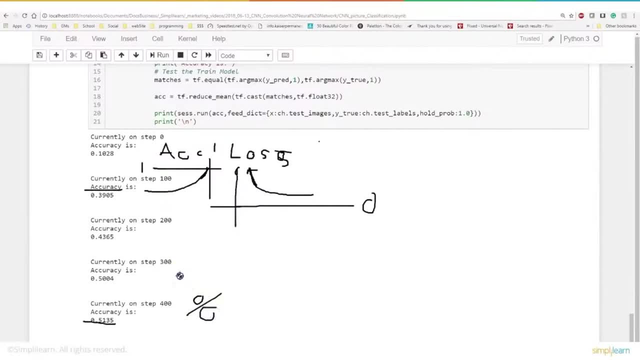 No, this is not percentage. Let me just put that in there. It is not percentage. This is logarithmic. What that means is that 0.2 is twice as good as 0.1. And when we see 0.4, that's twice as good. 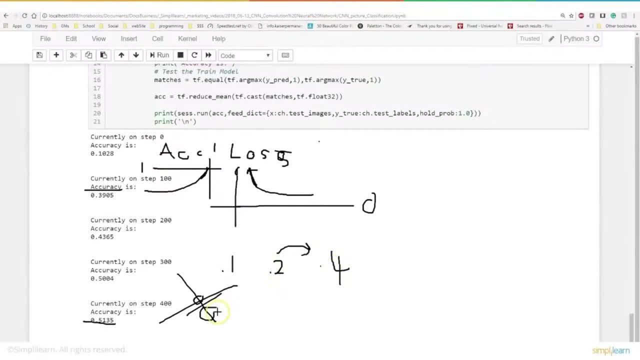 as 0.2.. Real way to convert this into a percentage. You really can't say this is a direct percentage conversion. What you can do, though, is in your head, if we were to give this a percentage, we might look at this as 50%- we're just guessing- equals 0.1., And if 50% roughly equals 0.1,. 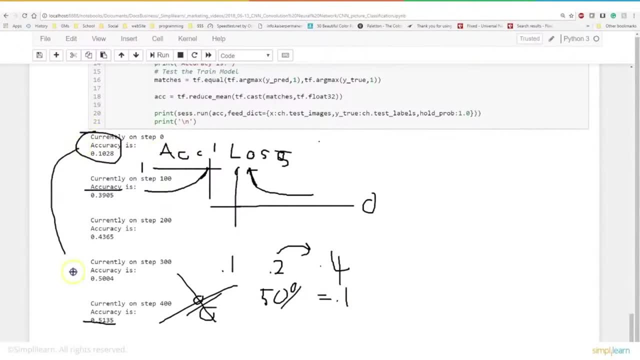 that's where we started up here at the top, Remember, at the top. here here's our 0.1028.. The accuracy of 50%, then 75% is about 0.2, and so on and so on. Don't quote those numbers. 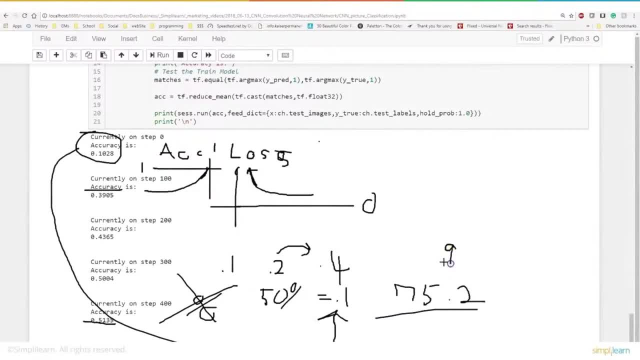 because that doesn't work that way. They say that if you have 0.95, that's pretty much saying 100%, And if you have 0.95, that's pretty much saying 100%, And if you have 0.95, that's pretty much saying 100%. 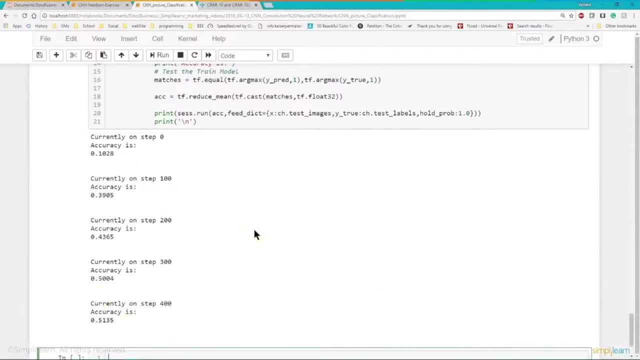 If you have anywhere between, you'd have to go look this up. Let me go ahead and remove all my drawings there. So the magic number is 0.5.. We really want to be over a 0.5 in this whole thing. 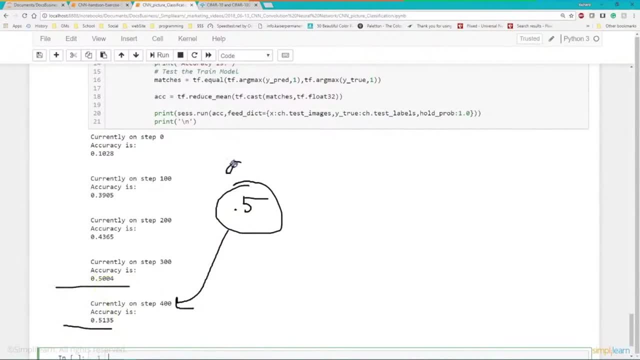 And we have both 0.5004.. Remember this is accuracy. If we were looking at loss then we'd be looking the other way. But 0.05, instead of how high it is, we want how low it is, But with. 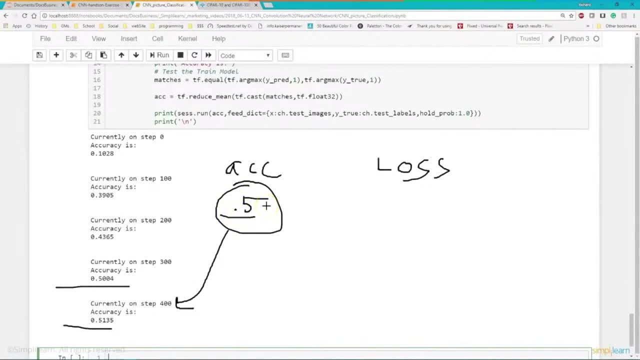 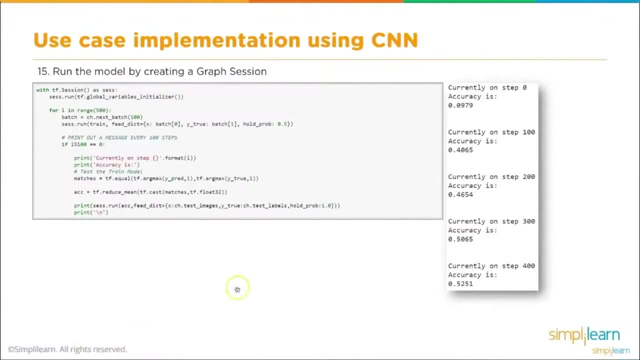 accuracy being over a 0.5 is pretty valid. That means this is pretty solid. And if you get to a 0.5, then it's a direct correlation. That's what we're looking for here. in these numbers And you can see, we finished with this model at 0.5135,, so still good. And if we look at when, 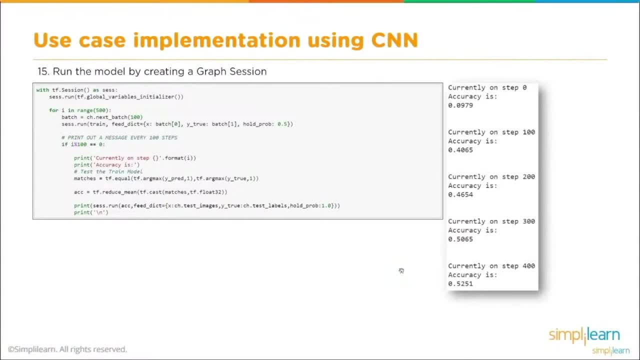 they ran this in the other end. remember there's a lot of randomness that goes into it. when we seed the weights, They got 0.5251, so a little better than ours, But that's fine. You'll find your own comes up a little bit better or worse depending on just that randomness. And so we've. 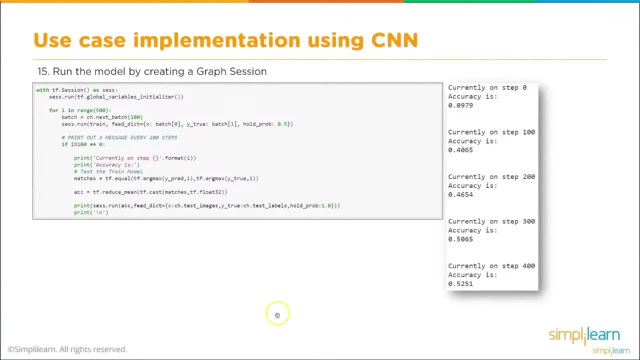 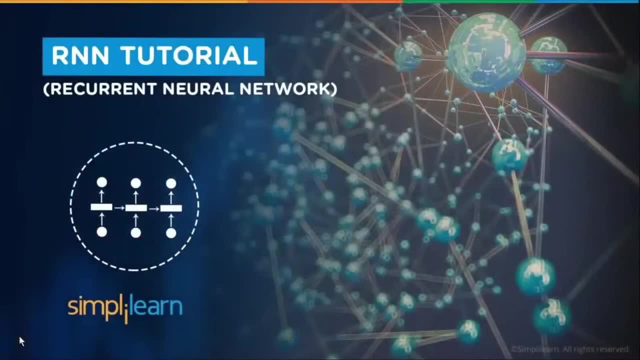 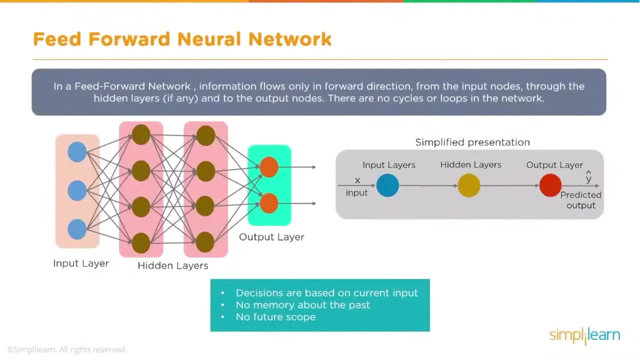 gone through the whole model We've created, we've trained the model and we've also gone through on the 100th run to test the model to see how accurate it is. Welcome to the RNN tutorial. That's the Recurrent Neural Network. So we talk about a feed-forward neural network In a feed-forward. 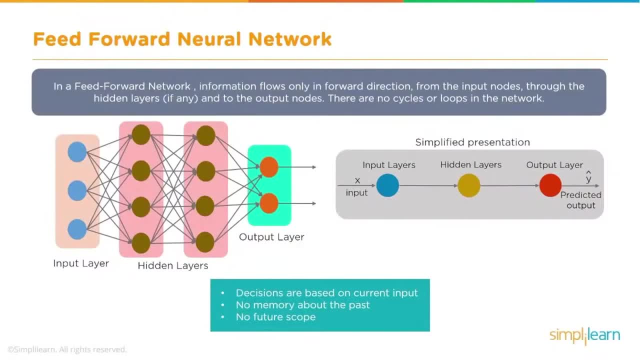 neural network, information flows only in the forward direction, from the input nodes through the hidden layers, if any, and to the output nodes. There are no cycles or loops in the network, And so you can see, here we have our input layer. I was talking about how it just goes straight forward. 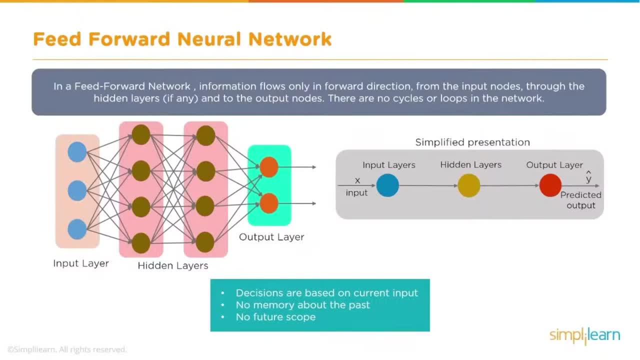 into the hidden layers, So each one of those connects and then connects to the next hidden output layer And of course we have a nice simplified version where it has a predicted output and they refer to the input as x a lot of times and the output as y. Decisions are based on current. 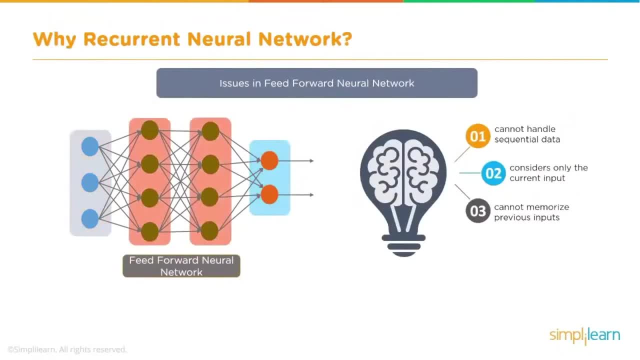 input, no memory about the past, no future scope. Why Recurrent Neural Network Issues in feed-forward neural network? So one of the biggest issues is because it doesn't have a scope of memory or time. a feed-forward neural network doesn't know how to handle sequential data. It only considers only the current input. So if you have an input that's out of sequence and you're not able to compute, you're simply going to have to go through the data, look through the data, look through the data and then look through the data. So if you have a 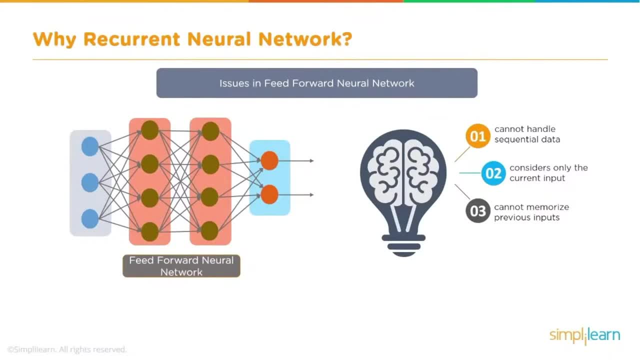 input that's out of sequence. do not concern about anything that you need to do. you don't let it do anything from the. So if you have a series of things, and because three points back affects what's happening now and what's your output affects what's happening, that's very important. 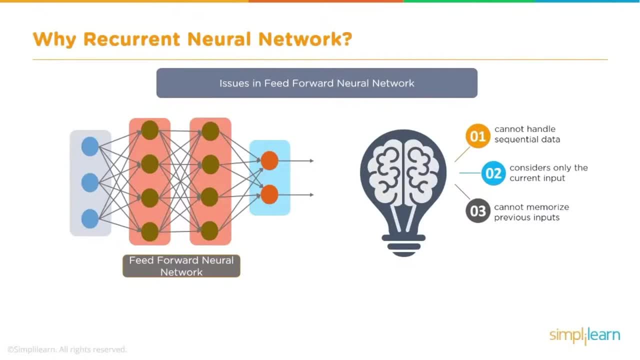 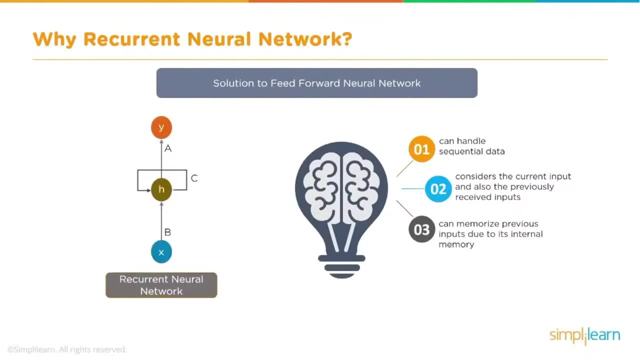 So whatever I put as an output is going to affect the next one. A feed forward doesn't look at any of that. It just looks at this is what's coming in And it cannot memorize previous inputs. So it doesn't have that list of inputs coming in. 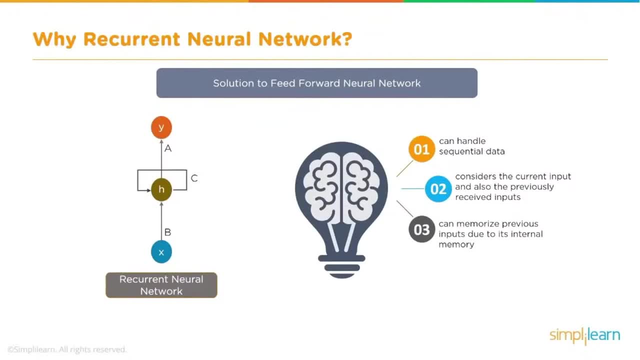 Solution to feed forward neural network. You'll see here where it says recurrent neural network and we have our X on the bottom, going to H, going to Y. That's your feed forward, But right in the middle it has a value C. 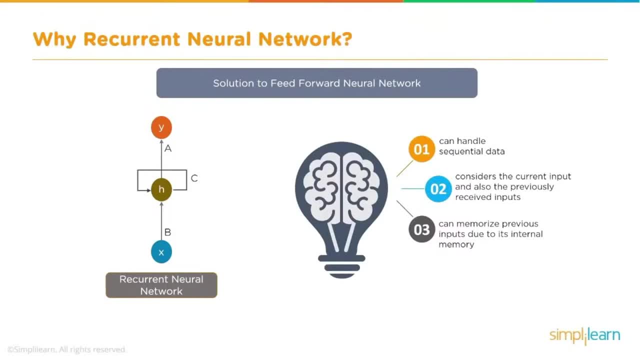 So there's a whole other process of memorizing what's going on in the hidden layers, And the hidden layers, as they produce data, feed into the next one. So your hidden layer might have an output that goes off to Y, but that output goes back into the next prediction coming in. 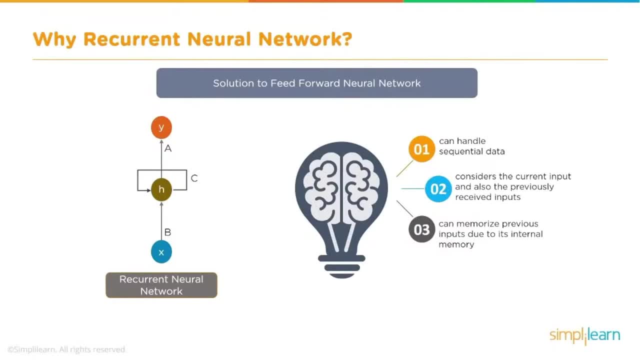 What this does is. this allows it to handle sequential data. It considers the current input and also the previously received inputs, And if we're going to look at general drawings and solutions, we should also look at applications of the RNN. Image captioning. 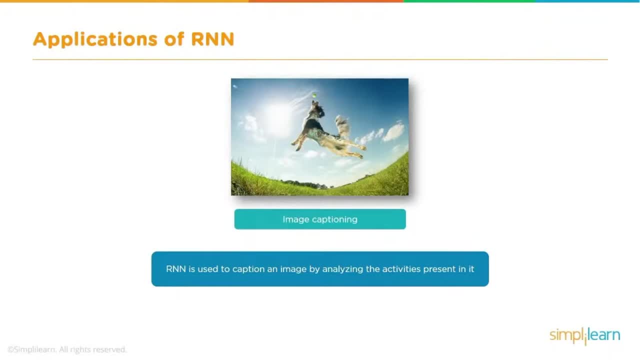 RNN is used to caption an image by analyzing the activities present in it. A dog catching a ball in midair. That's very tough. I mean, we have a lot of stuff that analyzes images of a dog and the image of a ball. 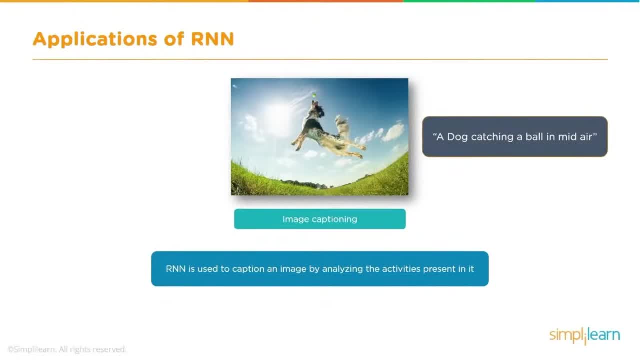 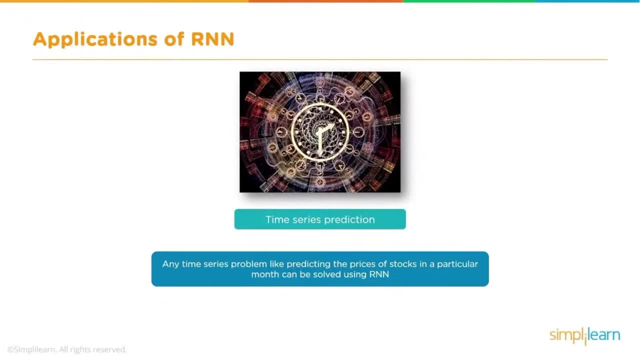 but it's able to add one more feature in there. that's actually catching the ball in midair: Time series prediction. Any time series problem, like predicting the prices of stocks in a particular month, can be solved using RNN And we'll dive into that. 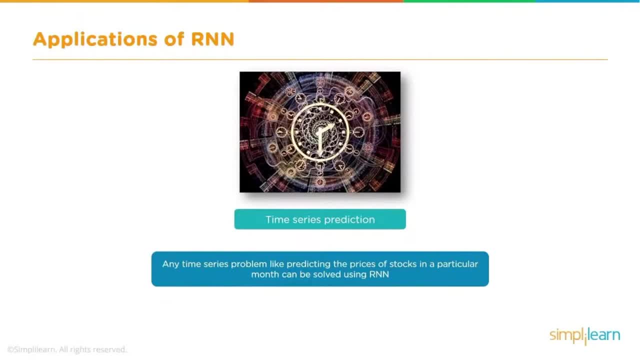 In our use case and actually take a look at some stock. One of the things you should know about analyzing stock today is that it is very difficult And if you're analyzing the whole stock, the stock market at the New York Stock Exchange in the US produces somewhere in the neighborhood. If you count all the individual trades and fluctuations by the second, it's like three terabytes a day of data. So we're going to look at one stock. Just analyzing one stock is really tricky. In here we'll give you a little jump on that. 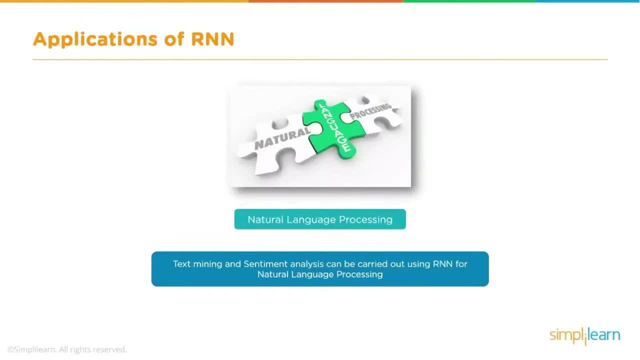 So that's exciting, But don't expect that, Don't expect to get rich off of it immediately. Another application of the RNN is natural language processing. Text mining and sentiment analysis can be carried out using RNN for natural language processing, And you can see right here the term natural language processing, when you stream those three words together, is very different than, if I said, processing language naturally. 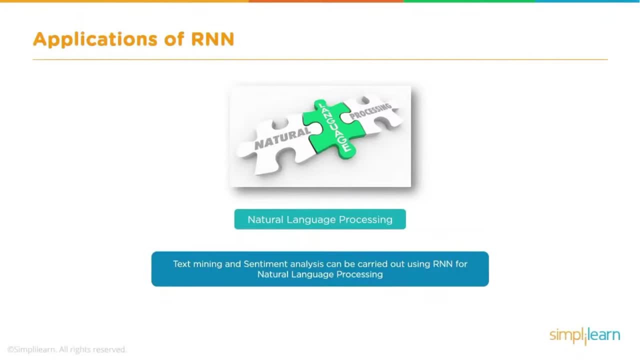 So the time series is very important when we're analyzing sentiments. It can change the whole value of a sentence just by switching the words around. Or if you're just counting the words, you may get one sentiment Where, if you actually look at the order, they're in. 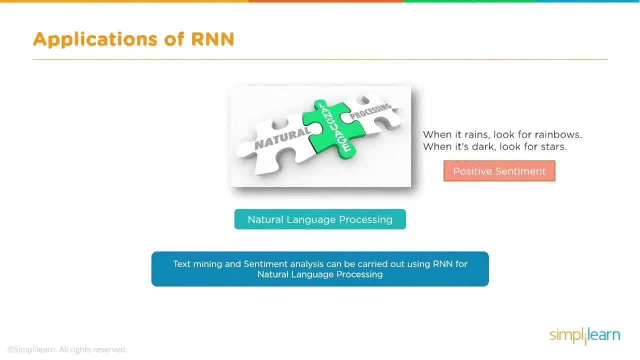 you get a completely different sentiment. When it rains, look for rainbows. When it's dark, look for stars. Both of these are positive sentiments And they're based upon the order of which the sentence is going in Machine translation, Given an input in one language. 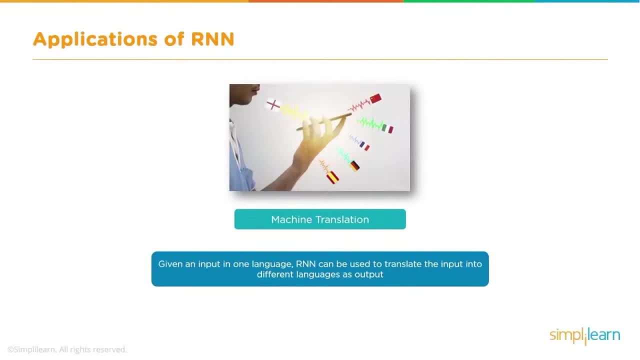 RNN can be used to translate the input into a different languages as output. I myself am very linguistically challenged, But if you study languages- and you're good with languages- you know right away that if you're speaking English you would say: 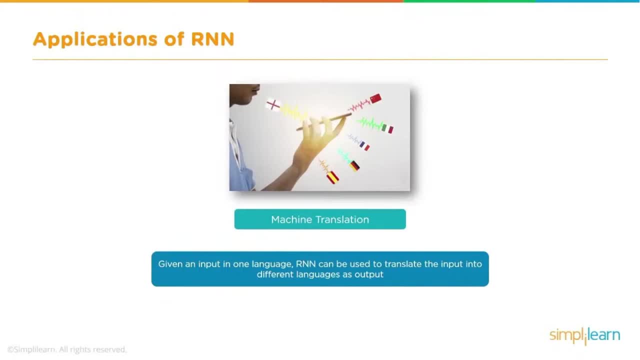 big cat And if you're speaking Spanish you would say cat big. So that translation is really important to get the right order to get. There's all kinds of parts of speech that are important to know by the order of the words. 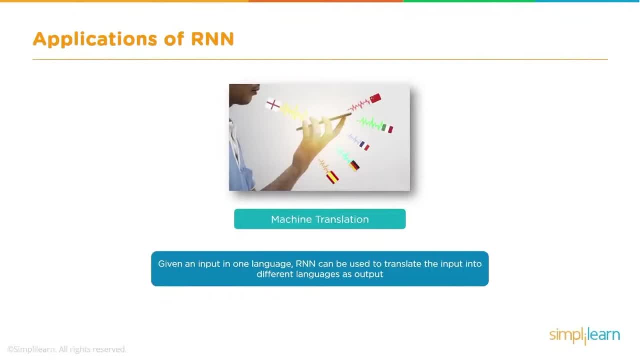 Here this person is speaking in English and getting translated, And you can see here a person is speaking in English in this little diagram. I guess that's denoted by the flags. I have a flag, I own it, No, But they're speaking in English and it's getting translated into Chinese. 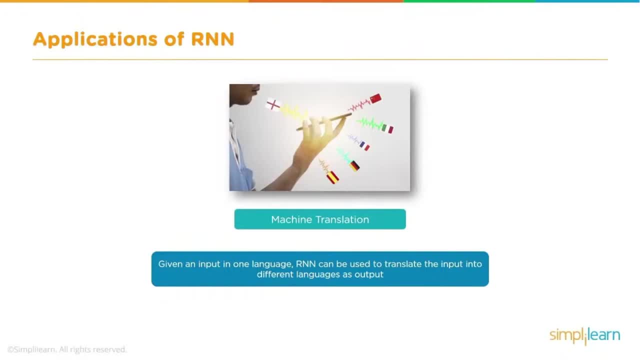 Italian, French, German and Spanish languages. Some of the tools coming out are just so cool. So somebody like myself, who's very linguistically challenged, I can now travel into worlds I would never think of, because I can have something translate my English back and forth readily. 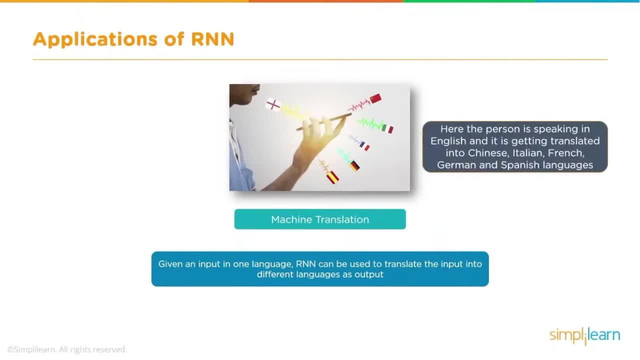 And I'm not stuck with a communication gap. So let's dive into what is a recurrent neural network. Recurrent neural network works on the principle of saving the output of a layer and feeding this back to the input in order to predict the output of the layer. 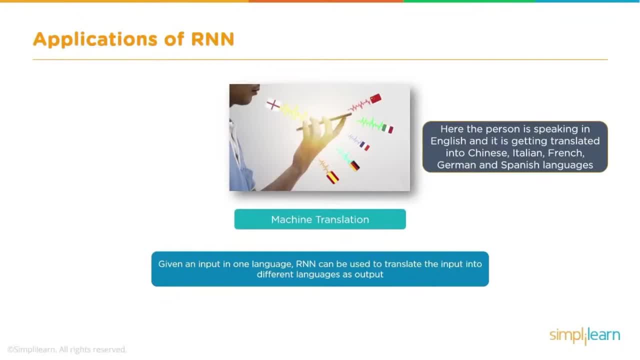 Sounds a little confusing, but when we start breaking it down it'll make more sense And usually we have a propagation forward neural network with the input layers, the hidden layers, the output layer. With the recurrent neural network we turn that on its side. 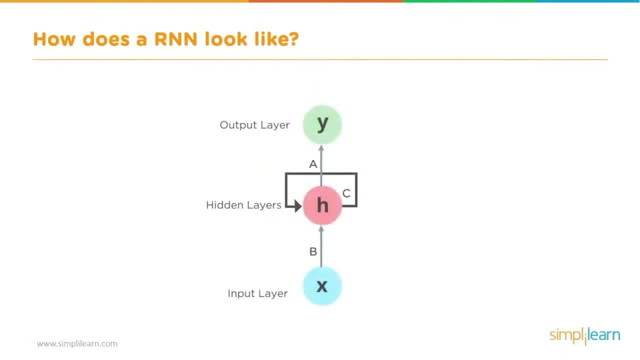 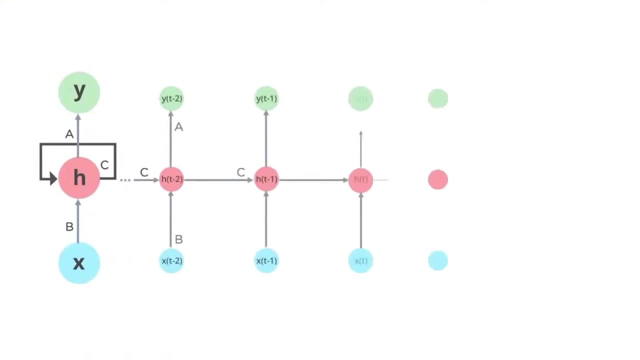 So here it is, And now our X comes up from the bottom, into the hidden layers, into Y, And they usually draw it very simplified: X to H with C as a loop, A to Y, where A, B and C are the perimeters. 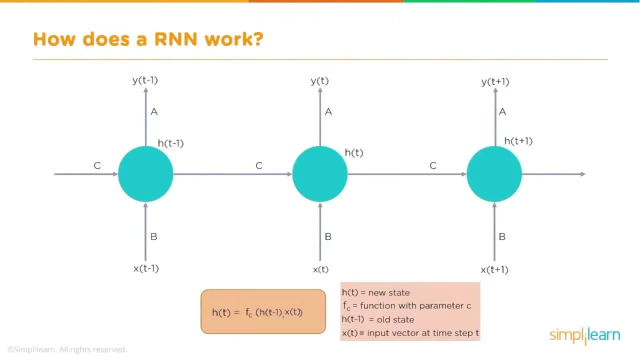 A lot of times you'll see this kind of drawing in here, digging closer and closer into the H and how it works, Going from left to right. you'll see that the C goes in and then the X goes in. So the X is going upward bound and C is going to the right. 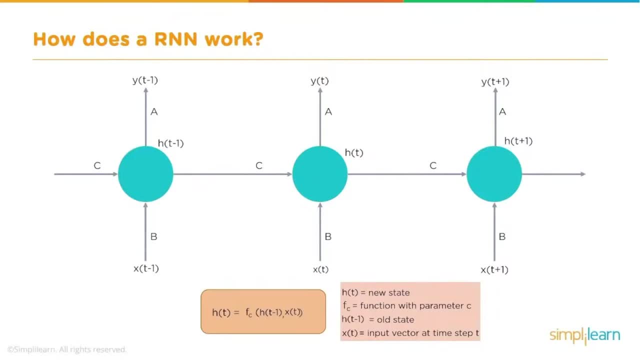 A is going out and C is also going out. That's where it gets a little confusing. So here we have X in, C in, and then we have Y out and C out, and C is based on HT minus one. So our value is based on. the Y and the H value are connected to each other. 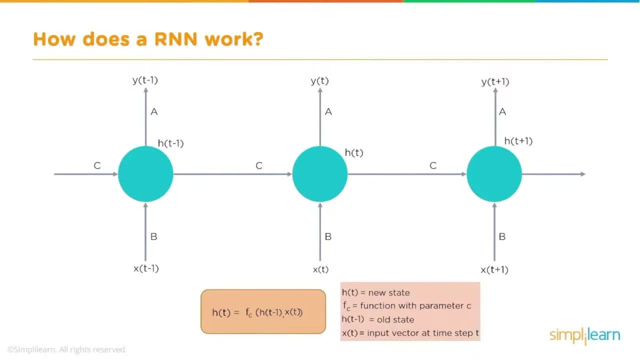 They're not necessarily the same value, because H can be its own thing And usually we draw this or we represent it as a function. H of T equals a function of C, where H of T minus one, that's the last H output and X of T going in. 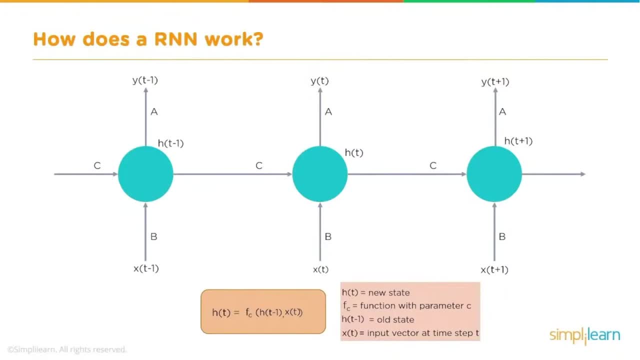 So it's the last output of H combined with the new input of X, where HT is the new state. FC is a function with the parameter C, That's a common way of denoting it. HT minus one is the old state coming out, and then X of T is an input vector at time of step T. 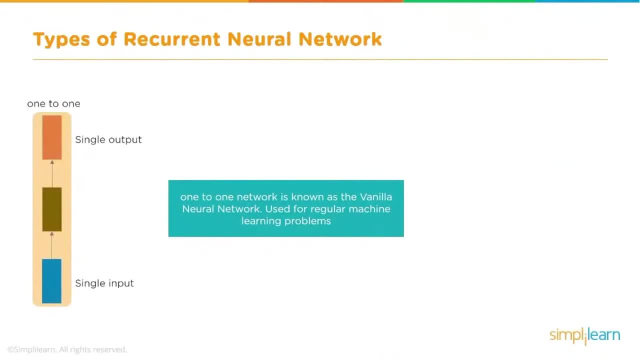 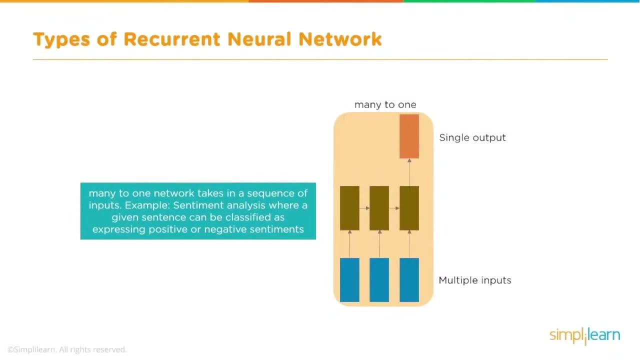 Well, we need to cover types of recurrent neural networks, And so the first one is the most common one, which is a one to one single output. One to one neural network is usually known as a vanilla neural network, used for regular machine learning problems. 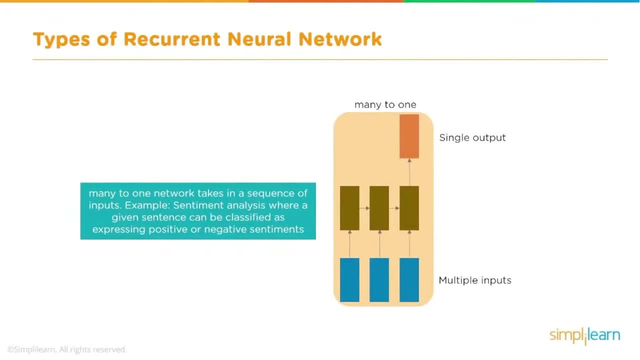 Why? Because vanilla is usually considered kind of a just a real basic flavor, But because it's very basic a lot of times they'll call it the vanilla neural network, which is not the common term but it is kind of a slang term. 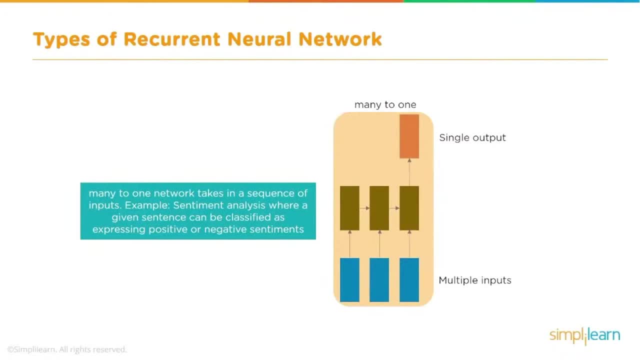 People will know what you're talking about. usually, if you say that, Then we run one to many, So you have a single input and you might have a multiple outputs- in this case, image captioning, as we looked at earlier, where we have not just looking at it as a dog. 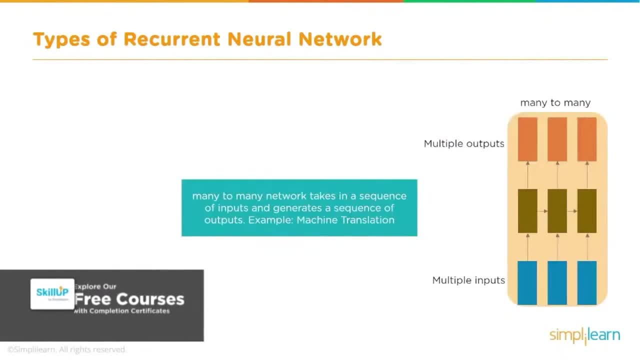 but a dog catching a ball in the air, And then you have many to one. network takes in a sequence of inputs. Examples: sentiment analysis, where a given sentence can be classified as expressing positive or negative sentiments, And we looked at that as we were discussing if it rains. 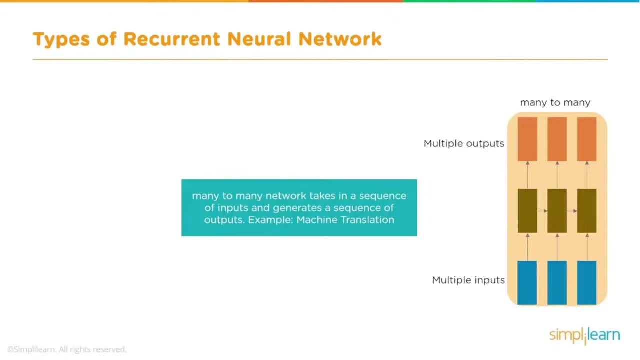 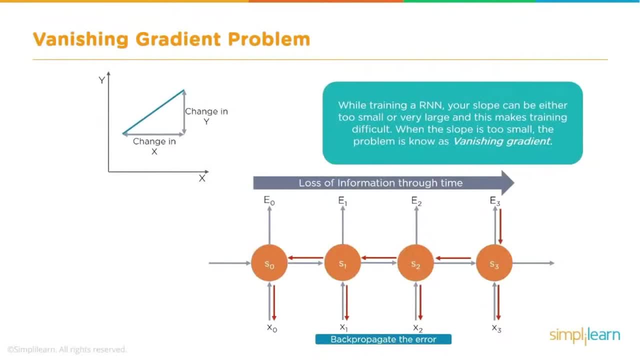 And then, of course, if you're going to do a one to one, many to one, one to many, there's many to many networks- takes in a sequence of inputs and generates a sequence of outputs. Example: machine translation. So we have a lengthy sentence coming in in English and then going out in all the different languages. 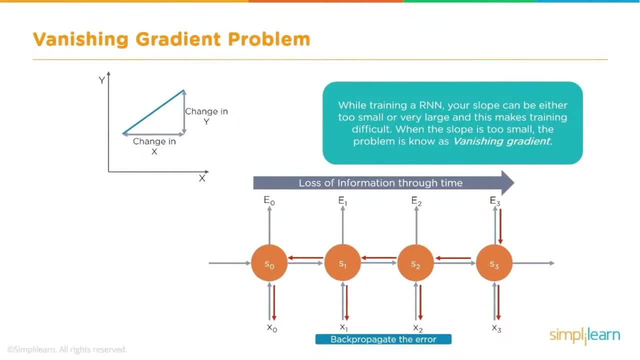 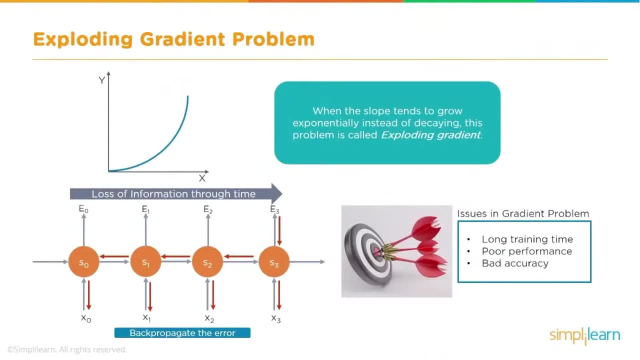 You know just a wonderful tool, very complicated set of computations. You know, if you're a translator, you realize just how difficult it is to translate into different languages. One of the biggest things you need to understand when we're working with this neural network. 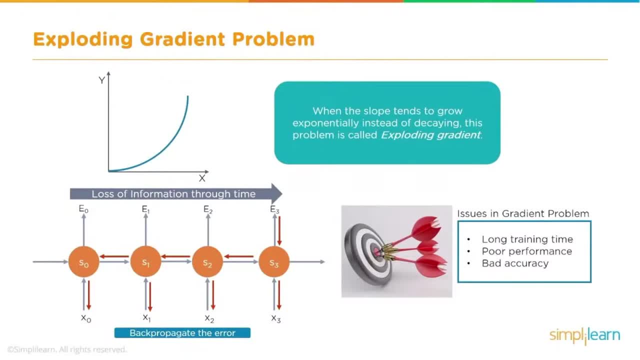 is what's called the vanishing gradient problem. While training an RNN, your slope can be either too small or very large, And this makes training difficult. When the slope is too small, the problem is known as vanishing gradient, And you'll see here. 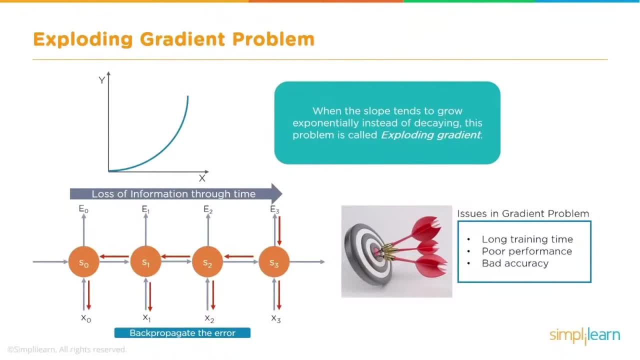 they have a nice image: loss of information through time. So if you're pushing not enough information forward, that information is lost, And then when you go to train it you start losing the third word in the sentence or something like that, or it doesn't quite follow the full logic. 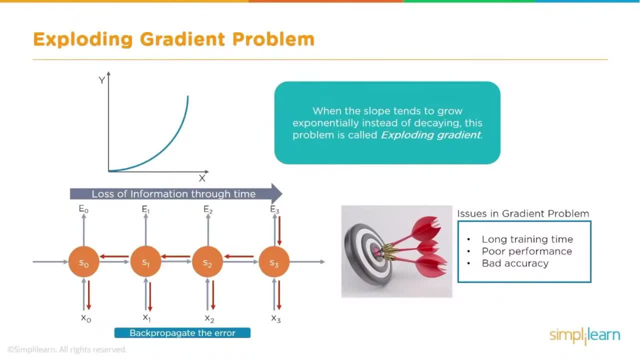 of what you're working on. Exploding gradient problem. Oh, this is one that runs into everybody. When you're working with this particular neural network, when the slope tends to grow exponentially instead of decaying, this problem is called exploding gradient. 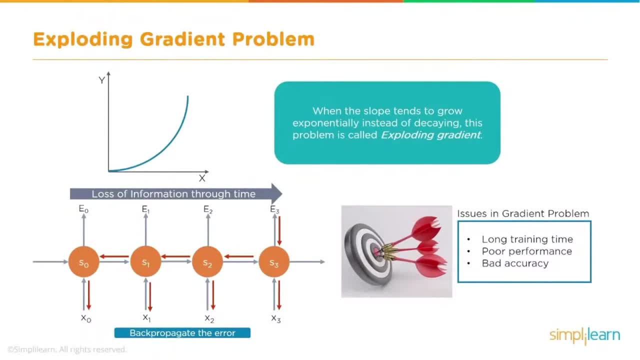 Issues in gradient problem: long training time, poor performance, bad accuracy. And I'll add one more in there: Your computer. if you're on a lower end computer testing out a model will lock up and give you the memory error Exploding gradient problem. 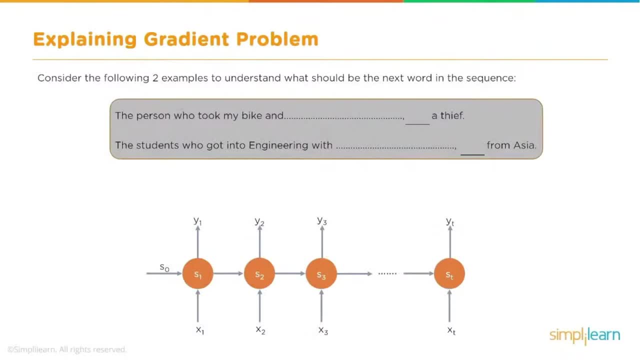 Consider the following Two examples to understand what should be the next word in the sequence: The person who took my bike and blank A thief, The students who got into engineering with blank from Asia, And you can see, in here we have our X value going in. 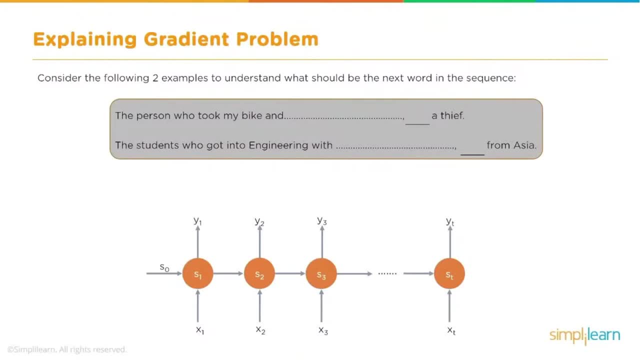 We have the previous value going forward And then you back, propagate the error, like you do with any neural network, And as we're looking for that missing word, maybe we'll have. the person took my bike and blank was a thief And the student who got into engineering with a blank were from Asia. 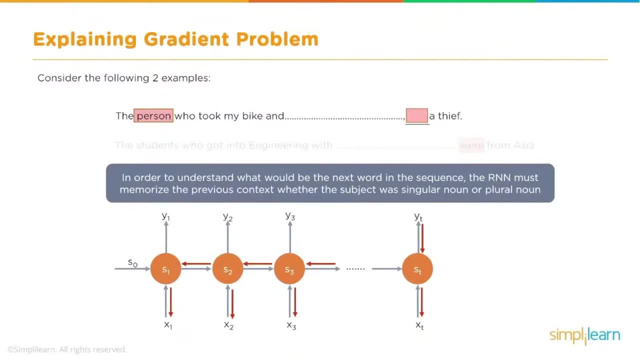 Consider the following example: The person who took the bike- So we'll go back to the person who took the bike- was blank a thief. In order to understand what would be the next word in the sequence, the RNN must memorize the previous context. 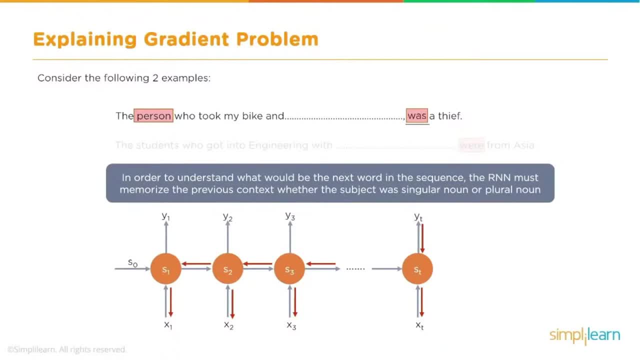 whether the subject was singular noun or a plural noun, So was a thief is singular The student who got into engineering. Well, in order to understand what would be the next word in the sequence, the RNN must memorize the previous context. 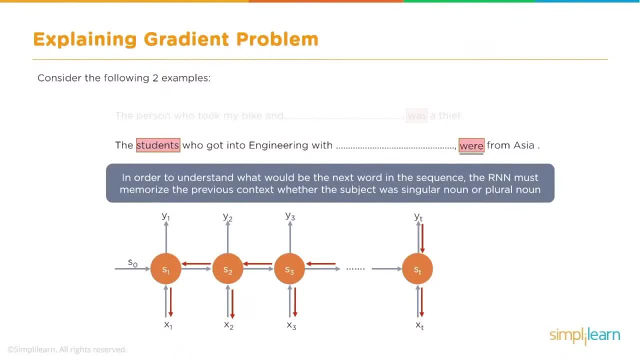 whether the subject was singular noun or a plural noun, And so you can see here, the students who got into engineering with blank were from Asia. It might be sometimes difficult for the error to back propagate to the beginning of the sequence, to predict what should be the output. 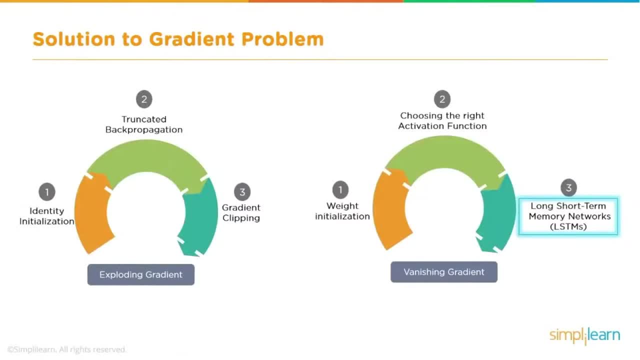 So when you run into the gradient problem, we need a solution. The solution to the gradient problem. First we're going to look at exploding gradient, where we have three different solutions, depending on what's going on. One is identity initialization. 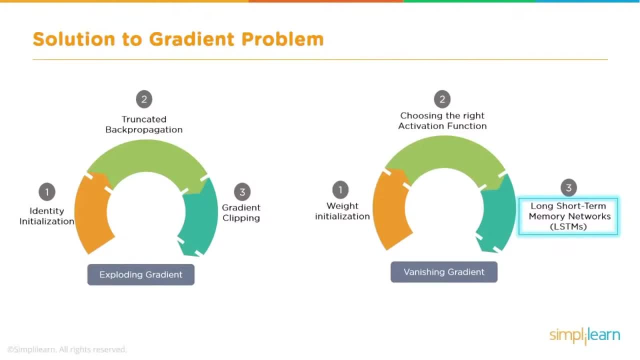 So the first thing we want to do is see if we can find a way to minimize the identities that are coming in, instead of having it identify everything just the important information. we're looking at Next is to truncate the back propagation. So, instead of having whatever information, it's sending to the next series. 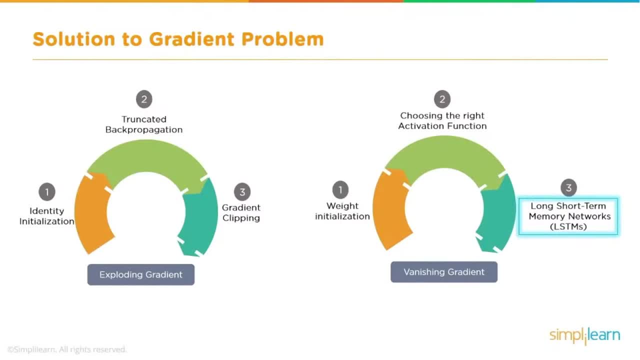 we can truncate what it's sending. We can lower that particular set of layers, make those smaller And finally is a gradient clipping. So when we're training it, we can clip what that gradient looks like and narrow the training model that we're using. 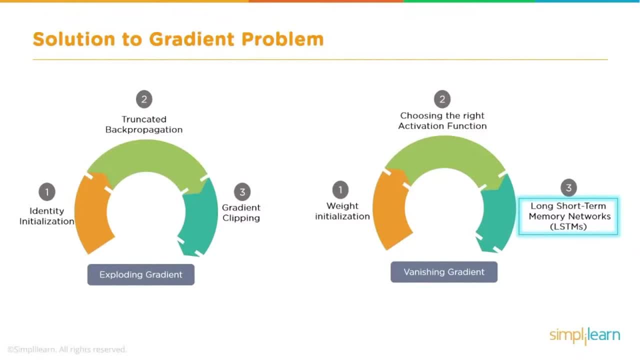 When you have a vanishing gradient, the option problem. we can take a look at weight initialization. Very similar to the identity, but we're going to add more weights in there so it can identify different aspects of what's coming in better. 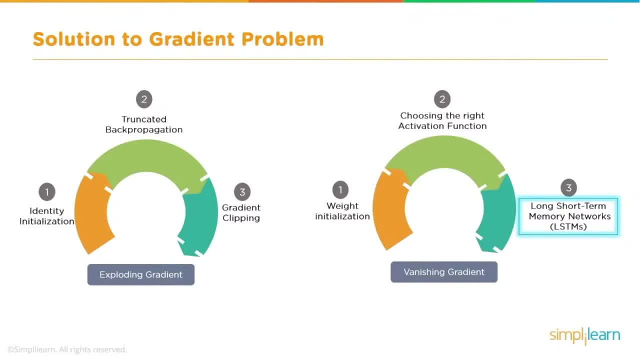 Choosing the right activation function. That's huge. So we might be activating based on one thing and we need to limit that. We haven't talked too much about activation functions, so we'll look at that just minimally. There's a lot of choices out there. 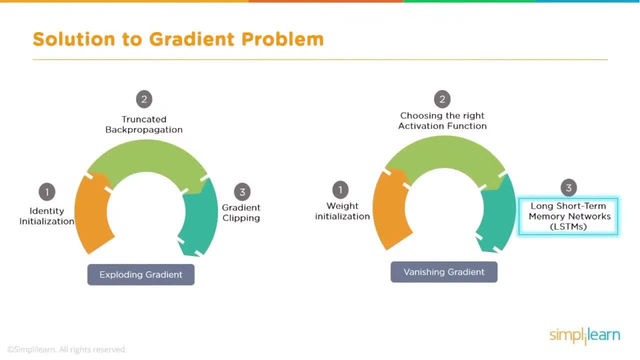 And then, finally, there's long short-term memory networks, the LSTMS. We can make adjustments to that. So, just like we did, just like we can clip the gradient as it comes out, we can also expand on that. We can increase the memory network, the size of it. 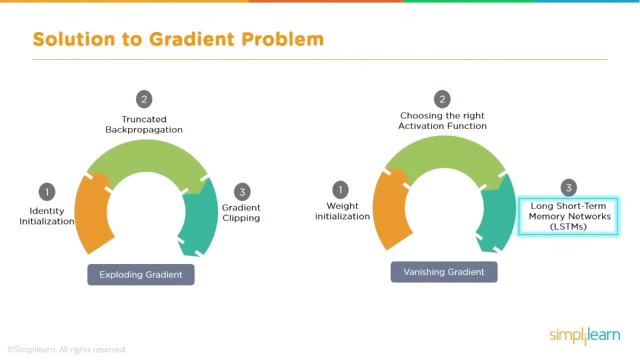 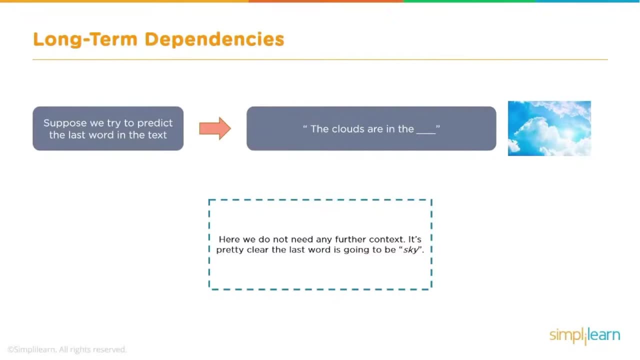 so it handles more information, And one of the most common problems in today's setup is what they call long-term dependencies. Suppose we try to predict the last word in the text, The clouds are in the- and you probably said sky Here. we do not need any further context. 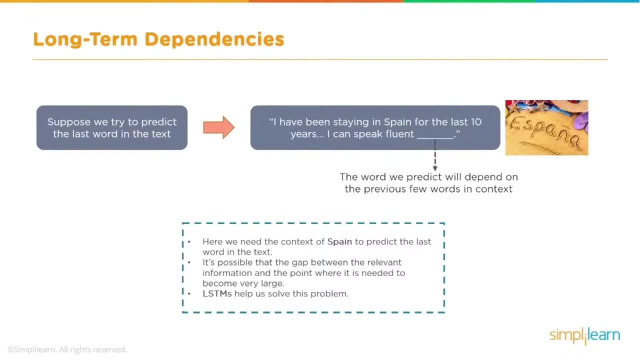 It's pretty clear that the last word is going to be sky. Suppose we try to predict the last word in the text. I have been staying in Spain for the last 10 years. I can speak fluent. Maybe you said Portuguese or French. 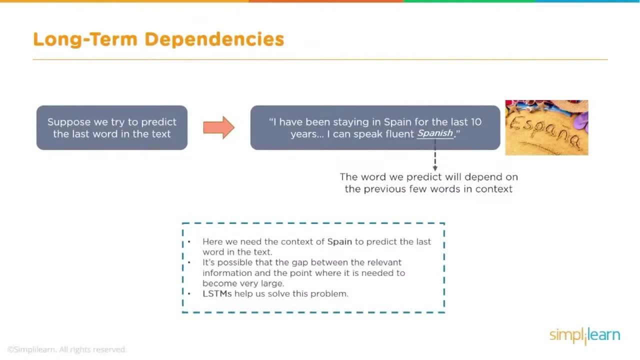 No, you probably said Spanish. The word we predict will depend on the previous few words in context. Here we need the context of Spain to predict the last word in the text. It's possible that the gap between the relevant information and the point where it is needed to become very large. 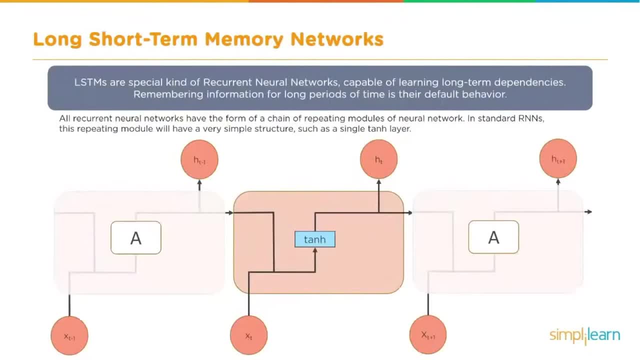 LSTMs help us solve this problem. So the LSTMS are a special kind of recurrent neural network capable of doing this, Capable of learning long-term dependencies. Remembering information for long periods of time is their default behavior. All recurrent neural networks have the form of a chain of repeating modules. 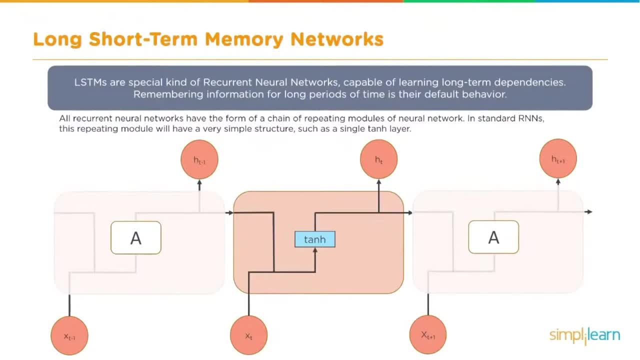 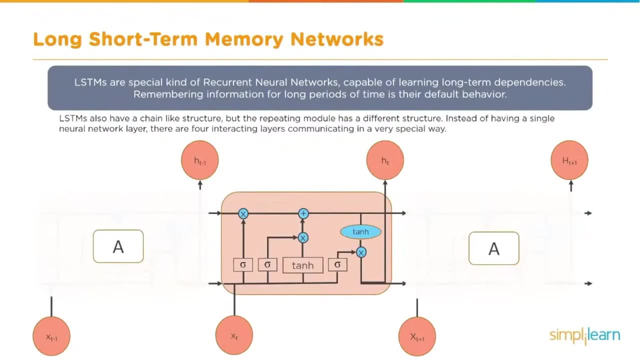 of neural network connections In standard RNNs. this repeating module will have a very simple structure, such as a single tangent H layer. LSTMSs also have a chain-like structure, but the repeating module has a different structure Instead of having a single neural network layer. 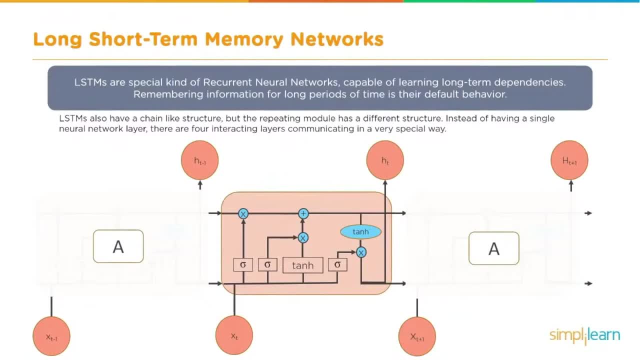 there are four interacting layers communicating in a very special way. LSTMSs are a special kind of recurrent neural network capable of learning long-term dependencies. Remembering information for long periods of time is their default behavior. LSTMSs also have a chain-like structure. 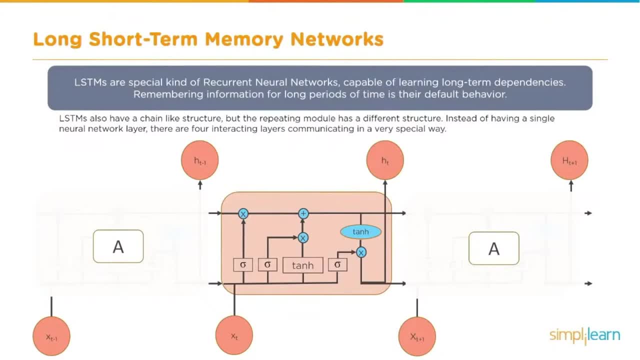 but the repeating module has a different structure. Instead of having a single neural network layer, there are four interacting layers communicating in a very special way. As you can see, the deeper we dig into this, the more complicated the graphs get In here. I want you to note that you have to be careful. 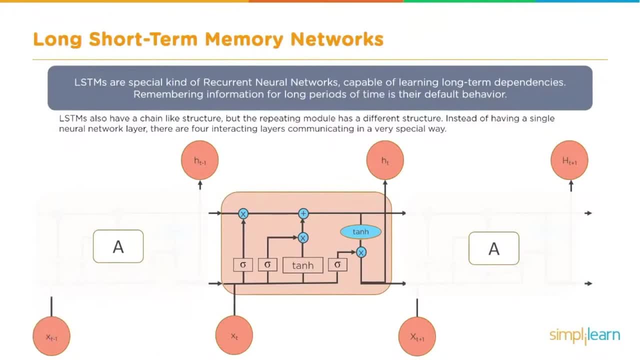 that you have x at t minus 1 coming in. you have x at t coming in and you have x at t plus 1.. And you have h at t minus 1, and h at t coming in and h at t plus 1 going out. 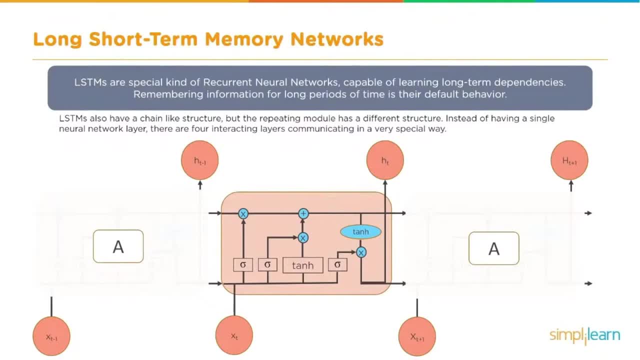 and of course, on the other side is the output A. In the middle we have our tangent H, but it occurs in two different places. So not only when we're computing the x at t plus 1 are we getting the tangent H from x at t. 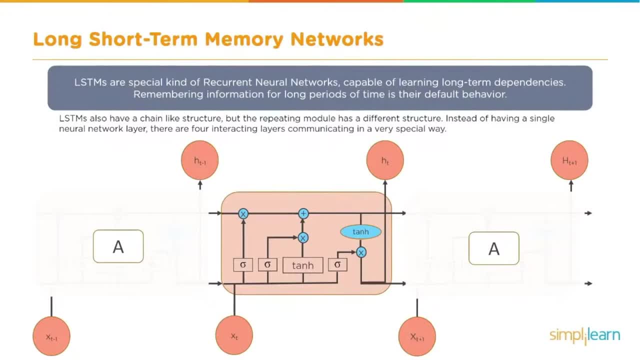 but we're also getting that value coming in from the x at t minus 1.. So the short of it is: as you look at these layers, not only does the propagate through the first layer goes into the second layer, back into itself, but it's also going into the third layer. 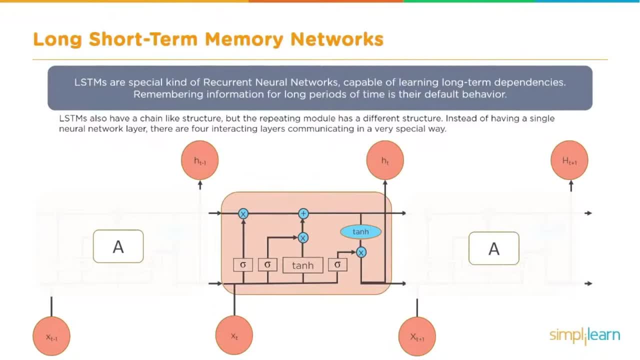 So now we're kind of stacking those up And this can get very complicated. as you grow that in size, It also grows in memory too and in the amount of resources it takes, But it's a very powerful tool to help us address the problem. 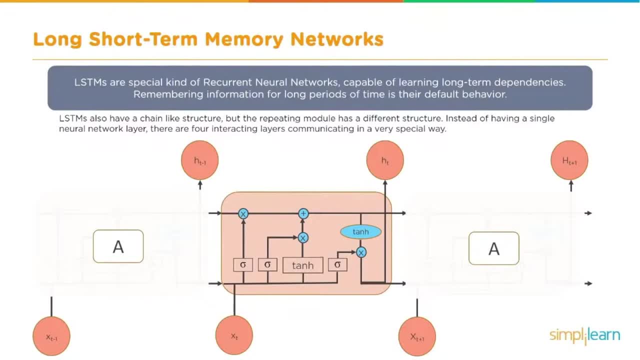 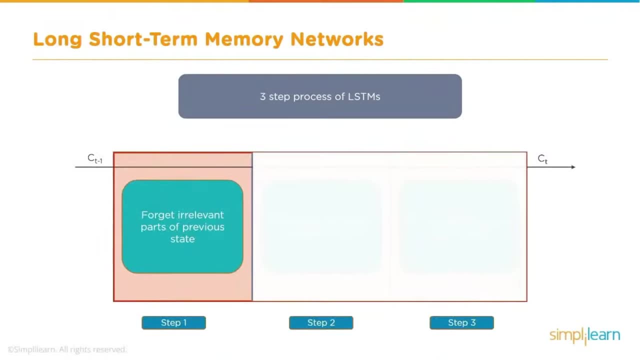 of complicated, long sequential information coming in, like we were just looking at in the sentence And when we're looking at our long short-term memory network. there's three steps of processing in the LSTMS that we look at. The first one is we want to forget irrelevant parts of the previous state. 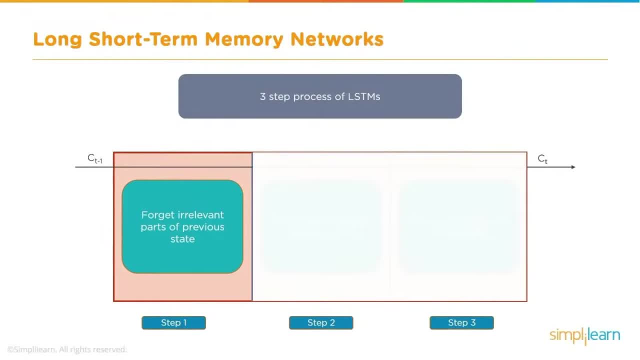 You know, a lot of times, like you know, is as in a, unless we're trying to look at whether it's a plural noun or not, they don't really play a huge part in the language, So we want to get rid of them. 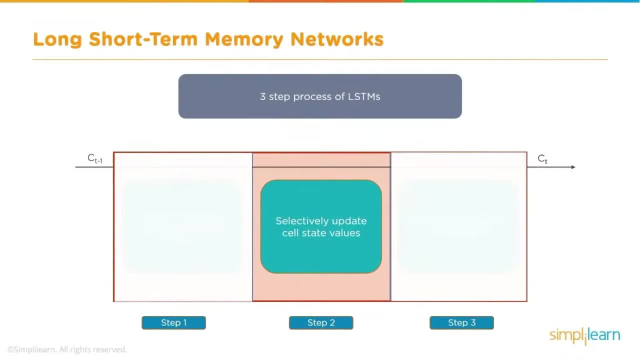 Then selectively update cell state values. So we only want to update the cell state values that reflect what we're working on. And finally, we want to put only output certain parts of the cell state. So whatever's coming out, we want to limit what's going out too. 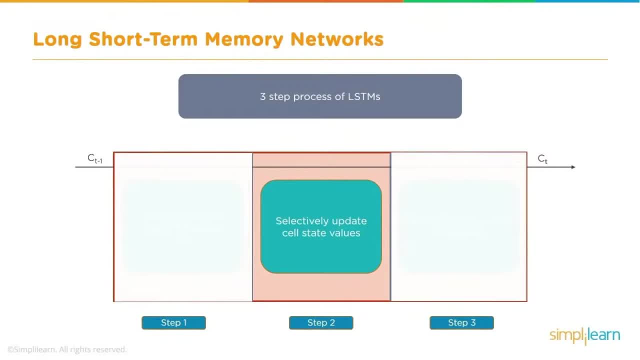 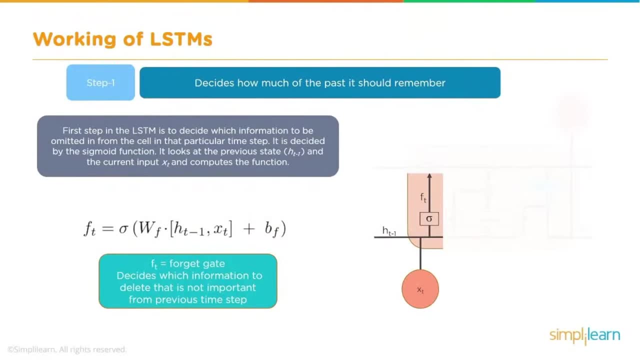 And let's dig a little deeper into this. Let's just see what this really looks like. So step one decides how much of the past it should remember. First step in the LSTM is to decide which information to be omitted in from the cell in that particular time step. 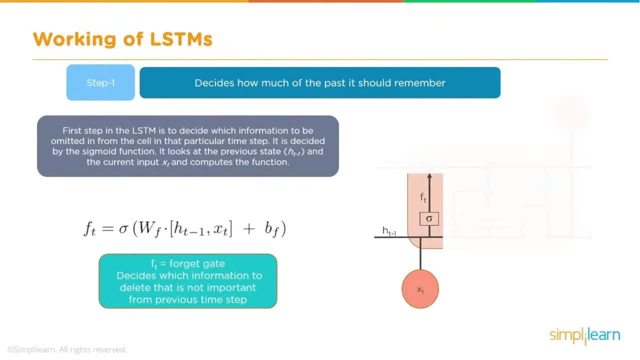 It is decided by the sigmoid function. It looks at the previous state h of t minus 1, and the current input x of t and computes the function. So you can see over here we have a function of t equals the sigmoid function of the weight of f. 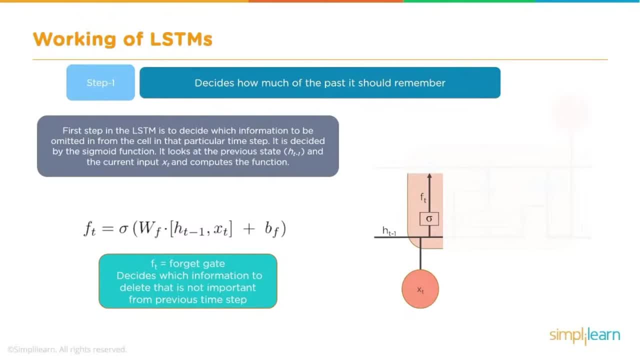 the h at t minus 1, and then x of t plus. of course you have a bias in there with any of your neural networks, so we have a bias function. So f of t equals forget. gate Decides which information to delete. 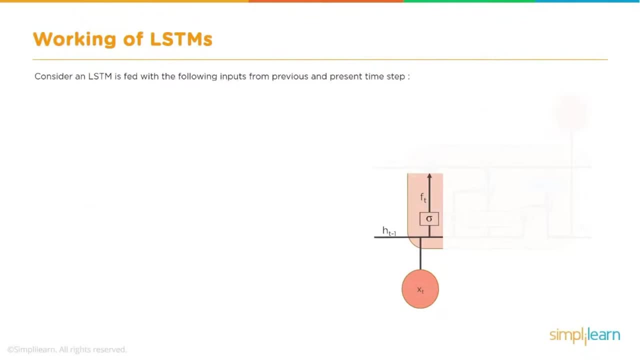 that is not important- from the previous time step. Considering an LSTM is fed with the following inputs: from the previous and present time step: Alice is good in physics. John, on the other hand, is good in math. John, on the other hand, is good in chemistry. 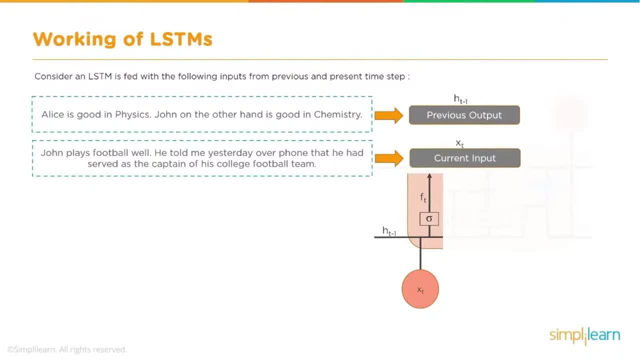 So previous output: John plays football. well, He told me yesterday over the phone that he had served as a captain of his college football team. That's our current input. So, as we look at this, the first step is the forget gate. 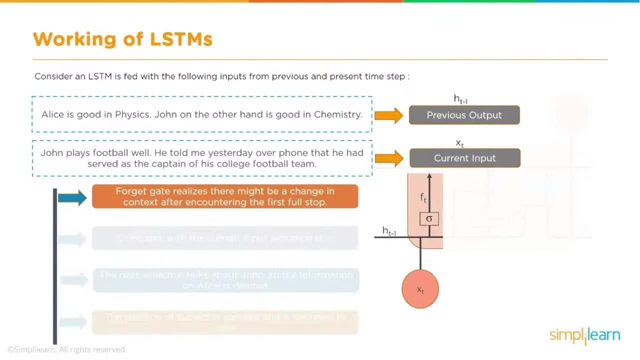 realizes there might be a change in context after encountering the first full stop, Compares with the current input sentence of x of t- So we're looking at that full stop- and then compares it with the input of the new sentence. The next sentence talks about John. 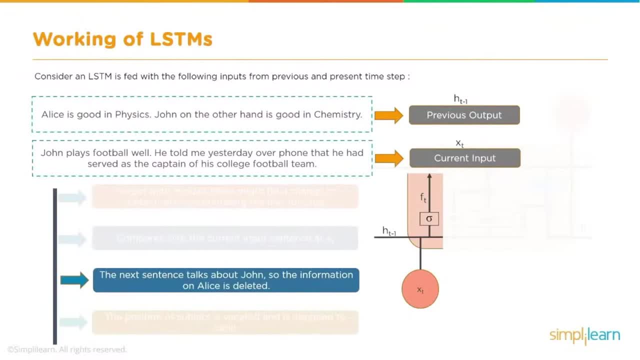 so the information on Alice is deleted. Okay, that's important to know. So we have this input coming in and if we're going to continue on with John, then that's going to be the primary information we're looking at. The position of the subject is vacated and is assigned to John. 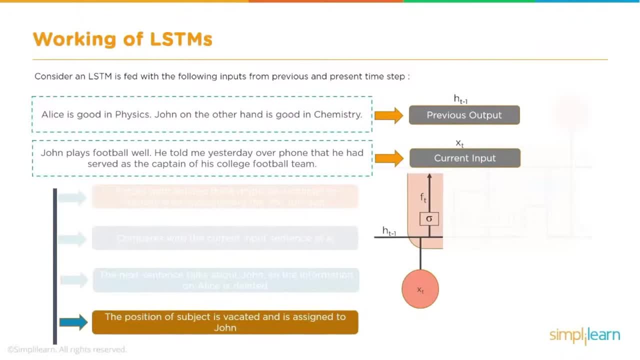 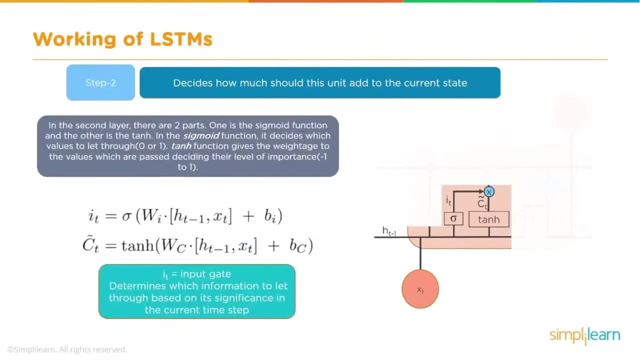 And so in this one, we've seen that we've weeded out a whole bunch of information, and we're only passing information on John, since that's now the new topic. So step two is then to decide how much should this unit add to the current state. 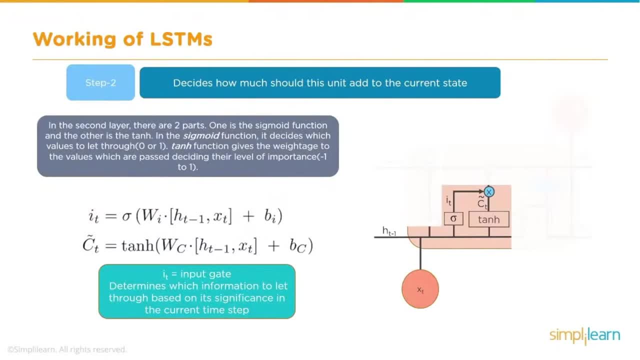 In the second layer there are two parts. One is the sigmoid function And the other is the tangent h. In the sigmoid function it decides which values to let through, zero or one. Tangent h function gives the weightage to the values which are passed. 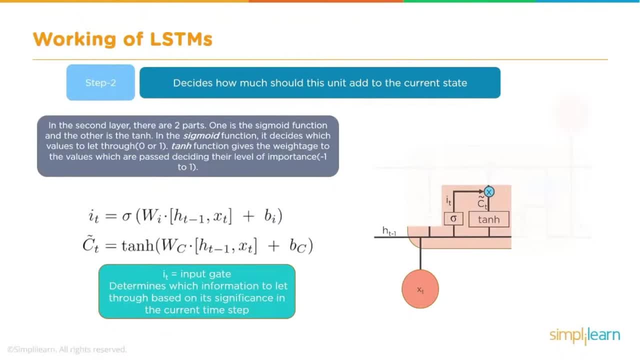 deciding their level of importance. minus one to one, And you can see the two formulators that come up. The i of t equals the sigmoid of the weight of i, h of t minus one, x of t plus the bias of i. 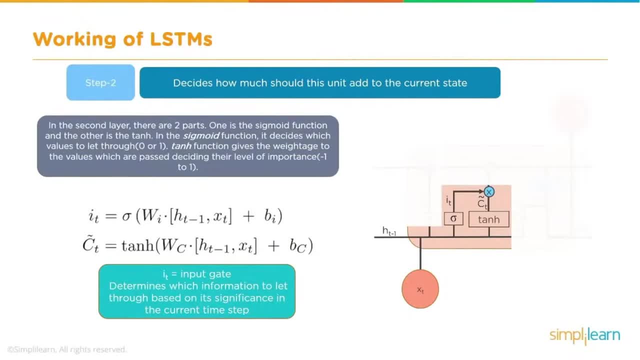 And the c of t equals the tangent of h, of the weight of c, of h of t, minus one x of t plus the bias of c. So our i of t equals the input gate determines which information to let through based on its significance in the current time step. 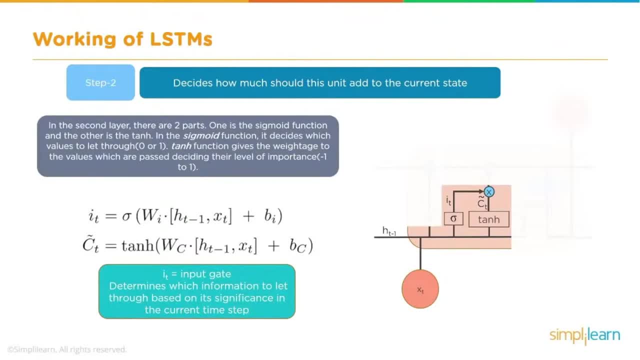 If this seems a little complicated, don't worry, because a lot of the programming is already done when we get to the case study. Understanding, though, that this is part of the program is important when you're trying to figure out what to set your settings at. 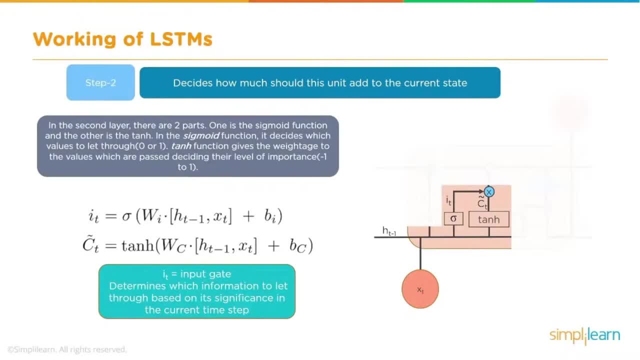 You should also note when you're looking at this. it should have some semblance to your forward propagation neural networks, where we have a value assigned to a weight plus a bias. This is another very important step in any of the neural network layers. 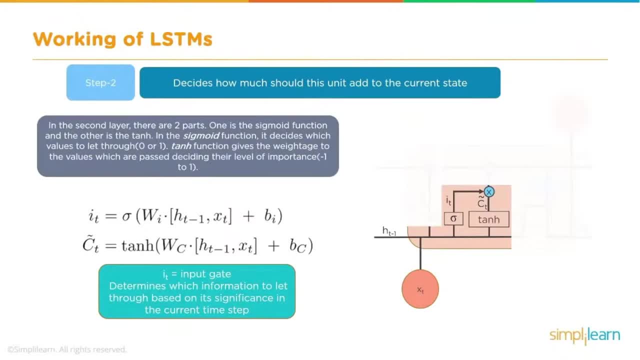 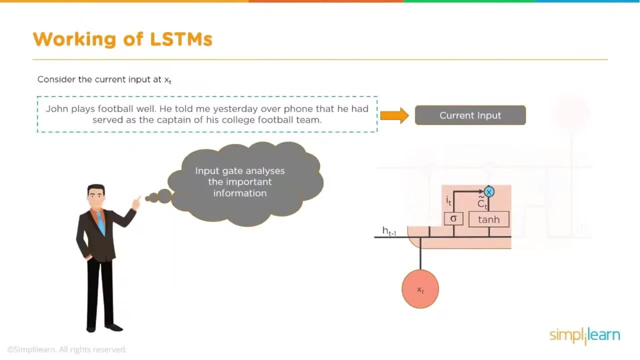 whether we're propagating into them the information from one to the next or we're just doing a straightforward neural network propagation. Let's take a quick look at this: what it looks like from the human standpoint. as I step out of my suit again. 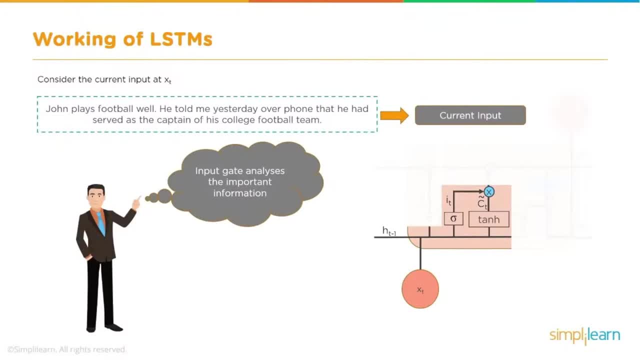 Consider the current input at x of t. John plays football. well, He told me yesterday over the phone that he has served as a captain of his college football team. That's our input Input gate analyses the important information- plays football and he was a captain of his college team is important, He told me. 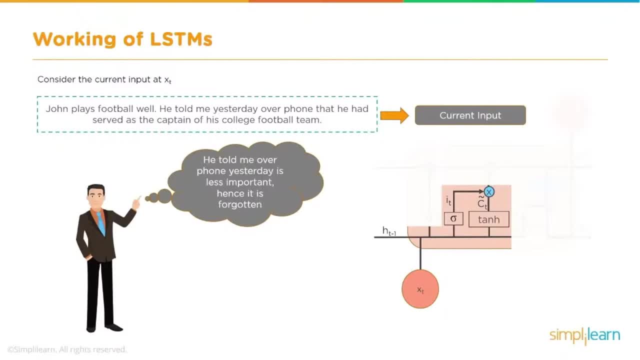 over the phone yesterday is less important, hence it is forgotten. This process of adding some new information can be done via the input gate. Now, this example is as a human form- and we'll look at training this stuff in just a minute- but as a human being. if I wanted to get this information from a 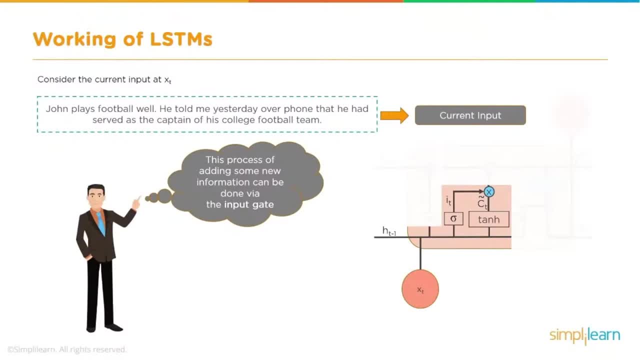 conversation. maybe it's a Google voice listening in on you or something like that. how do we weed out the information that he was talking to me on the phone yesterday? Well, I don't want to memorize that he talked to me on the phone. 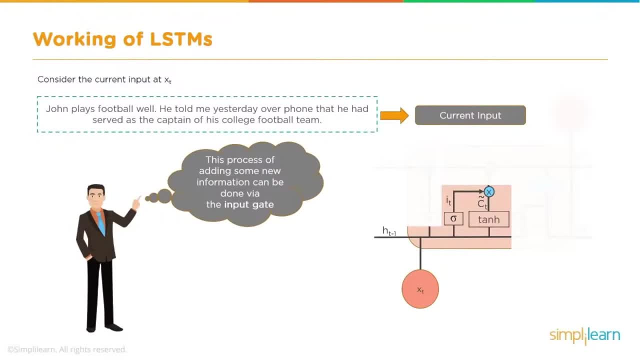 yesterday, or maybe that is important, but in this case it's not. I want to know that he was the captain of the football team. I want to know that he served. I want to know that John plays football and he was a captain of the college. 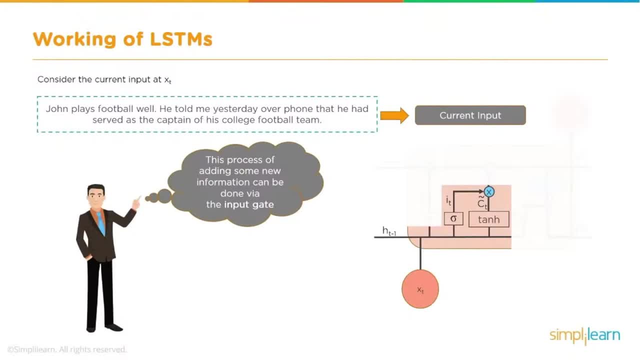 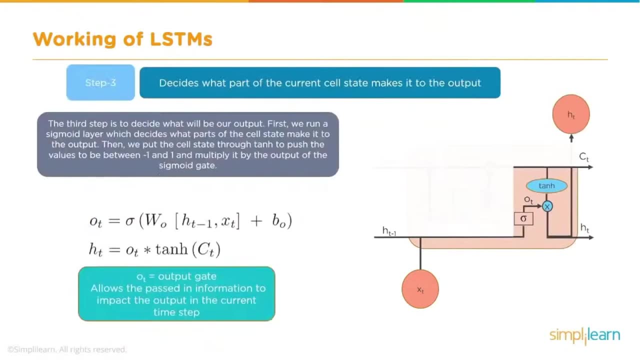 football team. Those are the two things that I want to take away as a human being. Again, we measure a lot of this from the human viewpoint and that's also how we try to train them so we can understand these neural networks. Finally, we get to step three. decides what part of the current cell state makes it to. 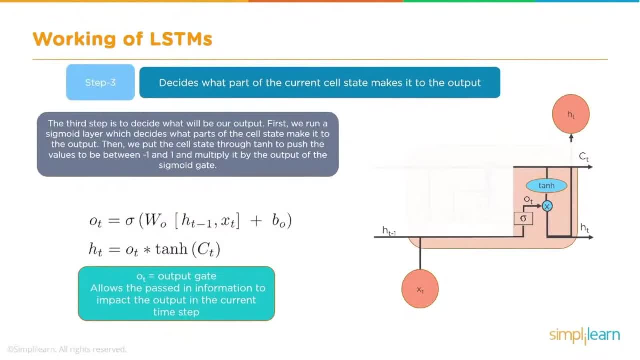 the output. The third step is to decide what will be our output. First we run a sigmoid layer which decides what parts of the cell state make it to the output. Then we put the cell state through the tangent H to push the values to be between minus one. 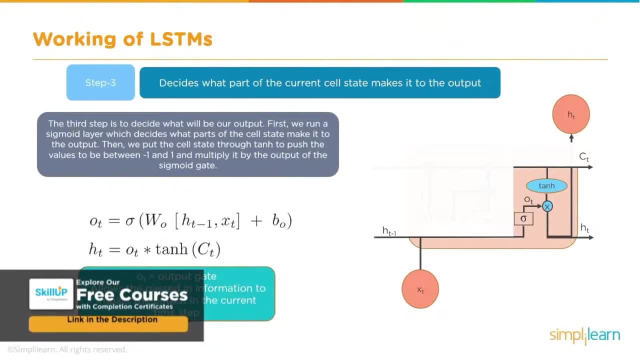 and one and multiply it by the output of the sigmoid gate. So when we talk about the output of T, we set that equal to the sigmoid of the weight of 0 of the H of T minus 1, and back one step in time by the X of T plus, of course, the bias, The H of T. 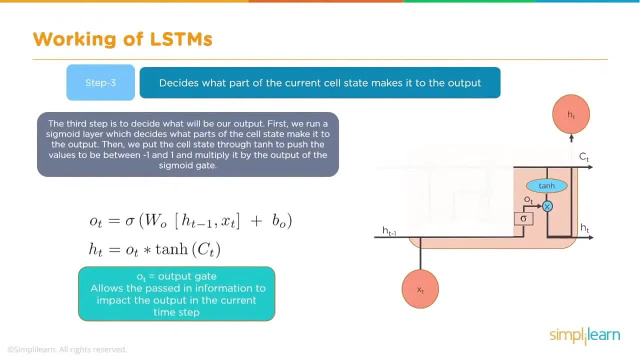 equals the out of T times the tangent of the tangent H of C of T. So our O of T equals the output gate allows the passed in information to impact the output in the current time step. Let's consider the example to predicting the next word in. 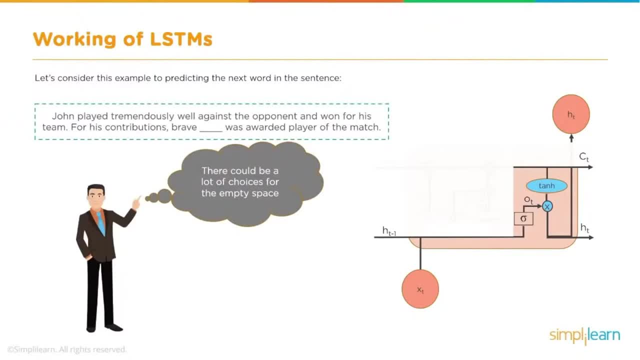 the sentence. John played tremendously well against the opponent and won for his team. For his contributions, brave blank was awarded player of the match. There could be a lot of choices for the empty space. Current input: brave is an adjective. Adjectives describe a noun. John could be the best output after brave Thumbs up. 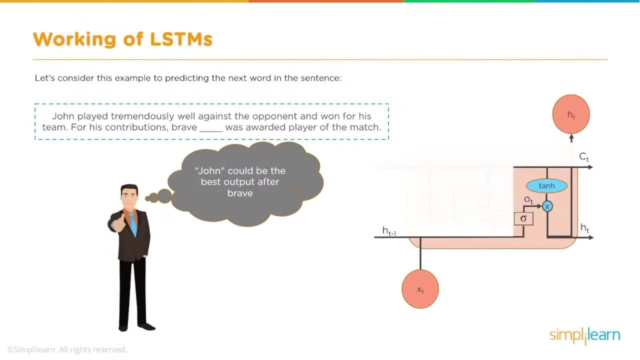 for John, awarded player of the match. And if you were to pull just the nouns out of the sentence team doesn't look right because it's not really the subject. we're talking about Contributions. you know, brave contributions or brave team. 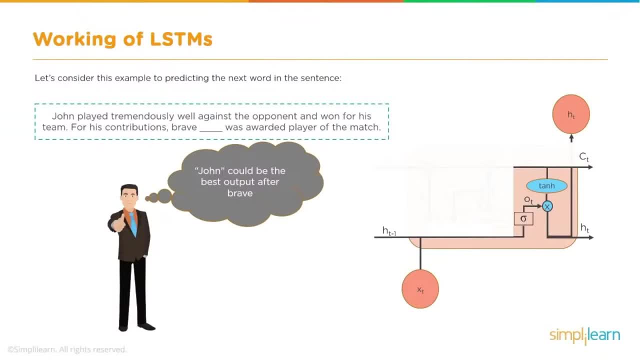 brave player, brave match. So you look at this and you can start to train this, this neural network. So it starts looking at it and goes, oh no, John is what we're talking about. So brave is an adjective, John's going to be the best output. and we give John a big thumbs up. And then of 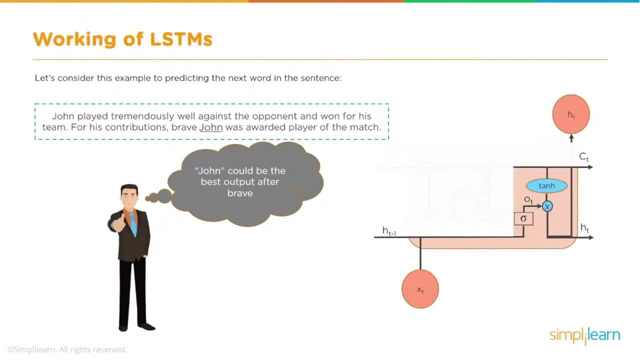 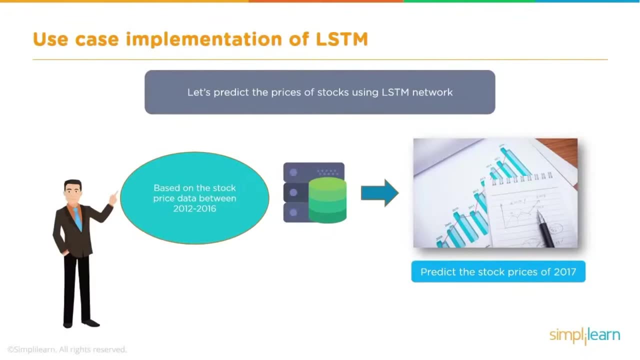 course we jump into my favorite part, the case study, Use case implementation of LSTM. Let's predict the prices of stocks using the LSTM network Based on the stock price data between 2012 and 2016.. We're going to try to predict the stock. 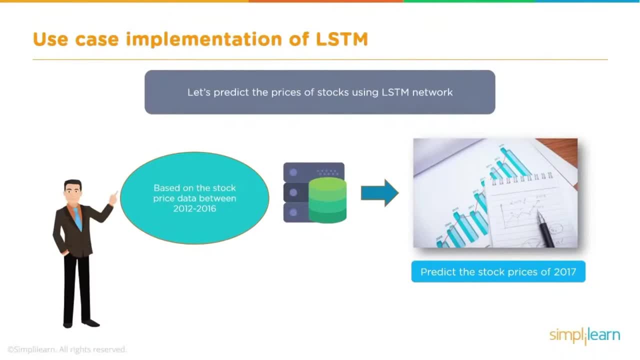 prices of 2017.. This will be a narrow set of data. We're not going to do the whole stock market. It turns out that the New York Stock Exchange generates roughly 1.5 million shares- three terabytes of data per day. That's all the different trades up and down of all the different. 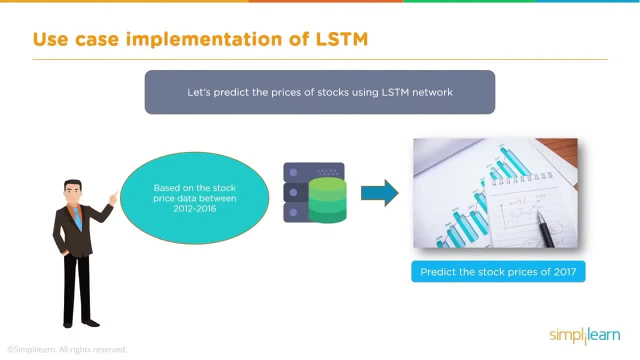 stocks going on and each individual one second to second or nanosecond to nanosecond. But we're going to limit that to just some very basic, fundamental information. so don't think you're going to get rich off this today, But at least you can give a step forward in how to start. 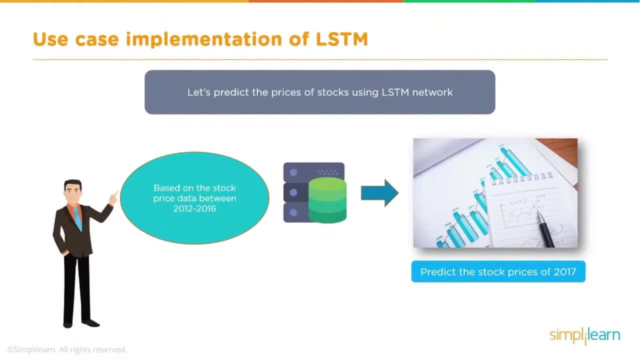 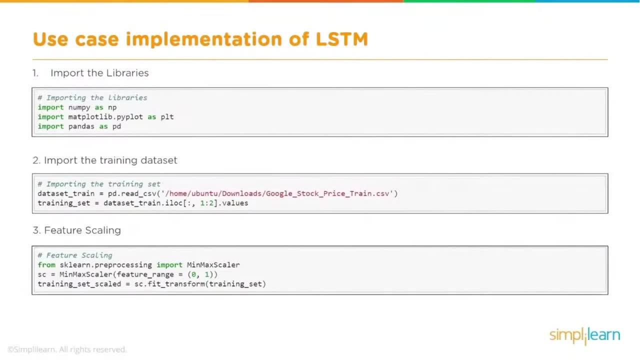 processing something like stock prices- a very valid use for machine learning in today's markets. Use case implementation of LSTM. Let's dive in. We're going to import our libraries. We're going to import the training set and get the scaling going. Now, if you watch any of our other tutorials, 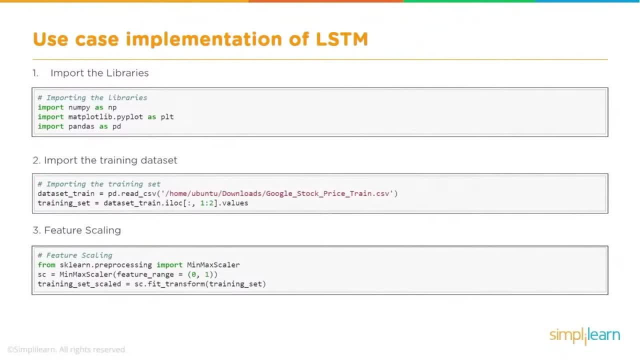 a lot of these pieces just start to look very familiar. It's a very similar setup. Let's take a look at that. and just a reminder: we're going to be using Anaconda, the Jupyter notebook, So here I have my Anaconda navigator When we go under environments. I've actually set up. 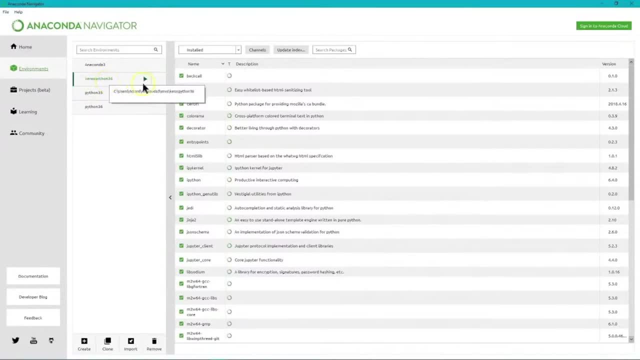 Anaconda When we go under environments, I've actually set up Anaconda. When we go under environments, I've actually set up Anaconda. When we go under environments, I've actually set up a cross, Python 3.6.. I'm in Python 3.6.. And the nice thing about Anaconda, especially the newer- 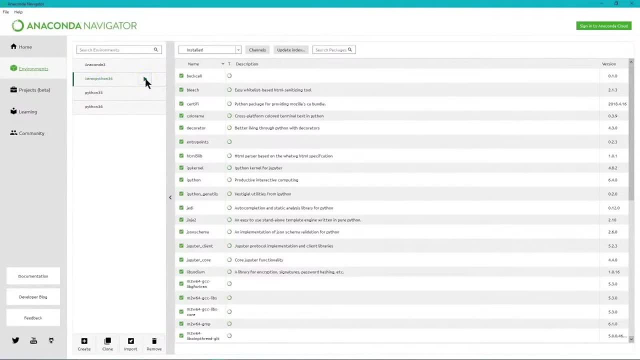 version. I remember a year ago messing with Anaconda and different versions of Python in different environments. Anaconda now has a nice interface and I have this installed both on a Ubuntu Linux machine and on Windows so it works fine on there. You can go in here and open a. 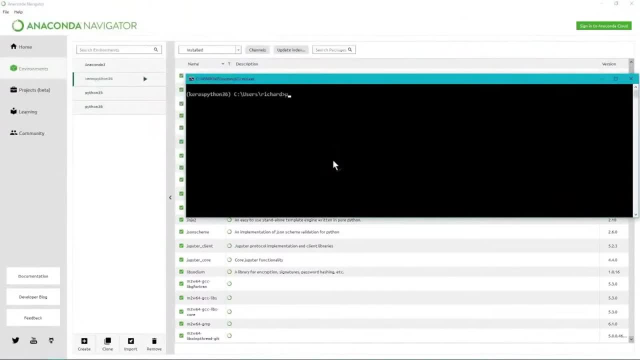 terminal window and then in here. once you're in the terminal window, this is where you're going to start installing, using PIP to install your different modules and everything. Now, we've already pre-installed them, so we don't need to do that in here. But if you don't have them, 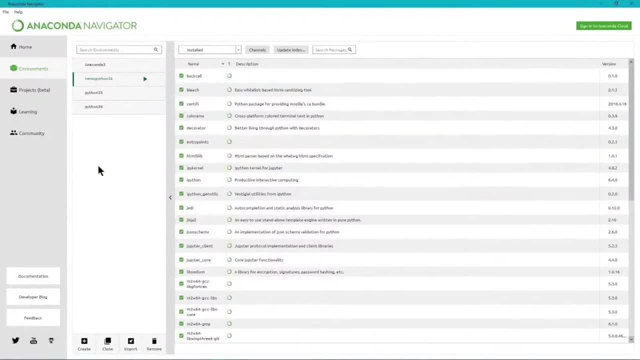 installed in your particular environment. you'll need to do that And of course, you don't need to use the Anaconda or the Jupyter. You can use whatever favorite Python IDE you like. I'm just a big fan of this because it keeps all my stuff separate. You can see, on this machine I have specifically 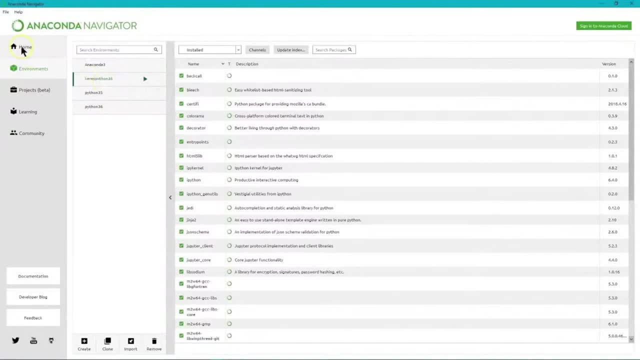 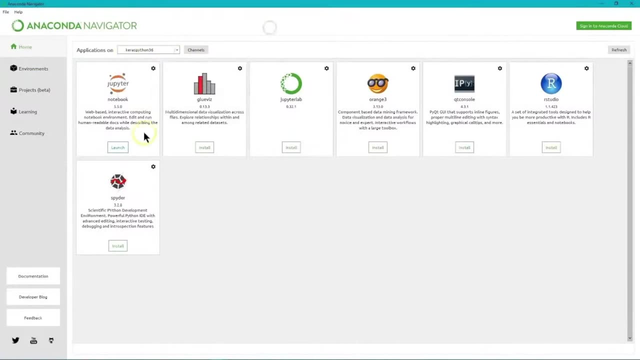 installed one for Keras. since we're going to be working with Keras under TensorFlow When we go back to home, I've gone up here to application and that's the environment I've loaded on here And then we'll click on the launch Jupyter notebook. Now I've already, in my Jupyter notebook, have set up a lot. 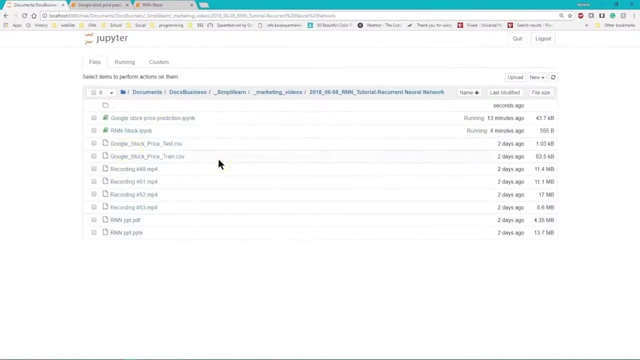 of stuff so that we're ready to go kind of like Martha Stewart's in the old cooking shows. We want to make sure we have all our tools for you so you're not waiting for them to load. And if we go up here to where it says new, you can see where you can create a new Python 3.. That's what we did. 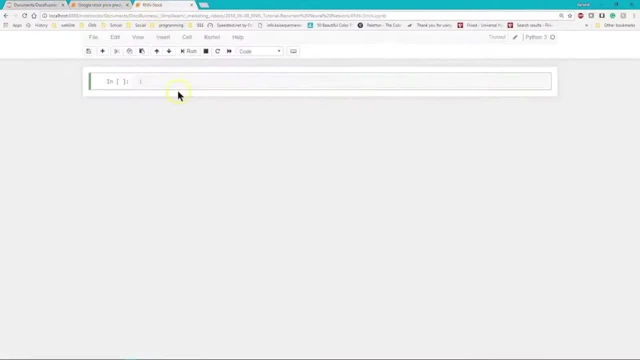 here underneath the setup. so it already has all the modules installed on it And I'm going to actually rename this. If you go under file, you can rename it. I'm calling it RNN stock And let's just take a look and start diving into the code. Let's get into the exciting part Now. we've 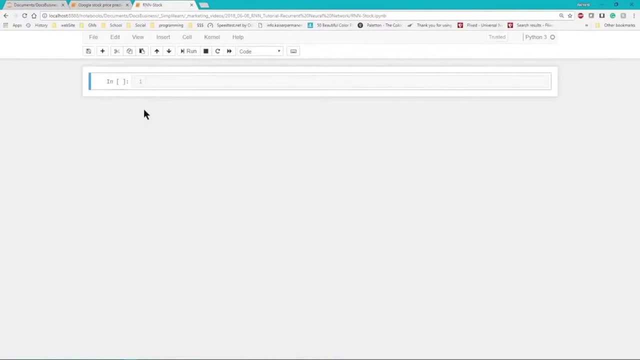 looked at the tool and of course you might be using a different tool, which is fine. Let's start putting that code in there and seeing what those imports and uploading everything looks like. Now, first half is kind of boring when we hit the run button because we're going to be importing numpy. 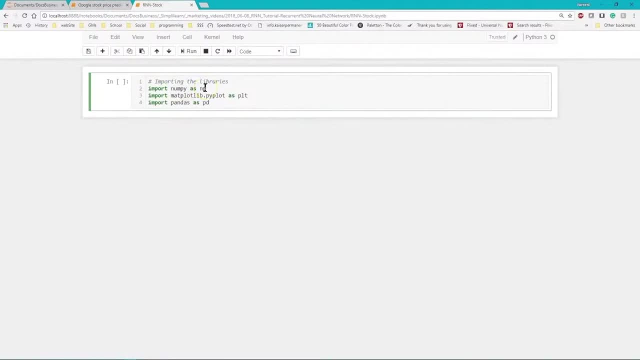 as np, That's the number- Python, which is your numpy array, and the matplot library. so we're going to do some plotting at the end And our pandas for our data set, our pandas as pd, And when I hit run, I'm going to be able to see what's going on And I'm going to be able to see what's. 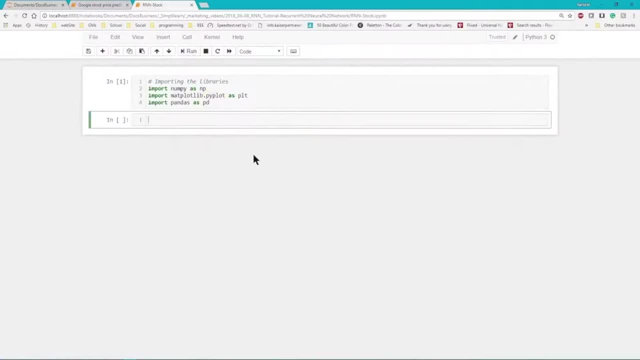 going on. So let's get started. Really doesn't do anything except for load those modules. just a quick note. let me just do a quick draw here. oh, Shift should be. If you stop here, you'll notice when we're doing this setup. if I was to divide this up, I'm going to actually 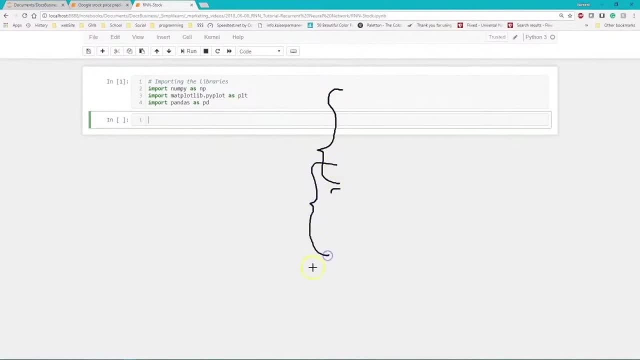 overlap these. Here we go. This first part that we're going to do is our data Prep. a lot of prepping involved is this one square line over here, And we need to do this with us pretty quickly involved, In fact, depending on what your system is. since we're using Keras, I put an overlap here. 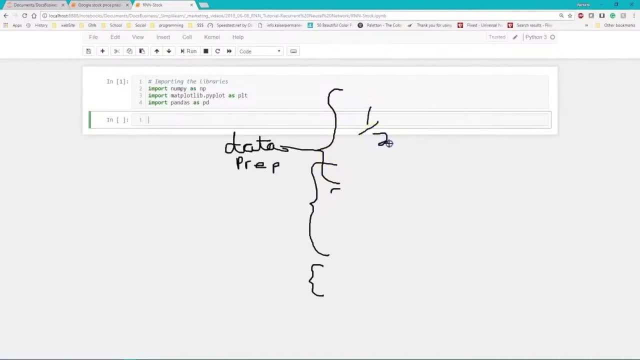 but you'll find that almost, maybe even half, of the code we do is all about the data prep, And the reason I overlap this with Keras- let me just put that down, because that's what we're working in- is because Keras has, like their own preset stuff, So it's already pre-built in, which is really nice. 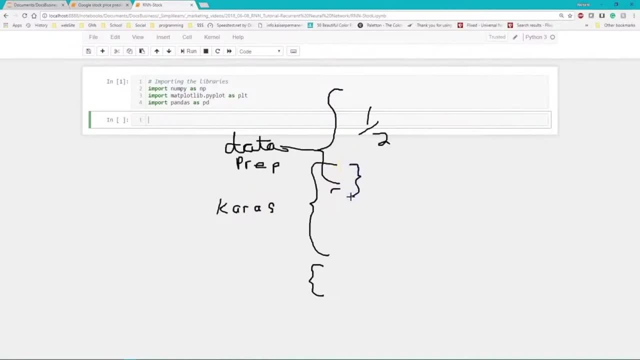 So there's a couple steps, a lot of times, that are in the Keras setup. We'll take a look at that to see what comes up in our code as we go through and look at stock. And then the last part is to evaluate And if you're working with shareholders or classroom whatever it is you're working with. 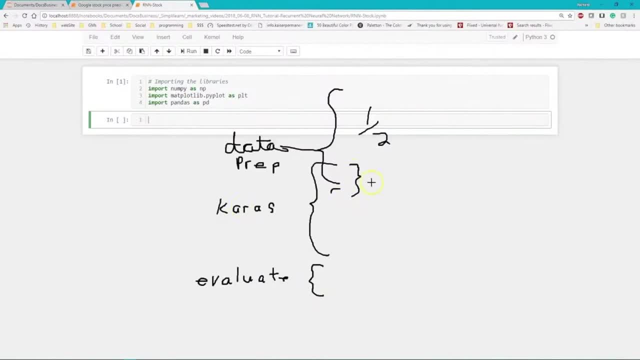 the evaluate is the next biggest piece. So the actual code here Keras is a little bit more, but when you're working with some of the other packages you might have like three lines. That might be it. All your stuff is in your pre-processing and your data, Since Keras is. 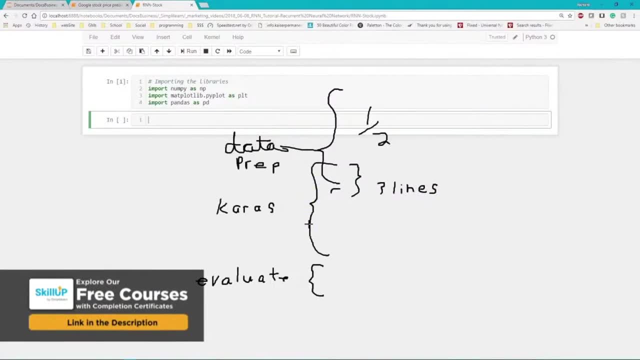 cutting edge and you load up your data. you're going to have to do a lot of processing. So the individual layers- you'll see that there's a few more lines here and cross is a little bit more robust, And then you spend a lot of times, like I said, with the evaluate you want to have. 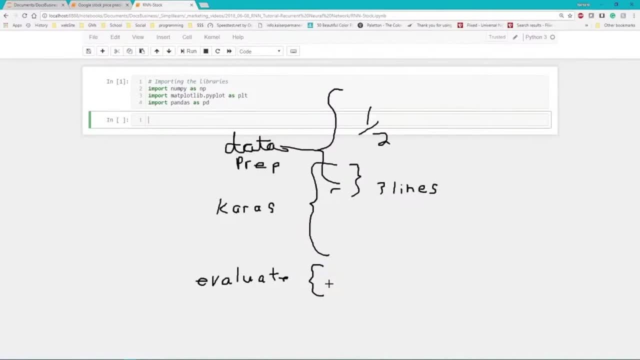 something you present to everybody else and say, hey, this is what I did, This is what it looks like. So let's go through those steps. This is like a kind of just general overview And let's just take a look and see what the next set of code looks like. And in here we have a dataset train. 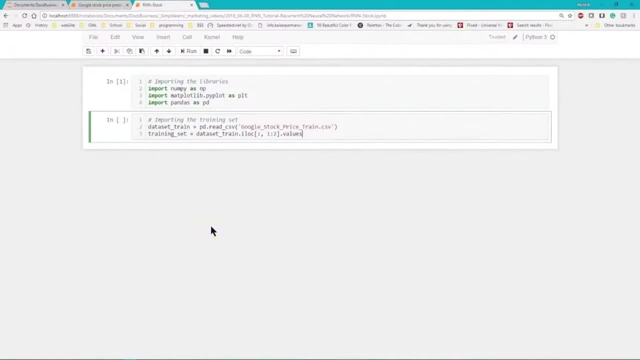 and it's going to be read using the PD or pandasreadcsv And it's a Google stock price traincsv And it's going to be read using the PD or pandasreadcsv And it's going to be read using: And so under this we have training set, equals dataset, train dot ilocation, And we've kind of 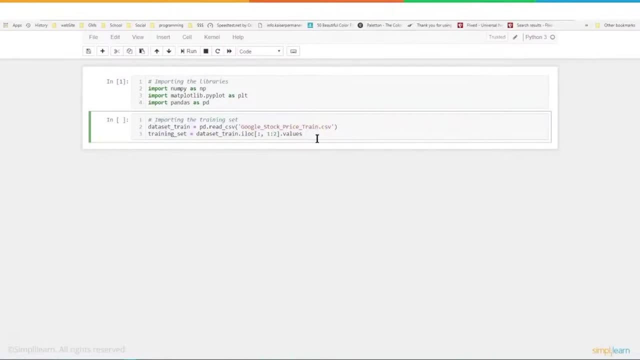 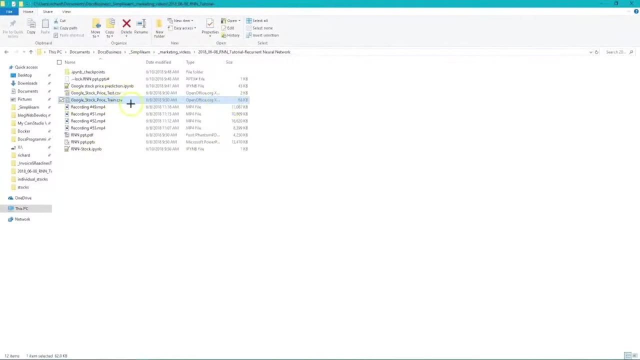 sorted out part of that. So what's going on here? Let's just take a look at the actual file and see what's going on there. Now, if we look at this, ignore all the extra files on this. I already have a train and a test set where it's sorted out. This is important to notice because a lot of times we 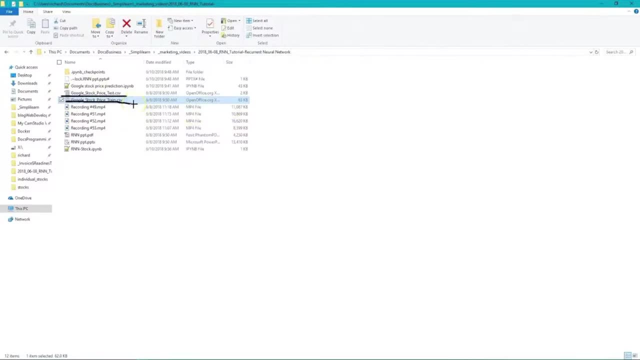 do that as part of the pre-processing of the data. We take 20% of the data out so we can test it, and then we train the rest of it. That's what we use to create our neural network. That way we can find out how good it is. But let's go ahead and just take a look and see what that looks like. 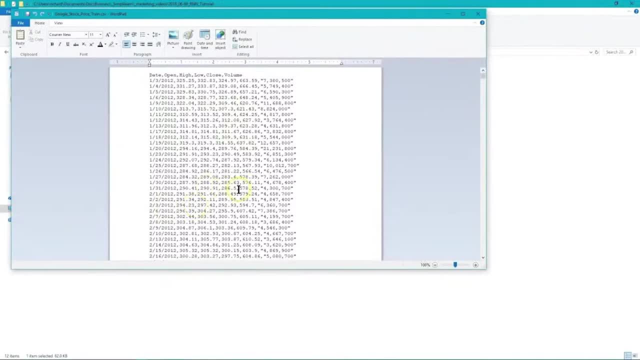 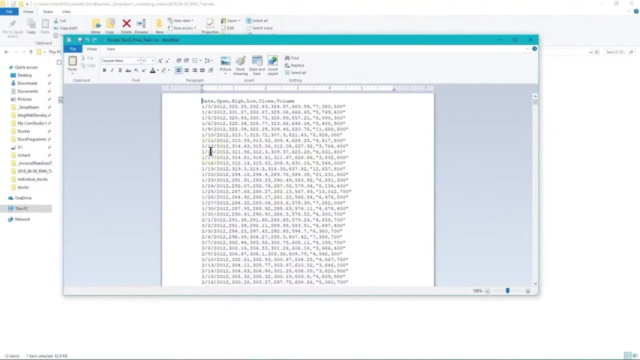 as far as the file itself, And I went ahead and just opened this up in a basic WordPad text editor just so we can take a look at it. Certainly you can open up an Excel or any other kind of spreadsheet, And we note that this is a comma-separated variables. We have a date. 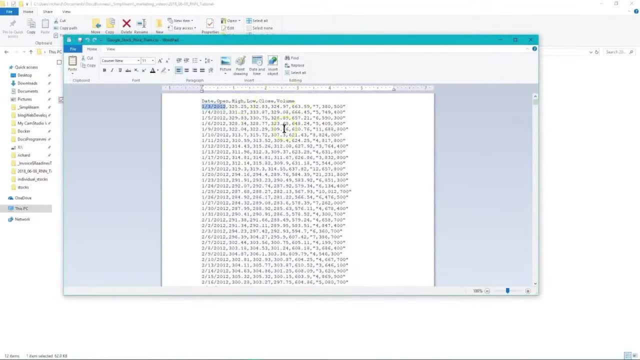 open high, low, close volume. This is the standard stuff that we import into our stock, One of the most basic set of information you can look at in stock. It's all free to download. In this case, we downloaded it from Google. That's why we call it the Google Stock Price. 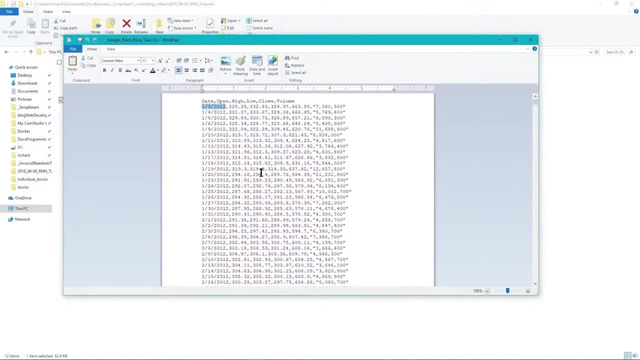 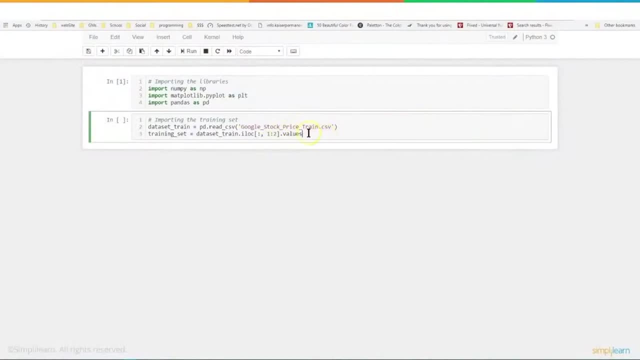 And it specifically is Google. This is the Google stock values from. as you can see here, we started off at 1-3-2012.. So when we look at this first setup up here, we have a data set. train equals pd, underscore, csv, And if you noticed on the original frame, let me just go back there. 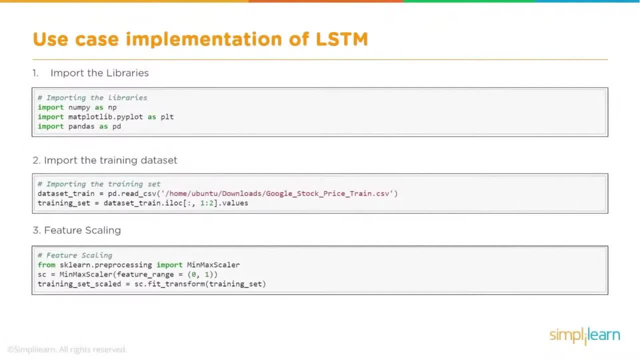 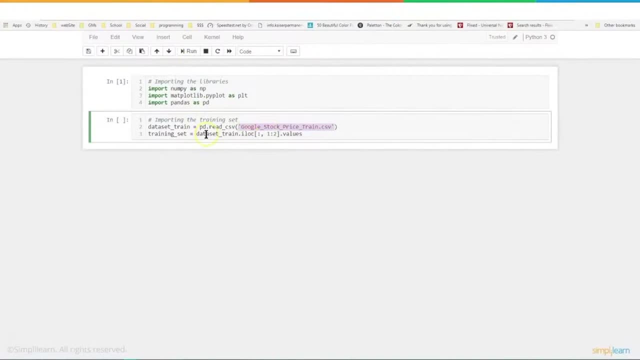 They had it set to home Ubuntu downloads- Google stock price train. I went ahead and changed that because we're in the same file where I'm running the code. So I've saved this particular Python code and I don't need to go through any special paths or have the full path on there And then. 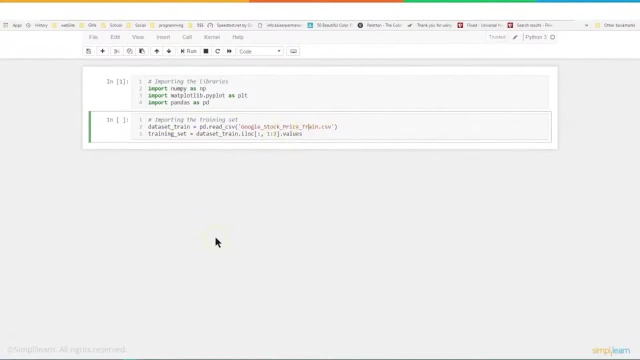 of course, we want to take out certain values in here And you're going to notice that we're using our data set And we're now in pandas. So pandas, basically it looks like a spreadsheet, And in this case, we're going to do ilocation, which is going to get specific locations. 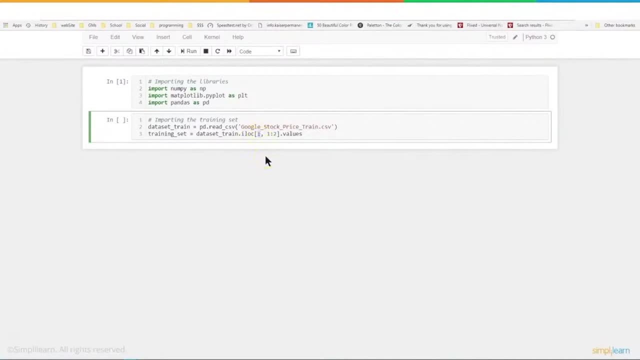 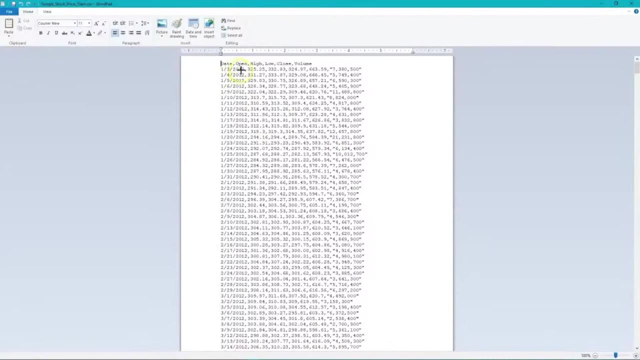 The first value is going to show us that we're pulling all the rows in the data And the second one is we're only going to look at columns one and two And if you remember, here from our data, as we switch back on over columns, we always start with zero, which is the date And we're. 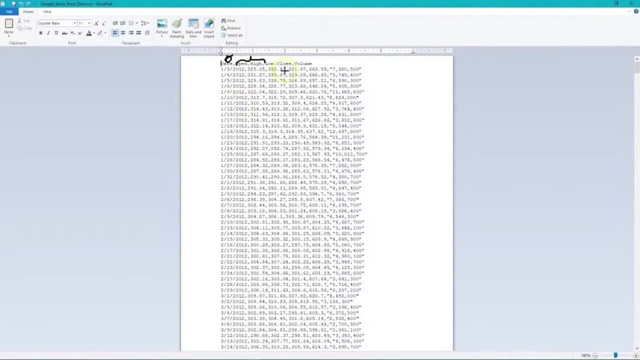 going to be looking at open and high, which would be one and two. We'll just label that right there and see Now when you go back and do this. you certainly can extrapolate and do this on all the columns, But for the example let's just limit a little bit here so that we can focus on just some. 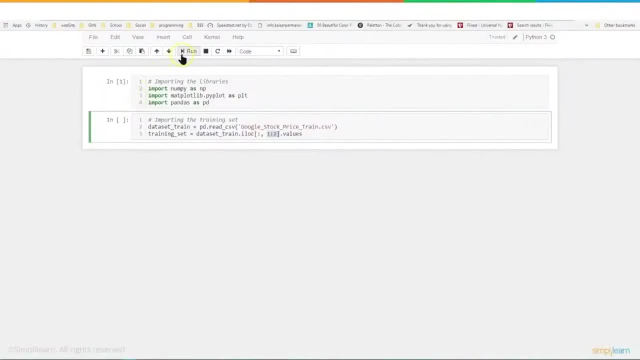 key aspects of stock, And then we'll go up here and run the code. And again I said, the first half is very boring. Whenever you hit the run button, it doesn't do anything because we're still just loading the data and setting it up. Now that we've loaded our data, we want to go. 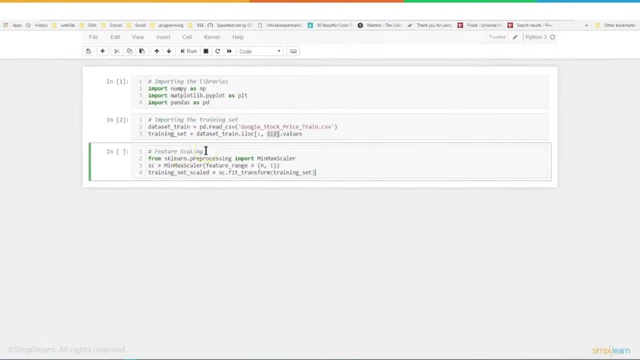 ahead and scale it. We want to go ahead and scale it And we want to go ahead and scale it And we want to do what they call feature scaling. And in here we're going to pull it up from the sklearn or the skkit, preprocessing import min max scaler. And when you look at this you got to remember: 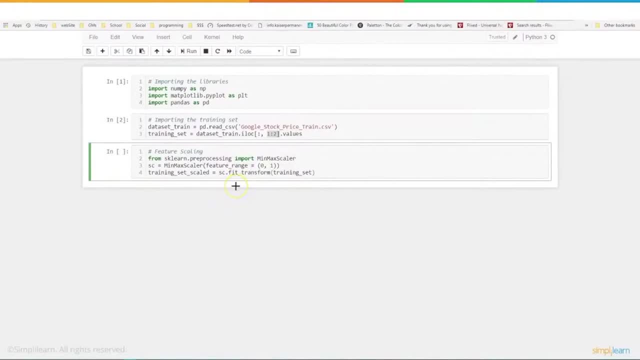 that biases in our data. we want to get rid of that. So if you have something that's like a really high value, let's just draw a quick graph And I have something here like: maybe the stock has a value. One stock has a value of 100.. And another stock has a value of 5.. 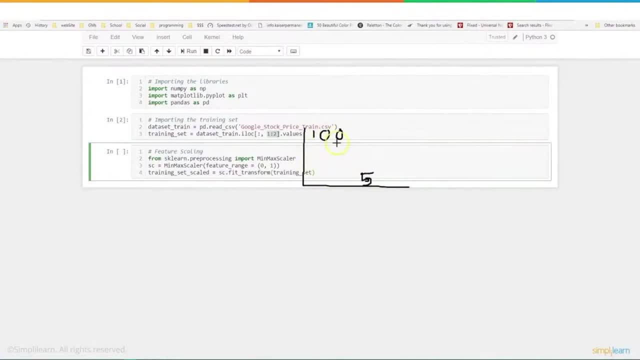 You start to get a bias between different stocks, And so when we do this, we go ahead and say: okay, 100 is going to be the max, And five is going to be the min, And then everything else goes, And then we change this, So we just squish it down. I like the word squish, So it's between: 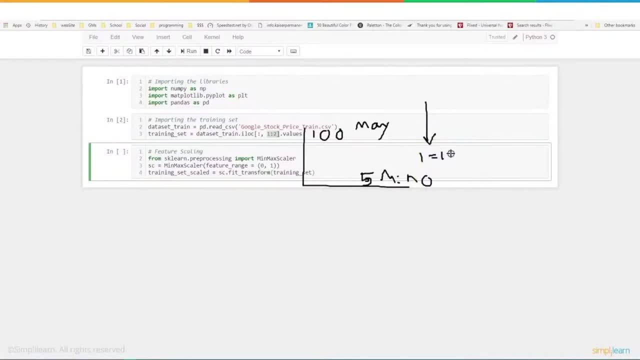 one and zero. So 100 equals one, or one equals 100. And zero equals five. And you can just multiply. It's usually just a simple multiplication. we're using Multiplication, So it's going to be minus five and then 100 divided or 95 divided by one. So whatever value, 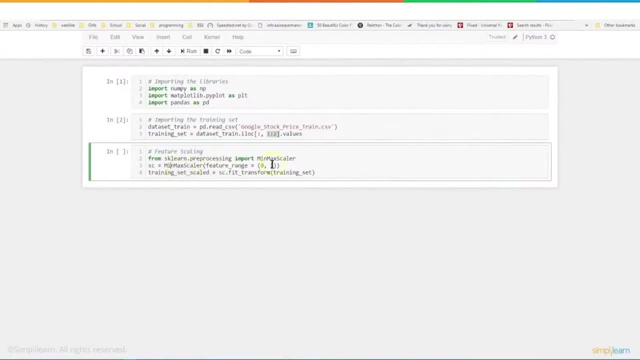 is is divided by 95. And once we've actually created our scale, we're telling it's going to be from zero to one. We want to take our training set and we're going to create a training set scaled And we're going to use our scaler SC and we're going to fit, We're going to fit and. 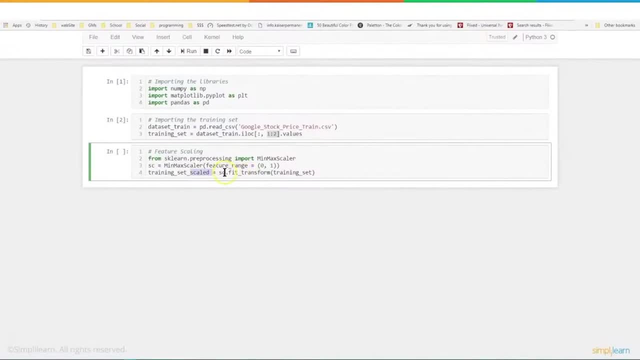 transform the training set So we can now use the SC, this particular object. We'll use it later on our testing set Because, remember, we have to also scale that when we go to test our model and see how it works, And we'll go ahead and 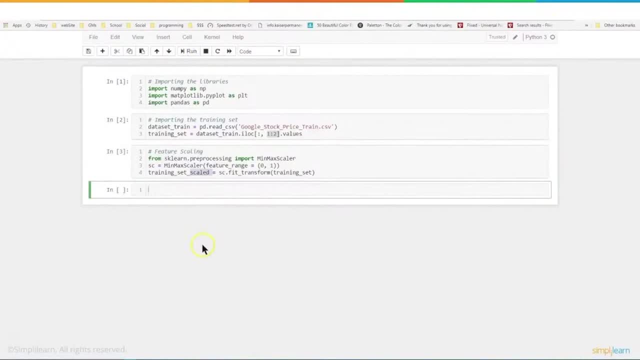 click on the run. Again, it's not going to have any output yet because we're just setting up all the variables, All right. so we paste the data in here And we're going to create the data structure with the 60 time steps and output. First note: we're running 60 time steps And that is where this 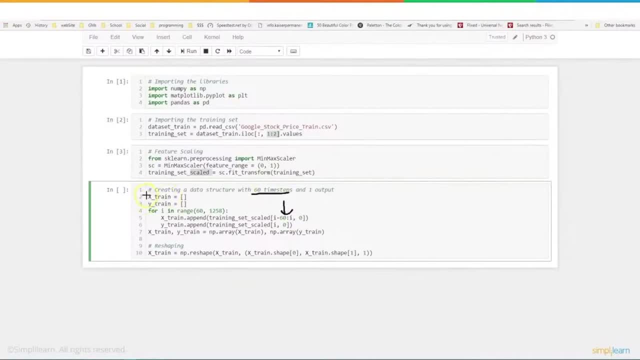 value here also comes in. So the first thing we do is we create our x train and y train variables And we're going to set them to an empty Python array- Very important to remember what kind of array we're in and what we're working with. And then we're going to come in here. We're going to go for 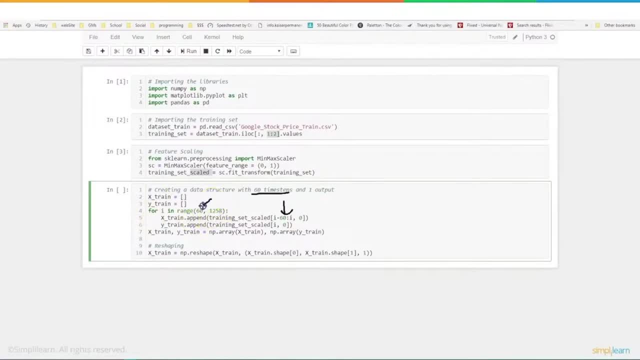 i in range 60 to 1258.. There's our 60, 60 time steps, And the reason we want to do this is, as we're adding the data in, there's nothing below the 60. So if we're going to use 60 time steps, 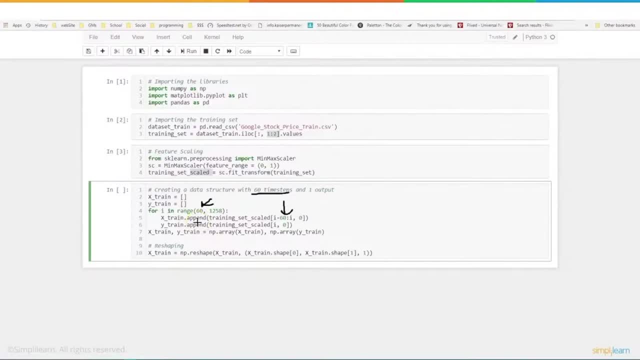 we have to start at point 60, because it includes everything underneath of it, Otherwise you'll get a pointer error. And then we're going to take our x train and we're going to append that to x train And we're going to set scale. This is a scaled value between 0 and 1.. And then 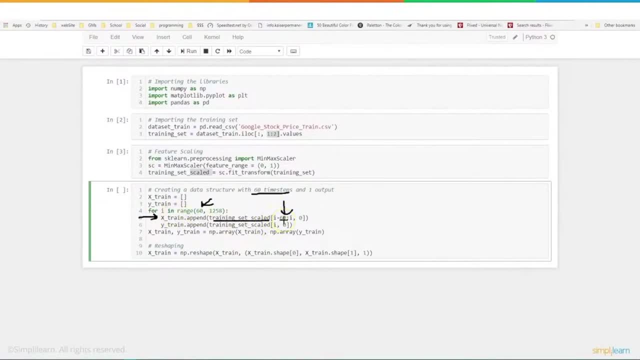 as i is equal to 60,, this value is going to be: 60 minus 60 is 0. So this actually is 0 to i, So it's going to be 0 to 60.. 1 to 61. Let me just circle this part right here: 1 to 61,, 2 to 62, and so on. 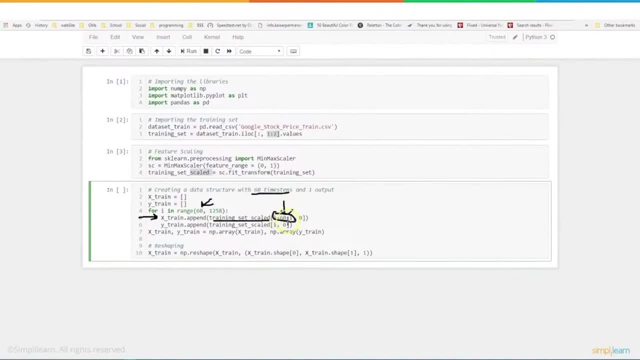 and so on. And, if you remember, I said 0 to 60. That's incorrect because it does not count. It doesn't count of 60.. So it's actually 59.. Important to remember that as we're looking at this And then the second part of this that we're looking at. So, if you remember correctly, here we 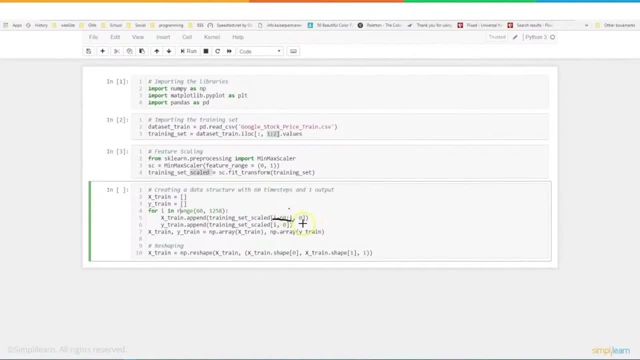 go. We go from 0 to 59 of i, And then we have a comma, a 0 right here. So finally, we're just going to look at the open value Now. I know we did put it in there for 1 to 2. If you remember. 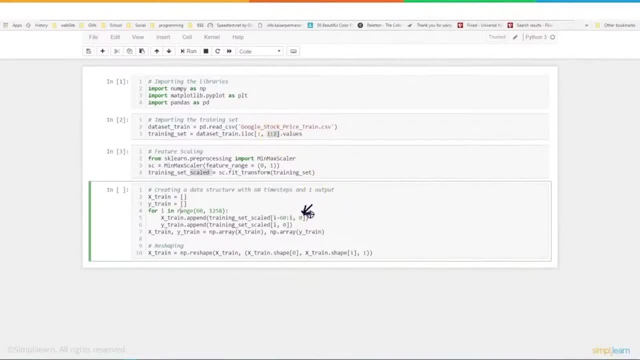 correctly. it doesn't count the second one, So it's just the open value. we're looking at just open, And then finally we have 1 to 2. And then we're going to look at the open value And then finally. 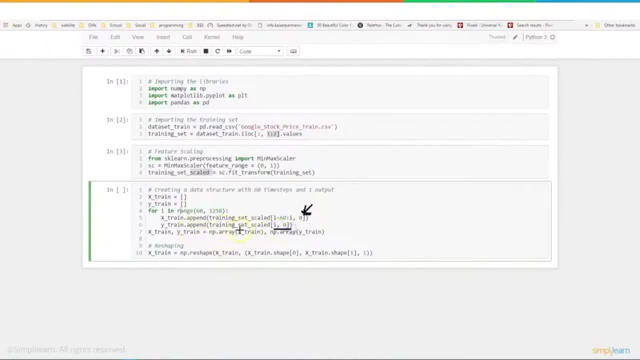 we have y train dot append training set i to 0. And if you remember correctly, i comma 0. If you remember correctly, this is 0 to 59. So there's 60 values in it. So when we do, i down here this is: 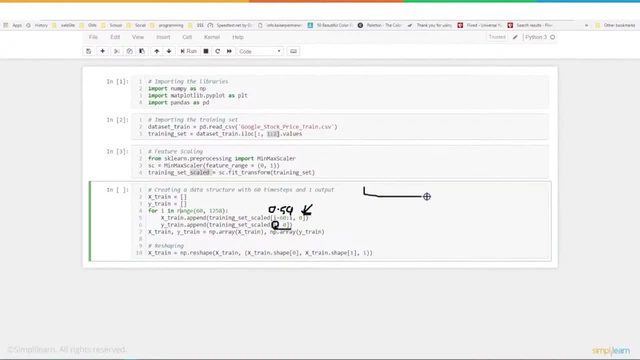 number 60.. So we're going to do this as we're creating an array And we have 0 to 59. And over here we have number 60, which is going into the y train. It's being appended on there, And then this: 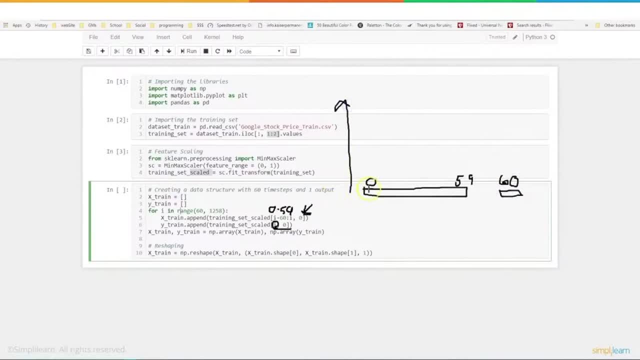 goes all the way up. So this is down here- is 0 to 59. And we'll call it 60,, since that's the value over here, And it goes all the way up to 1258.. That's where this value here comes in. That's the. 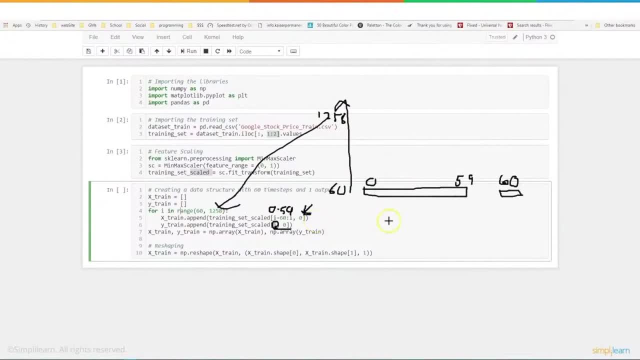 length of the data we're loading. So we've loaded two arrays. we've loaded one array that has, which is filled with arrays from 0 to 59. And we loaded one array, which is just the value And what we're looking at. you want to think about this as a time sequence? 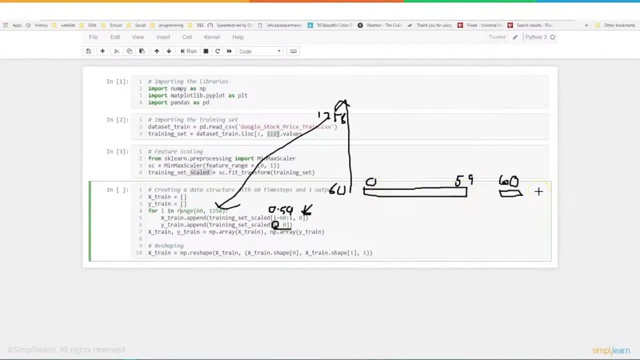 If I open, open, open, open, open, open, what's the next one in the series? So we're looking at the Google stock And each time it opens, we want to know what the next one? 0 through 59,? what's 60?? 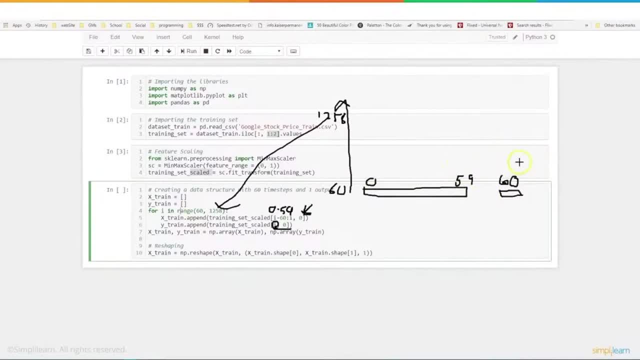 1 through 60,, what's 61?, 2 through 62,, what's 62?, And so on and so on going up, And then, once we've loaded those in our for loop, we go ahead and take x train and y train equals nparray. 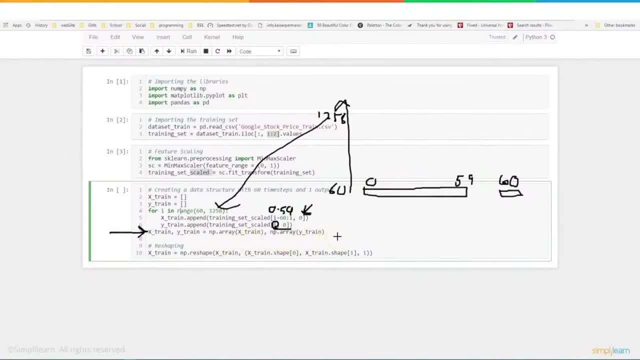 x trainnparray y train. We're just converting this back into a numpy array. That way, we can use all the cool tools that we get with numpy array, including reshaping. So if we take a look and see what's going on here, we're going to take our x train, we're going to reshape it, Wow. 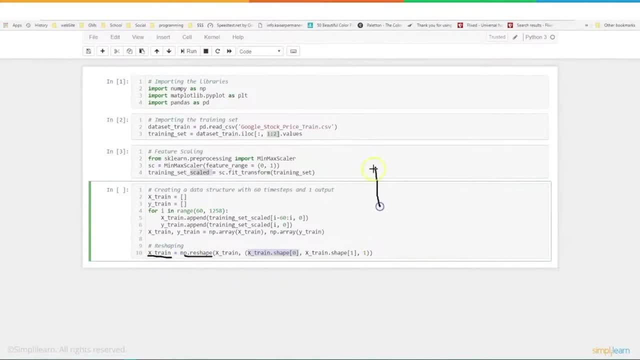 what the heck does reshape mean? That means we have an array- if you remember correctly- so many numbers by 60. That's how wide it is. And so when you do x train dot shape, that gets one of the shapes And you get x train dot shape of one. 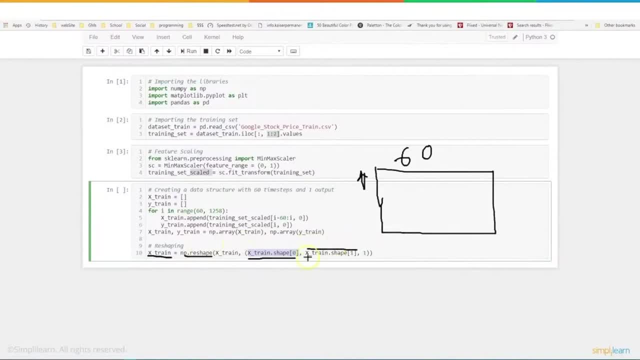 and the other shape. Now we're just making sure the data is formatted correctly, And so you use this to pull the fact that it's 60 by. in this case, where's that value? 60 by 1199.. 1258 minus. 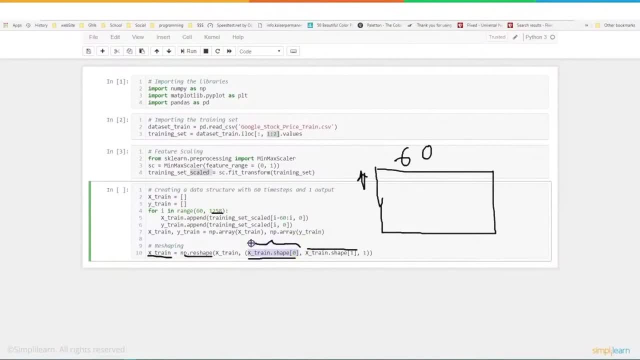 60, 1199.. And we're making sure that that is shaped correctly. So the data is grouped into 1199 by 60 different arrays, And then the one on the end just means at the end, because when you're dealing with shapes and numpy, 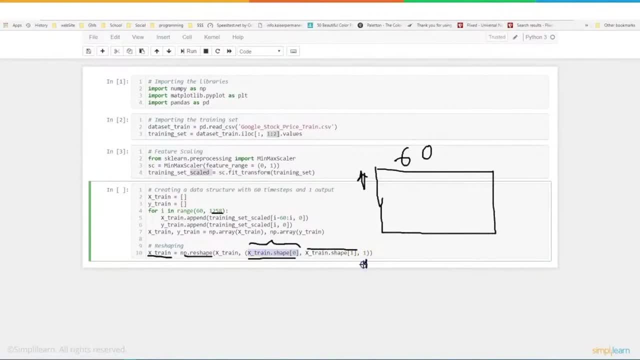 at this as layers, and so the end layer needs to be one value. That's like the leaf of a tree, where this is the branch and then it branches out some more and then you get the leaf npreshape comes from and, using the existing shapes to form it, We'll go ahead and run this piece of code Again. 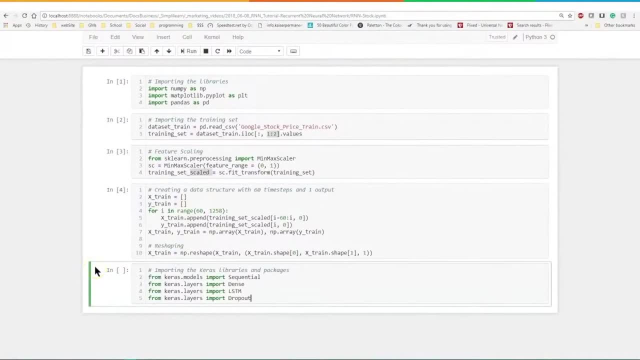 there's no real output and then we'll import our different cross modules that we need. So, from cross models, we're going to import the sequential model. We're dealing with sequential data. We have our dense layers. We have actually three layers. we're going to bring in Our dense, our LSTM, which 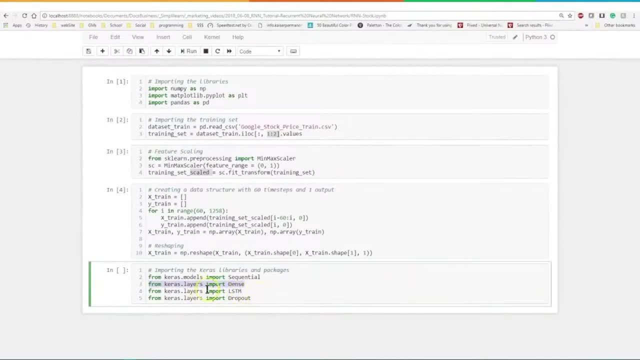 is what we're focusing on- and our dropout, And we'll discuss these three layers more in just a moment. But you do need the with the LSTM, you do need the dropout and then the final layer will be the dense. But let's go ahead and run this and that'll bring import our modules And you'll see. 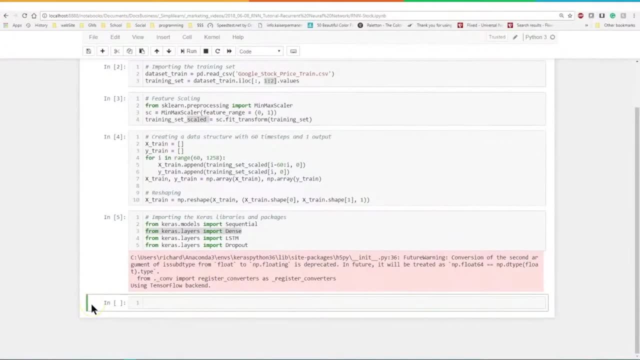 we get an error on here And if you read it closer, it's not actually an error, it's a warning. What does this warning mean? These things come up all the time when you're working with such cutting edge modules that are completely being updated all the time. We're not going to worry too much about the warning. All it's saying. 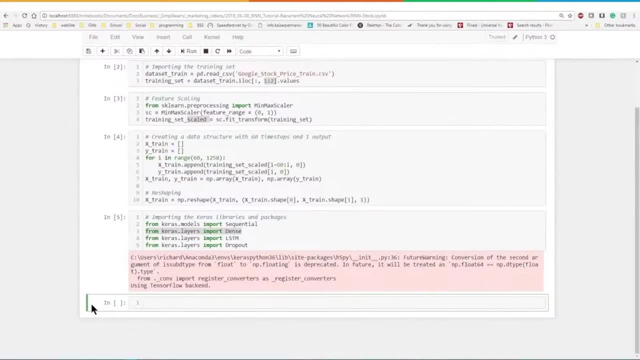 is that the H5PY module, which is part of cross, is going to be updated at some point, And if you're running new stuff on cross and you start updating your cross system, you better make sure that your H5PY is updated too. Otherwise you're going to have an error later on And you can actually just 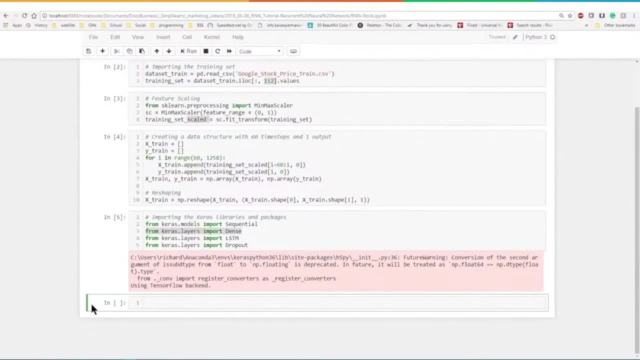 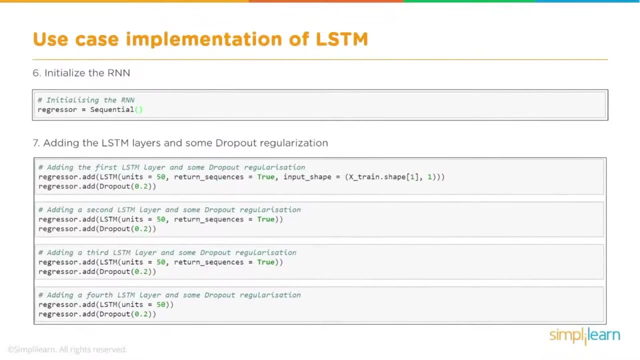 run an update on the H5PY now if you wanted to. Not a big deal, We're not going to worry about that today, And I said we were going to jump in and start looking at what those layers mean. I meant that, And we're going to start off with initializing the RNN And then 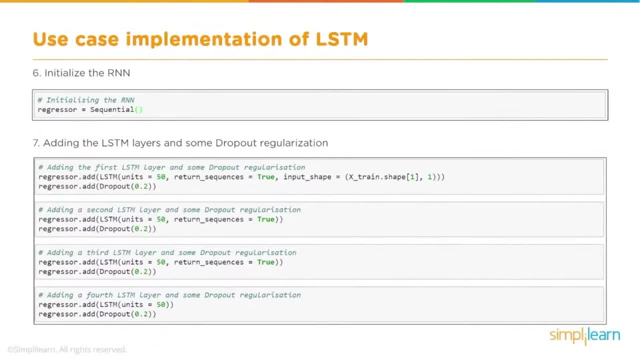 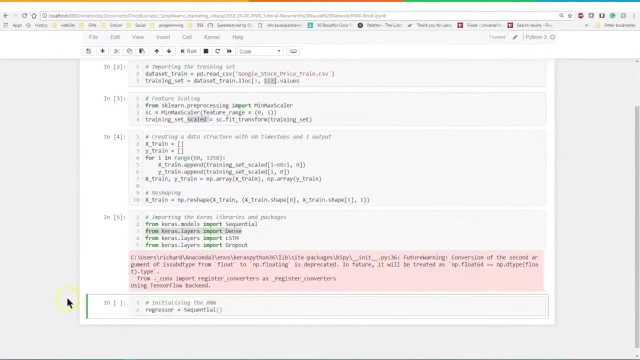 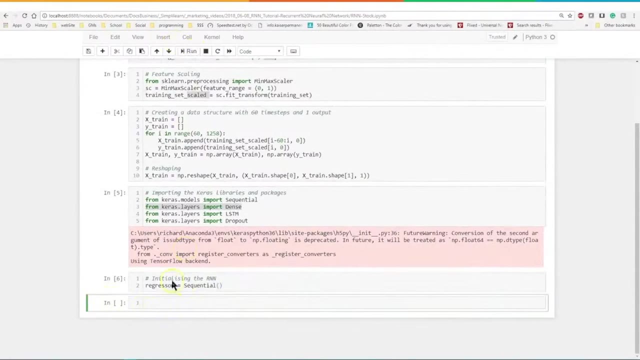 we'll start adding those layers in And you'll see that we have the LSTM and then the dropout, LSTM, then dropout, LSTM, then dropout. What the heck is that doing? So let's explore that. We'll start by initializing the RNN. Regressor equals sequential, because we're using the sequential model, And we'll 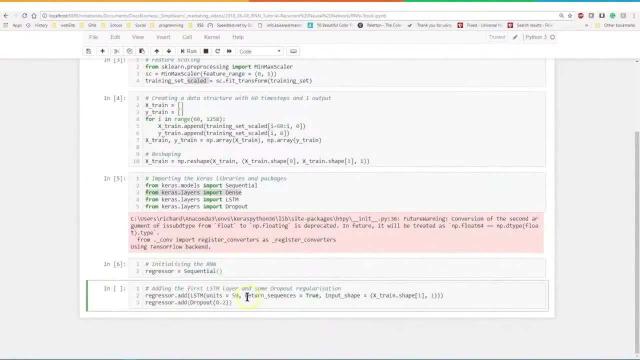 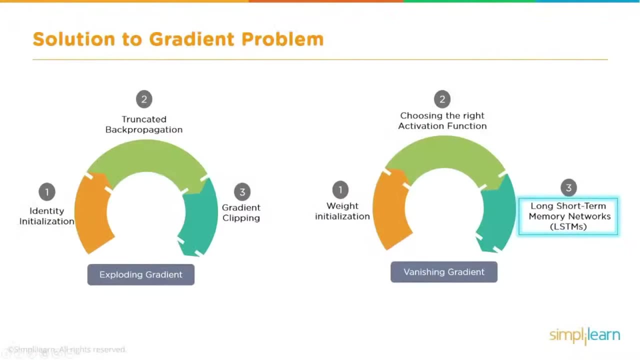 run that and load that up, And then we're going to start adding our LSTM layer and some dropout regularization and, right, there should be the Q dropout regularization and if we go back here and remember our exploding gradient, well, that's what we're talking about. the 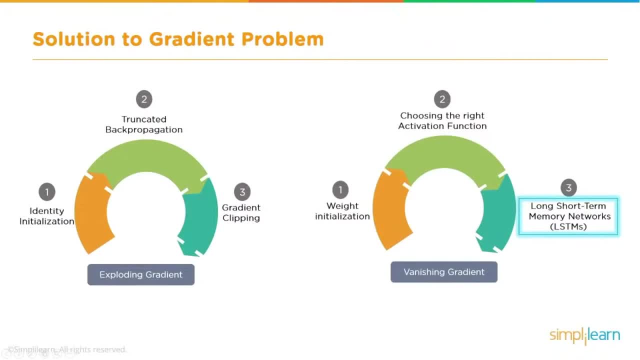 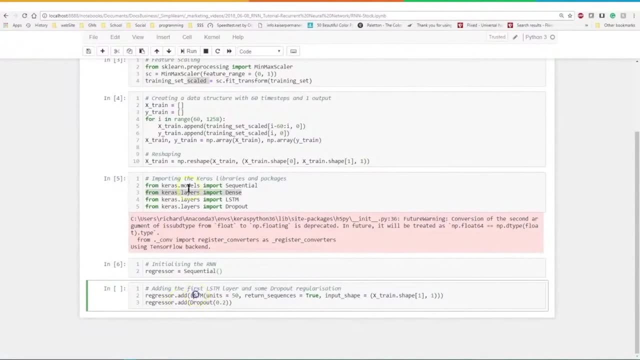 dropout drops out unnecessary data, so we're not just shifting huge amounts of data through the network, so, and so we go in here. let's just go ahead and add this in. I'll go ahead and run this and we had three of them, so let me go ahead and put. 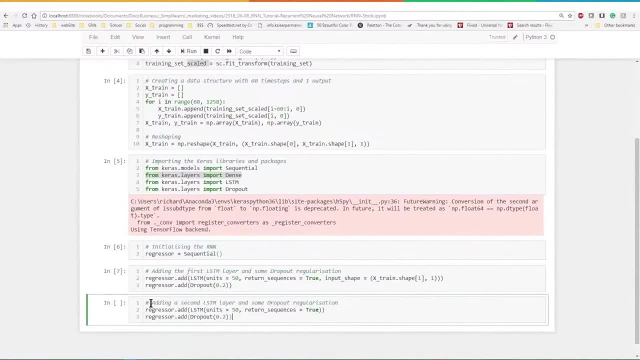 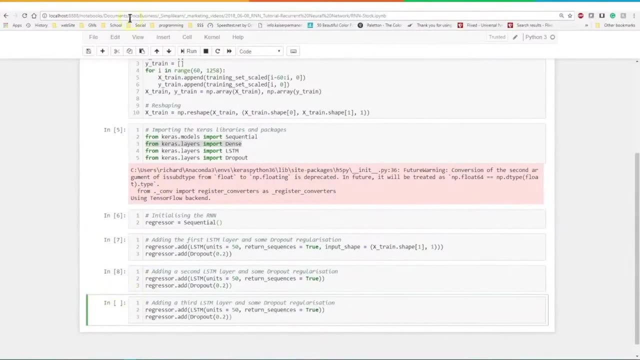 all three of them in, and then we can go back over them. there's the second one, and let's put one more in. let's put that in, and we'll go ahead and put two more in. I meant to, but I said one more in, but it's actually two more in, and then let's 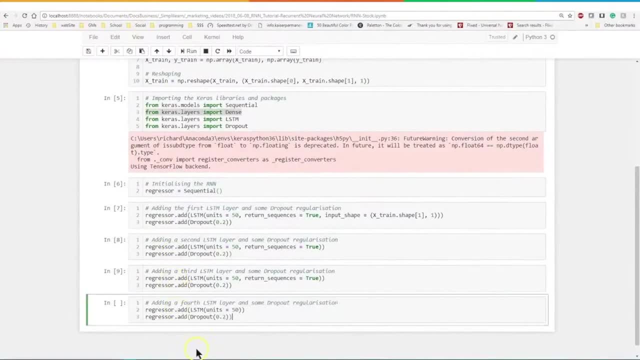 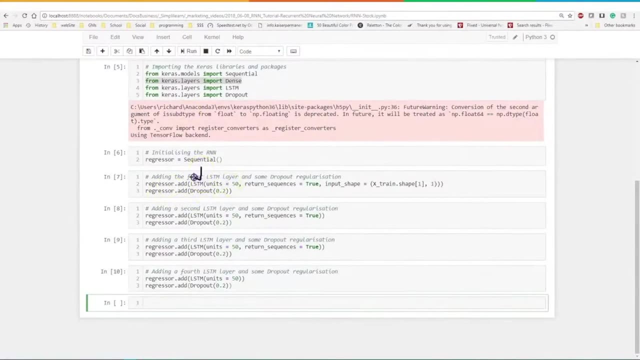 add one more after that and, as you can see, each time I run these they don't actually have an output. so let's take a closer look and see what's going on here. so we're gonna add our first LSTM layer in here. we're gonna have units 50, the 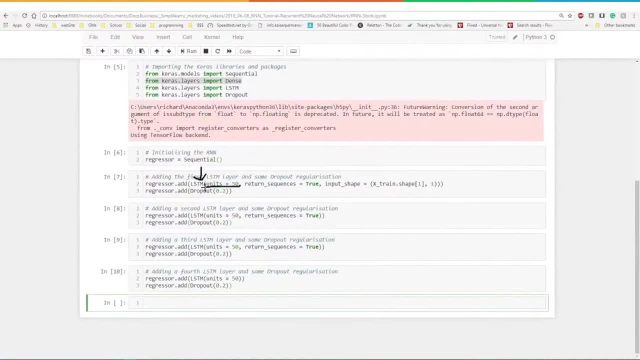 units is the positive integer and it's the dimensionality of the output space. this is what's going out into the next layer, so we might have 60 coming in but we have 50 going out. we have a return sequence because it is a sequence data, so we want 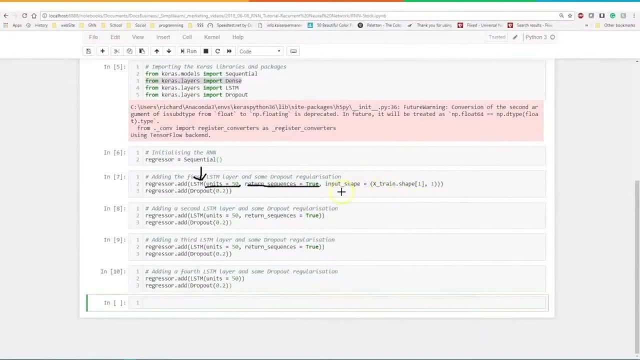 to keep that true. and then you have to tell it what shape it's in. well, we already know the shape by just going in here and looking at X train shape. so input shape equals the X train shape of 1 comma 1. makes it real easy, you don't? 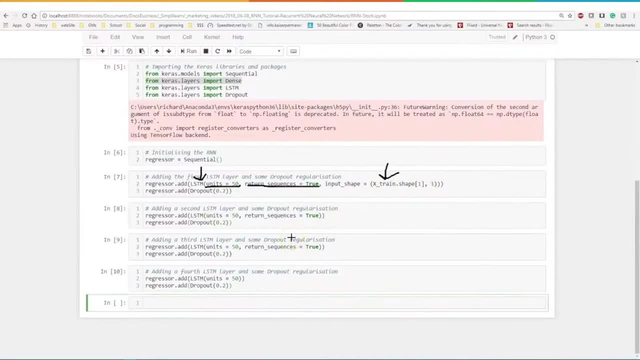 have to remember all the numbers that put in 60 or whatever else is in there. you just let it tell the regressor what model to use and so we follow our STM with a dropout layer. now understanding the dropout layer, it's kind of exciting because one of the things that happens is we can over train our network. 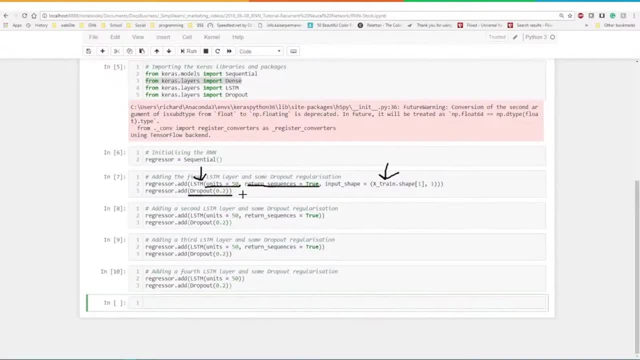 that means that our neural network will memorize such specific data that it has trouble predicting anything that's not in that specific realm. to fix for that, each time we run through the training mode we're going to take point two or twenty percent of our neurons. they just turn them off. so we're only gonna train. 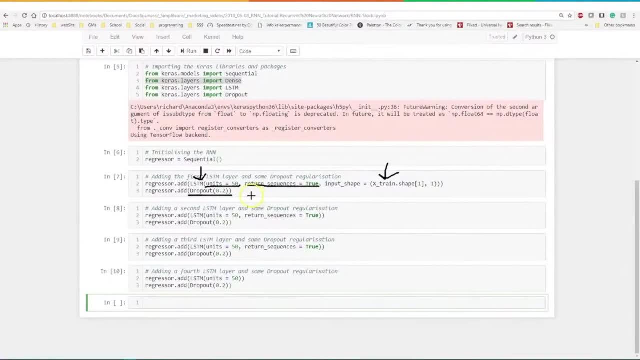 on the other ones and it's gonna be random that way. each time we pass through this we don't over train. these nodes come back in the next training cycle, we randomly pick a different 20. And finally they see a big difference as we go from the first. 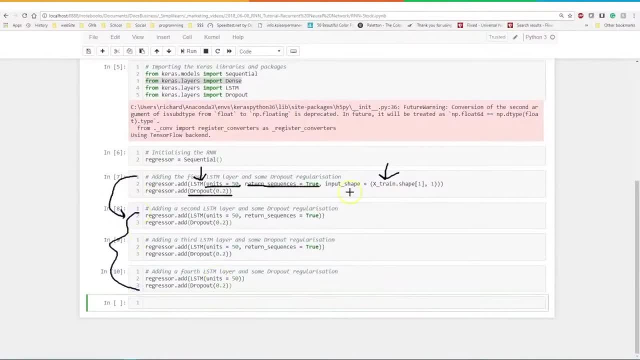 to the second and third and fourth. The first thing is we don't have to input the shape, Because the shape's already. the output units is 50 here. this out of the next step automatically knows this layer is putting out 50. And because it's the next layer, it automatically sets that. and 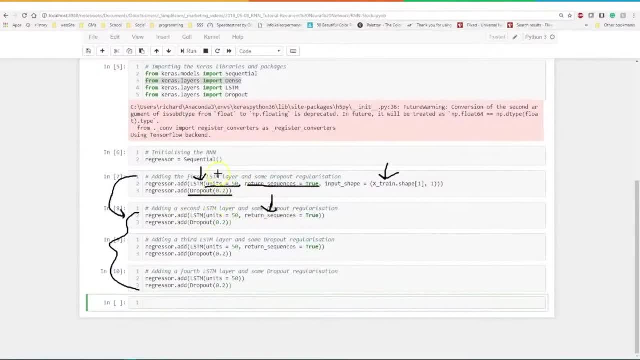 says: oh, 50 is coming out from our last layer. It's coming out, you know, goes into the regressor, and of course we have our dropout And that's what's coming into this one, and so on, and so on. 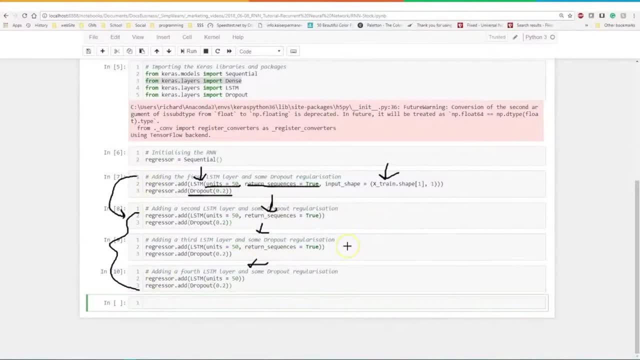 And so the next three layers. we don't have to let it know what the shape is. It automatically understands that And we're going to keep the units the same. We're still going to do 50 units. It's still a sequence coming through 50 units and a sequence. Now the next piece of code is what? 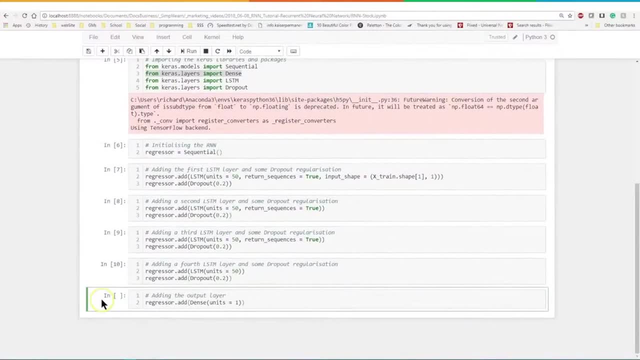 brings it all together. Let's go ahead and take a look at that And we come in here, we put the output layer, the dense layer And, if you remember, up here we had the three layers, We had LSTM, dropout and dense. Dense just says we're going to bring this all down into one output instead of 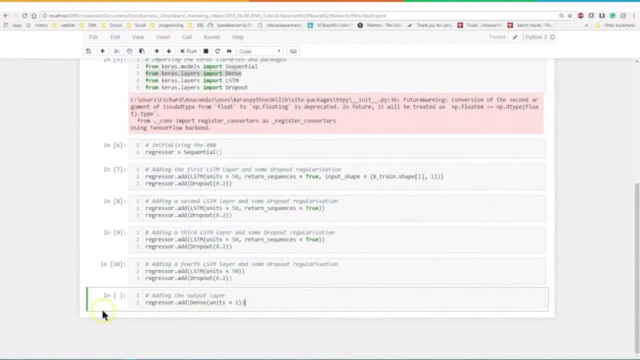 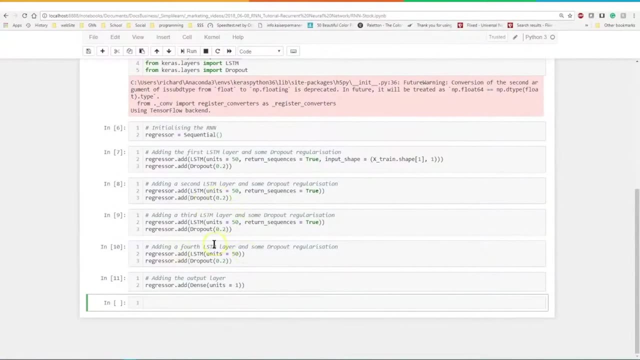 putting out a sequence. We just want to know the answer at this point, And let's go ahead and run that. And so in here you notice, all we're doing is setting things up one step at a time. So far, we've brought in: 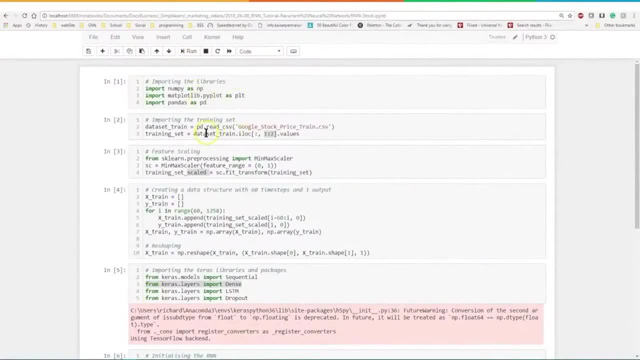 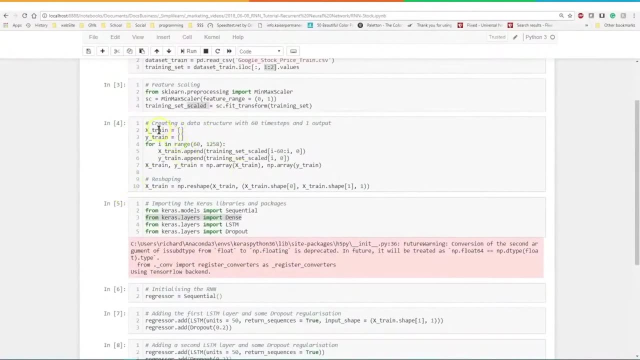 our way up here. We brought in our data, We brought in our different modules. We formatted the data for training it. We set it up. You know we have our YX train and our Y train. We have our source of data and the answers we know so far that we're going to put in there. We've reshaped that, We've 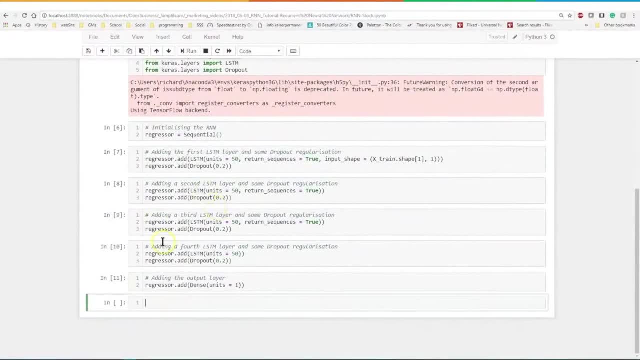 come in and built our cross. We've imported our different layers And we have in here. if you look, we have what? five total layers. Now, Keras is a little different than a lot of other systems, because a lot of other systems put this all in one line and do it. 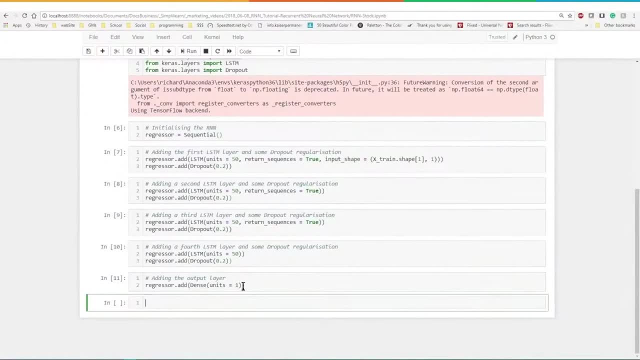 automatic, But they don't give you the options of how those layers interface And they don't give you the options of how the data comes in. Keras is cutting edge for this reason. So, even though there's a lot of extra steps in building the model, this has a huge impact on the output and 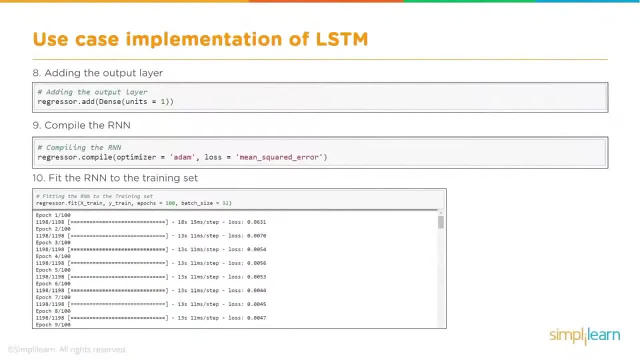 what we can do with these new models from Keras. So we brought in our Ops. We have our full model put together, our regressor, So we need to go ahead and compile it And then we're going to go ahead and fit the data, We're going to compile the pieces. 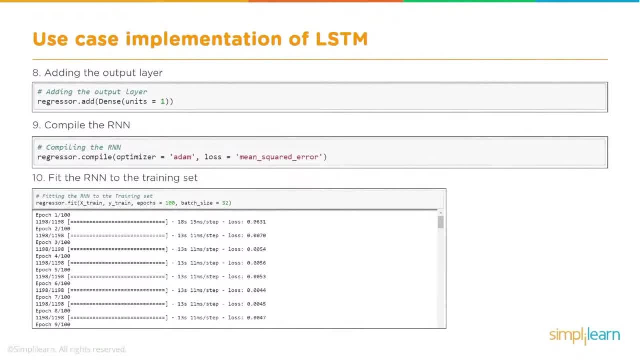 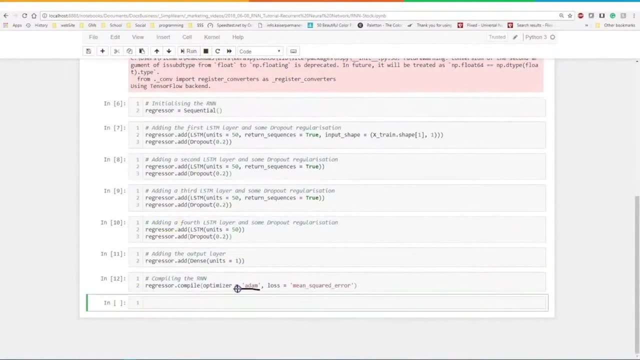 so they all come together and then we're going to run our training data on there and actually recreate our regressor, so it's ready to be used. So let's go ahead and compile that and I can go ahead and run that. And if you've been looking at any of our other tutorials on neural networks, 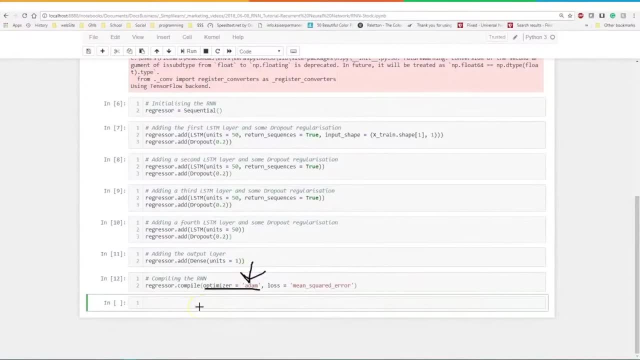 you'll see, we're going to use the optimizer Atom. Atom is optimized for big data. There's a couple other optimizers out there, a couple other optimizers out there beyond the scope of this tutorial, but certainly Adam will work pretty good for this, and loss equals mean squared value. 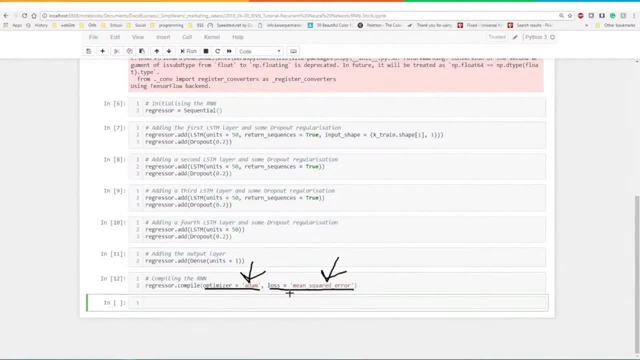 so when we're training it, this is what we want to base the loss on. how bad is our error? we're going to use the mean squared value for our error and the atom optimizer for its differential equations. you don't have to know the math behind them, but certainly it helps to know what they're doing and where they fit into. 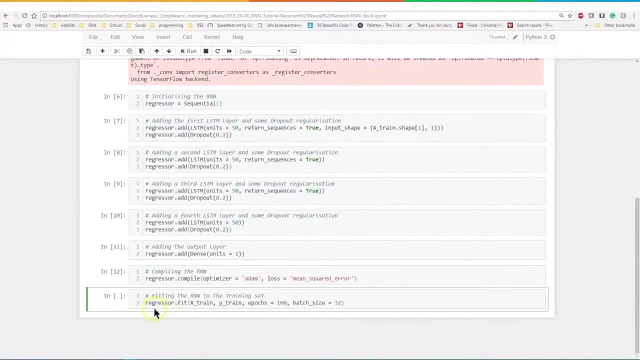 the bigger models. and then, finally, we're going to do our fit, fitting the RNN to the training set. we have the regressor dot fit, x-train, y-train, epics and batch size, so we know where this is. this is our data coming in for the x-train, our y. 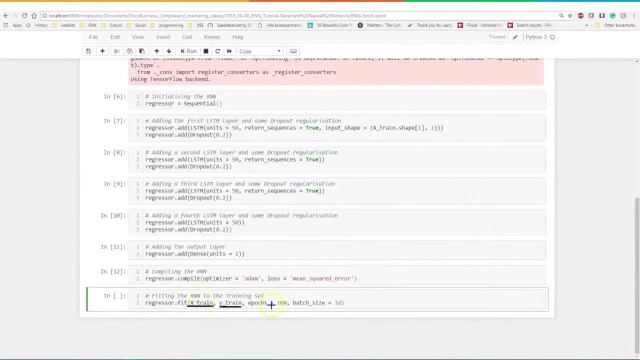 train is the answer we're looking for of our data. our sequential input, epics, is how many times we're going to go over the whole data set. we created a whole data set of x-train, so this is each, each of those rows, which includes a time. 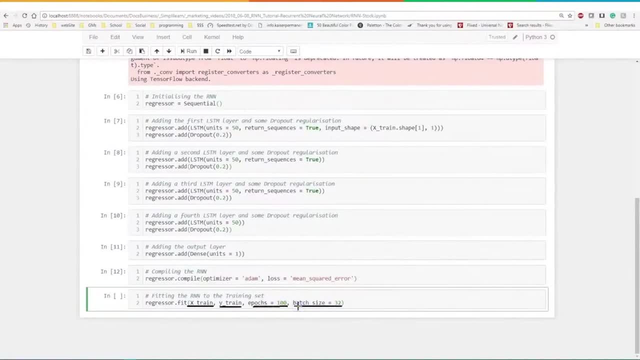 sequence of 60 and batch size. another one of those things were cross really shines is if you were pulling this a from a large file. instead of trying to load it all into RAM, it can now pick smaller batches up and load those indirectly. we're not worried about pulling them off a file today. this isn't big enough to cause the. 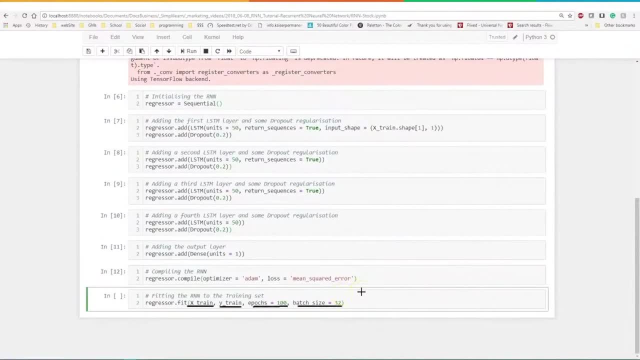 computer too much of a problem to run, not to straining on the resources, but as we run this, you can imagine what happened. I was doing a lot more than just one column in one set of stock, in this case Google stock. imagine if I was doing this across all the stocks and I had, instead of just the open, I had open. 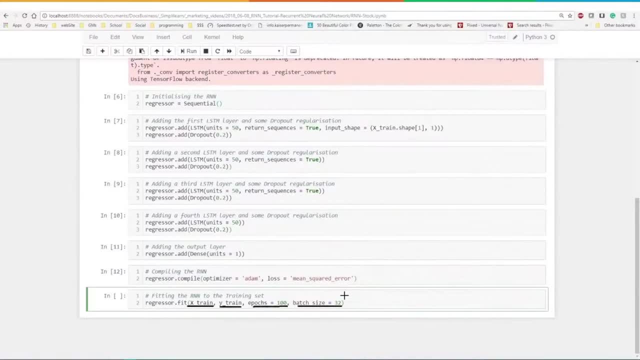 close. you can actually find yourself with about thirteen different variables, times sixty, X's a time sequence, suddenly find yourself with a gig of memory loading into your RAM which will just completely- you know if it's just, if you're not on multiple computers or cluster- start running into resource problems. but for 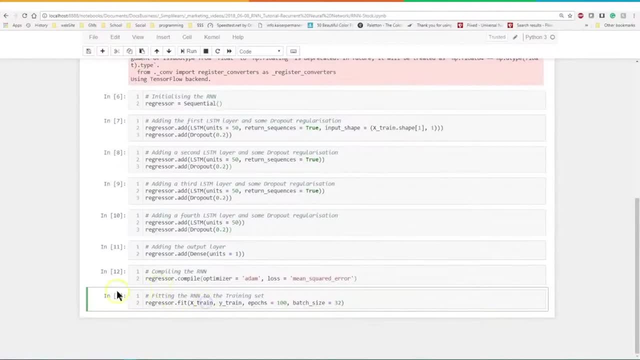 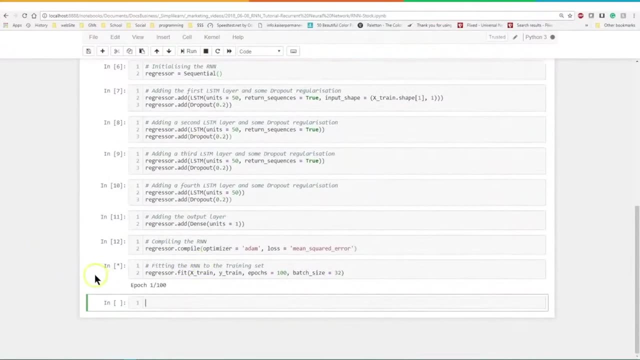 this, we don't have to worry about that. so let's go ahead and run this, and this will actually take a little bit of my computer is an older laptop. give a second to kick in there. there we go, alright, so we have epic. so this is gonna. 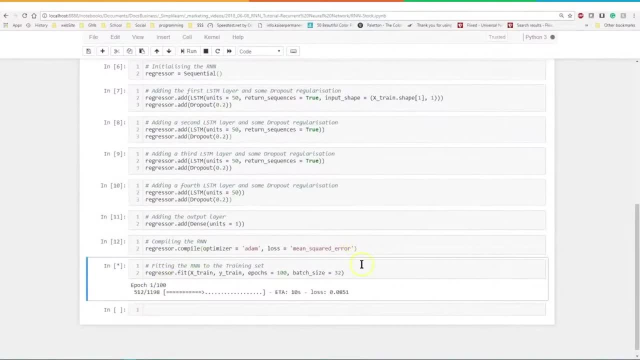 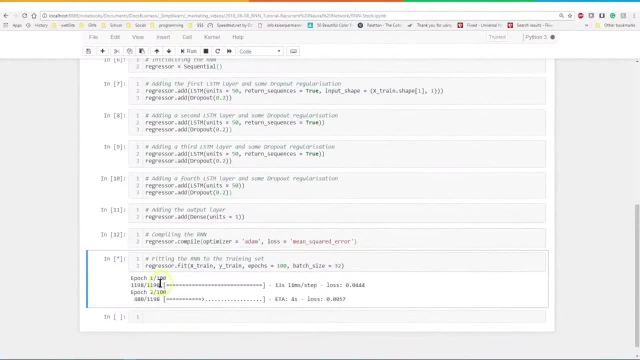 tell me it's running the first run through all the data And as it's going through, it's batching them in 32 pieces, So 32 lines each time And there's 1198.. I think I said 1199 earlier, but 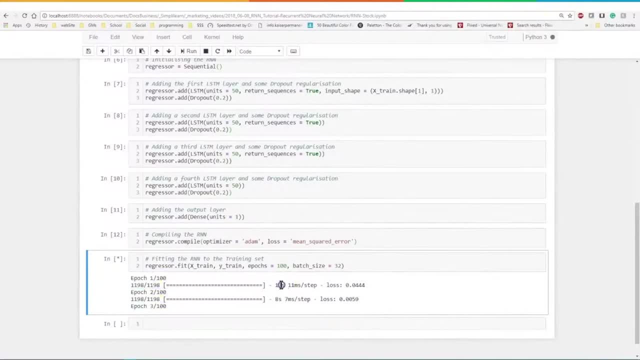 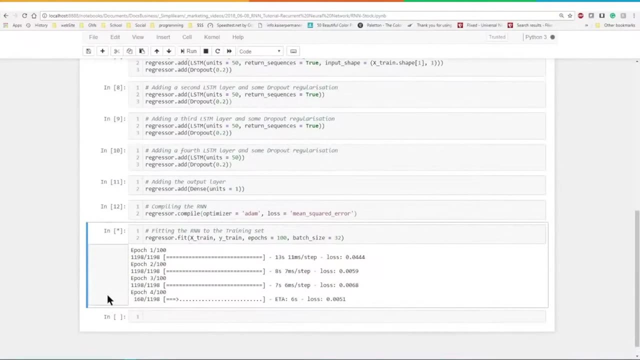 it's 1198.. I was off by one And each one of these is 13 seconds, So you can imagine this is roughly 20 to 30 minutes runtime on this computer. Like I said, it's an older laptop running at 0.9 gigahertz. 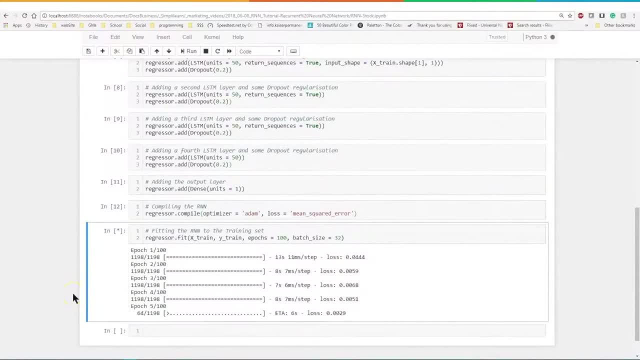 on a dual processor, And that's fine. What we'll do is: I'll go ahead and stop, go get a drink of coffee and come back And let's see what happens at the end and where this takes us. And, like any, 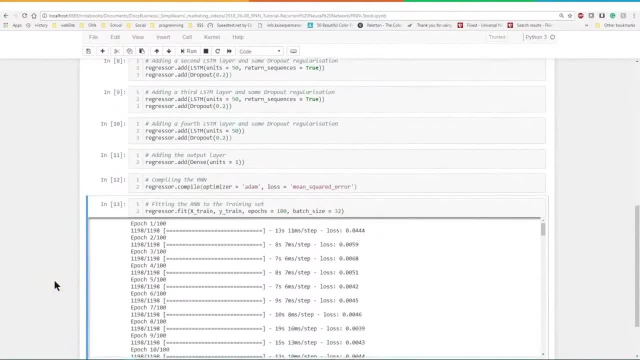 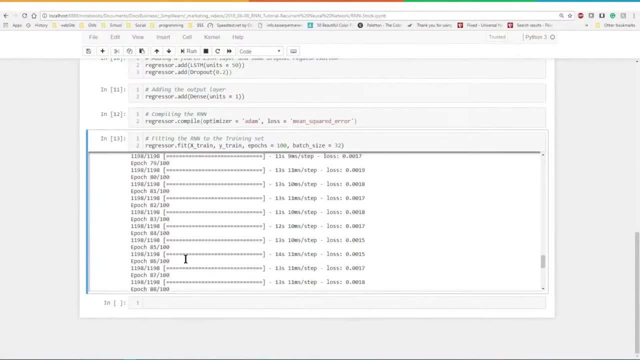 good cooking show. I've kind of gotten my latte. I also had some other stuff running in the background, So you'll see these numbers jumped up to like 19 seconds- 15 seconds, But you can scroll through and you can see we've run it through 100 steps or 100 epics. So the question is: what does? 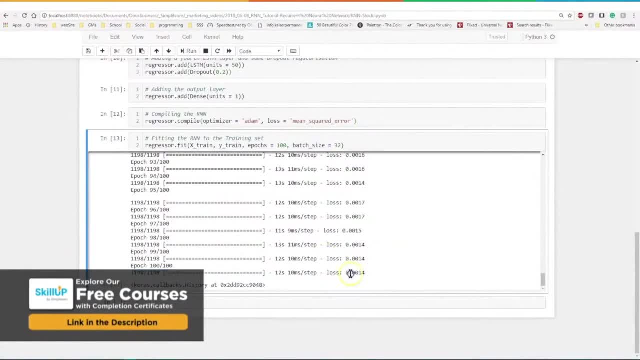 all this mean? One of the first things you'll notice is that our loss is over here. It kind of stopped at 0.0014, but you can see it kind of goes down until we hit about 0.014 three times in a row. 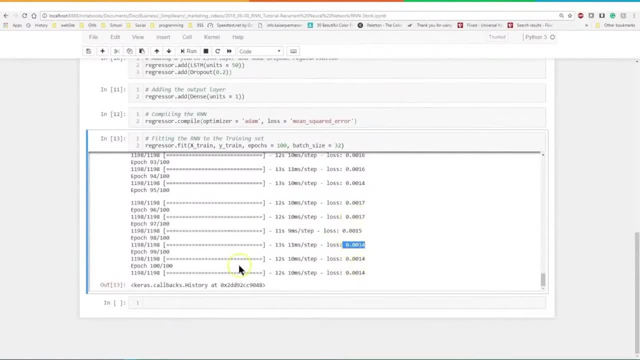 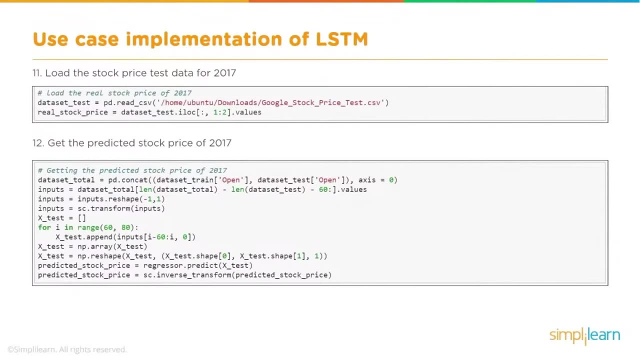 So we guessed our epic Pretty close, since our loss has remained the same on there. So to find out what we're looking at, we're going to go ahead and load up our test data- the test data that we didn't process yet, And a 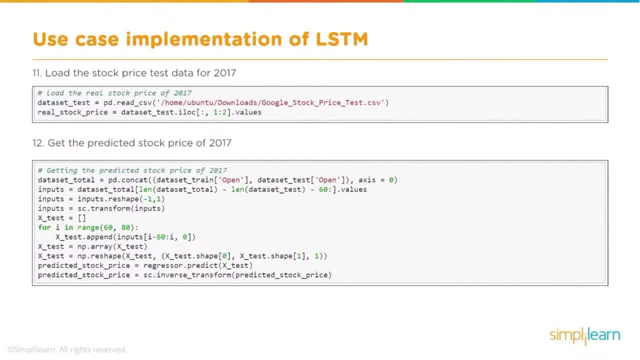 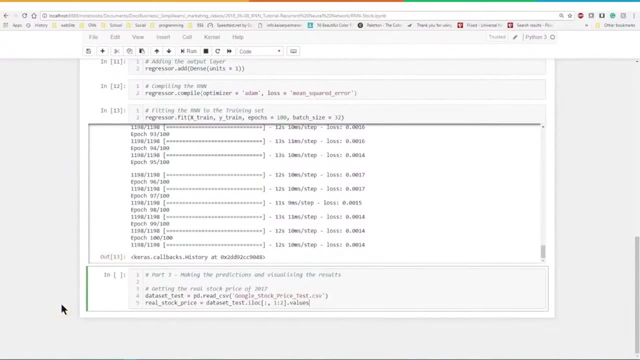 real stock price data set test allocation. This is the same thing we did when we prepped the data in the first place. So let's go ahead and go through this code And we can see. we've labeled it. part three: making the predictions and visualizing the results. So the first thing we need to do is go. 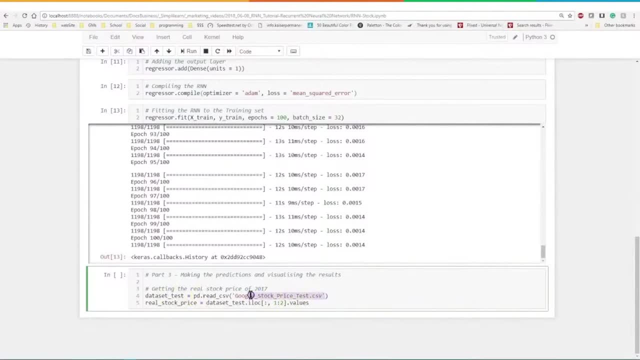 ahead and read the data in from our test CSV And you see, I've changed the path on there And we're going to call it the real stock price. And we're going to call it the real stock price And again we're doing just the one column here and the values from I location, So it's all the rows and 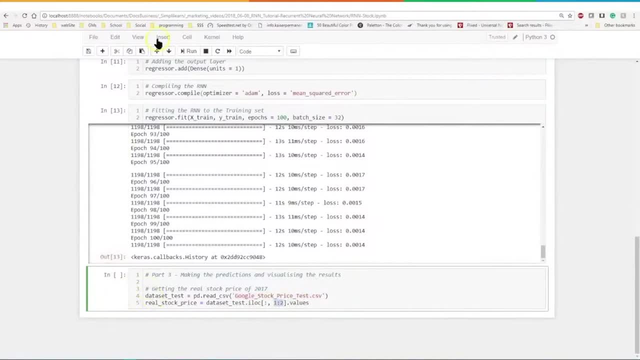 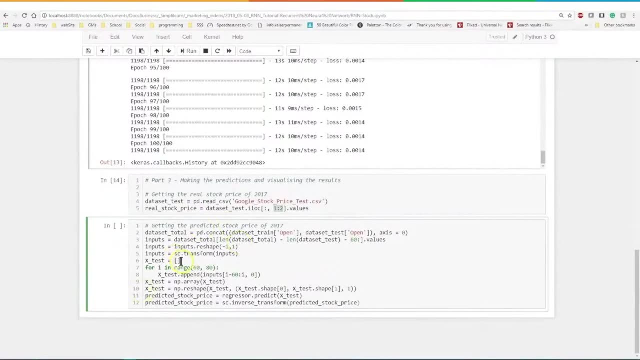 just the values from these, that one location- That's the open stock- open. Let's go ahead and run that, So that's loaded in there, And then let's go ahead and create. we have our inputs, we're going to create inputs here, And this should all look familiar because this is the same thing we 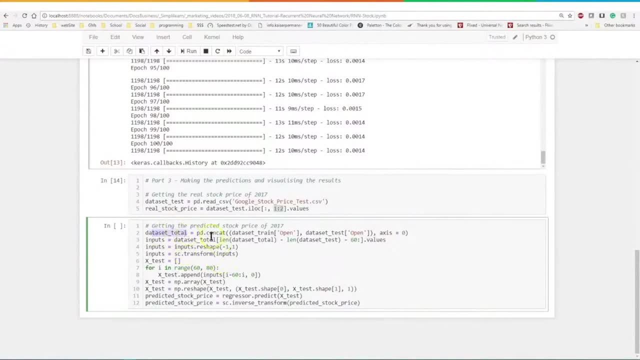 did before. we're going to take our data set total. we're going to do a little pandas can cap from the dataset train. Now, remember, the end of the dataset train is part of the data going in And let's just visualize that just a little bit. Here's our train data. Let me just put tr for train And. 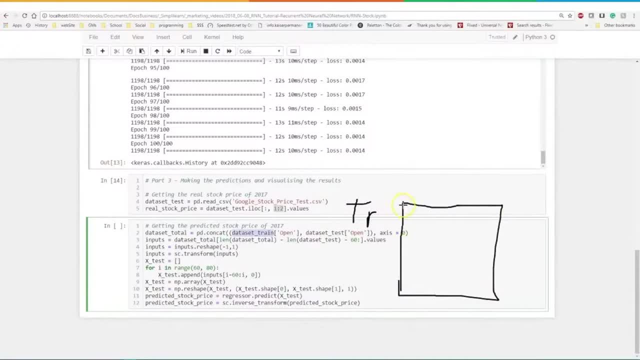 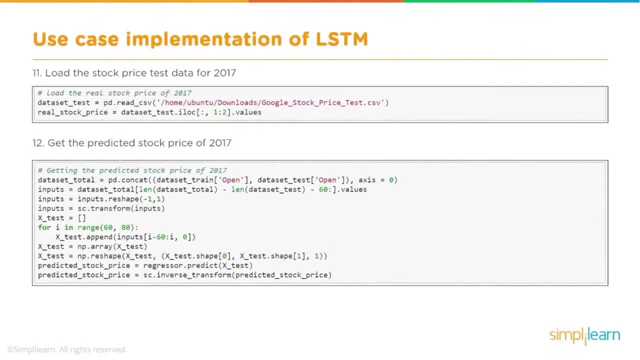 it went up to this value here, But each one of these values generated a bunch of columns, So it's 60 across, And this value here equals this one, And this value here equals this one, And this value here equals this one, And so we need these top 60 to go into our new data, So to find out what we're. 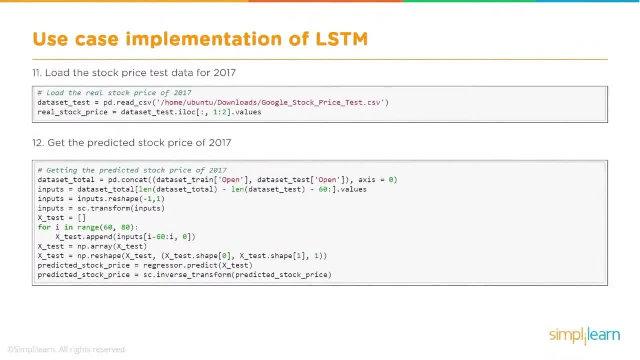 looking at. we're going to go ahead and load up our test data, the test data that we didn't process yet, And a real stock price dataset, test allocation. This is the same thing we did when we prepped the data in the first place. So let's go ahead and go through this code And we can see we've labeled it. 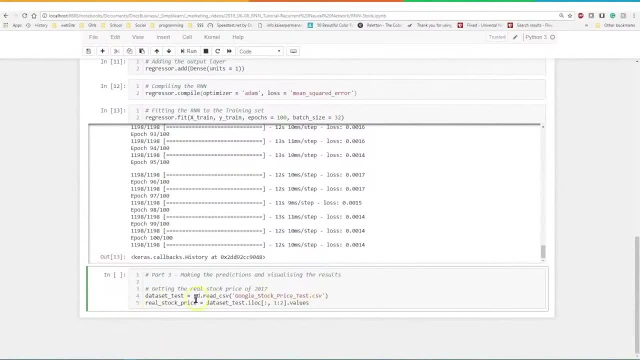 part three, making the predictions and visualizing the results. So the first thing we need to do is go ahead and read the data in from our test CL- And you see, I've changed the path on it for my computer- And then we'll call it the real stock price. 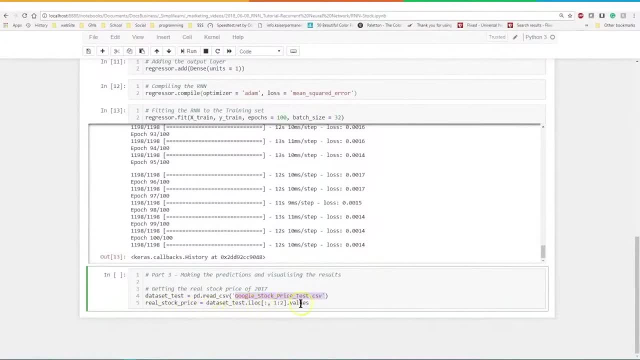 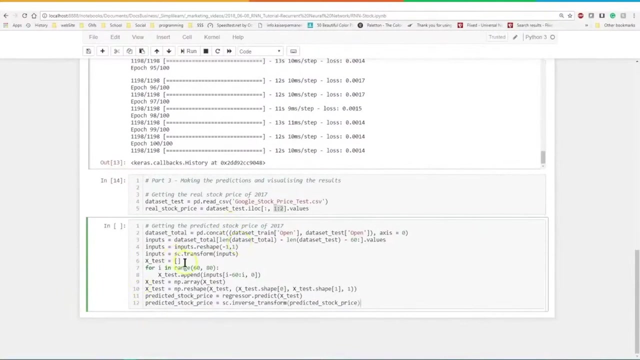 And again we're doing just the one column here and the values from iLocation. So it's all the rows and just the values from these. that one location, That's the open stock open, And let's go ahead and run that, So that's loaded in there, And then let's go ahead and create. we have our inputs, We're going to. 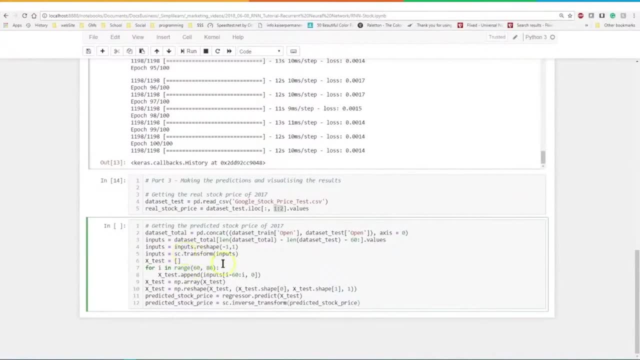 create inputs here, And this should all look familiar because this is the same thing we did before. We're going to take our data set total. We're going to do a little pandas concat from the data set train. Now remember the end of the data set. 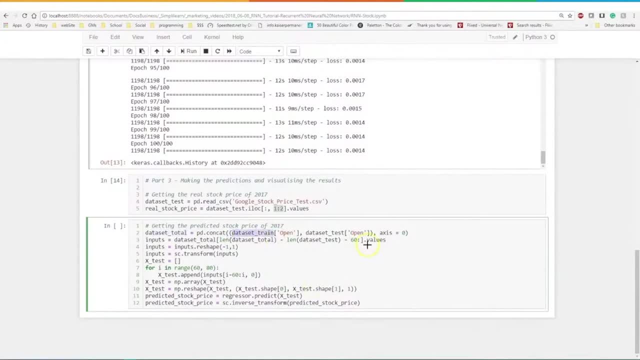 train is part of the data going in, And let's just visualize that just a little bit. Here's our train data. Let me just put tr for train And it went up to this value here, But each one of these values generated a bunch of columns, So it was 60 across And this value here equals this one And this. 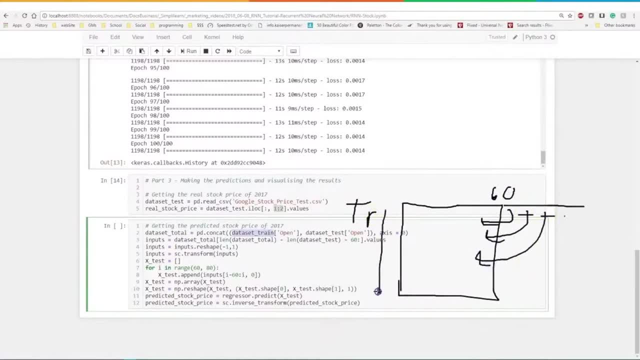 value here equals this one, And this value here equals this one, And so we need these top 60 to go into our new data, Because that's part of the next data, Or it's actually the top 59. So that's what this. 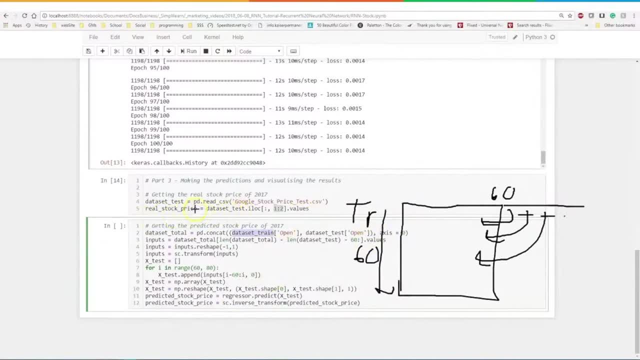 first setup is over. here Is we're going in, we're doing the real stock price And we're going to just take the data set test And we're going to load that in And then the real stock price is our data test, dot test. 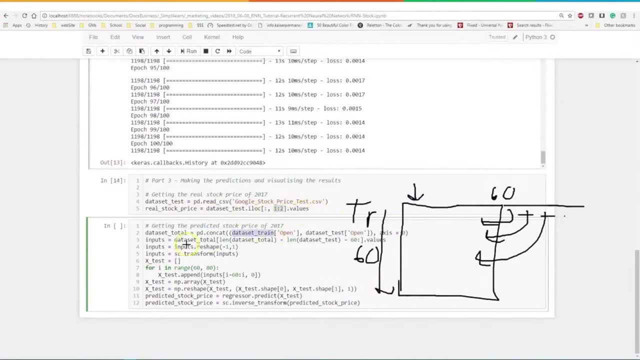 location. So we're just looking at that: first column, the open price And then our data set total. we're going to take pandas and we're going to concat And we're going to take our data set train for the open and our data set test open And this is one way you can reference these values. So let's go ahead and run. 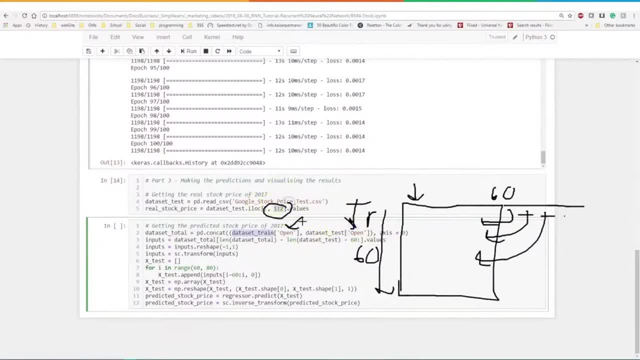 these columns. We've referenced them a couple different ways. We've referenced them up here with the one two, But we know it's labeled as a pandas set, as open. So pandas is great that way. Lots of versatility there. And we'll go ahead and go back up here and run this. There we go And you'll notice this is the same. 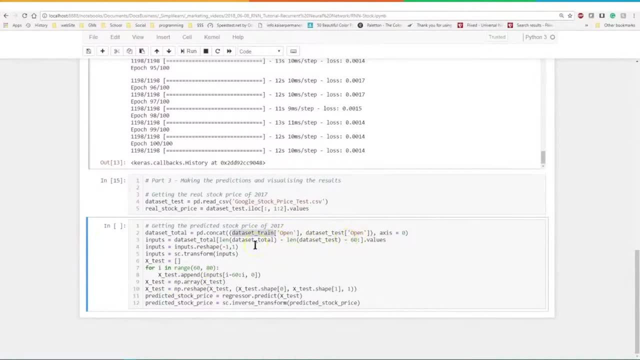 as what we did before. We have our open data set. We've pended our two different or concatenated our two data sets together. We have our inputs: equals data set, total length, Data set total minus length of data set, minus test minus 60 values. So we're going to run this over all of them And you'll see why. 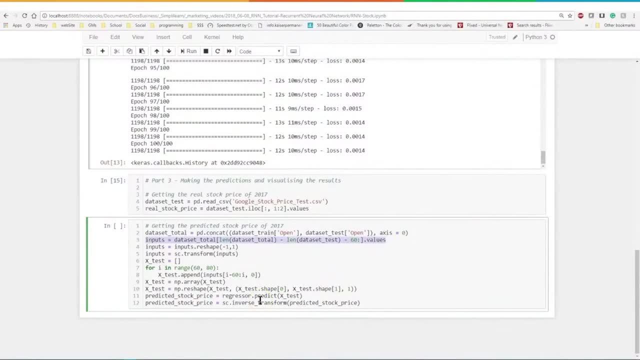 this works Because normally when you're running your test set versus your training set, you run them completely separate. But when we graph this, you'll see that we're just going to be looking at the part that we didn't train it with to see how well it graphs, And we have our inputs equals inputs dot reshapes. 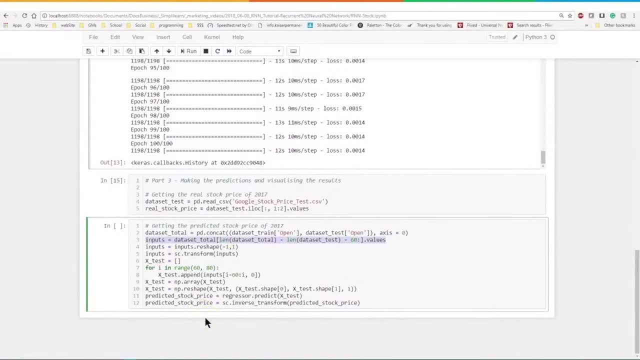 or reshaping like we did before. We're transforming our inputs. So if you remember, from the transform between zero and one, And finally we want to go ahead and take our X test And we're going to create that X test And for i, in range 60 to 80.. 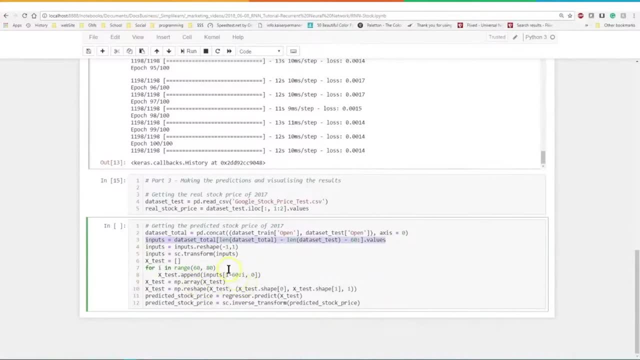 So here's our X test And we're appending our inputs i to 60, which, remember, is zero to 59. And i comma zero on the other side. So it's just the first column which is our open column And once again, we take our X test, We convert it. 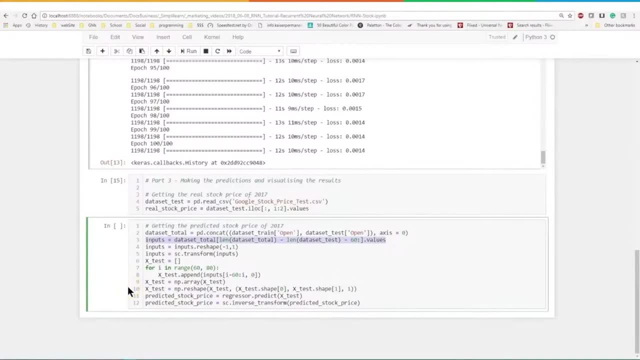 to a numpy array. We do the same reshape we did before, And then we get down to the final two lines, And here we have something new, Right here on these last two lines, Let me just highlight those or mark them. Predicted stock price equals regressor dot. predicts X test. So we're predicting all the stock. 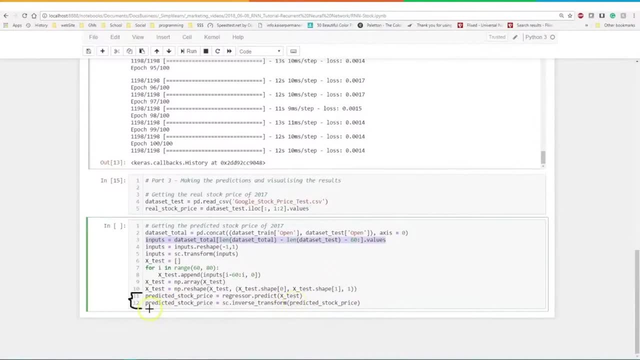 including both the training And the testing model here. And then we want to take this prediction And we want to inverse the transform. So, remember, we put them between zero and one. Well, that's not going to mean very much to me to look at a. 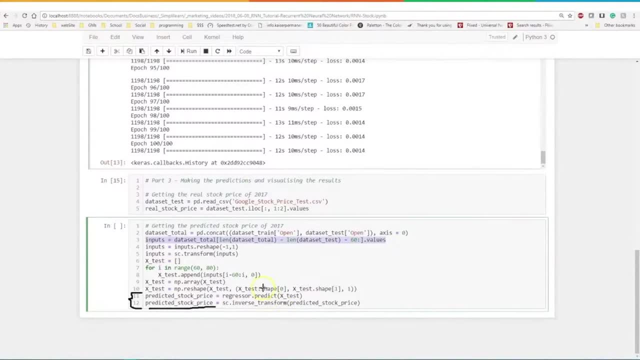 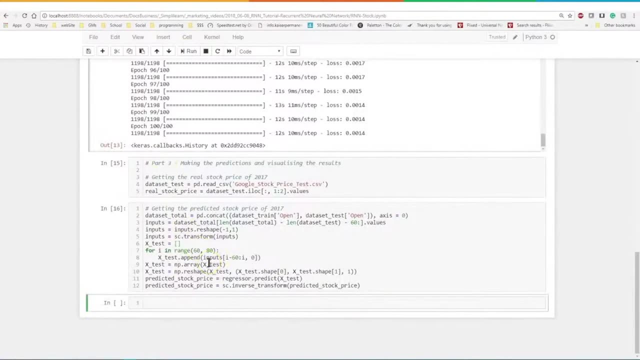 float number between zero and one. I want the dollar amounts, I want to know what the cash value is, And we'll go ahead and run this And you'll see it runs much quicker than the training. That's what's so wonderful about these neural networks: Once you put them together, it takes just a second to run the same neural 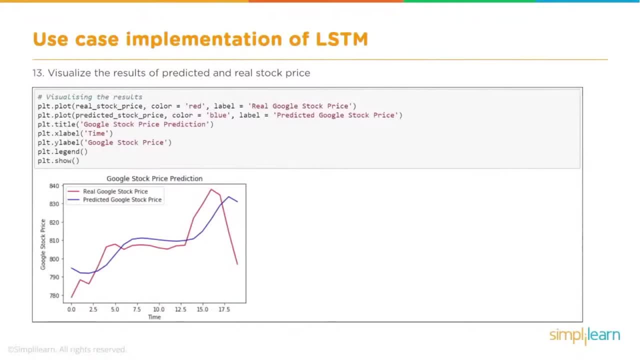 network. that took us what a half hour to train And plot the data. We're going to plot what we think it's going to be And we're going to plot it against the real data- What the Google stock actually did. So let's go ahead and take a look at that in code. 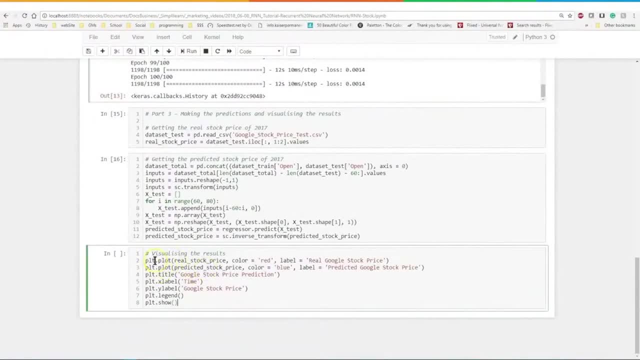 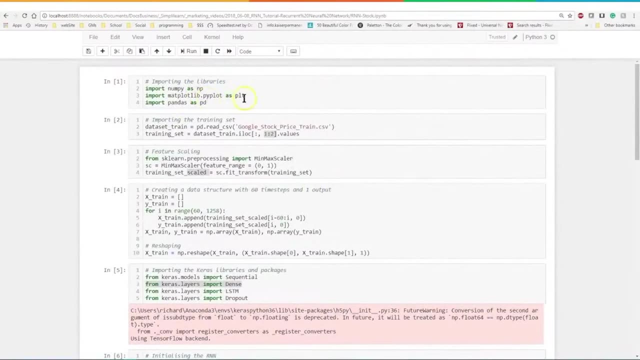 And let's pull this code up. So we have our PLT. That's our. oh, if you remember from the very beginning, Let me just go back up to the top. We have our matplotlibrarypiplot as PLT. That's where that comes in And we come down here We're going to plot. Let me get my. 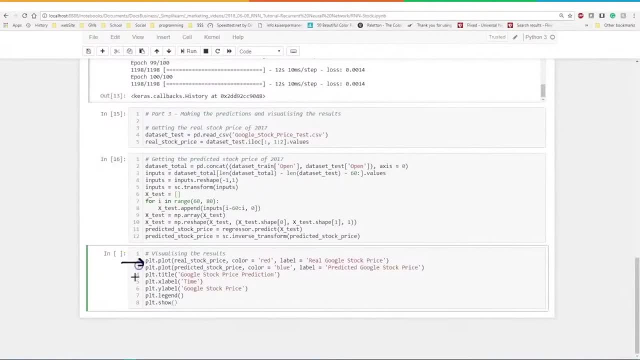 drawing thing out again. We're going to go ahead And PLT is basically kind of like an object. It's one of the things that always threw me when I'm doing graphs in Python, Because I always think you have to create an object And then it loads that class in there. Well, in this case, PLT is like a canvas, you're. 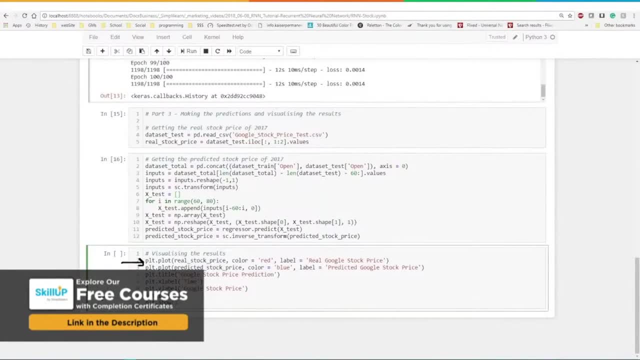 putting stuff on. So if you've done HTML5, you'll have the canvas object. This is the canvas, So we're going to plot the real stock price- That's what it actually is- And we're going to give that color red, So it's going to be a bright red And we're going to label it real Google. 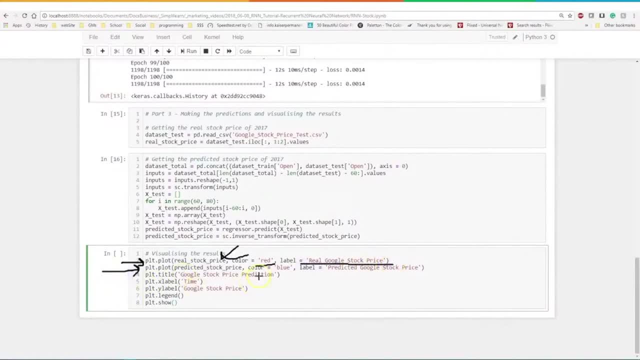 stock price And then we're going to do our predicted stock And we're going to do it in blue And it's going to be labeled predicted And we'll give it a title. It's always nice to give a title To your graph, Especially if you're going to present this to somebody, to your shareholders in the office, And the X label is going to be time. 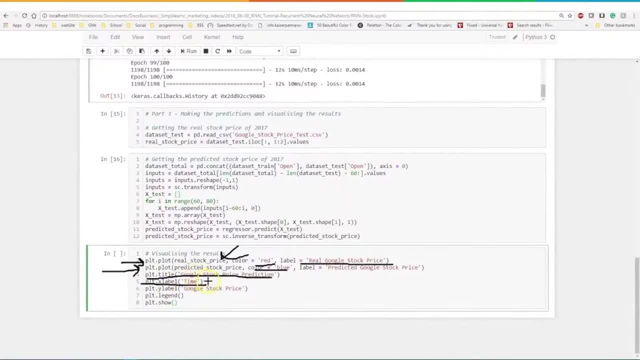 Because it's a time series And we didn't actually put the actual date and times on here. But that's fine, We just know they're incremented by time. And then, of course, the Y label is the actual stock price. PLTLegend tells us to build the legend on here, So that the color red and real 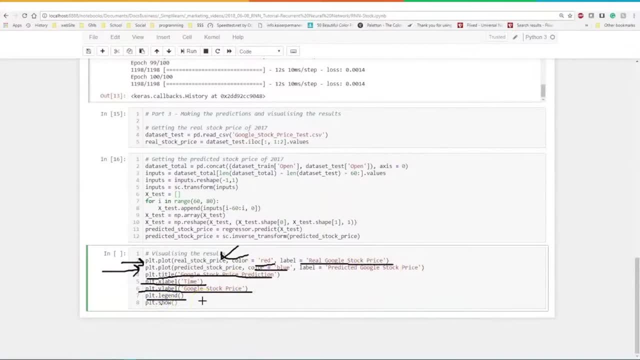 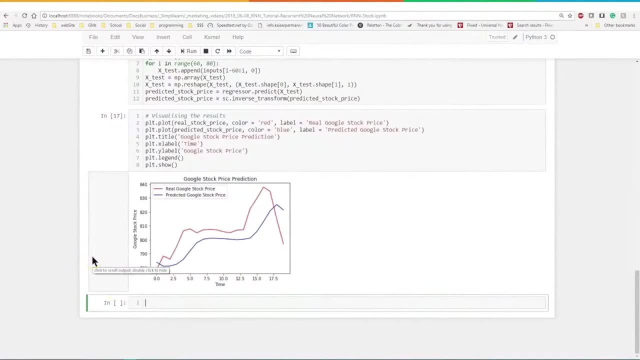 Google stock price show up on there And then the plot shows us that actual graph. So let's go ahead and run this and see what that looks like, And you can see, here we have a nice graph. And let's talk just a little bit about this graph before we wrap it up. Here's our legend. I was 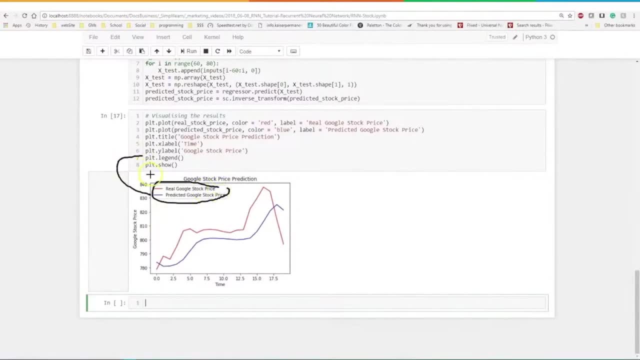 telling you about. That's why we have the legend to show the prices. We have our title and everything, And you'll notice on the bottom we have a time sequence. We didn't put the actual time in here. Now we could have. We could have gone ahead and plotted the X, since we know what the dates are. 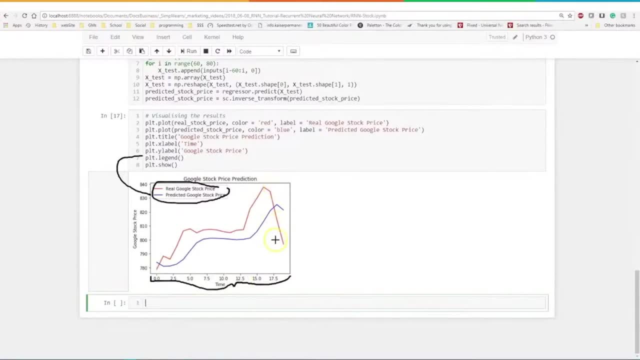 And plotted this to dates, But we also know that it's only the last piece of data that we're looking at. So last piece of data which ends somewhere, probably around here on the graph, I think it's like about 20% of the data, Probably less than that. We have the Google price And the Google price has this: 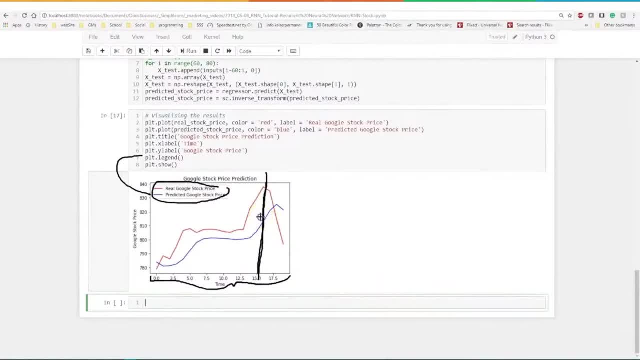 little up jump and then down And you'll see that the actual Google, instead of a turn down here, just didn't go up as high and didn't go down. So our prediction has the same pattern, But the overall value is pretty far off as far as stock. But then again, we're only looking at one column, We're only 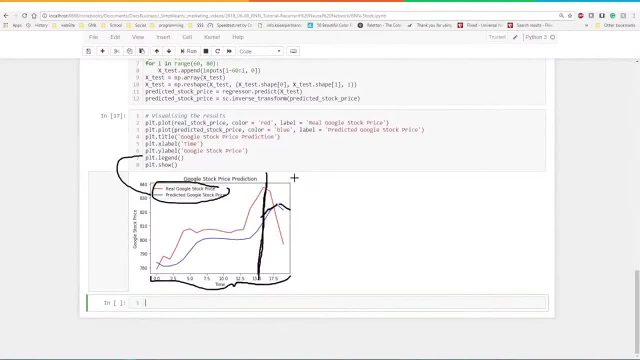 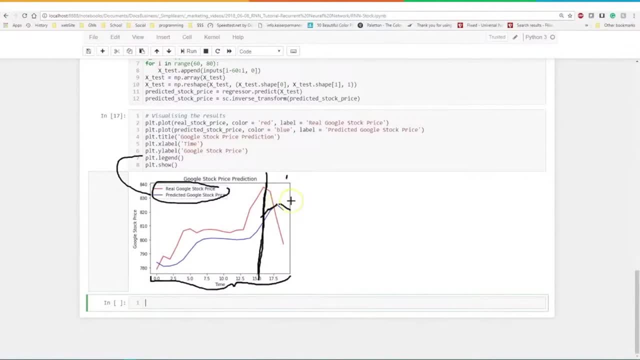 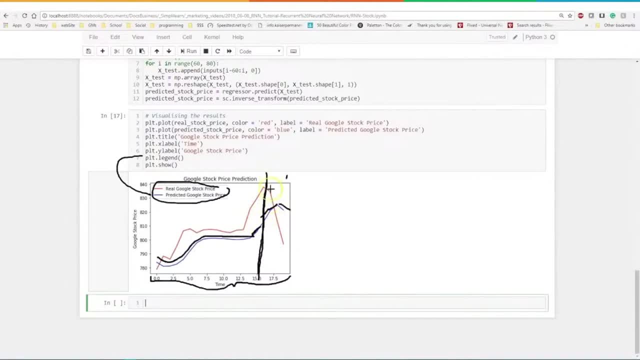 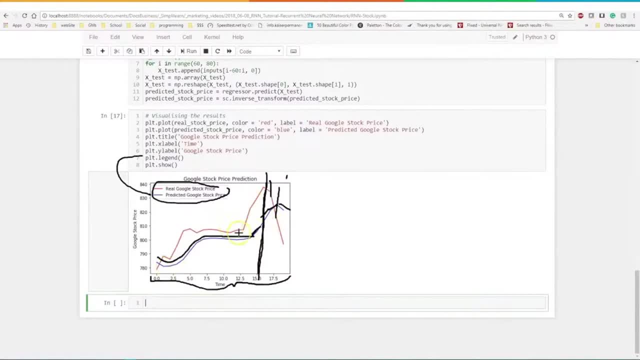 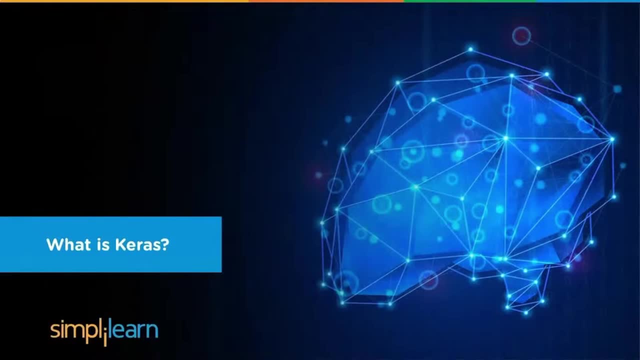 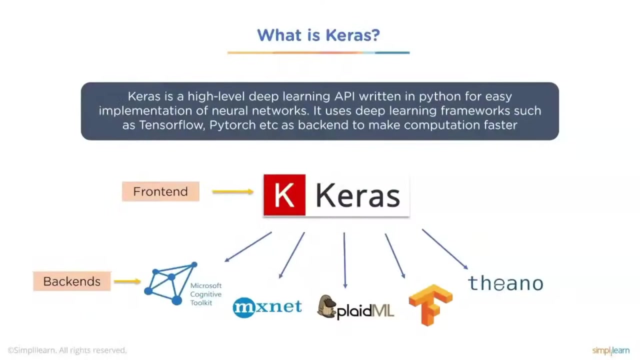 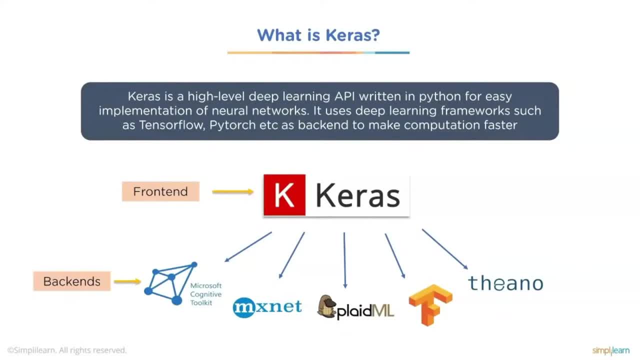 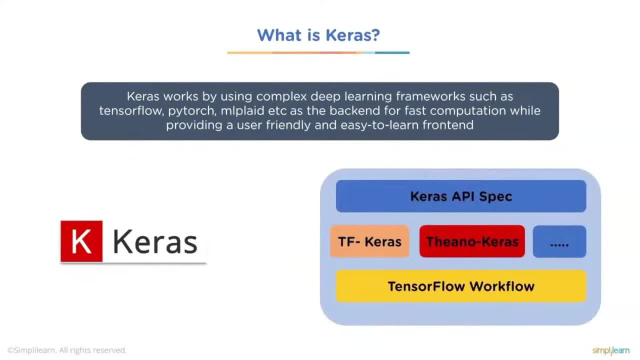 So Keras works by using complex deep learning frameworks such as TensorFlow, PyTorch, ML, Played, etc. as a backend for fast computation while providing a user-friendly and easy-to-learn front-end. And you can see, here we have the Keras API specifications and under that you'd have, like TF Keras for TensorFlow, Thano Keras and so on, And then you have your TensorFlow workflow that this is all sitting on top of. 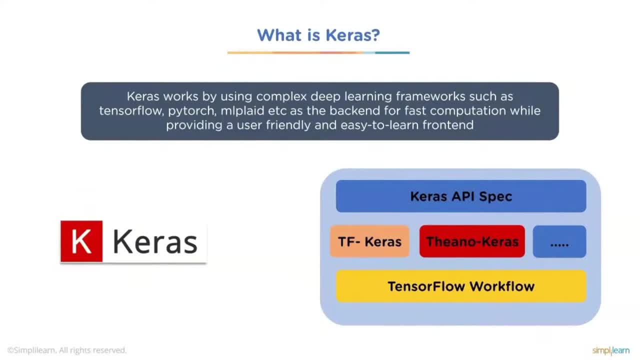 And this is like I said. it organizes everything. The heavy lifting is still done by TensorFlow or whatever you know underlying package you put in there, And this is really nice because you don't have to dig as deeply into the heavy end stuff while still having a very robust package. you can get up and running rather quickly. 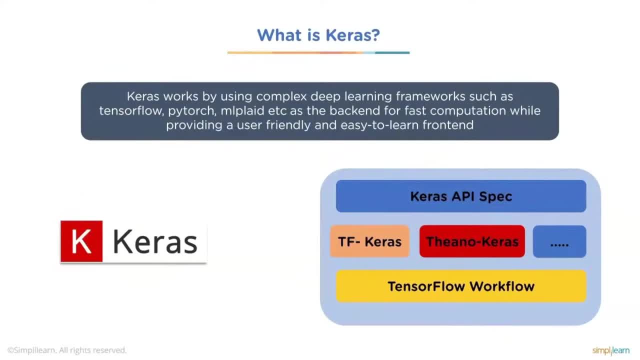 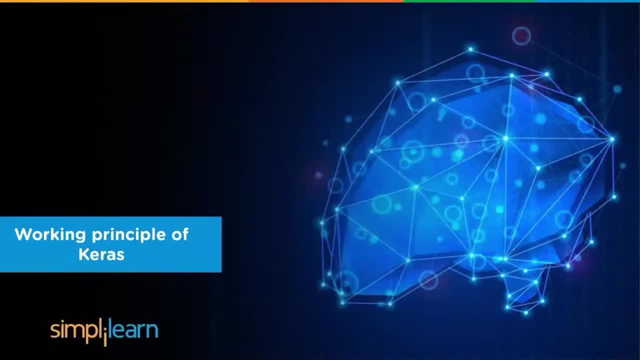 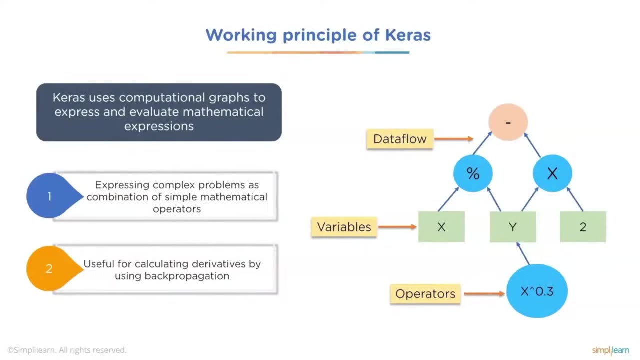 And it doesn't distract from the processing time, because all the heavy lifting is done by packages like TensorFlow. This is the organization on top of it. So the working principle of Keras, The working principle of Keras is: Keras uses computational graphs to express and evaluate mathematical expressions. 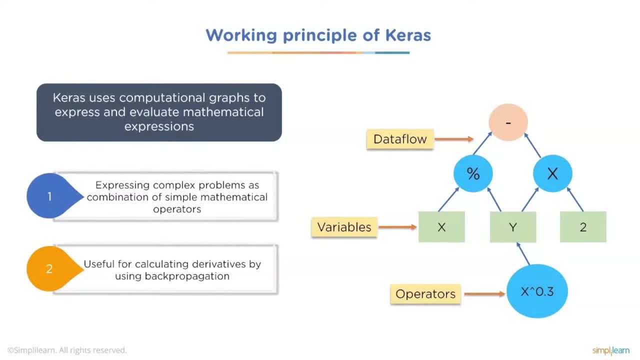 And you can see here we put it in blue- they have the expression expressing complex problems as a combination of simple mathematical operators. where we have, like the percentage- or in this case in Python that's usually your remainder or multiplication, You might have the operator of x. 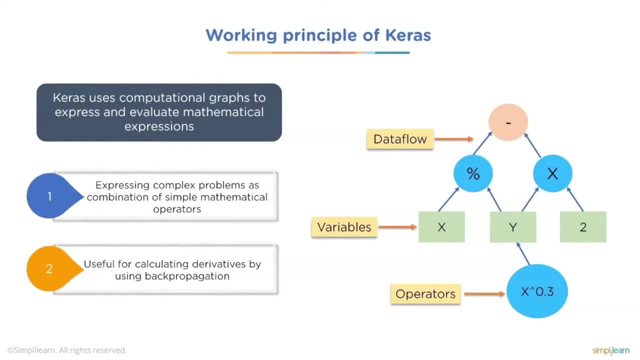 You might have the operator of x to the power of 0.3.. And it is useful for calculating derivatives by using back propagation. So if we're doing it with neural networks, we send the error back up to figure out how to change it. 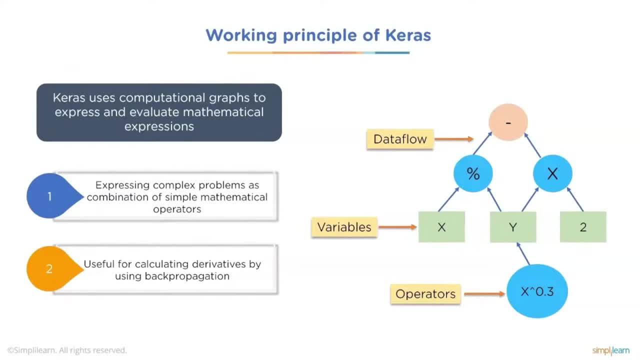 This makes it really easy to do that without really having not banging your head and having to handwrite everything. It's easier to implement distributed computation And, for solving complex problems, specify input and outputs and make sure all nodes are connected, And so this is really nice. as you come in through is that, as your layers are going in there, you can get some very complicated, different setups nowadays, which we'll look at in just a second. 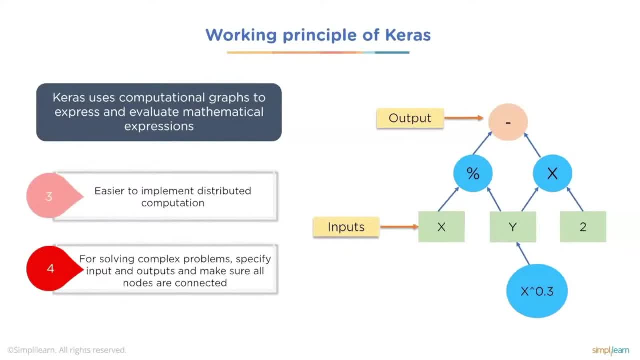 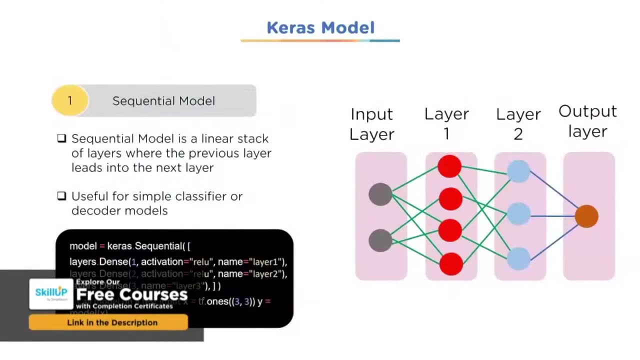 And this just makes it really easy to start spinning this stuff up and trying out the different models. So we look at Keras models. Keras model we have a sequential model. Sequential model is a linear stack of layers where the previous layer leads into the next layer. 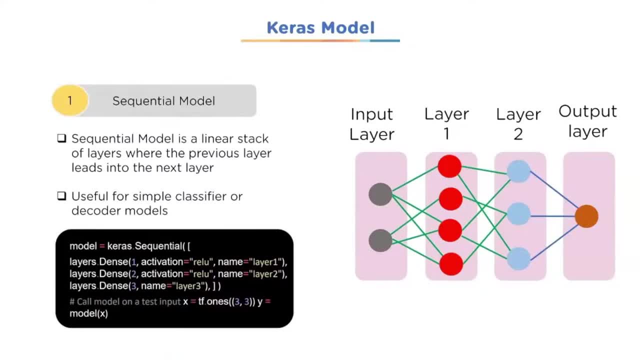 And this: if you've done anything else, even like the sklearn with their neural networks and propagation and any of these setups- this should look familiar. You should have your input layer. it goes into your layer 1,, layer 2, and then to the output layer. 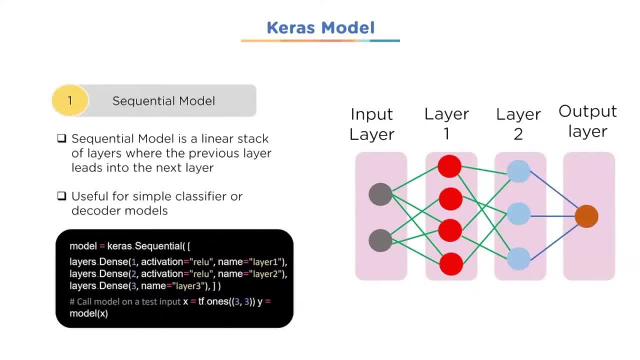 And it's useful for simple classifier decoder models And you can see down here we have the model: equals across sequential. This is the actual code. You can see how easy it is. We have a layer that's dense. Your layer 1 has an activation. 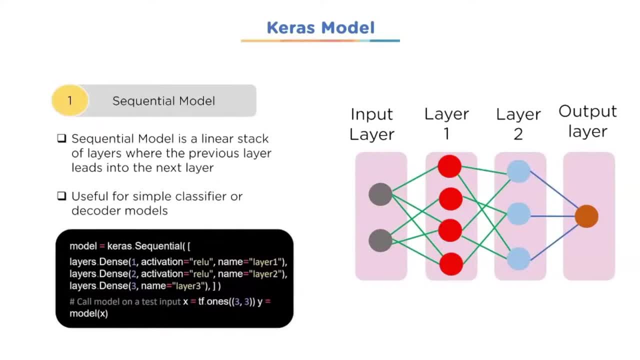 They're using the ReLU in this particular example- And then you have your name, layer 1, layer dense ReLU name, layer 2, and so forth, And they just feed right into each other. So it's really easy just to stack them, as you can see here, and it automatically takes care of everything else for you. 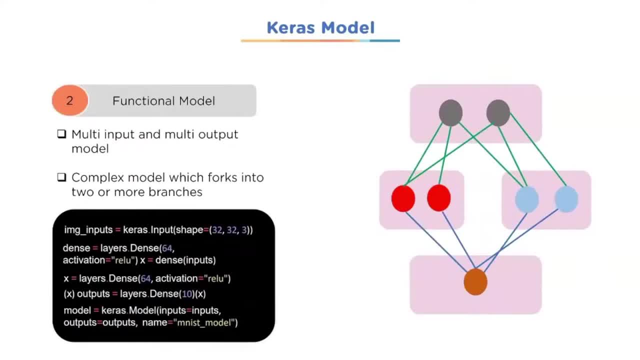 And then there's a functional model, And this is really where things are at. This is new. Make sure you update your Keras or you'll find yourself running this doing the functional model. You'll run into an error code because this is a fairly new release. 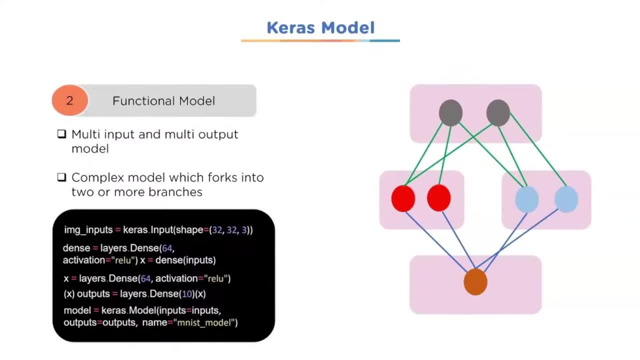 And it uses multi-input and multi-output model. The complex model which forks into two or more branches- And you can see- here we have our image- inputs equals your Keras input shape equals 32 by 32 by 3.. You have your dense layers: dense 64, activation ReLU. 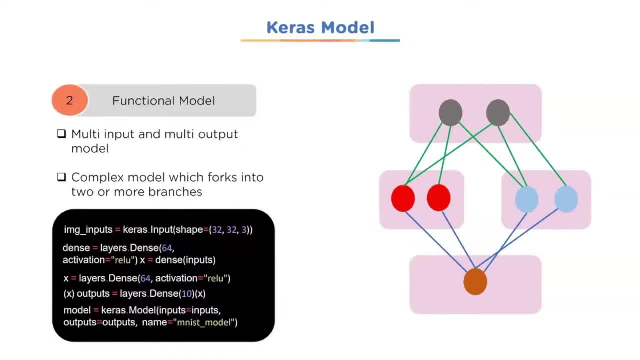 This should look similar to what you already saw before, But if you look at the graph on the right, it's going to be a lot easier to see what's going on. You have two different inputs And one way you can think of this is: maybe one of those is a small image and one of those is a full-sized image. 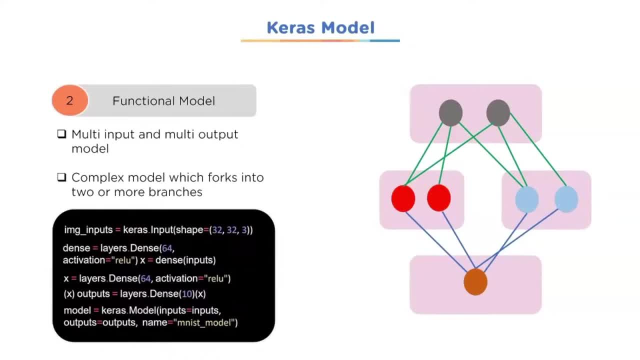 And that feedback goes into. you might feed both of them into one node, because it's looking for one thing, And then only into one node for the other one, And so you can start to get kind of an idea that there's a lot of use for this kind of split and this kind of setup. 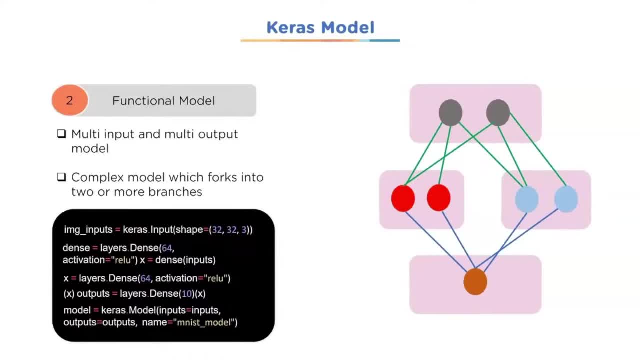 We have multiple information coming in, but the information is very different, even though it overlaps, And you don't want it to send it through the same neural network. And they're finding that this trains faster and also has a better result, Depending on how you split the data up and how you fork the models coming down. 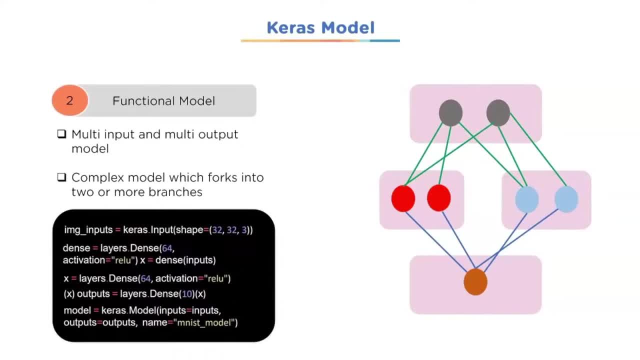 And so in here we do have the two complex models coming in. We have our image inputs, which is a 32 by 32, by 3 or 3 channels or 4. if you have an alpha channel, You have your layers dense 64. activation using the ReLU. 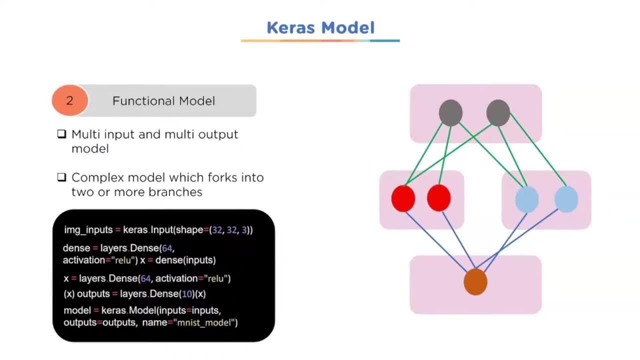 Very common: X equals dense inputs, X layers. dense. 64. activation equals ReLU. X. outputs equals layers. dense. 10X Model equals Keras Model. inputs equals inputs, Outputs equals outputs. Name equals ninst model. So we add a little name on there. 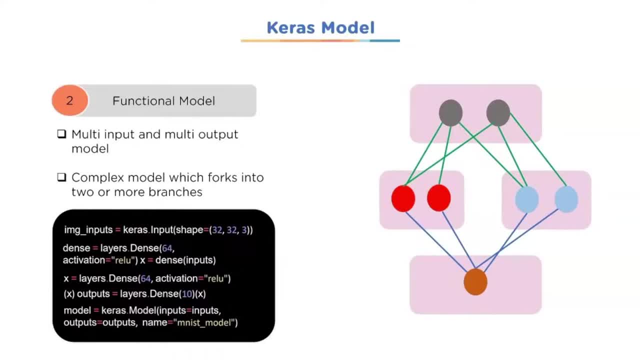 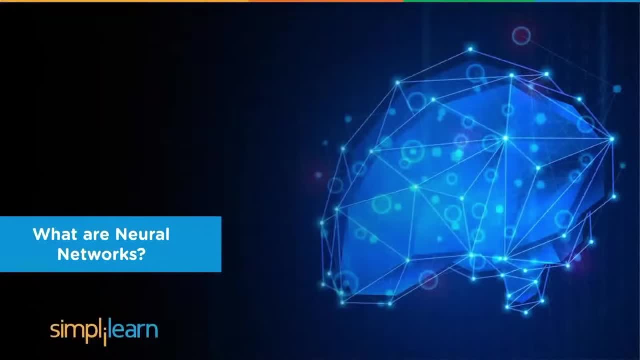 And again, this is this kind of split here. This is setting us up to have the input go into different areas. So if you're already looking at Keras, You already have this answer: What are neural networks? But it's always good to get on the same page. 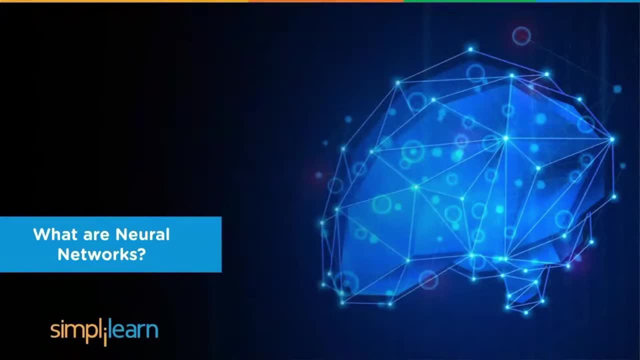 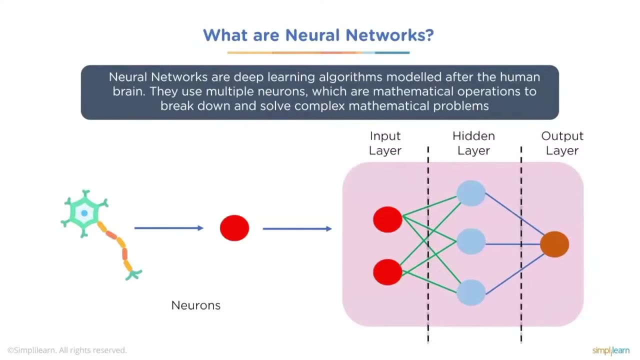 And for those people who don't fully understand neural networks, to dive into them a little bit Or do a quick overview. Neural networks are deep learning algorithms modeled after the human brain. They use multiple neurons, which are mathematical operations, to break down and solve complex mathematical problems. 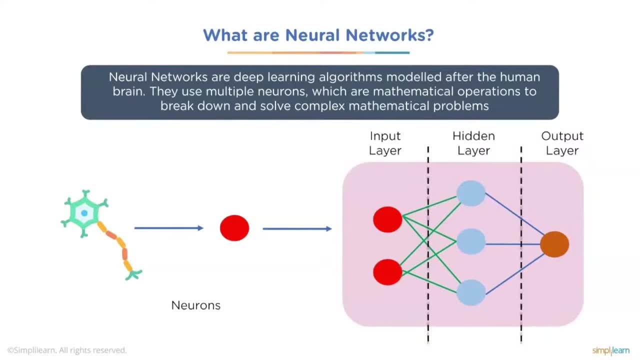 And so, just like the neuron, One neuron fires in and it fires out to all these other neurons, or nodes as we call them, And eventually they all come down to your output layer. And you can see, here we have the really standard graph input layer. 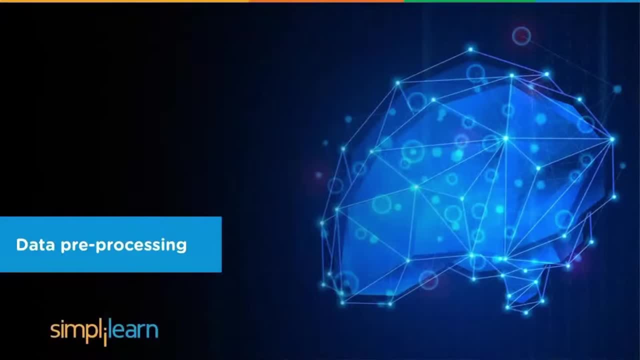 A hidden layer and an output layer. One of the biggest parts of any data processing is your data preprocessing, So we always have to touch base on that With a neural network. like many of these models, They're kind of when you first start using them. 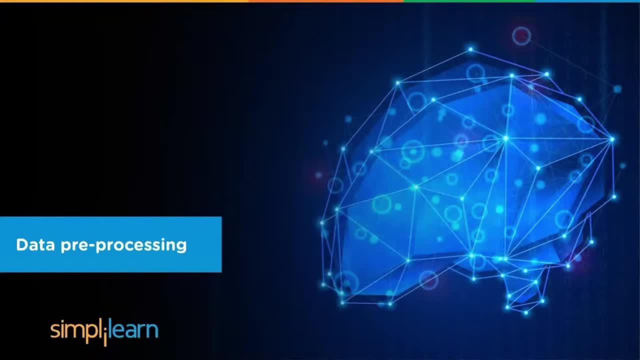 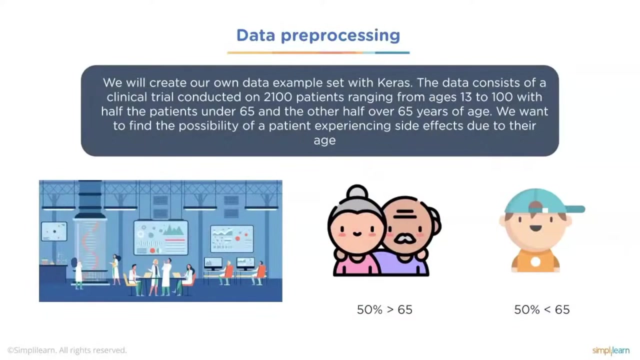 They're like a black box. You put your data in, You train it And you test it And see how good it was, And you have to preprocess that data because bad data in is bad outputs. So in data preprocessing we will create our own data examples, set with Keras. 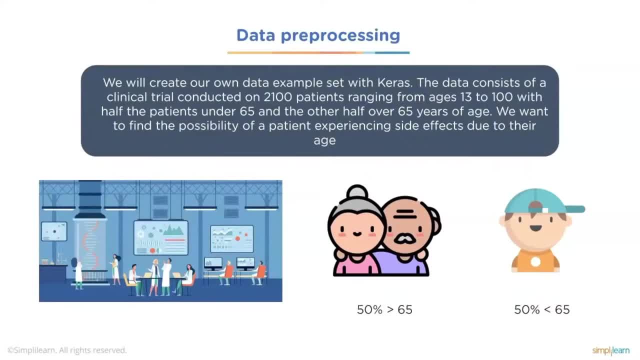 The data consists of a clinical trial conducted on 2100 patients Ranging from ages 13 to 100.. With the patients under 65 and the other half over 65 years of age, We want to find the possibility of a patient experiencing side effects. 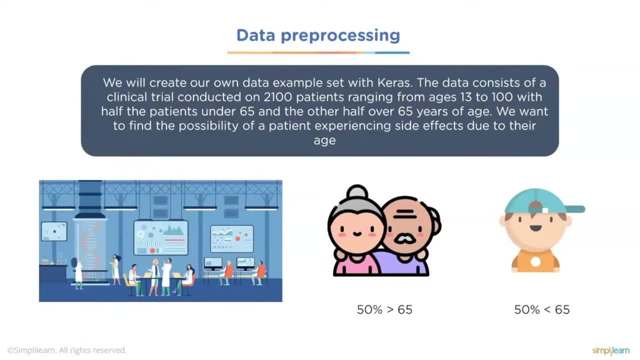 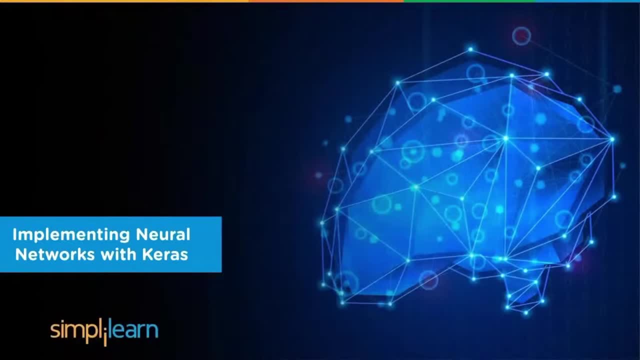 Due to their age, And you can think of this in today's world with COVID. What's going to happen on there? And we're going to go ahead and do an example of that in our live hands on. Like I said, most of this you really need to have hands on to understand. 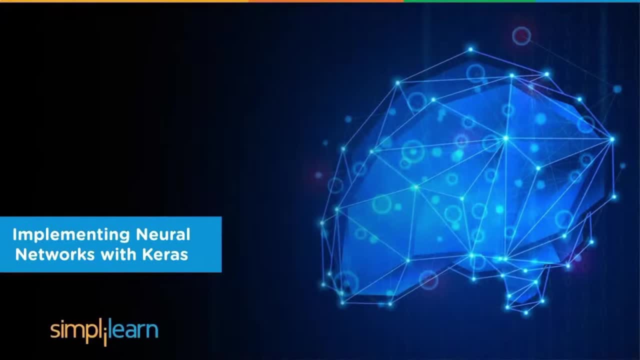 So let's go ahead and bring up our anaconda And open that up and open up a Jupyter notebook for doing the Python code in. Now, if you're not familiar with those, you can use pretty much any of your setups. I just like those for doing demos. 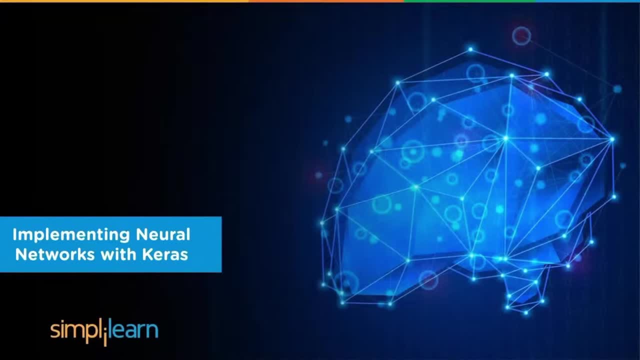 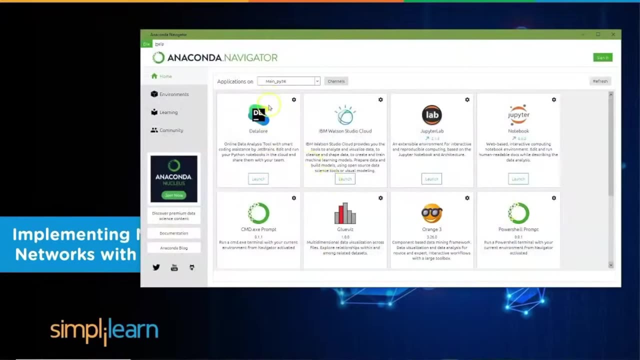 And showing people, especially shareholders. It really helps because it's a nice visual. So let me go ahead and flip over to our anaconda. And the anaconda has a lot of cool tools. They just added Datalore and IBM Watson Studio, clad into the anaconda framework. 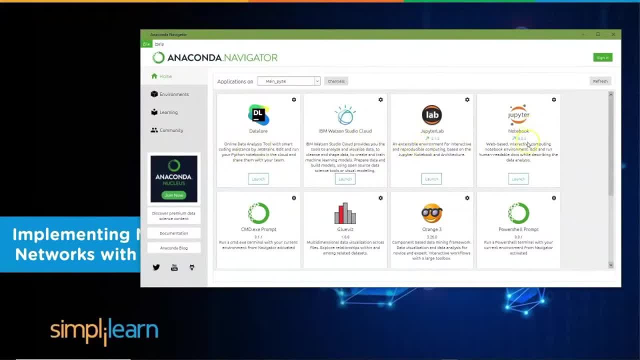 But we'll be in the Jupyter lab or Jupyter notebook. I'm going to do Jupyter notebook for this Because I use the lab for, like, large projects with multiple pieces, Because it has multiple tabs, Where the notebook will work fine for what we're doing. 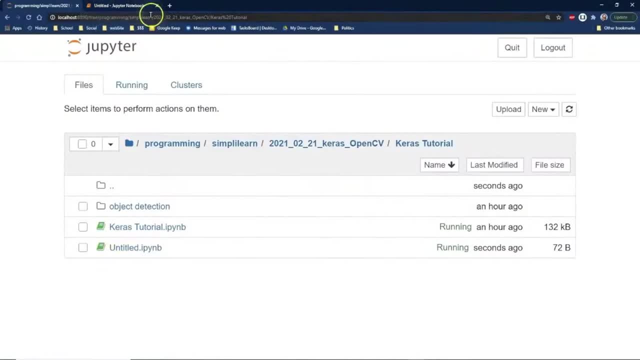 And this opens up in our browser window, Because that's how Jupyter notebook is set to run, And we'll go under new. Create a new Python 3.. And it creates an untitled Python. We'll go ahead and give this a title. 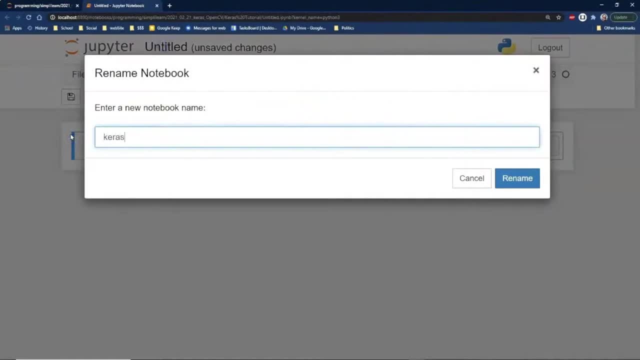 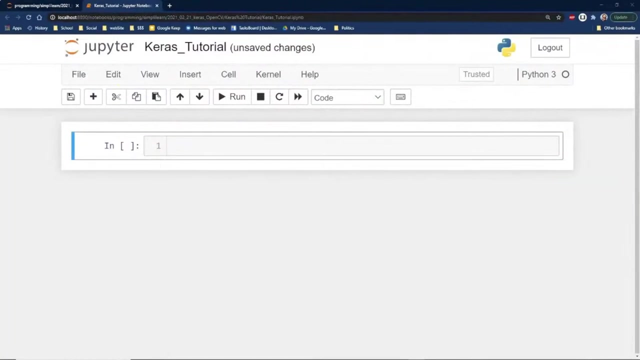 And we'll just call this cross tutorial And let's change that to capital. There we go. We'll go ahead and just rename that, And the first thing we want to go ahead and do is get some pre-processing tools involved, And so we need to go ahead and import some stuff for that. 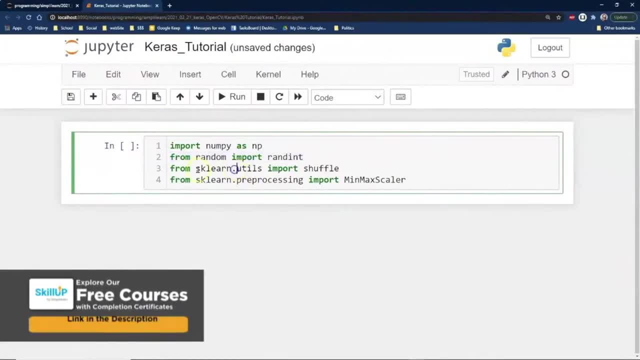 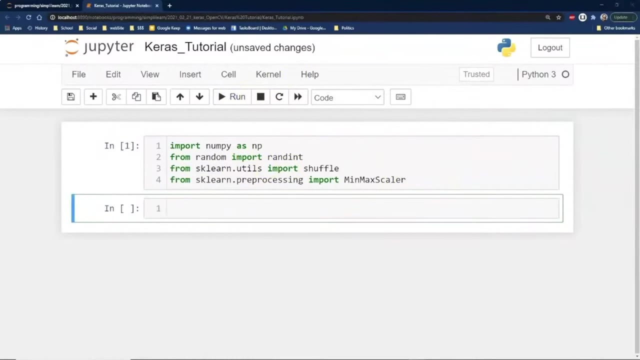 Like our numpy, Do some random number generation. I mentioned sklearn or your scikit. If you're installing sklearn- The sklearn stuff- It's a scikit you want to look up. That should be a tool of anybody who is doing data science. 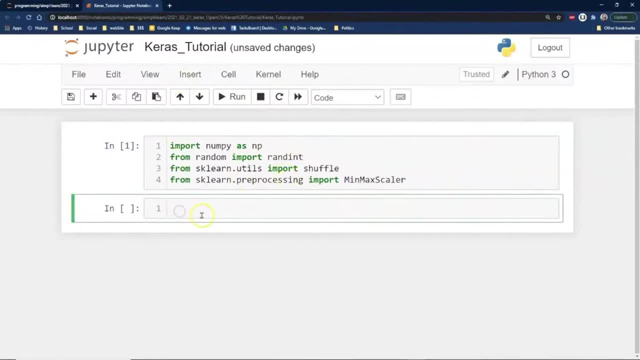 If you're not, If you're not familiar with the sklearn toolkit, It's huge, But there's so many things in there that we always go back to And we want to go ahead and create some train labels and train samples for training our data. 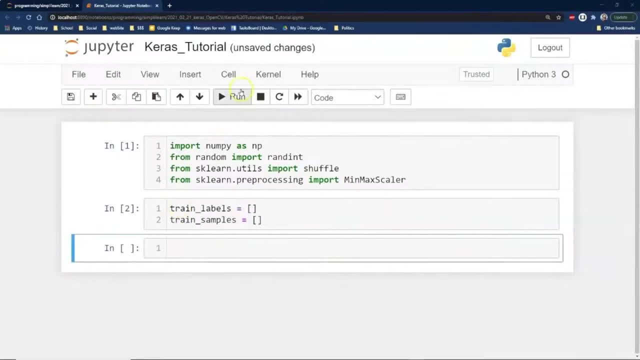 And then just a note of what we're actually doing in here. Let me go ahead and change this. This is kind of a fun thing you can do. We can change the code to markdown And then markdown code is nice for doing examples. 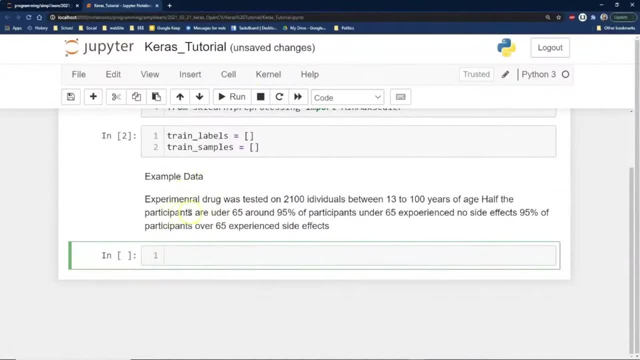 Once you've already built this, Our example data, We're going to do experimental. There we go. Experimental drug was tested on 2100 individuals between 13 to 100 years of age. Half the participants are under 65. And 95% of participants are under 65.. 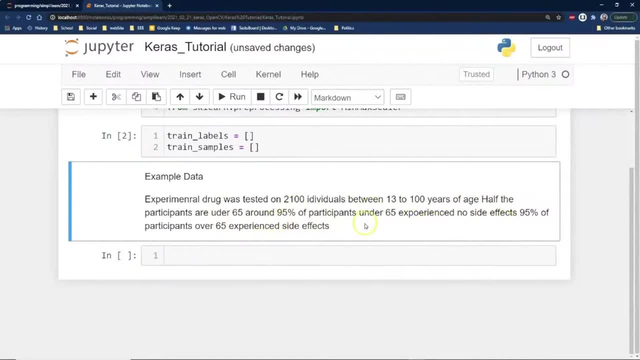 Experienced no side effects, While 95% of participants over 65 experienced side effects. So that's kind of where we're starting, And this is just a real quick example, Because we're going to do another one with a little bit more complicated information. 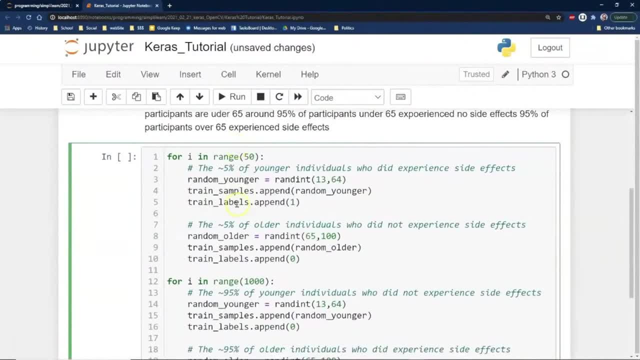 And so we want to go ahead and generate our setup. So we want to do for i in range And we want to go ahead and create. If you look here we have random integers, Train the labels, Append. So we're just creating some random data. 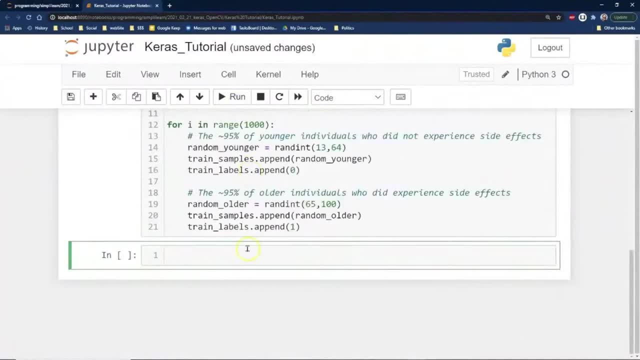 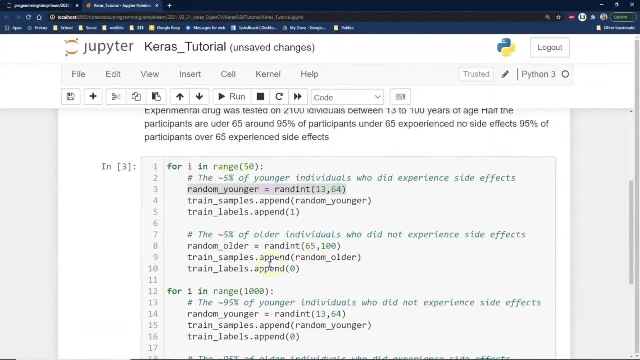 And let me go ahead and just run that. And so once we've created our setup, Once we've created our random data- And you can certainly ask for a copy of the code from Simply Learn- They'll send you a copy of this. 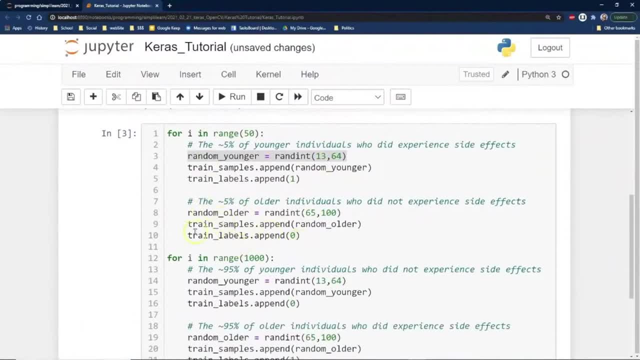 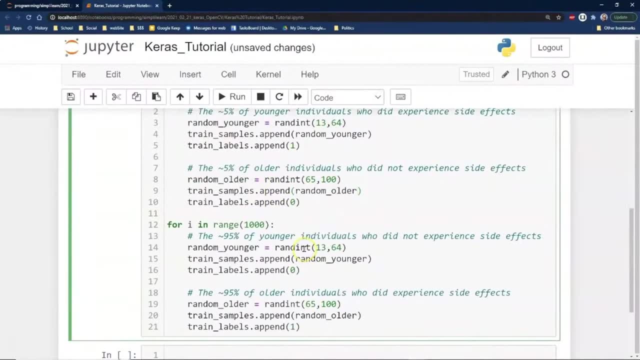 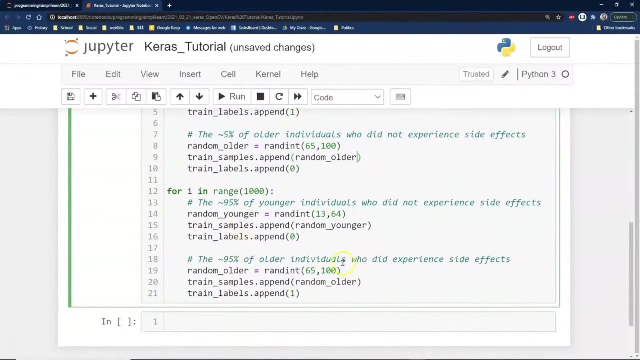 Or you can zoom in on the video and see how we went ahead and did our train samples Append, And we're just using this. I do this kind of stuff all the time. I was running a thing that had to do with errors following a bell shaped curve on a standard distribution error. 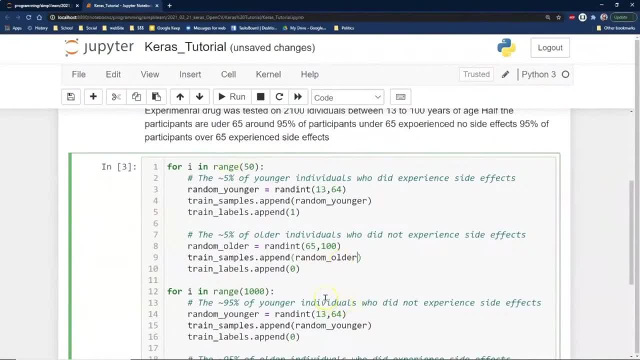 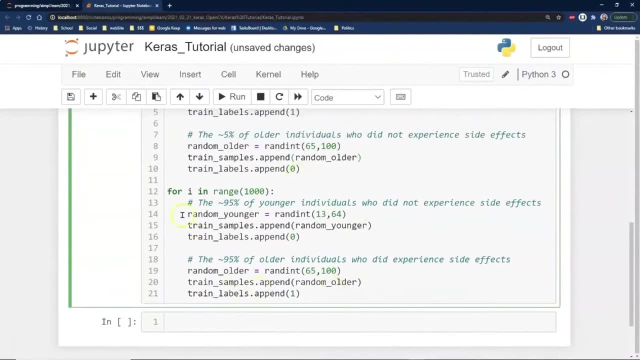 And so what do I do? I generate the data. I do the standard distribution error to see what it looks like And how my code processes it, since that was the baseline I was looking for In this. we're just generating random data for our setup on here. 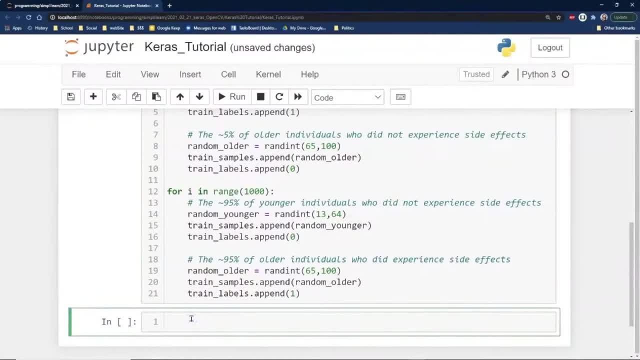 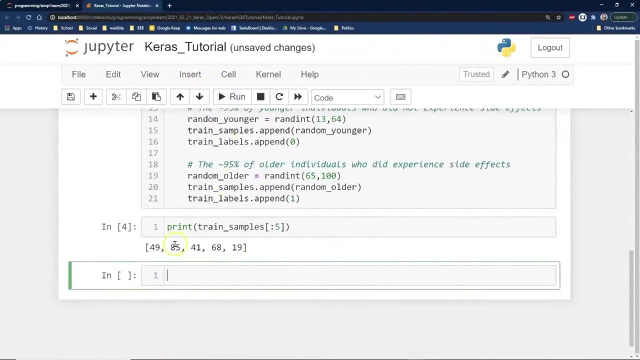 And we could actually go in and print some of the data up. Let's just do this Print, We'll do train samples And we'll just do the first five pieces of data in there to see what that looks like. And you can see the first five pieces of data in our train samples is 49,, 85,, 41,, 68,, 19.. 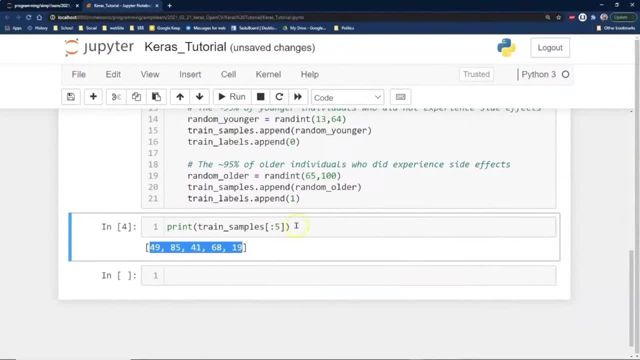 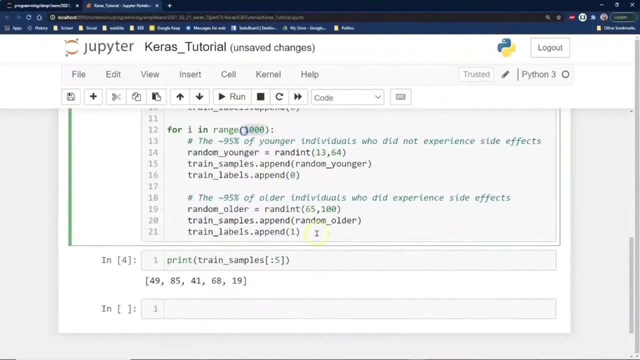 Just random numbers generated in there. That's all that is, And we generated significantly more than that. Let's see 50 up here, 1,000.. Yeah, So there's 1,000 here. 1,000 numbers we generated. 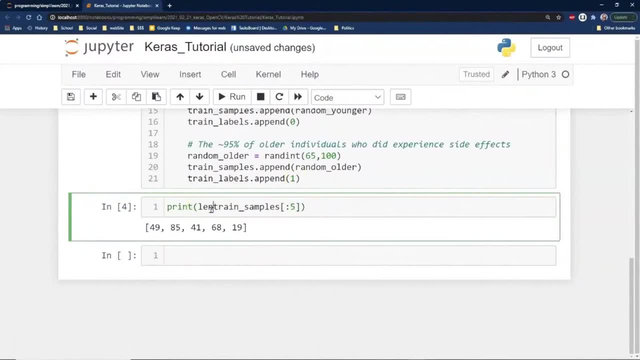 And we could also, if we wanted to find that out, we could do a quick print the length of it, Or you could do a shape kind of thing. And if you're using NumPy- although the length for this is just fine- 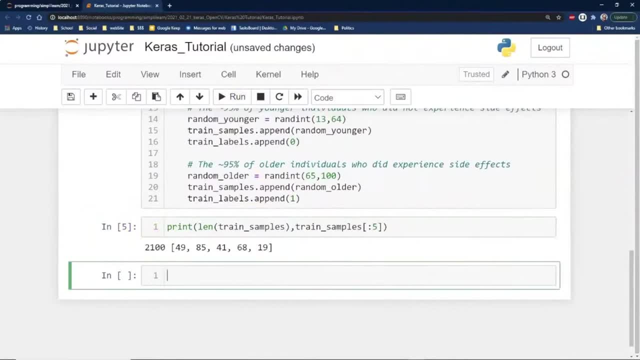 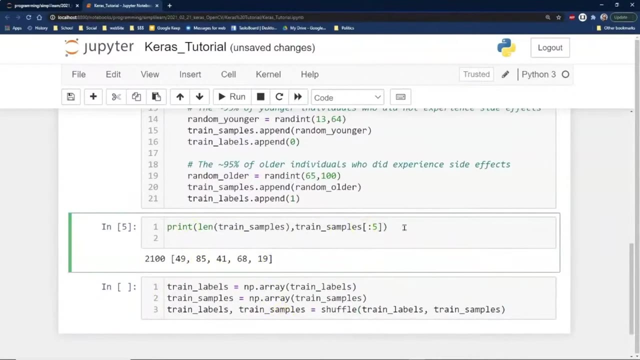 And there we go. It's actually 2,100, like we said in the demo setup in there. And then we want to go ahead and take our labels. That was our train labels. We also did samples, didn't we? So we could also print, do the same thing. 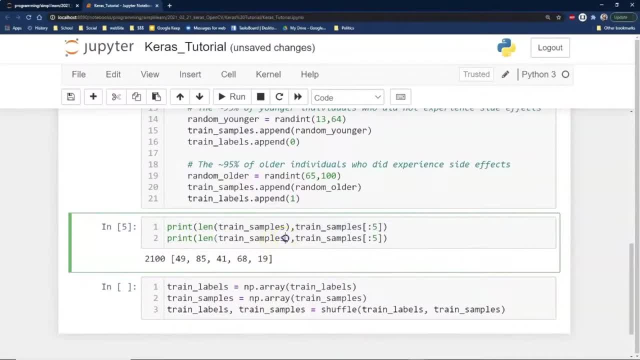 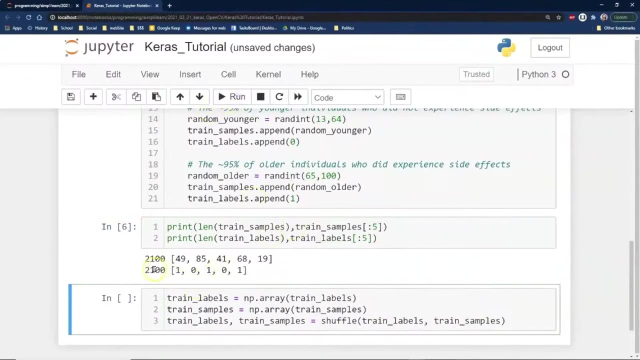 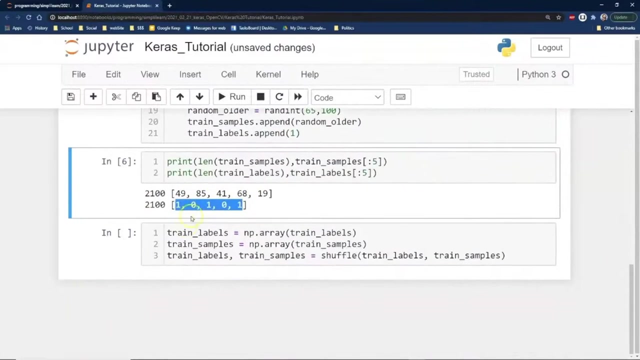 Labels, And let's change this to labels And labels And run that Just to double check And sure enough, we have 2,100.. And they're labeled 101010.. I guess that's if they have symptoms or not. 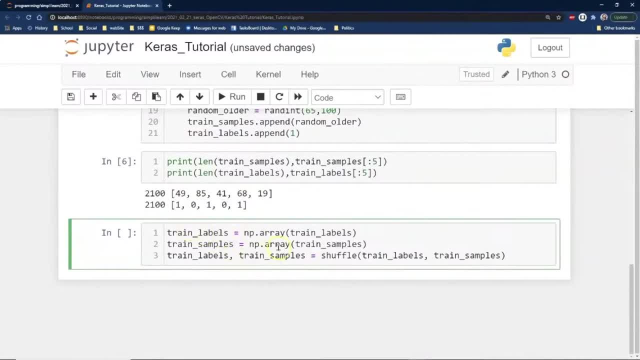 One symptoms, zero, none. And so we want to go ahead and take our train labels and we'll convert it into a NumPy array, And the same thing with our samples, And let's go ahead and run that, And we also shuffle. 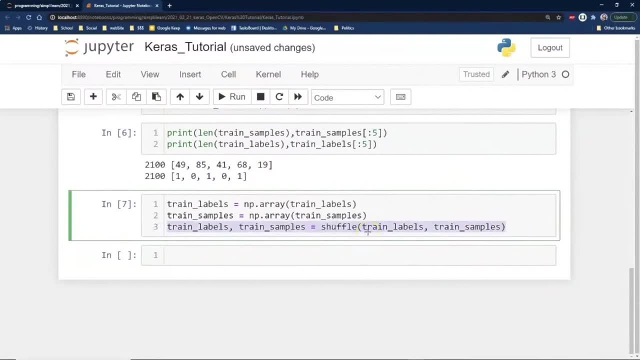 This is just a neat feature you can do in NumPy right here, Put my drawing thing on, which I didn't have on earlier. I can take the data and I can shuffle it. So we have our, so it just randomizes it. 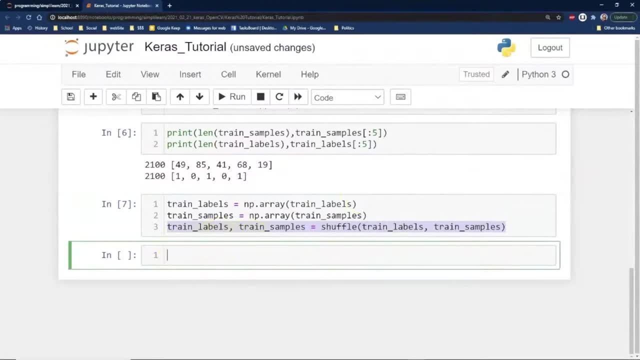 That's all that's doing. We've already randomized it, so it's kind of an overkill. It's not really necessary, But if you're doing a larger package where the data is coming in and a lot of times it's organized somehow. 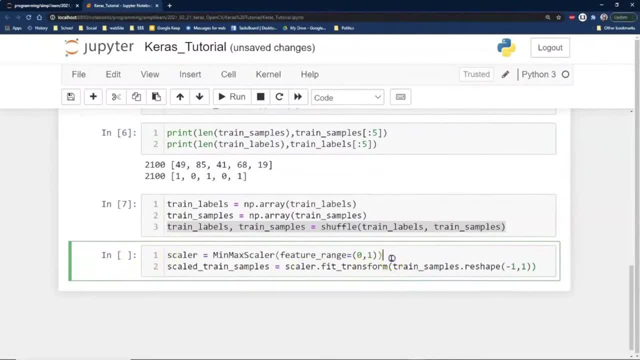 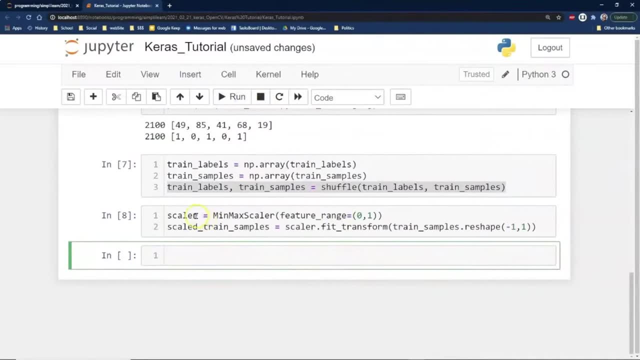 And you want to randomize it, just to make sure that you know the input doesn't follow a certain pattern that might create a bias in your model. And we go ahead and create a scalar, The scalar range minimum max scalar. Feature range: zero to one. 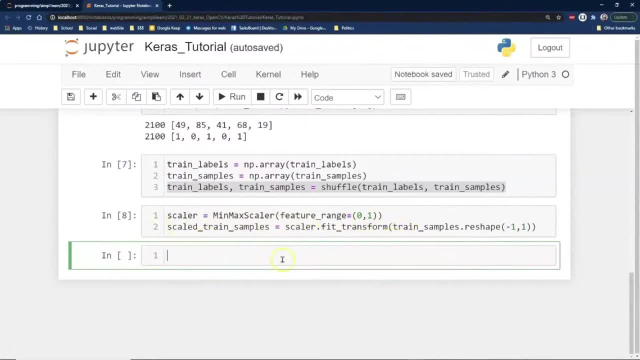 Then we go ahead and scale the scale train samples. So we're going to go ahead and fit and transform the data. So it's nice and scaled. And that is the age. So you can see up here we have forty-nine, eighty-five, forty-one. 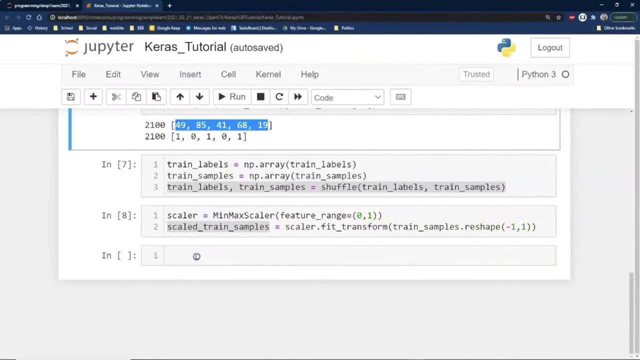 We're just moving that, so it's going to be between zero and one, And so this is true with any of your neural networks. You really want to convert the data to zero and one, Otherwise you create a bias. So if you have like a hundred creates a bias versus the math behind it gets really complicated. 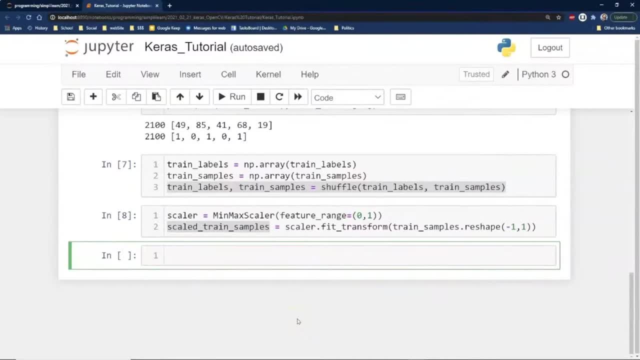 If you actually start multiplying stuff- there's a lot of multiplication and addition going on in there- That higher end value will eventually multiply down And it will have a huge bias as to how the model fits it, And then it will not fit as well. 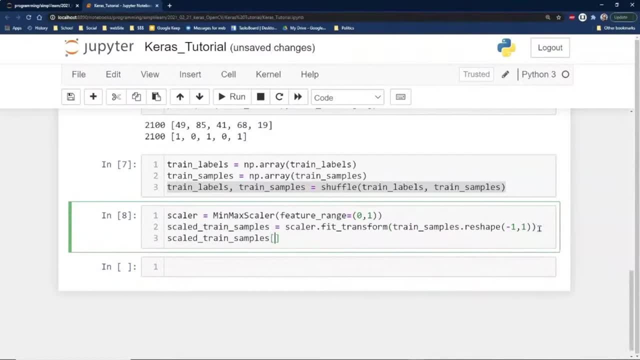 And then one of the fun things we can do in Jupyter Notebook is that if you have a variable and you're not doing anything with it, it's the last one on the line. It will automatically print. And we're just going to look at the first five samples on here. 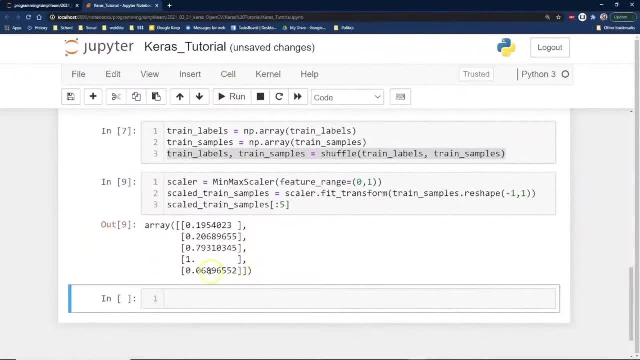 And so it's going to print the first five samples And you can see here we go .195, .791.. So everything's between zero and one, And that just shows us that we scaled it properly and it looks good. It really helps a lot to do these kind of printups halfway through. 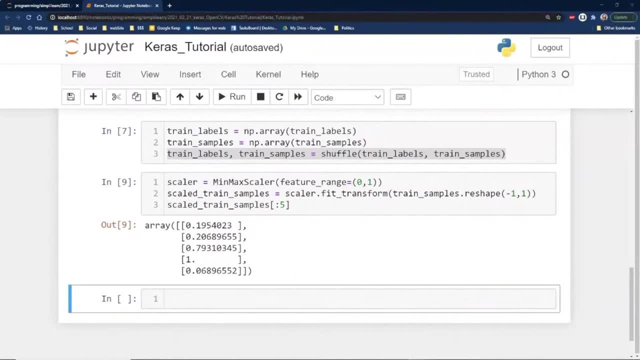 You never know what's going to go on there. I don't know how many times I've gotten down and found out that the data sent to me that I thought was scaled was not, And then I have to go back and track it down and figure it out on there. 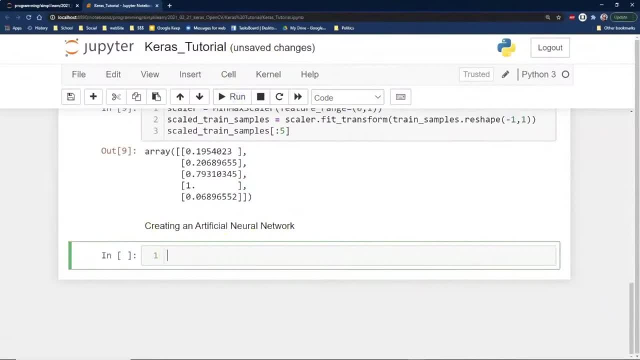 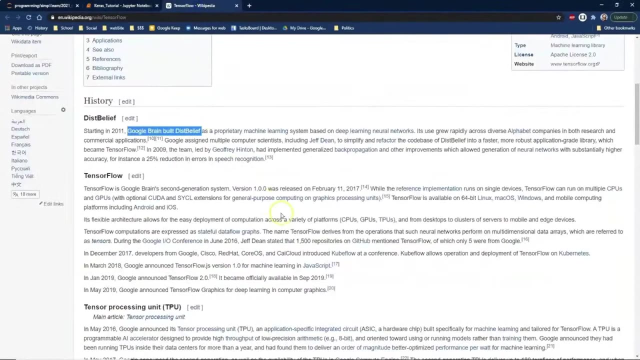 So let's go ahead and create our artificial neural network, And for doing that, this is where we start diving into TensorFlow and Keras TensorFlow. if you don't know the history of TensorFlow, it helps to jump into- we'll just use Wikipedia. 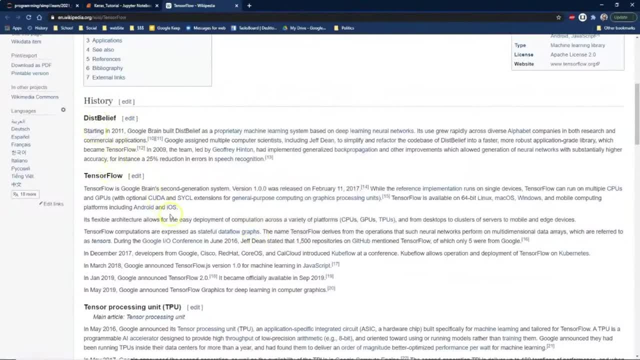 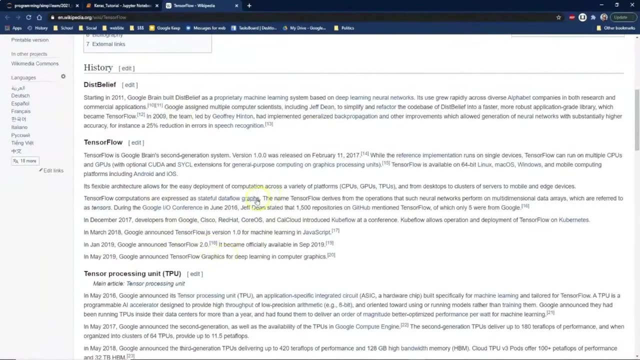 Be careful, Wikipedia, on these things, because you get in trouble, But it's a good place to start. Back in 2011,, Google Brain built Disbelief as a proprietary machine learning setup. TensorFlow became the open source for it, So TensorFlow was a Google product. 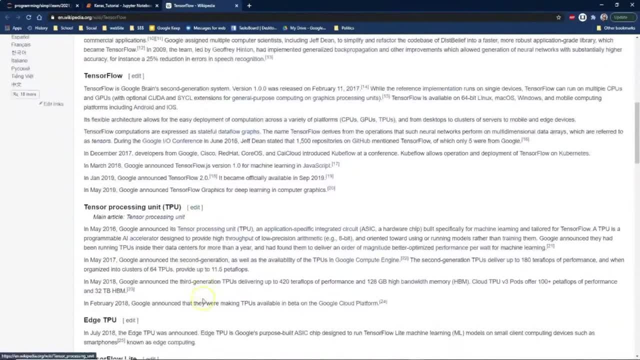 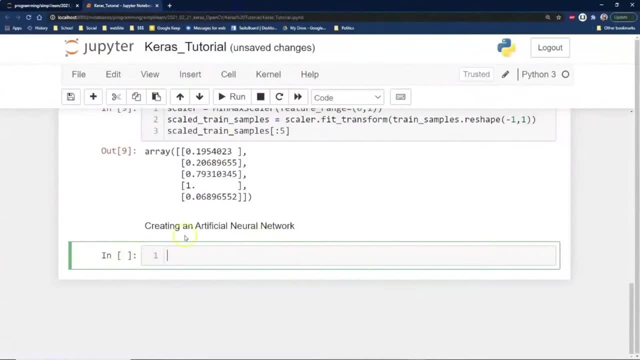 And then it became open sourced And now it's just become probably one of the de facto's when it comes for neural networks, as far as where we're at. So when you see the TensorFlow setup, it's got like a huge following. There are some other setups, like the side kit under the sklearn has their own little neural network. 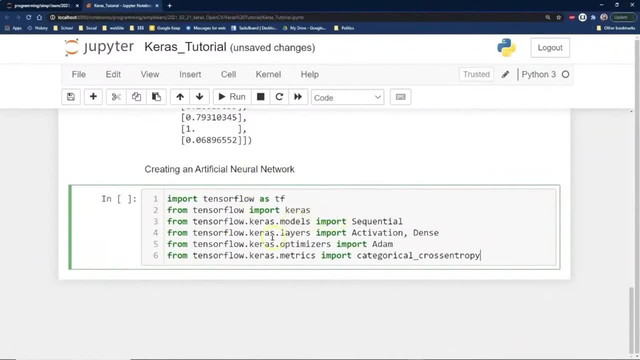 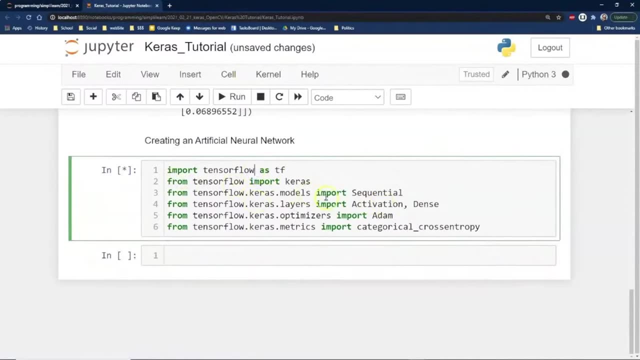 But the TensorFlow is the most robust one out there right now And Keras sitting on top of it makes it a very powerful tool. So we can leverage both the Keras easiness in which we can build a sequential setup on top of TensorFlow. 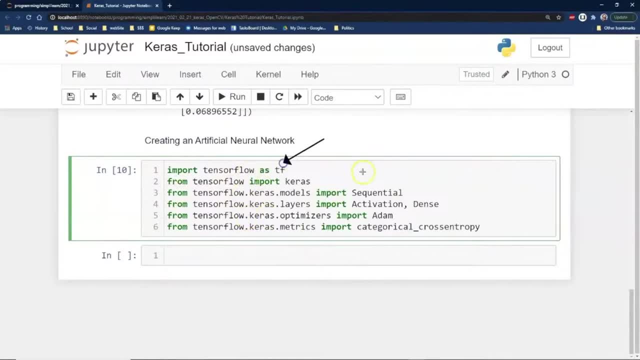 And so in here we're going to go ahead And do our input of TensorFlow And then we have the rest of this is all Keras here, from number two down We're going to import from TensorFlow the Keras connection And then you have your TensorFlow Keras models import sequential. 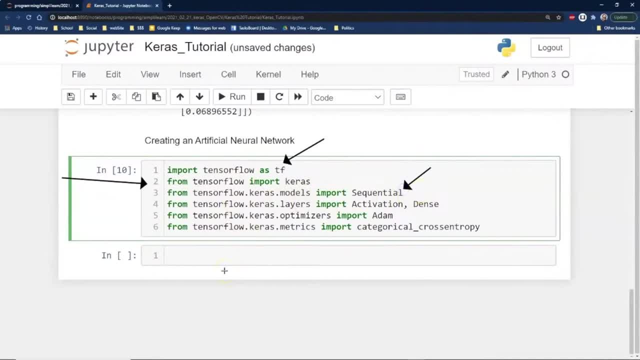 It's a specific kind of model. We'll look at that in just a second. If you remember from the files, that means it goes from one layer to the next layer to the next layer. There's no funky splits or anything like that. 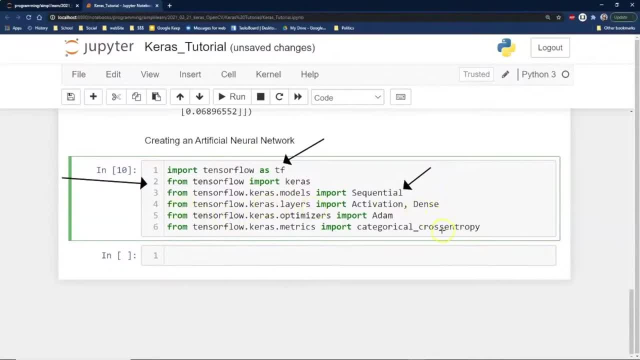 And then we have from TensorFlow. From TensorFlow Keras layers, we're going to import our activation and our dense layer And we have our optimizer Atom. This is a big thing to be aware of how you optimize your data. When you first do it, Atom's as good as any. 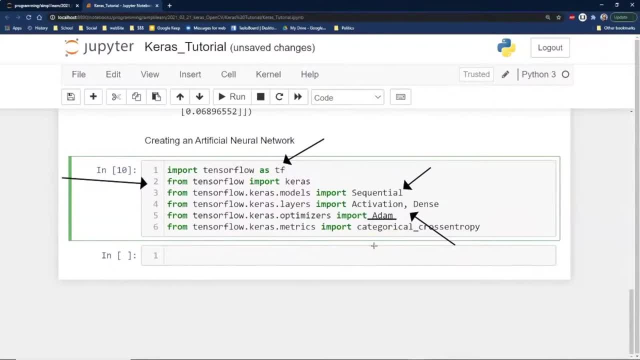 Atom is usually. there's a number of optimizer out there. There's a couple of main ones, But Atom is usually assigned to bigger data. It works fine Usually. the lower data does it just fine, But Atom is probably the mostly used. 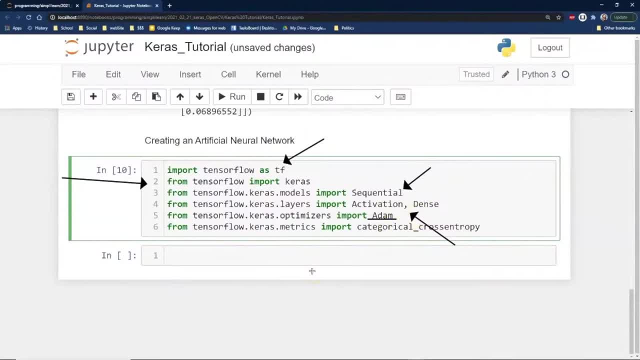 But there are some more out there And, depending on what you're doing with your layers, your different layers might have different activations on them. And then finally, down here you'll see our setup, where we want to go ahead and use the metrics. 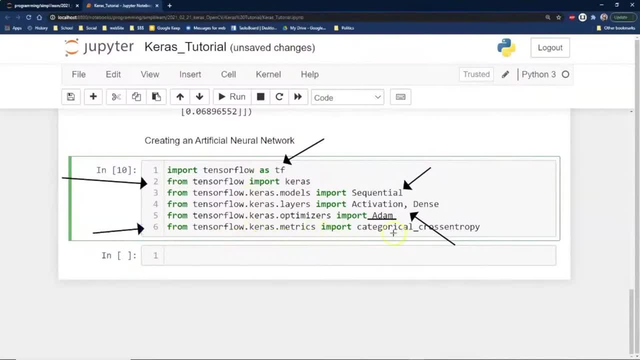 And we're going to use the TensorFlow Keras metrics for categorical Keras entropy So we can see how everything performs when we're done. That's all that is. A lot of times you'll see us go back and forth between TensorFlow and then Scikit has a lot of really good metrics also for measuring these things. 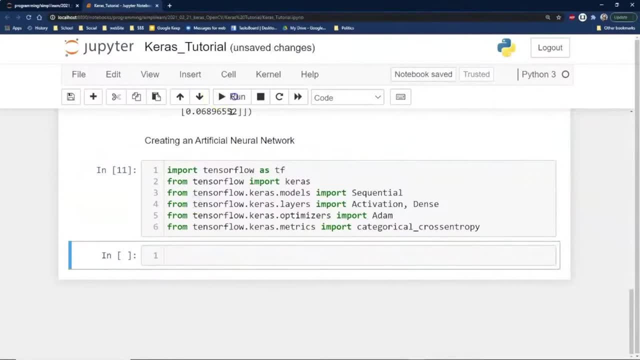 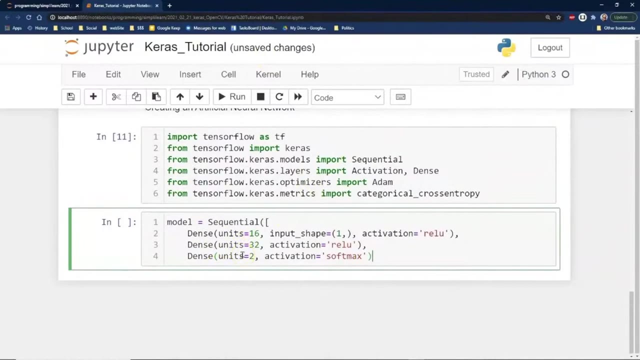 Again at the end of the story: how good does your model do? And we'll go ahead and load all that. And then comes the fun part. I actually like to spend hours messing with these things And four lines of code. You're like, ah, you're going to spend hours on four lines of code. 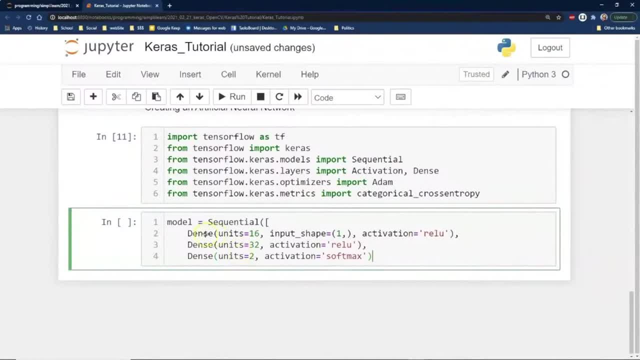 No, You don't spend hours on four lines of code. That's not what we're talking about when I say spend hours on four lines of code. What we have here- and I'm going to explain that in just a second- we have a model. 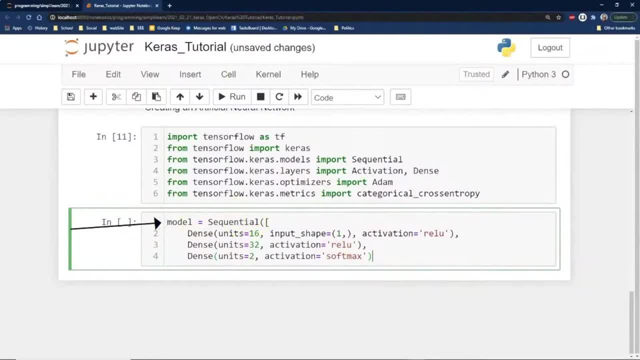 And it's a sequential model, If you remember correctly- we mentioned the sequential up here- where it goes from one layer to the next And our first layer is going to be our input. It's going to be what they call dense, which usually is just dense. 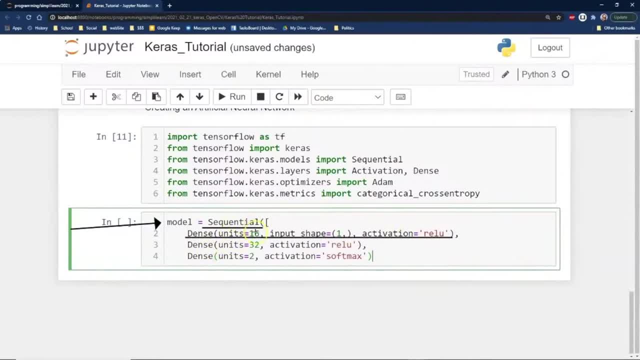 And then you have your input and your activation. How many units are coming in? We have 16.. What's the shape? What's the activation? And this is where it gets interesting, because we have in here ReLU on two of these and Softmax activation on one of these. 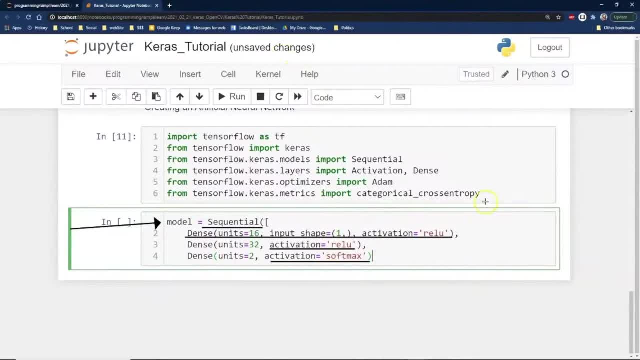 There are so many different options for what these mean and how they function. How does the ReLU, how does the Softmax function? And they do a lot of different things. We're not going to go into the activations in here. That is. what really you spend hours doing is looking at these different activations. 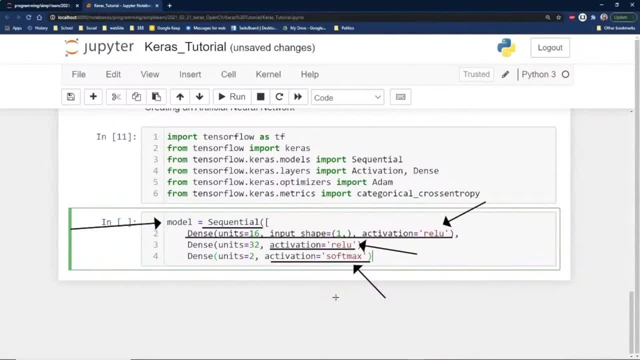 And just some of it is just almost like you're playing with it Like an artist. you start getting a feel for like an inverse tangent activation or the tanh activation takes up a huge processing amount, So you don't see it a lot. 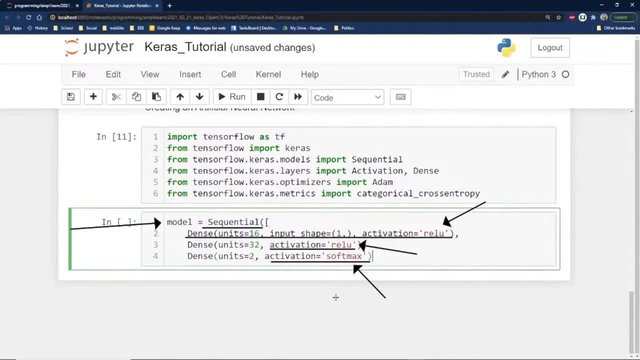 Yet it comes up with a better solution, especially when you're doing, when you're analyzing word documents, and you're tokenizing the words, And so you'll see this shift from one to the other, because you're both trying to build a better model. 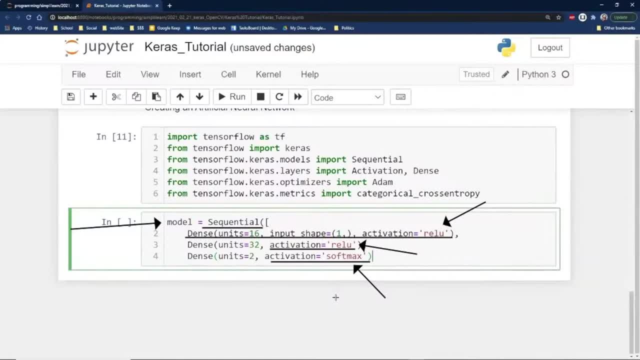 And if you're working on a huge data set, you'll crash the system. It'll just take too long to process. And then you see things like Softmax, Softmax. Softmax Generates an interesting setup. Where a lot of these? when you talk about ReLU? 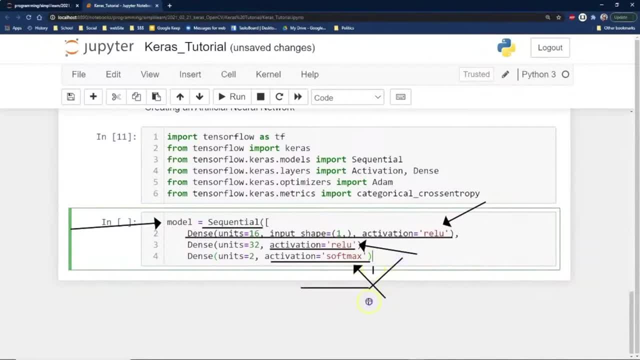 Oops, let me do this ReLU. There we go. ReLU has a setup where if it's less than zero, it's zero, And then it goes up. And then you might have what they call lazy setup, where it has a slight negative to it so that the errors can translate better. 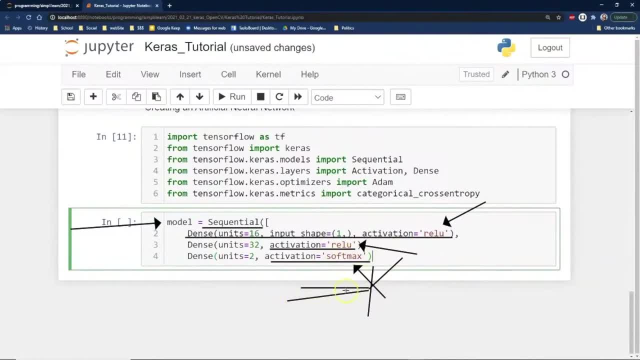 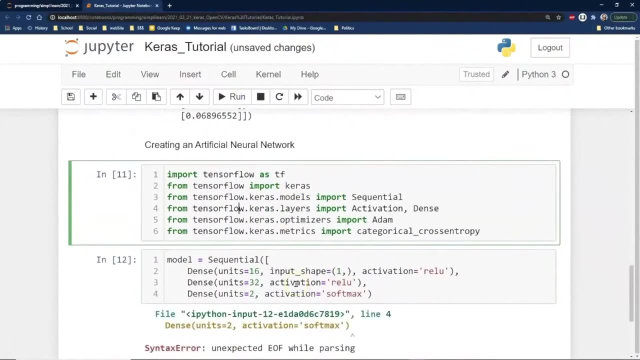 Same thing with Softmax. It has a slight laziness to it So that errors can translate better. translate better. all these little details make a huge difference on your model. so one of the really cool things about data science that I like is you build your, what they call you build to fail, and it's an interesting design set. 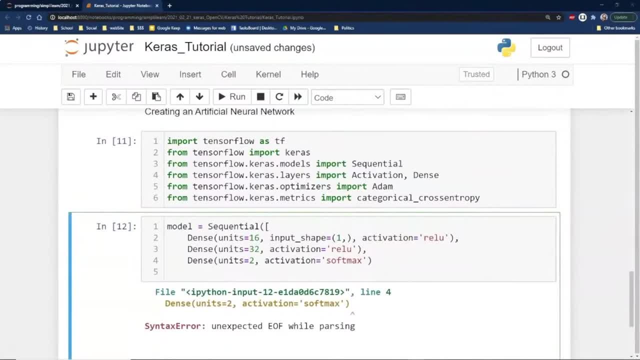 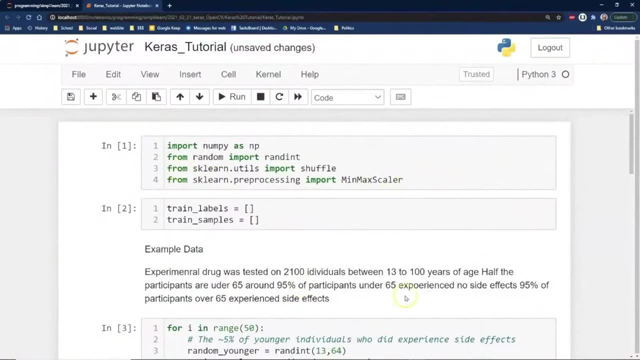 up. oops, I forgot the end of my code here. the concept of build to fail is: you want the model as a whole to work, so you can test your model out, so that you can do, you can get to the end and you can do. your see, where was it? 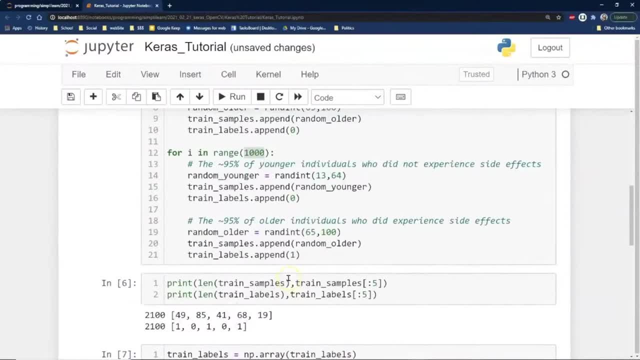 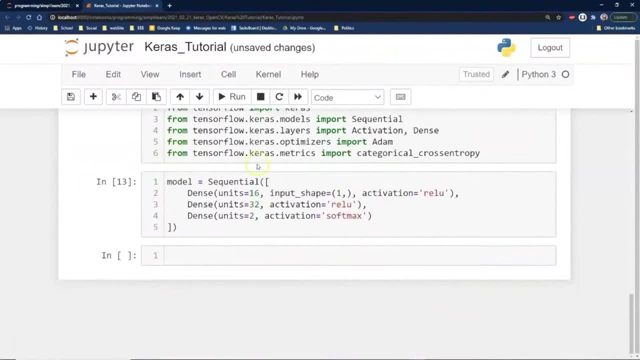 hovershot down here. you could test your test out, out the quality of your set up on there and see what did I do? my tensorflow? oh, here we go, I did. it was right above me. there we go, we started doing your cross entropy and stuff like that is. you need a full functional set of code. 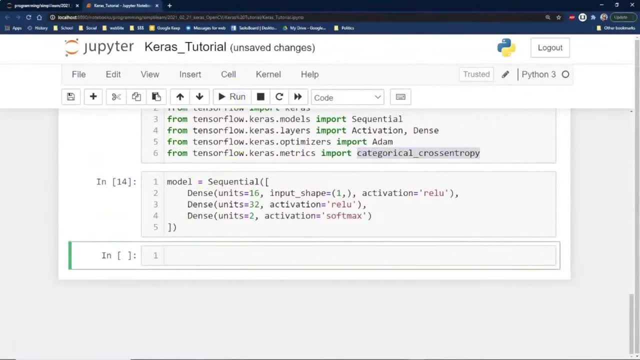 you. well, you can do your tests, you can see, do local code, you can see things like everything you just added here- you just added string stuff here you can show, So that when you run it you can then test your model out and say, hey, it's either this model works better than this model, and this is why 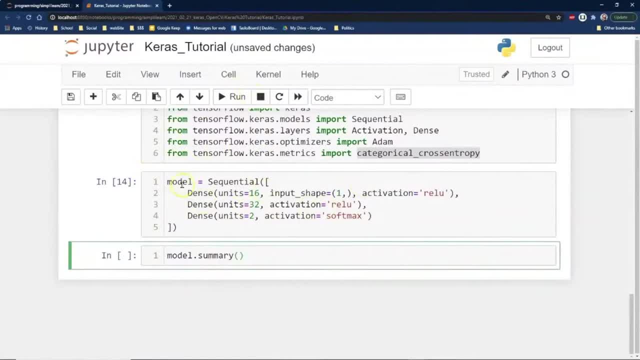 And then you can start swapping in these models. And so when I say I spend a huge amount of time on preprocessing data, it's probably 80% of your programming time. Well, between those two it's like 80-20.. 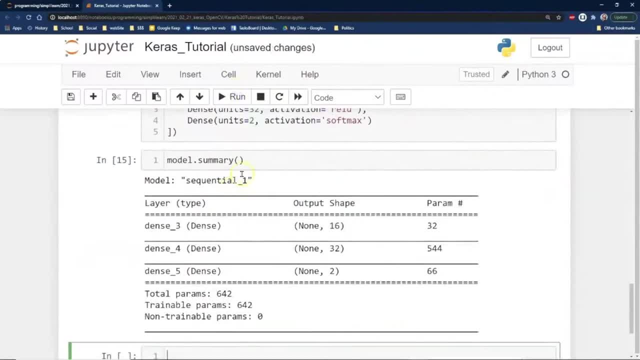 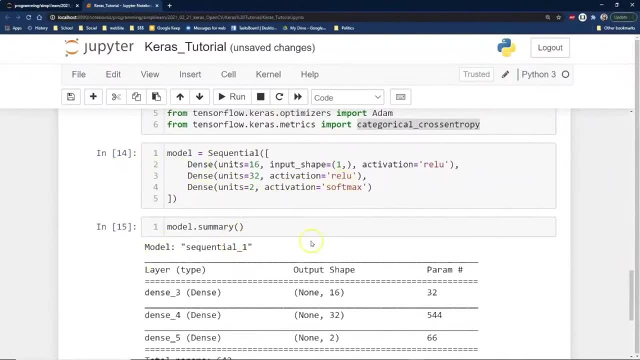 You'll spend a lot of time on the models. Once you get the model down, once you get the whole code and the flow down set depending on your data, your models get more and more robust as you start experimenting with different inputs, different data streams and all kinds of things. 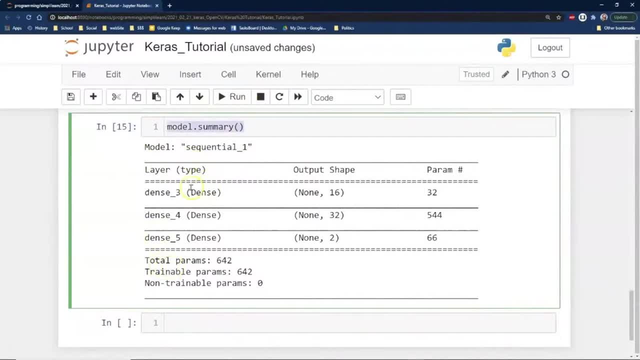 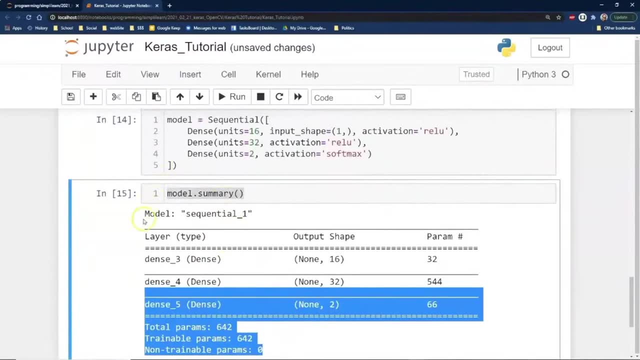 And we can do a simple model summary here. Here's our sequential, Here's our layer, our output, our parameter. This is one of the nice things about Keras You can see right here. here's our sequential one model: Boom, boom, boom, boom. 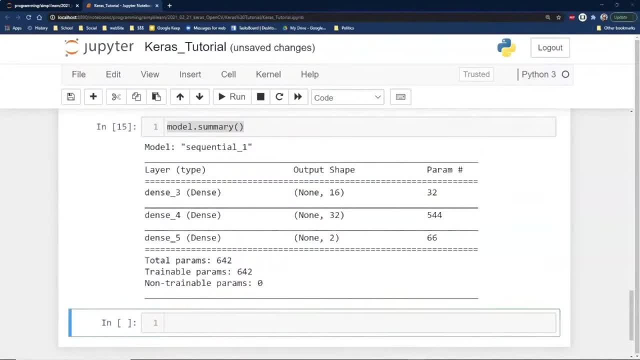 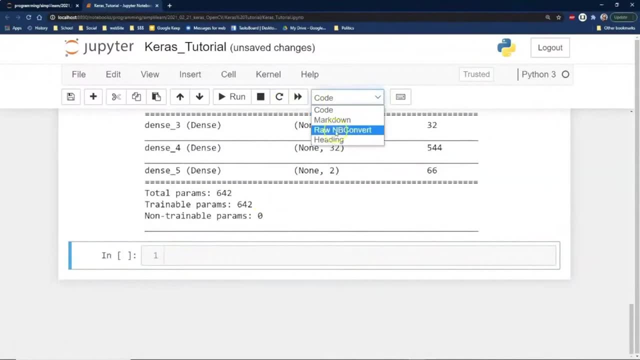 Everything is set and clear and easy to read. So, once we have our model built, the next thing we're going to want to do is we're going to want to go ahead and train that model, And so the next step is, of course, model training. 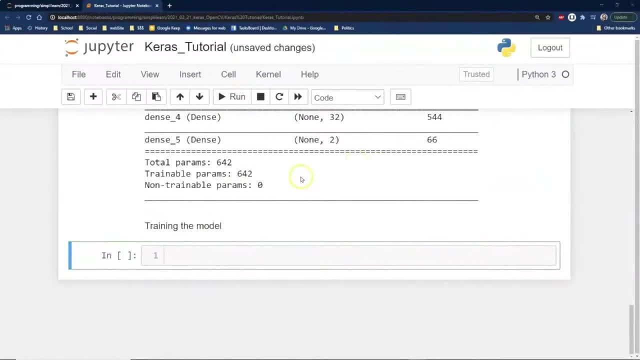 And when we come in here, this a lot of times is just paired with the model because it's so straightforward. It's nice to print out the model setup so you can have a tracking. But here's our model. The key word in Keras is compile. 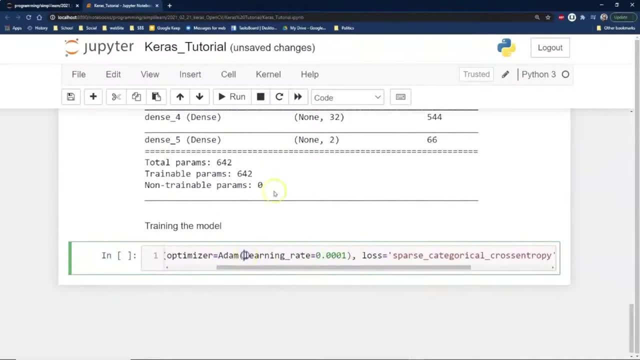 Optimizer, atom learning rate- another term right there that we're just skipping right over- that really becomes the meat of the setup- is your learning rate. So whoops, I forgot that I had an arrow, but I'll just underline it. 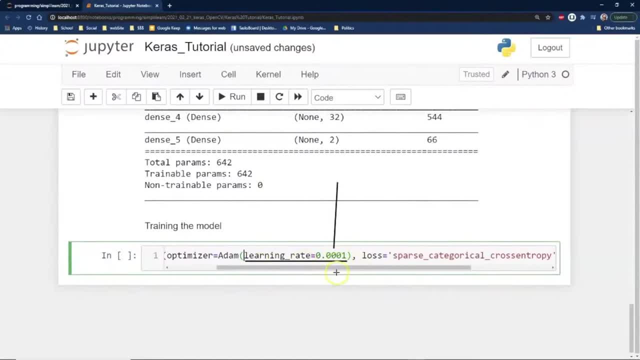 A lot of times the learning rate is set to 0.01,. depending on what you're doing. This learning rate can overfit and underfit, so you'd want to look up. I know we have a number of tutorials out on overfitting and underfitting that are really worth reading once you get to that point in understanding. 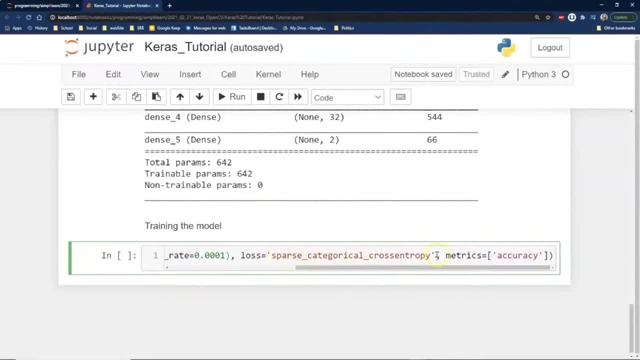 And we have our loss: sparse, categorical cross entropy. so this is going to tell Keras how far to go until it stops, and then we're looking for metrics of accuracy. So we'll go ahead and run that, and now that we've compiled our model, 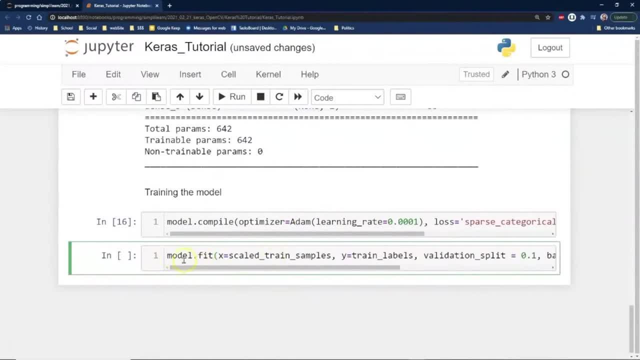 we want to go ahead and run it, fit it. So here's our model: fit. We have our scale to train samples, our train labels, our validation split. In this case, we're going to use 10% of the data for validation. 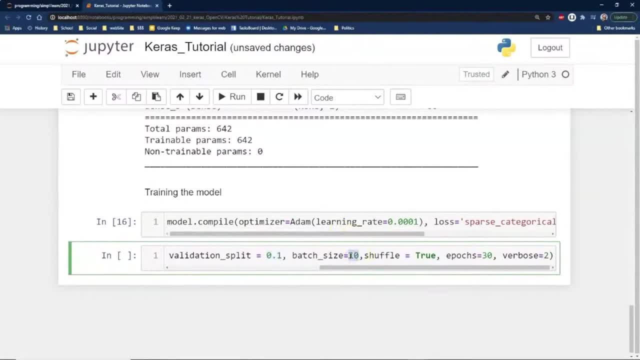 Batch size, another number you kind of play with. Not a huge difference as far as how it works, but it does affect how long it takes to run, and it can also affect the bias a little bit. Most of the time, though, a batch size is between 10 to 100, depending on just how much data you're processing in there. 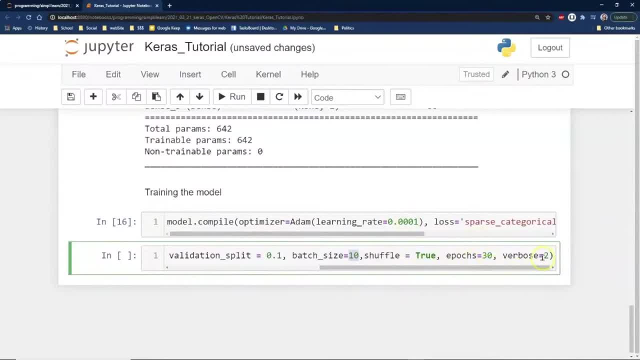 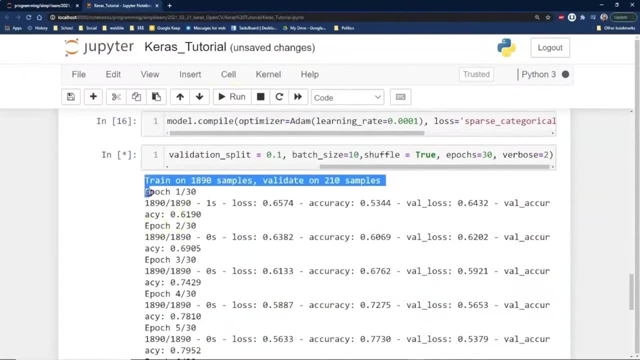 We want to go ahead and shuffle it. We're going to go through 30 epics and put a verbose of 2, and let me just go ahead and run this And you can see right here: here's our epic, here's our training, here's our loss. 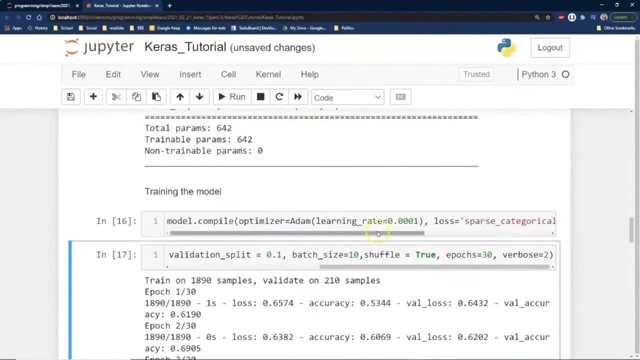 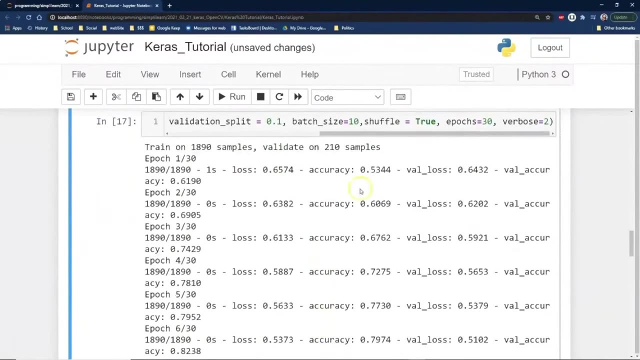 Now, if you remember correctly, up here we set the loss. Let's see where was it Compiled, our data, There we go Loss. So it's looking at the sparse categorical cross entropy. This tells us that, as it goes, how much does the error go down is the best way to look at that. 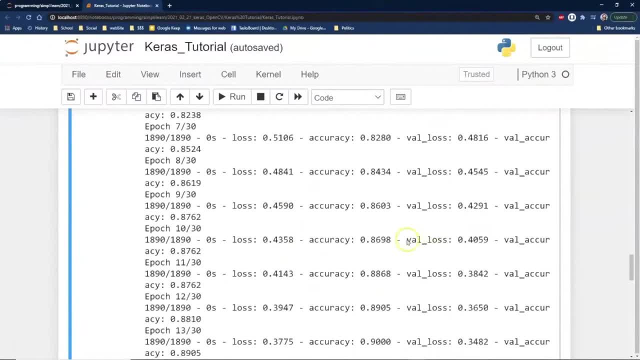 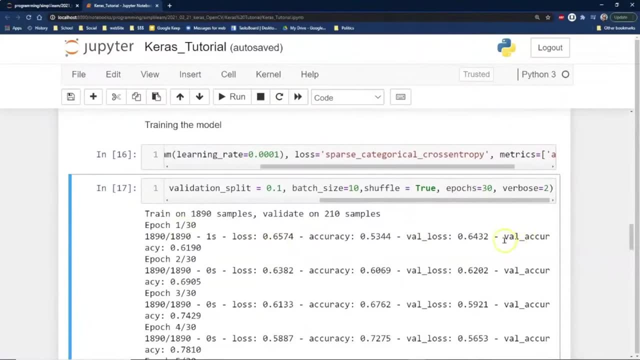 And you can see here, the lower the number, the better. It just keeps going down And vice versa. accuracy we want. Let's see where's my accuracy, Value, accuracy at the end, And you can see 0.619, 0.66.. 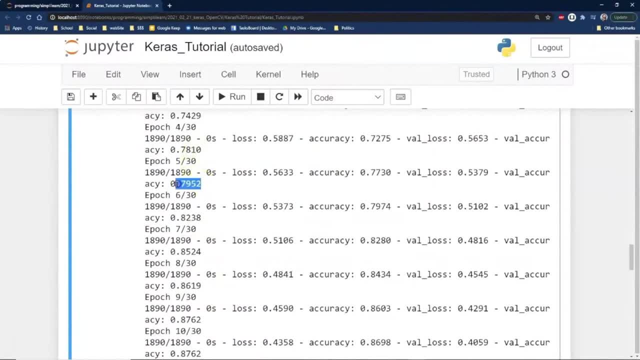 9.74,. it's going up. We want the accuracy- would be ideal if it made it all the way to 1.. But we also the loss is more important because it's a balance. You can have 100% accuracy and your model doesn't work because it's overfitted. 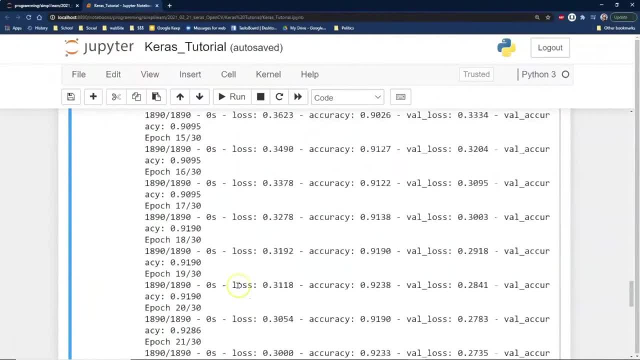 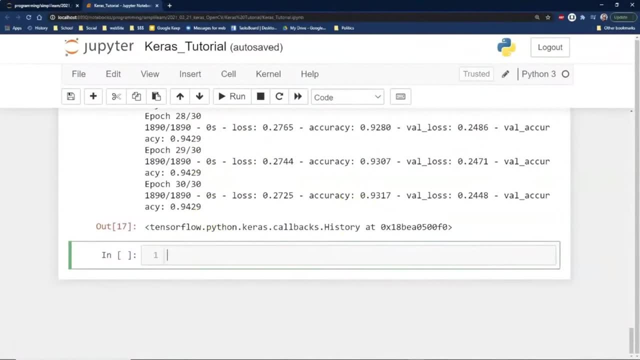 Again, you won't look up overfitting and underfitting models And we went ahead and went through 30 epics. It's always fun to kind of watch your code going. To be honest, I usually, the first time I run it, I'm like, oh, that's cool. 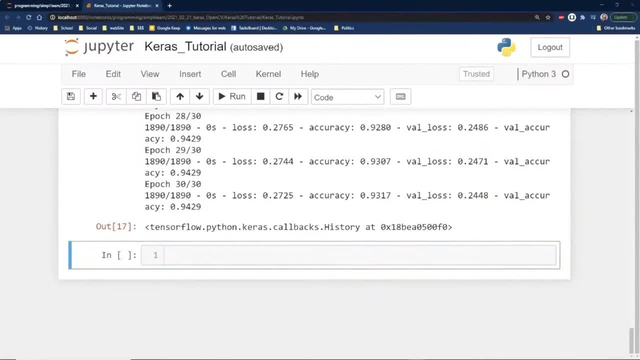 I get to see what it does And after the second time of running it I'm like I like to just not see that And you can repress those, of course, in your code. Repress the warnings in the printing. 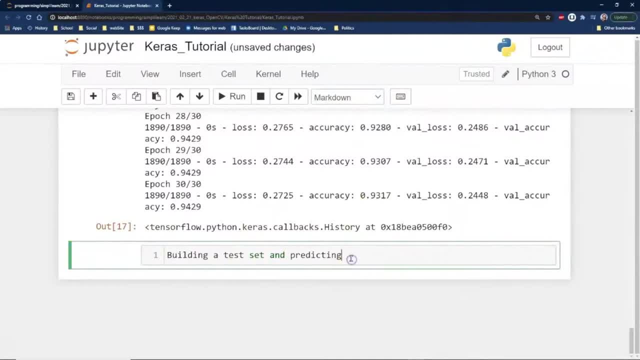 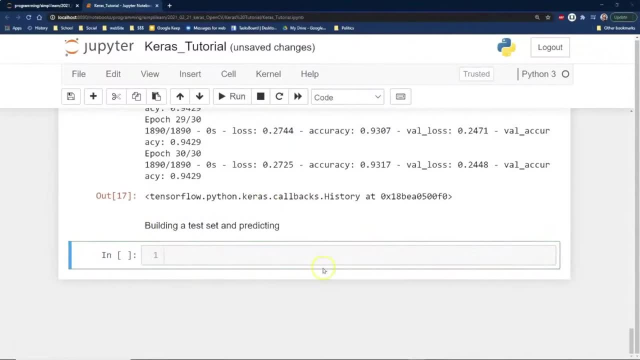 And so the next step is going to be building a test set and predicting it now. So here we go: We want to go ahead and build our test set And we have, just like we did, our training set. A lot of times, you just split your initial set up. 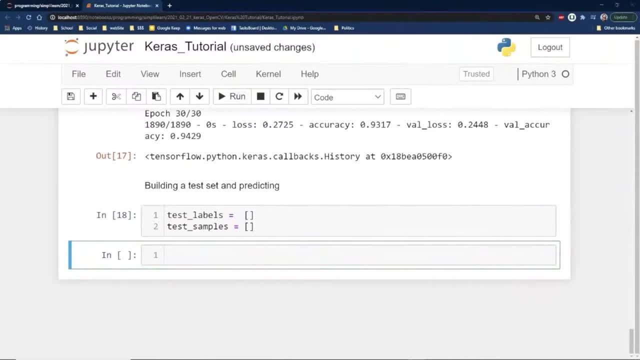 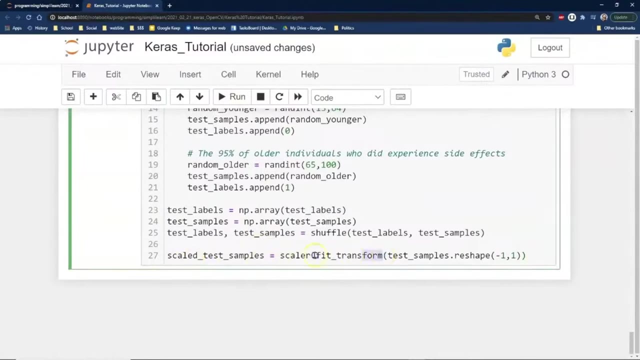 But we'll go ahead and do a separate set on here, And this is just what we did above. There's no difference as far as the randomness that we're using to build this set on here. The only difference is that we already did our scalar up here. 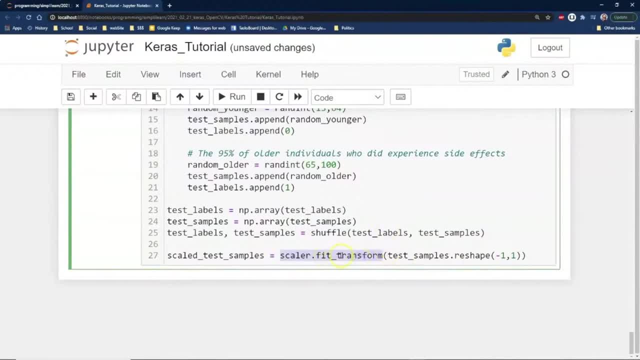 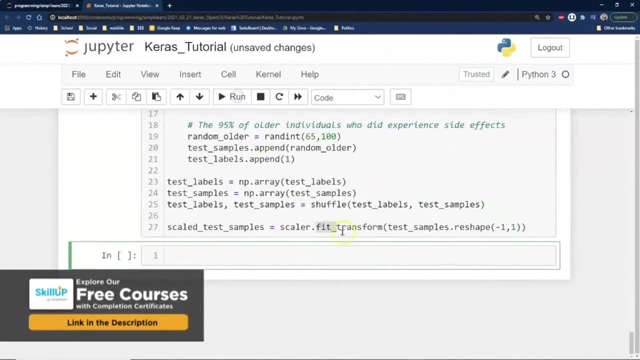 Well, it doesn't matter because the data is going to be across the same thing, But this should just be just transform down here instead of fit transform Because you don't want to refit your data on your testing data. There we go. 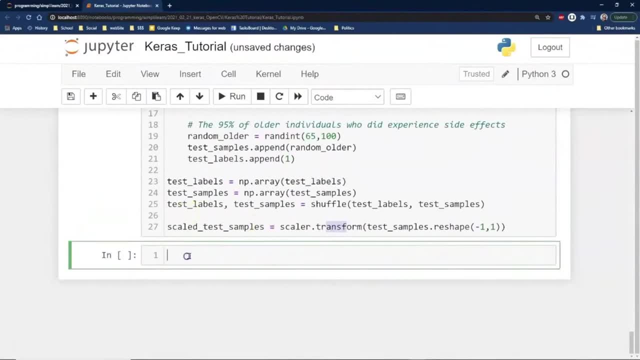 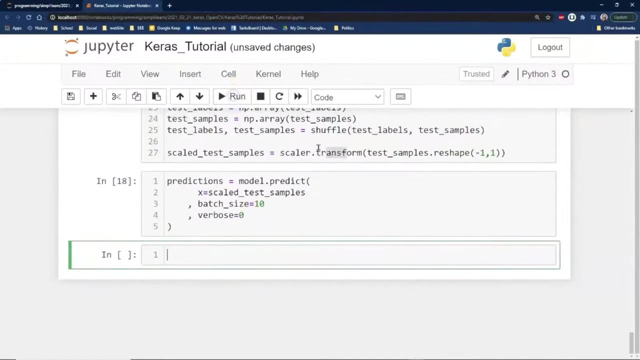 And now we're just transforming it because you never want to transform the test data- Easy mistake to make, especially on an example like this where we're not doing. you know we're randomizing the data anyway, So it doesn't matter too much because we're not expecting something weird. 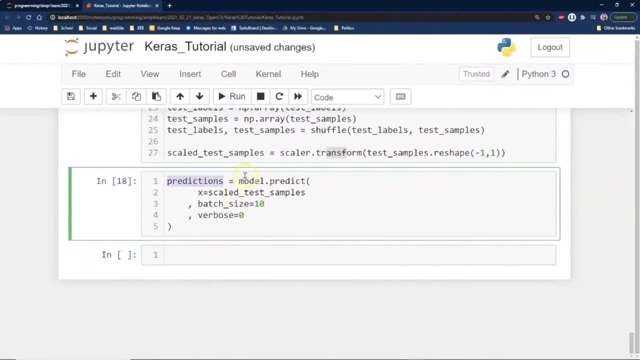 And then we went ahead and do our predictions. The whole reason we built the model is: we take our model, we predict And we're going to do: here's our X scale data: batch size 10,, verbose. And now we have our predictions in here. 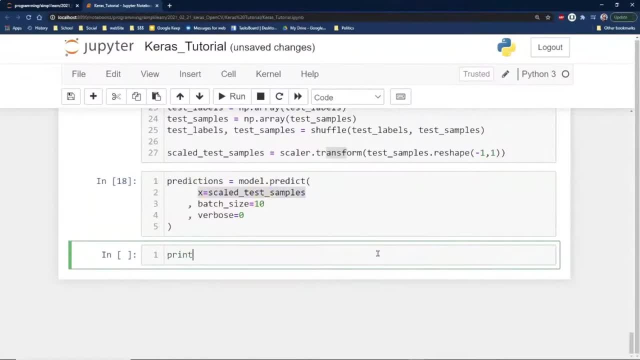 And we could go ahead and do a we'll print predictions And then I guess I could just put down predictions in five, So we can look at the first five of the predictions. 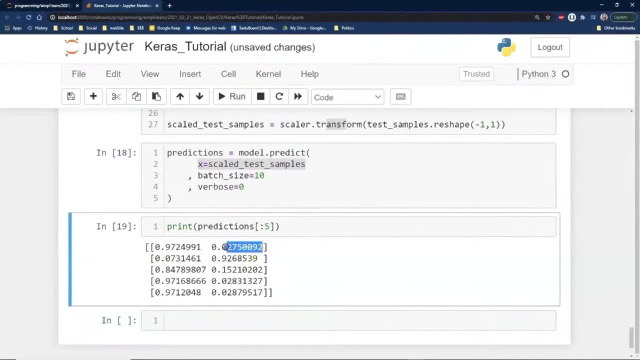 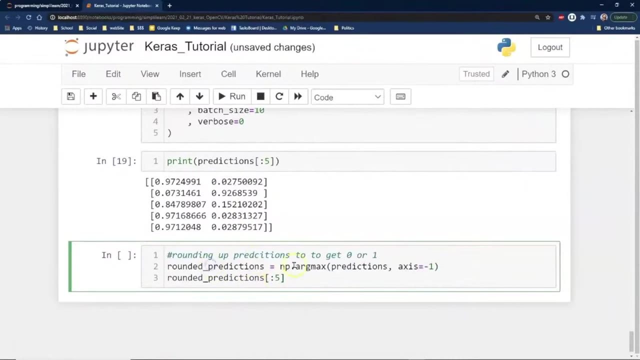 So what we have here is we have our age and the prediction on this age versus what we think it's going to be, What we think they're going to have- symptoms or not- And the first thing we notice is it's hard to read, because we really want a yes, no answer. 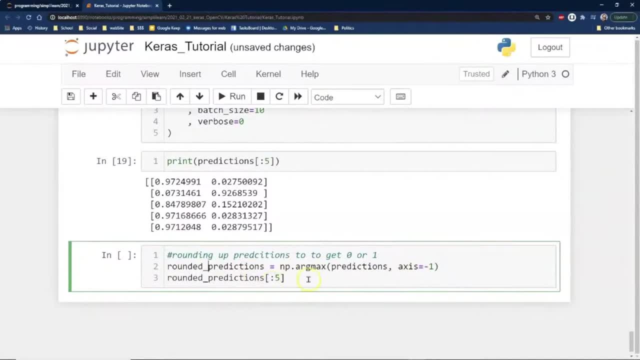 So we'll go ahead and just round off the predictions using the argmax, the numpy argmax for predictions, So it just goes to a zero one. If you remember, this is a Jupyter notebook, so I don't have to put the print. 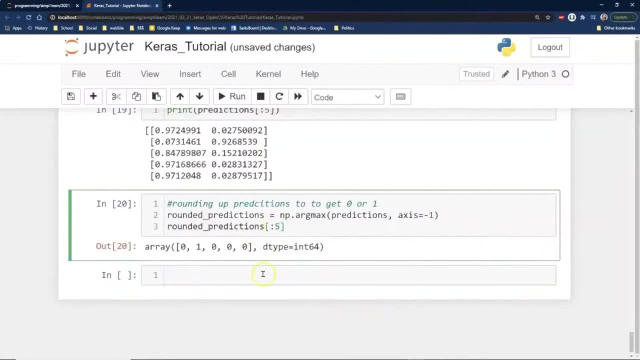 I can just put in rounded predictions and we'll just do the first five And you can see here: zero one, zero, zero, zero. So that's what the predictions are. that we have coming out of this Is no symptoms, symptoms, no symptoms, symptoms, no symptoms. 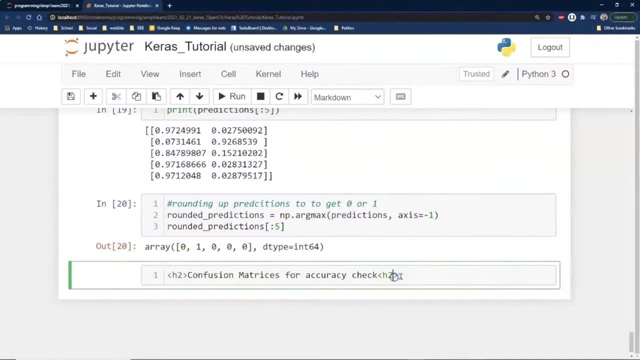 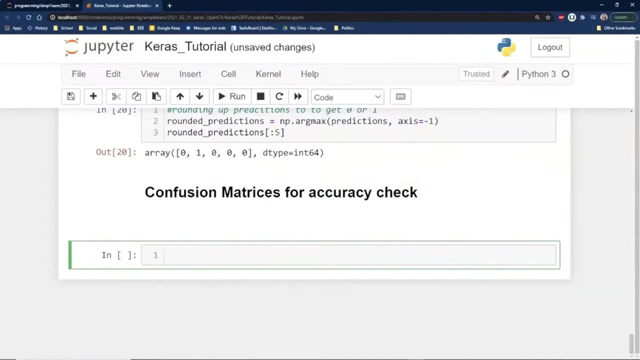 And, just as we were talking about at the beginning, we want to go ahead and take a look at this. There we go: Confusion matrixes for accuracy. check Most important part, when you get down to the end of the story, how accurate is your model? 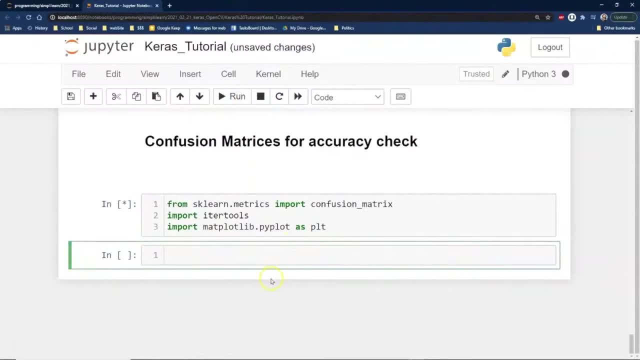 Before you go and play with the model and see if you can get a better accuracy out of it. And for this we'll go ahead and use the scikit, the sklearn metrics- Scikit being where that comes from- Import confusion matrix, some iteration tools and, of course, a nice matplotlib. 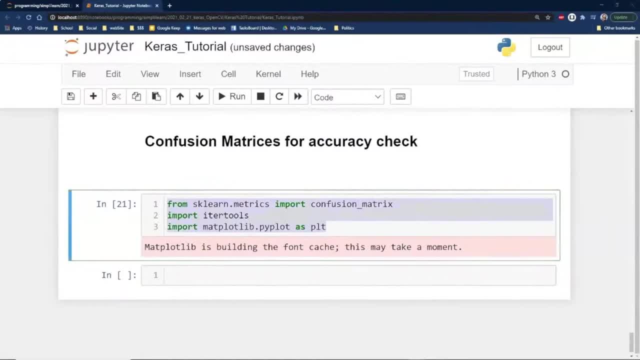 That makes a big difference. So it's always nice to, It's a nice graph to look at. Picture's worth a thousand words. And then we'll go ahead and call it cm for confusion. matrix. Why true equals test labels? Why predict rounded predictions? 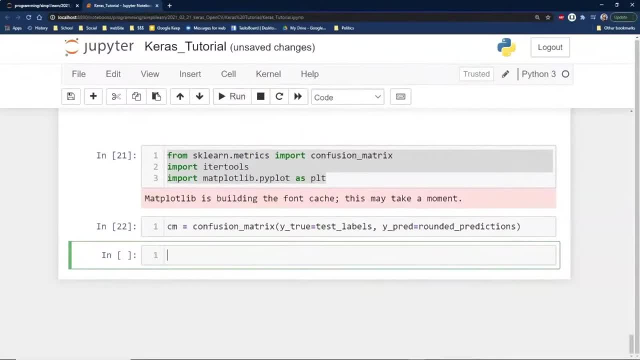 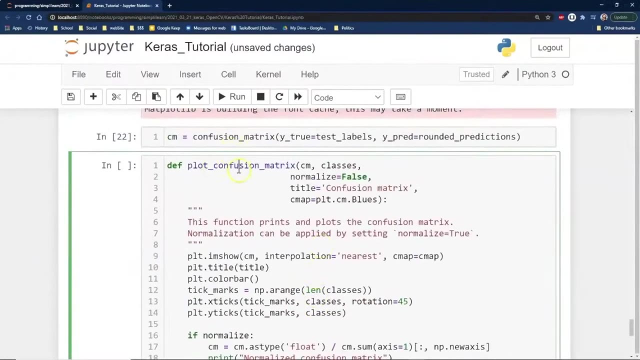 And we'll go ahead and load in our cm And I'm not going to spend too much time on the plotting Going over the different plotting code You can spend. We have whole tutorials on how to do your different plotting on there But we do have here is we're going to do a plot confusion matrix. 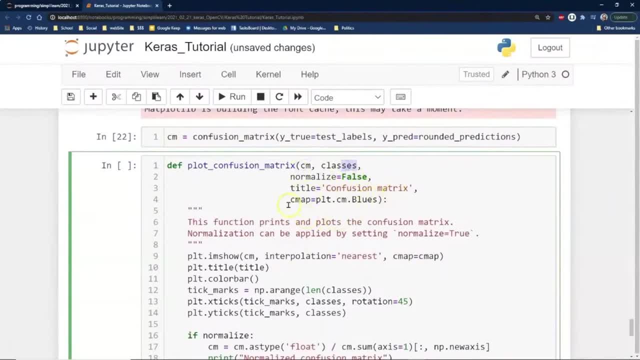 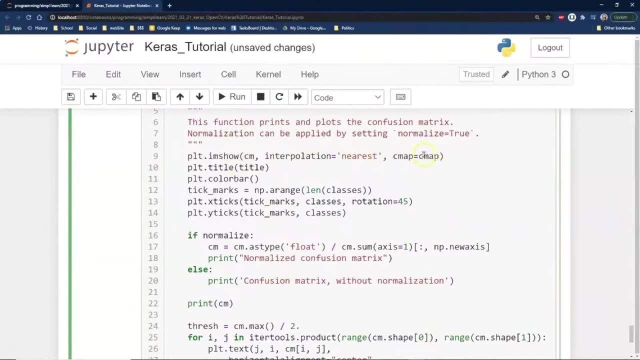 There's our cm, our classes, normalized false title confusion. matrix Cmap is going to be in blues And you can see here we have, to the nearest cmap titles, all the different pieces, Whether you put tick marks or not. 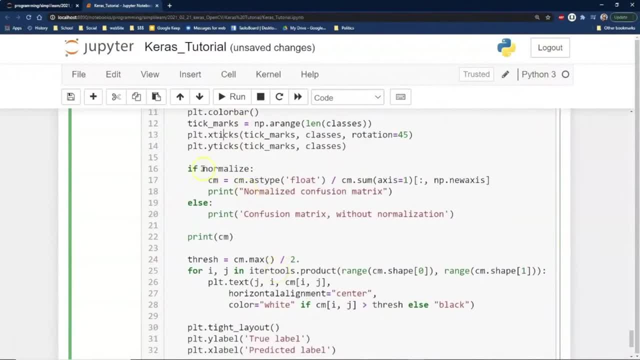 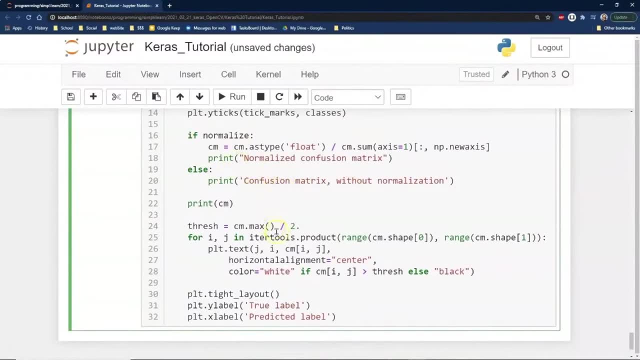 The marks, the classes, the color bar. So a lot of different information on here. As far as how we're doing the printing of the confusion matrix, You can also just dump the confusion matrix into a seaborn And real quick get an output. 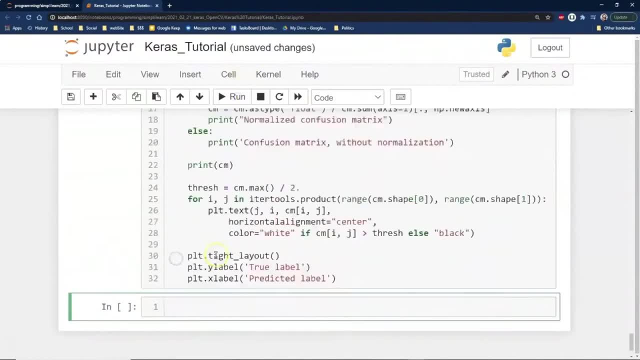 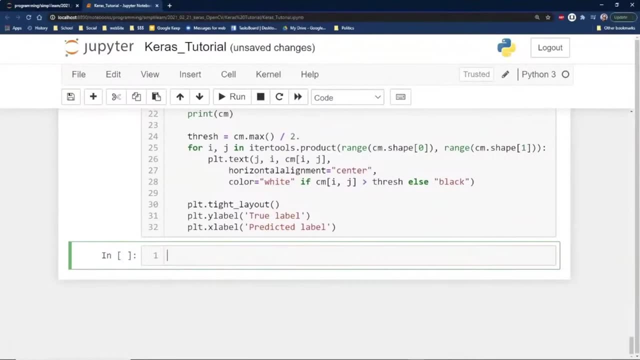 It's worth knowing how to do all this When you're doing a presentation to the shareholders. You don't want to do this on the fly. You want to take the time to make it look really nice, Like our guys in the back did. 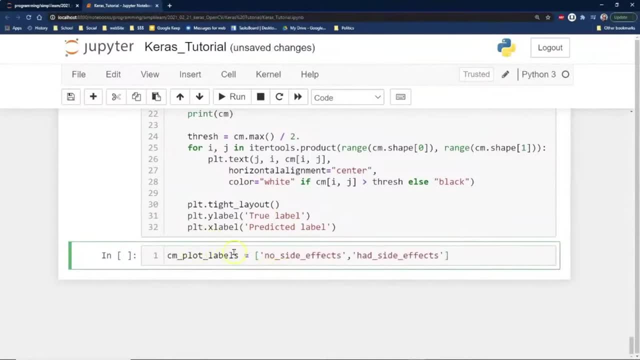 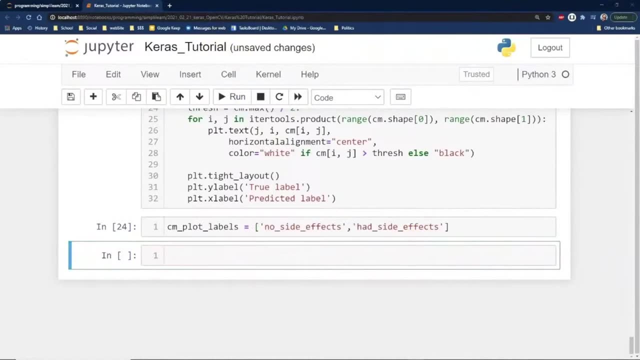 And let's go ahead and do this. We've got to put together our cm plot labels. We'll go ahead and run that. We'll go ahead and call the definition for our mapping And you can see here plot confusion matrix. That's the little script we just wrote. 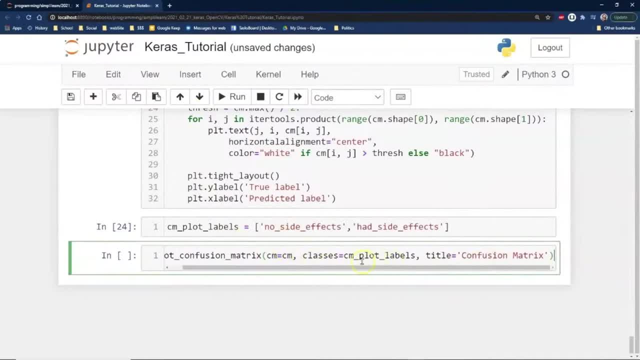 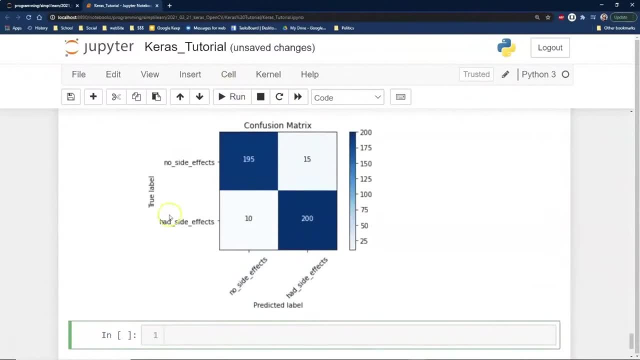 And we're going to dump our data into it. So our confusion matrix, our classes title confusion matrix, And let's just go ahead and run that And you can see, here we have our basic setup. No side effects: 195.. Had side effects: 200. 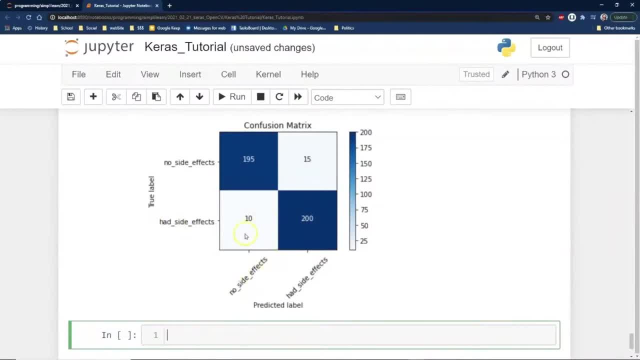 No side effects. that had side effects. So we predicted the 10 of them Who actually had side effects And that's pretty good. I mean, I don't know about you, But that's 5% error on this And this is because there's 200 here. 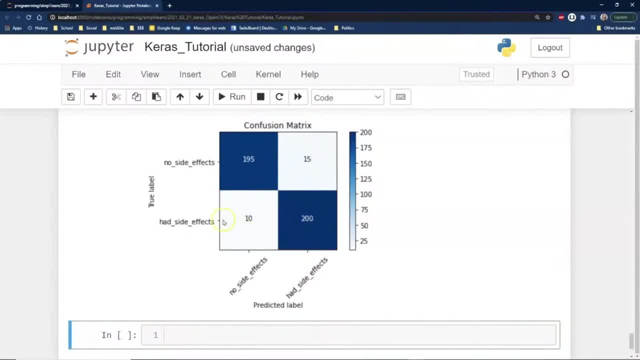 That's where I get 5%. Divide these both by 2. And you get 5 out of 100.. You can do the same kind of math up here, Not as quick on the fly, because it's 15 and 195. 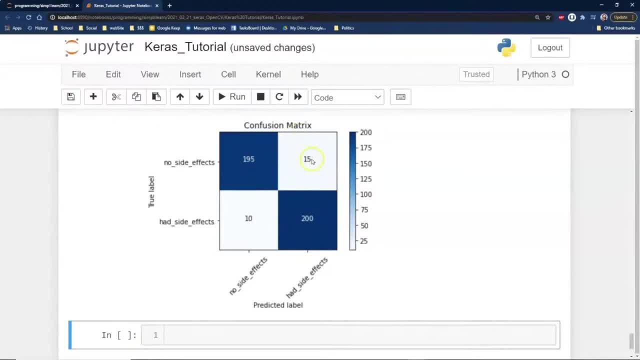 Not an easily rounded number But you can see here where they have 15 people Who predicted to have no With the no side effects, but had side effects Kind of setup on there And these confusion matrix are so important at the end of the day. 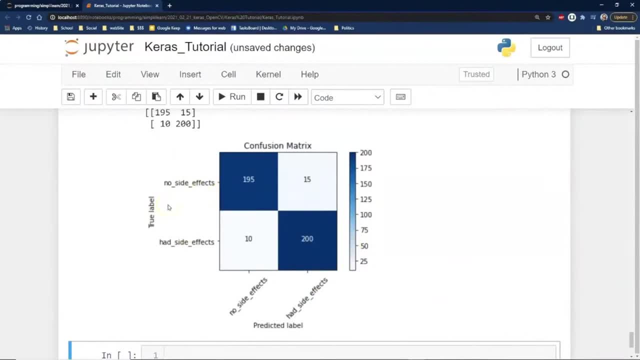 This is really where you show whatever you're working on comes up And you can actually show them. hey, this is how good we are or not. How messed up it is. So this was a. I spent a lot of time on some of the parts. 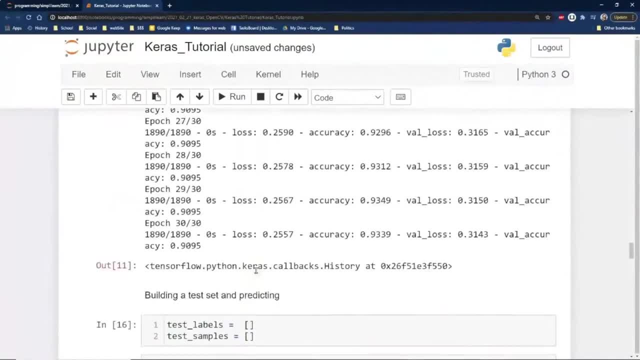 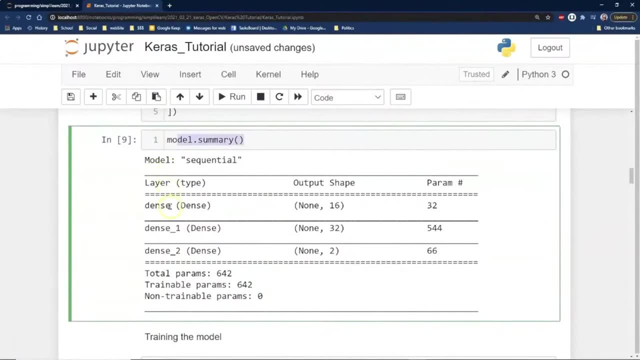 But you can see here it's really simple. We did the random generation of data But when we actually built the model coming up here, Here's our model summary And we just have the layers on here that we built with our model on this, 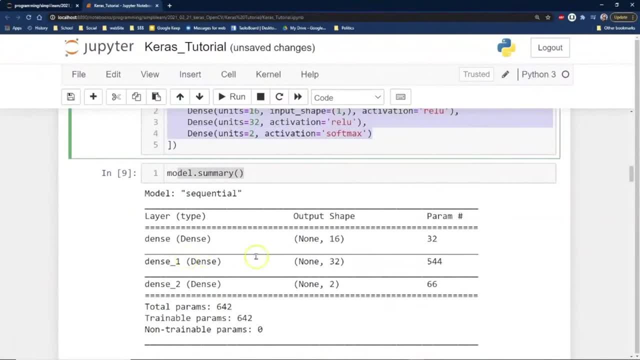 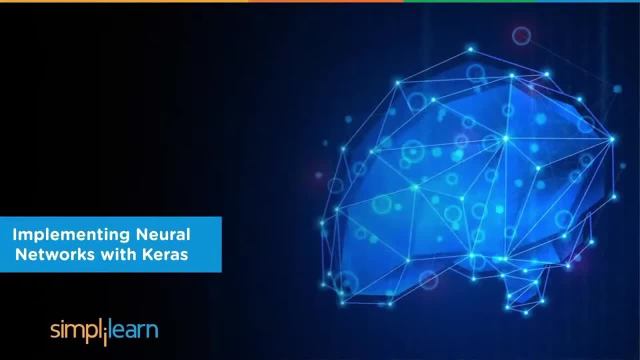 And then we went ahead and trained it and ran the prediction. Now we can get a lot more complicated. Let me flip back over here because we're going to do another demo. So that was our basic introduction to it. We talked about the 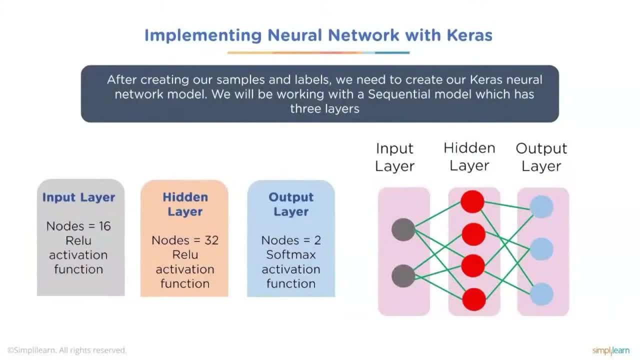 So implementing a neural network with Keras. After creating our samples and labels, We need to create our Keras neural network model. We will be working with a sequential model which has three layers, And this is what we did. We had our input layer. 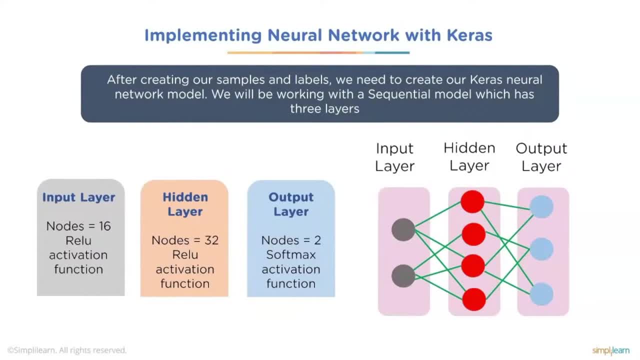 Our hidden layers And our output layers And you can see the input layer coming in Was the age factor. We had our hidden layer And then we had the output. Are you going to have symptoms or not? So we're going to go ahead and go with something a little bit more complicated. 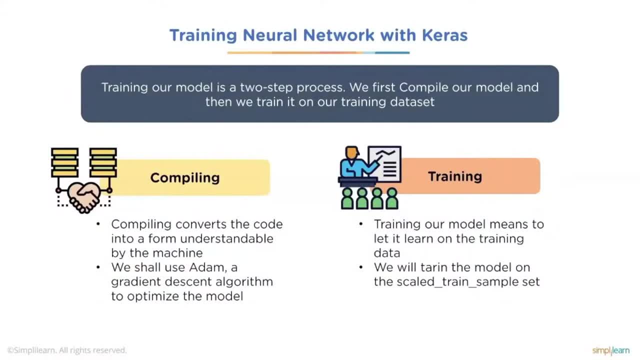 Training our model is a two-step process. We first compile our model And then we train it in our training data set. So we have compiling. Compiling converts the code into a form of understandable by machine. We use the atom in the last example. 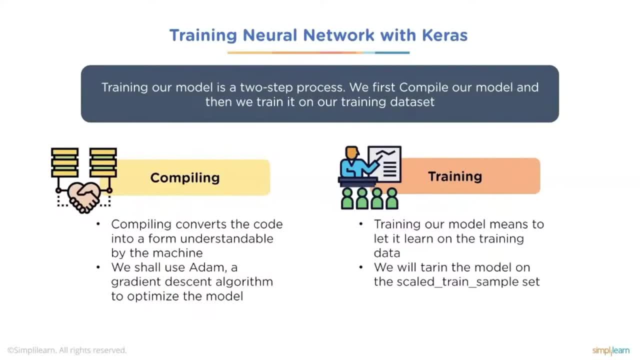 A gradient descent algorithm to optimize a model. And then we trained our model, Which means it let it learn on training data, And I actually had it a little backwards there, But this is what we just did. If you remember from our code, we just had 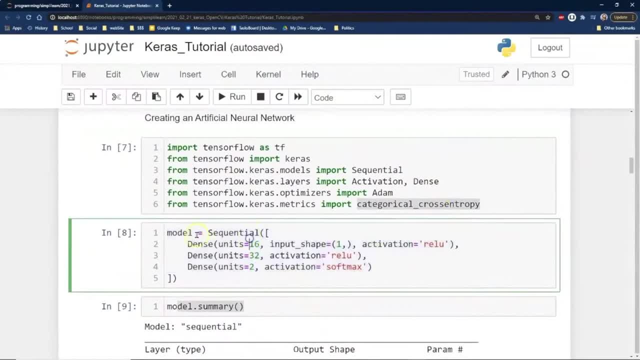 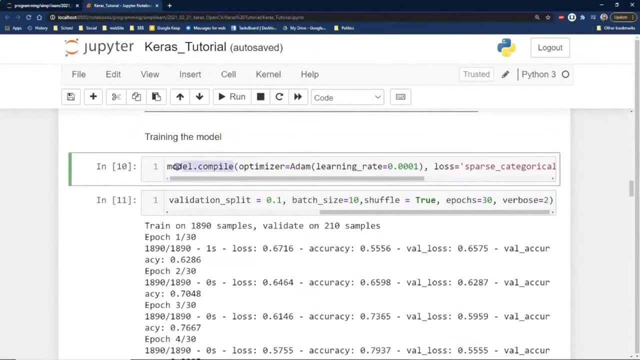 Let me go back here. Here's our model that we created Summarized. We come down here and we compile it. So it tells it: hey, we're ready to build this model and use it, And then we train it. This is the part where we go ahead and fit our model. 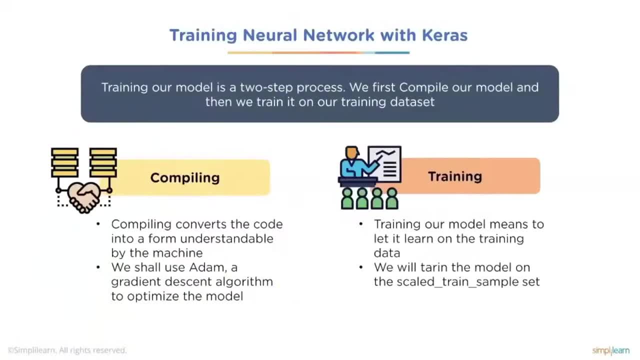 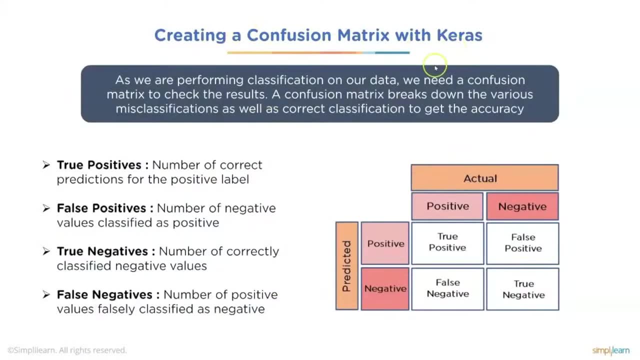 And put that information in here And it goes through the training on there And of course, we scaled the data, which was really important to do, And then you saw we did the creating a confusion matrix with Keras As we are performing classifications on our data. 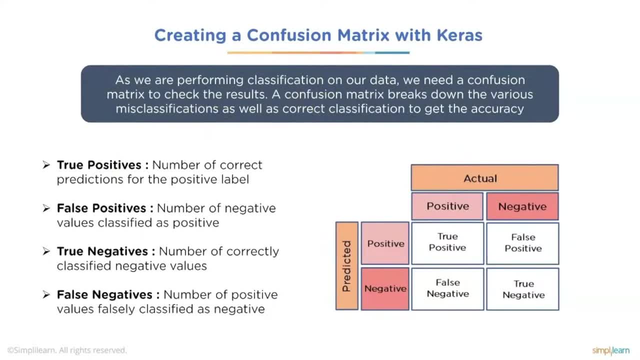 We need a confusion matrix to check the results. A confusion matrix breaks down the various misclassifications As well as correct classifications to get the accuracy. And so you can see here: This is what we did with the true positive, False positive. 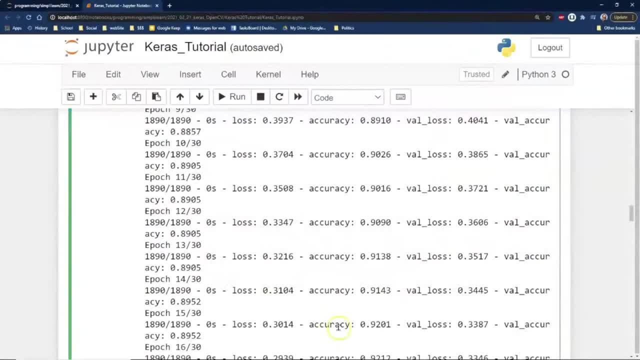 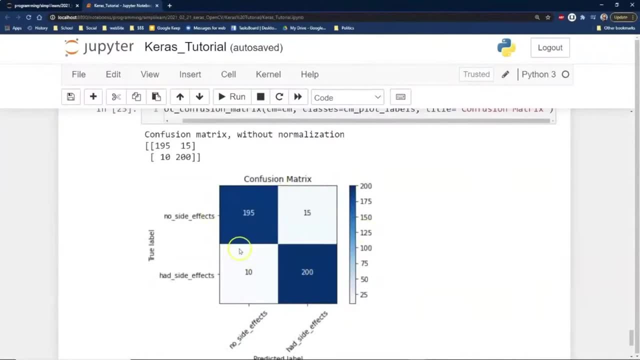 True negative, False negative, And that is what we went over. Let me just scroll down here On the end. We printed it out And you can see we have a nice printout of our confusion matrix With the true positive, False positive. 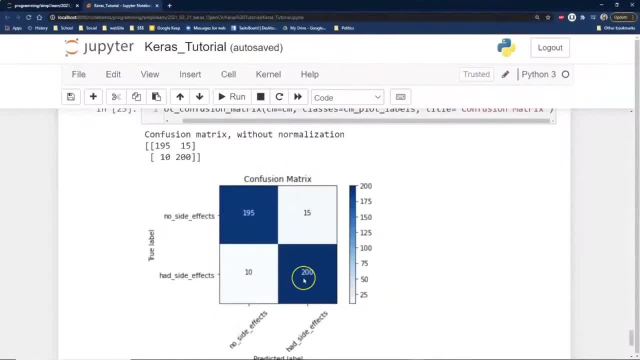 False, negative, True, negative. So the blue ones: We want those to be the biggest numbers, Because those are the better side. And then we have our false predictions on here, As far as this one. So it had no side effects, But we predicted. 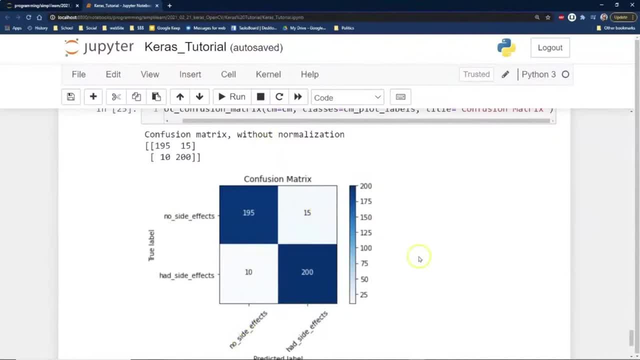 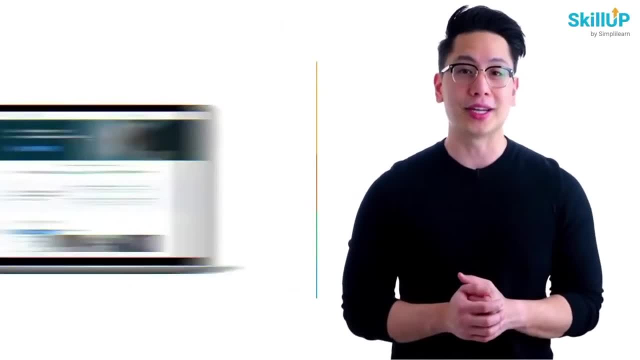 Let's see No side effects Predicting side effects And vice versa. If getting your learning started is half the battle, What if you could do that for free? Visit ScaleUp by SimplyLearn. Click on the link in the description to know more. 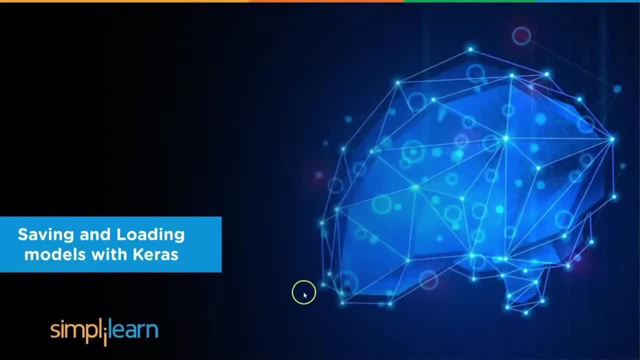 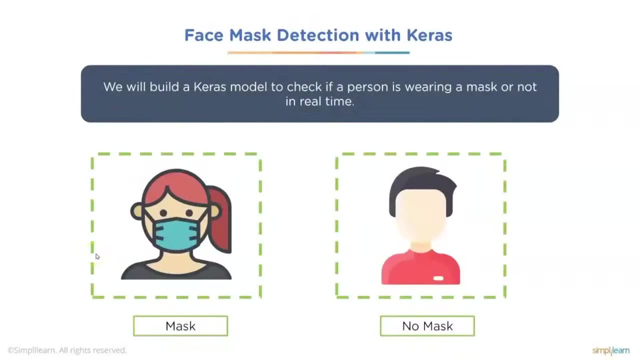 Now saving and loading models with Keras. We're going to dive into a more complicated demo And you're going to say, Oh, that was a lot of complication before. Well, if you broke it down, We randomized some data, We created the Keras setup. 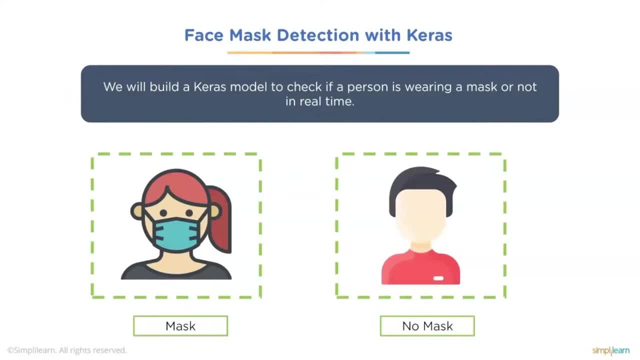 We compiled it, We trained it, We predicted And we ran our matrix. So we're going to dive into something a little bit more fun. We're going to do a face mask detection with Keras, So we're going to build a Keras model. 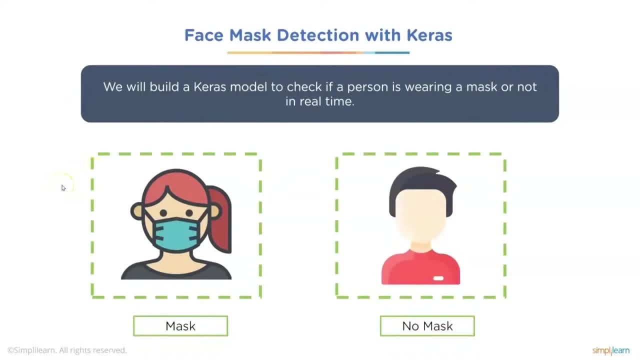 To check if a person is wearing a mask or not In real time, And this might be important If you're at the front of a store. This is something today Which might be very useful As far as making sure people are safe. 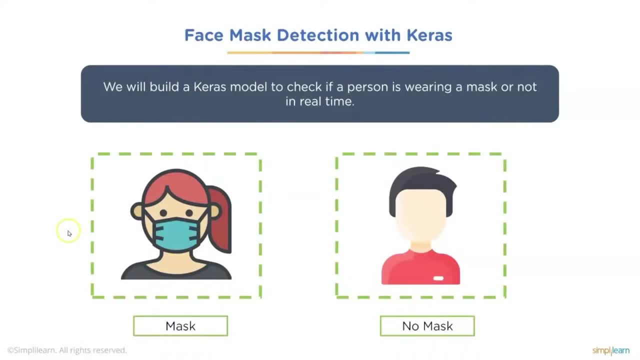 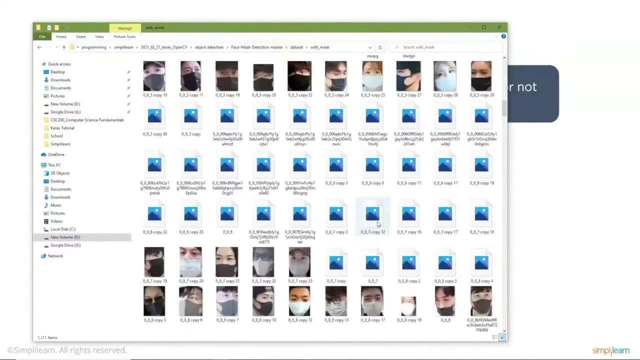 And so we're going to look at mask and no mask. And let's start with a little bit on the data. And so MID I have with a mask You can see they just have a number of images Showing the people in masks. 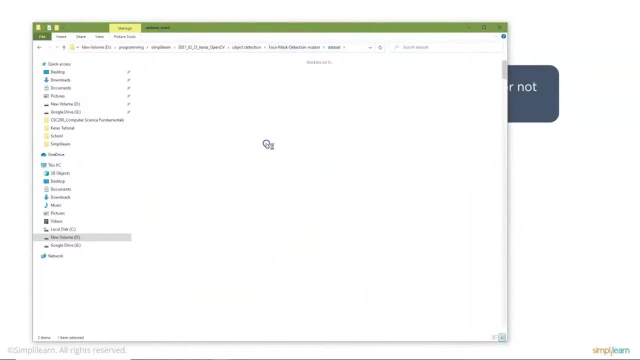 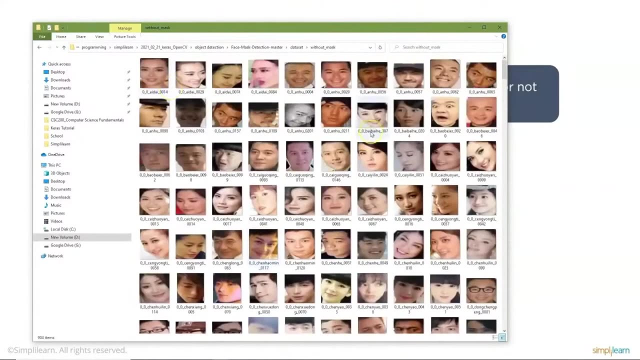 And again, If you want some of this information, Contact, Simply Learn, And they can send you some of the information As far as people with and without masks, So you can try it on your own, And this is just such a wonderful example. 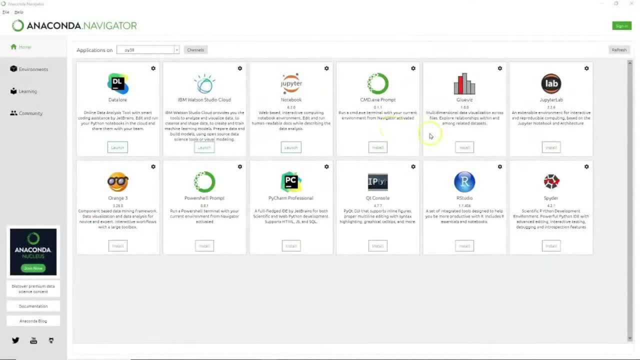 Of this setup on here. So before I dive into the mask detection, Talking about being in the current with COVID And seeing if people are wearing masks- This particular example I had to go ahead and update to a Python 3.8 version. 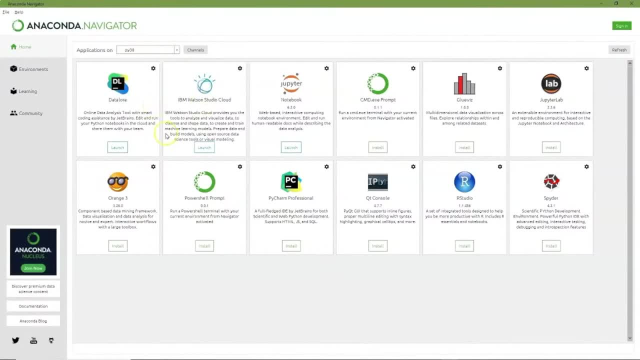 It might run in a 3.7.. I'm not sure. I kind of skipped 3.7 and installed 3.8.. So I'll be running in a Python 3.8.. And then you also want to make sure your TensorFlow is up to date. 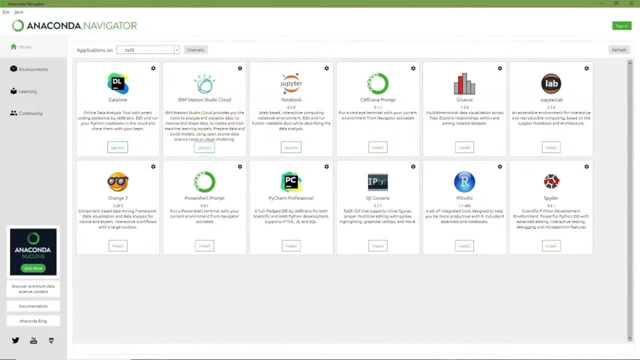 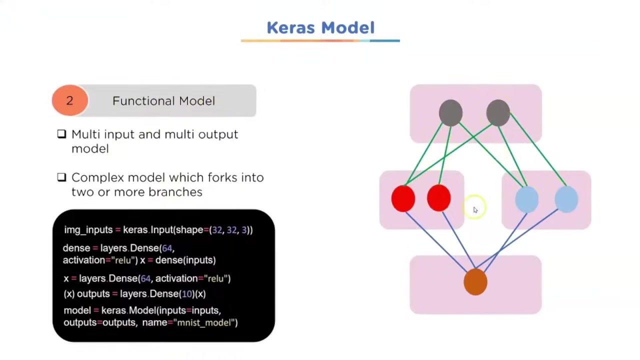 Because the call functional layers. That's where they split, If you remember correctly from back. Let's take a look at this. Remember from here The functional model And a functional layer Allows us to feed in the different layers Into different nodes. 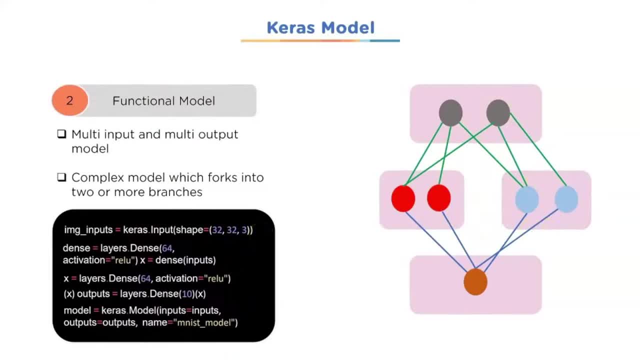 Into different layers And split them. Very powerful tool, Very popular right now In the edge of where things are with neural networks And creating a better model. So I've upgraded to Python 3.8.. And let's go ahead and open that up. 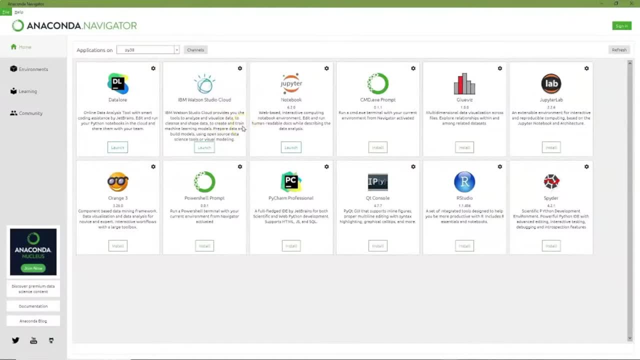 And go through our next example, Which includes multiple layers: Programming it to recognize whether someone wears a mask or not And then saving that model so we can use it in real time. So we're actually almost a full end-to-end development of a product here. 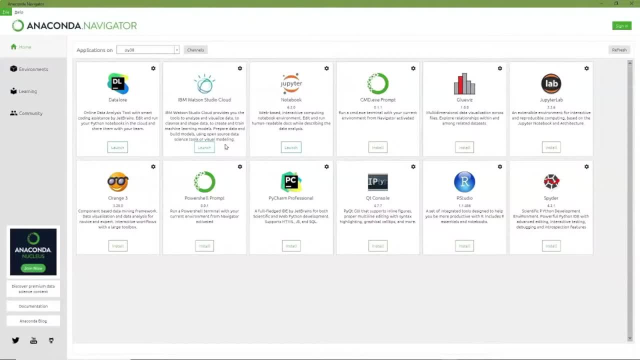 Of course, this is a very simplified version, And there'd be a lot more to it. You'd also have to do like recognizing whether it's someone's face or not. All kinds of other things go into this, So let's go ahead and jump into that code. 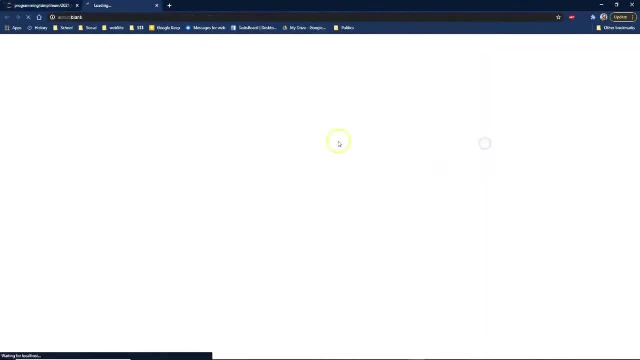 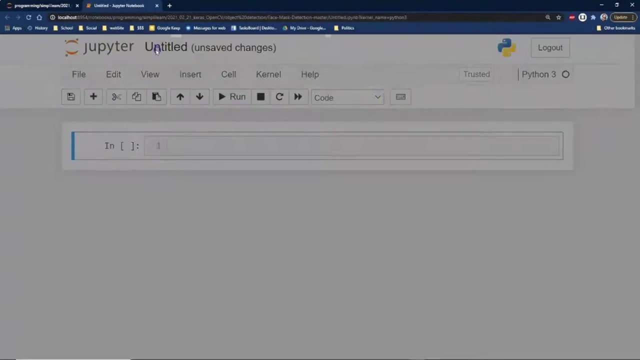 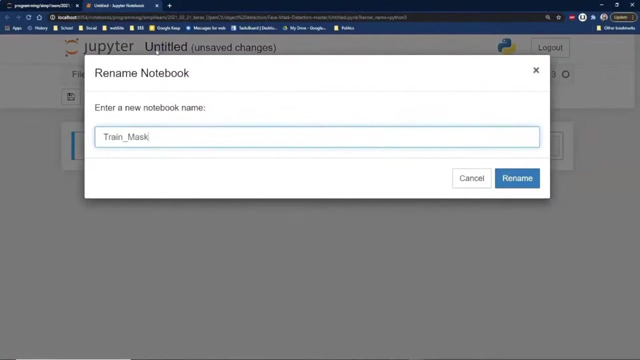 And we'll open up a new Python 3.. Python 3.. It's working on it. There we go. And then we want to go ahead and train our mask. We'll just call this train mask And we want to go ahead and train mask and save it. 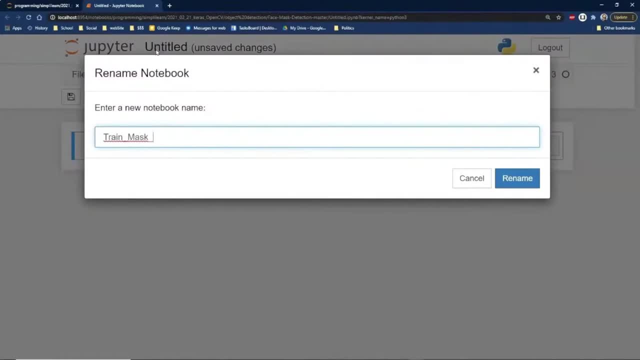 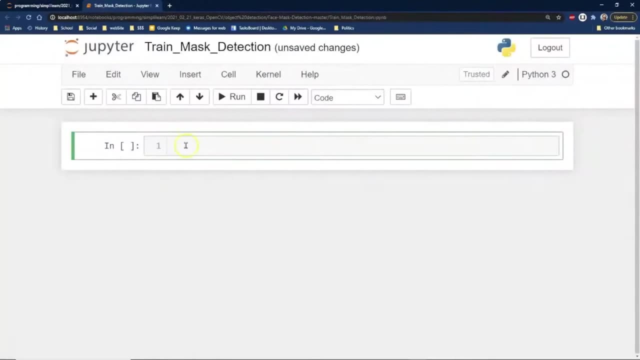 So it's save mask Train, mask detection, Not to be confused with masking data. A little bit different. You're talking about a physical mask on your face And then, from the cross standpoint, We've got a lot of imports to do here. 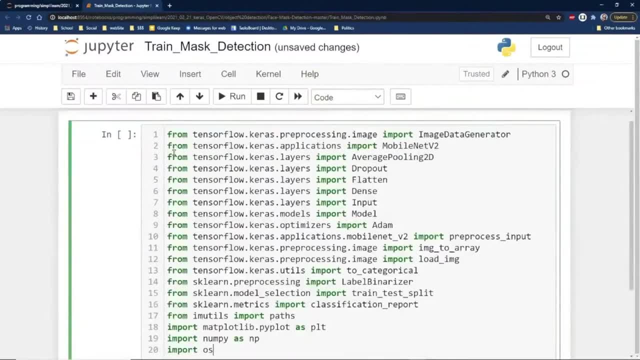 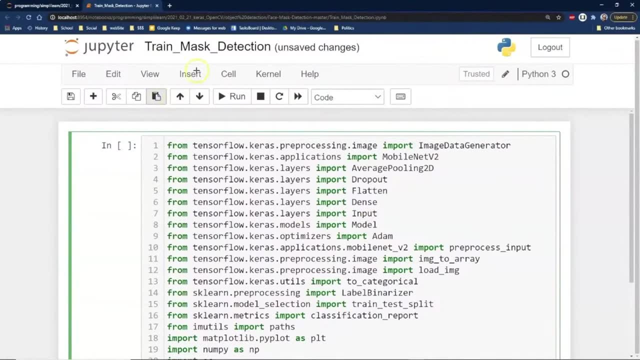 And I'm not going to dig too deep on the imports, We're just going to go ahead and notice a few of them. So we have in here- Oops, I'm going to go alt D, There we go, Have something to draw with a little bit here. 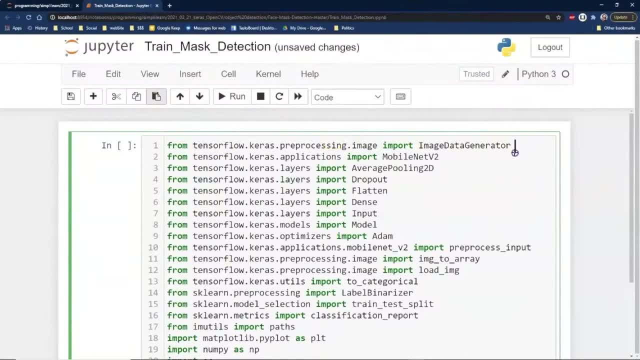 We have our image processing, And the image processing- right here, Let me underline that- Deals with how do we bring images in, Because most images are like a square grid And then each value in there has three values for the three different colors. 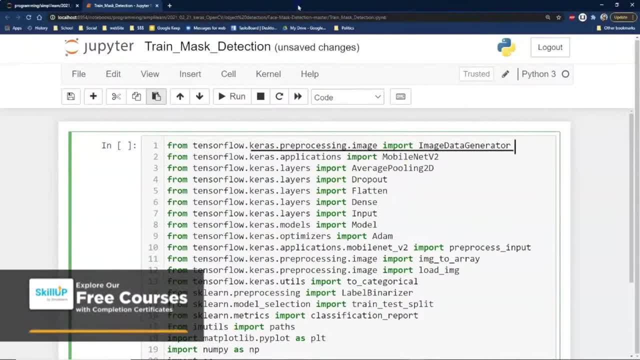 Cross and TensorFlow do a really good job of working with that, So you don't have to do all the heavy listening and figuring out what's going to go on. And we have the mobile net average pooling 2D. This again is: How do we deal with the images and pooling them? 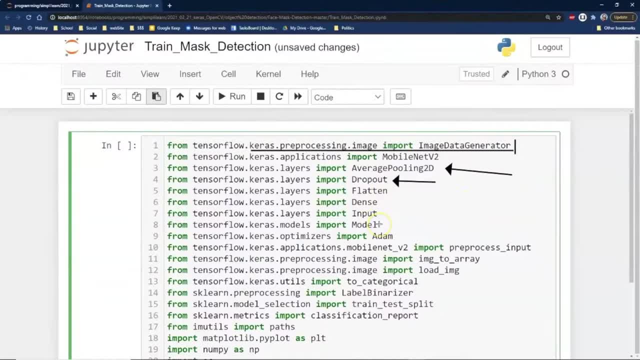 Dropout's a cool thing Worth looking up. If you haven't, As you get more and more into Keras and TensorFlow, It'll auto drop out certain notes. That way you'll get a better. The notes just kind of die. They find that they actually create more of a bias than a help. 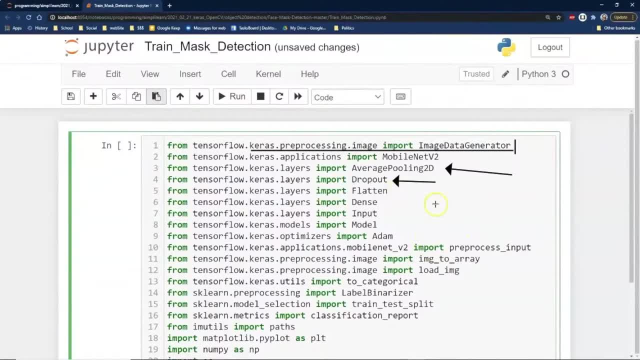 And they also add processing time, So they remove them And then we have our flatten. That's where you take that huge array With the three different colors And you find a way to flatten it. So it's just a one dimensional array. 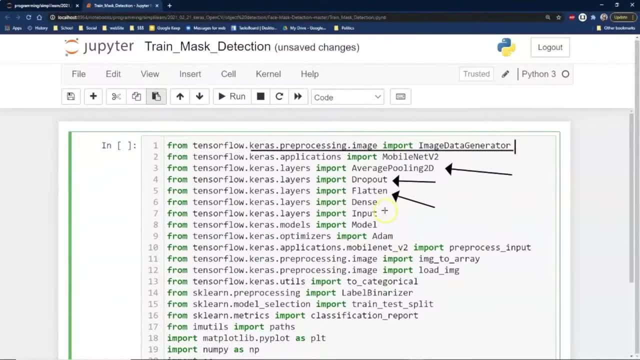 Instead of a two by two by three Dense input. We did that in the other one, So that should look a little familiar. Oops, There we go, Our input, Our model. Again, these are things we had in the last one. 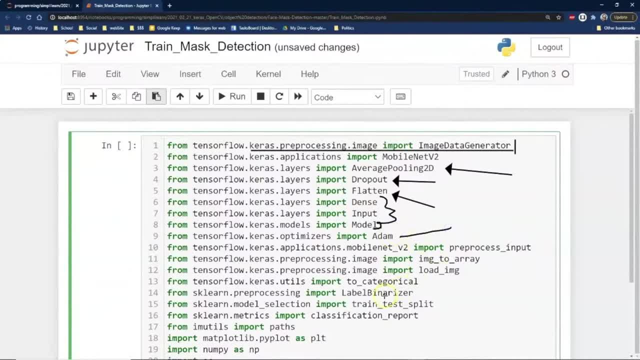 Here's our optimizer with our atom. We have some pre-processing on the input That goes along with bringing in the data in. More pre-processing with image to image. More pre-processing with image to array, Loading the image. This stuff is so nice. 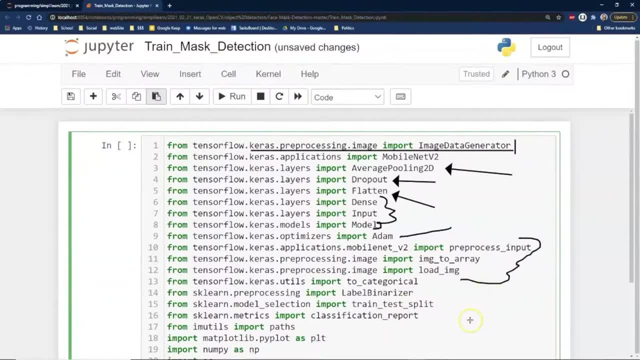 It looks like a lot of work. You have to import all these different modules in here, But the truth is it does everything for you. You're not doing a lot of pre-processing, You're letting the software do the pre-processing. And we're going to be working with the 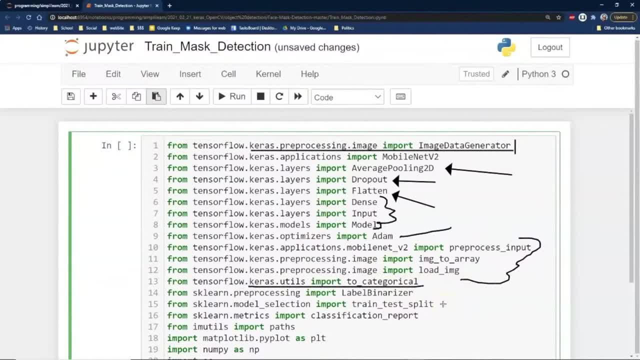 Setting something to categorical Again. that's just a conversion from a number to a category Zero one doesn't really mean anything. It's like true, false, It's. There's our label. by as a The same thing, We're changing our labels. 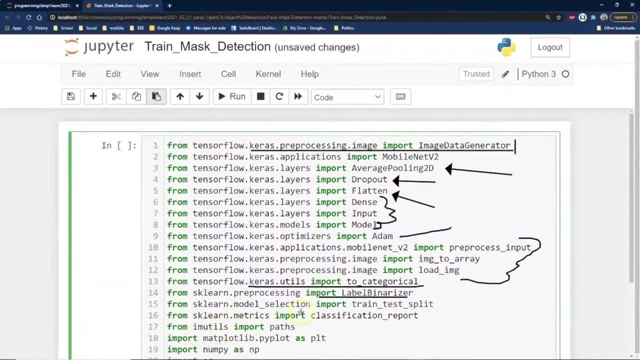 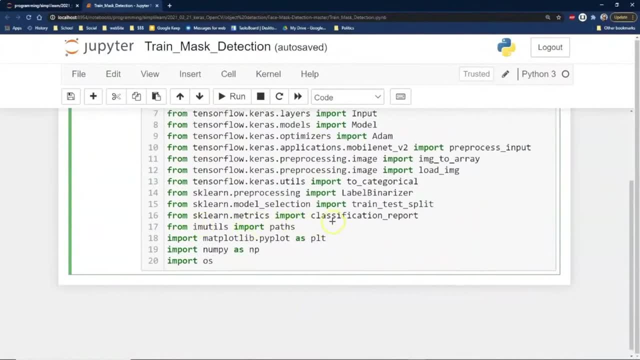 Around. And then there's our train test Split classification report, our I, I am utilities. Let me just go ahead and scroll down here, not for these. This is something a little different. going on down here. This is not part of the. 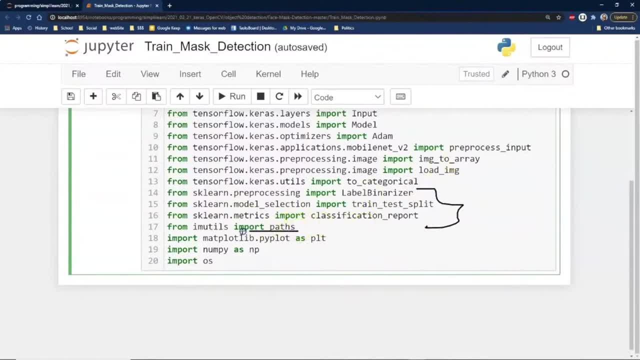 TensorFlow or the SK learn. This is the side kit setup of open CV and we'll actually have another tutorial going out with the open CV. so if you want to know more about open CV, you'll get a glance on it in this software, especially the second piece when we reload up the data and 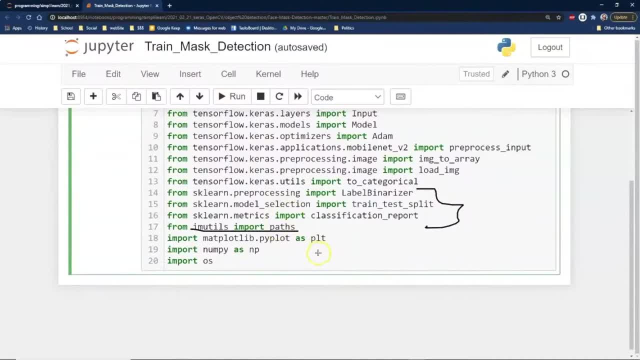 hook it up to a video camera. we're going to do that on this round, but this is part of the open CV thing and you'll see cv2 is usually how that's referenced. but the IM utilities has to do with how do you rotate pictures around and stuff. 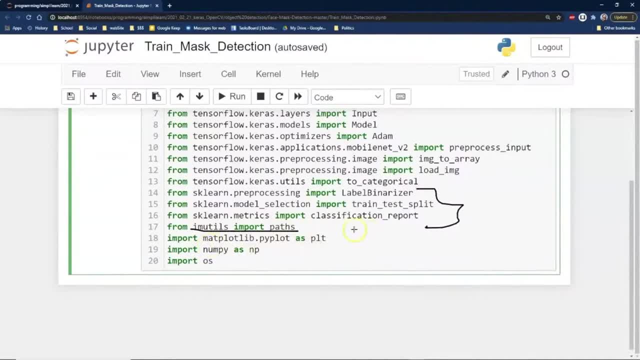 like that and resize them. and then the matplotlib for plotting- cuz it's nice to have a graph tells us how good we're doing- and then, of course, our numpy numbers array and just a straight OS access. Wow, so that was a lot of imports. like I said, I'm not gonna spend. I spent a. 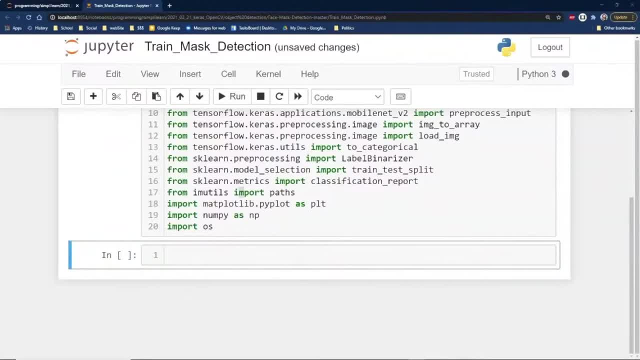 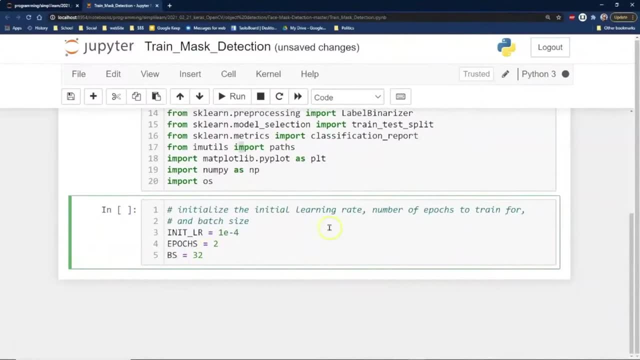 little time going through them, but we didn't want to go too much into them, and then I'm gonna create some variables that we need to go ahead and initialize. we have the learning rate, number of epics to train for, and the battery time and the return to the other one. so that's going to use the 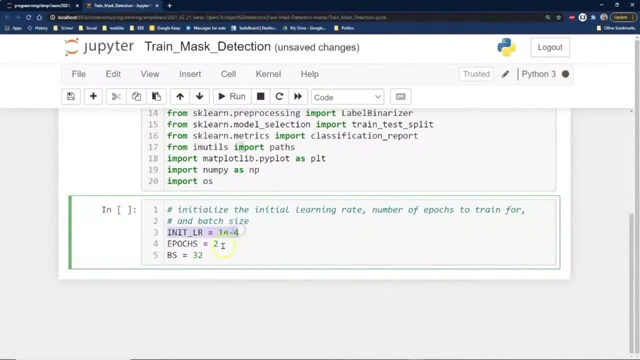 size and if you remember correctly we talked about the learning rate- to the negative four: point oh oh oh one. a lot of times is point oh oh one or point oh oh one. usually it's in that variation, depending on what you're doing and how many epics and they kind of play with the epics. the epics is how many times. 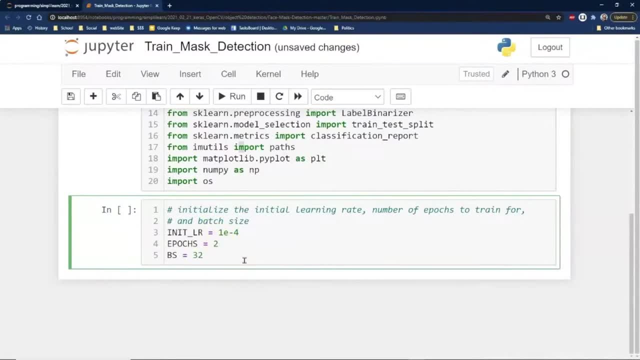 we're going to go through all the data and now I have it. as to, the actual setup is for 20, and 20 works great. the reason I have it for two is it takes a long time to process. one of the downsides of Jupiter is that Jupiter isolates it to a 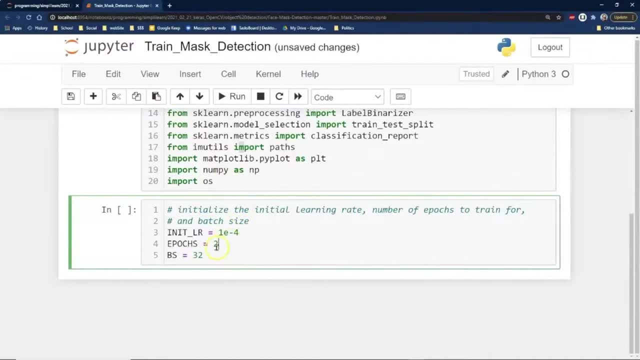 single kernel. so even though I'm on an eight core processor with 16 dedicated threads, only one thread is running on this, no matter what, so it doesn't matter. so it takes a lot longer to run, even though tensorflow really skills up nicely and the batch size. 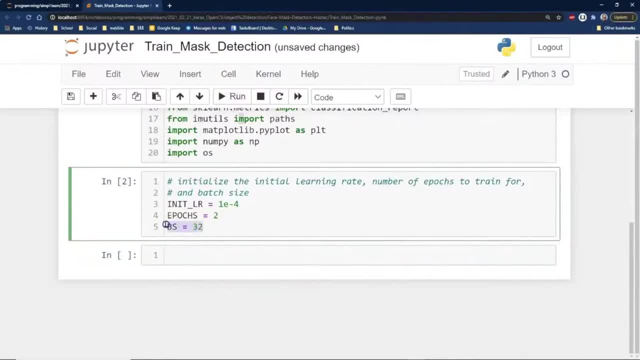 is how many pictures we load it once in process. again, those are numbers you have to learn to play with, depending on your data and what's coming in, and the last thing we want to go ahead and do is there's a directory with the data set we're going to run and this just has images of bass and not masks. and if we 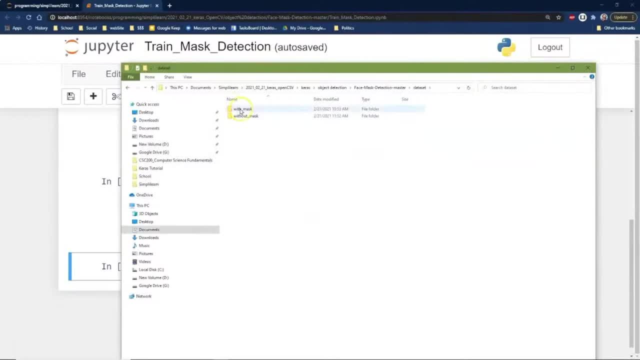 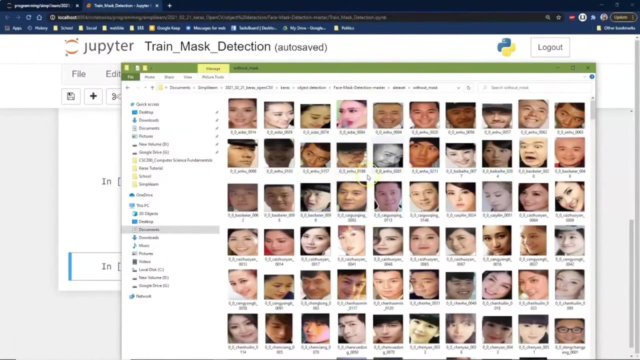 go in here you'll see data set and you have pictures with mass. they're just images of people with mass on their face and then we have the opposite and go back up here without masks. so it's pretty straightforward. they look kind of askew because they tried to format them into very similar setup on there. so 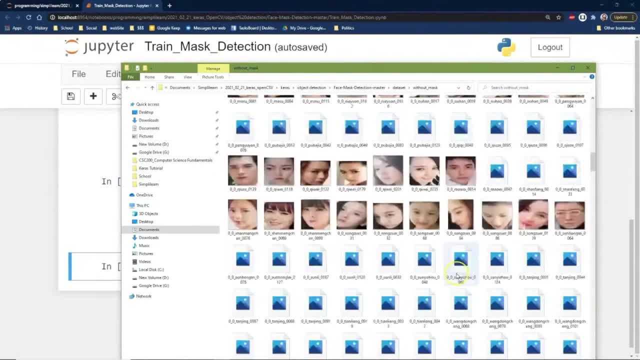 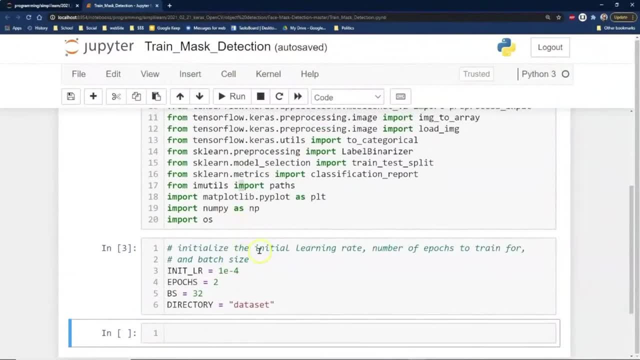 they're. they're mostly squares. you'll see some that are slightly different on here, and that's kind of important thing to do on a lot of these data sets: get them as close as you can to each other and we'll- we actually will- run in the in. 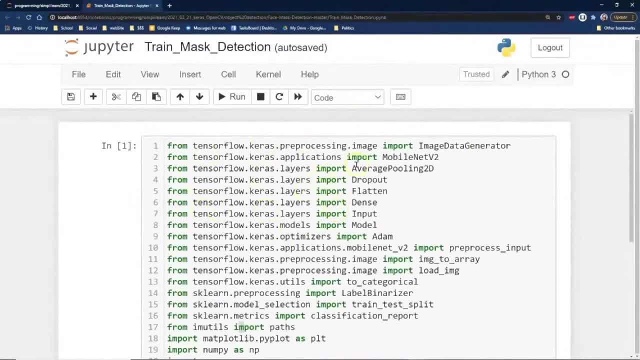 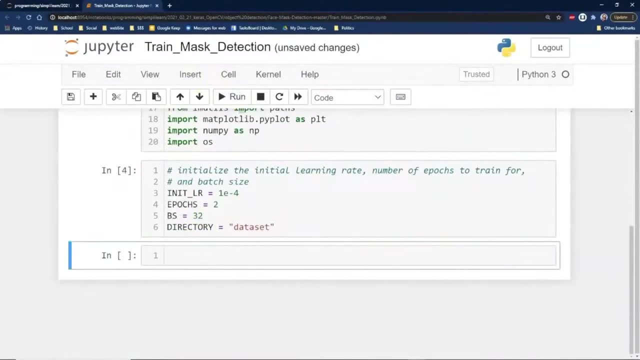 this processing of images up here and the cross layers and importing and dealing with images. it does such a wonderful job of converting these that a lot of it we don't have to do a whole lot with. so you have a couple things going on there, and so we're now going to be. this is now. 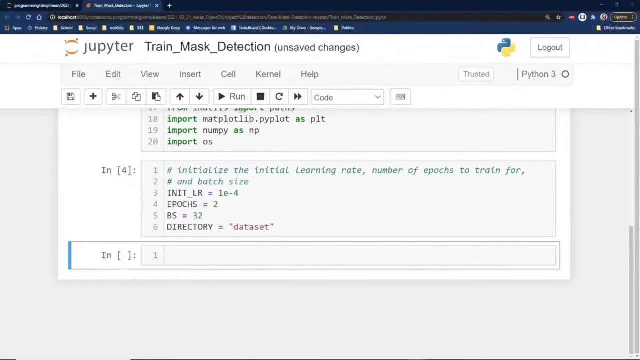 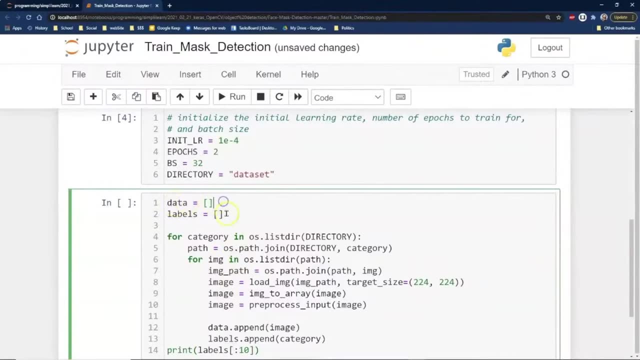 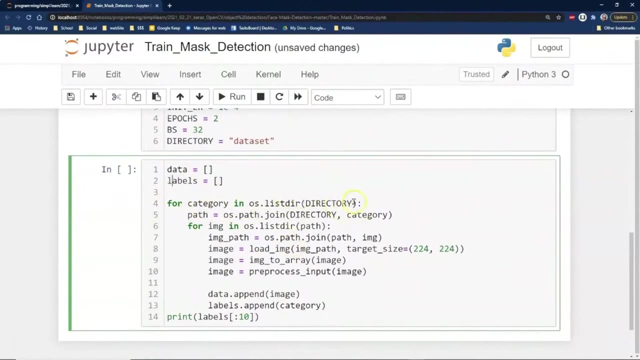 loading the images and let me see, we'll go ahead and create data and labels. here's our, here's the features going in, which is going to be our pictures and our labels going out, and then for categories, in our list, directory, directory, and if you remember, I just flashed that at you, it had. 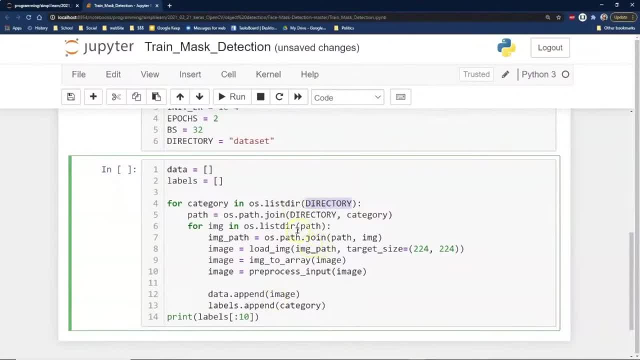 face mask or no face mask. those are the two options and we're just going to load in to that. we're going to pin the image itself and the labels. so we'll just create a huge array and you can see right now this could be an issue if you. 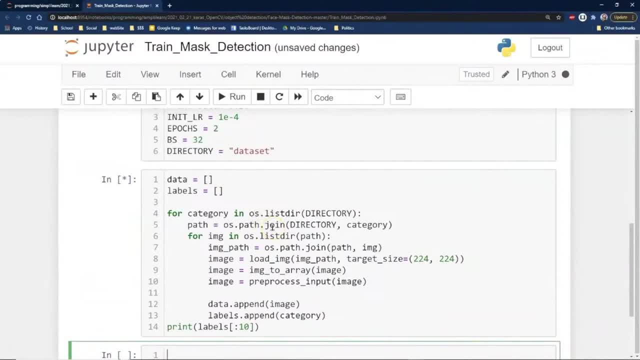 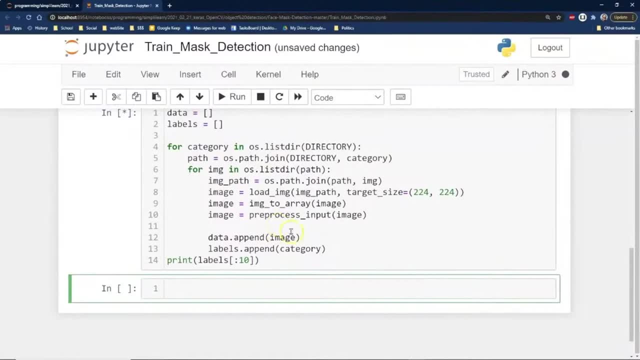 had more data at some point. thankfully, I have a 32 gig hard drive or RAM. even that doesn't, you could do with a lot less of that. probably under 16 or even 8 gigs would easily load all this stuff, and then we'll go ahead and create a new. 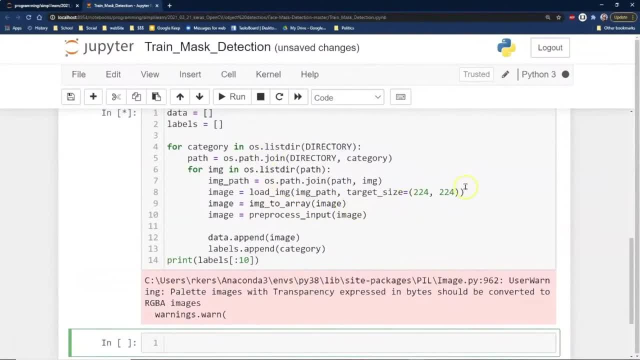 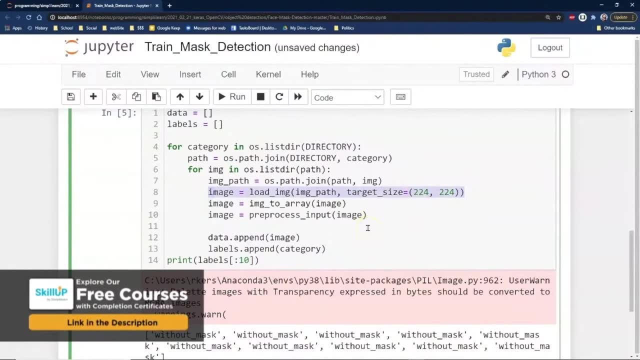 image here and we'll go ahead and create a new image here and we'll go ahead and a conversion going on in here. i told you about how we are going to convert the size of the image so it resizes all the images and that way our data is all identical the way it comes in and you can see. 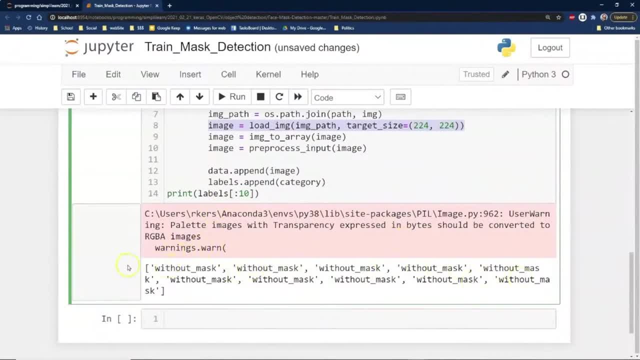 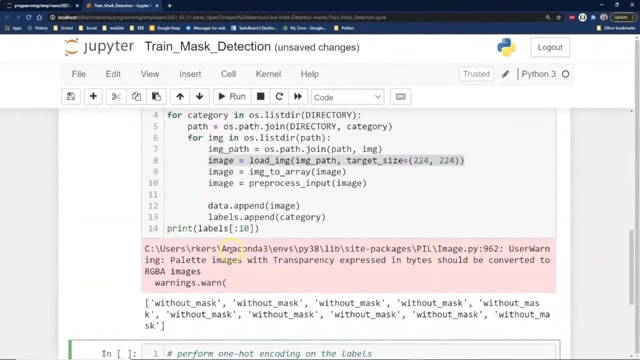 here with our labels we have without mask, without mask, without mask. the other one would be with mask. those are the two that we have going in there and then we need to change it to the one hot encoding and this is going to take our up here we had, was it labels and data. we want the labels to be. 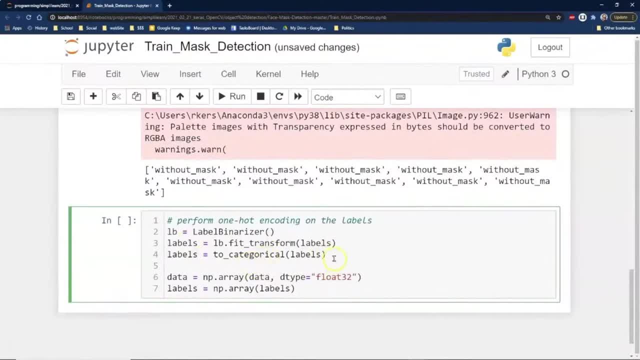 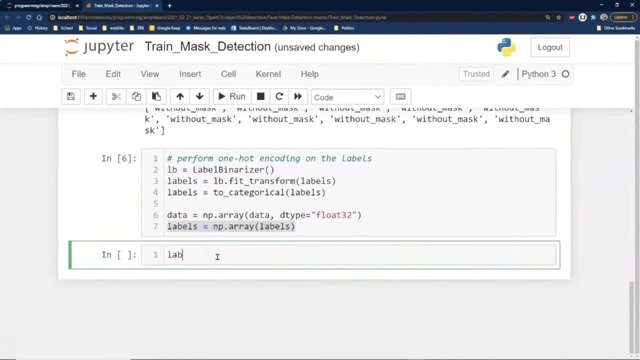 categorical. so we're going to take labels and change it to categorical and our labels then equal a categorical list. we'll run that and again, if we do labels and we just do the last or the first 10, let's do the last 10 just because minus 10 to the end. there we go. 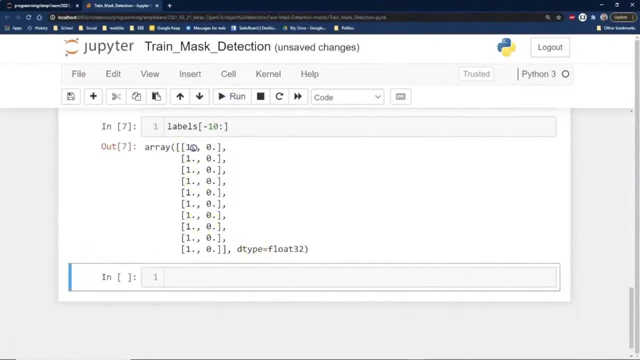 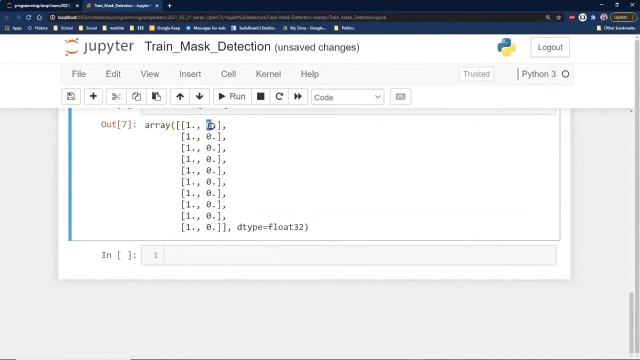 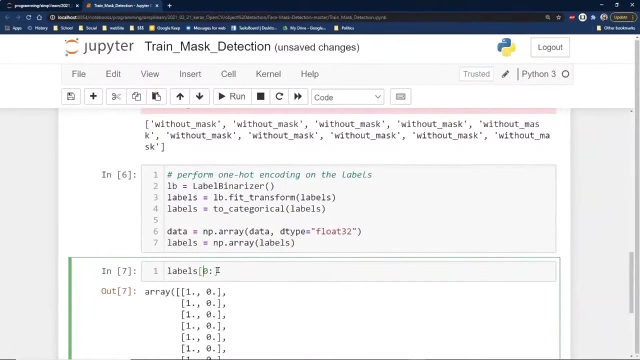 and So we can see where the other side looks like. we now have one. that means they have a mask, one 0, 1, 0. so on one being, they have a mask and zero no mask. and if we did this in reverse, i just realized that this might not make sense if you've never done this before. 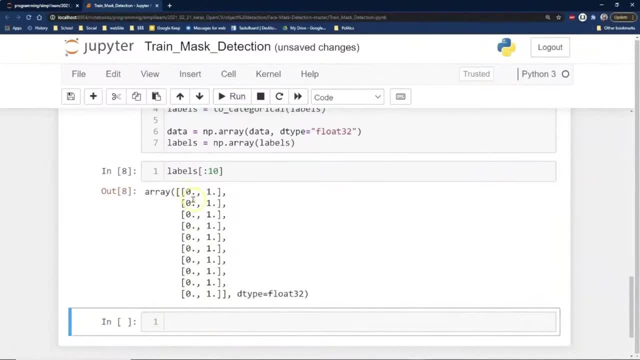 let me run this zero one. so zero is: uh, do they have a mask on zero? do they not have a mask on? they don't have a mask, and then we're going to do the rest of the ones we want to use have a mask on one. so this is the same as what we saw up here, without mask. one equals the second. 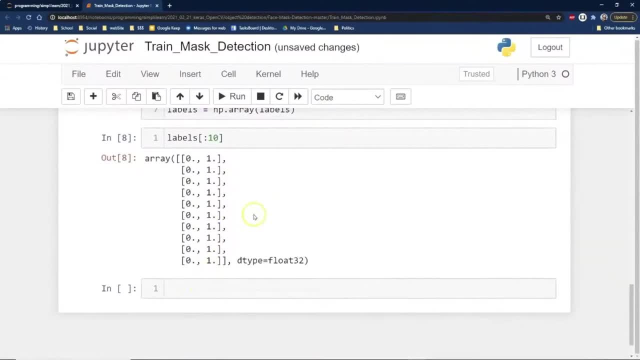 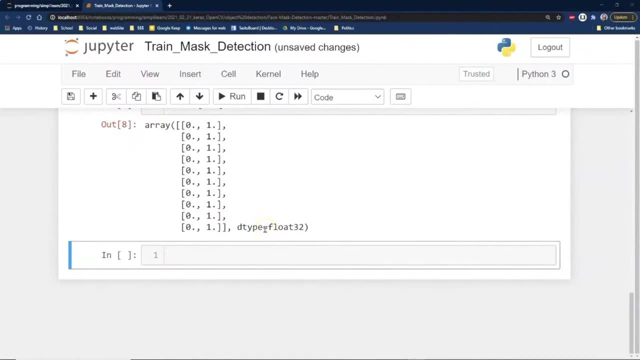 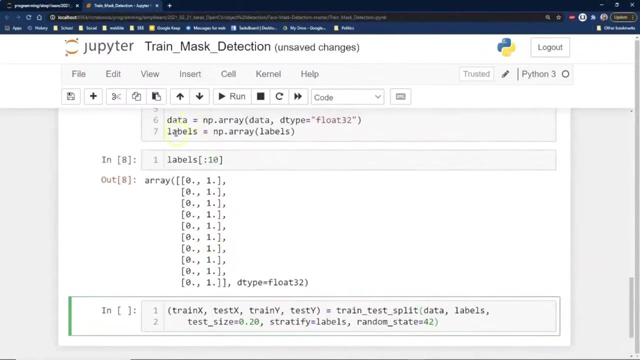 value is without mass. so with mass, without mask, and that's just a. with any of your data processing we can't really zero. if you have a zero one output, uh, it causes issues as far as training and setting it up. so we always want to use a one hot encoder if the values are not actual. 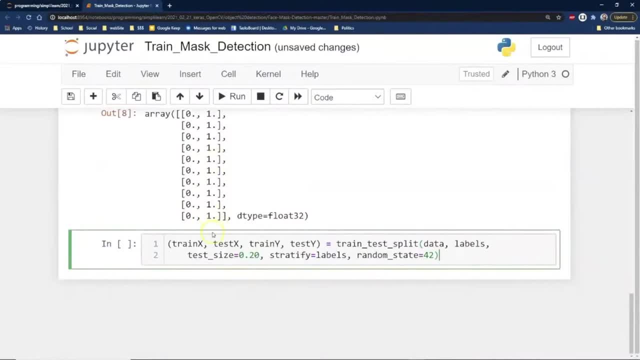 linear value or regression values. they're not actual numbers if they represent a thing, and so now we need to go ahead and do our train x test, x, train y test, y, train split test data and we'll go ahead and make sure it's going to be random and we'll take 20 of it for testing. 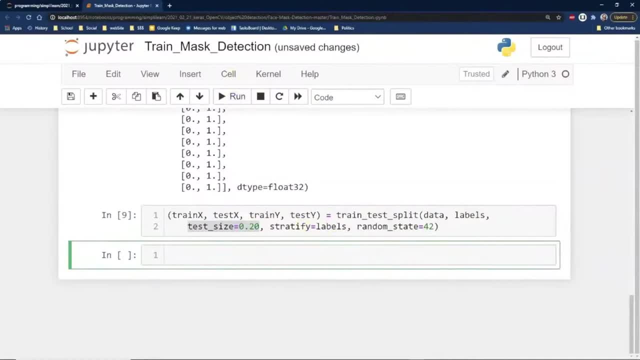 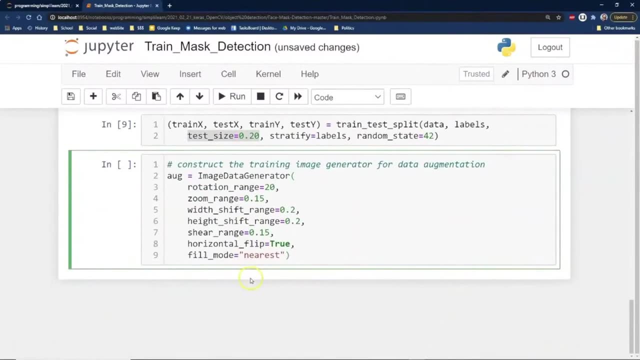 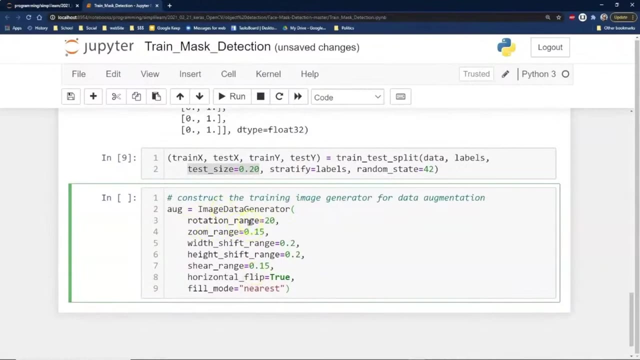 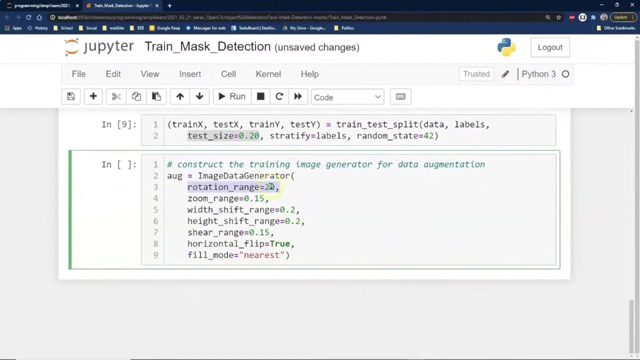 and the rest for setting it up. as far as training their model, this is something that's become so cool. when they're training these set, they realize we can augment the data. what does augment mean? well, if i rotate the data around and i zoom in, i zoom out, i rotate it, share it a little bit, flip it horizontally, fill mode, as they do all. 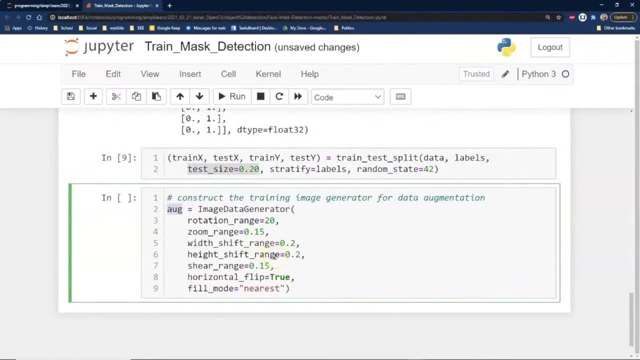 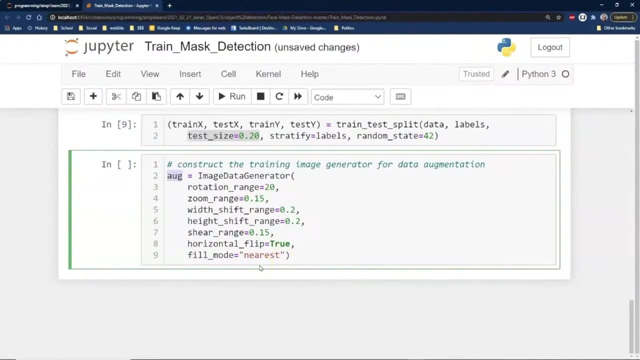 these different things to the data it is able to. it's kind of like increasing the number of samples i have. so if i have all these perfect samples, what happens when we only have part of the face, or the face is tilted sideways, or all those little shifts cause a problem. if you're doing just a standard. 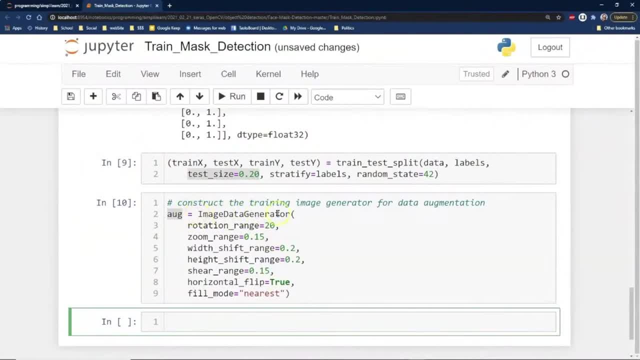 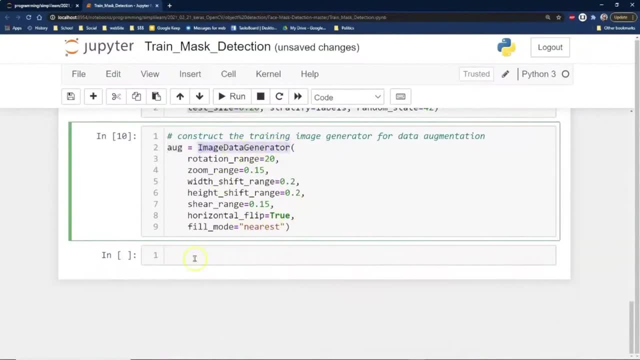 set of data. so we're going to create an augment in our image data generator which is going to rotate, zoom and do all kinds of cool things, and this is worth looking up: this image data generator and all the different features it has. a lot of times i'll the first time through my models. i'll leave that. 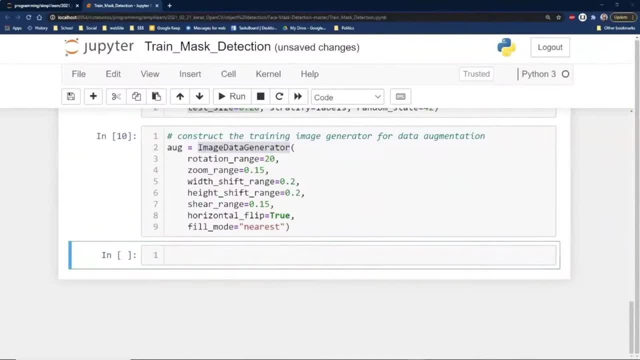 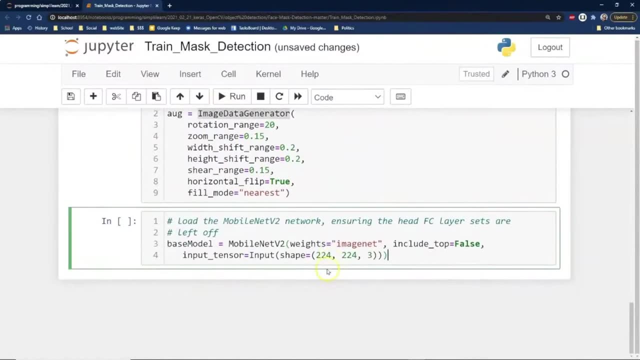 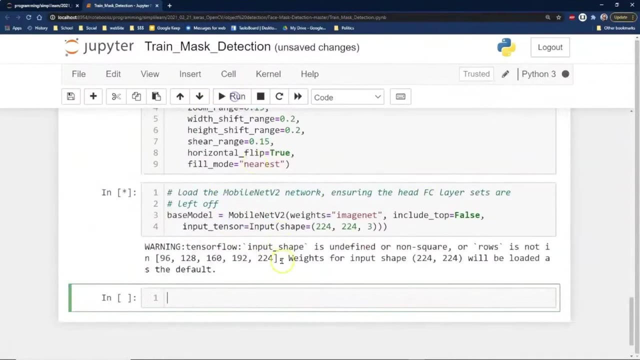 out because i want to make sure there's a thing we call build to fail, which is just cool to know that something is going to happen from a photo like aircraft uber to my row and they're just making sure you don't loop files in between yourannitals. 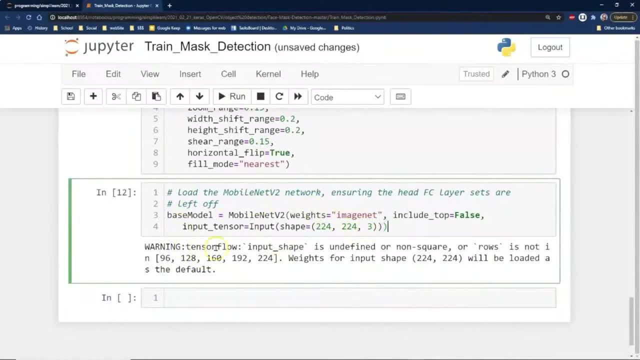 it really depends on the model. so it's not your model. you're making all of the technical changes, but anything well built obviously. so one thing i always look at when i build a model- you know, kind of a trademarks model- is i keep leaving this good little path over here. 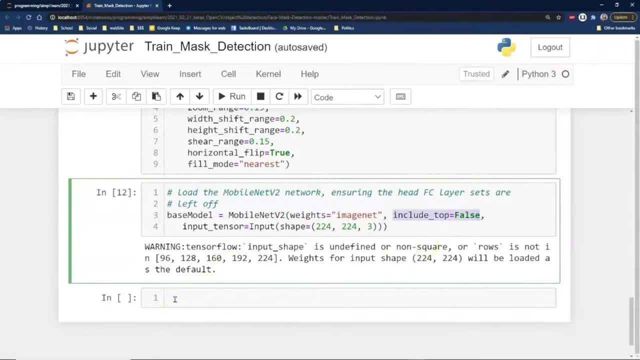 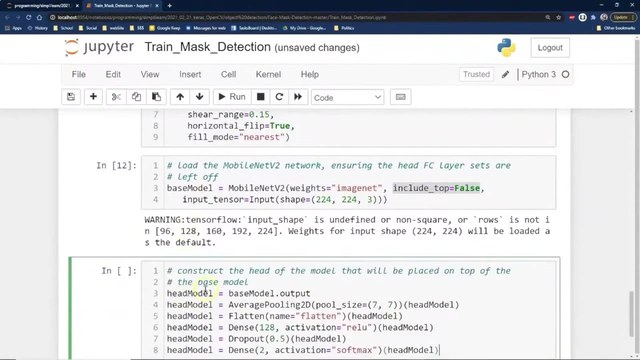 just it's because i'll put my model in the top right corner, in with the label on the top row, so we want to make sure that that is not the case. and then the construction of the head of the model that will be placed on the top of the base model. we want to go ahead and set that up. 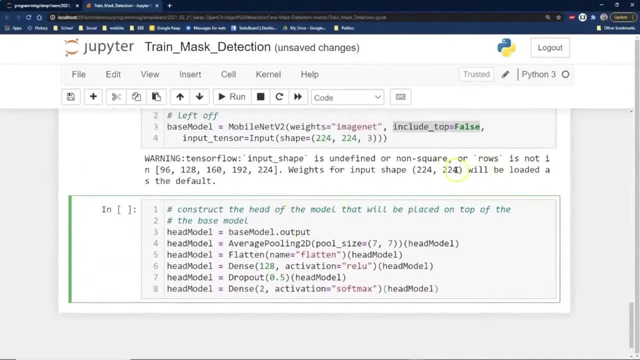 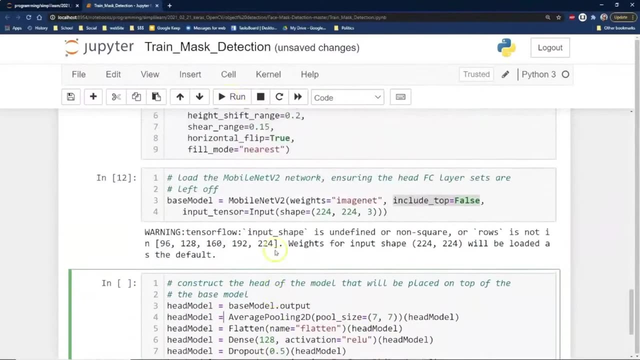 and you'll see a warning here. I'm kind of ignoring the warning because it has to do with the size of the pictures and the weights for input shape. so they'll switch things to defaults, just saying, hey, we're gonna auto shape some of this stuff for you. you should be aware of that. with this kind of imagery, we're 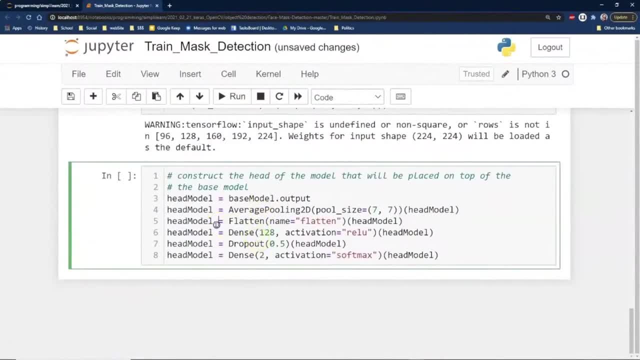 already augmenting it by moving it around and flipping it and doing all kinds of things to it. so that's not a bad thing in this, but another data it might be if you're working in a different domain, and so we're gonna go back here and we're gonna have- we have our base model, we're gonna do our head. 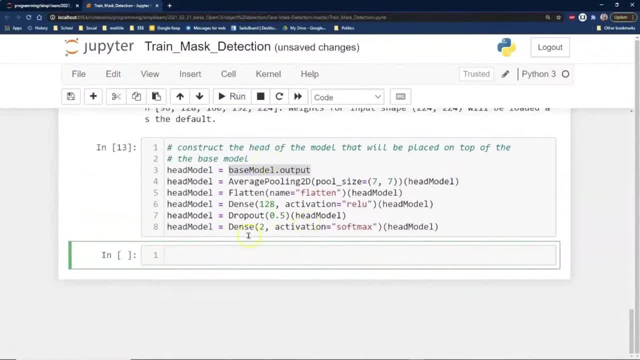 model equals our base model output and what we got here is we have an average pooling: 2d, 2d, 2d, 2d, size 7, 7 head model, head model flattened. so we're flattening the data. so this is all processing and flattening the images, and the pooling has to do with some of 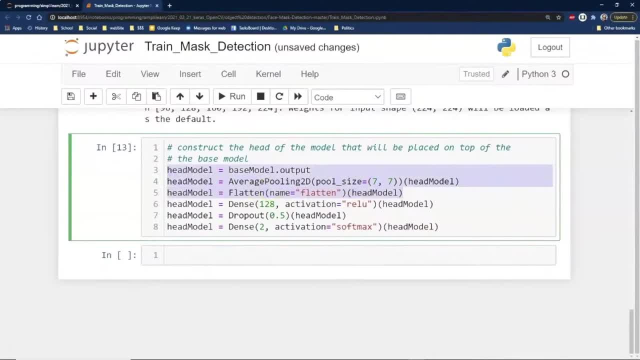 the ways that can process some of the data. we'll look at that a little bit when we get down to the lower level on this processing it. and then we have our dense. we've already talked a little bit about a dense, just what you think about, and 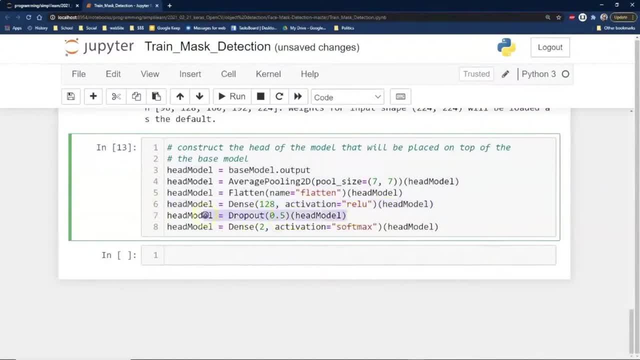 then the head model has a dropout, a point five. what do we can do with a dropout? the dropout says that we're going to drop out a certain amount of nodes while training. so when you actually use the model it will use all the notes, but this drops certain ones out and it helps stop. 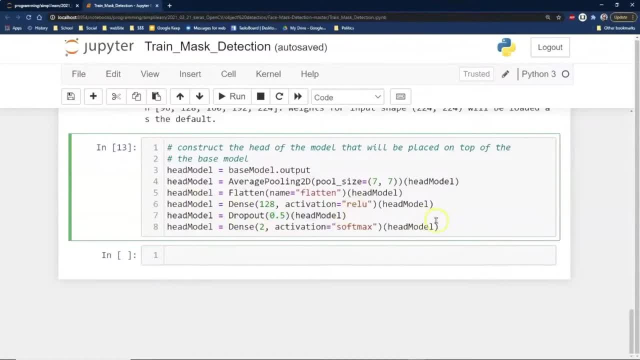 biases from a forming, so it's really a cool feature in here. they discovered this a while back. we have another dense mode and this time we're using soft max activation- lots of different activation options here. soft max is a real popular one for a lot of things. so is their Reilu and you. 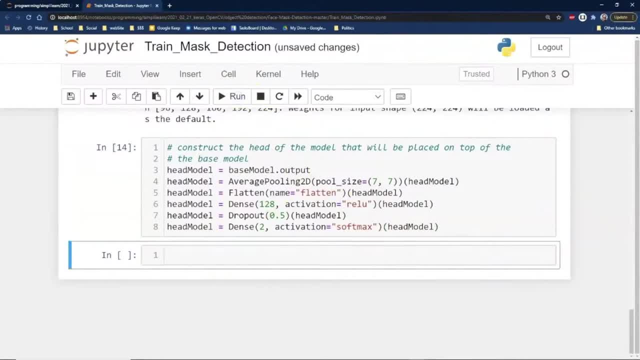 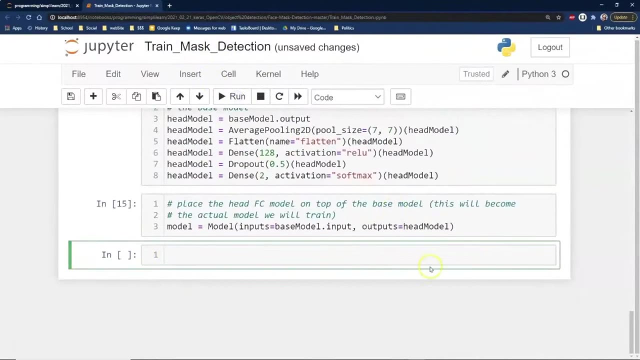 know there's. we do a whole talk on activation formulas and why, what their different uses are and how they work. when you first start out you'll you'll use mostly the Reilu and the soft max for a lot of them, just because they're there's some of the basic setups. it's a good place to start and then we have our 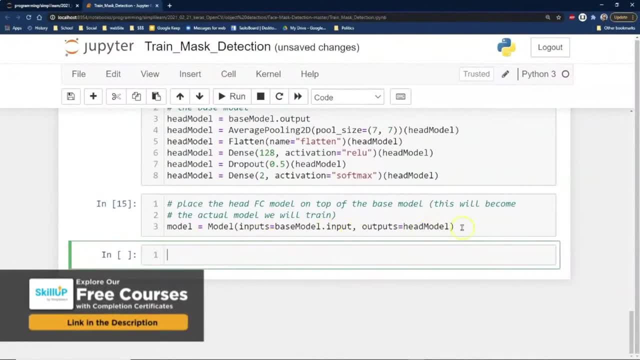 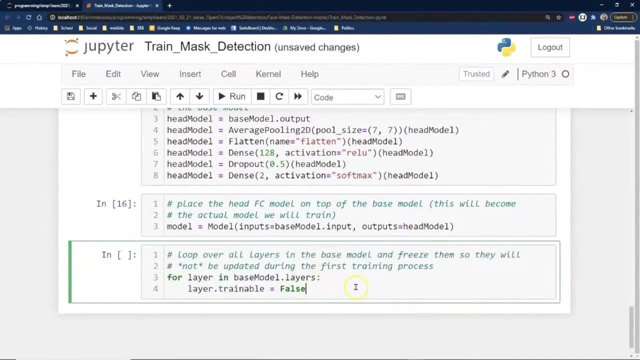 model equals model. inputs equals base model. dot input outputs equals head model. so again, we're still building our model here. we'll go ahead and run that and then we're going to loop over all the layers in the base model and freeze them, so they will not be updated. 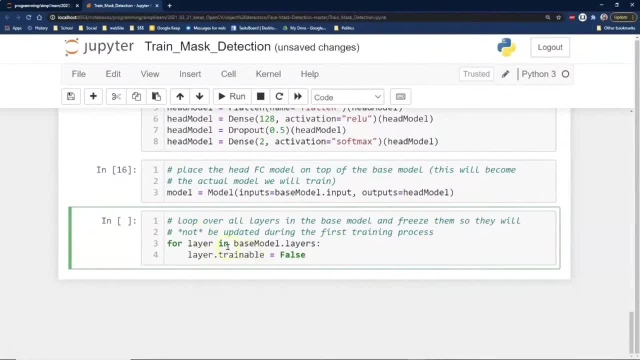 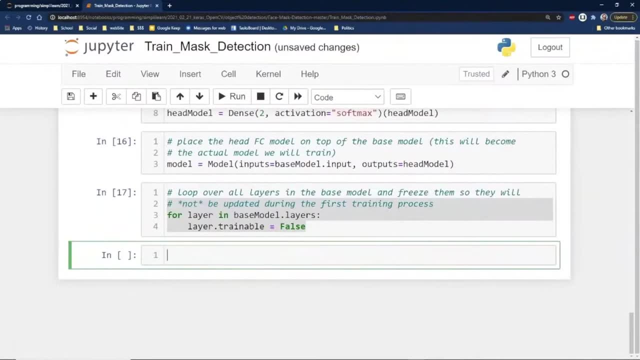 during the first training process. so for layer and base model layers, layers, dot trainable- equals false. a lot of times when you go through your data you want to kind of jump in part way through. I I'm not sure why in the back they did this for this particular example, but I do this a lot when 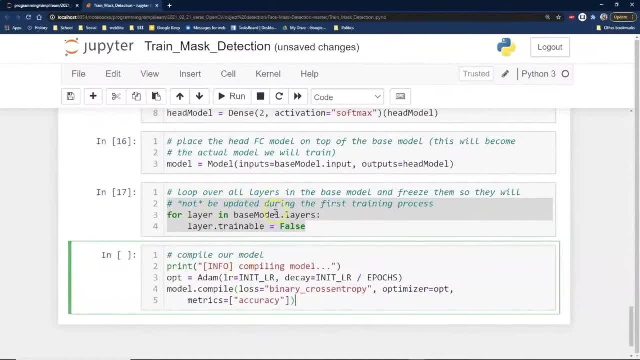 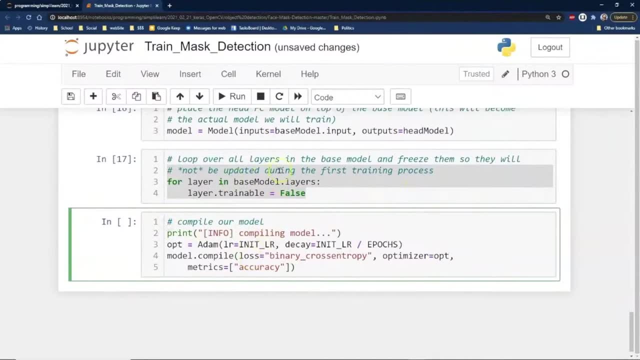 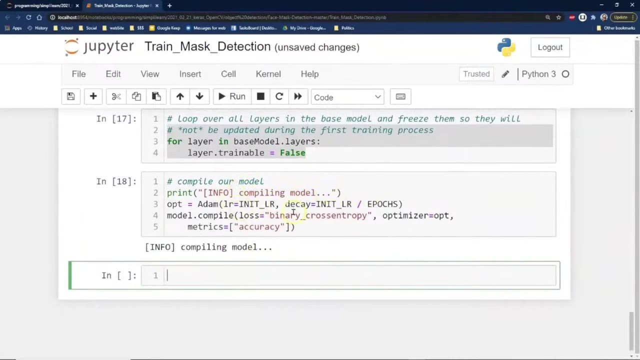 I'm working with series and specifically in stock data. I wanted to iterate through the first set of 30 data. before it does anything, I would have to look deeper to see why they froze it on this particular one, and then we're going to compile our model. so compiling the model Adam and knit. 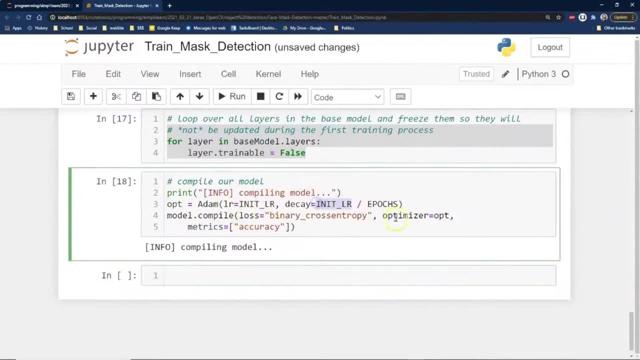 layer decay, initial learning rate over epics, and we go ahead and compile. our loss is going to be the binary cross entropy which will have that print out. optimizer for opt metrics is accuracy- same thing we had before, not a huge jump as far as the previous code. and then we go ahead and we've gone through all this and now we 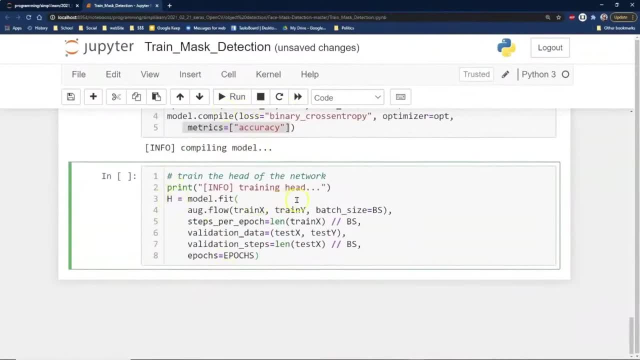 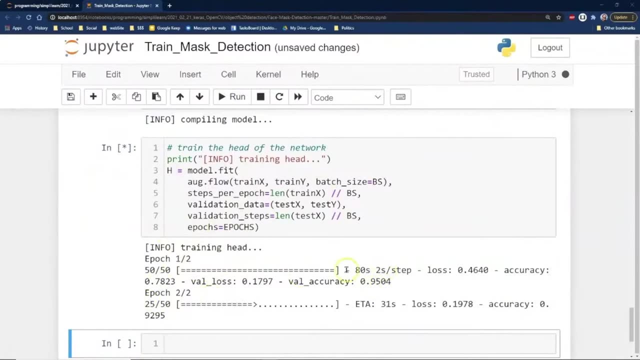 need to go ahead and fit our model. so train the head of the network. print info. training head run now. I skipped a little time because it to you'll see. the run time here is at 80 seconds per epic. takes a couple minutes for it to get. 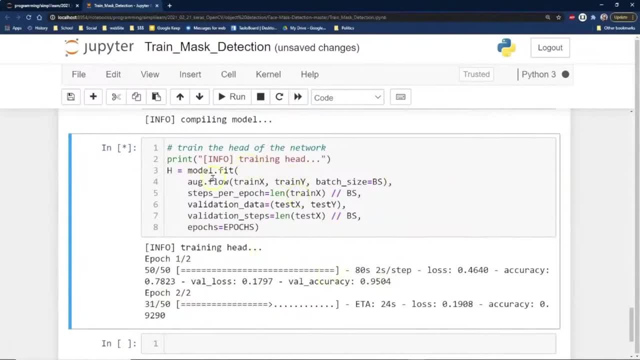 through on a single kernel. one of the things I want you to notice on here while we're well it's finishing the processing, is that we have up here our augment going on, so anytime the training next and trading, why go in? there's some randomness going on there and is 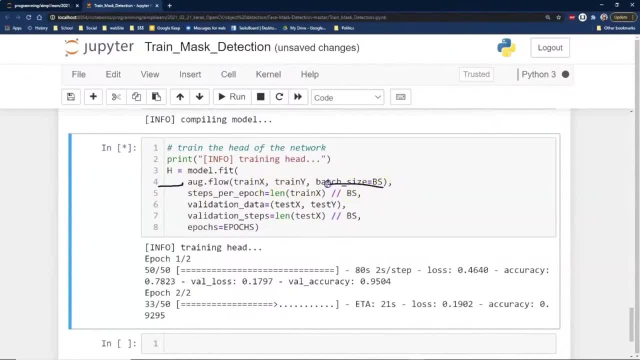 jiggling it around. what's going into our setup? of course we're batch sizing it, so it's going through whatever we set for the batch values, how many we process at a time, and then we have the steps per epic, the train X, the batch size. 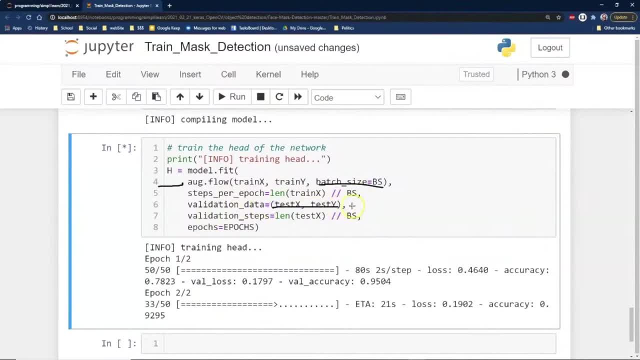 validation data. here's our test X and test Y, where we're sending that in, and this, again, it's validation. one of the important things to know about validation is our when both our training data and our test data have about the same accuracy. that's when you want to stop. that means that our model isn't biased. 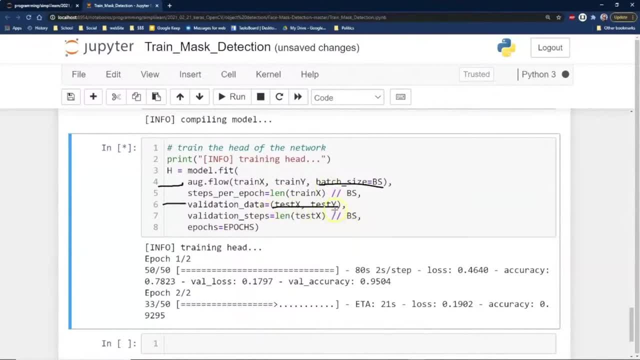 if you have a higher accuracy on your testing- you've trained it- and your accuracy is higher on your actual test data, then something in there is probably has a bias and it's over fitted. so that's what this is really about. right here with the validation data and validation data. 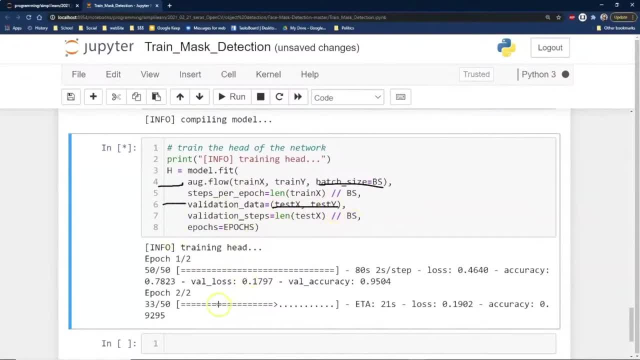 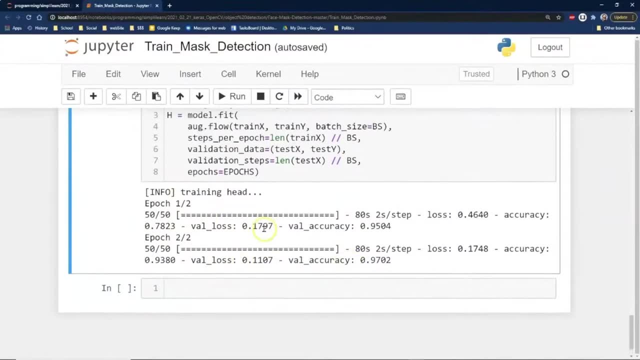 elimination steps. so it looks like it's go ahead and see if it's done. processing looks like we've gone ahead and gone through two epics again. you could run this through about 20 with this amount of data and it would give you a nice refined model at the end. we're going to stop at two because I 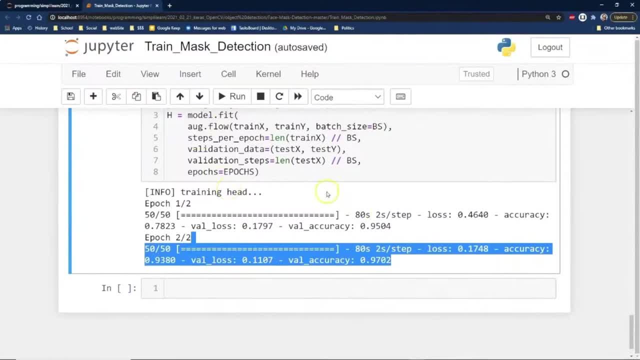 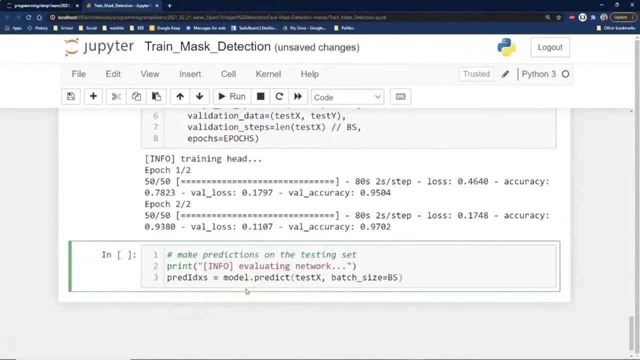 really don't want to sit around all afternoon and I'm running this on a single thread. so now that we've done this, we're going to need to evaluate our model and see how good it is, and to do that, we need to go ahead and make our 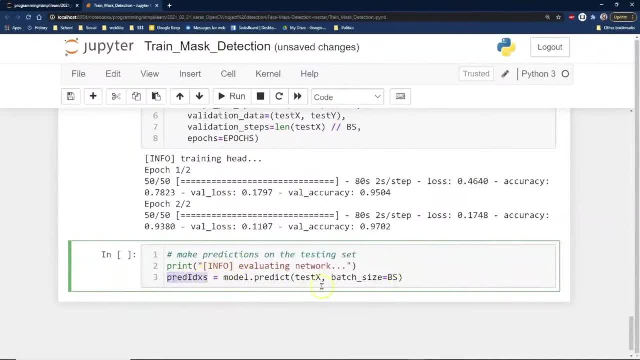 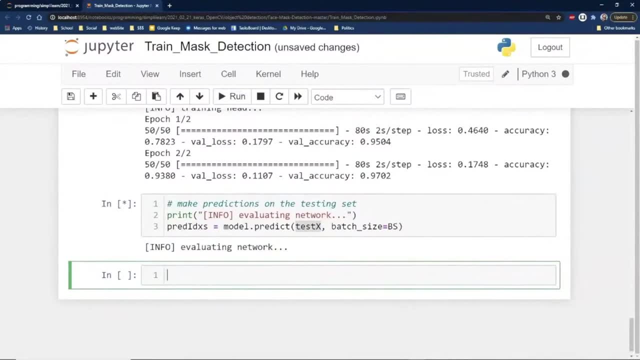 our predictions. these are predictions on our test X to see what it thinks are going to be. so now it's going to be evaluating the network and then we'll go ahead and go down here and we will need to turn the index in because, remember, it's either zero or one. it's a zero one, zero one. so you have two outputs, not 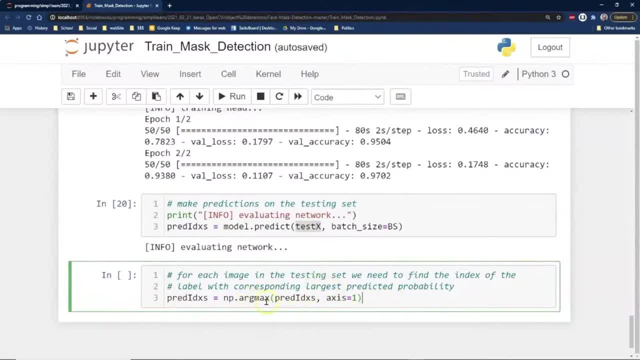 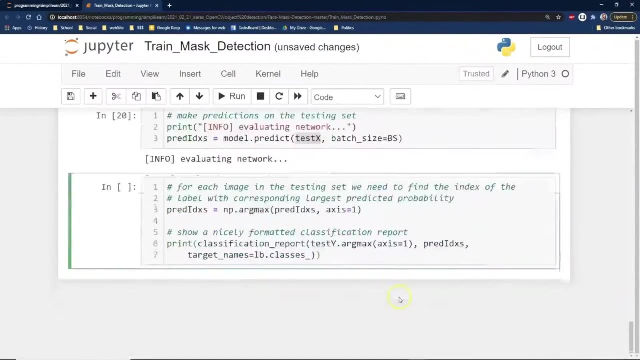 wearing wearing a mask and not wearing a mask, and so we need to go ahead and take that argument at the end and change those predictions to a zero or one coming out, and then, to finish that off, we want to go ahead and let me just put this right in here and do it all in one shot. we want to show a nicely formatted 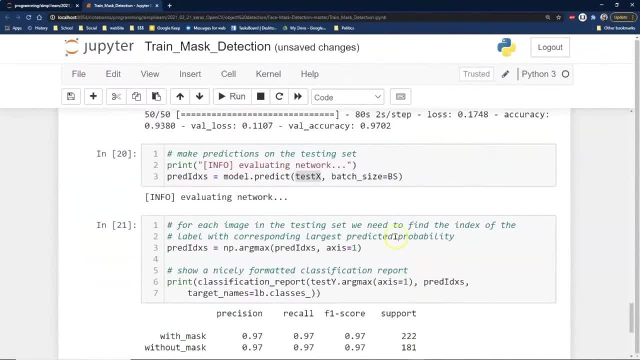 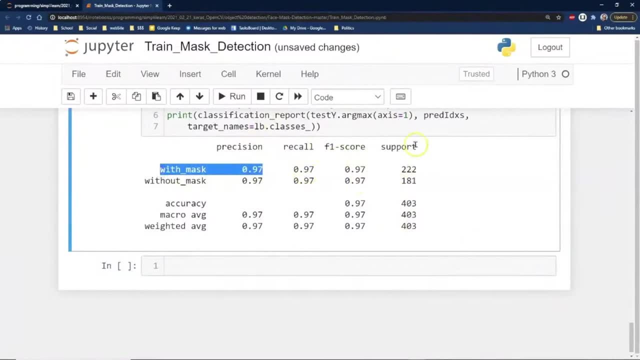 classification reports. we can see what that looks like on here and there we have it. we have our precision: it's 97% with a mask. there's our f1 score: support without a mask: 97%. so that's pretty high, high setup on there. you know you three people are going to sneak into 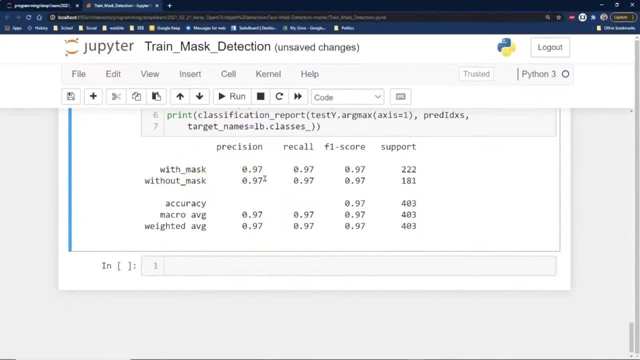 the store who are without a mask and thinks they have a mask, and there's going to be three people with a mask that's going to flag the person at the front to go. oh hey, look at this person. he might not have a mask. that's if. i guess it's a setup in front of a store. so there you have it. 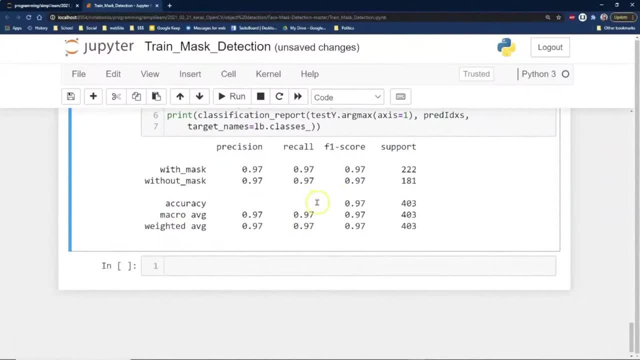 and, of course, one of the other cool things about this is if someone's walking into the store and you take multiple pictures of them- you know this is just an- it would be a way of flagging- and then you can take that average of those pictures and make sure they match or don't match. if you're on 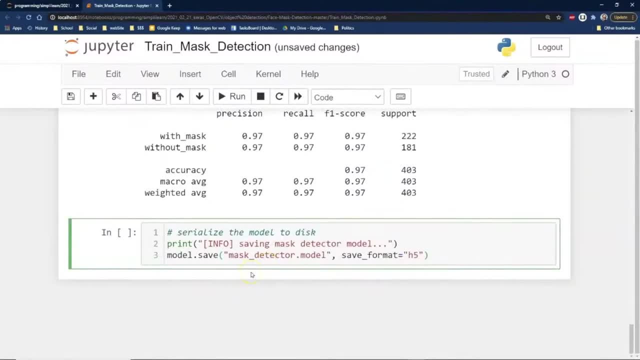 the back end and this is an important step because we're going to: this is just cool, i love doing this stuff. so we're going to go ahead and take our model and we're going to save it. so, model save, mass detector dot model. we're going to give it a name. we're going to save the format, in this case. 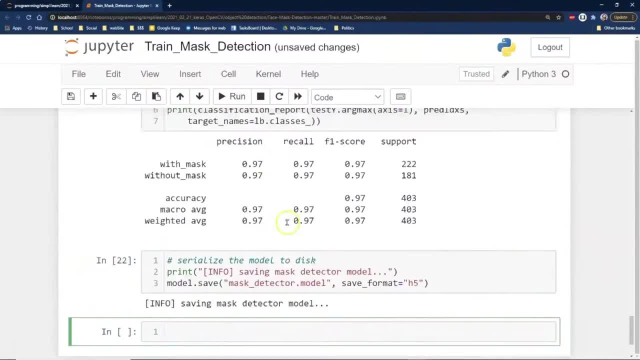 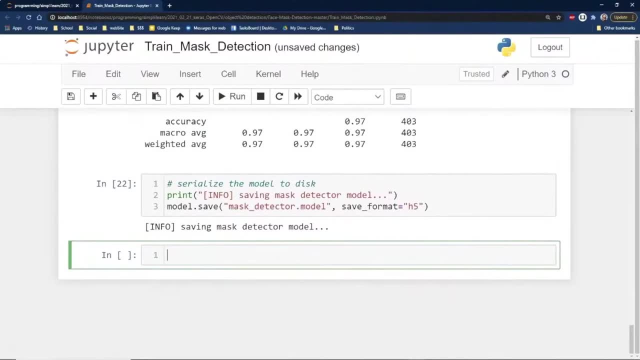 we're going to use the h5 format and so this model we just programmed has just been saved. uh, so now i can load it up into, say, another program. what's cool about this is, let's say, i want to have somebody work on the other part of the program. well, i just save the model. they upload the model. now they can use it for. 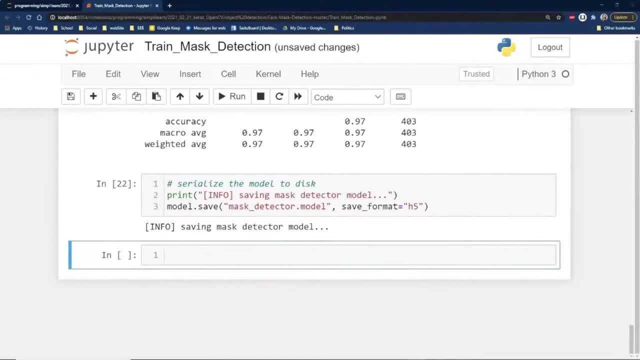 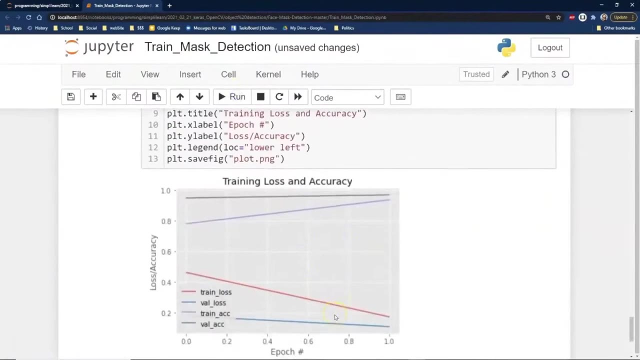 whatever, and then if i get more information and we start working with that at some point, i might want to update this model and make a better model, and this is true so many things where i take this model and maybe i'm running a prediction on making money for a. 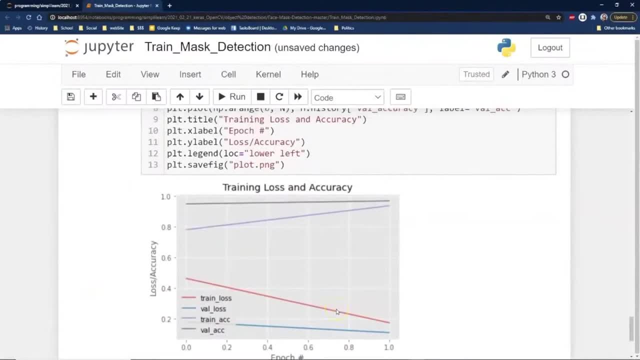 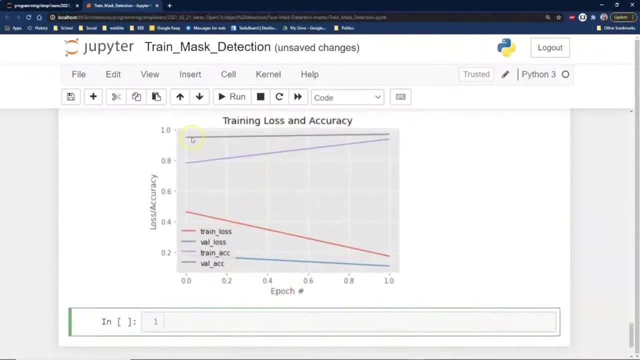 company and as my model gets better i want to keep updating it and then it's really easy just to push that out to the actual end user. and here we have a nice graph. you can see the training loss and accuracy as we go through the epics. we only did the, you know, only shows just the one epic. 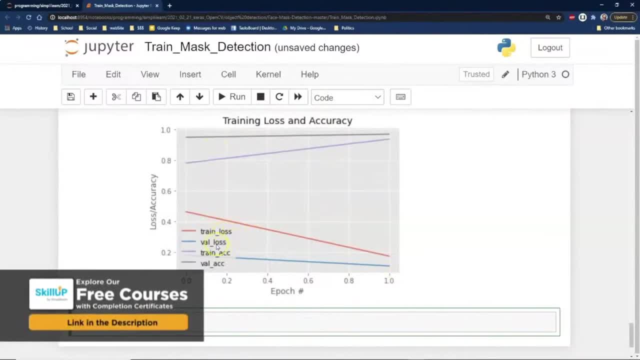 coming in here. but you can see right here as the value loss train accuracy and value loss accuracy starts switching and they start converging and you'll hear converging. this is a convergence they're talking about when they say you're, you're. i know when i work in the scikit with sk learn. 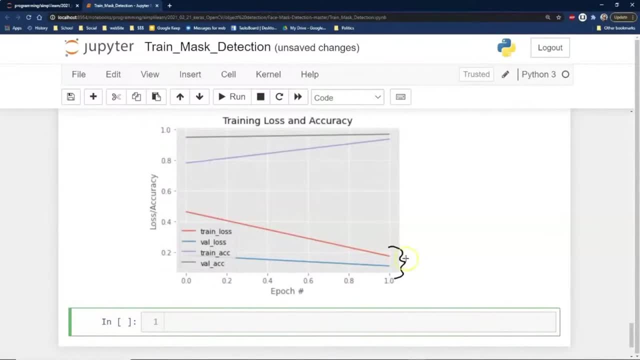 neural networks. this is what they're talking about. a convergence is our loss, and our accuracy come together and also up here, and this is why i'd run it more than just two epics. as you can see, they still haven't converged all the way, so that would be a cue for me to keep going. but what we want to do is we want to go ahead and 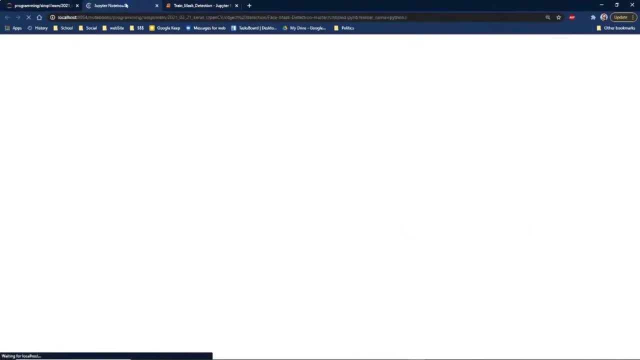 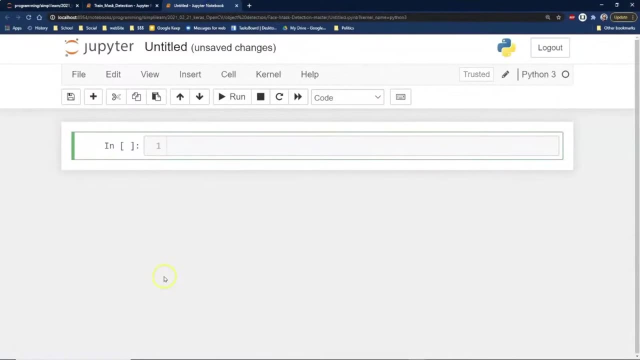 create a new python 3 program and we just did our train mask. so now we're going to go ahead and import that and use it and show you in a live action. get a view of both- myself in the afternoon, along with my background- of an office which is in the middle still of reconstruction for another. 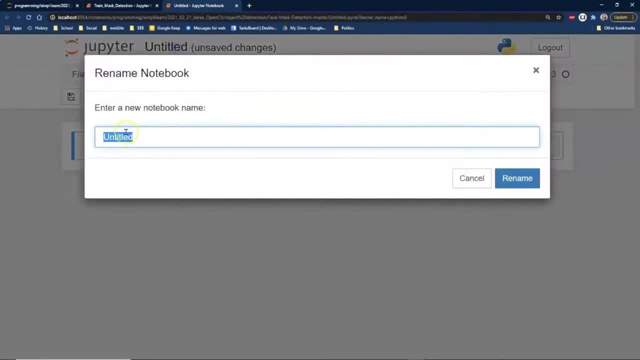 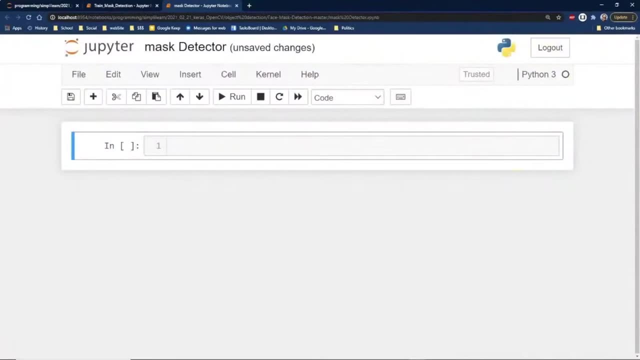 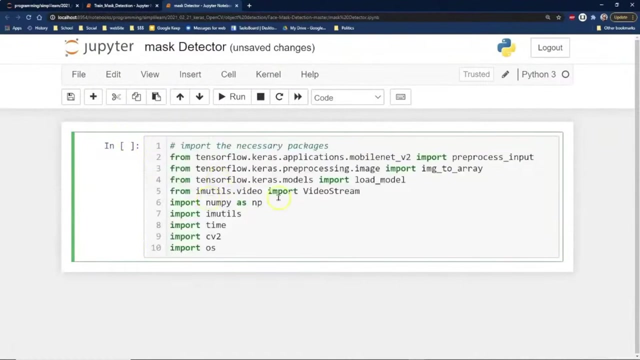 month and we'll call this a mask detector, and then we're going to grab a bunch of a few items coming in. we have our mobilenet v2 import pre-processing input, so we're still going to need that. we still have our tensorflow image to array. we have our load model. that's where most of the 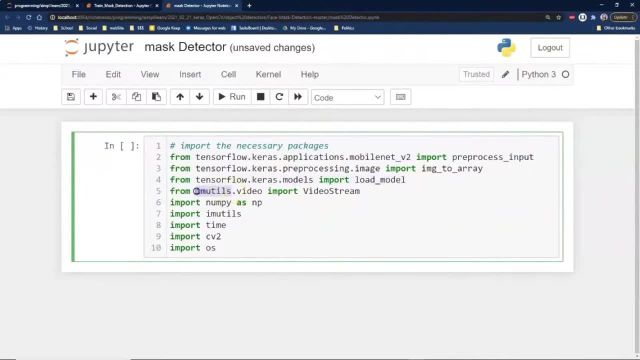 stuff's going on. this is our cv2 or opencv again. i'm not going to dig too deep into that. we're going to flash a little opencv code at you and we actually have a tutorial on that coming out: our numpy array, our im utilities. 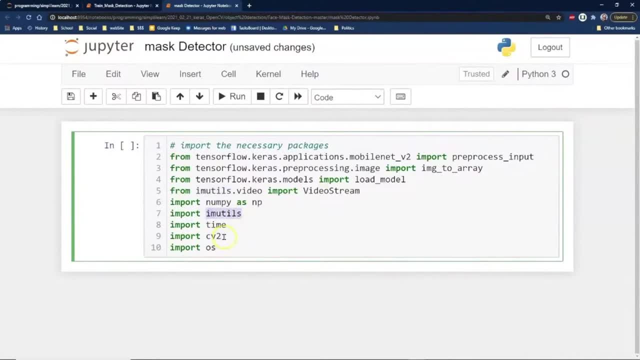 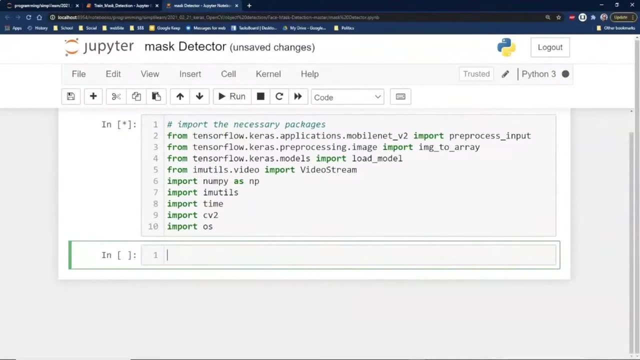 which is part of the opencv or cv2 setup, and then we have, of course, time and just our operating system. so those are the things we're going to go ahead and set up on here and then we're going to create. this takes just a moment. 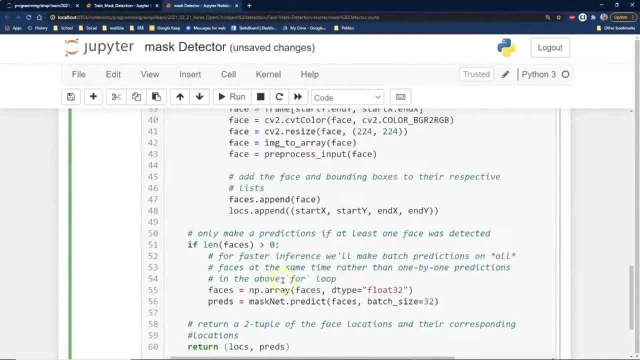 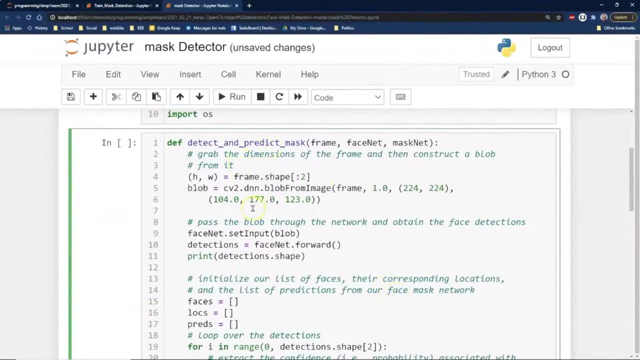 our module here which is going to do all the heavy lifting. so we're going to detect and predict a mask. we have frame, face net, mass net. these are going to be generated by our opencv. we have our frame coming in and then we want to go ahead and 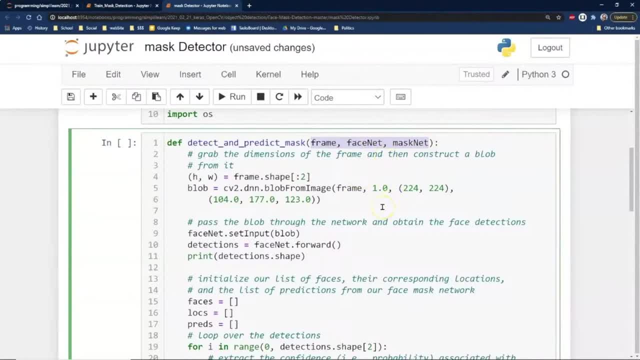 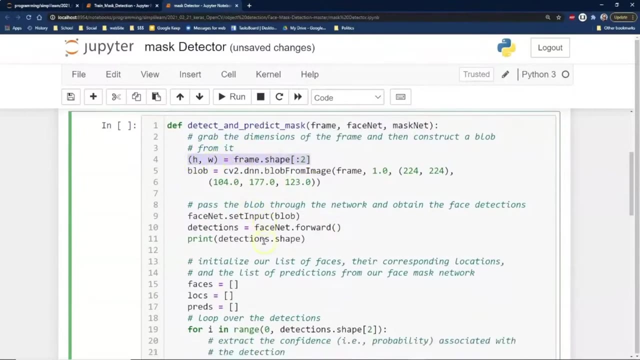 create a mask around the face. it's going to try to detect the face and then set that up so we know what we're going to be processing through our model. and then there's a frame shape here. this is just our height versus width. that's all hw stands for. 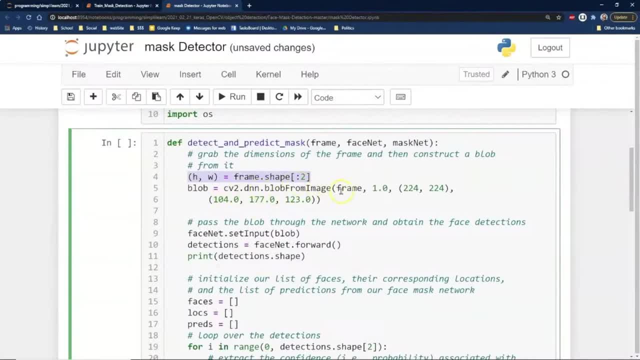 they've called it blob, which is a cv2 dnn blob form image frame. so this is reformatting this frame that's going to be coming in literally from my camera and we'll show you that in a minute- that little piece of code that shoots that in here and we're going to pass the blob through the network. 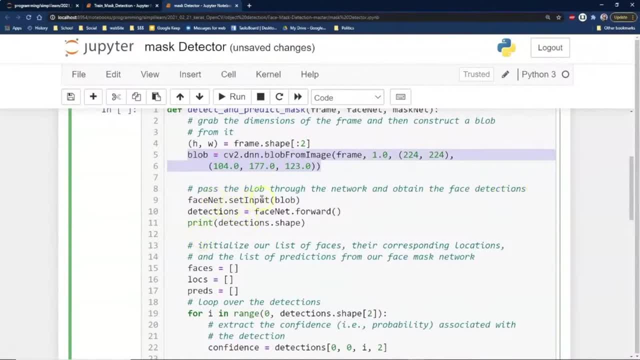 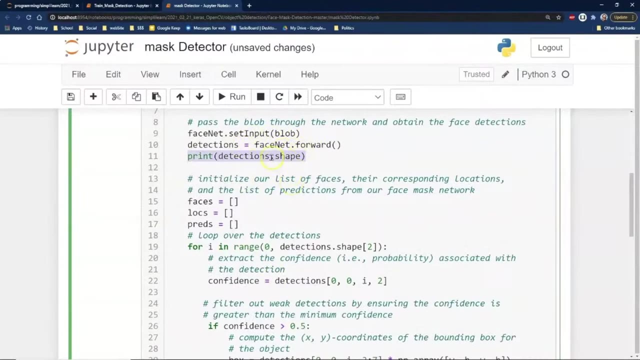 and obtain the face detections. so face net dot set import blob detections. face net forward print detections, shape, uh. so these is. this is what's going on here. this is that model we just created. we're going to send that in there and i'll show you in a second where that is, but it's going. 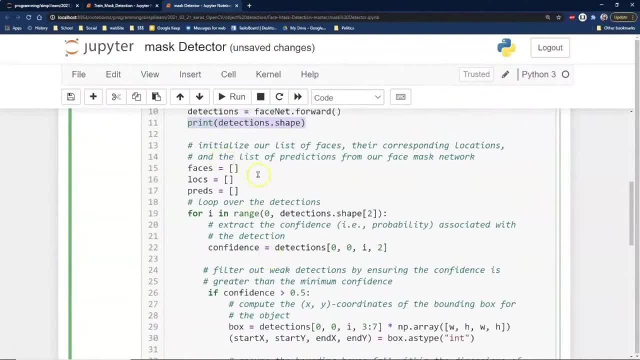 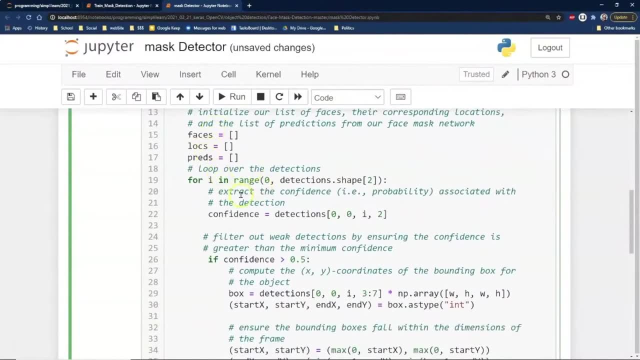 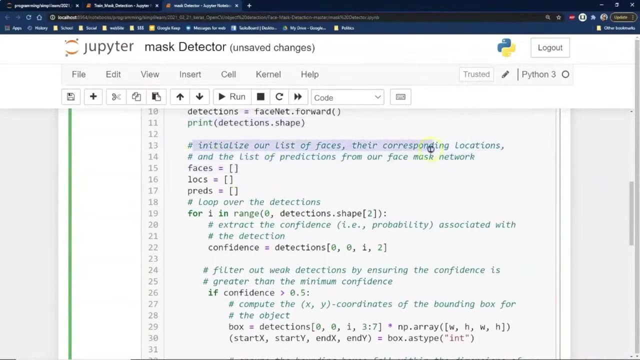 to be under facenet and then we go ahead and initialize our list of faces- they're corresponding locations and the list of predictions from our face mask network. we're going to loop over the detections and this is a little bit more work than you think as far as looking for different 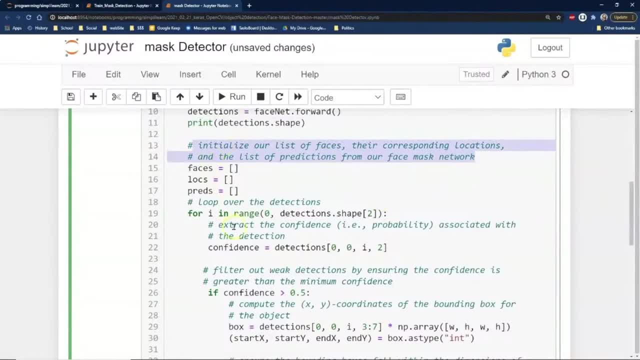 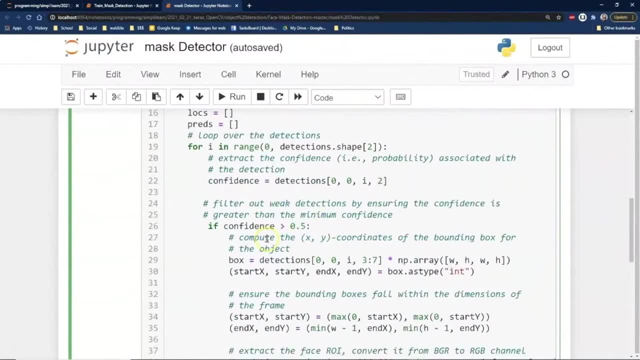 faces. What happens if you have a crowd of faces? So we're looping through the detections and the shapes going through here and probability associated with the detection. Here's our confidence of detections. We're going to filter out weak detection by ensuring the confidence. 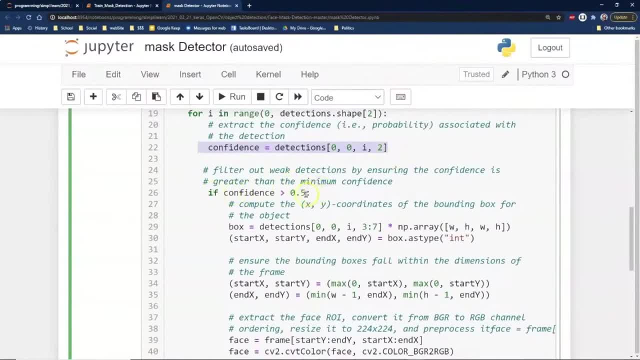 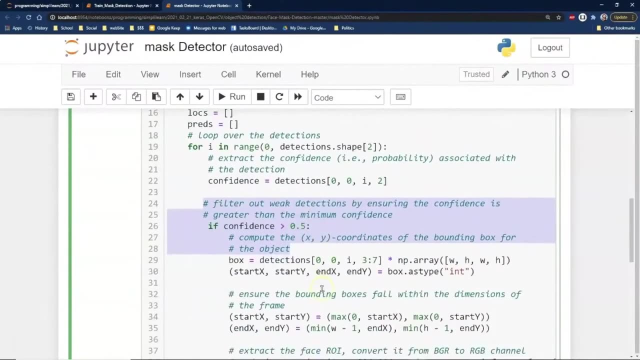 is greater than the minimum confidence. So we've set it- remember, zero to one. so 0.5 would be our minimal confidence. probably is pretty good. And then we're going to put in compute bounding boxes for the object. If I'm zipping through this, it's because we're going to do an OpenCV. 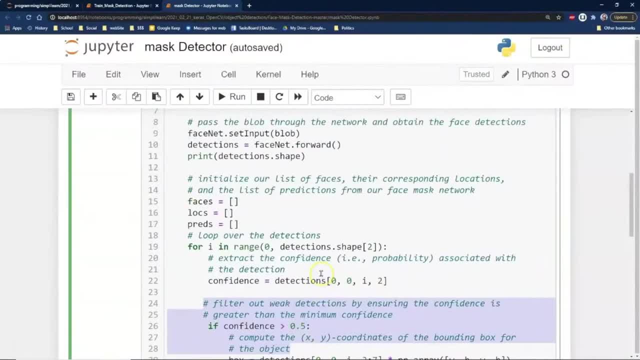 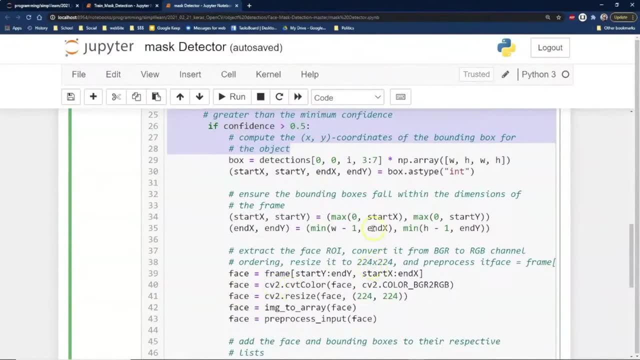 and I really want to stick to just the Keras part, And so I'm just kind of jumping through all this code. You can get a copy of this code from SimplyLearn and take it apart, or look for the OpenCV coming out And we'll create a box. The box sets it around. 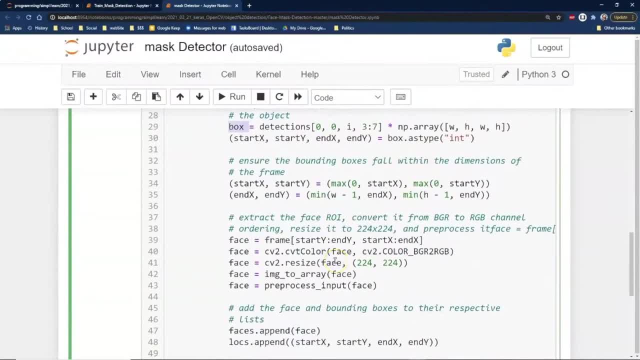 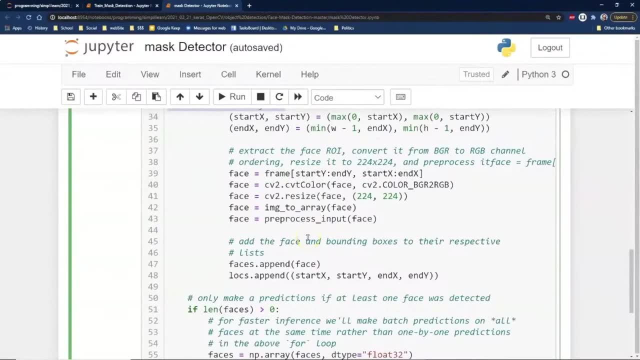 The image Ensure. the bounding boxes fall within the dimensions of the frame. So we create a box around what we hope is going to be the face. Extract the face ROI, Convert it from BGR to RGB channel. Again, this is an OpenCV issue, Not really an issue, but it has to do with the order. 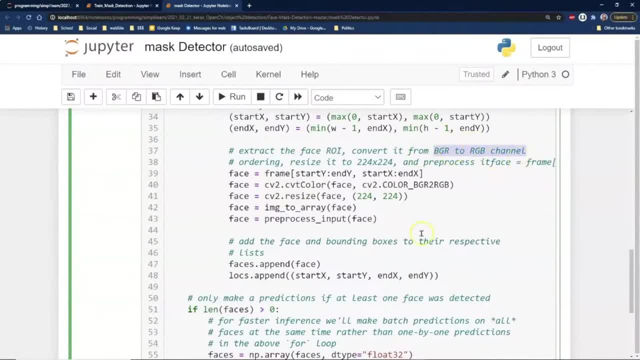 I don't know how many times I've forgotten to check the order colors when working with OpenCV, because there's all kinds of fun things when red becomes blue and blue becomes red And we're going to go ahead and resize it, process it, frame it, Face frame setup Again. 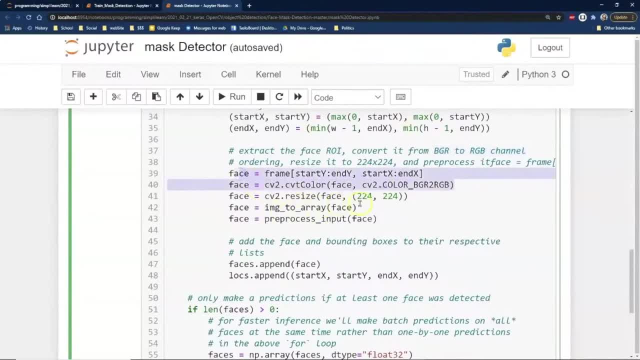 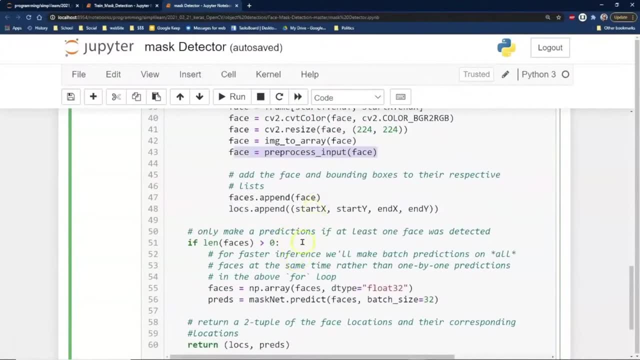 the face, the CVT color. We're going to convert it, We're going to resize it. Image to array. Pre-process the input: Pin the face, Locate face, start X, start Y and X. Boy, that was just a huge. 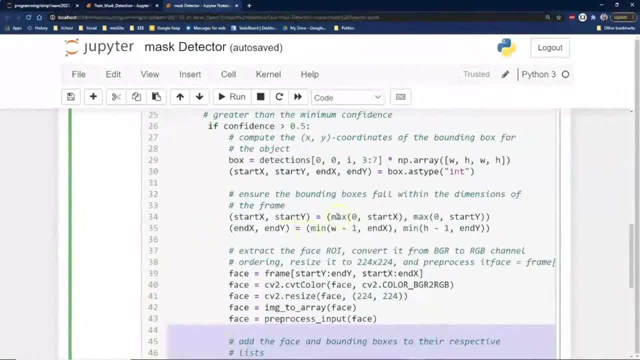 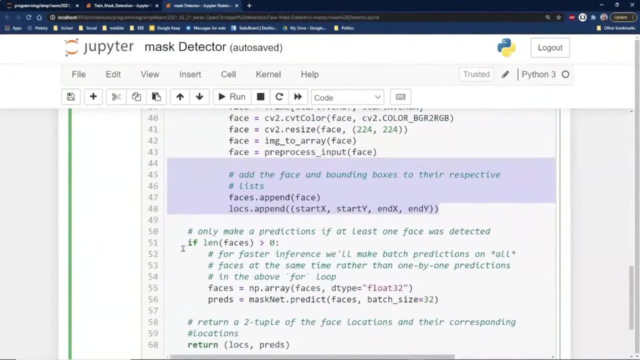 amount And I skipped over a ton of it. But the bottom line is we're building a box around the face And that box because the OpenCV does a lot of work. it's going to be a lot of work, It does a decent job of finding the face And that box is going to go in there and see hey. 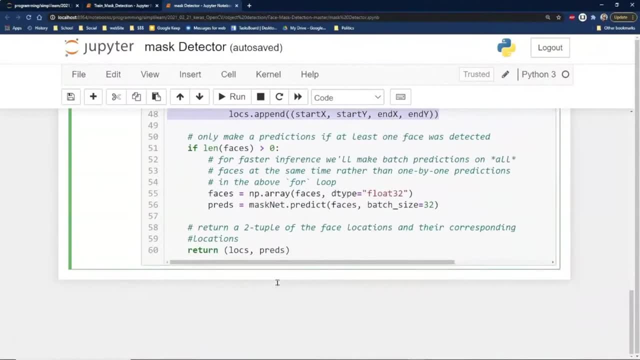 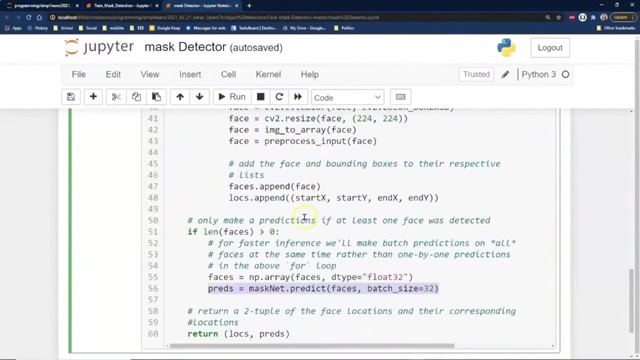 does this person have a mask on it, And so that's what all this is doing on here. And then, finally, we get down to this, where it says: predictions equals masknetpredict faces- batch size 32.. So these different images of where we're guessing where the face is are then going to go through. 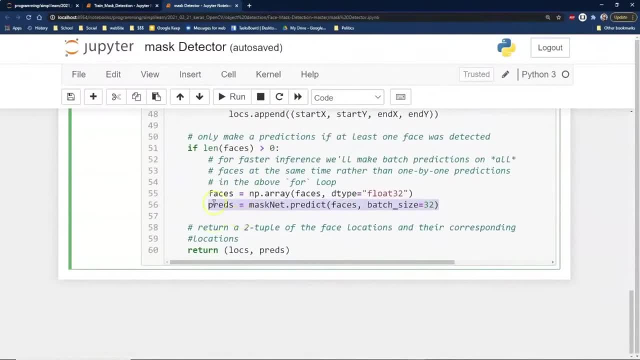 and generate an array of faces, if you will, And we're going to look through and say: does this face have a mask on it? And that's what's going right. here is our prediction. That's the big thing that we're working for. 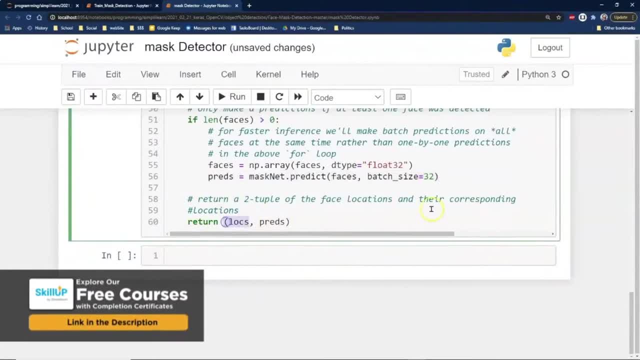 And then we return the locations and the predictions. The location just tells where on the picture it is, And then the prediction tells us what it is. Is it a mask or is it not a mask? All right, so we've loaded that all up. 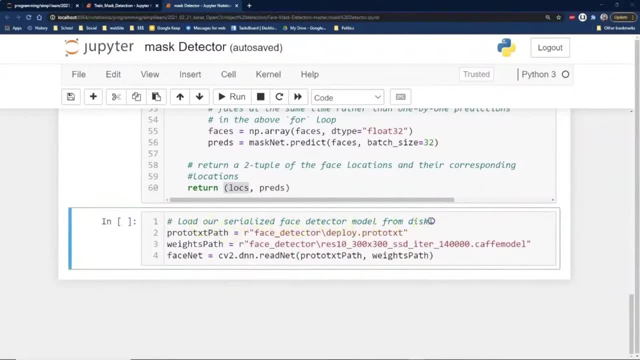 So we're going to load our serialized face detector model from disk And we have the path that it was saved in. Obviously, you're going to put it in a different path depending on where you have it or however you want to do it and how you saved it on the last one. 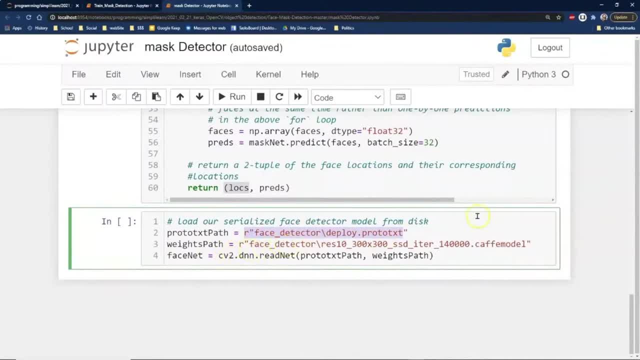 where we trained it, And then we have our weights path And so, finally, our face net. here it is equals cv2.dnnreadnet- prototext path- weights path, And we're going to load that up on here. So let me go ahead and run that. 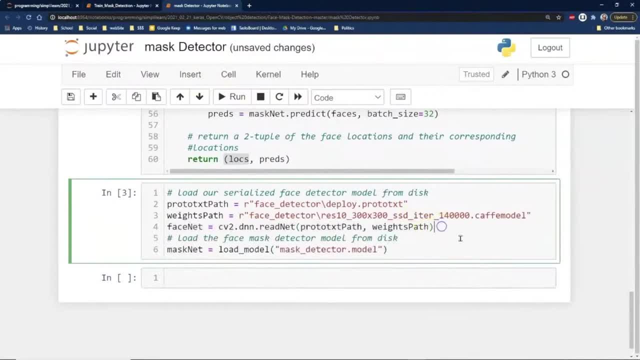 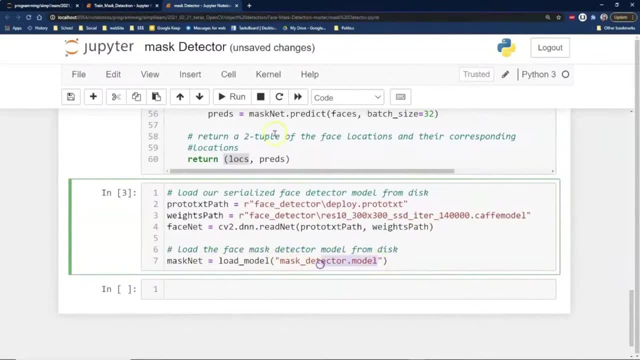 And then we also need to. I'll just put it right down here. I always hate separating these things in there- And then we're going to load the actual face detector model from disk. This is the model that we saved, So let's go ahead and run that on there also. 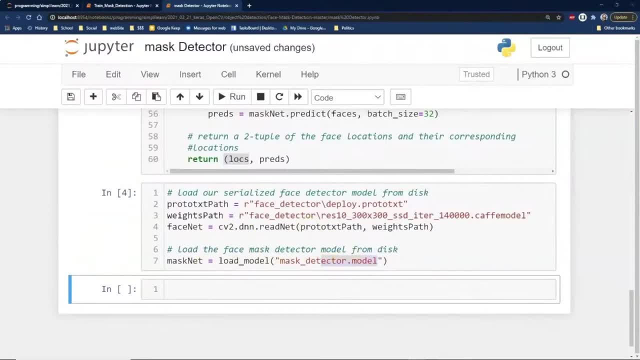 So this is pulling in all the different pieces we need for our model, And then the next part is we're going to create open up our video, And this is just kind of fun because it's all part of the OpenCV video setup. 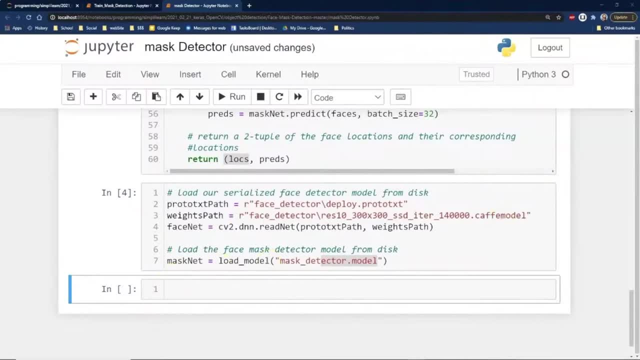 And we just put this all in as one. There we go. So we're going to go ahead and open up our video, We're going to start it And we're going to run it until we're done, And this is where we get some real, like kind of live action stuff, which is fun. 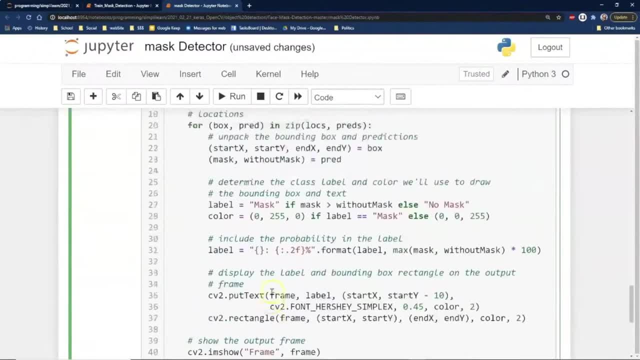 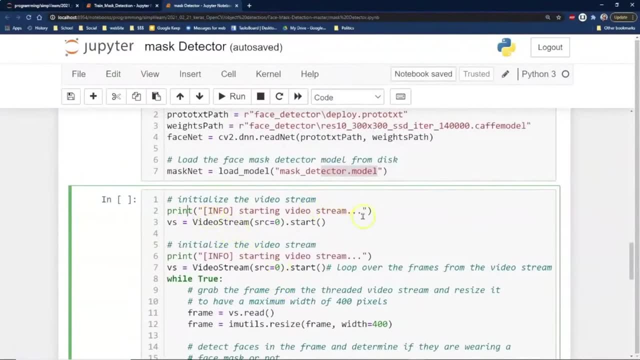 This is what I like working about with images and videos is that when you start working with images and videos, it's all like right there in front of you. It's visual and you can see what's going on. So we're going to start our video streaming. This is grabbing our video stream. source: zero start. That means it's grabbing my main camera. I have hooked up. 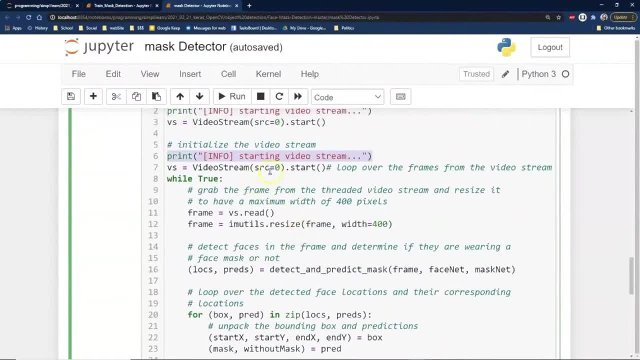 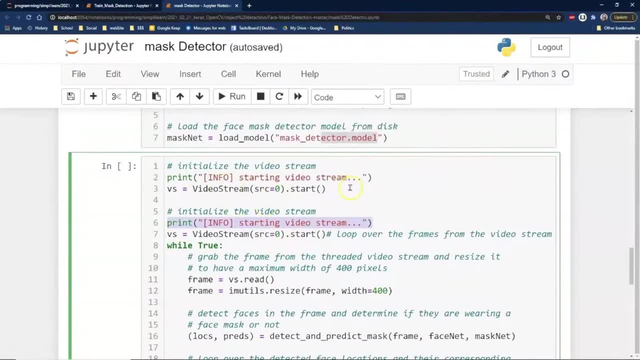 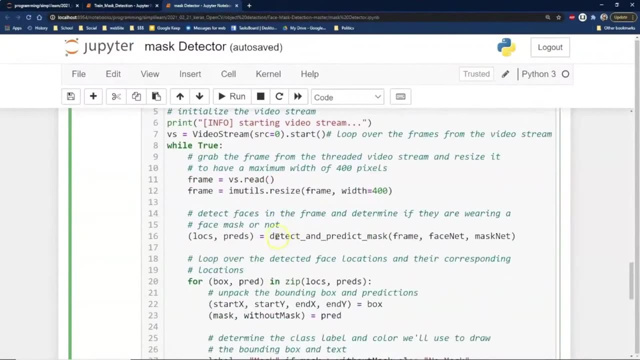 And then you know starting video. you're going to print it out. Here's our video source. equals zero start. Loop over the frames from the video stream. Oops, a little redundancy there. Let me close, I'll just leave it. That's how they had it in the code. So so, while true, we're going to grab the frame from the threaded video stream and resize it to have the maximum width of 400 pixels. 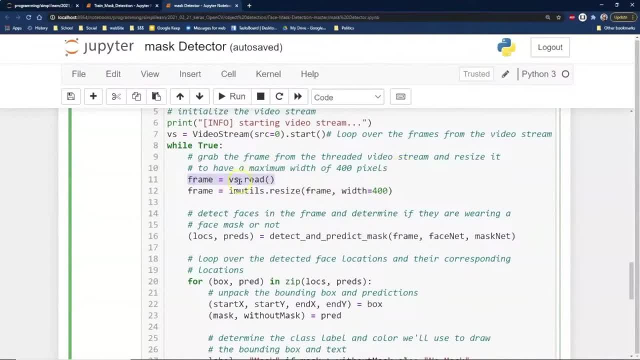 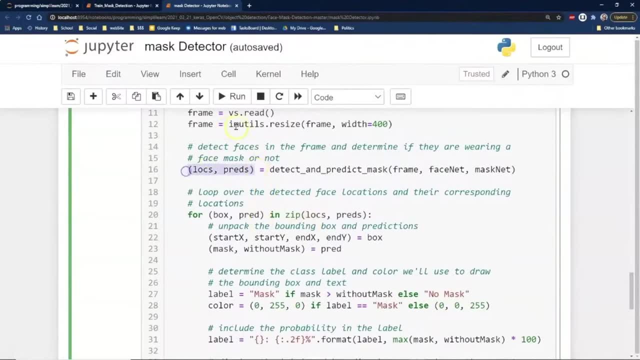 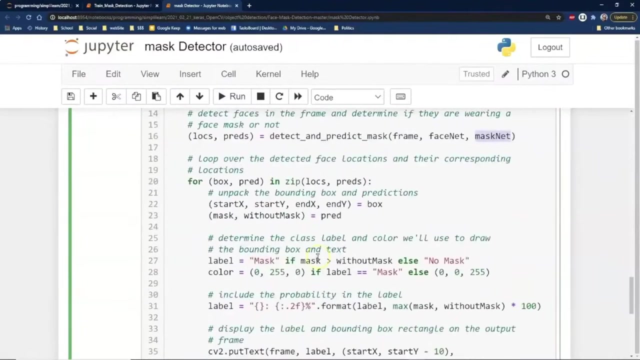 So here's our frame. We're going to read it from our visual stream, We're going to resize it And then we have, we're returning- Remember we return from the appropriate procedure, the location and the prediction. So detect, predict, mask. we're sending at the frame, we're sending at the face net and the mask net. so we're sitting, all the different pieces that say this is what's going through on here. 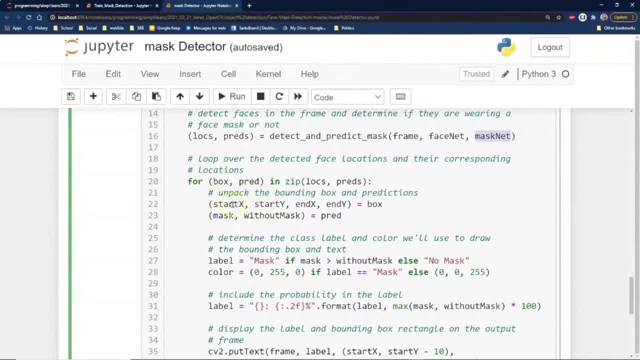 And then he returns our location and predictions and then for our box and predictions in the location and predictions, Uh huh, And the box is again: this is an open CV set that says, hey, this is a box coming in from the location. 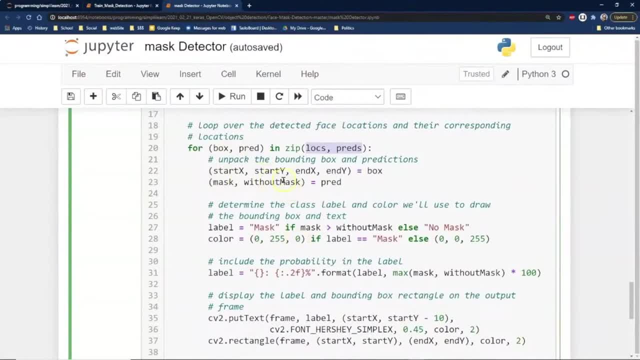 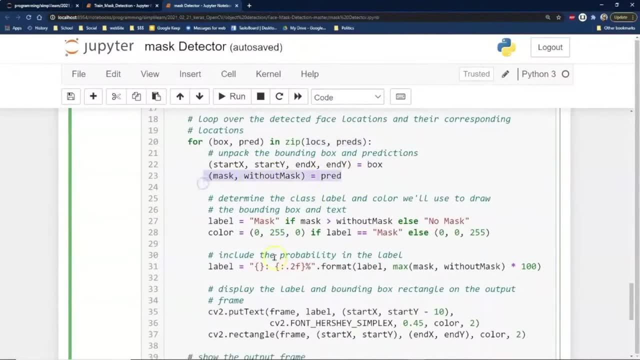 Because you have the two different points on there And then we're going to unpack the box in predictions And we're going to go ahead and do: mask without a mask equals prediction. We're going to create our label. No mask would create color if the label equals mask. L00225.. 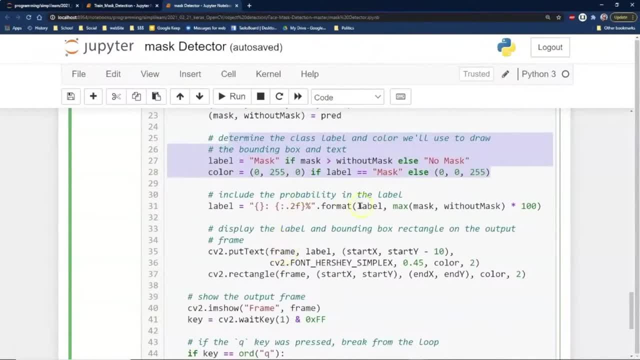 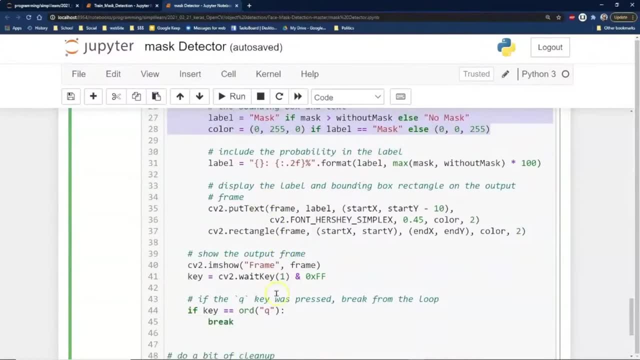 And you know this is going to make a lot more sense when I hit the run button here. But we have the probability of the label. We're going to display the label and bounding box rectangle on the output frame And then we're going to go ahead and show the output from the frame CV2, I am show frame frame. 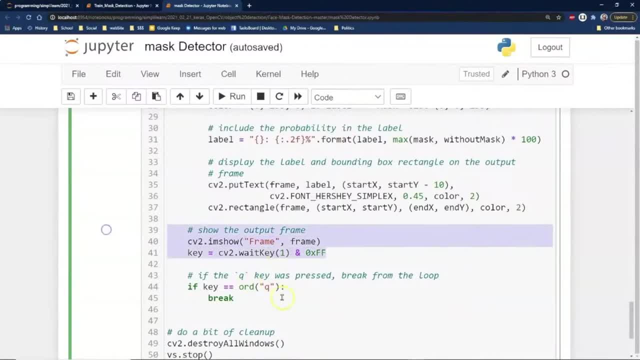 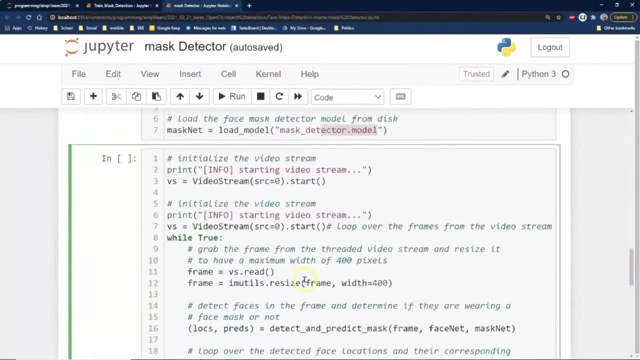 And then the key equals CV2, wait, key 1.. We're just going to wait until the next one comes through from our feed And we're going to do this until we hit the stop button. pretty much. So are you ready for this? 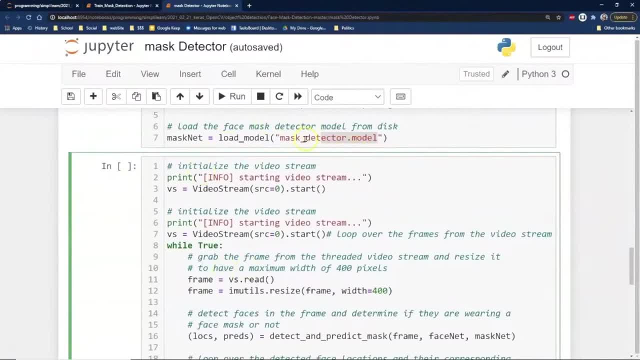 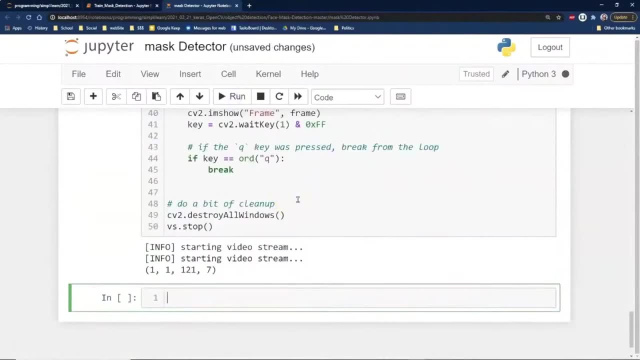 Let's see if it works. We've distributed our model, We've loaded it up into our distributed Uh code. here We've got a hooked into our camera and we're going to go ahead and run it, And there it goes. 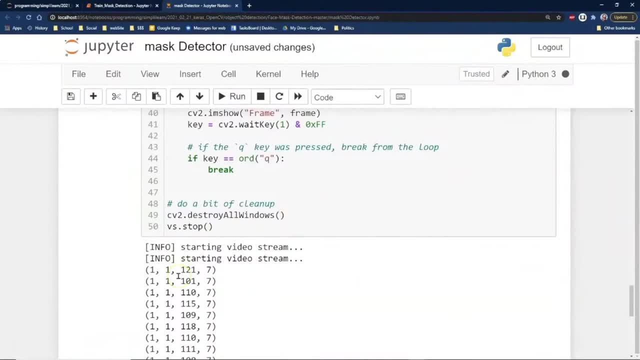 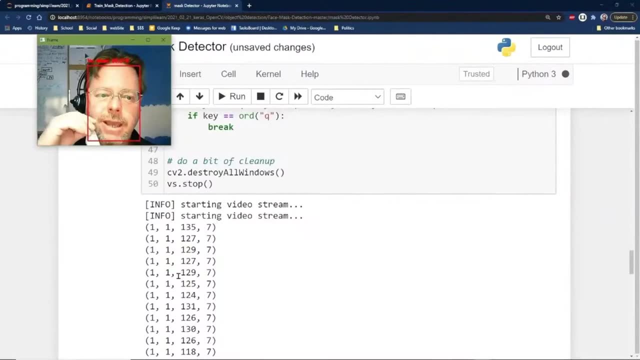 It's going to be running and we can see the data coming down here and we're waiting for the pop up And there I am in my office with my funky headset on uh, and you can see in the background my unfinished wall. 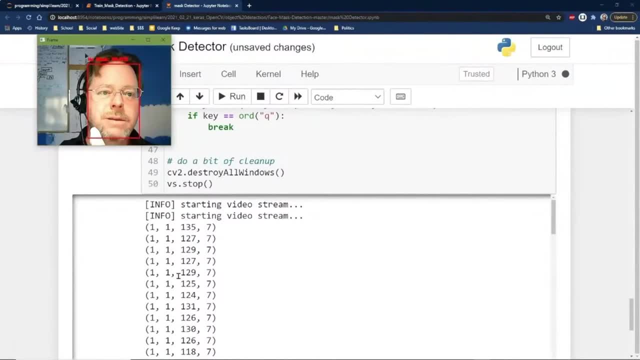 And it says up here: no mask. Oh, no, I don't have a mask on. Uh, I wonder if I cover my mouth, what would happen? Uh, you can see my no mask goes down a little bit. I wish I'd brought a mask into my office. 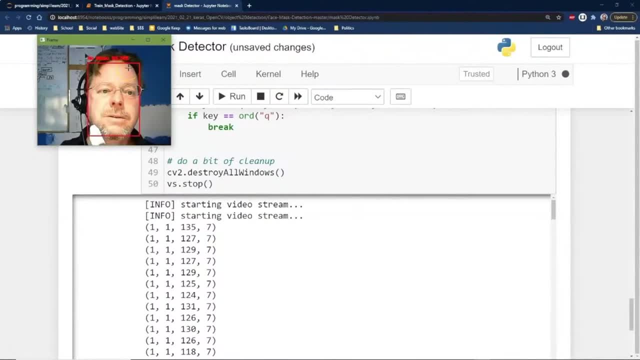 Uh, it's up at the house, but you can see here that this says: you know, there's a 95, 98% chance that I don't have a mask on, And it's true, I don't have a mask on right now and this could be distributed. 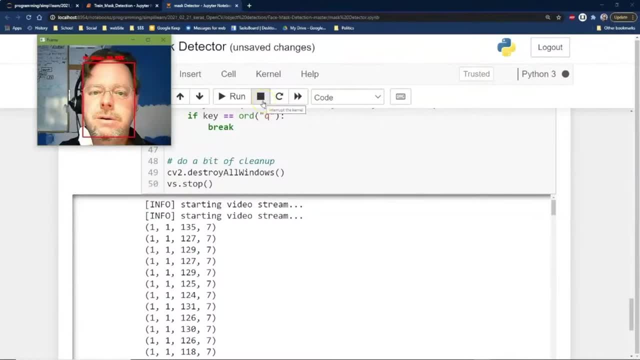 This is actually an excellent little piece of script that you can start. you know, you install somewhere on a video feed, on a, on a security camera or something, And then you'd have this really neat uh setup saying: Hey, do you have a mask on? 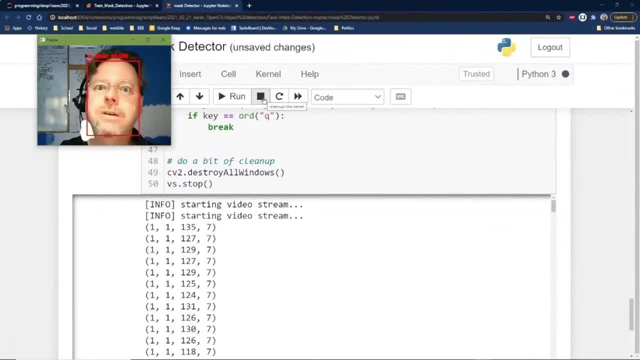 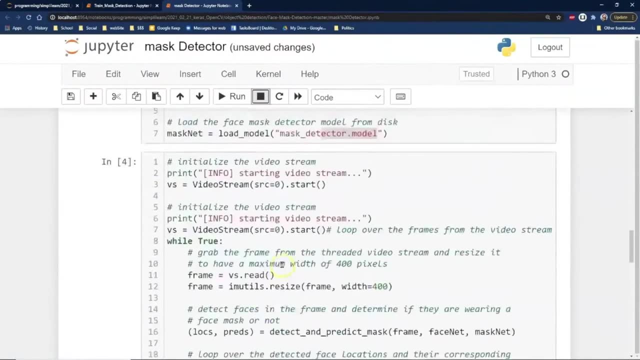 When you enter a store or a public transportation or whatever it is where they're required to wear a mask. Uh, let me go ahead and stop that Now. if you want a copy of this uh code, definitely give us a holler. 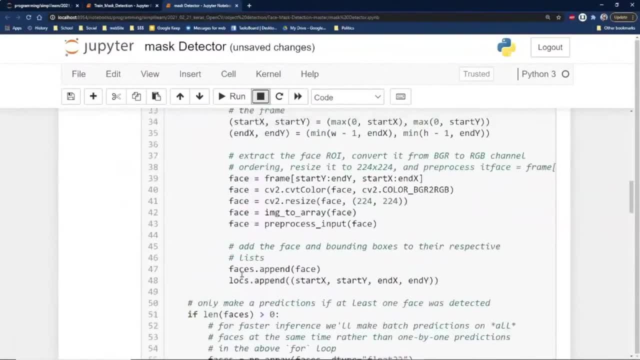 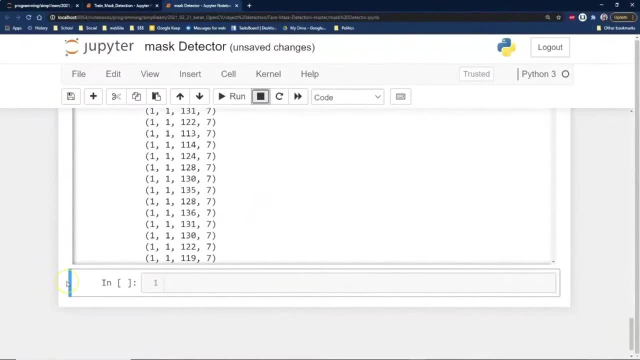 We will be going into open CV and another one, So I skipped a lot of the open CV um code in here. as far as going into detail, really focusing on the cross uh- saving the model, uploading the model and then processing- 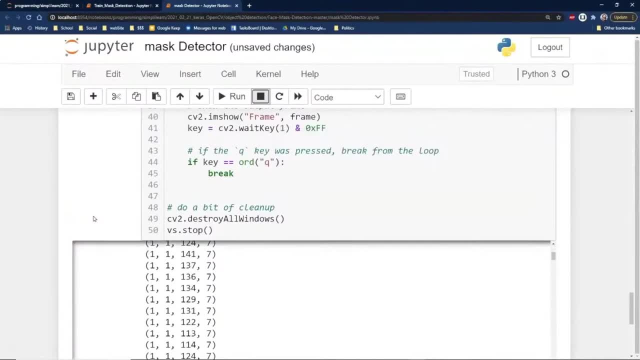 Uh, streaming video through it So you can see it that the model works. We actually have this working model that hooks into the video camera, which is just pretty cool and a lot of fun. So I told you we're going to dive in and really roll up our sleeve and do a lot of coding today. 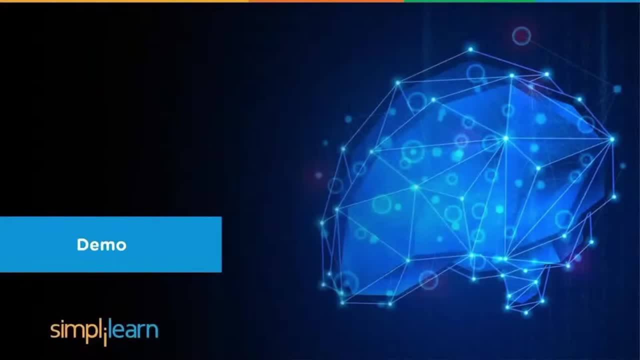 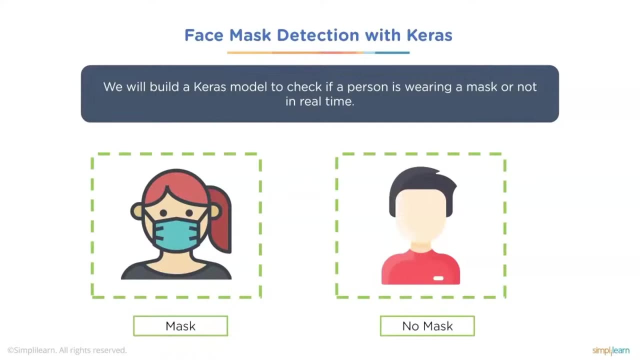 Uh, we did the basic- uh, demo up above for just pulling in a cross- And then we went into a cross model uh, where we pulled in data to see whether someone was wearing a mask or not. So very useful in today's world as far as a fully 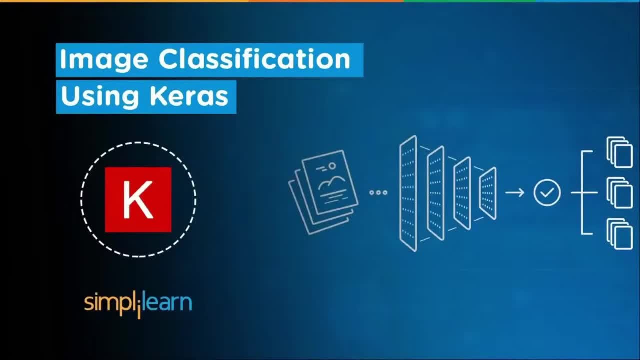 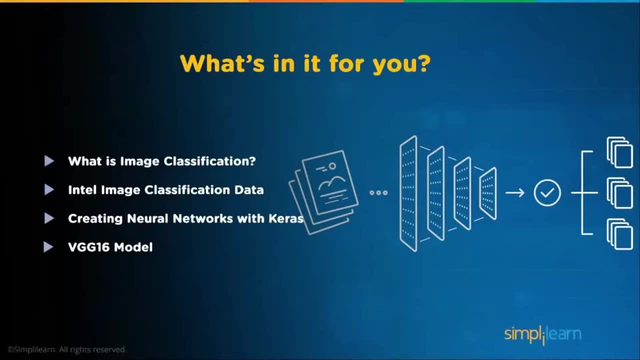 Running application and we're going to take a look at image classification using cross and the basic setup, And we're actually looking at two different demos on here. Uh, what's in it for you today? What is image classification? Intel image classification data, creating neural networks with cross and the VGG 16 model? 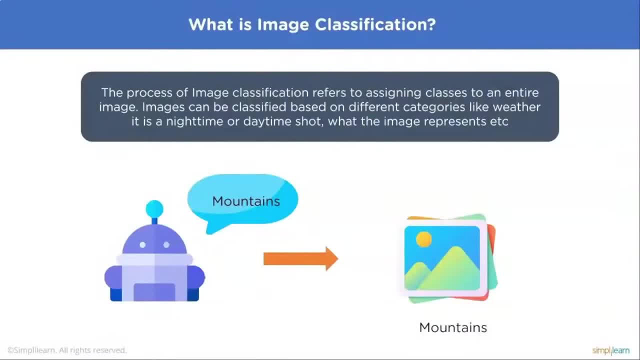 What is image classification? The process of image classification refers to assigning classes to an entire image. Images can be classified based on different categories, like whether it is a nighttime or daytime shot, what the image represents, et cetera. And you can see here we have uh, mountains looking for mountains. 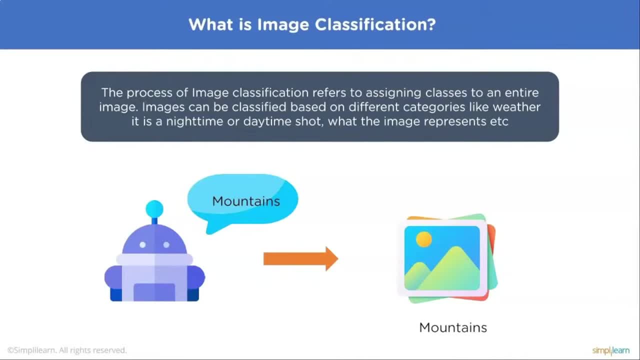 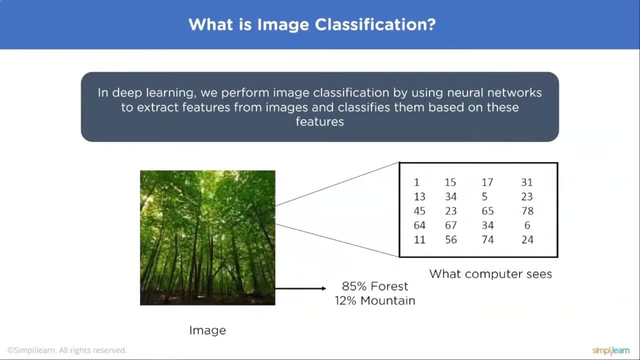 We'll actually be doing some uh uh pictures of scenery and stuff like that. In deep learning. we perform image classification by using neural networks to extract features from images and classifies them based on these features. And you can see here where it says like what computer sees, and it says: oh yeah, we see mostly forest, maybe a little bit of mountains, because of where the image is. 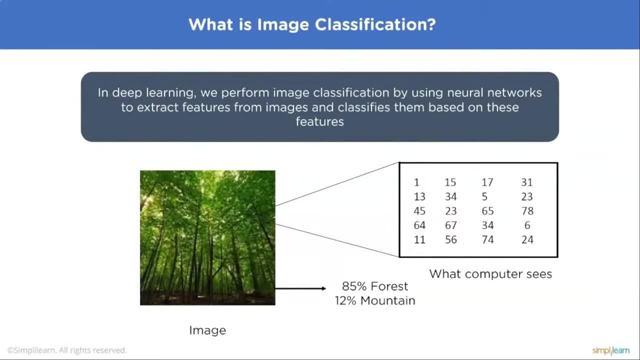 Um, and this is really where one of the areas that neural networks really shines- Um, if you try to run this stuff through, uh, more like a linear regression model, you'll still get results, uh, but the results kind of miss a lot of things as they, as the neural networks get better and better at what they do with different tools we have out there. 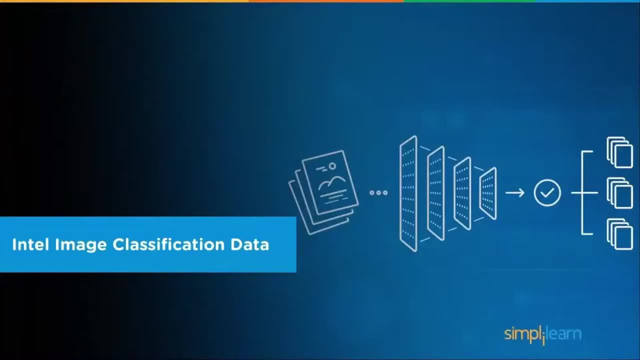 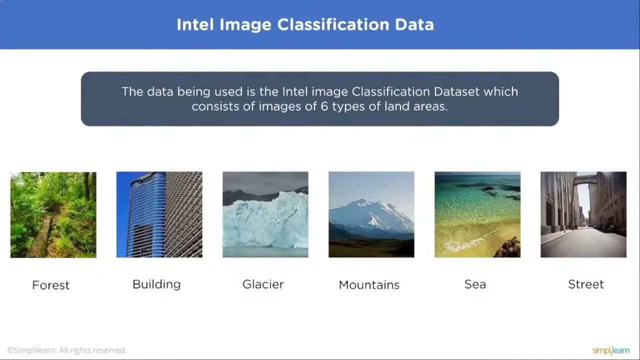 Uh, so Intel image classification data. the data being used is the Intel image classification data set, which consists of images of six types of land areas, And so we have forest building, glaciers and mountains, sea and street. uh, and you can see here is a couple of the images out of there as a setup in the in the um uh Intel image classification data that they use. 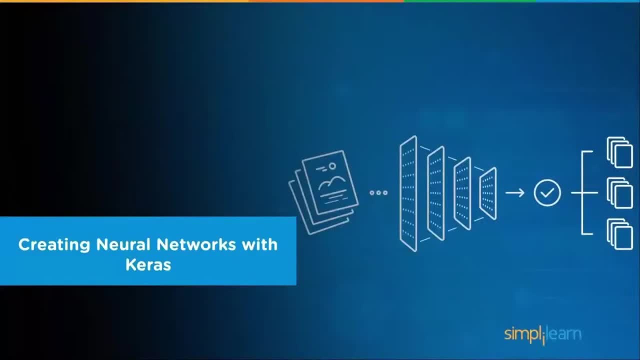 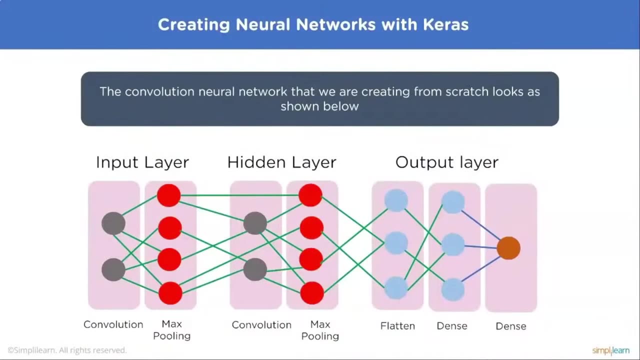 And then we're going to go into creating a network. So we're going to go into creating a network, So we're going to go into creating neural networks with Keras. The convolutional neural network that we are creating from scratch looks uh, as shown below. 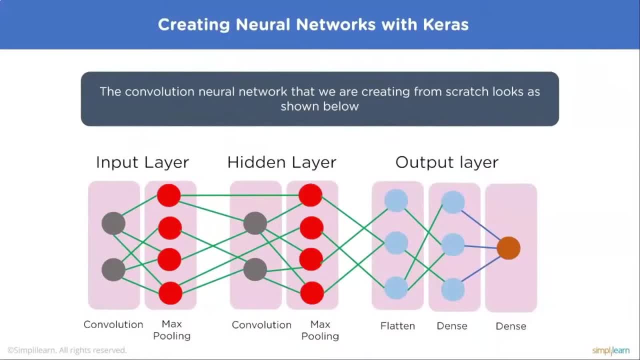 You can see, here we have our input layer. Um, they haven't listed max pooling, Uh, so you have, as you're coming in, with the input layer and this. the input layer is actually um before this, but the first layer that it's going to go into is going to be a convolutional neural network. 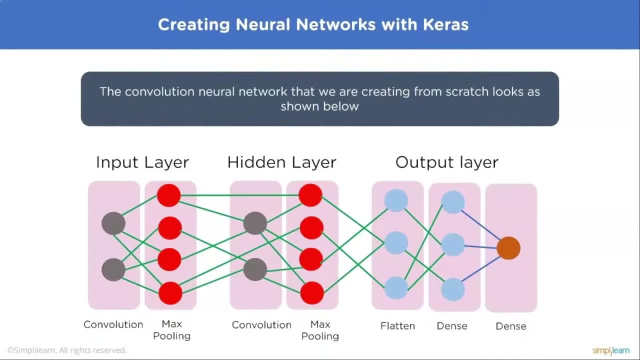 Then you have a max pooling that pools those the the convolutional neural networks returns. Uh, in this case they have two of those. That is very standard with convolutional neural networks. Uh, one of the ones that I was looking at earlier that was standard being used by um, one of the larger companies- I can't remember which one- for doing a large amount of identification, had two convolutional neural networks, each with their max pooling and then about 17 dense layers after it. 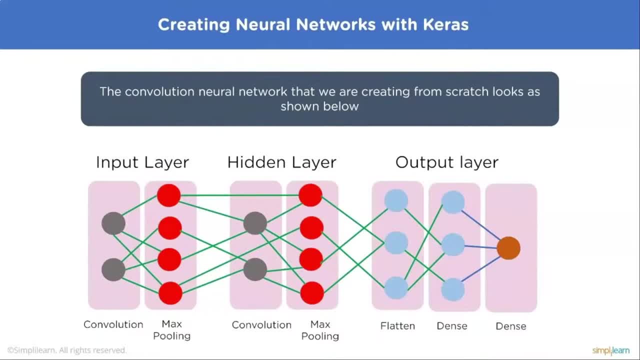 We're not going to do that heavy duty of a of a code, but we'll get you headed in the right direction and that gives you an idea of what you're actually going to be looking at when you look at the flattened part and then the dense. 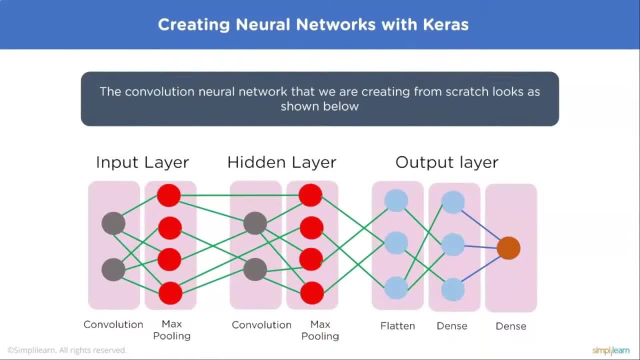 We're talking like 17 dense layers afterwards. Uh, I find that a lot of the stuff I've been working on, I end up maxing it out right around nine dense layers. It really depends on what you have going in and what you're working with. 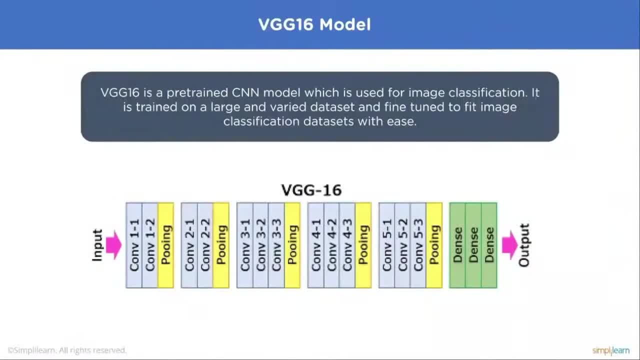 And the VGG16 model. Uh, VGG16 is a 3D model. It's a pre-trained CNN model which is used for image classification. It is trained on a large, varied data set and fine-tuned to fit image classification data sets with ease. 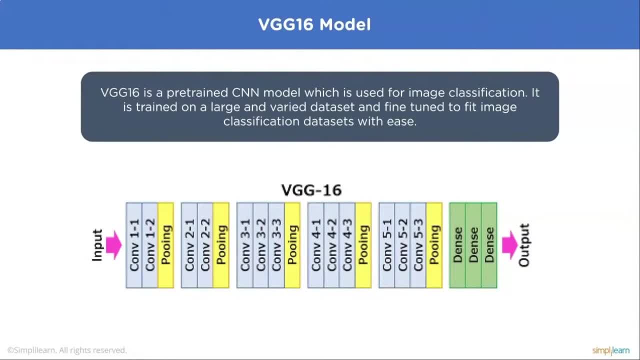 And you can see down here we have the input coming in, uh, the convolutional neural network one to one, one to two and then pooling. And then we do two to one, two to two, convolutional neural network, then pooling. 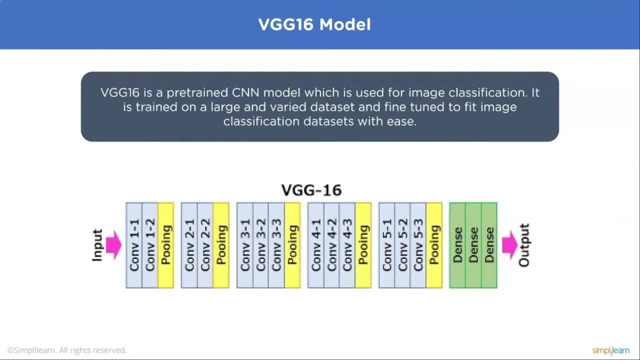 Three to two and you can see there's just this huge layering of convolutional neural networks And in this case they have five such layers going in And then you have three dense going out, or uh more. Now, when they took this setup, this actually won an award, uh, back in 2019 for this particular setup. 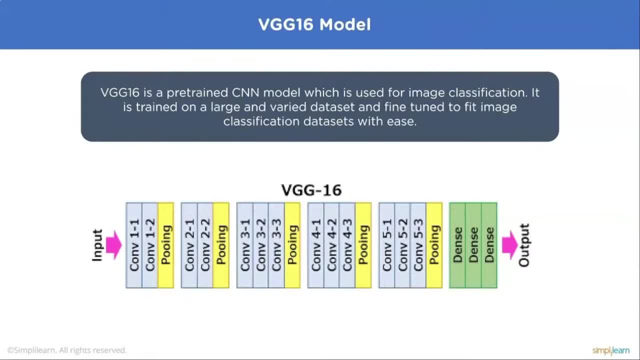 Uh, and it does. it does really good, except that, again, um, we only show the three dense layers here And, as you find out, depending on your data going in and what you have set up, uh, that really isn't enough on one of these setups. Uh, and it does. it does really good, except that, again, um, we only show the three dense layers here And, as you find out, depending on your data going in and what you have set up, uh, that really isn't enough on one of these setups. 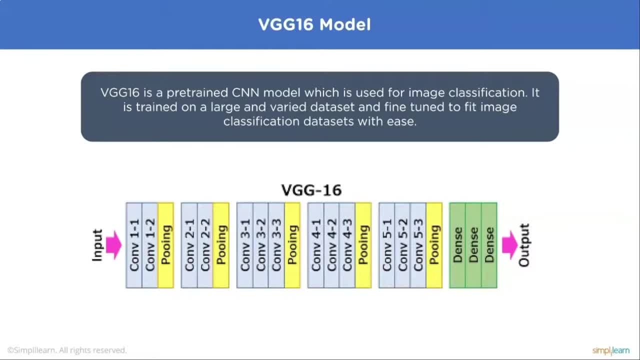 And I'm gonna show you why we restricted it, because it does take up a lot of processing power in some of these things. And I'm gonna show you why we restricted it, because it does take up a lot of processing power in some of these things. 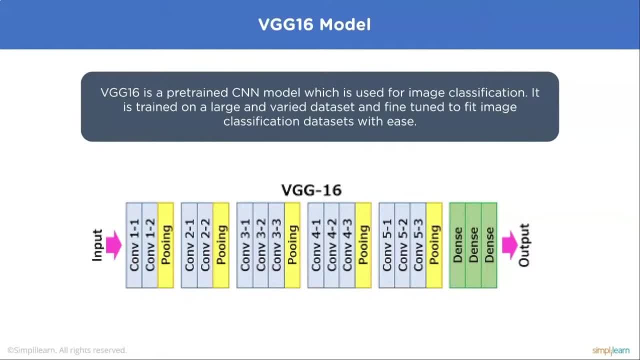 And I'm gonna show you why we restricted it, because it does take up a lot of processing power in some of these things. So let's go ahead and roll up our sleeves and we're gonna look at both the setups. So let's go ahead and roll up our sleeves and we're gonna look at both the setups. 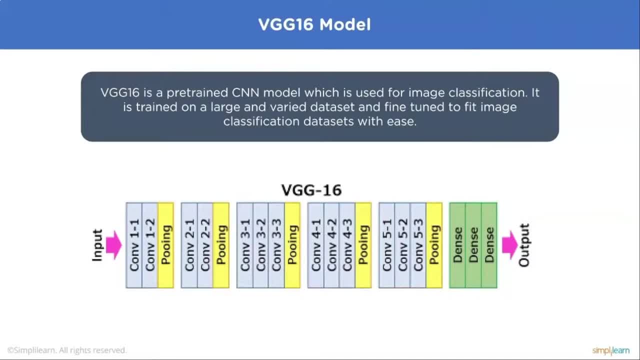 We're gonna start with the um- uh, the first classification, um- and then we'll go into the VGG16 and show you how that's set up. We're gonna start with the um and then we'll go into the VGG16 and show you how that's set up. 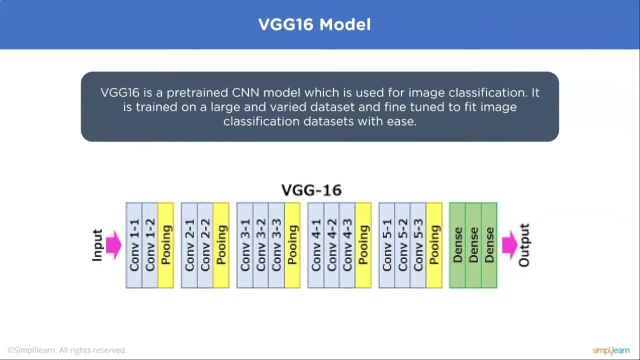 We're gonna start with the um and then we'll go into the VGG16 and show you how that's set up. Now I'm gonna be using Anaconda, and let me flip over to my Anaconda so you can see what that looks like. 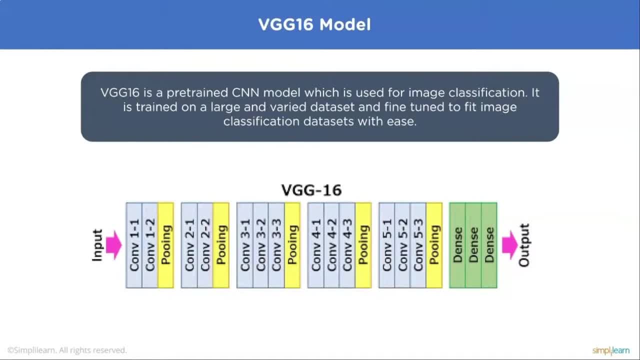 Now I'm gonna be using Anaconda, and let me flip over to my Anaconda so you can see what that looks like. Now I'm gonna be using Anaconda, and let me flip over to my Anaconda so you can see what that looks like. 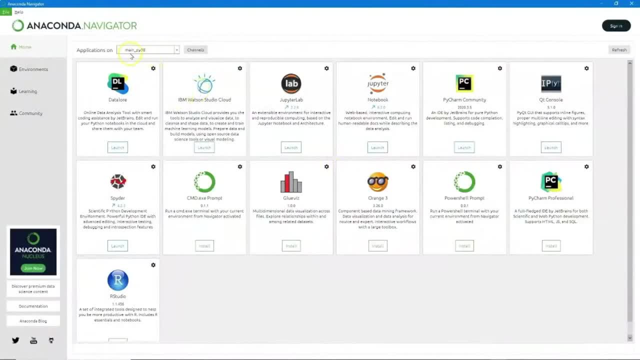 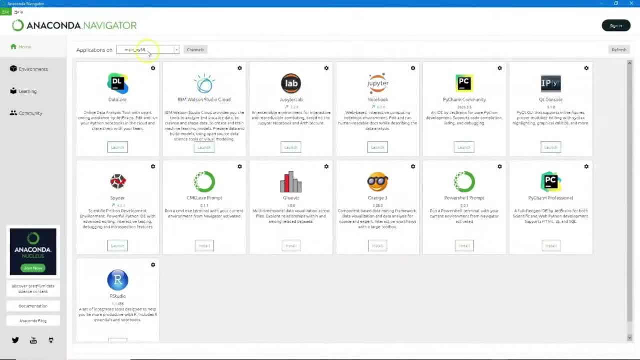 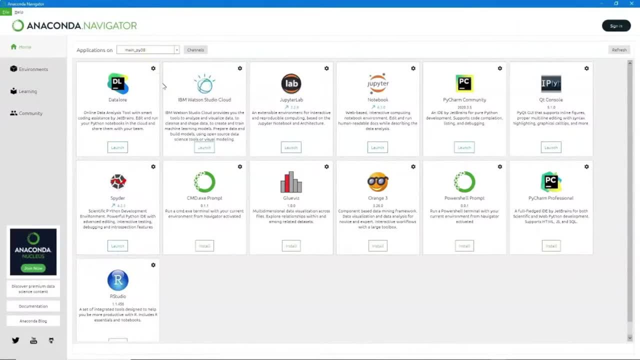 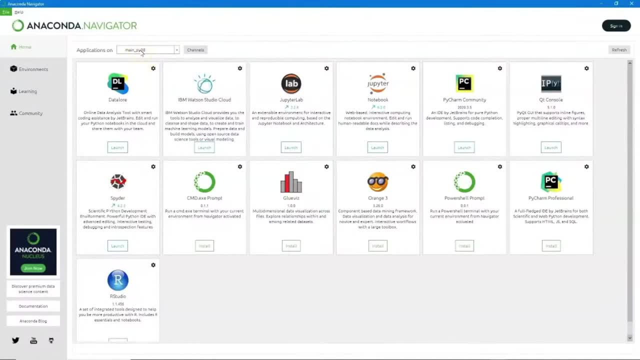 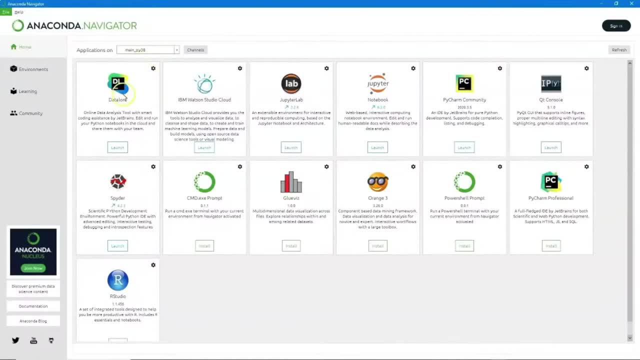 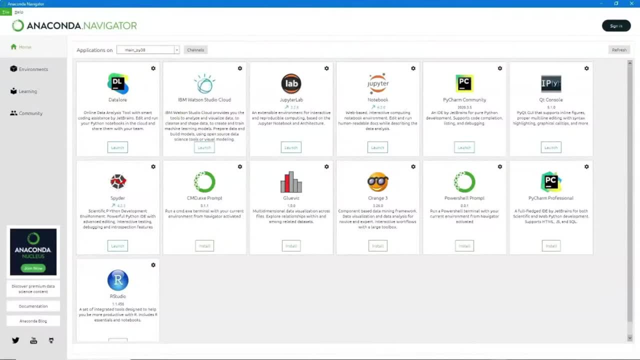 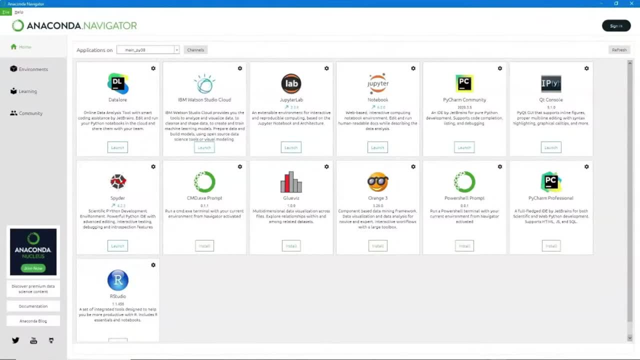 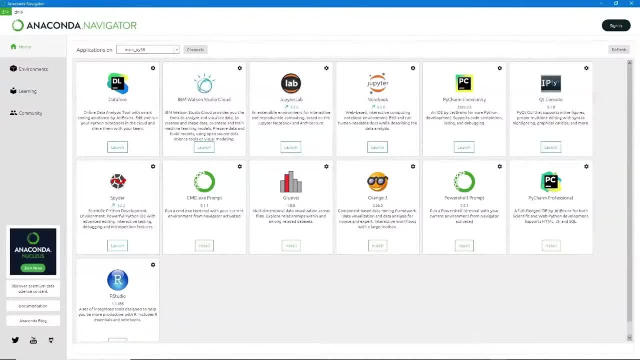 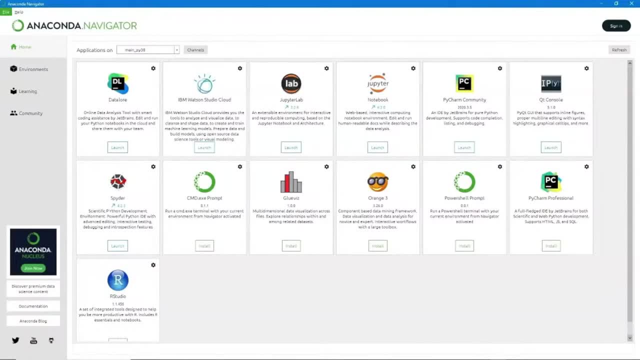 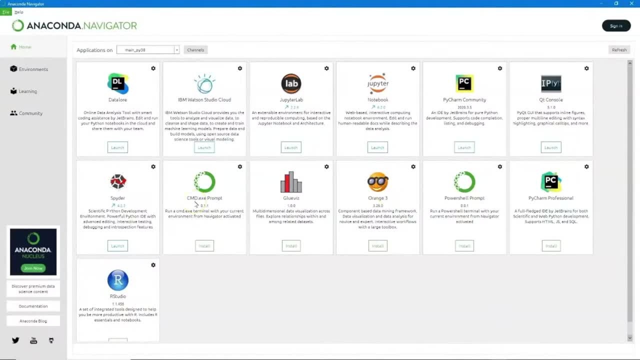 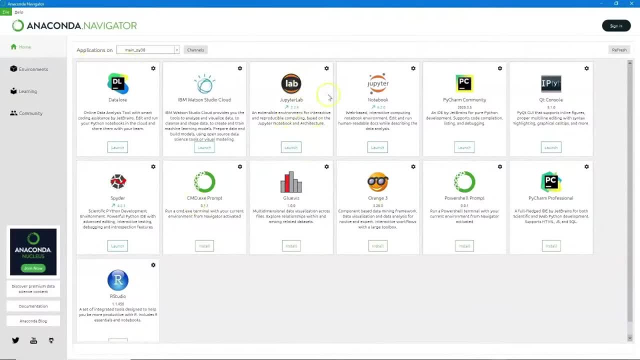 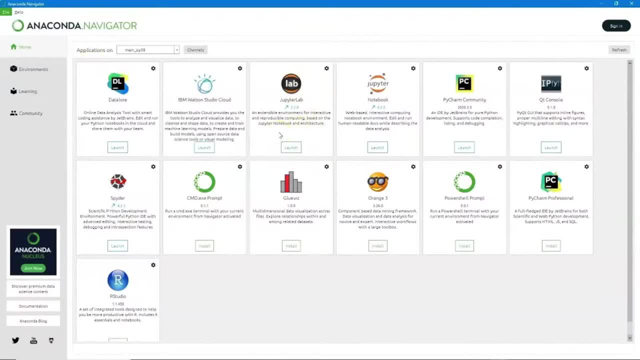 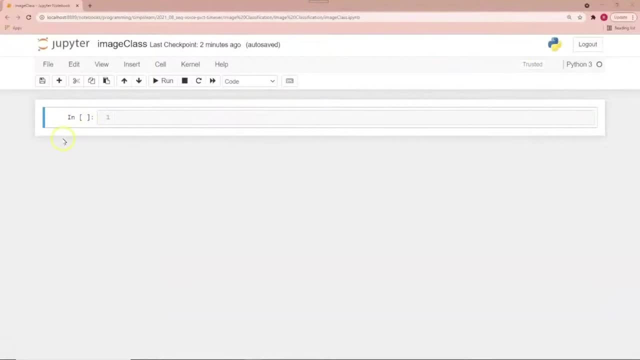 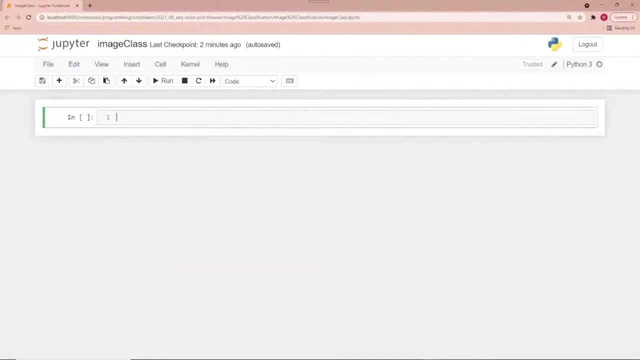 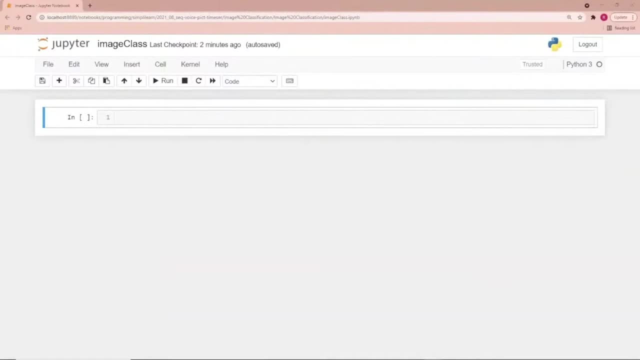 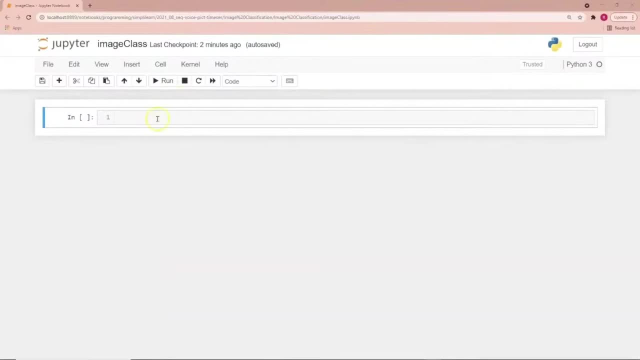 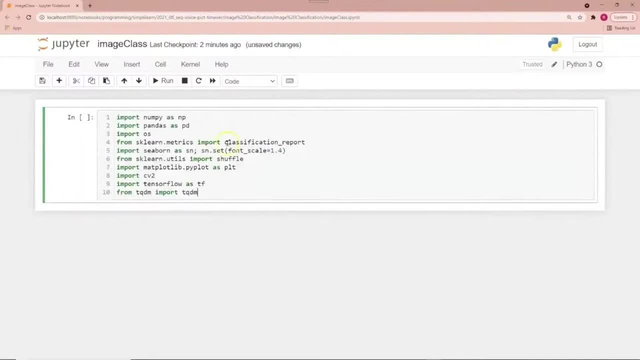 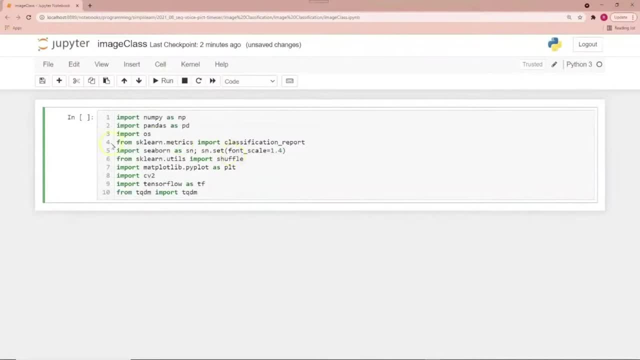 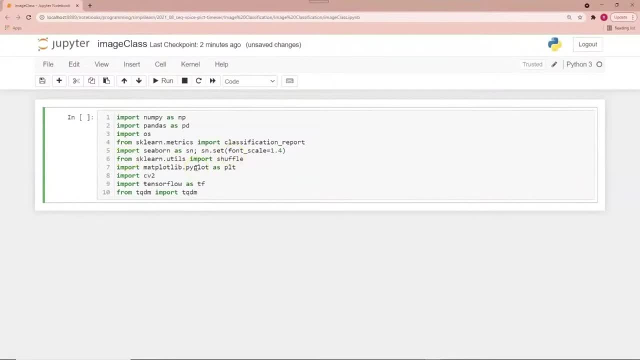 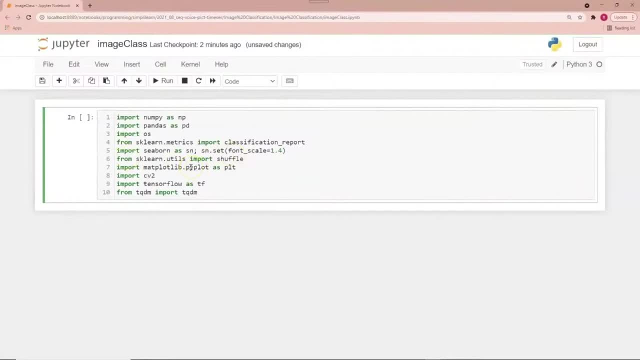 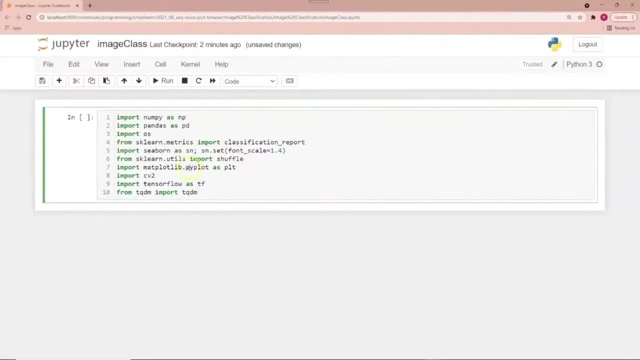 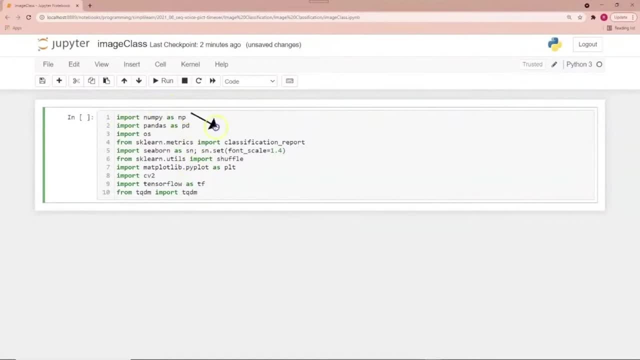 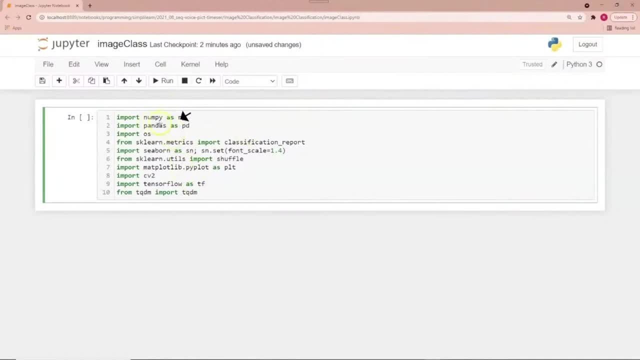 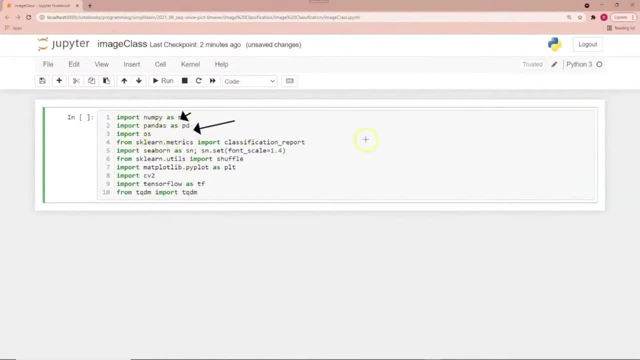 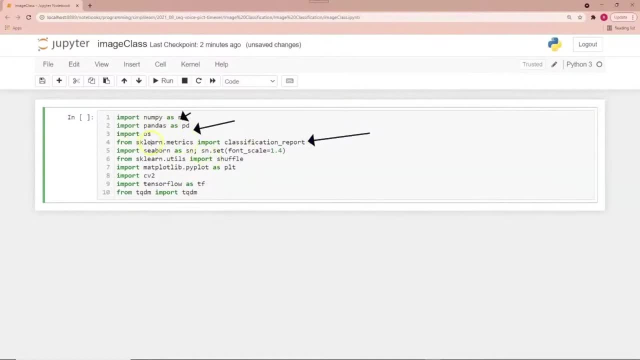 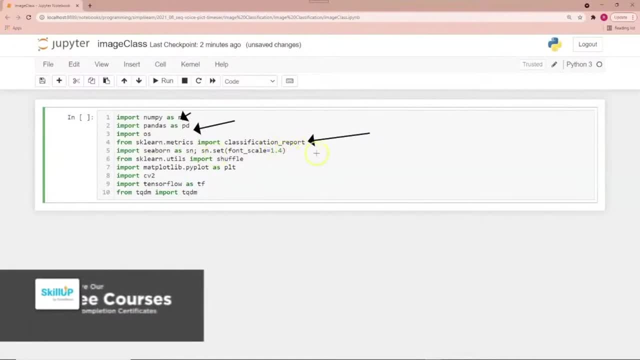 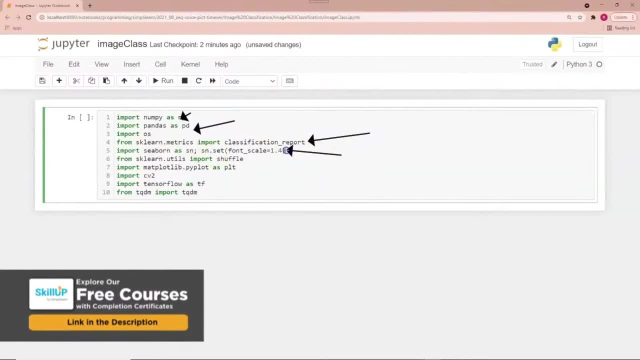 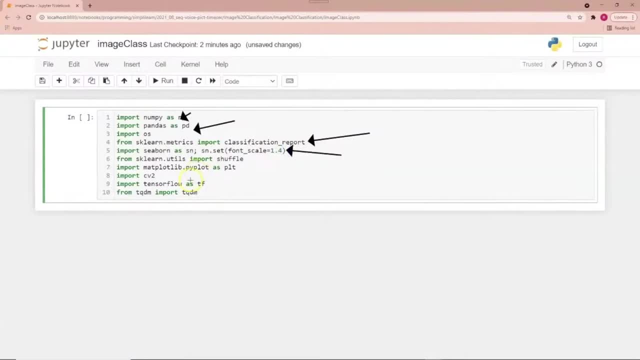 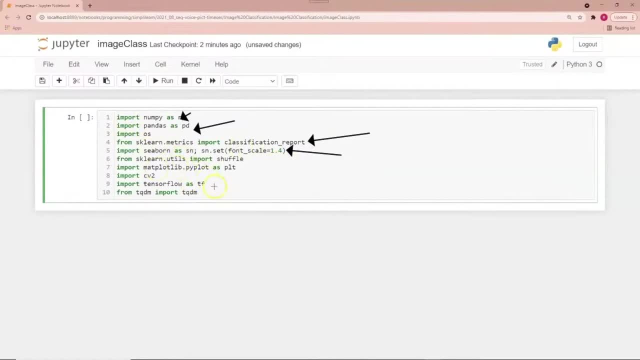 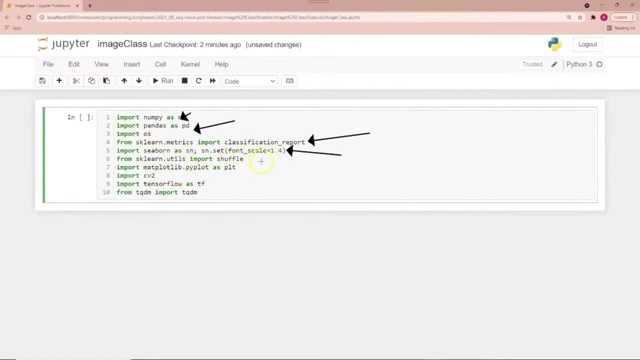 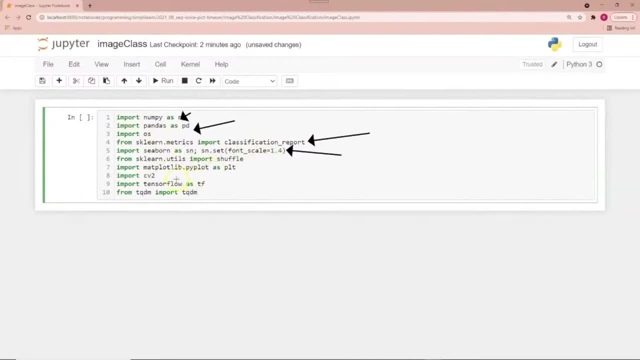 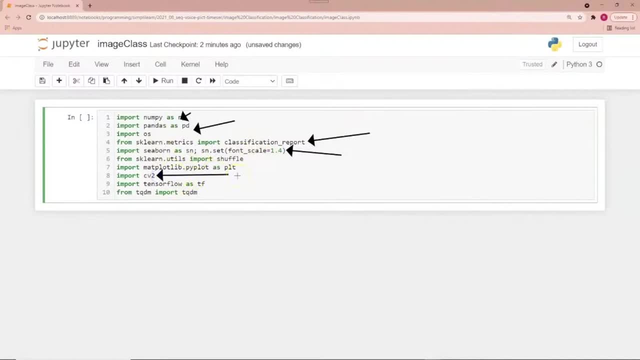 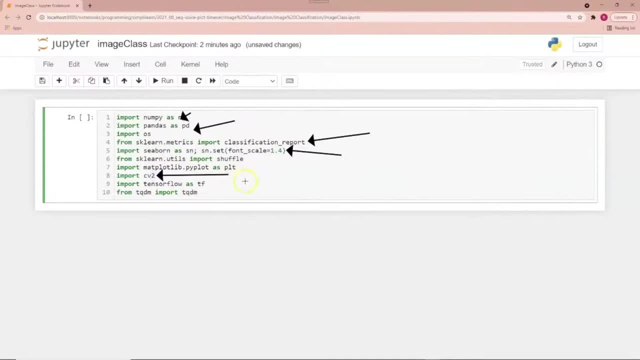 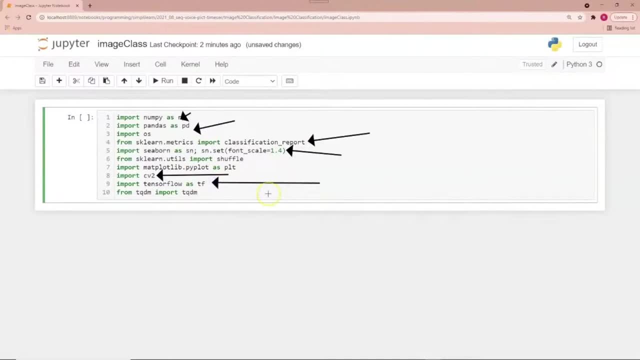 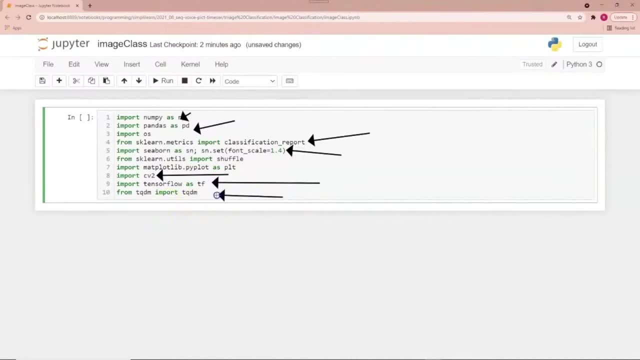 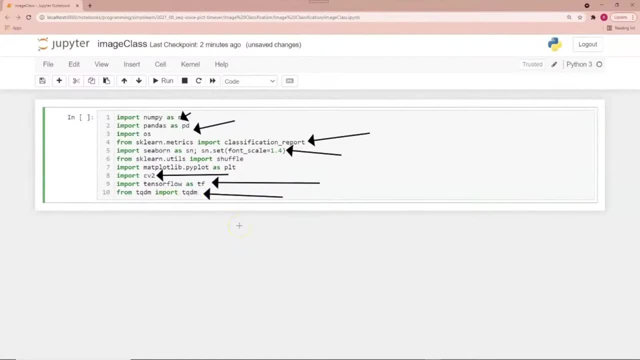 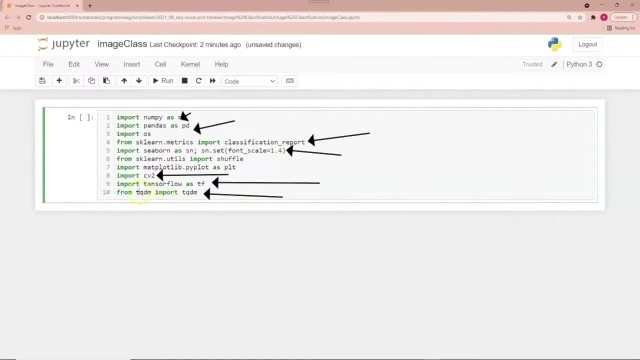 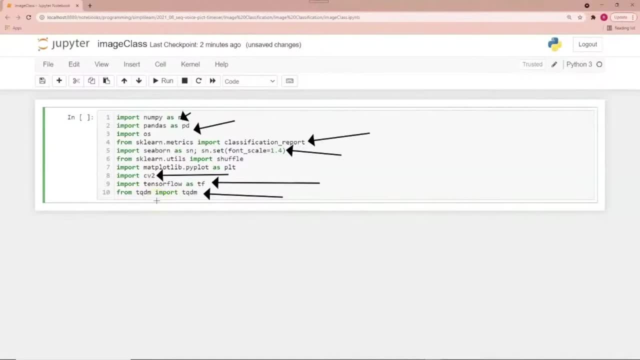 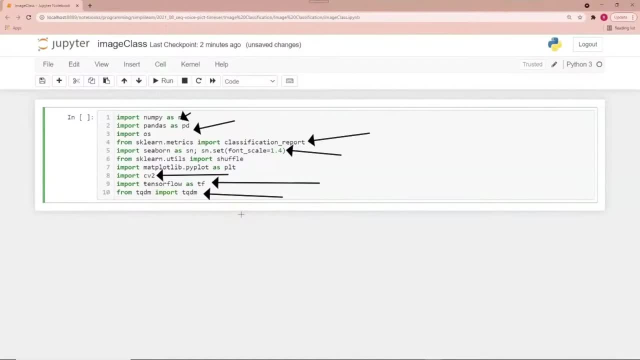 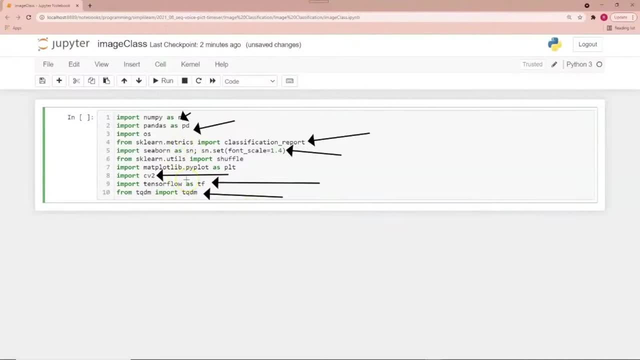 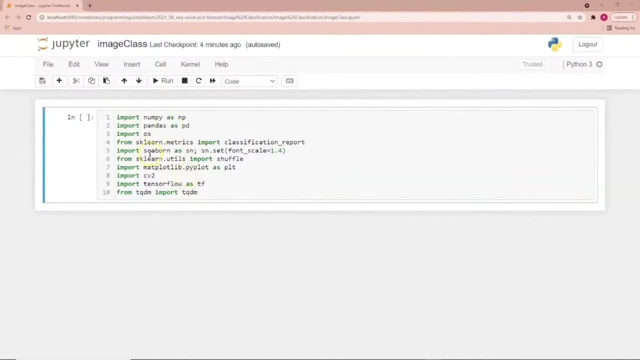 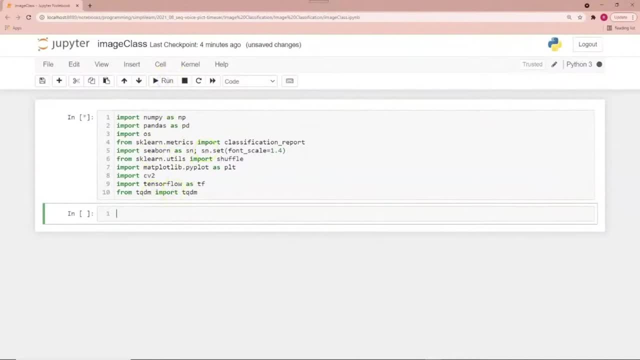 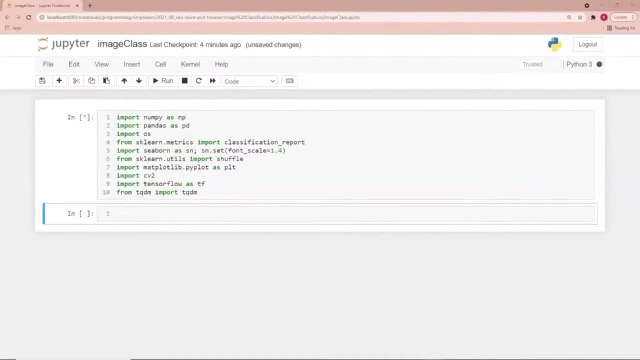 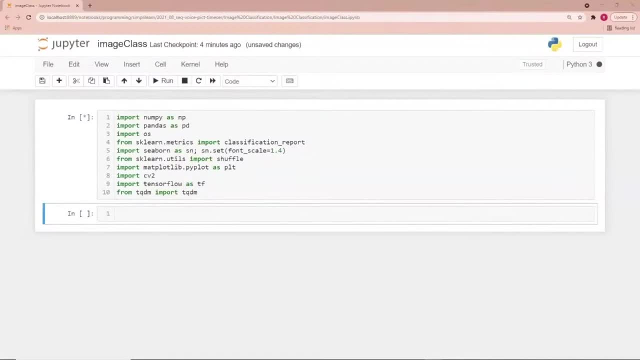 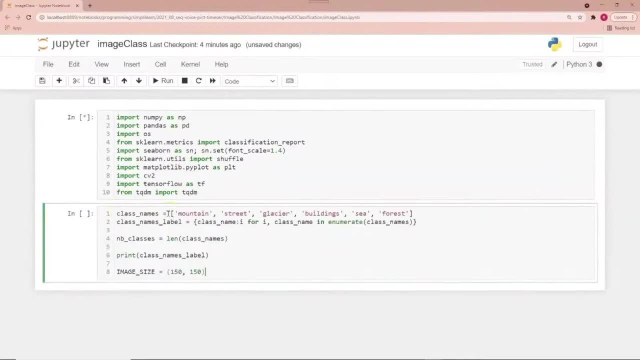 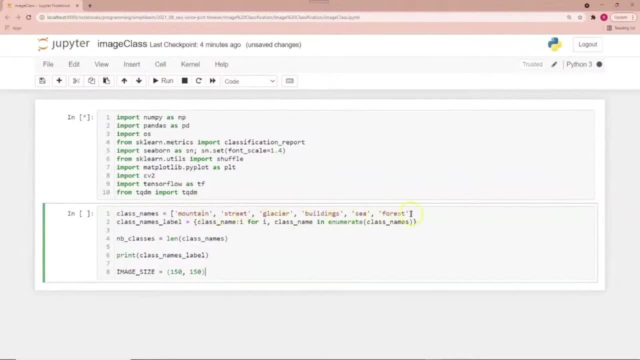 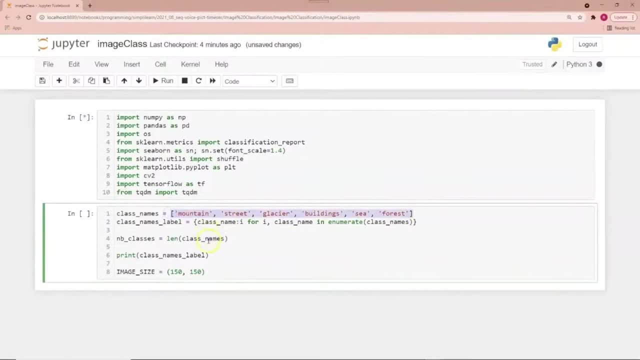 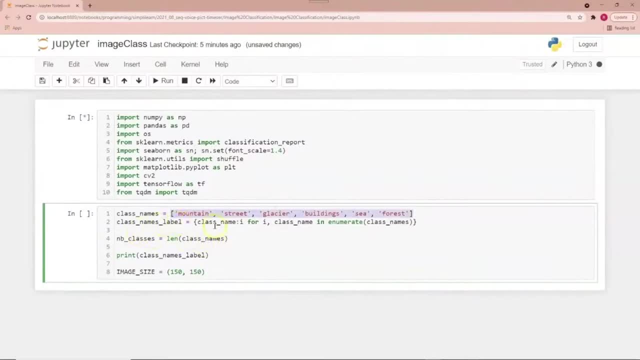 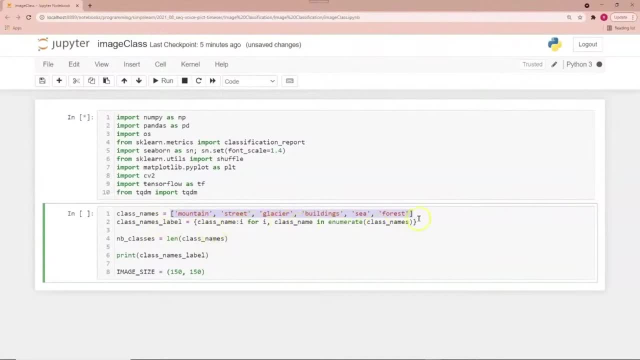 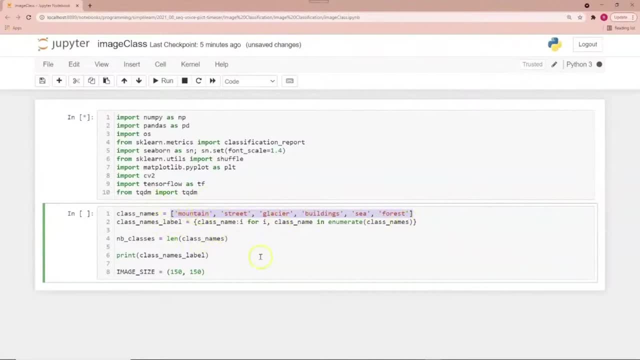 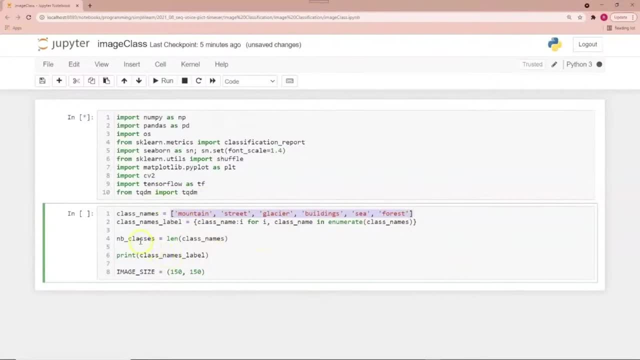 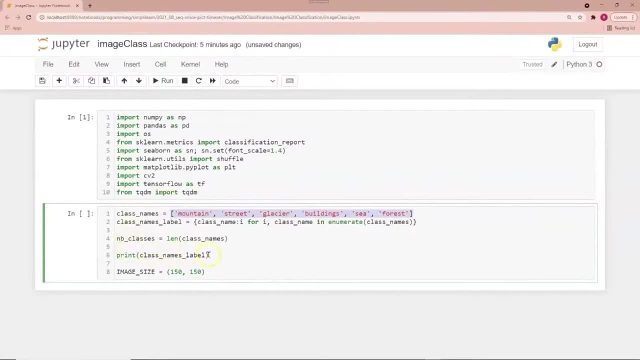 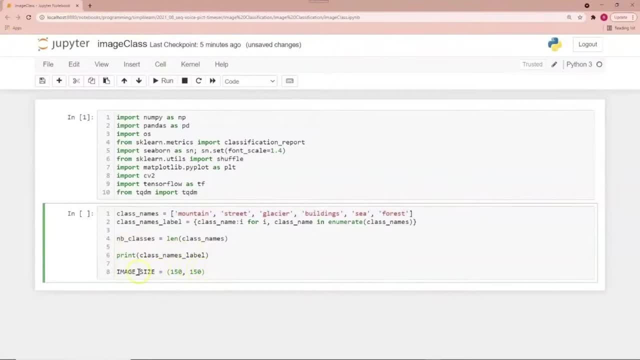 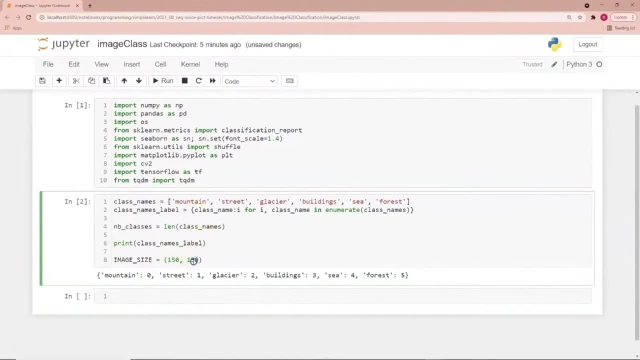 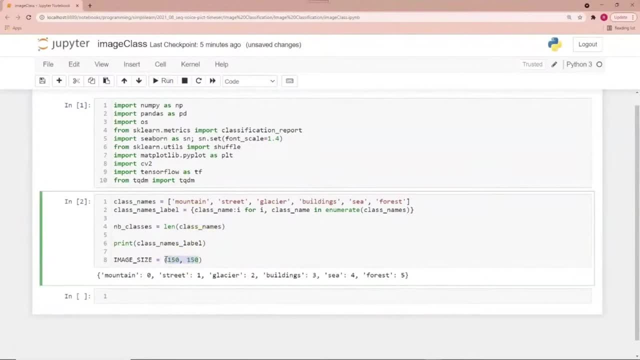 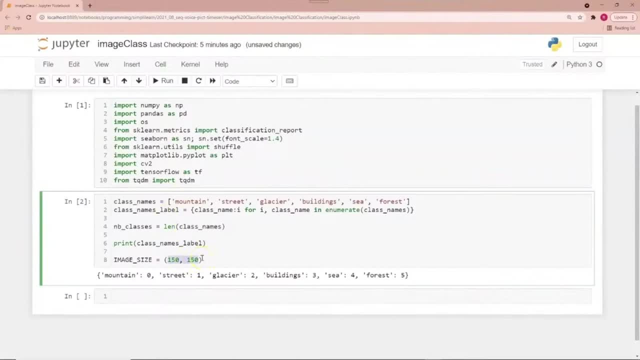 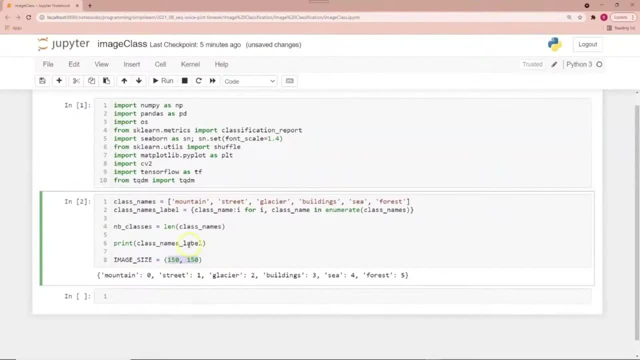 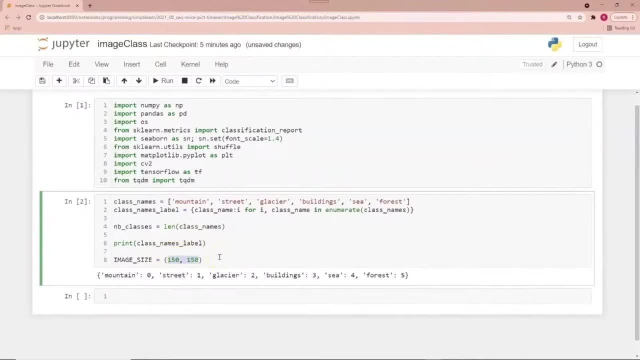 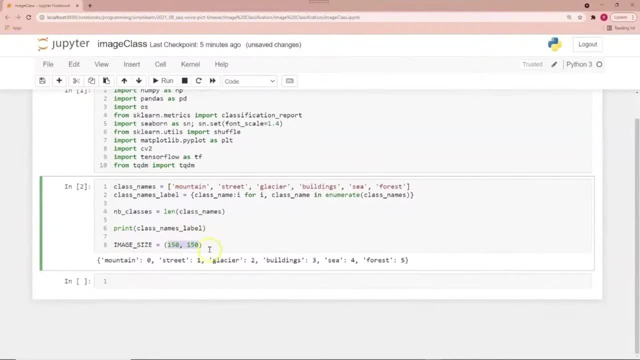 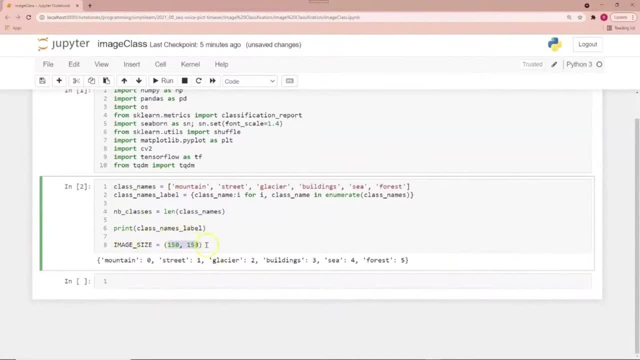 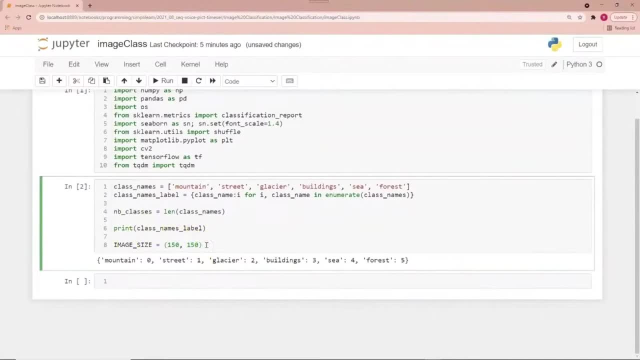 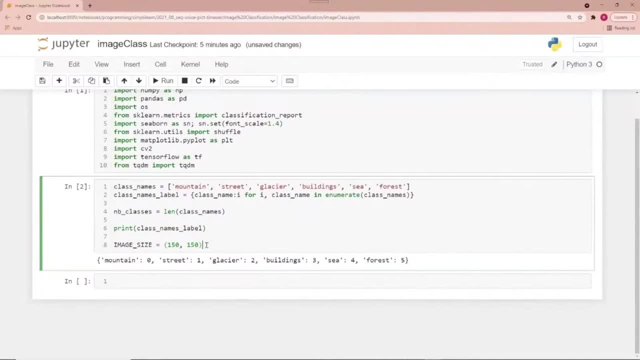 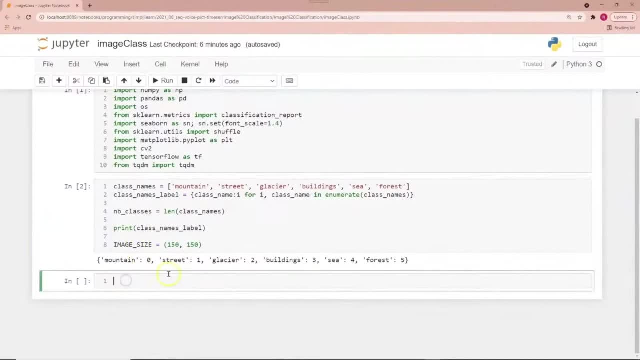 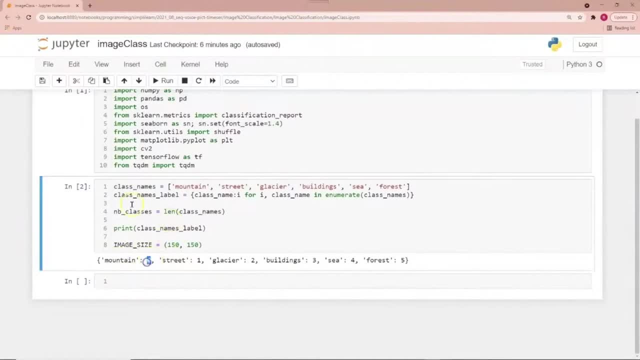 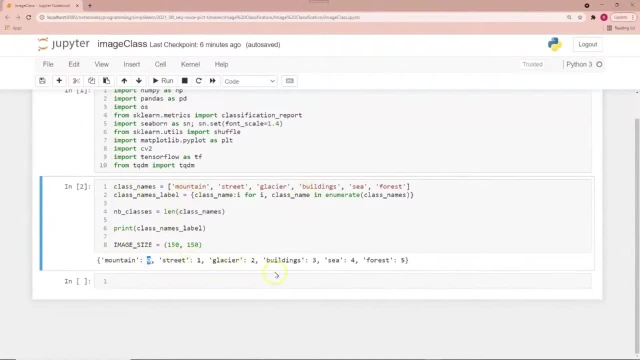 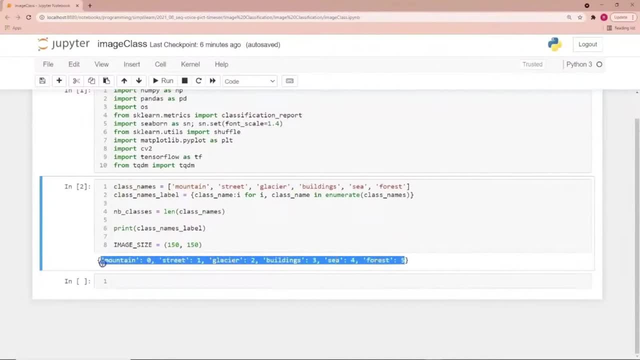 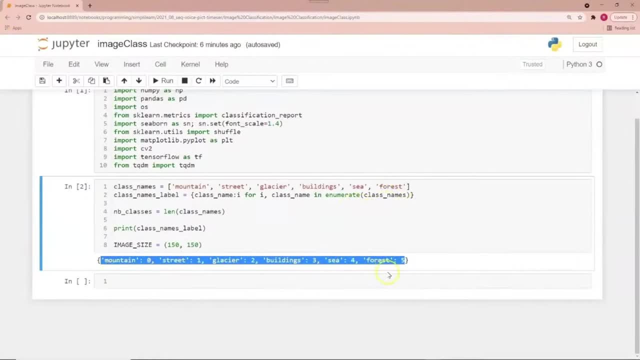 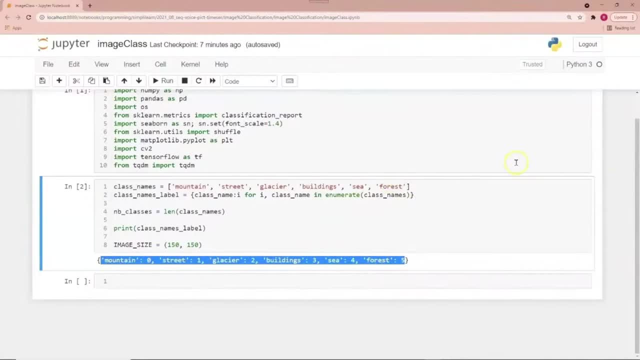 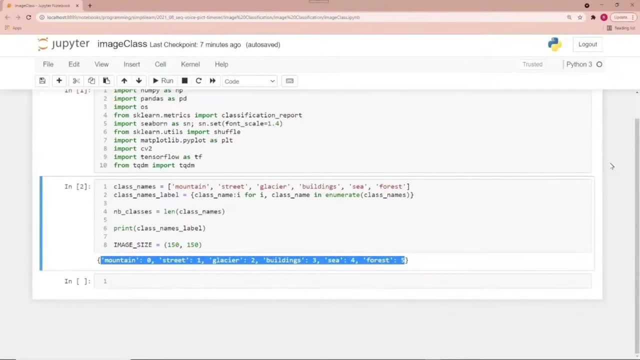 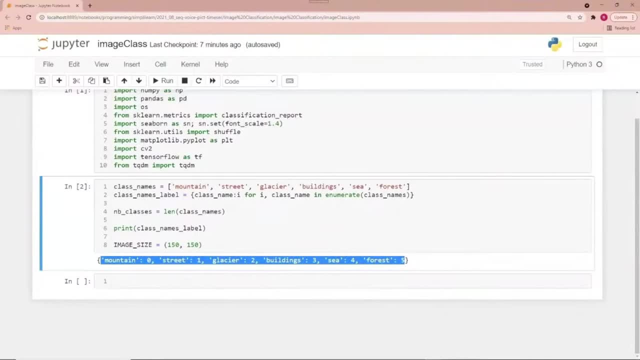 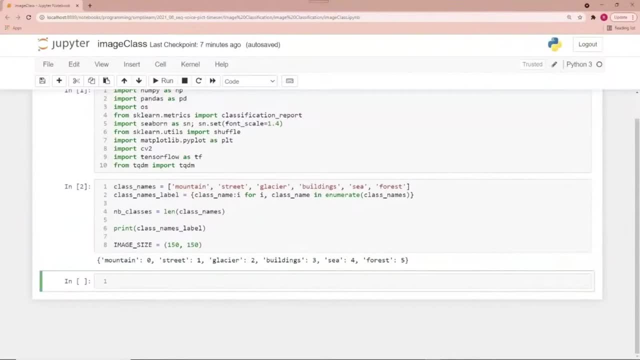 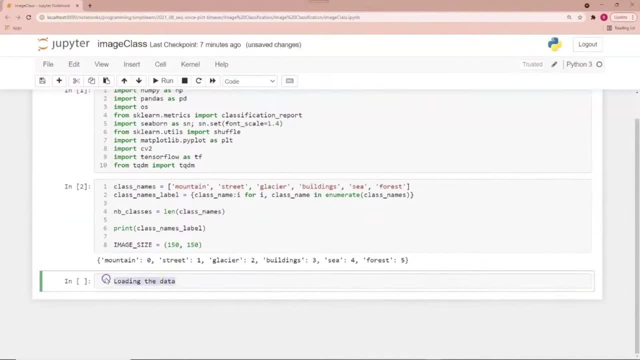 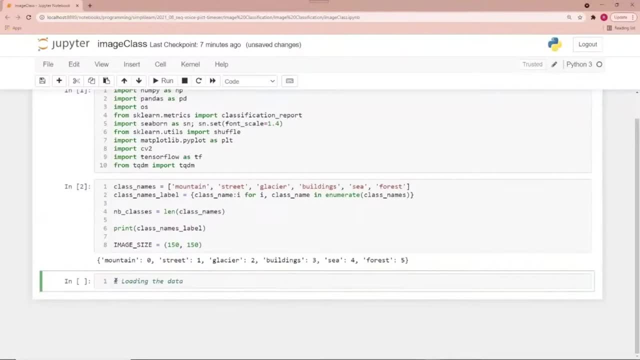 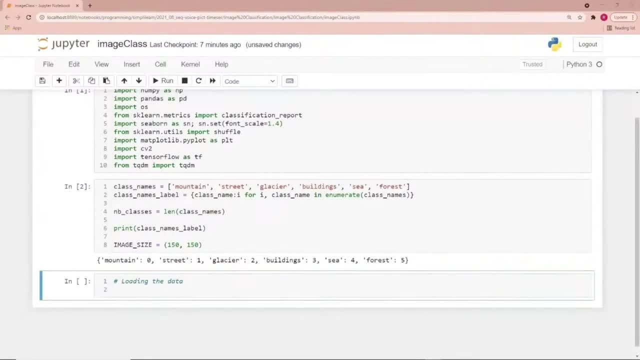 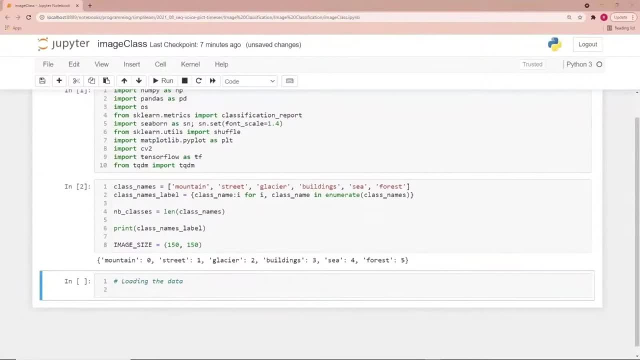 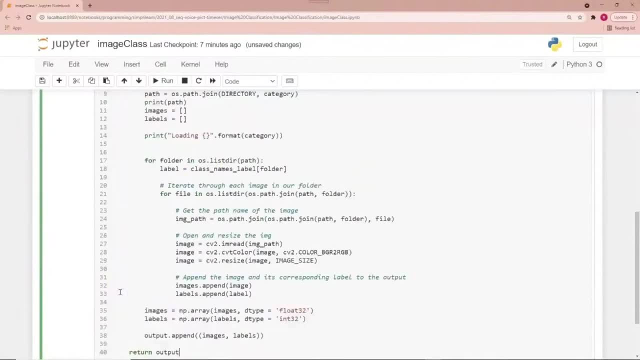 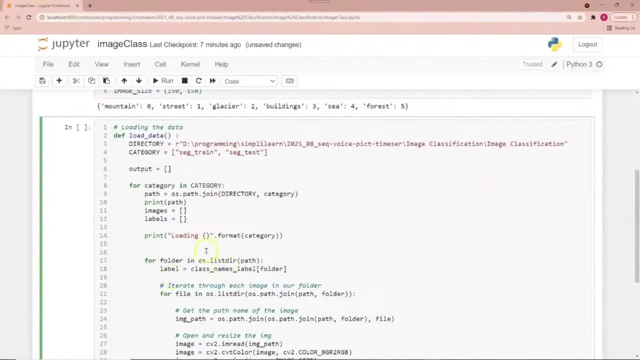 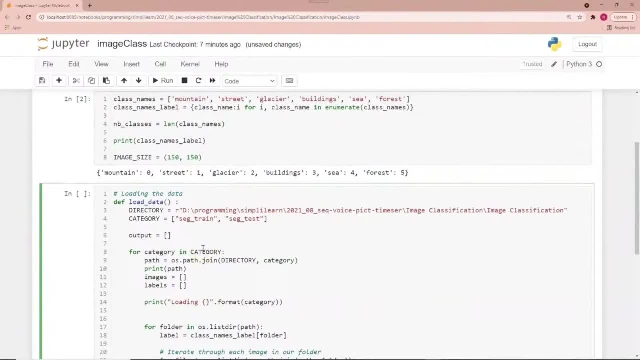 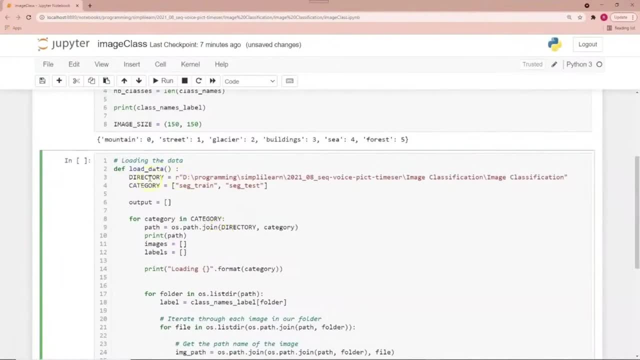 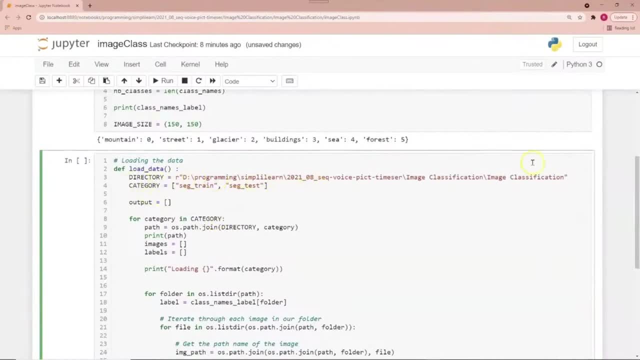 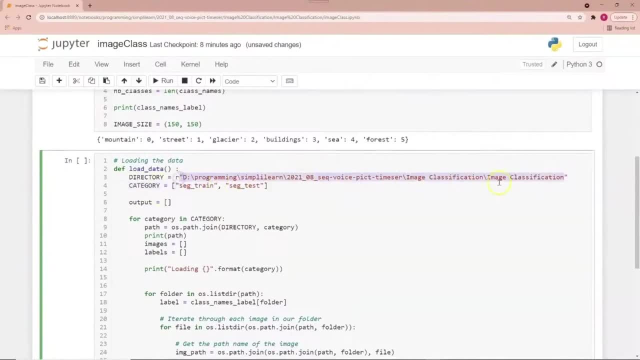 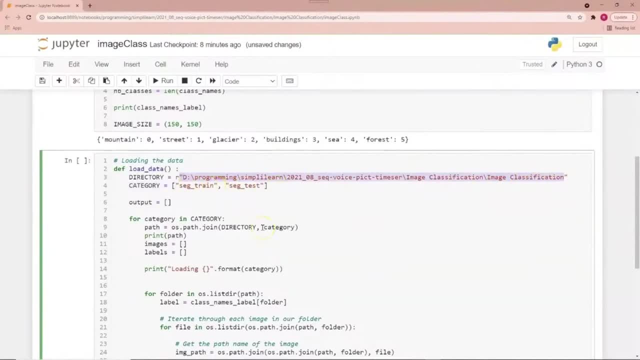 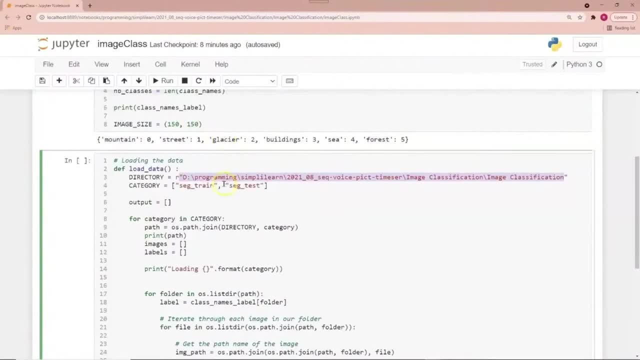 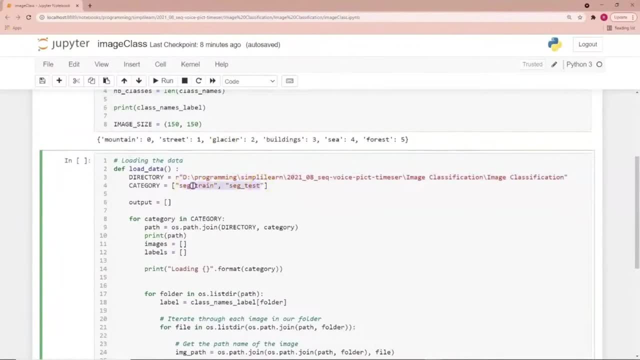 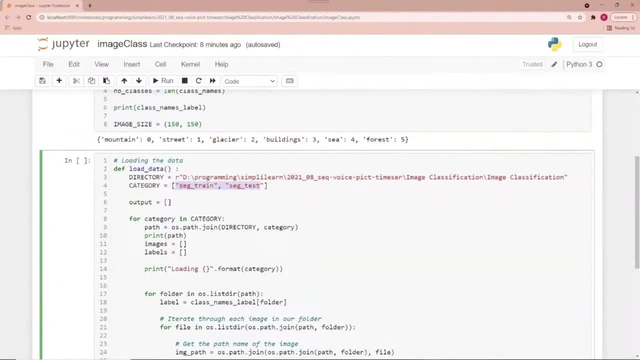 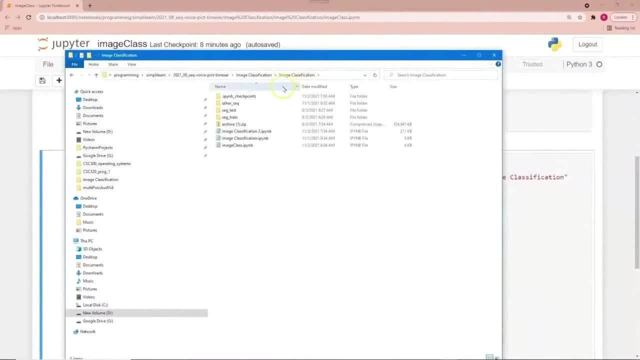 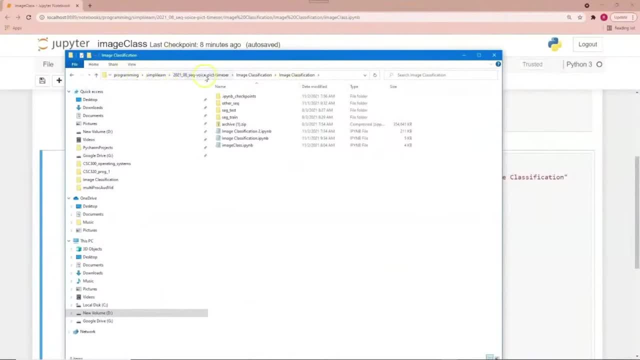 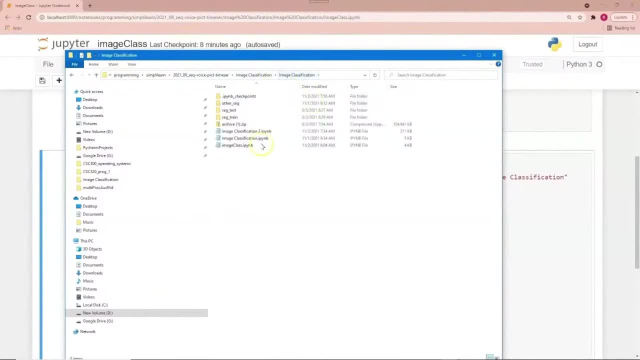 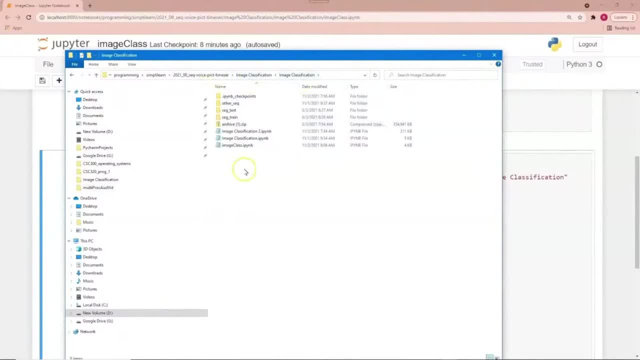 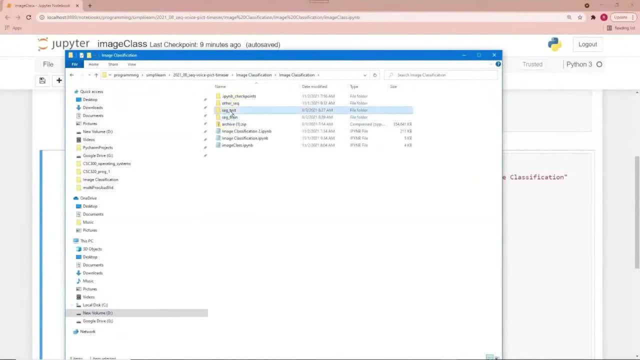 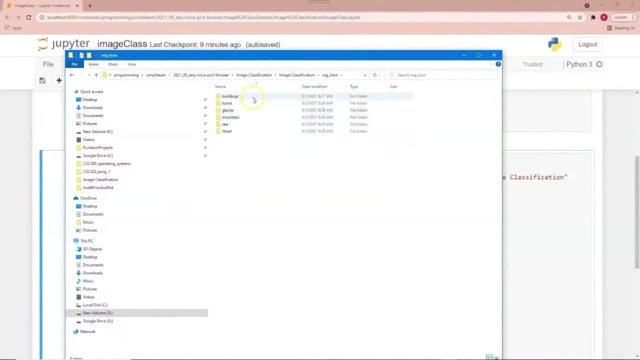 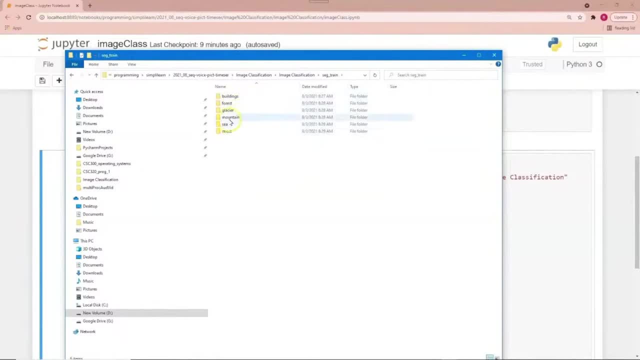 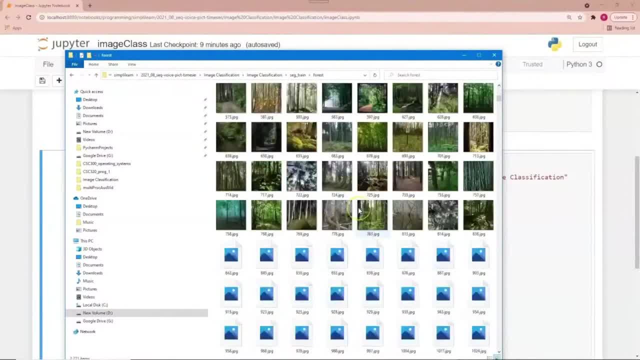 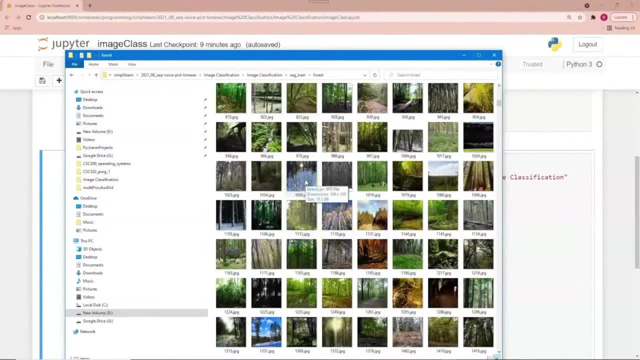 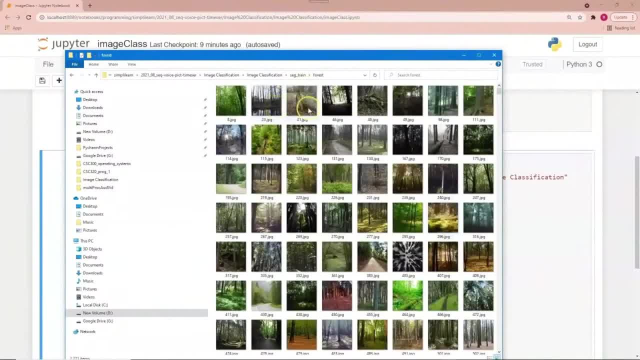 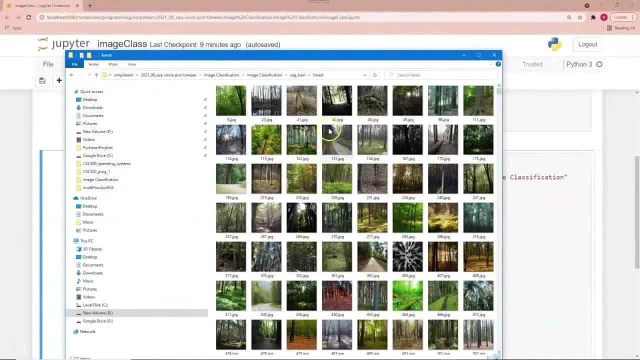 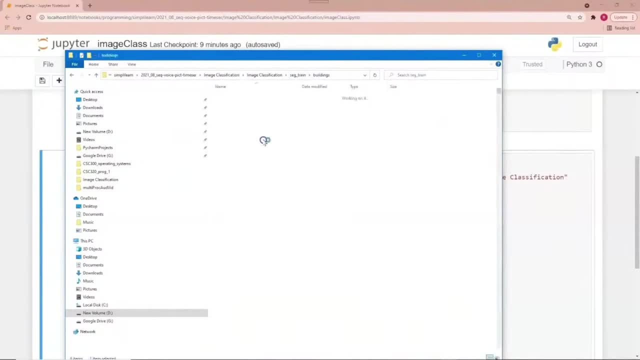 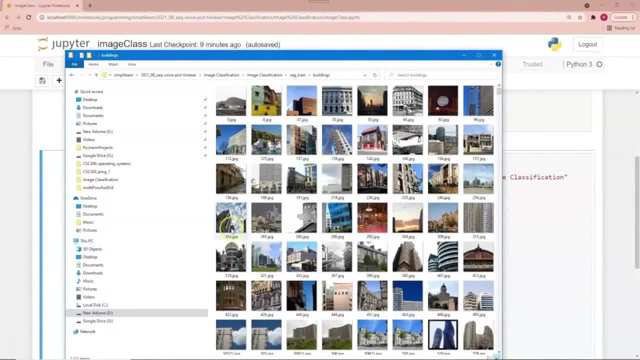 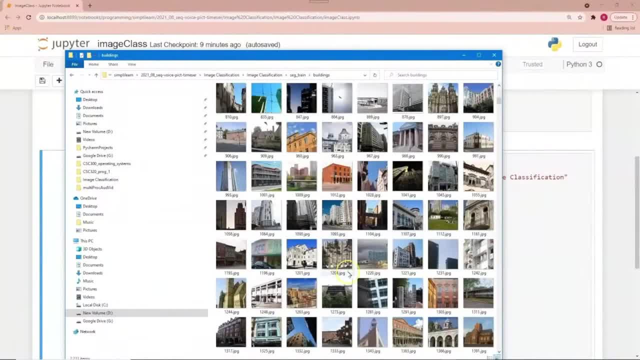 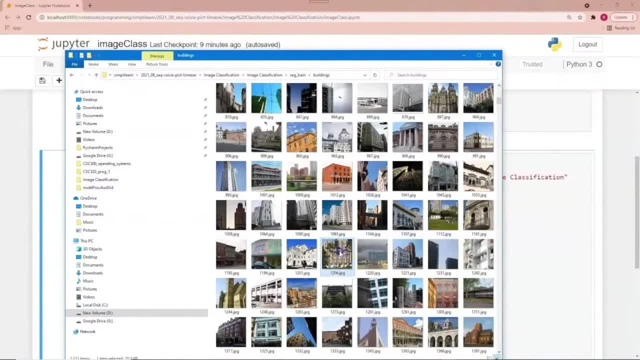 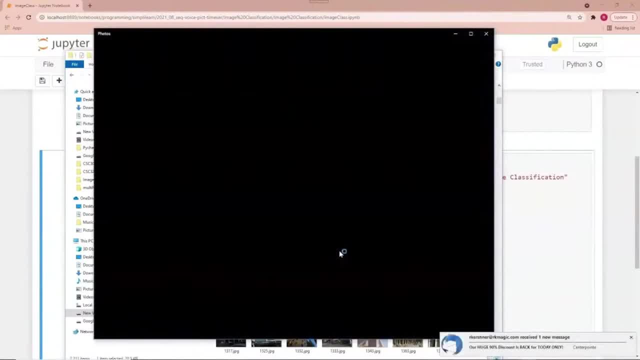 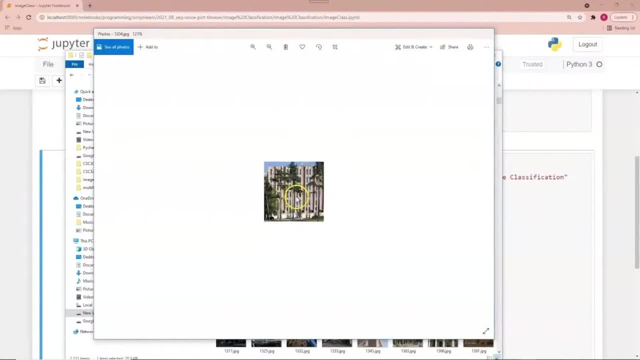 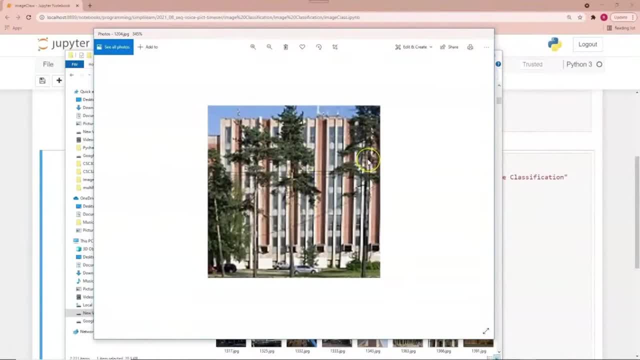 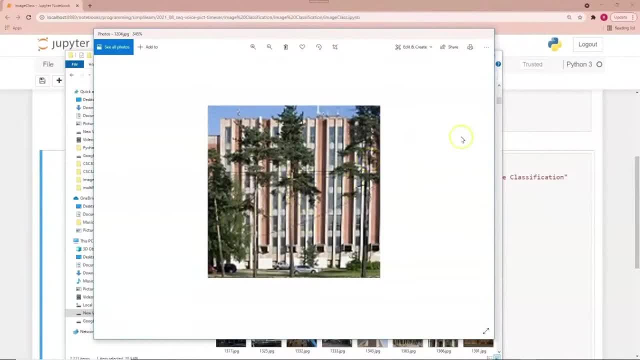 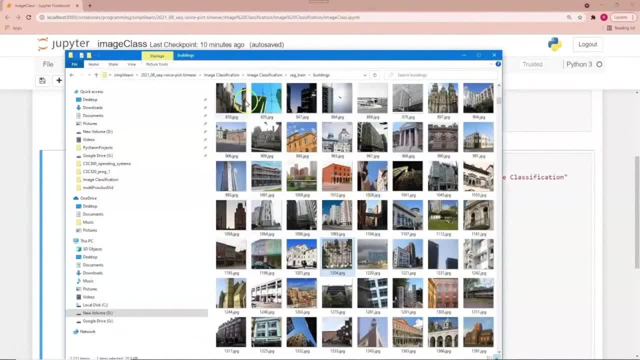 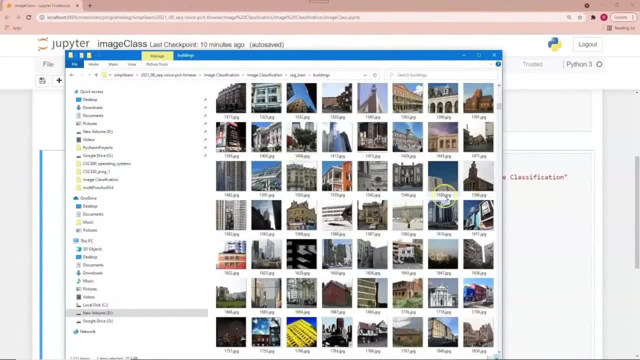 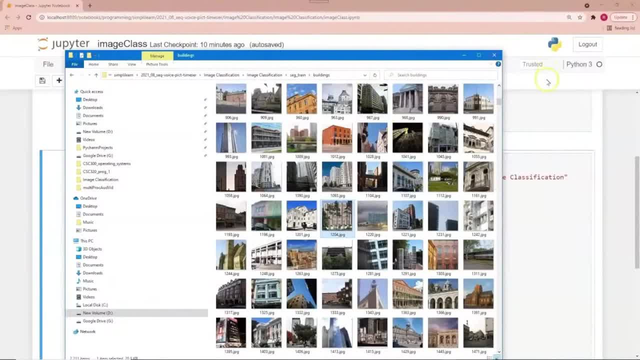 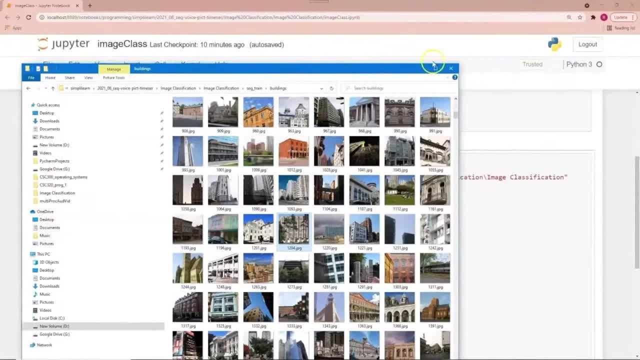 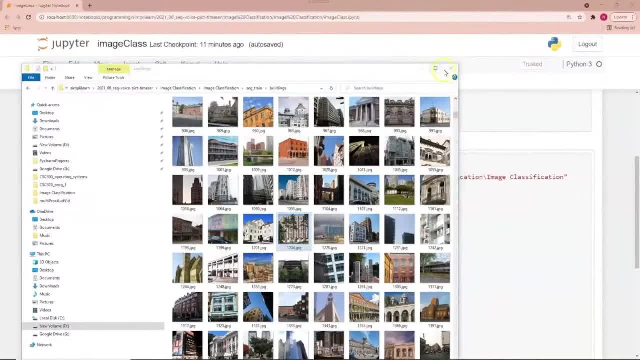 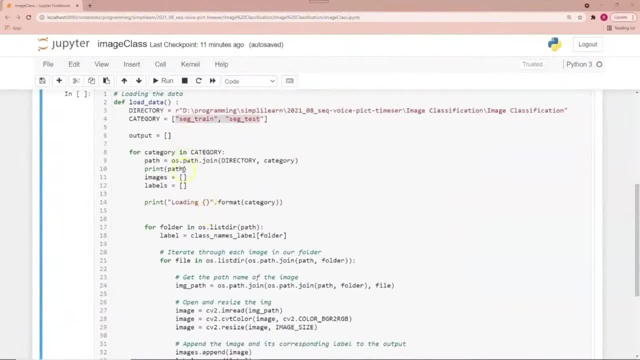 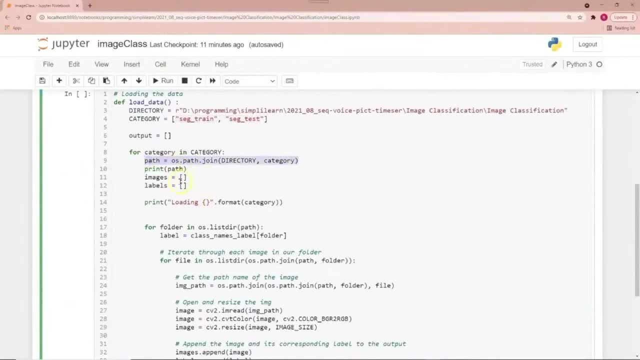 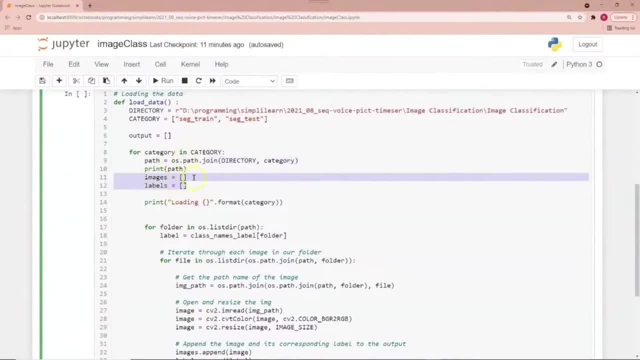 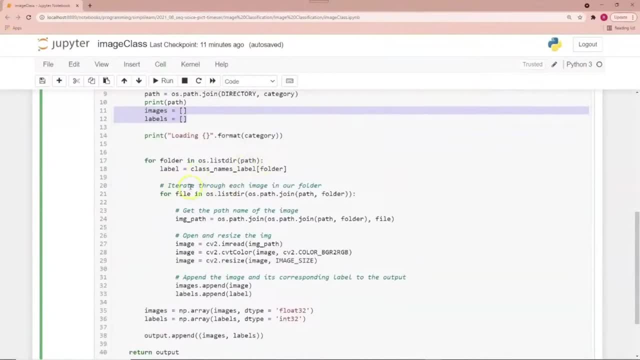 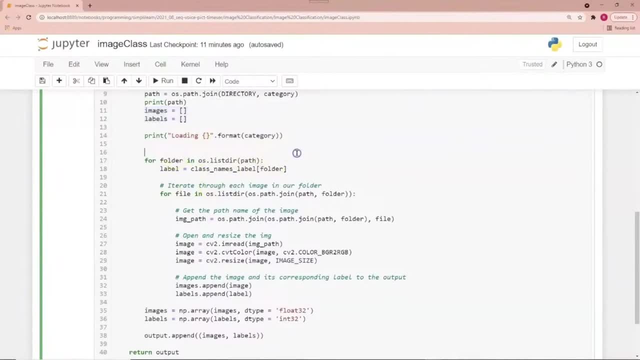 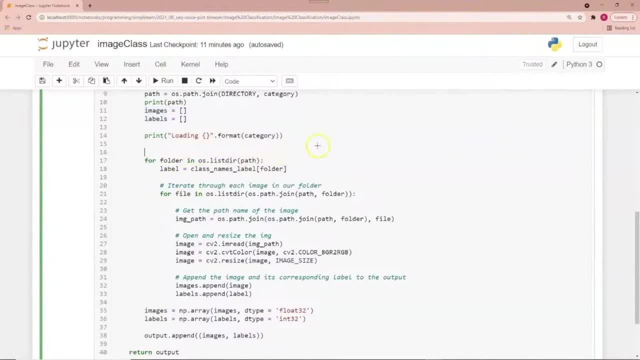 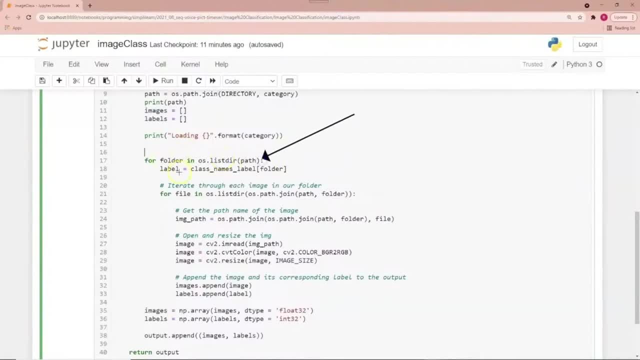 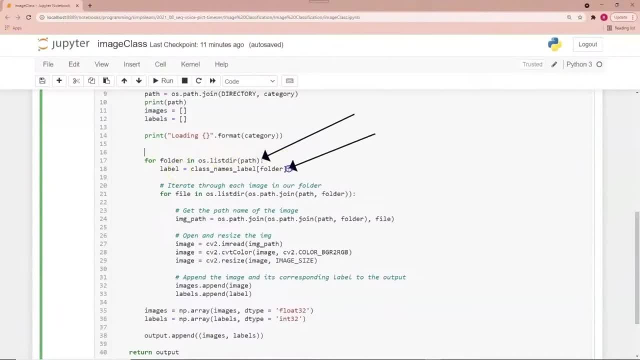 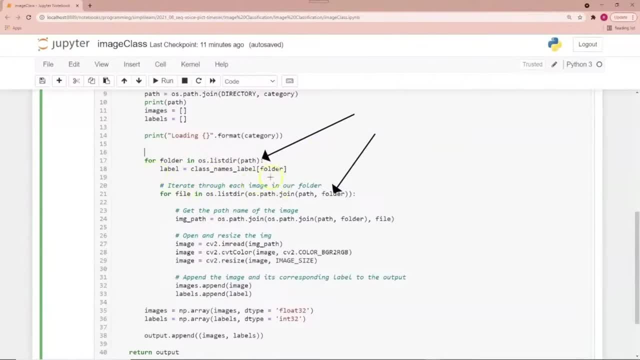 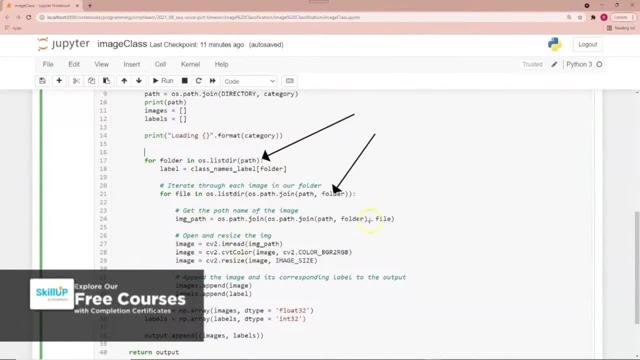 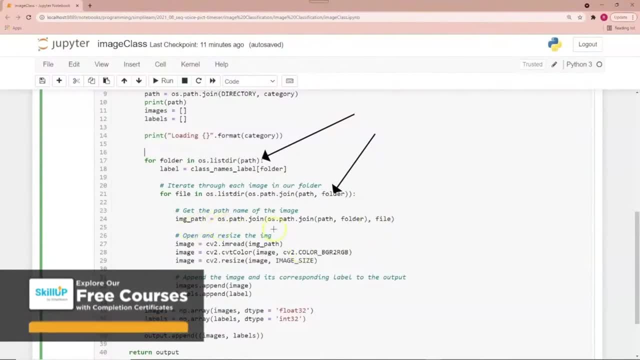 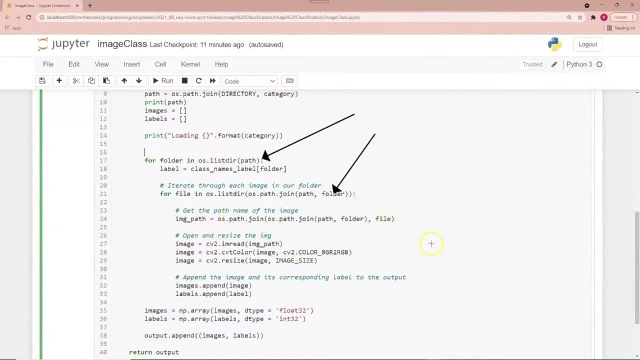 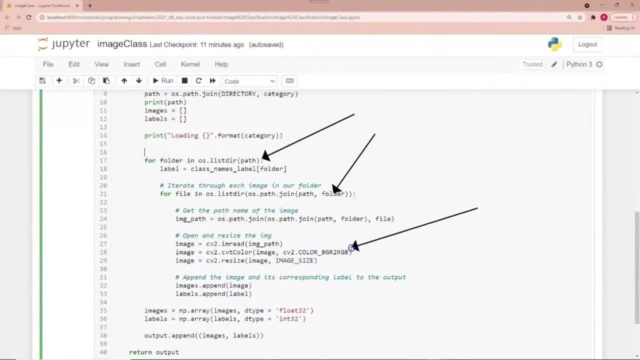 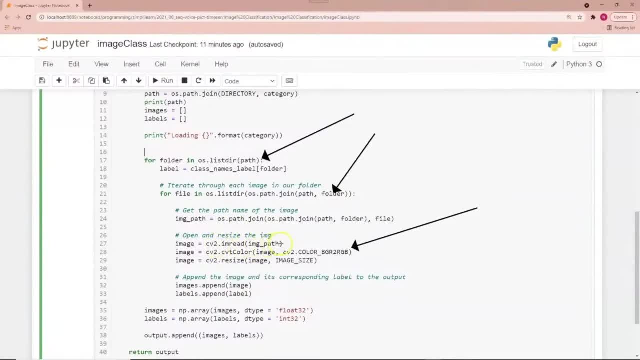 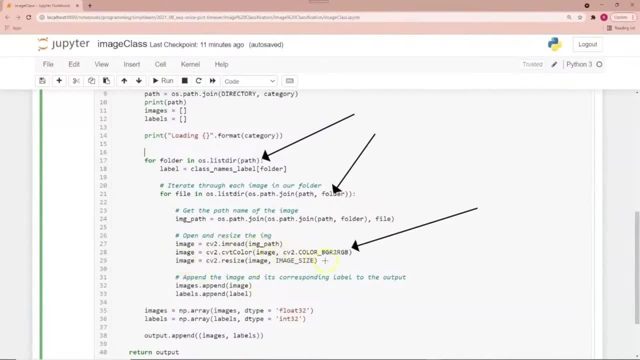 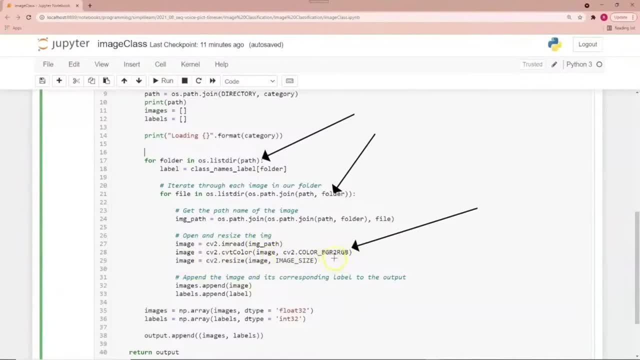 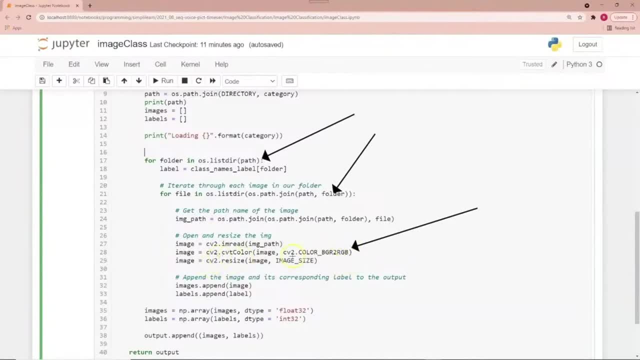 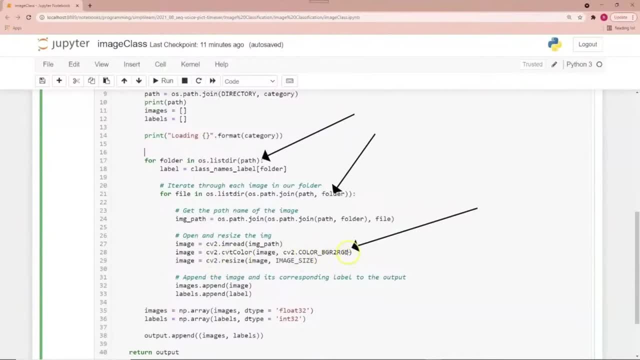 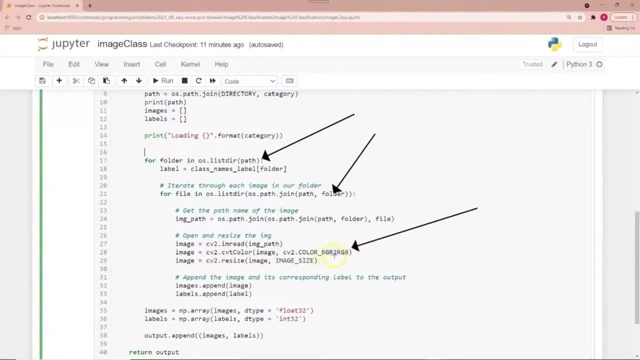 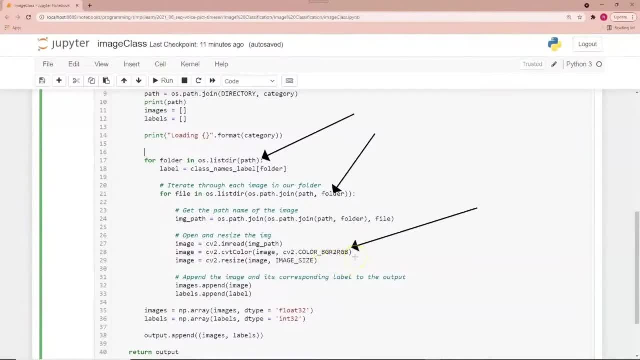 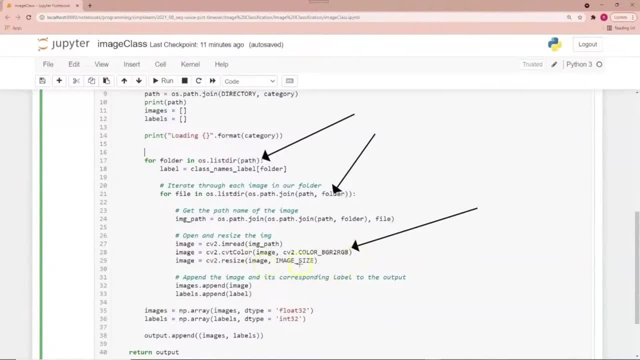 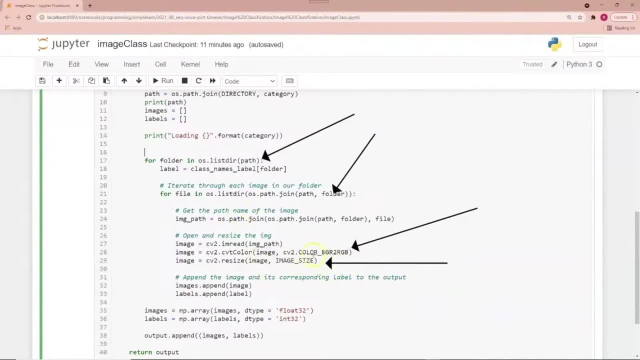 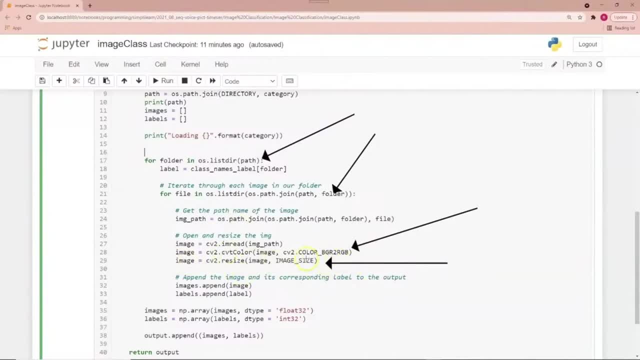 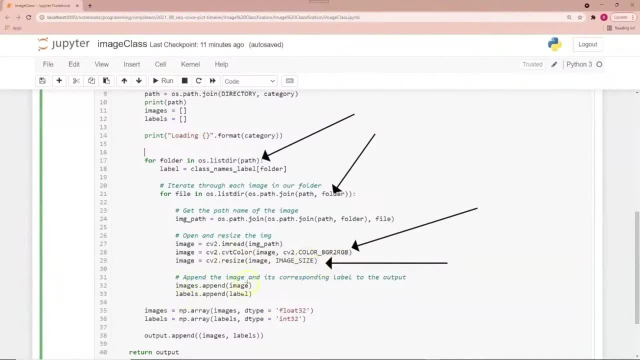 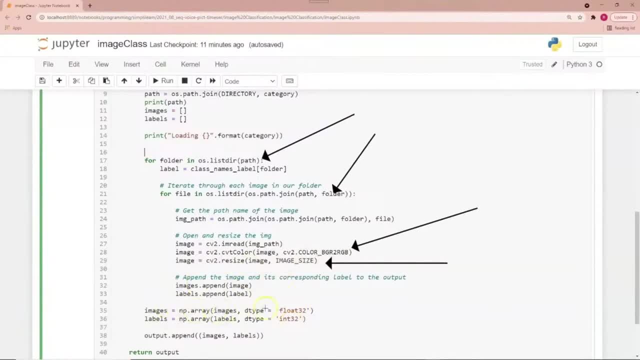 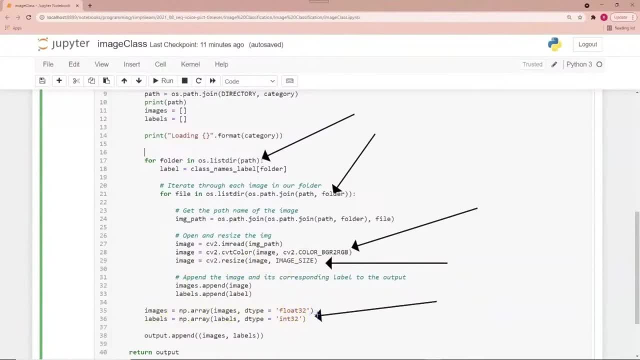 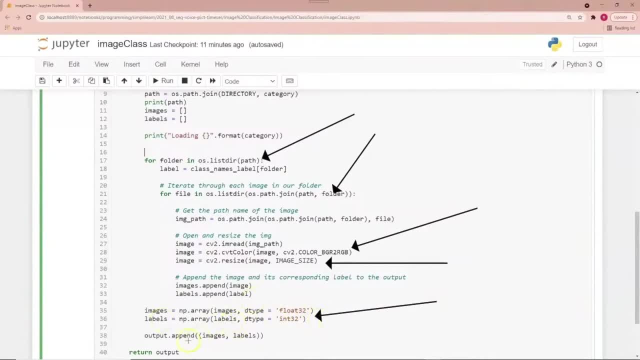 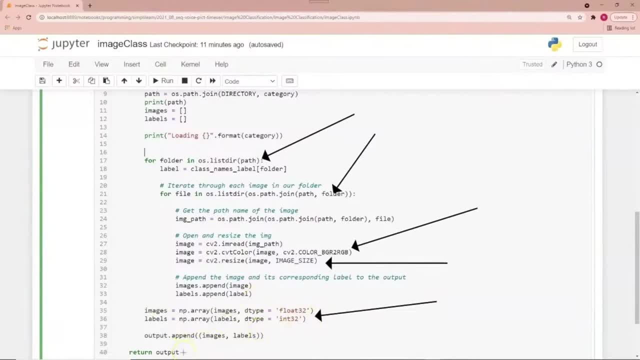 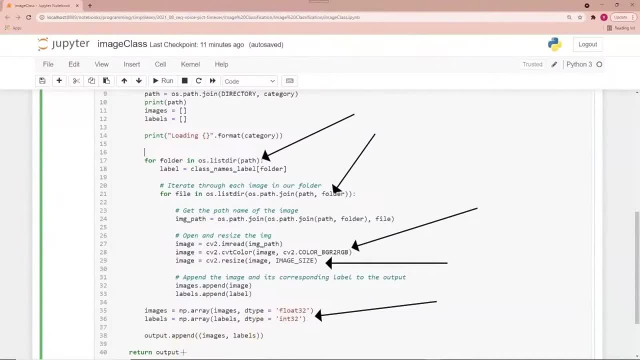 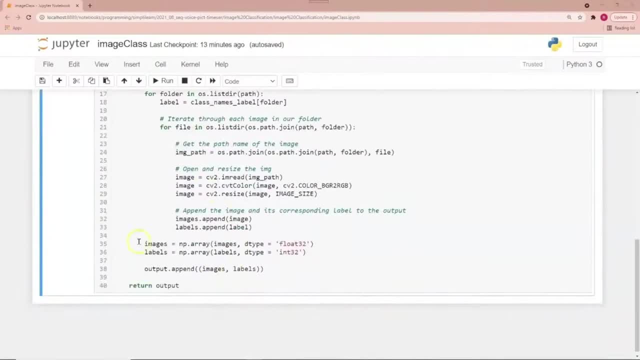 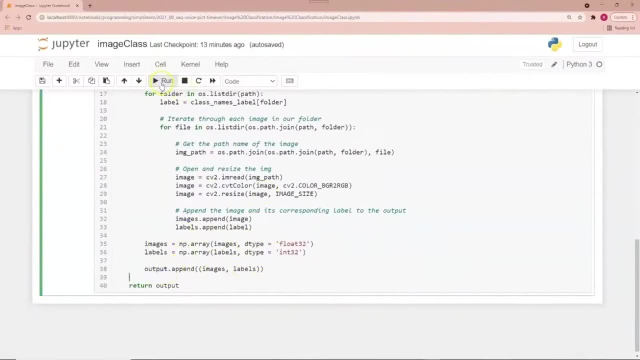 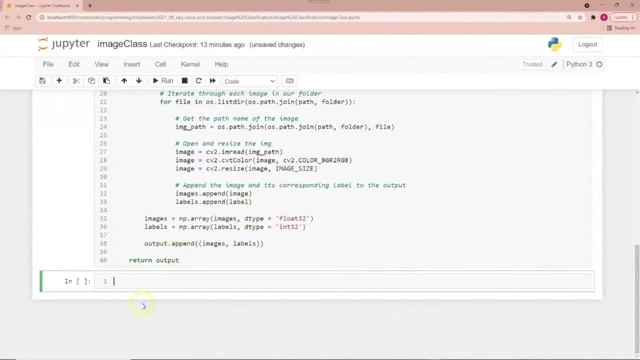 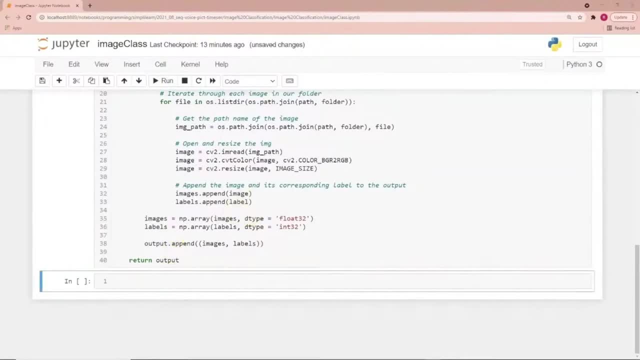 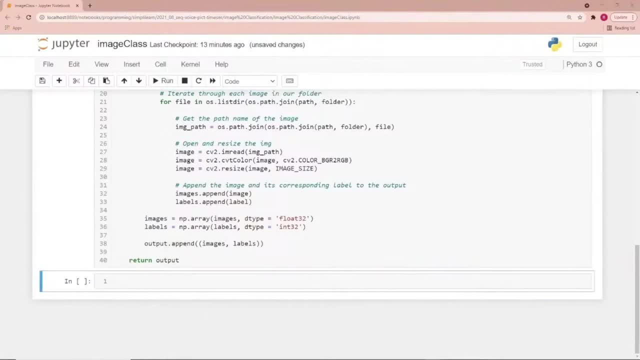 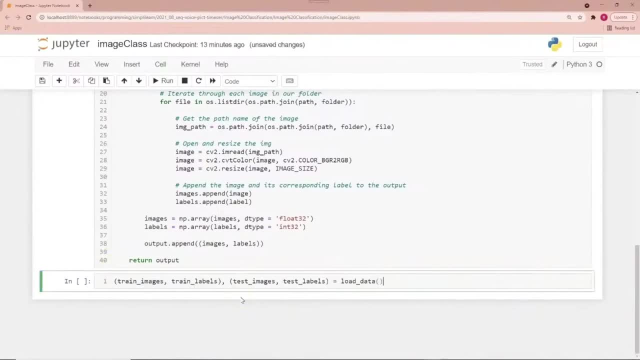 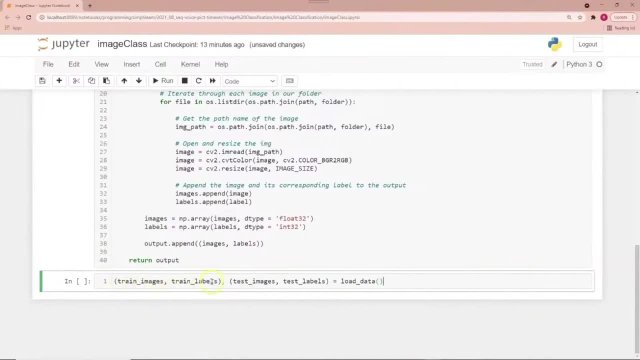 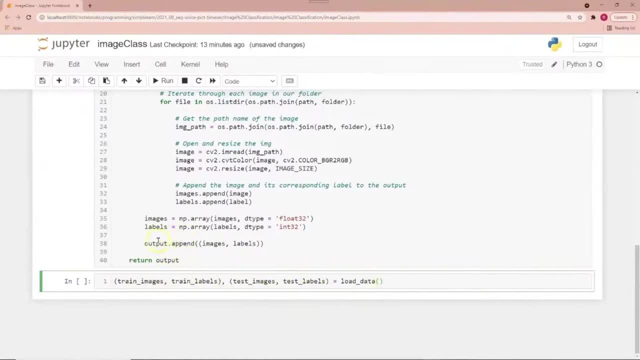 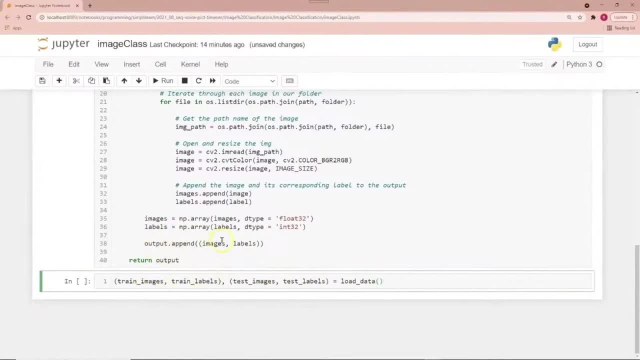 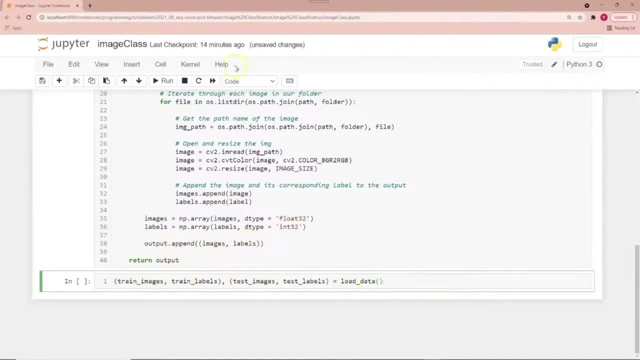 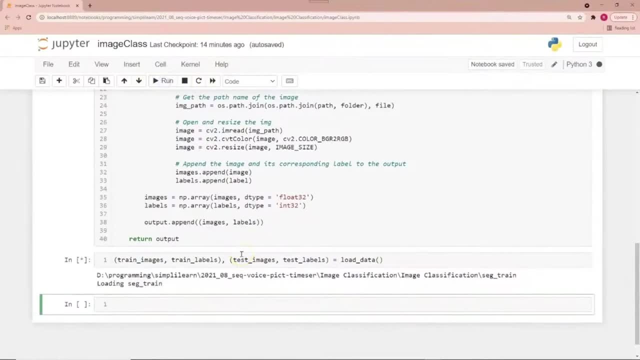 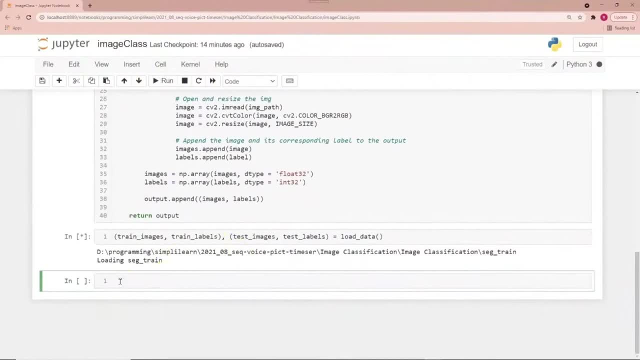 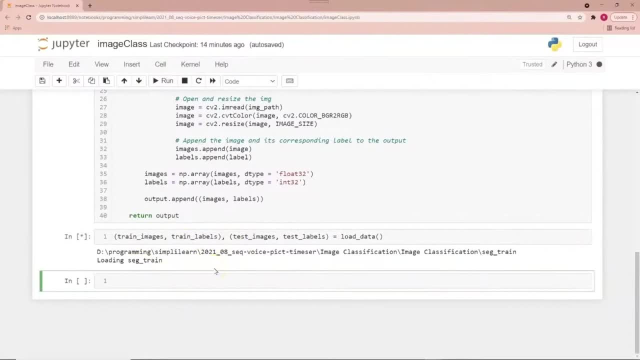 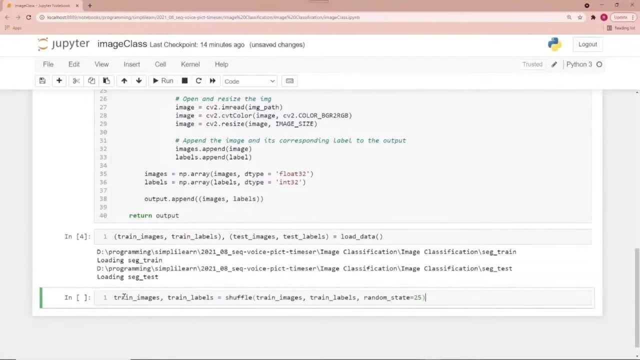 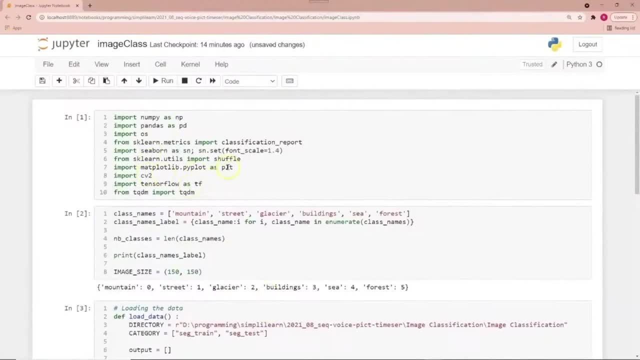 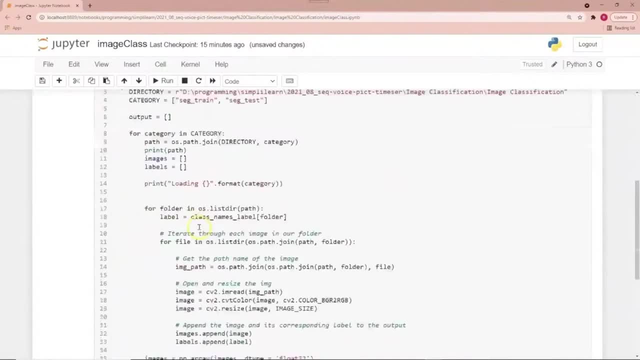 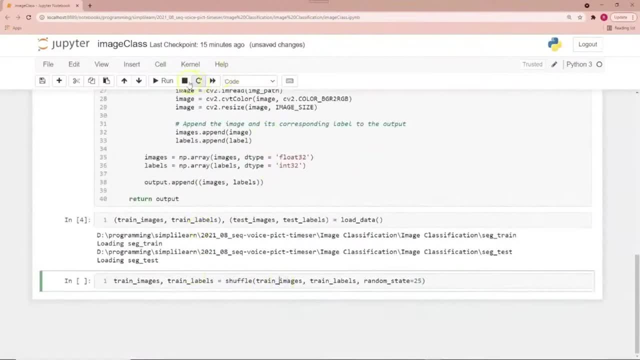 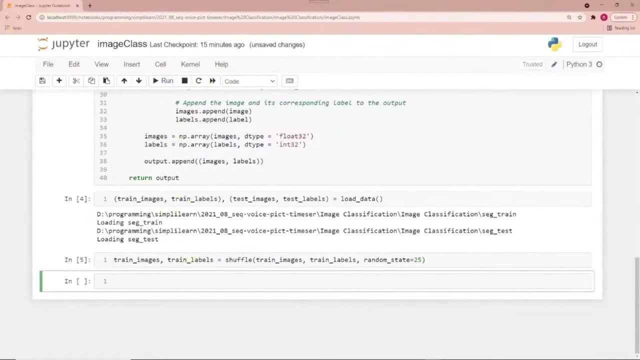 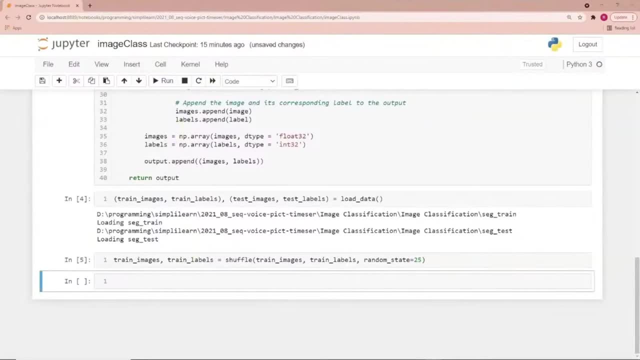 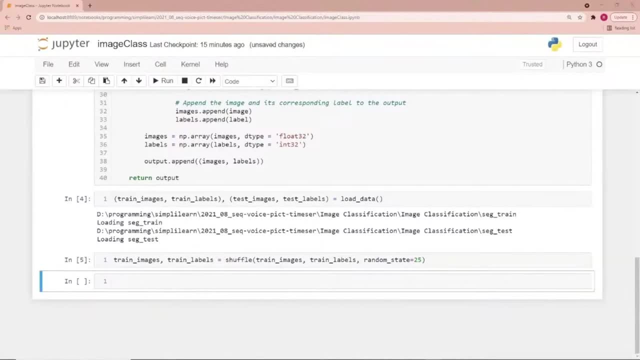 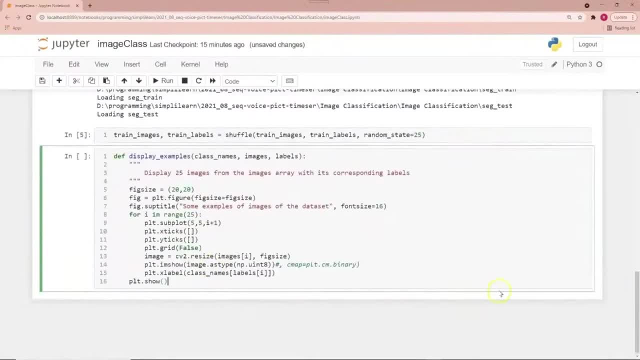 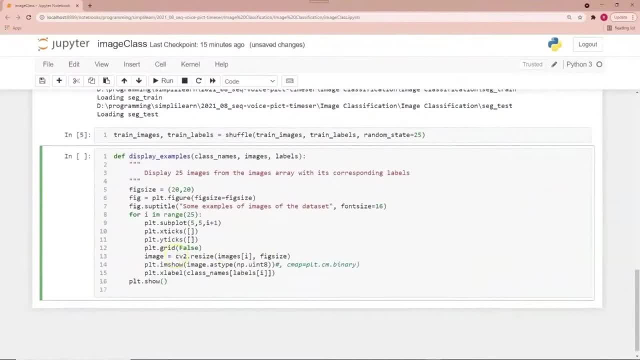 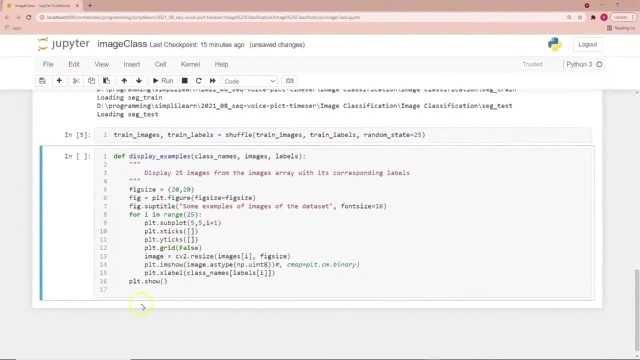 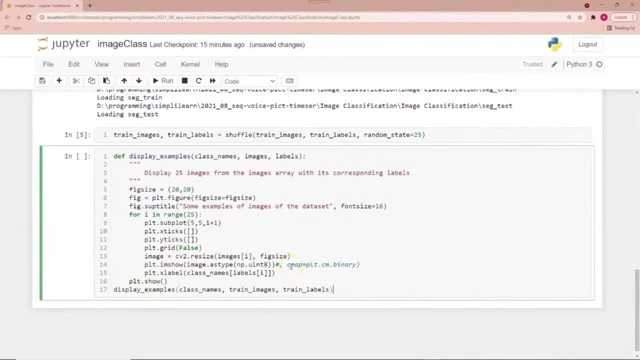 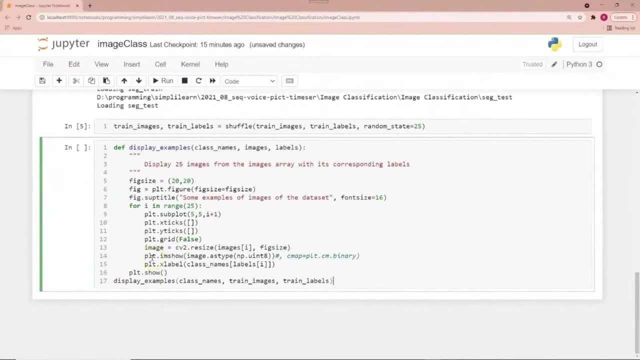 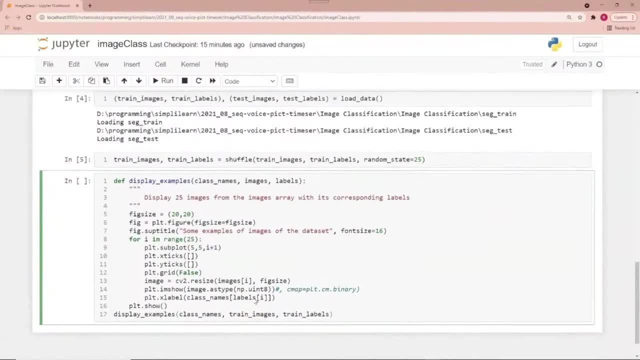 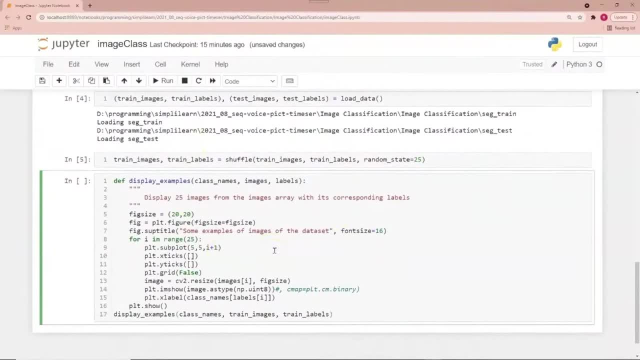 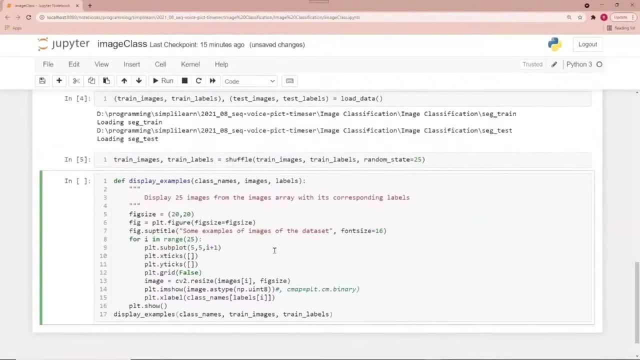 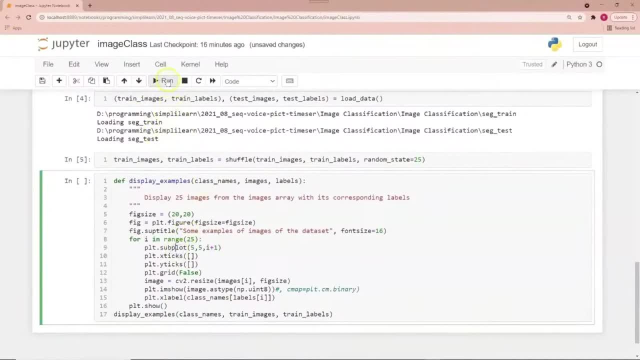 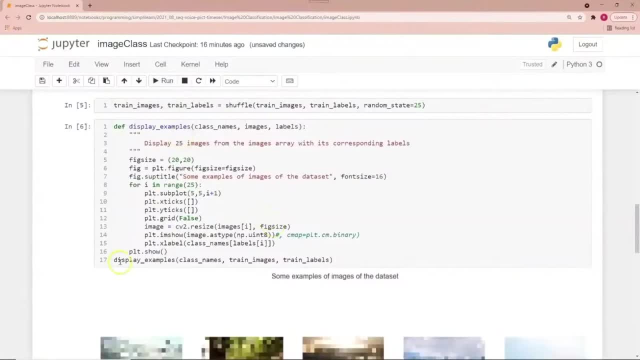 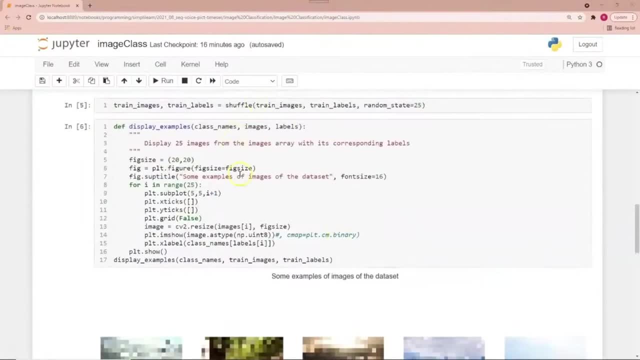 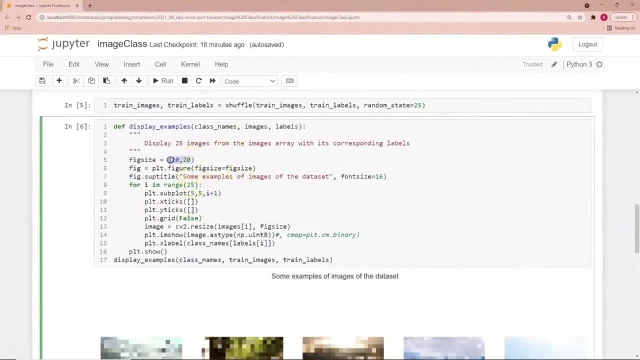 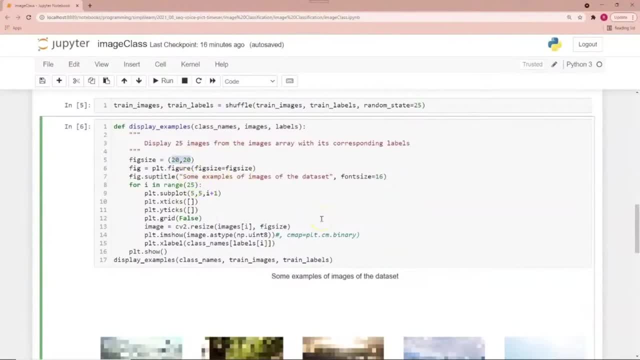 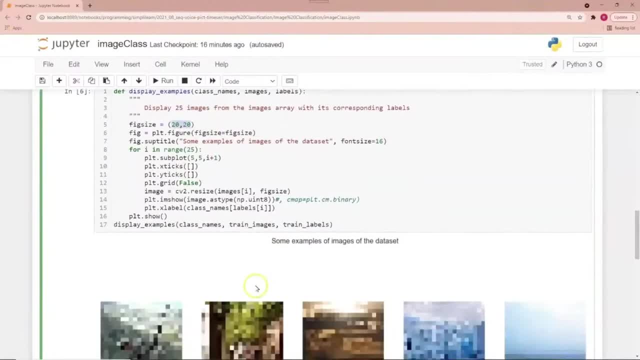 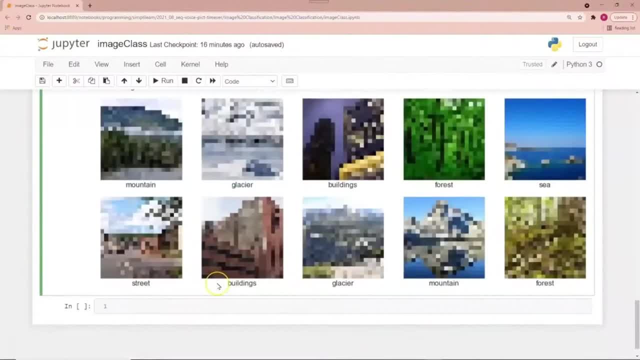 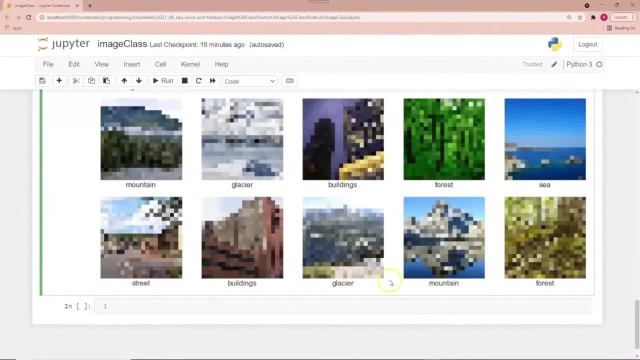 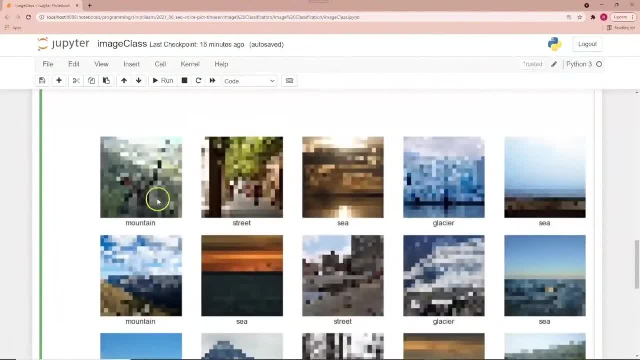 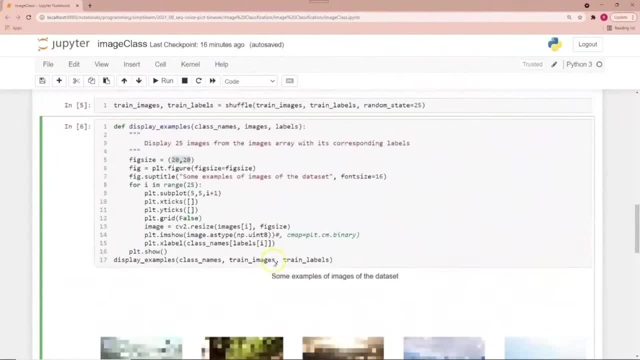 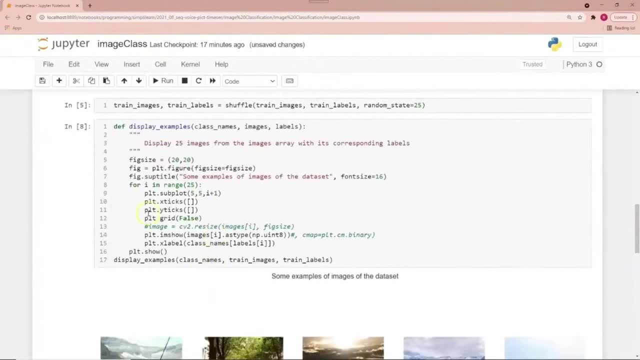 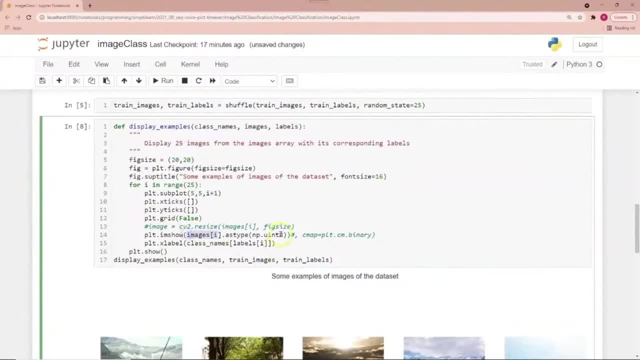 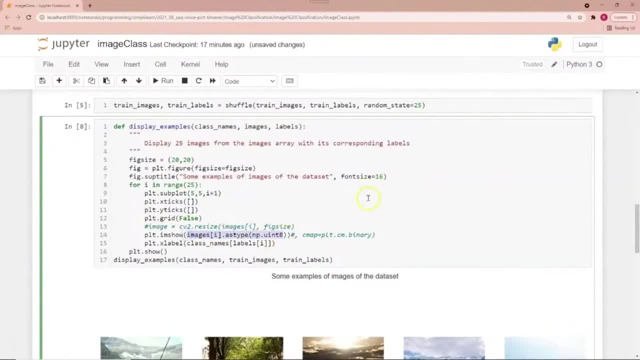 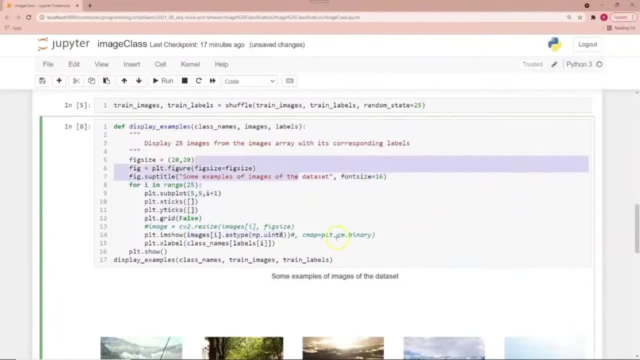 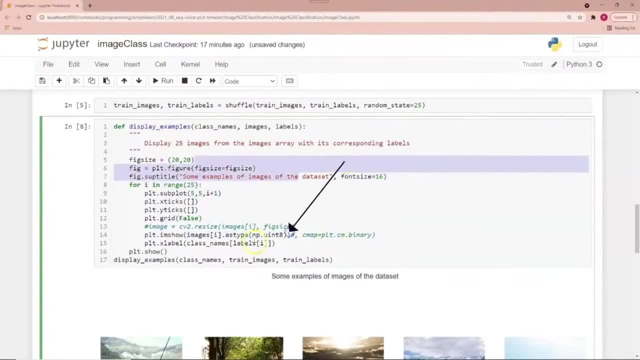 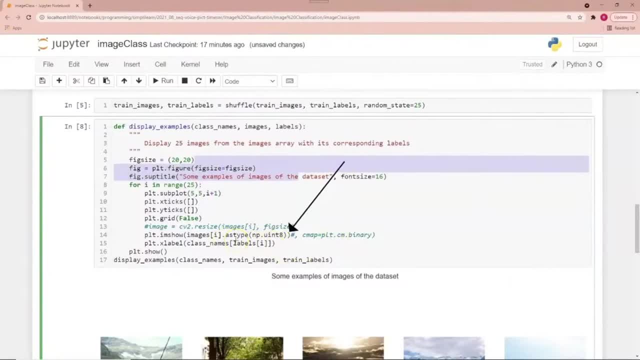 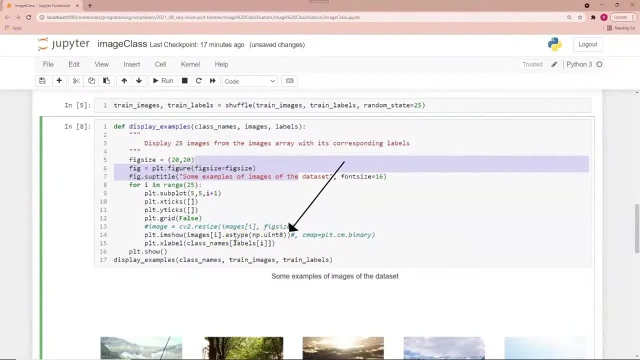 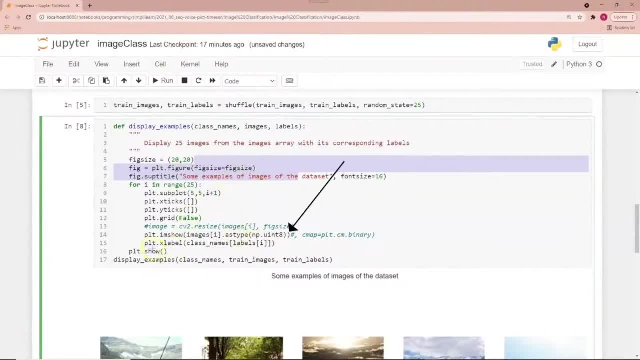 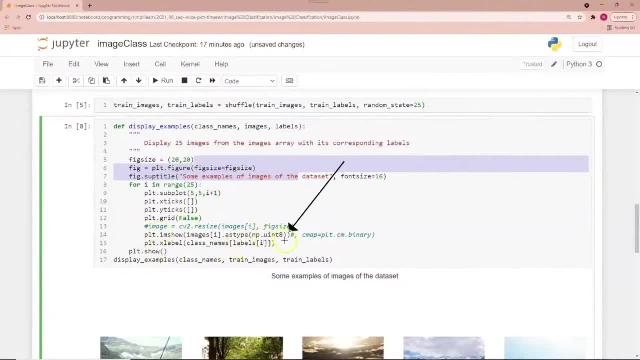 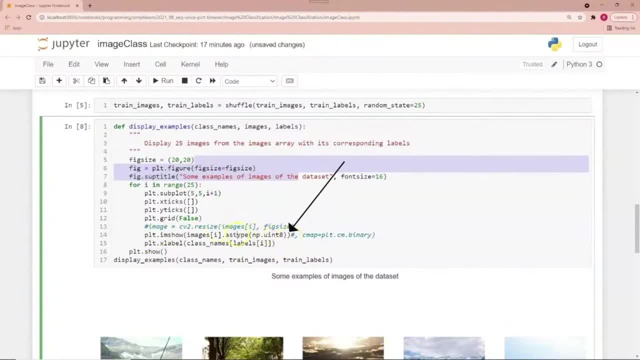 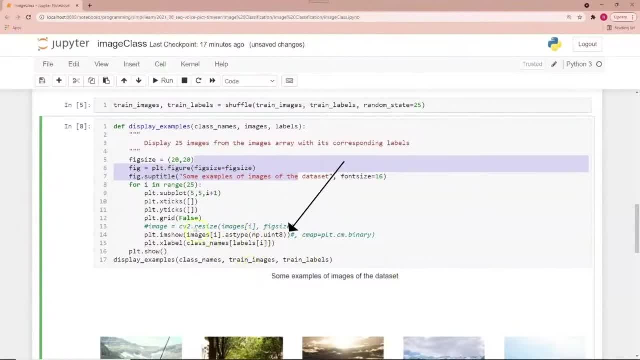 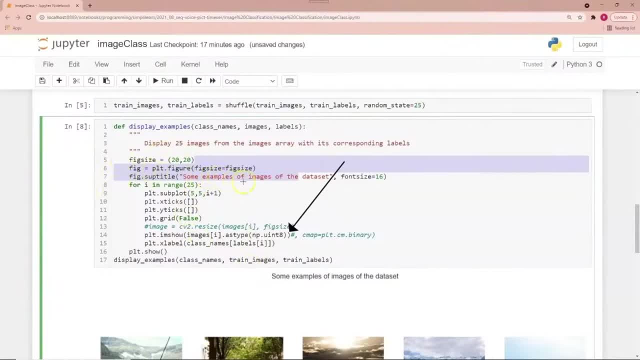 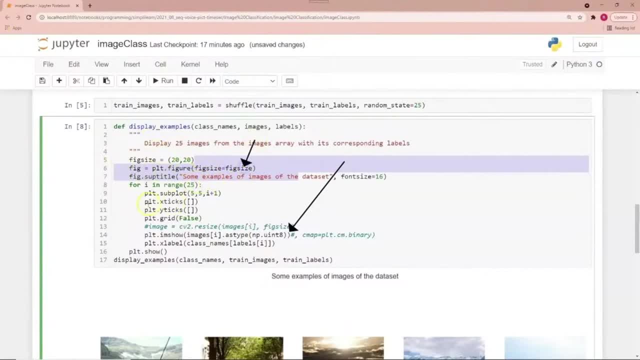 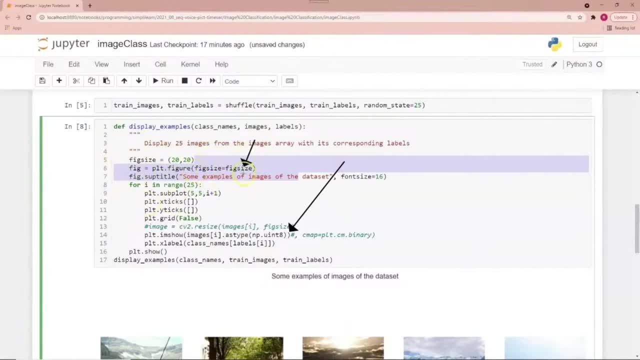 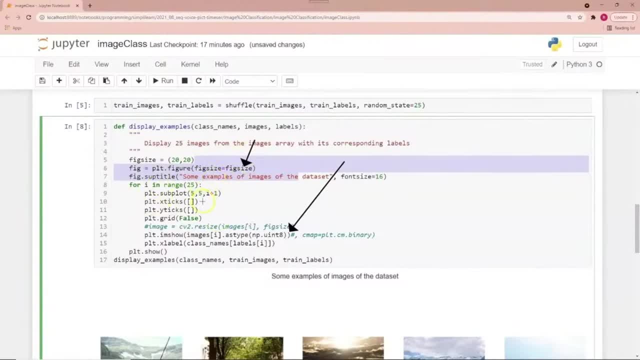 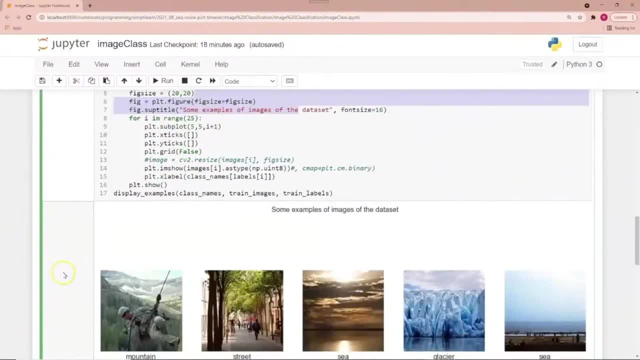 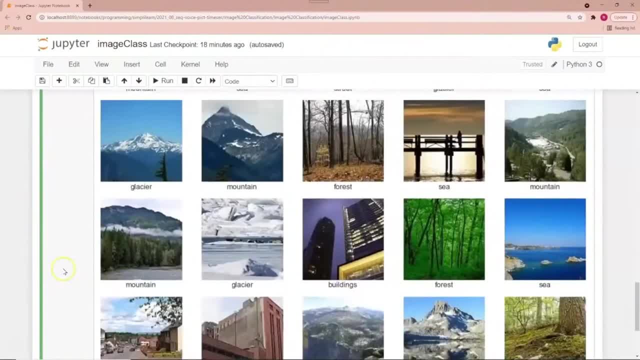 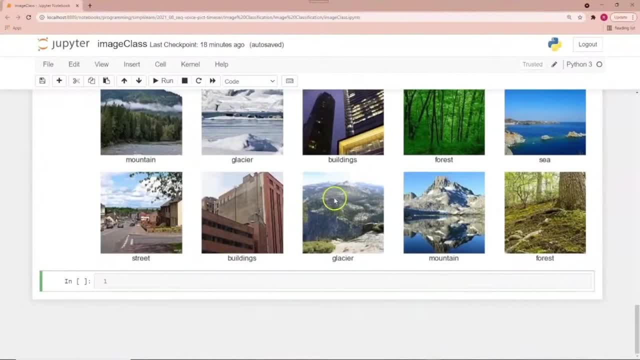 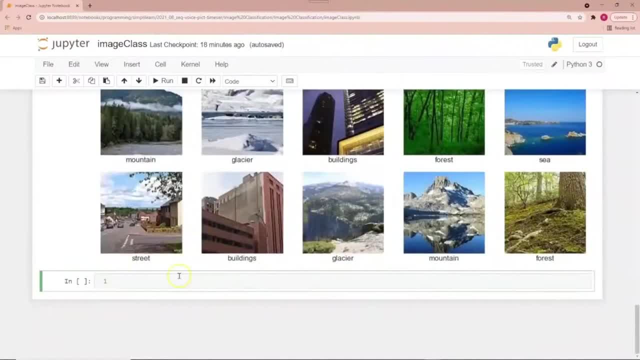 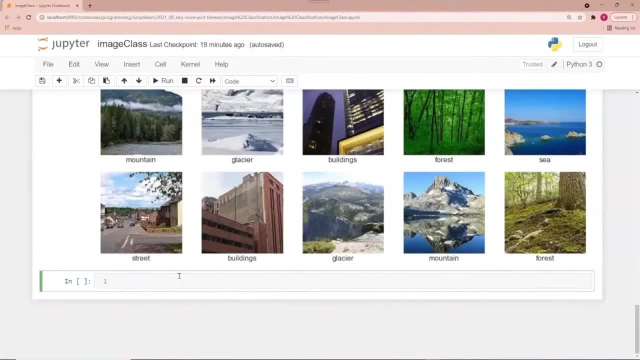 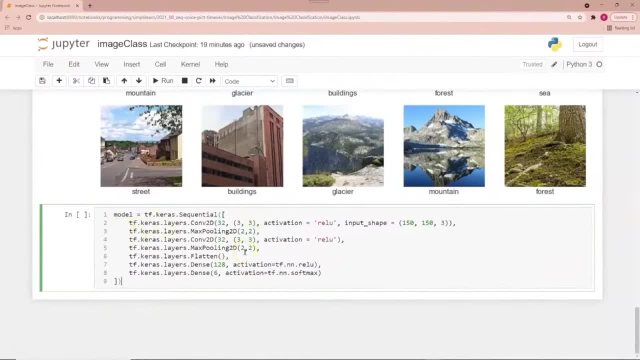 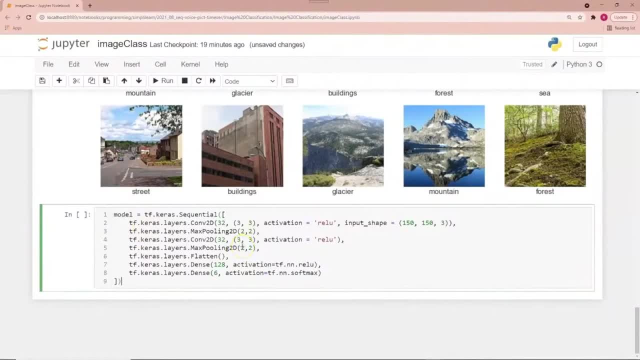 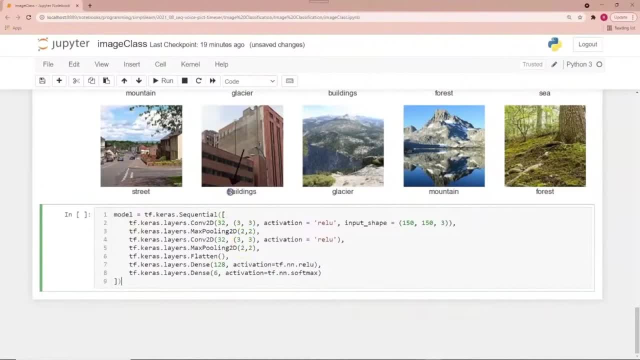 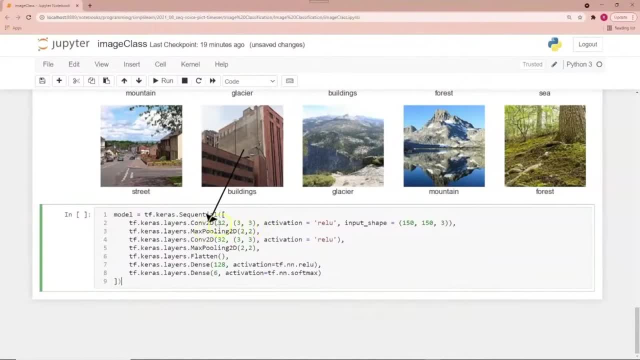 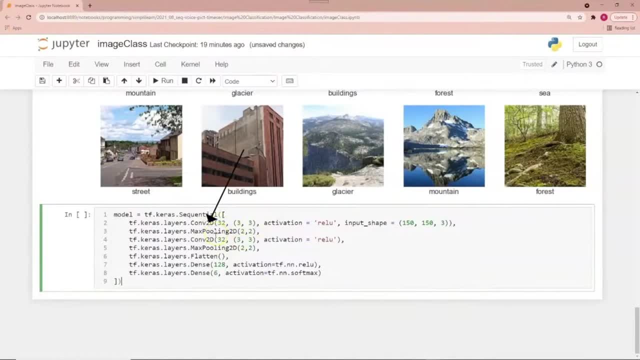 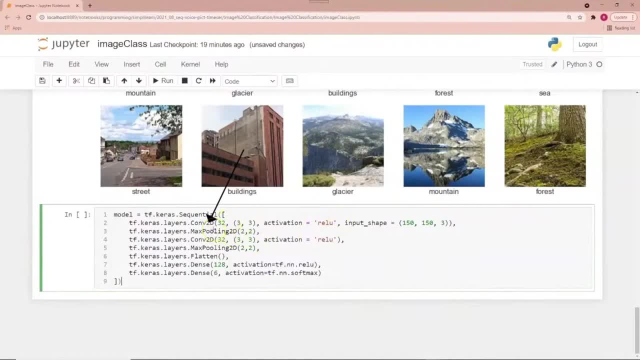 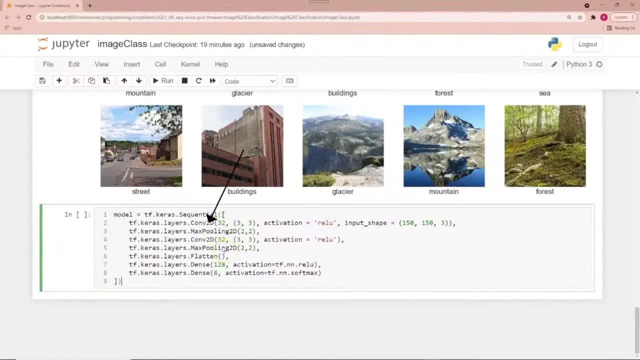 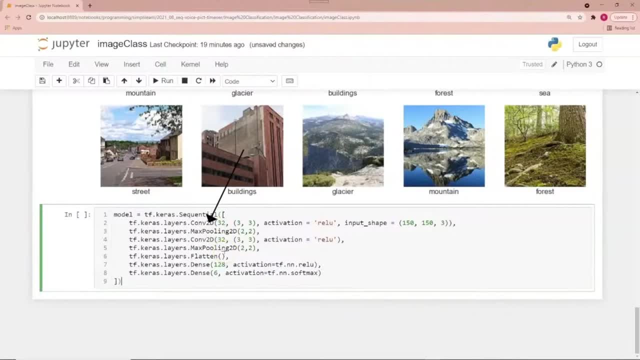 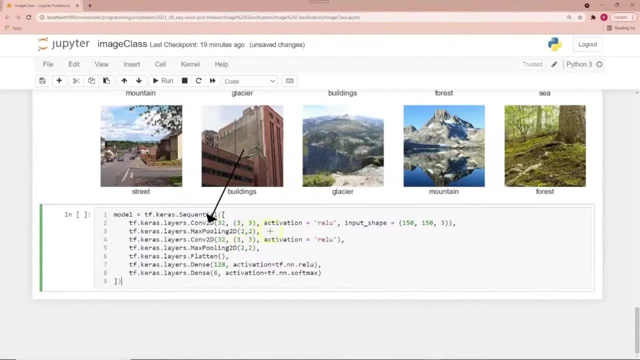 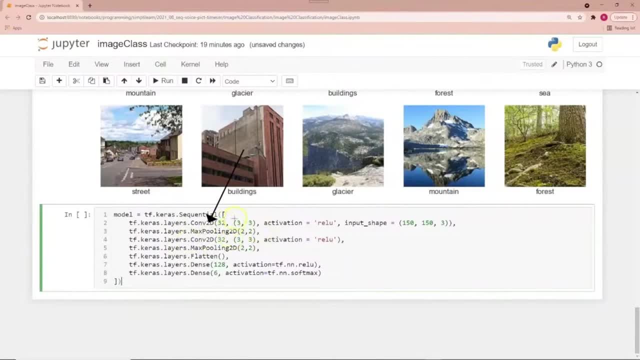 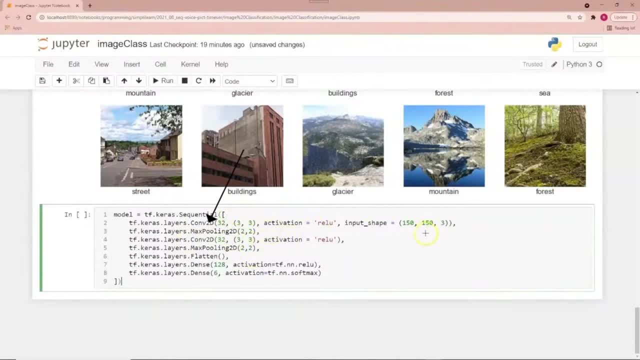 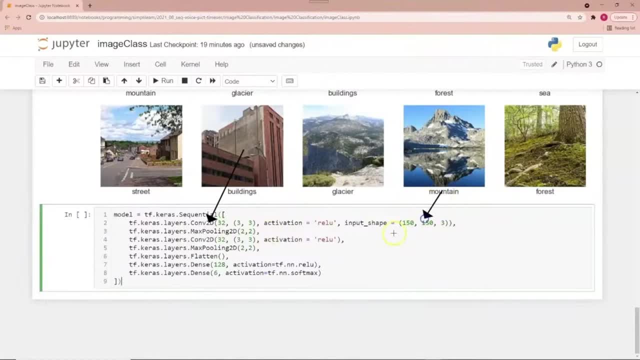 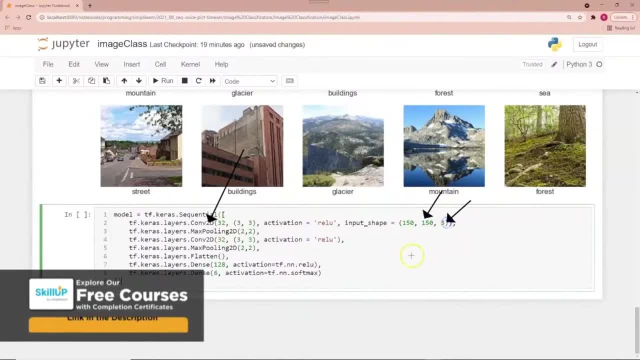 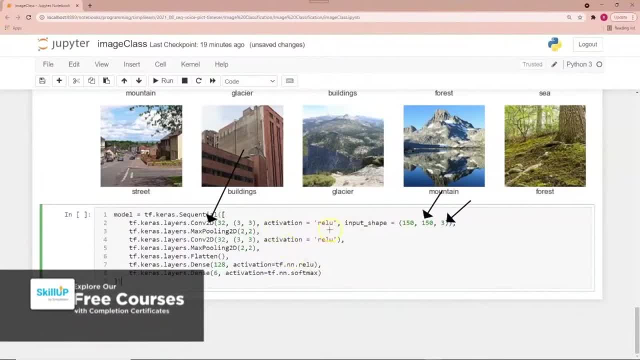 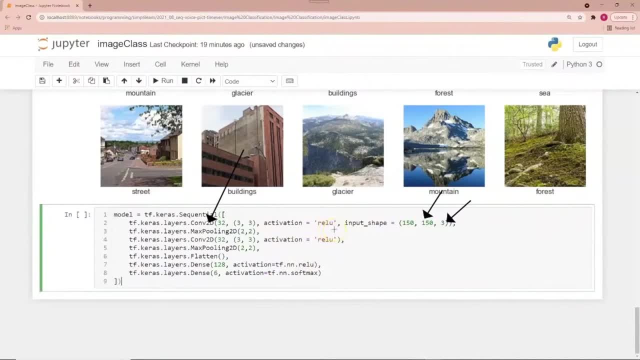 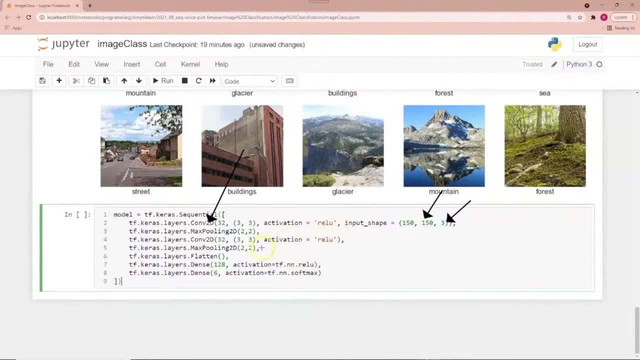 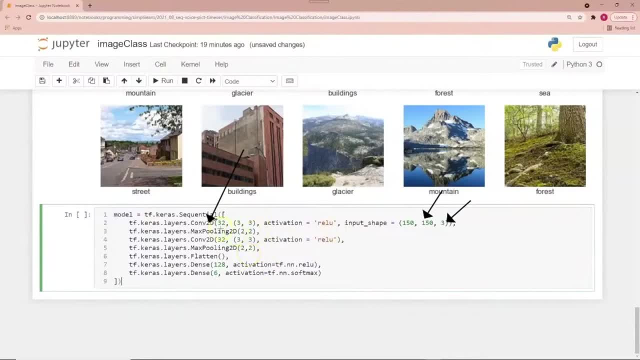 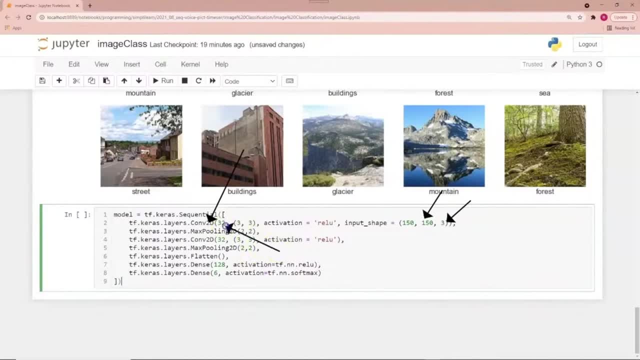 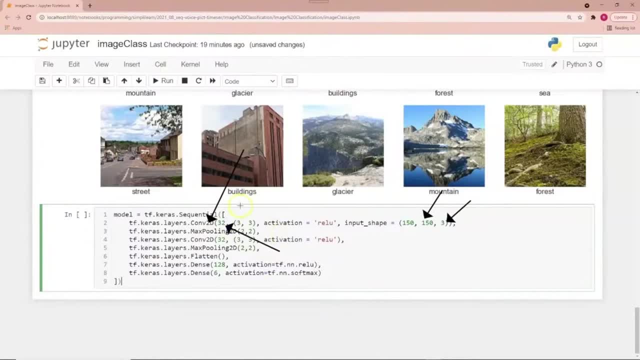 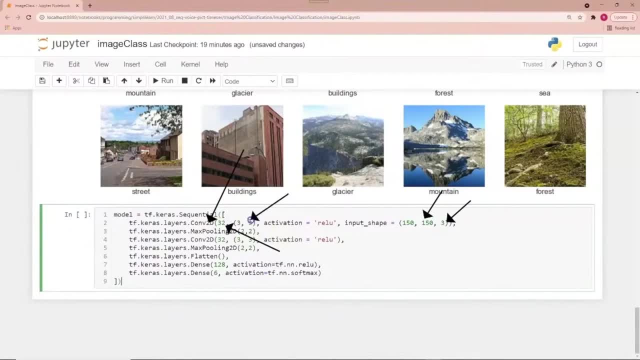 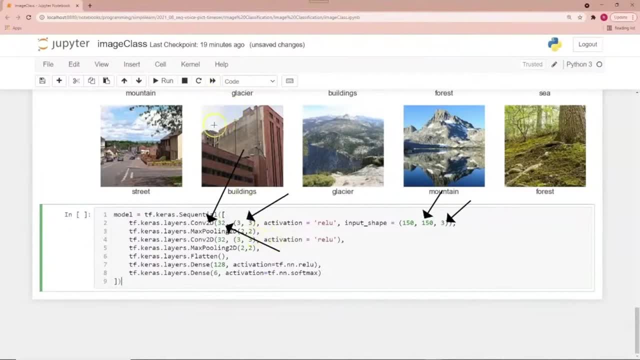 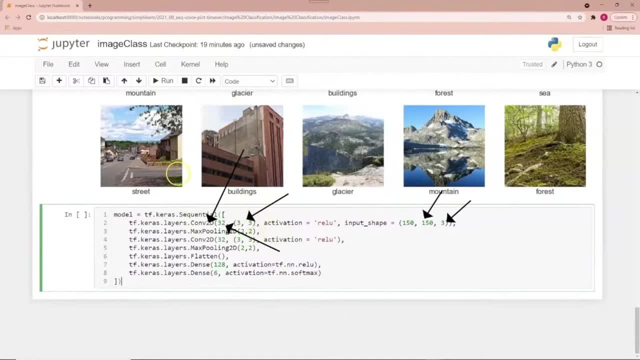 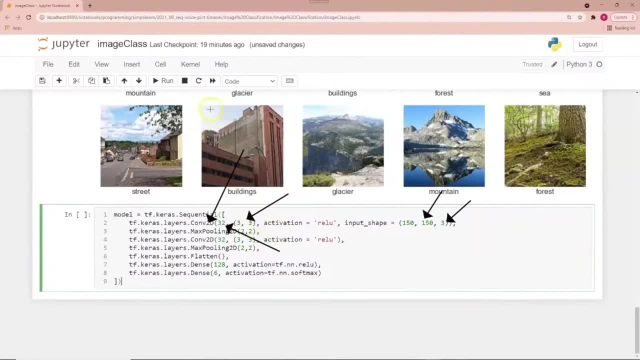 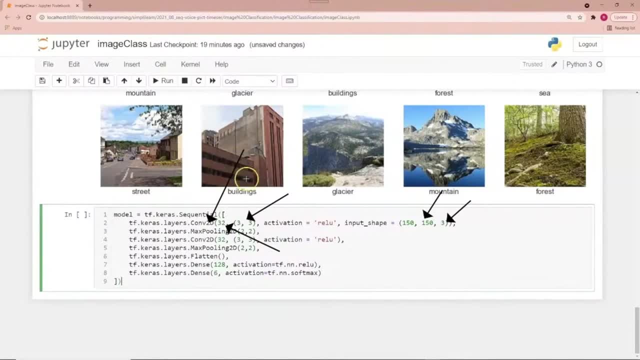 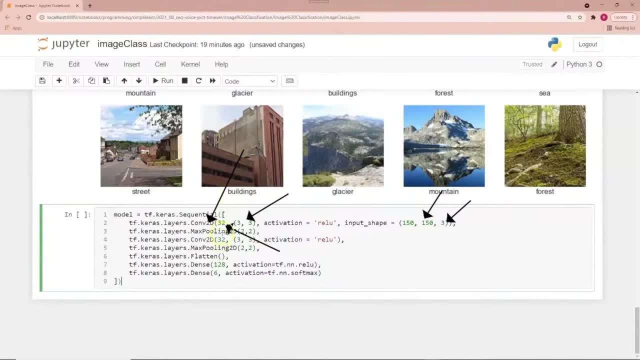 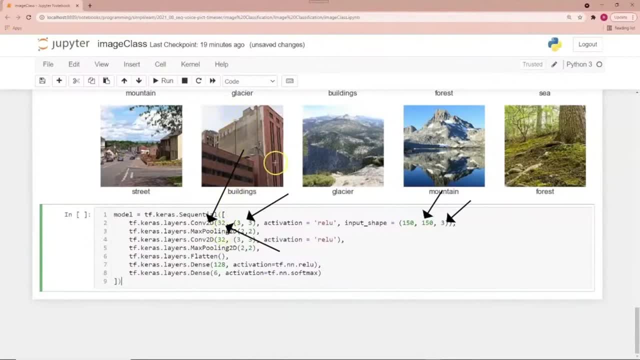 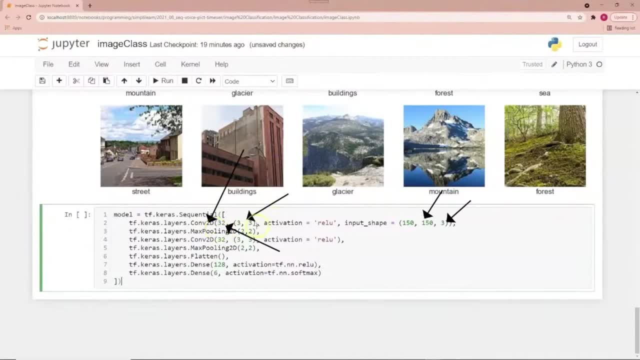 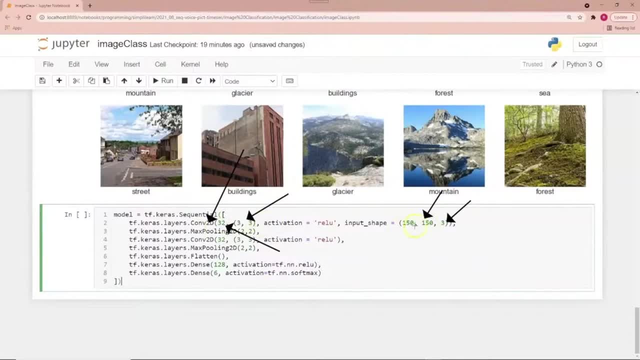 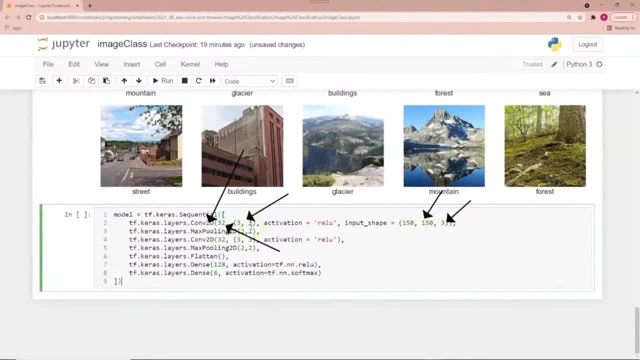 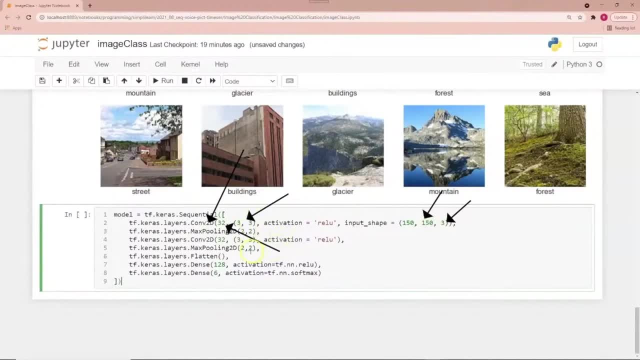 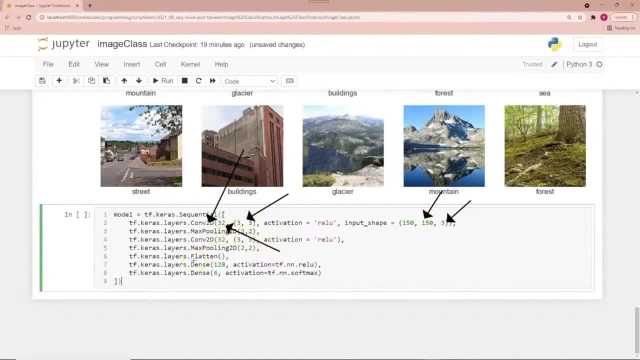 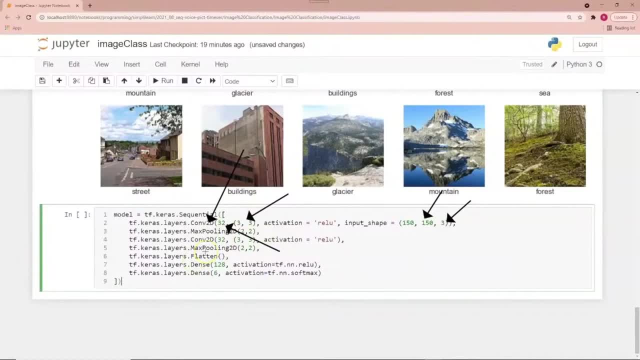 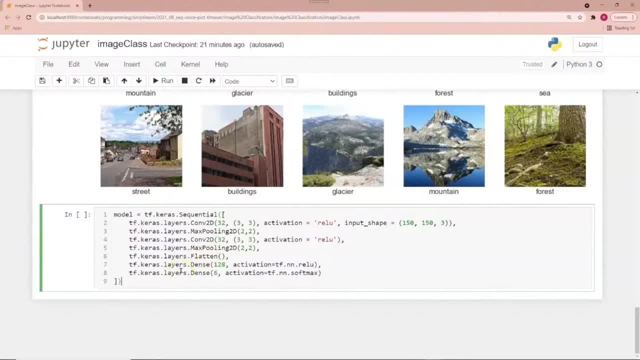 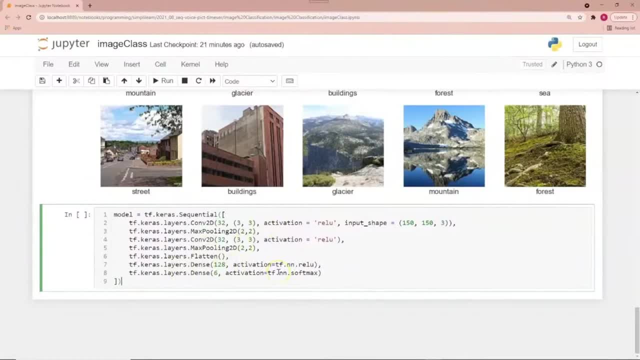 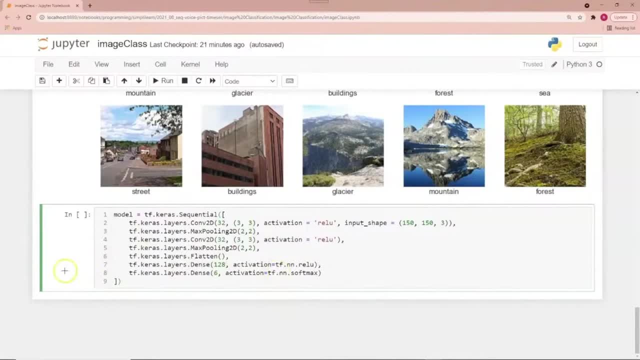 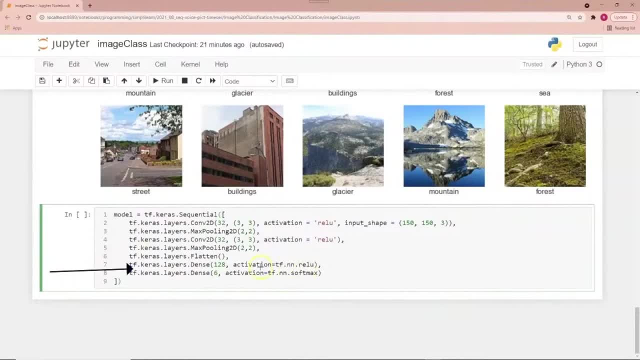 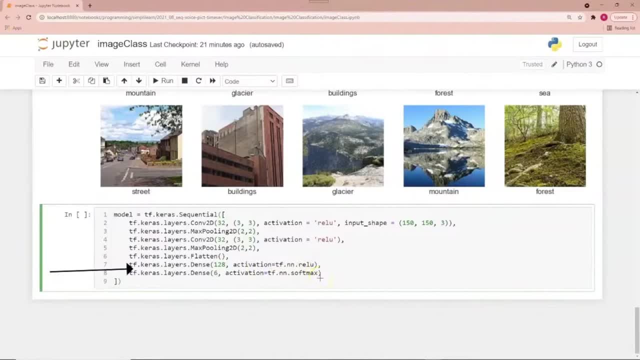 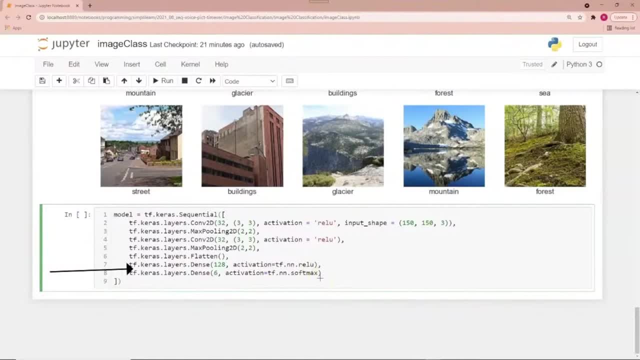 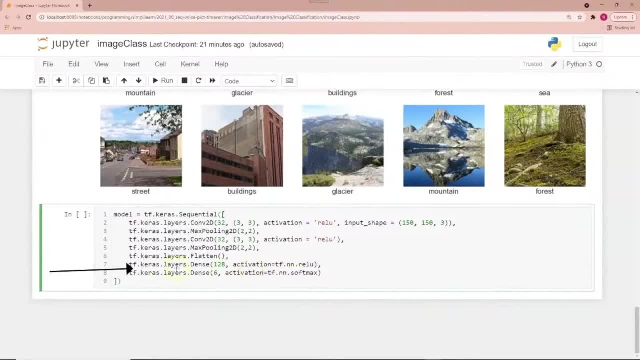 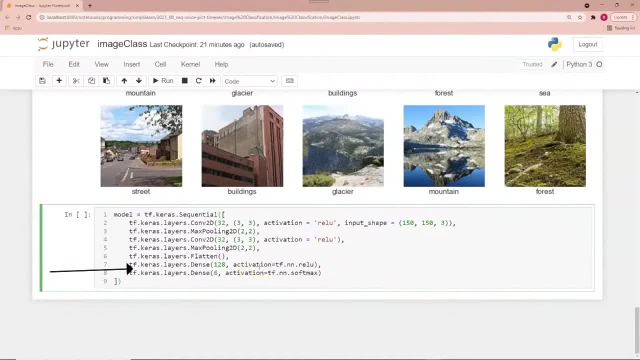 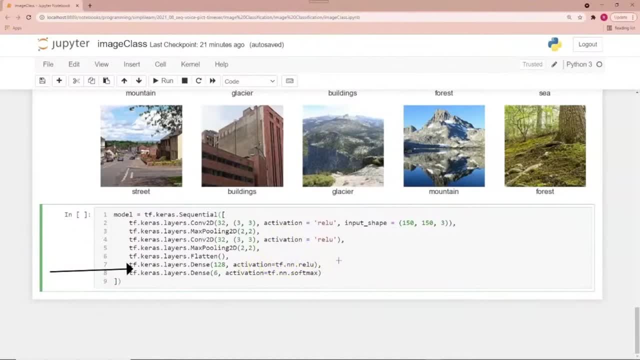 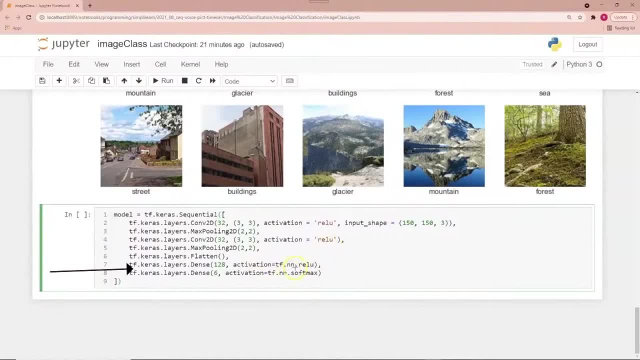 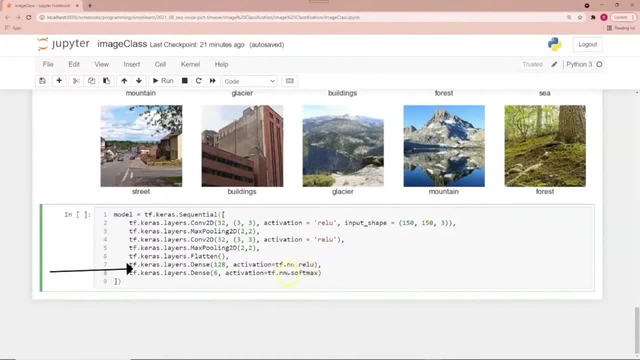 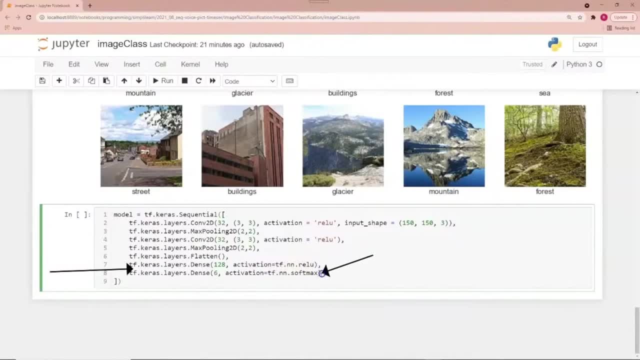 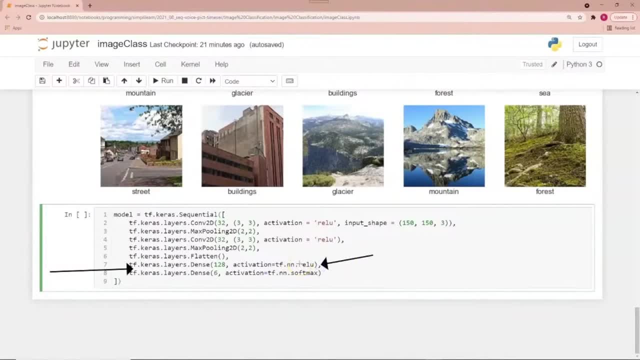 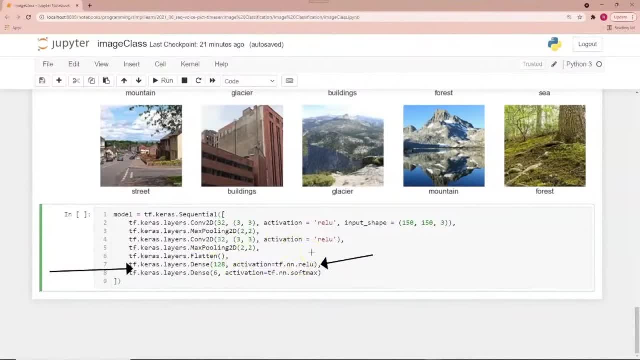 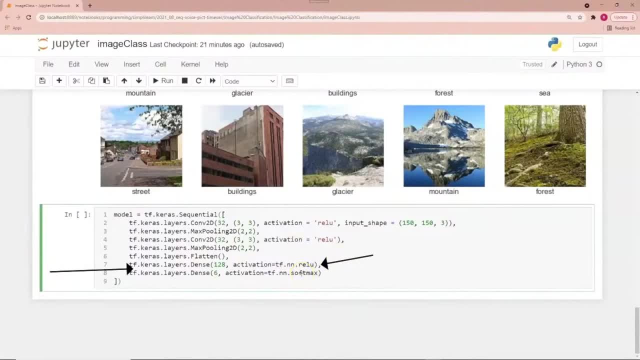 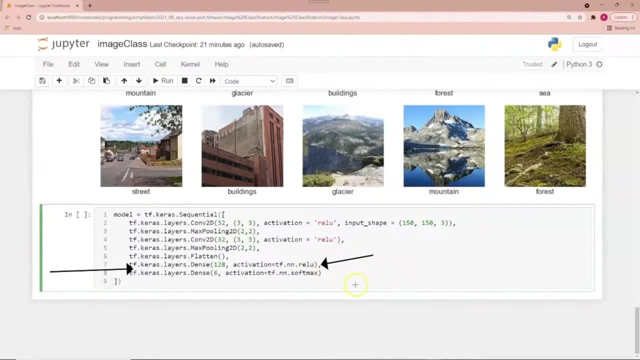 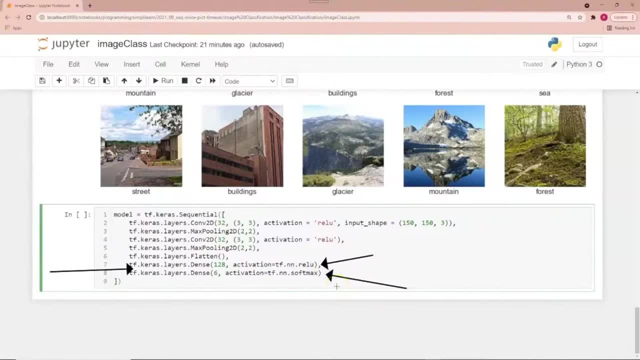 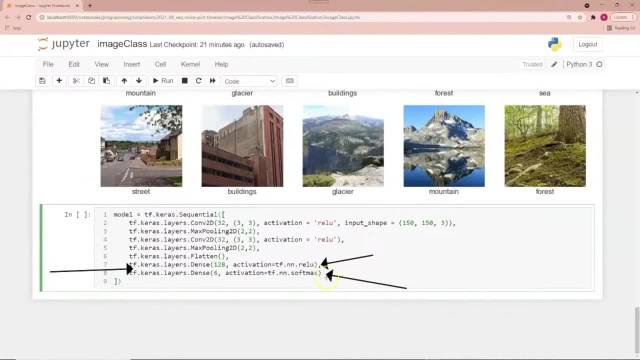 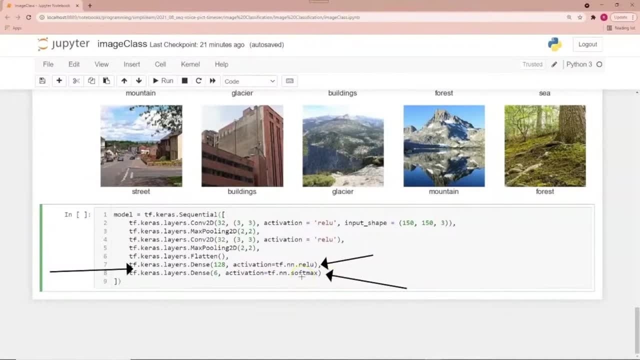 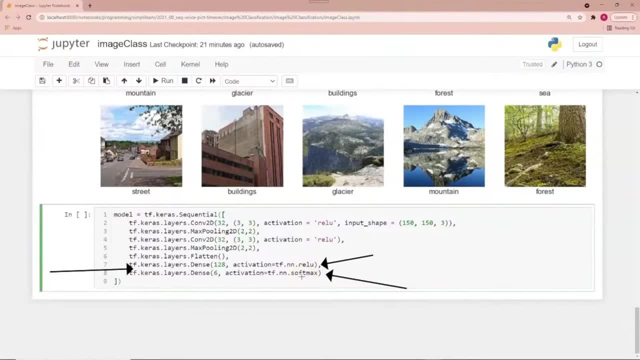 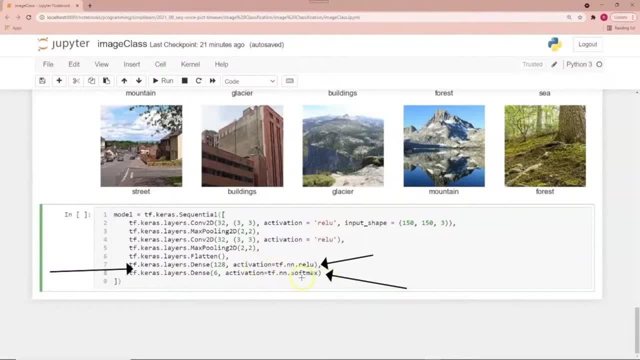 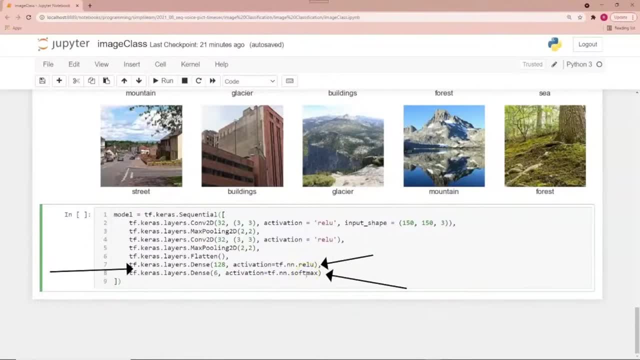 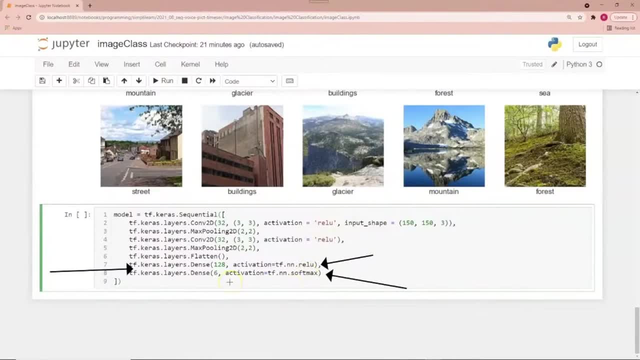 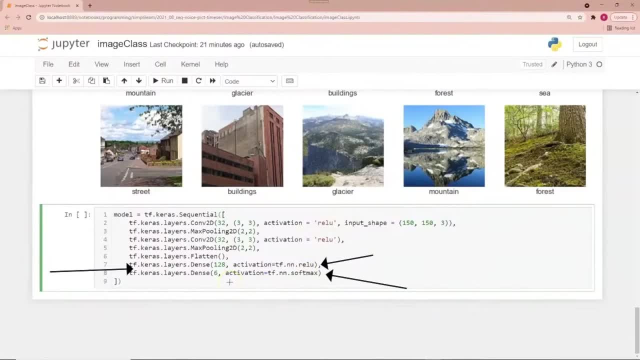 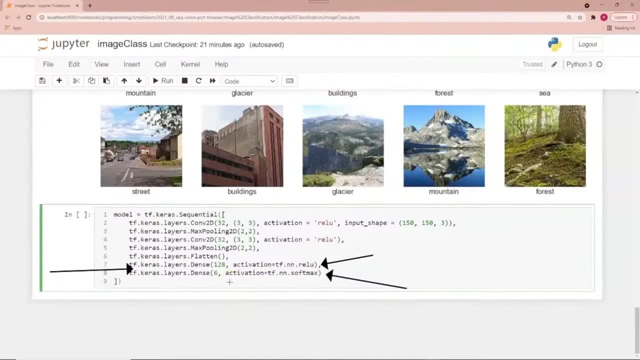 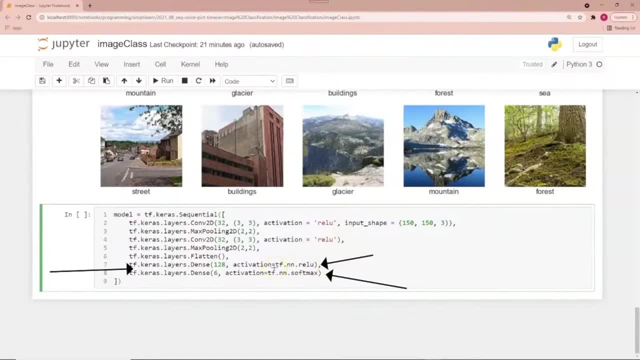 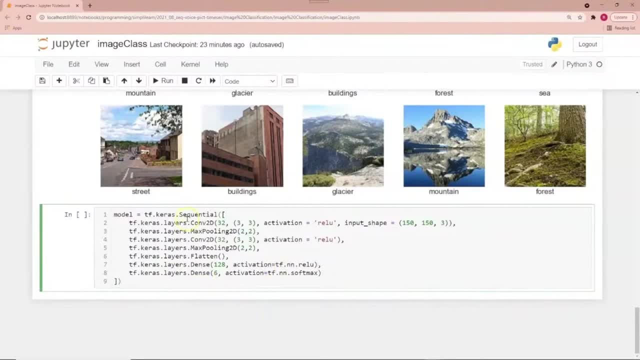 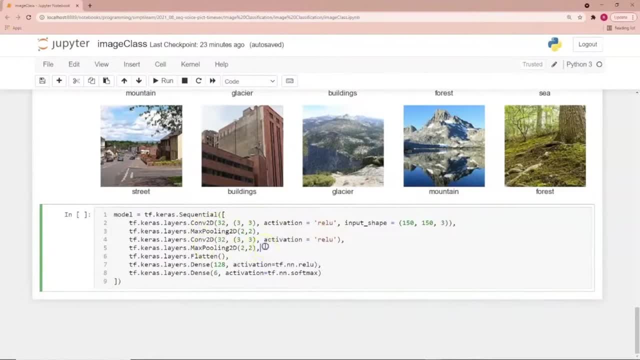 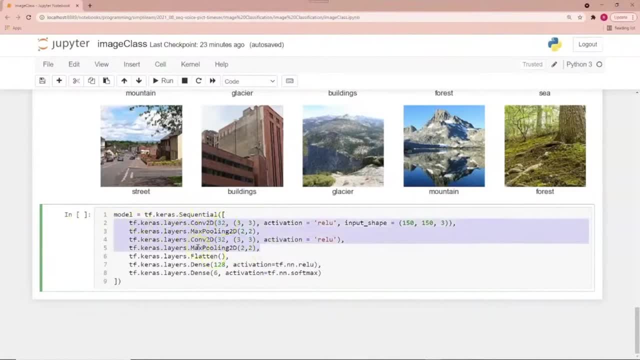 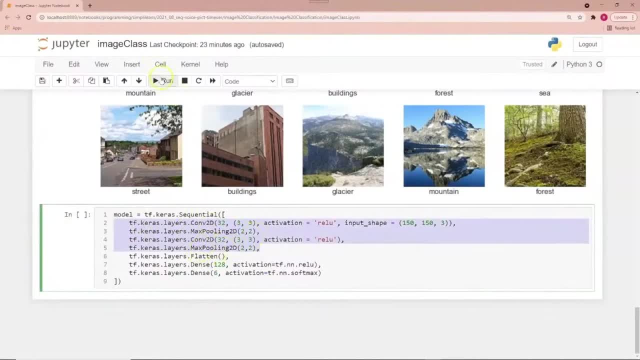 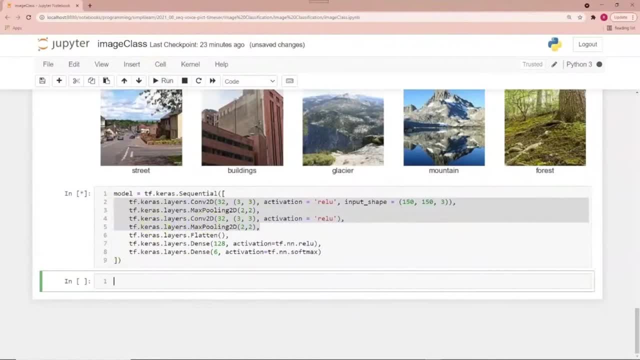 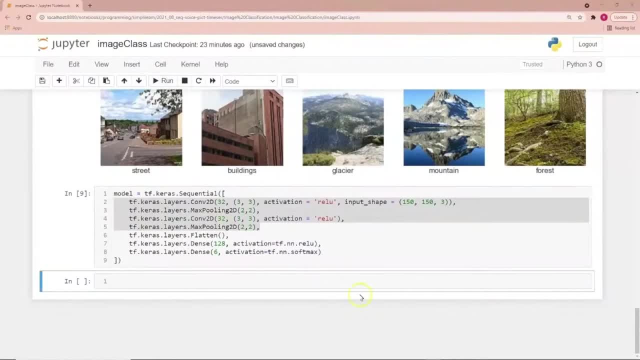 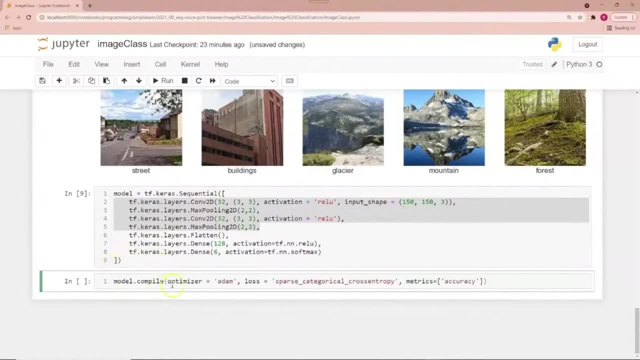 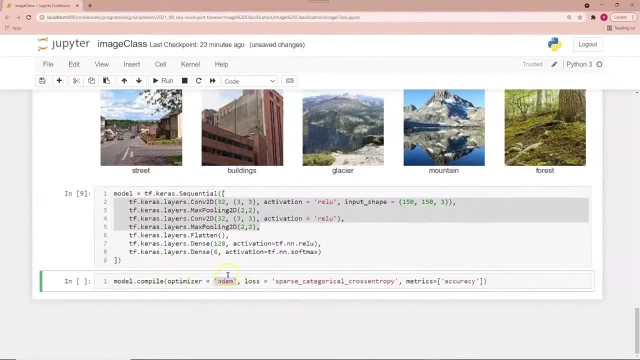 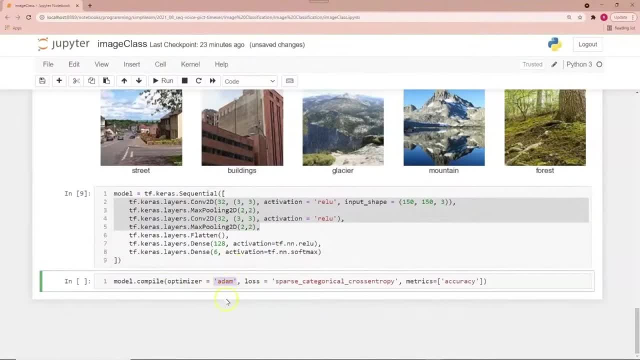 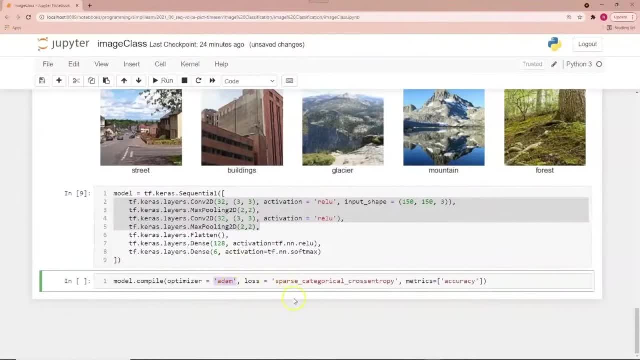 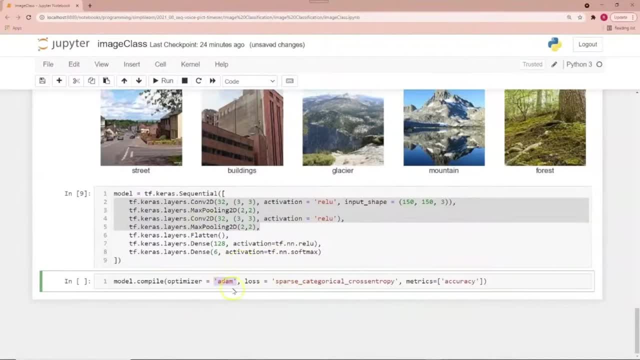 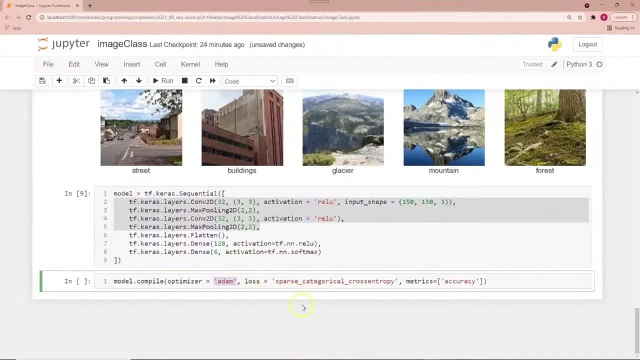 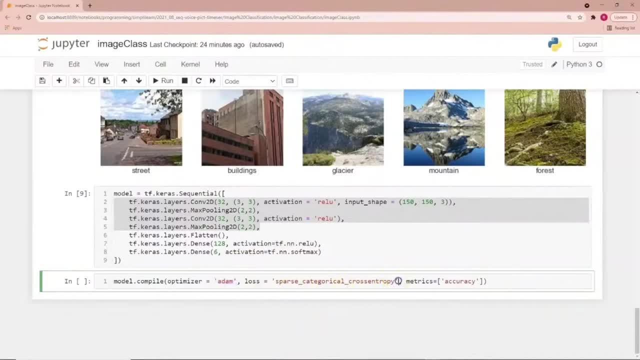 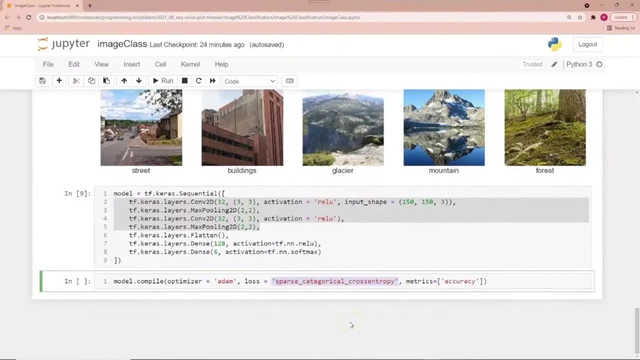 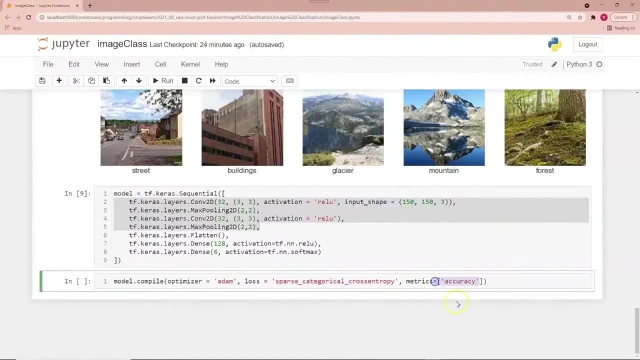 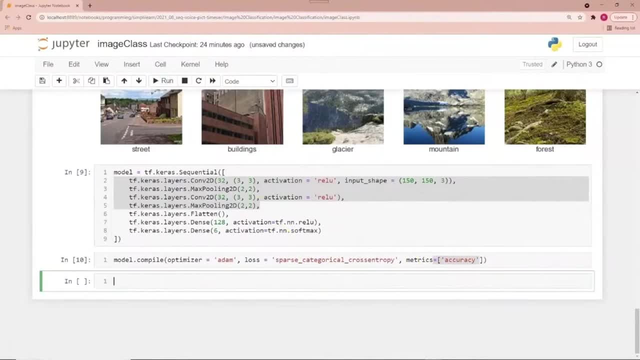 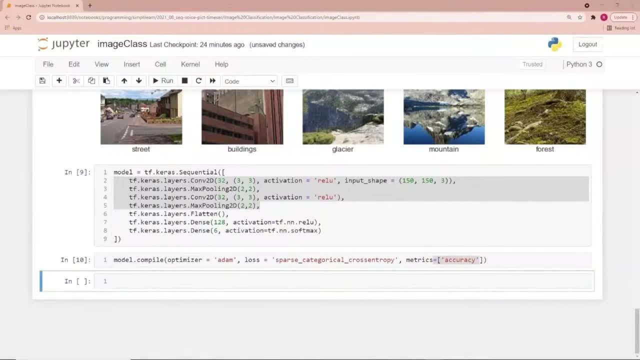 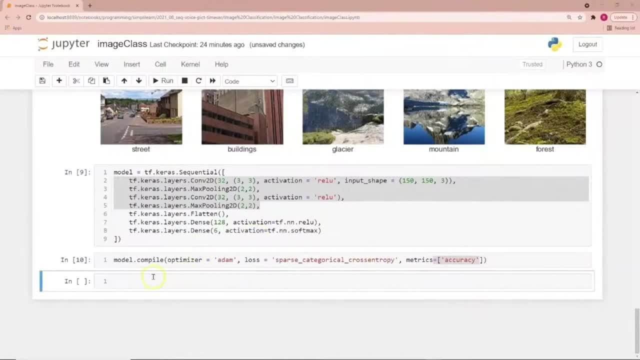 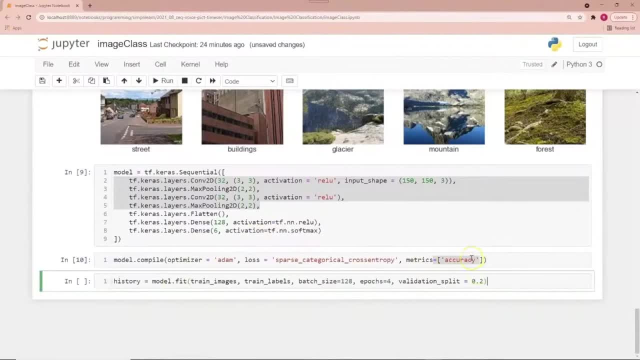 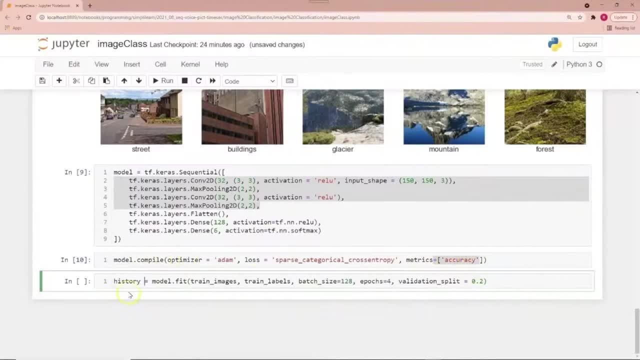 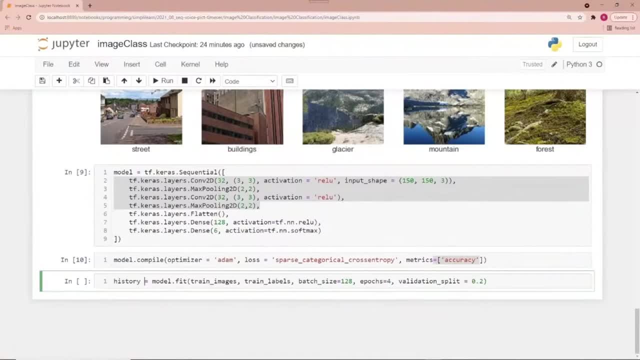 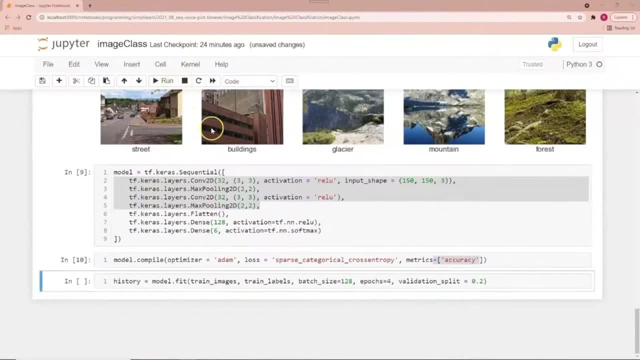 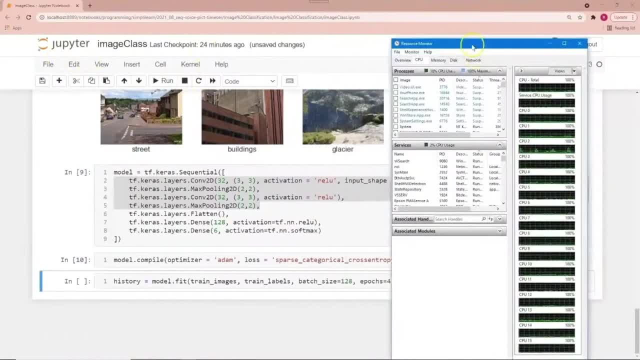 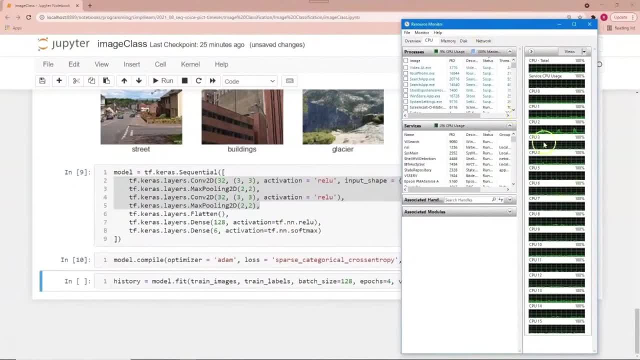 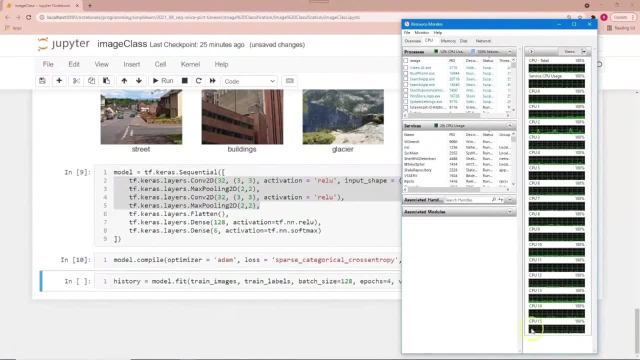 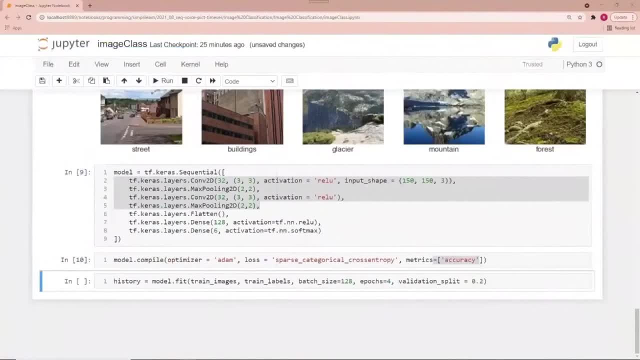 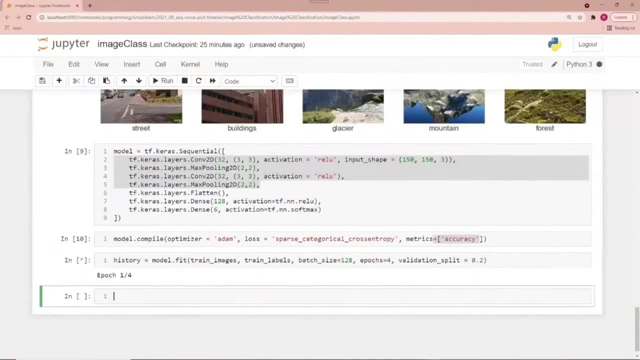 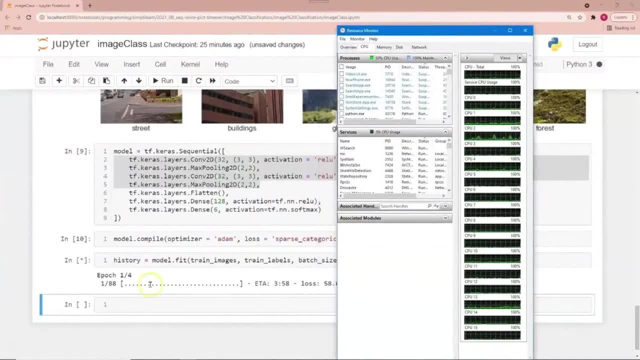 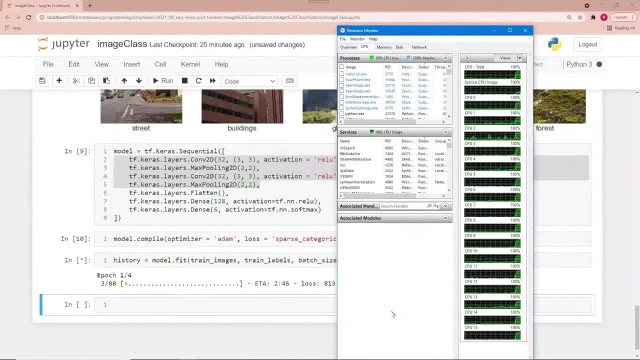 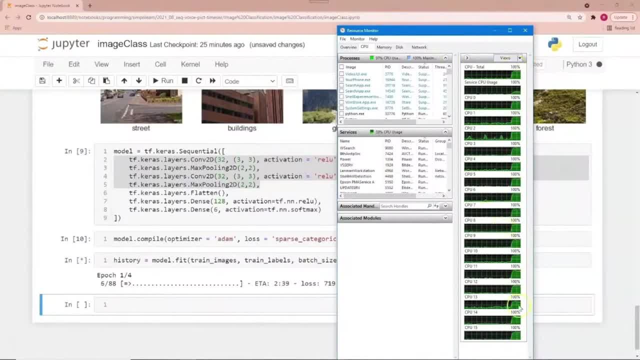 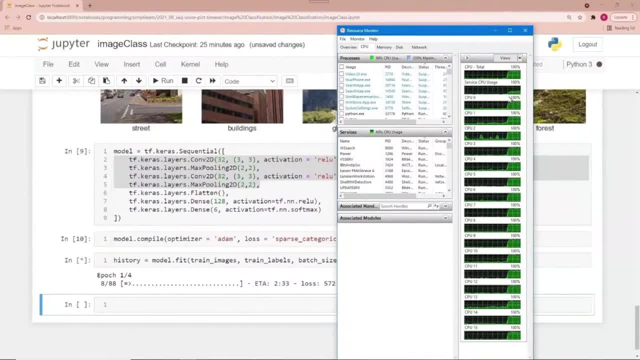 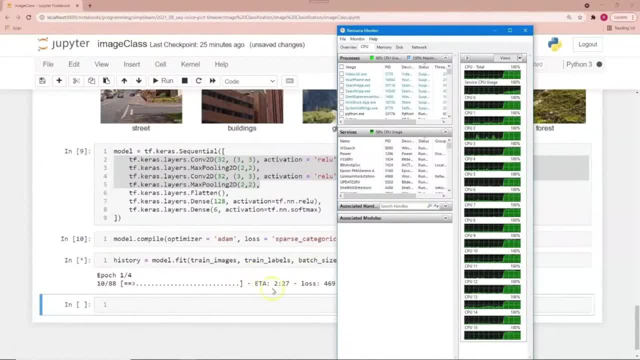 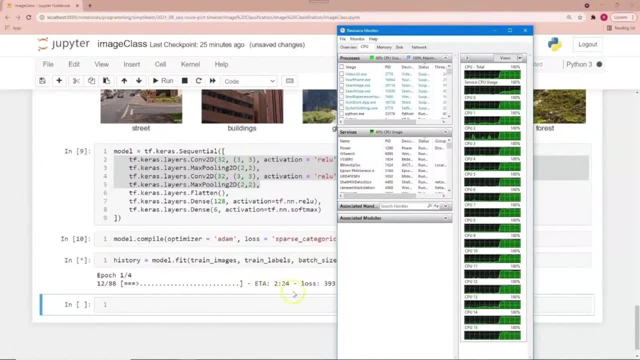 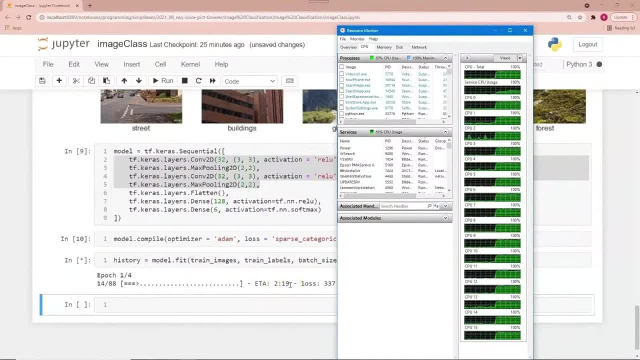 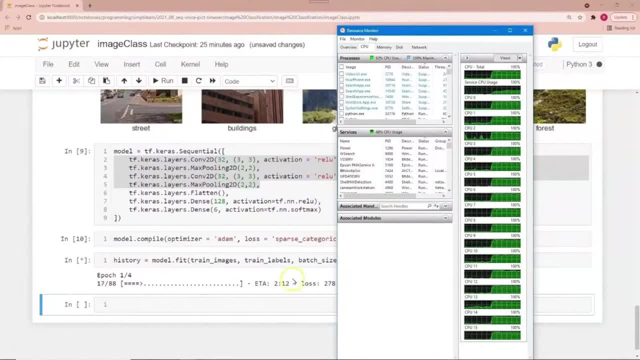 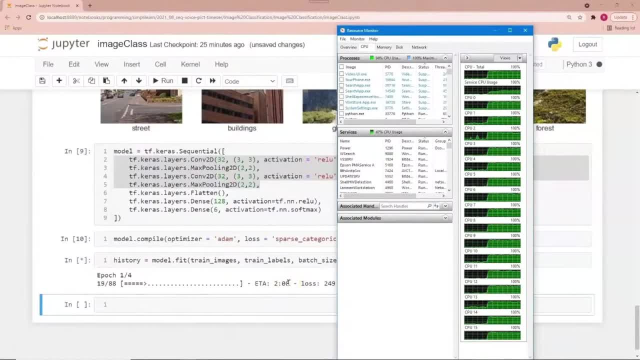 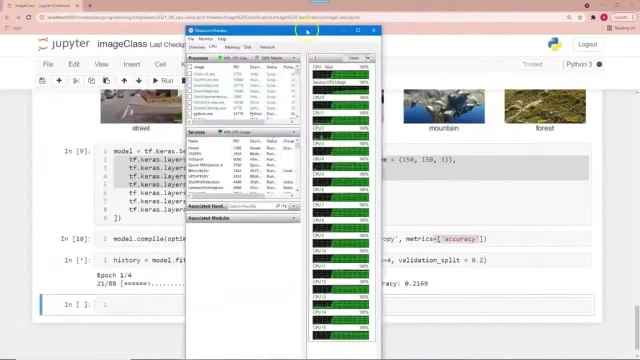 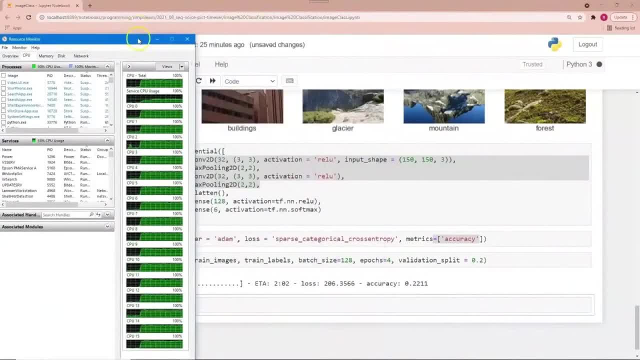 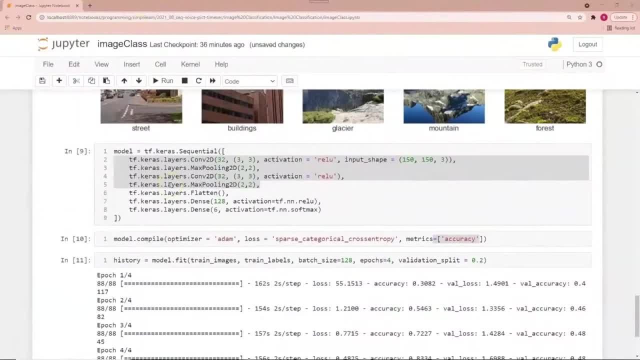 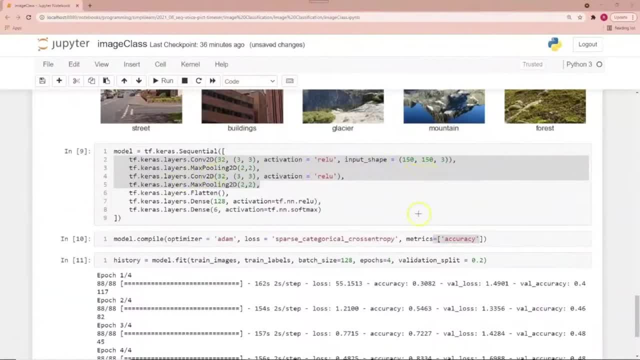 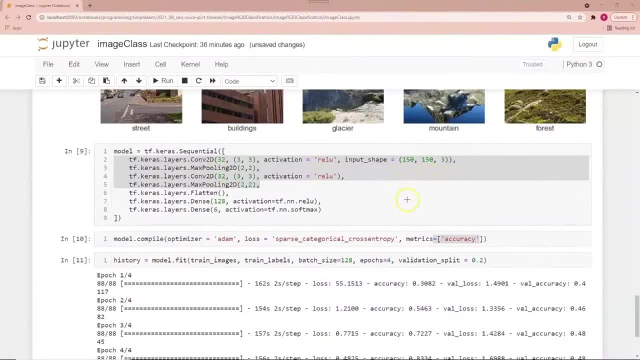 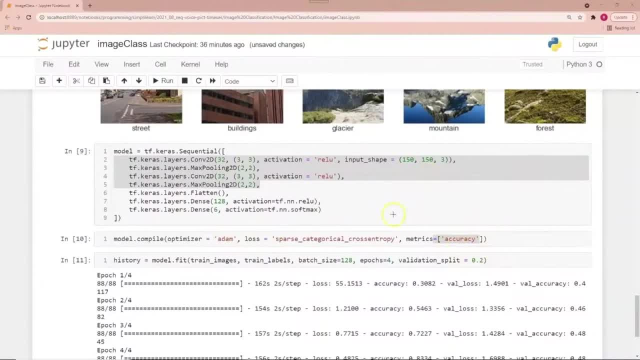 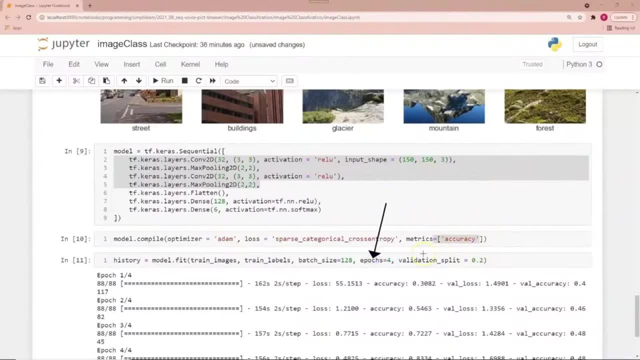 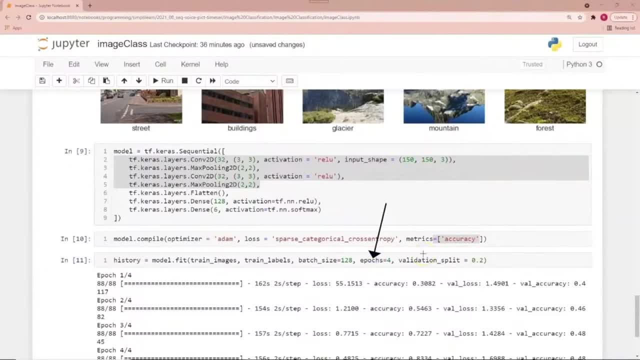 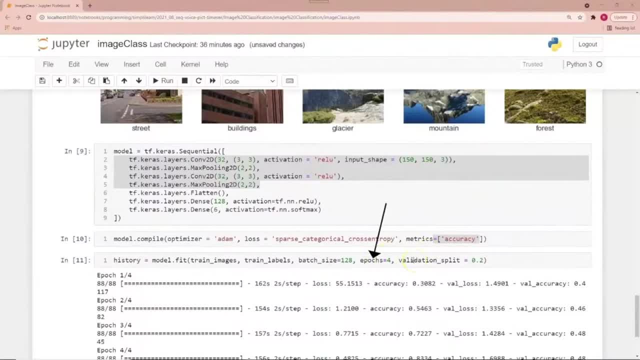 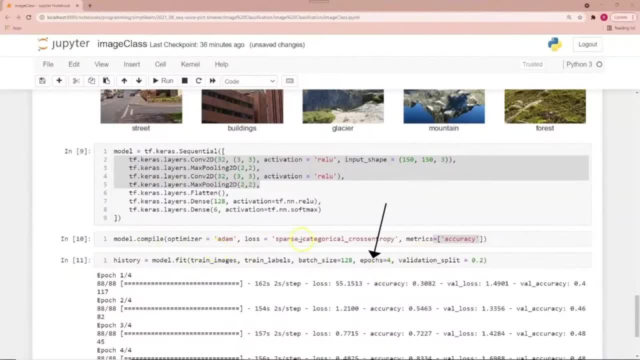 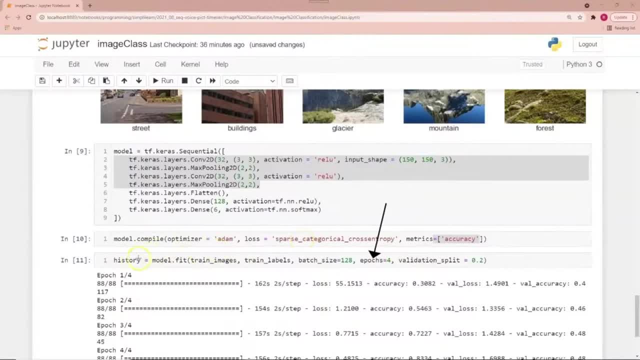 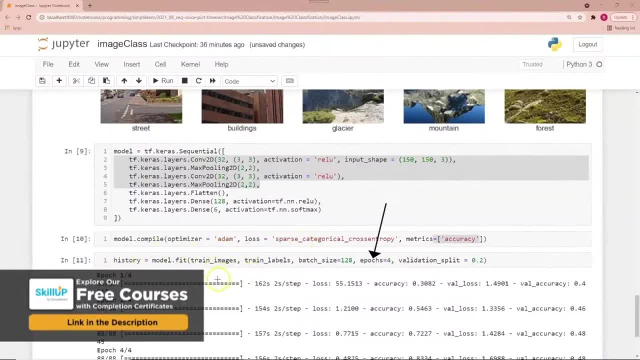 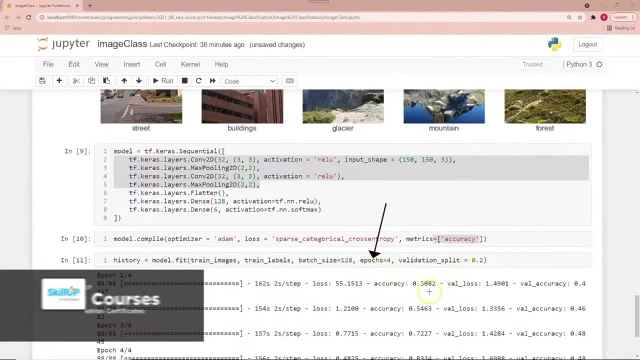 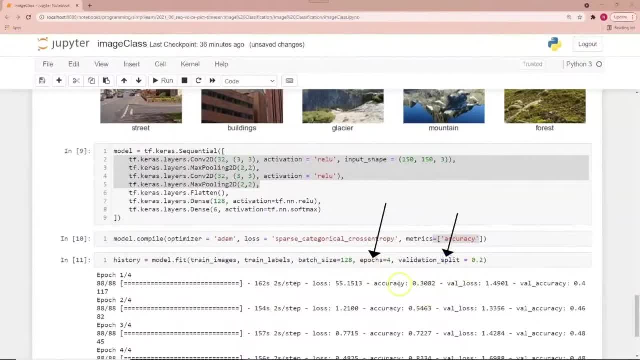 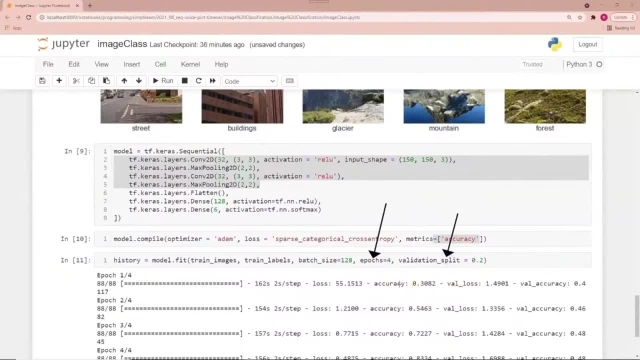 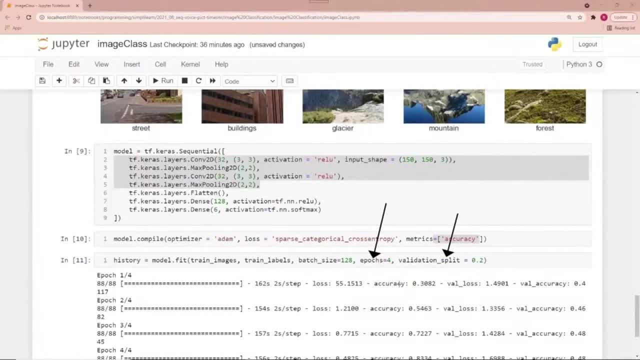 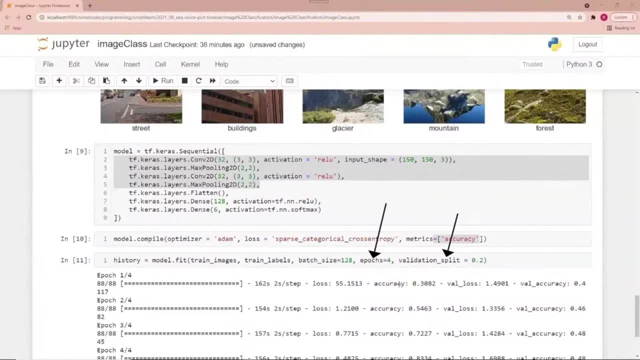 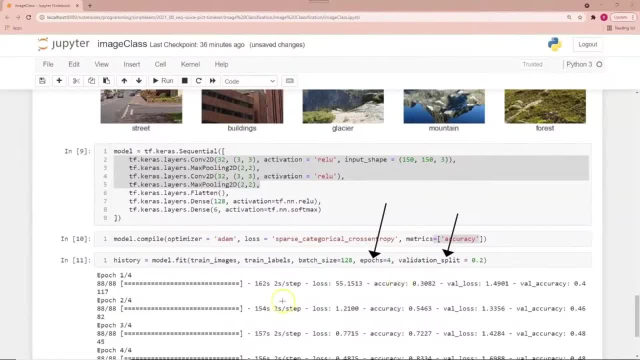 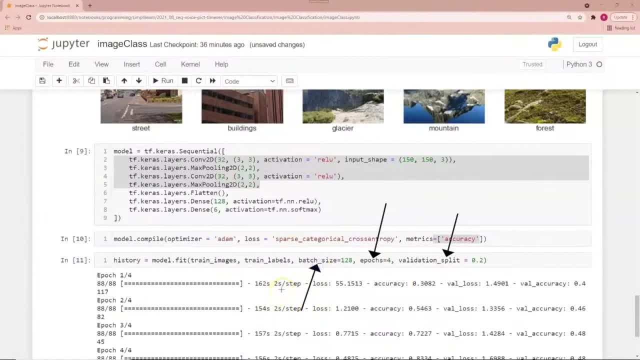 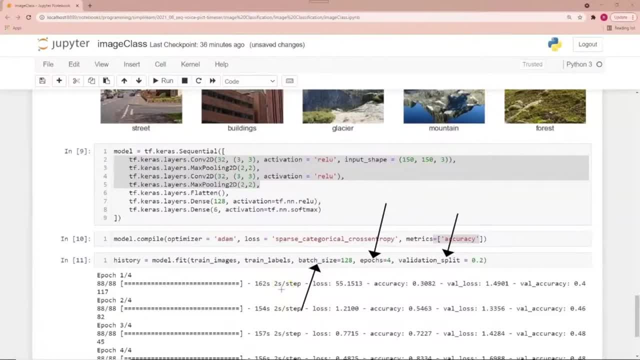 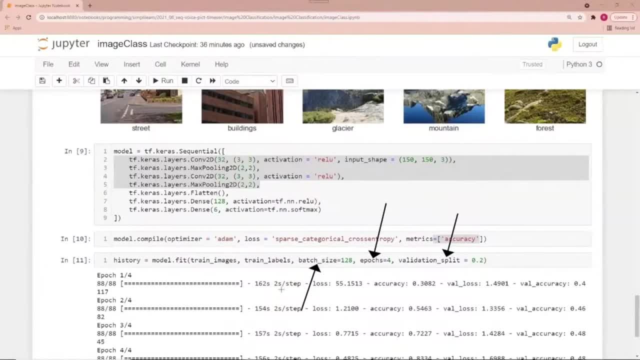 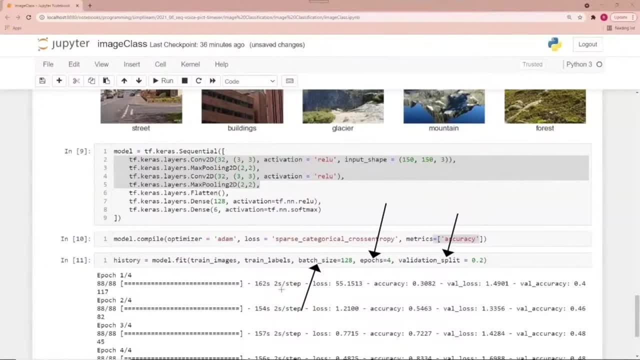 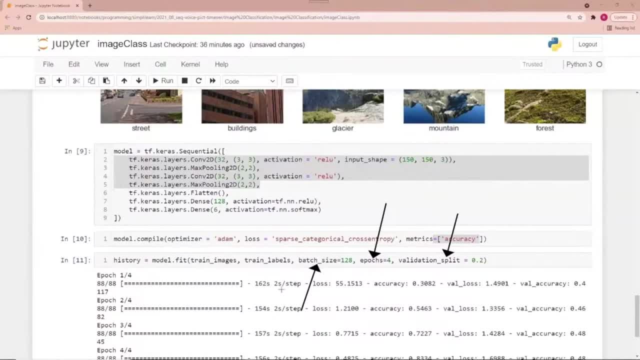 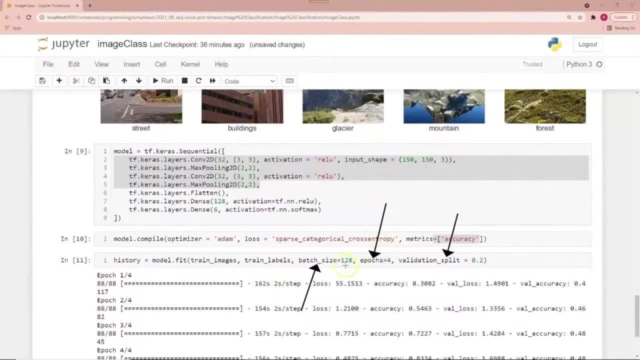 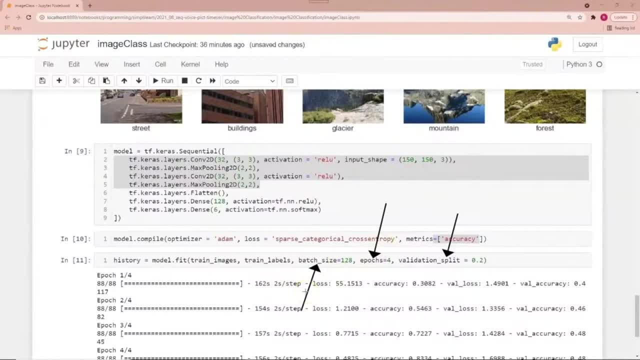 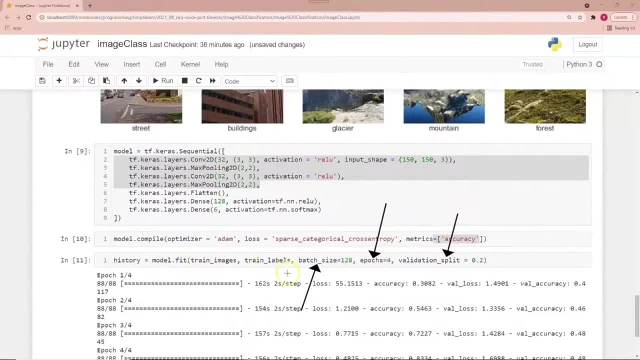 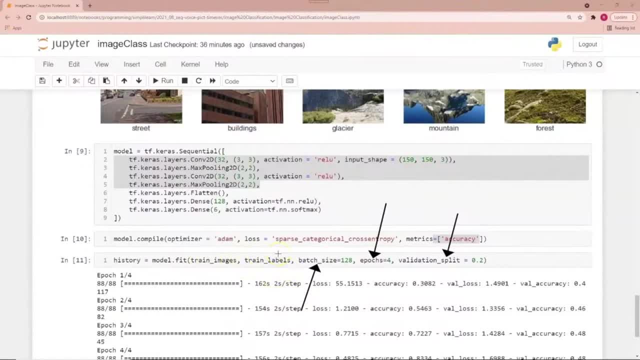 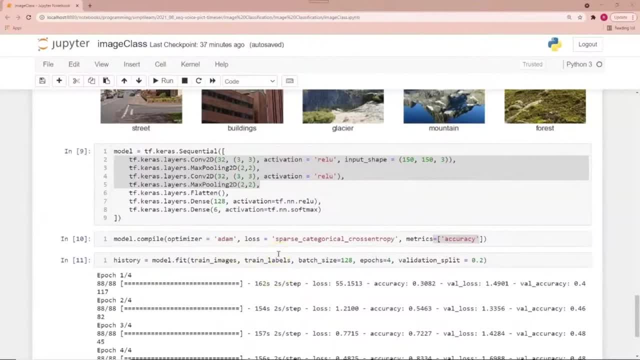 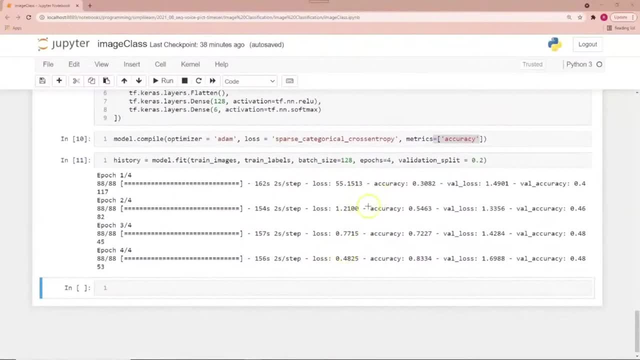 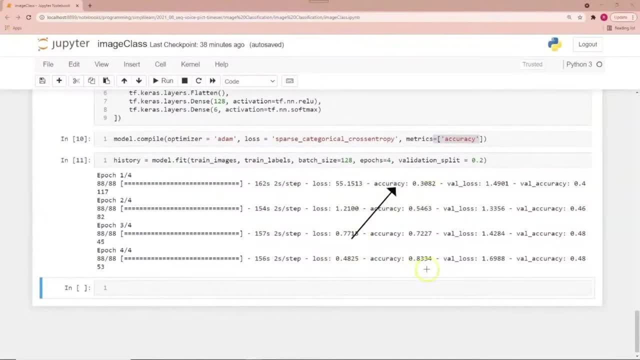 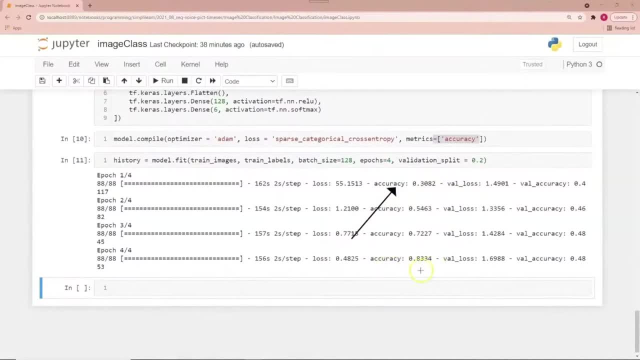 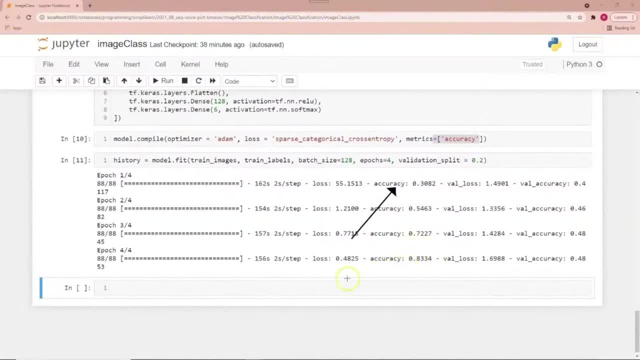 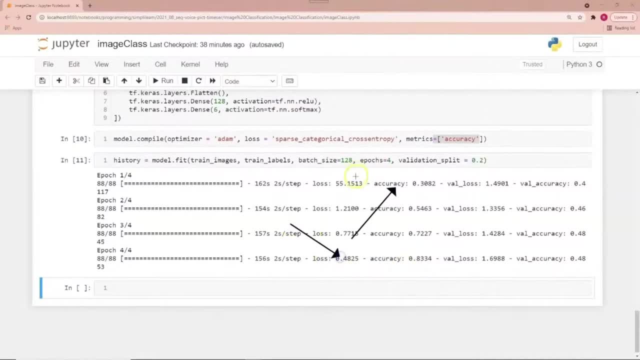 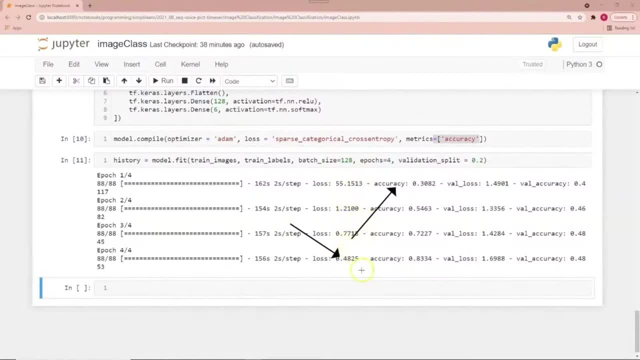 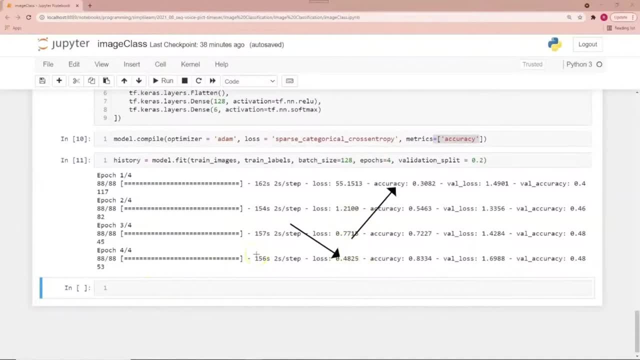 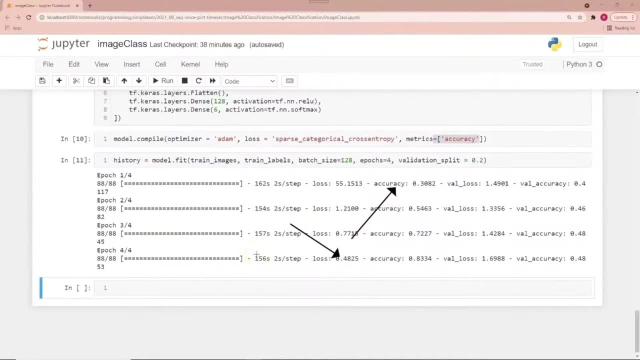 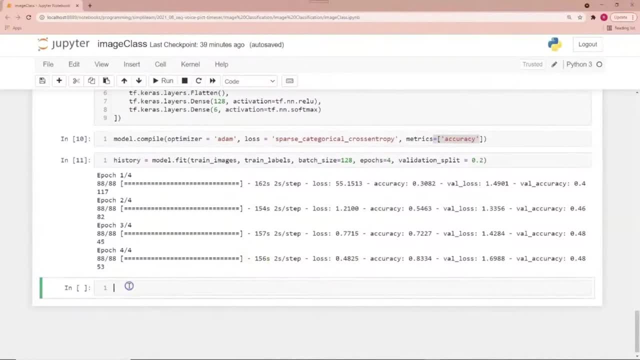 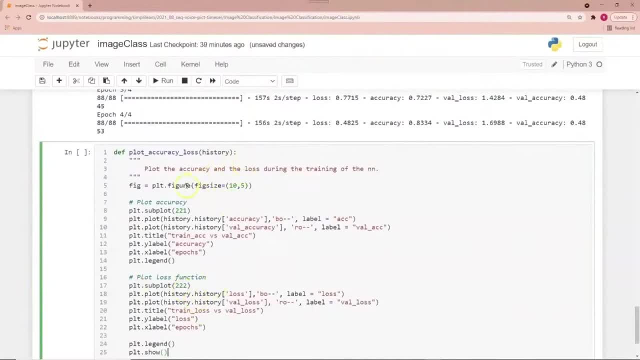 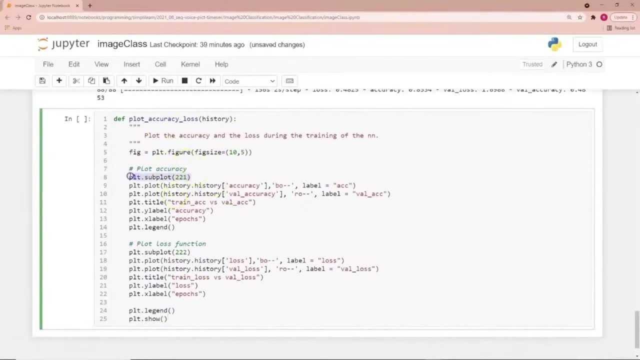 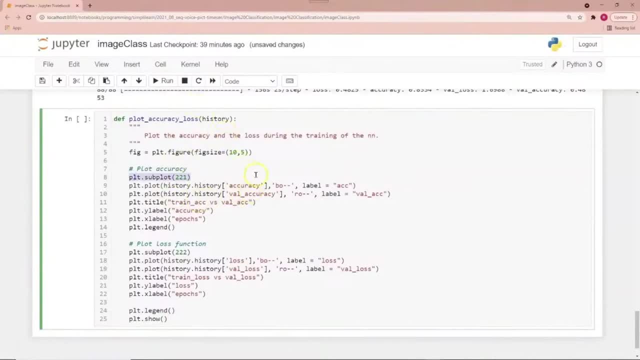 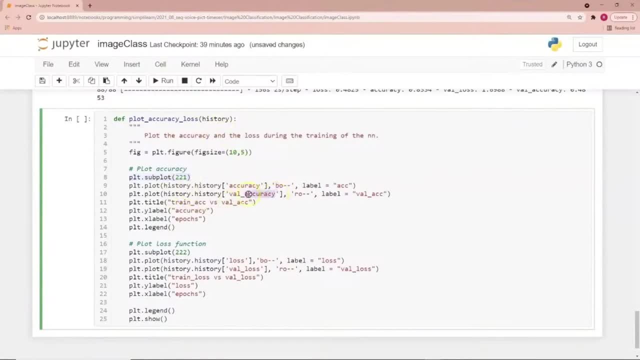 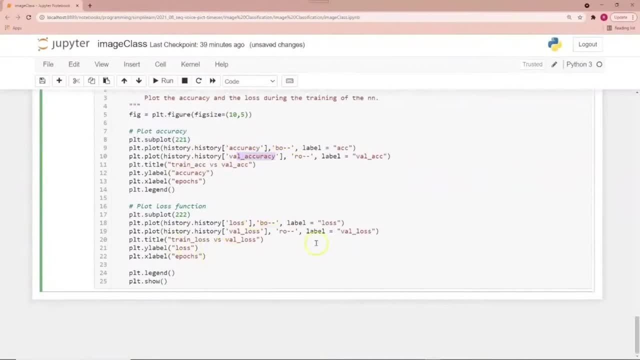 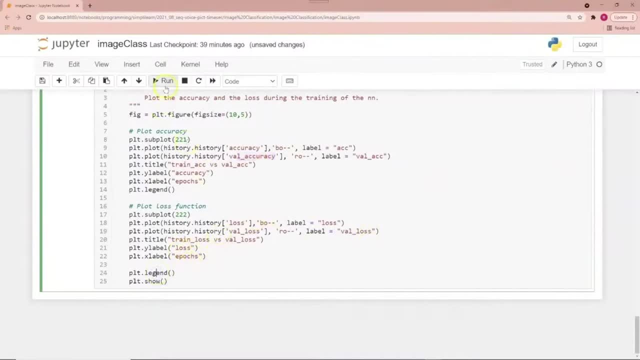 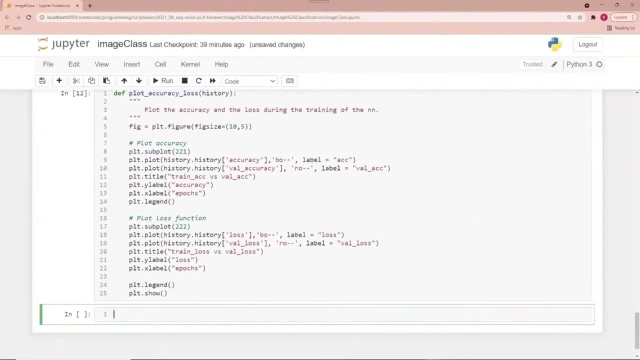 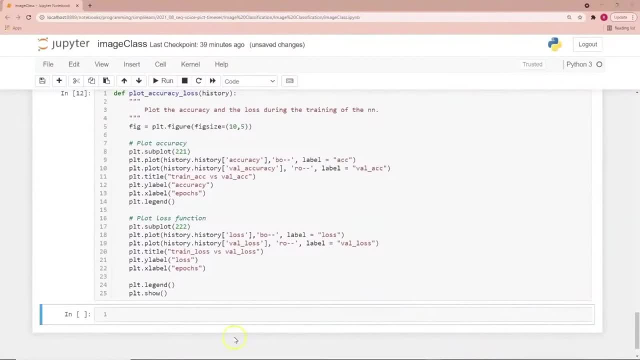 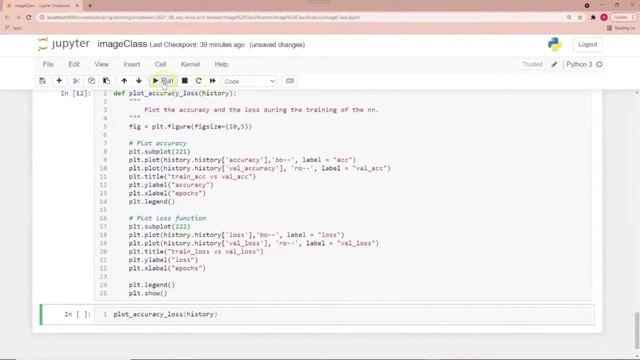 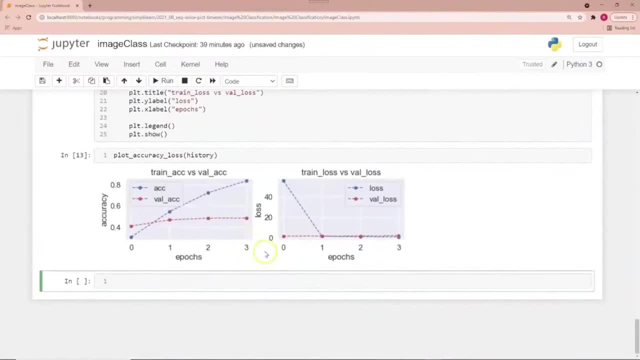 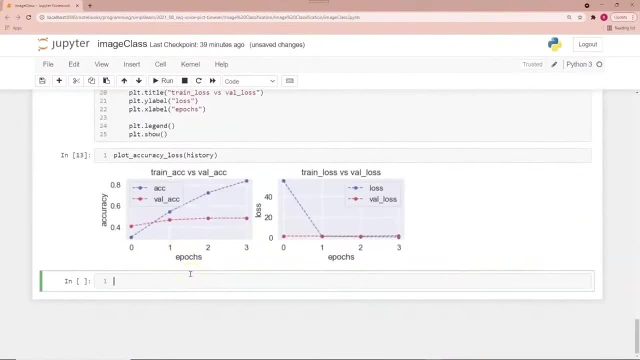 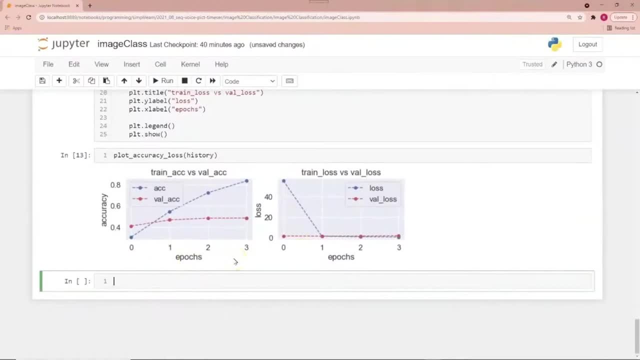 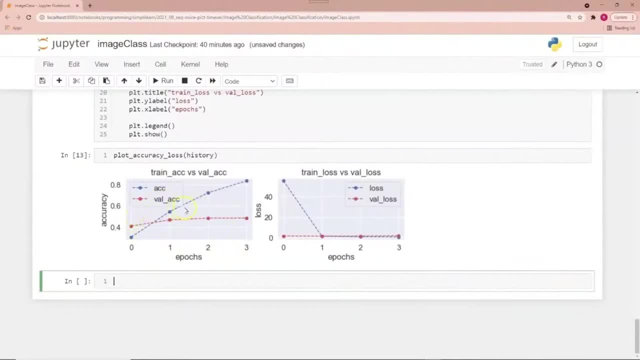 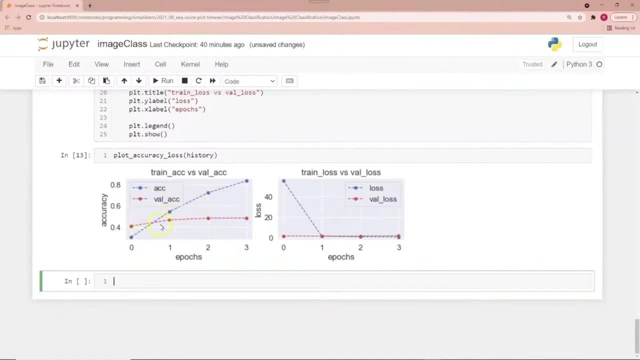 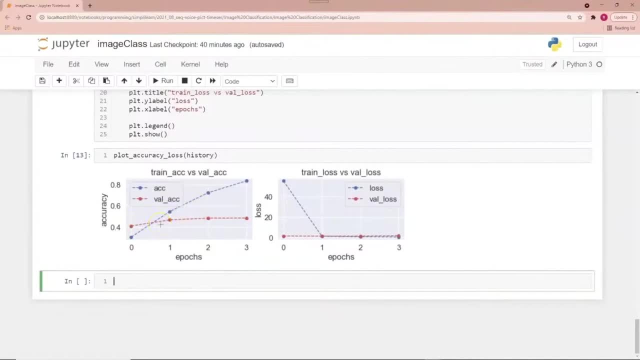 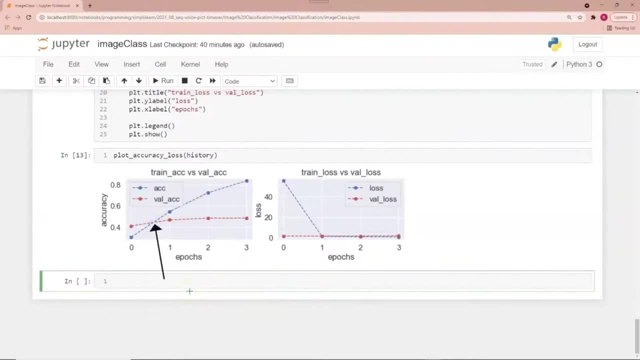 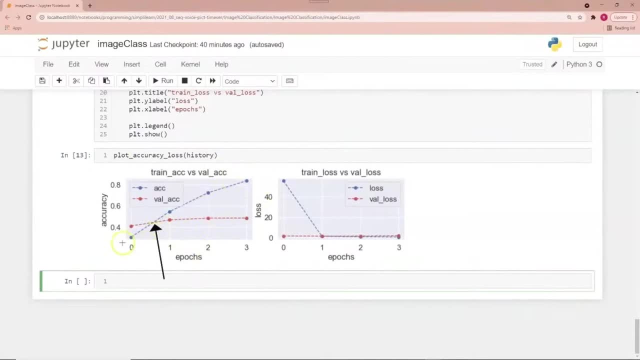 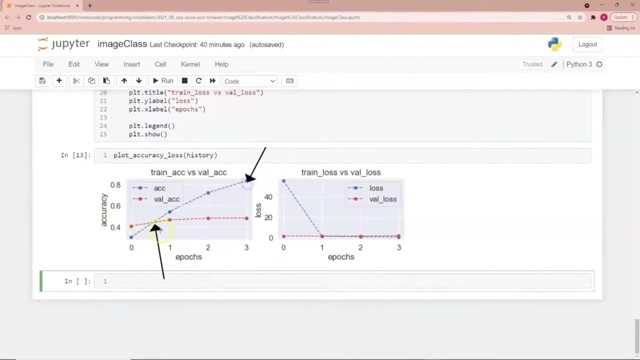 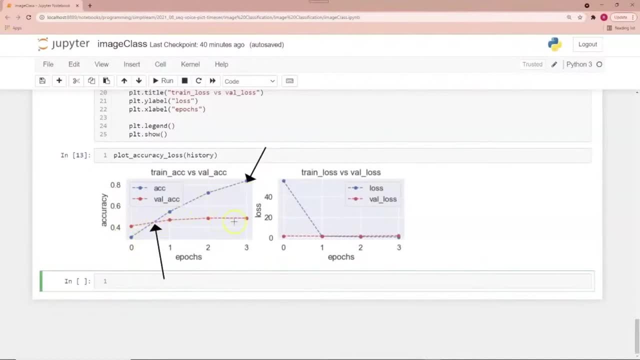 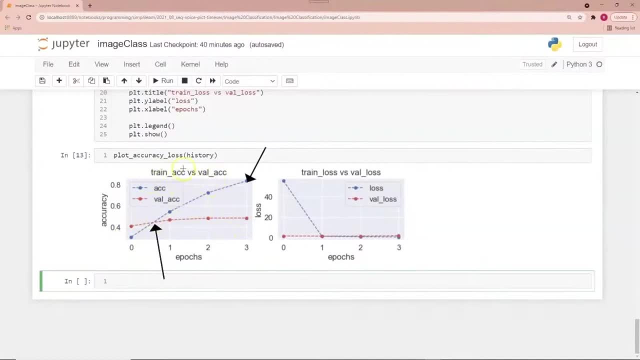 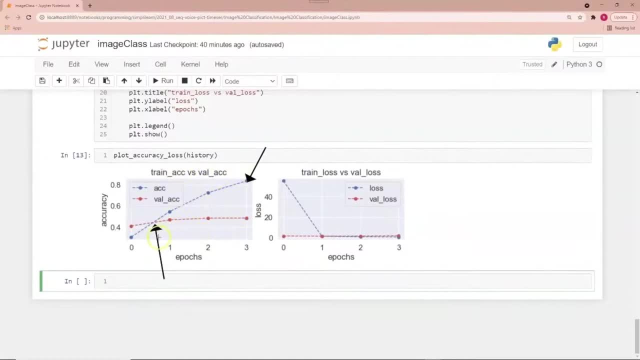 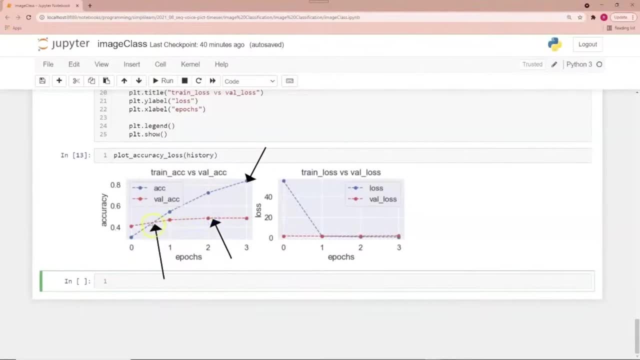 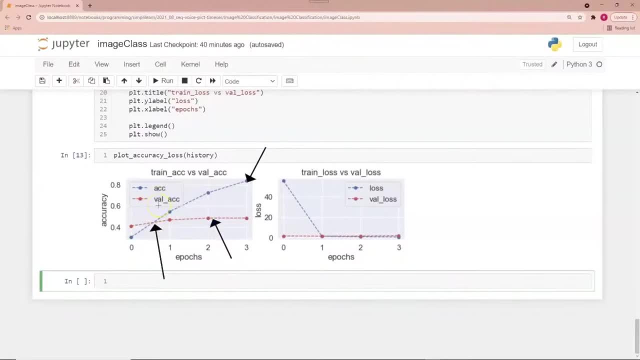 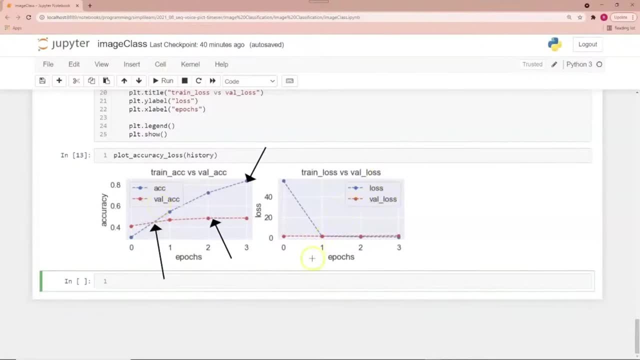 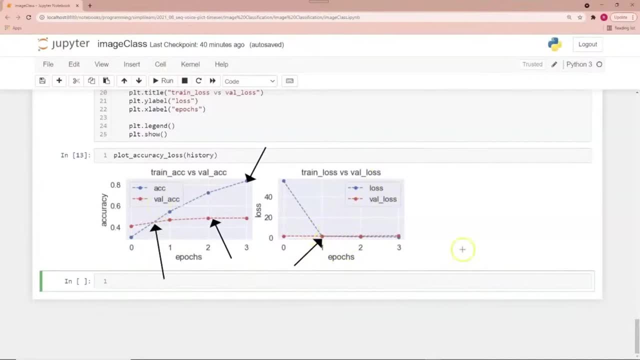 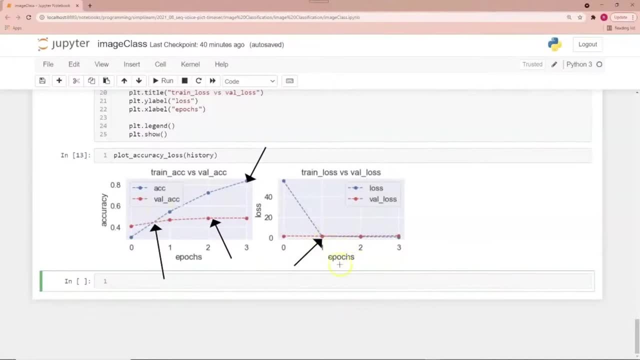 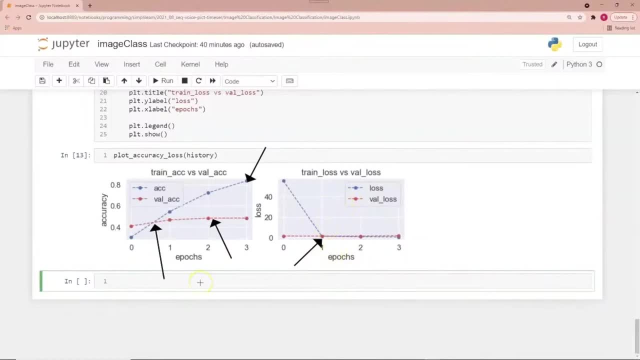 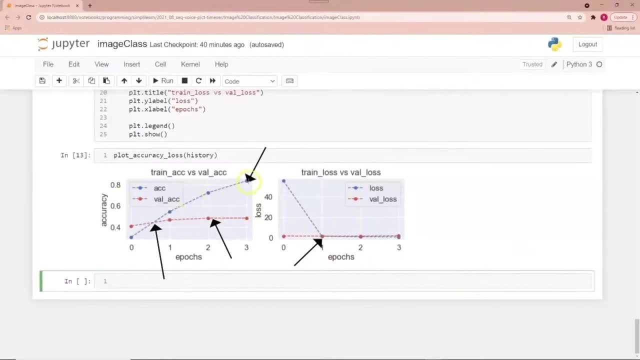 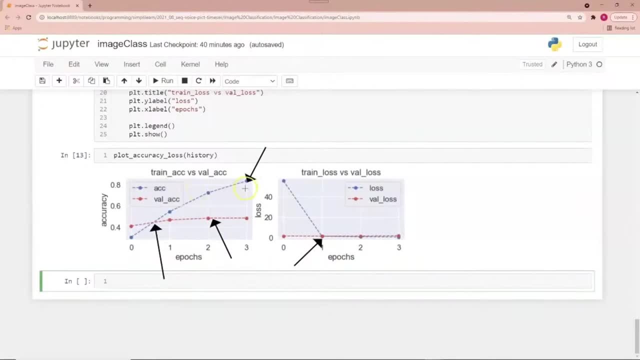 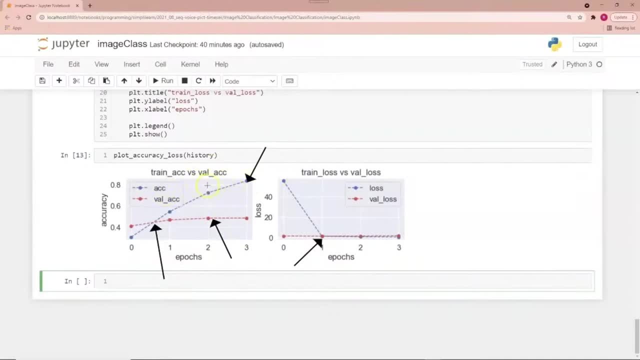 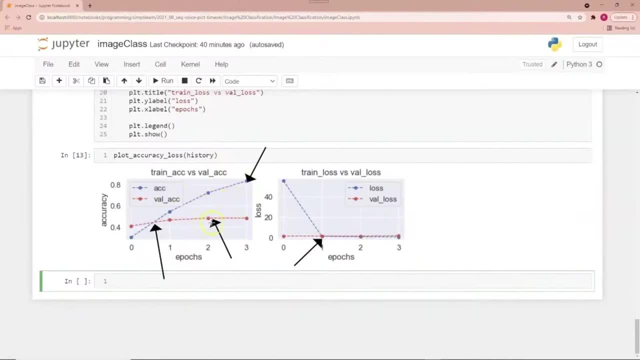 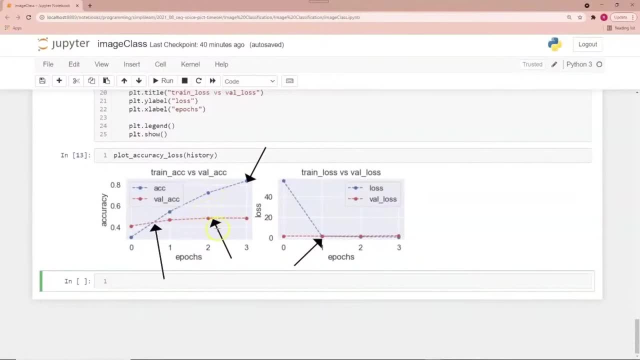 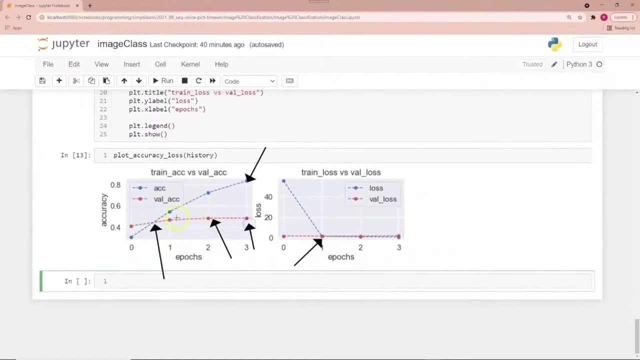 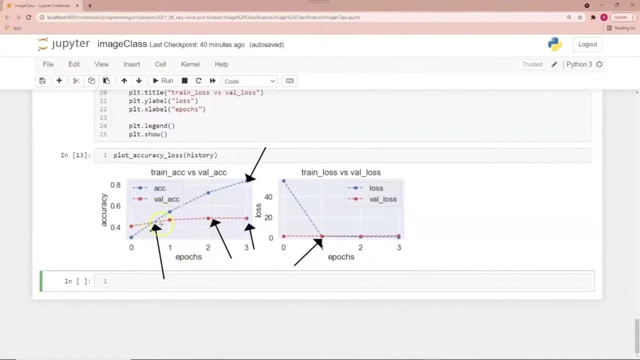 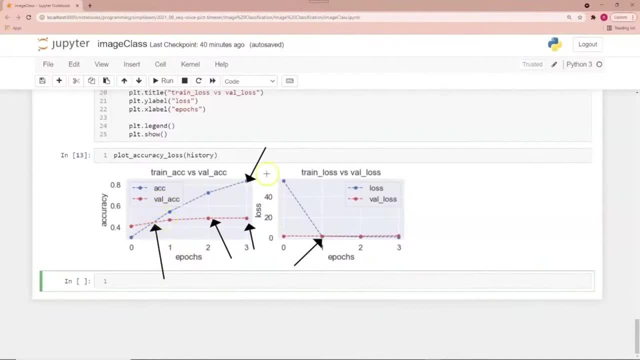 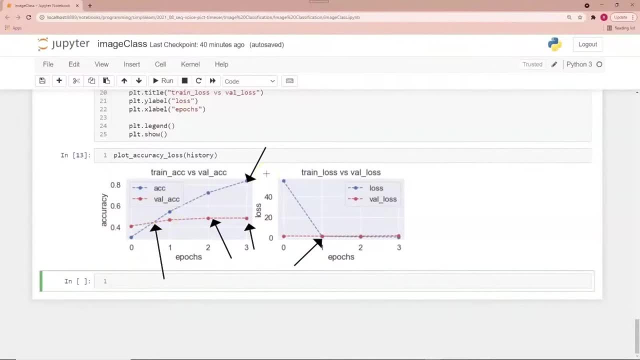 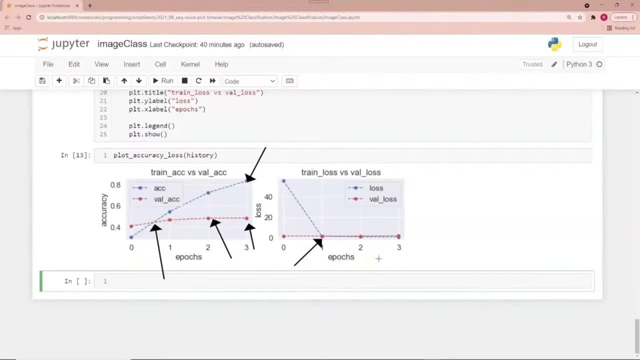 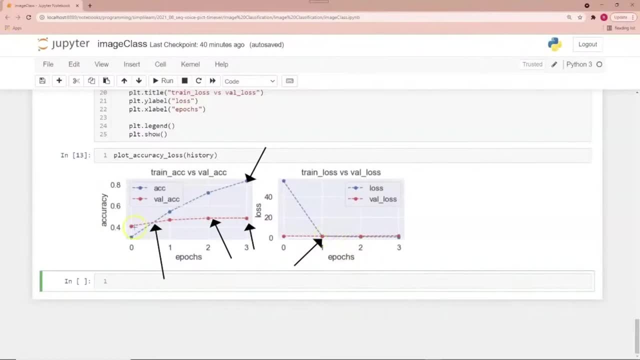 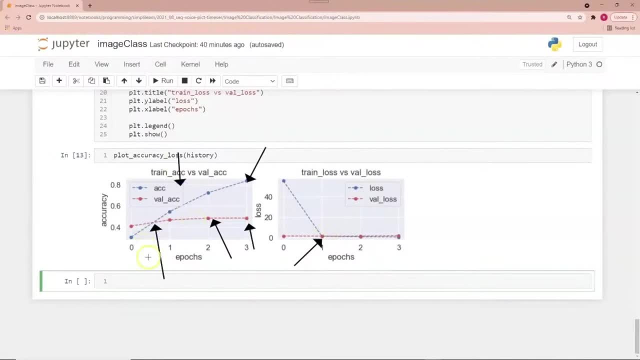 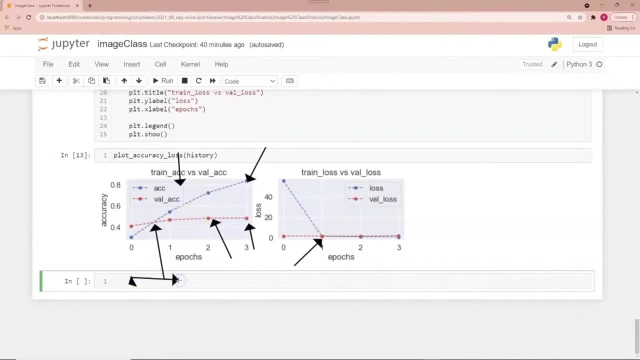 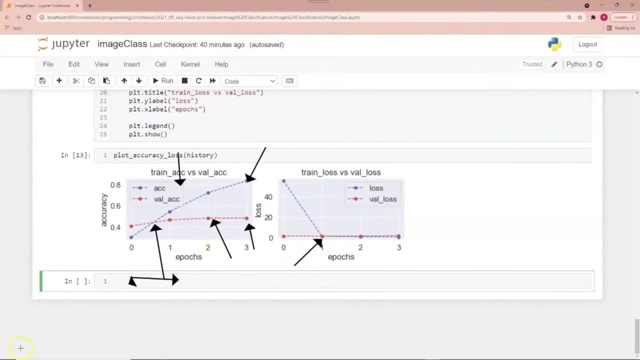 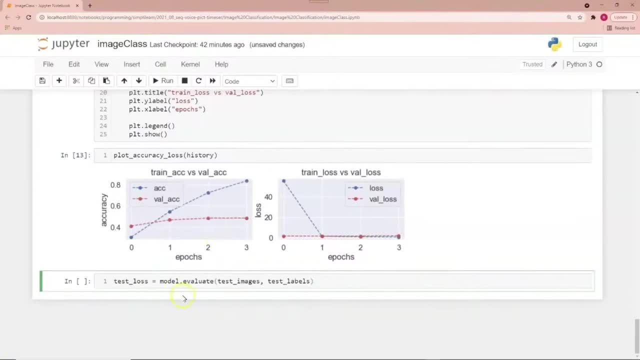 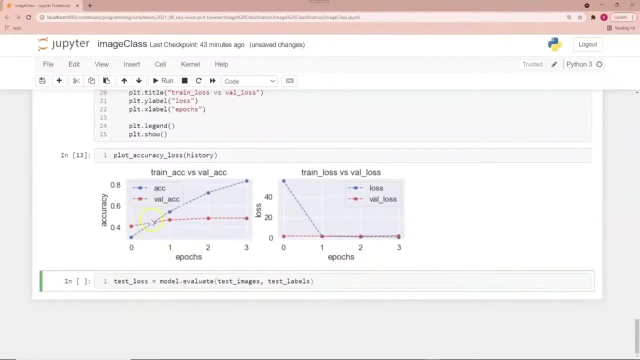 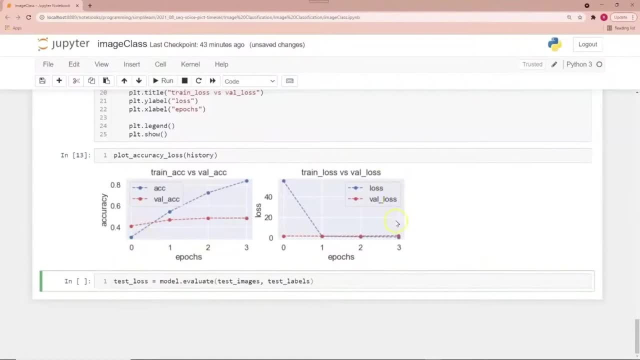 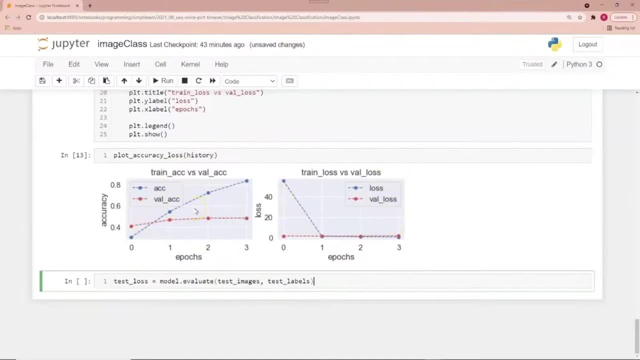 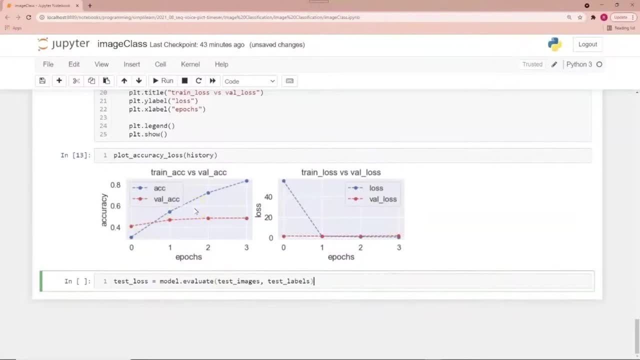 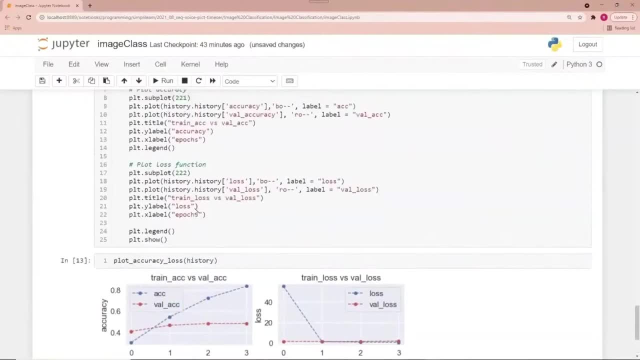 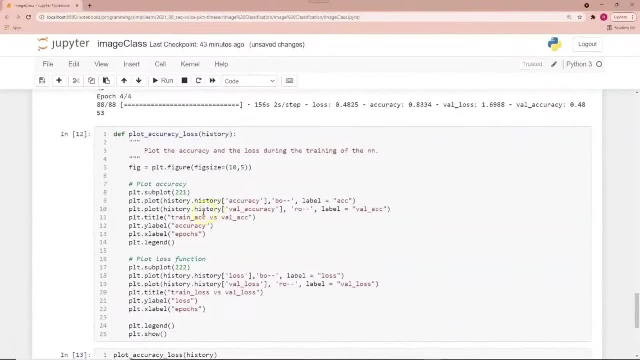 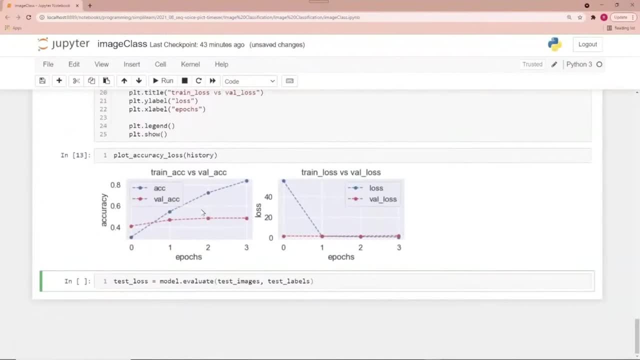 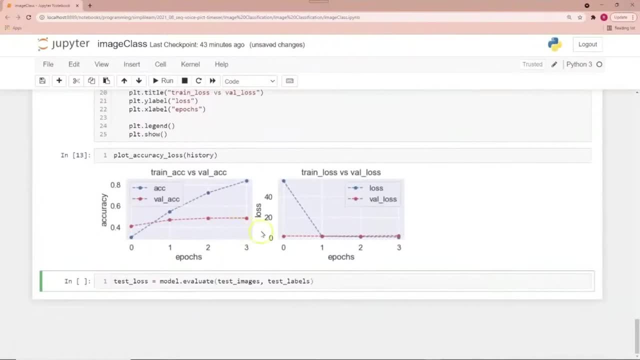 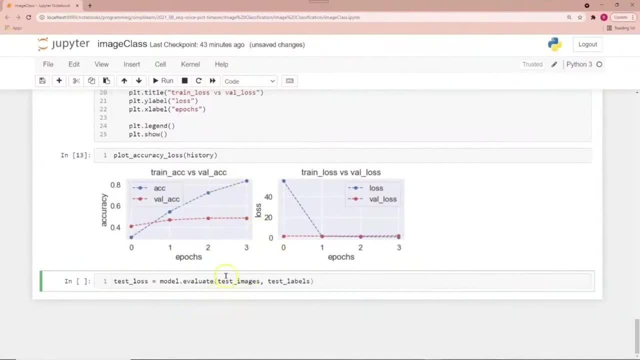 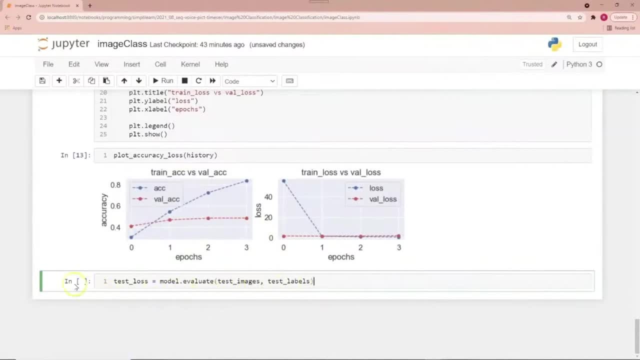 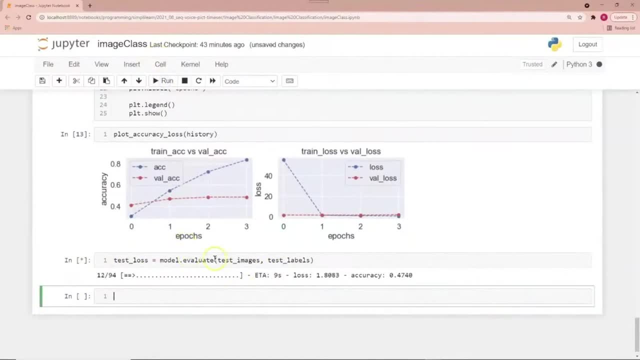 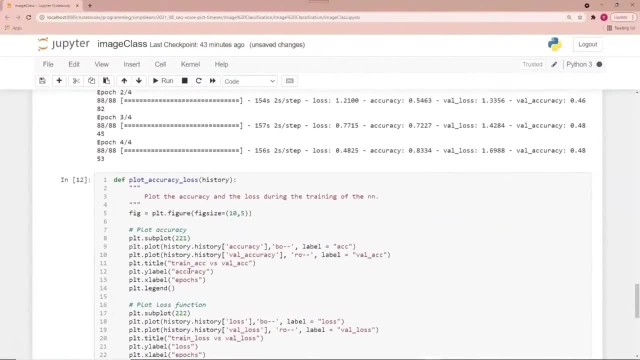 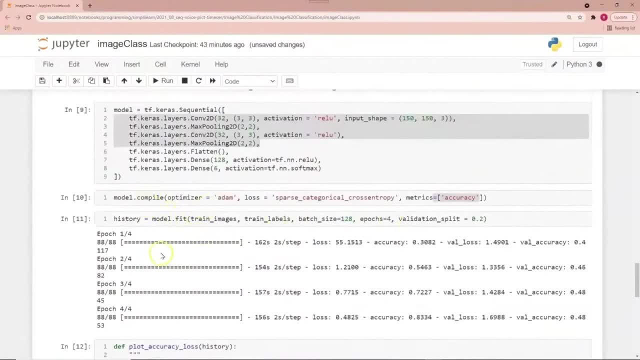 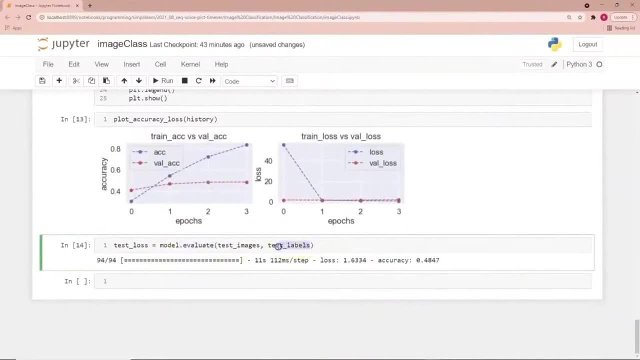 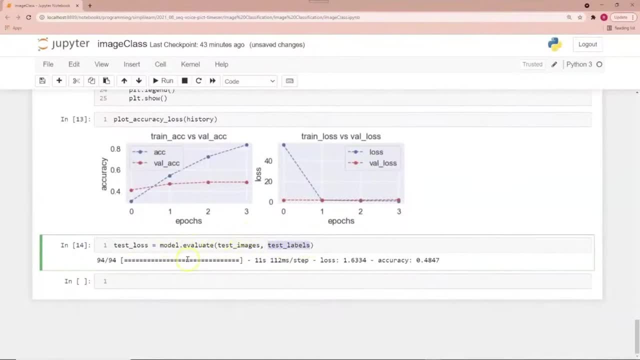 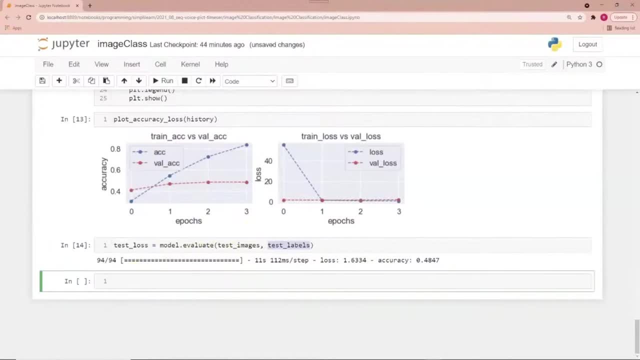 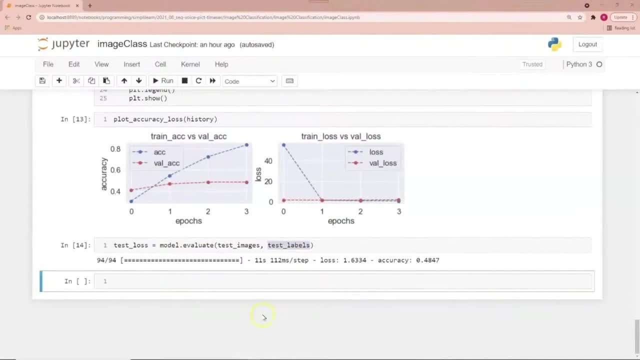 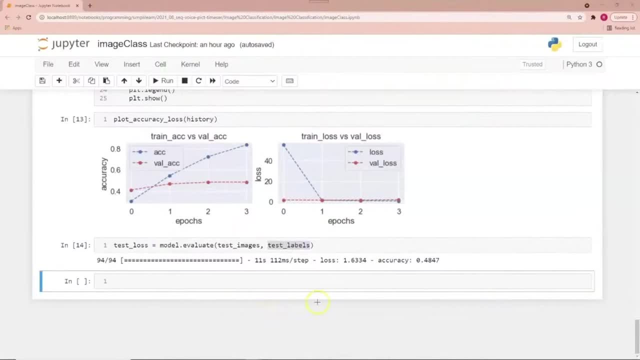 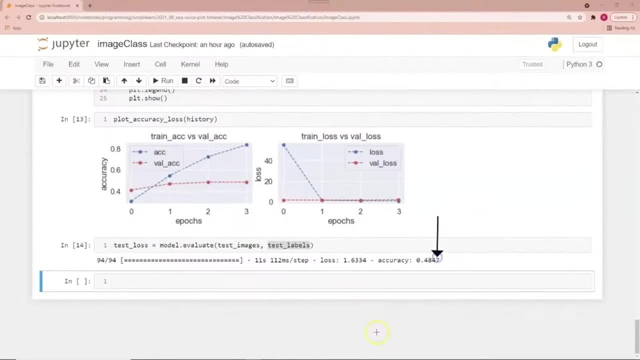 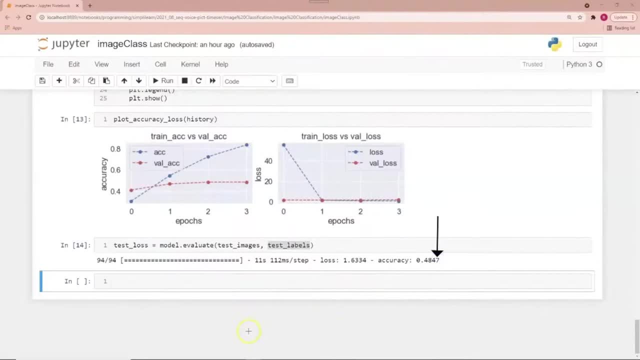 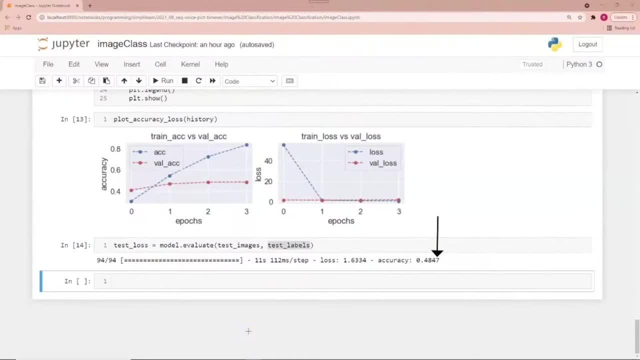 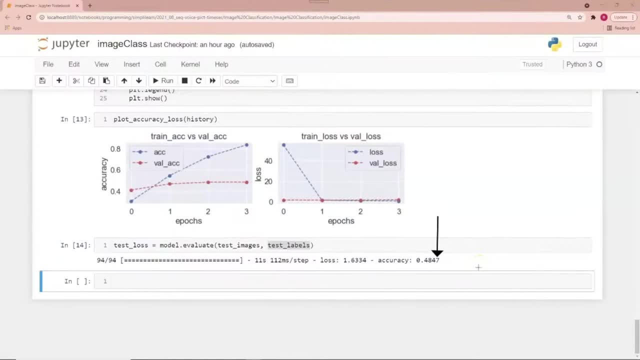 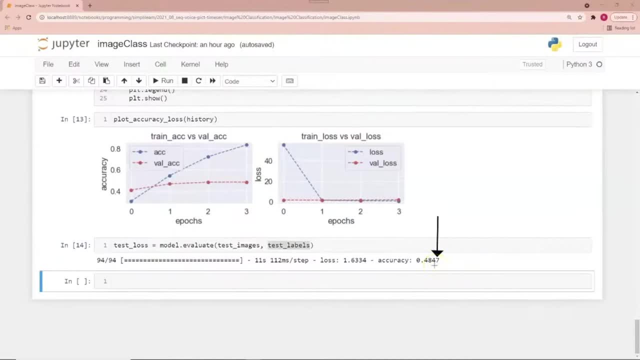 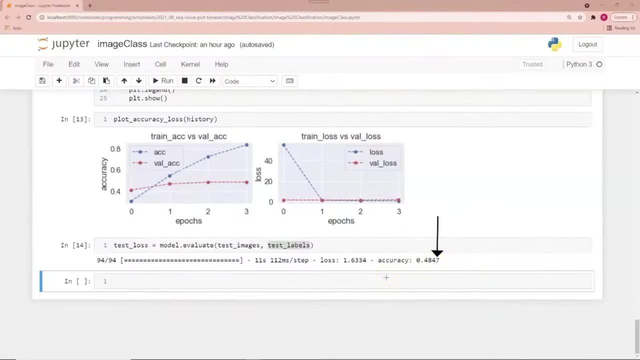 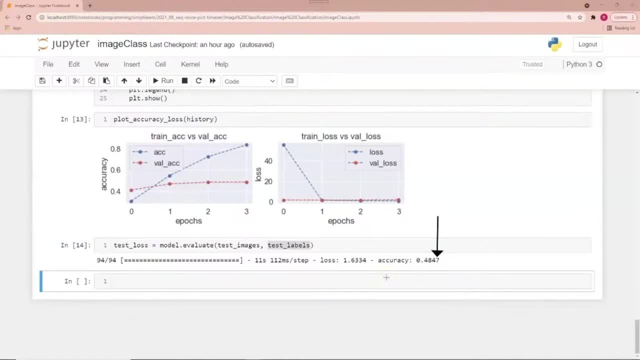 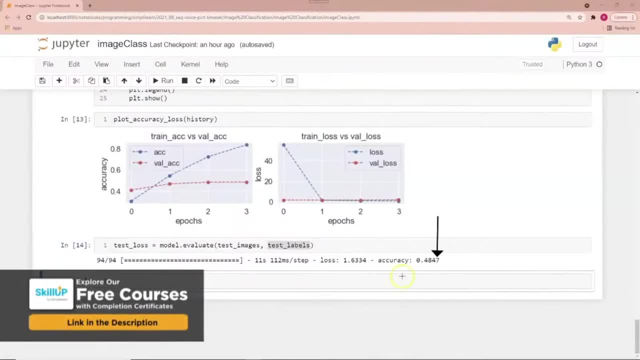 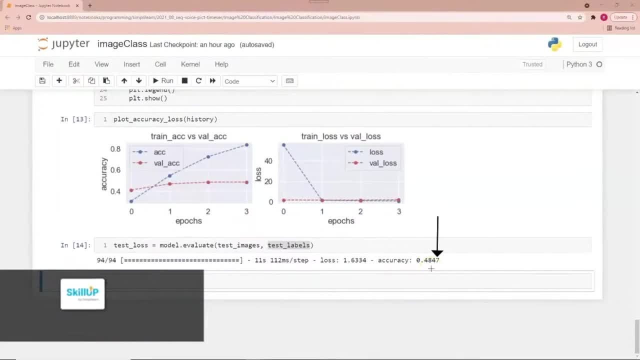 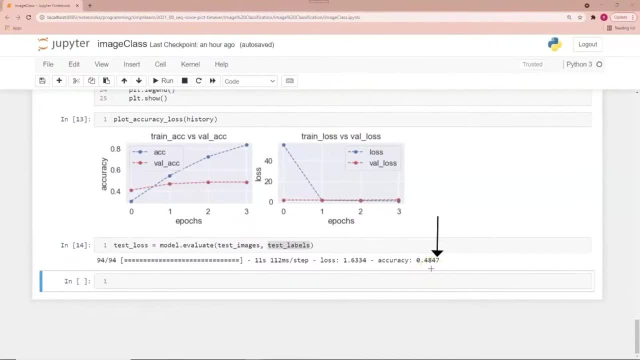 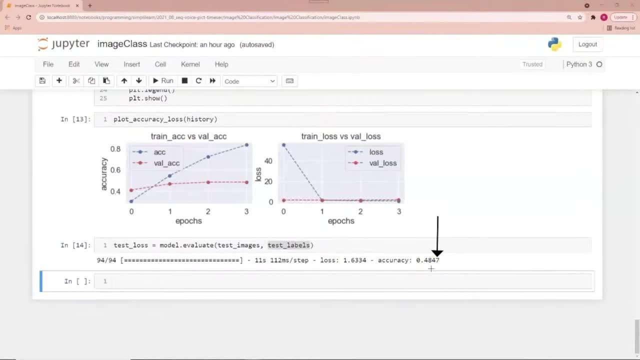 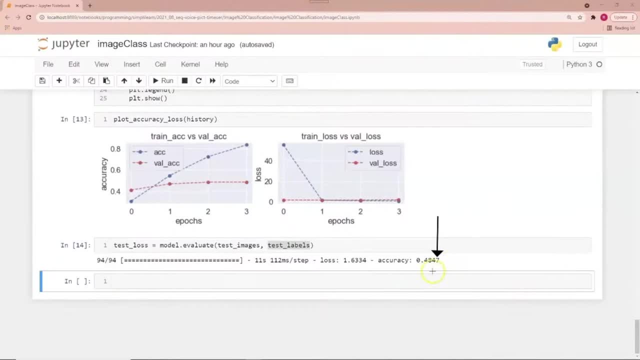 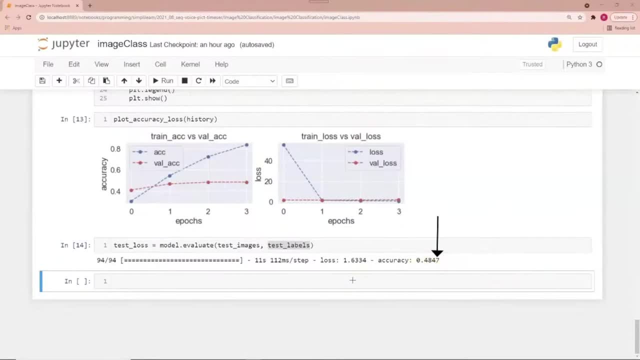 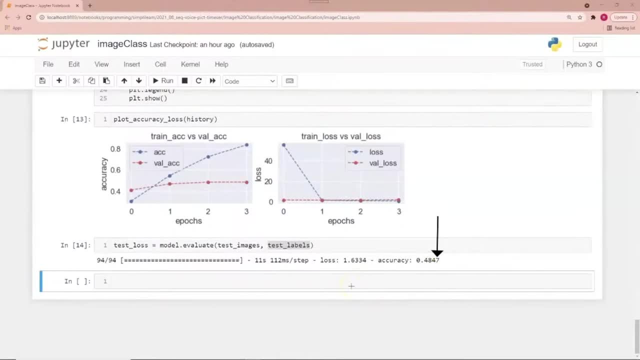 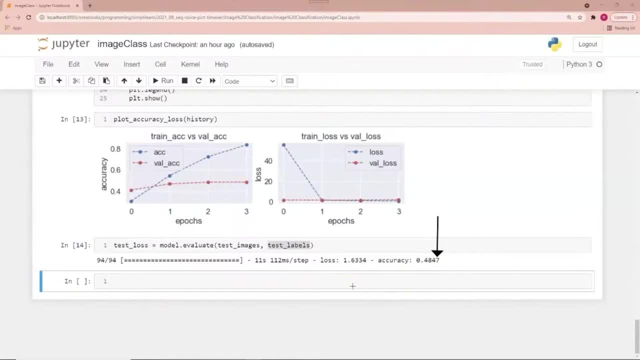 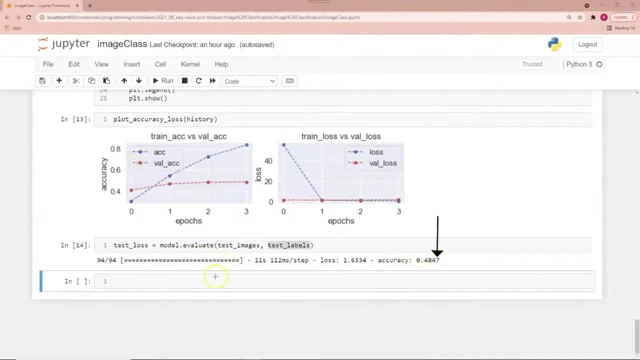 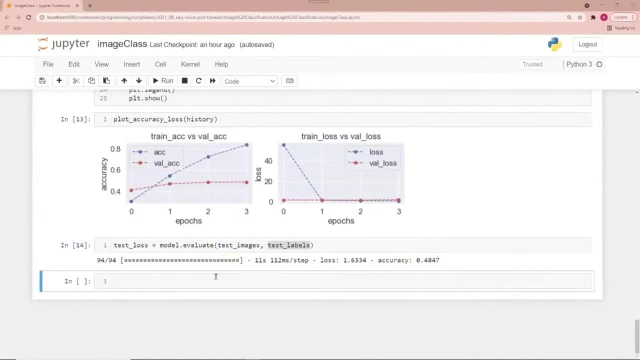 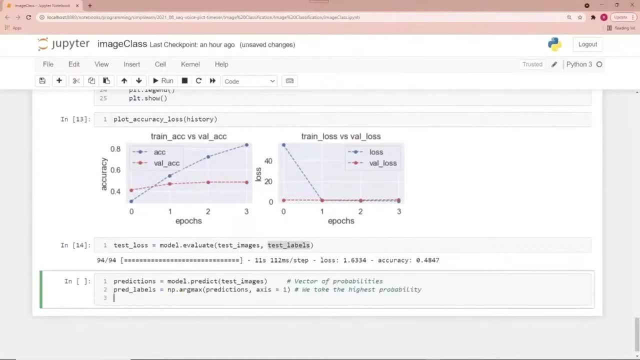 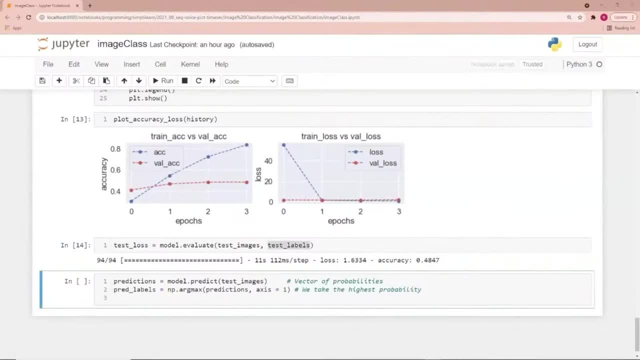 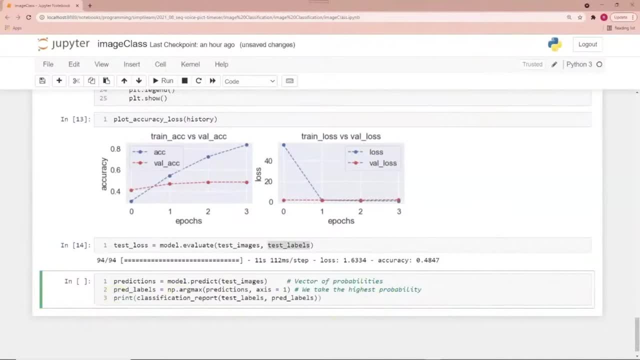 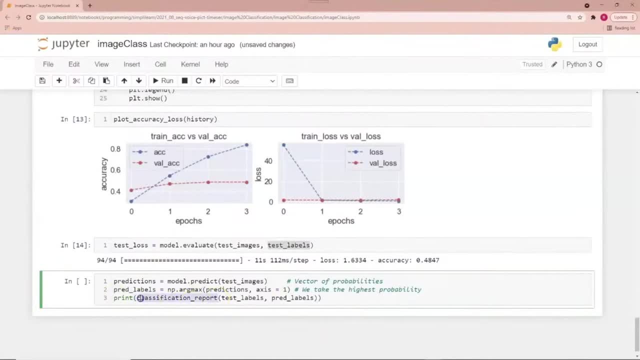 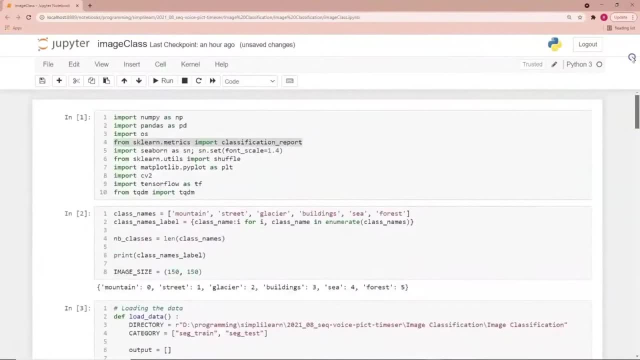 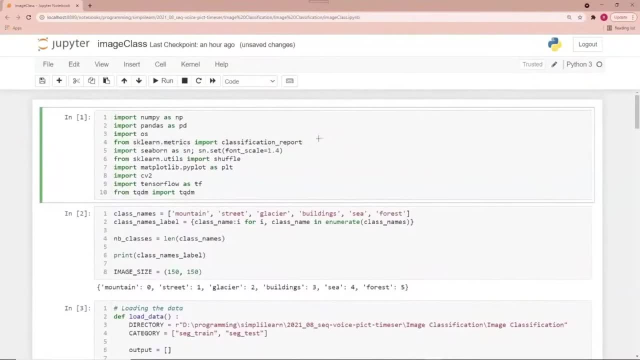 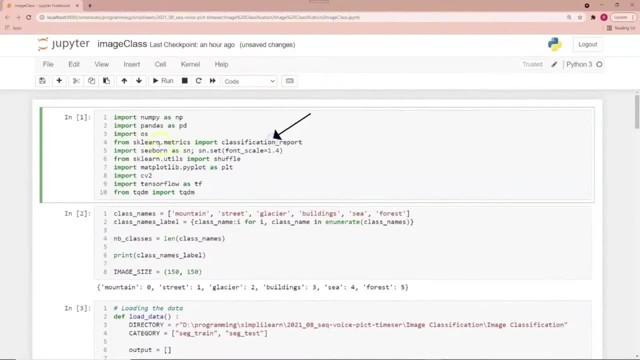 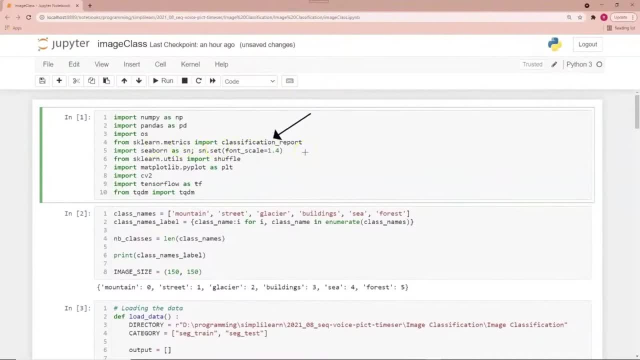 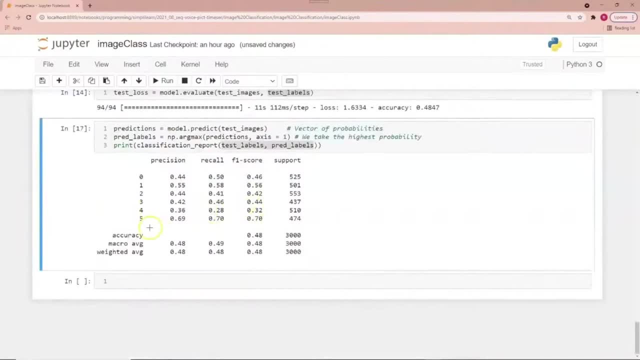 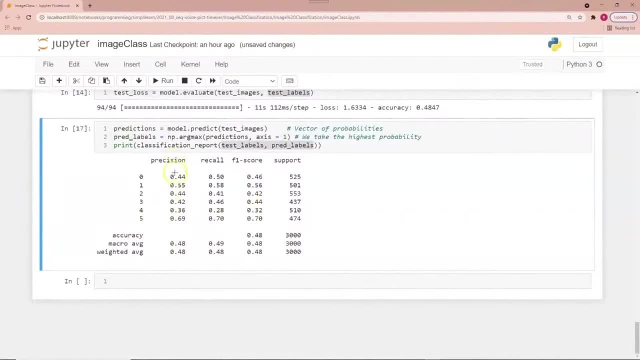 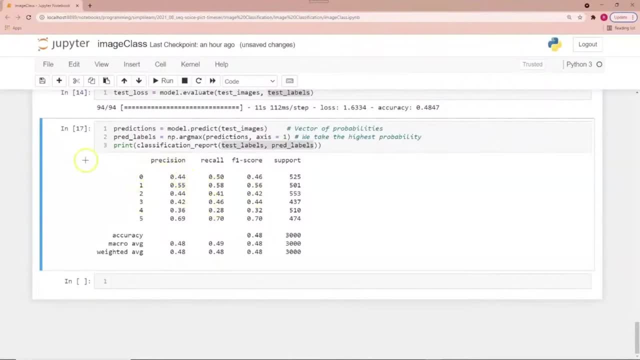 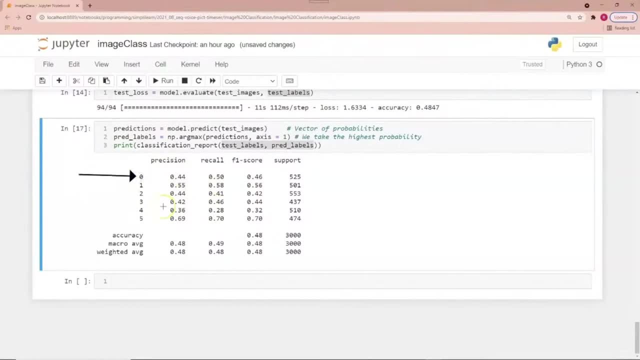 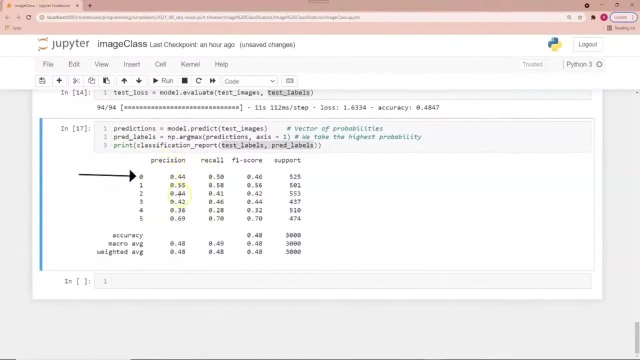 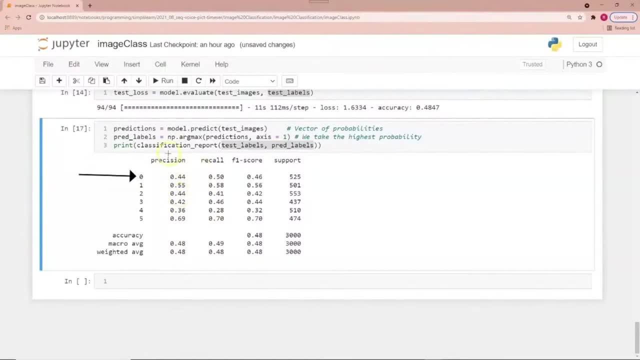 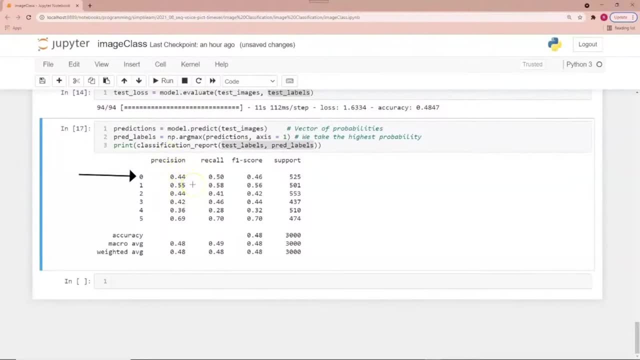 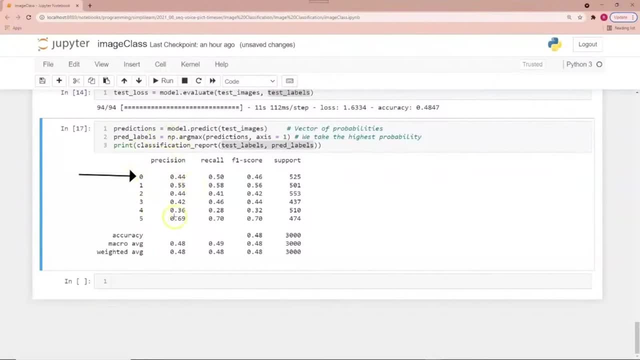 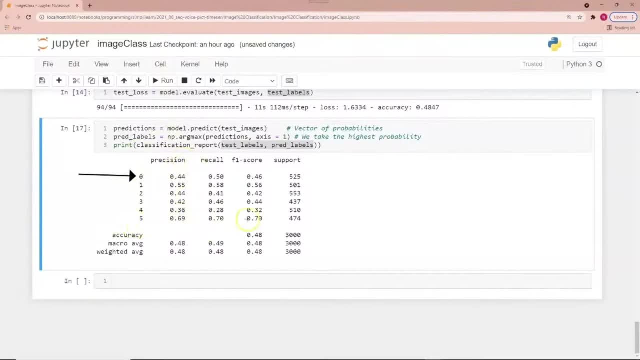 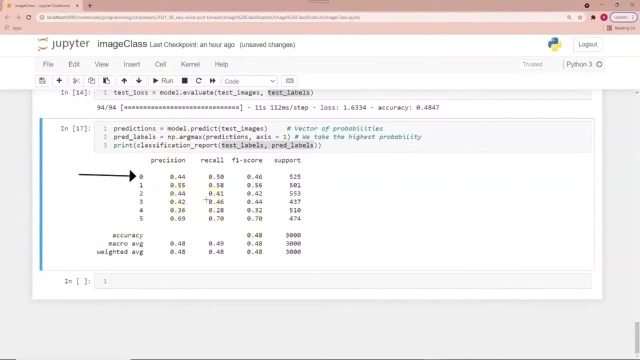 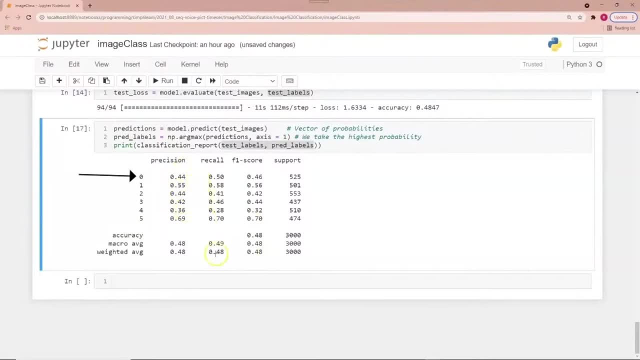 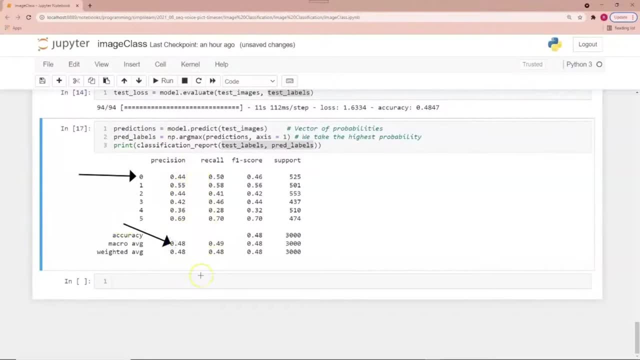 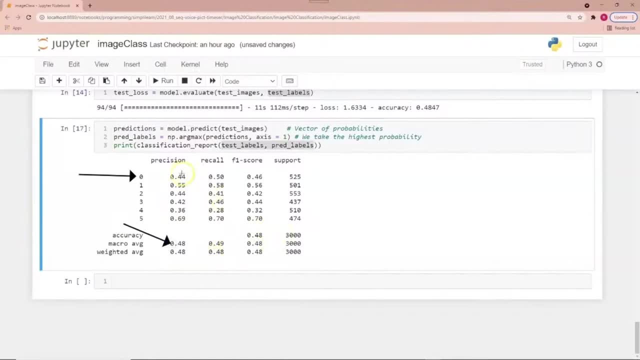 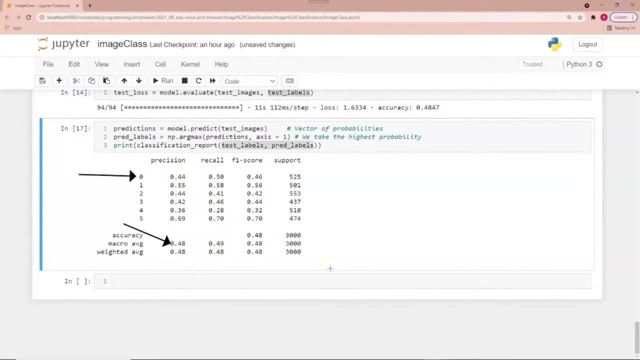 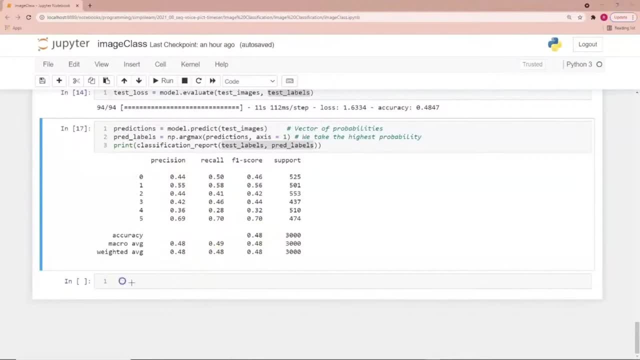 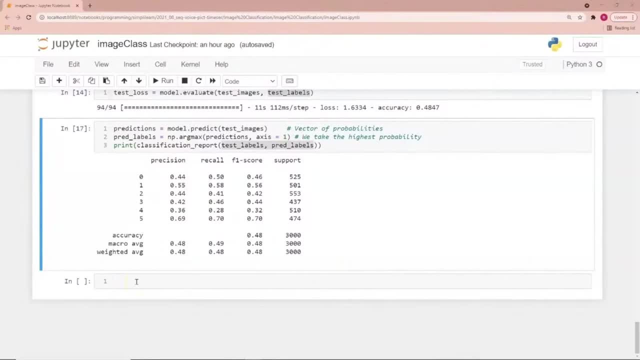 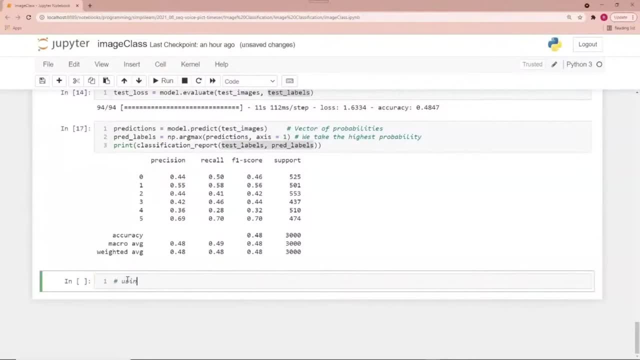 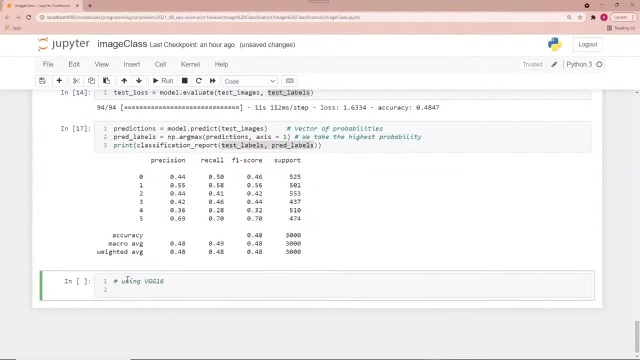 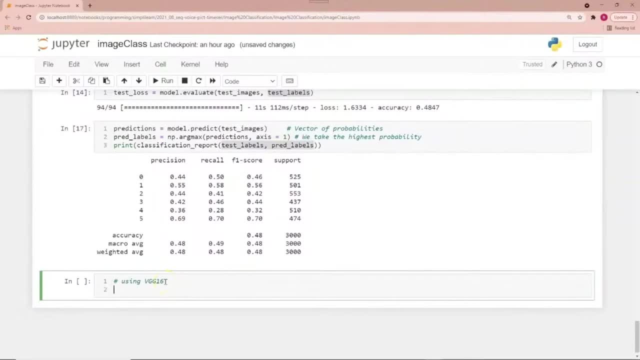 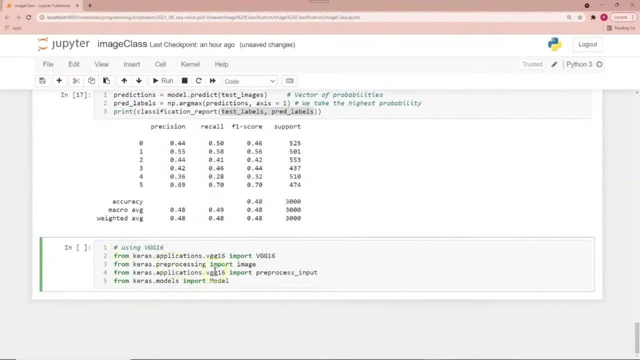 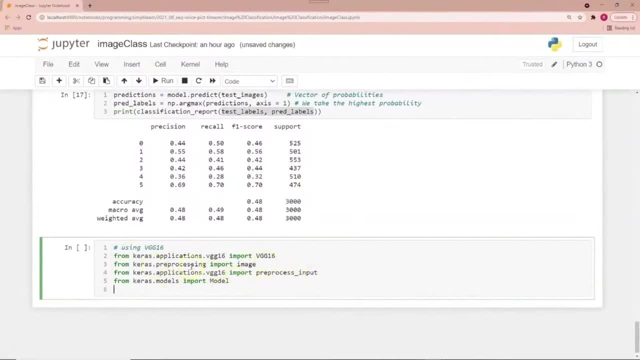 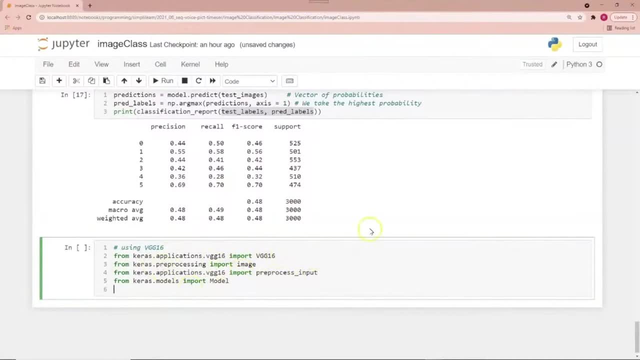 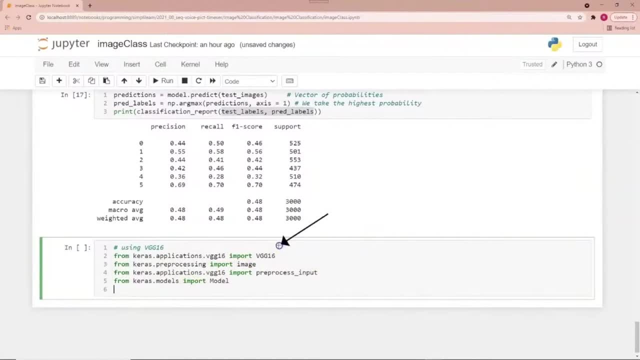 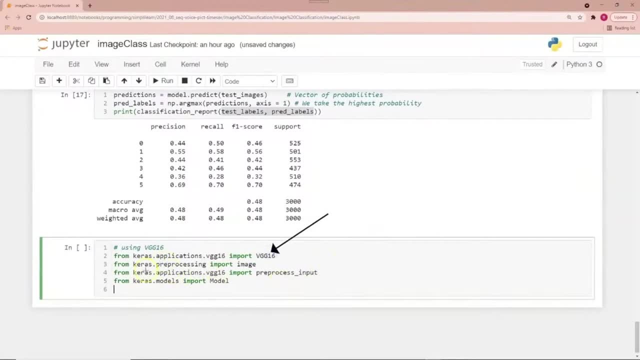 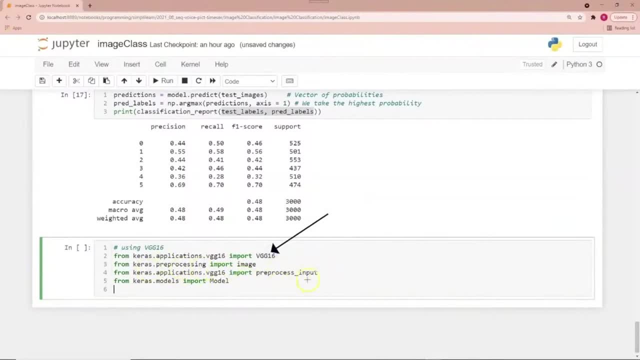 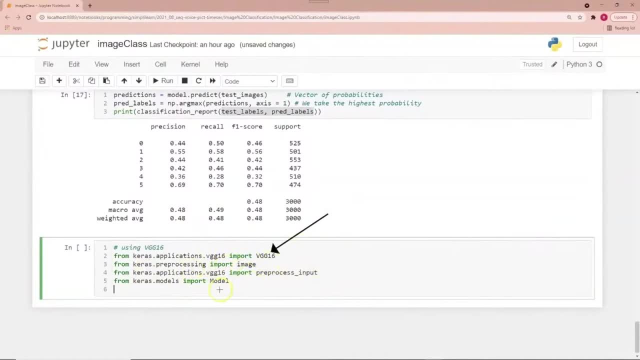 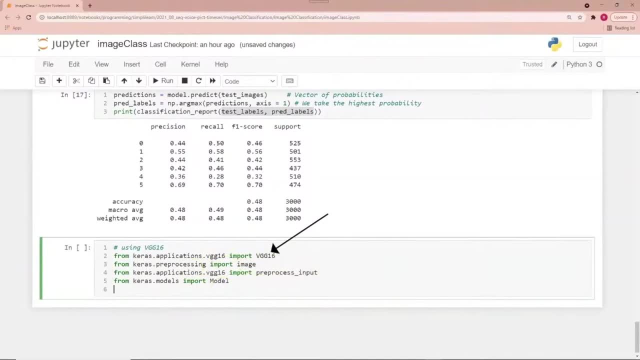 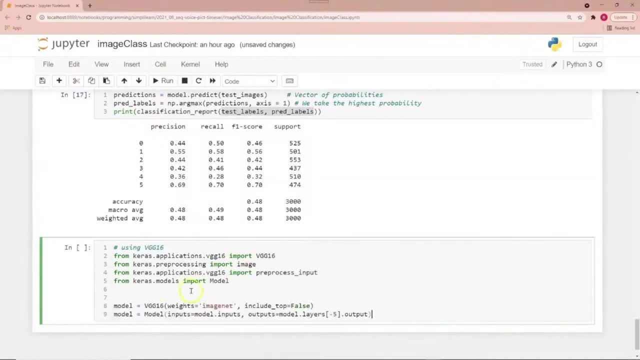 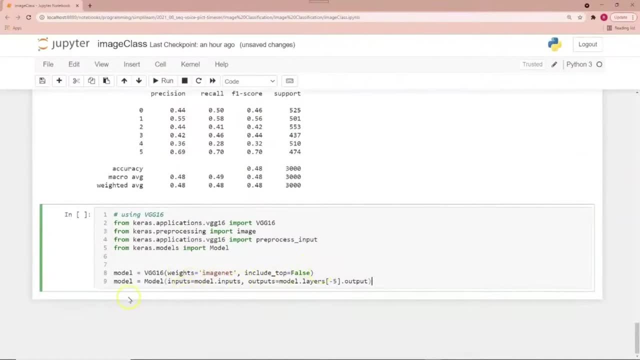 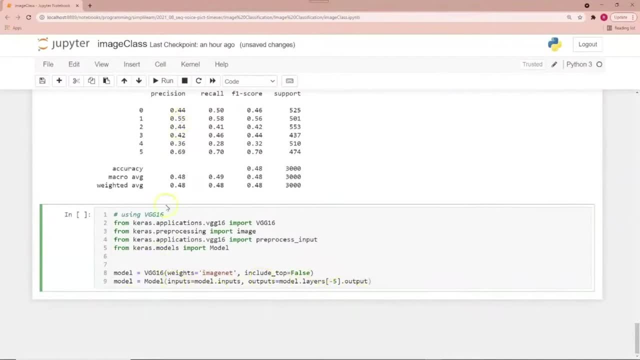 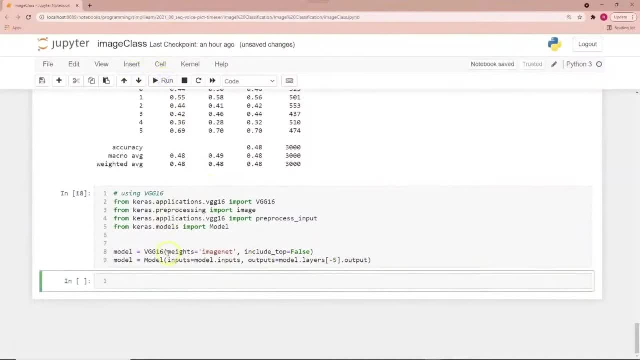 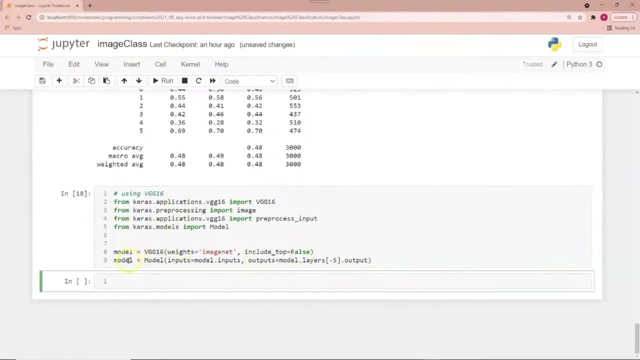 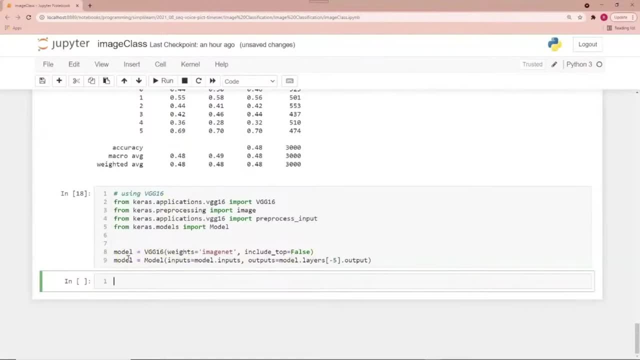 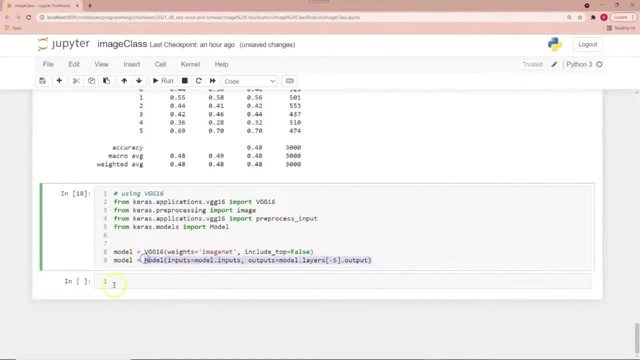 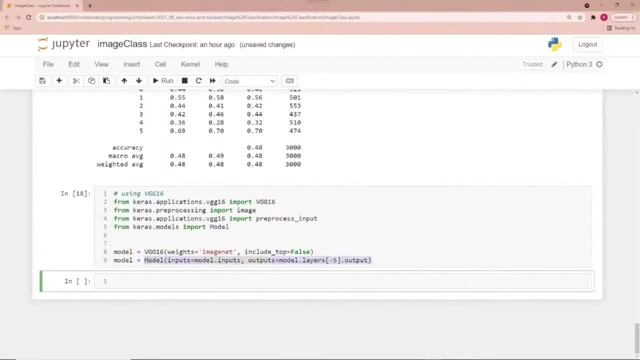 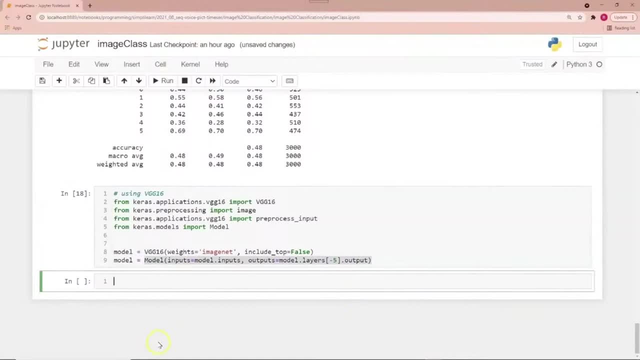 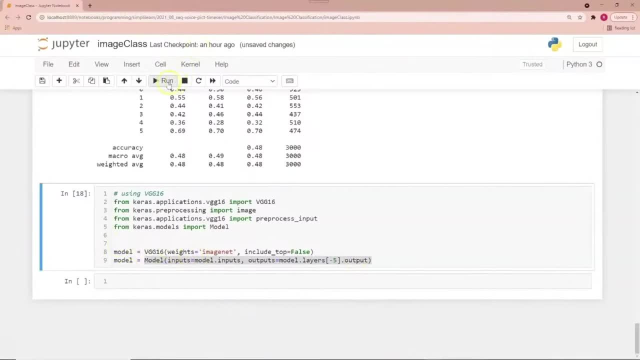 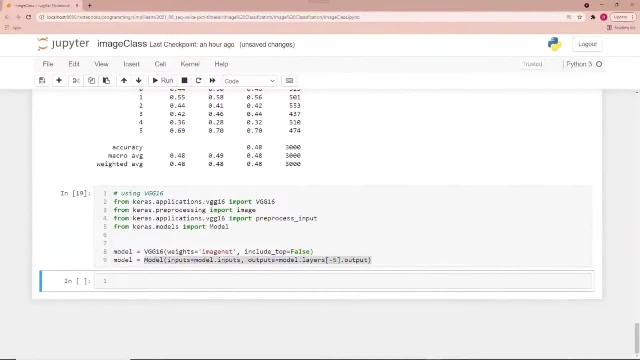 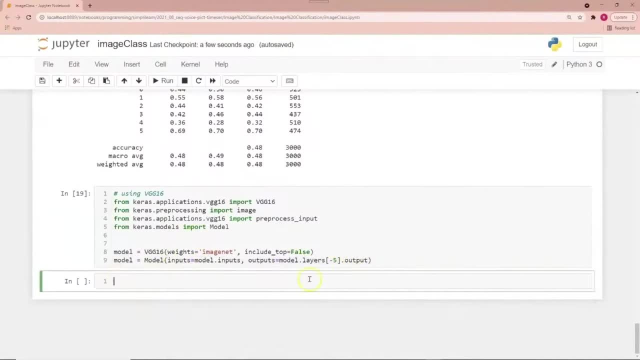 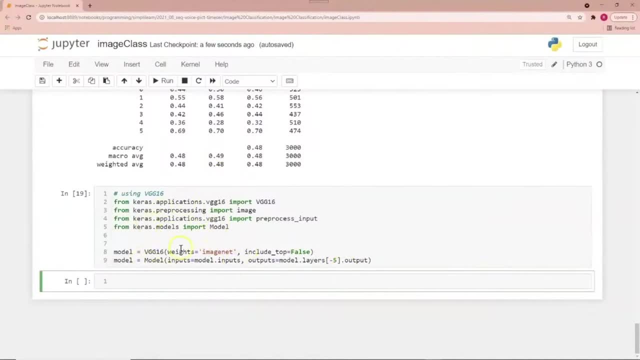 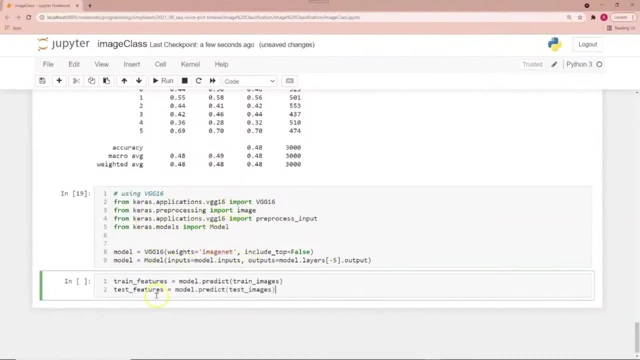 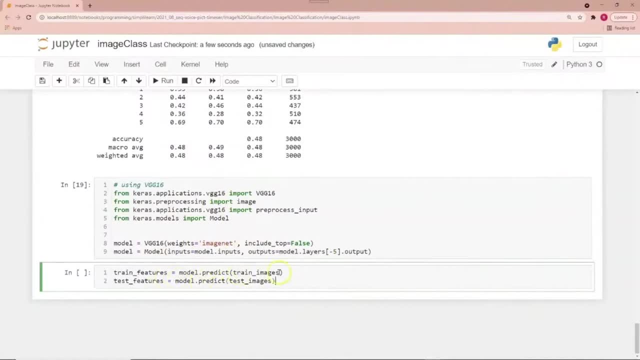 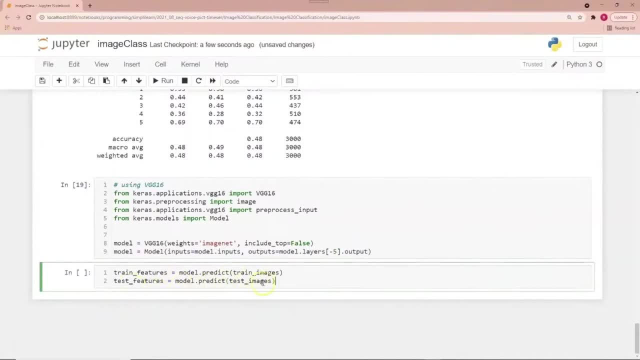 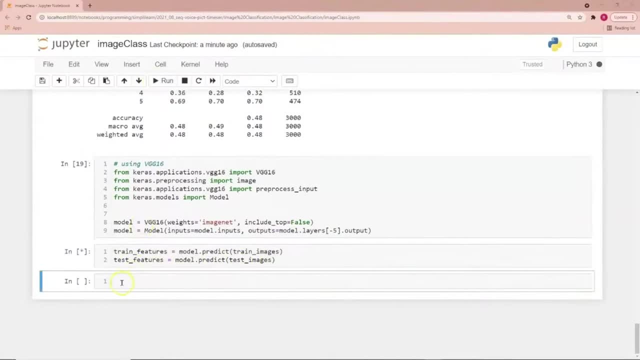 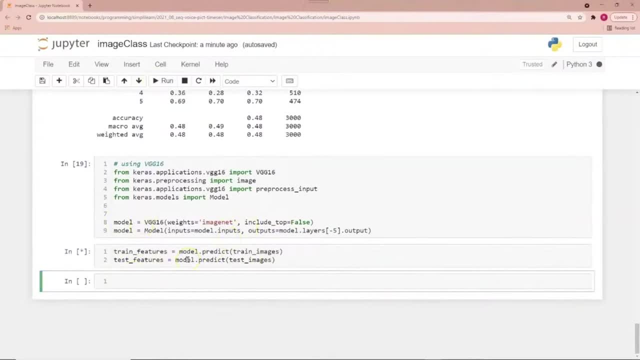 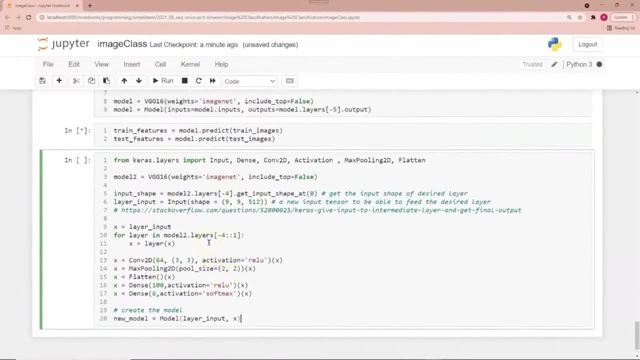 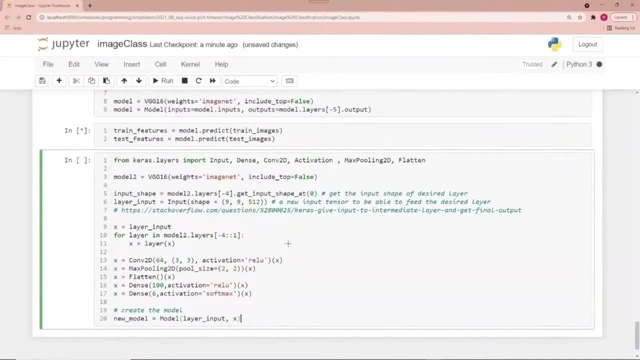 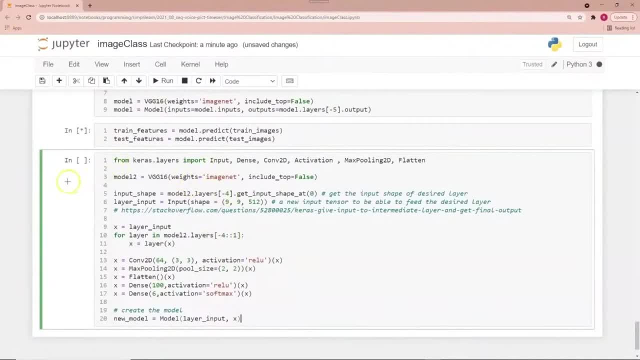 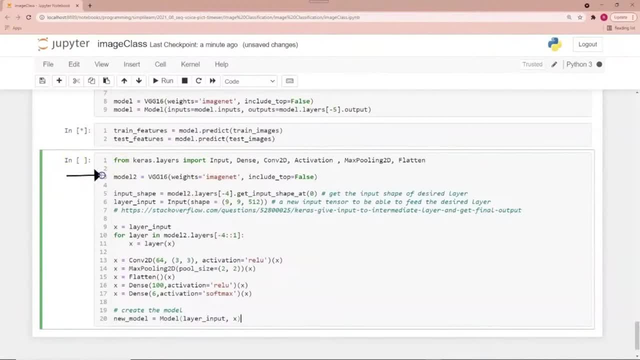 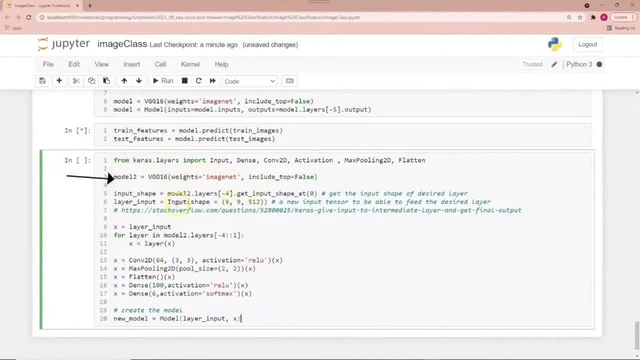 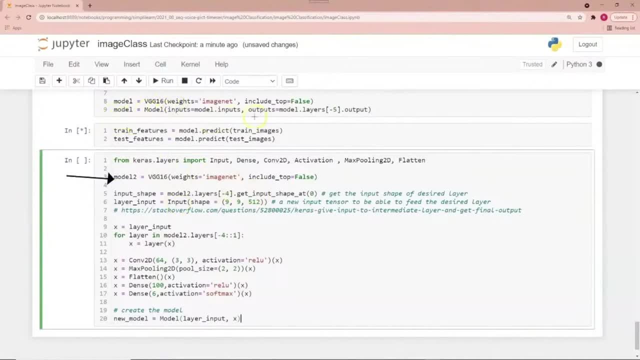 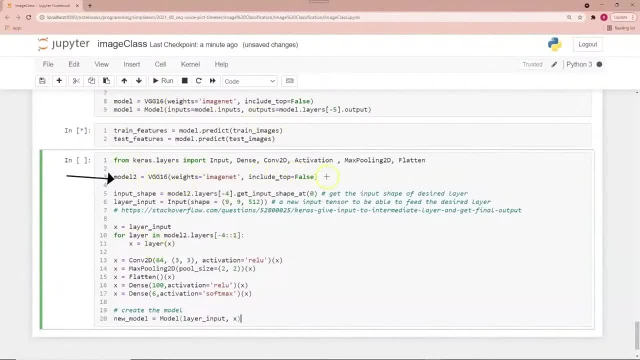 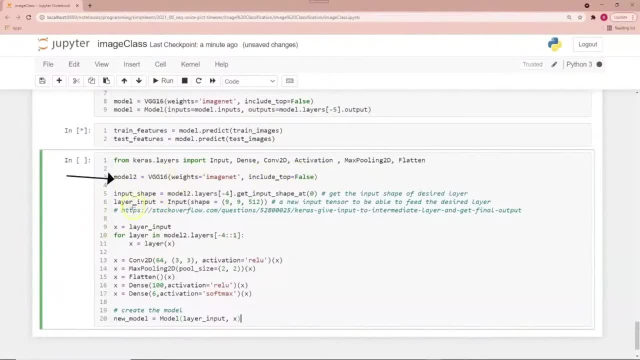 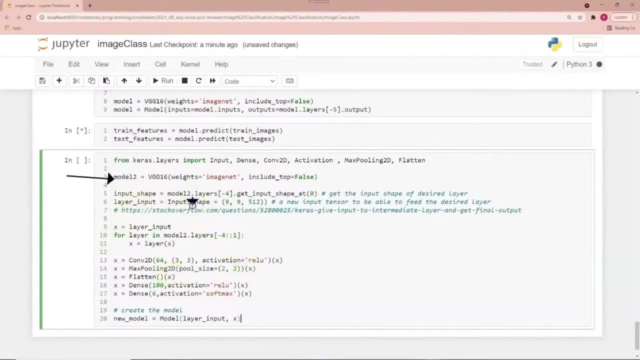 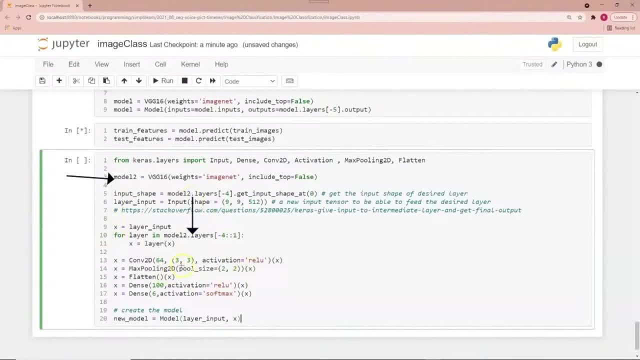 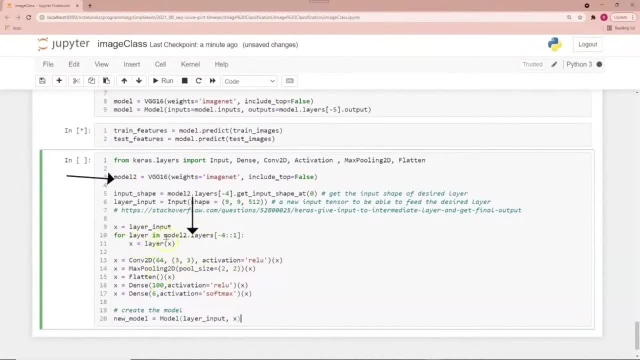 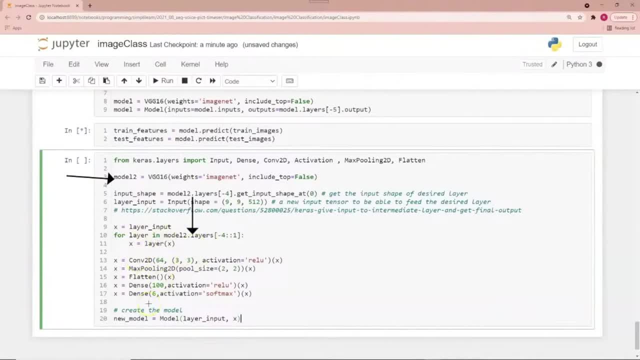 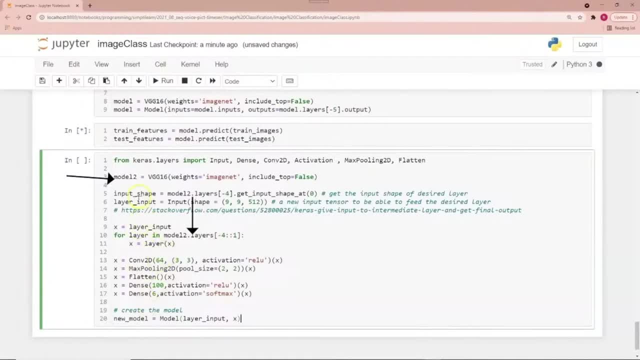 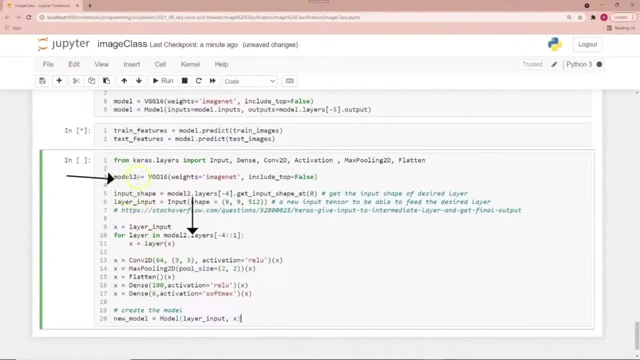 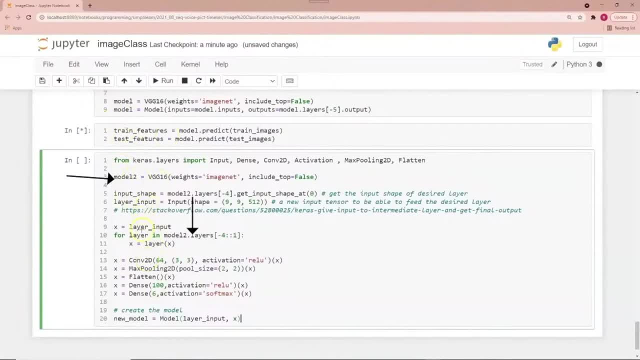 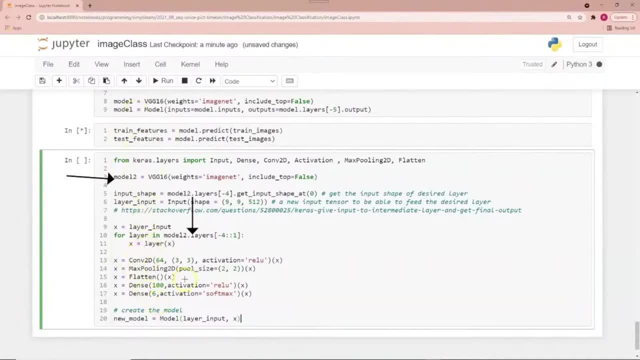 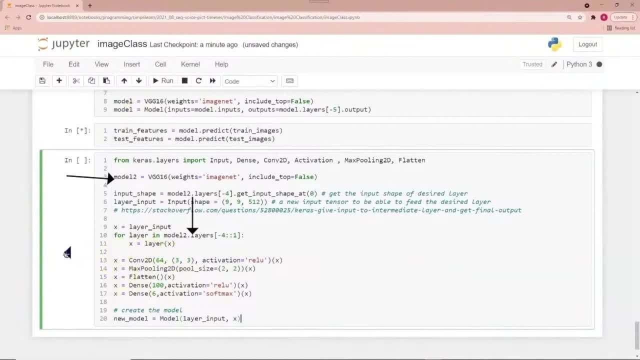 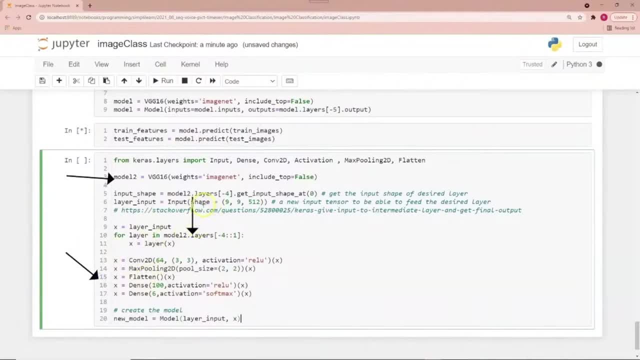 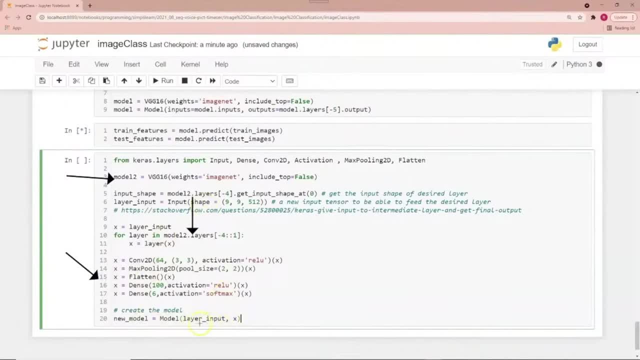 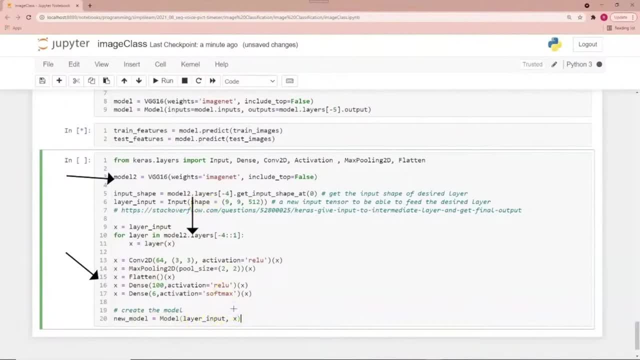 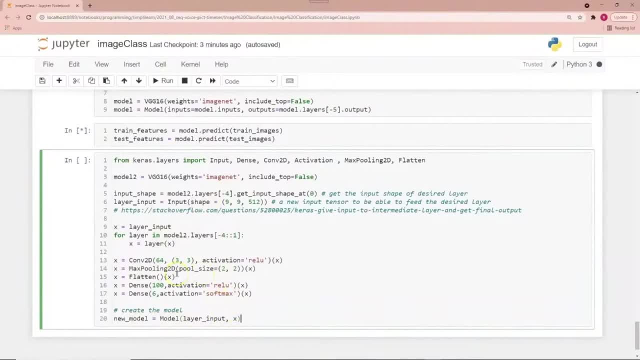 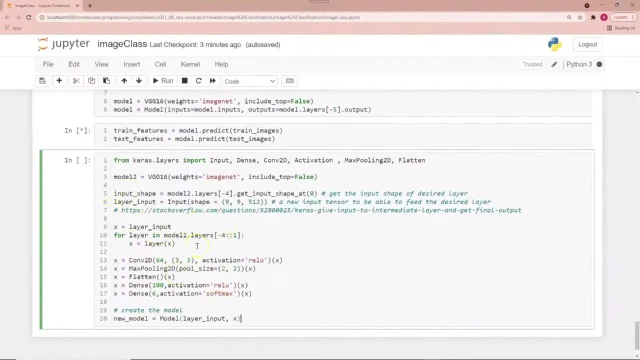 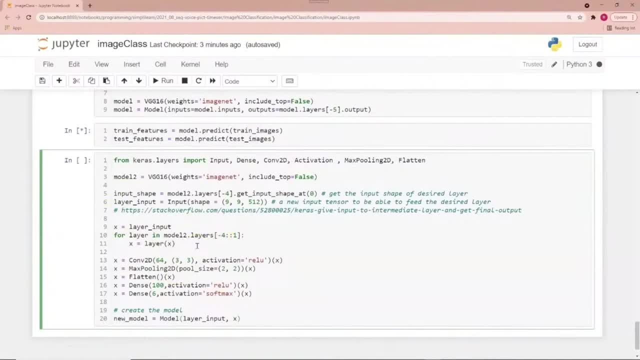 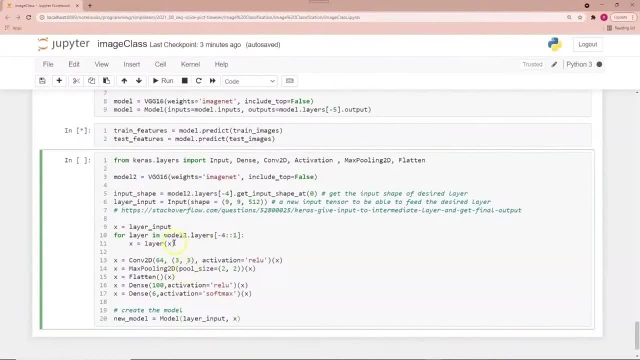 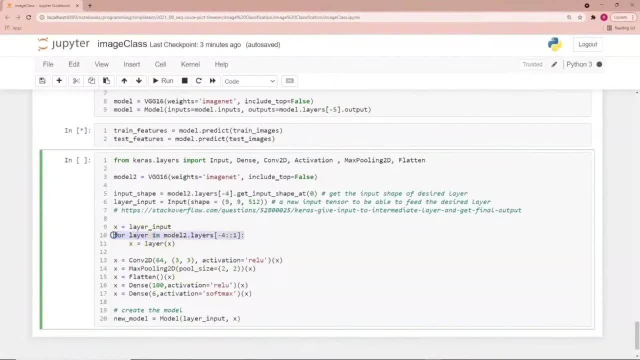 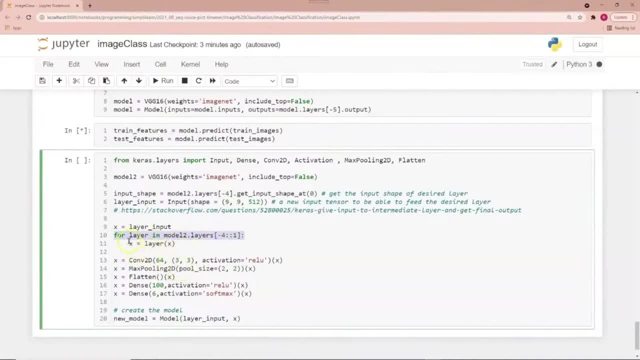 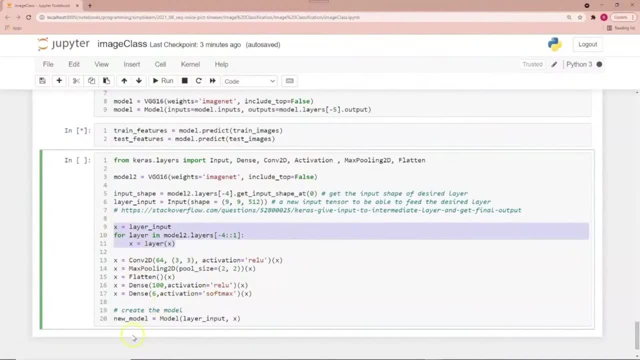 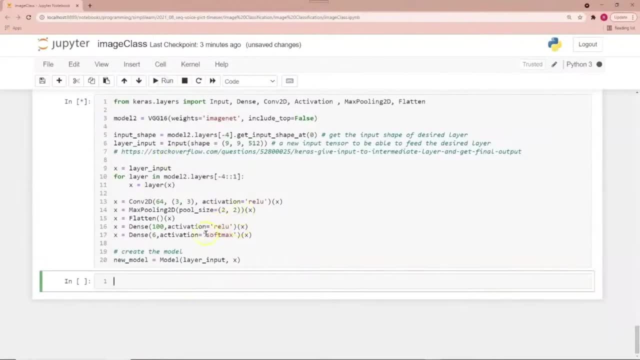 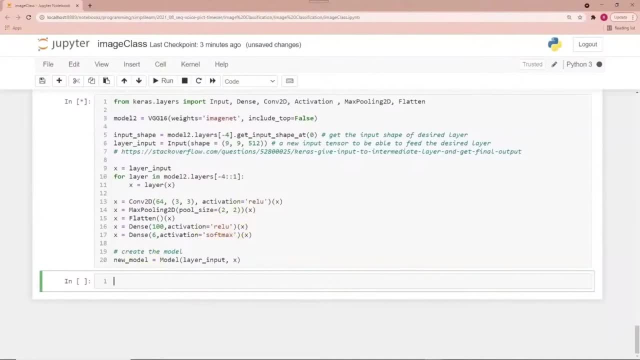 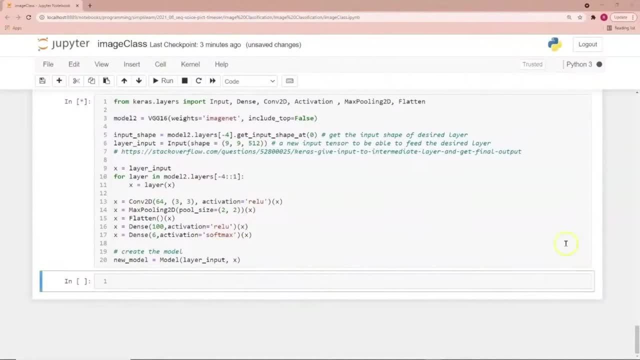 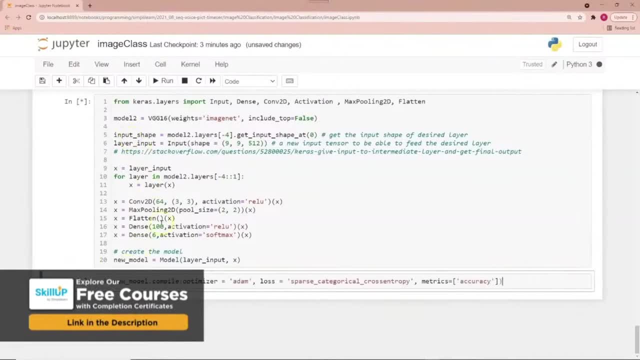 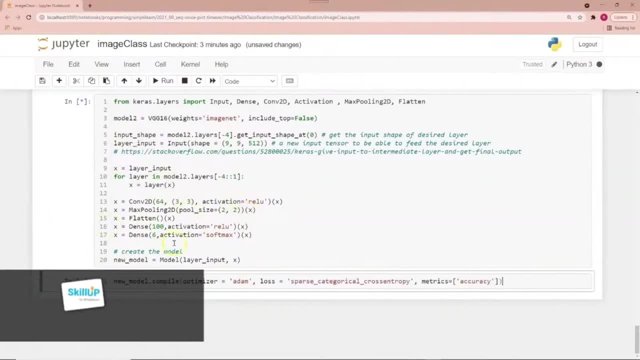 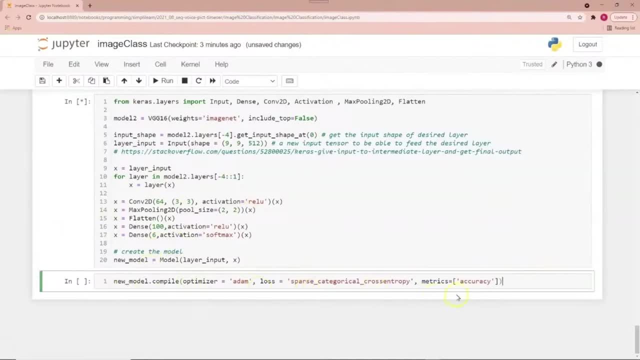 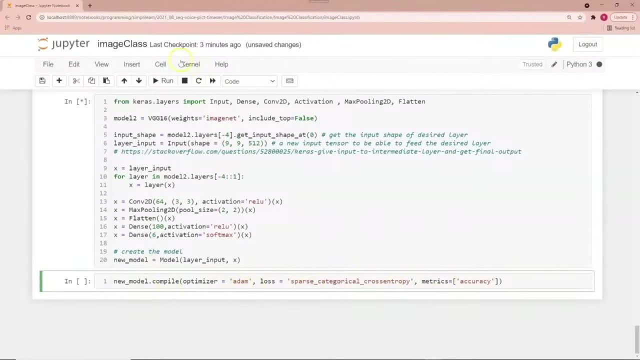 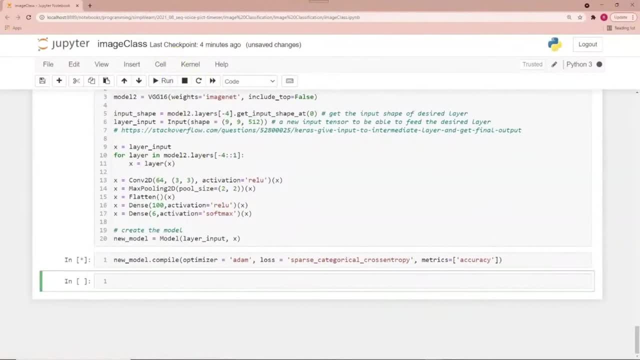 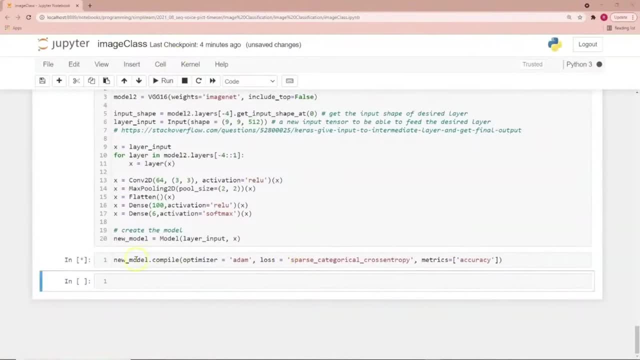 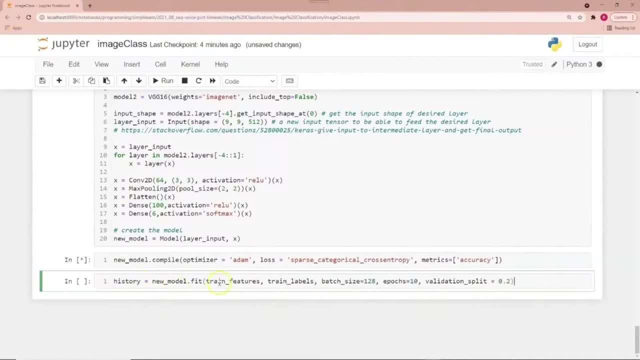 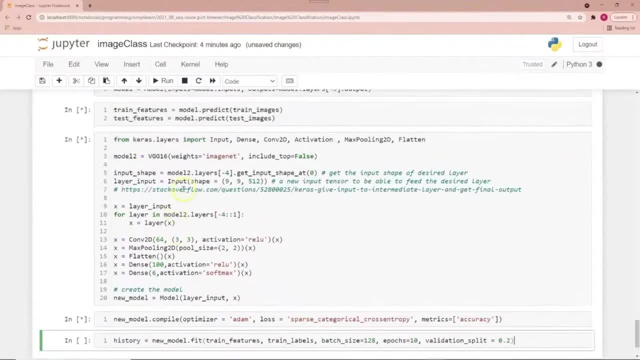 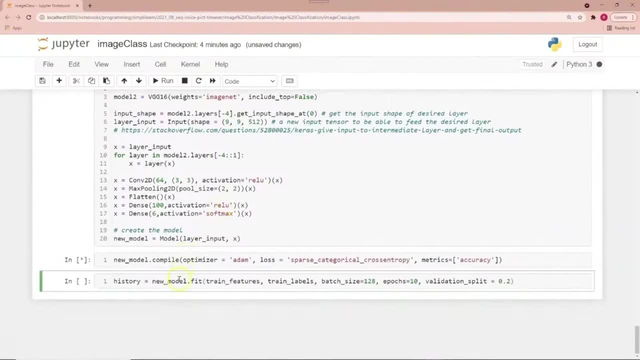 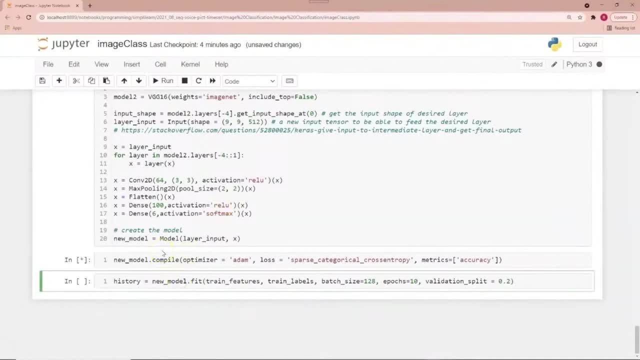 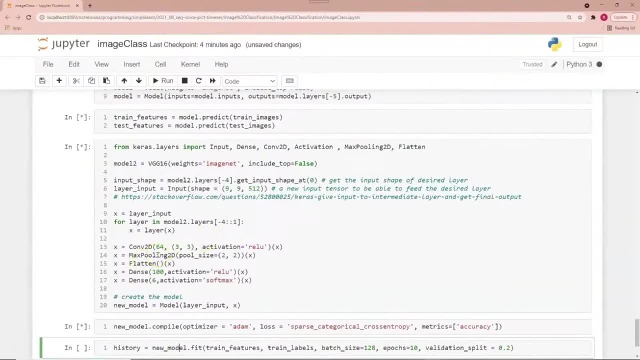 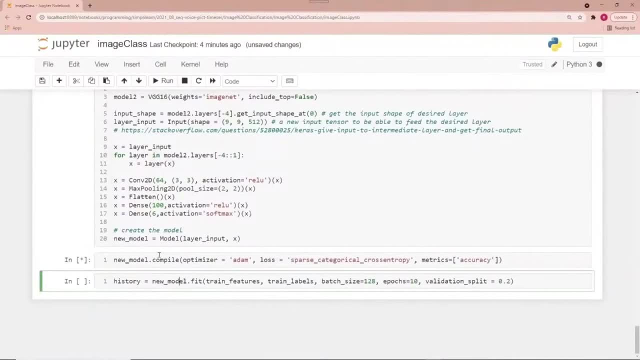 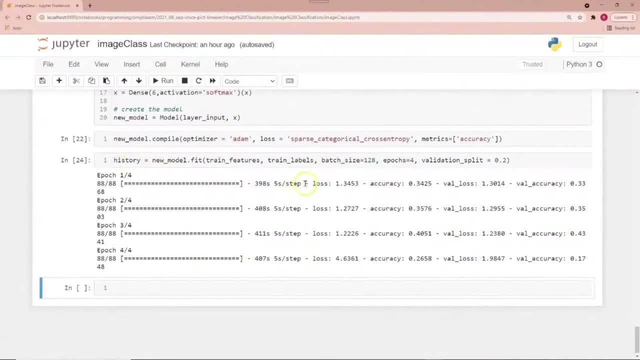 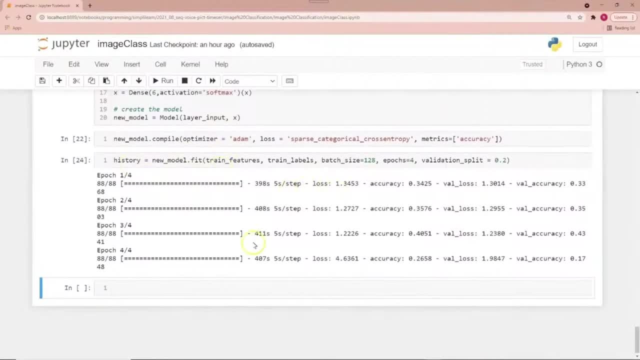 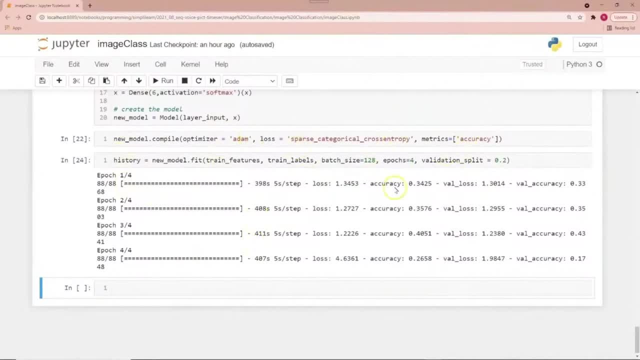 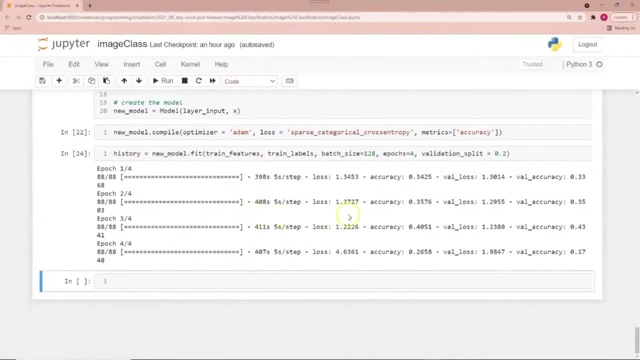 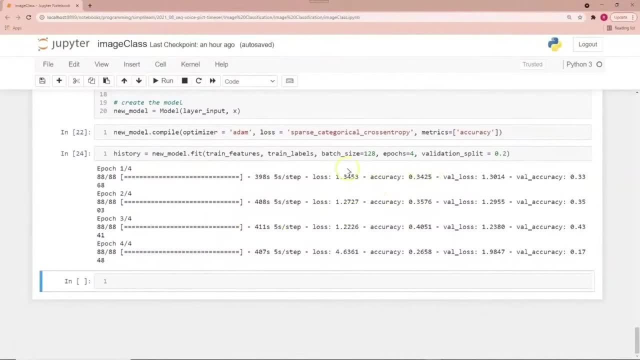 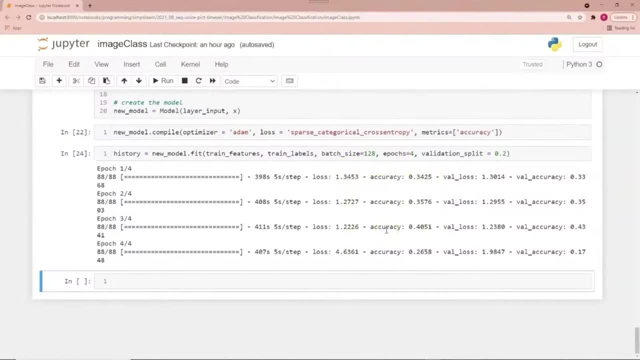 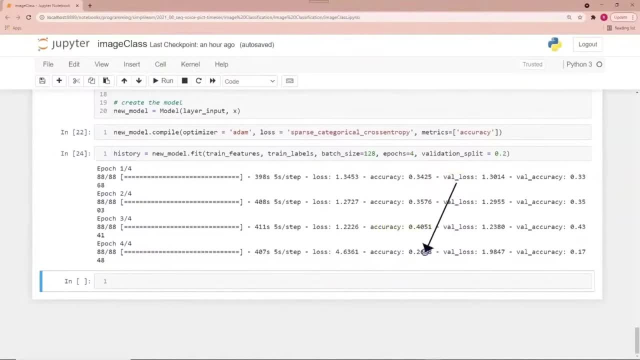 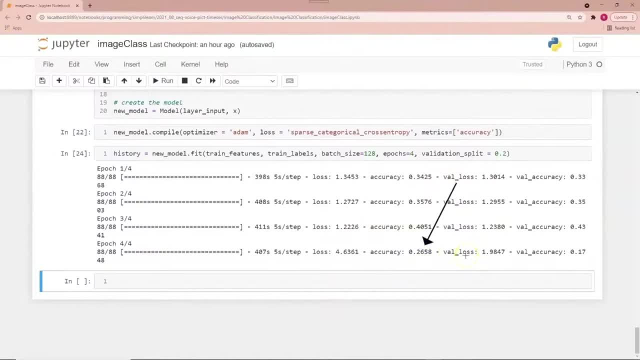 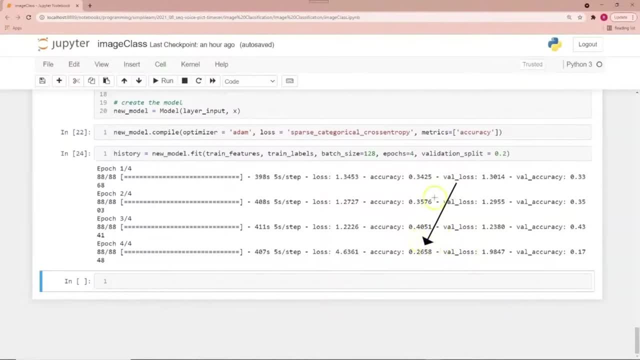 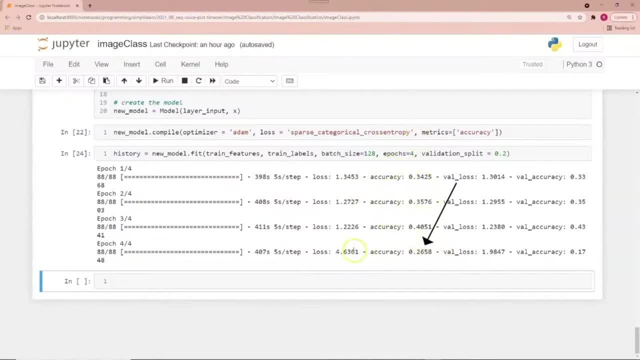 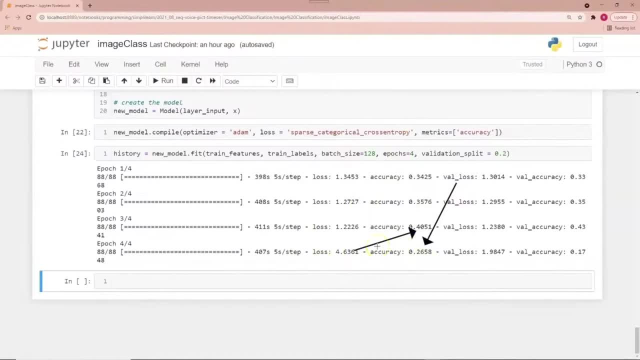 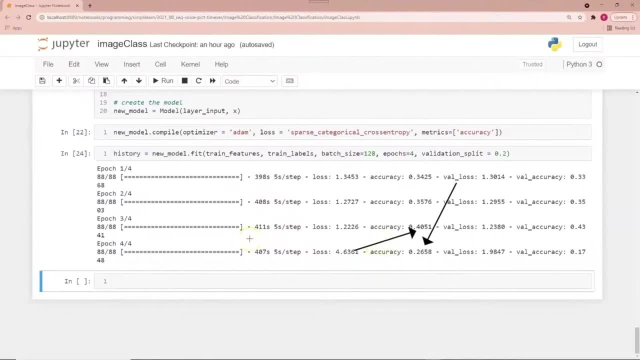 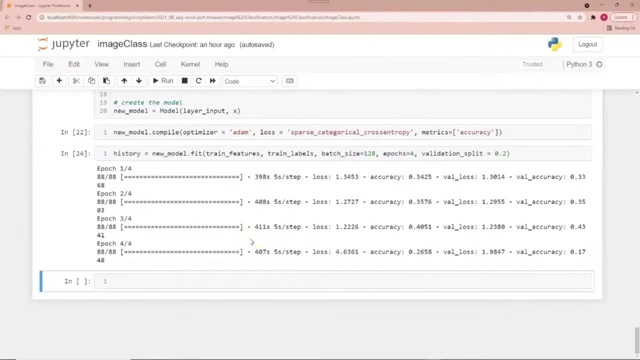 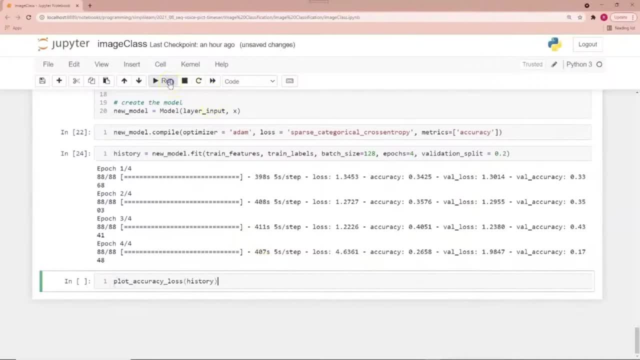 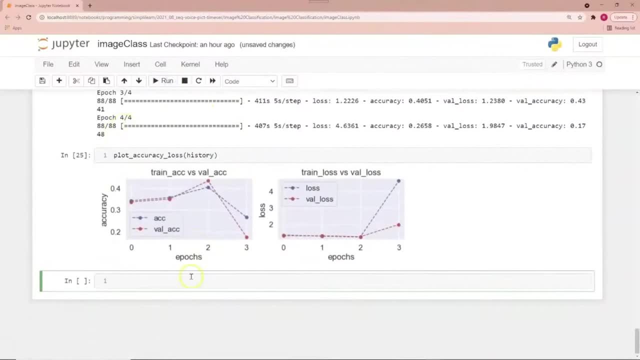 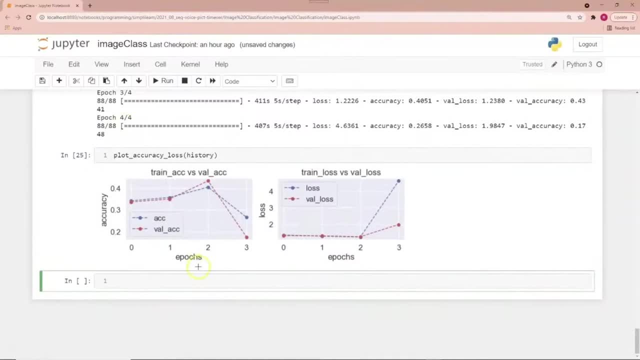 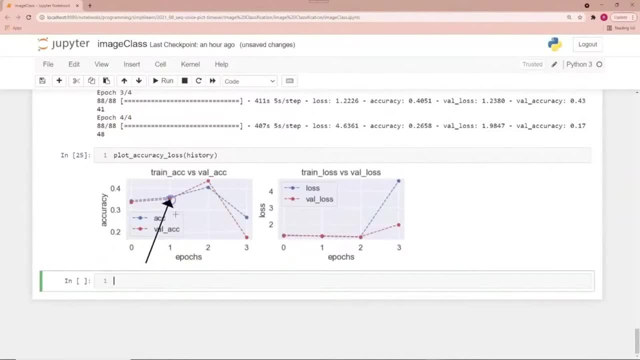 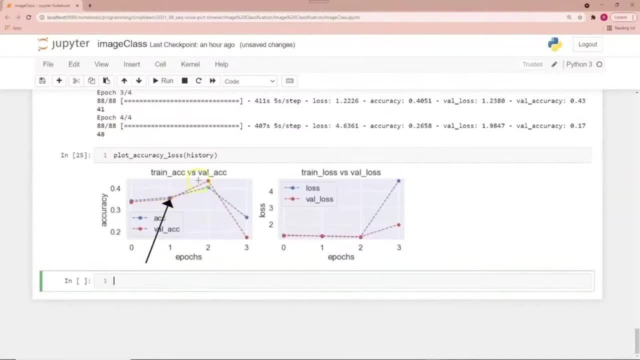 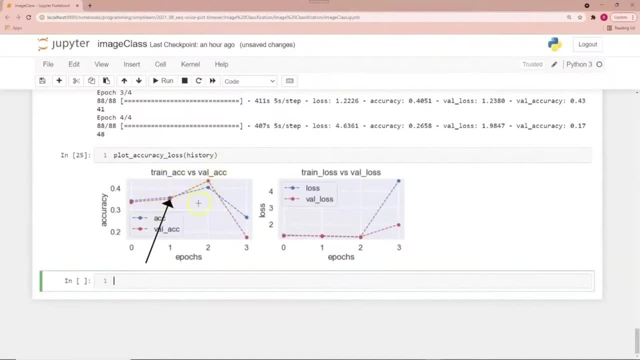 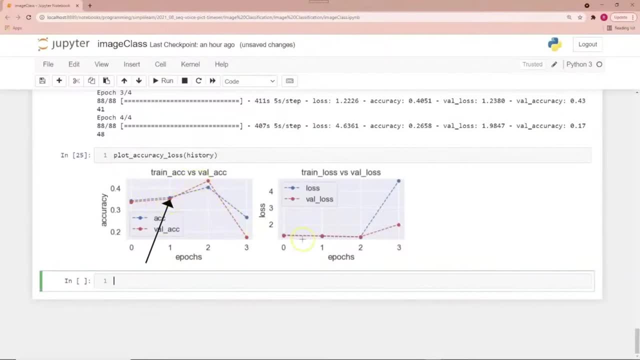 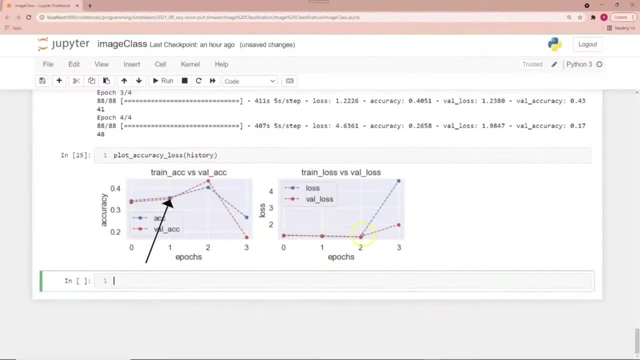 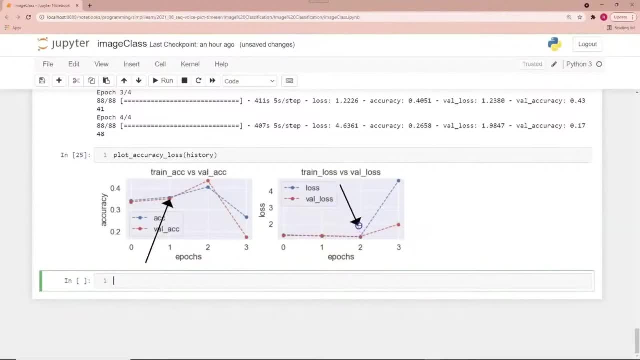 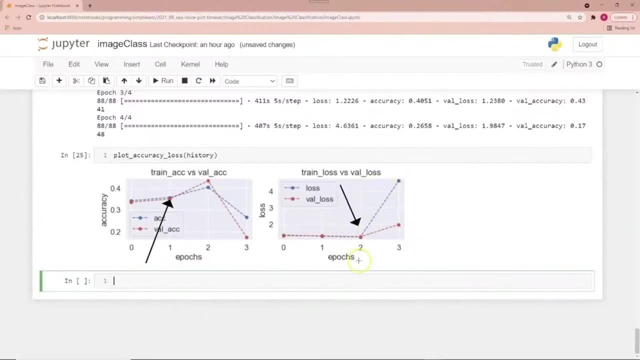 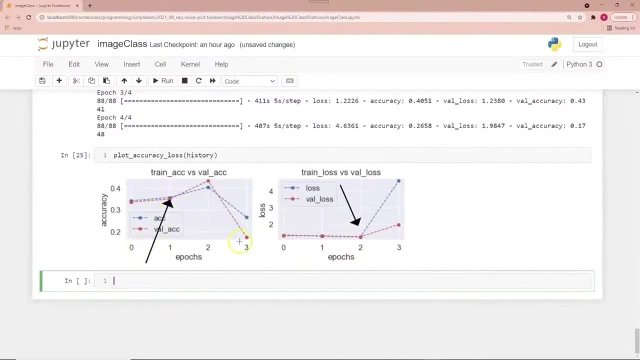 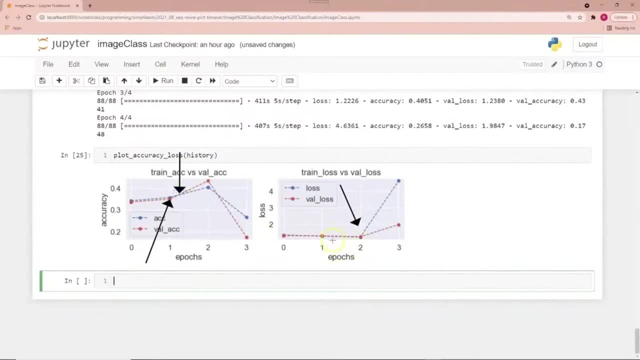 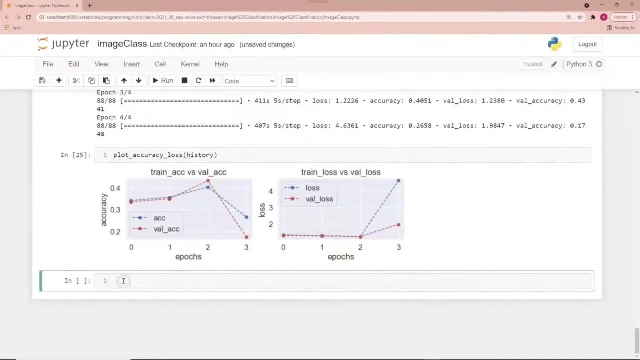 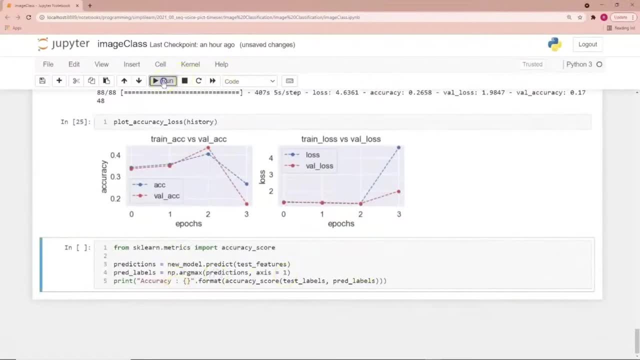 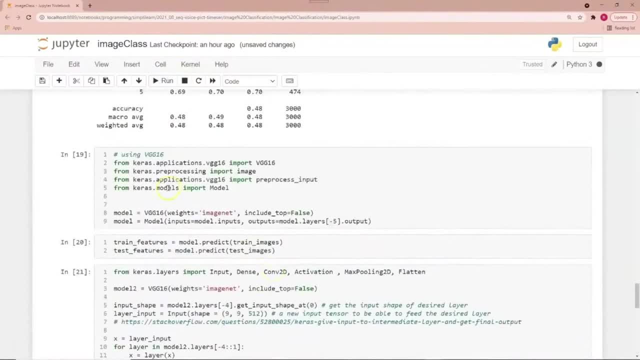 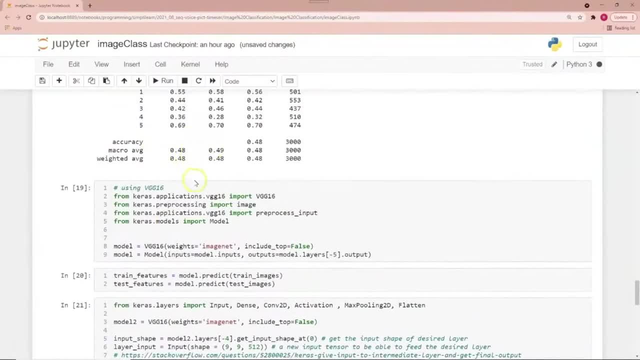 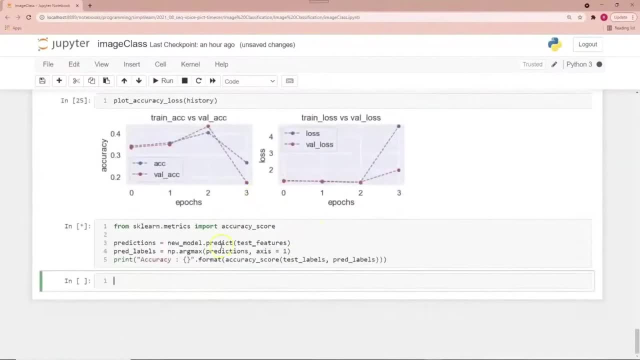 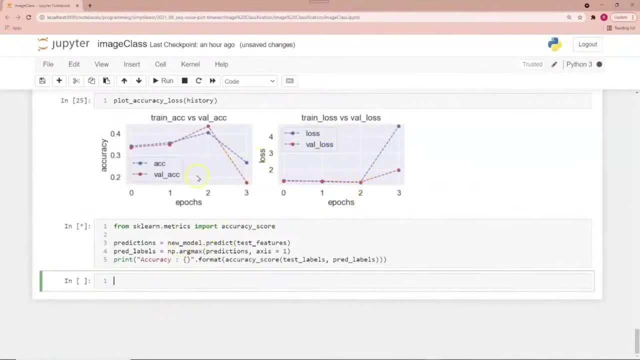 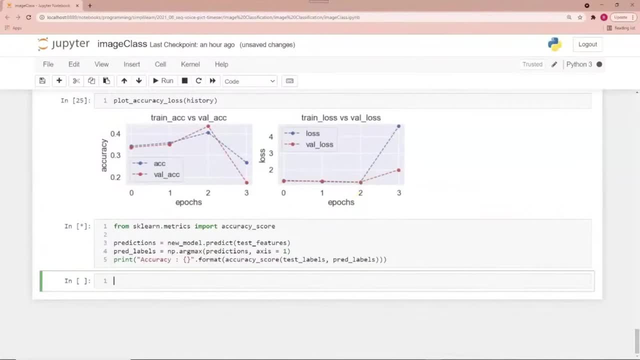 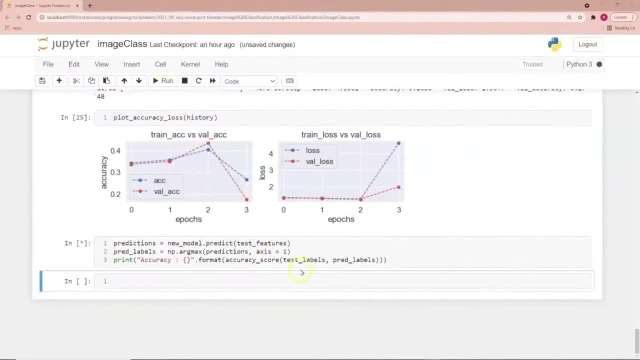 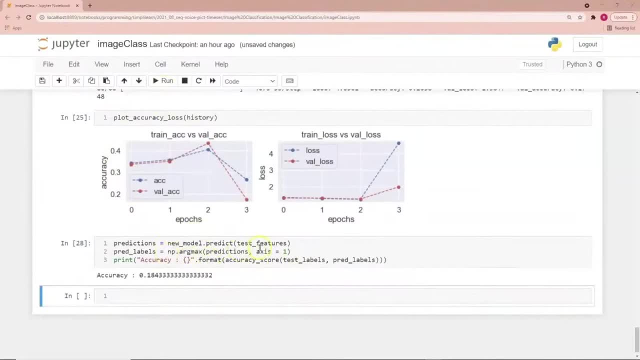 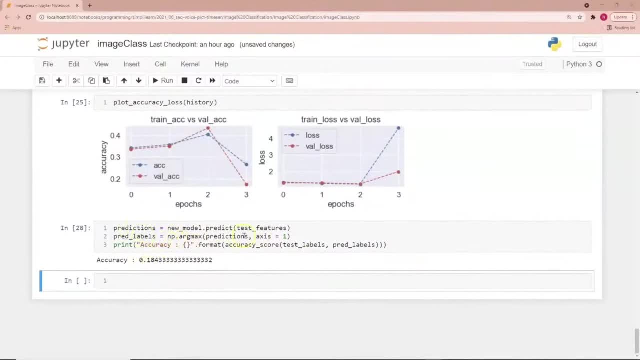 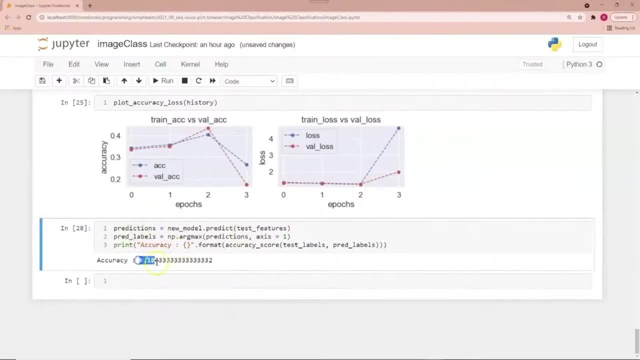 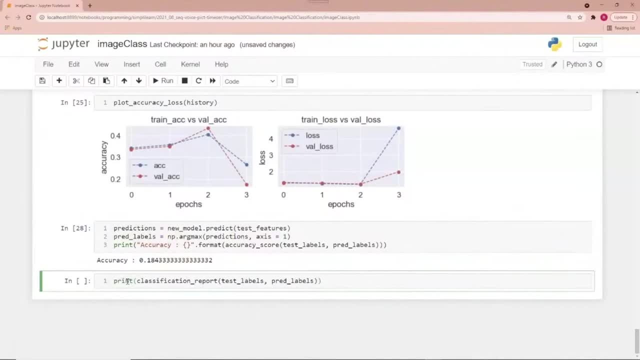 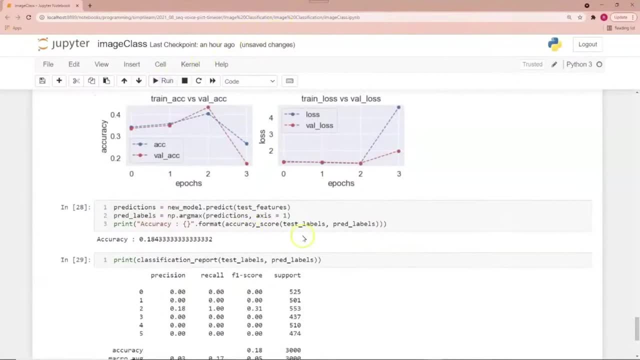 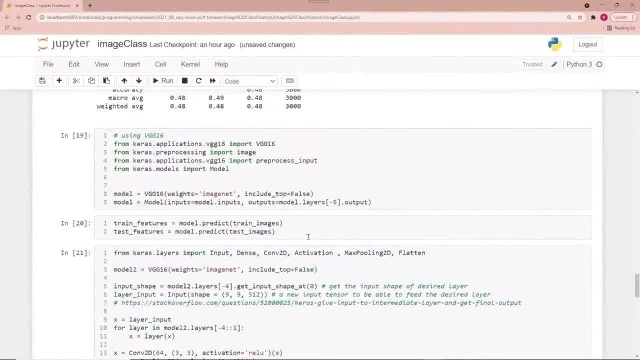 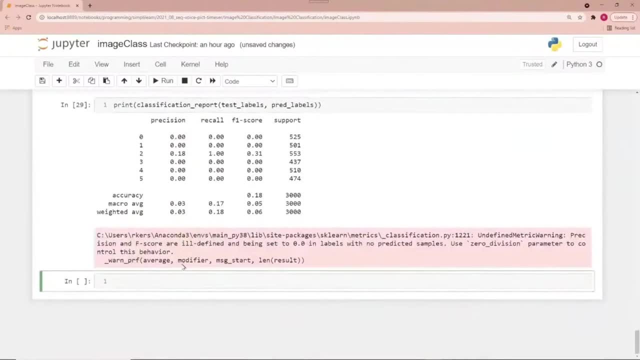 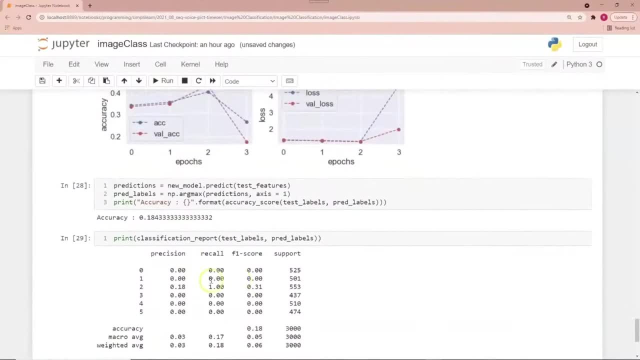 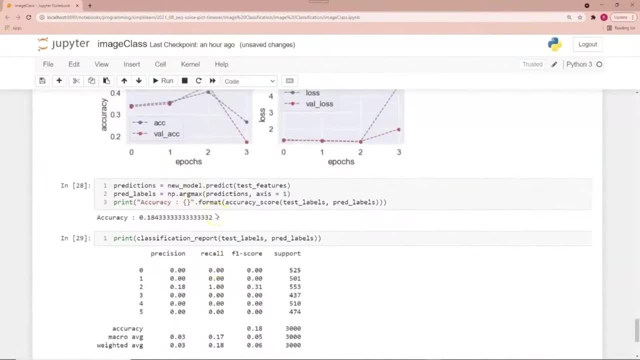 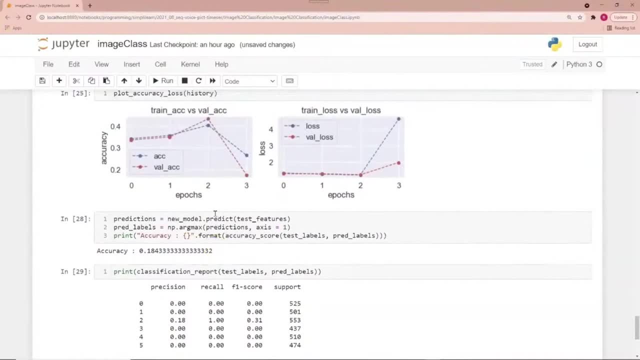 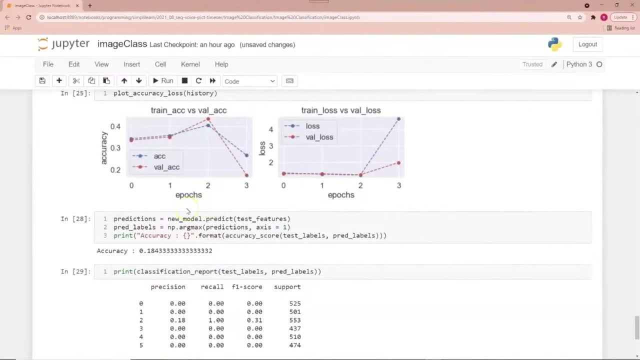 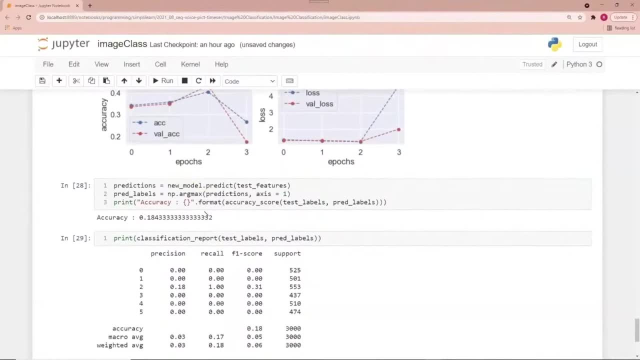 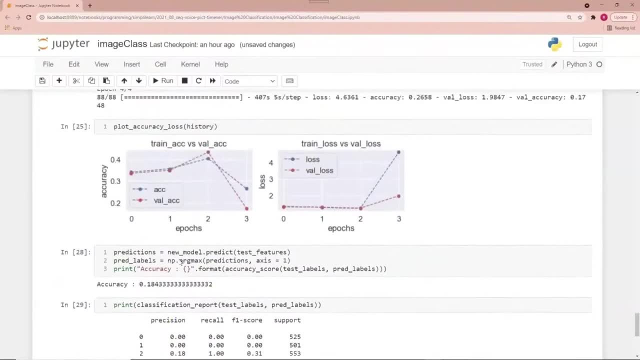 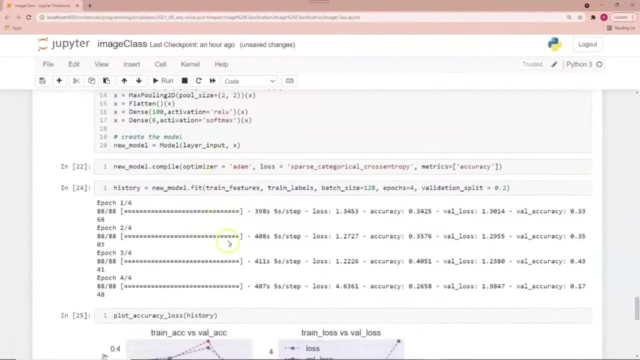 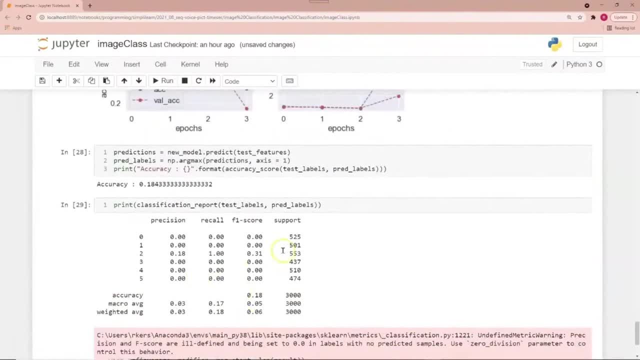 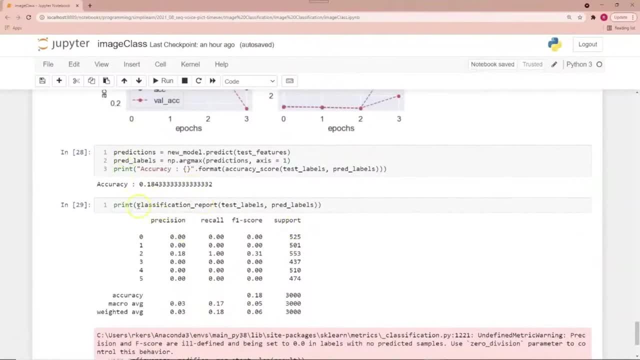 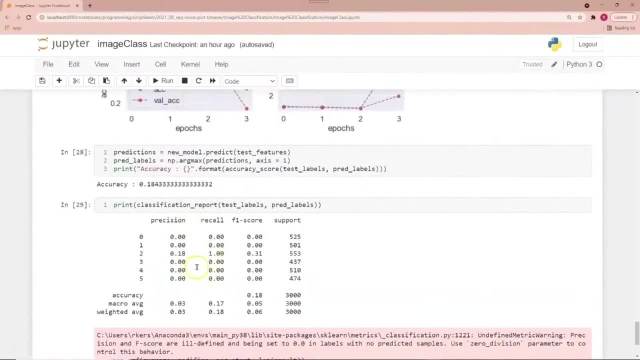 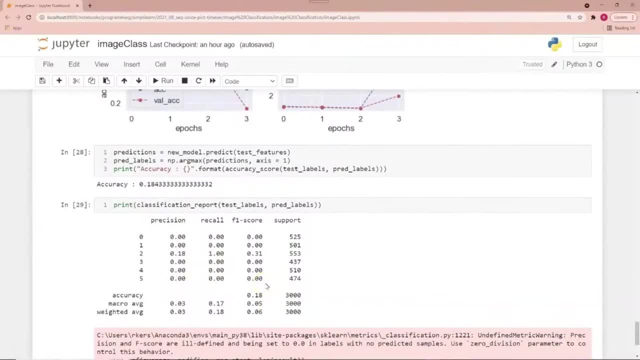 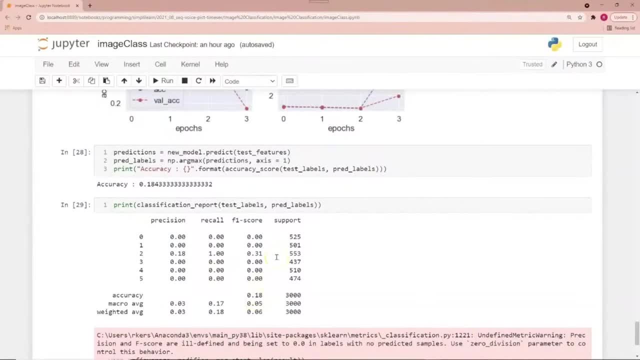 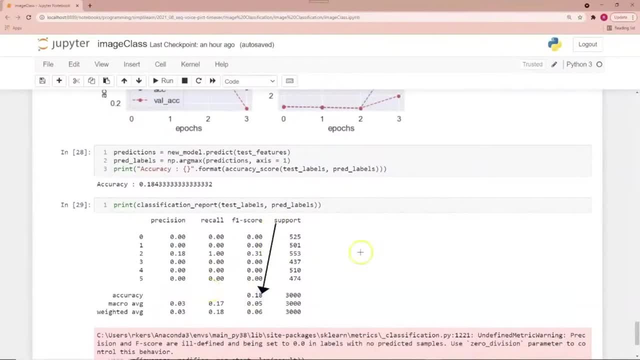 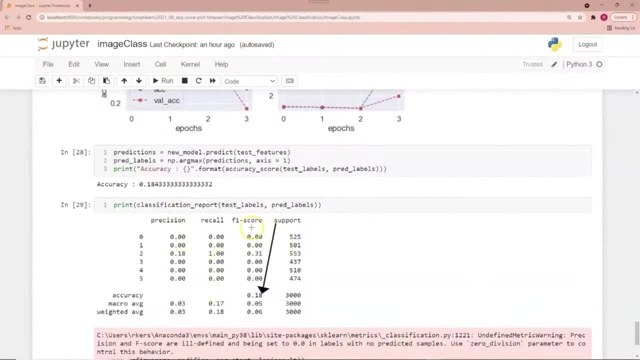 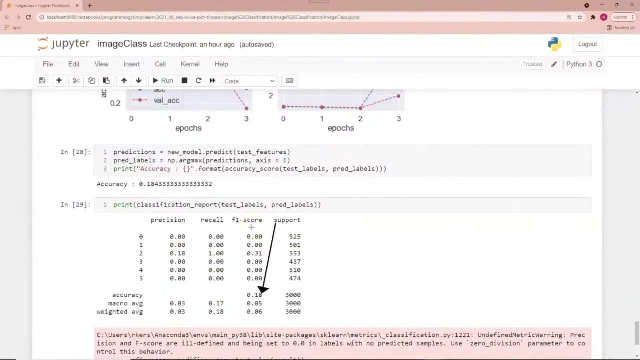 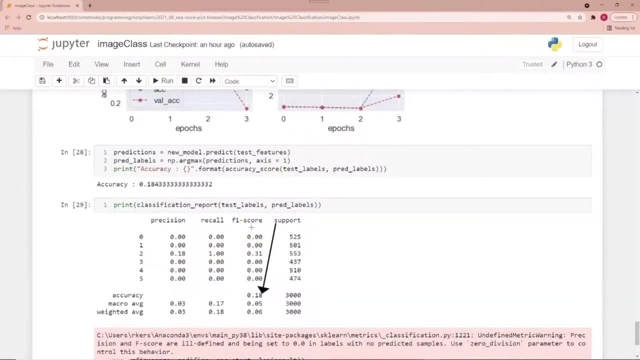 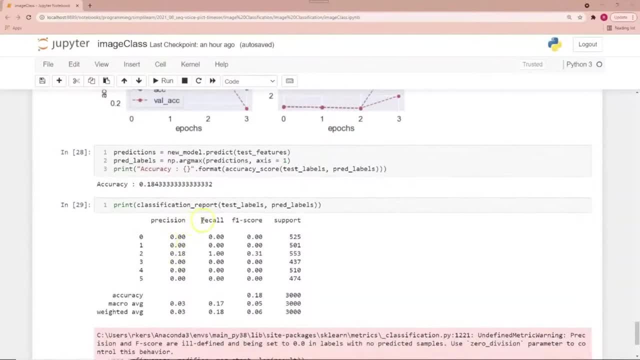 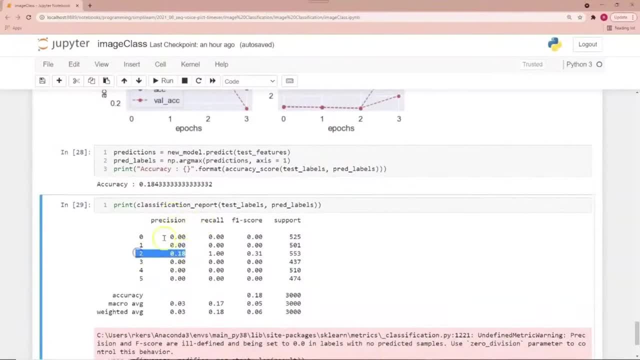 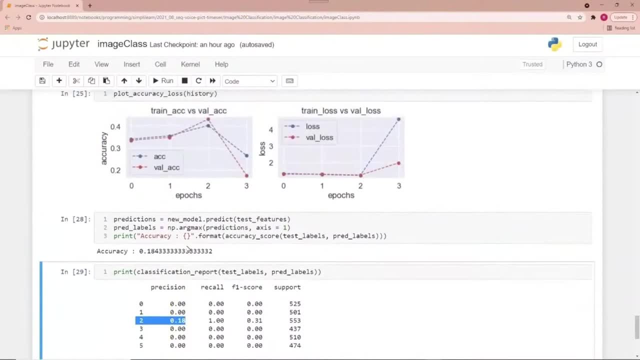 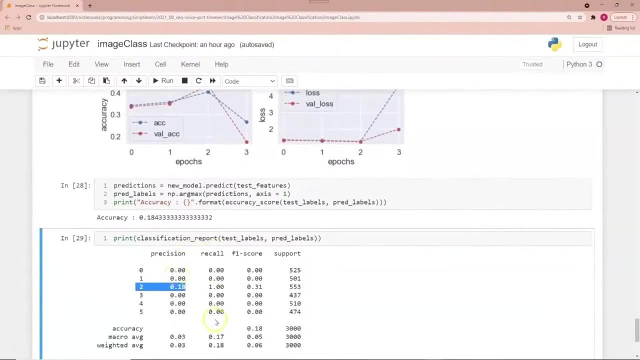 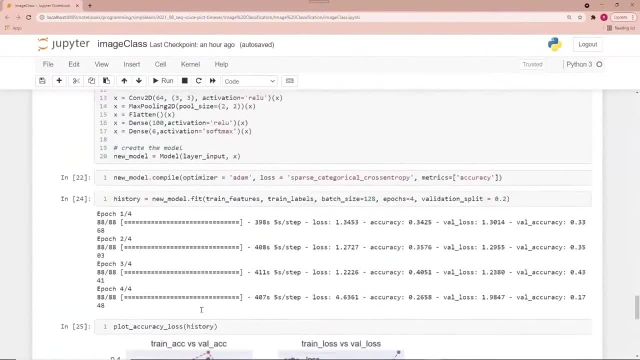 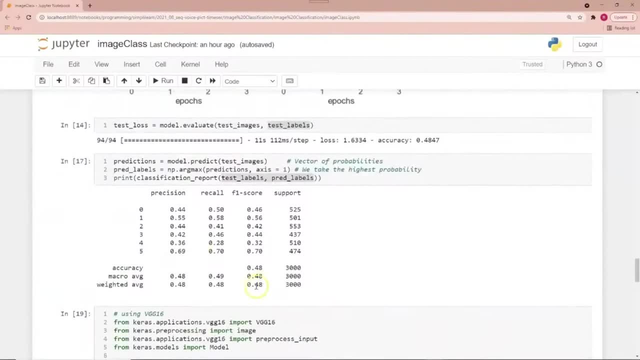 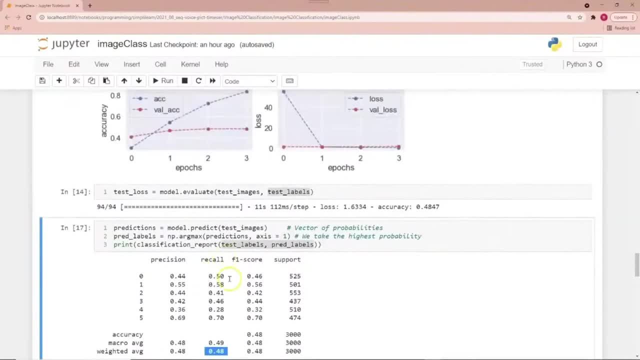 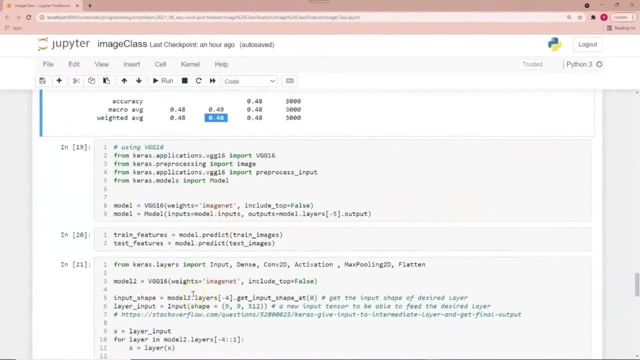 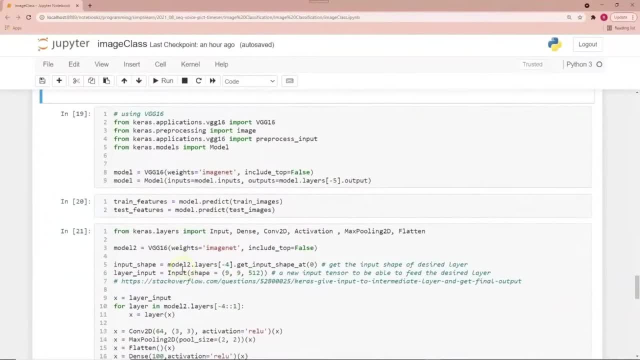 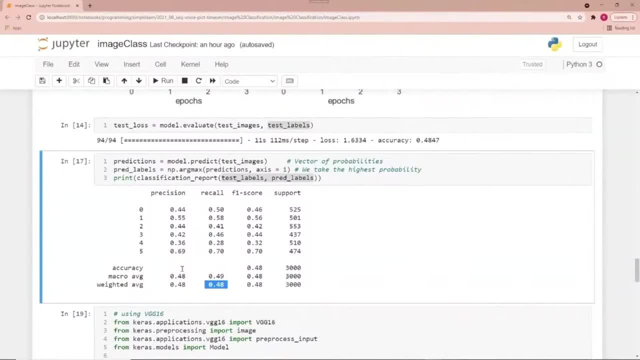 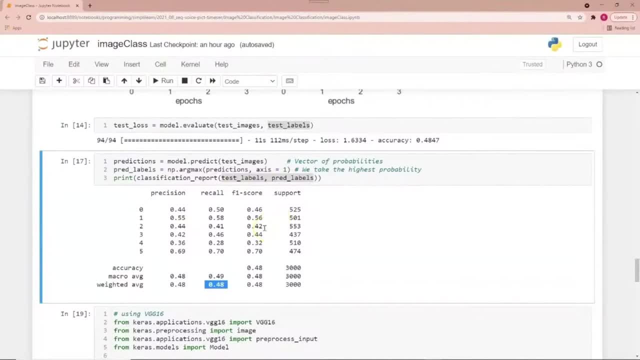 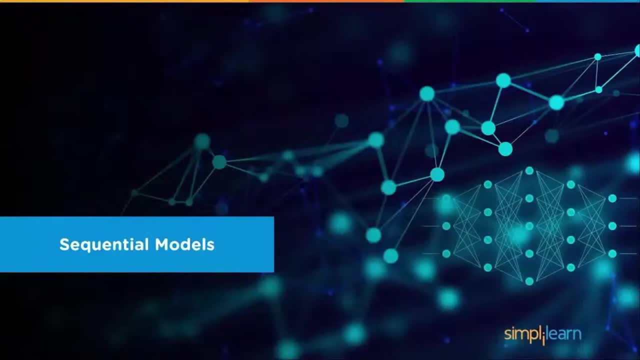 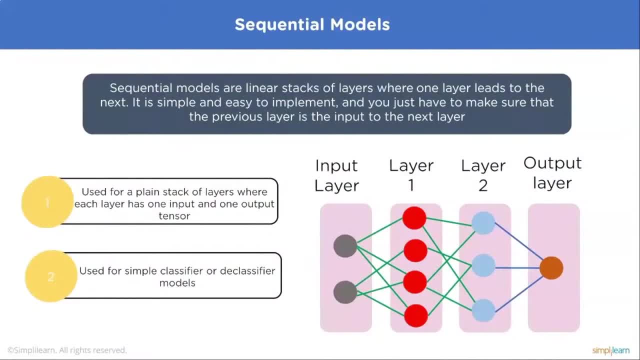 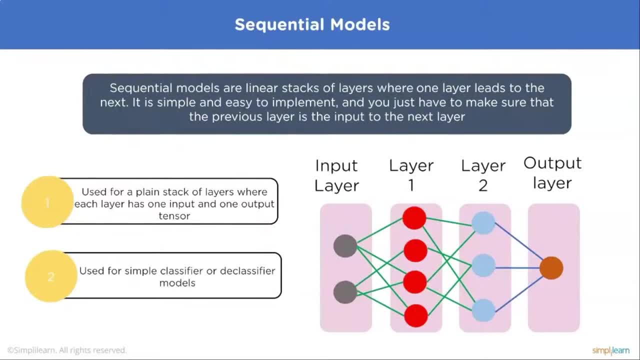 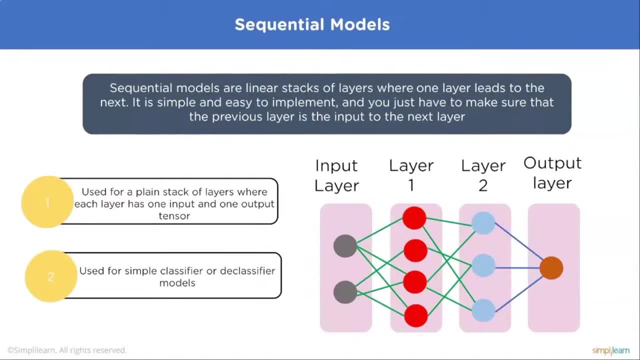 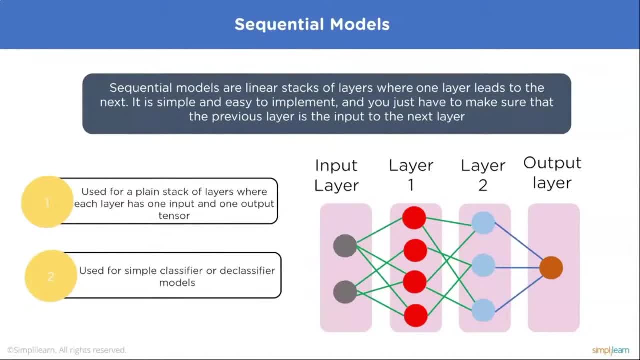 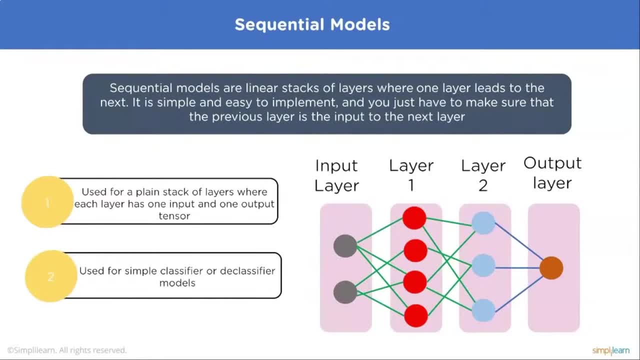 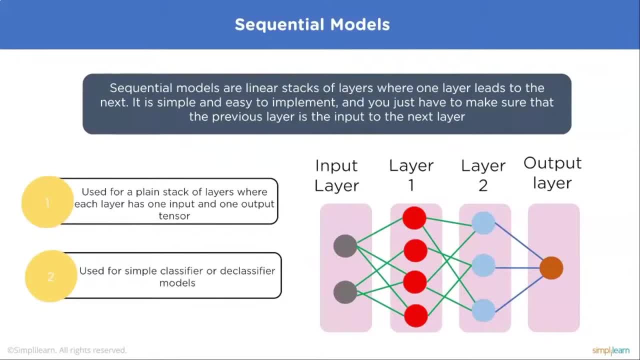 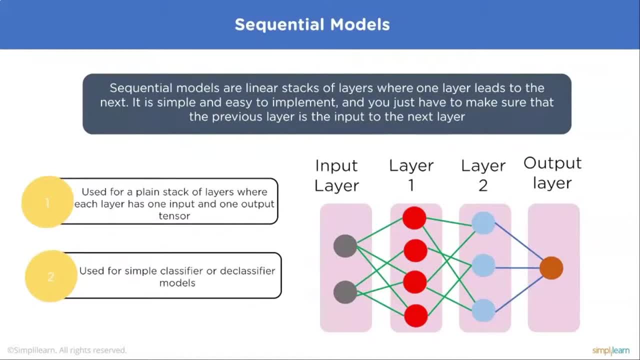 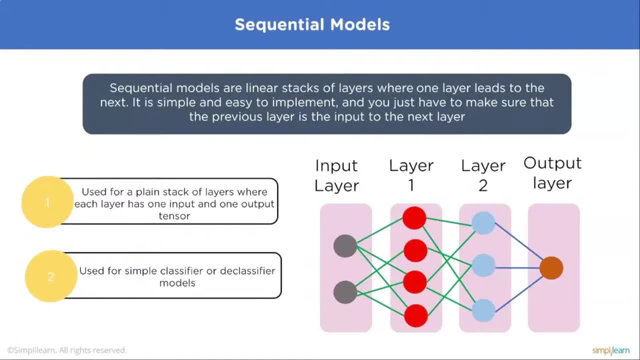 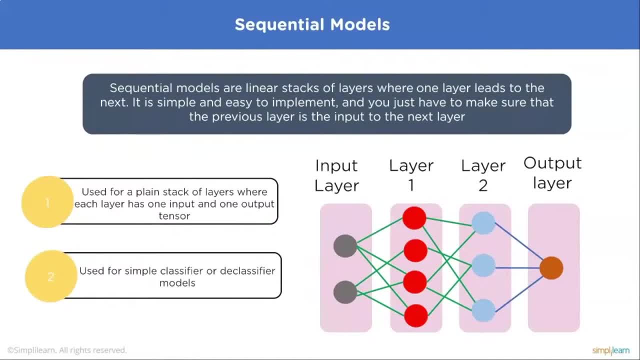 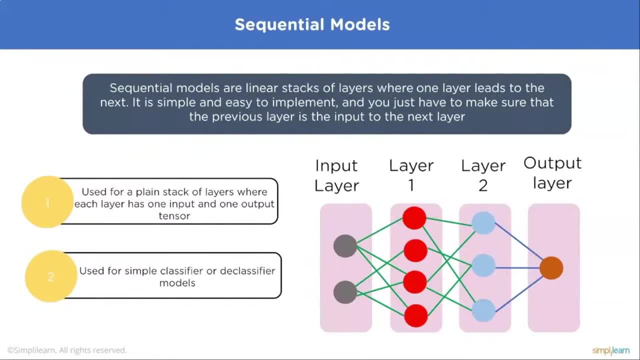 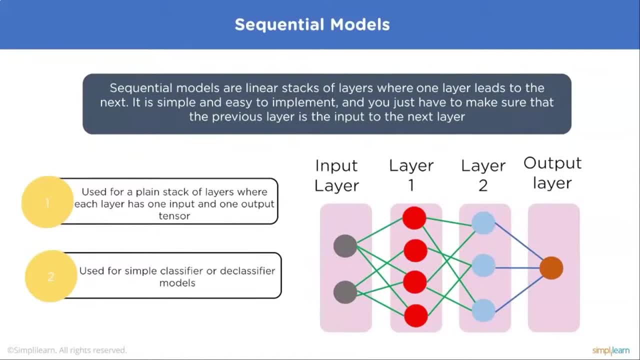 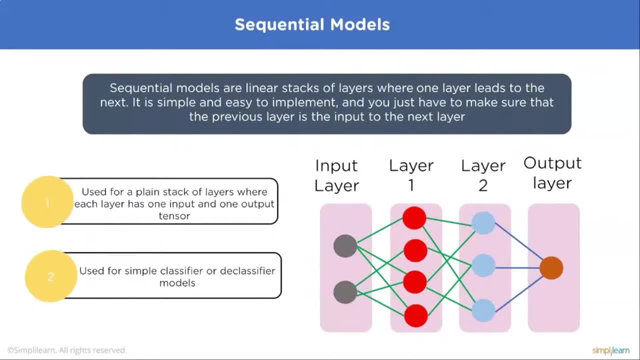 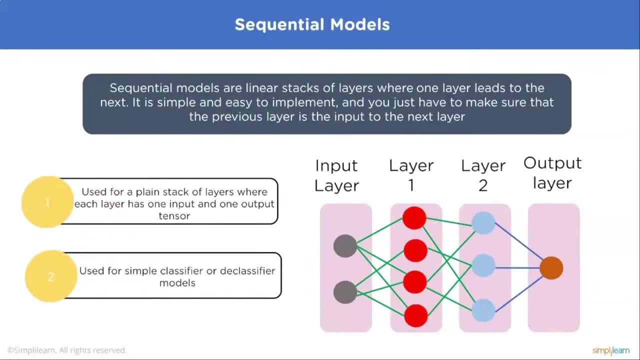 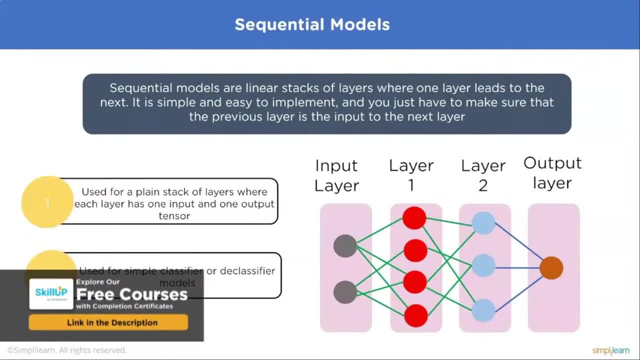 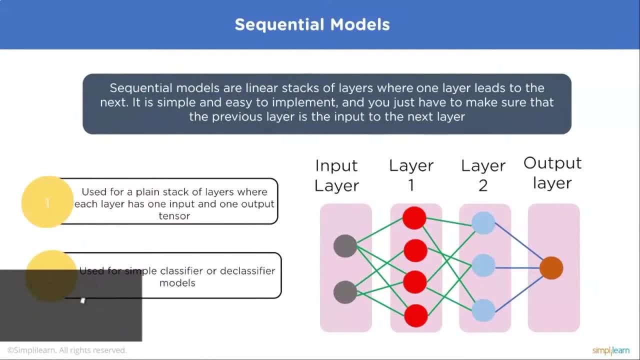 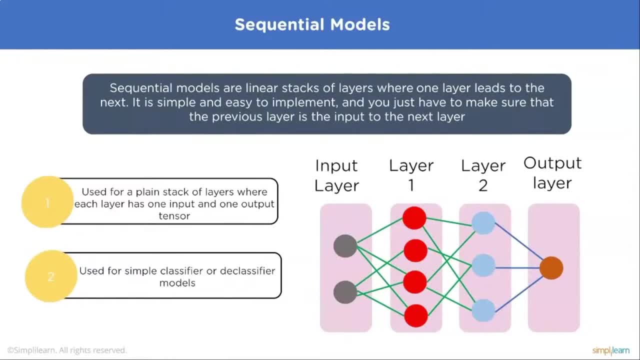 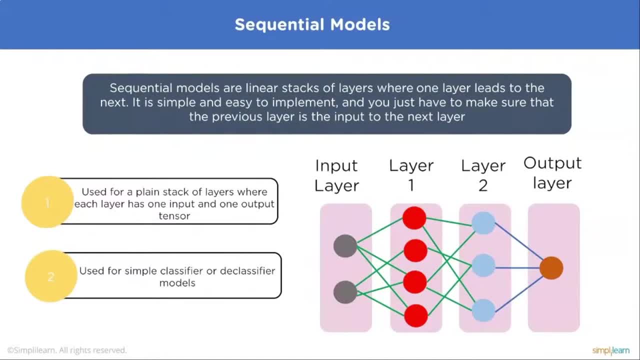 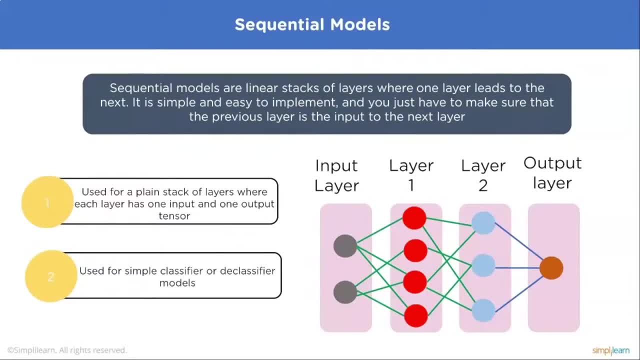 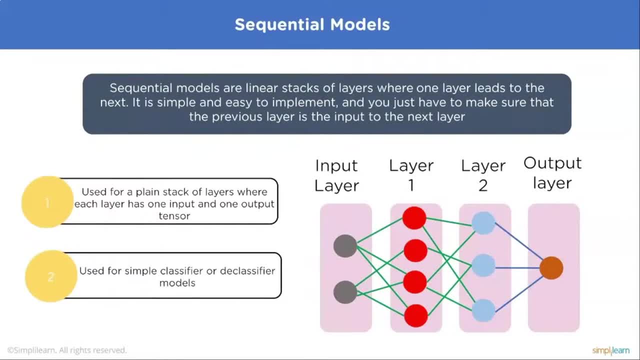 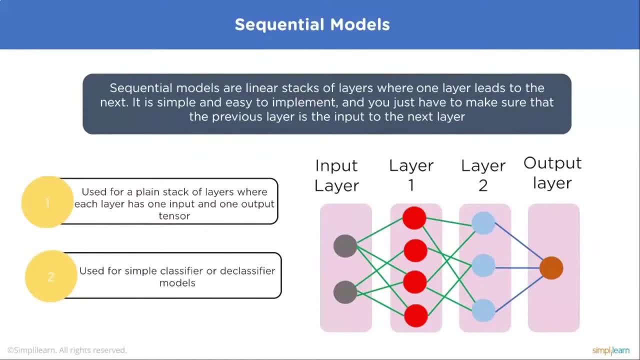 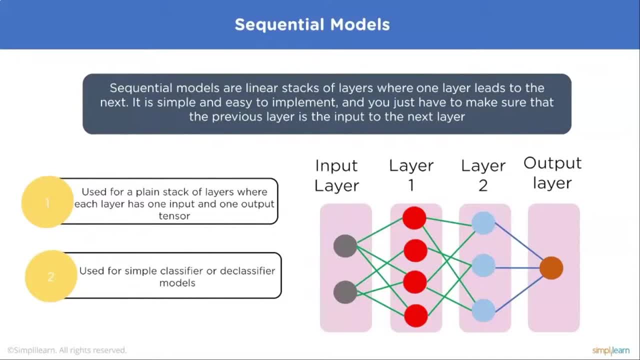 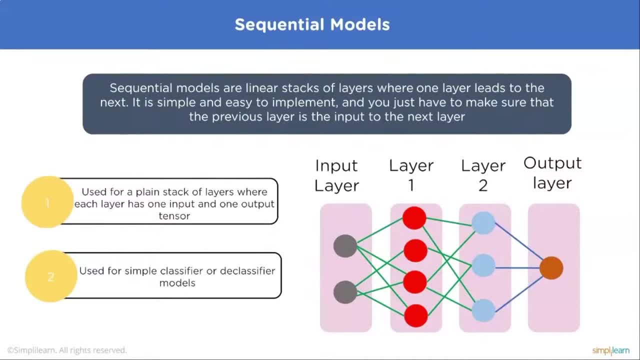 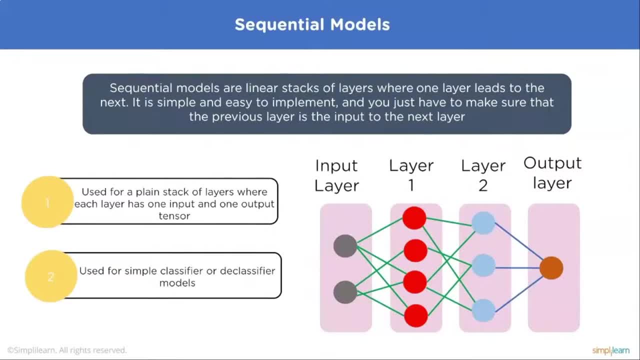 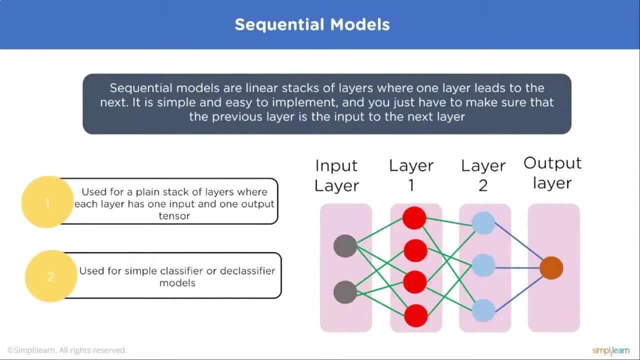 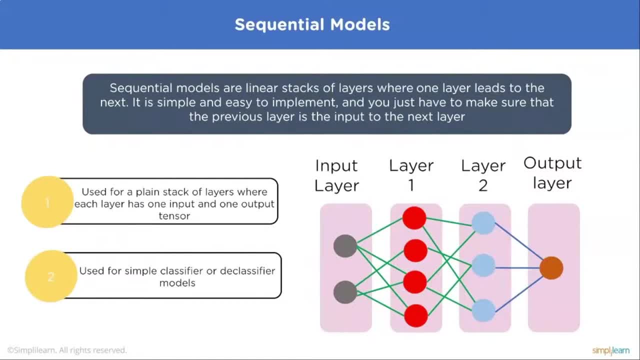 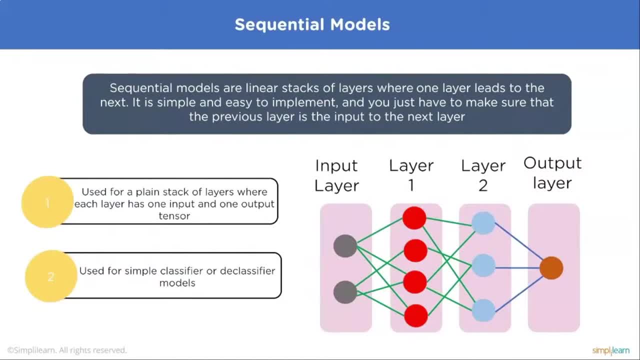 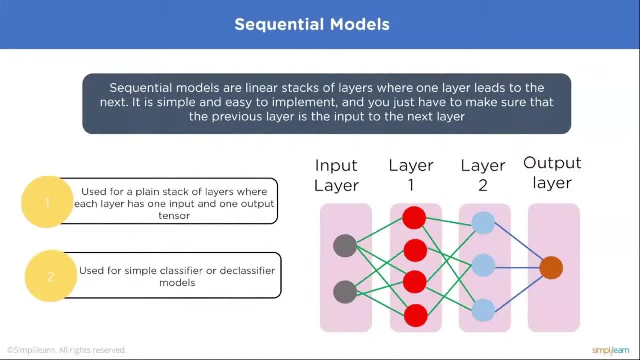 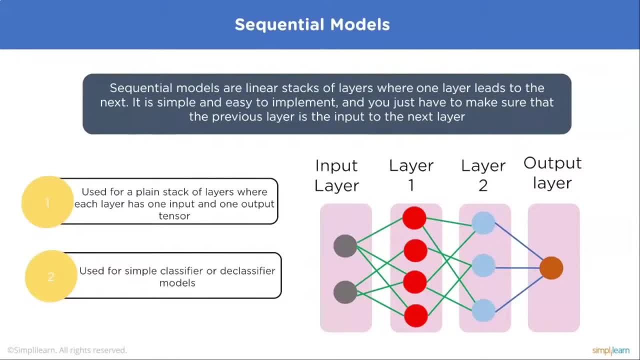 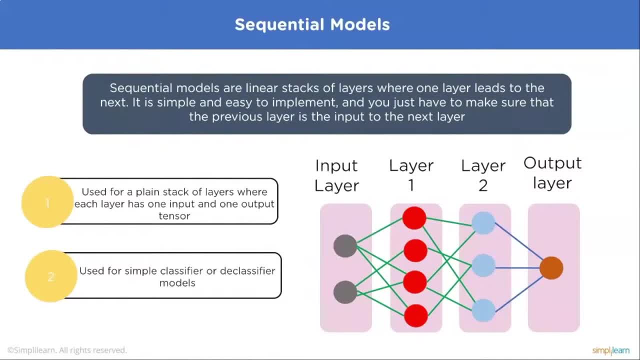 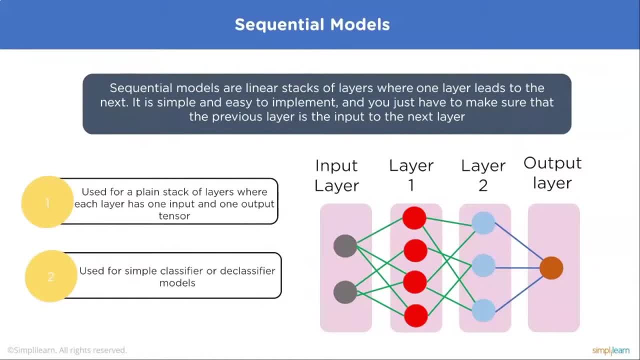 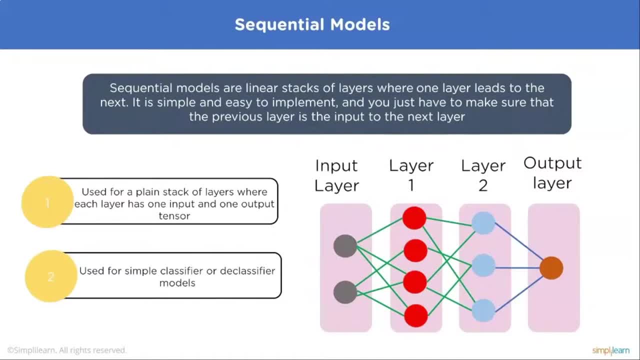 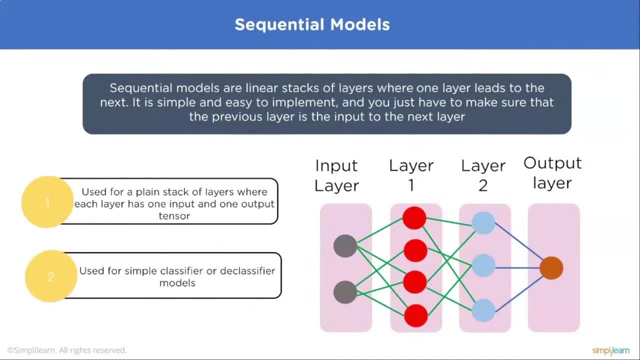 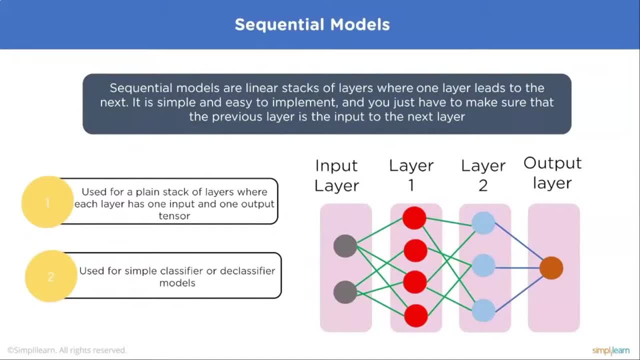 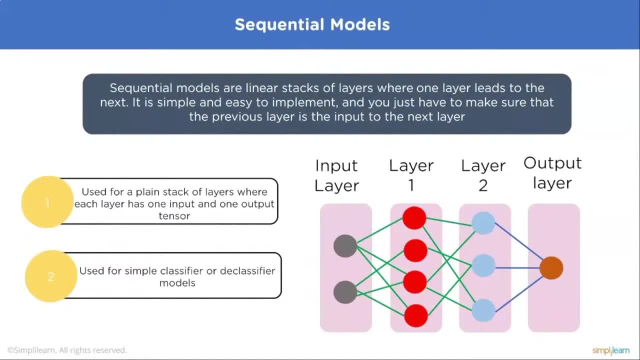 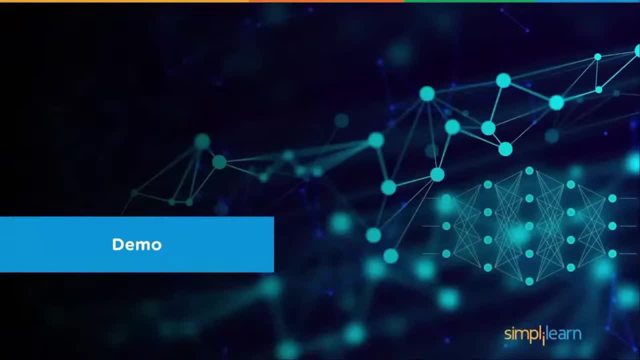 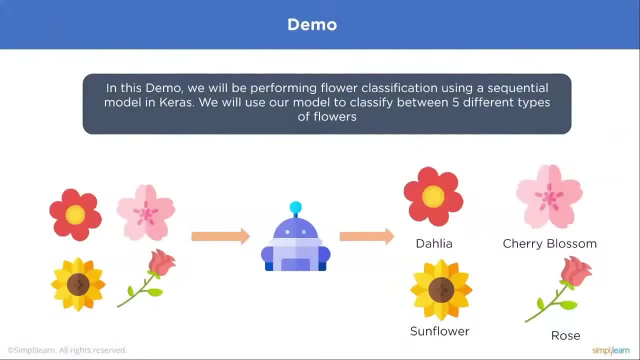 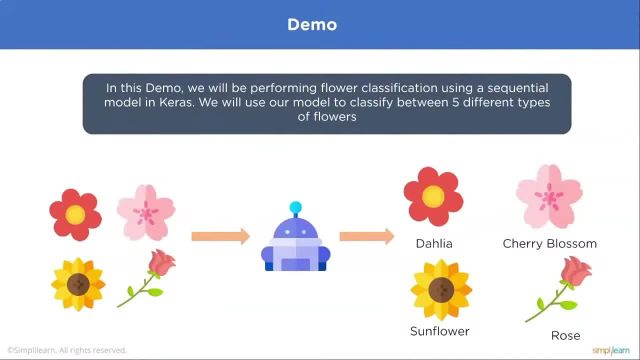 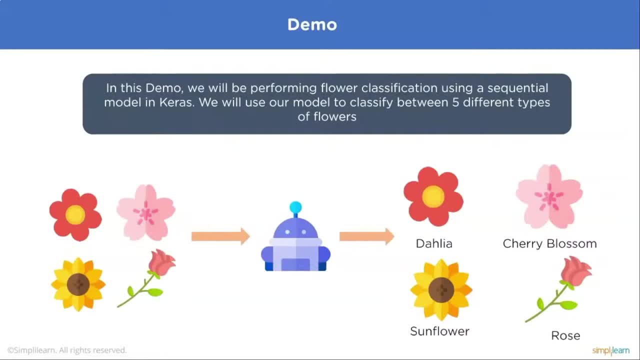 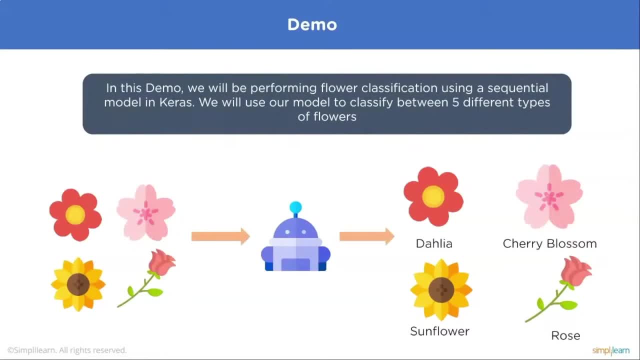 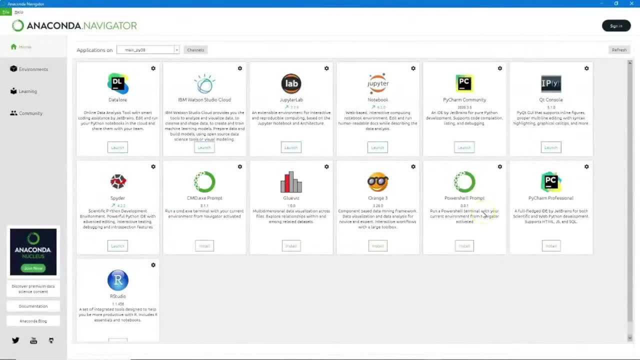 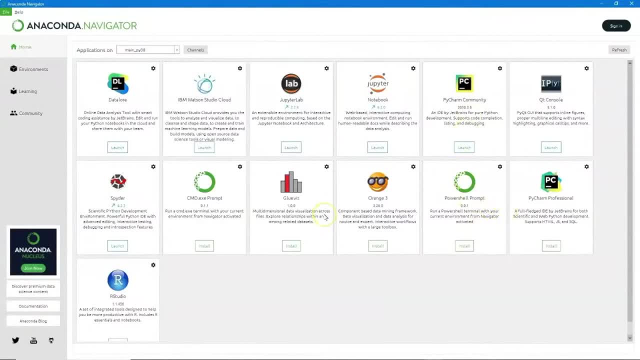 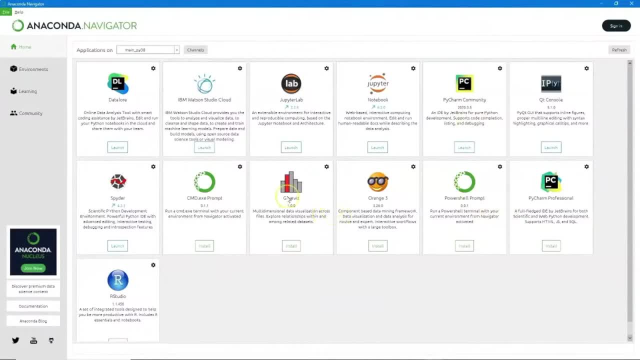 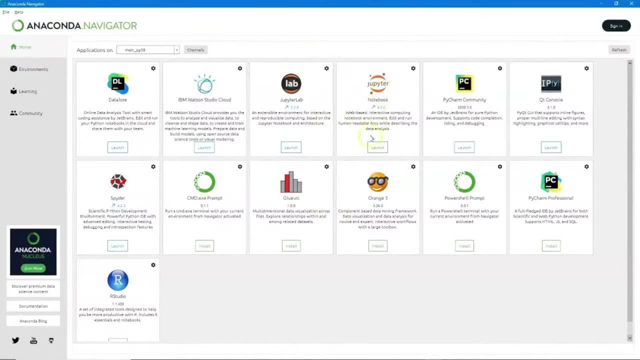 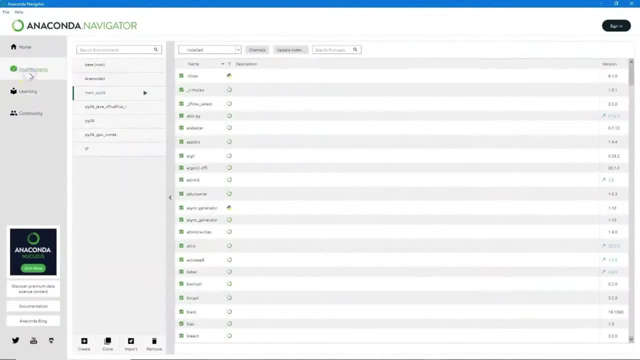 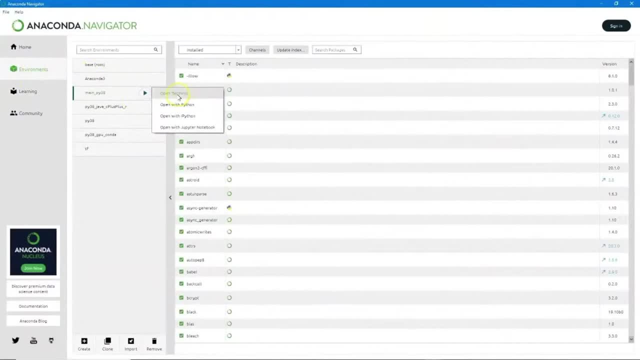 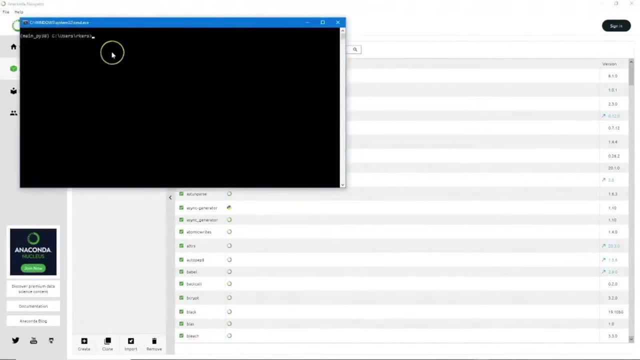 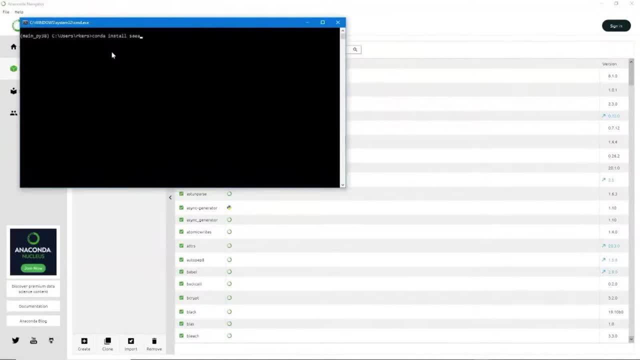 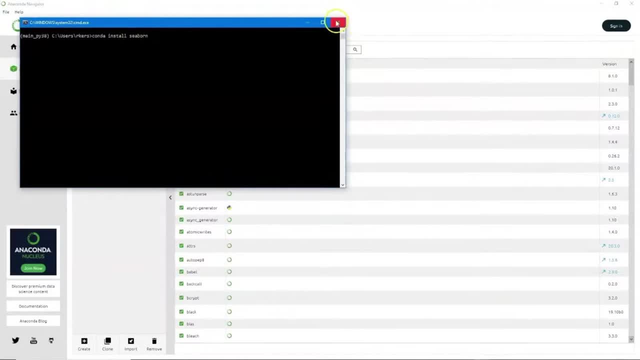 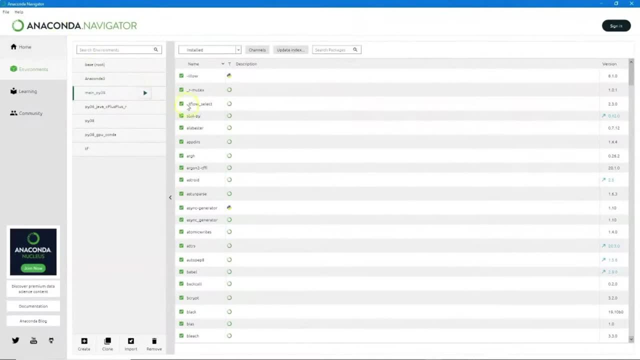 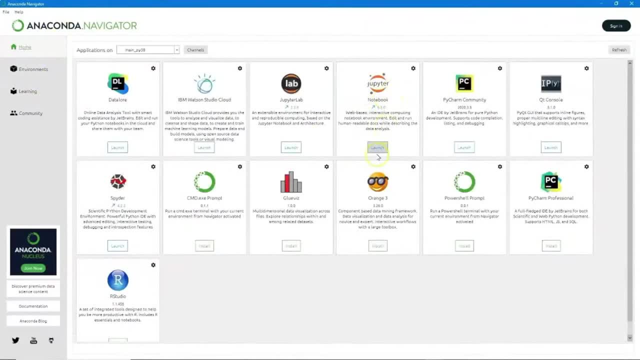 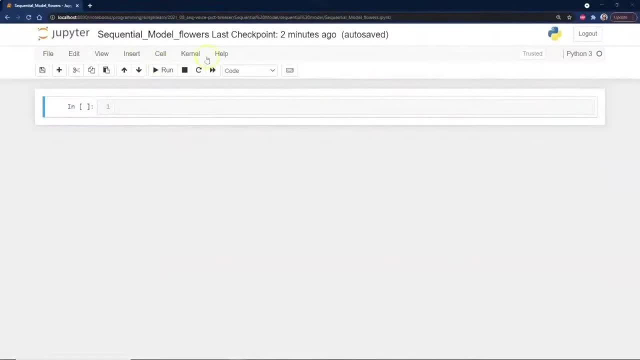 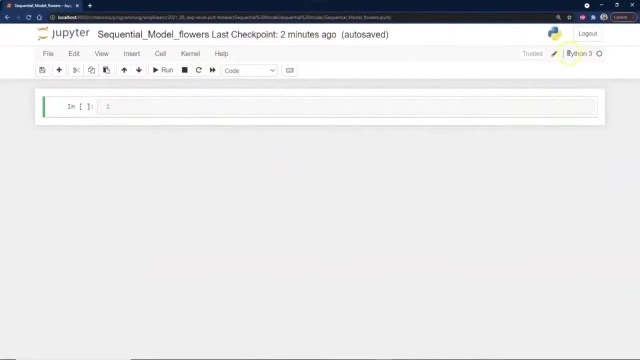 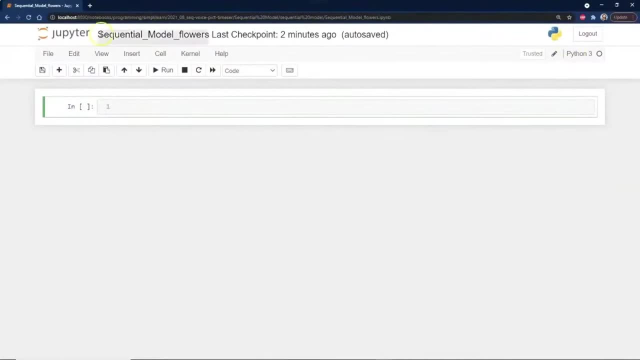 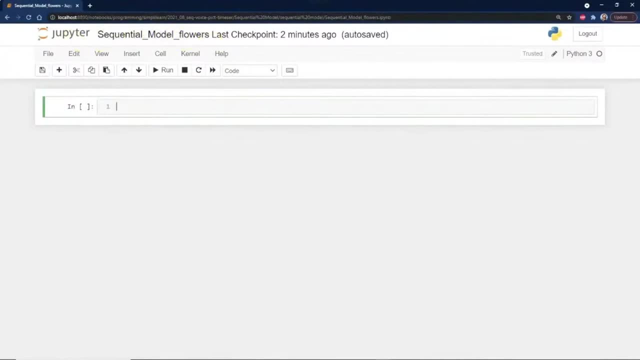 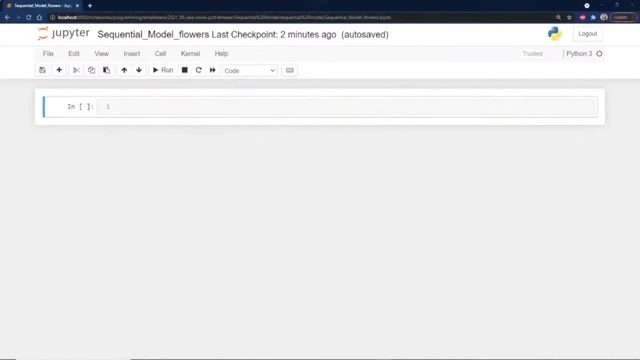 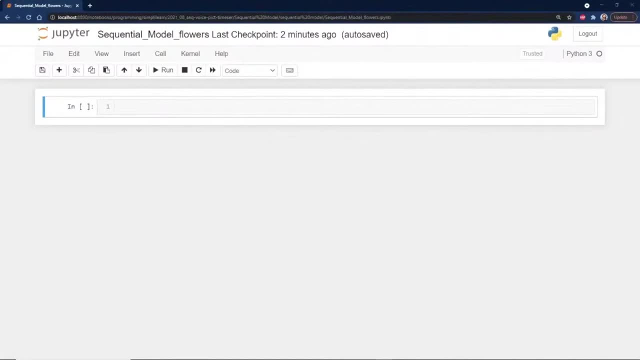 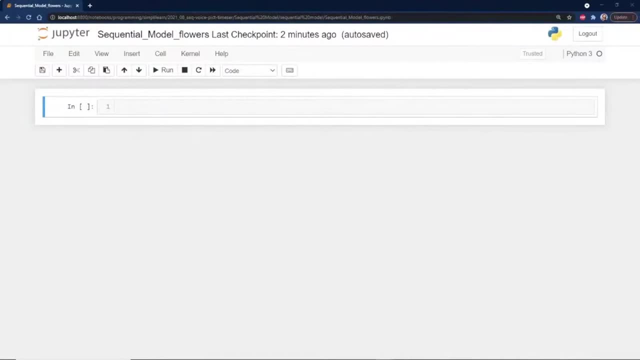 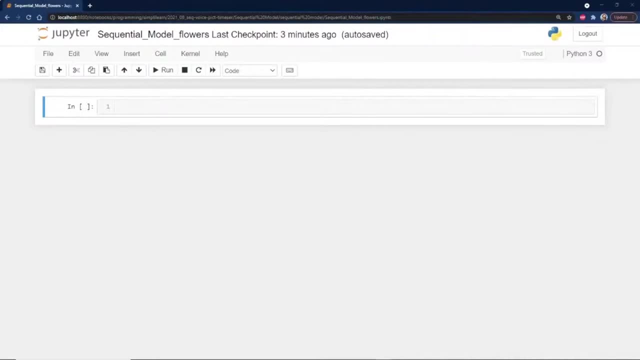 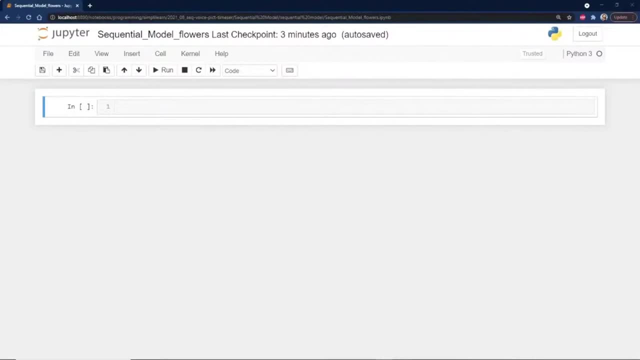 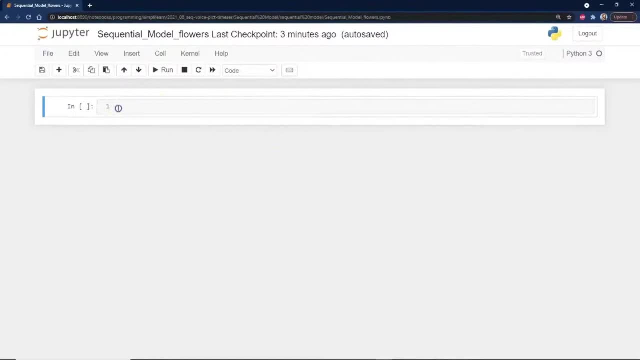 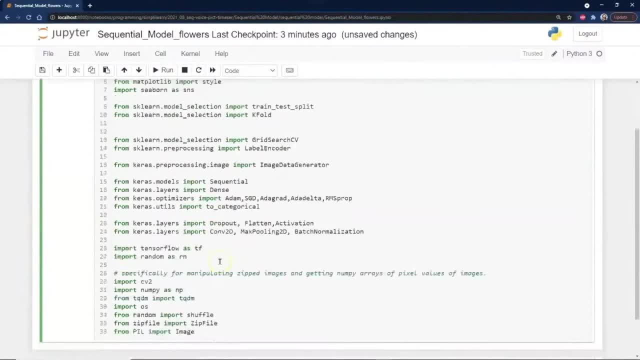 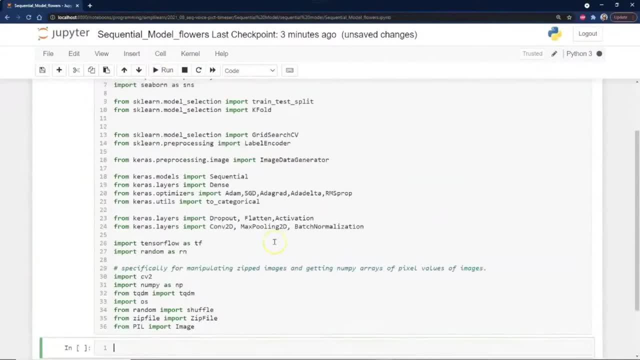 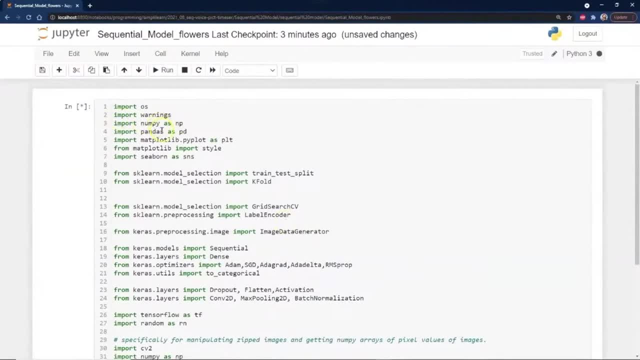 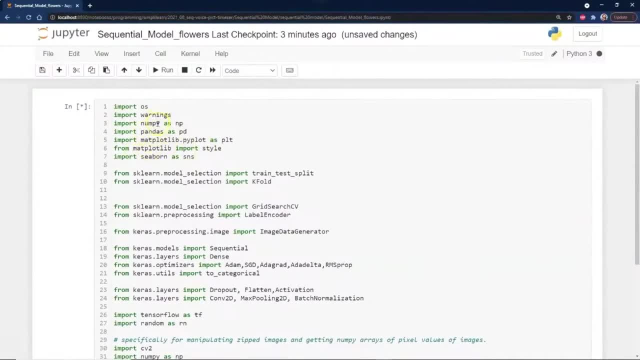 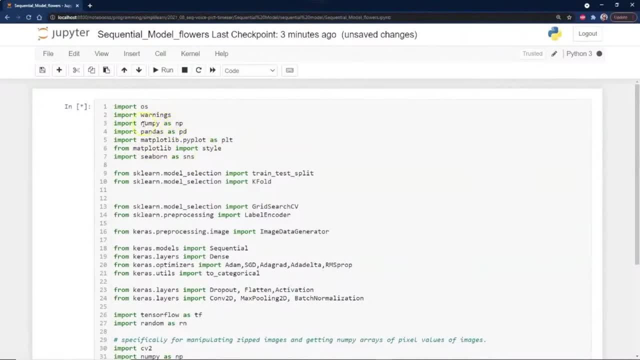 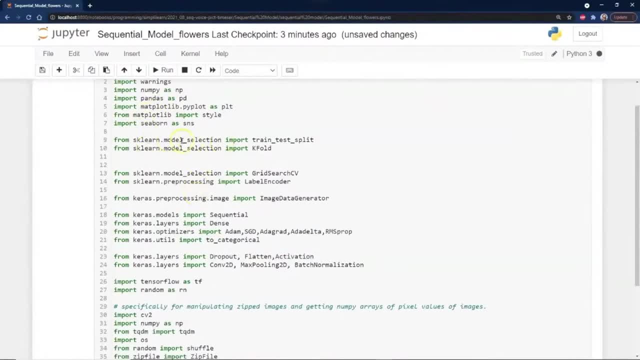 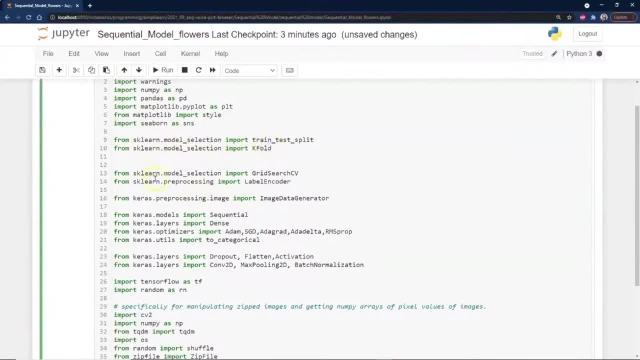 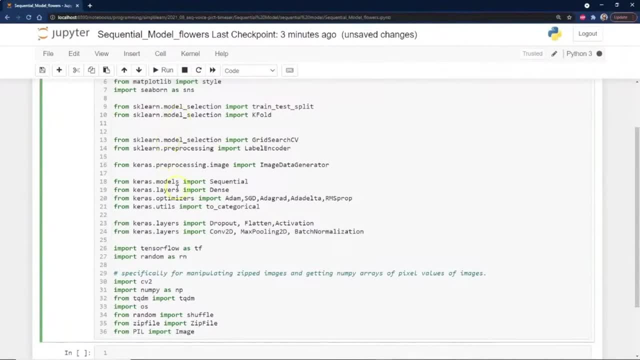 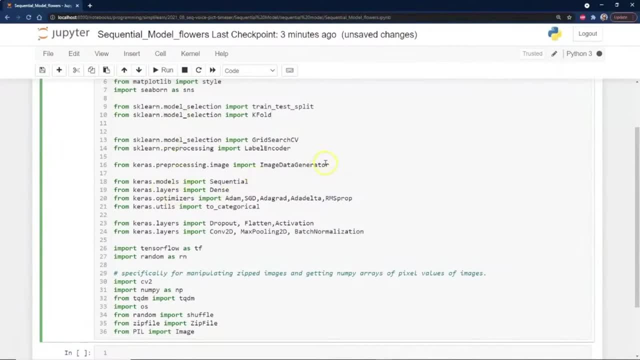 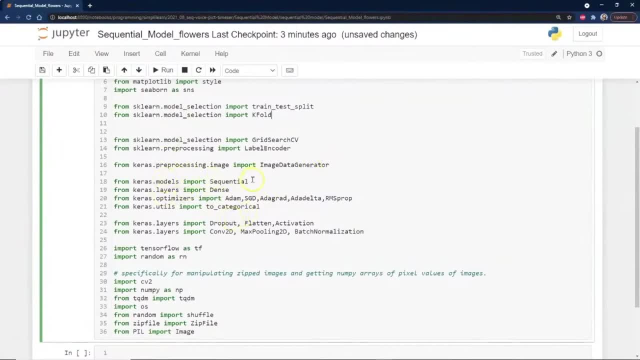 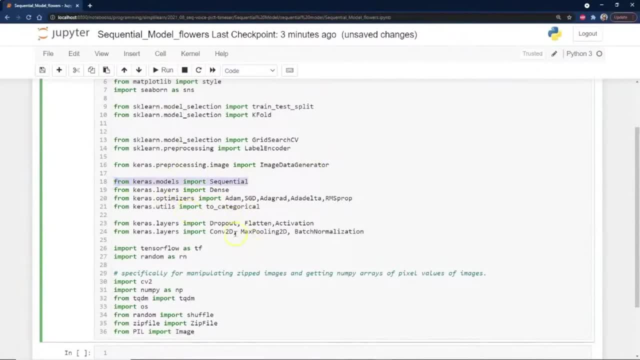 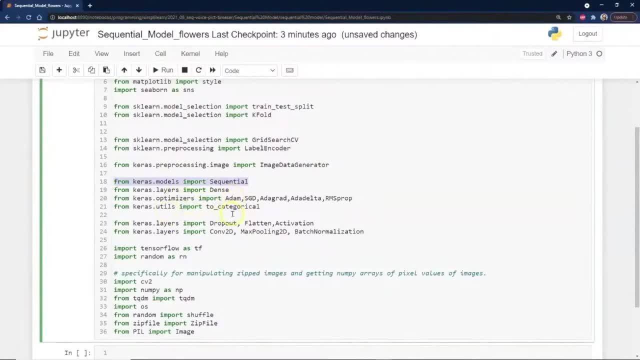 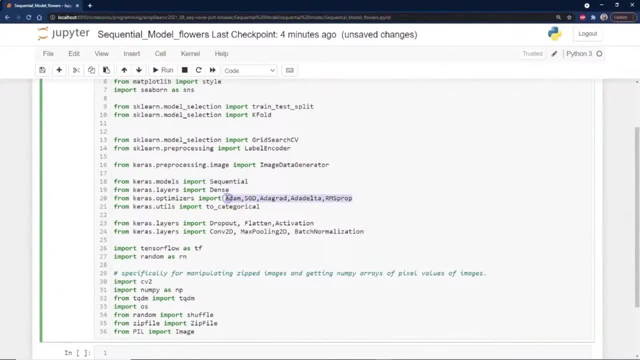 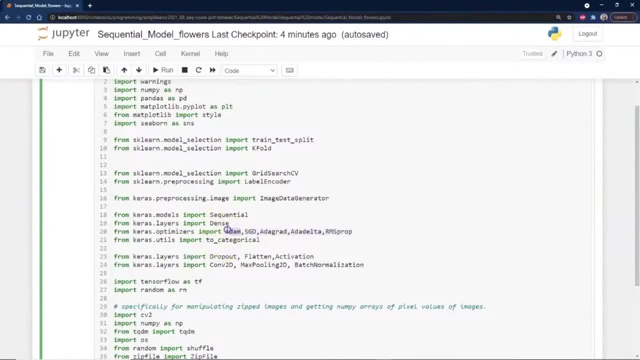 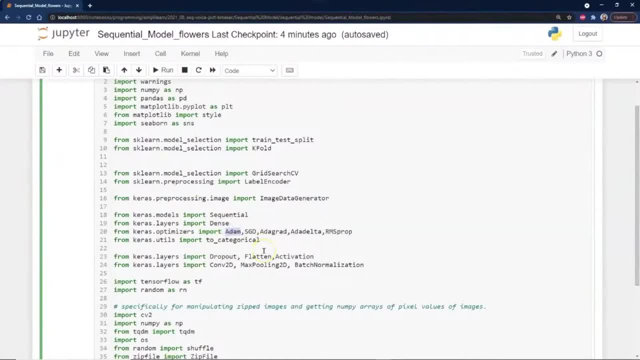 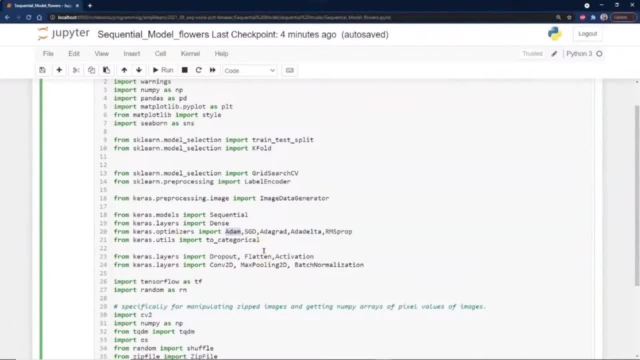 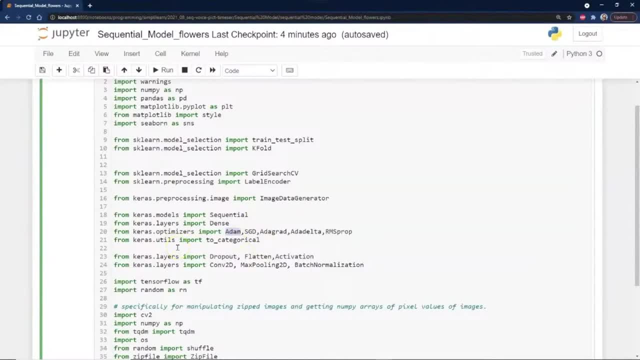 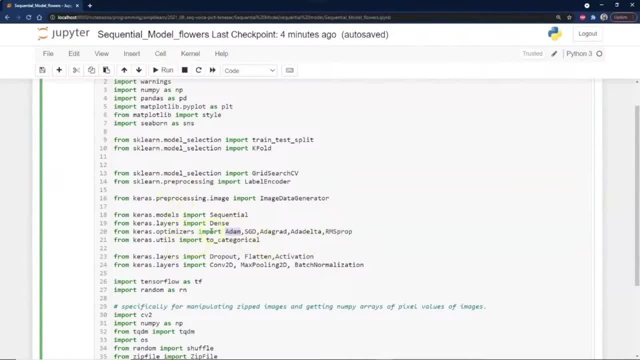 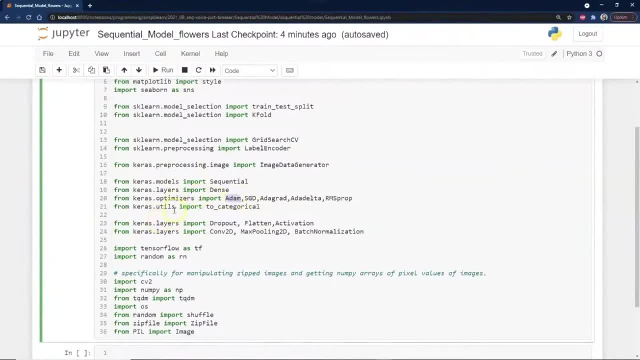 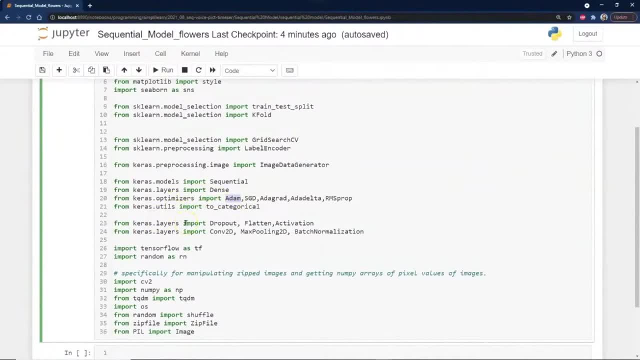 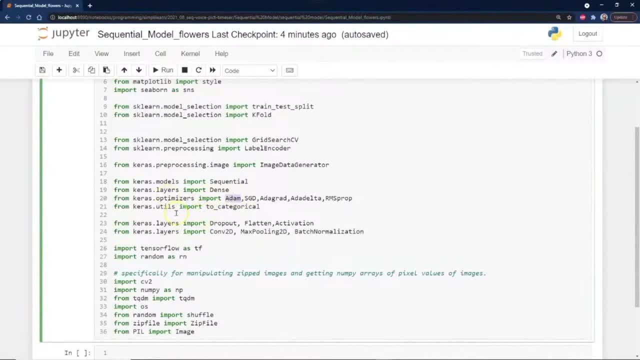 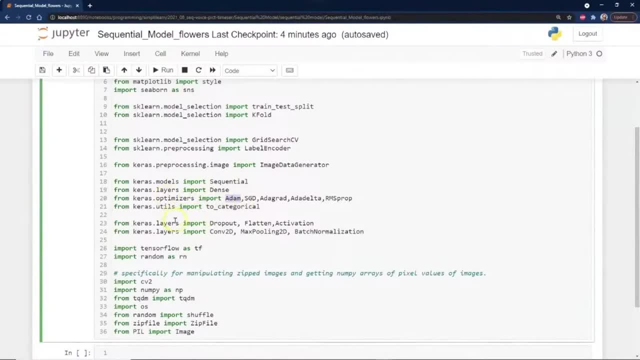 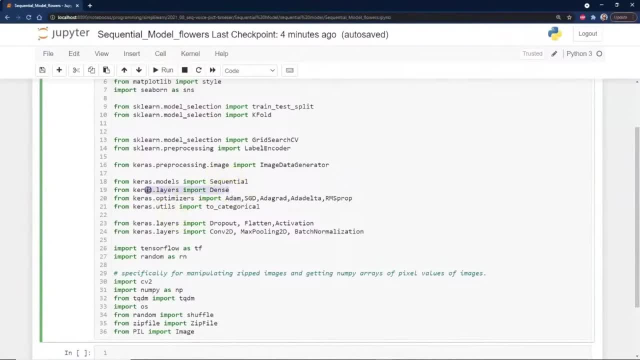 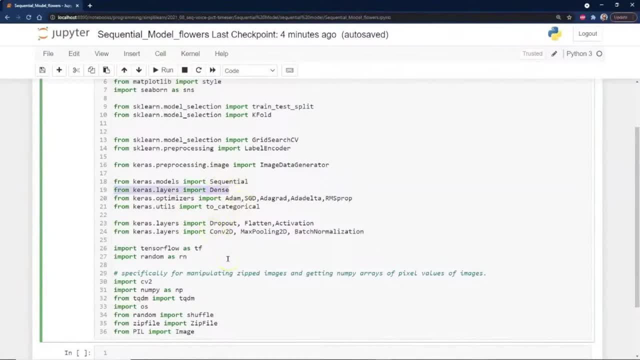 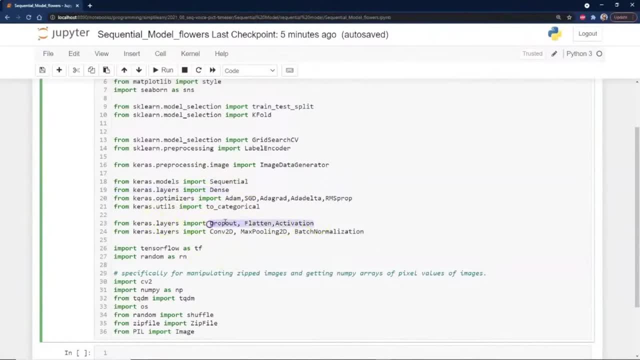 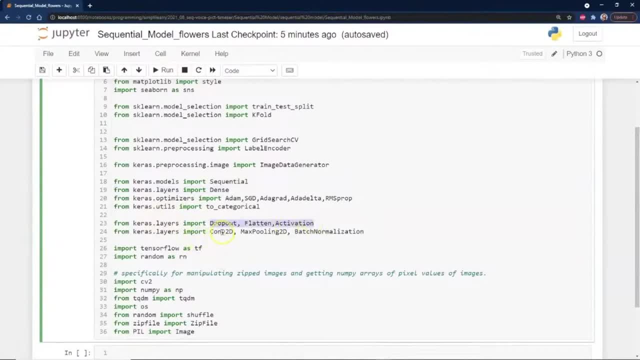 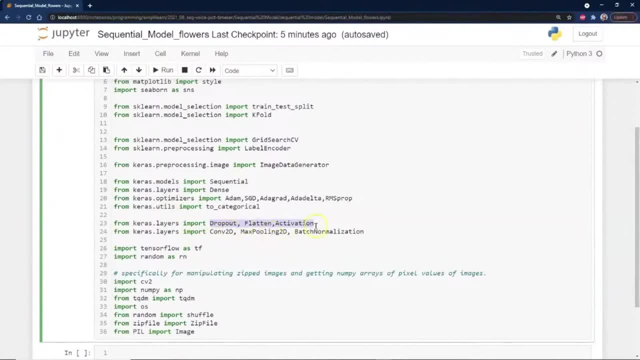 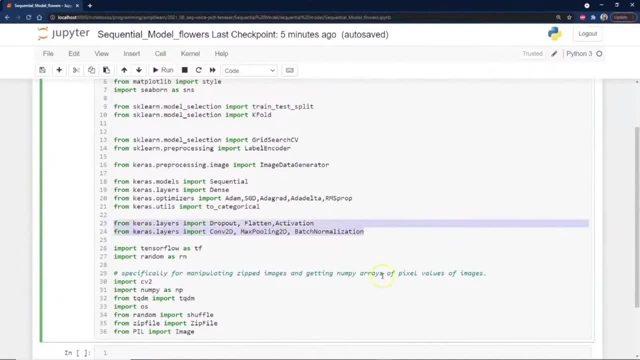 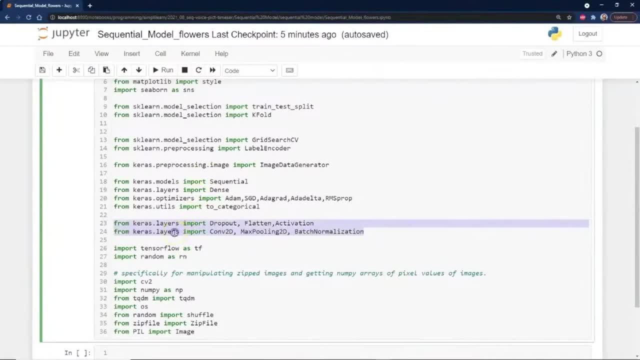 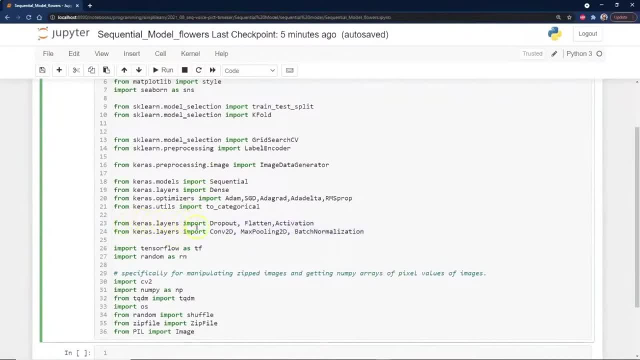 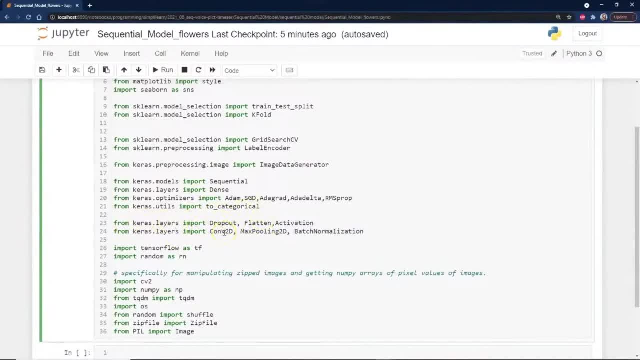 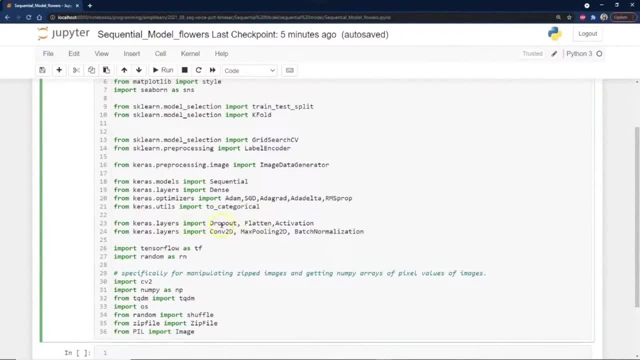 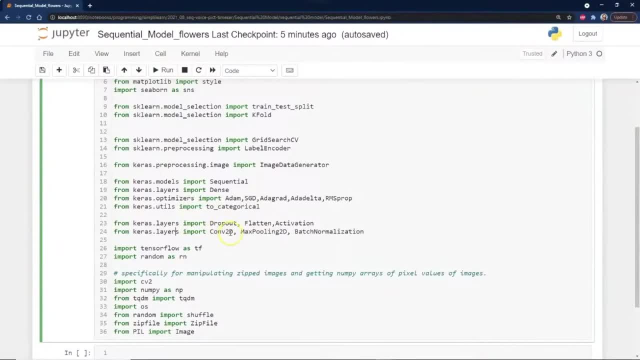 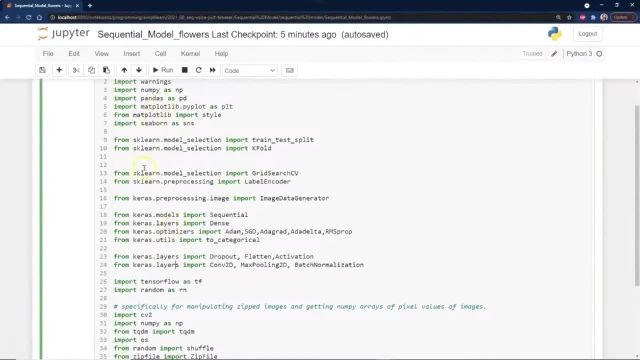 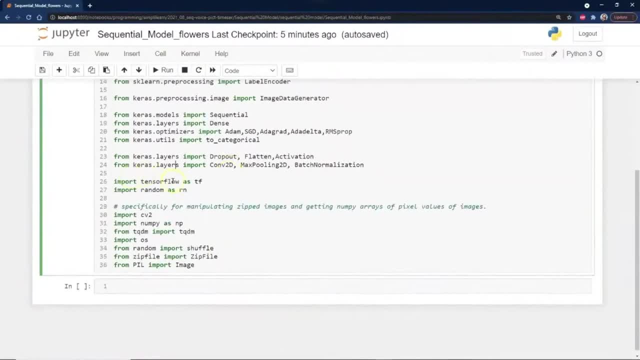 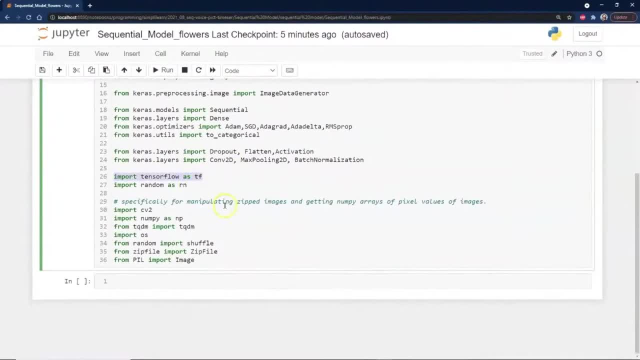 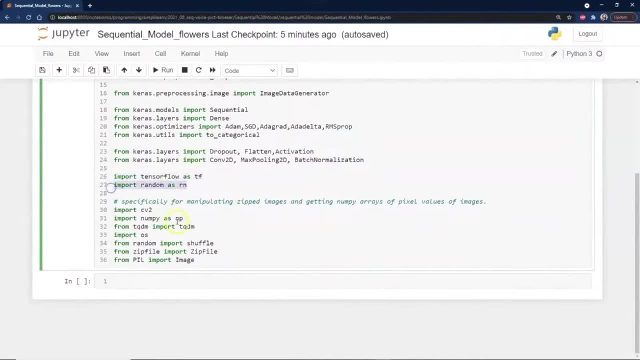 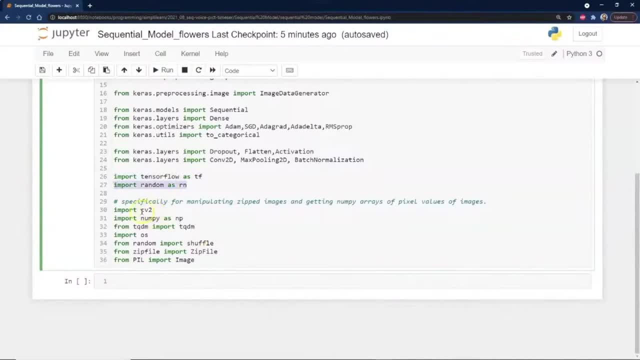 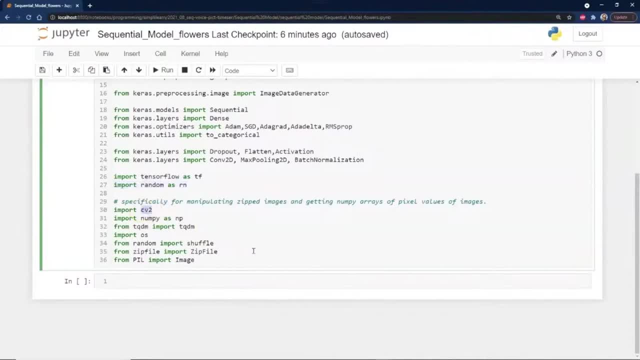 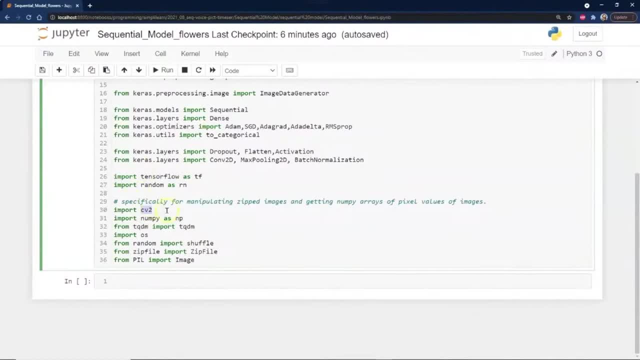 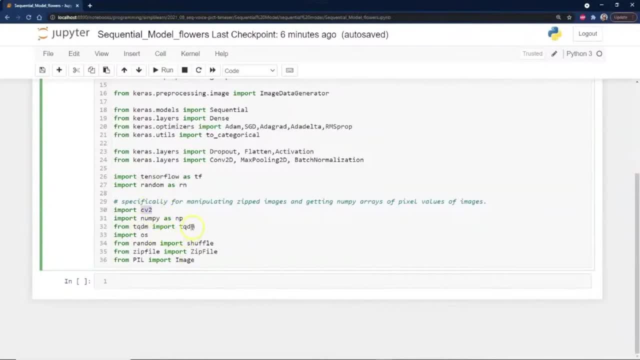 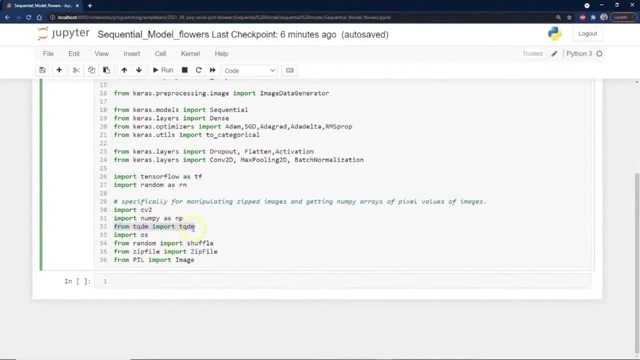 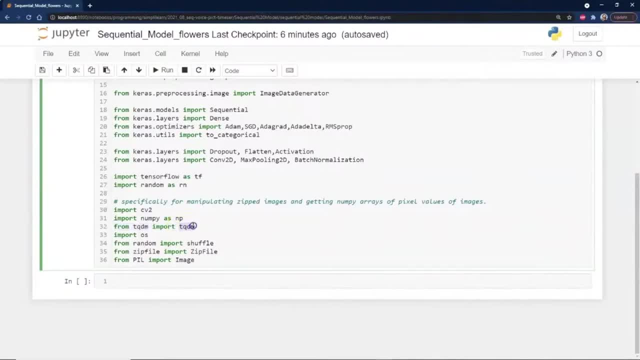 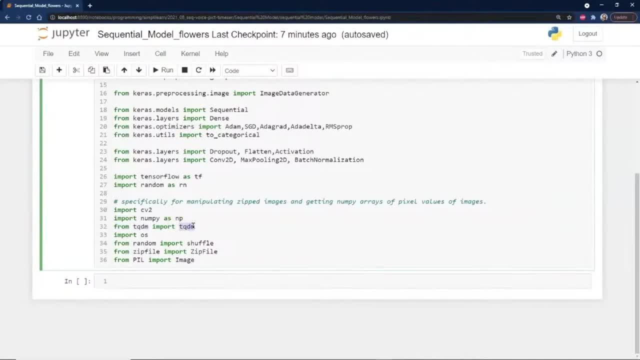 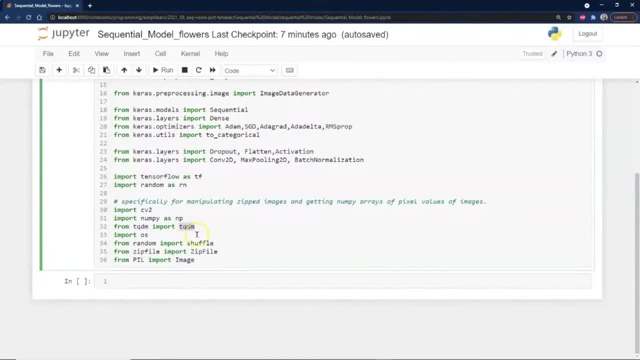 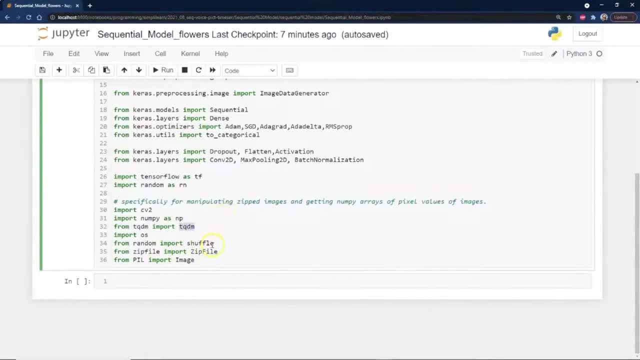 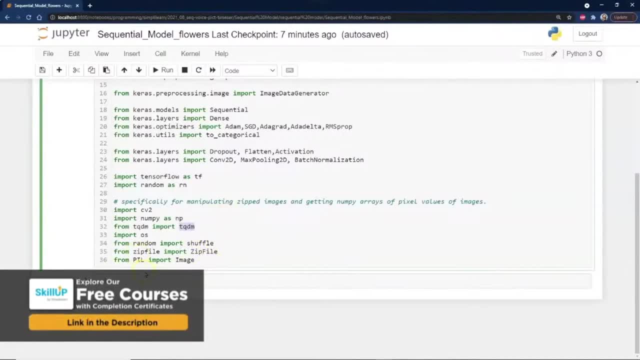 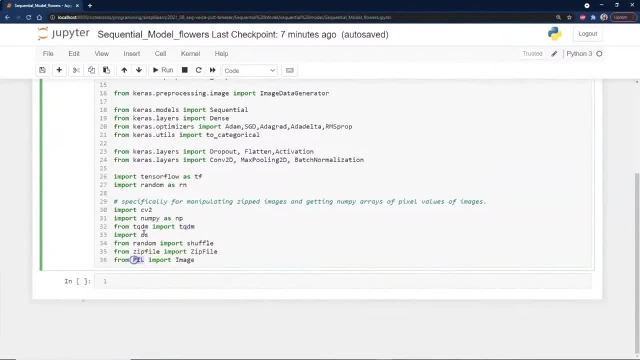 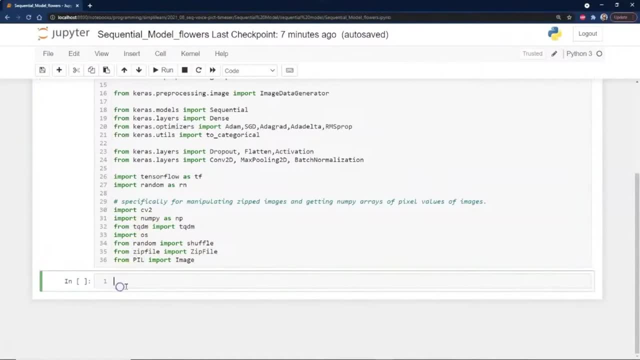 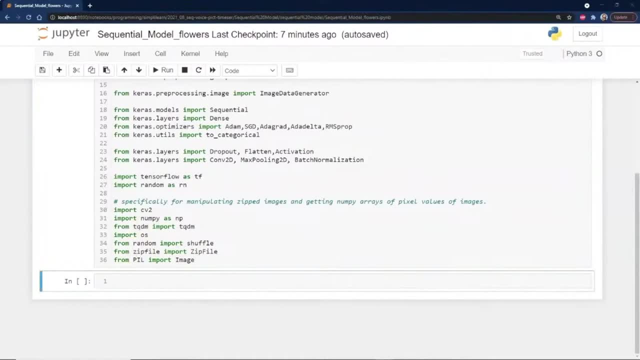 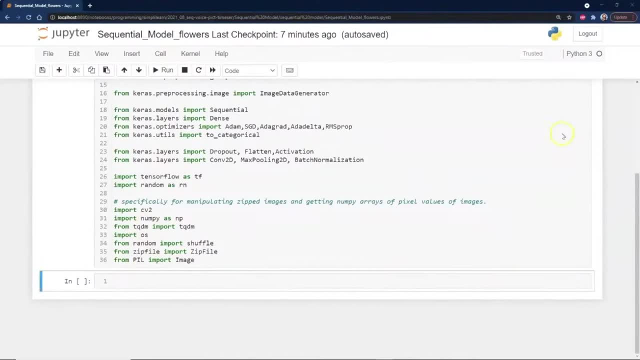 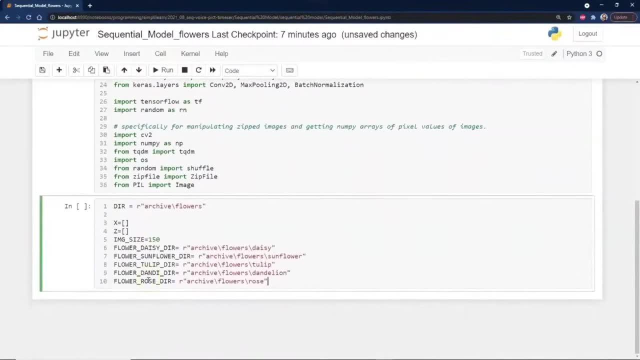 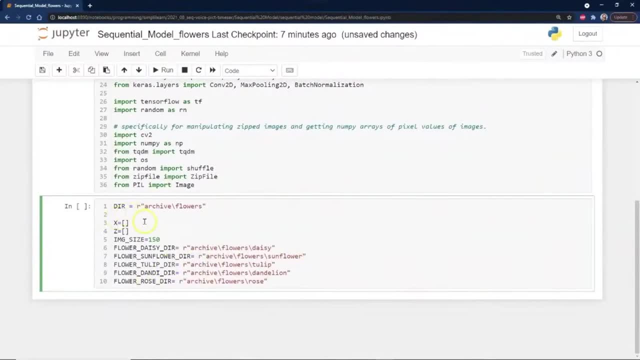 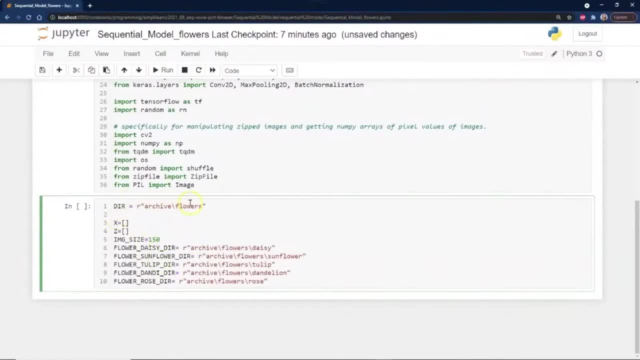 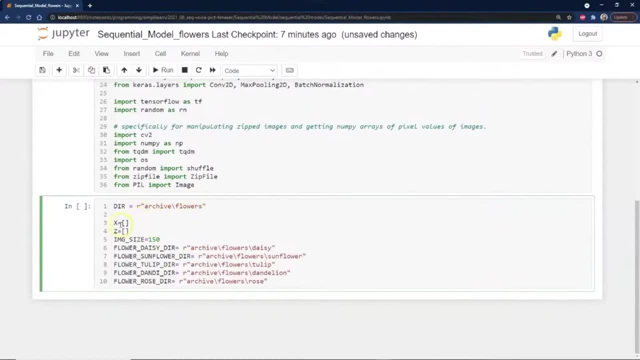 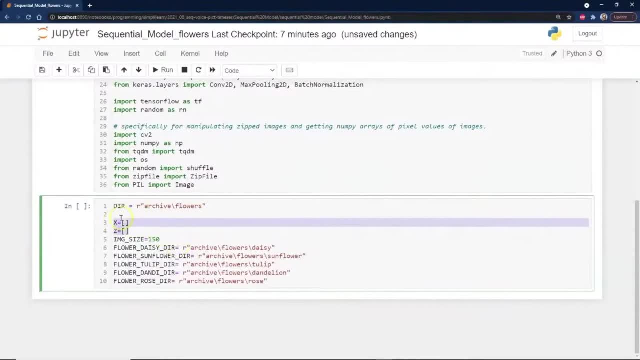 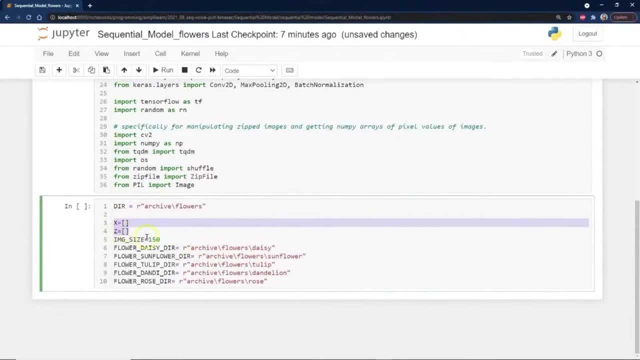 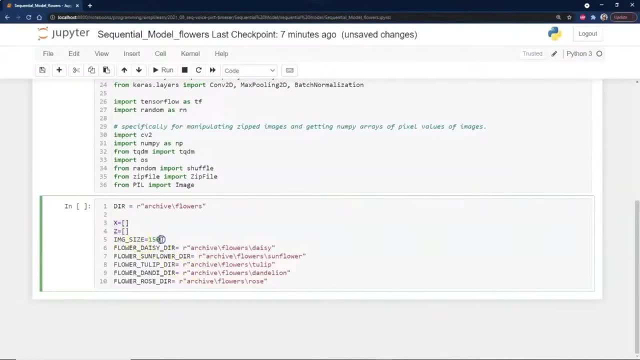 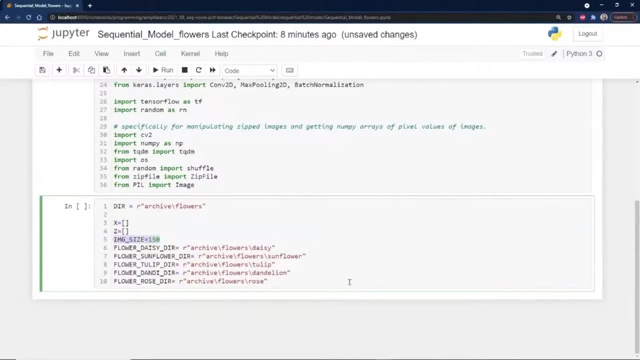 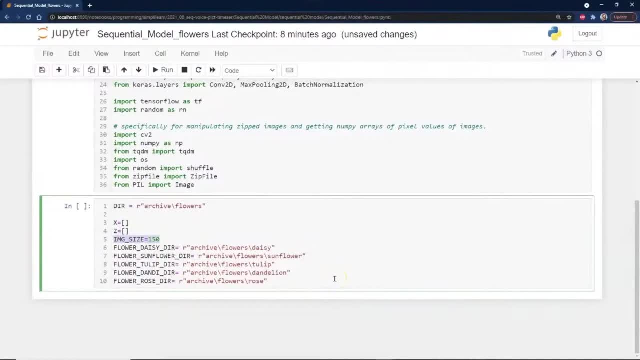 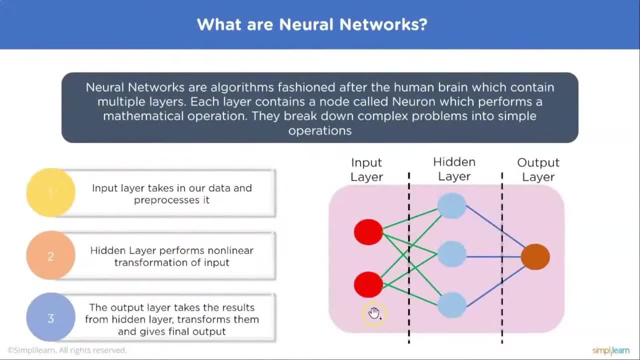 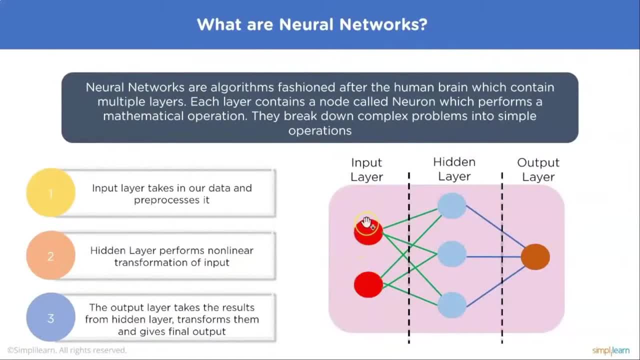 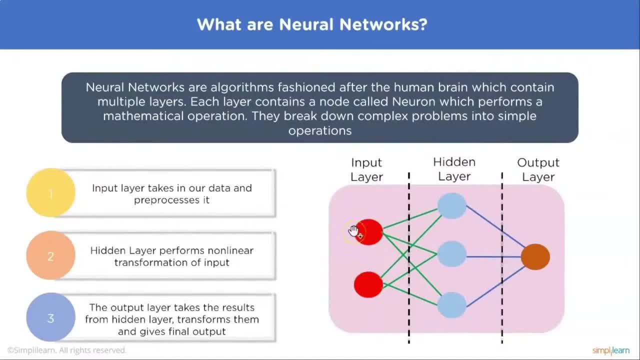 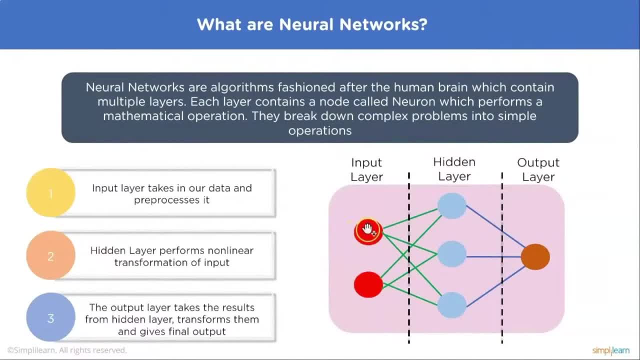 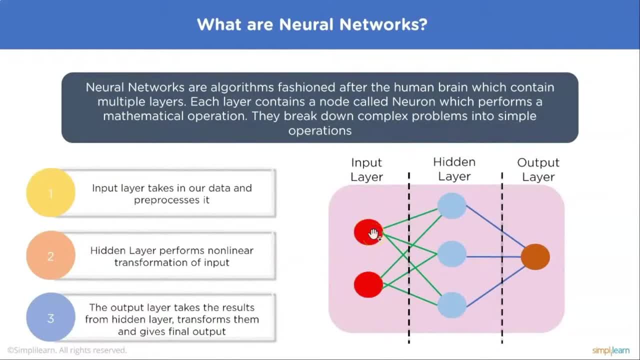 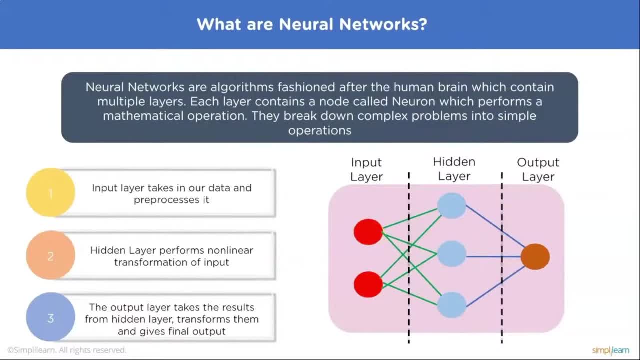 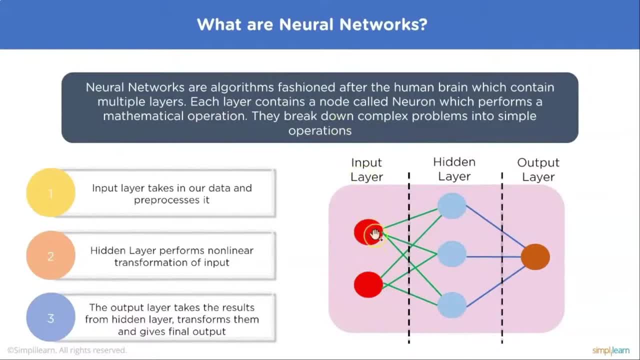 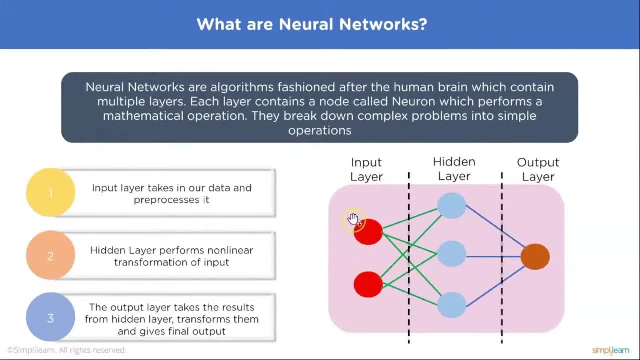 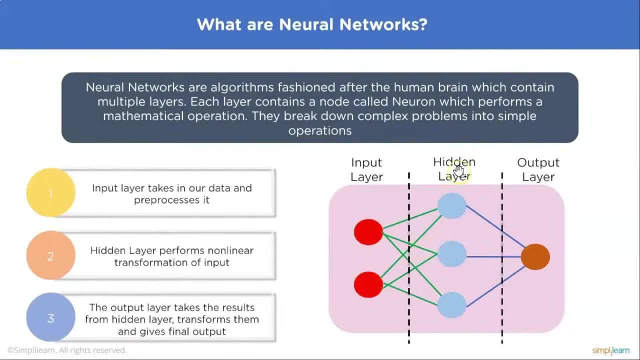 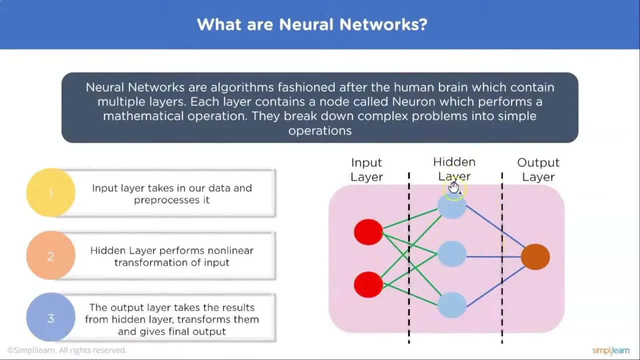 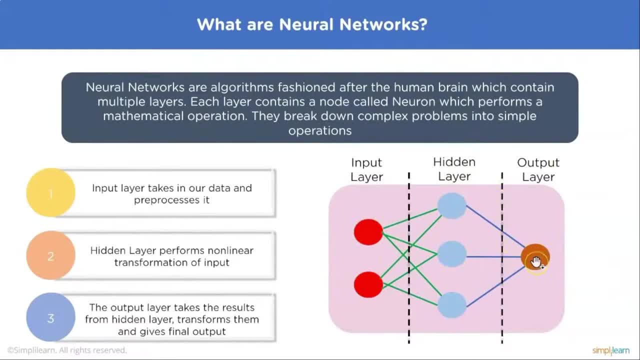 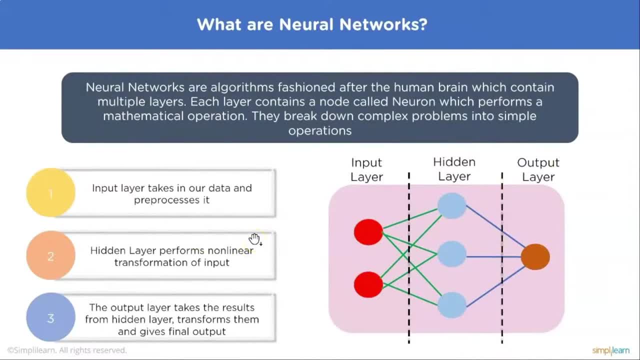 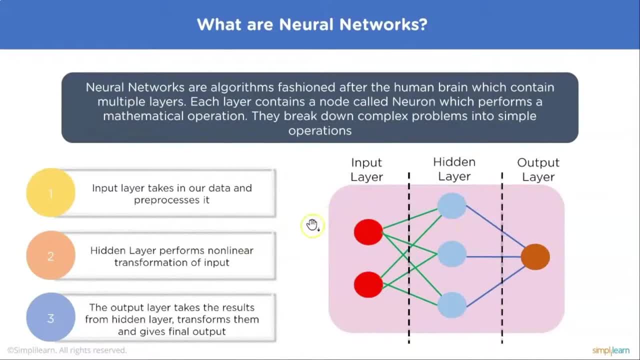 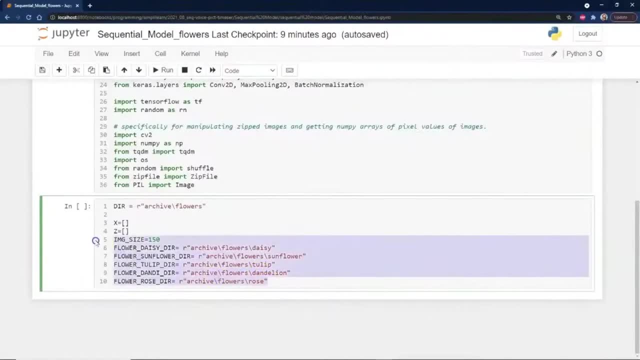 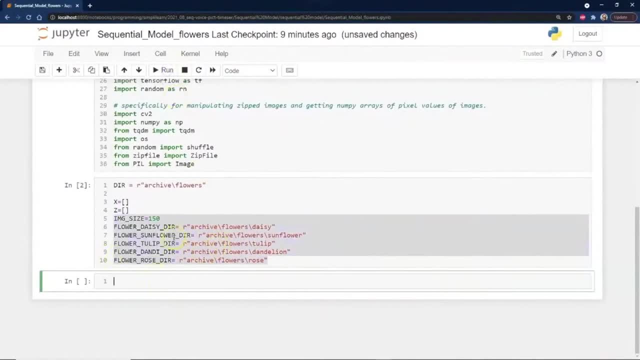 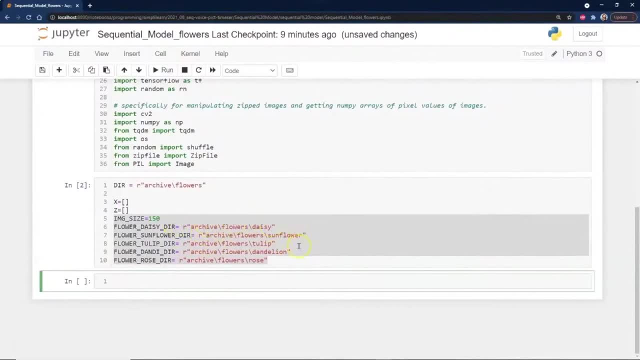 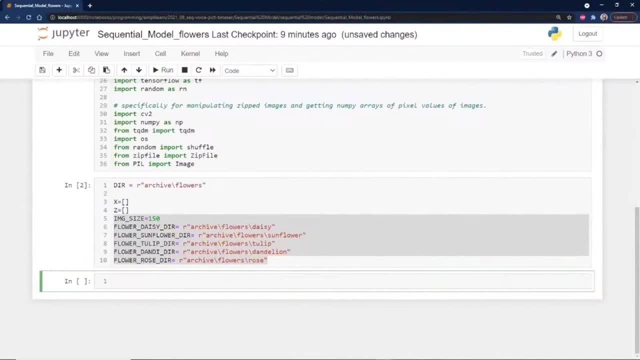 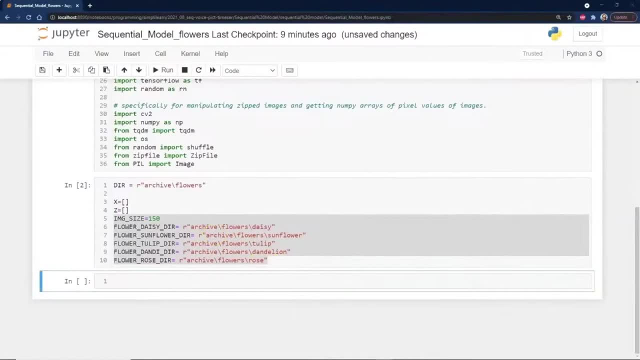 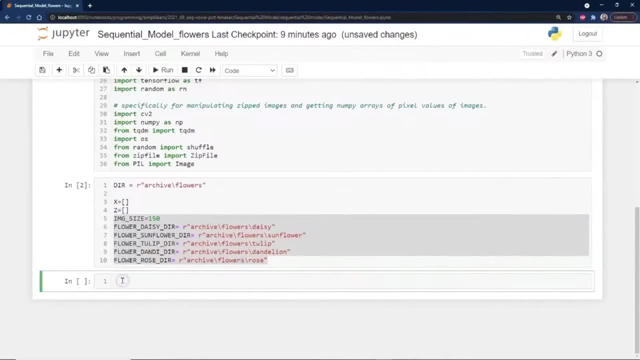 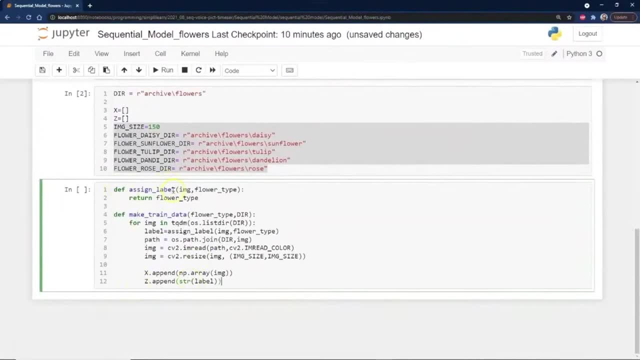 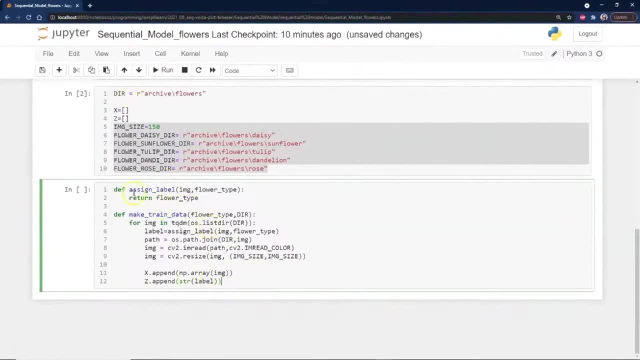 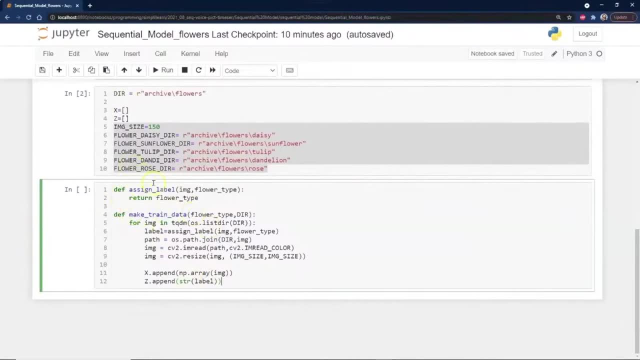 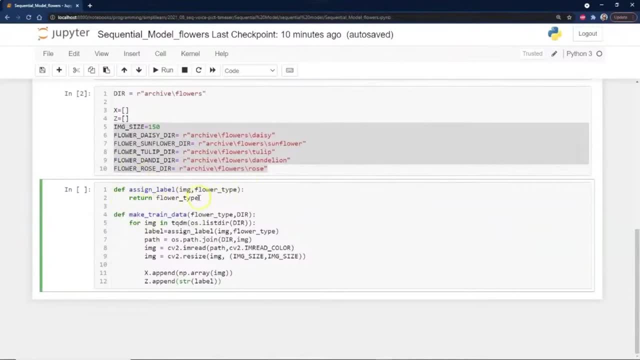 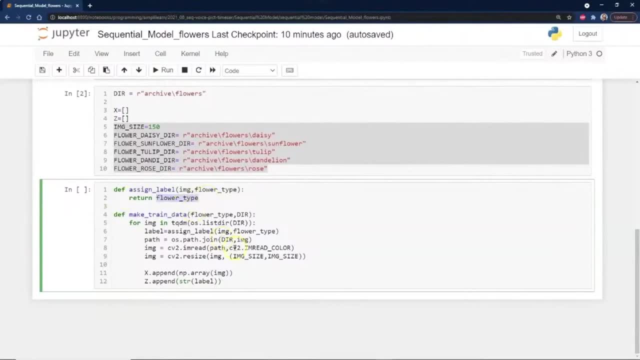 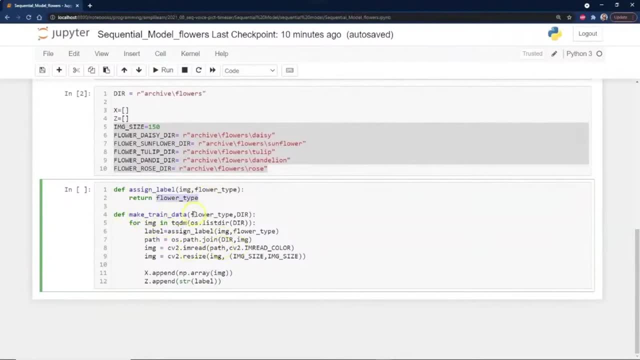 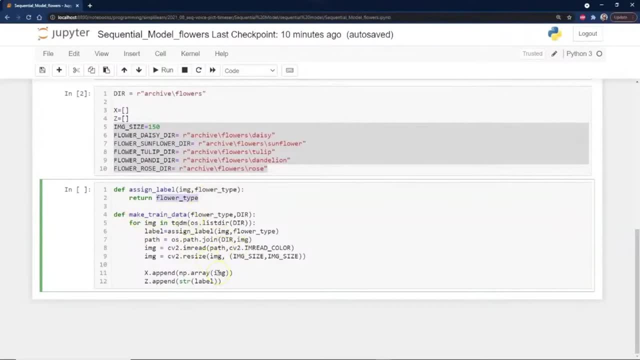 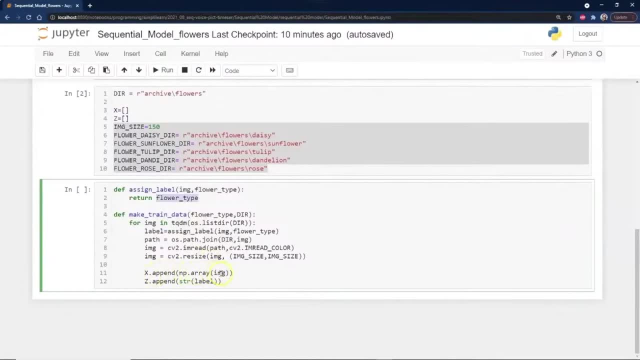 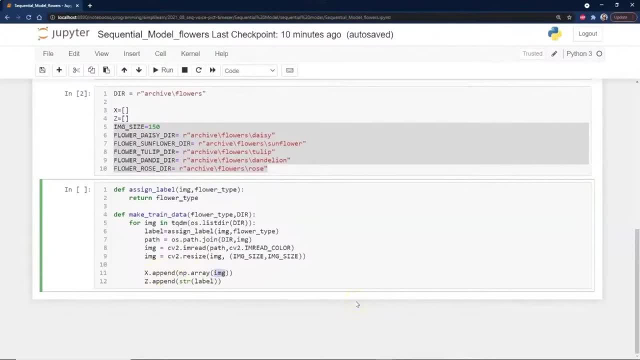 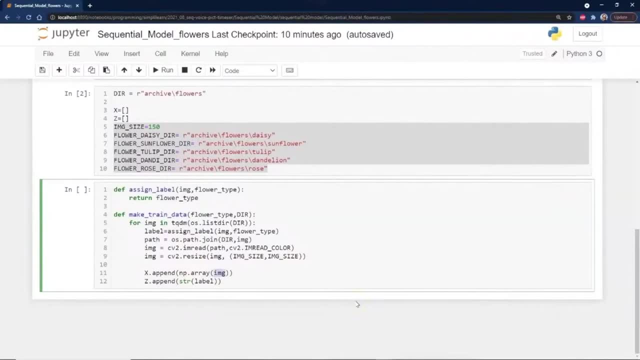 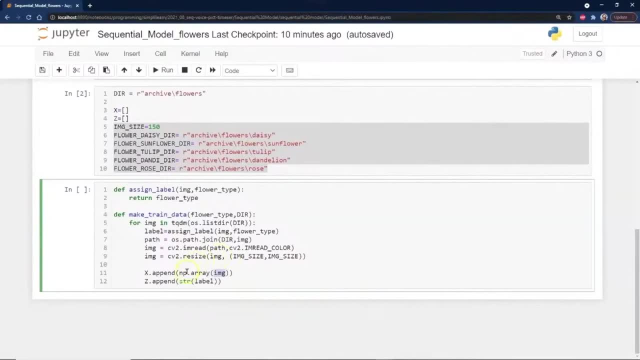 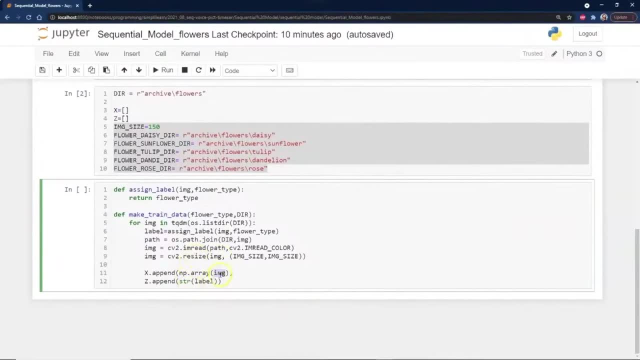 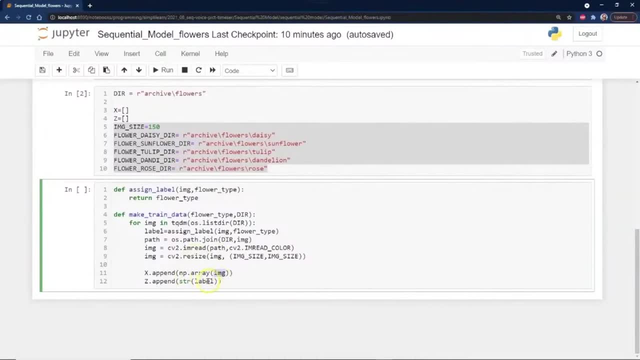 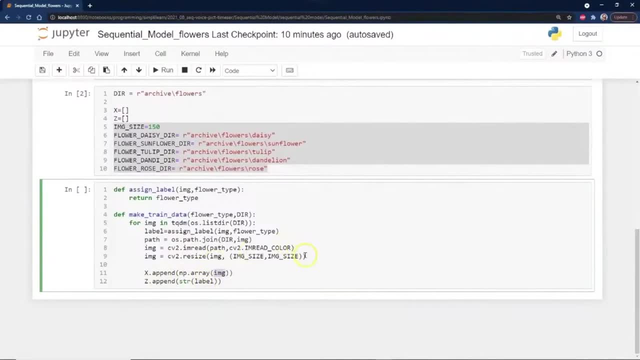 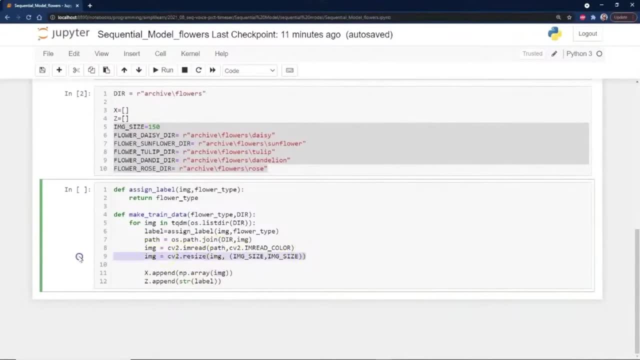 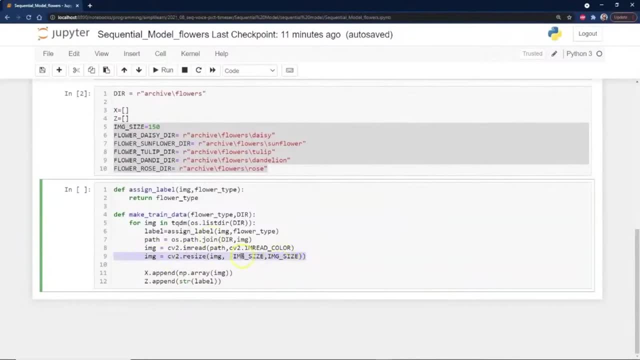 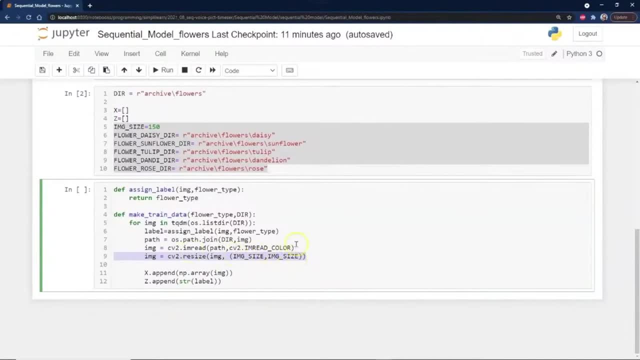 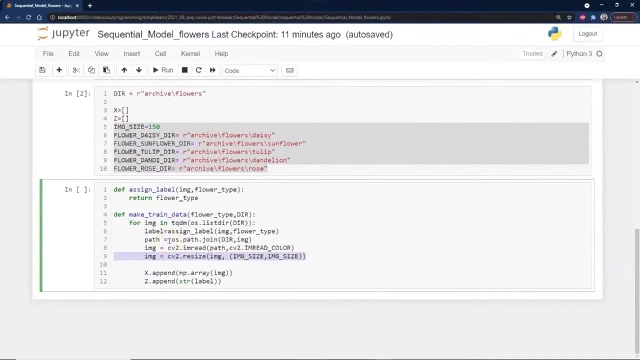 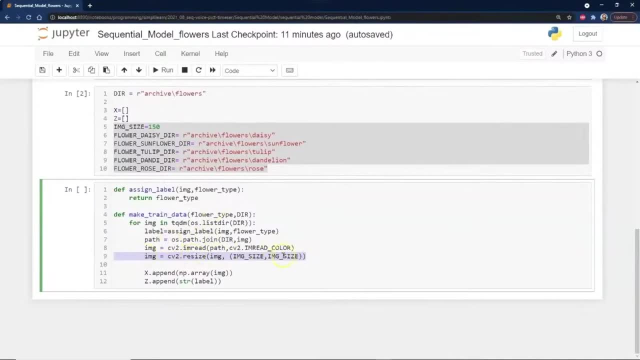 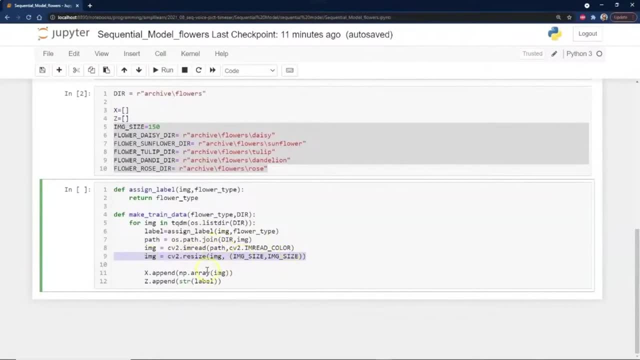 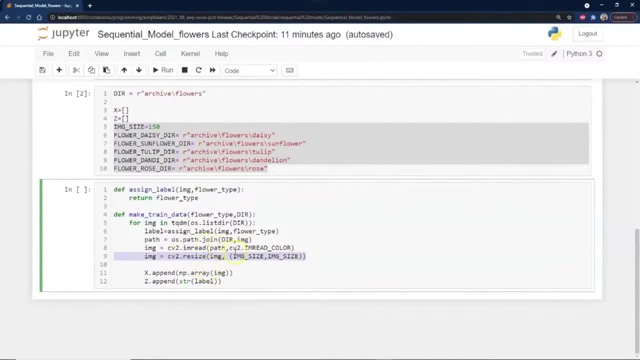 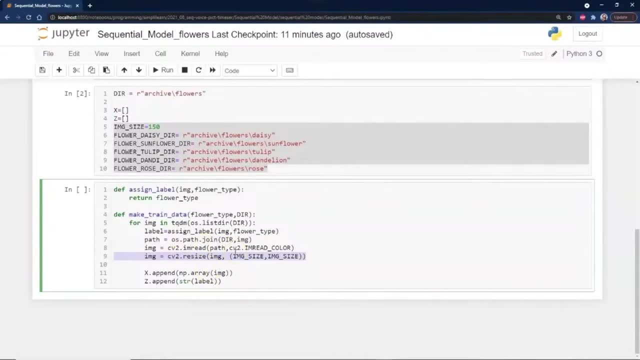 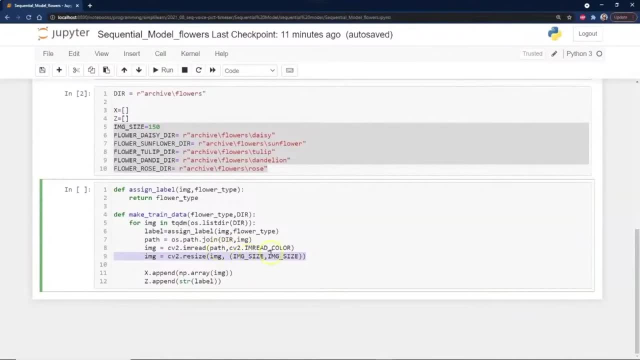 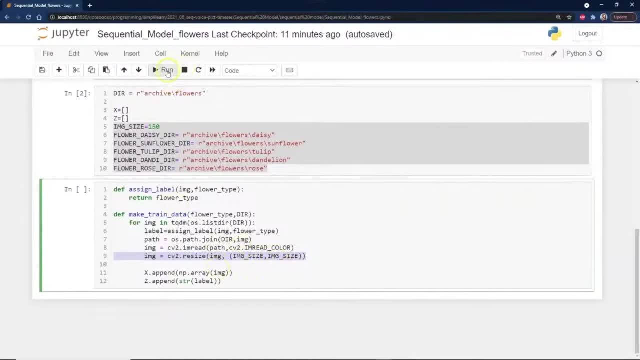 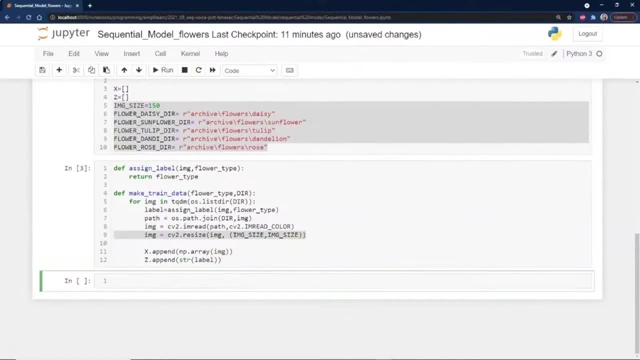 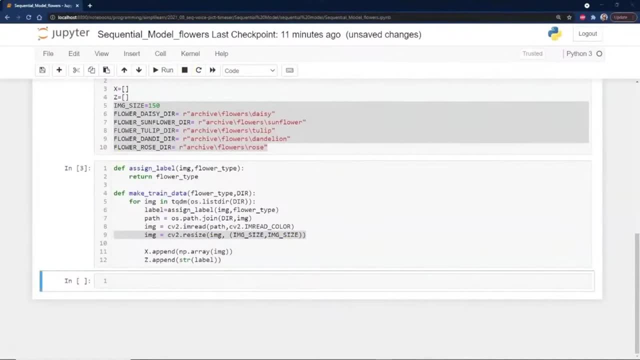 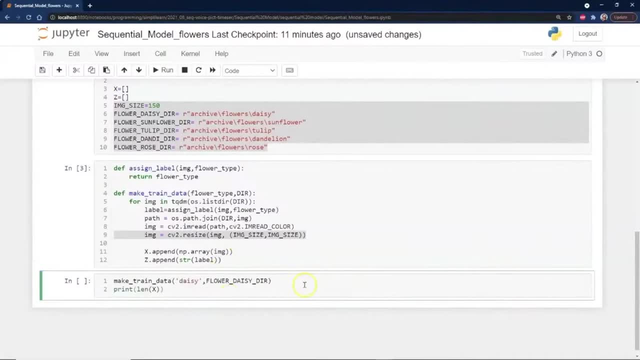 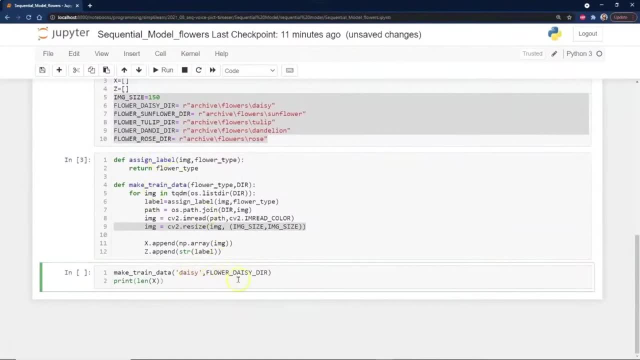 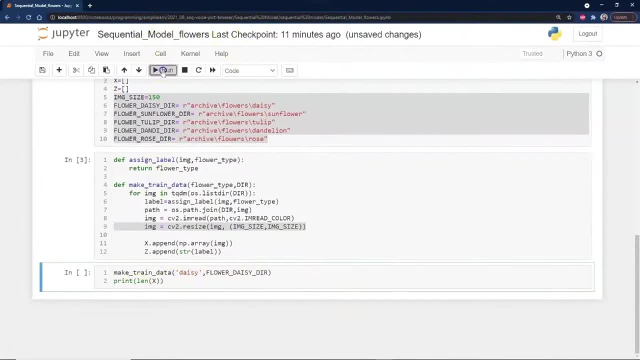 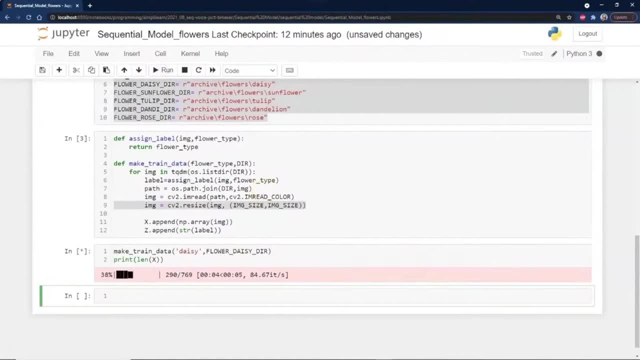 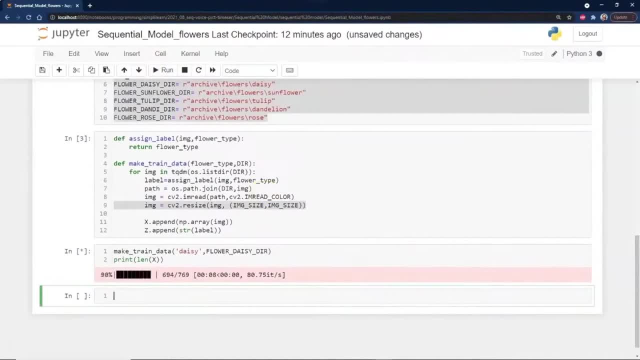 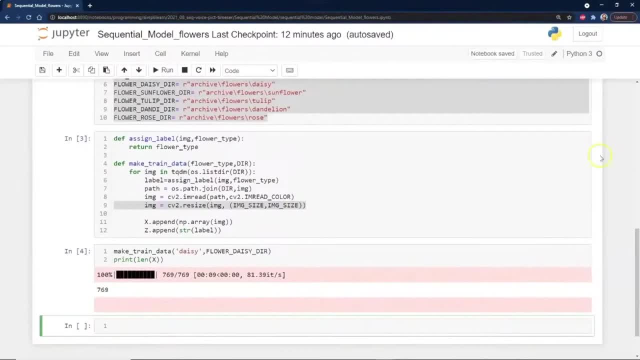 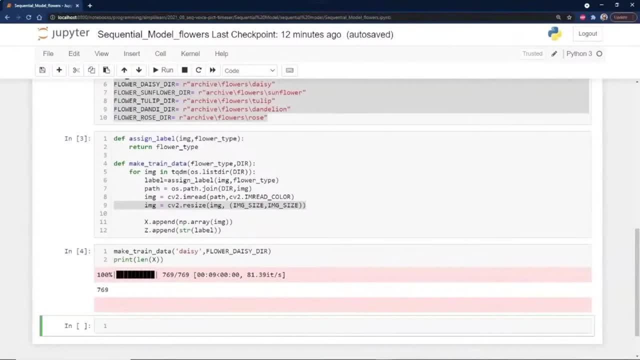 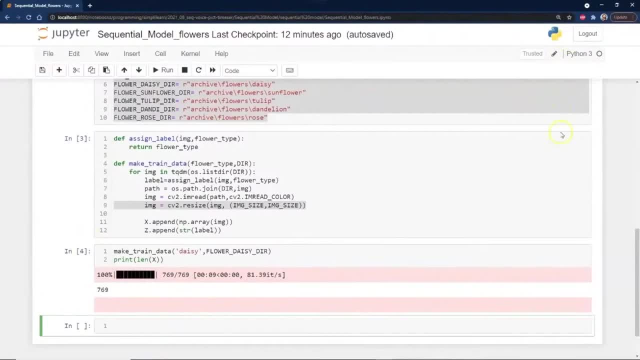 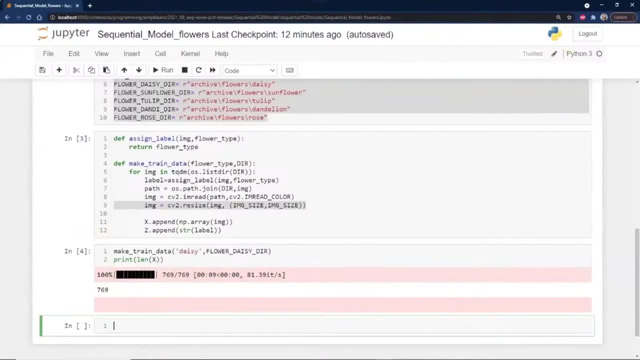 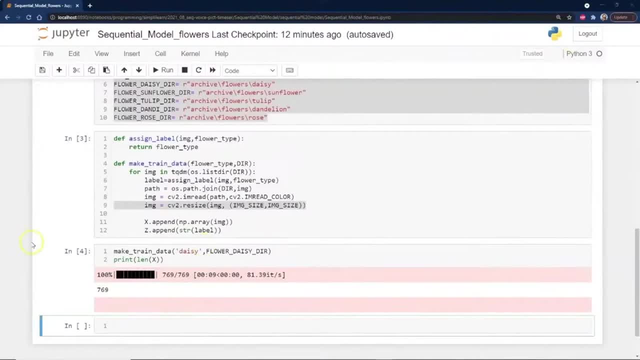 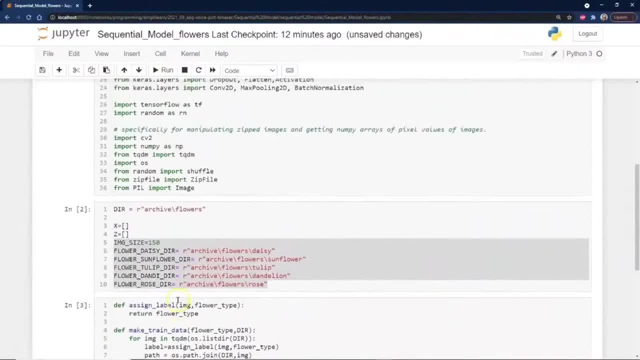 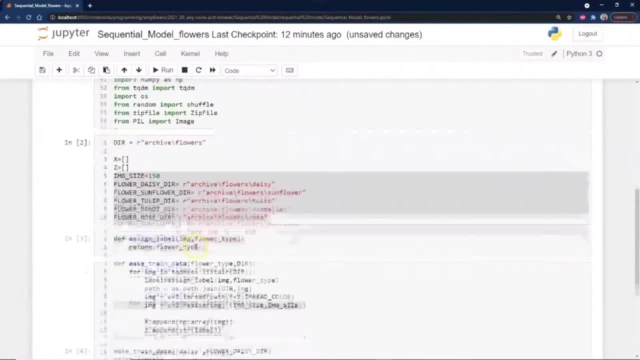 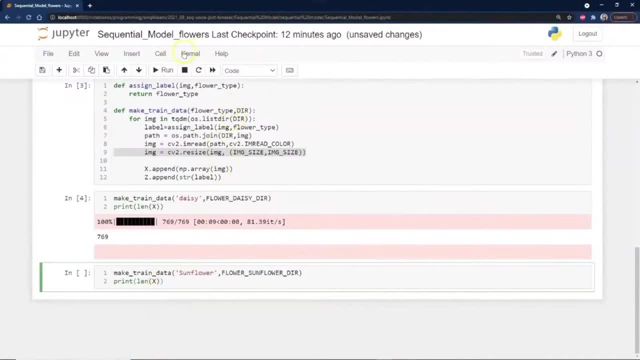 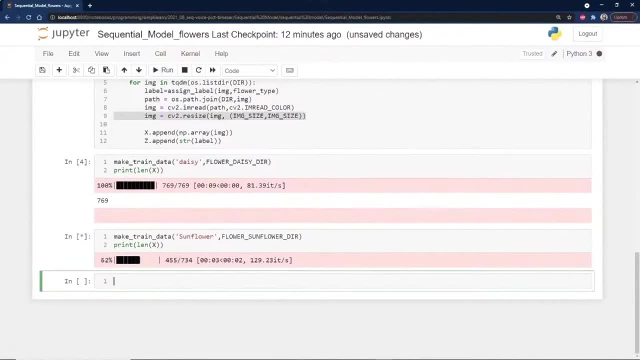 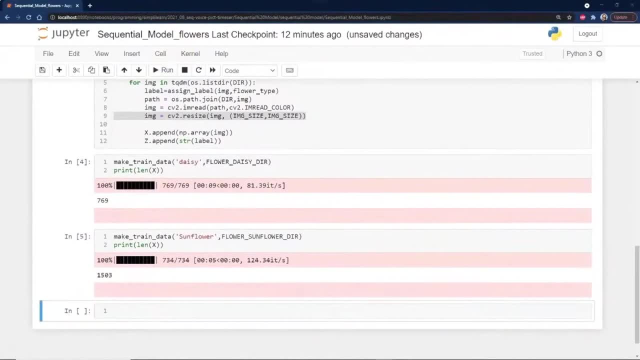 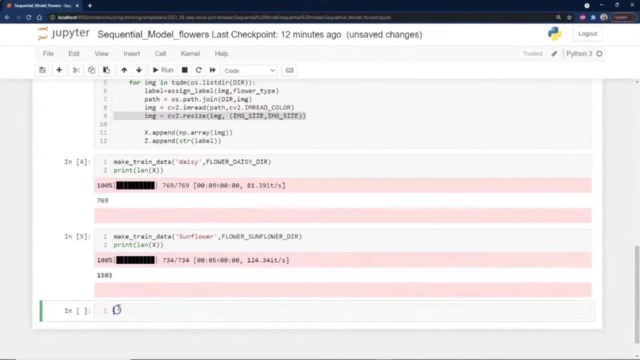 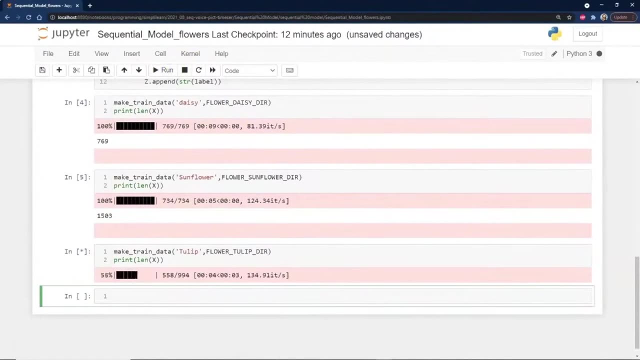 to show you something: It doesn't matter how good the people in the back are or how good you are programming. Errors are going to come up, and you got to figure out how to handle them. And so when we get all the way down to the where is it? Dandelion? Here's our dandelion directory. we're 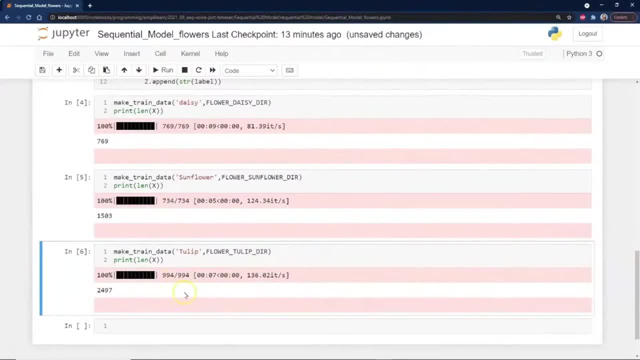 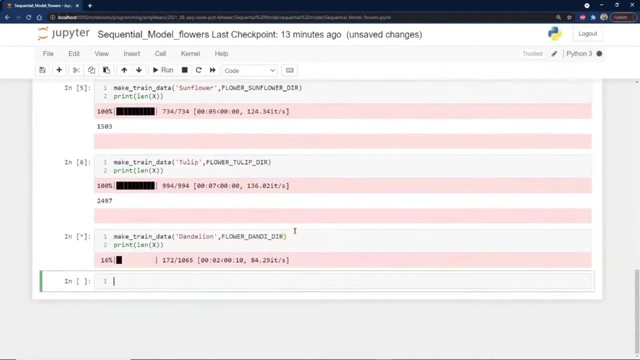 going to build. Jupyter has some cool things it does, which makes this really easy to deal with, But at the same time, you would want to go back in there, depending on how many times you rerun this, how many times you pull this, So when you're finding errors going in here there's a couple. 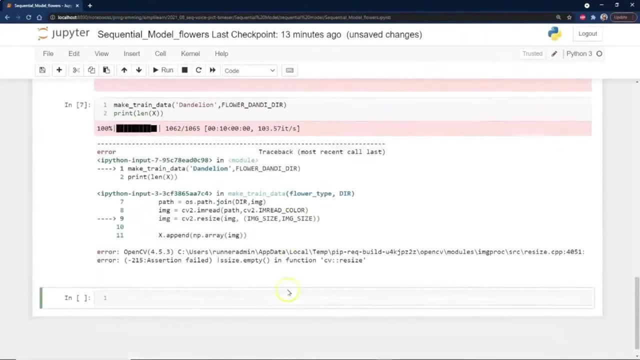 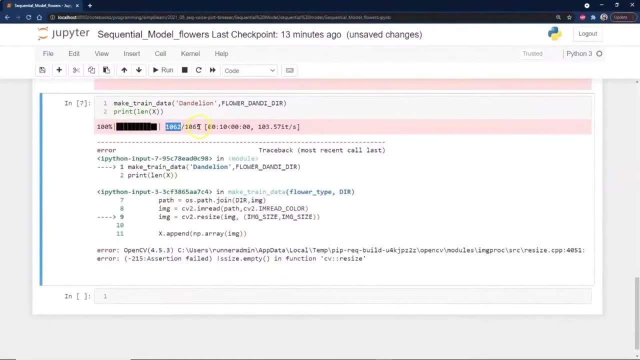 things you can do And we're just going to. oh, it wasn't, no, there it is. There's our error. I knew there was an error. This processed 1,062 out of 1,065.. Now I can do a couple things. One I could. 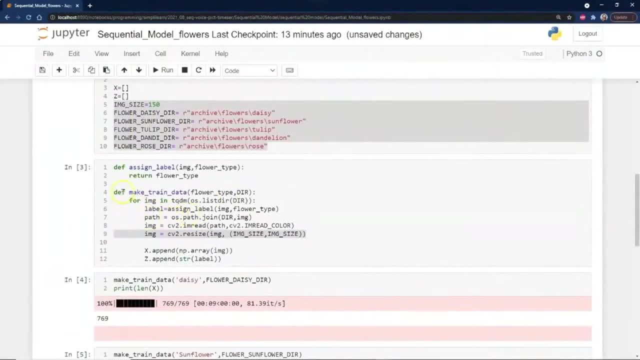 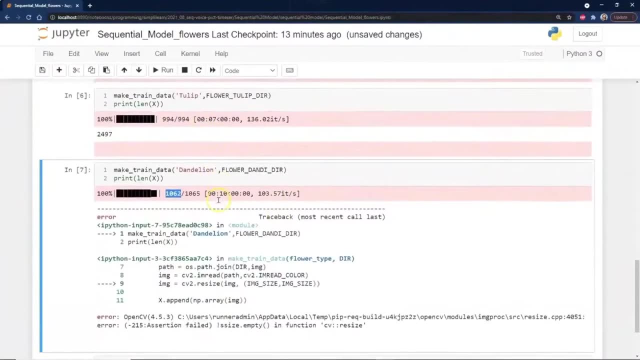 go back into our definition and I can just put in here: try And so if it has a bad conversion- because this is where the error is coming from- just skip it. That's one way to do it. When you're doing a lot of work in data science and you look 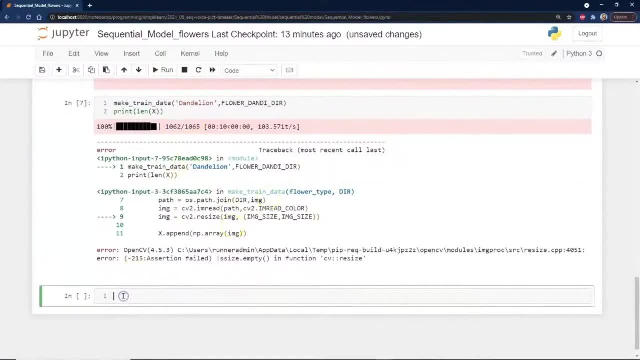 at something like this, where you're losing three points of data. at the end you just say, okay, I lost three points, Who cares? Or you can go in there and try to delete it. It really doesn't matter for this particular demo, And so we're just going to leave that. 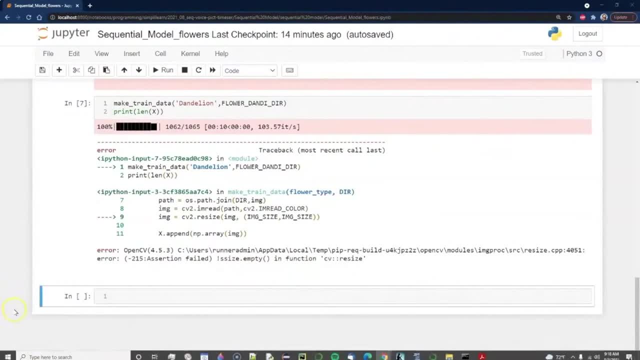 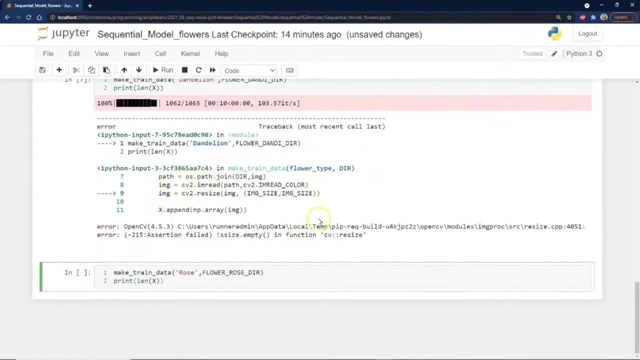 error right alone and skip over because it's already added all the other files in there. And this is a wonderful thing about Jupyter Notebook is that I can just continue on there and the X and Z which we're creating is still running And we'll just go right into the next. 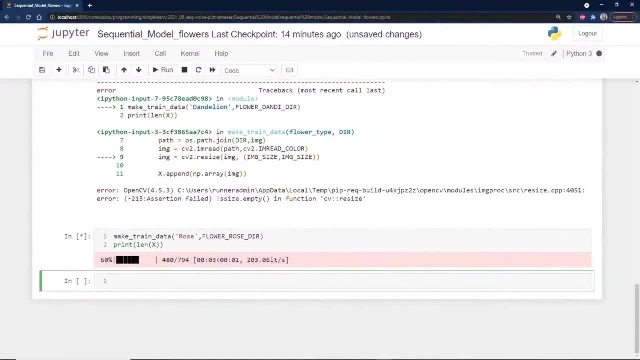 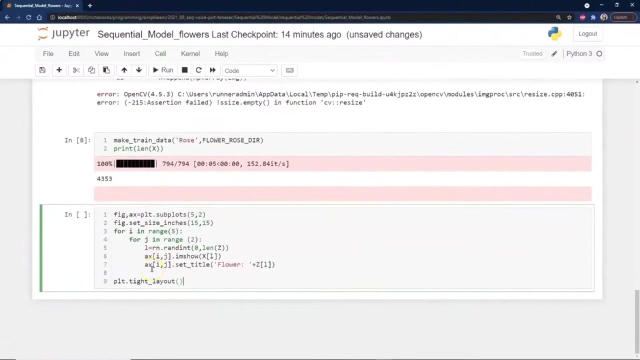 flower row, So all these flowers are in there. That's just a cool thing about Jupyter Notebook, And then we can go ahead and just take a quick look and see what we're dealing with- And this of course, really when you're dealing with a. 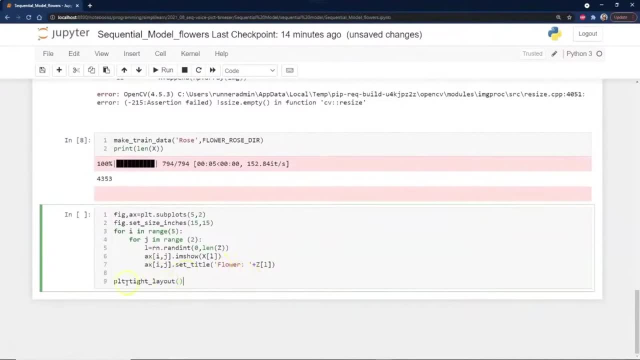 other people and showing them stuff. this is just kind of fun where we can display it on the plot library here And we're just going to go through and let's see what we got here Looks like we're going to do like five of each of them, I think. Is that how they set this up? 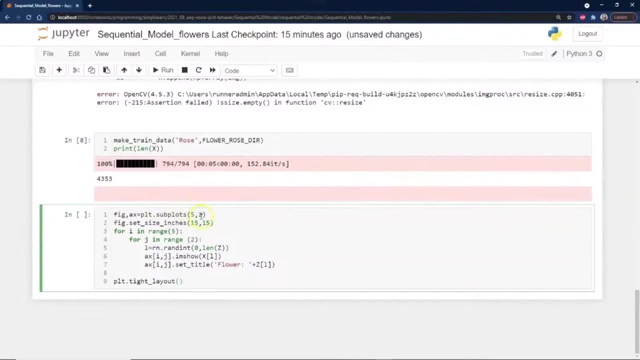 Plot library. five by two- Okay, Oh, I see how they did it. Okay, So two each. So we have five by two set up on our axes and we're just going to go in and look at a couple of these flowers. 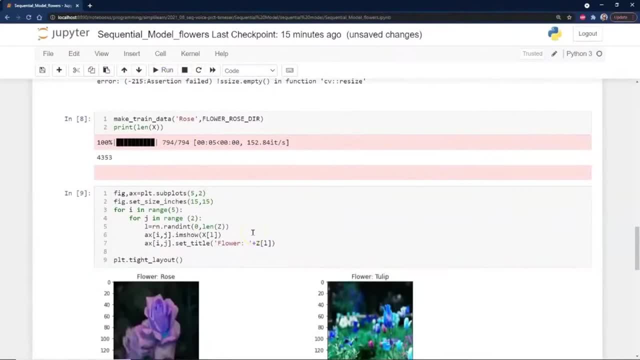 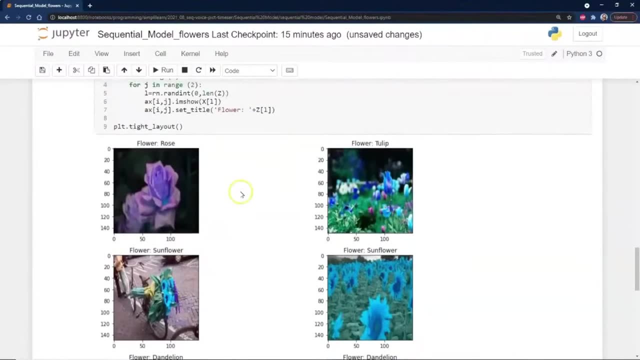 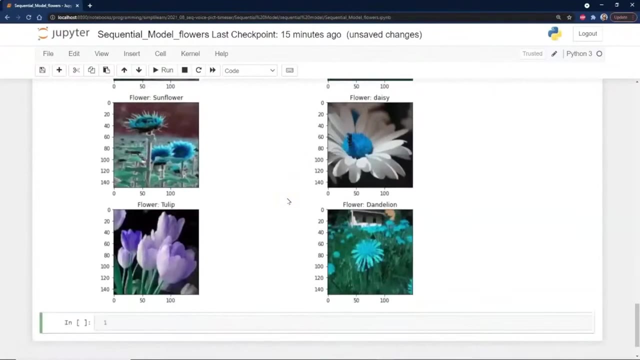 It's always a good thing to look at some of your data, No matter what you're doing. we reformatted this to 150 by 150.. You can see how it really blurs this one up here on the tulip. That is that resize to 150 by 150. And these are what's actually going in. These are: 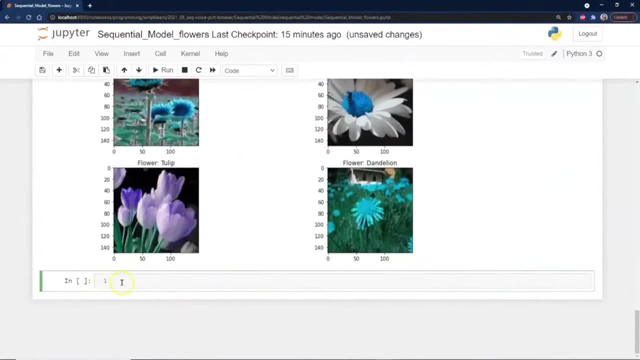 all 150 by 150 images. You can check the dimensions on the side and you can see just a quick sampling of the flowers we're actually going to process on here And again. like I said, we're not going to go into detail, But every single one of our things can be properly placed. 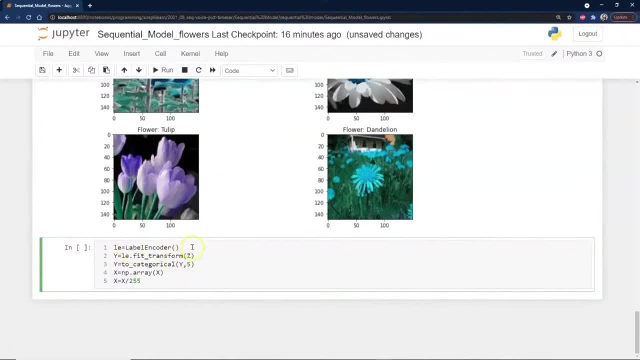 on here. Then we put in just a second of those five by four Click Play. And now it's here in the des Furthermore it module And again, like I said, all of this is leg CHTS and this is going to know- says focal. 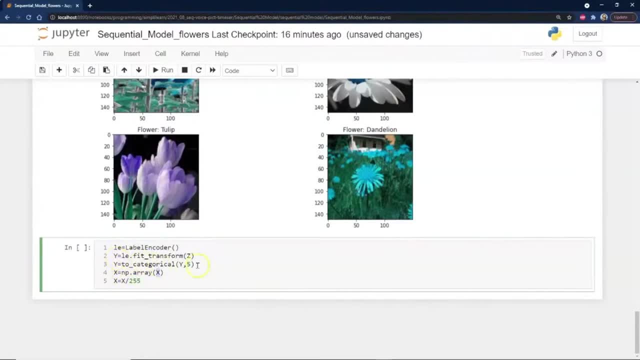 behavior of this item. It's now categorized. This is a style underences 樹. that's our z array we created, and then we have y, which equals that, and then we go ahead and do to categorical. we want five different categories and then we create our x in p array of x, x equals. 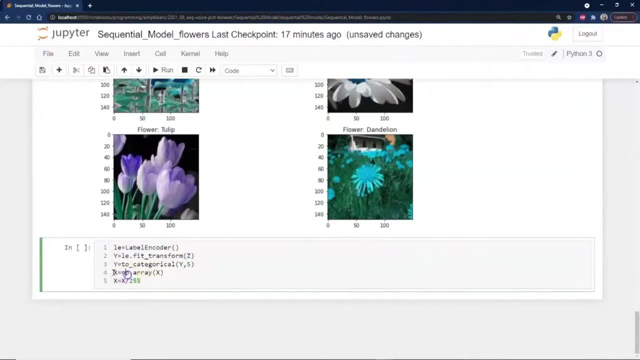 x over 255. so what's going on here? there's two different transformations. one, we've turned our categories into 0, 1, 2, 3, 4, 5 as the output and we have taken our x array. and remember, the x array is three values of your different colors. this is so important to understand when we do this. 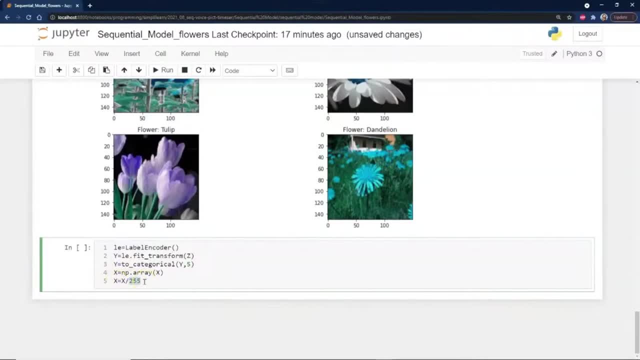 across a numpy array. this takes every one of those three colors. so we have 150 by 150 pixels. out of those 150 by 150 pixels, they each have three color arrays, and those color arrays range from zero to five. so we have two colors and then we have three colors and then we have 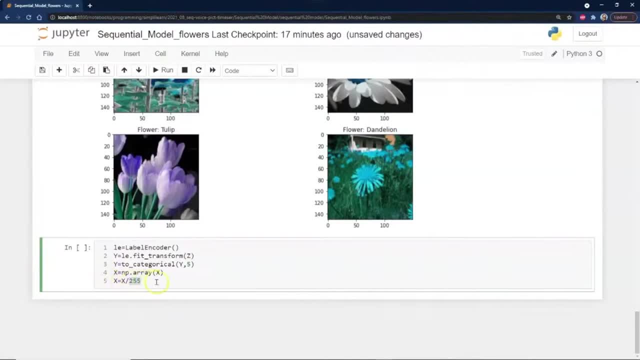 three color arrays and those color arrays range from zero to five. so we have three color arrays and 0 to 250.. So when we take the x equals x over 255,. I'm sorry, range from 0 to 255,. this converts. 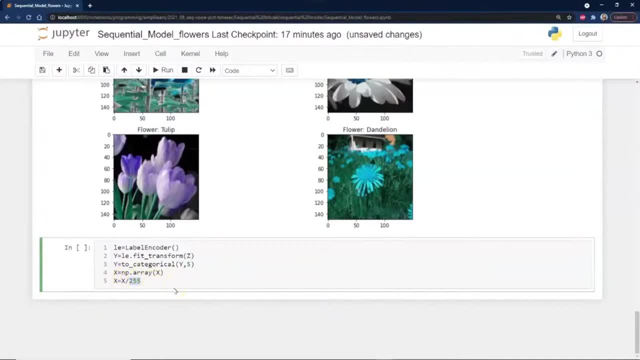 all those pixels to a number between 0 and 1. And you really want to do that when you're working with neural networks. Now, if you do a linear regression model, it doesn't affect it as much, and so you don't have to do that conversion if you're doing straight numbers. But when you're 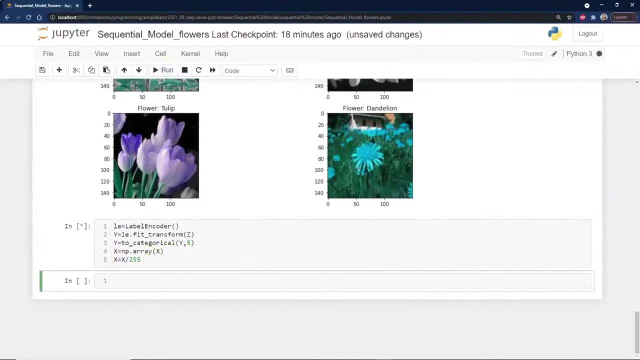 running neural networks. if you don't do this, you're going to create a huge bias And that means it'll do really good on predicting one or two things and they'll just totally die on a lot of other predictions. So now we have our x and y values, x being the data in, y being our. 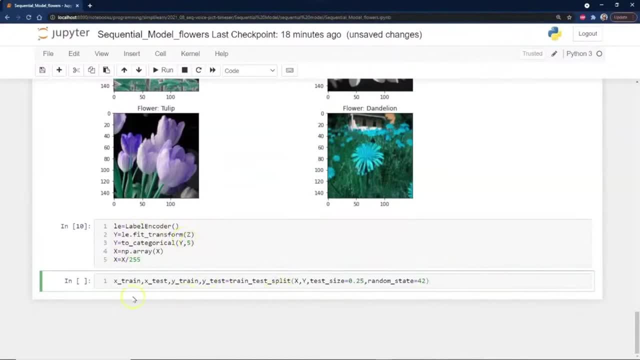 known output And, with any good setup, we want to divide this data into our training. So we have x train, we have our x test. This is the data. we're not going to program the model with And, of course, your y train course. 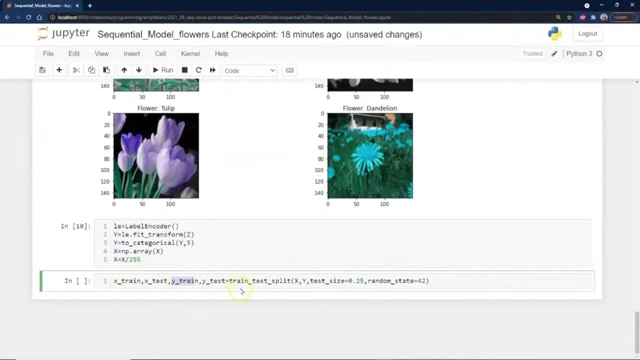 corresponds to your x train and your y test corresponds to your x test. the outputs, And this is when we do the train test split. this was from the scikit sklearn. We imported train test split and we're just going to go ahead and do the test size at about a quarter of the data: 0.25.. 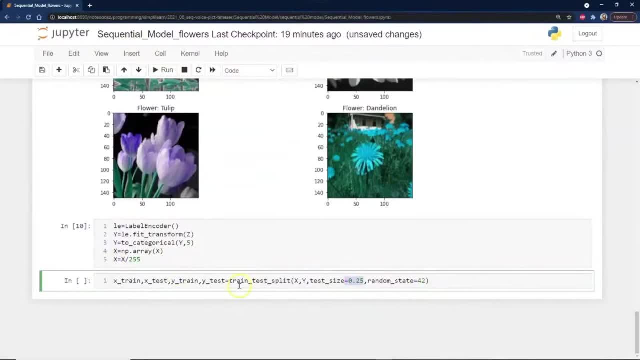 And of course random is always good. This is such a good tool. I mean certainly you can do your own division. You know you could just take the first, you know, 0.25 of the data or whatever do the length of the data. Not real hard to do. 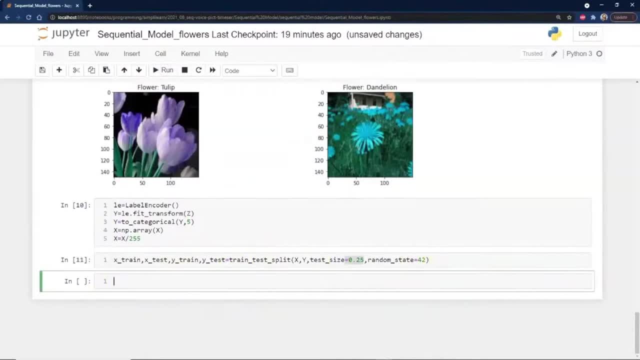 But this is randomized so that if you're running this test a few times, you can kind of get an idea whether it's going to work or not. Sometimes what I will do is I'll just split the data into three parts and then I'll test it on two, with one being the, or train it on two of those parts with one. 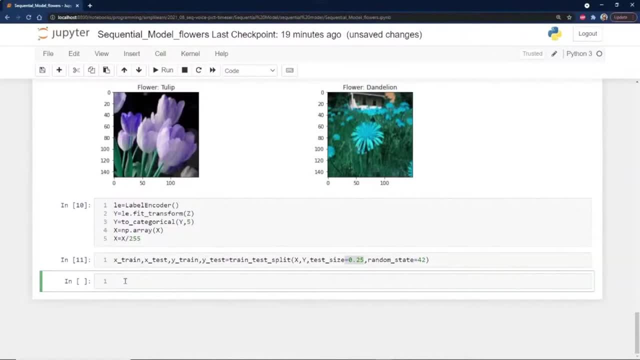 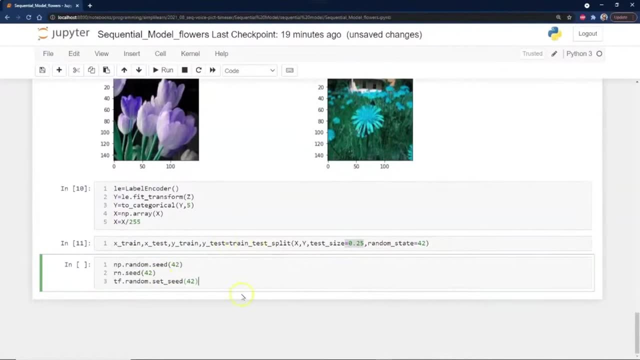 being the test, and I rotate it, So I come up with three different answers, which is a good way of finding out just how good your model is. But for setting up, let's stick with the x train, x test and the sklearn package. 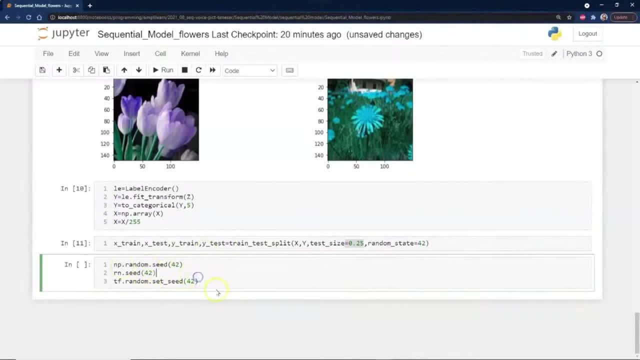 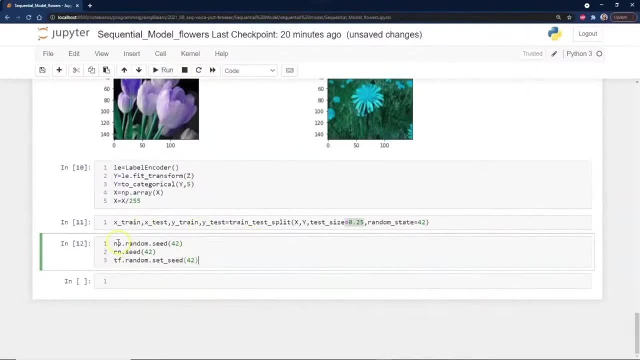 And then we're going to go ahead and do a random seed. Now, a lot of times across actually does this automatically, but we're going to go ahead and set it up on here And you can see, we did an NP random seed from 42, and we get a nice RN number And then we do tf random. we set the seed So you can set. 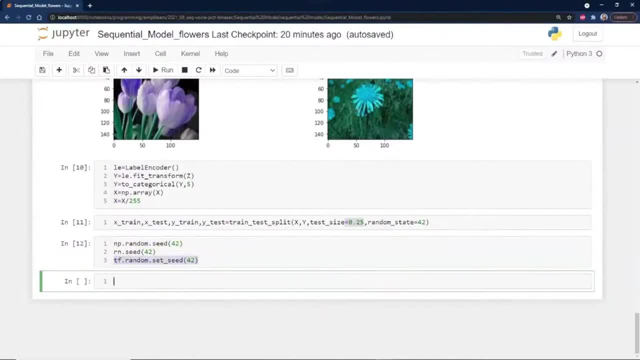 your randomness at the beginning of your tensor flow And that's what the tfrandomset is. So that's a lot of progress, All this prep, and then we finally get to the exciting part. This is where you probably spend once you have the data prepped and you have your pipeline going and you have everything set up on. 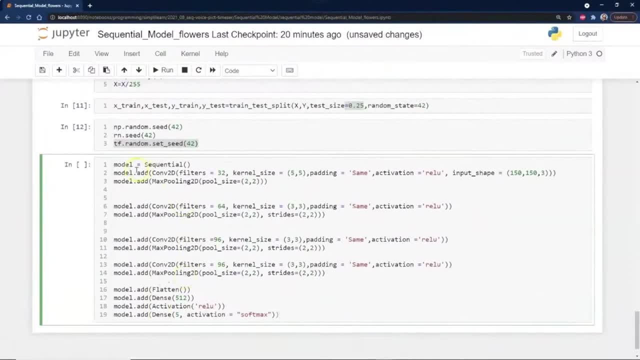 there. this is the part that's exciting- is building these models, And so we look at this model, one we're going to designate as sequential. They have the API, which is across the cross TensorFlow API. versus sequential, Sequential means we're going one layer to the next. 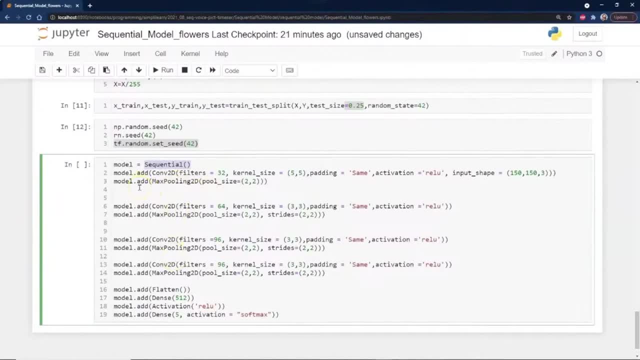 So we're not going to split the layer and bring it back together. It looks almost the same, with the exception of bringing it back together, So it's not a huge step to go from this to an API. And the first thing we're going to look at is our convolutional neural network in 2D. So what's going on here? 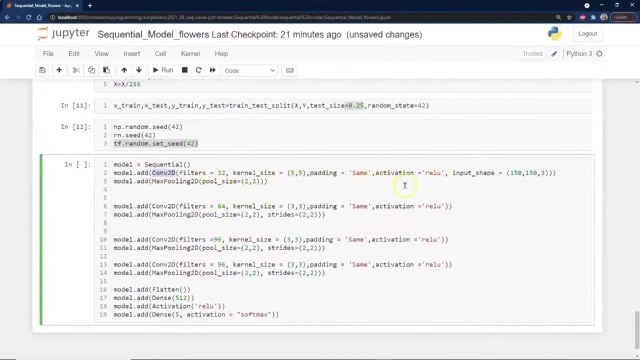 There's a lot of stuff that's going on here. The default for? well, let's start with the beginning. What is a convolutional 2D network? Well, a convolutional 2D network creates a number of small windows, And those small 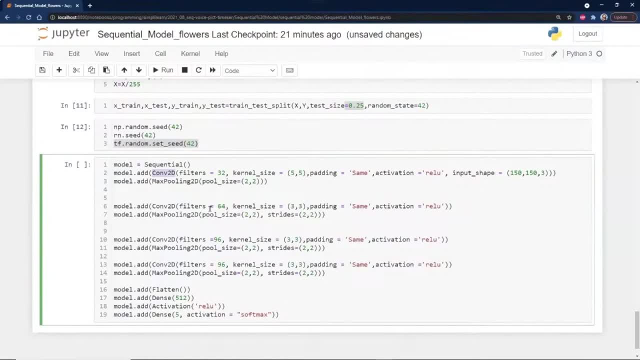 windows float over the picture and each one of them is their own neural network And this basically becomes like a categorization. And then it looks at that and it says, oh, if we add these numbers up a certain way, we can find out whether this is the right flower based on this little. 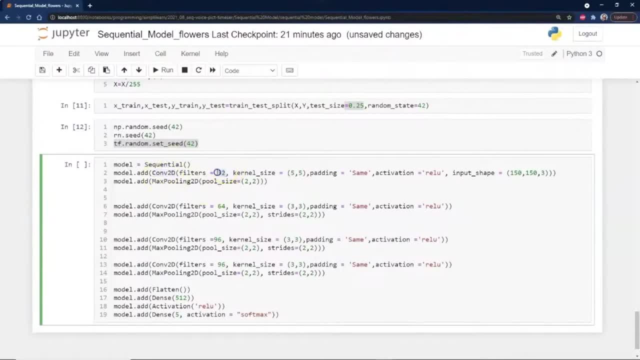 window floating around which looks at different things, And we have filters 32.. So this is everything that's going on here. So we have filters 32.. So this is everything that's going on here, And we have filters 32.. So this is everything that's going on here. So we have filters 32.. So this is. 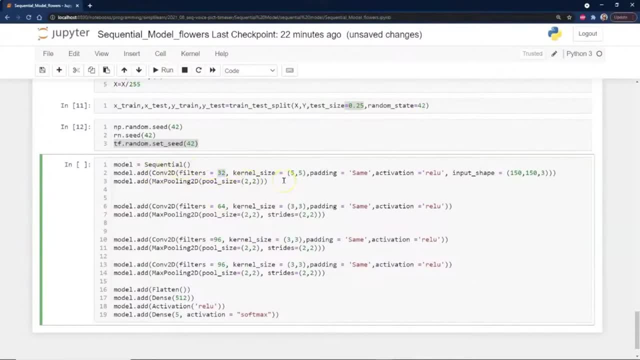 actually creating 32 windows is what that's doing. And the kernel size is five by five, So we're looking at a five by five square. Remember it's 150 by 150.. So this narrows it down to a five by. 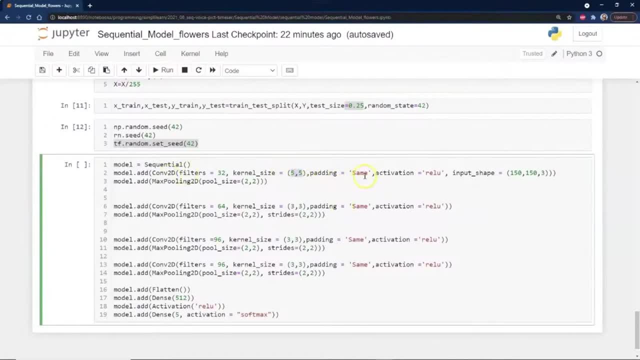 five. It's a 2D, So it has your x- y coordinates And we look at this five by five. Remember, each one of these is actually looking at five by five, by three, So we're actually looking at 15 by 15. 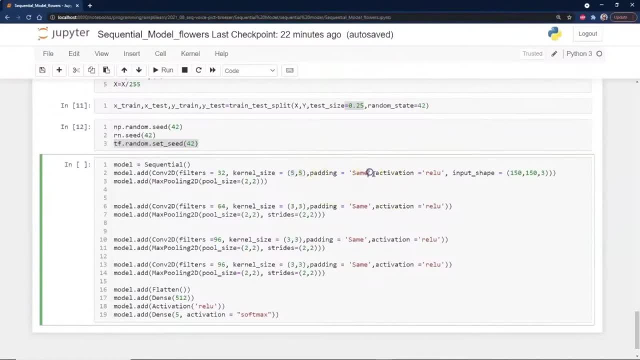 different pixels And padding is just usually. I just ignore that. Activation by default is ReLU. We went ahead and put the ReLU in there. There's a lot of different activations. ReLU is for your smaller. Remember I mentioned Atom. When you have a lot of data, use an Atom kind of activation or use an Atom. 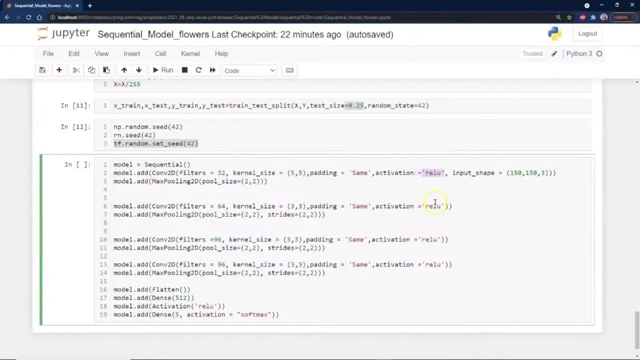 processing. We're using the ReLU here. It kind of gives you a yes or no, but it doesn't give you a full yes or no. It has a zero and then it kind of shoots off at an angle Very common- It's the most common one- And then of course here's our input shape: 150 by 150 by three pixels. 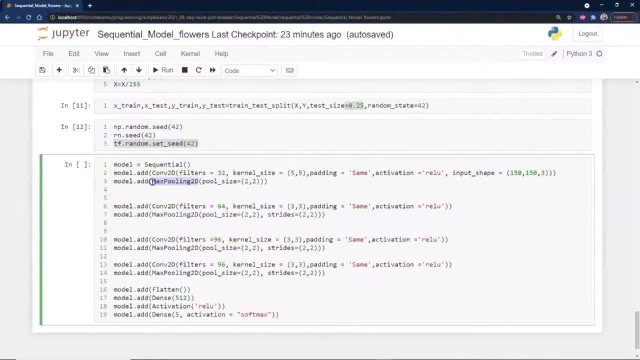 And then we have to pool it. So whenever you have a convolutional 2D layer, we have to bring this back together and pool this into a neural network, And then we're going to go ahead and repeat this, So we're going to add another network here. One of the cool things if you look at this is that, as it 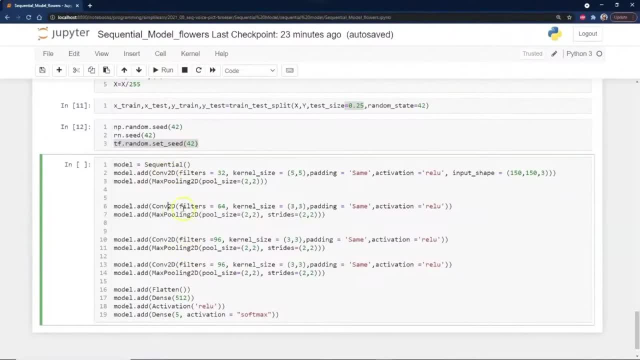 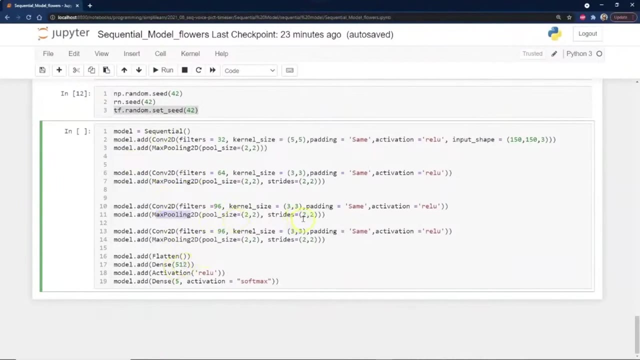 comes in, it just kind of automatically assumes you're going down to the next layer, And so we have another convolutional neural network 2D. Here's our max pooling again. We're going to do that again, max pooling, And we're just going to filter on down. Now, one of the things they did on this one. 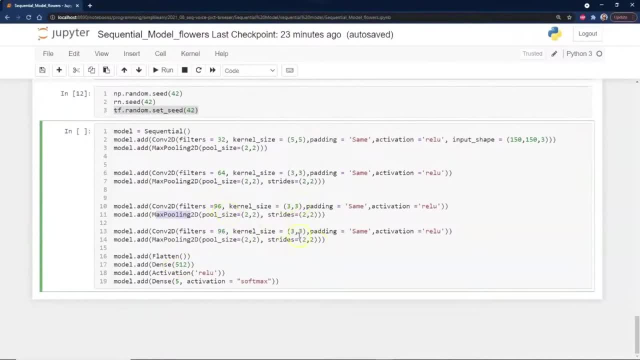 is they changed the kernel size, They changed the number of filters, And so each one of these steps kind of looks at the data a little bit differently. And that's kind of cool, because then you get a little added filtering on there. This is where you start playing with the model You might be looking. 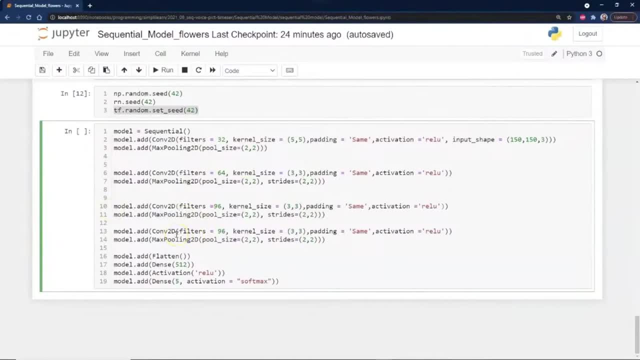 at a convolutional neural network, which is great for image classifications. We get down to here. One of the things we see is flattened, So we just flatten it. Remember, this is 150 by 150 by three. Well, and actually the pool size changes. It's actually smaller than that. Flatten just puts that. 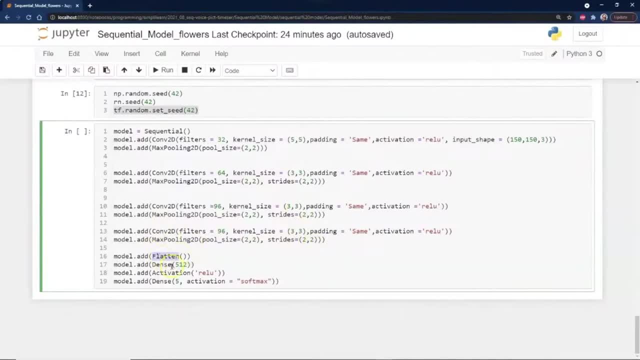 into a 1D array. So instead of being, you know, a tensor of this really complexity with the pixels and everything, it's just flat. And then the dense is just another activation on there. By default, it is probably ReLU as far as this activation. And then, oh yeah, here we go In sequential. 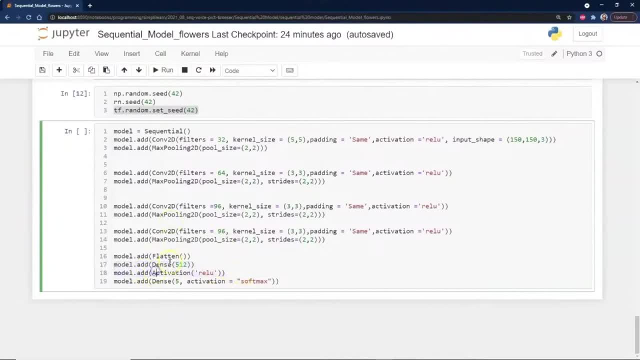 they actually added the activation as ReLU. So this just because this is sequential. this activation is attached to the dense And there's a lot of different activations, but ReLU is the most common one. And then we also see a softmax. Softmax is similar but it has its own kind of variation. 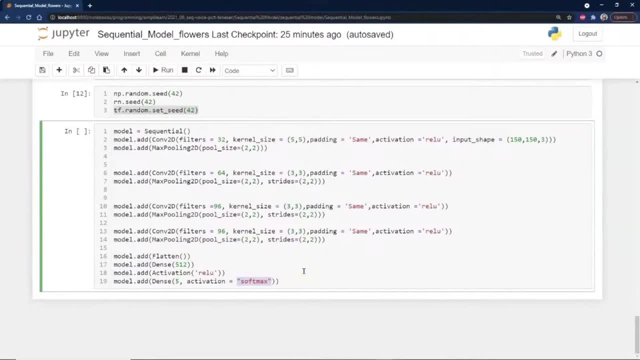 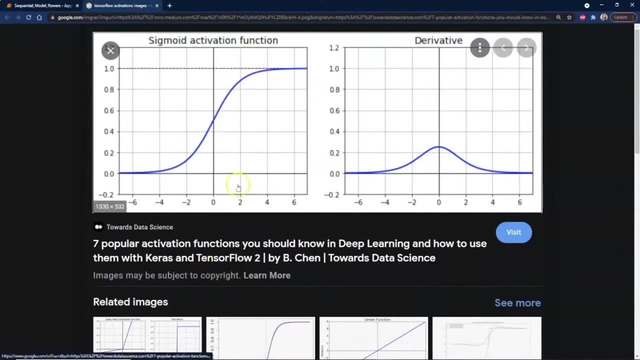 And one of the cool things you know what. let me bring this up because if you don't know about these activations, this doesn't make sense, And I just did a quick Google search on images of TensorFlow activations. I should probably look at which website this is, But this is the output of 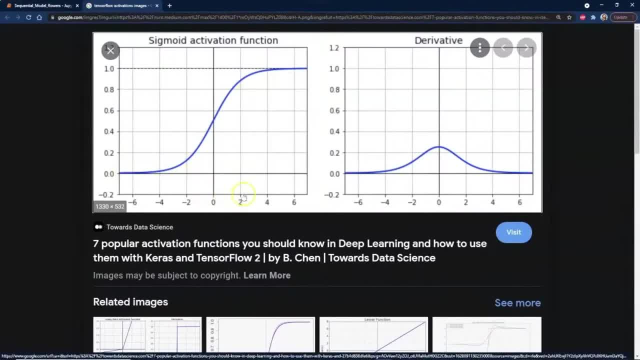 the values. So as your X, as it adds in all those weights, it adds in all those weights. So you can see it's going to activate it a certain way And that's a sigmoid activation And you can see it goes between 0 and 1 and has a nice curve there. This also shows the derivatives. And if we come 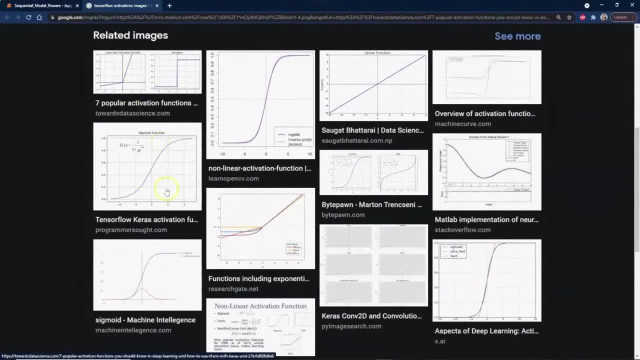 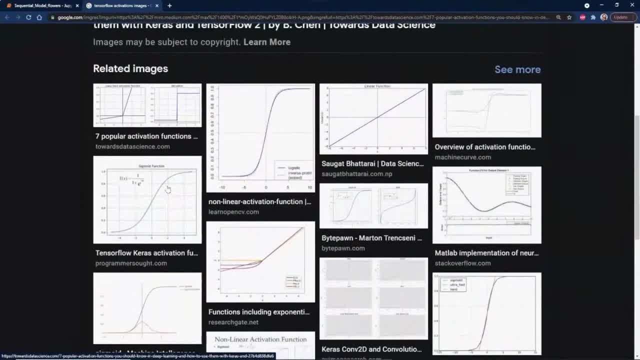 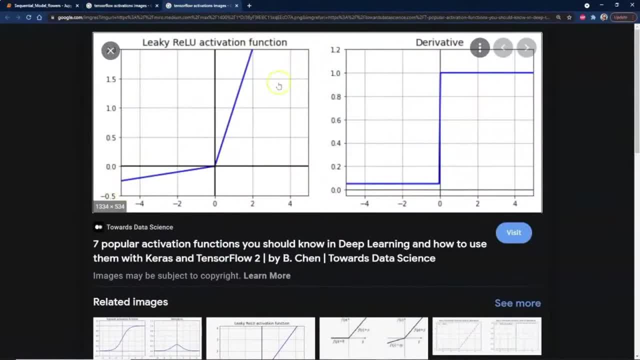 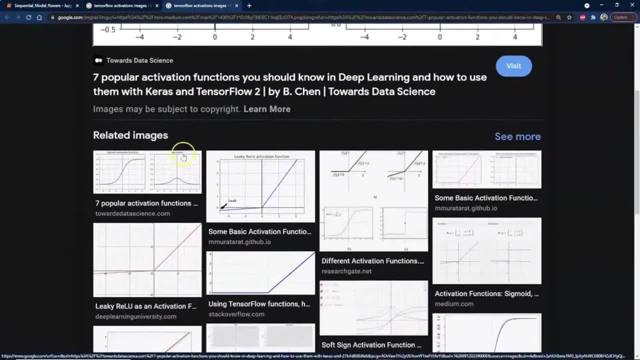 leaky ReLU And you can see, instead of it just being 0 and then a value between going up, it has a little leaky there. Otherwise your ReLU loses some nodes. They just become inactive. But you can see there's a lot of different options here. Here's a good one right here with the ReLU. You can see. 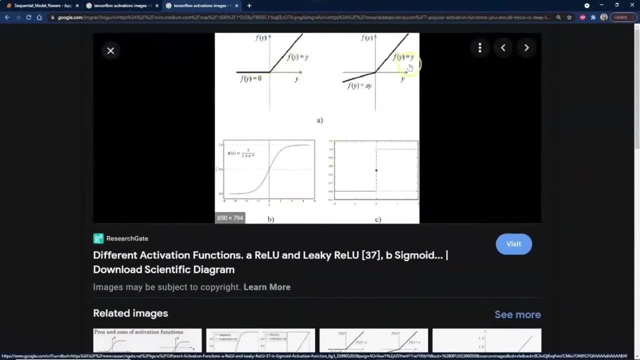 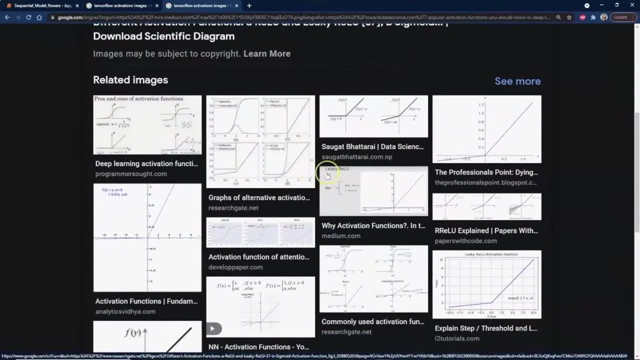 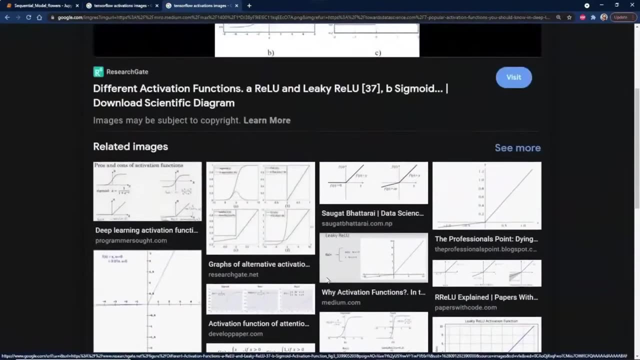 the ReLU function on the upper left here And then the leaky ReLU over here on the right, which is very commonly used also. One of the things I use with processing language is the, you know, the exponential one, or the tangent H, the hyperbolic tangent, because they have that nice funky curve. 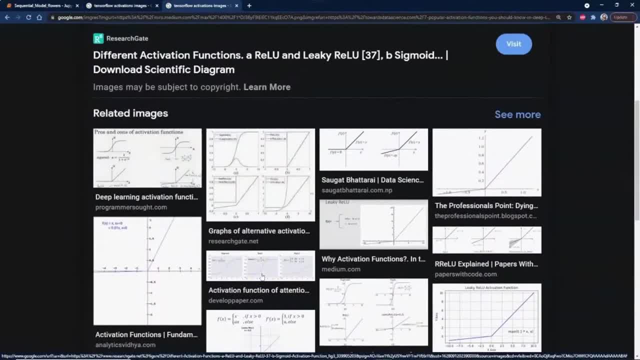 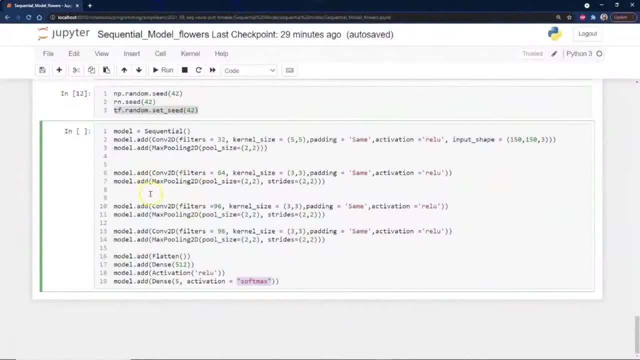 that comes in that has a whole different meaning and captures word use better. Again, these are very specific to domain and you can spend a lot of time playing with different models. For our basic model, we'll stick to the ReLU and the Softmax on here And we'll go ahead and run and build this. 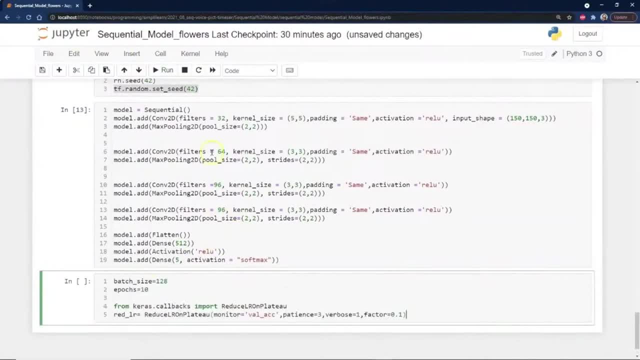 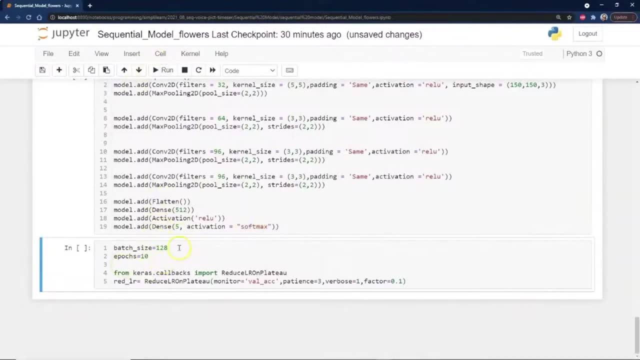 model. So now that we've had fun playing with all these different models and different models that we can add in there, we need to go ahead and have a batch size on here: 128, Epyx 10.. This means that we're going to send 128 rows of data or flowers at a time to be processed And the 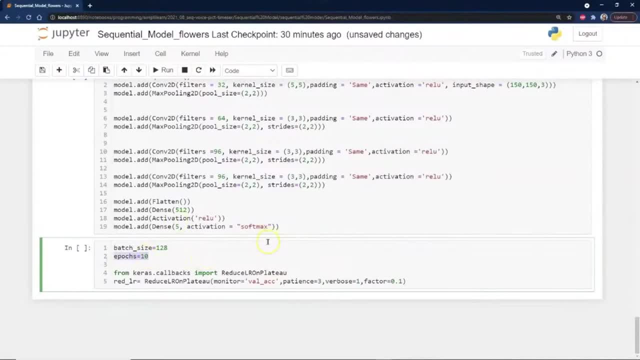 Epyx 10, that's how many times we're going to loop through all the data, And then there's all kinds of stuff you can do Again. this is now built into a lot of cross models already. You can see here that it's actually by default, So there's different ways to reduce the values And verbose equals. 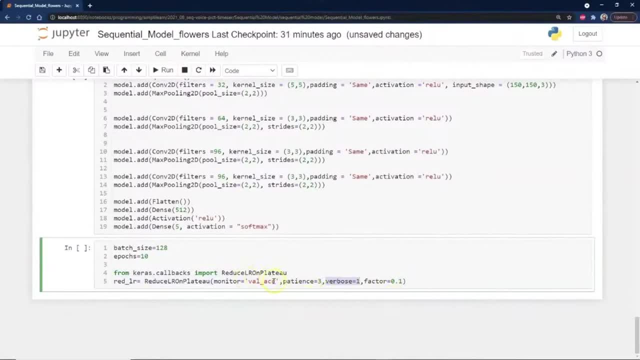 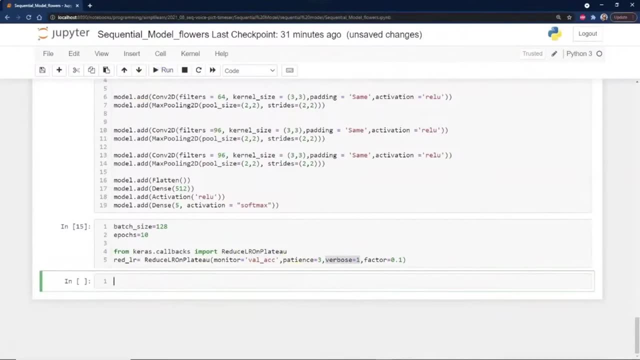 one means that we're going to show what's going on, Value, what we're monitoring. We'll see that as we actually train the model, This is what's going to come out of there. If you set the verbose equal to zero, you don't have to watch it train the model, although it is kind of nice to actually. 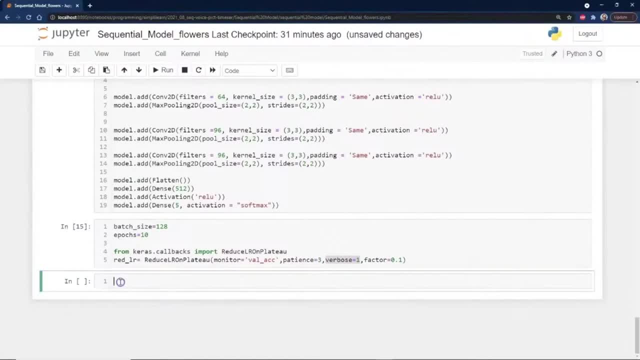 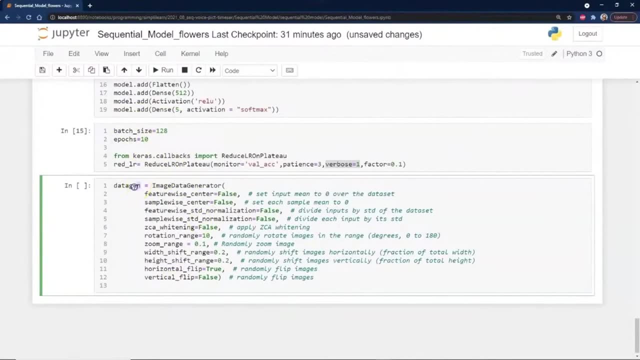 know what's going on sometimes, And since we're still working on bringing the data in- here's our batch size, here's our Epyx- we need to go ahead and create a data generator. This is our image data generator And it has all the different settings in. 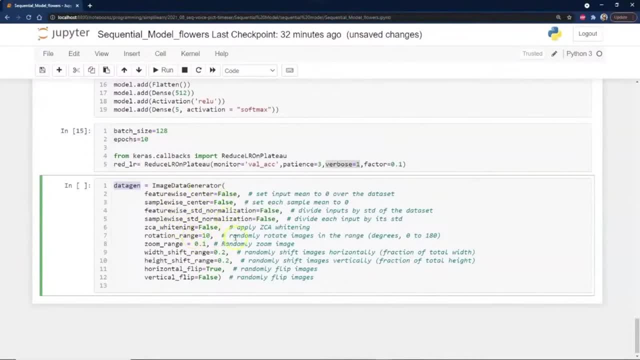 here. Almost all of these are defaults. So if you're looking at this going, oh my gosh, this is confusing. most of the time you can actually just ignore most of this Vertical flip so you can randomly flip pictures. You can randomly horizontally flip them, You can shift the picture around. 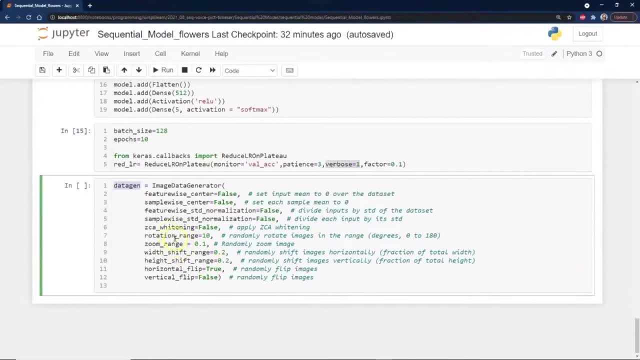 This kind of helps gives you multiple data off of them. Zooming rotation- there's all kinds of different things you can do with images. Most of these we're just going to leave as false. We don't really need to do all. 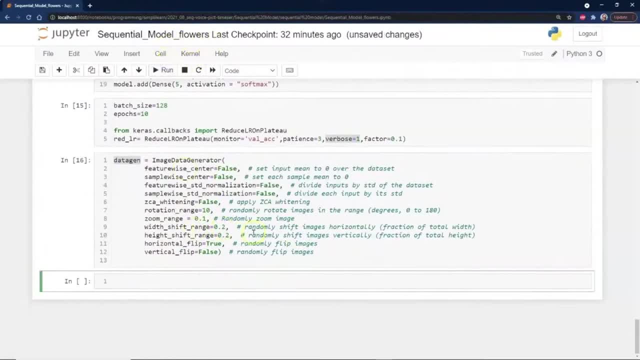 that setup because we already have a huge amount of data. If you're short data, you can start flipping like a horizontal picture and it will generate. it's like doubling your data almost, So the upside is you double your data. The downside is that if you already have a bias in your data, you already have. 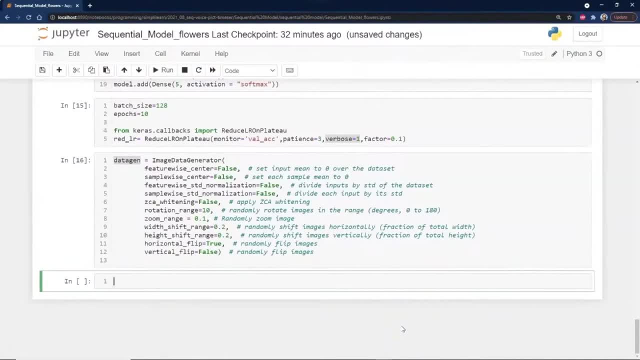 5,000 sunflowers and only two roses. that's a huge bias. It's also going to double that bias. That is the downside of that. And so we have our model compile and this you're going to see in all the Keras We're going to take. 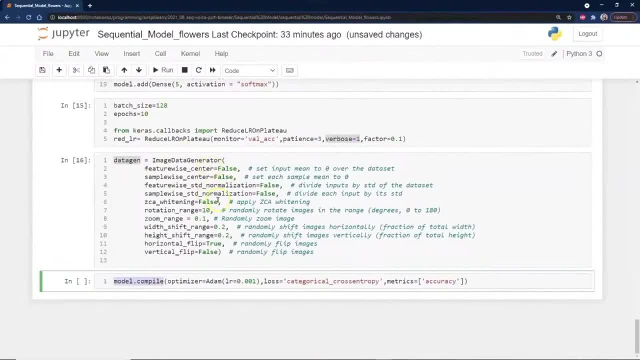 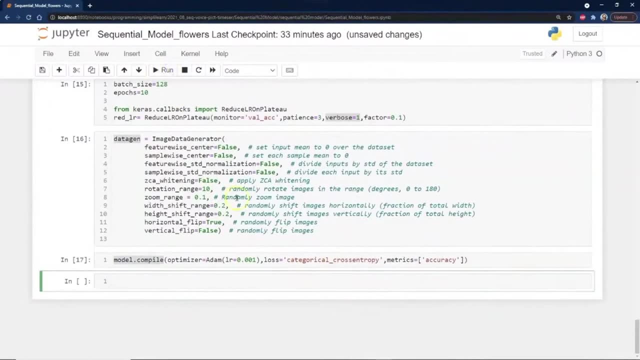 this model here. We're going to take all this information as far as how we want it to go and we're going to compile it. This actually builds the model and so we're going to run that And I want you to notice there we have the default learning rate, Very important. this is the default: 0 0 1.. 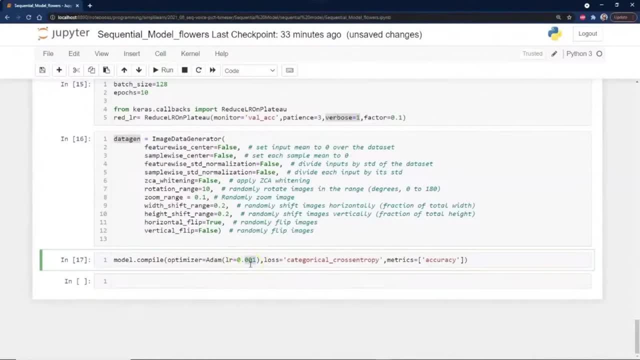 There really don't change. It's how slowly it adjusts to find the right answer, And the more data you have, you might actually make this a smaller number. you have a very small sample of data. you might go even larger than that, And then we're going to look at 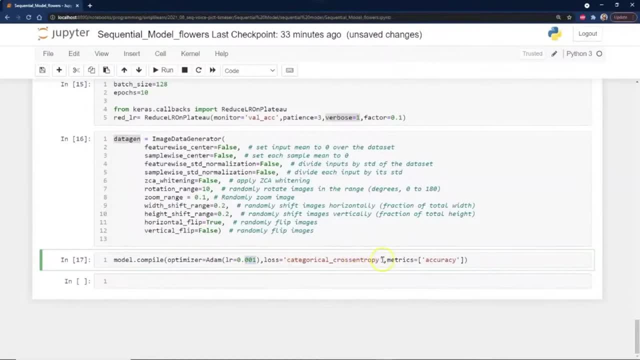 the loss: categorically Categorical cross-entropy most commonly used, and this is how we're used in a lot of This is how much it improves the model is. improving is what this number means. That's important on there, And then the accuracy. 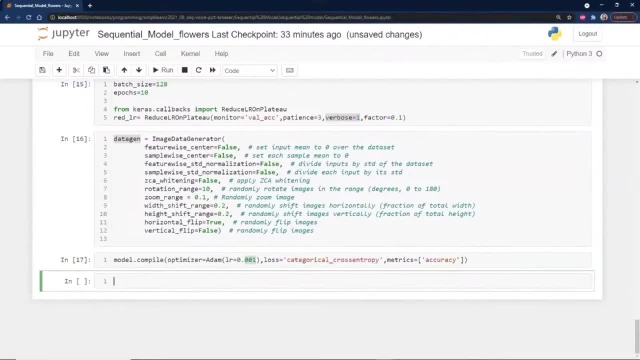 We want to know just how good our model is on the accuracy, And then one of the cool things to do is if you're in a group of people who are studying the model. if you're in shareholders you don't want to do this is you can run the model. 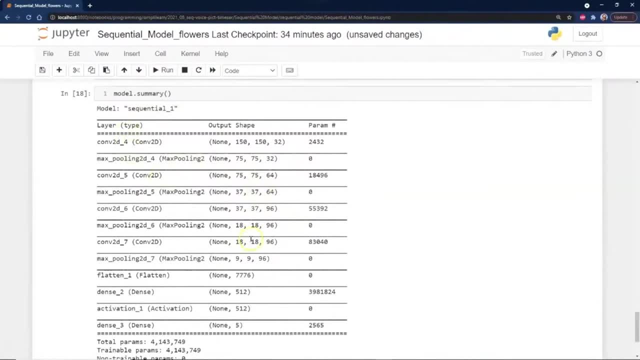 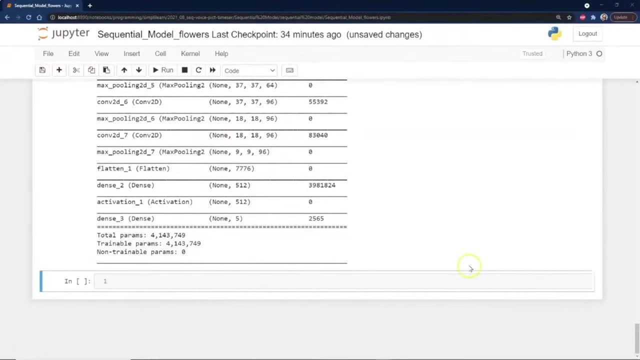 summary. I do this by default and you can see the different layers that you built into this model. Just a quick summary on there. So we went ahead and we're going to go ahead and create a. we'll call it history, but we. 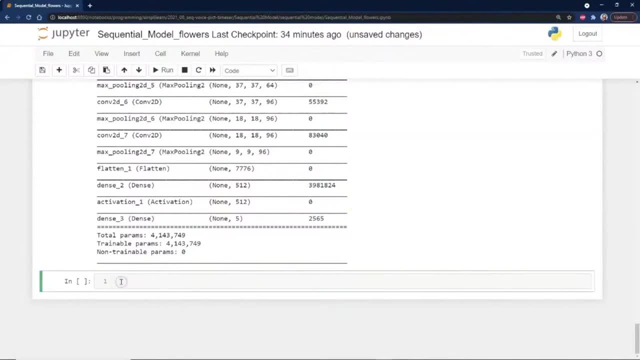 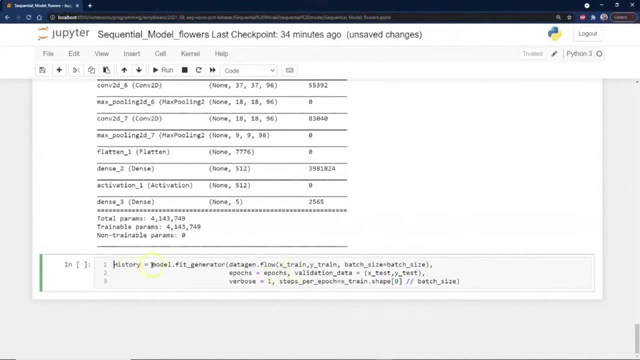 want to do a model fit generator, And so what this history is doing is this is tracking what's going on as while it fits the model. Now there's a lot of new setups in here where they just use fit and then you put the generator. 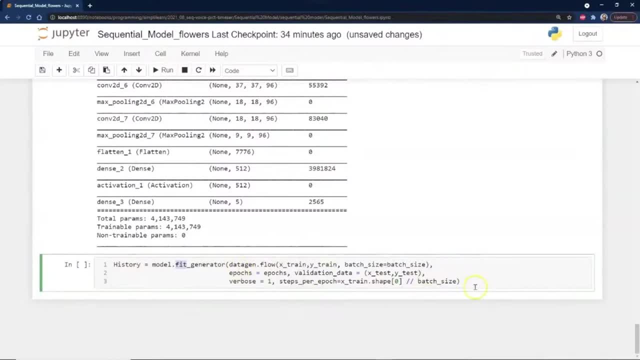 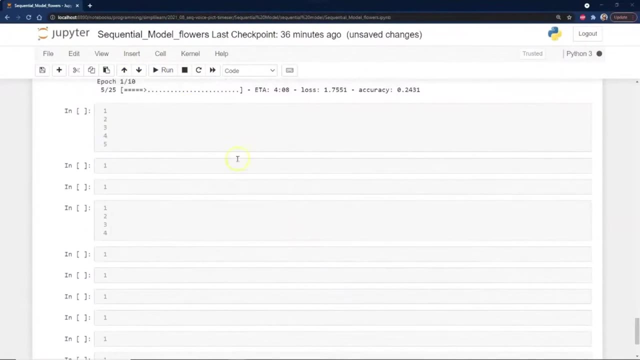 in here. We're going to leave it like this, Even though the new default There's a little different on. that Doesn't really matter, Does the same thing? And we'll go ahead and just run that You can see while it's running. right here we're going through the epics. 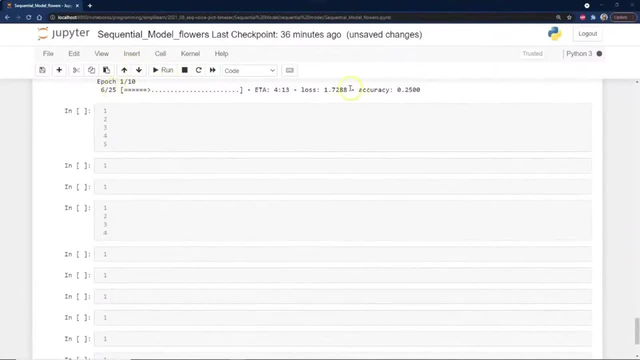 We have one of 10.. Now we're going through six to 25.. Here's our loss. We're printing that out so you can see how it's improving and our accuracy. The accuracy gets better and better. And this is six out of 25.. 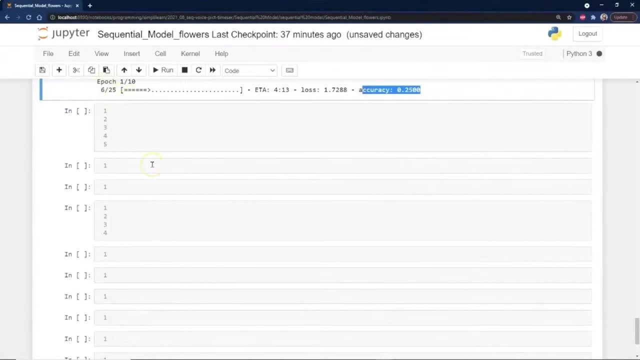 This is going to take a couple minutes to process Because we are training 150 by 150, by three pixels, across six layers or eight layers, whatever it was. That is a huge amount of processing, So this will take a few minutes to process. 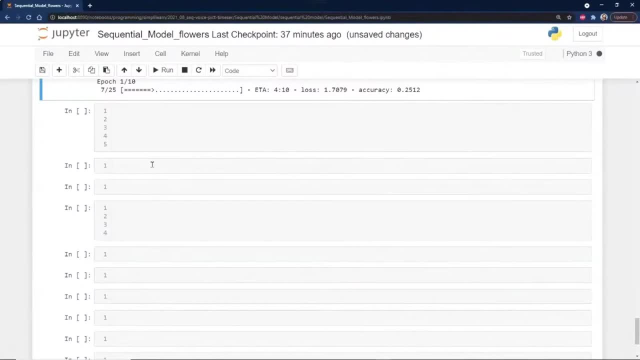 This is when we talk about the hardware and the problems that come up in data science and why it's only now just exploding being able to do neural networks. This is why this process takes a long time. Now you should have seen a jump on the screen here. 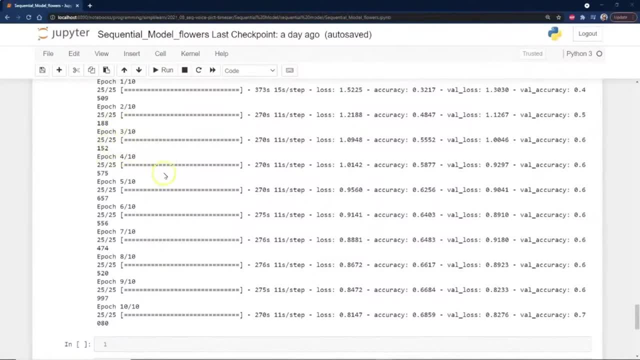 Because I did pause the recorder to let this go ahead and run all the way through its epics. Let's go ahead and take a look and see what these epics are, And if you set the verbose to zero instead of one, it won't show what's going on in the 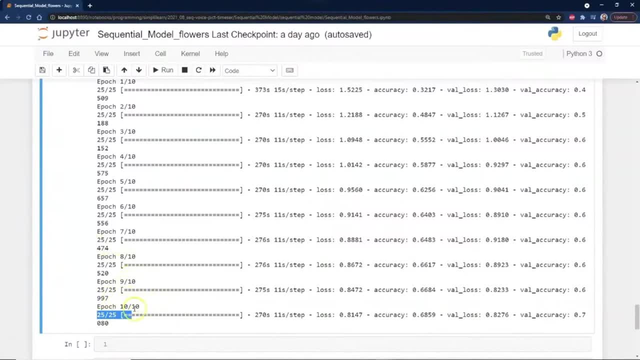 behind the scenes as it's training it. So we look at this epic: 10 epics. We went through all the data 10 times. If I remember correctly, there's roughly a gig of data there, so that's a lot of data. 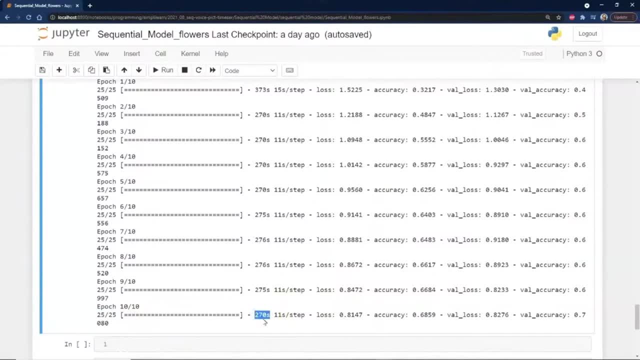 The first thing you're going to notice is the 270 seconds. That's how much each of those epics took to run, And so if you divide 60 in there, you roughly get about five minutes worth of each epic. So if I have 10 epics, that's 50 minutes, almost an hour of runtime. 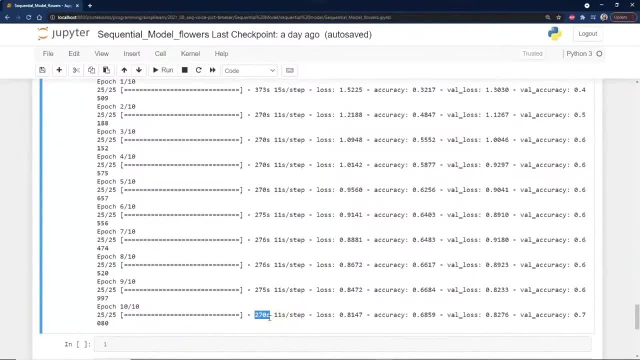 That's a big deal when we talk about processing. On this particular computer I actually have- what is it? eight cores with 16 dedicated threads, So it runs like a 16-core computer. It alternates the threads going in And it still takes it five minutes for each one of these epics. 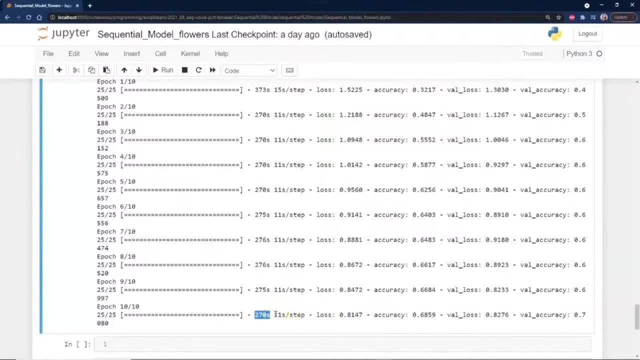 So you start to see that if you have a lot of data, this is going to be a problem. if you have a number of models, you want to find out how good the models are doing and what model to use, And so each of those models could take all night to run. 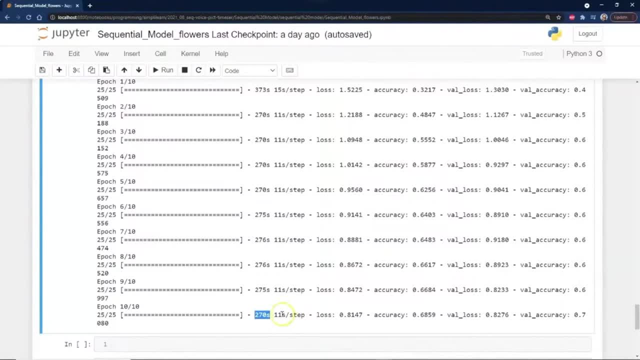 In fact I have a model I'm running now that takes about a day and a half to test each model. It takes four days to do the whole data. So what I do is I actually take a small piece of the data, I test it out to find out, get an idea of how the different setups are going to do. 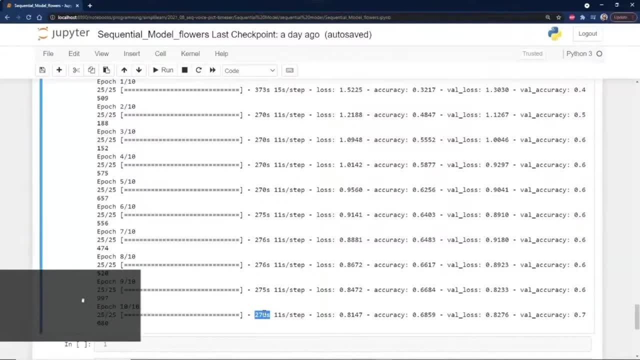 And then I increase that size of the data and then increase it again And I can just take that curve and kind of say, okay, if the data is doing this, then I need to add in more dense layers or whatever. So you can do small chunks of data and then figure out what it costs to do a large set. 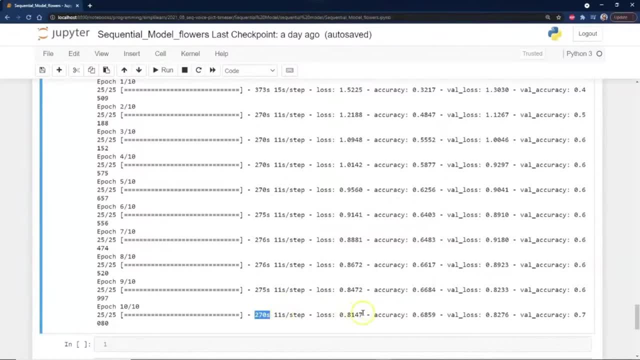 of data and what kind of model you want. The loss, as we see here, continues to go down. This is the error. This is the error. This is how much error is in there. It really isn't a user-friendly number, other than the more it trends down, the better. 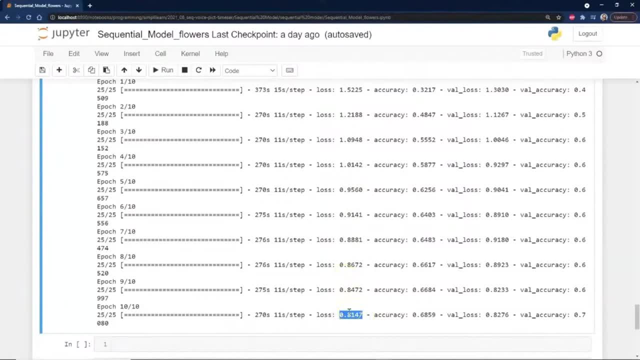 And so if you continue to see the loss going down, eventually you'll get to the point where it stops going down and it goes up and down and kind of wavers a little bit. At that point you know you've run too many epics. 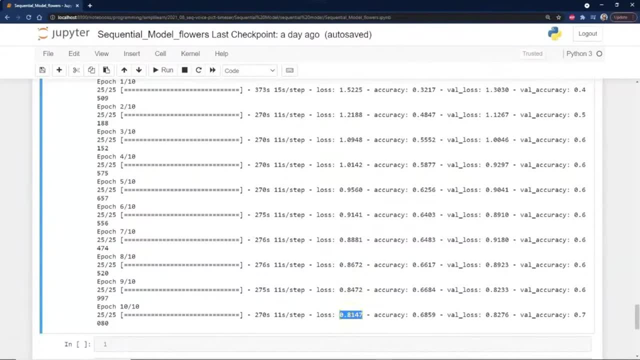 You're starting to get a bias in there, and it's not going to give you a good model fit. The accuracy just turns this into something that we can use, And so the accuracy is: what percentage of guesses? in this case, it's categorical, so 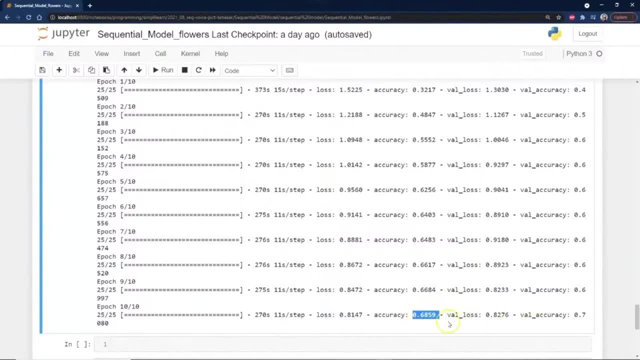 this is the percentage of guesses are correct. Value loss is similar, you know, minus a value loss, And then you have the value accuracy and you'll see the value accuracy is pretty similar to the accuracy, Just rounds it off, basically. 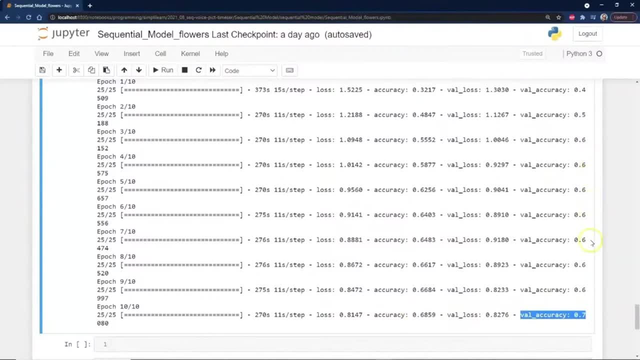 And so a lot of times you come down here and you go: okay, we're doing 0.5, 0.6, 0.7.. And that is 70% accuracy, or in this case, 68.7.. 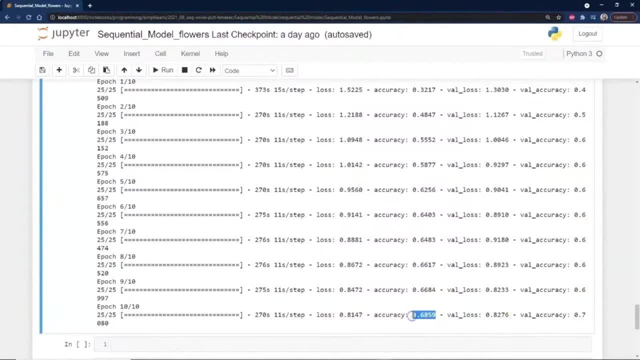 So that's pretty good. Okay, So that's 5, 9% accuracy. That's a very usable number and it's very important to have If you're identifying flowers. that's probably good enough if you can get within a close. 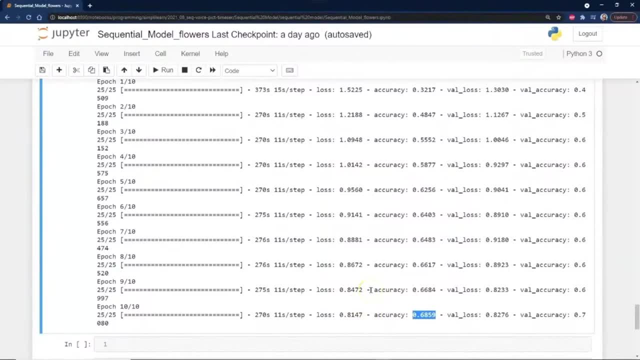 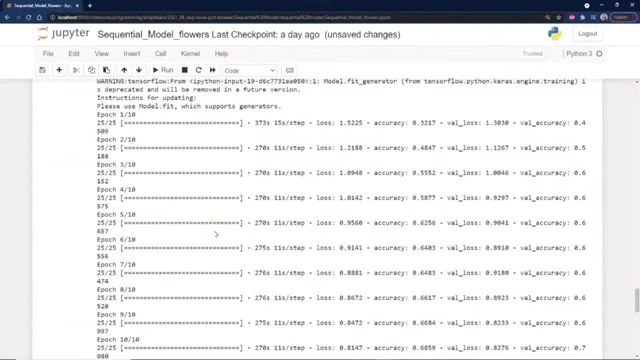 distance and knowing what flower you're identifying. If you're trying to figure out whether someone's going to die from a heart attack or not, you might want to rethink it a little bit or rekey how you're building your model. So if I'm working with a group of clients, shareholders in a company, or something like, 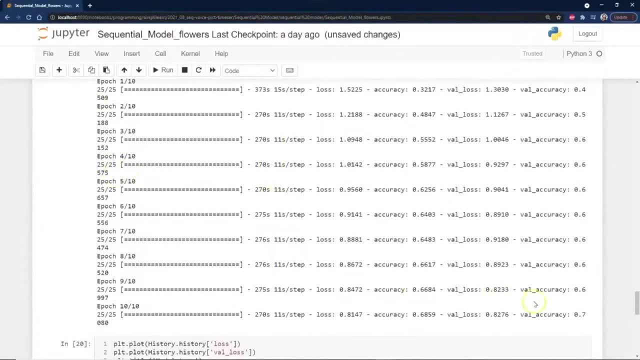 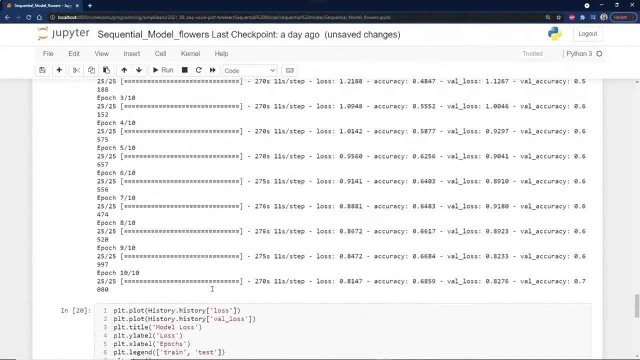 that You don't really want to show them this. You don't want to show them? hey, this is what's going on with the accuracy. These are just numbers, And so we want to go and put the finishing touches, just like when you are building a. 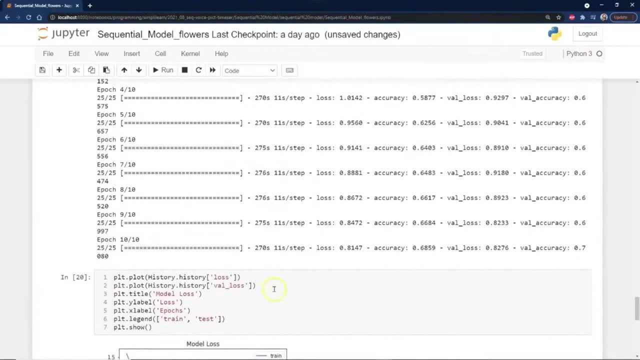 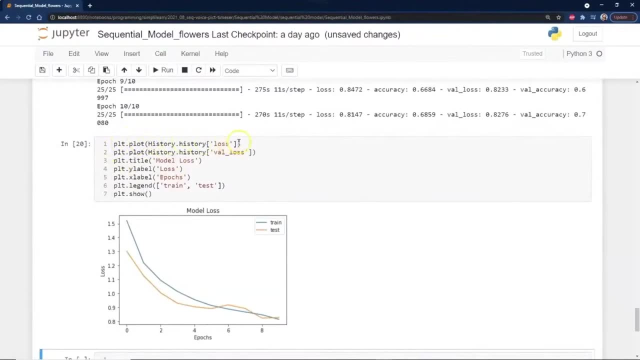 house and you put in the frame and the trim on the house. It's nice to have something, a nice view of what's going on, And so we'll go ahead and do a pie plot and we'll just plot the history of the loss. the 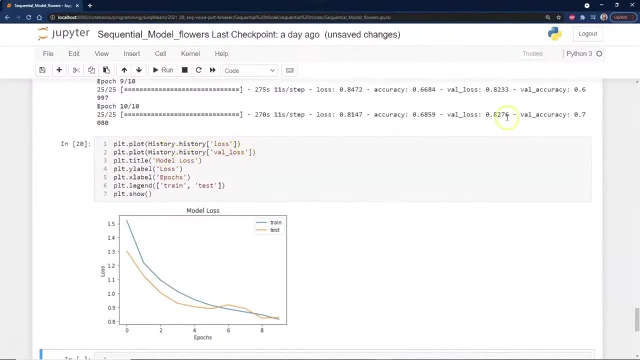 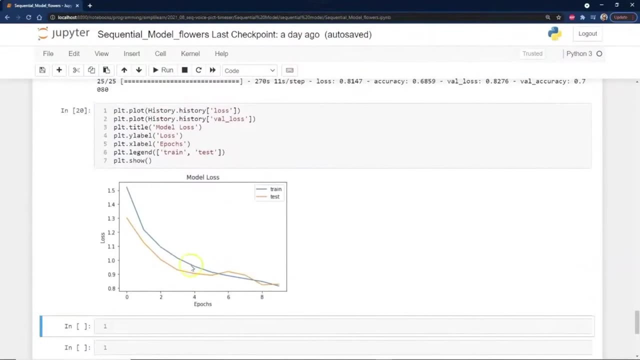 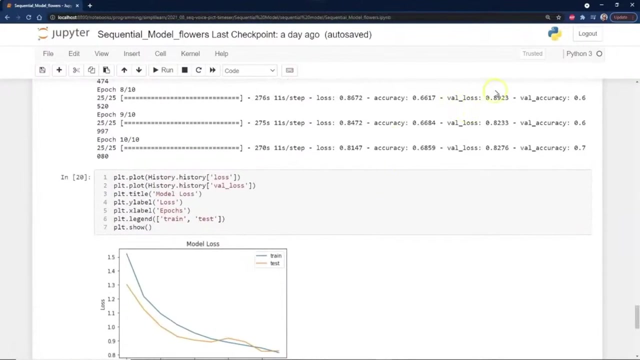 history of the value loss over here- Epic's, train and test, And so we're just going to compute these. This is really important, And what I want you to notice right here is when we get to about five epics- a little more than five, six epics- you see a crossover here and it starts crossing as far as the. 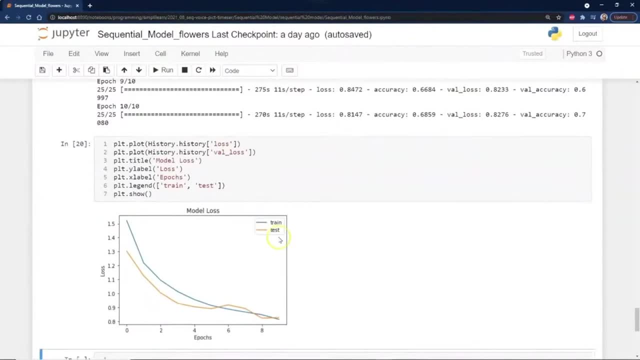 value loss And what's going on here is you have the loss in your actual model and your actual data and you had the value loss where it's testing it against the test data. the data wasn't used to program your model wasn't used to train your model on. 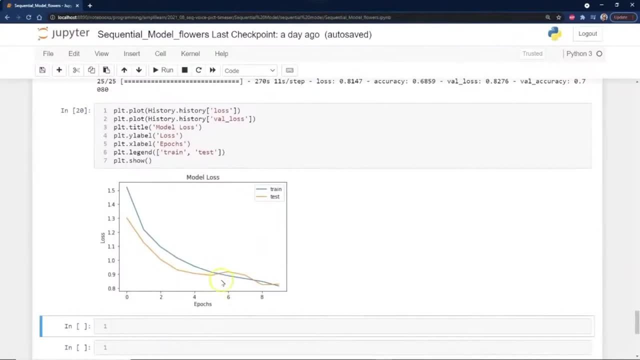 And so when we see this crossing over, this is where the bias is coming in. This is becoming over fitted, And so when you put these two together right around five and six, you start to see how it does this switch over here.